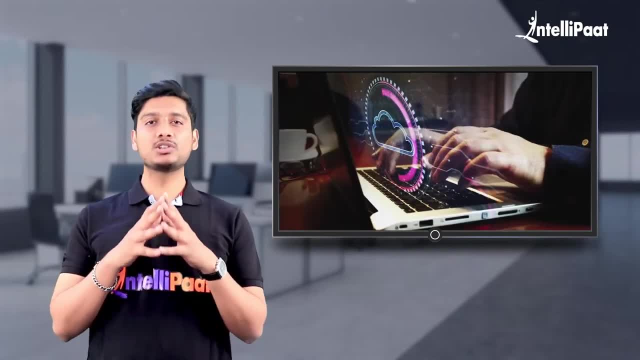 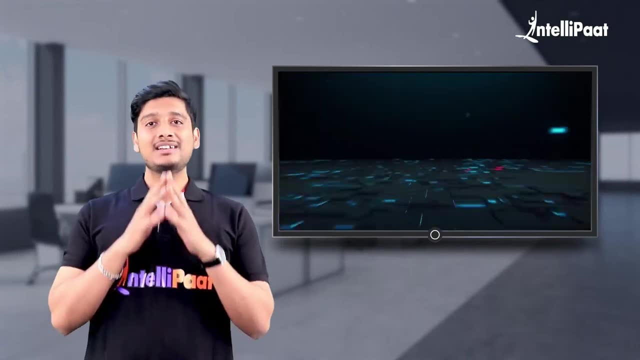 about Microsoft Azure, an industry leader in cloud computing domains, With a 22% market share and approximate 45,000 plus job openings in the world. today, learning this technology will definitely seal the deal for you if you want to become a successful IT professional. 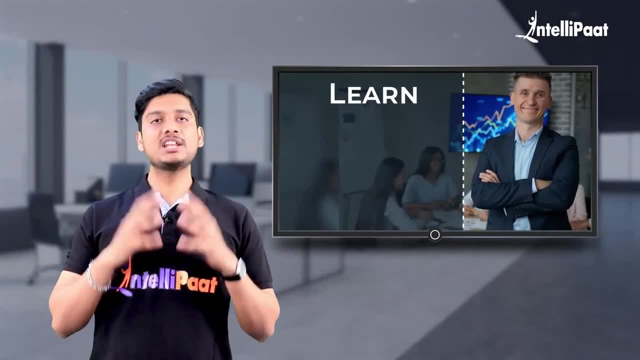 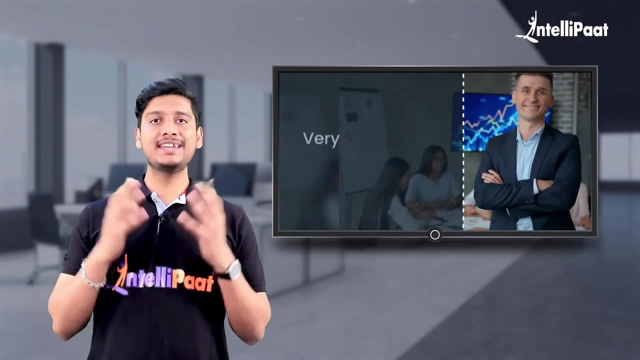 In this session you will get to learn, as well as master, some of the most important Azure services through extensive hands-on sessions. You will get to learn through very interesting case-based quizzes, and we will also discuss about some very frequently asked interview questions that can help you crack your code. 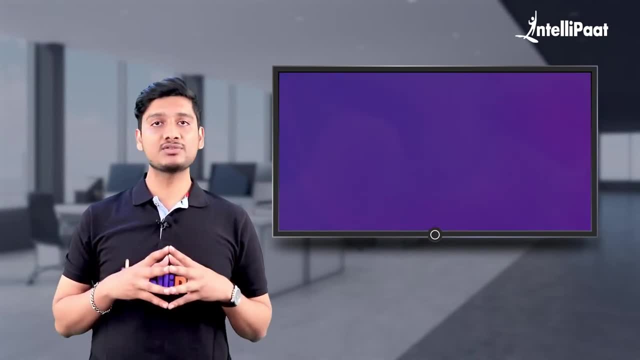 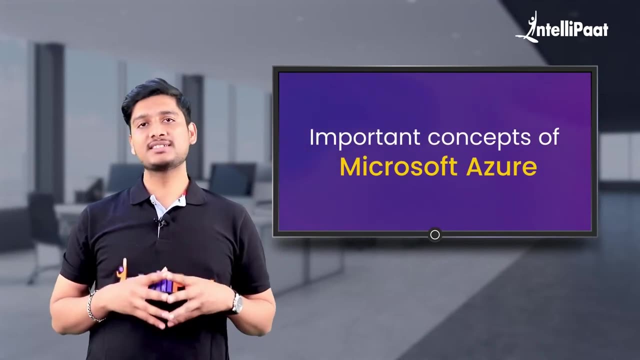 Thank you for watching this video. If you have any questions, feel free to ask them in the comments below. Stay with us till the end of the session as we sail through the very important concepts of Microsoft Azure. There is a lot to learn and a lot to discuss in this session, so let's quickly move on. 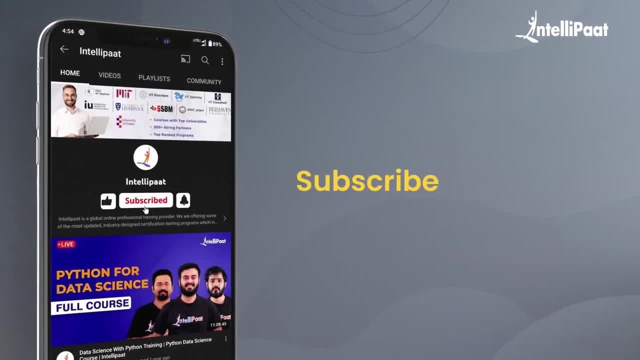 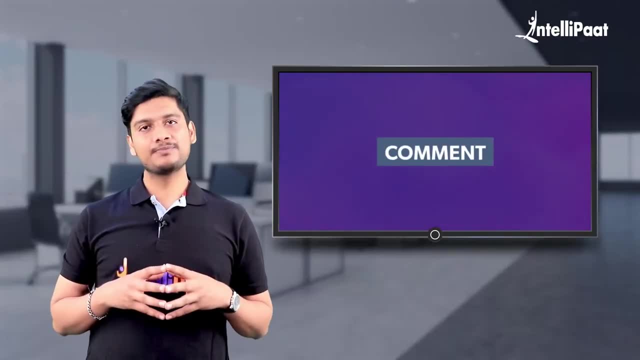 to the agenda of the video. Before that, make sure to subscribe to our channel and hit the bell icon for regular updates. Also, don't forget to mention below in the comments how you liked the video. Now, without any further ado, let's discuss the agenda. 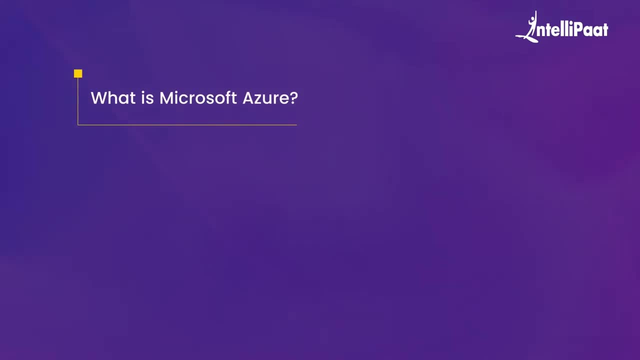 So we are going to start with. what is Microsoft Azure? Moving further, we will discuss about Microsoft Azure. First, we will discuss the story of startup companies using Azure, Azure services and Azure pricing. After that, we will discuss website architecture in Azure and end-to-end. 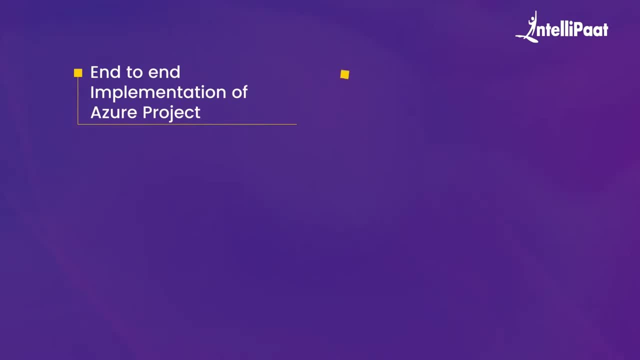 implementation of Azure projects. After that, we will discuss what is cloud computing, various cloud models, top three cloud providers and we will also learn how to deploy an e-commerce website app on Azure. And to end this session, we are going to discuss very crucial Azure. 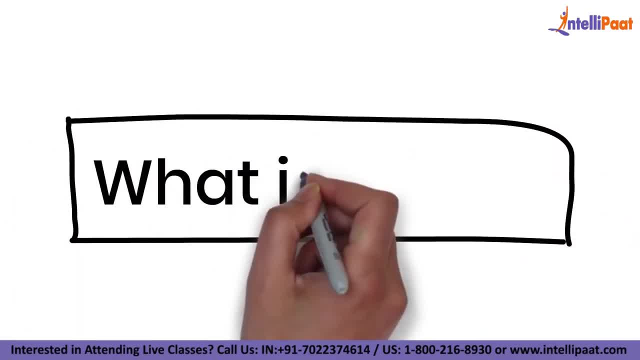 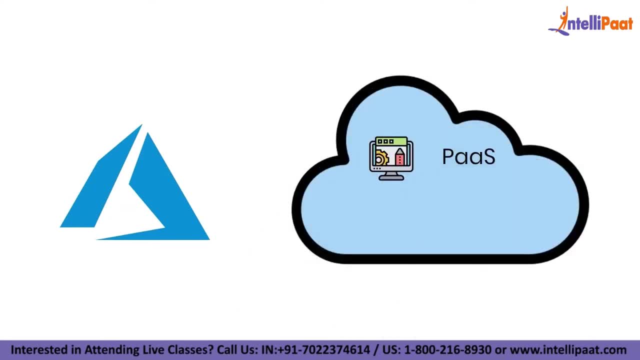 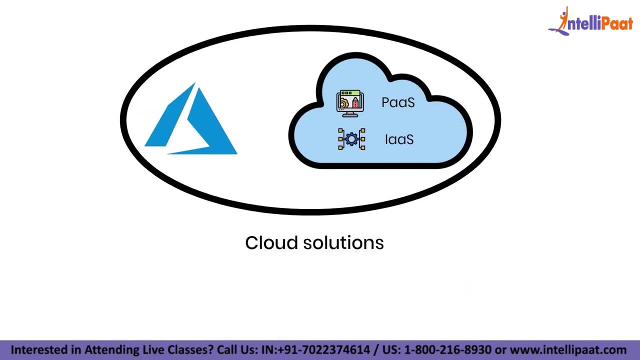 interview questions and answers. So what is Microsoft Azure? So what is Microsoft Azure? Microsoft Azure? Microsoft Azure is a cloud provider that provides various platform as a service and infrastructure as a service. products. Azure has cloud solutions to all the infrastructural problems by providing services in. 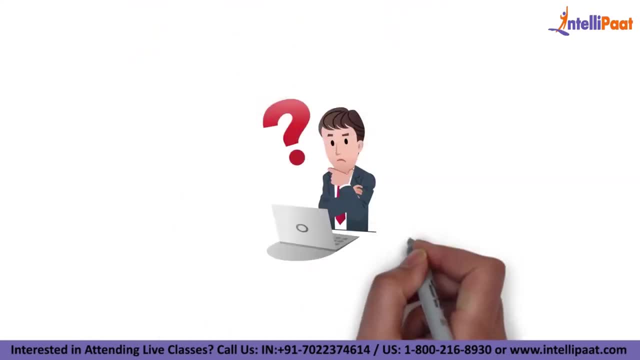 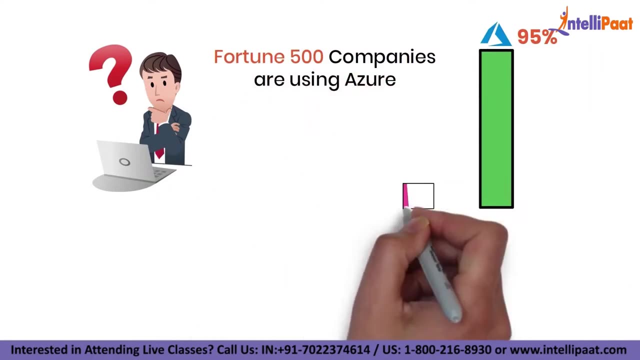 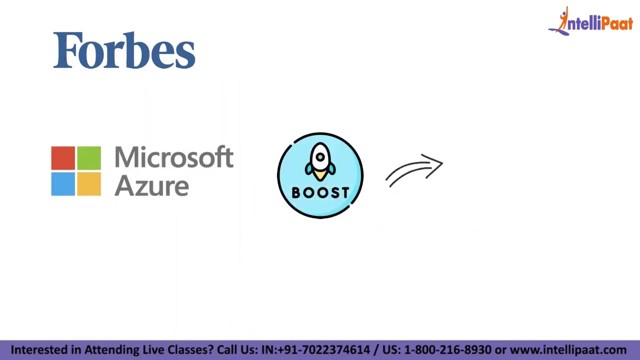 various domains. Did you know that almost 95% of fortune 500 companies are using Azure? Also, it is five times cheaper than AWS in terms of windows and sql server, because there are also Microsoft products. Forbes say that Microsoft Azure is set to boost the size of the IT market by 10 trillion dollars in the 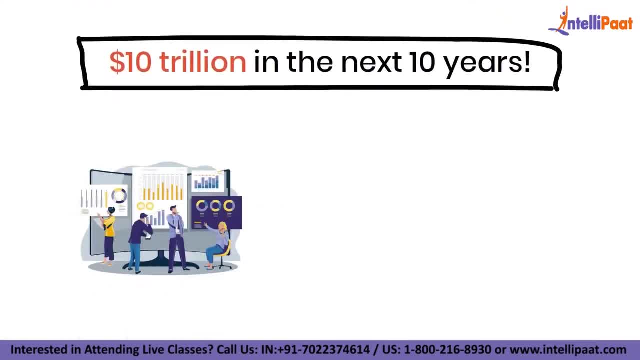 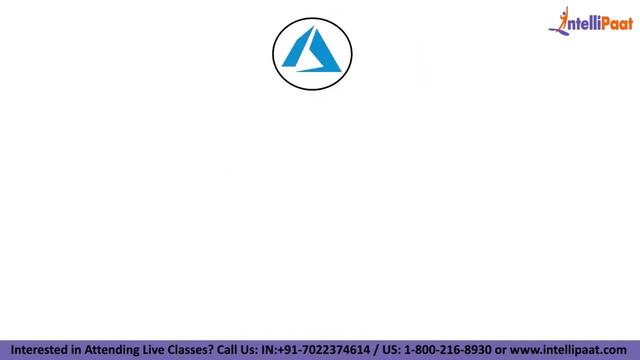 next 10 years As, per predictions, 80% of the businesses will move their workload to cloud by 2025. Thus making it a major company in the future, major career to consider transitioning to. for a better understanding of azure, let us start at the 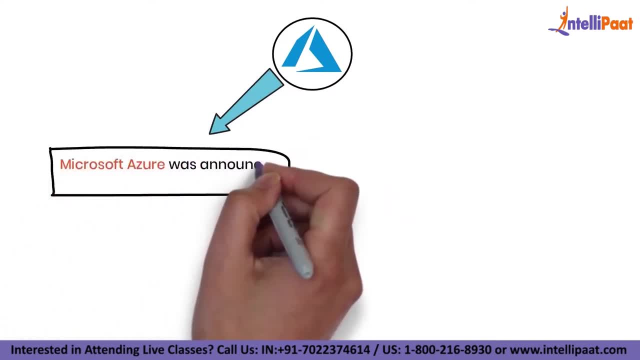 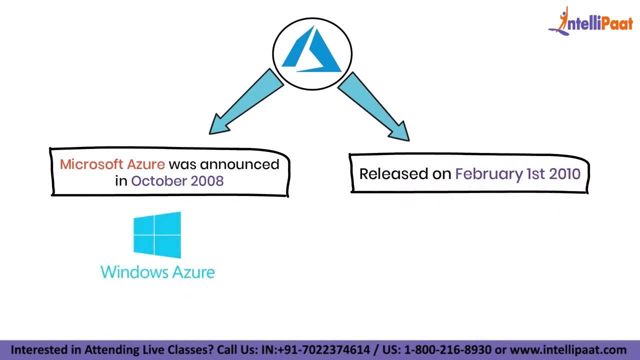 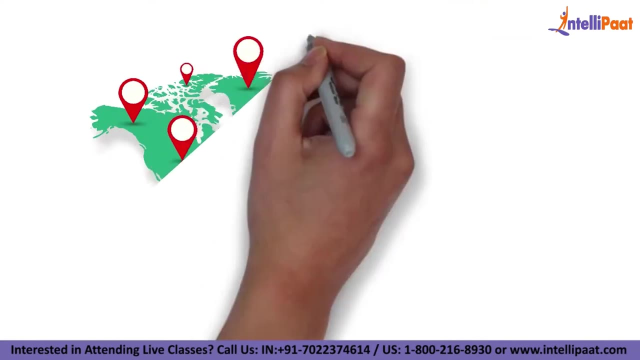 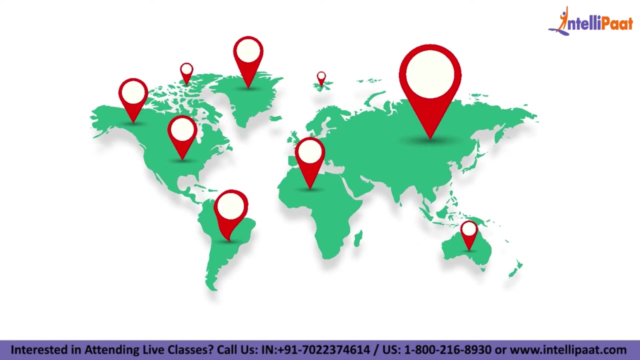 very beginning. microsoft azure was announced in october 2008 and released on february 1 2010 as windows azure first, and later named as microsoft azure on 25th march 2015. in today's scenario, its reach is in 140 countries and is still expanding, which is pretty impeccable in simpler. 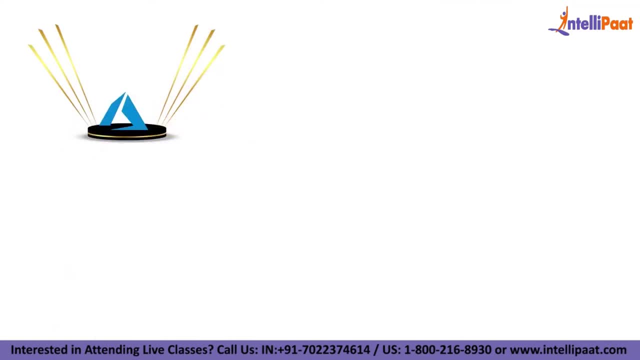 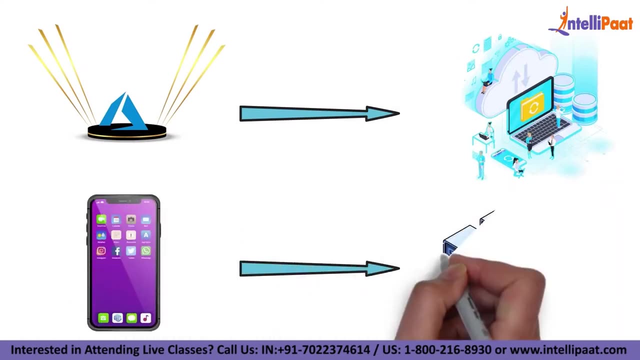 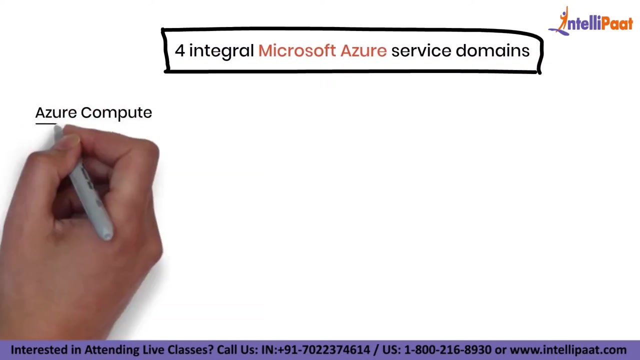 terms, microsoft azure is a platform that enables users to engage in agile cloud computing and is designed for creating and managing apps through microsoft's data center. now there are four integral microsoft azure service domains. the first one is azure compute. compute is the most important domain in azure. as it is the most important domain in azure, as it is the most. 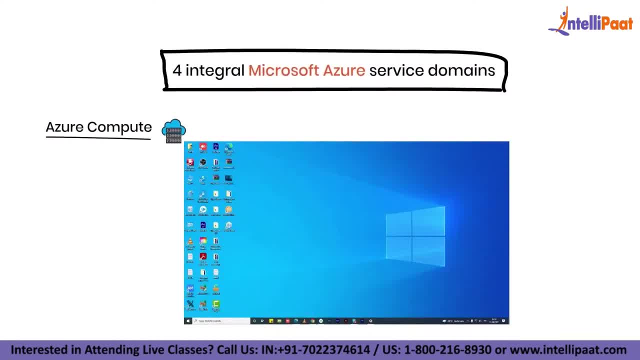 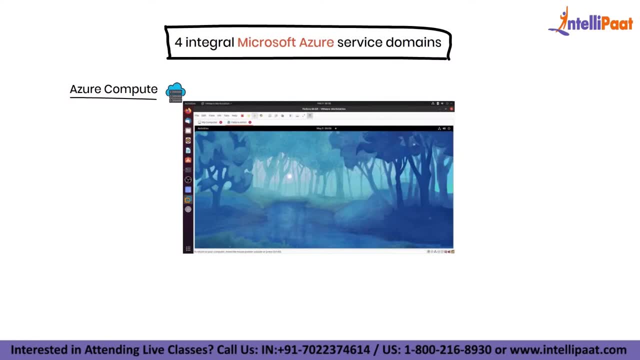 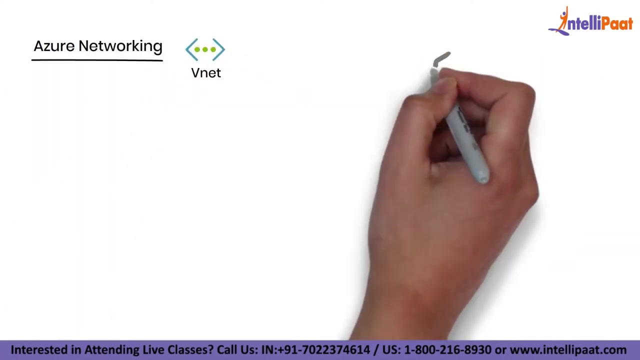 integral domain in azure as it brings everything together. with azure virtual machines you can get on-demand scalable compute resources. azure virtual machines, app services and container instances are some popular compute services. second, we have azure networking networks from the cloud networks. in azure, vnet is the networking tool that connects all azure resources together. these 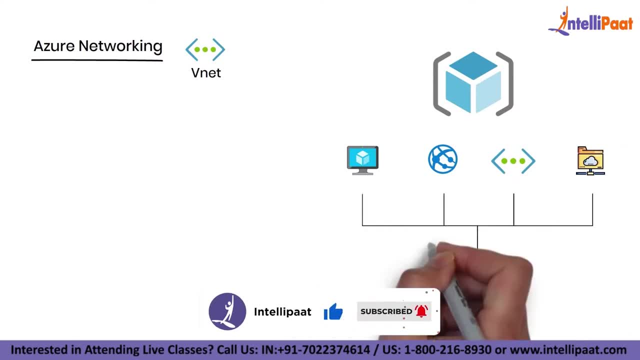 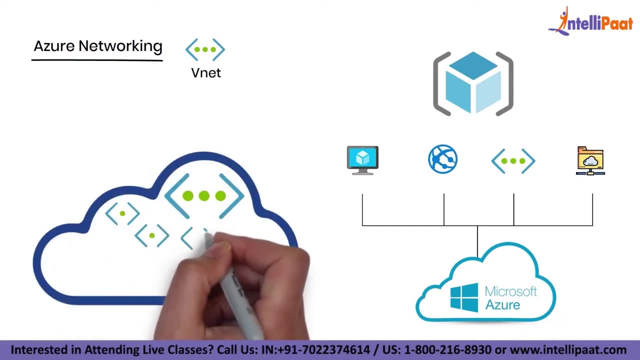 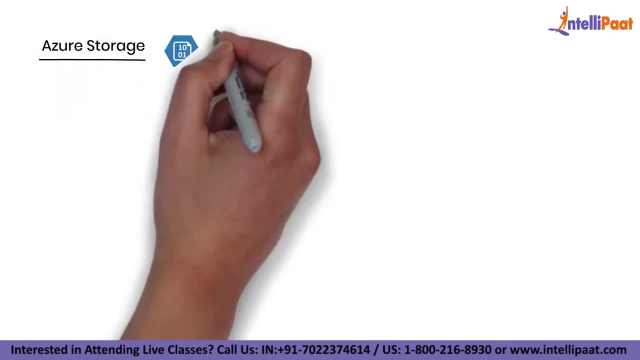 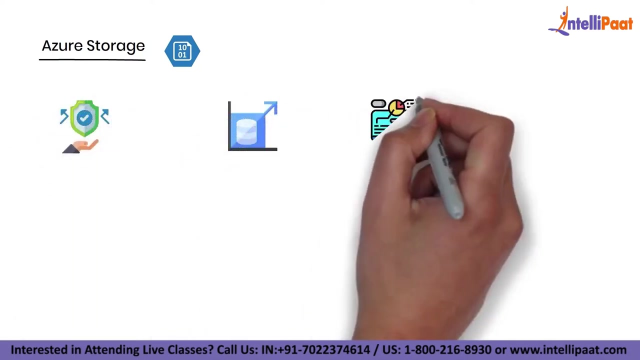 networking services are used to connect all azure resources together and to connect all azure resources to the azure cloud. it is also used to manage virtual private networks and further create multiple virtual networks on the cloud. the third one is azure storage. azure storage provides storage solutions that are more durable and large-scale applications. data-driven applications can be. 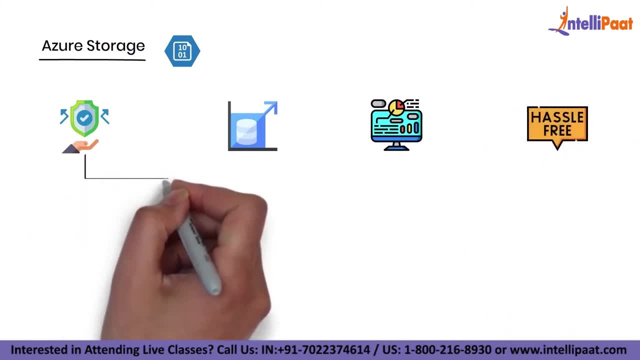 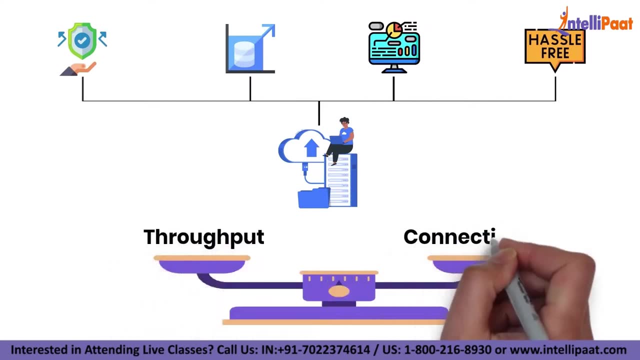 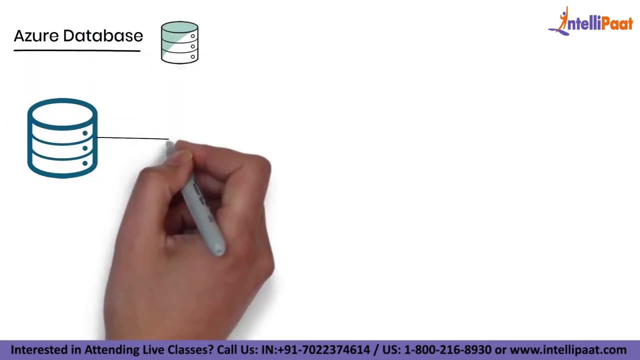 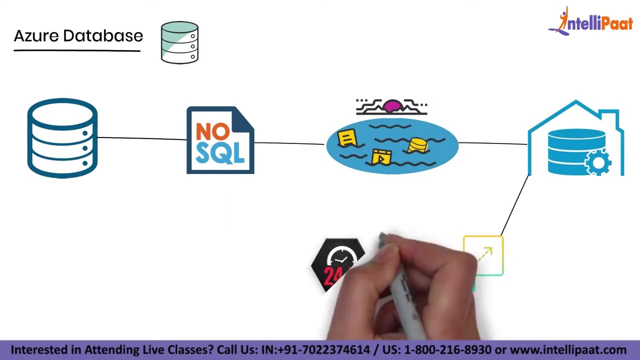 built without any hassle. azure automatically connects all azure services to the azure cloud, it automatically scales the storage requirements according to the usage and it automatically balances throughput according to the connections made. and the last one is azure database. azure provides relational databases, no sql databases, data lakes and data warehouses. it provides a scalable, high 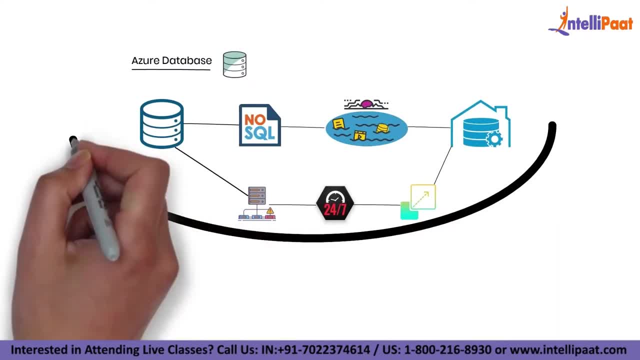 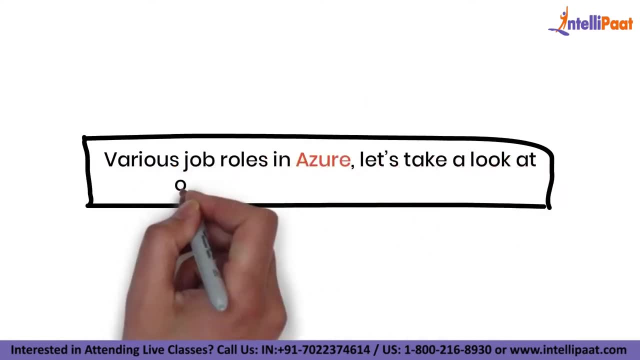 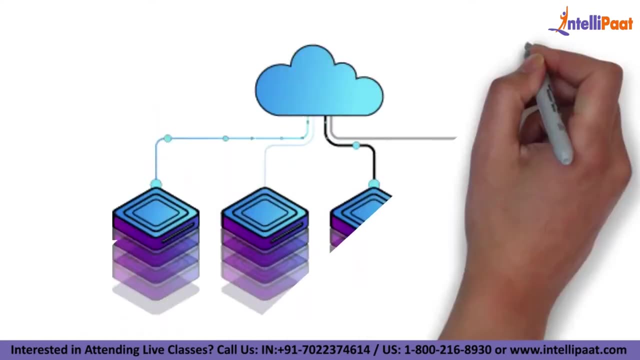 available and fault tolerant database server and lets you scale according to the incoming data. there are various job roles in azure. let's take a look at one of the most popular job roles: azure developer. an azure developer is a cloud professional who creates cloud-based applications making use of the 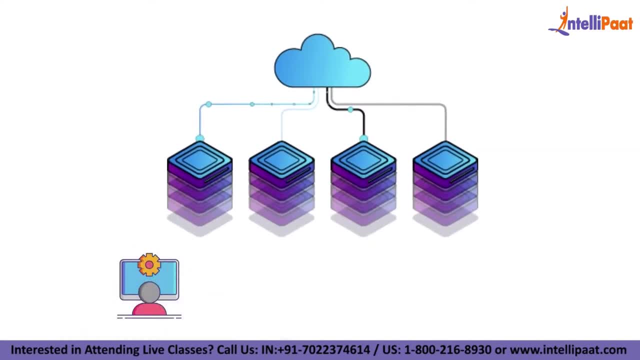 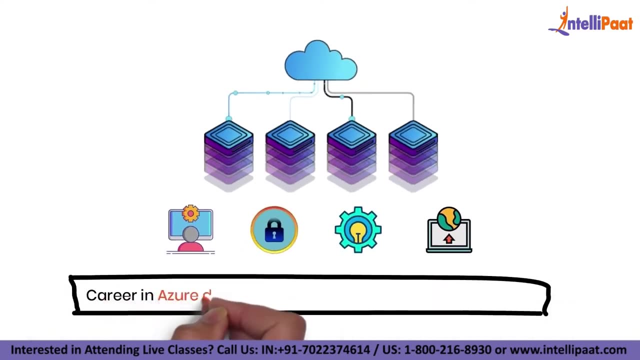 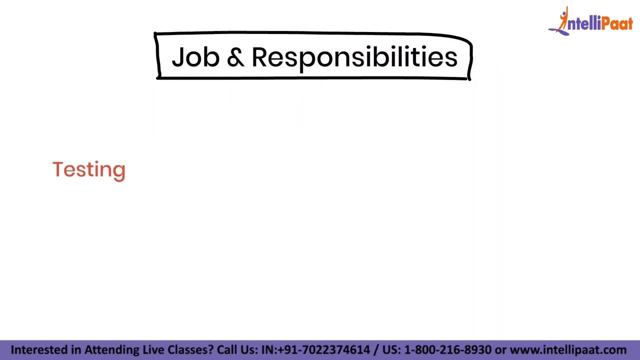 benefits of the cloud architecture. if you are proficient in testing, security, development and deployment, then a career in azure development is somewhere you will fit in well. the job includes responsibilities like testing and monitoring of the azure cloud and the cloud architecture. it also includes the testing of applications, maintaining, developing and deploy them on azure. 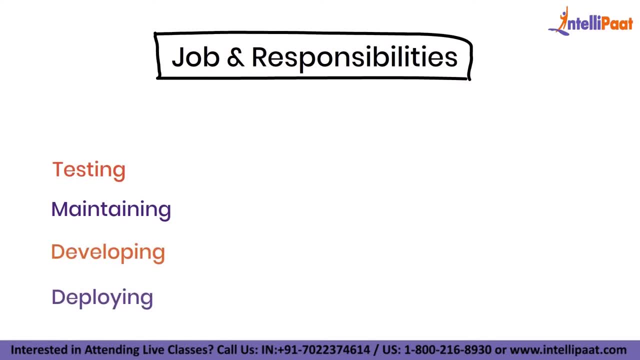 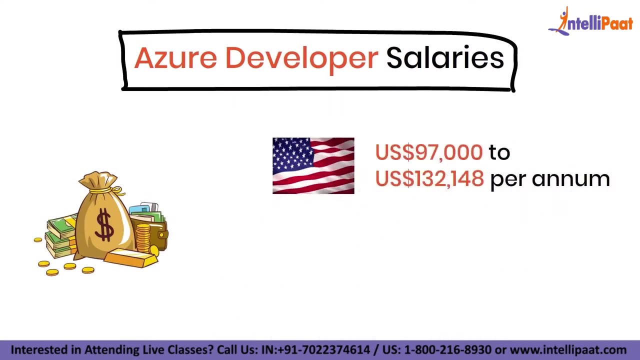 it also includes participating in all phases of development and having the ability to work side by side with cloud administrators, clients and cloud architects in united states. on average basis, an azure developer gets paid 132 148 dollars per annum. however, for an entry-level developer, its 97. 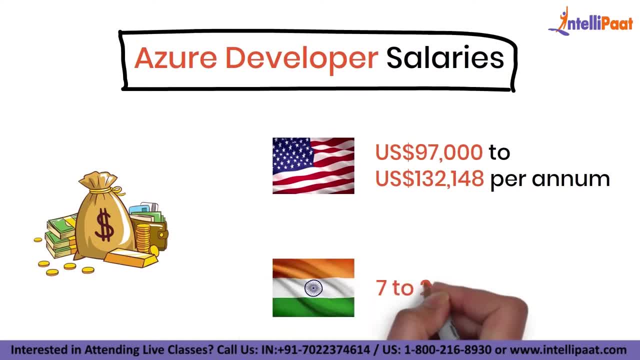 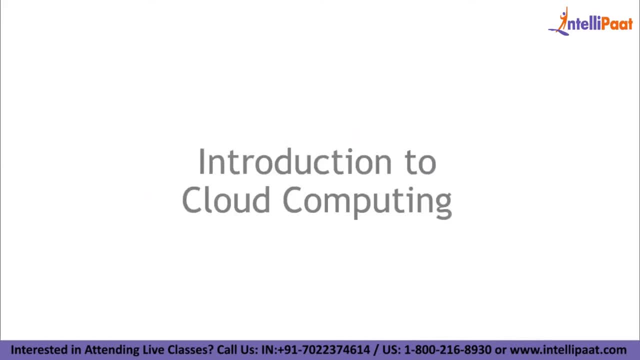 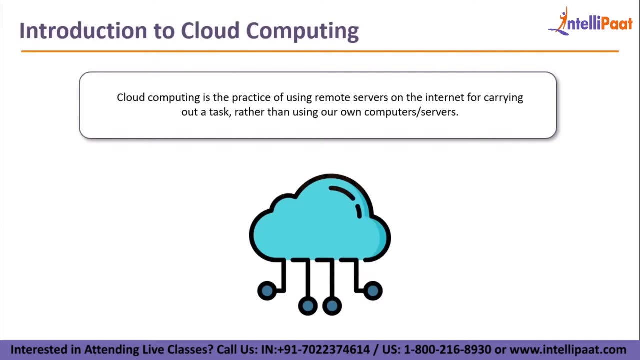 000, whereas in india the salary offered ranges from 7 lakhs to 25 lakhs per annum. that's all about azure. what is cloud computing right? so let's go ahead and understand first cloud computing by its definition. so, guys, by definition, cloud computing is nothing but the use of remote servers on the 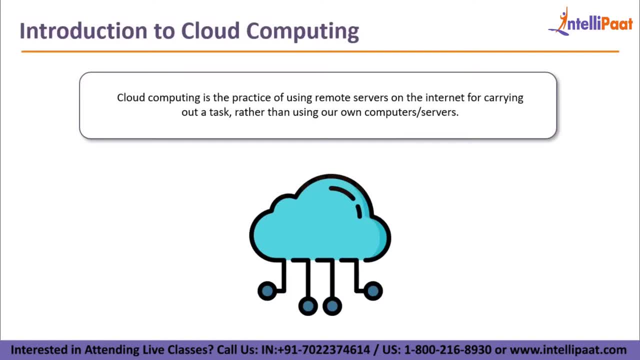 internet to do your tasks. it could be basically hosting an application. it could be hosting your database server and sometimes it's the application itself rather than the server itself. essentially, it could be your database server or service server. orively, you could have programs like secure costsos or problems like that. it could be social and 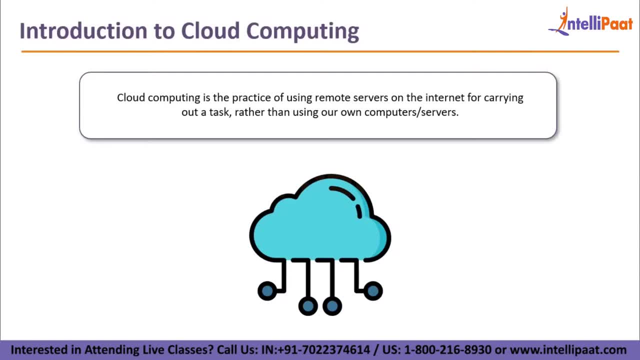 it could be anything right when you use servers on the internet, when you use somebody else's servers on the internet rather than using your own servers or computers. when you use somebody else's computer on the internet. that is called cloud computing right, and the person or the 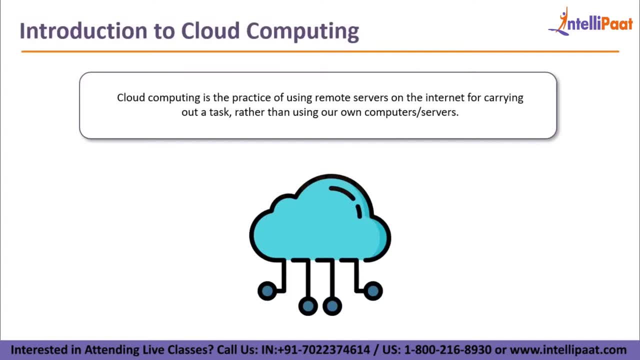 company who provides you with that kind of server is called a cloud provider. this is a gist of what cloud computing is now. obviously, cloud computing has more things to it, and we will discuss that as we move along. right now, to give you an example as to how you can imagine how cloud works is like, 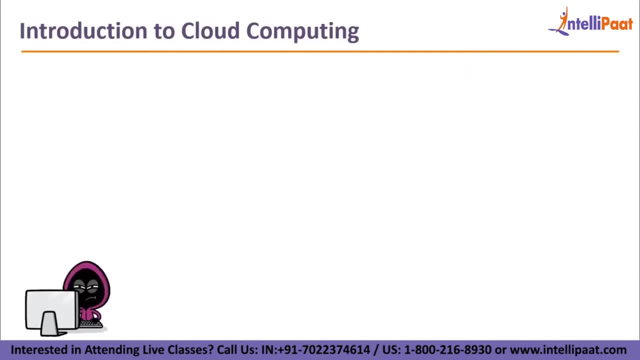 this. let's say you're a developer- okay, and what you want to do is you want to host an application. so you basically start up a company and you have an idea which is similar to, let's say, instagram, and that idea is a billion dollar idea. right, and what you want to do is you want to start off by 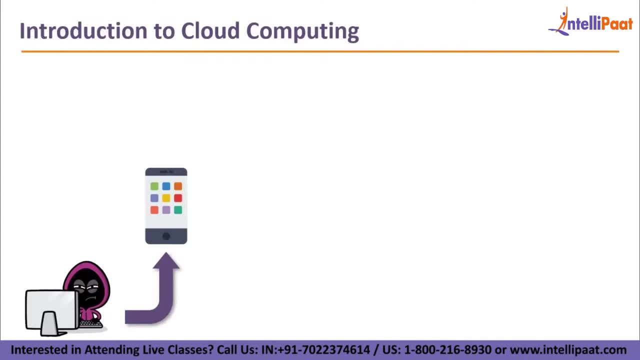 just creating the application by yourself. you don't want to hire any people, right? because you want to keep the cost minimum. so you develop the code by yourself and now the application is ready. but you have to make this application available to the world. so how do you do that? so the first thing that you would have to 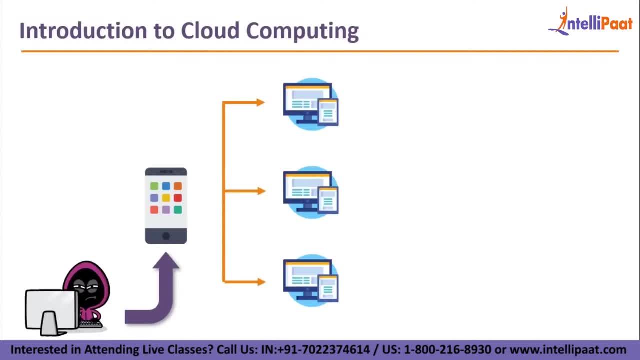 do is you'll have to buy some servers and you'll have to put that application on those servers. so once your application is on those servers, the next top task would be to basically make that application available on the internet. right, and how would you make it available on the internet? 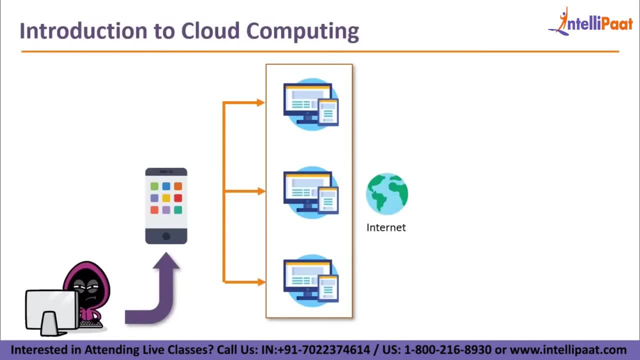 you basically connect internet to these servers and you assign a public ip to these servers, and now your, your application is basically available on ip address. next thing that you would do is you would buy a domain and the next thing that you know is now the domain is ready, and now your. 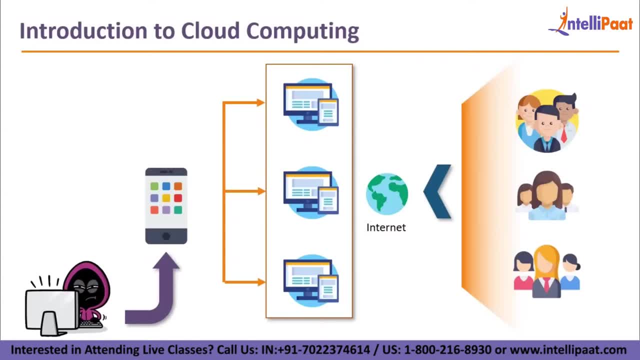 application. anybody on the internet who goes to your particular domain would be able to access your application. okay, so, guys, this is the normal life science of how applications were launched before cloud computing. now, the problem over here, guys, is that you invested some money on these servers and guys servers. 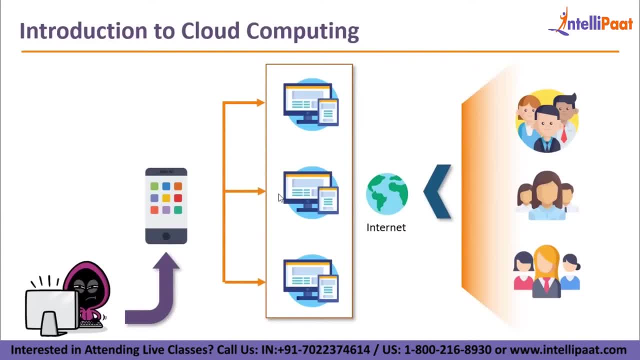 are not cheap. they're very, very expensive. right, and as a guy who is starting up with their company, you might think that an idea is worth a billion dollars, but if you actually think about it, there's a lot of risk, and there's a lot of. I mean, there's a 50% probability, because you are just starting off now. 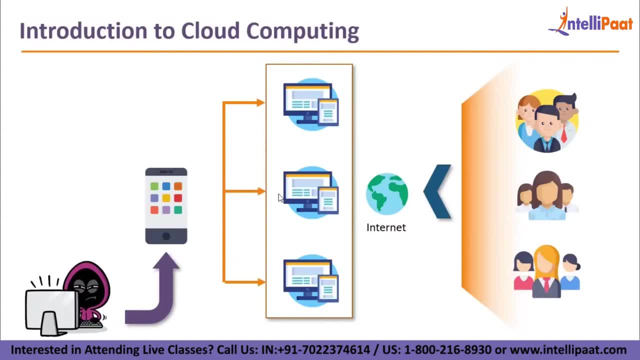 that you might fail, although there's a probability of a 50% probability that you might succeed as well- but there are a lot of risks that are involved and there's a lot at stake over here, because you're investing a lot of money on these servers, right? so this was the general way of starting up a business before. 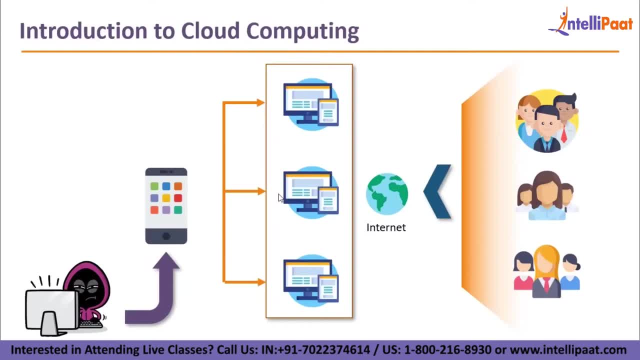 cloud computing emerged. now, after cloud computing, it has become very simple. now, let's say, you come up with an idea and now you want to deploy your application. all you have to do is you will go on cloud, cloud computing and you will go on cloud computing, and you will go on cloud. 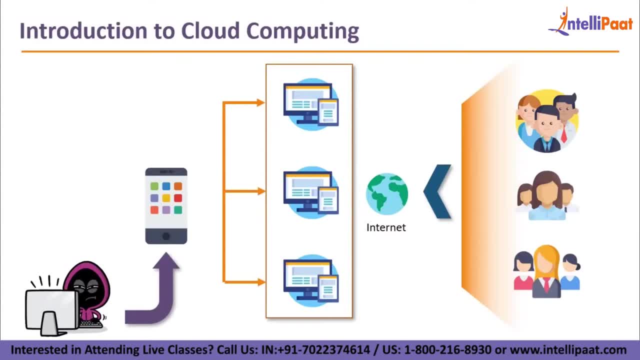 cloud computing and you will go on cloud computing. and you will go on cloud and you would say, hey, I need some servers for deploying my application. so you would get those servers, which would already be connecting to the internet, or everything would be set up by the cloud provider. you just have to use them, right. 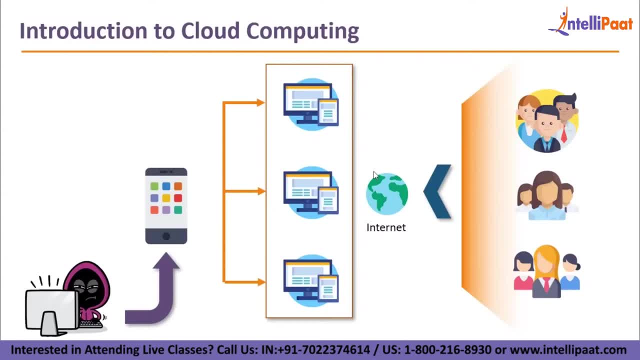 and the only thing the cloud provider would expect from you is he would say, like: hey, you know what. you just have to pay me for the time that you're using the servers for, and that's about it. I don't need anything else from you right now. that's an awesome thing now, the kind of pricing that cloud computing gives. 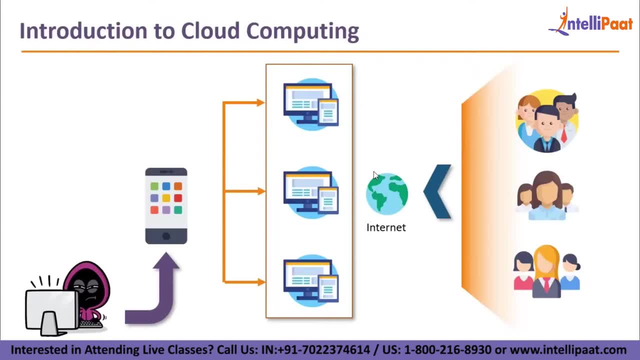 you is a pay as you go pricing. that basically means you just pay for the amount of time that you're using servers for. in case of Azure, it counts in terms of minutes, right, so the number of minutes that you would be using the servers for it will charge you according to that. right now, if you again think about what? 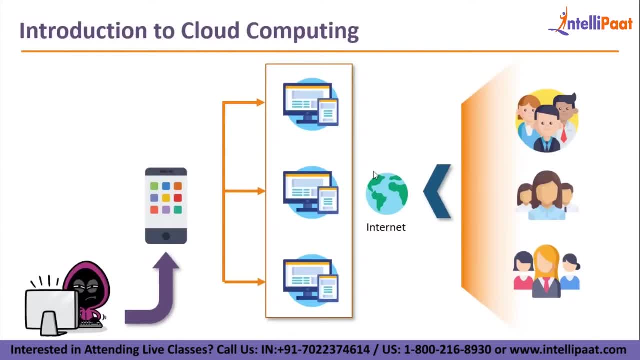 all changes came about over here when I was not using cloud, and when I'm using cloud now. the first change that would come about here is if, let's say, you know you were not using cloud computing and you bought these servers. now, obviously somebody has to manage these servers for you as well, right and now, when somebody 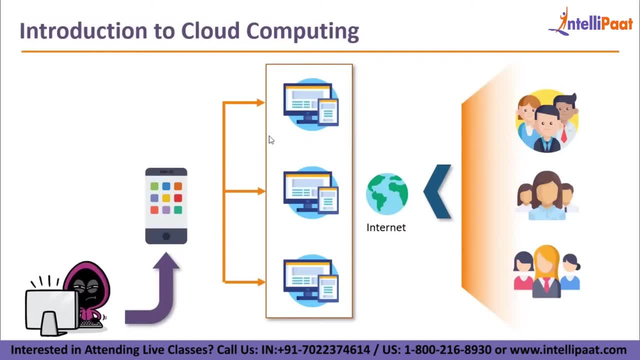 has to manage them. for you. there's always a chance of downtime as well, so you always at your back of your mind. you will always be thinking of whether my servers are up and running or not. do I need more people to handle these kind of servers? when your application becomes big, you will also have to scale these. 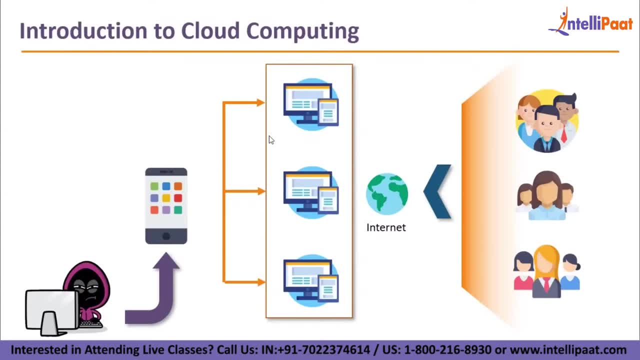 servers. all these problems would be at the back of your mind, and at the same time, you also have to develop code for it, and at the same time, you also have to develop code for it, right? so that's a lot on your plate now. what cloud does for you is it says you. 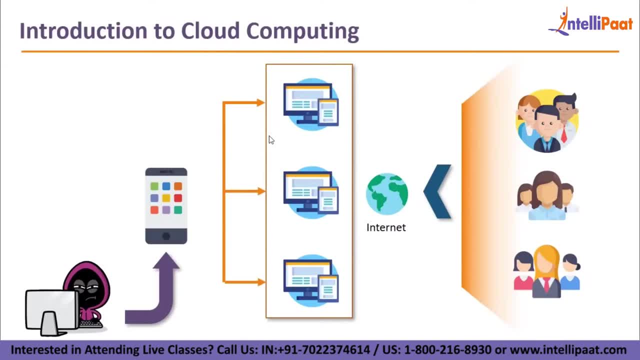 know. you just pay me for the amount of time you're using the servers for. I, on the other hand, will hire the workforce that is required to manage these servers. I, on the other hand, as a cloud provider, will also scale your servers as and when required, when the demand increases on the application you just 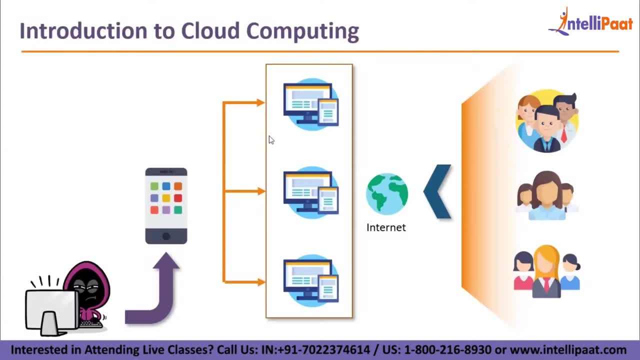 sit back, relax and you code your application. that's all you have. right and guys? this is the biggest advantage that you get with cloud computing. right and focus on the work that you have to do. everything logistical or everything operational with respect to managing servers, is handled by your cloud. 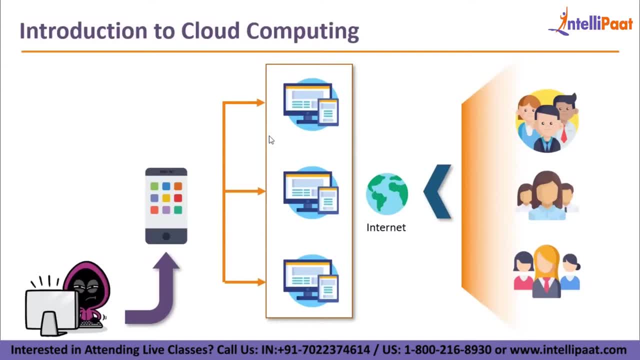 provider, and what is better than paying less for that right you pay? you're paying less, you're hiring less workforce and at the same time, you're getting a better quality of internet hosting available. I mean, you do basically, like literally- imagine now if you have to secure an. 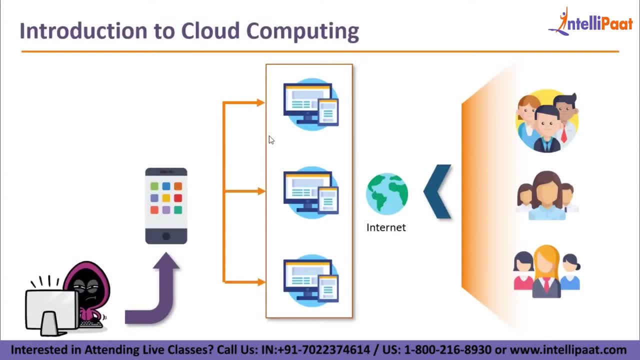 application you'll have to buy. you'll have to hire a security engineer who will basically secure your application. you will also have to hire people who will ensure that your application is up and running. but how? by basically scaling them up and down. that your number of servers. so you would need deployment engineers. you would also have to keep some. 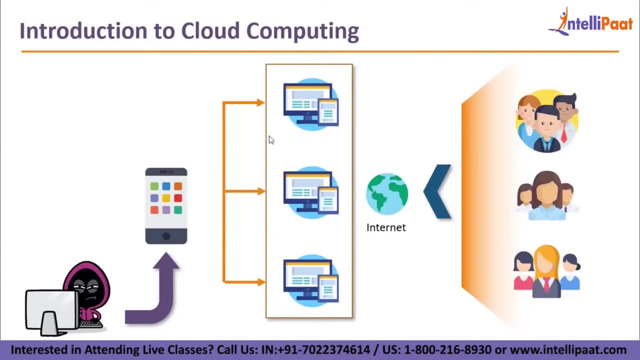 servers in your stack, so that whenever new servers are required, whenever the demand goes up, those can be plugged and played as and when required. right, so these are all the things that you had to do, but now, with cloud computing, you don't have to do that, because everything is managed by the cloud. 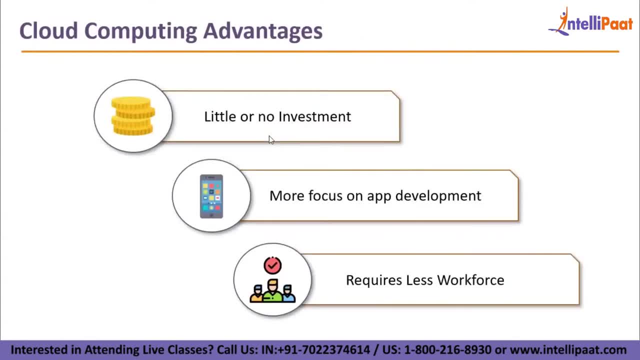 provider. you just have to code your application. so summarizing the advantages that you get with cloud computing is that while you're starting up, you don't have to invest a lot. right? that is the number one advantage. number two advantages: you can focus on your app development. you don't have 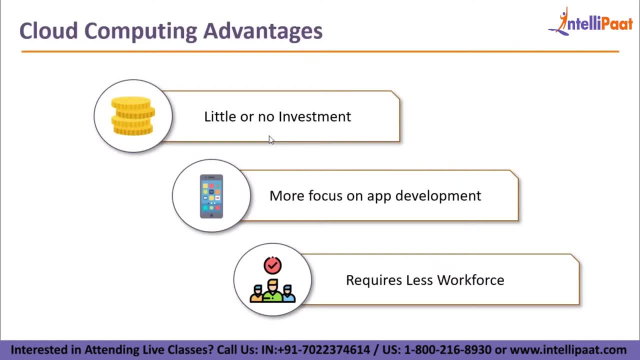 to focus on. you know what is happening on my server. are my servers running fine or not? are security patches updated or not? everything will be managed by your cloud provider. and the third thing is that it requires like a workforce, because obviously you're not hiring anyone to manage. 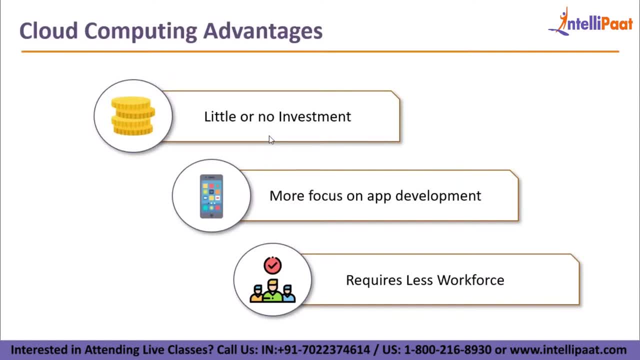 your servers. everything is being done by the cloud provider. if you want to hire people, you can actually hire more developers so that your coding work is distributed among them, right? so these are the advantages, guys, that you get with cloud computing. now, cloud computing is offered in various, in various types of services and that we will discover as we move along, but those types. 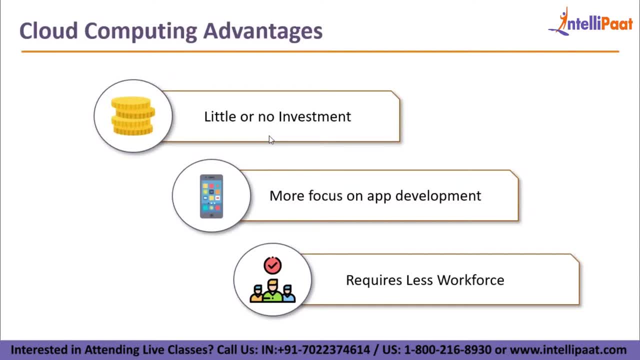 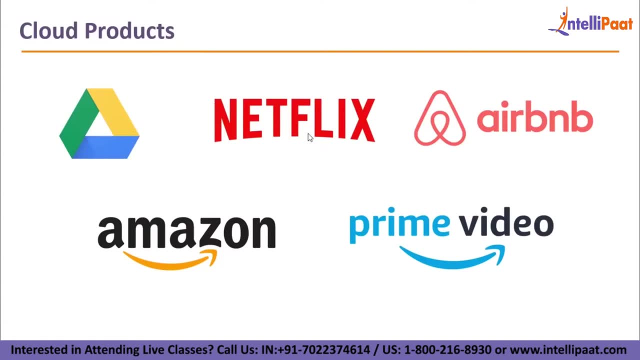 of services leads to different kind of applications or different kind of products on the cloud, for example. you might have heard about this, you might have heard about google drive, you might have heard about netflix, airbnb. all these applications are basically hosted on cloud and you might not even 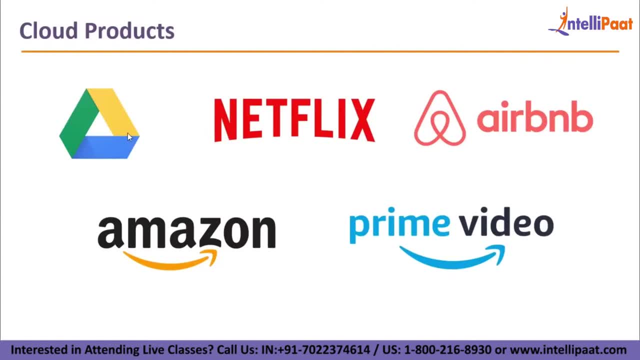 realize it right now, if we talk about google drive, google drive is nothing, but it's it's it's kind of service. it's software as a service that is given to you by cloud provider. what is the software service? we'll discuss that as we move along, but just understand that google drive is. 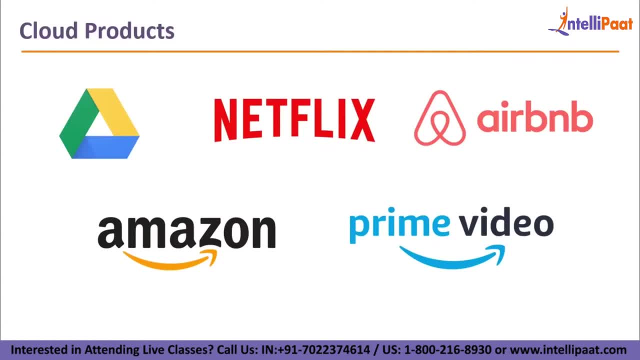 a cloud product. it is basically hosted on google's infrastructure, right? you don't care about where. if you are uploading a file on google drive, you don't care about where. on which server is it being stored, right? you don't care about which operating system is that server running? you don't? 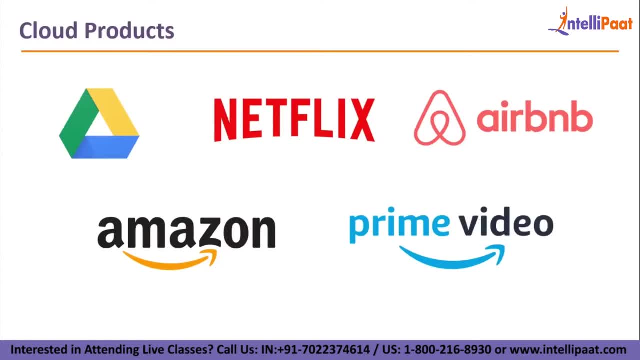 care about. you know whether the hardware on that server is good enough to basically handle the speed with which you want to work. you don't care about anything right? you just care about your file being there on google drive and you know it's gonna be there. why? because you trust google with 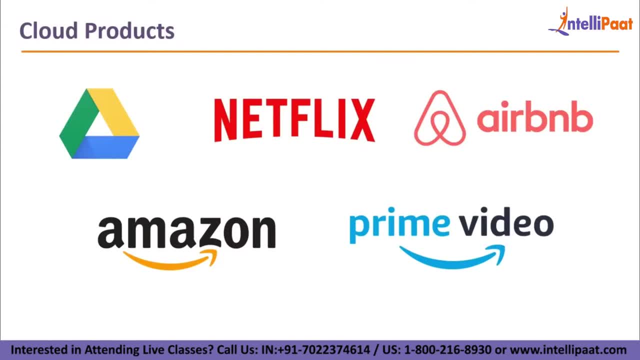 your things. you trust google that it'll manage everything on the infrastructure side, and that is exactly what cloud computing is all about. similarly, when you talk about netflix, netflix is a very popular video streaming surface. i'm sure all of you must have used it. that is itself. 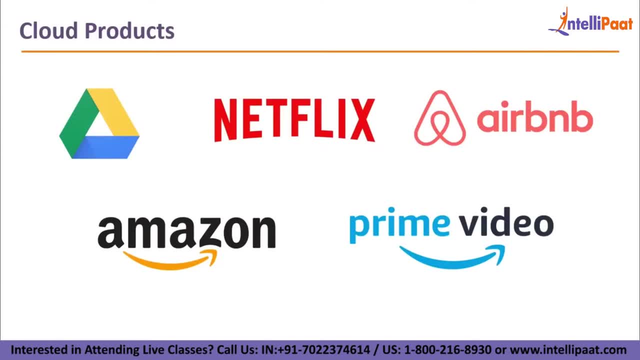 also hosted onto cloud right. so netflix. we rely on netflix to be always up and running, and netflix itself relies on the cloud provider on which it is hosted. that you know. they will ensure that i'm up and running always right. so that is how cool. 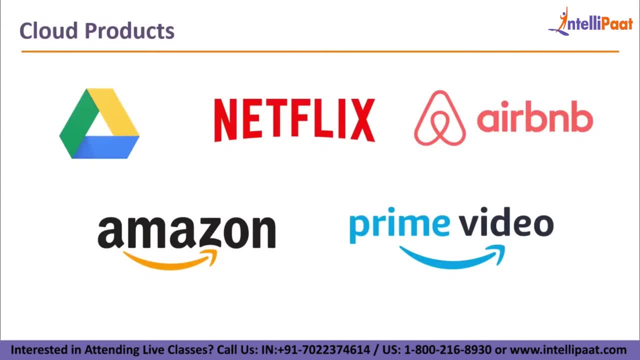 you can do this one way by one way. that's exactly what you see happening, right? it also has to do with that. you can do this one way by one way, right, you can do this one way by one way. that you you know. the concept of cloud is that a popular service such as netflix is also not caring about. 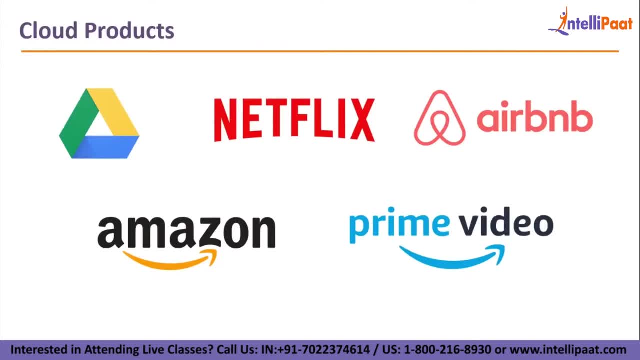 how these servers are managed. all of that is managed by your cloud provider. similarly, you must have also heard about abnb. you must have also heard about the e-commerce company, the giant, which is amazon. then there is also prime video, all of these products. they are basically hosted. 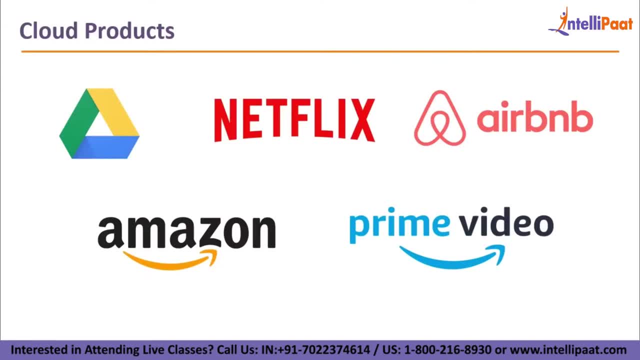 on cloud right. so if you have remained there, you would also recognize flipkart. flipkart is again an e-commerce giant, which was recently taken over by walmart right. flipkart also is completely hosted on a cloud provider. in flipkart's case, it's basically hosted on microsoft azure right. 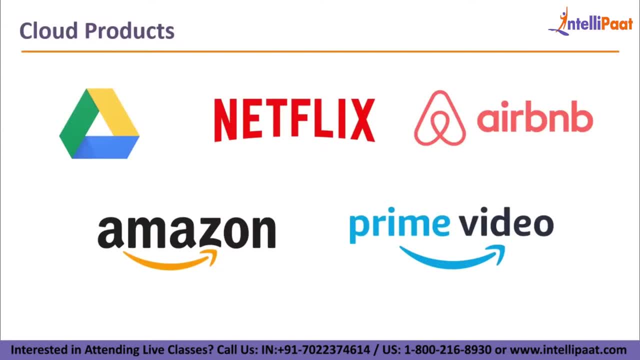 so we'll be talking more about azure as we move along, but, guys, these are some of the products that you might be using in your everyday life which are based, basically hosted, on the cloud. right now you 're moving forward, guys. we were talking about cloud computing services. there are various kind. 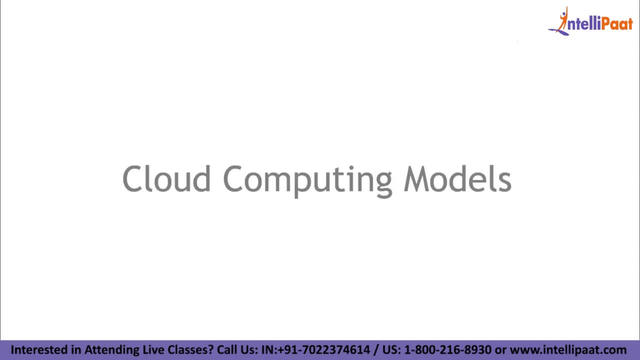 of services that cloud computing has to offer us. there are. basically, the cloud computing business is based on two kind of models, and we'll discuss those models in this section, which is cloud computing models. all right, guys, now let's discuss the various cloud models which, on which, basically, 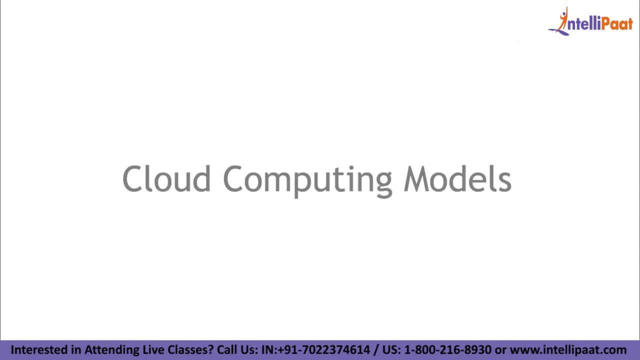 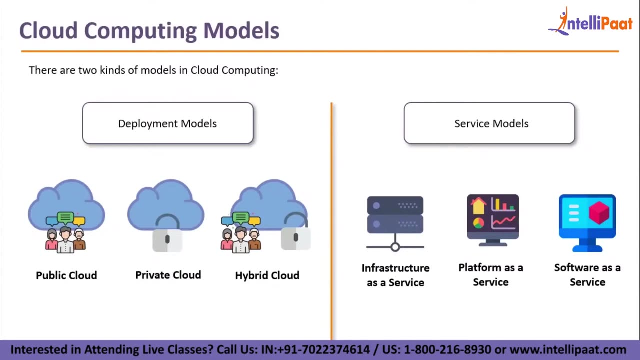 cloud companies are working and are earning right. so, basically, cloud computing gives us two models. the first model is the deployment model and the next model are the service models. now, what are these? let's discuss them one by one. so, guys, deployment models are basically the way you can deploy your application on cloud right, the 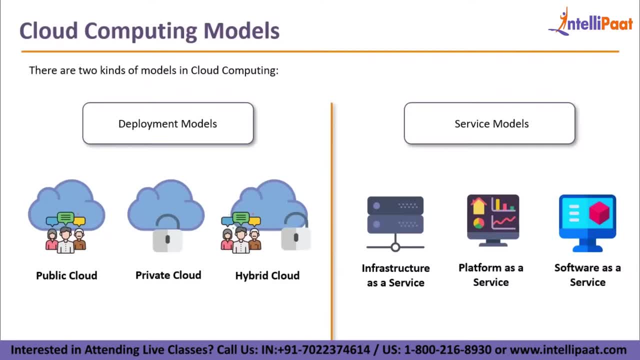 various ways you can apply. deploy your application on cloud are basically called deployment models, right? so that's a thing that you choose. how do you want your application to be deployed? how are they deployed? we'll discuss that in a few moments, but first let's discuss how is it different from? 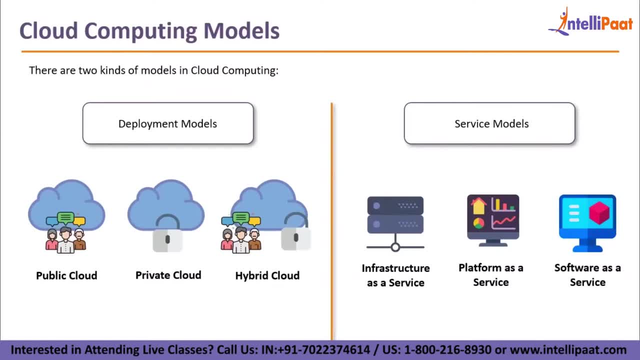 service models. so, guys, service models are different, like service models are different, and service and Service models are: how do you want your service to be, or how do you want the cloud provider to give you a particular service? Do you want an infrastructure from the cloud provider? Do you? 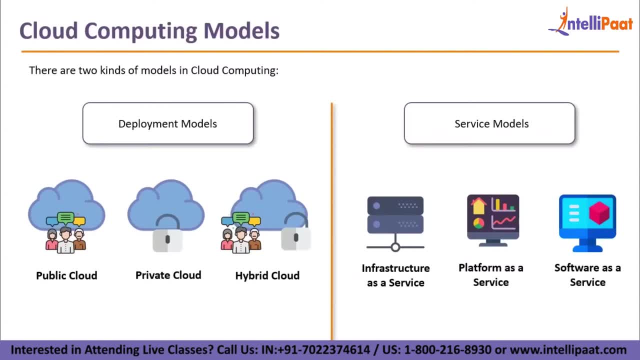 want a platform from a cloud provider, or do you want a software from a cloud provider right Now? what does these three things mean? So when you talk about infrastructure as a service, you basically expect that you would be given a machine to work on from the cloud provider. That 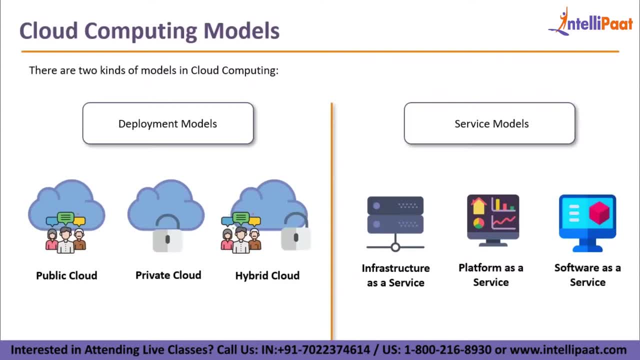 basically means you will get access to the operating system. In case of platform as a service, what you do get is basically a dashboard kind of thing, where you will not get access to the operating system, but you get access to a dashboard on which you can upload your application. 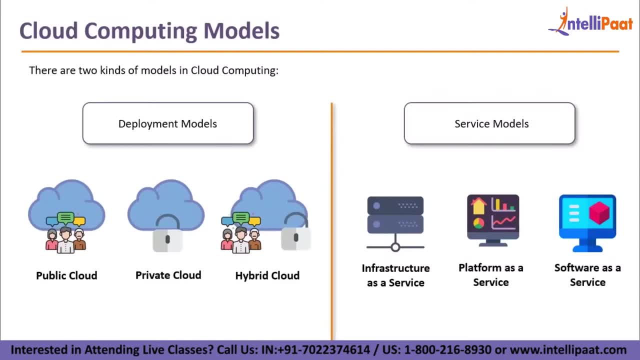 and basically see whether your application is up and running right. So, software installation, everything is handled by the cloud provider, And the next thing is software as a service, wherein you do not get access to the operating system, You do not get access to a dashboard. 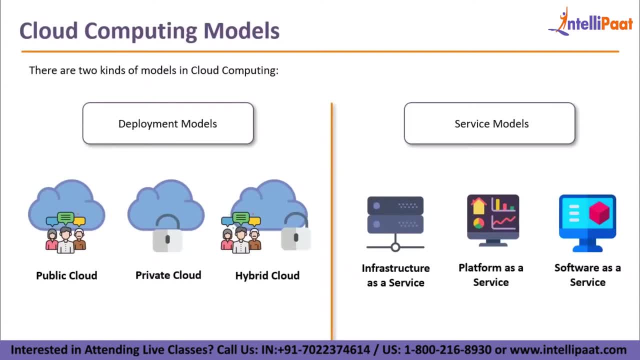 where you can upload your code, But what you do get is a software that has been made by the cloud provider, which you can use to cater to your needs. For example, there are various CRM softwares out there which are hosted on cloud, For example, Zoho CRM. it's a cloud product, right? Google Drive. 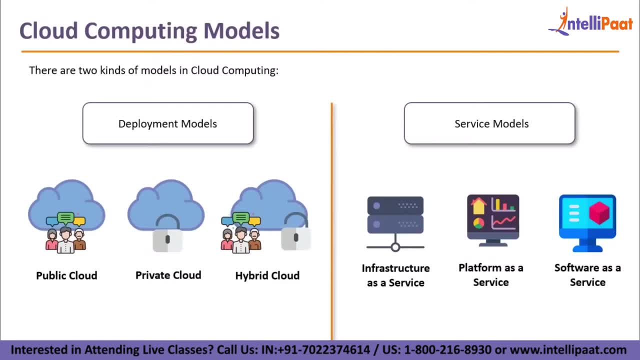 on which you basically use for solving your storage needs, is again a software as a service. Similarly, you can think of a lot of things which are basically softwares that you use in your day-to-day life, on which you can basically not upload your code. 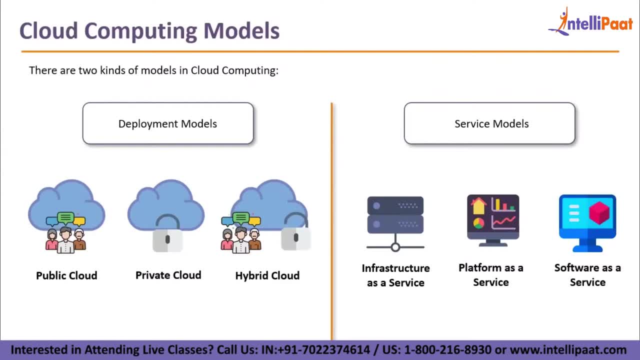 but you can actually use that software. For example, Facebook is also a software and it's hosted on cloud, So that also falls under software as a service. Instagram is a software that you use. That also is hosted on cloud. That also falls under software as a service. Platform as a service is a little. 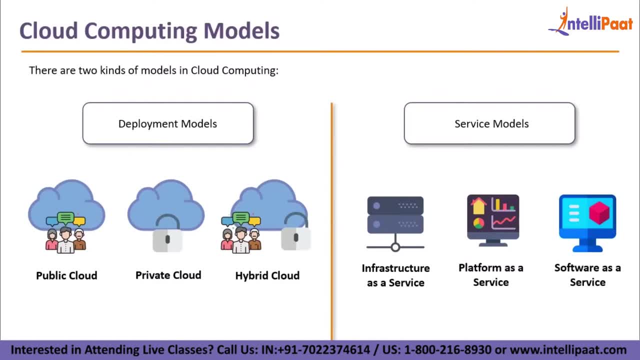 different, basically because you will be uploading code on it and that will be deployed on a server that you would not be aware of, right? So that's why it's a platform. It gives you a platform to code and that's why it's a platform as a service. And, on the other hand, 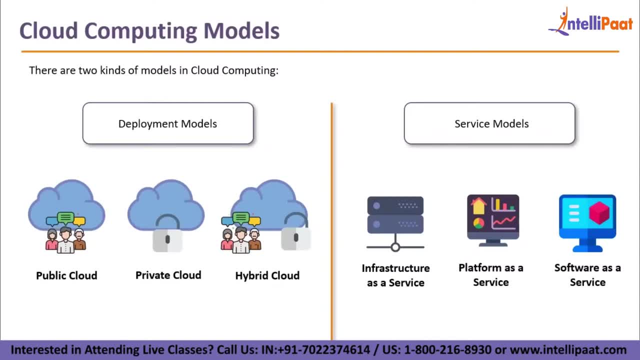 when we talk about infrastructure as a service, like I said, you get the access to the operating system. similarly, when we talk about deployment models, public cloud is nothing but when you share your code or when you share your machine with other people on the network as well. right more? 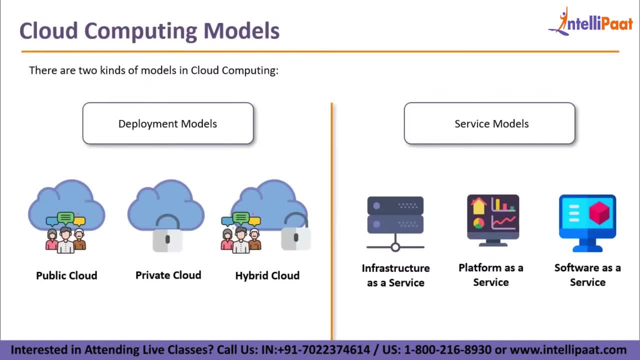 about that. i'll talk as you move along, right, but let me first tell you the difference between private, public and hybrid cloud. so private cloud is nothing but when you are, when you do not want to share your machine with anybody else, right, you just want your code to exist on the machine and 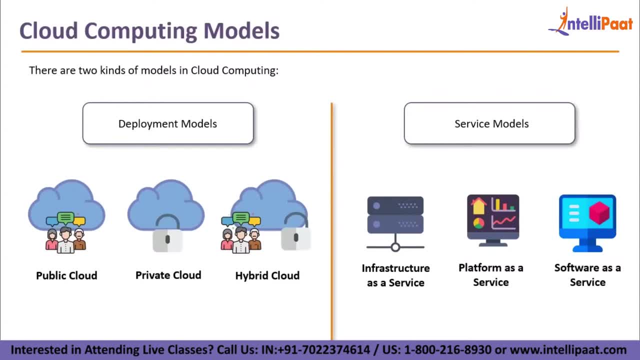 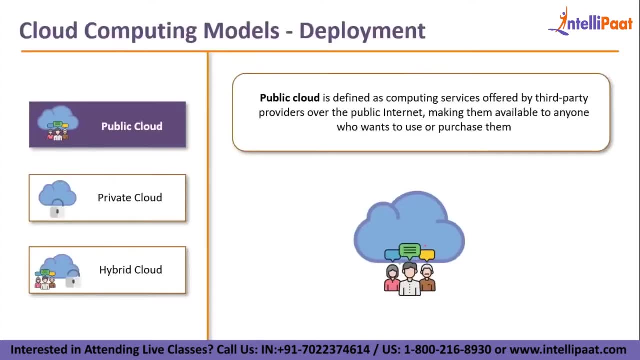 then you have something called as hybrid cloud, which is basically a mixture of both of them, right? so let's go ahead and discuss each of them in detail as you move along, right? so let's first talk about the deployment models. so the deployment models, like i said, there are public, private and 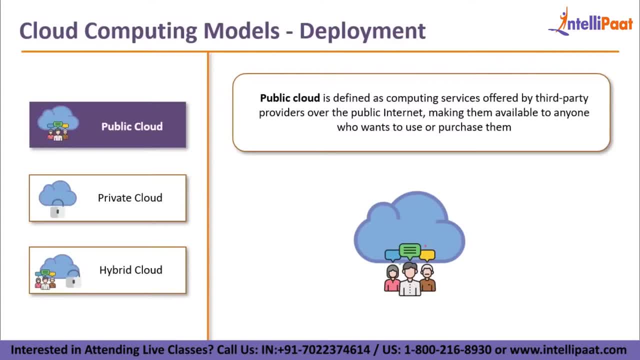 hybrid. the first one is public cloud. so what basically happens is that when you deploy a machine on cloud, when you deploy a virtual machine on cloud, it is not a separate machine which gets deployed on cloud. so what basically happens is that each cloud provider they buy machines which are humongous in size. right, it could have around 30 petabytes of storage. 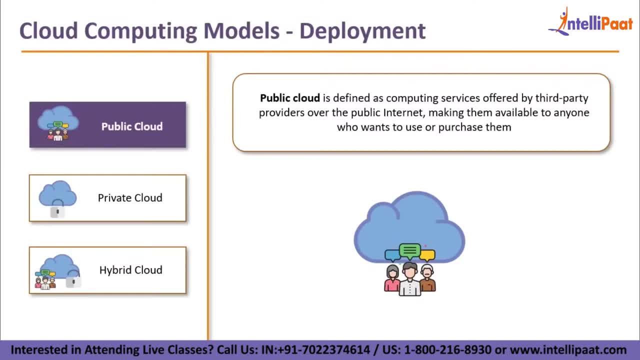 and it can have around, let's say, 200 gb of ram or 300 gb of ram or even more than that. right, so each machine has this kind of a specification. now, what they do is they install hypervisors on these machines. and what do hypervisors or virtualization softwares do, is that they launch. 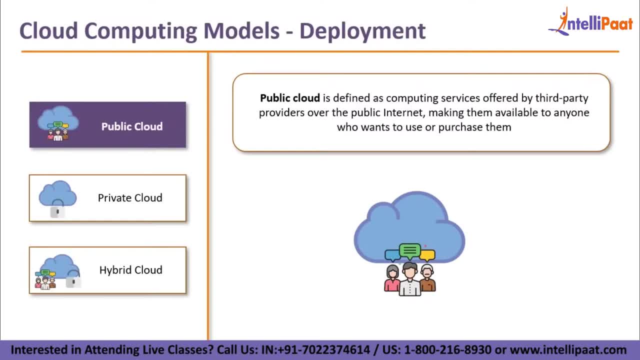 multiple machines on this very same system, right? so let's say, you launch a machine on cloud and you launch five machines on microsoft azure, so that could mean that all your five machines which are launched may be hosted on one particular server as well. that's a possibility, right so? 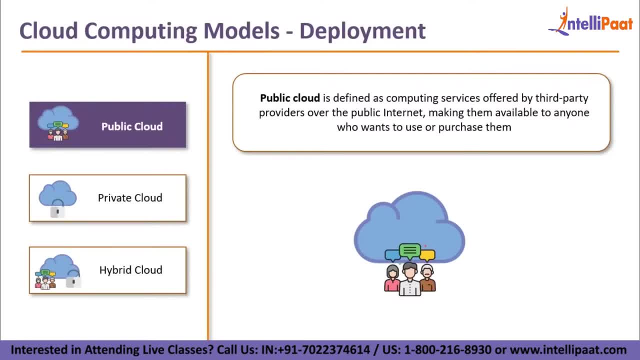 this is how cloud provides you with different kind of specification machines. they basically buy one kind of machine. they buy all their servers with one kind of specification, but according to your needs, according to what kind of specification you want, they virtualize a machine from that very server and obviously they will launch five machines on microsoft azure, so that 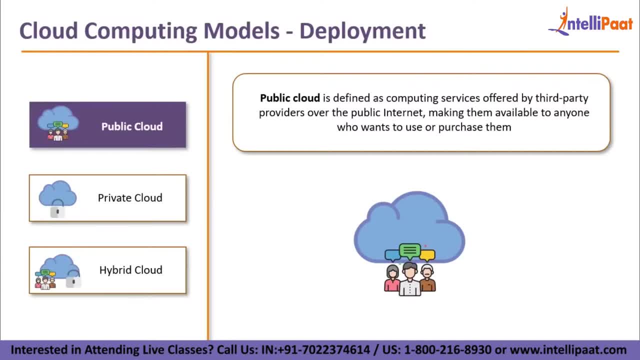 they launch more virtual machines also from that very server. if the resources are free, right. this is how cloud works. now what happens in case of public cloud is that let's say, you're launching a virtual machine, right, and you have launched it, let's say, on microsoft azure. so if there is 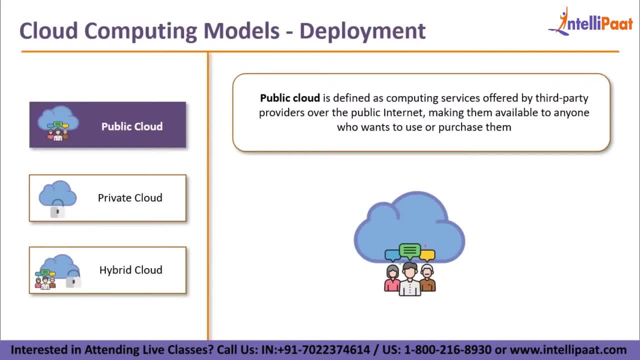 one more company. let's say you're amazon, okay, and there's one more company, let's say it's flipkart, or let's say it's walmart. so if they come up to microsoft azure and they say that you know what, you're launching a virtual machine on your cloud platform, it could be that both of your websites 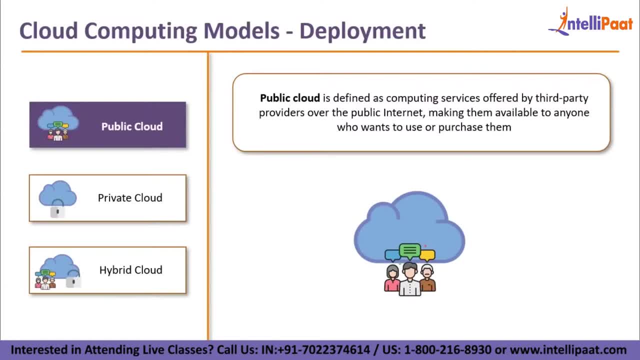 are actually being hosted from the same server right now. this might sound okay to you because you believe in your cloud provider and you know they guarantee you security to your applications. they guarantee you that no data of yours will be hacked from the other people who are also. 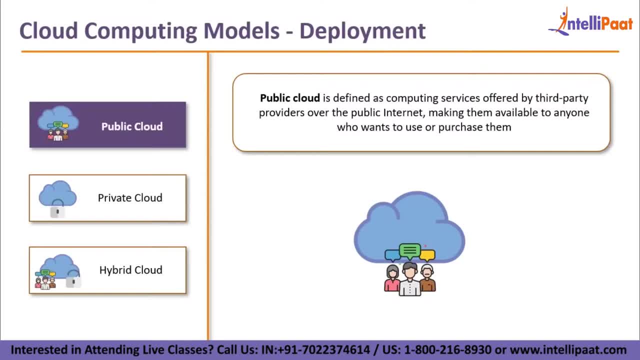 sharing the same hardware as you. but some companies, they basically say, or they have some confidential data which they do not want to share with anyone. right, so we'll come to that. but if you are okay with this kind of first setup wherein you know your application could be on the same, 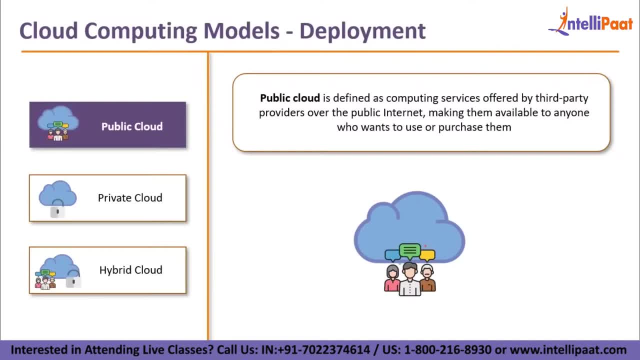 hardware on which other applications are also there or other people are also using it, then you term it as public cloud because you are on the cloud, which where all the public can basically come up and they can launch their own servers, and it could be that you are existing on the 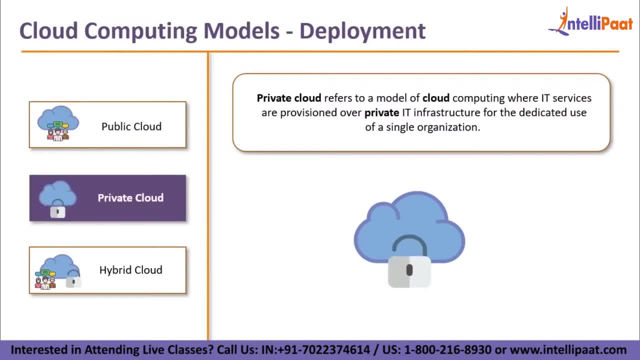 same server as well, but you don't care about that. that is public cloud. next type of cloud is private cloud. so private cloud is for those companies that i was talking about, which basically want confidentiality and they want security in the utmost manner that they can. right so, let's talk about some government agencies. right so, because 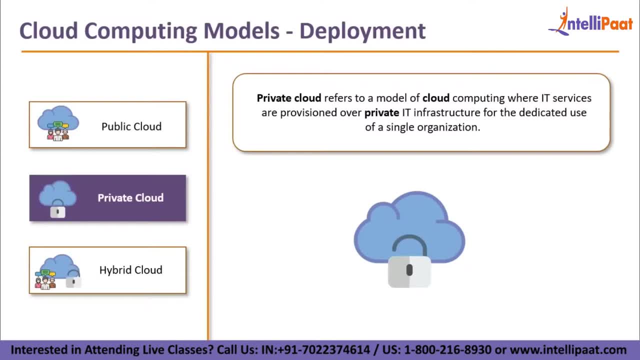 if some government agency have to host their data on cloud- and let's say they turn on to microsoft azure, for that matter. so they would say: okay, so we don't care about the money that we have to pay you, but we want security in the most highest regards possible. so what microsoft azure tells them is you. 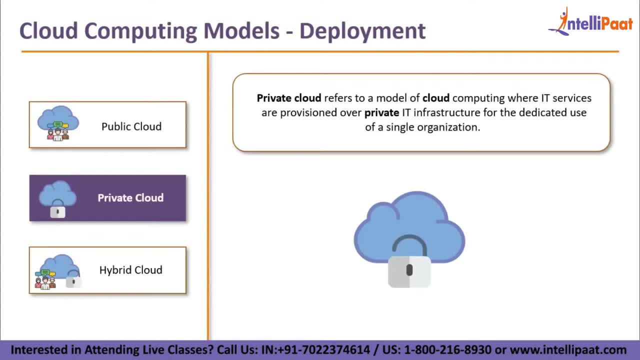 know what? uh, although we have this system in place, which is unhackable? uh, it's, it's technically unhackable. no other person who is hosted on the same server as you would be able to get into your website. but if you are still concerned because, you know, in technology actually there is nothing. 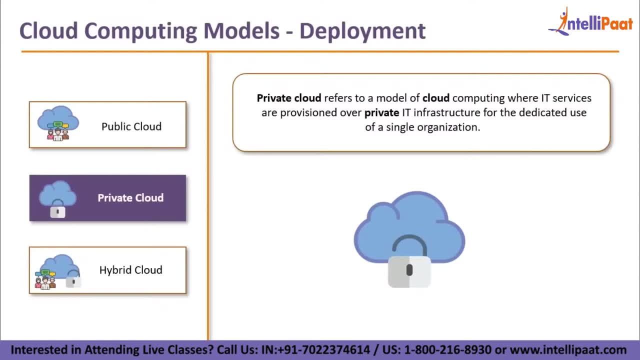 called as unhackable. everything can be hacked, right, it's just, uh, it's just hardware, right? if earlier people can like, you would have heard about people jailbreaking iphones and apple. every time it comes up with a new phone, it says it's the most secure device on the planet and 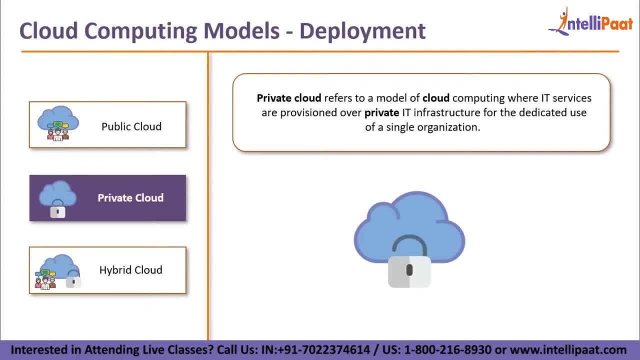 still, people manage to hack it right. so same as the situation here as well. even though your cloud provider is guaranteeing you that you know your hardware, that you own, and if there are other companies also on that hardware, they will not be able to hack into your data, still, you know the. 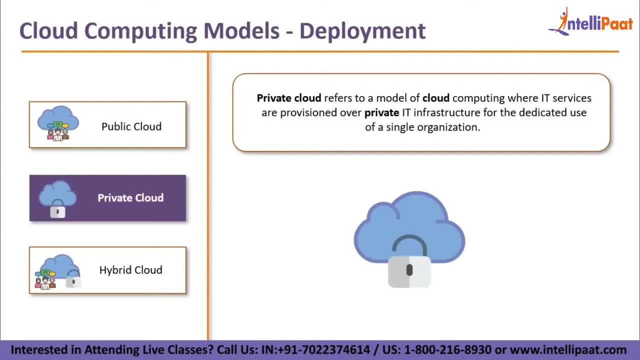 company. they do not want to take any chance, so they are being hacked. do not want to take any chance, so they opt for private cloud. so i was taking the example of government agencies which have very- you know- volatile data with them, data which is very, very confidential, so they don't take any. 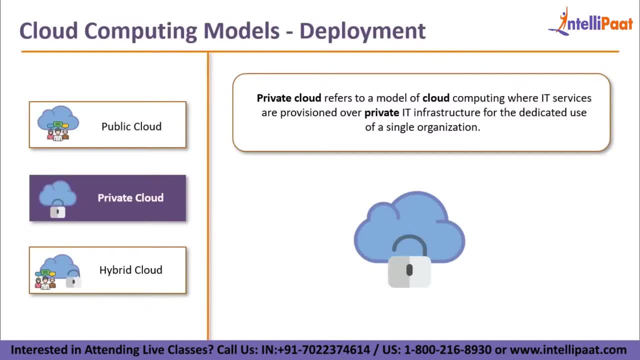 risk, they also opt for a private cloud. a private cloud basically means is that they would give you one unit of their server for your use right. you use that server as you own it. no other company will be posted on that particular server. that the cloud provider guarantees you right. so that is. 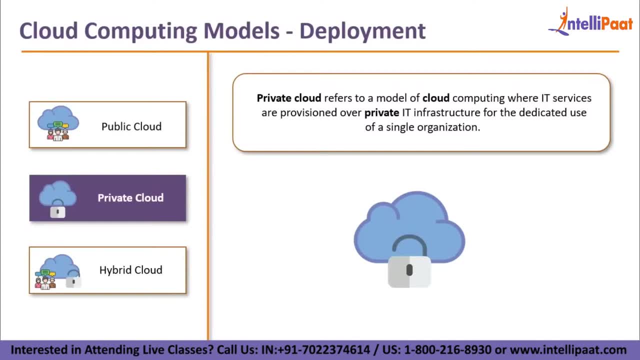 termed as a private cloud. one other way that you can create a private cloud is that you can buy your own servers right and you can set up. set them up in a data center and what you can do is you can install the hypervisor, the virtualization software, on top of it and you can use those servers as if. 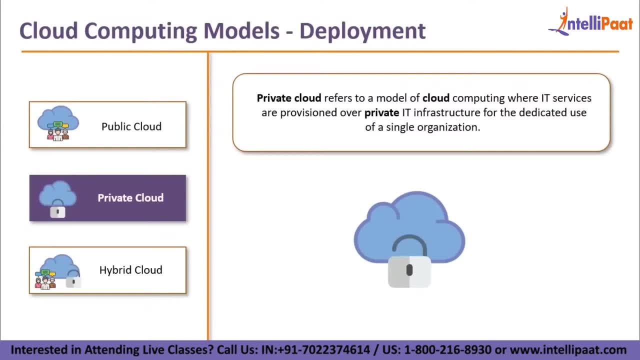 you are using any other cloud provider, for that matter, like if you use microsoft azure, you can deploy machines with various specifications. similarly, you will be able to do that in your data center as well, but the scene is over there. you have bought your own servers right on the other side of the second 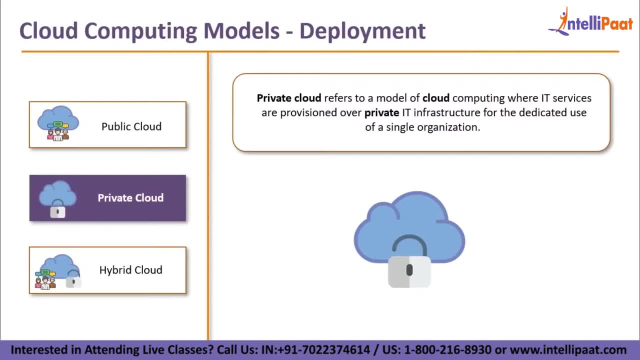 type of private cloud that i discussed with you is when your cloud provider, that is a company like microsoft, azure, they would say: okay, you know what, i can provide you a server on which i will not be putting any other company and you can use that server as your own, and that is also termed as. 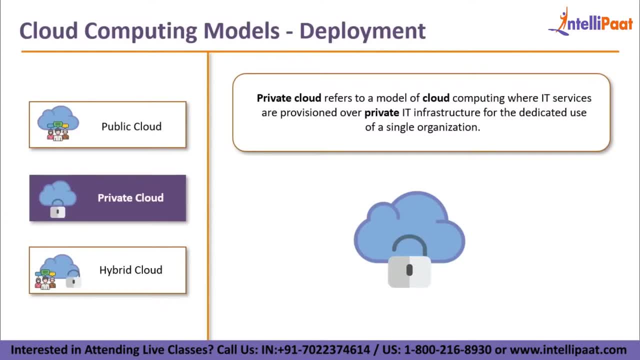 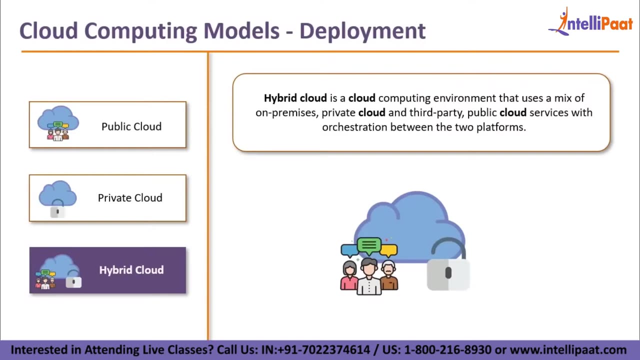 private cloud. okay, so these are the two deployment models. first we discussed private cloud- sorry, public cloud- and then we discussed private cloud. and then we discussed private cloud and then we discussed private cloud. the third type of cloud which exists in terms of deployment, in terms of how you can deploy your applications on cloud, is called hybrid cloud. now, what is hybrid cloud? as? 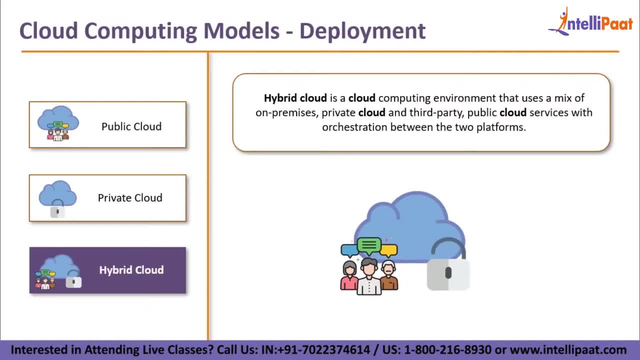 the name suggests it's basically a mixture of public and private cloud. now why would you use a deployment model like this? so one use case that i can tell you guys is: let's say: you know, because i told you, private clouds are expensive. let's say you have a distributed kind of an application. 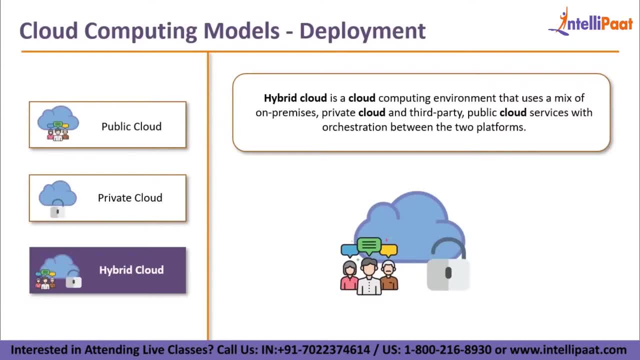 on which storage is done? on one server, the website hosting is, let's say, done on the other server. so what you do is because your website is already facing the internet. what you do is on the private cloud. you basically just store your files right and you know all the confidential data is stored. 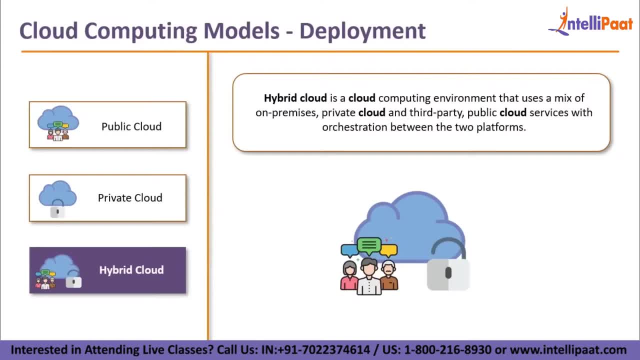 on the private server. on the other hand, the website is actually hosted on the public server because, anyways, it has to be exposed onto the internet, and what you do is you create a private connection between your server, that is, your website server, and your back-end storage, which 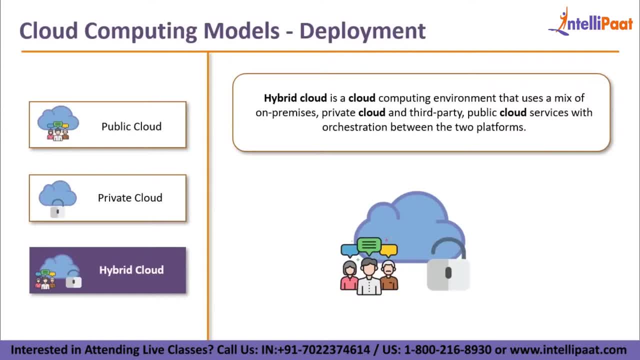 is basically on private cloud and then they interact. so it basically gives you an advantage of saving some money because now your website exists on the public cloud. so if there is anything related to website, anything related scaling related to website or anything for that matter, everything will happen on the public cloud, and if there is any extra space or extra resources, 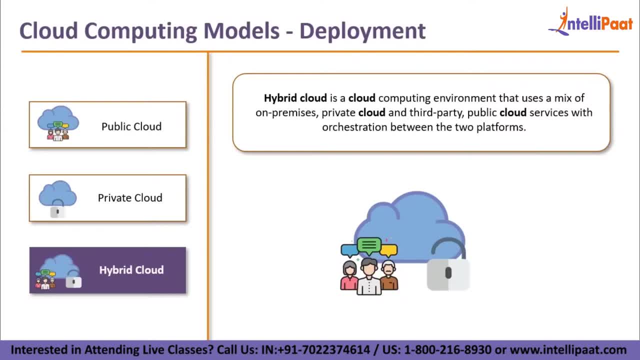 required. on the private cloud, you will actually be able to do that, and you will be able to do that. you actually have to set up a new server which will be storing the extra data for you. you do not have the option of choosing the cheaper option, which is public cloud in this case, because now 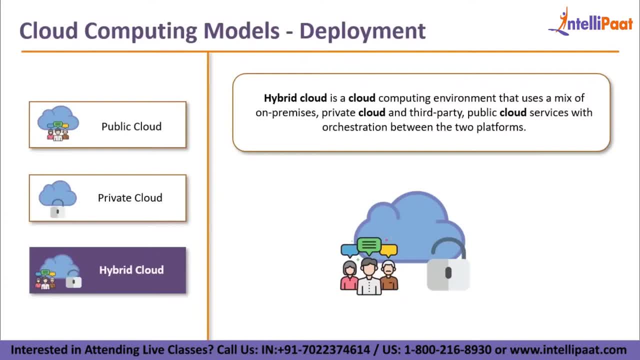 private cloud is very expensive, and the cloud provider told you that in beforehand- that if i, if you put your application on private cloud, i'll give you one whole server for your own use and nobody else will be deployed on it, right? so if scaling in that sense has to happen, but only your, 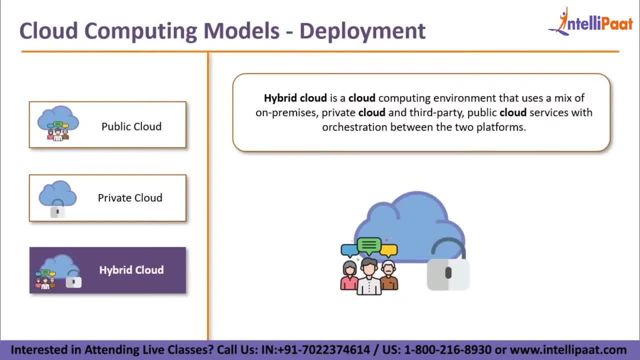 data will be stored on it and you don't have to do that. so you don't have to do that, so you do not, or you cannot have a control on how much specification do you need on that computer, because obviously you will be buying that own, buying that computer or server for yourself right on the other. 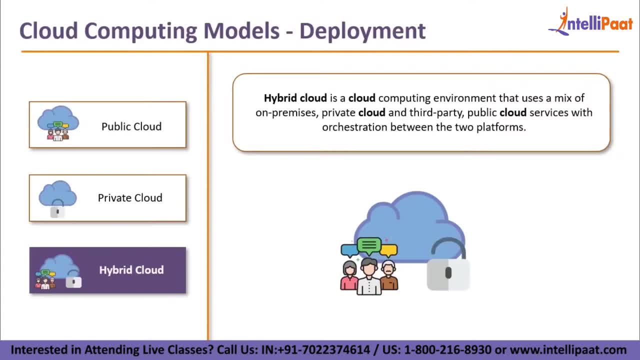 hand, if you deploy it on a using a cloud provider, that is, you buy a private cloud or you host or you ask your cloud provider to basically give you a private cloud on their own premises so they might give you a server which is configurable, but again, that is more expensive than what is there on your. 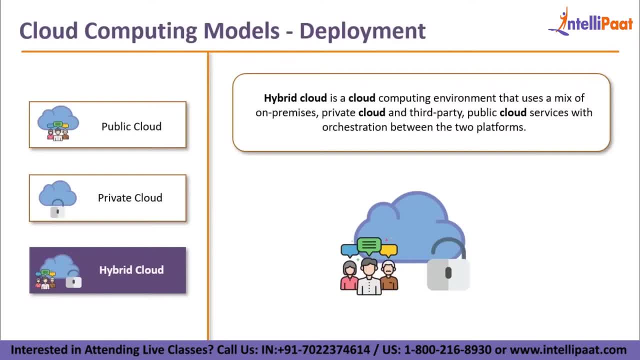 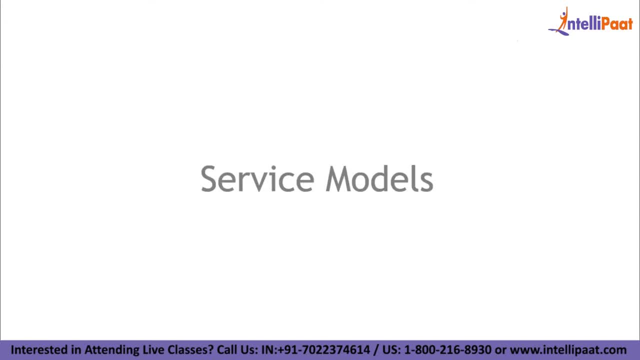 public cloud. so this is how a hybrid implementation guys works. uh, moving forward guys. now we have discussed about the various deployment models, the various ways you can deploy your application on cloud. now let's discuss the various service models which exist on uh cloud. right? so we have already discussed there. 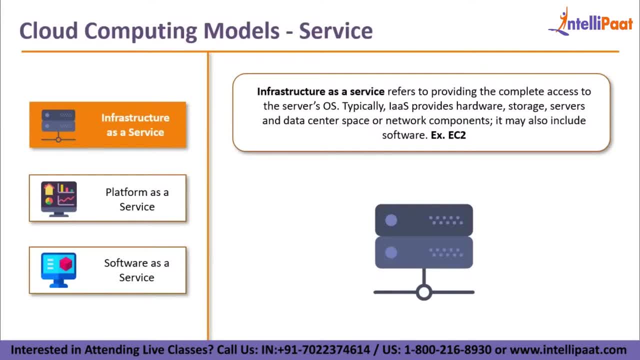 are three kind of services that can be offered to you on cloud. uh, you might get an infrastructure as a service, a platform as a service or a software as a service. now, guys, infrastructure as a service, uh, like you already know, i've already explained to you guys, when you get access to the 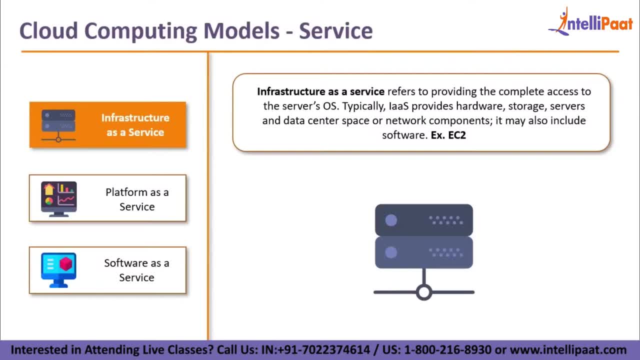 operating system right of an application or of your server, that is, you can configure or you can install anything on that server of your choice. you can install a database, you can install web applications, you can install any back-end applications. whatever you want to install, you can install, and it's your server. do whatever you want with it, right? that is called infrastructure. 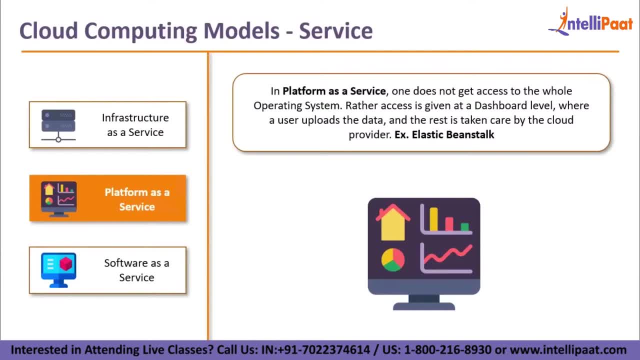 as a service. on the other hand, when you come as to platform as a service, in that case they do not give you an access to the operating system. in fact, they do not give you the access to the machine as well. I will give you a dashboard. you upload your code over there and I will host your application for. 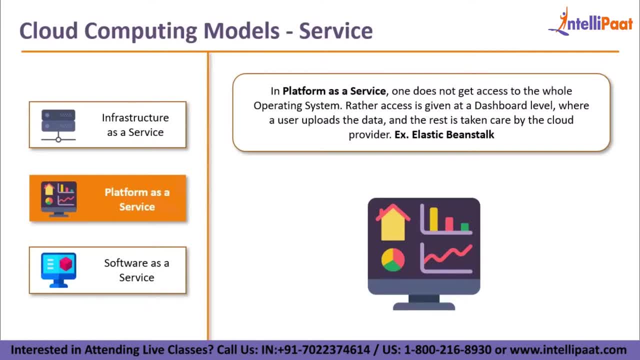 you, let me handle all the operations, let me install the required software needed for your code, let me do everything, let me do scaling, let me do everything for you, right? so in that kind of a scenario, that kind of a service is called platform as a service. okay, and the third type is: 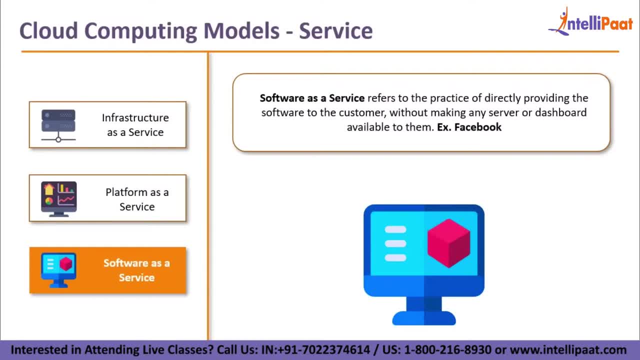 software as a service, where we have already discussed that when you get access to a software rather than a platform or the whole machine as a service, you call it as software as a service, and the examples were google drive. the examples were facebook, instagram, gmail, anything of that sort. 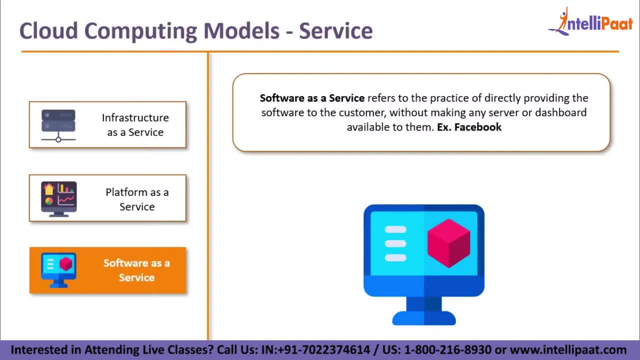 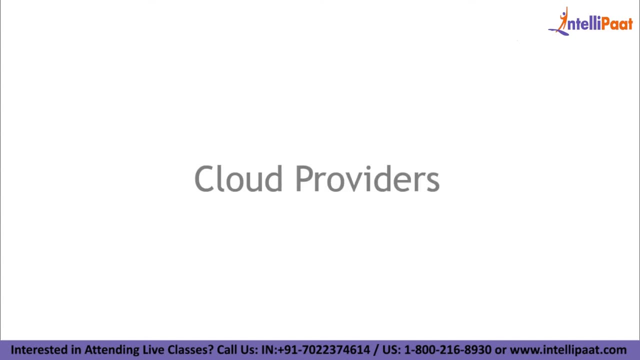 on which you you do not have the option of uploading your code to host your application. you basically can just use that application- that's termed as software- as a service. now moving on forward, guys, let's talk about who provides these kind of services right now. this was cloud. 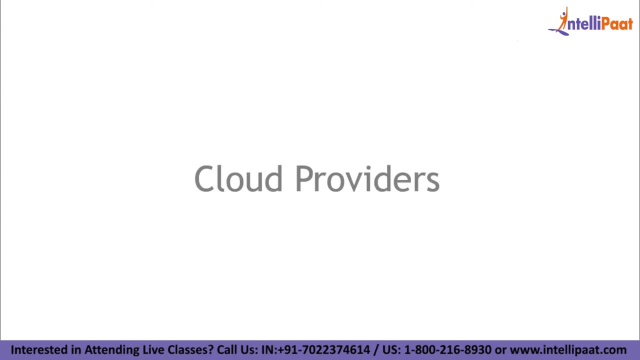 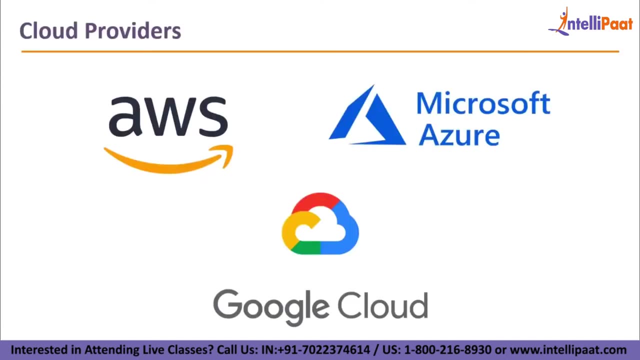 industry in general, right, but today's session is about microsoft azure. so how does microsoft azure fit into this kind of a story is? let us explore that. so, guys, the top three cloud providers in the whole world are basically aws, and then you have microsoft azure, and then you have google. 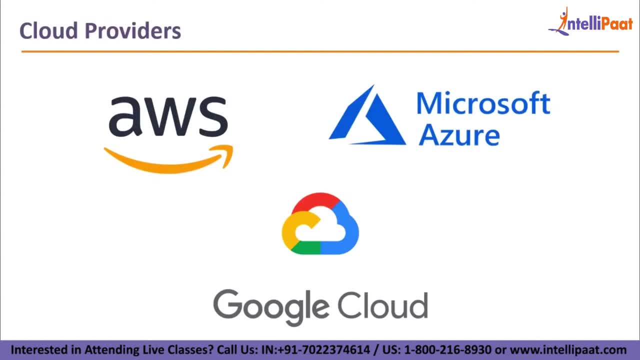 cloud. so all these three companies, they provide the cloud business model on their own infrastructure, right? so every concept that we studied is provided by these three cloud providers. and lets, lets put it out there that aws is the most used cloud provider in the world. right, it's just popularкивido the largest market share. 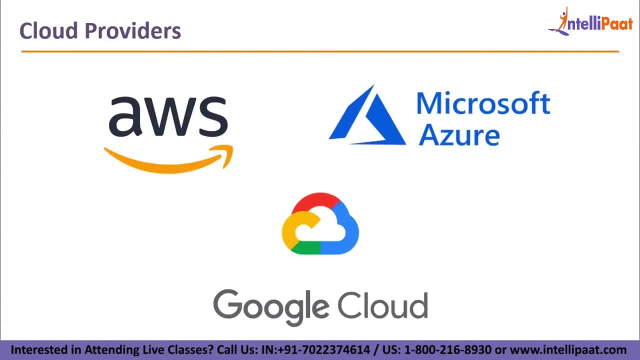 but that is not mean that microsoft is here on google cloud, a little less operational order on not that great as aws. it's just that aws was launched way back in 2006 and that's why most of the companies who got weird and do you know, okay, so they understand cloud, and they said, Ok, Let's believe them. 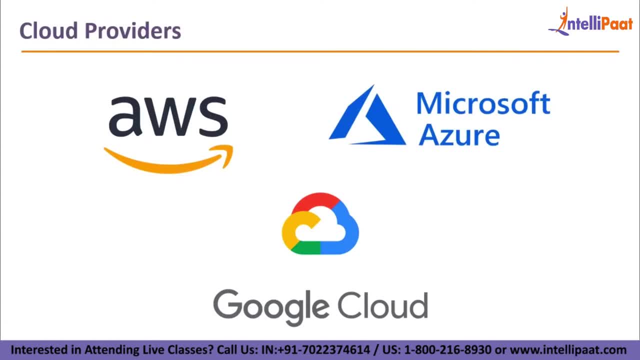 here, So it's actually going to save a lot of costs for us. They moved on to AWS and, because there was no other cloud provider at that particular time, they are now still on AWS, because now, of course, those companies that shifted at 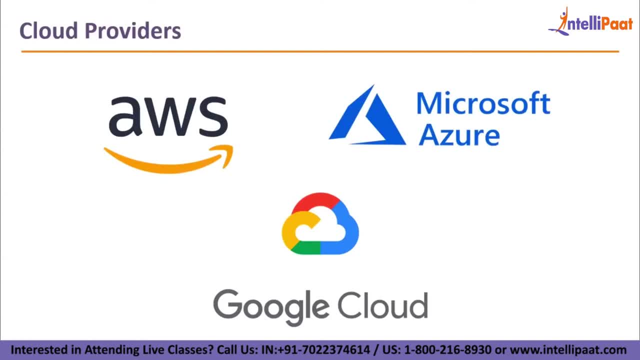 that time. they are now completely dependent on the cloud provider And if they try to migrate, that will actually cost them a lot, right, And that is why AWS has the largest market share. Reason being: it came here first And hence there are more and more people who are actually hosting their applications. 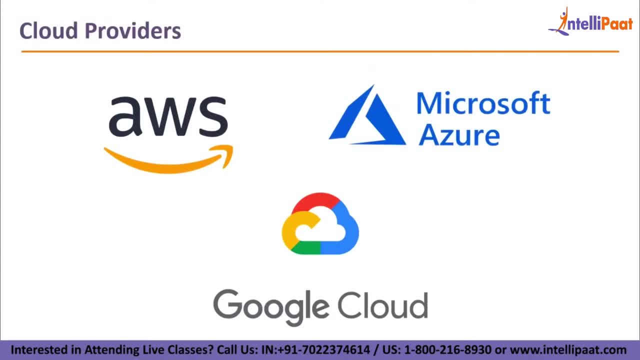 from AWS, The second largest cloud provider is Microsoft Azure, right? So, guys, Microsoft Azure was recently launched. I guess it was launched in 2012,. right, And since then it has grown a lot. right, So it has around 13 or 14% of the whole market share, right, of the whole cloud paradigm. 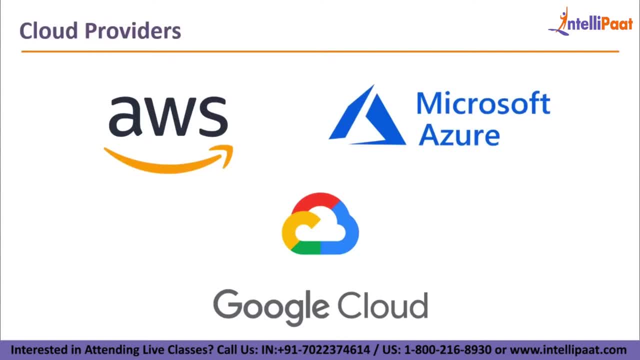 And it is growing exponentially every year. right, Why are we studying about Microsoft Azure? I will give you a lot of facts, you know, in the upcoming slides, But what I want to point out over here is the growth of Microsoft Azure is more than. 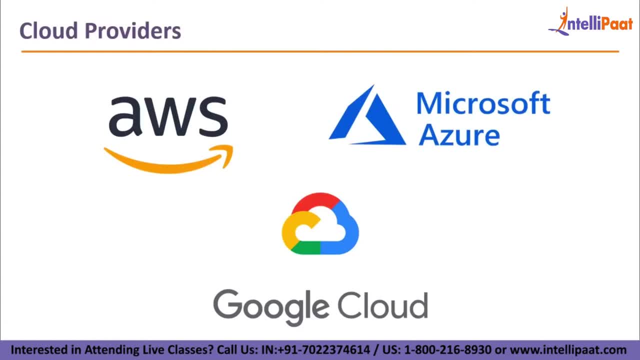 the growth of AWS right. So at the growth rate at which AWS is growing, Microsoft Azure is growing at a triple speed than the growth of AWS. So that just shows that people have started adopting Microsoft Azure, People have started using Microsoft Azure. 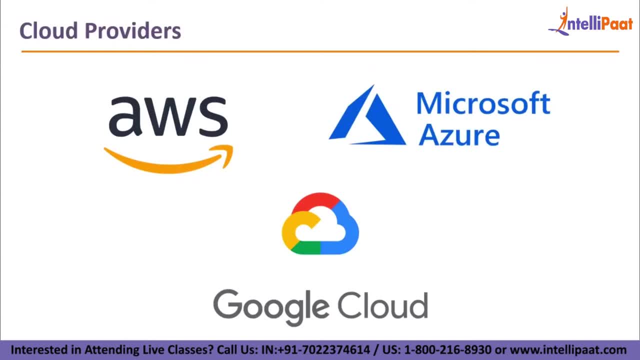 And that, but that does not point that you know people have stopped using AWS. That basically means Now, the shift that I see in the industry right now is: everyone wants their application up and running. They do not want any discontinuation in the business processes, which are running 24-7. 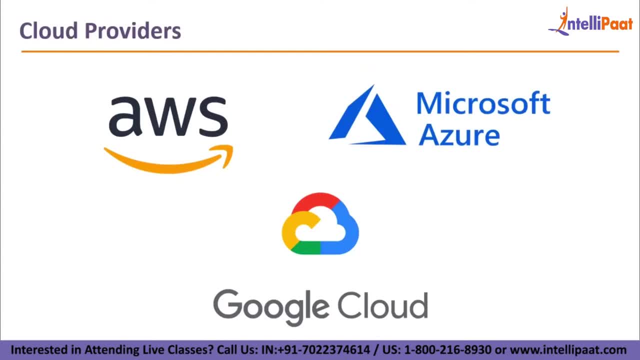 in their organization, So for having that kind of availability. so basically SLAs. when you deal with SLAs, SLAs are basically service level agreements. So when companies get in partnership with cloud providers and they say: you know, you host our cloud, 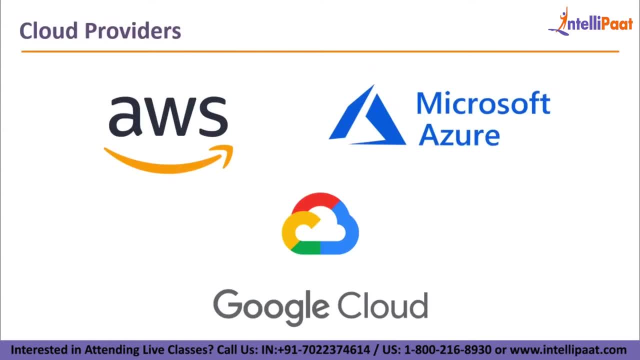 Our servers for us. They also sign service level agreements where the cloud provider says: you know, this is the amount of guarantee that I can give you that you know your servers will be up and running. So the SLAs are usually 97,, 98,, 99 percent, which basically means your cloud provider. 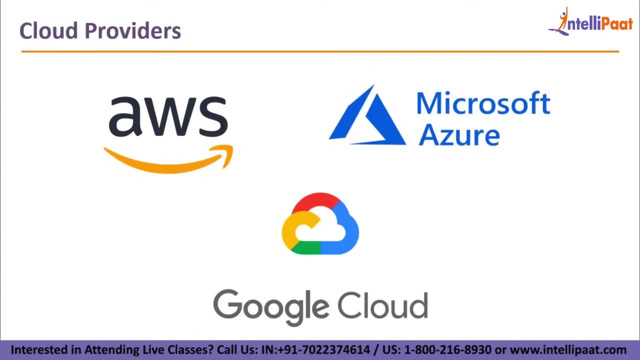 is guaranteeing 99 percent of your uptime throughout the lifecycle that you will be on that cloud provider. But you know companies they still do not like the number 99. They feel you know why should I take a risk for that one percent? 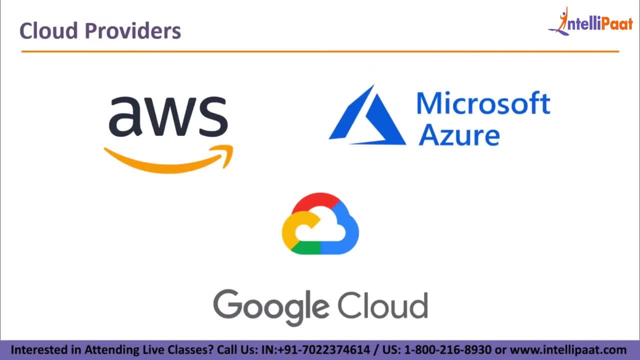 So what they do is they actually rely on other cloud providers as well, Right? So if, let's say, your application is hosted on Microsoft Azure and what you want to do is your Microsoft Azure is saying: you know your application is going to be up 99 percent. 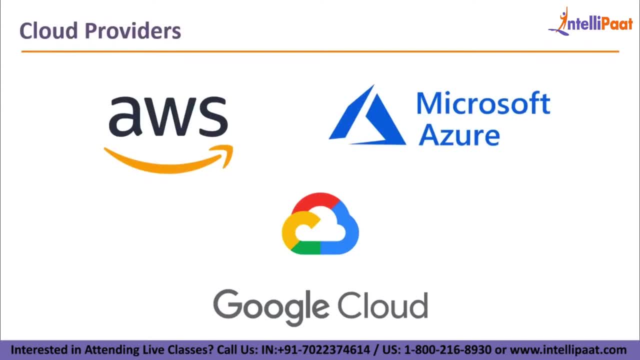 of the times. So what you do is you replicate your architecture and you deploy it on a secondary cloud provider as well, because whenever your cloud provider will be down- let's say your Microsoft Azure- your cloud computing service goes down. Right, So if that goes down, you at least have a backup which will serve as your main website. 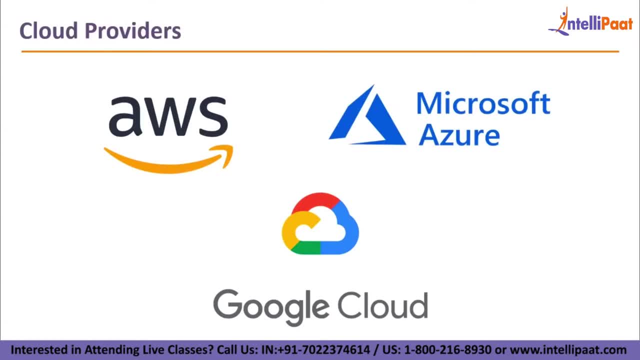 again, or your main application again, which is hosted on some other cloud provider, And hence you know, even if Microsoft Azure is down, your other cloud provider does not get affected Right, And hence your business still continues. So this is a shift that I'm seeing in the industry: that people are not only on cloud. 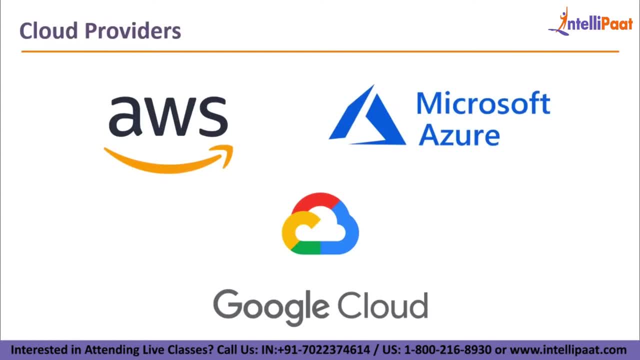 but they are now on multiple cloud providers as well, so that you know their application, their application, never go down. So, guys, like I said, the three top cloud providers are AWS, Microsoft Azure and Google Cloud. But now let's go ahead and talk about why are we learning about Microsoft Azure today? 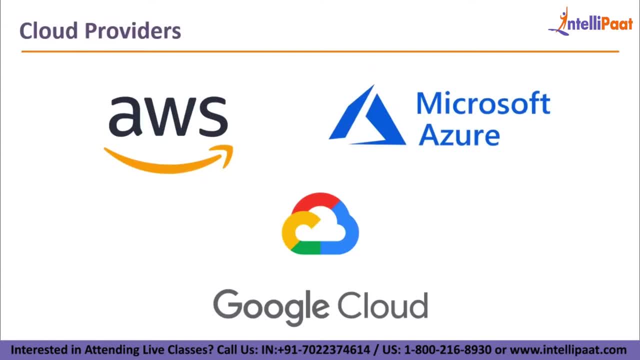 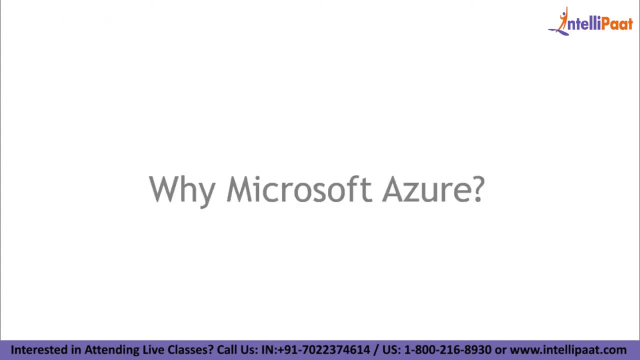 When I mentioned that you know, AWS is the largest cloud provider in the market. why am I not studying about AWS? Why am I studying about Microsoft Azure? So let me go ahead and tell you guys why, Right? So the reason for that is that Microsoft Azure, in terms of Microsoft products, like you and 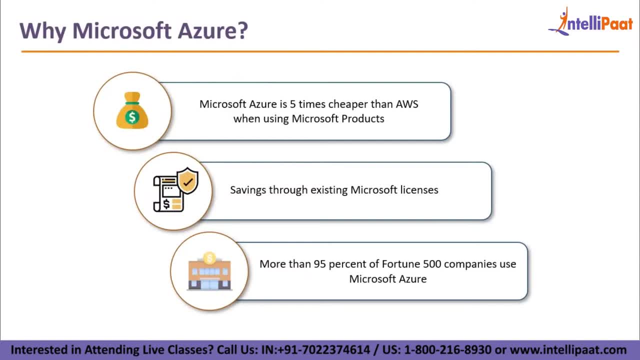 I, we both know that Right At some point of your life, in IT or at home, you would have used a Microsoft product. That's how well they have integrated, or that's how well they've designed their products, that each and every person on this planet, if they are into IT, they must have used Microsoft. 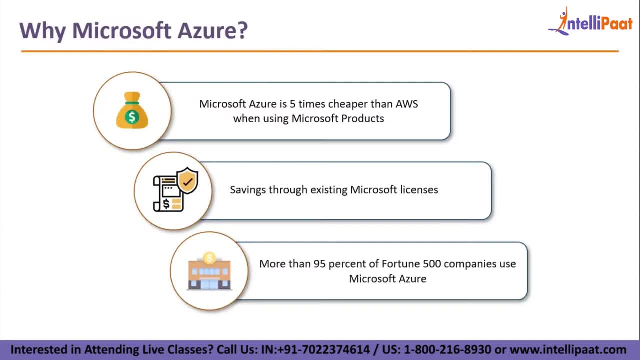 products at one point in their life Right And Microsoft Azure gives you a benefit in terms of using Microsoft products. that it says that if you are on cloud and if you want to use any Microsoft products Like Windows or SQL, for that matter, AWS- whatever price AWS gives- Azure can give you. 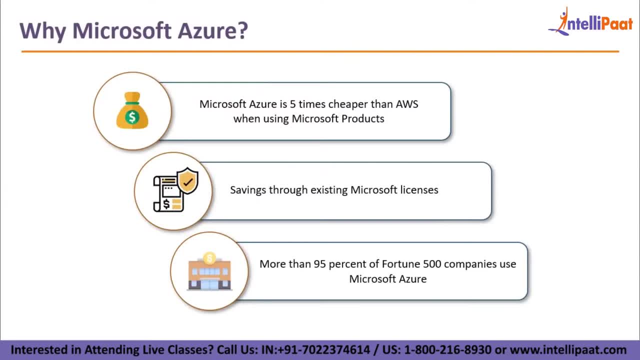 a price which is five times cheaper than that price. The reason for that is very simple: that Microsoft owns the licenses and hence a license which is basically being bought by Amazon would be, you know, costlier to them. And when they give you that license on a shared basis, that is on a timely basis, obviously. 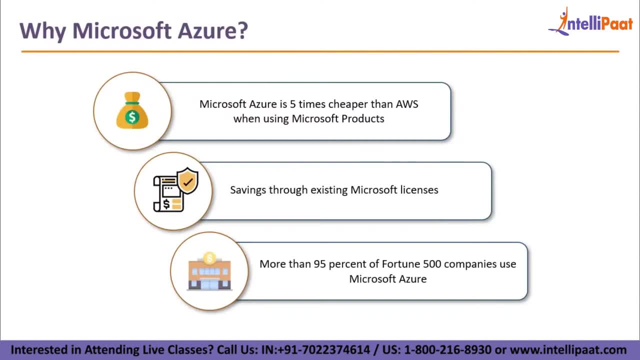 they'll charge you more, Right. But when it comes to Microsoft, they have Those charges in hand because it's their own license, Right? So what they tell you is that, dude, you know what, whatever AWS is charging you for that? 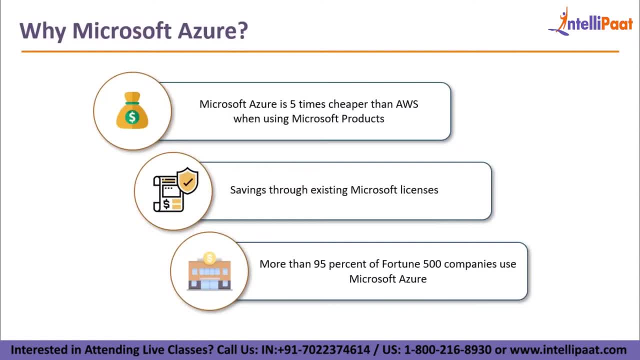 particular instance, for a product, for a software which is by Microsoft, which is running on that server, I'm going to give you that same server in one fifth of the price. So this is the first advantage that you get with Microsoft Azure, that, if you are into, 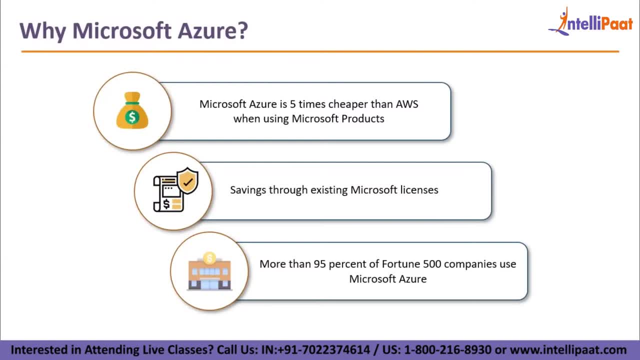 Microsoft products. if your application is using any kind of Microsoft product, you will find it one fifth of the price when compared to AWS. The second thing is that if you have Microsoft licenses, then obviously, if you are, let's say, in a business and you are using some Microsoft software, you obviously would have. 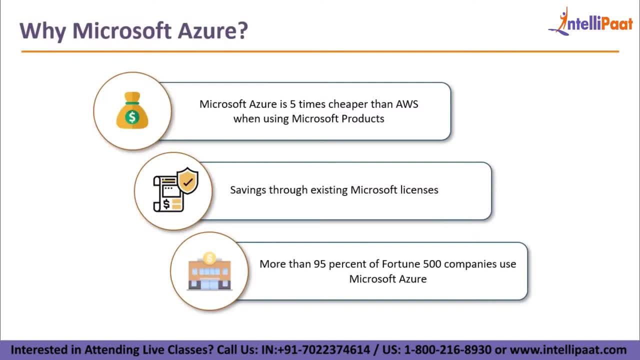 bought some licenses And when you want to go on to cloud, you know you do not want to pay for the licenses as well. You just want to pay for, let's say, the server that you're using. Why should you pay for the operating system when you have actually paid for that operating? 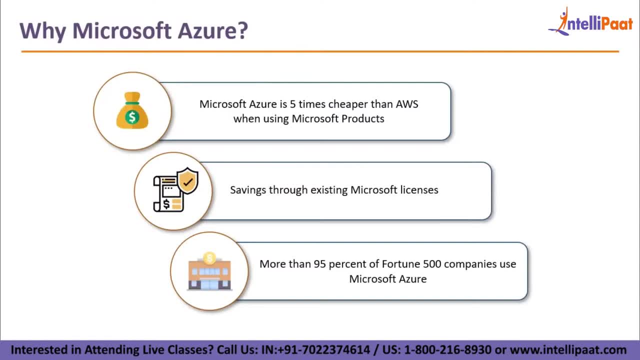 system before when you purchased it for your office laptop or your office server. So what you can do is, or what option Microsoft Azure gives you is the bring your own license option. So you bring your own license, you give the license key to them and they will not charge. 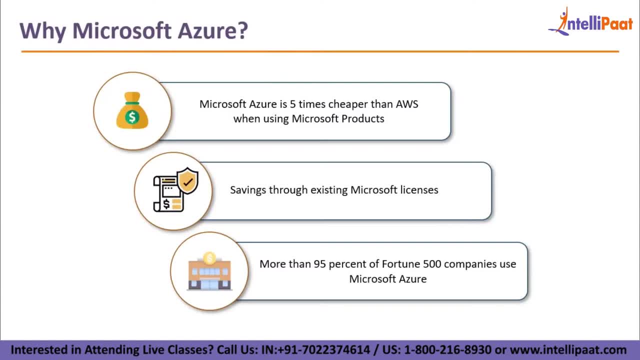 you anything for their licensing, Even the one fifth cost that they were charging. they will not charge you that if you have your own license, if you have your own Microsoft license and you bring that to the Microsoft Azure cloud, OK. so that is the second advantage that you get with Microsoft Azure. 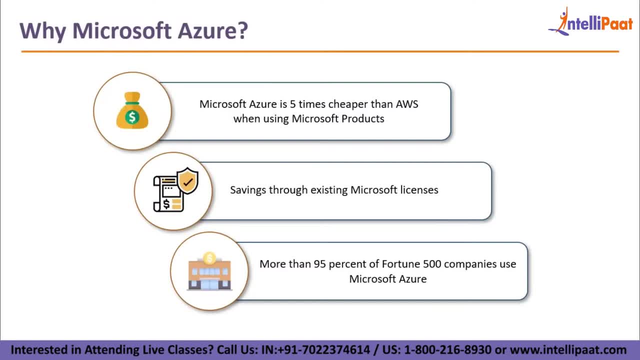 And the third advantage that you get is that Even 95% of Fortune 500 companies are actually using Microsoft Azure. Now, that could be either in the case of a primary cloud provider, or it could be using Microsoft Azure as a secondary cloud provider, or it could be using some products of Microsoft. 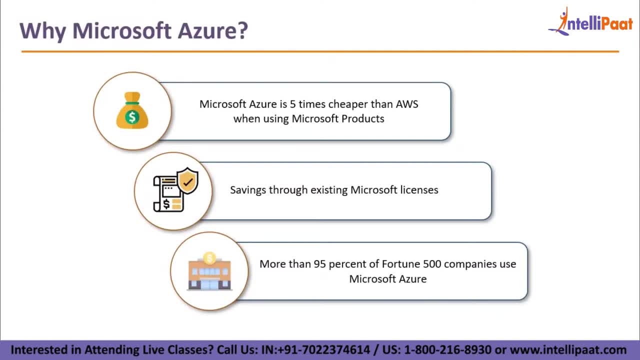 Azure. But if we talk about the companies, the Fortune 500 companies, 95% of them are using Microsoft Azure right. So if you get yourself certified In Microsoft Azure, you have a 95% probability of hitting a company. 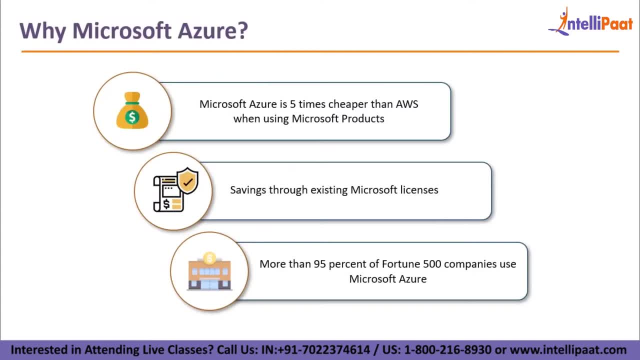 If you go to 100 companies, you have a 95% chance that you will be actually landing up in a company which will be using some kind of a Microsoft Azure service, right? So that's a pretty huge number And that actually gives you a higher probability of getting a job as well in these Fortune. 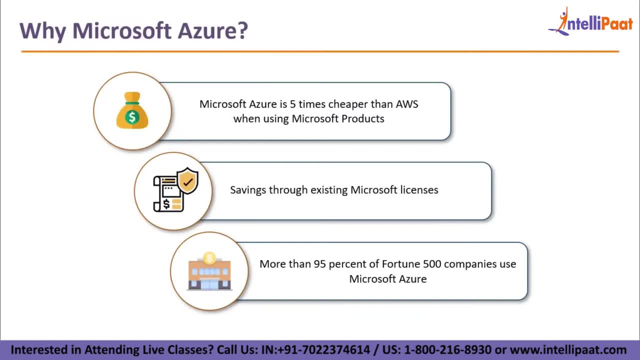 500 companies. So these are the three main advantages as to why Microsoft Azure is being preferred by businesses for their work right, And that's what companies have now started to shift to Microsoft Azure as well, And that is why it is seeing such a huge exponential growth rate when compared to AWS. 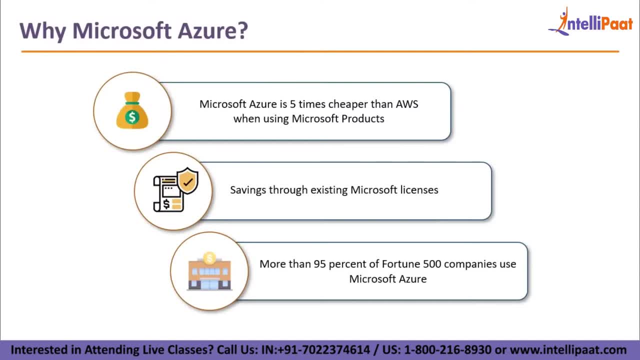 Now, now that you know that, you know why are we learning Microsoft Azure. The reason for that is obviously the chances of getting yourself a job in Microsoft Azure is more great. Now let's move on and talk about what exactly Microsoft Azure is right. 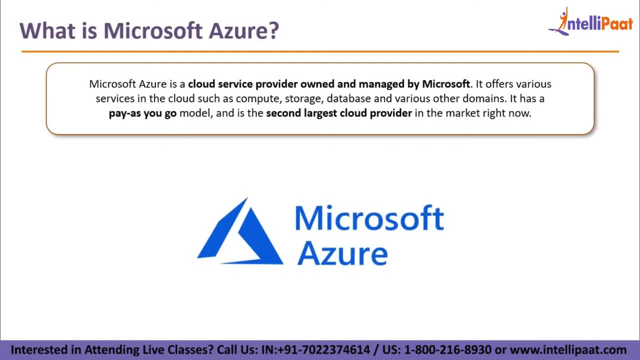 So, guys, Microsoft Azure is? It's basically a cloud service which is developed by Microsoft, right, It is owned and managed by Microsoft and it offers you its services in a pay as you go model, and it is the second largest cloud provider in the world, right? 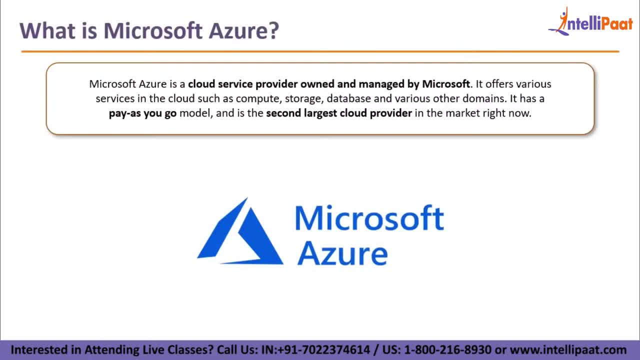 So this is what Microsoft Azure is. So whatever I've taught you with regards to the concepts of cloud, all of them are given to you by Microsoft Azure, right Along with the advantages that I told you. all of that you get with Microsoft Azure, and 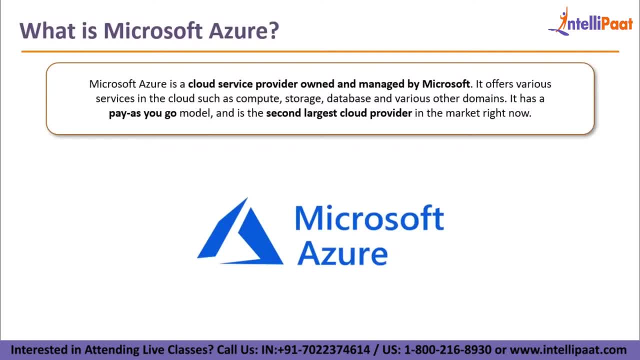 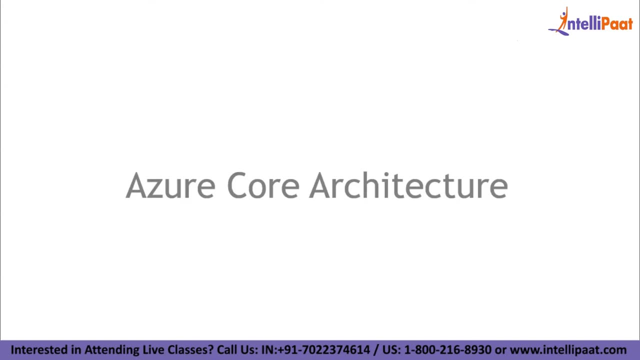 all you pay for, So that particular service is based on the number of minutes that you're using its services for, right? That's how amazing cloud is, And that's how amazing even Microsoft Azure is. right Now let's move forward and talk about how Microsoft Azure basically works, right? 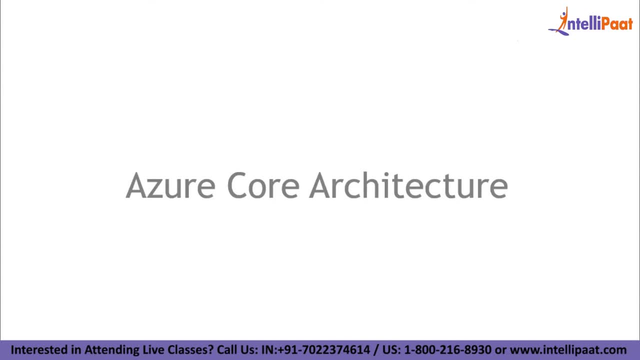 So we have discussed enough about what cloud computing is. what is Microsoft Azure? We are all clear with that. why we're using it, why we're learning it today- We're all clear with that. Now let's get into the technical aspects of Microsoft Azure and understand. 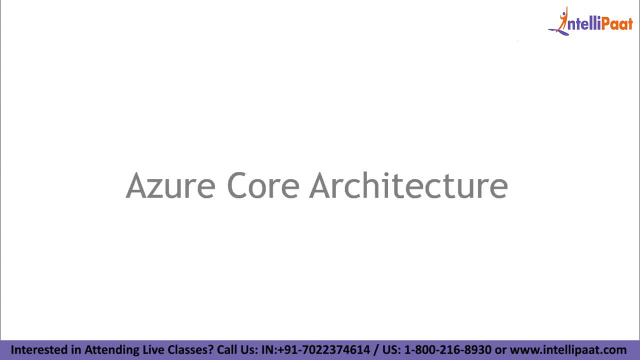 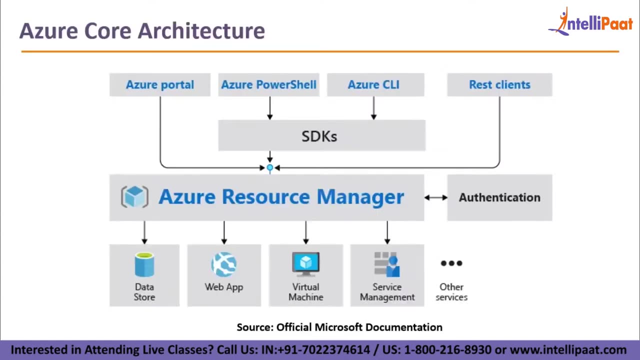 How does basically Microsoft Azure is structured in terms of its architecture. All right, guys. now let's go ahead and understand the Azure core architecture. So, guys, this is the core architecture for Azure. As you can see, there are four ways of accessing Azure, right? 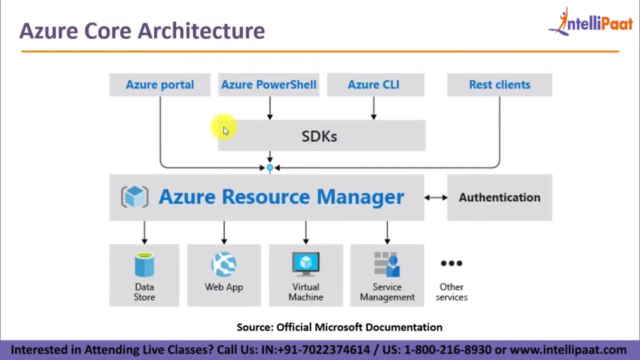 These four components are basically nothing but four different ways of accessing the Azure resources. right, So the Azure resource manager is basically a mediator Between the Azure resources and the external agents which can interact with the Azure resources. Now, to interact with the Azure resource manager, you need these four ways. 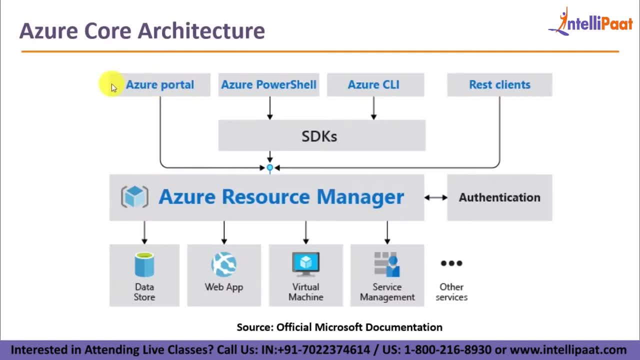 Now, what are these four ways? The first way is the Azure portal. Now, what is the Azure portal? The Azure portal is nothing but the GUI website that you get provided with right. For example, if you go to portalazurecom once you have signed up on Azure, you can basically go to that portal and 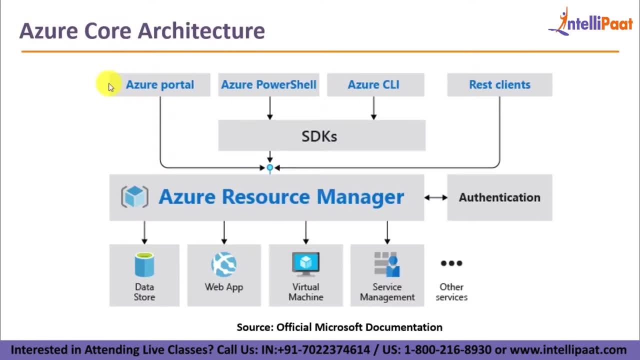 You can deploy any kind of resource that you want, right? So you can control and manage the resources from that interface. So that interface is called the Azure portal, right? The next thing is Azure PowerShell. Now, what is Azure PowerShell? So there is a thing called Microsoft PowerShell. 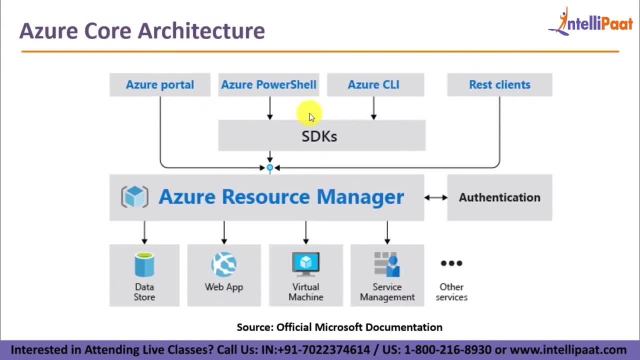 So that exists in a Windows system. So if you're using a Windows system, you can just type in your start bar PowerShell and you would be able to see what PowerShell is. right, It's a native Microsoft product. Now What Azure or what Microsoft's provide you with, is. it also gives you an extension for making your PowerShell interact with Microsoft Azure, right. 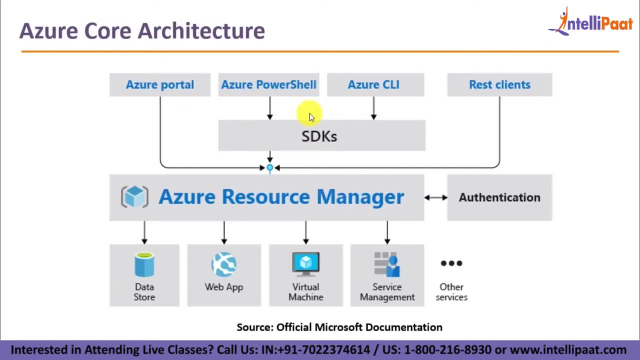 And once you install that extension, once it's installed on your system, your PowerShell would be able to connect to Microsoft Azure, which would basically give you the ability of controlling or deploying resources on Microsoft Azure using the command line. So that's Azure PowerShell. 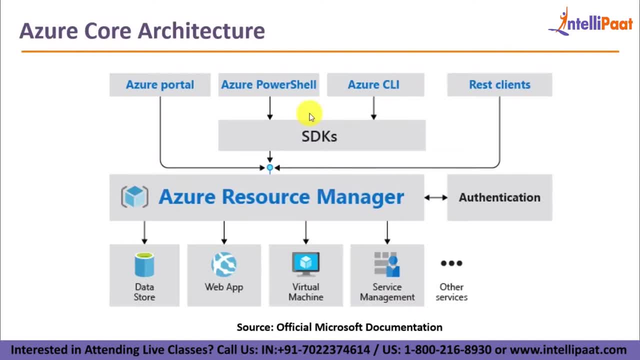 Similarly, You have something called as Azure CLI. Now PowerShell, like I said, is a product from Microsoft. Azure CLI is basically done on the DOS prompt, right. So DOS is altogether a different software which has been there since ages on Windows right. 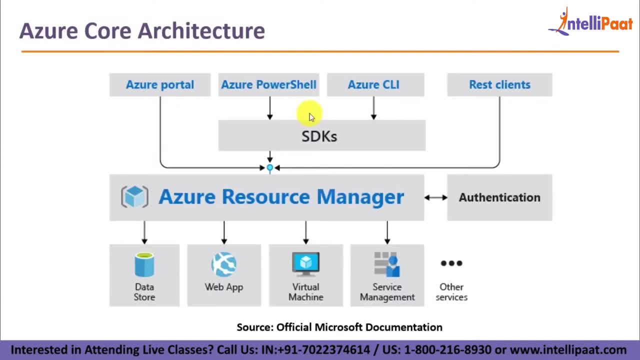 So if you want, if you're more inclined towards using the DOS prompt, you can actually install the necessary software for Azure and then you can use the DOS commands to use, And then you can also just manage or deploy Azure resources. This is a third way of accessing your Azure resources, and then you have something called as REST clients. 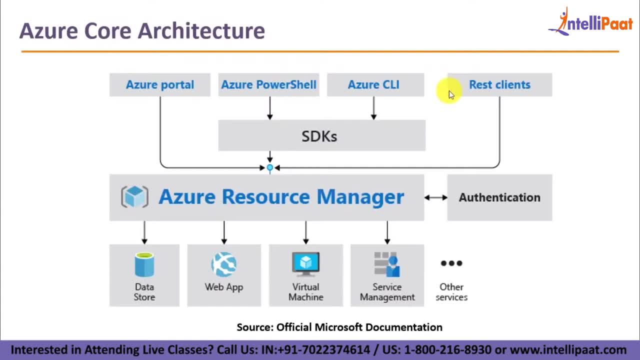 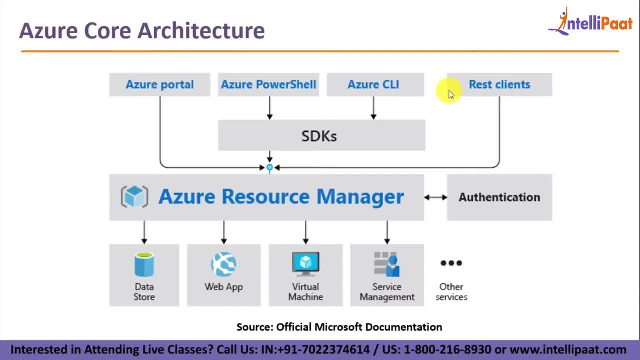 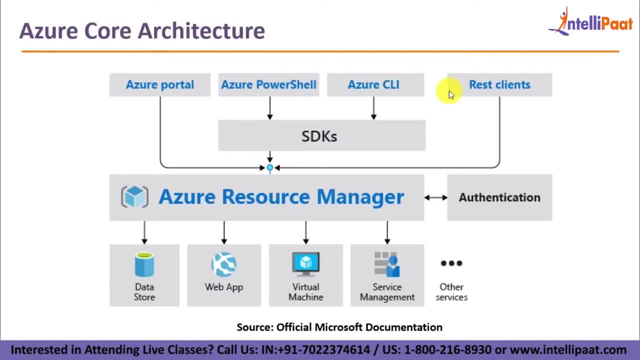 from the Azure portal, or you're not doing it- that through the PowerShell, or you're not doing that through as your CLI. what you have done is you have created your own application and you have linked your application to your Azure account and you're making. or you're making that website, or you're. 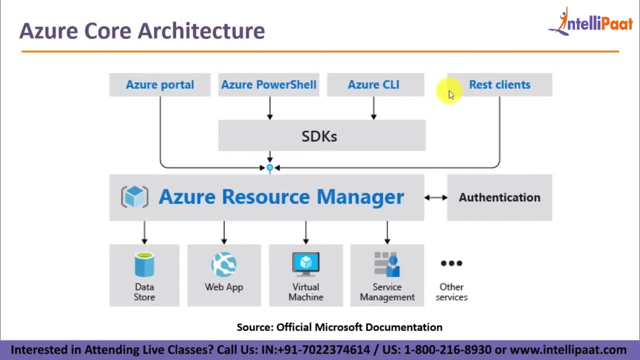 allowing that website basically to control your Azure resources, and this is possible using APIs, which are also called rest lines. right now, these resources, in case of Azure PowerShell and Azure CLI, they would interact with the help of SDKs to connect. was your resource manager, your Azure portal? any? 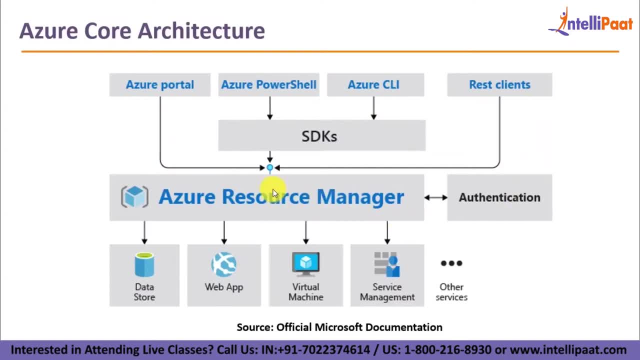 rest, clients can directly interact with the Azure Speaker 5 resource manager. and what is an azure resource manager? like i previously stated, it's nothing but a mediator. so, basically, what happens is all the resources which are deployed on azure they are. they are not directly accessible by the user, even if he's using the website or using the power shell. 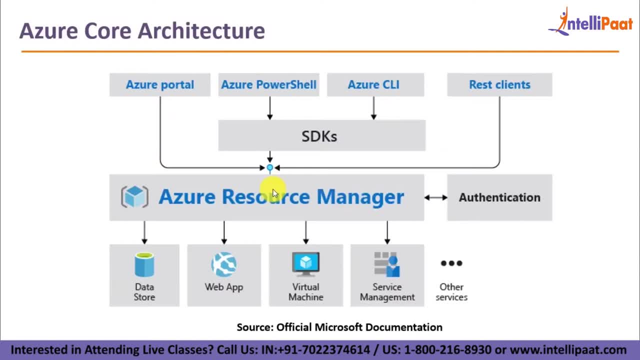 or using the cli or using the rest lines. every request has to go to the azure resource manager, and what the azure resource manager does is it basically authenticates your request. it will check whether you, as a user of a microsoft azure account, have the necessary permissions to do a certain. 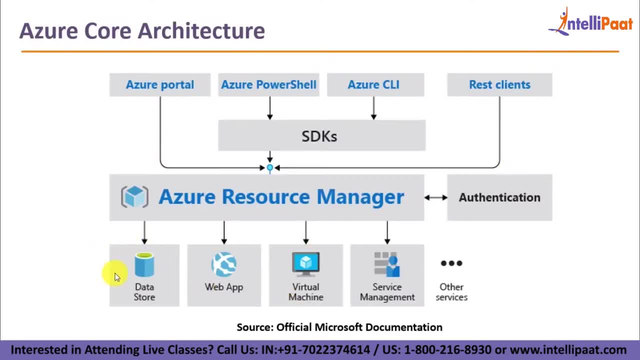 task which you're trying to do with your application. for example, when you create a microsoft azure account, you would have the option of creating multiple users in that same account so that multiple people can work on your own account. for example, let's say you're start a startup or you open a startup right and now you've hired a tech team. now what you want to 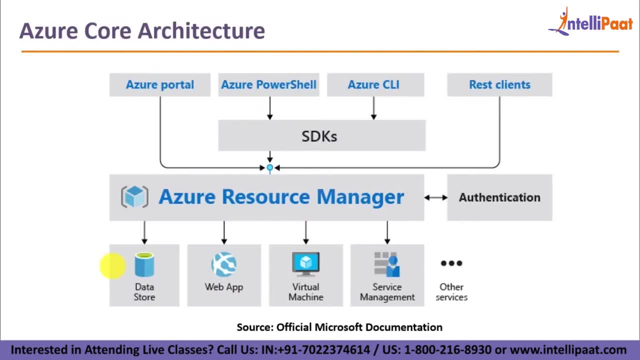 do is you want your cto or the person who's going to be managing your tech team, uh, the admin access of your azure account and, on the other hand, the developers, who probably? let's say if, if one of the developers is going to work on the azure storage, right, so you just want him to access your storage. 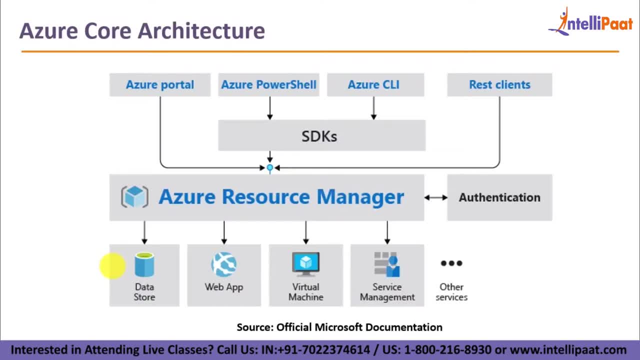 you don't want him to access your vms or any other kind of azure service. uh, so what you can do is you can create a user and you can give definite permissions as to what he can access and what he cannot access. okay, now, how will this be helpful? now, let's say, your technical manager. he signs in. 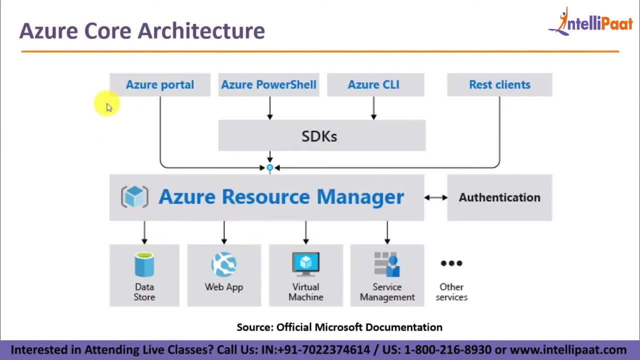 as a user right and he signs in, let's say, through the azure portal, and then he tries to deploy a vm resource or a virtual machine, or he tries to use the storage account. he would be able to do so. why is that possible? because he has the permission to do so and that's why he has the ability to do so. 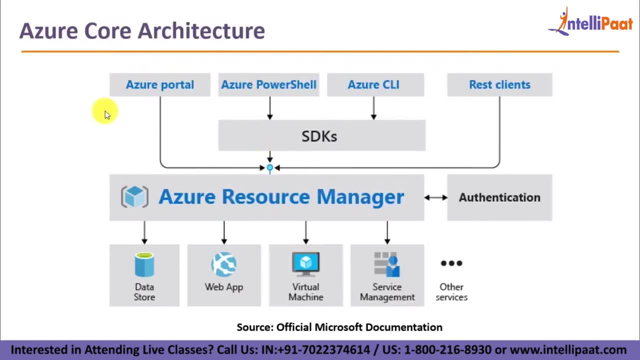 and he's able to do everything that you have given him, and he'd be able to do everything that you can do. on the other hand, let's say now your developer comes in, he also logs in through the azure portal, he also sees everything which is there, right, but the moment he tries to deploy a virtual machine, 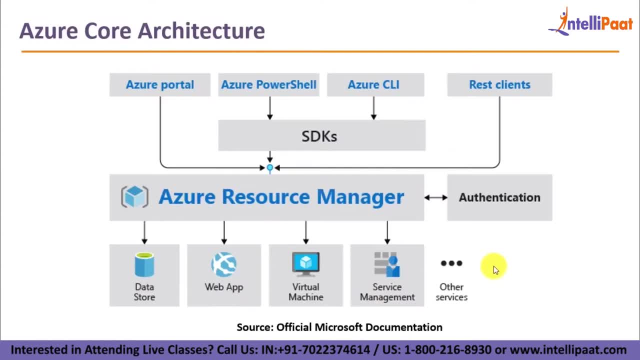 because he has to go through all his requests would be going through the azure resource manager. when the azure resource manager authenticates this guy and sees whether he has the permissions to so, the authenticator will basically say no, this guy does not have that permission. so azure resource. 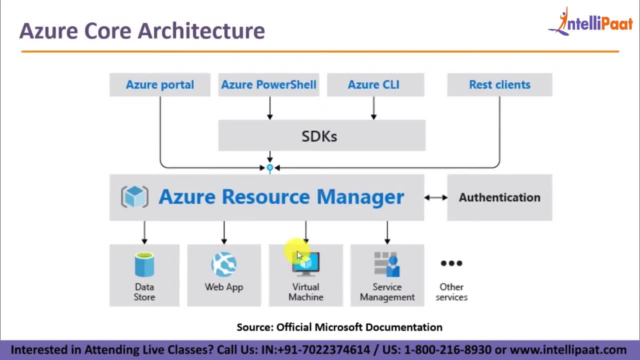 manager will not take a request forward. it will basically revert you back with error message saying you do not have the sufficient permissions to carry out this task right, and this is the sole reason we need a mediator between our azure resources and the and the various ways through. 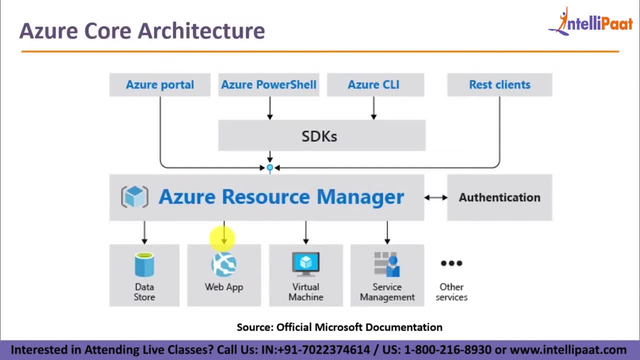 which we can use azure now this would be the same case with azure powershell. this would be the same case with azure cli. when you use azure powershell with your azure account, you obviously have to enter your credentials. in case of a developer, he will be entering his credentials that you have. 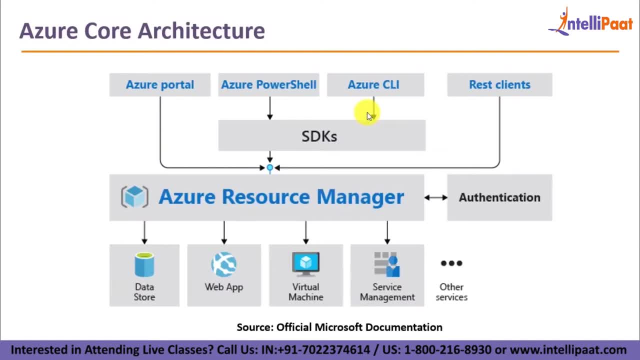 given to him, right, and those basically just have the access to the storage. and again, you would also get the same kind of message in azure powershell. similarly, you will get the same kind of message in azure cli and even in the rest. you clients, right. so when you connect your website to your azure account, again you will get a key. 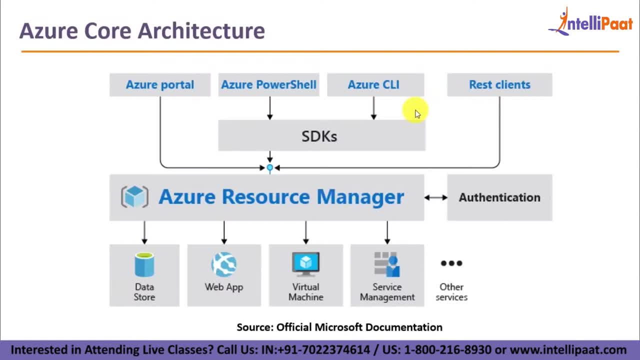 and a secret access key right, or, in other case, what you'll have to do is you'll have to include some metadata on your server on which you're hosting that website, and that metadata would basically authenticate you to the azure account. so for every user, you get a different kind of 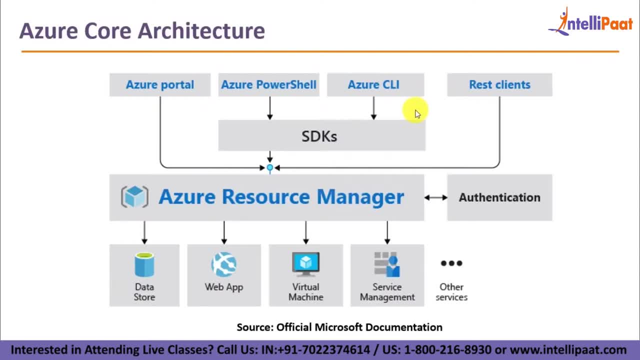 credentials for your metadata. in case of your developer, you will get a different set of credentials and those credentials would basically, when they'll be authenticated, they would get, or they will inherit, the same properties or the same permissions that the developer account has and, accordingly, your azure resource manager will authenticate and check whether you do you do you. 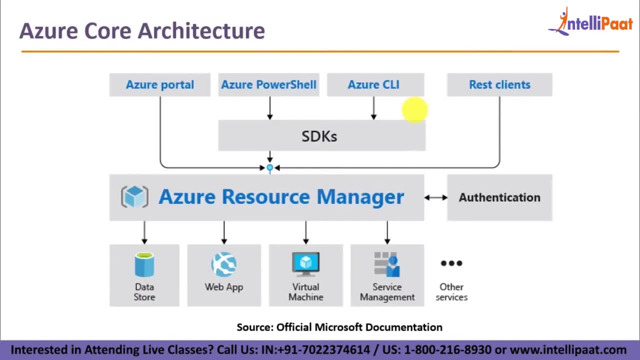 have the required permissions, or not, right, and accordingly you would be able to do the operations. so, guys, uh, summing up or just revisiting what we just studied, so there are basically four ways to access azure. you have azure portal, azure powershell, azure cli and you have rest clients. 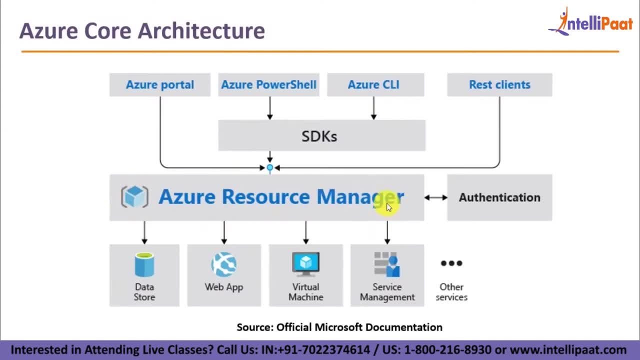 right all of these. they interact through the azure resource manager and the azure resource manager based on what kind of permissions you have. it basically routes your request to the necessary service and carries out the task for you, right? so this is a gist of how azure works in the back end. 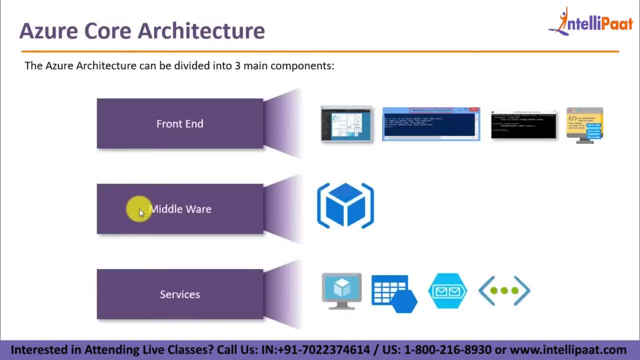 now let's move forward and talk about the front end, the middleware and the services. right, so the front end as a whole is the middleware and the services. right so the front end as a whole is the. as we discussed, there were four ways of accessing azure uh services, which were: this is the azure. 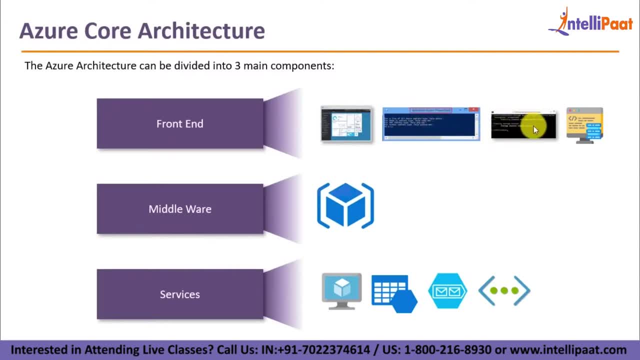 portal. this is the azure powershell. um, this is the azure cli, and then you have the rest lines. the middleware was nothing, but it was the azure resource manager. we'd be discussing that. and then you have the services. uh, that we'll be discussing in a few moments. 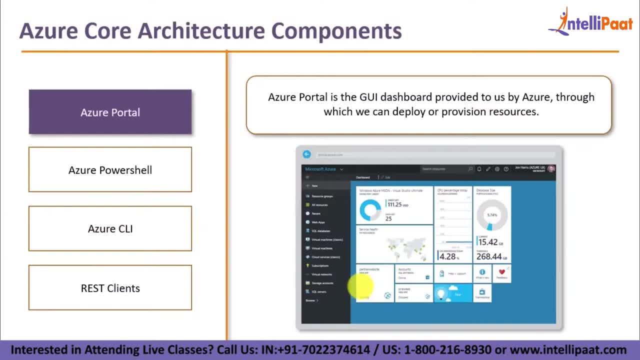 right, so let's start off with the front end part, the front end components. so what is the azure portal? so, guys, the azure portal looks something like this, right, so it's a g? ui component that you get on your web browser, and on your web browser you can, basically, you can. 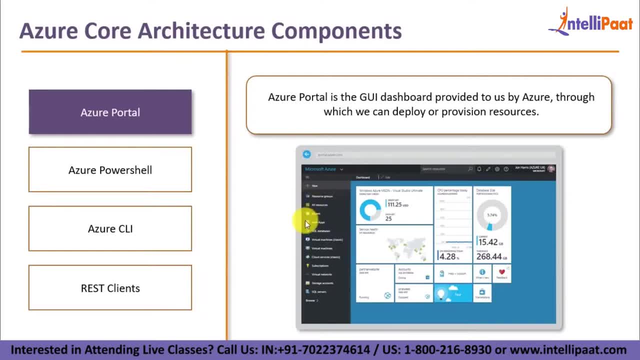 see that on the left hand side, you have things as all resources. you have web apps, you have sql databases. you can just select the service that you want and you can subsequently launch it. we'll be discussing more on this as we move along. i'll be showing you guys the portal. i'll be showing you. 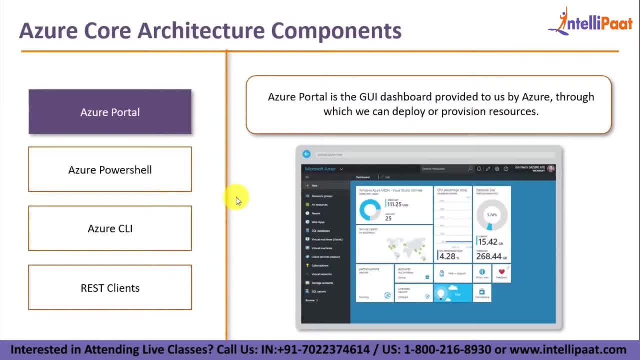 guys how you can use it to deploy resources. for now, we're just understanding what the azure portal looks like, and this is what it looks like. right on the right hand side you can see that the azure portal looks like this and you get all kind of widgets. so these are widgets. these are called. 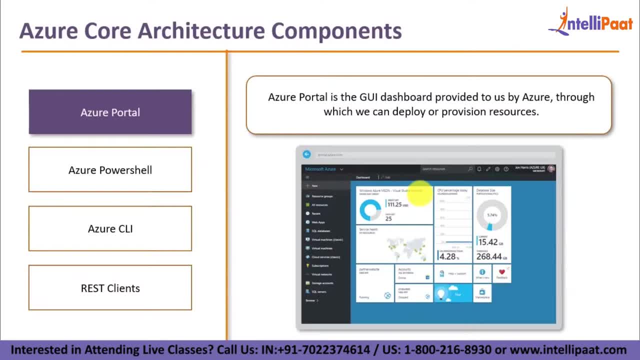 widgets which show different kind of information, right, so you'll have the option of including these widgets on your dashboard. more on this we will talk as you move along in the session. so, guys, this was the azure portal, this is the azure powershell. so i told you, guys, microsoft. 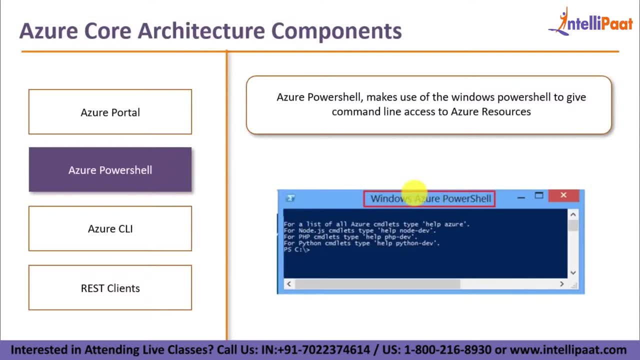 has launched its own command line, which now comes with windows integrated, which is called powershell. if you want to use that powershell with your azure account, what you'll have to do is you'll have to download some libraries which will help your powershell to basically. 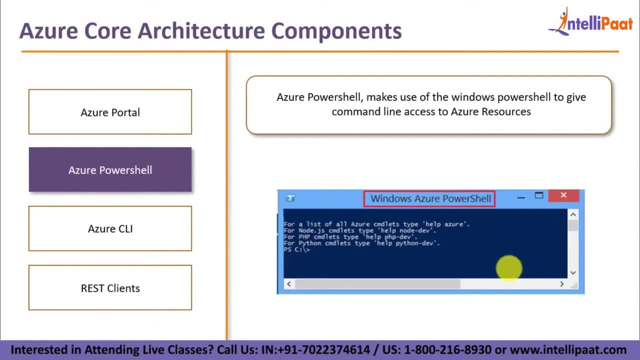 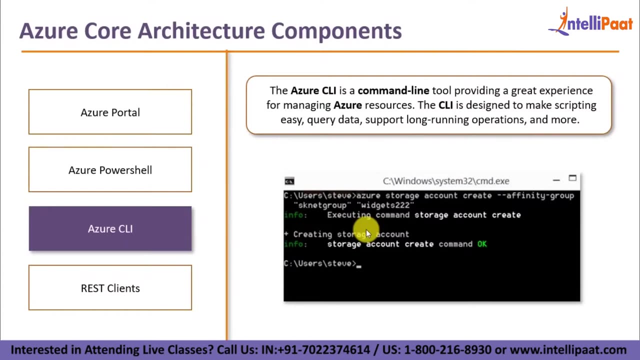 connect to azure and once you do that, you would basically see something like this windows azure powershell and now you can enter the powershell commands, which should basically help you to connect to your azure account and carry out whatever you want in a command line fashion, right. similarly, if you are into dos, you can actually go ahead and use azure cli, so dos. 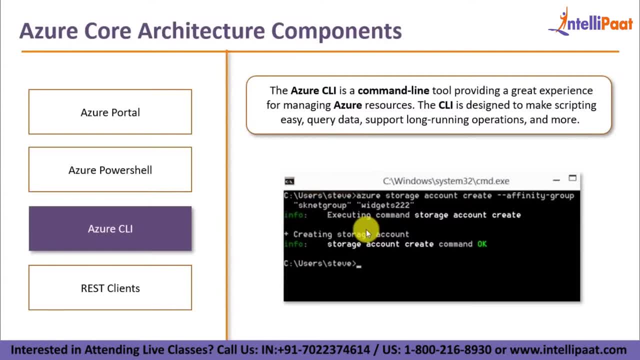 commands are different from powershell, and there could be a command line that you want to use in a scenario wherein you're better at dos commands than your powershell commands, and if that is the case, you can actually go ahead and just install the libraries for azure cli, and then you can. 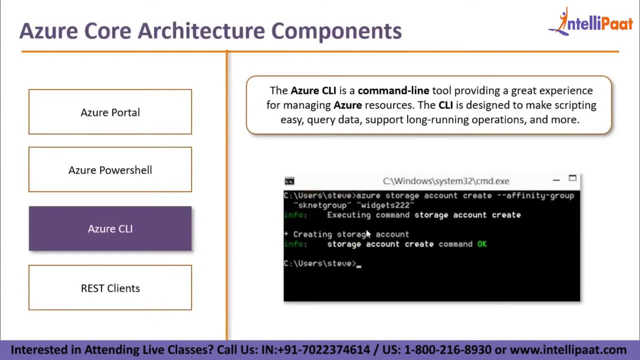 actually use it in the dos environment, right in this case? also, if you want to manage your azure resources like you were managing it through powershell, through command line statements, you can do a similar kind of way in azure cli as well, but the commands that you'd be entering over here 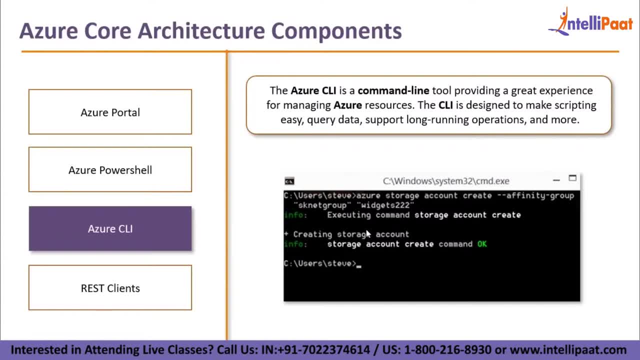 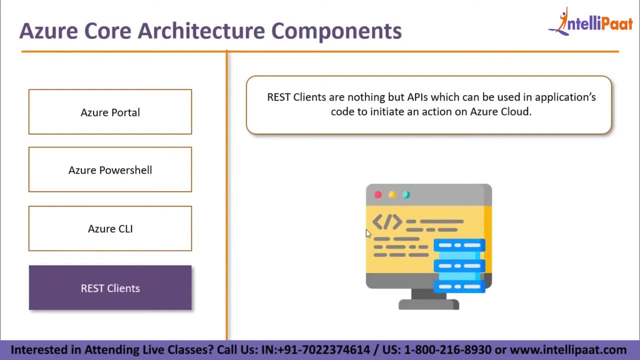 would be more in line with dos commands. on the other hand, when we talk about powershell, we would be using powershell commands to control azure in that case. okay, so this was azure cli guys. in the next and the last topic is rest clients. so rest clients, as i already told, these are nothing but. 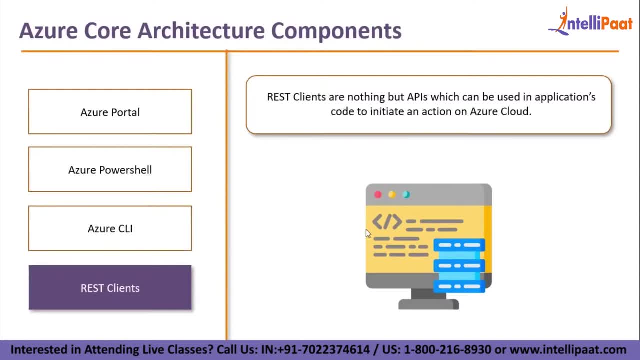 apis that you use on your website, so you'll have to authenticate them using the metadata credentials, and these credentials would be available for all the accounts that are created under a root microsoft azure account, so each credential would be different from each other based on if there are more users. for example, in our case, we created a user for our it manager. 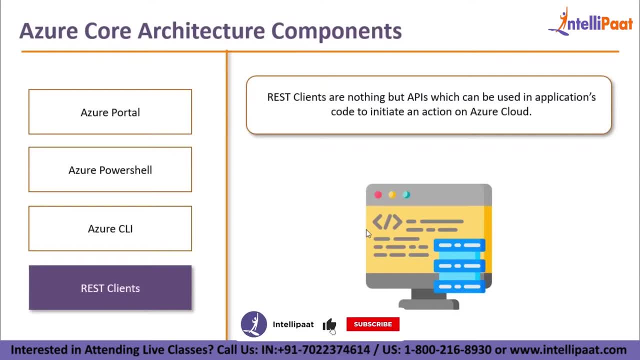 and then we created a user for a software developer. for our software developer, we just gave him the storage access for our it manager. we basically gave him the administrator access. so when they put their credentials down, the code of their web application, they try to connect to azure. based on the permissions that they have, they would be able to access the. 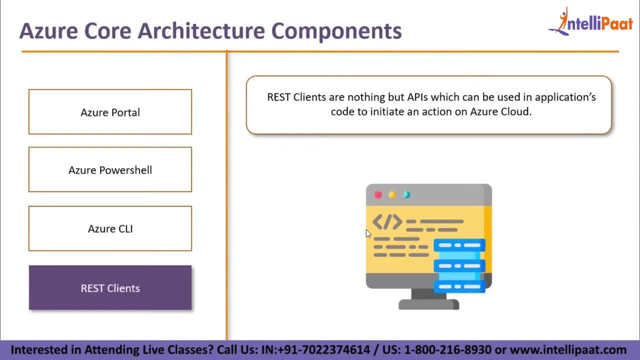 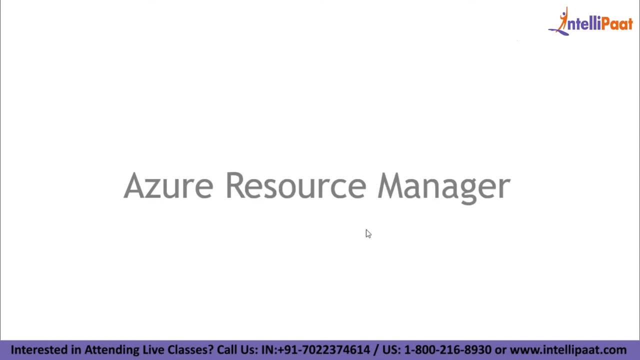 resources in case they do not have the permission, you will get a corresponding error to that that this particular user does not have the necessary permissions to access that particular resource. all right, guys. so these were the front-end components of the azure core architecture. now let's talk about the middleware, uh, the component which basically acts as a mediator between your 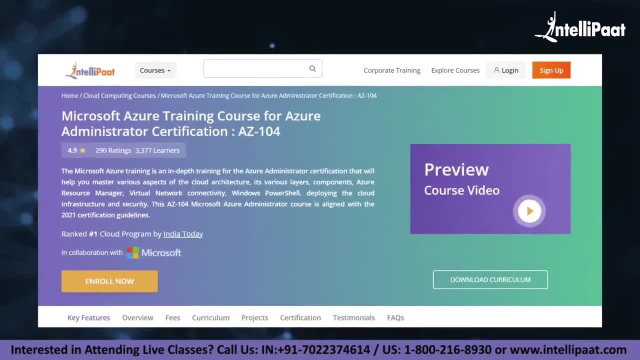 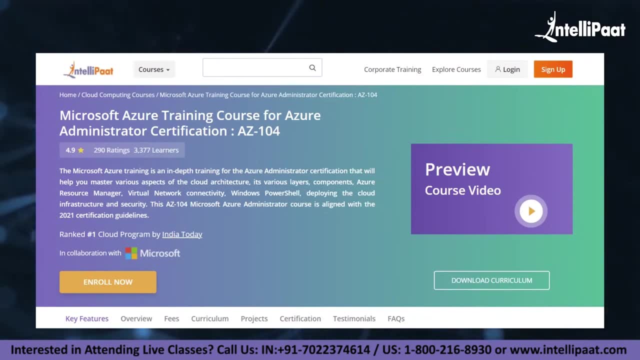 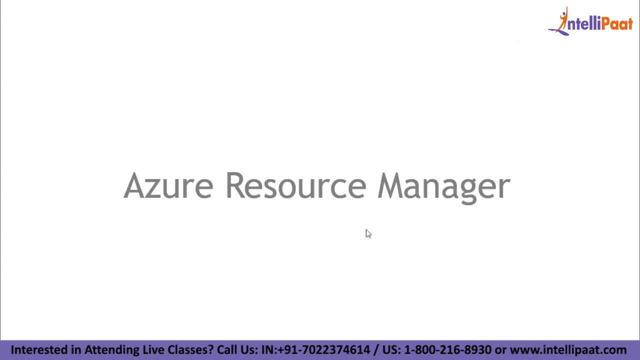 resources and the azure resource manager. just a quick info, guys. intellipaat provides microsoft azure certification training in partnership with microsoft, mentored by industry experts, the course link of which is given in the description below. now let's continue with the session touch points, that is, your front-end components and the core components, which is 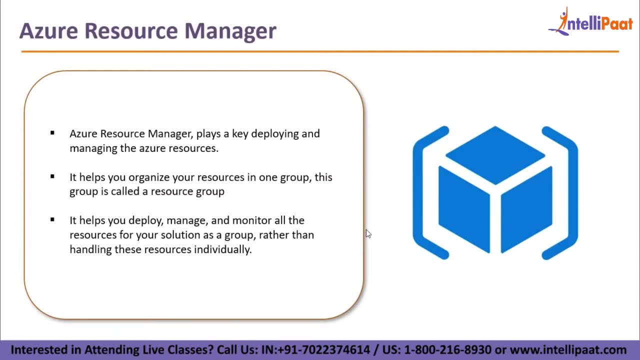 the azure resources, so it acts as a mediator. the azure resource manager, so azure resource manager it and manage the Azure resources right. it also helps you to organize resources in Azure. for example, it will help you in grouping resources together. let's say I'm launching a web application- okay- and I'm also, at the same time, launching some. 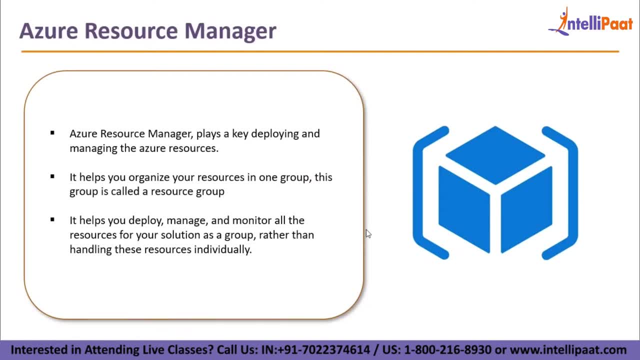 other application. let's say, I'm also launching my Android app back-end service. so what I can do is, let's say, if I'm launching a web application, I would need certain components. I would need, let's say, I need a separate storage for my web application, right, so I can create a storage account. I would create a web. 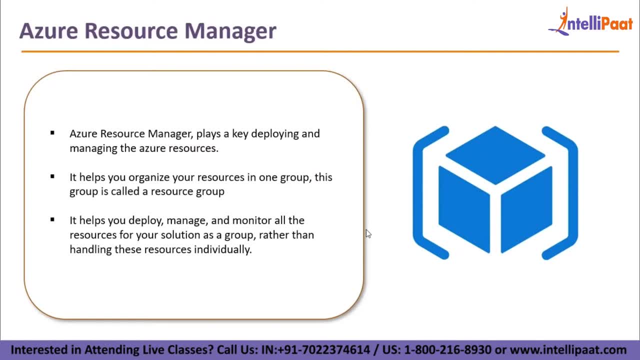 app and then I would create a database server. now, if I create it just like that in Azure and you try to see all the resources, you would not be able to make out as to which resources are there for my Android application and which resources are there for my web application. what you can do is probably: 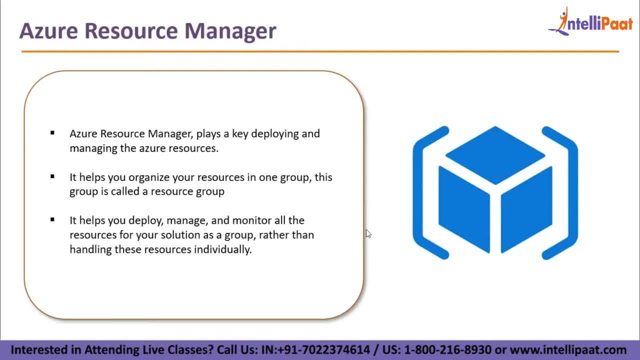 you can define a nomenclature and then you can create a web application and then you can say: probably you can name your instances like, let's say, for Android database you can say Android underscore database. for your web application you can say web app underscore database. so that's one way of 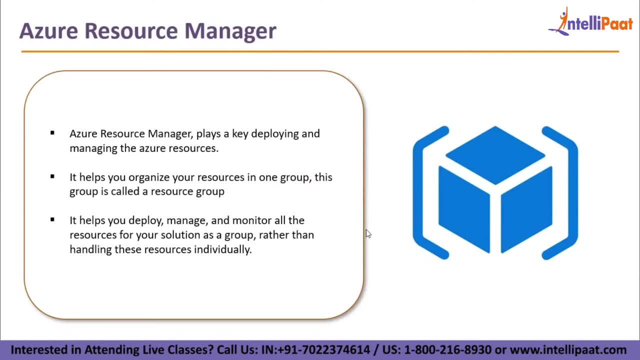 sorting it out, but as your resource manager makes it easy for you. how does it make it easy? it basically gives you the ability to create groups, right? so if you're creating one kind of an application, what you can do is you can create a group and inside that group you can basically just map the resources, or 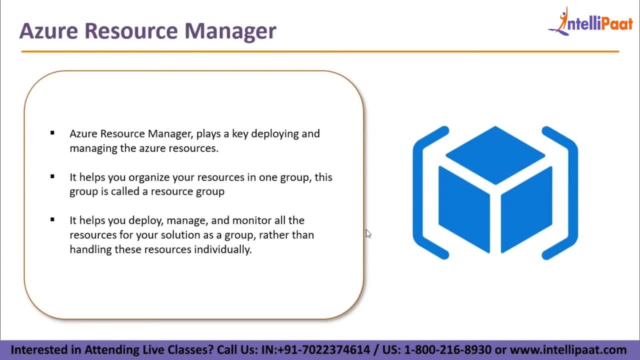 launch the resources that are specifically there for that particular application. for example, for a web application. I can launch all the resources that I want and I can group them together in the web application group. right, I can name the group anything. it's just like a folder, guys, if you were to understand it more, simply understand, it's just for sorting. 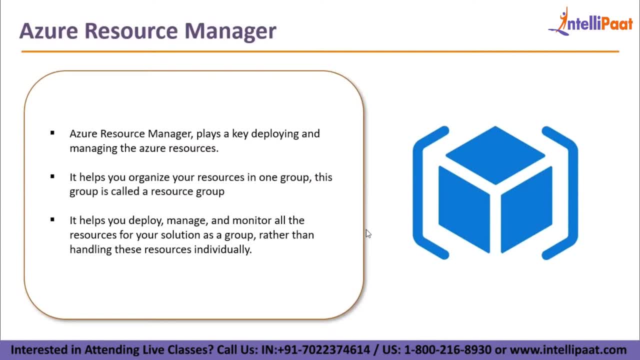 out resources. let's say you have a desktop full of files and those files are PDFs, TXTs and doc documents. so what you can do is you can just create three folders and inside those three folders you can put your doc folders and your files in the inside the PDF folder, you can put PDF files inside the text files. 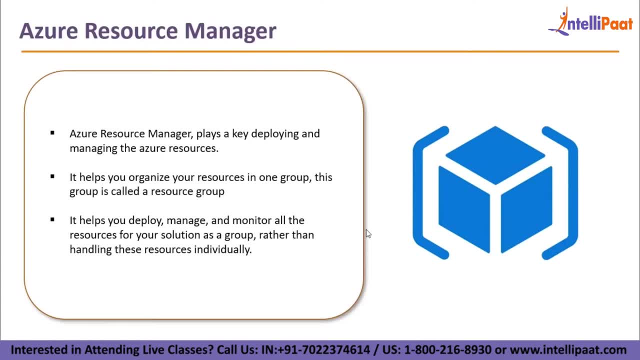 you can put the text files right. so this is the way of sorting on your desktop. similarly, if you want to sort your resources in Azure, you can use the ability of creating resource groups using the Azure resource manager right and, at the same time, the third point or the third feature of Azure resource. 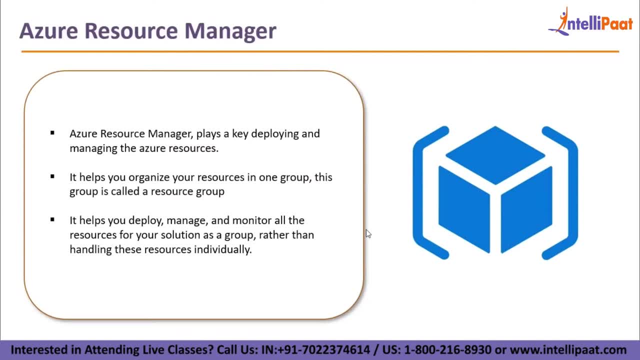 manager is. it authenticates, it checks what all permissions you have and, based on that, it gives you the ability to create a group. based on that, it gives you the ability to control your Azure resources. right. so it also authenticates your calls to the Azure resources, and only through the Azure resource manager would. 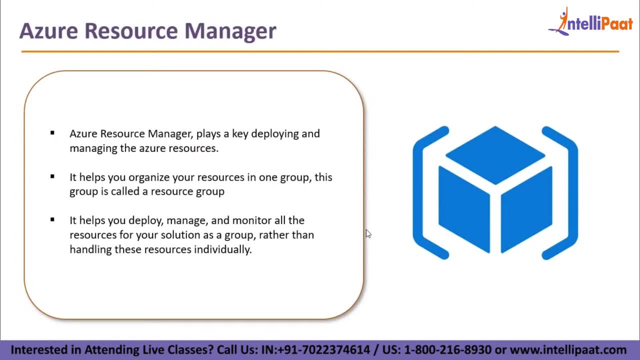 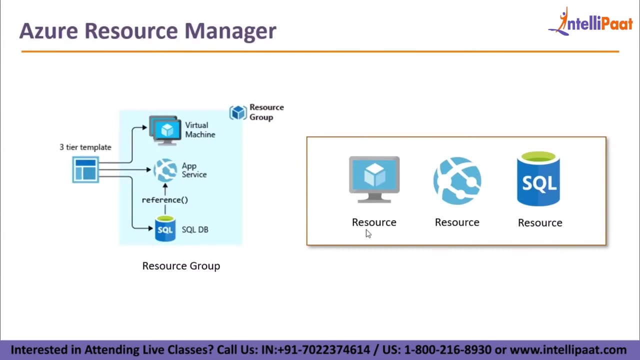 your calls go and if they are accepted by the Azure resource manager, only then they will be forwarded. otherwise, they would be rejected and you would get an appropriate message for that. all right. so, guys, this was all about the Azure resource manager. so I was talking to you about what a resource group is, and 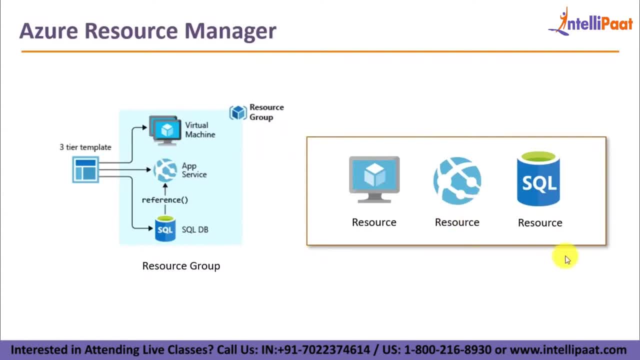 what I mean by that is I want to do, is I want to group all these three resources. so, as you can see, let's say this is a resource group of mine and what I want to do is I want to group all these three resources. so my VM instance, that I 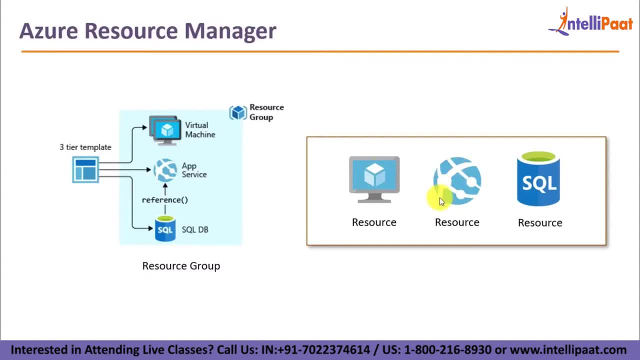 launched, that is termed as a resource. if I launch a web app, that is also termed as a resource. don't worry if you don't understand what is a virtual machine, what is a web app? I will talk more about this as we move along in this session. 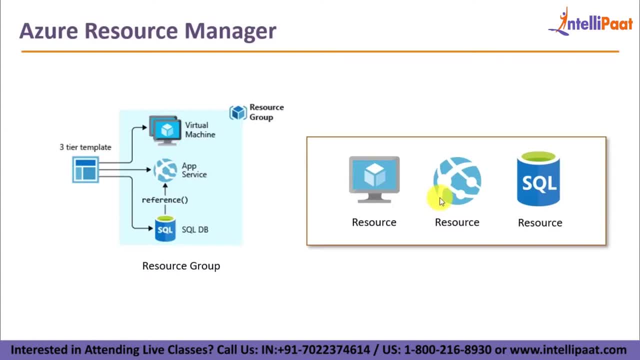 but for now, understand that any service in Azure, any instance that you launch in Azure, is basically a resource right. and when you group one or more resources together, or I should say two or more resources together for a particular thing- which so I gave you the analogy of folders- if you group them together and 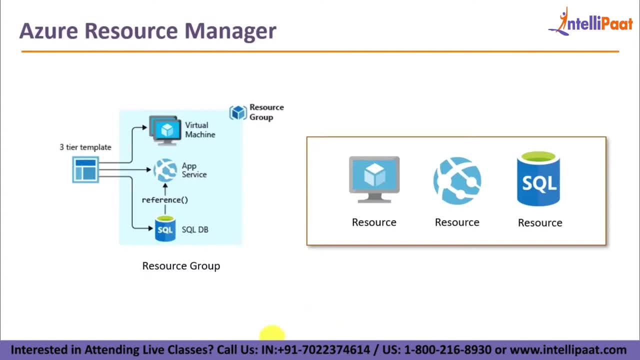 that symbolizes something that basically can be done using resource groups, and that is exactly what is specified in the figure as well. right? so you have some virtual machines, you have app servers and you have a SQL database and you have all grouped them together in a resource group and probably you have a. 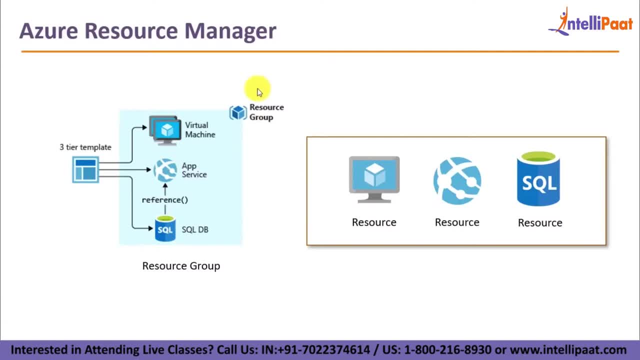 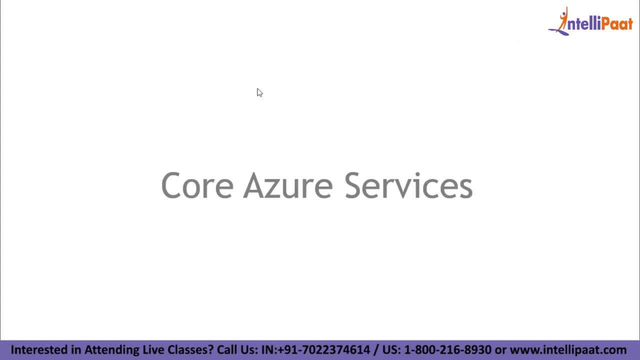 resource group and you have a database and you have a resource group and probably you can call it, let's say, the production environment. you can create a test environment, call the resource group a test environment and deploy the necessary resources inside that as well. so, guys, with this we come to an end of 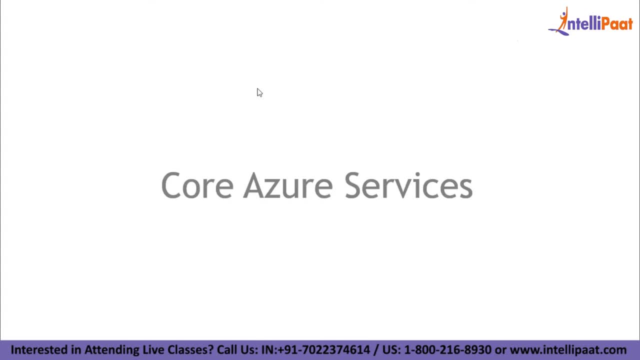 the Azure core architecture. so by now you understand the nitty-gritties of how, as your works in the backend, right, how things are structured inside Azure. moving forward, guys. now we will be talking about the Azure services, right? so we'll be talking about the resources that we just saw. 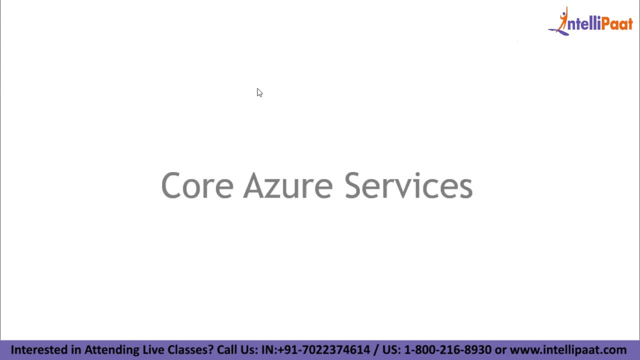 the resources that we were grouping inside the resource group, or the resources which, basically, the Azure resource manager was managing. we're going to talk about those, and those are nothing but services in Azure, right? so it'll become more clear as we move along. so let's start off now with core Azure. 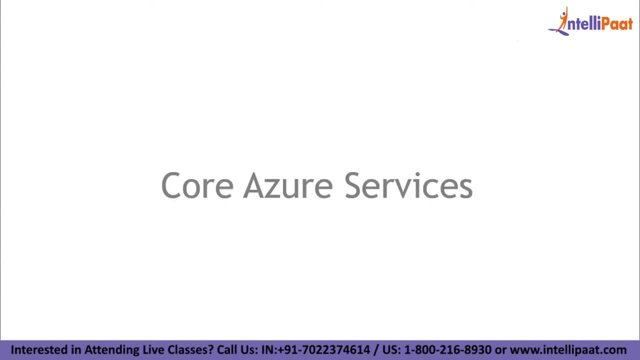 services. all right, guys. so before starting off with the services, guys, there's again a simpler way to understand all the services in this. your, what is your has done is, let's say, there are around 300 plus services in a right now. it is difficult to actually remember all those services or to 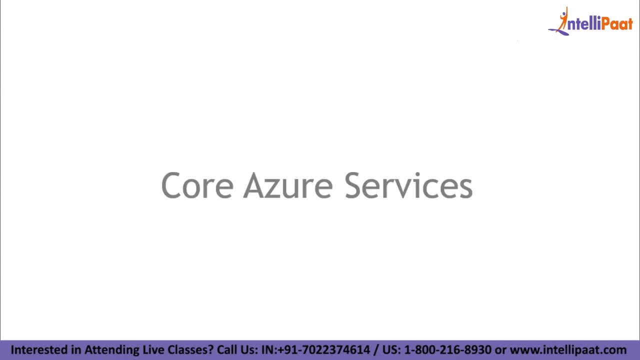 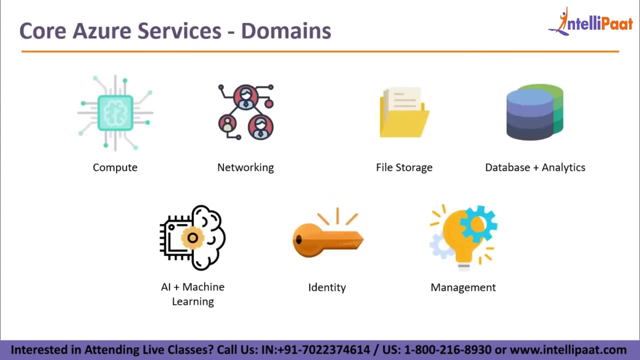 basically know how one service is different from the other. so what, as your has done, is it has actually divided its services based on what the services does, or what the services do, right? so the major sections that it has divided its services in are these right? so these are not all the sections that, as your gives. 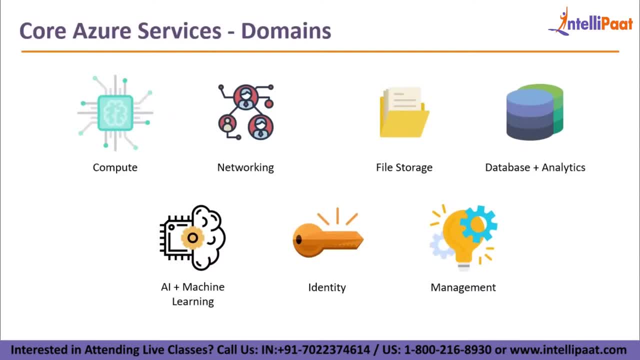 us the services in. but these are all the important sections or the important domains in which, as your provides you services, and as a cloud engineer or as a azure engineer, when you'll be working in companies, mostly you would be working on services which are included in these domains, right? so we'd be covering these. 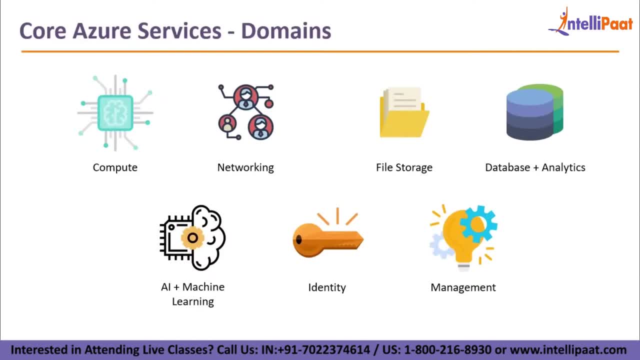 guys, there is no as your engineer out there who would be knowing each and every service in a jar right, but what we as learners can do is we can learn all the important services which are basically used in your everyday life when you become a cloud engineer, right and as and when you apply. 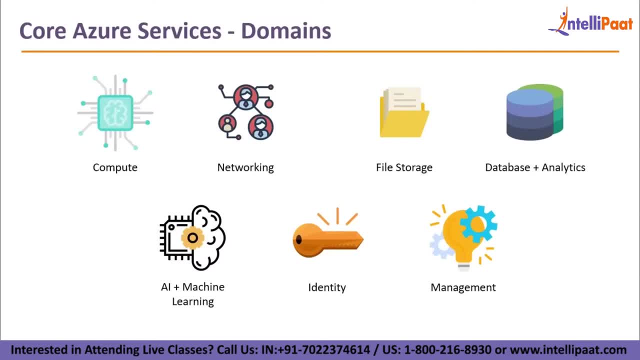 to companies. probably you can tell them you know all the basic services, all the important services in Azure and if there is any special requirement for a particular service that they use, it is obviously going to be an easier task for you, since you understand how is your works. so understanding, one more service. 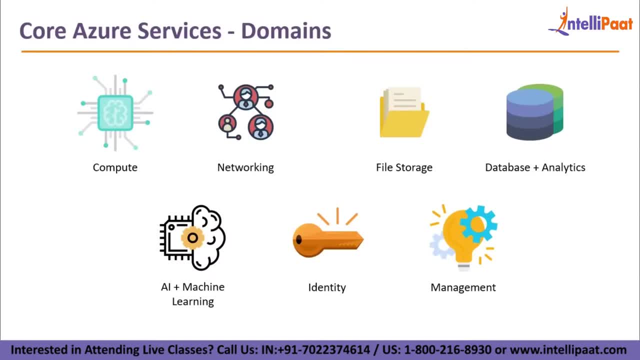 in Azure would not be a great deal, but most of the times, I would say nine percent of the things that you will be doing as a cloud engineer, or ninety percent of the services that you will be using or working on as a cloud engineer would be covered under these two. so now let's go ahead and start off with the. 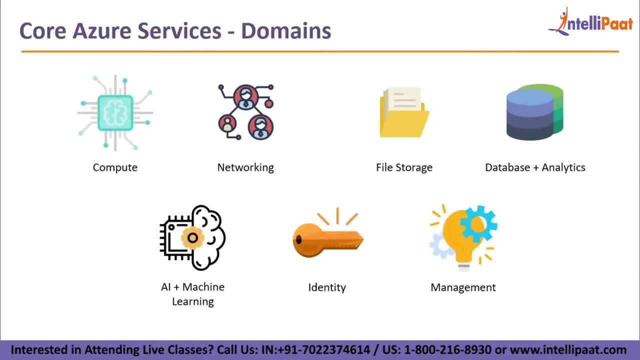 first domain, which is compute. but before that let me give you a brief about all of these domains. right, so the first domain is compute. so in compute you have compute intensive resources wherein you get the raw processing part. more on this we will talk about as we move along. then the second kind of 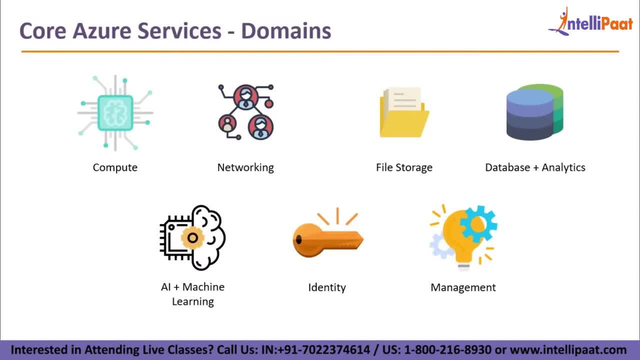 domain is networking, so this particular domain would include all the services which provide you with networking capabilities. right, then we have the storage domain, which basically gives you all the services in Azure which can basically give you the capability of storing some files. right, and obviously there are a lot of services in storage and each service is targeted at a 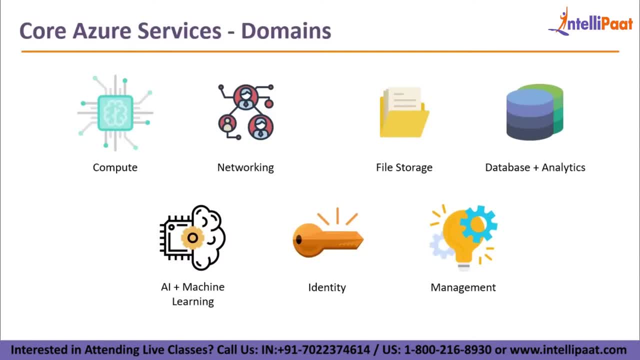 different kind of use case. so we're going to discuss some of the storage services in Azure which are very prominent. then you have services related to database and analytics, right? so if you want to store textual data, which also you want to analyze using graphs or using flowcharts, right, you can do that in. 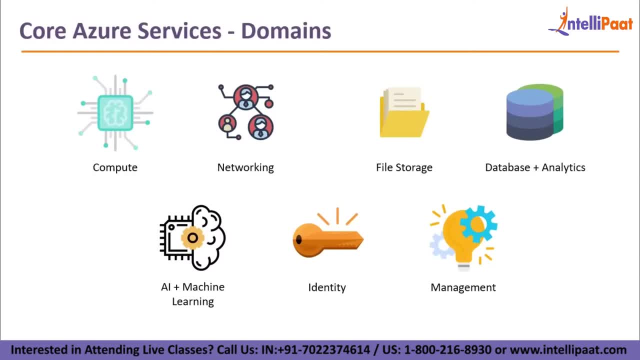 Azure in the domain database, plus analytics, then our next domain comes out to be AI and machine learning. now, this is a very important domain, guys, and I've seen actually people who are data scientists, people who are researching on data science. so, basically, when you're working on data science or when you're 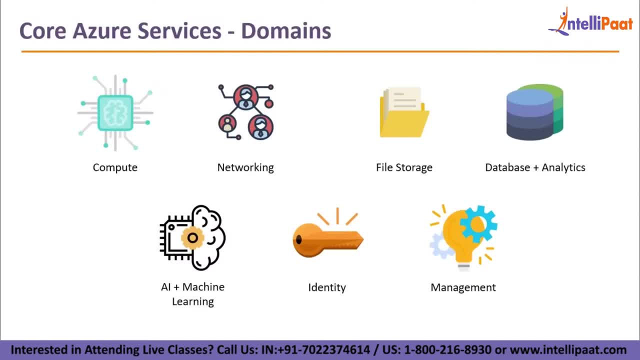 working with AI, you need a lot of computing power right now. the good thing about cloud is that it offers you a pay-as-you-go model, which basically means you only pay for the time you use the resources for right, and nobody can afford, you know, a high spec machine. if you need an i7, an octa-core processor. 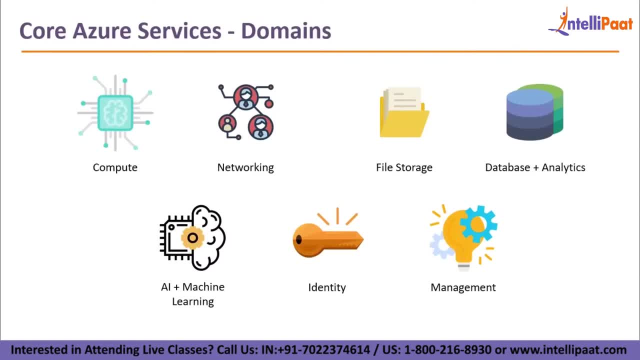 and a 32 GB RAM. it's very difficult for a layman to get hold of such kind of a machine. so what researchers and what data scientists can do is they can actually launch a machine on Azure with a similar spec that they want for their use case, use it for the time they want and shut it off. 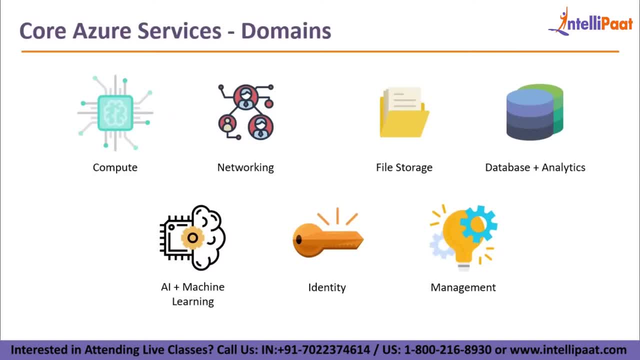 and you'll be charged as low as around 0.05 or 0.06 dollars, I guess, for if you use it for around half an hour or so, right? so I guess half an hour or 45 minutes should be enough if you want to do a POC or if you even into researching. 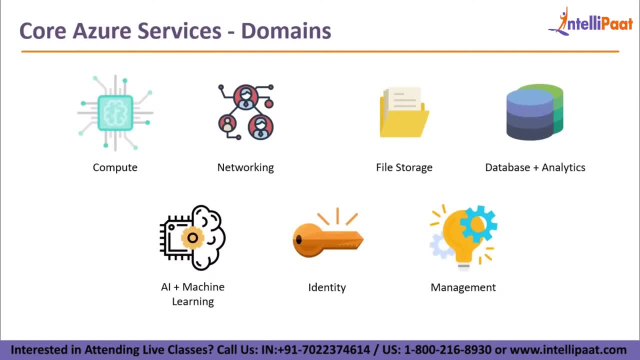 or if you're into testing. I guess this would be the cheapest option for you, rather than a pay-as-you-go model. So you can get a full-blown server or a full-blown laptop with high specs, and all that will be more expensive for you. so it's better if you use services from cloud for your compute. 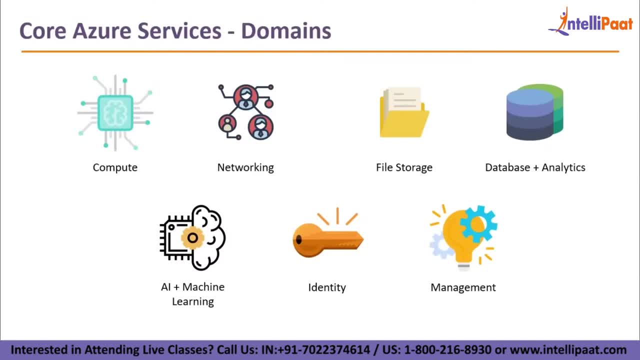 intensive needs. but that is not it. what you get in AI and machine learning domain is you get, you know, you get a pre-built dashboard kind of a thing, so you don't have to feed in algorithms. everything is pre-built in Azure. you basically get a drag-and-drop kind of thing. 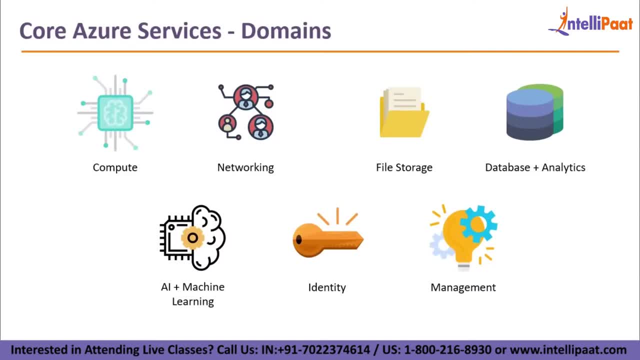 So if you're looking for the best for post functionality, when you're particularly using Azure ML- because I've used that- I'm telling you it's pretty drag-and-drop if you compare it with its counterpart. let's say, if you want to do a regression test in our, you would actually have to write a long. 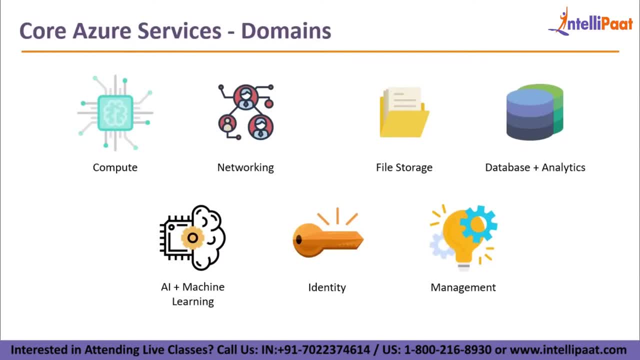 script to do a particular thing, but the the kind of services that, as your has launched, for example, like I mentioned as your ML, all you have to do is drag and drop and you can get your results right. so that's how convenient it is and that's why people are more and more to save their time, to save on their time. 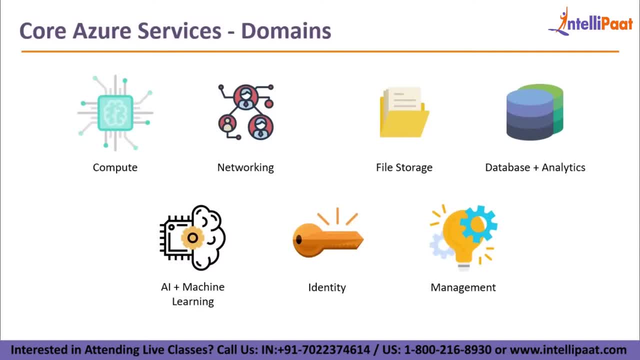 So that's how convenient it is and that's why people are more and more to save their time, to save on their time, their costs. they're actually using the ai and machine learning capabilities of the cloud and, in particular, we are talking about azure, so azure also has ai and machine learning services. 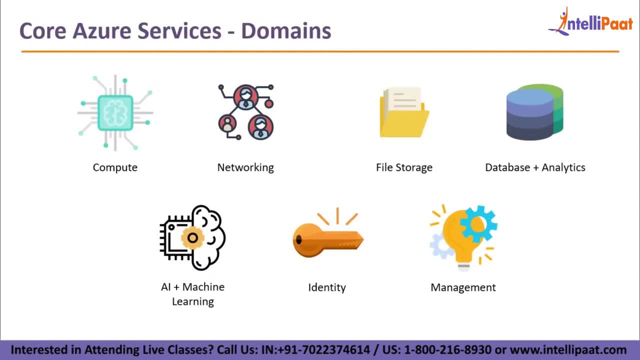 which also we will be discussing as we move along in the session. right then, the next domain is identity. so identity domain domain would basically include services which will help you in authenticating users. it will help you to basically get the metadata credentials that we discussed earlier for your website. so all the authentication part, the authorization part, uh, whenever you want. 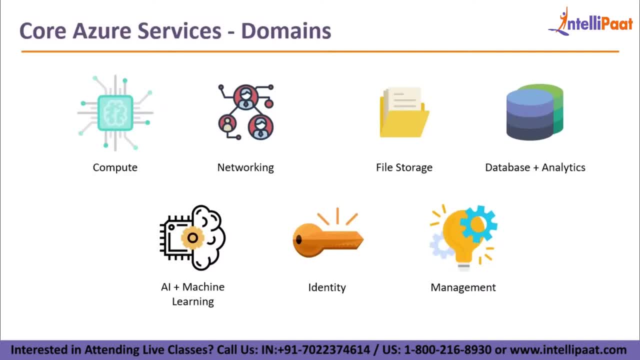 to give specific permissions to particular users. all of that can be managed with the identity services. and, lastly, we would be discussing the domain which is management, which would basically include services such as monitoring. it would include services, uh, such as infrastructure, as code, right? uh, don't worry about these big words, guys. as we move along, everything will 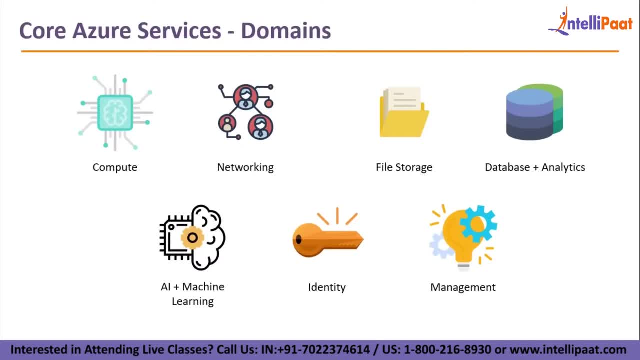 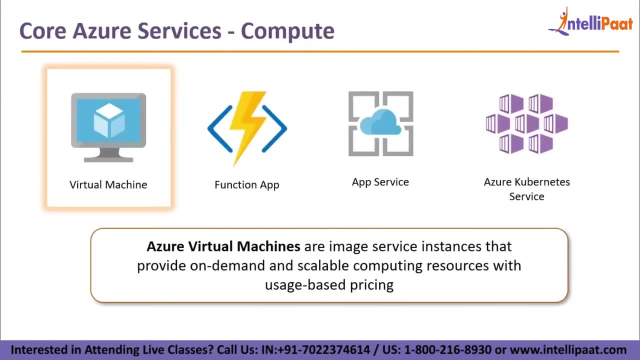 be clear, but without wasting time, let's jump on to our first domain, which is compute, and let's understand what are the different services that we're going to understand in that right. so in compute guys, you basically have four prominent services. you have virtual machines, you have 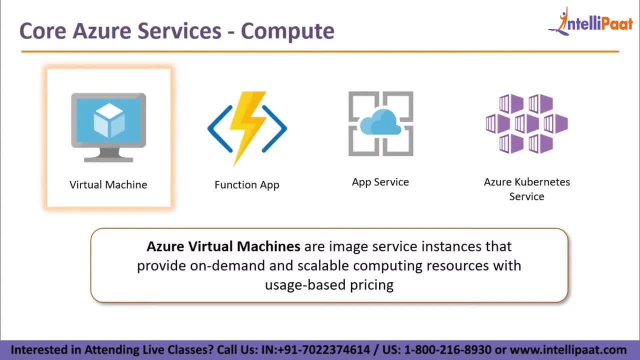 function apps. you have app service, and then you have the azure kubernetes service. so the first service that we're going to discuss about is the azure virtual machine service. now, what is that now, guys? azure virtual machines are nothing, but it's- it's basically a server. 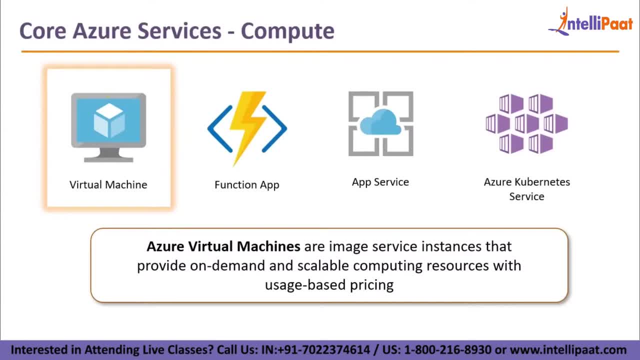 or i can say, uh, the most layman terms possible. let's just say it's a computer, uh, just like a laptop, which has just installed windows on it and nothing else is there, right? for example, let's say you buy a laptop, what are the first thing that you see? you see, uh, your windows there. or you see: 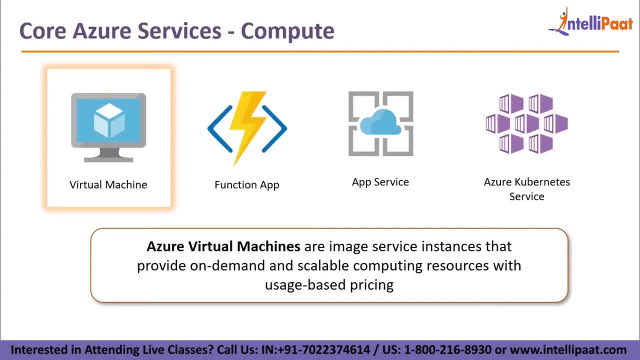 your mac os there or you see your linux operating system there and basically no, no, no software is installed. it's just a bare minimum operating system which is given to you and whatever you want to do on your laptop, you install it. it's a very, very basic step, so you have to becomes a full App: 800 for an app, or. 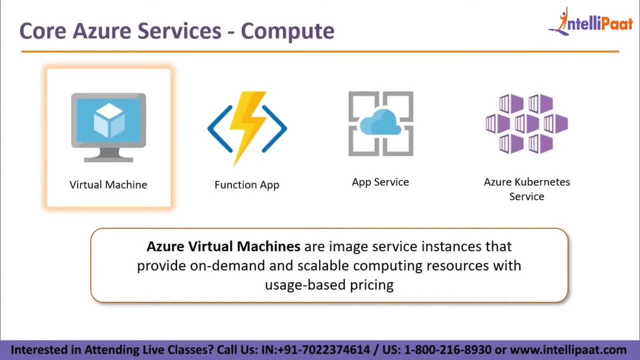 you install a zip file and it's important to have that system, so then, basically, you can deal with the sort of anything that's install it and then you work on right. so, similarly, virtual machines are there. virtual machines are nothing, but they are machines that are launched by your cloud provider, which in our case is azure. 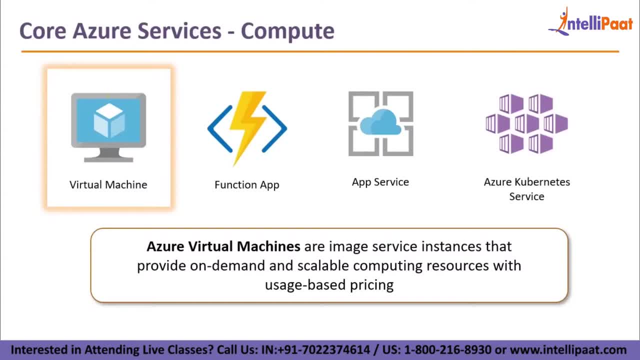 and they launch it for you, so you don't have to worry about where are they getting it from. they launch it for you and what they do is they give you the remote access to it, right. so it's basically like working on your own laptop, but working on it from a remote location. so, similarly, 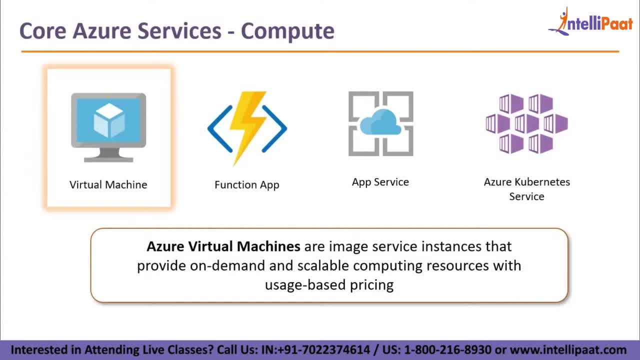 you get your own machine on azure which is freshly made right. you have a fresh operating system on it, there are no softwares installed and whatever you want you can install on this particular server. so we call it server because basically you would be using it for deploying applications which would 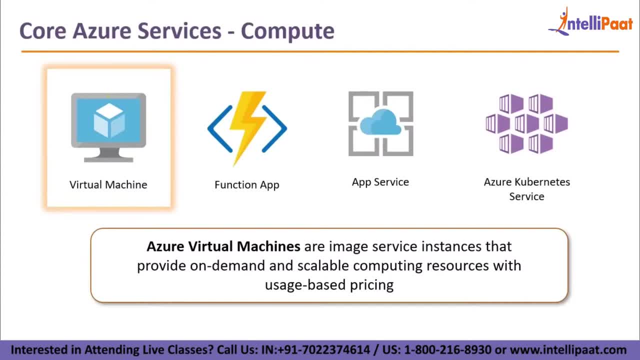 be basically be available to the user. so that's why we call it a server right. so basically, these are server or computers that are launched by azure for your own personal use, but you would be accessing it remotely if it's a Windows machine. in a GUI case you can. 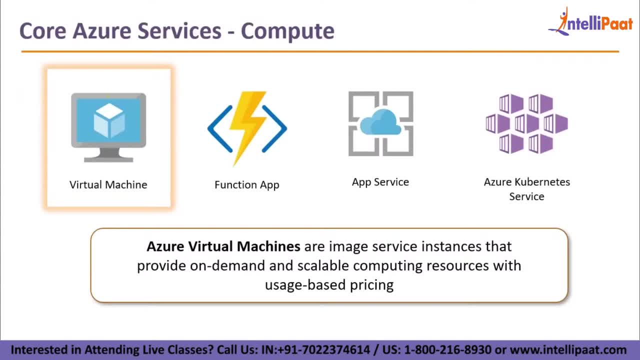 basically do an RDP and use it. if it's a Linux machine, you can do. basically do an SSH and you can work on the command line for it. but remember, guys, there are no softwares installed on it. there are no extra softwares installed on it. so anything that you want the server to do, for example, let's: 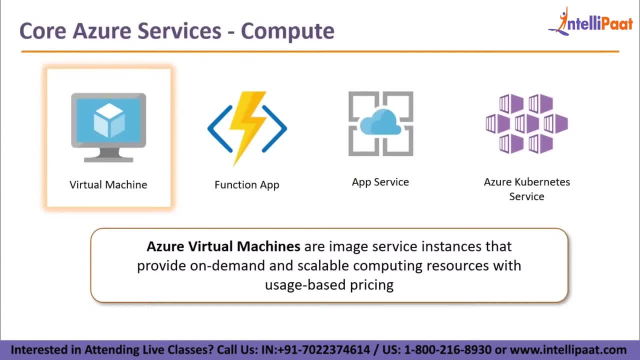 say, you want to create a database server, you can just install database on it and it'll be ready, right, and it will be ready for accepting requests for the database service, if you want to. if you want it to be a web server, you can basically install Apache, PHP etc. and then you can put your. 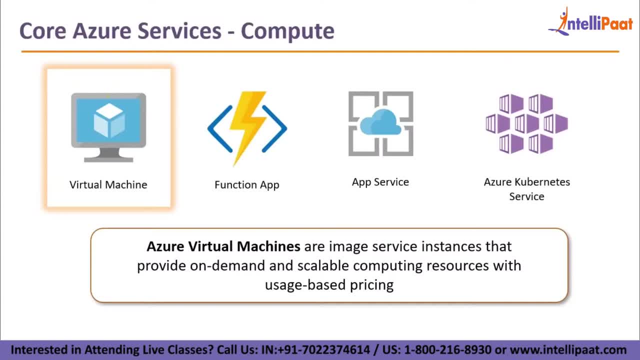 website on it. it'll become a web server. anything and everything that you want or that you can do on your laptop, you can do on virtual machines. so this is what Azure virtual machines is, guys. now the next kind of service is similar to virtual machines, but it's actually an advanced version of virtual. 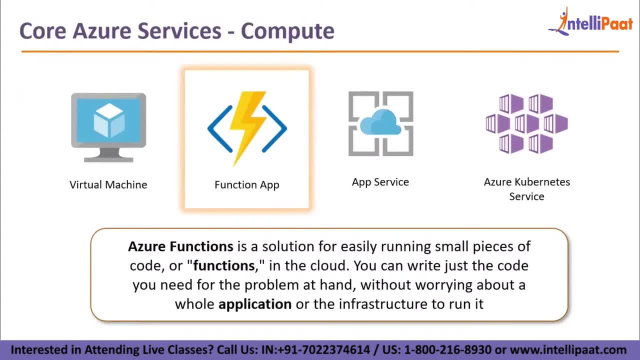 machines. so what are function apps? so, guys, function apps is, uh, like I said, it's an advanced version of the virtual machine in which you do not get the access of the operating system. okay, so let me give you an example. for example, let's say you are, let's say, doing some work on a website and that website. 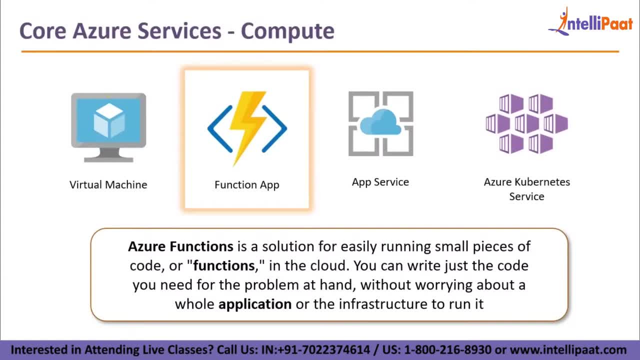 basically, let's say, does processing for you? for example, let's say you are on Facebook and what you do is you upload a profile picture. and once you upload a profile picture, let's say you want to crop that profile picture to a particular size, and then you can use it for fucking video editing. you can definitely do it, and you can just go to your website any time of the year to actually update your profile picture, and then you can do all the the other stuff that's happening in the middle of the year. or you can just like you can, you can apply it, and then you can do everything, have all the different things that you need to do, and then you can just like. 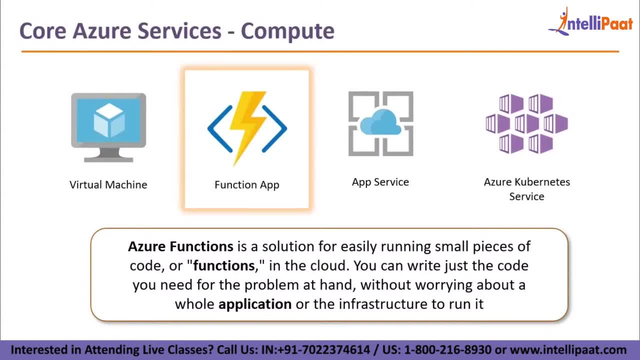 want to upload it as a image on your facebook. so what will happen? so you will upload your image on the facebook app. you will do the cropping part. let's say you want to add a filter as well. you add that filter and then you click on save and then you want it to be uploaded as a profile picture. 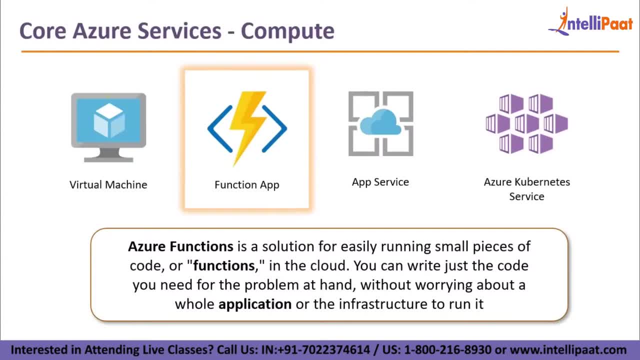 on your facebook, right? so there is a minimum amount of processing that would have to be done on your image. some processing has to be done on your image, right? and basically how that works, is that processing is actually not done on your phone or on your computer on which you are accessing? 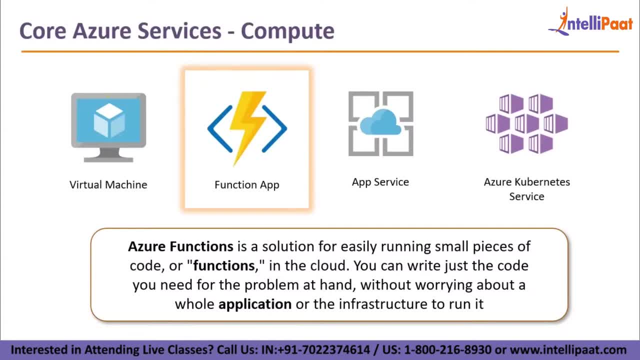 facebook. that is actually done on the facebook servers, but the way they handle it is, they basically would have a web server in place. they would separately have a database server in place which would be interacting with your web server, and for the processing they have a separate server. 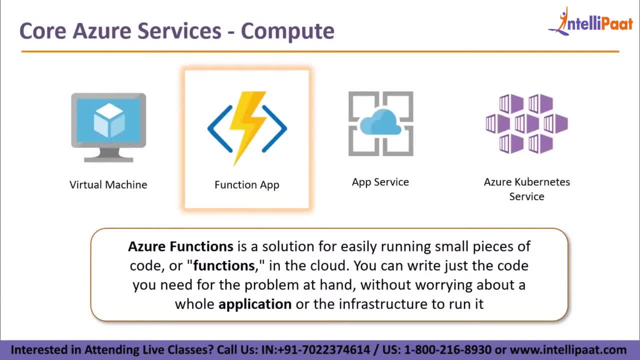 okay, and that separate server is basically called a back-end server. and what does that back-end server do? all the requests which comes in, it basically processes it and gives out the result. that's the sole job of a back-end server. and why is it separate? why is it not integrated with the web server? the simple reason for that is, let's say, 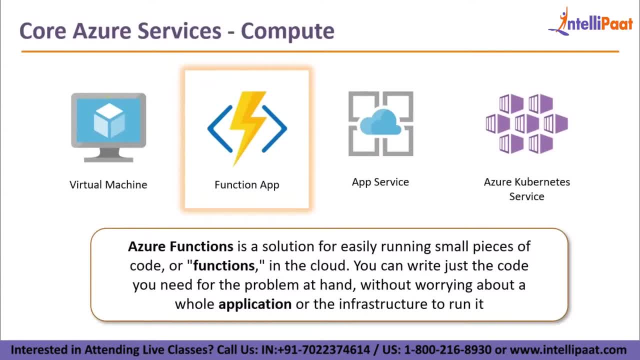 there are 100 users who are using your website, right, and they're constantly exploring your website, going through the ui, doing uploading images, doing processing and everything. now your back-end component is doing the image processing and the front-end component of yours, which is the website component of yours, is basically serving the website to the users. 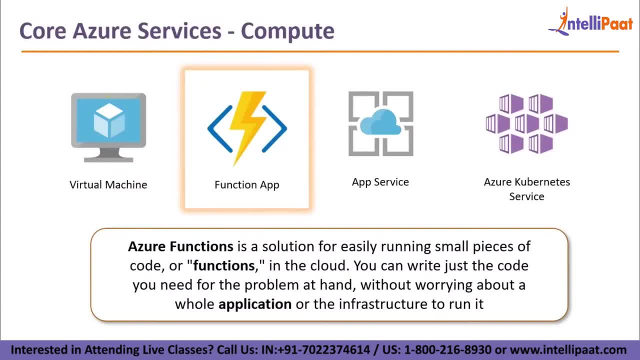 right. so there are two tasks happening over there and, let's say any one of them, they get overloaded with some work, right? that would hamper the performance of the second component. let's say there are more users on the website, right? so obviously your web component, or the website, 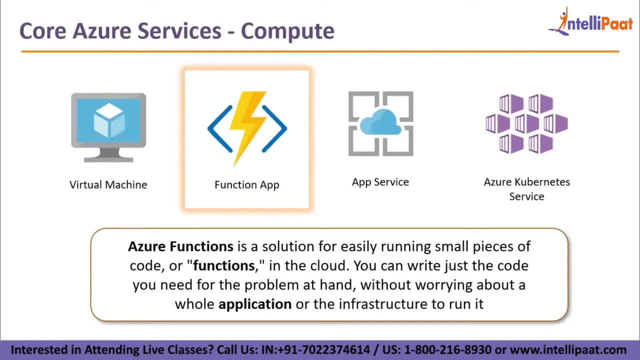 component of your server would require more processing power. so let's say it takes up 60% of the processing and let's say what happens is all these people who came in, they upload their profile pictures and they put some filter on and they now want to. 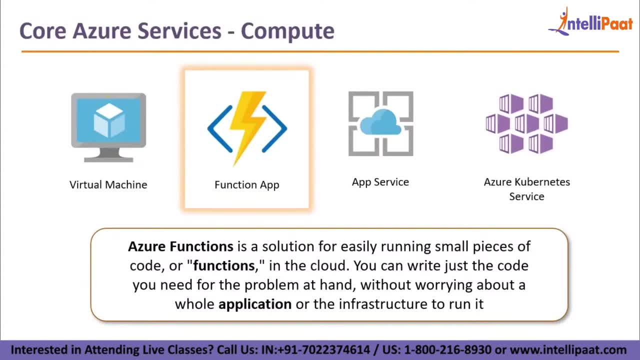 process it. so one thing is your server is already busy serving these hundred people. your website and the cpu mark is at 60% now because of the processing load which is coming onto your back-end component. that also requires around 80% cpu to work efficiently, but now because 60%. 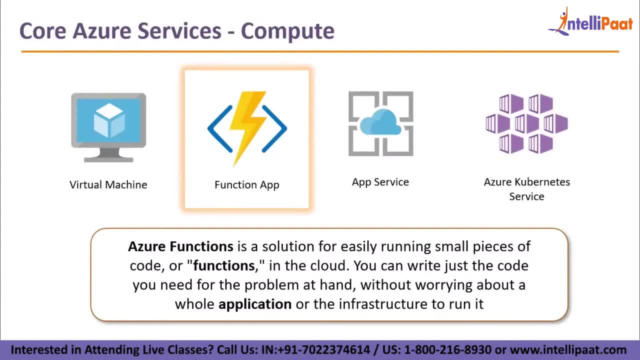 has already been taken by your website server. there's only 40% left. so what will happen in this? your server will inadvertently become slow. right, it'll become slow and it might even crash in case a deadlock situation happens. right, and this was usually the case when we were not aware of distributed computing. but nowadays what happens is we are. 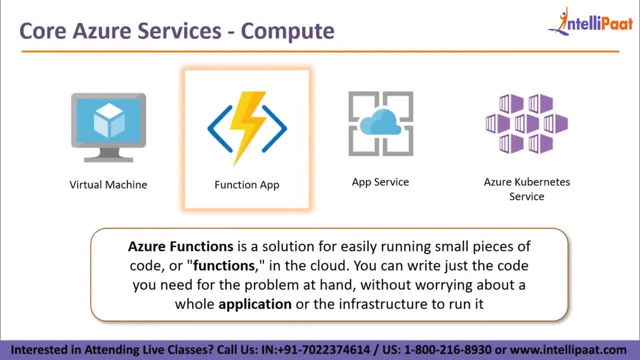 dealing in a world where we cannot afford downtime, and that is the reason everything has been distributed right. so if there is more load on my back-end server, my back-end server is going to handle it. it will not hamper the performance of my website server or my database server. so 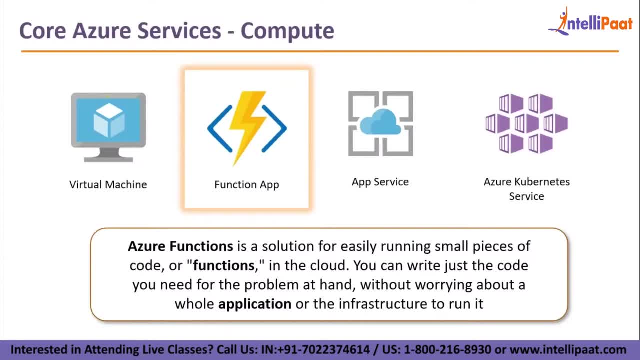 every software component is now distributed. and why are we discussing this? we are discussing this because we are talking about function app. now, what is a function app? function app is nothing but a back-end service on which you do not have to deal with the operating system like you do in virtual machines. you do not get an access to the operating system. 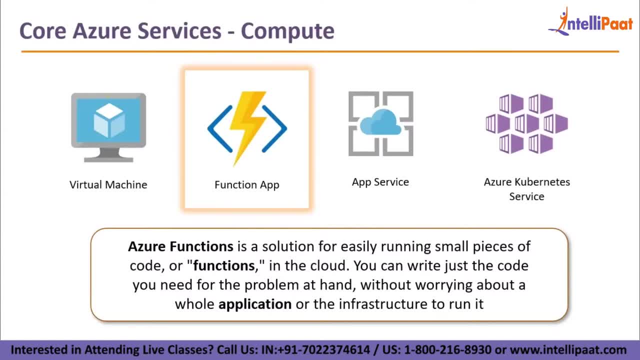 you cannot install any kind of software on it, whatever you choose. let's say you have an option of choosing what kind of back-end code you want to run on the function app, let's say your image processing, whatever code you have written for the image processing app. let's say: 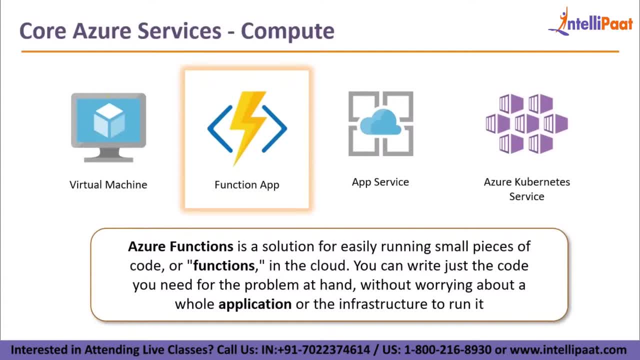 you have written it in python. so when you will be deploying a function app, what you'll be choosing is: what kind of code would i be uploading on the function app? let's say you choose python, the next thing that you would be doing is you'll be clicking on next and then it will make your function app. 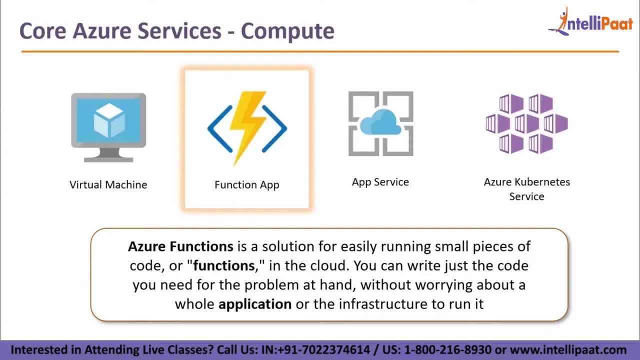 ready and then it'll ask you for the code for the image processing. you're given the code, you click on save and now your back-end server is ready to accept requests. that's it. so now all your functions ping the back-end server with the required information, with the image, it will. 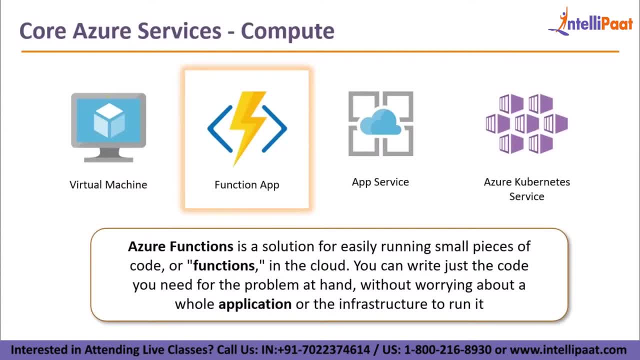 basically take the image. it will run through the code. see what it has to be done, do the processing on the image and give the image back to the website server or to the facebook servers, which will basically upload the profile picture right. so in a just what is function. 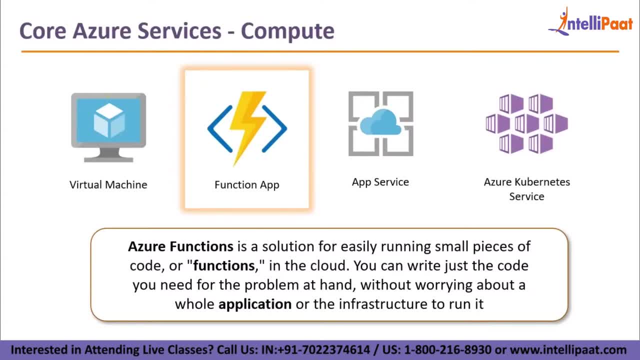 app, a function app is basically a service which will not give you access to the operating system. it will basically give you one dashboard on which you can upload code, and it can do any task for you. all you have to do is give it work. it will do for you and that's about it. you. 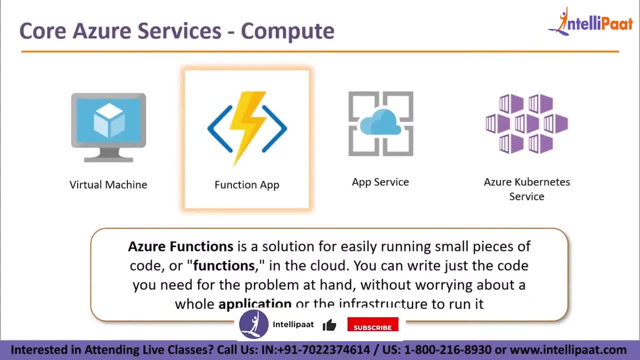 don't have to mess around with anything else. you don't have to worry about what machine size i should give to my function app. you don't have to worry about how many machines should i run so that my function app never gets overloaded. everything is managed by azure. all you have to do is given 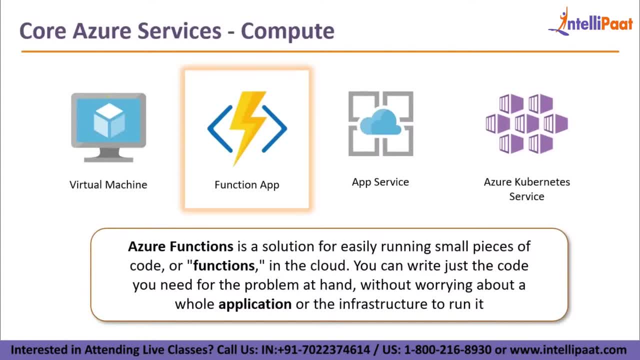 the code and see your application working. so these kind of applications are basically called platform as a service, and the earlier service that we discussed was virtual machine- is basically called infrastructure as a service. why infrastructure as a service? because in that case you got access to the operating system right. you can do anything on that server. you can install anything you can. 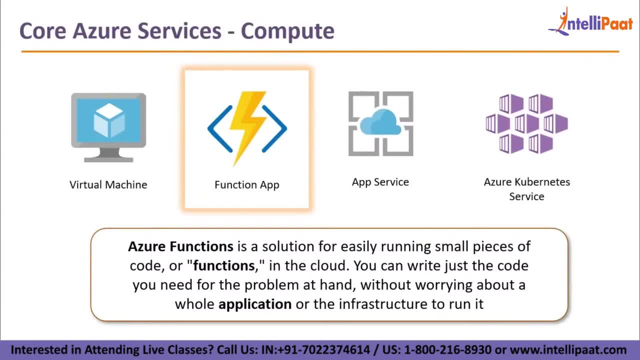 actually delete everything also, and you can make that server hang, or you can make that server not working. you can actually uninstall the installation files of the operating system as well. that is something that you can do with your server, but what will happen is it will not cause any harm. 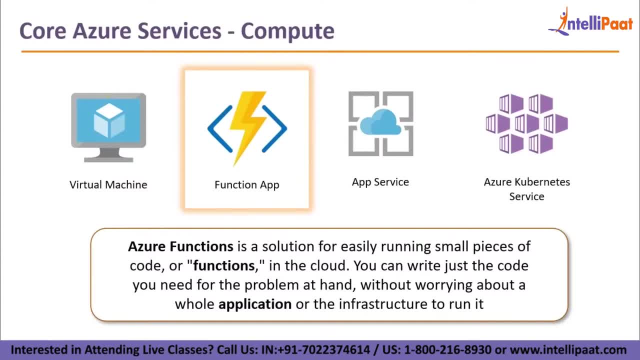 to azure. basically, you would not be able to use the server and in the far end time you will basically have to delete it because it's going to be usable. that's the most extreme thing which could happen. but the case with function app is because it's a platform as a service. it's giving you a dashboard on which you can upload. 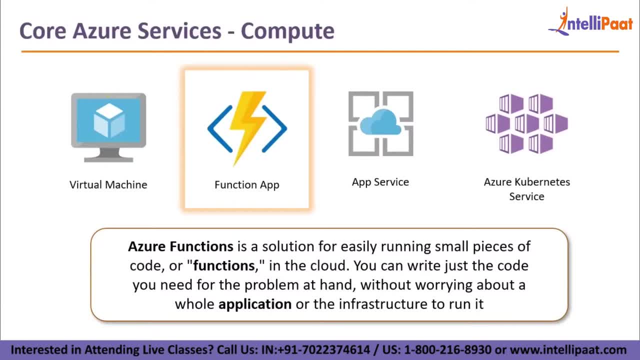 code and hence it's a platform right. it is not giving you access to the operating system. it is not giving you access to what softwares you can install. you just choose the environment in which your code can run and that's it. that's what a function app is all about. it's a back-end server. 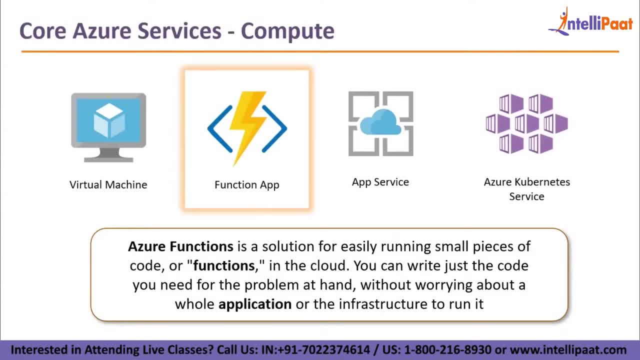 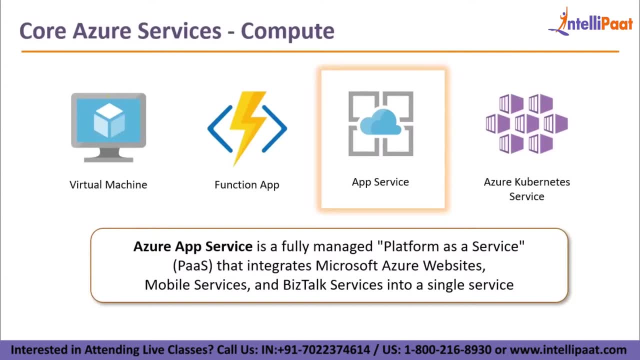 without choosing or worrying about the underlying infrastructure. moving forward, the next server is that we have is app service. app service is yet another uh platform as a service kind of resource that we have in azure. and what you can do with app services you can basically launch or deploy. 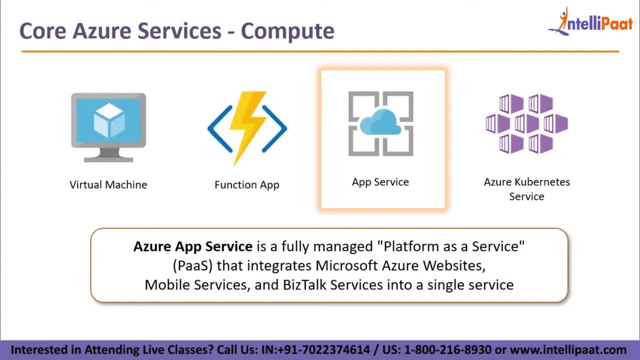 websites. now you would be wondering that in function app also i can just give my code and probably i can give my website code and it will deploy the website for me. no, your function app can only give outputs based on the inputs, it cannot deploy a web application for you. if you want to deploy a web application, you would have to use. 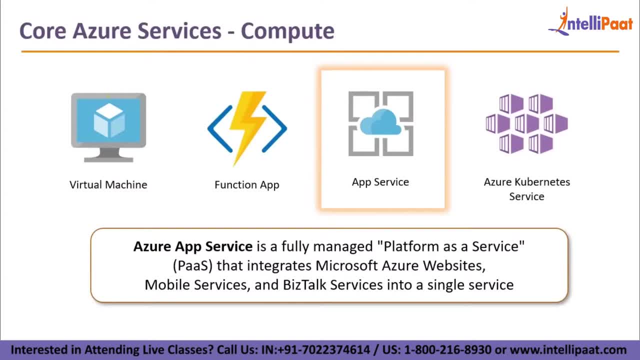 app service. in app service you would find a resource called web app. you'll have to deploy that and on that you will basically get again a dashboard, since it's a platform as a service, you will again get a dashboard where you will be able to upload your website files and once you do, 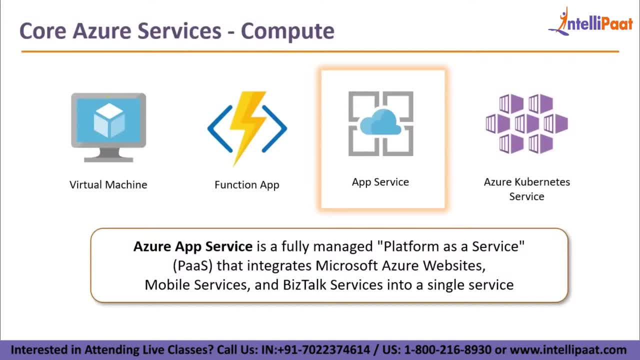 that once the process is finished, you will basically get a link, and if you click on that link, you can see your website right. so then we did not get access to the operating system. we do not have control on what softwares are installed. the basic way the app service works is- or in our case, since we are discussing about 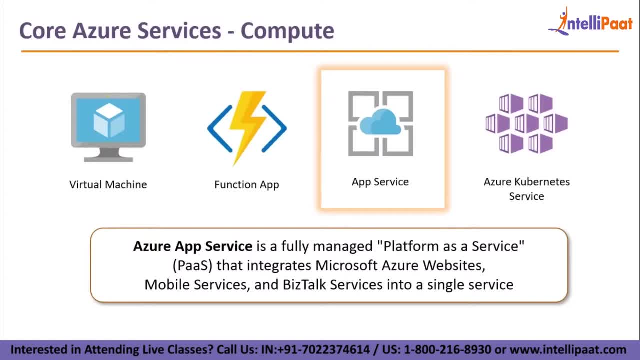 websites. our web app works is. it'll ask you: uh, what kind of code is your website written in? let's say, my website is written in nodejs, so i'll just say i'll just select nodejs and i'll click on next. and the next question they'll ask is: uh, do you want to auto scale? 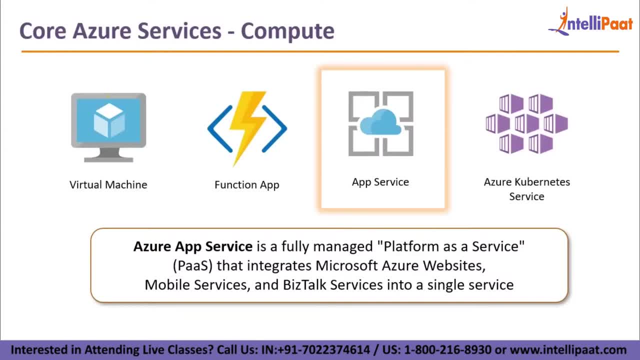 when the cpu increases or when the memory is low. do you want to auto scale? you will say: yes, i want to auto scale. you'll click on next and it does everything for you, and at the end, what you get is again a web ui on which you will have a button called upload, on which you just have to upload your website and 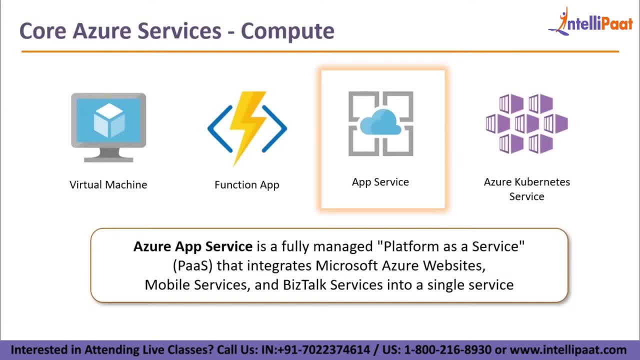 everything would be set for you right. there is also an option to just directly mention the github link. it'll pull the code from github and it'll deploy whatever code was there on github, but the application for you in function app. so this is a very tricky thing. that what is the difference? 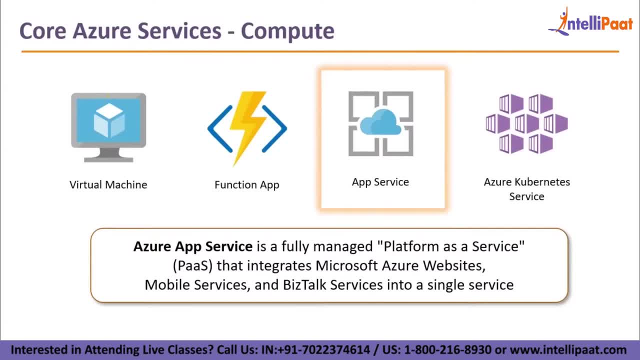 between function app and a web app. so function app only does the back-end tasks for you. you give it code, it will take an input, it will give you the output. that's it. it is not used to deploy an application app service. on the other hand, it is only used to deploy an application. okay, so this. 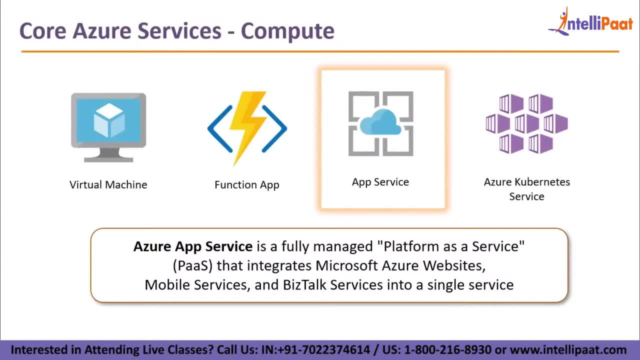 is the main difference between a function app and an app service. a next service is probably the, a important service when you're working in a containerization environment. so i'm sure most of you know about what docker is. if you don't know, just type on youtube docker tutorial by intellipaat. 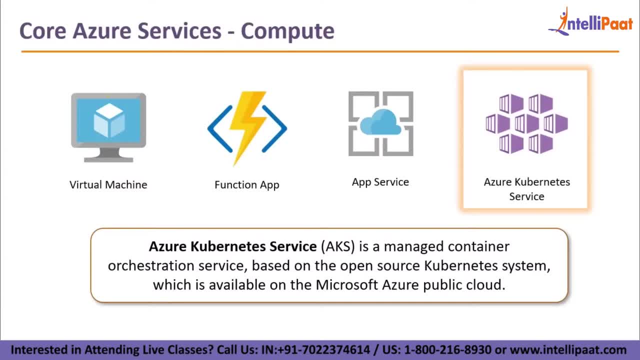 go through that video and you will be able to understand. you know what docker is. so docker is nothing but a containerization platform on which you can deploy applications. so we were talking about distributed computing, right? so containers are nothing, but they act as separate virtual entities, which are 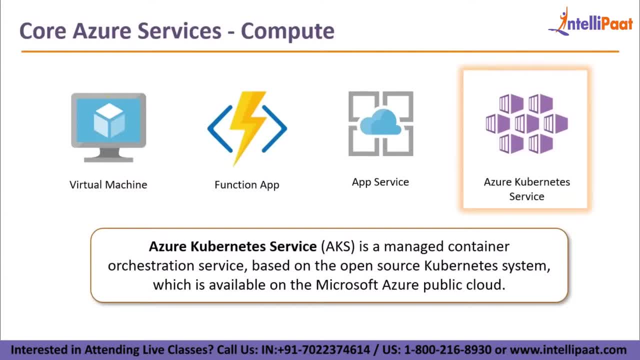 isolated from each other. so i can launch an ubuntu container, i can launch a centos container, i can launch a different flavor of linux container as well. right in them i can install any software i want and exactly whatever code files i want i can put on those containers and these containers can. 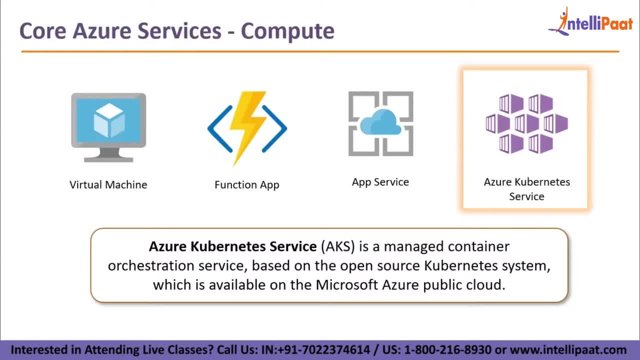 then interact and mimic a distributed application kind of a scenario. right now, what kubernetes is? it manages these containers. for you, it's an automatic service which manages these containers. what? what does it manage? let's say, uh, you know, i deploy three containers: one is my website container, one is my backend container and one is my database container. 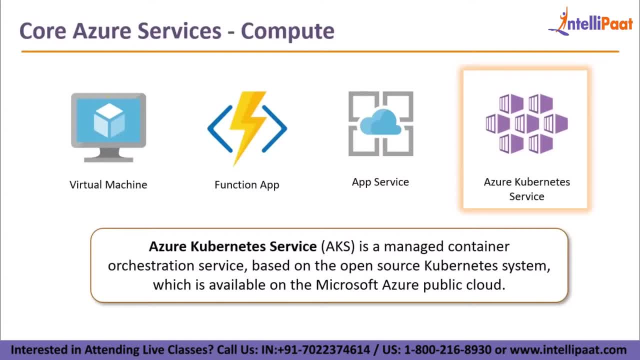 now, for some reason, my backend container is not working. okay, it stops working. now what will happen? what should ideally happen, ideally my? if my backend server stops working, i need to get an alert. i will go there, i will see what the problem is, i will fix it and then my backend container or backend server. 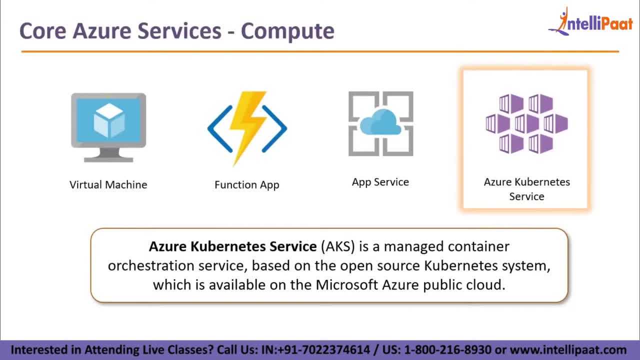 and my application would serve normally. but what happens is you cannot monitor application 24 by 7. so what kubernetes does for you is it does all the manual tasks for you. so it automatically detects that a fault has occurred in a particular container, and what it does is it deletes that. 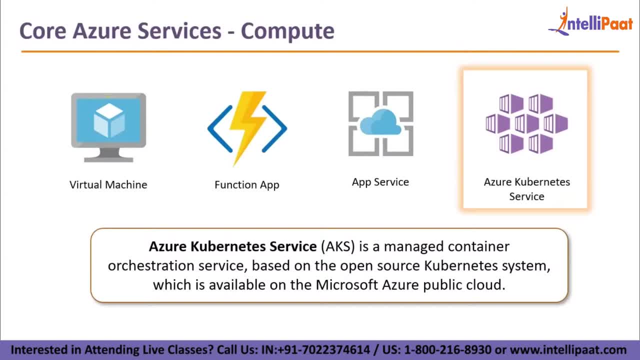 container and launches a new copy of it automatically. right, and this is just one of the tasks that kubernetes does automatically for you. you can also configure kubernetes to scale your containers for you, and you can also configure kubernetes to scale your containers for you, and. 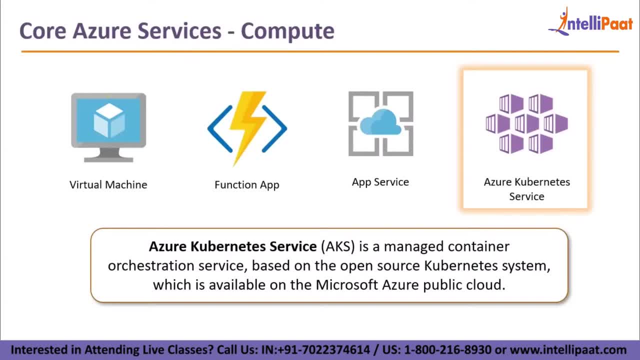 it can do a host of other things and we would discuss it probably. uh, when we move along and we just when we just are focusing on azure kubernetes for service, we can actually talk more about it because there are loads of features in it, but this is again a very important service. 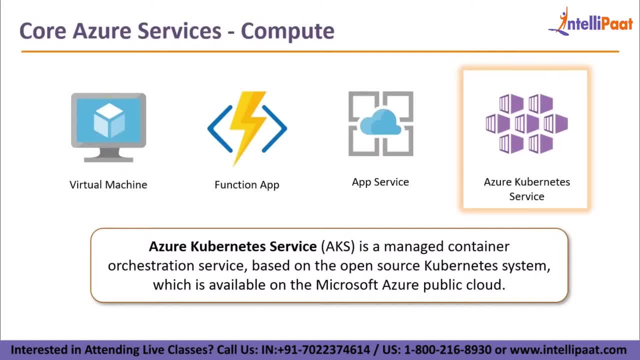 so most of the startup companies- uh, not, not mncs, but most of the startup companies- have now adopted the container architecture or have now uh made their code into, uh fit into- containers, and now they are using the kubernetes service. if i want to give you a little background of the kubernetes service: the kubernetes service was actually 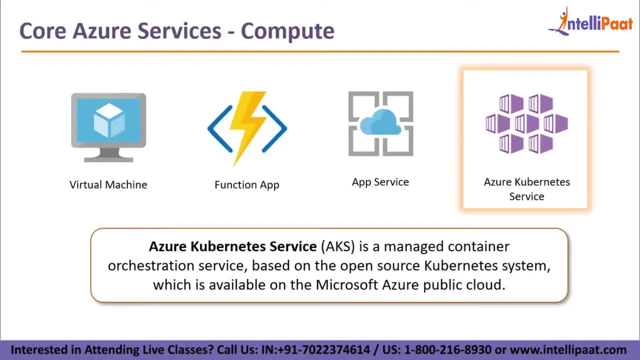 developed by the google company. later they made it open source and now it's available to the world. anybody can use it or download for free and can actually install it on their system. right, but when you install it on your system, you actually have to manage kubernetes all by yourself. so what? 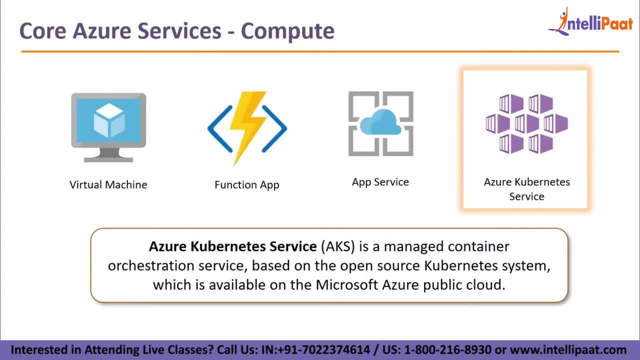 azure does is. it has created platform as a service again and it says: i will handle the kubernetes installation, i will handle the kubernetes configuration. you just tell me what you want and i will deploy that in a kubernetes cluster for you, right? so all the advantages of kubernetes you get and you also don't have to deal with kubernetes. 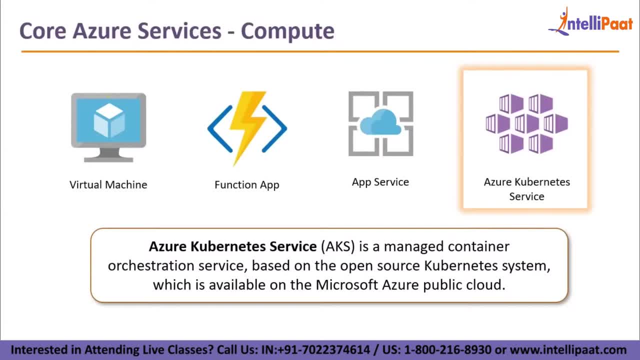 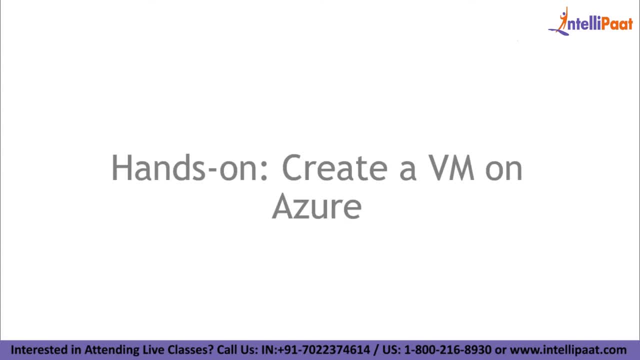 so this is the power of cloud. this is what azure is giving you as a service, right? and this is what azure kubernetes service was all about. all right, guys. so now let's get down to the interesting part. let's now start off with a hands-on. 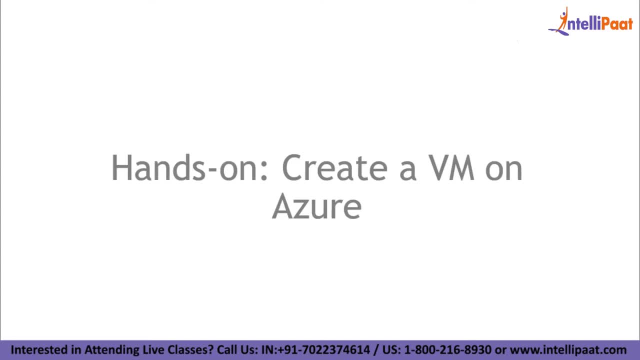 where you will get an taste of how, as basically, azure portal looks like, and also how things work out, how you deploy resources on azure and basically, in the most essence, we learned about what a vm is. so we're gonna see how we can actually launch a vm inside microsoft azure. all right, so just give me. 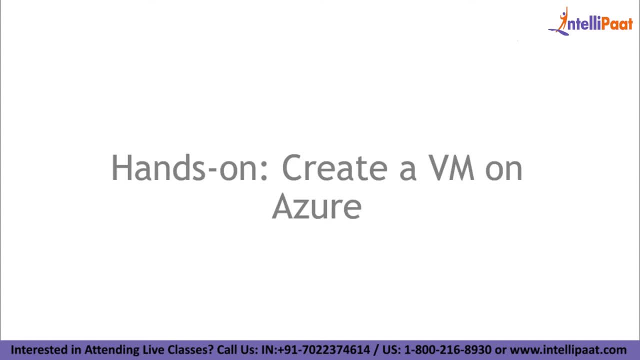 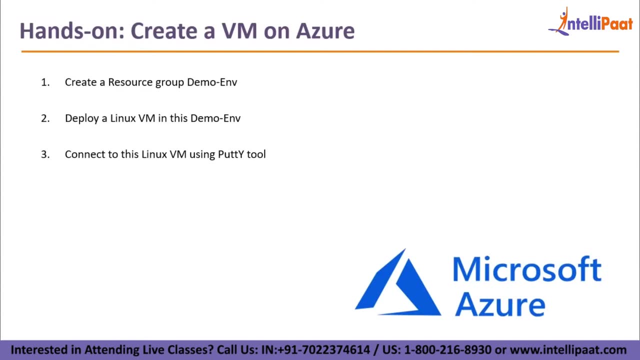 a minute. i'll just switch on to my portal and then we will start on with the demo now, before moving over there. guys, these are the three things that we're gonna do. so, uh, when we were learning the software and the infrastructure, i told you guys that basically all the resources that 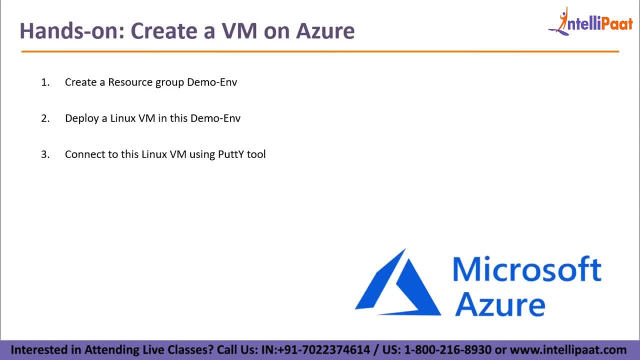 are deployed on in azure can be managed, or they can be grouped together using resource groups. so the first thing that we're going to do is we're going to create a resource group, which will have the name demo environment. okay, then, what we're going to do is in this demo. 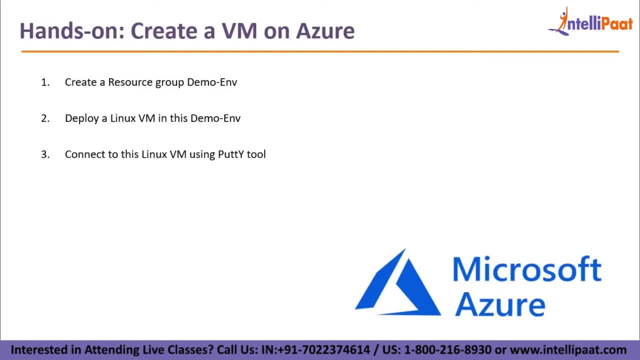 environment. basically, we're going to launch a virtual machine which will have a linux operating it. now, once it is deployed, we will try to connect to this virtual machine using the putty tool that is available for doing SSH on Linux. so basically, when you're, whenever you're installing or whenever you're launching a Linux, Linux 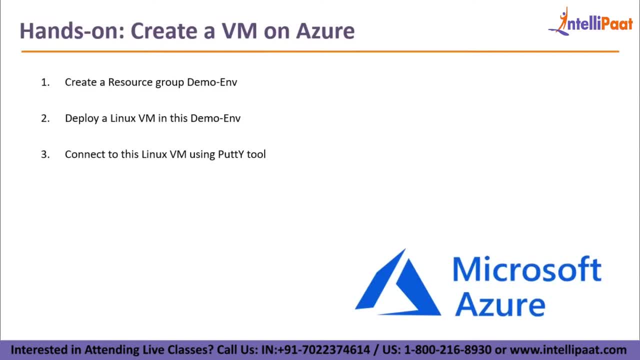 instance, a way to connect to a Linux instance is using SSH, right, because it's a command-line operating system and all, everything and anything that you want to do on this operating system, you can do it on the command line. on the contrary, if you deploy a Windows machine, in that case you have to use the remote desktop. 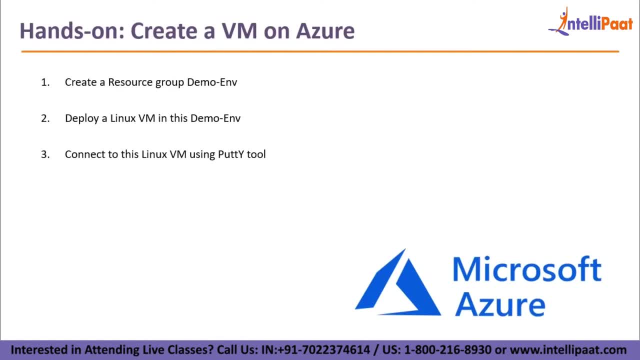 protocol, so it's basically called RDP and there's a software for that which can basically connect using RDP. so that is inbuilt in Windows. so if you are on a Windows machine, just type on type remote desktop right, and you will get that application. the only thing it will ask is the IP address. click on connect and 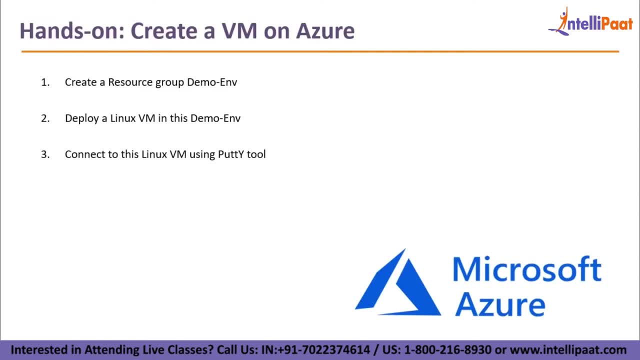 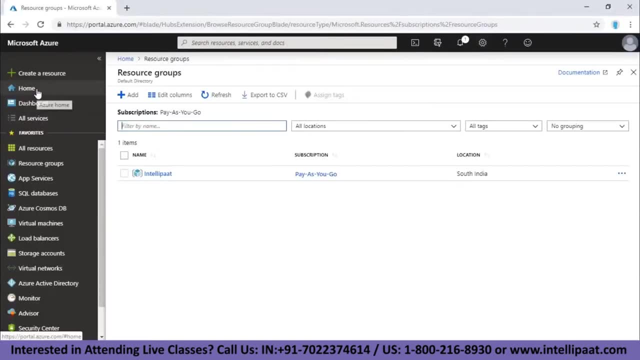 then last for the password. alright, guys. so, without going any further, let's get started. okay? so, without wasting any more time, let's go ahead, switch to my Azure portal and let's see how it looks like. right? so, guys, this is my Azure portal, so let me just go to home and let me show you how it actually looks like. 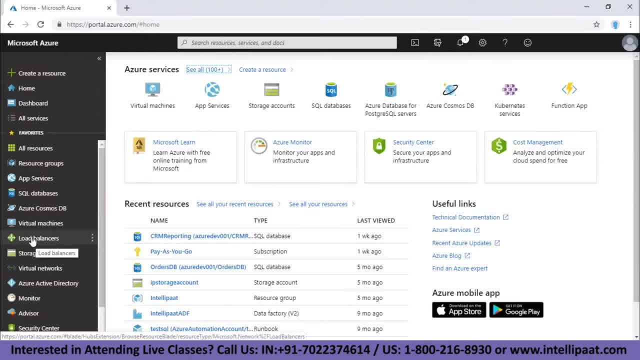 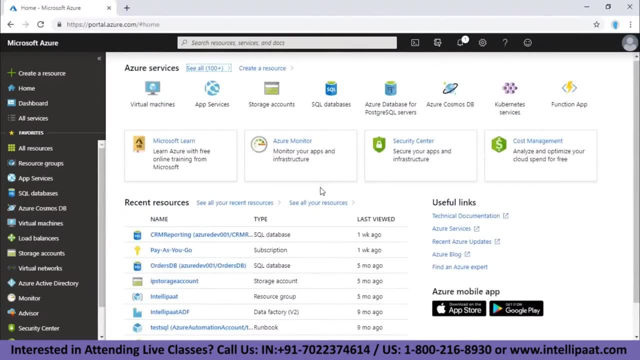 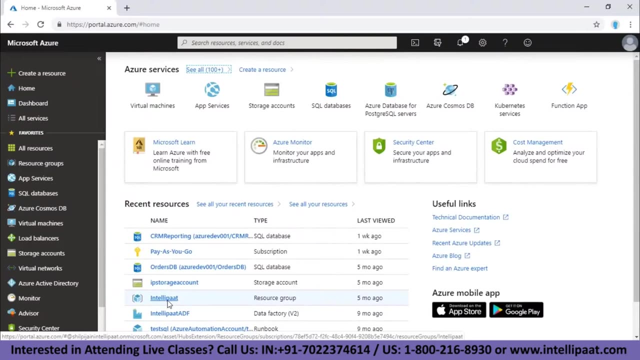 so this is how your portal looks like. guys, this is the web UI that we were talking about. now there are some resources that are already launched in my Microsoft Azure right. so, as you can see, I've named my resources something like this. but let's say, I'm going to deploy a Linux VM now. 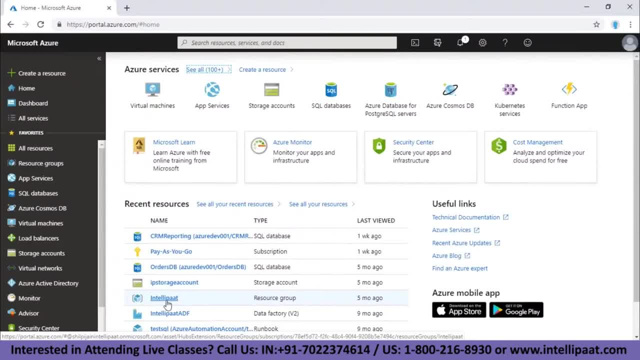 right and I'm going to deploy it to my Microsoft Managed Elements- that Linux VM is only for demo purposes. now this will actually give you a take as to how you can, or how resource groups basically can, help you guys. now, if I go to all resources right now, you can see these are all the resources which are. 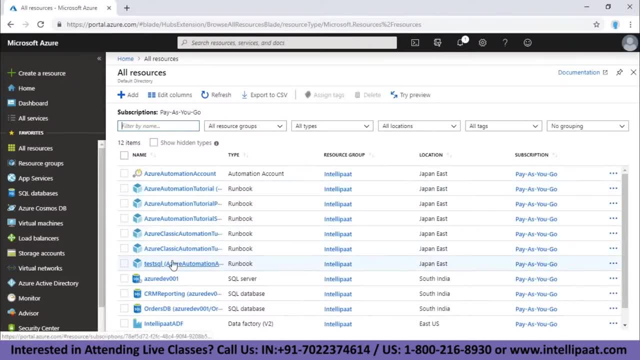 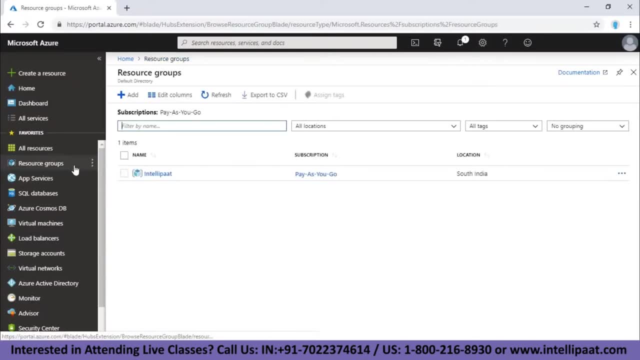 deployed on as your right now, but I do not know which resource is doing what or which resource is contributing to what application. on the contrary, if I go to resource groups, you can see that there is a group which is called Intel apart, which exists on my Microsoft Azure portal, and if I go inside this resource, 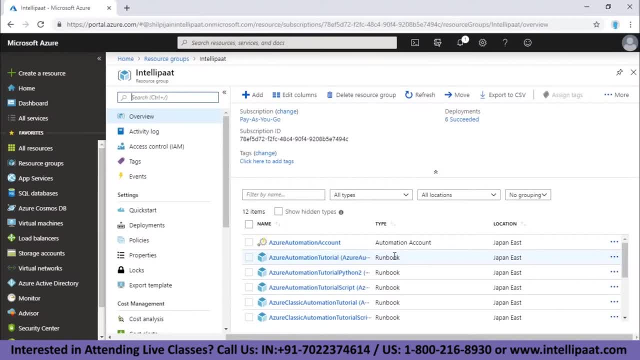 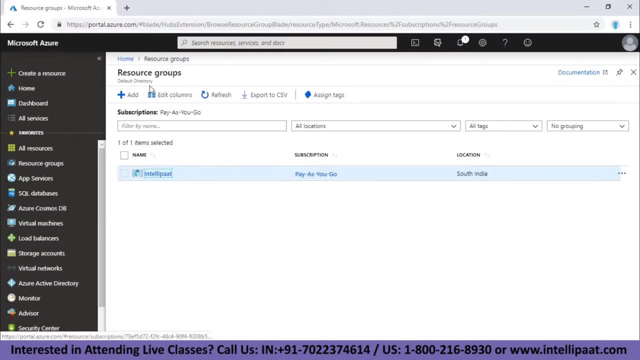 group, I would be able to see all the resources which have been deployed. so now, what I'm going to do is because what I am doing right now is just for demo purpose. so what I'm gonna do is I'm gonna add a resource group. so let me. 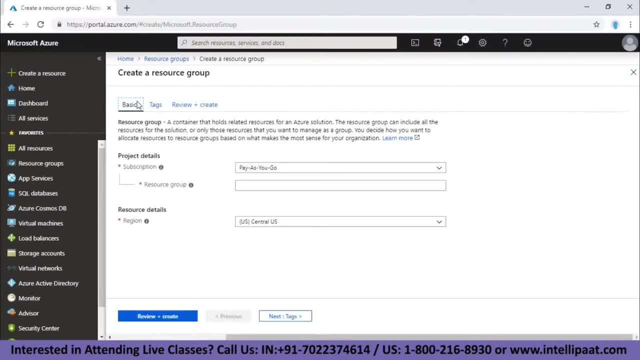 just click on add and let us create a resource group by the name demo environment. so I will type in demo, demo, demo env. right, and let's say the region that we have to choose: always choose a region, guys, which is nearer to you. so what do you mean by region? so region? 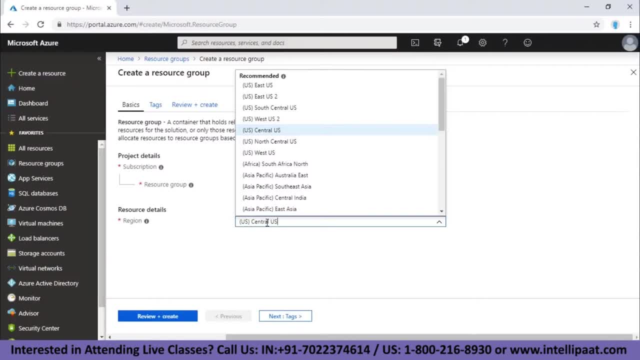 basically means now Microsoft Azure is so huge that it has deployed or it has set up its data centers in different countries. the reason they have done so is because, let's say, you have your application and you have a startup and you have actually started it up in, let's say, India. right, and your application is. 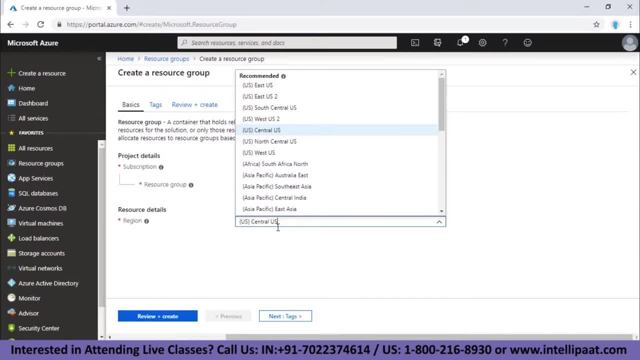 actually only accessed by the Indian audience, right? so that's whom you cater to. so what you can do is, rather than deploying so it makes more sense to deploy your application or your website on in in a region which is nearer to your audience, because in that case, if the internet routes, it'll be far lesser when. 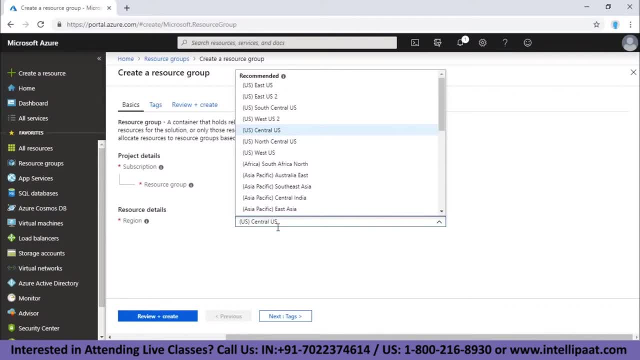 you compare it with launching your application in some other country. for example, let's say we launch this resource over, create this resource group in, let's say us right. so we create this resource group in, let's say, the US, right, but my target audience is basically in India. now, what is gonna happen now, when? 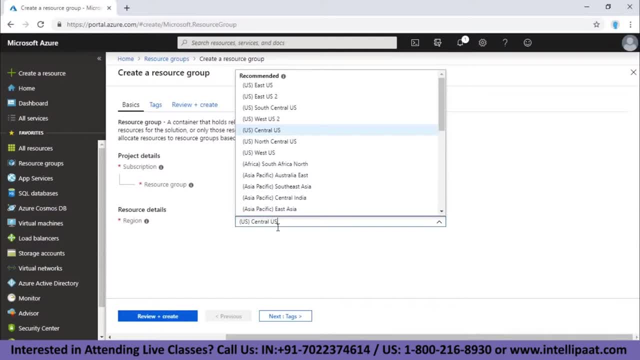 my target audience audience is in India and let's say I'm going to the intellipaatcom website. that is my application. every time. the data is being fetched from the US and it is being transferred to the Indian servers and then from your ISP, you are getting the data on your system. now, if we were to 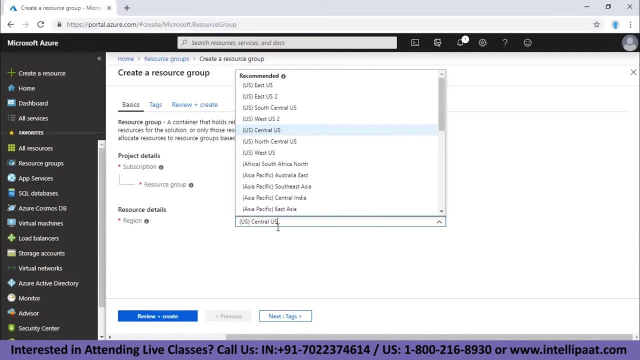 make, or if you were to deploy our application in India itself, what will happen is that the distance that the data has to be cover data will cover will be less, and that will significantly increase your response time of the website, right? so that is why choosing a region is very important. you can choose. 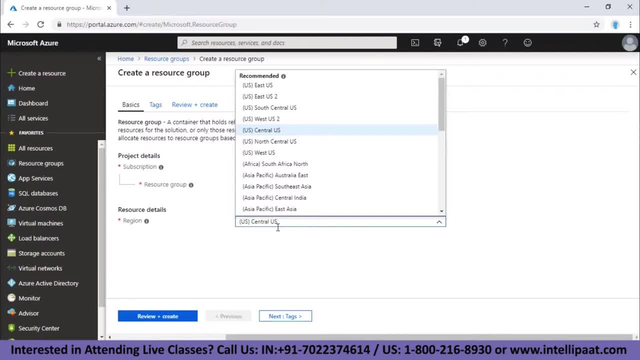 any region you want, but I would suggest you choose a region which is more nearer to you, right? so in our case, let's scroll down and see if we have any region which are nearer to me. so I can see that we have a region in India is called South. 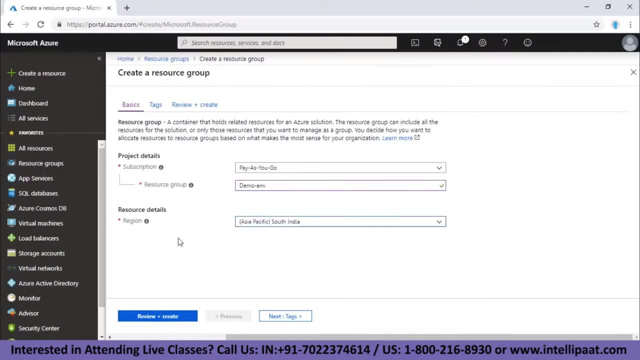 India. so let us select that, and then I can see that we have a region in India, right? all right, so now the region that my resource is getting deployed is in south india, right? so that's what i've selected. the name that i've given is demo environment, and now let's go ahead and 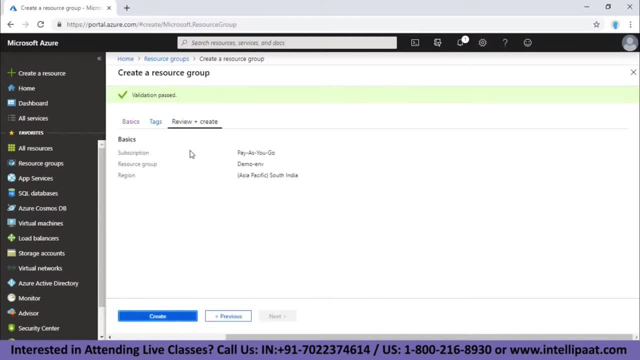 click on review plus right. so this is what is going to happen. the subscription is going to be pay as you go. if you are under free tier, you will see free tier, the resource group. this is the name that i've given, and the region on which this is being deployed is south india. let's click on. 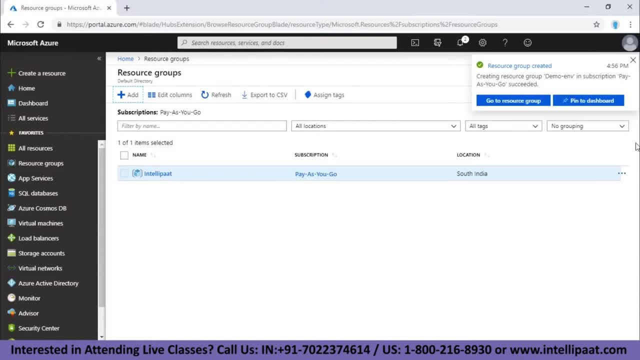 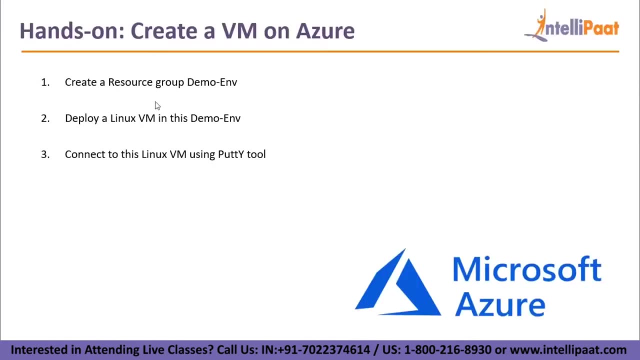 create. so now my resource group is being created right, and if i do a little refresh over here, i can see that my demo environment resource group is present here. now what i want to do- the next step that i have to do- let me just go back to my slide- is to deploy a linux vm in this demo. 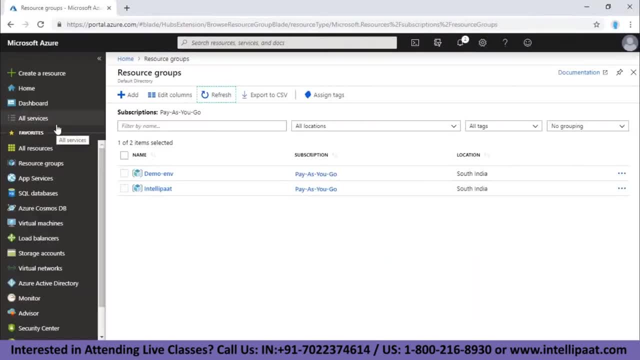 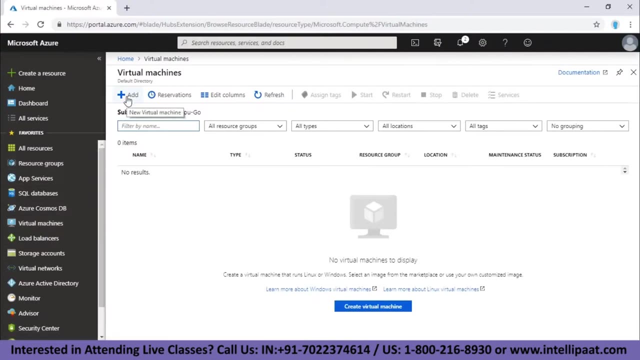 environment resource group. so let's do that. let us come back to our azure portal, and now what we want to do is we want to deploy a virtual machine. so you will see on the left hand side that there is a service called virtual machines. let's select that. and now what i have to do is i have to click on add right. so 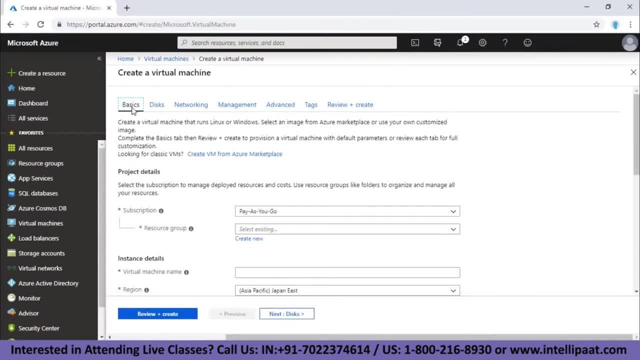 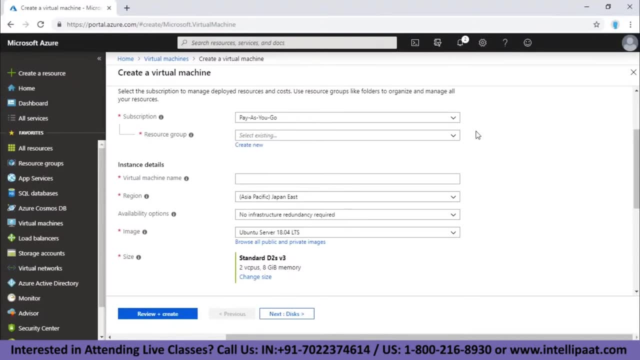 because i want to create a virtual machine. so i'll click on add. now it'll ask you which resource group do you want to make this server available in? so i want to basically make it available in demo environment. so this is what i've selected. what do i want my virtual machine name to be? 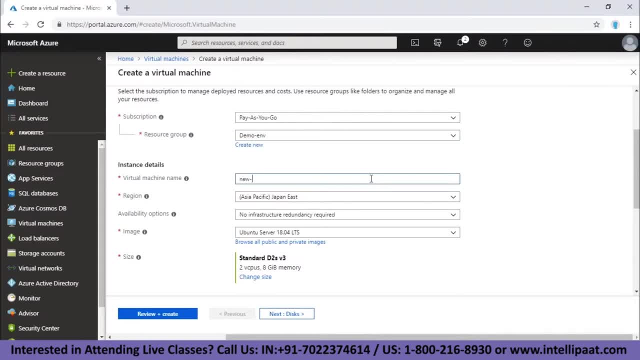 let's say i want my virtual machine name to be new vm hyphen linux. okay, this is what the name is, the region i want it to be nearer to me, so i'll select as south india right availability options. if you go ahead and choose it, you will have an option. 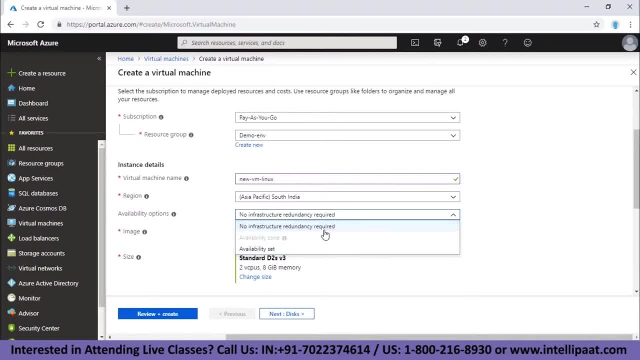 between availability set or no infrastructure redundancy required. so what is redundancy? redundancy basically means: do you want a copy of your server somewhere else as well, so that, let's say, in the data center where this server is going to be deployed, that data center goes down, something happens and the data gets corrupted. so if you choose that, you know you want to replicate. 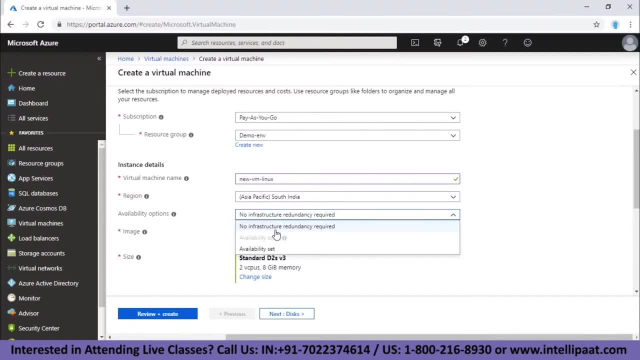 your server. what will happen is, even if there is a downtime in a particular data center in which your vm was deployed, your redundant server will come into power and that is from where you will get your data. so, basically, it increases the availability of your application. and even if 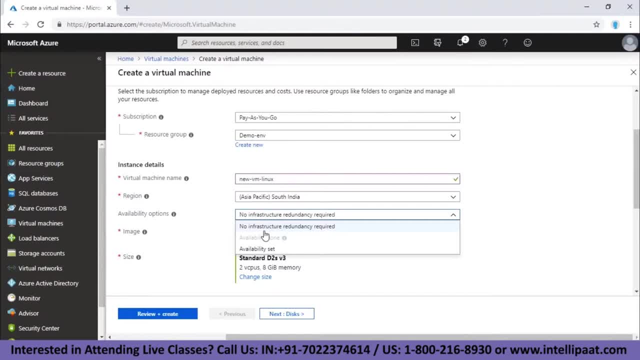 there is a problem from the azure side. your application will not go down, but since we are doing a demo, what we will select is no infrastructure redundancy required. uh, what is the image that you want? so by image we mean the operating system. which, what? what kind of 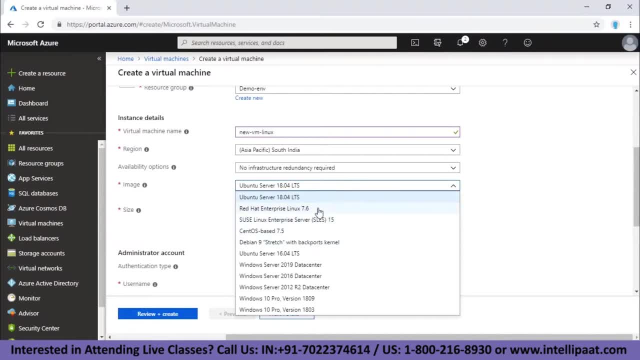 operating system do you want to connect to? right? so you have all these operating systems over here. i can actually launch a windows 10 pro. i can launch a windows server. i can launch ubuntu 16. i can launch dbn 9, centos, suzy linux, red hat, ubuntu server, right. so for our sake, let's consider ubuntu. 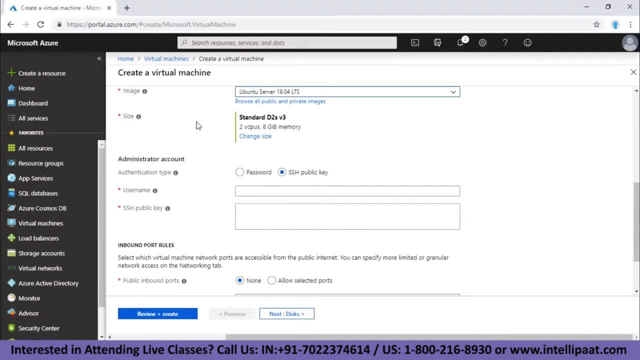 what we want to deploy. and now it'll ask me: what is the size of the machine that you want to give right? so what you can do is you can actually change the size. so by default it will say you should deploy a 2 cpu and a 8 gb machine. you can just click on change size and you will have all. 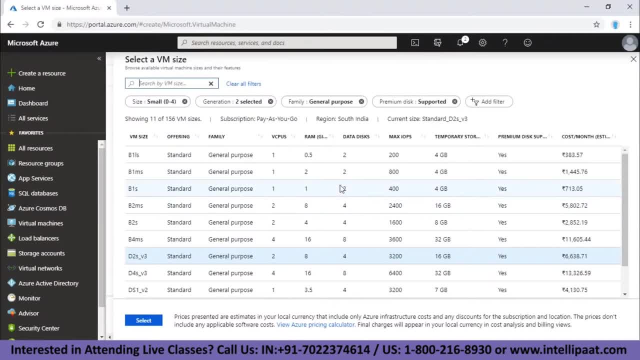 these options available to you. right, so you can see that, because what we are doing going to do is a demo, so what you can see over here is 0.5 gb ram and a 1 cpu will basically cost me around 83 rupees per month, right, so let's go ahead and try to deploy this machine. right, so this makes. 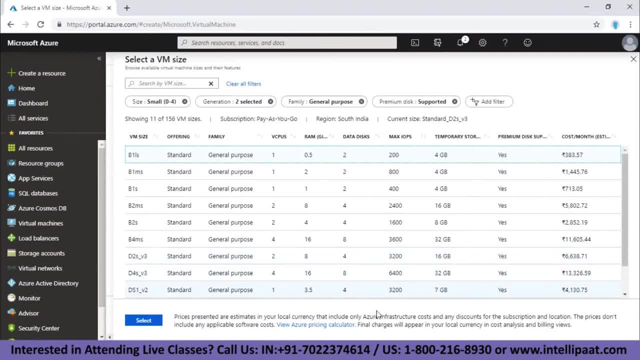 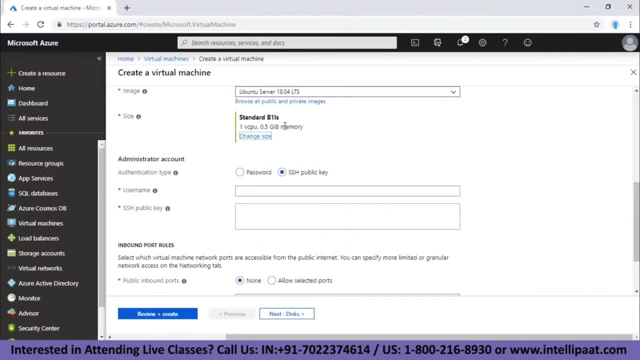 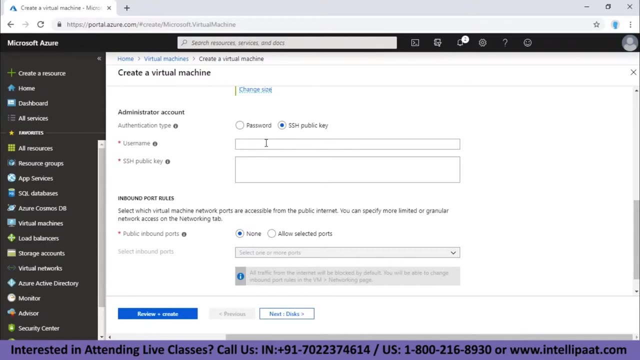 more sense, because we are only doing a demo and probably i'll delete it after this session, right? so i've selected this and i click on select now so you can see it's one vcpu and 0.5 gb memory- great. next thing it is asking me is: what is the authentication type that you want to give on? 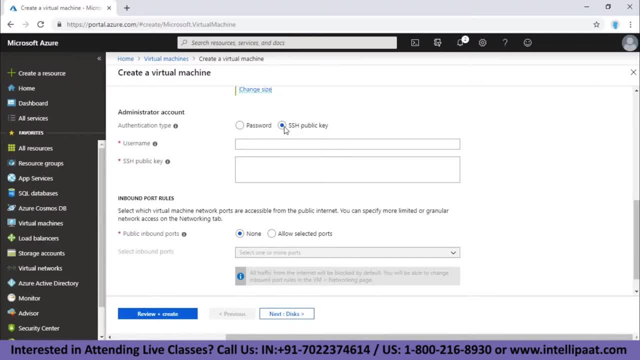 this particular machine. you can either choose the ssh public key, or you can choose the public key, or what you can choose is password right. so if you want to choose ssh public key, what you'll have to do is you'll have to generate a ssh public key right. if you choose password, what it will ask is: 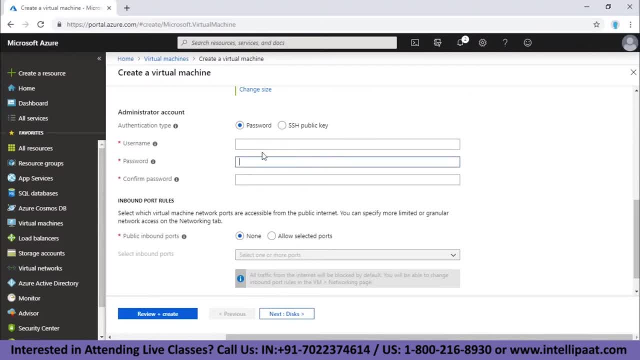 the username and the password if you- and this is basically the most standard way of doing it, but if you want to give security to your instance, the suggested method would be to create a public key. now, how can you create a public key? there is a software called. 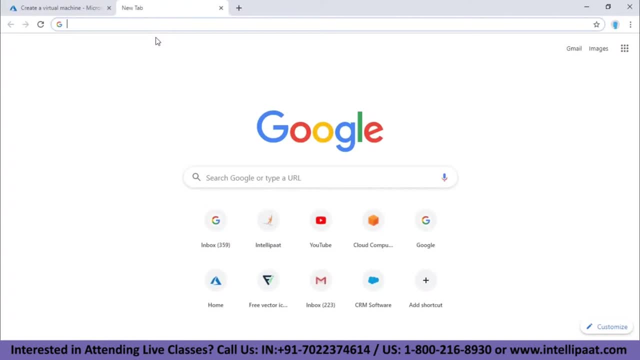 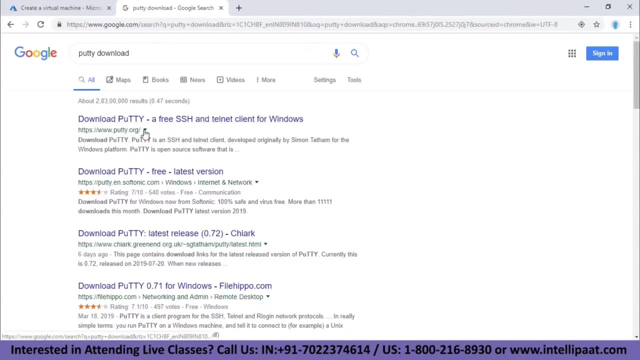 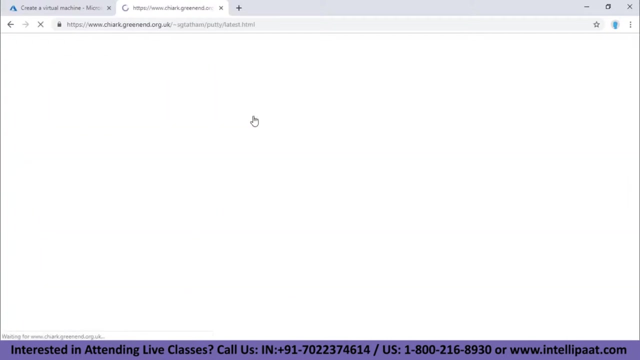 puttygen right and the way you can download it is just type on google putty, download right, and then you will get a link from puttyorg. just click on that and you can say. you will see this link which says download putty. just click over here right now. you will get all the versions on which you can. 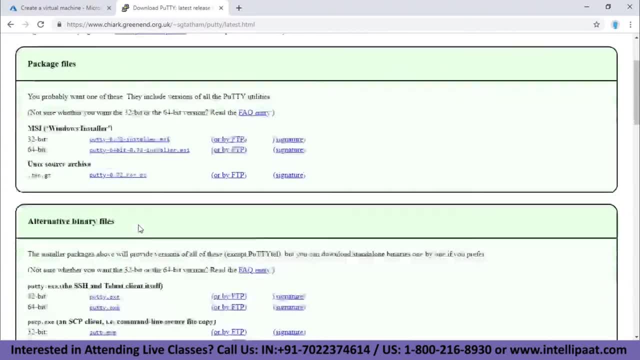 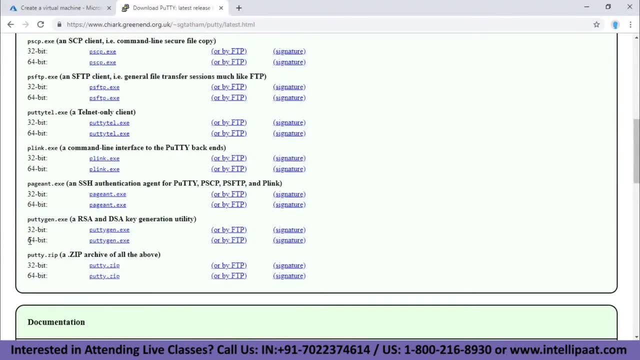 basically using which you can basically install putty. now, what we're basically looking for is puttygen, right, so you will find it over here. based on your cpu architecture, you can basically select puttygen and then you can download. once puttygen is downloaded, it will. 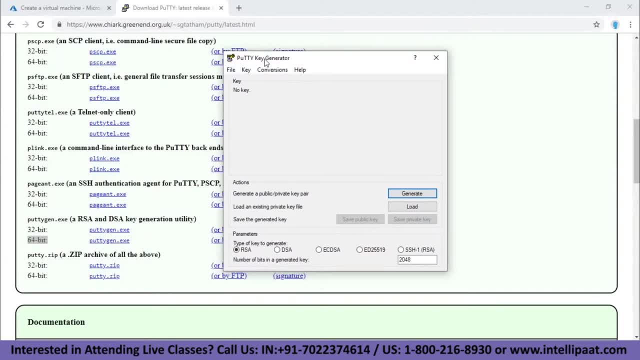 look something like this. so, as you can see, it's putty: key generator. what i want to do is i want to generate a public private key, so let's click on generate now. what it will ask is you'll have to hover your mouse here for some randomness and it will create a key based on that. so let's hover. 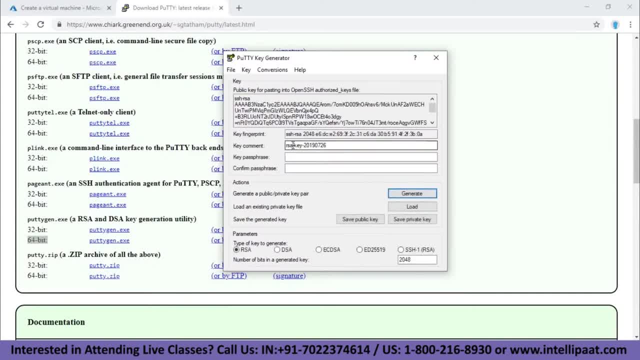 our mouse in this region and now it has created the key for me. now it says the public key is the key for pasting into open ssh authorized key file. so this is the public key, basically right, and you will have to copy this. let's copy it, right. so this is my public key. now let's come back. 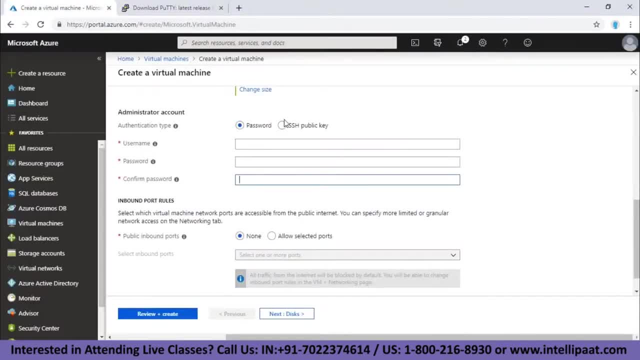 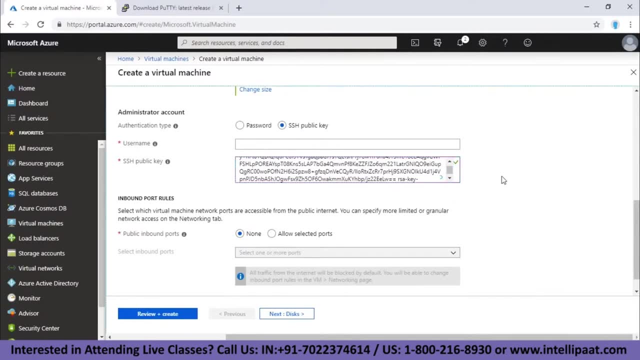 to my portal, so i can just choose ssh public key and i can paste the public key over here, and this is how it works. now, if your key is verified, what you will get is a tick mark over here, which basically means that a key has been verified and now you can go ahead, right. so my key is now. 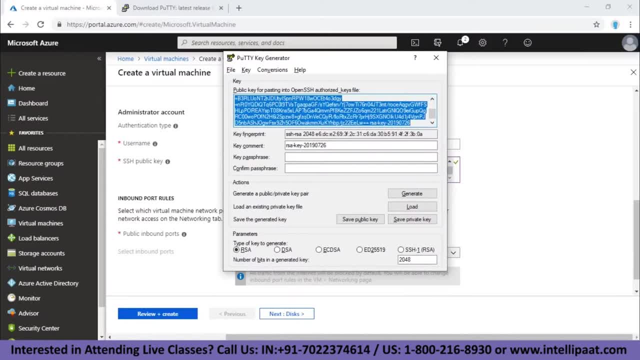 verified what that is the next step that i'll have to do. the next step that i'll have to do is i'll have to save the private key. okay, so this is the public key which has been generated. what i have to do is i have to save the private key which i'll be using to connect to my instance. so in this case, 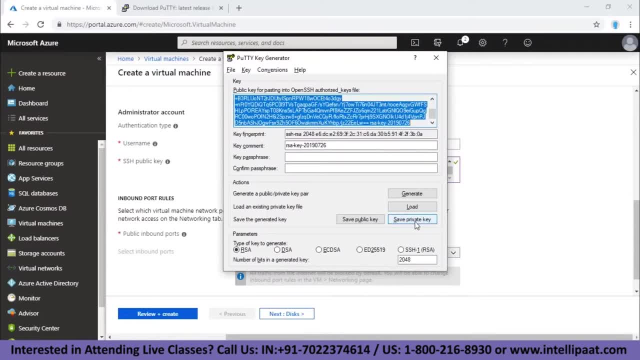 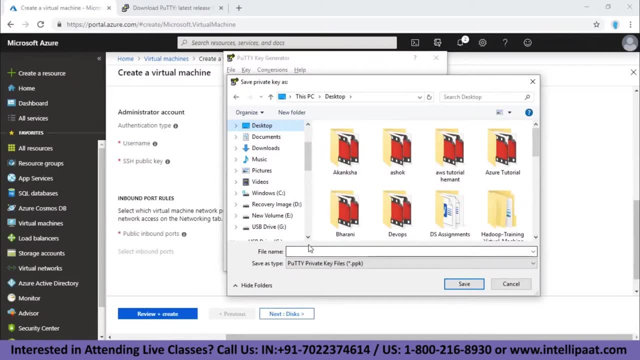 you basically do not have to use, you know, any password if you have this particular file, which i have on my device. but i've been using my device to do this. so now here, let me go to my browser and let me click on yes. let's say i save it on the desktop, or let me actually save it somewhere else. 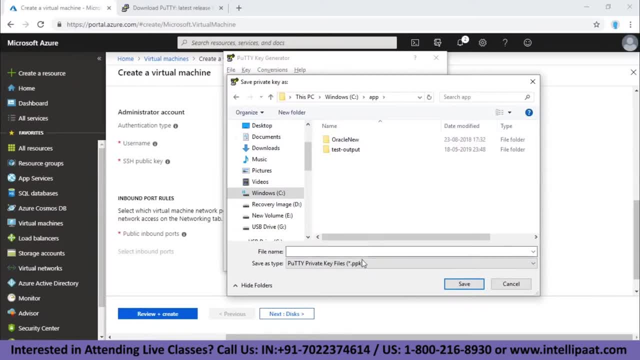 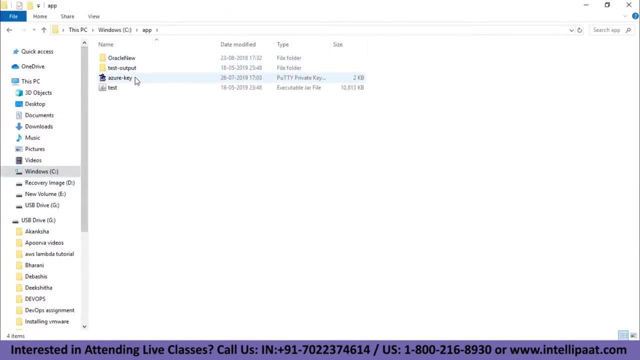 let me save it in c drive and let me actually create, uh, let's say, in the app folder, i'm just creating this private key file and let's name it as azure hyphen key, okay, and now i'll click on save. so my ppk has now been saved. if i want to go there, i can just go to see. i'll go to app and i can see that azure hyphen key. okay, so that's not a very high. 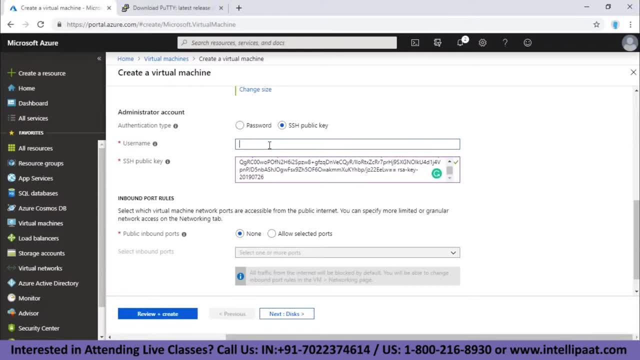 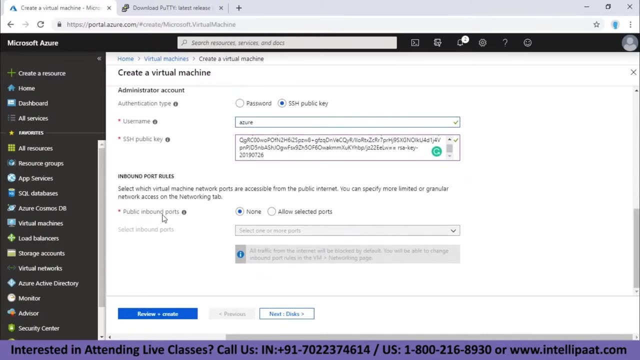 PPK is now present over here, Great. So this is done. Now I'll have to specify the username. So let's specify the username as Azure. you can specify any username that you want, Right? So we have specified it as Azure. Now the next thing that it is asking is: do you want any inbound ports? 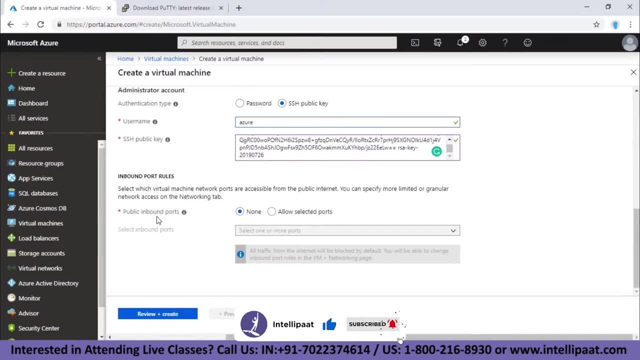 to be enabled on this particular instance. Now we will be connecting to this instance from our machine right and the protocol that we'll be using is SSH, So we'll have to open the SSH port. So we'll have to click on allow selected ports And what port do I want to allow? I want. 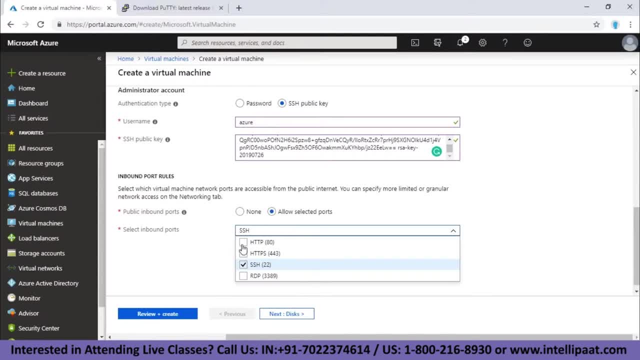 to allow SSH port. Okay, let's select HTTP also. Why? I'll tell you that in a few moments, once you have the Linux machine up and running- right In case this was a Windows machine- I will also have to enable the RDP port, which you can just tick over here. In my case, I don't need the RDP port. 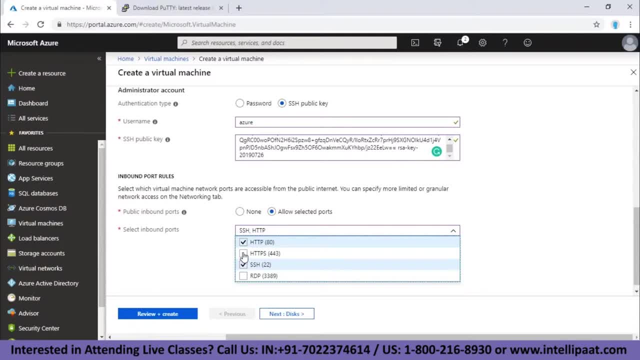 I just need SSH And I need HTTP to the use for it. I'll tell you As we move along. All right, So I want SSH and HTTP to be enabled, And what I can now do is I can just click on review plus create, And now it will basically just show me all the configuration for. 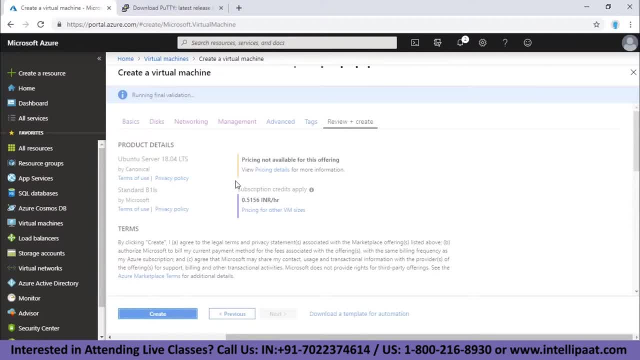 my VM, which is going by default right. I can just review it And that will be it. Right Now. I will show you something very interesting over here. Let's, once this loading is complete. So, as you know, cloud computing, it doesn't charge you per month, But basically the pricing model. 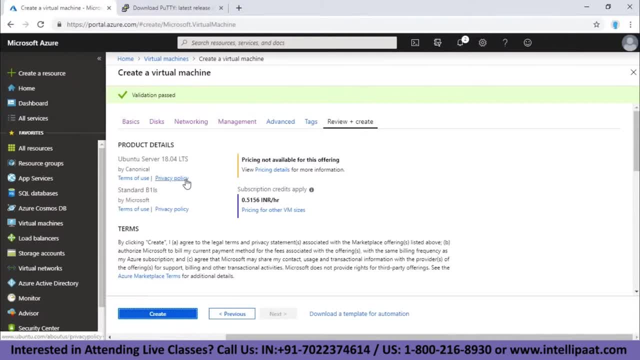 is 50 per hour kind of a thing, right? So, as you can see, the machine that I'm launching right now is, right now, 50 Pesa per hour. This is the rate, or this is basically the pricing of my machine that I'm going to launch. So that's awesome, Right. The next thing is the OS which is being launched is 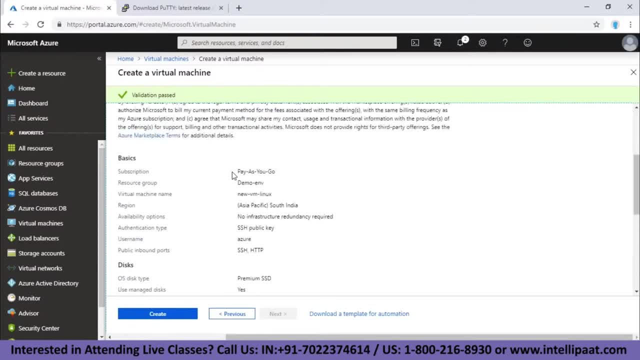 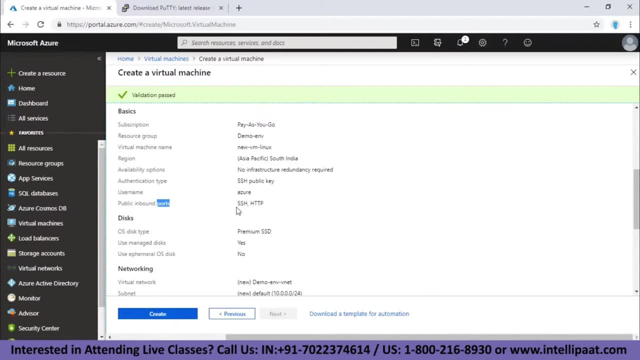 Ubuntu server 18.04.. That is also great And, if you want, you can actually look at the username, which is Ubuntu. sorry, Azure. what are the public inbound ports? it's SSH and HTTP. The disk type is SSD. Is it a managed disk? Yes, The network it's basically creating. 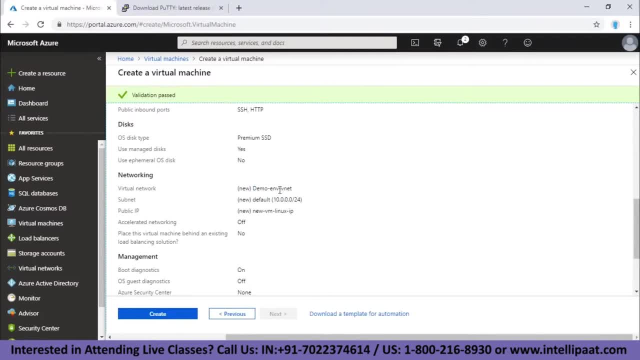 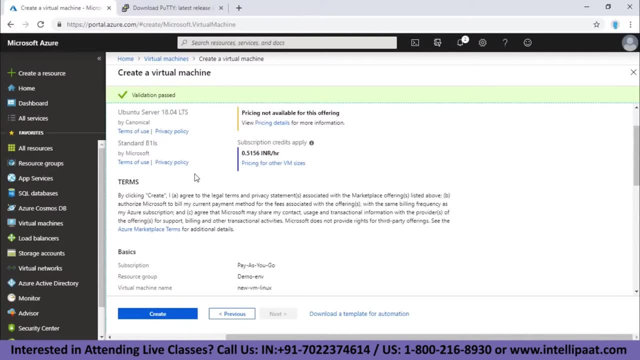 a new network for me, which is which goes by the same resource group name, which is demo hyphen ENV. So what is going to happen is, guys, when I launch this particular VM, a lot of things will be created. it will create disks, it will create networks and everything related to it will. 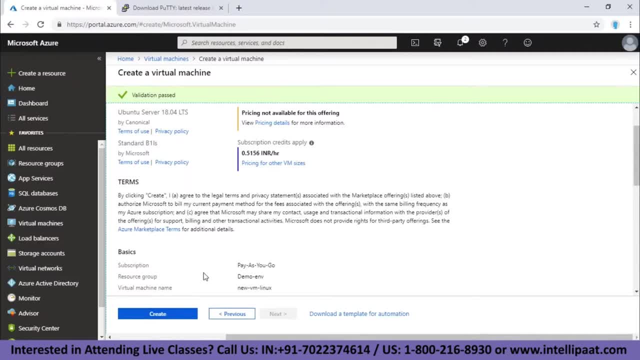 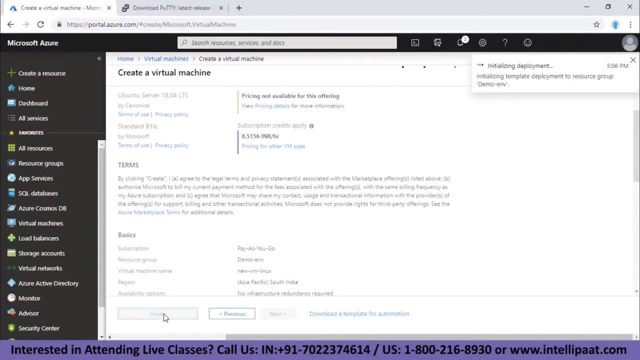 actually go inside that particular resource group, right? So I'll show you how to do that. Just click on Create once you feel everything is right And now my machine is basically getting created. Okay, so let's wait for a few while. it will take like a 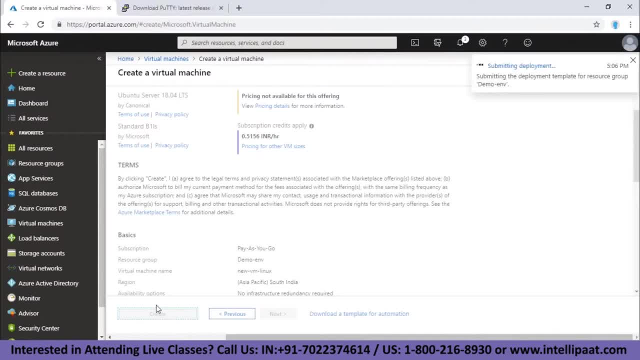 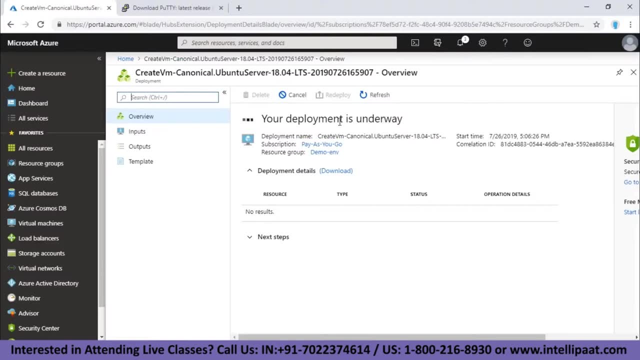 minute or so to deploy a machine. So let's wait for that time And let's hope this deploy soon. So, as you can see, it says your deployment is underway. Once it's complete, you will see a different message over here, So let's wait for that message to appear. 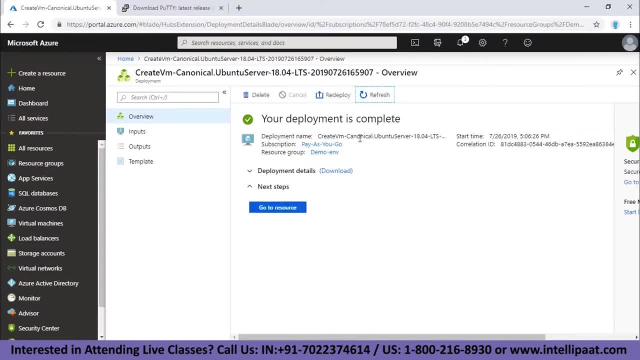 All right, guys, so my deployment is complete. As you can see, the message is being told over here, So the next thing that I'm going to do is I'm going to go to resource groups, And now I can see that I 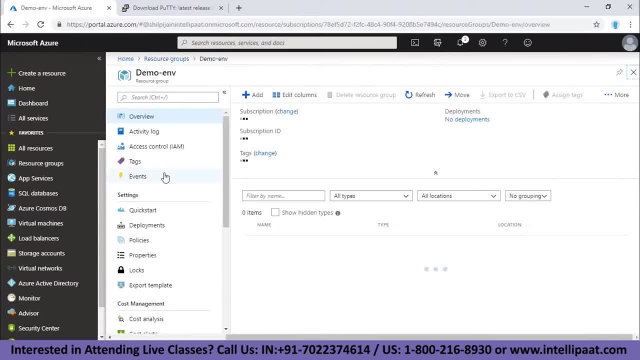 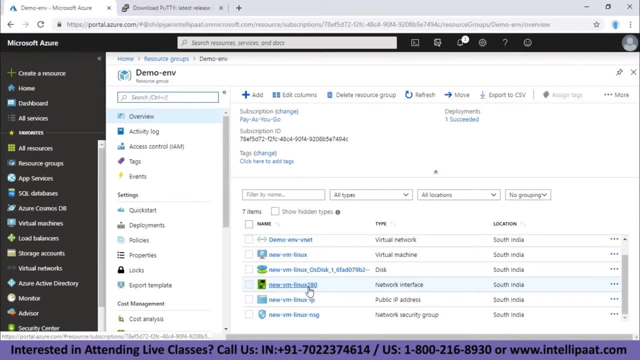 have something called as demo hyphen ENV. I will go inside that, And over here I have all the related resources to my VM. Okay, so, guys, as you can see, my virtual machine is this particular resource, So let me go inside that. 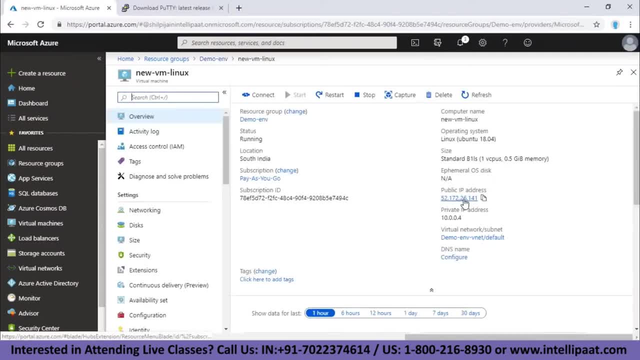 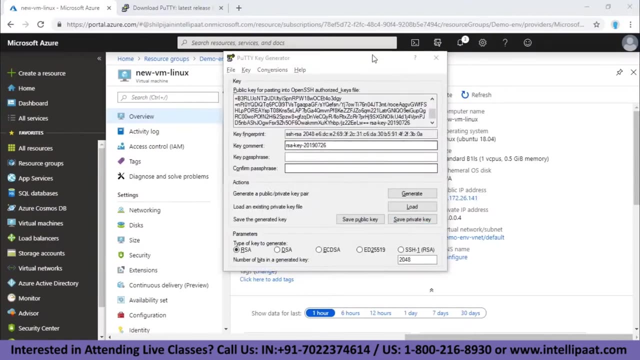 And now what I'll have to do is I'll have to select this IP address. This is the IP address on which the instance is available. So let's copy this IP address. And now let's open the putty tool. Now, what is the putty tool? We used putty gen before to create the key, Now for connecting. 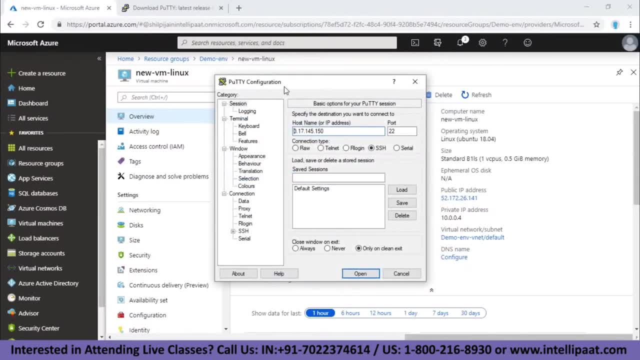 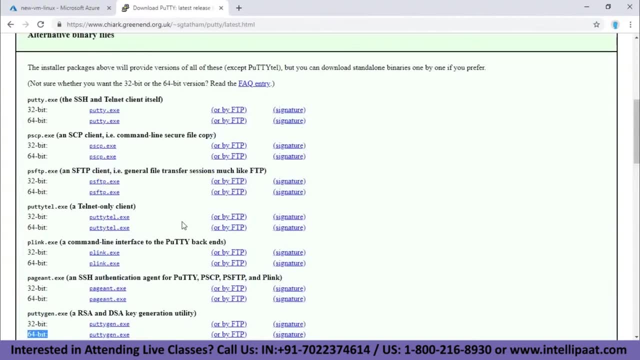 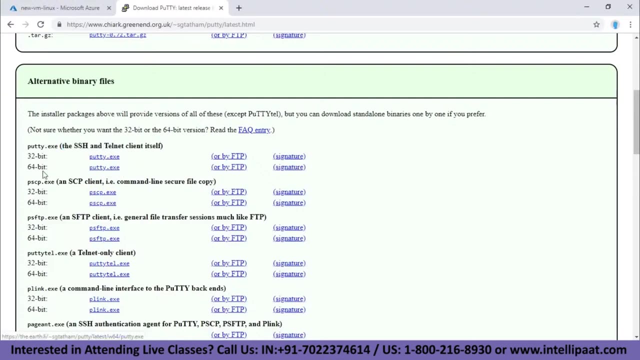 to the instance, you will have to use the putty tool. Now how do you download the putty tool? Again back to your tab where you open the download web page. Now over here you will have to select the puttyexe. It says the SSH and telnet client itself. You'll have to download this according to your 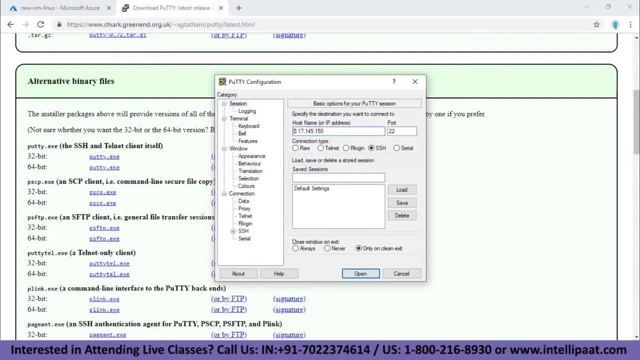 architecture, And then you will have a tool which looks something like this. Now what I want to do is I want to connect to this IP address, which I've just copied from the Azure portal, And I will have to go inside SSH And I'll have to go inside auth, And now I will have to select the PPK, which 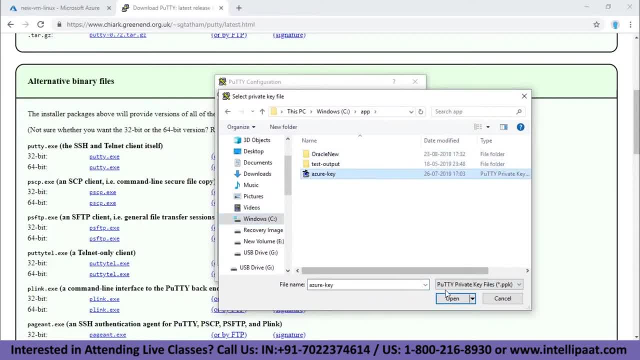 will basically be used to connect to my machine, which is Azure hyphen key. Let's click on open. And now I will have to select the PPK, which will basically be used to connect to my machine, which is Azure hyphen key. Let's click on open. 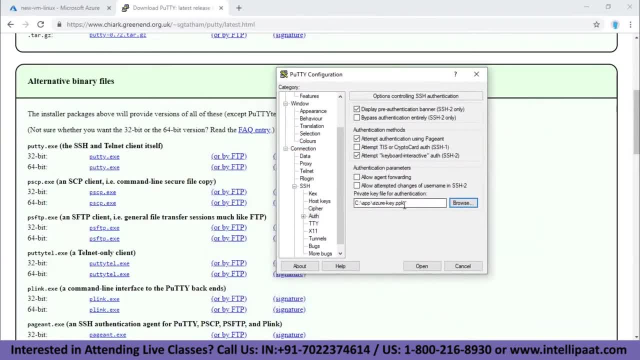 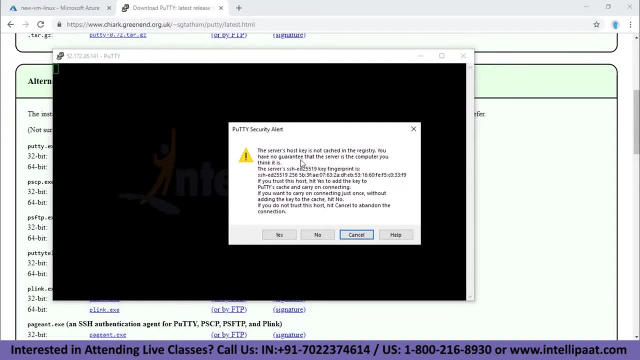 And now everything is ready, guys. So I have selected the PPK, I have inserted the IP address And now let's click on open. So it will ask: So whenever you connect to a new IP address, it will give you this warning. Don't worry about it, Just click on yes. 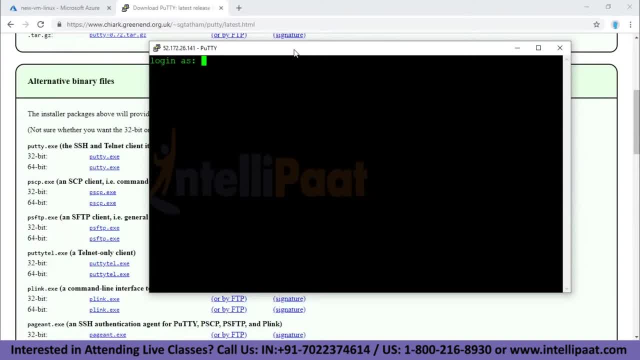 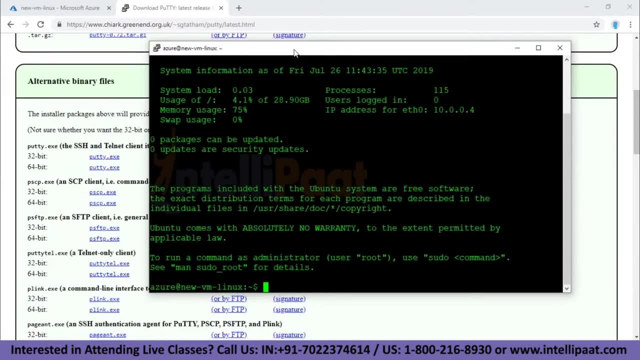 And now it is asking: what do you want to log in as? So remember, the username that we gave was Azure, So let's select that and hit enter, And that's it. That's about it, guys. Now you're inside your. 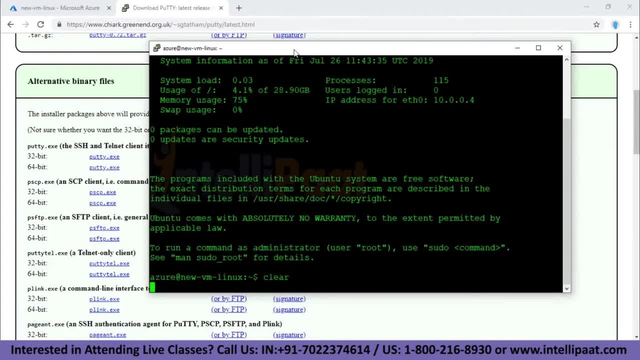 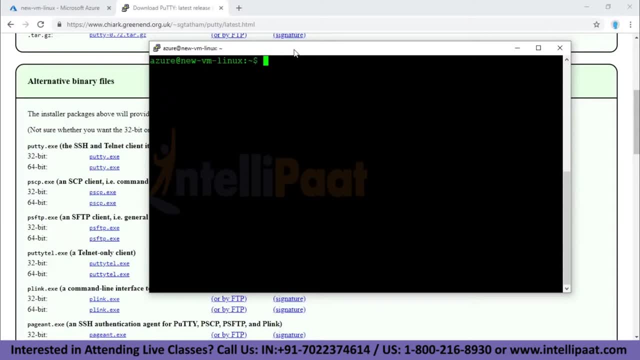 Linux machine, which is the Ubuntu machine, And now you can do anything with it as you feel necessary. right Now, you will ask me one thing that you know: we deployed, we allowed HTTP connection. Why did I do that? Just to show you one very awesome thing. 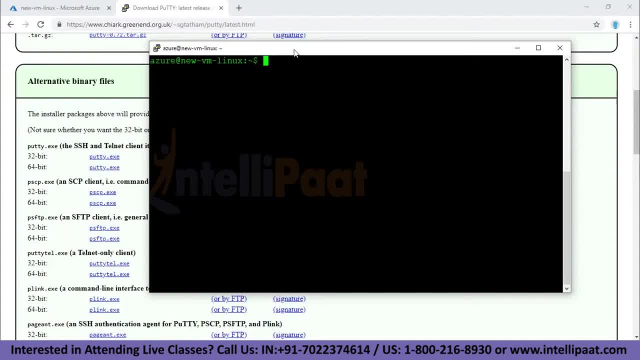 Now, since this is Ubuntu, the commands that I'll be entering now is basically for Ubuntu, And if you want to copy these commands, you will also have to install or you will have to launch Ubuntu OS, Right? So what I'm going to do is I'm going to make this server as a web server. So in order to do that, I'll pass on the commands sudo, apt-get. 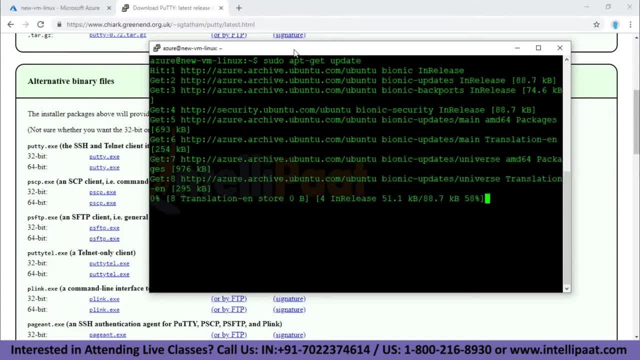 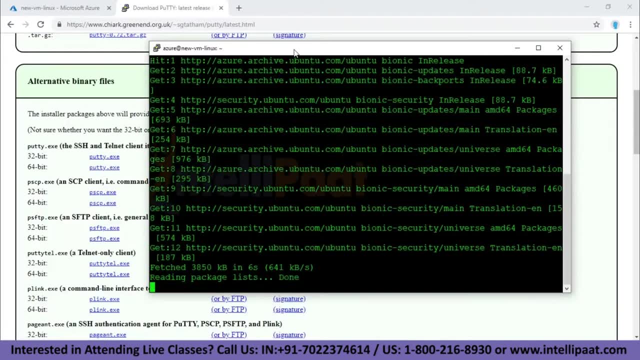 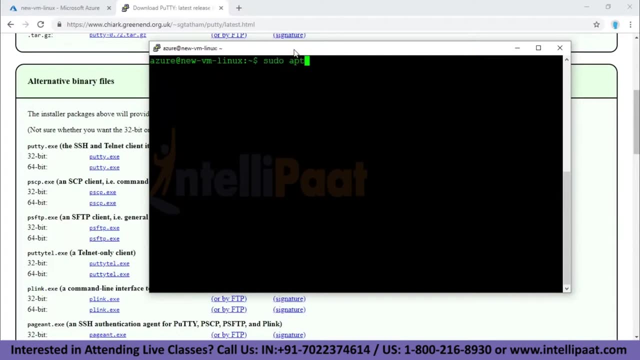 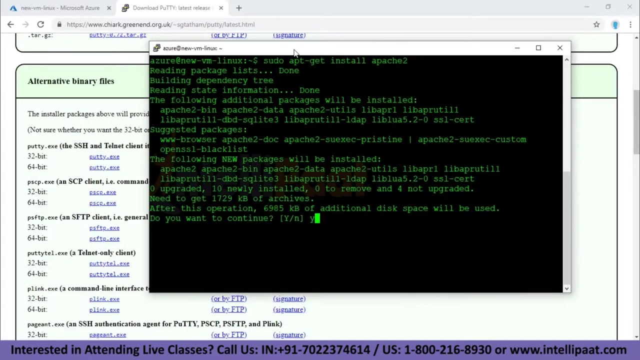 So let's update this machine. first, sudo apt-get update, And this will now update the machine. All right, So my machine is now updated. Now let's go ahead and install Apache. So sudo apt-get: install Apache 2.. So, guys, what is Apache? Apache is basically a software for web server, And what is? 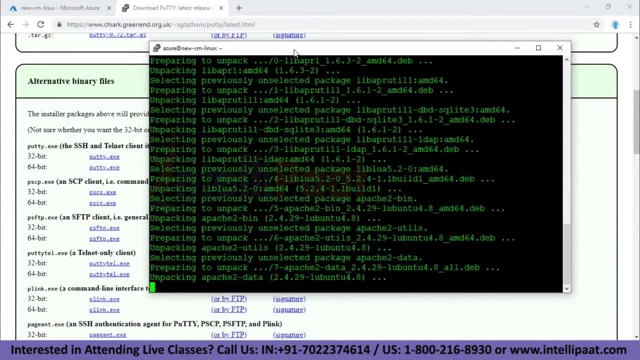 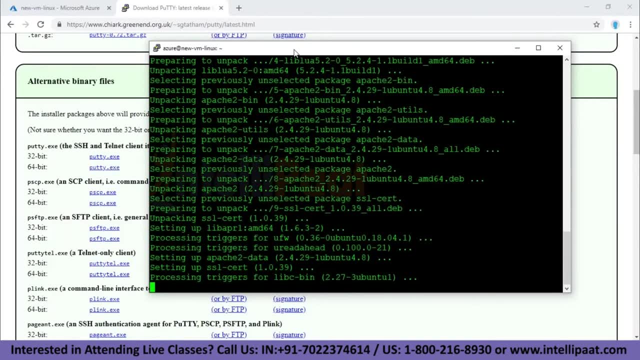 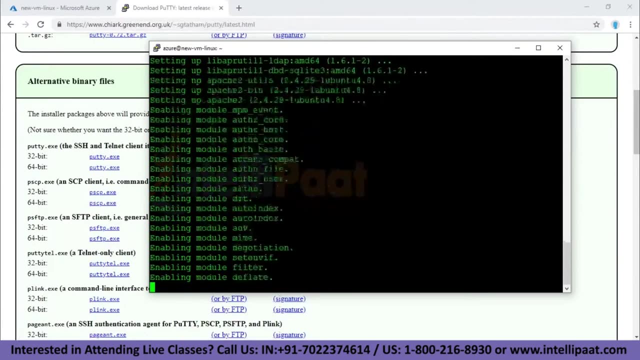 right now happening is it is being installed on my Ubuntu machine. Once it gets installed on my Ubuntu machine, all I have to do is I'll have to go to the IP address of my VM instance, And then I will be able to see a web page over there, Right? So it's almost complete, guys. So let's. 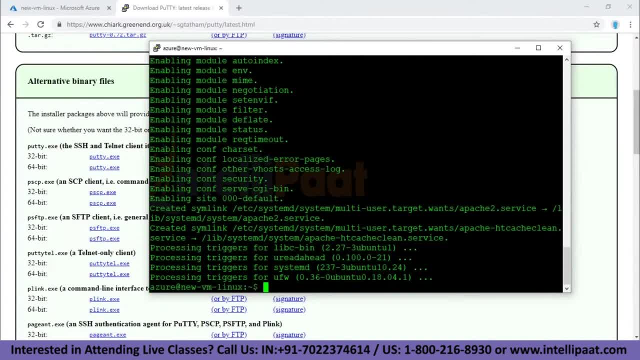 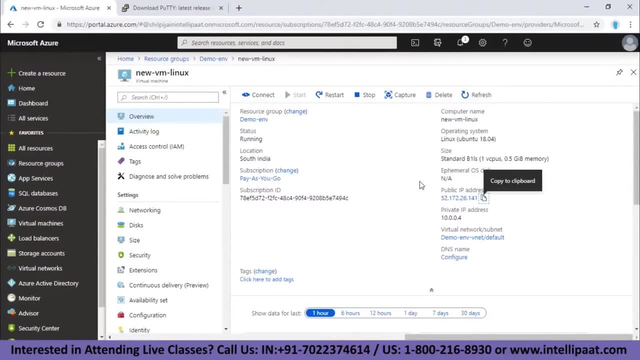 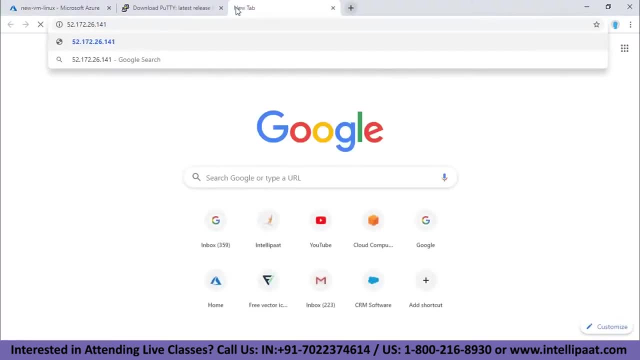 wait for this to complete and then we'll move forward. All right, So my Apache has now been successfully installed, And now, if I go back to my machine or my portal, my Azure portal, I'll just copy this IP address, And now let's paste it in a new tab and hit enter. Can you see? This is. 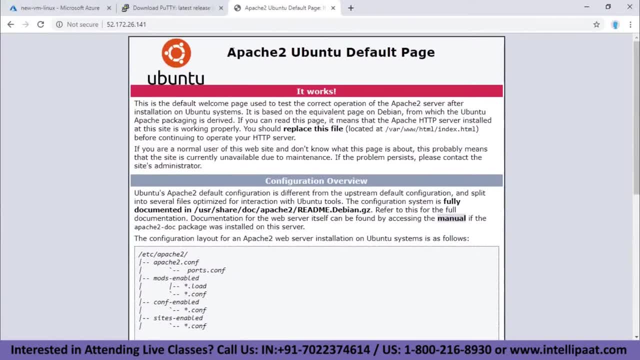 basically a website which has been created by Apache 2.. It's basically a default page which you have installed, Apache 2.. But nevertheless, guys, if you guys go to this IP address- given that I would not shut off this machine- you will be also able to see this particular page, which is: 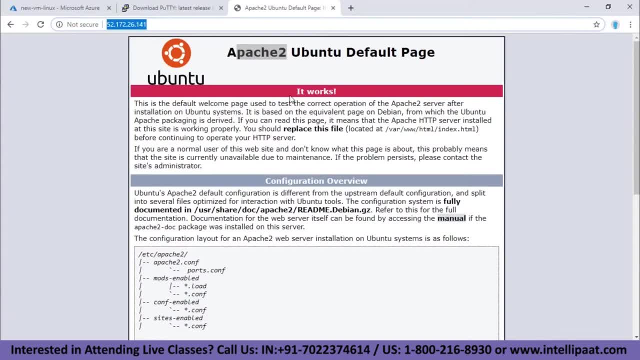 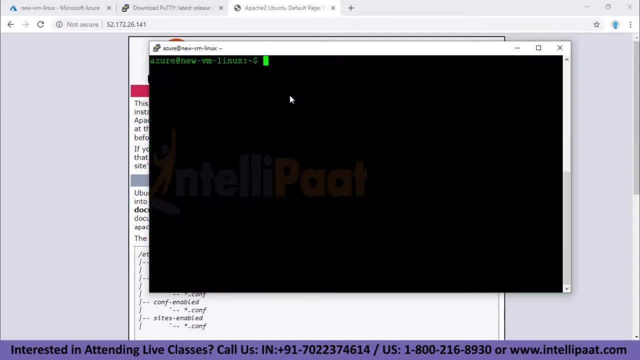 basically the Apache 2.1.2 default page. Now what I can do is I can also go ahead and edit this web page, Right? So let's go ahead and go to the location where this web page is basically stored. So it's stored inside. 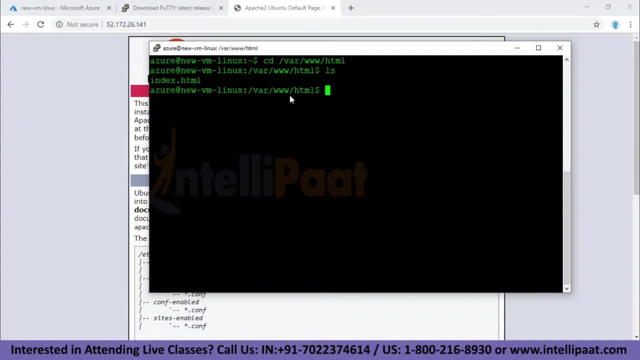 that wwwhtml, And this is the indexhtml file which is being shown over here. So what I'll do is I'll just change the name of this indexhtml file to, let's say, 1.html file, And I'll have to give sudo in order to do that. And now let's create one more indexhtml And let's say this: 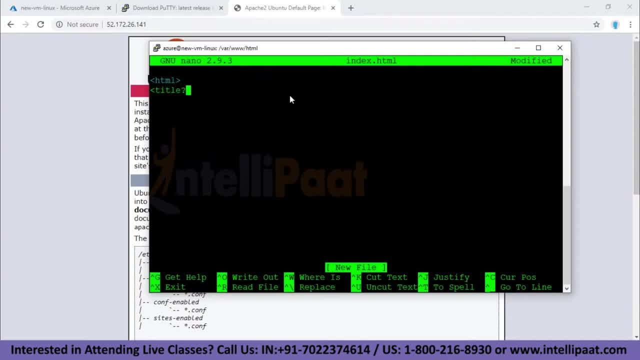 is an HTML page whose title would be demo website- Right, And the body of this would basically have a heading which would go like: welcome to Intellipaat's Azure. Okay, So this is what I specify. I close the headers and I close the body. 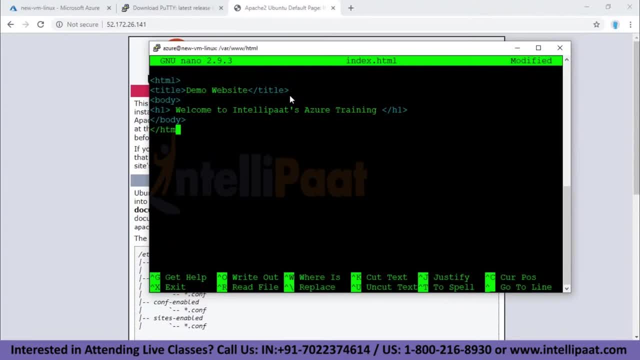 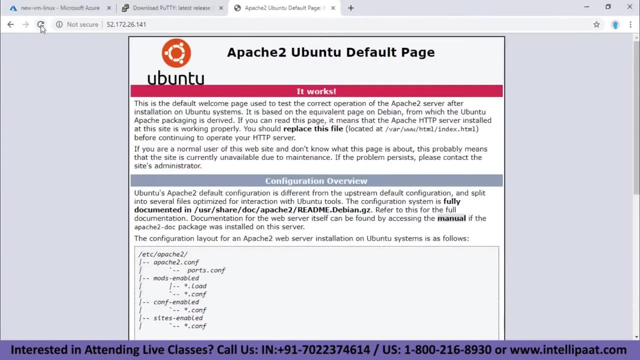 and I close the HTML as well. Okay, So I've closed the HTML, I've closed the body, I've given the edge one, I've given the title as demo website. let's save it. and if I do an LS now, I can see that there is an index dot HTML present. now, if I do a 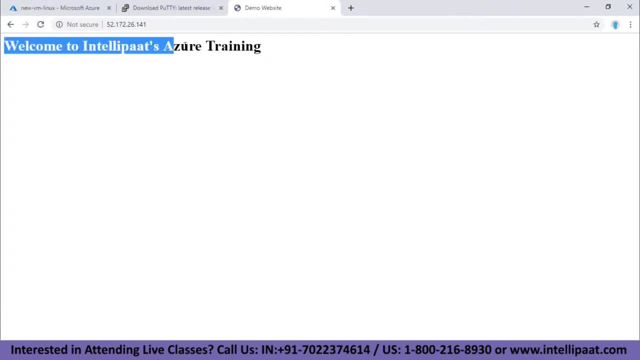 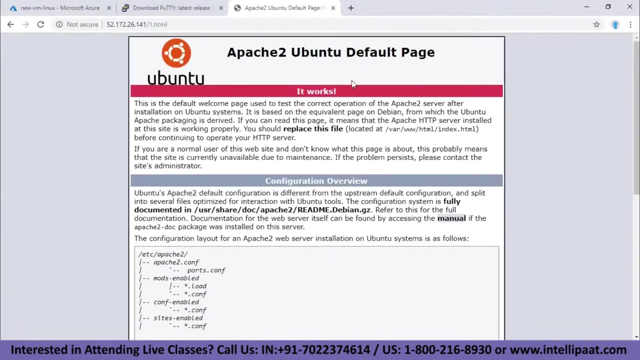 refresh. you can see I'm getting this. welcome to intellipaat is your training and the title of my page is demo website. right now, you would have also noticed I made the Apache page as one dot HTML. so if I go to one dot HTML, this is the. 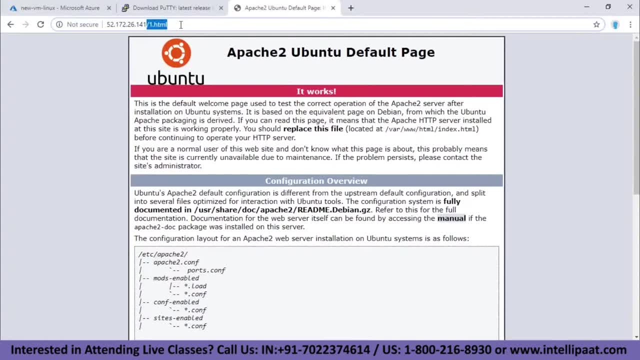 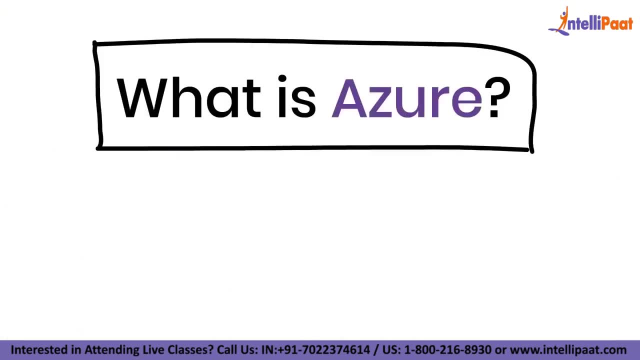 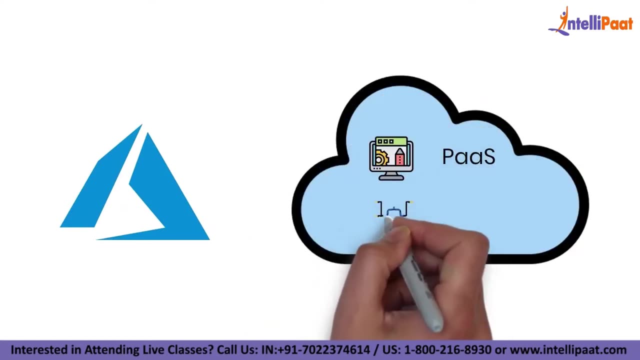 Ubuntu default page and if I simply go on the IP address, it will open the extra HTML, which is basically this: so what is Microsoft Azure? Microsoft Azure is a cloud provider that provides various platform as a service and infrastructure as a service. products as your. has cloud solutions to all the infrastructural. 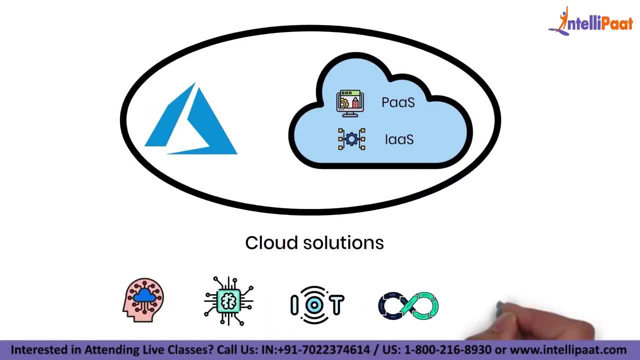 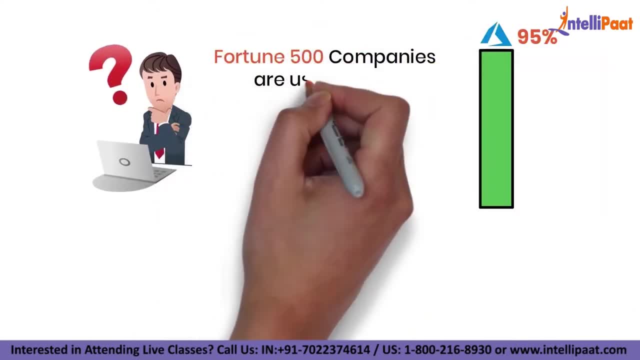 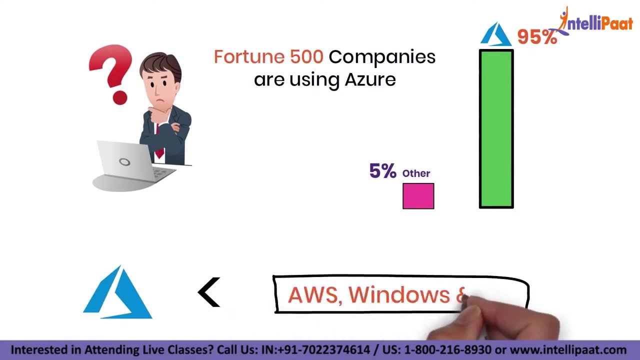 problems by providing services in various domains. did you know that almost ninety five percent of all the services in Microsoft Azure are based on Azure and, by the end of fortune, 500 companies are using as your? also, it is five times cheaper than AWS in terms of windows and SQL server, because there are also 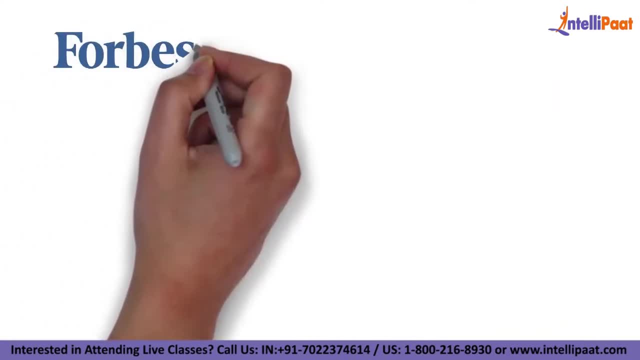 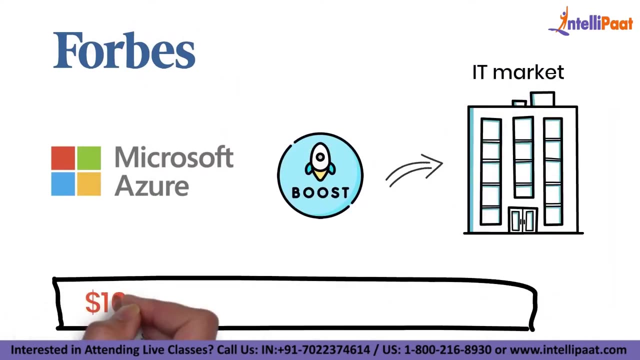 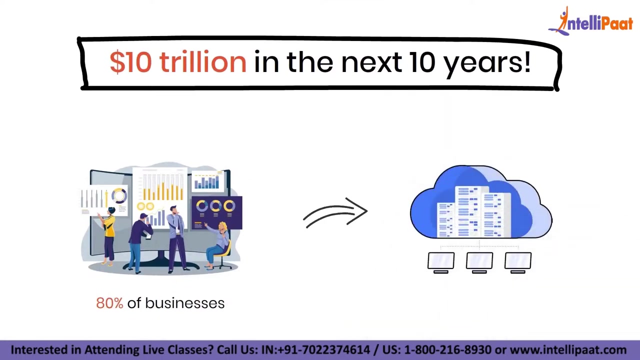 Microsoft products. Forbes say that Microsoft Azure is set to boost the size of the IT market by ten trillion dollars in the next ten years. as per predictions, eighty percent of the businesses will move their workload to cloud by 20% 2025, thus making it a major career to consider transitioning to. 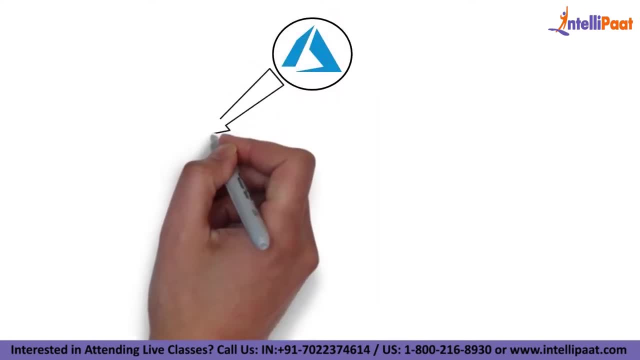 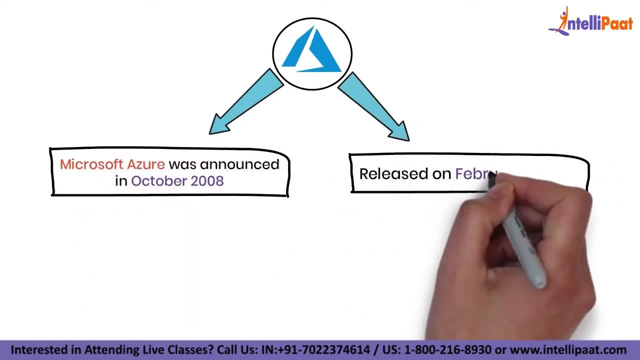 For a better understanding of Azure, let us start at the very beginning. Microsoft Azure was announced in October 2008 and released on February 1, 2010 as Windows Azure first, and later named as Microsoft Azure on 25th March 2015.. 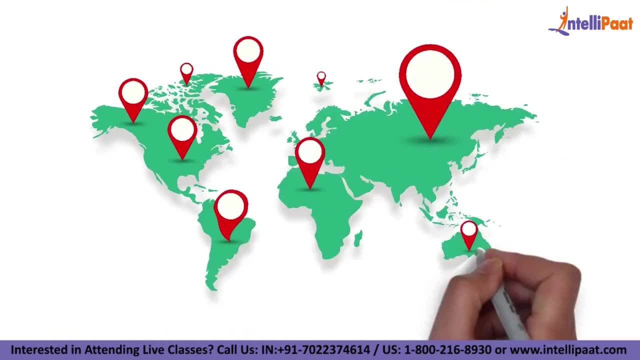 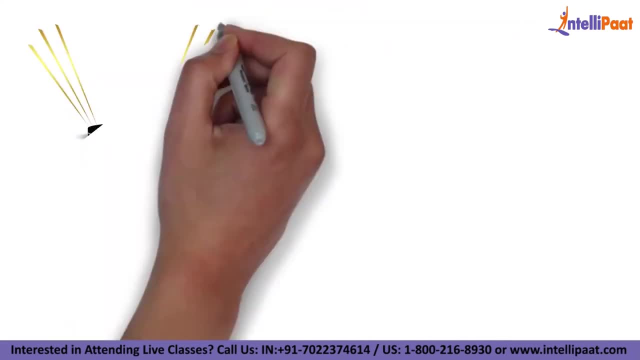 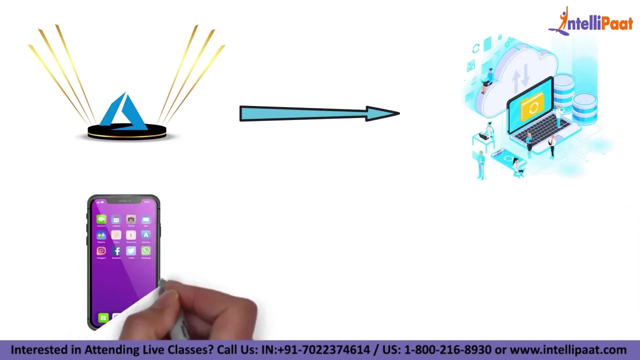 In today's scenario, its reach is in 140 countries and is still expanding, which is pretty impeccable. In simpler terms, Microsoft Azure is a platform that enables users to engage in agile cloud computing and is designed for creating and managing apps through Microsoft's data center. 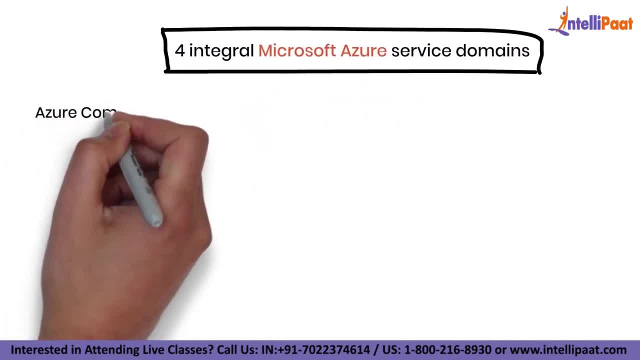 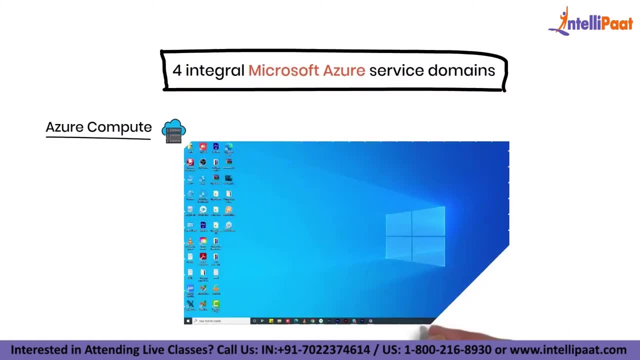 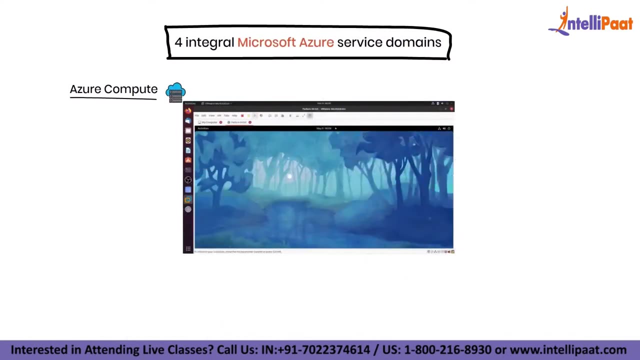 Now there are four integral Microsoft Azure service domains. The first one is Azure Compute. Compute is the most integral domain in Azure, as it brings everything together with Azure Virtual Machines. You can get on-demand scalable compute resources. Azure Virtual Machines, App Services and Container Instances are some popular compute services. 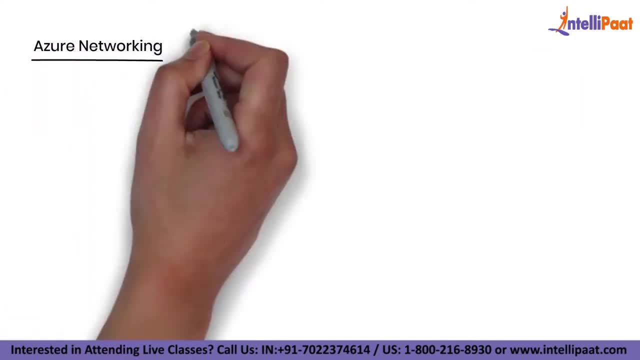 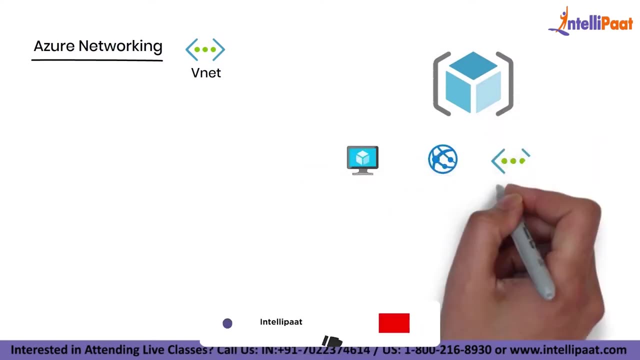 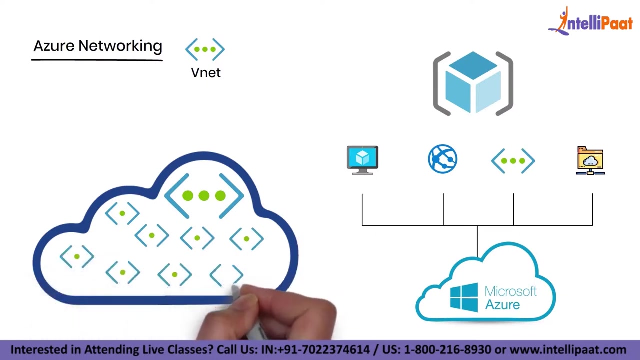 Second, we have Azure Networking Networks from the cloud networks. In Azure, VNet is the networking tool that connects all Azure resources together. These networking services allow enterprises to safely connect their on-premises services to the Azure cloud. It is also used to manage virtual private networks and further create multiple virtual 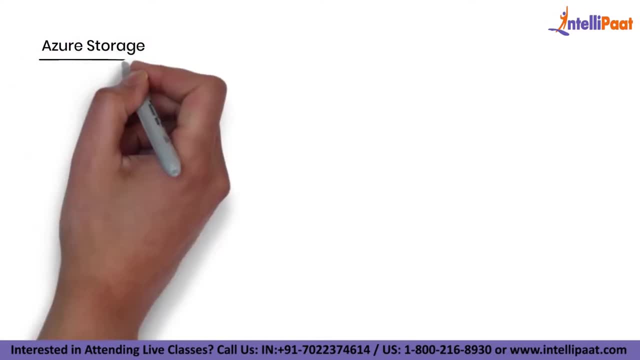 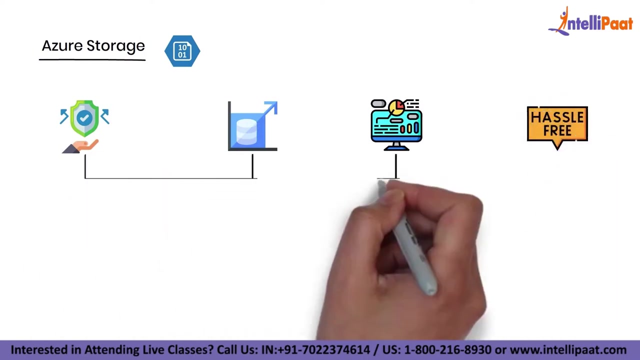 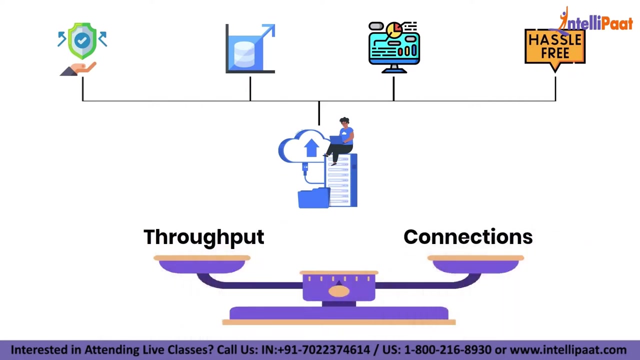 networks on the cloud. The third one is Azure Storage. Azure Storage provides storage solutions that are more durable and large-scale applications. data-driven applications can be built without any hassle. Azure automatically scales the storage requirements according to the usage and it automatically balances throughput according to the connections made. 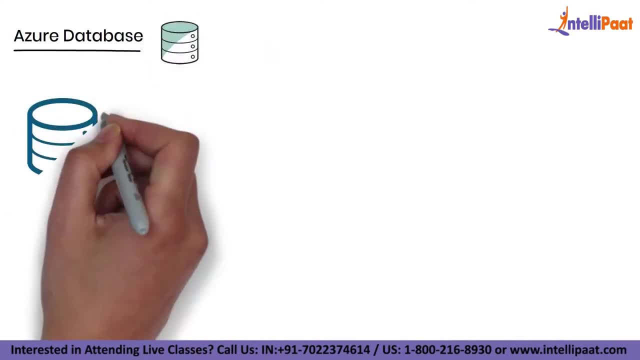 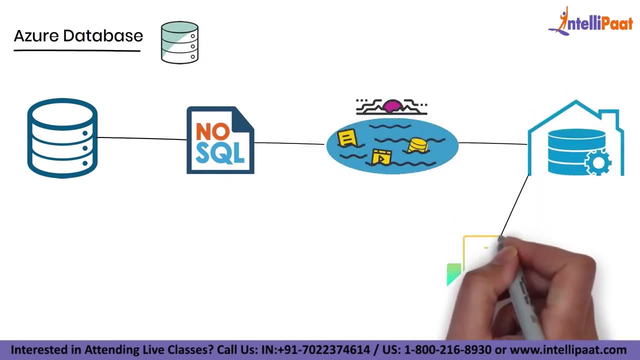 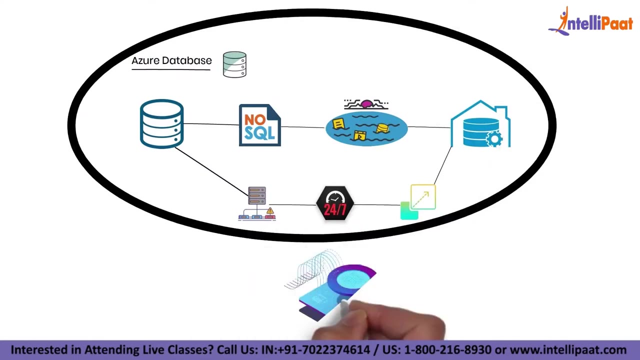 And the last one is Azure Database. Azure provides relational databases, NoSQL databases, data lakes and data warehouses. It provides a scalable, high-available and fault-tolerant database server and lets you scale according to the incoming data. There are various job roles in Azure. 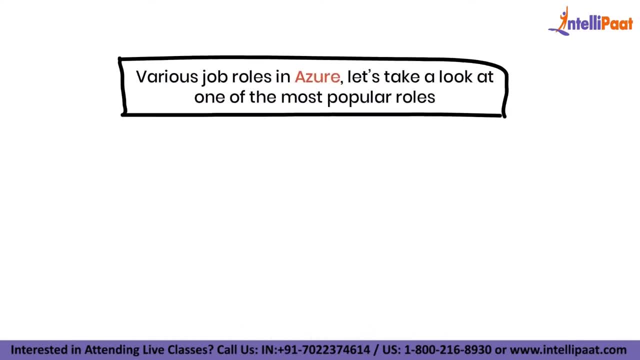 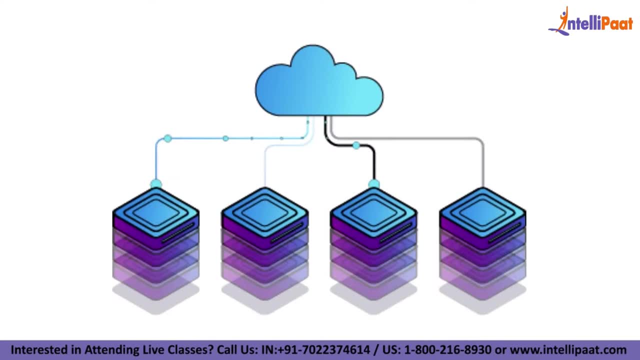 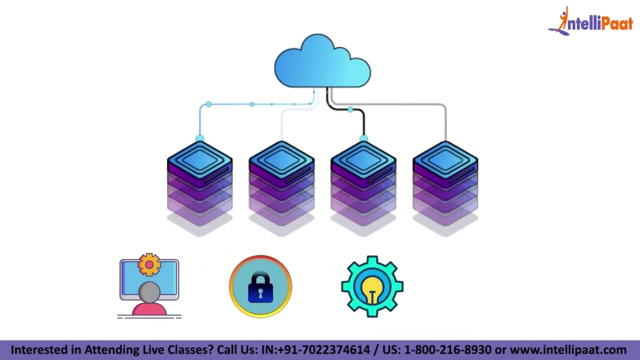 Let's take a look at one of the most popular job roles: Azure Developer. An Azure Developer is a cloud professional who creates cloud-based applications making use of the benefits of the cloud architecture. If you are proficient in testing, security, development and deployment, then a career. 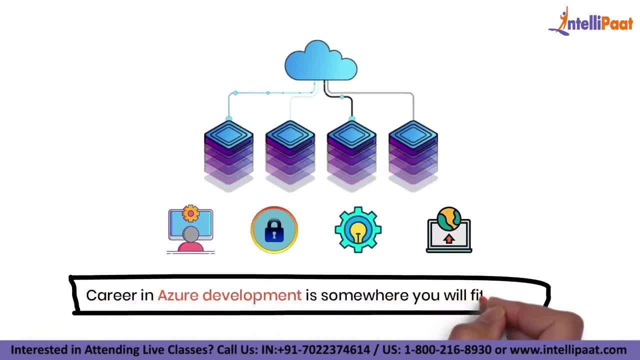 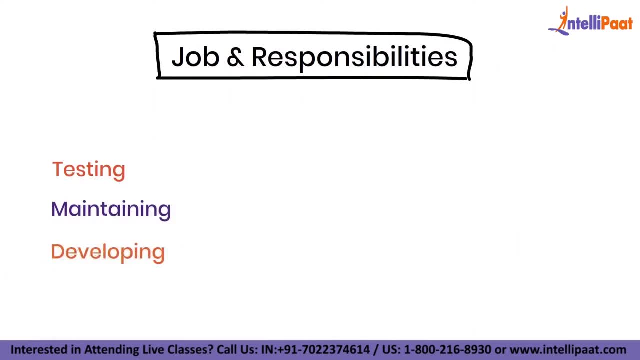 in Azure. Development is somewhere you will fit in well. The job includes responsibilities like testing, security and deployment. The job includes responsibilities like testing, security and deployment. The job also includes the existing of applications: maintaining, developing and deploying them. 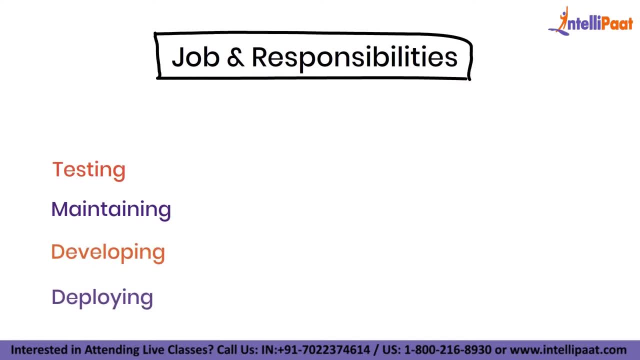 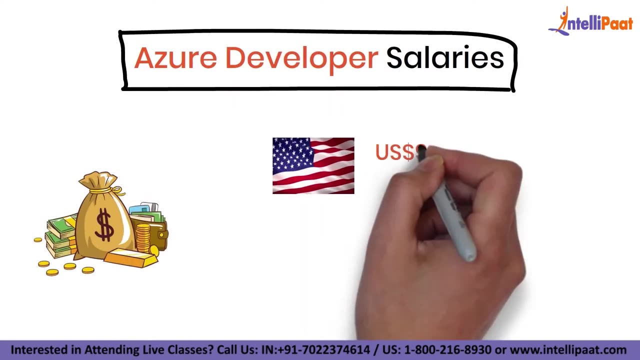 on Azure. It also includes participating in all phases of development and having the ability to work side-by-side with cloud administrators, clients and cloud architects In the United States, on average basis, an Azure Developer gets paid $132,148 per annum. 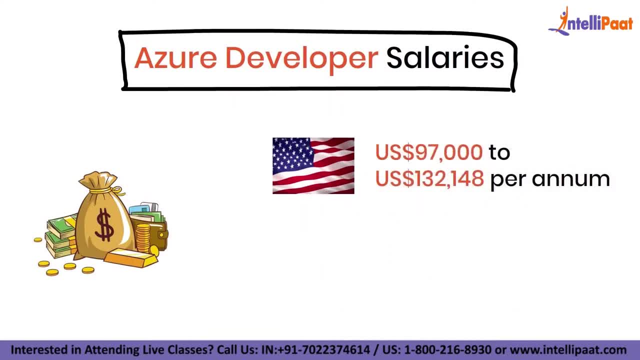 However, for an entry-level developer it's $97,000 and $ Dok함 annually. For the fossils, it costs $200,000.. $97,000, whereas in India the salary offered ranges from 7 lakhs to 25 lakhs per annum. 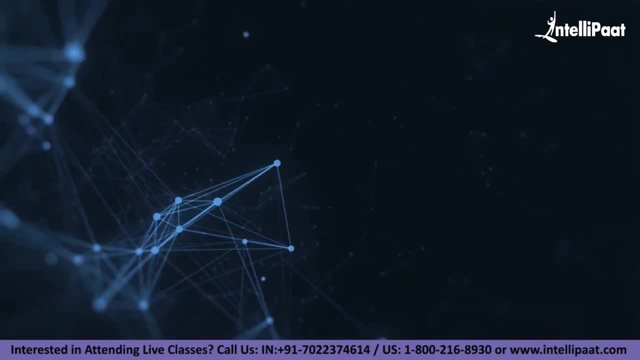 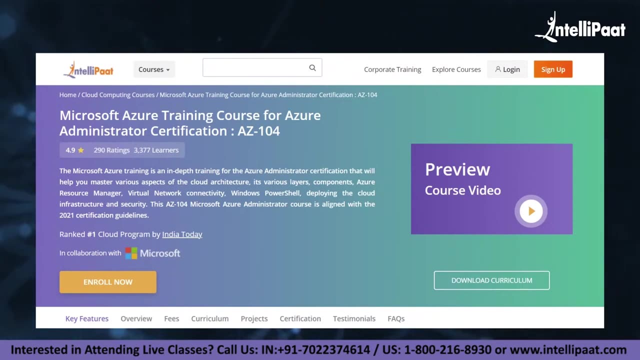 That's all about Azure. Just a quick info, guys. Intellipaat provides Microsoft Azure certification training in partnership with Microsoft, mentored by industry experts, The course link of which is given in the description below. Now let's continue with the session. 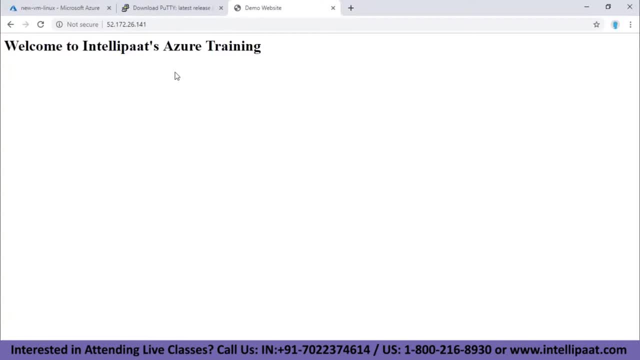 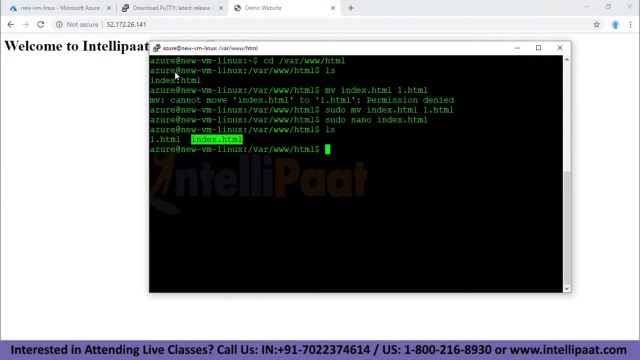 So, guys, we have successfully deployed our Linux VM on Azure and we have successfully hosted a website, also on this particular server. Now, guys, remember that this is infrastructure as a service. Now, what I've done is I had the access to the operating system. 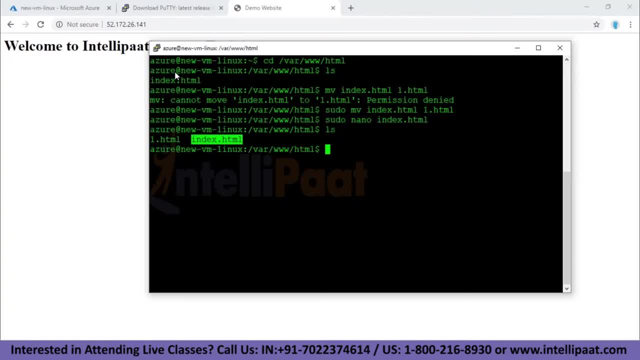 I basically installed Apache 2 and then I put a website over there in that particular folder which is var- wwwhtml, and then I got the website Right. So this is infrastructure as a service. You're getting the whole operating system and you can do anything with it. 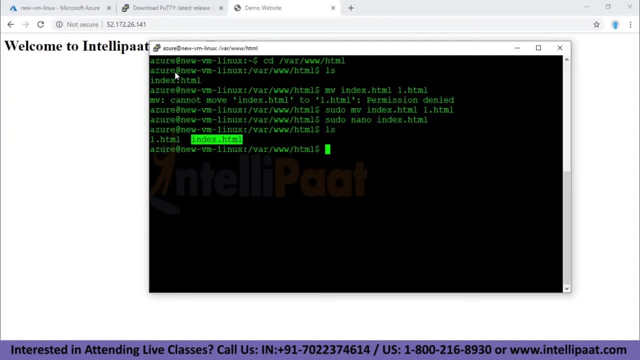 I can also install MySQL on it and I can configure my website to basically talk to the MySQL server. Right, I can do anything with this server. Now, when you compare it with app services, which we saw earlier, that app services are basically platform as a service or function as a service. 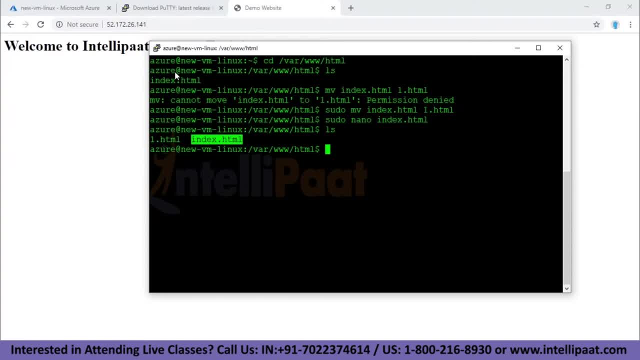 Functions app is also a platform as a service. Now, how is it different From the hands on point of view? you would basically not be using Putty. You will basically just deploy that app, that is the web app, and you will get a URL instead. 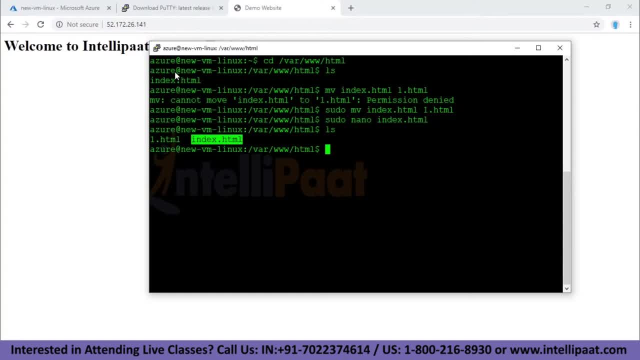 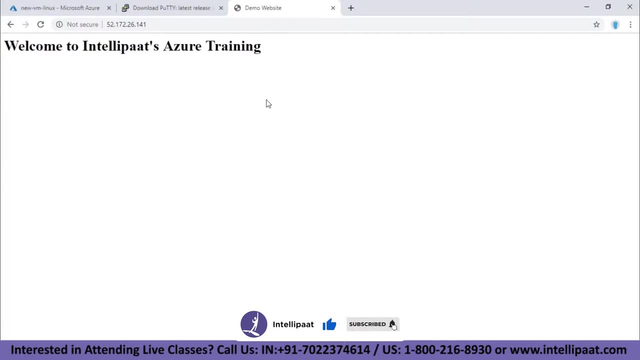 of an IP address, You will get a URL and if you go to that URL you will see a default page. So let's say you saw a default page when you installed Apache 2.. You will see a default page from Azure when you go to that link that this is a default. 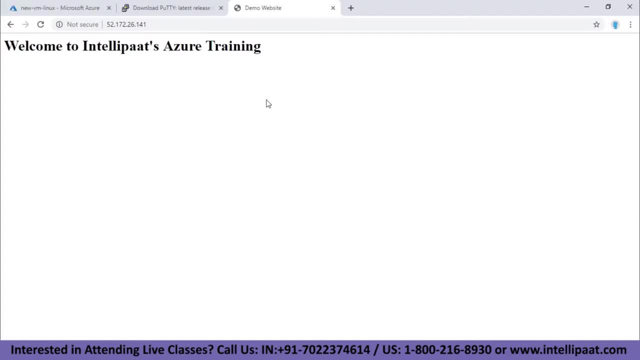 page for the web app that you have deployed Right, And if you find the dashboard, you will see a button called upload Right. So what you can do is like: I created this indexhtml file, you can also create yours, and you will just have to upload it. 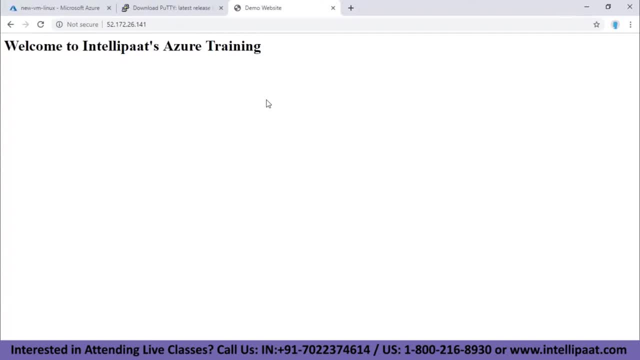 Now Azure will take care where that file has to go inside the file system, Right, And it will take care that on the link when you go now you will see your website. It will take care what software it has to install, whether it wants to install Apache. 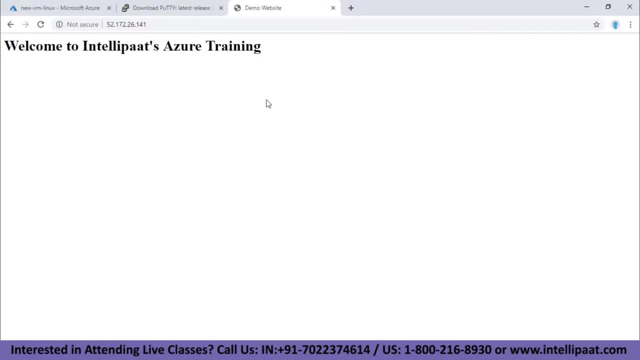 2, which is basically the web server, or there are several other web servers as well. You have Nginx, You have Tomcat, So anything that you want, Anything that you want or anything which is configured in Azure, would be automatically installed, and all you will get is a button which will ask you to upload the website. 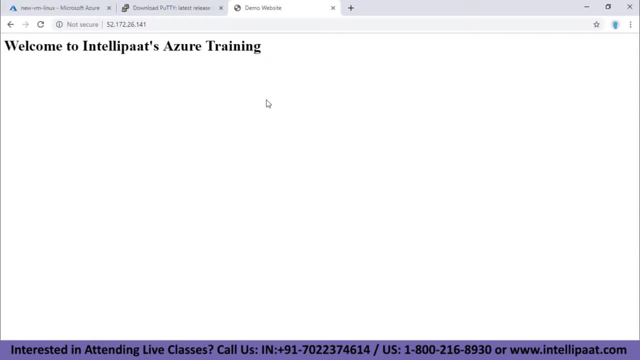 So you would not get direct access to the operating system and hence it is called platform as a service. Similarly with functions app in app services. basically, you can deploy applications in function app. You cannot deploy an application. It is simply a place where you just put your code and that code will be done. 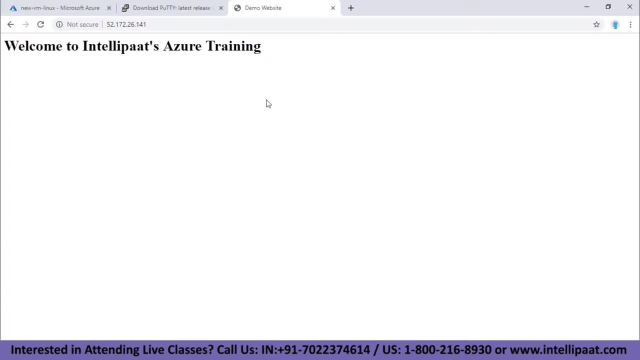 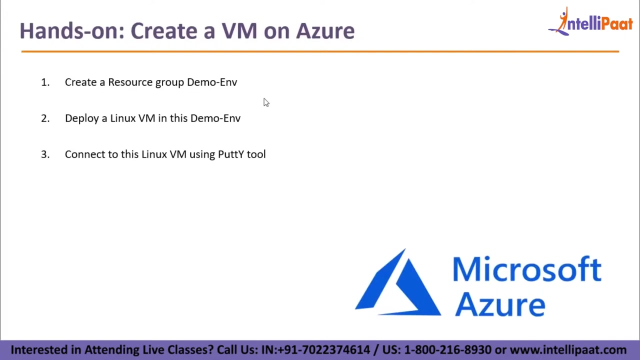 Right, So if, in short, I will have to tell you what functions app is, it basically does processing. Okay, guys, So guys. this was our demo. This was our first demo as to how the you can launch virtual machines on Azure. Now let's go ahead to our next topic. 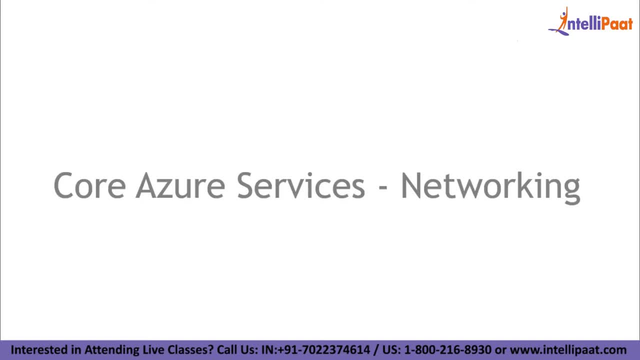 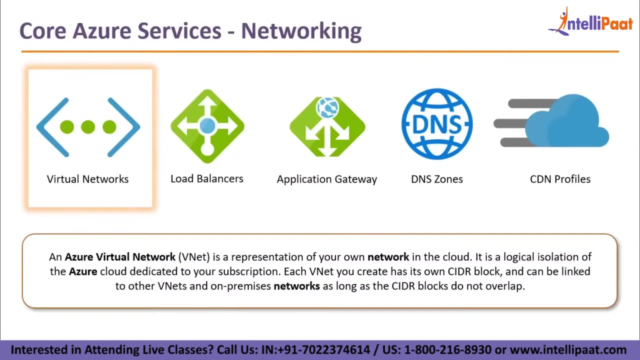 Alright, guys. so next in our list are the networking services of Azure, So let's go ahead and start with them. So, guys, basically there are five core services in networking that you should know of, The first one being the very important one, Which is virtual networks. 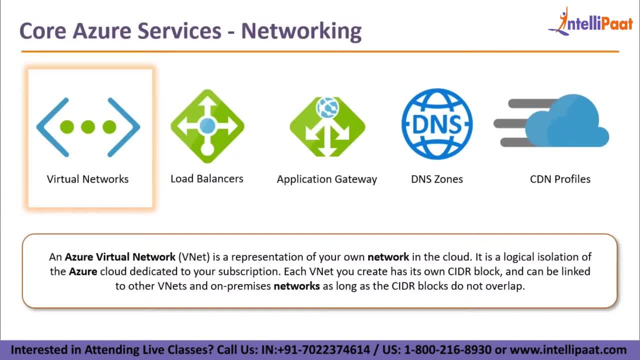 Now, what are virtual networks? Virtual networks are basically isolated environments or isolated networks on the Azure infrastructure for whatever machines or whatever VMs that you launch in Azure and if you want them to talk to each other. For example, I deployed an application where probably I would have a database I would 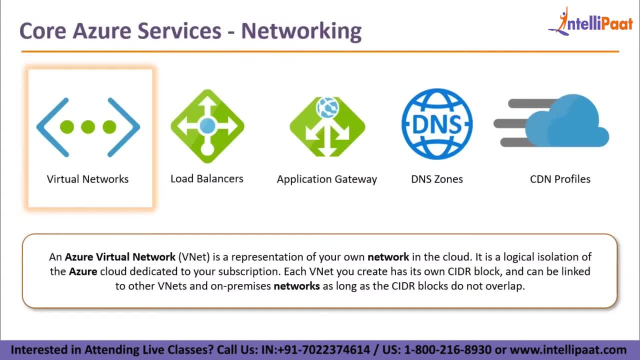 have a backend server, I would have a frontend server. Now all these servers have to interact with each other so that the whole application can basically function. Now, How do they interact with each other? They can interact with each other only when they are on one network. 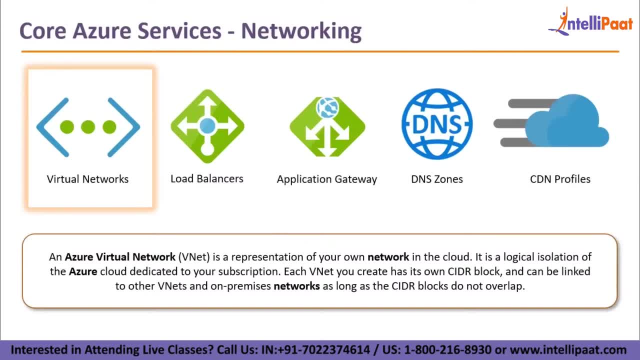 Right, So that is very important. Otherwise, they will have to interact with each other over the internet, but that is not a secure thing to do, Right. A secure thing to do is when instances or when servers interact on their own private network, which is basically not accessible to the outside world. 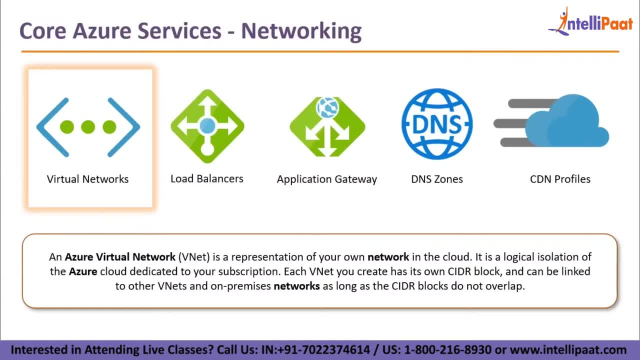 It is only accessible to the administrator who has possibly launched those instances. So in those cases We need virtual networks. and also one more thing: that when you are using virtual networks or if you are using private networks in Azure, You basically get a bandwidth of around 1 GB per second. 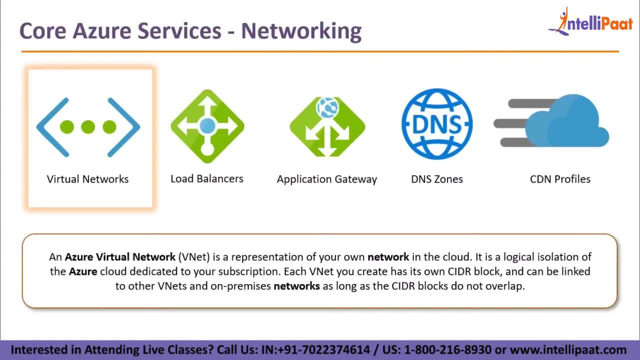 Right. That is the kind of bandwidth that you get when you are dealing with instances which are in the same network, that is, in the same virtual network. But if instances have to interact over the internet, obviously the bandwidth will go down and at the same time it is not secure. 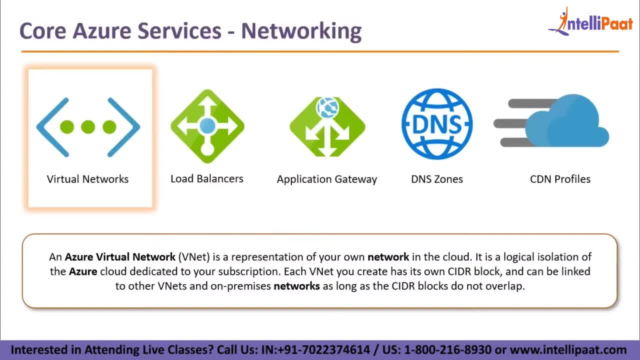 Right. So If you want to launch any resource in Azure which basically can be launched inside a network, They are launched inside a virtual network And you do not have the option of launching an instance or a server without a virtual network. You have to launch it inside a virtual network. now that if you don't want to use it and want 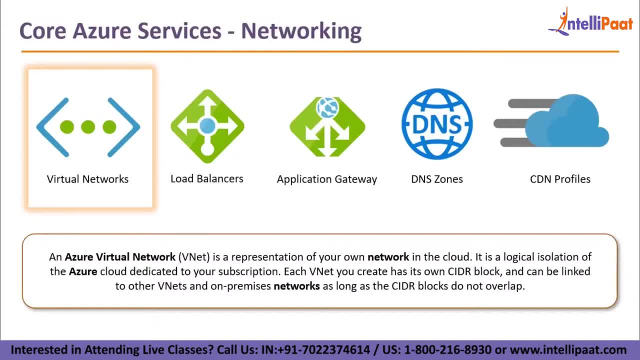 to have instances, talk over the internet, that is your choice, But Azure does not give you an option of deploying an instance without it being a part of a virtual network. Right? So, guys, this is a virtual network Moving forward. now let's talk about load balancers. 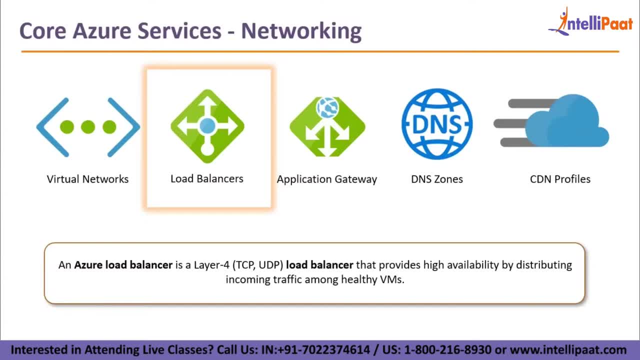 Now, what are load balancers? Now, this is a very important service, Reason being when you deploy your application on cloud. one of the most popular reasons of deploying applications on Azure is because you can get high availability, which basically means you can launch your application on multiple servers so that, even if one server fails, the 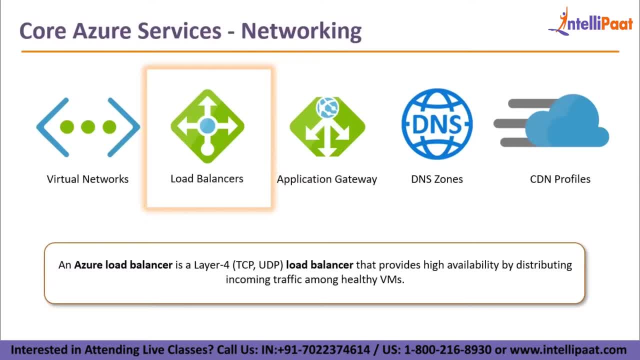 other server can basically be their replica And they can serve the application right. So this results in a high availability of your application. Now, what is a load balancer? A load balancer basically sits in front of multiple virtual machines which have the same. 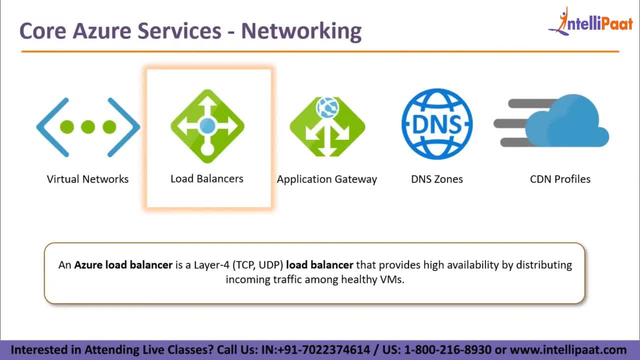 application running on them. right, And it sits in front of it. Now, obviously, if you are a customer, you do not realize whether an application has been made redundant on multiple servers, right? If you go to facebookcom or if you go to intellibarcom, you wouldn't realize how many. 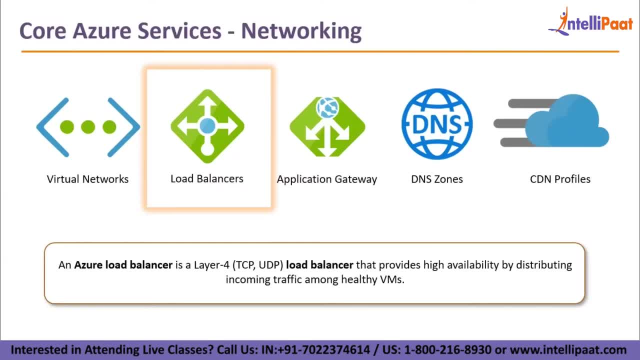 servers are actually working. So how is it possible? right, You have to know, basically, servers. they have IP addresses, right? So you, as a customer, should know which IP address you should ping. But all you do is you go to a particular domain, let's say intellibarcom, and you get the website. 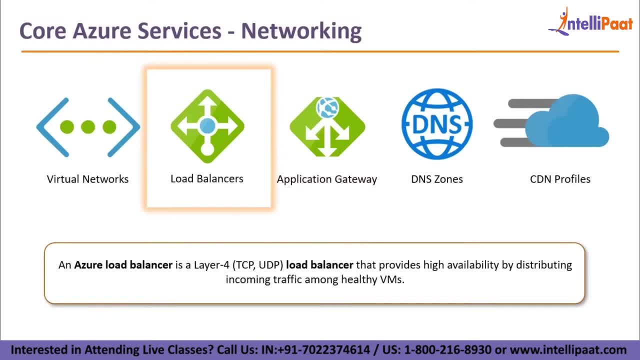 So how is it actually working? So, basically, the way it works is that load balancer has its own IP address or domain name, And what the load balancer does is it basically randomly spreads the required IP address to the end number of servers it has. 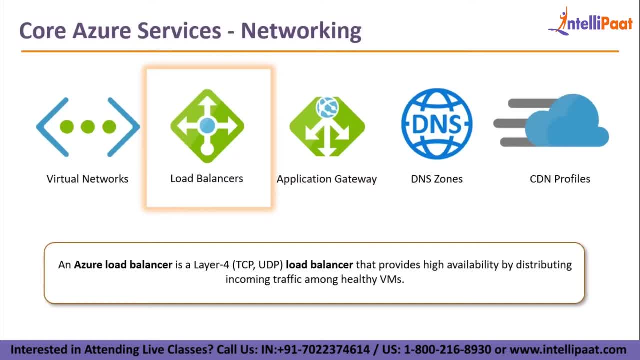 Let's say, my intellibar website resides on five servers, wherein one is the primary server and four are the redundant servers, But all these five servers are basically serving my website. Now, when a customer comes onto intellibarcom, his request is processed in this fashion that: 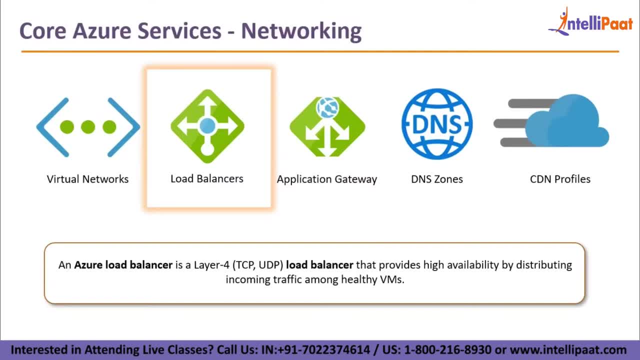 whenever he comes to intellibarcom. basically he is routed to the load balancer's domain name or IP address And once a request reaches the load balancer, the load balancer sees which server basically has less load right And the server which has less load it sends the request to it right. 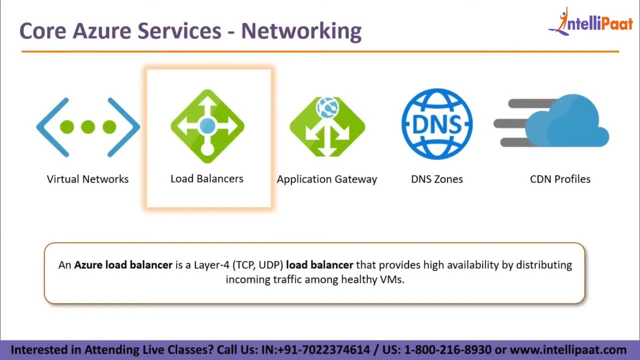 Now, load balancer is also an important concept. You must have heard about auto scaling, right? or, if we talk it in terms of Azure, it's basically called VM scale sets. So what happens in that particular scenario is we specify a threshold limit. We specify that whenever the CPU usage goes beyond 80 percent of the aggregate number. 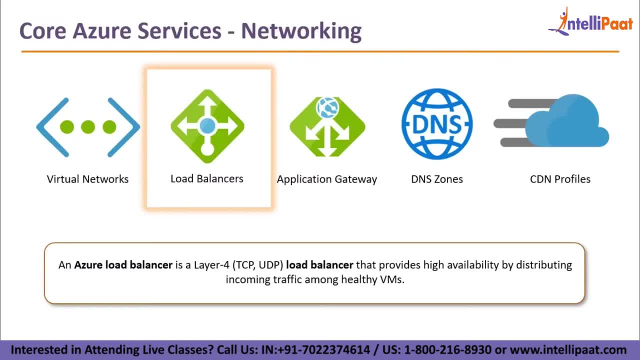 of servers. Let's say there are four servers and the average CPU load on all these four servers has gone beyond 80 percent, right? So what happens in that case? it will basically launch a new instance. Now, when it launches a new server with the same application, your load balancer should. 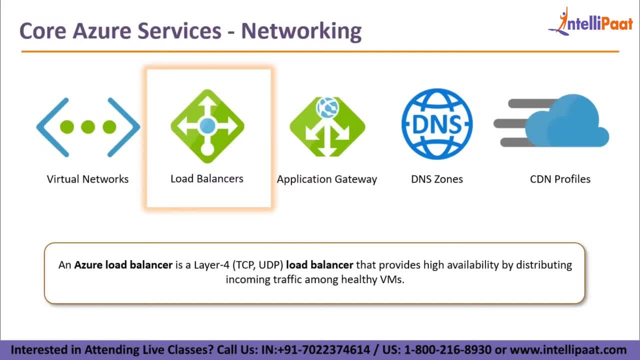 also route traffic to it, And that is when load balancer plays a key role. It plays a key role When you're doing auto scaling and, at the same time, it plays a key role when you have multiple servers which are basically serving the same application and you want to equally. 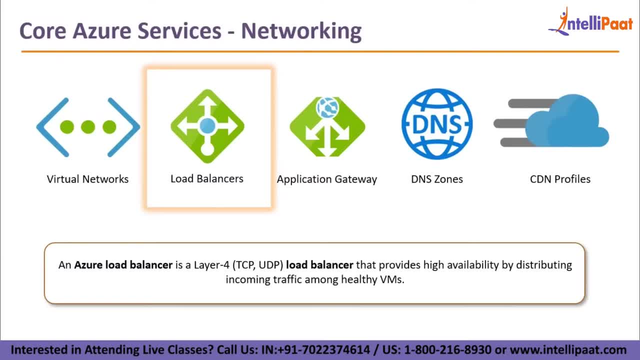 divide the traffic coming onto your servers, or basically coming onto your load balancer on your servers, Right? So this is what a load balancer is, as the name suggests. Right, But the load balancer in its most basic sense? it basically does it randomly, right? 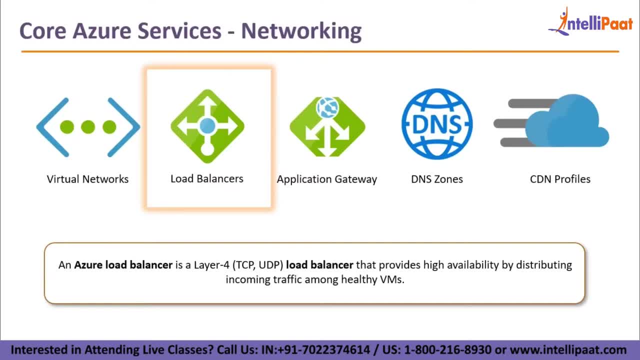 It randomly equally distributes the traffic among all the servers, Right. So it doesn't follow any protocol or rule as in how it has to basically divide the traffic, Right. So this kind of process or this kind of procedure, when it is followed, it is basically called. 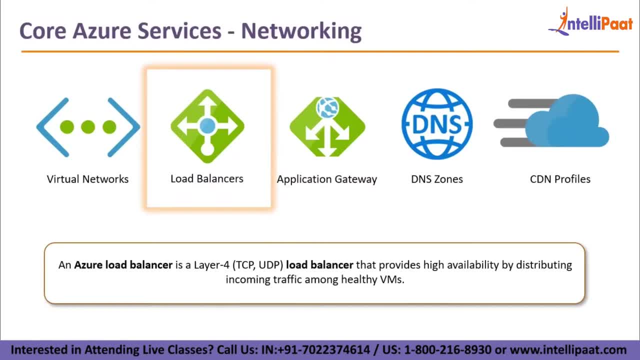 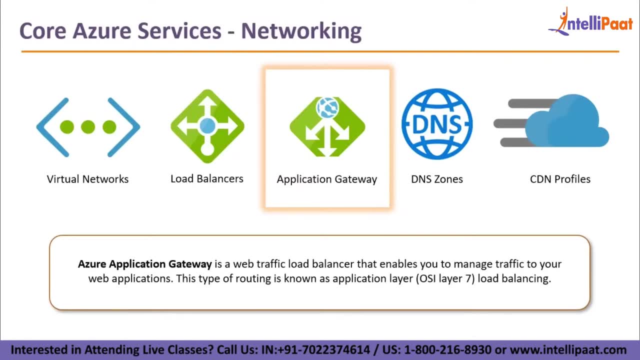 a round robin fashion of distributing traffic Right. The next kind of load balancer is the application gateway load balancer. Now, what is application gateway load balancer? The application gateway load balancer basically works a little different from the normal load balancer that we discussed earlier. 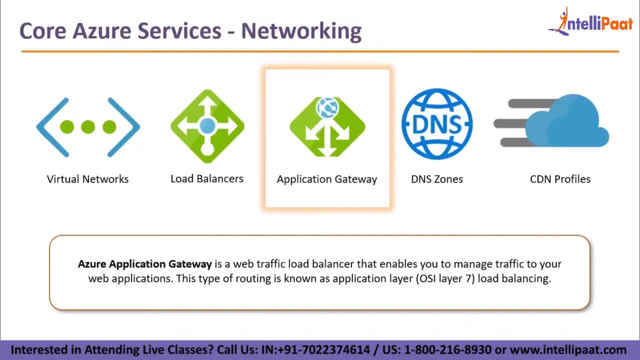 So in the application gateway load balancer, Basically the load is distributed based on rules. Now, what are those rules? Those rules are basically paths. Now, for example, if I go to Intellipaatcom, slash blog, right, What will happen? I get to see the blogging Web site. and if I go to Intellipaatcom, slash all courses. 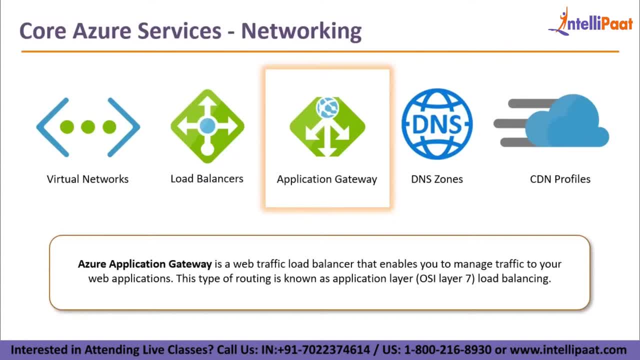 I basically see all the courses which are there on the Web site. Now, how does that work? Now you, if you, if you are from an IT background, You understand how servers work. You might say that there must be two folders inside the root document of the web, of the 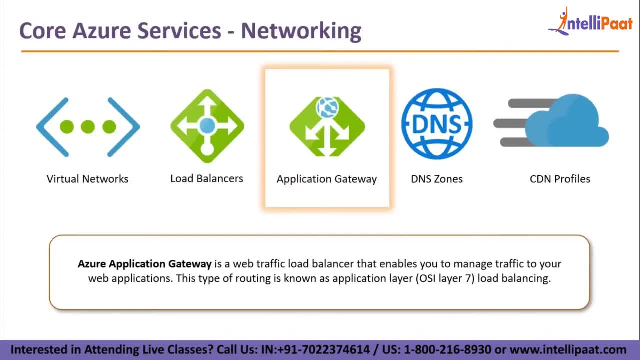 server where in inside the all course folder, you have the code for displaying all the courses and inside the blog folder, you have the code for showing all the blogs. But that is not actually how it works, Right? So, basically, if you, if I, were to talk about our infrastructure, the Intellipaat infrastructure, 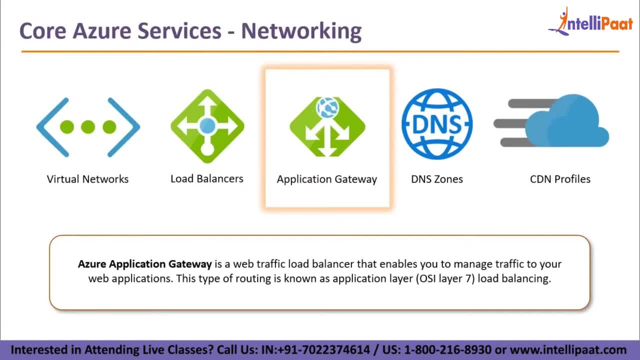 we have a separate server for blogs And we have a separate server for all the courses that we have. right Now, the load balancer that we use is an application gateway load balancer, It's kind of like that. So basically, what happens is whenever it sees that in the URL there is a path which says: 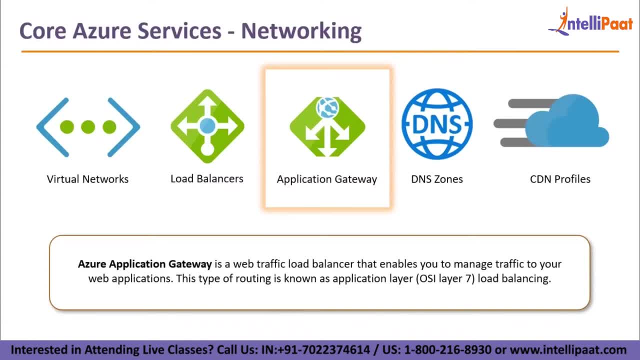 slash blog. it basically routes the traffic onto the blogging server and whenever it sees that the path is slash- all courses- it routes the traffic to my courses server. So this is how it works. This is called path based routing and basically it works on the layer seven. 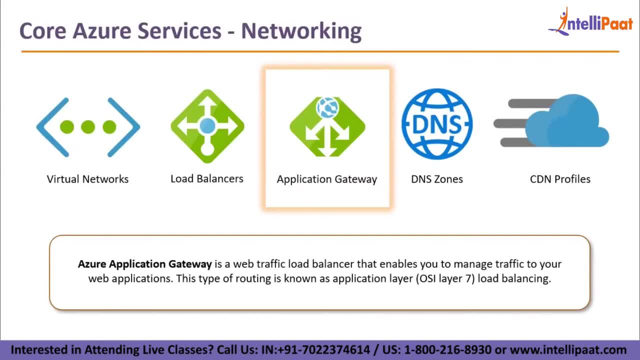 So if you guys are aware of the OSI model, right? So according to the OSI model, the application gateway load balancer works on layer seven Right Now. if you are not from CS background and if you didn't understand what what I just said, it is OK. 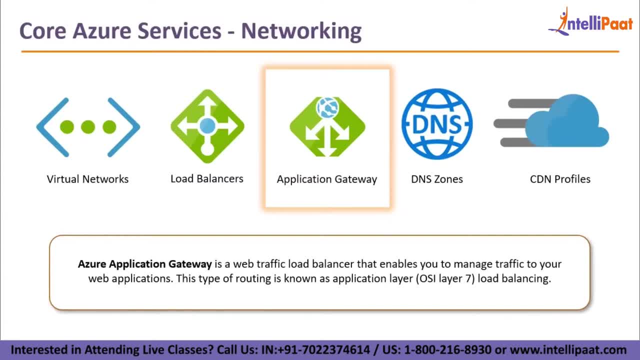 So, in the most basic sense, what the application, the layer seven, that it works on, in the most basic, basic sense, What that means is that application gateway load balancer does path based routing right. Whatever path is there in the request. based on that path, it basically routes the request. 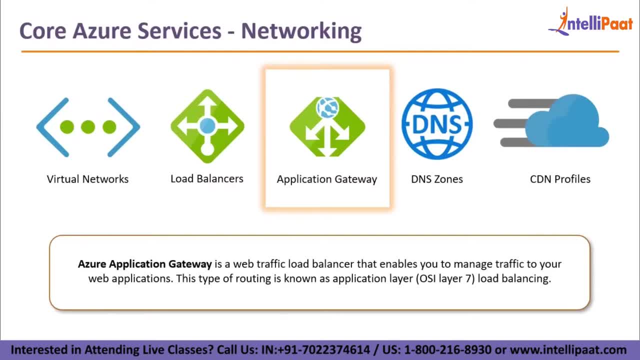 to a particular server. You can also define a default rule in case anything which is there except slash blog and slash all courses. if there is a default server that you want to send your request to, that is also possible. Like, for example, you would have seen that some websites 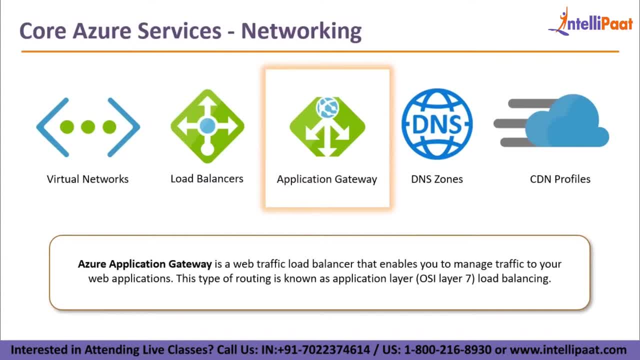 If the link is not found on that website, they basically route to a 404 page. right Now, how? how does a typical 404 page look like, right? If you look a 404 page, it basically says error 404 content not found right. But some websites like if you, if you would have visit flipkartcom or amazoncom, or even 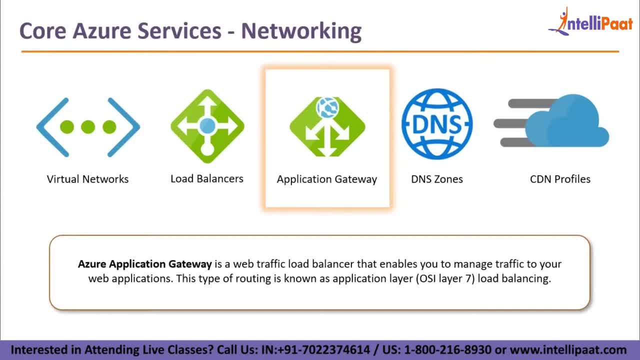 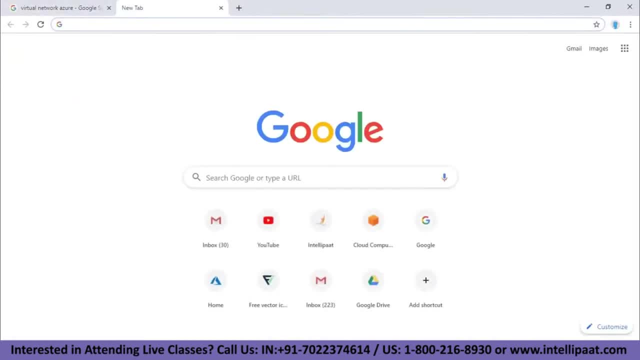 intellipartcom. in that case, if you try to search for something which is not there on the blog, for example, let me just switch to my browser right And let us go to, Let's say, intellipartcom and let's say slash azure, right. 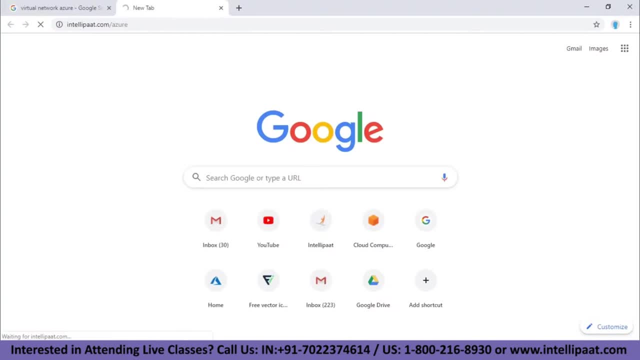 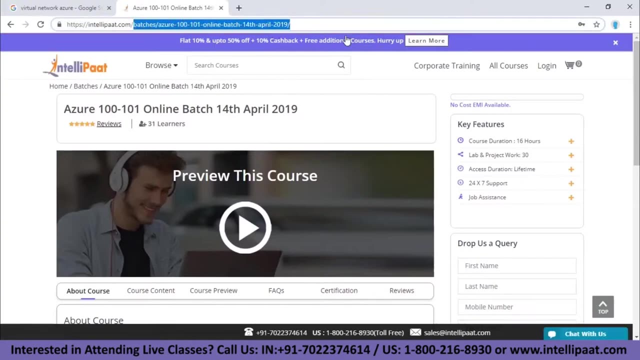 Now what will happen? It will basically give me a 404 page, and let's see how that looks like. OK, so there is a slash azure thing. Let me do one thing. Let me type in some gibberish content and let me just search for that. 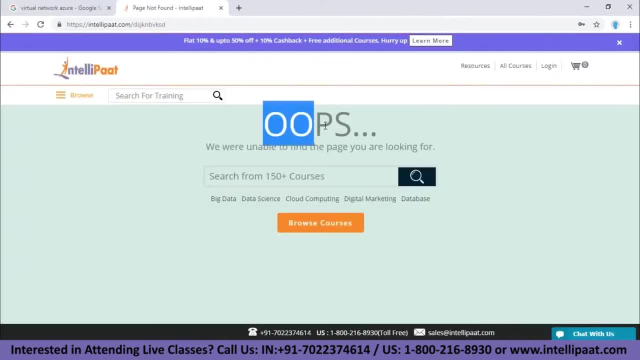 So this should give me a 404 right. So you can see I've got an oops page which says we were unable to find the page you are looking for. So if I go to content also over here, let's say we enter some random text again, I will. 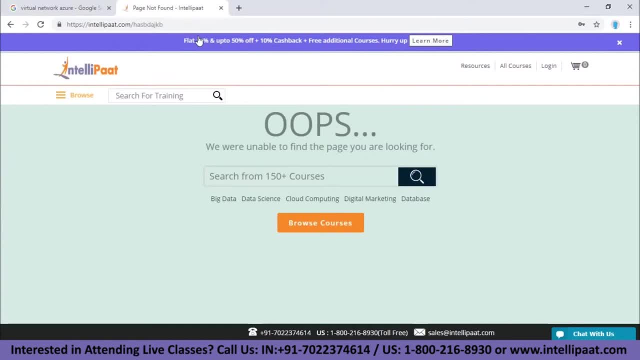 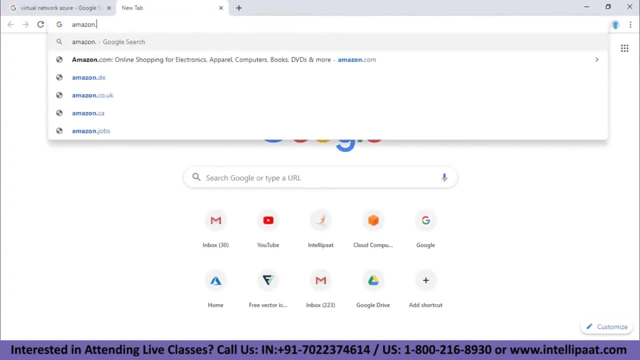 again see this page. can you see? it says page not found. And this is similarly the way it happens for other websites as well. For example, if I go to amazonin and I again search for something gibberish, Let's see what happens. 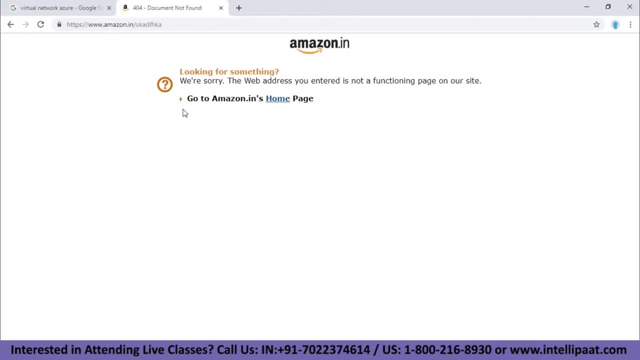 It says 404- document not found. and this is basically a custom page, right? And if I again go to anything other, Any other gibberish URL, I again get this page. Now, how is that working? So that is working because they also are using an application load balancer, which basically 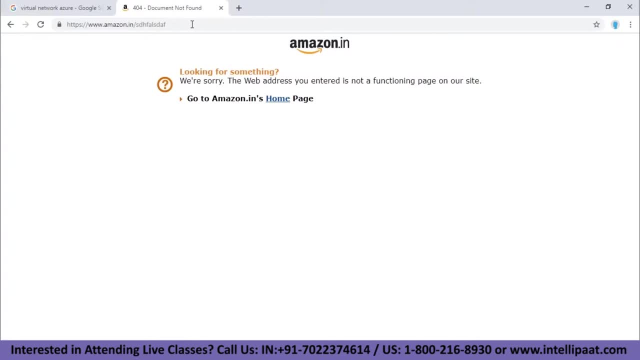 says anything other than the rules that we have specified. if someone goes or tries to go to a particular URL like the one that we have specified, route them to the 404 page, which is this right, And that's how the application load balancer is bringing you to this particular 404 page. 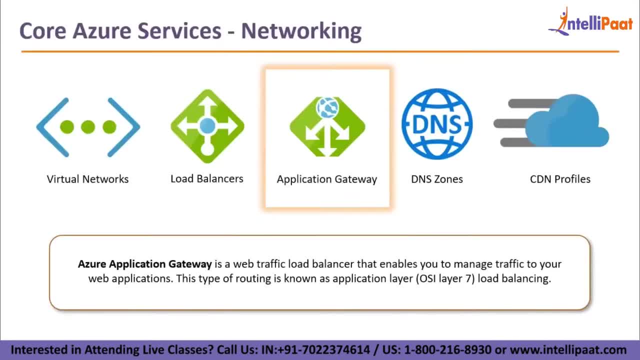 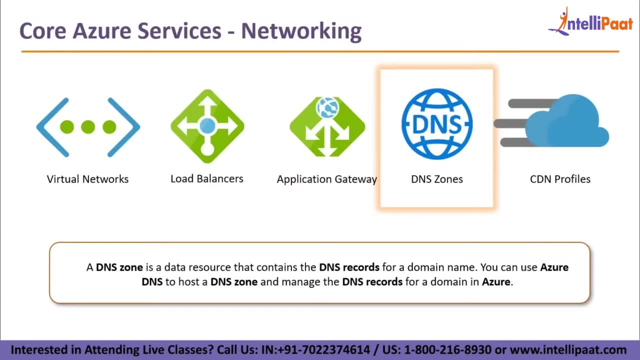 right? So, guys, this is the application gateway. The next service that we have in networking is called the DNS zones. Now, what is the DNS zone? Now, any website that you go to, guys, you do not enter the IP address for that website, right? 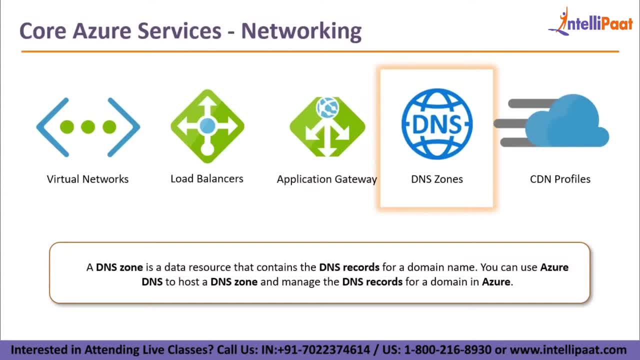 You basically enter a domain name and that domain name basically gets you to the website. right, You never enter the IP address. So similar is the case with DNS zones as well. So what DNS zones helps you in is basically it helps you to Route your domain to the Azure resource where your application basically resides. 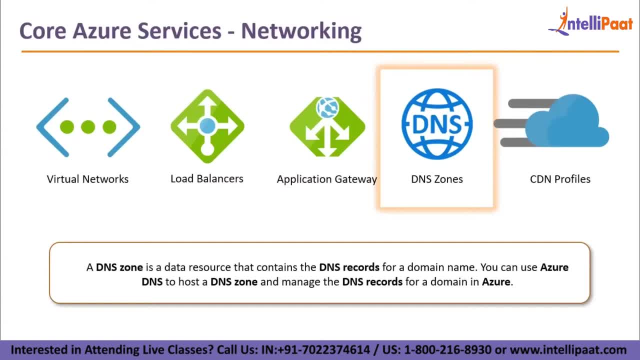 For example, you go to any domain website and you buy a domain. Let's say you buy a domain which is a personal website- dot, X, Y, Z. Let's say, you buy this domain. Now you want to route what, whoever is going to this domain. you want to route the traffic. 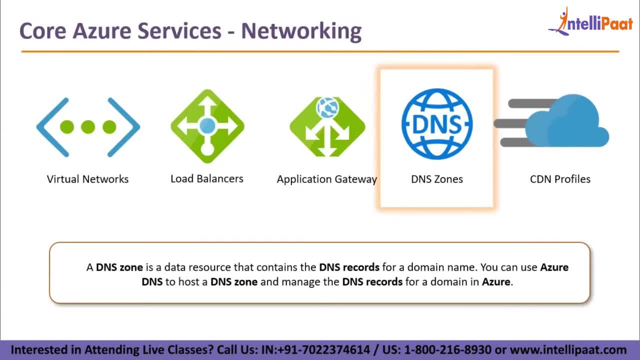 to one of the virtual machines that you have launched in your portal. Now how would you do that? For doing that, you will have to go inside the DNS zones service of Azure and you basically will get some name servers right. Those name servers are basically DNS servers that Azure owns, and those DNS servers you 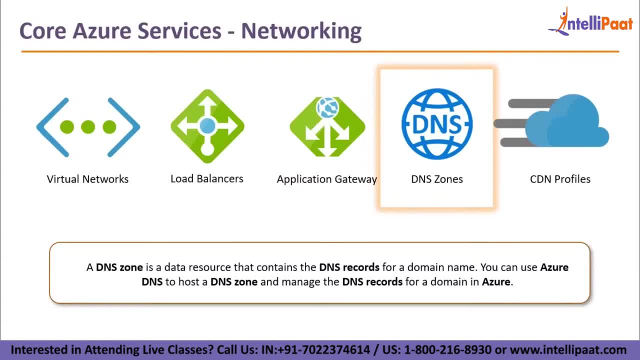 would have to specify in your domain So where you bought your domain. you would basically get a dashboard where then you can put the DNS servers which the domain that you have bought Will ping on right. For example, whoever would be going to personal website, dot X, Y, Z would basically be routed. 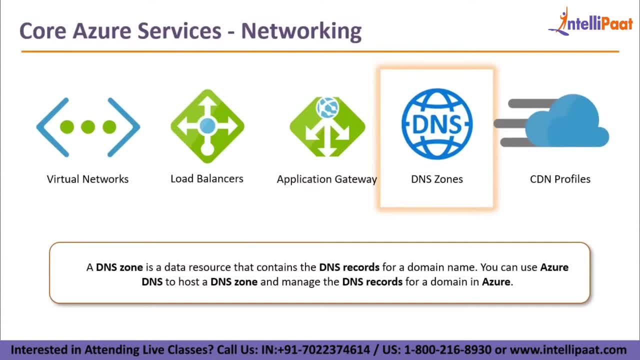 to those DNS servers that you will be mentioning over there, right, And those DNS servers you get from DNS zones. The next thing that you do is you specify in the DNS zones that whatever traffic is coming from the domain that basically I've specified, route them to this particular VM. 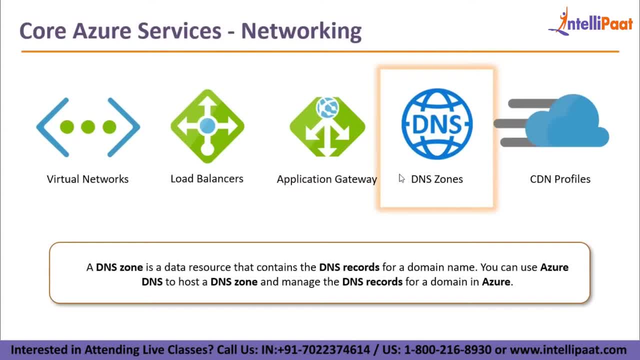 instance, I'll have to specify that in DNS zone service So it will work. So whenever you need a use or whenever you have a use case- like you have the domain with you- or even if you want to buy a domain, you can actually buy the domain at the Azure dashboard. 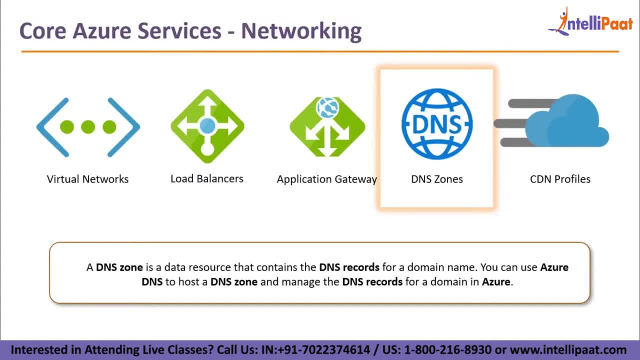 as well. But let's say you have the domain itself, right, And you want to point it to any Azure resource which is existing in your dashboard. So the way to do that is going inside DNS zone, right? Our next service, guys, is again a very important service which is called CDN. 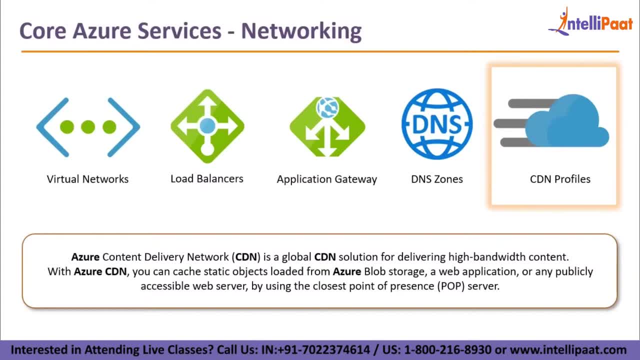 Now, what is CDN? CDN basically means content delivery network. Now, how does that work? What is a content delivery network? A content delivery network, basically, it basically improves the time taken to basically serve you a website. For example, if you go to Amazon dot com or if you go to Facebook dot com, let's say 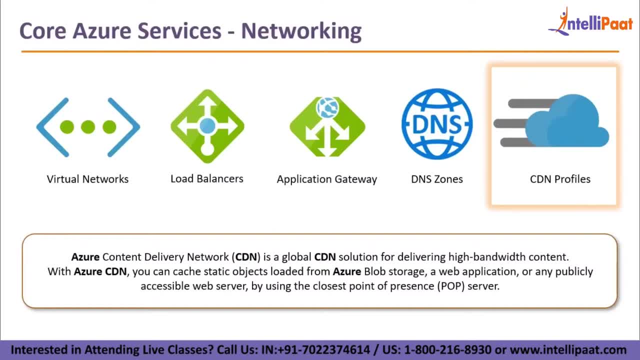 Do you happen to see the speed with which the website loads? if you have a good Internet connection, It loads very fast right Now. where do you think the Facebook website is actually hosted Right Now? what happens is now Facebook is a multinational corporation, right? 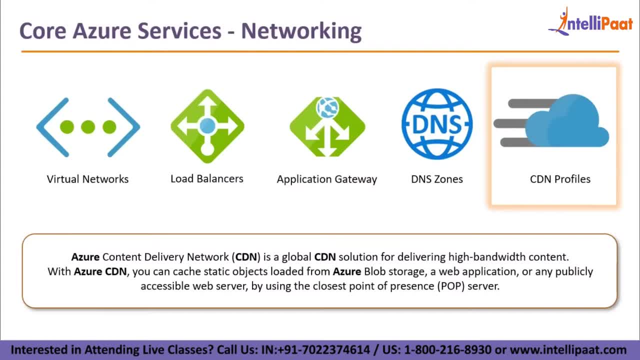 It's a big Web site which is actually being used for the whole world, right? So they have different data centers across the globe from where the requests are basically served. But let's talk about a smaller scale Web site. Let's talk about Intellipaat dot com, right? 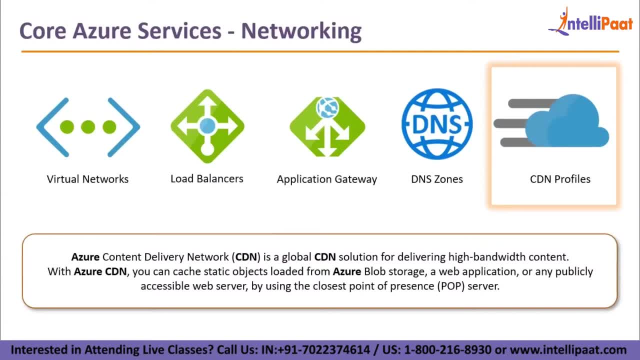 We don't serve the whole world. we basically might have around 400 to 500 people at a particular time. Right Now, what happens is we get traffic from across the globe, right. We want everyone to have a speedy experience when it comes to them using a Web site, right? 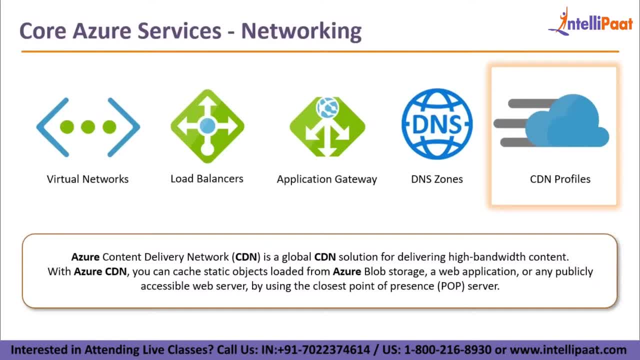 Now, what is what? what are the ways that I can ensure that, let's say, my traffic is coming from US? right, The traffic that comes from US is like, let's say, 60 percent of my overall traffic. So what I can do is I can set up my data center in the US so that the US people will actually 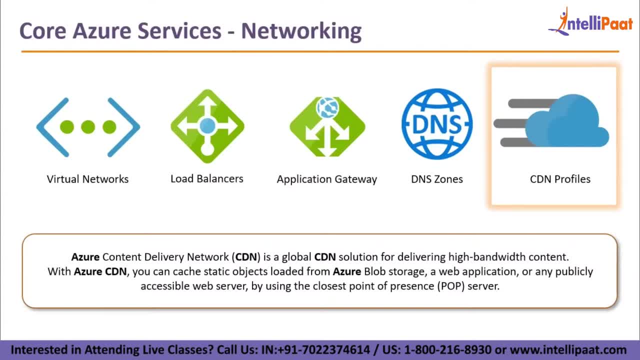 get the Web site First right. But let's say someone is accessing the Web site from Japan, So in that case what he will have to do is, whenever he goes to Intellipaat dot com, the request will basically be sent to the US servers and from the US servers the request. 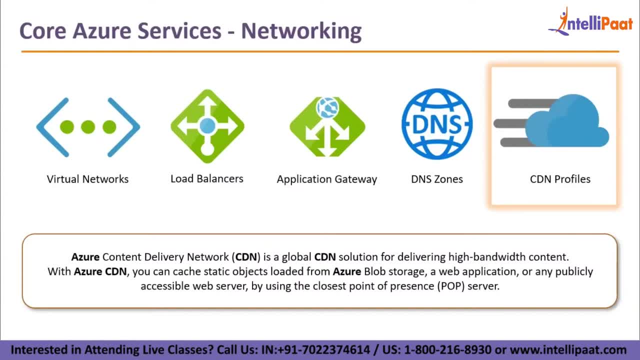 will come back and that's when his Web site will start to load, Right. So this basically increases latency. latency is basically response time of a particular application. In our case, it's a Web site: Intellipaat dot com. Now, if you want to reduce latency, 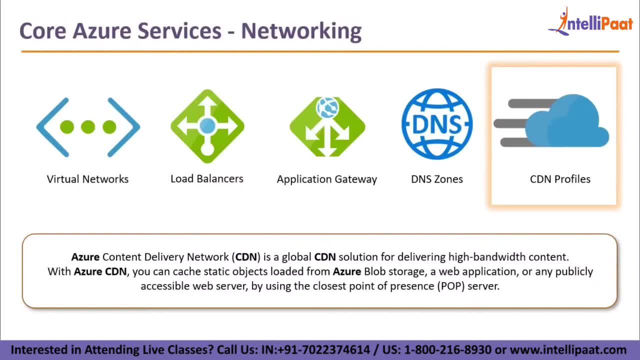 What are the different ways To do that? The different ways to do that is. the first way that you can do it is: you can basically open a data center in Japan as well and load all your scale up the number of servers that you have and then also put a Web site over there. 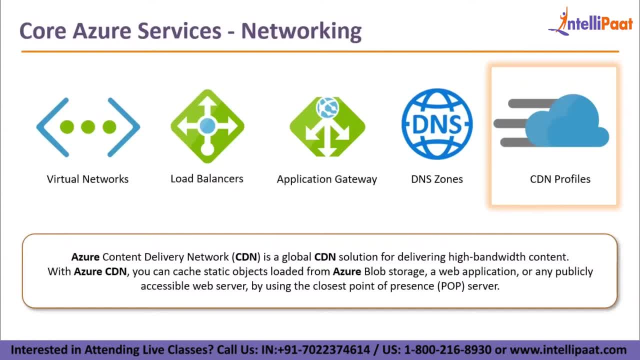 And whenever people from Japan will basically be accessing your Web site, they should be seeing the Japanese version of the Web site, and the people in the US? they should be seeing the US version of the Web site. The people in India should be seeing the Indian version of the Web site. 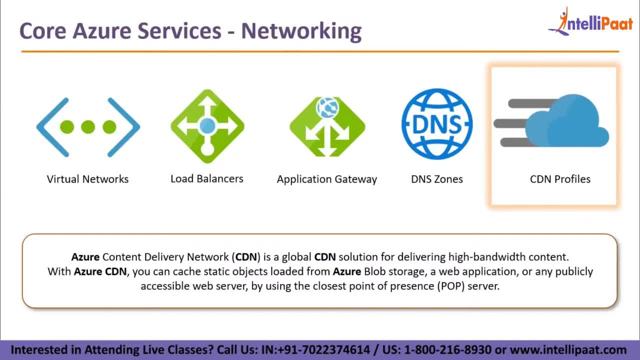 Right. So, of course, when you use an e-commerce Web site like Amazon, So you have Amazon dot and you have Amazon dot com. For Australian people it's Amazon dot au Right? So for different countries it has the different extension, which basically means that that. 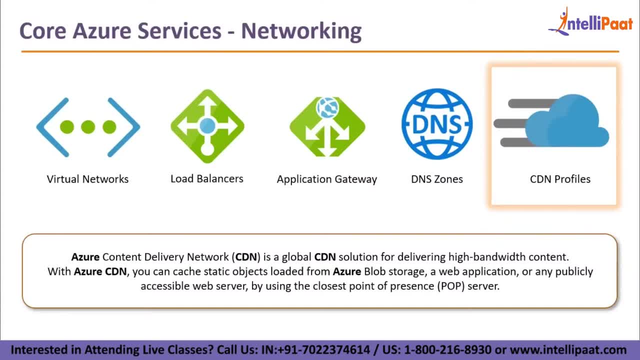 particular Web site is being served from their home countries- data center, Right. But there is another way to basically serve your Web site faster, and that way is basically called CDN. Now, what is CDN? CDN basically caches all your state static data, Right. 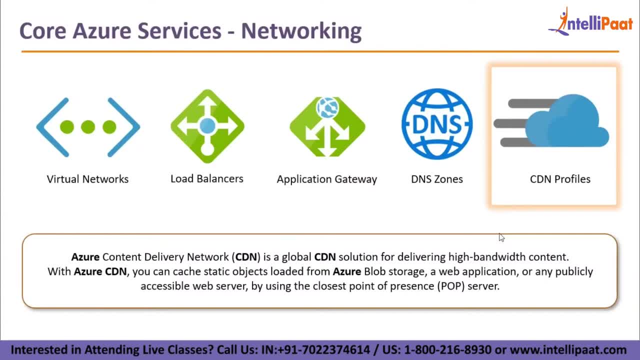 For example, what kind of static data are we talking about? Let's talk about videos. Let's say, my Intellipaat Web site also plays videos in the self-paced courses. Now, if you are a person who is in Japan and let's say, my servers are there in the US, 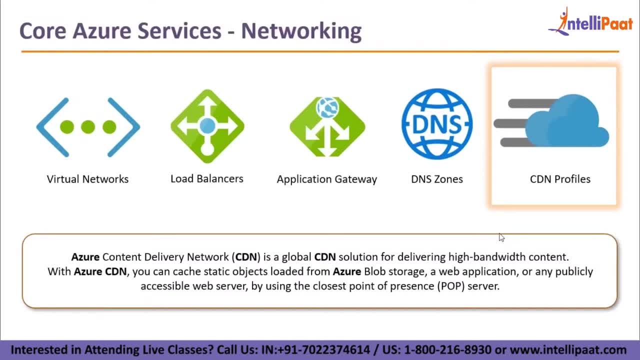 So what will happen is, the moment you try to play a video on my Web site, that video will get downloaded to the nearest location of an Azure data center, Right. So while you're watching that video, that video has been downloaded on the data center. 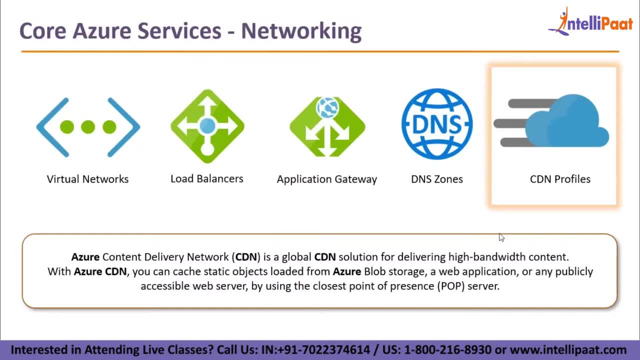 Right That data center of the Azure premises in Japan, And what happens later is basically, whenever any other person in Japan would try to exit that Web site, he will get access to it through the Japan server rather than the US server. So what you have done is you have set up your servers in US. you have not set up your servers. 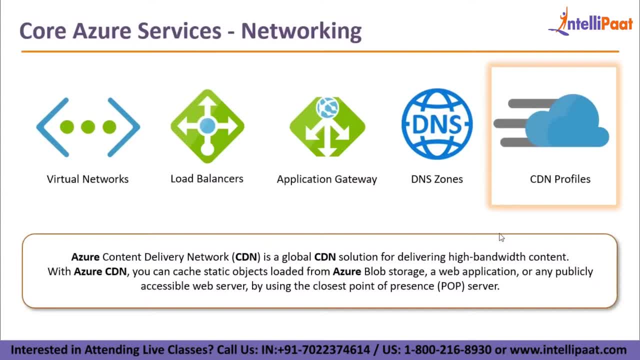 in Japan. but what you have done is you have basically enabled CDN on your Web site And what happens in that case is all the static content is basically loaded. It's basically loaded onto edge servers of Azure. So whatever servers are used to cache data, cache static data in the CDN services are 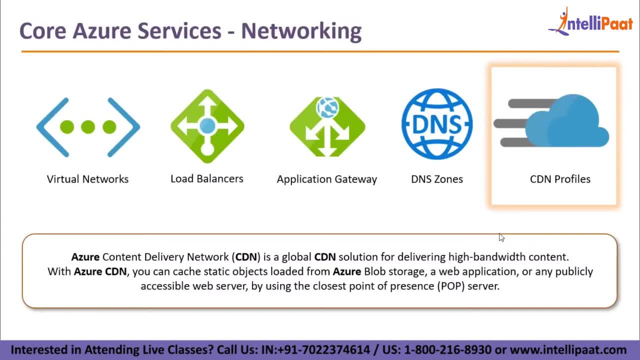 called the edge servers, Right? So whoever is accessing my Web site from whatever part of the world, if they have your data center near them, my content will basically automatically get downloaded over there And, whenever there is the next person who is trying to access it, that already downloaded. 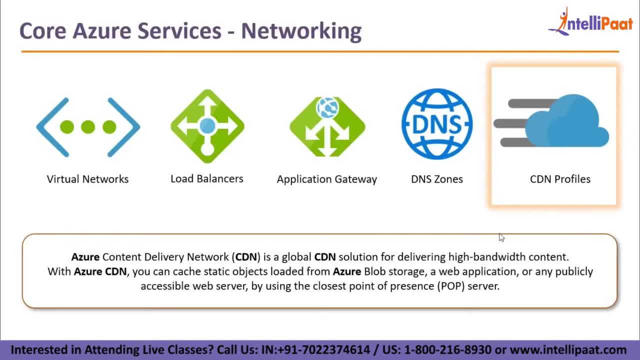 data will be served to him directly And that's how I reduce the latency of my application, without setting up servers in different locations for different kind of traffic that I get Right. So this is how it drastically reduces cost, because I'm not launching new servers and 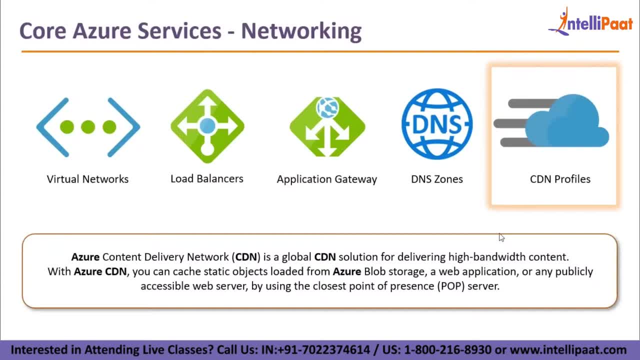 at the same time, it serves the purpose of reducing your latency of your application. So this is what CDN profiles is guide. So these were the core services in networking of Azure. Right Now, let's move forward and talk about a next set of services, which are basically the storage. 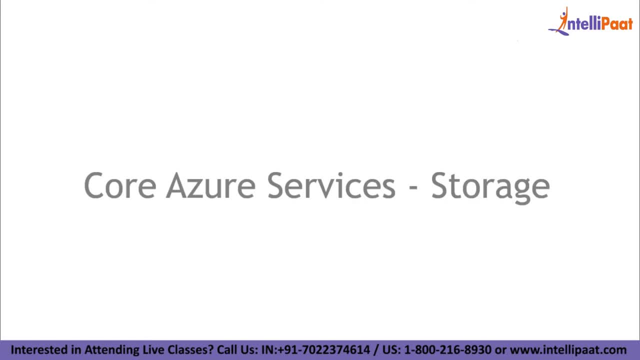 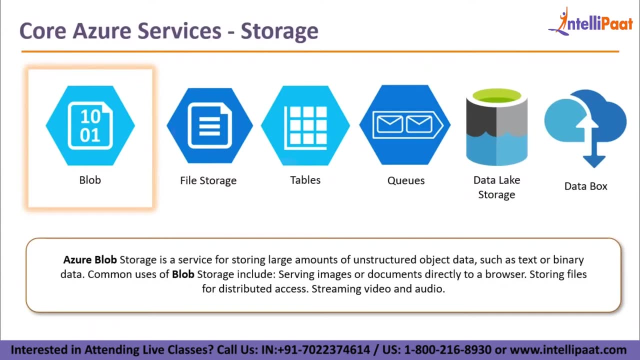 services. All right. So, guys, next in the list, we have the storage services of Azure, So let's go ahead and have a look at them. So, guys, essentially there are six services that you should know of while you're using Azure in terms of storage. 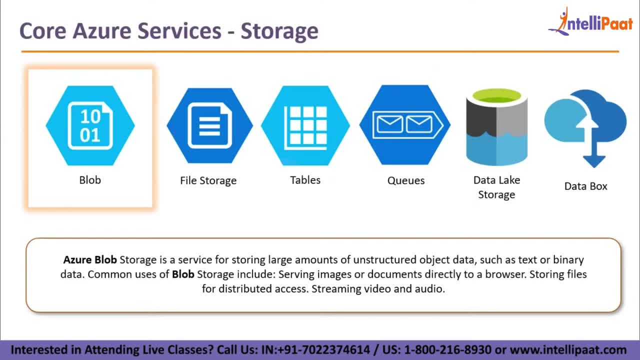 Six services are blob, file storage, tables, queues, data lake storage and data box. So let's discuss them one by one, The first one being blob. Now, what is blob? So, guys, blob basically means binary, large objects, Right? So if you have binary files and you want to store them on Azure, blob storage is the answer. 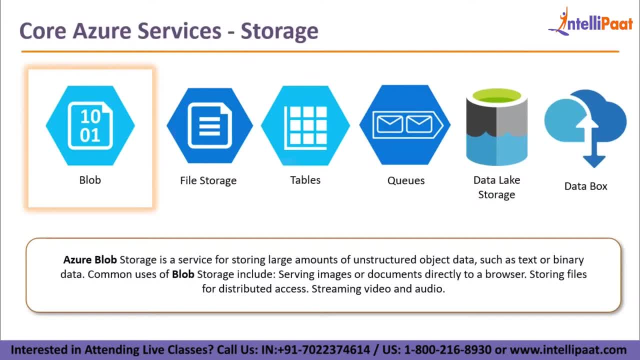 for you, Right? So it can store anything from music files or it can store video files. it can also store text documents. any kind of file that you want to store on Azure can be stored on blob. Now blob also can be used with your, in conjunction with your websites. 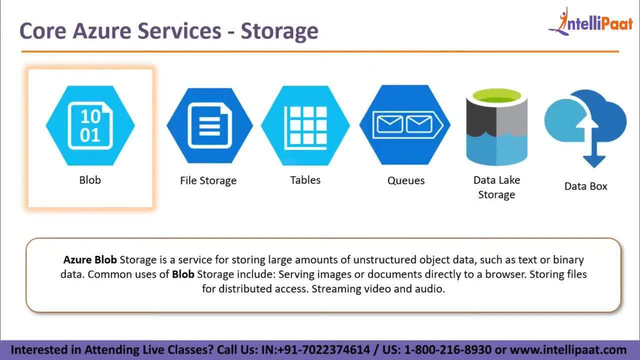 And it can basically act as a storage server for you, Right? It also enables you to host content which is publicly accessible over a link. It can also host static websites on its storage. So that is what blob is, guys, right? So most of the time, you would see that companies, if they have a website, all its static content. 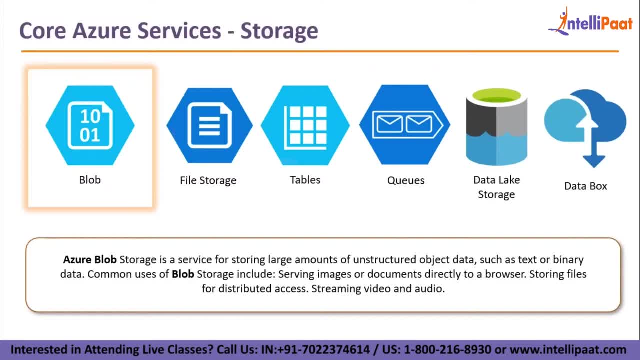 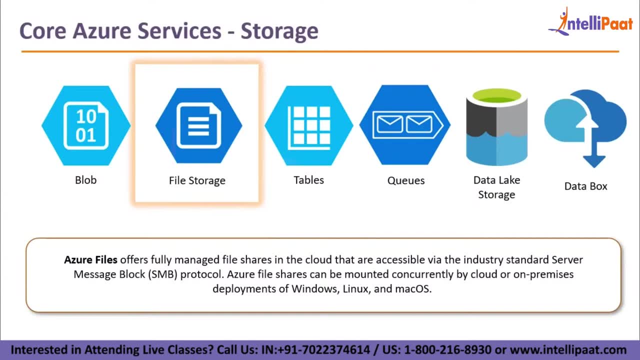 is actually picked up from the blob Right, So this was about the blob guys. Now the next service is file storage. Now, what is file storage? File storage is basically a shared file storage that can be used with multiple computers. That basically means if I have five servers- right. 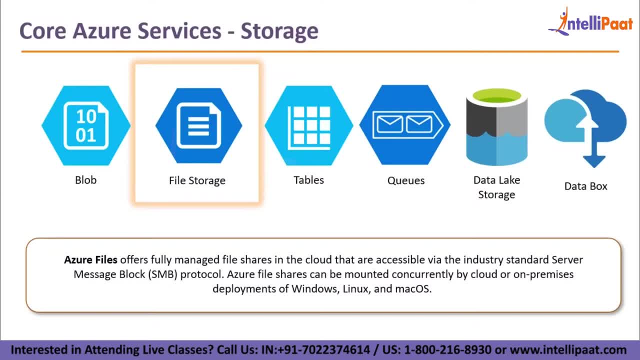 And let's say they need a particular file for their working and all these five servers basically need the same file. So what I can do is I can basically create a drive or I can create a storage Point on file storage and all all these five servers can be used or can be used to basically. 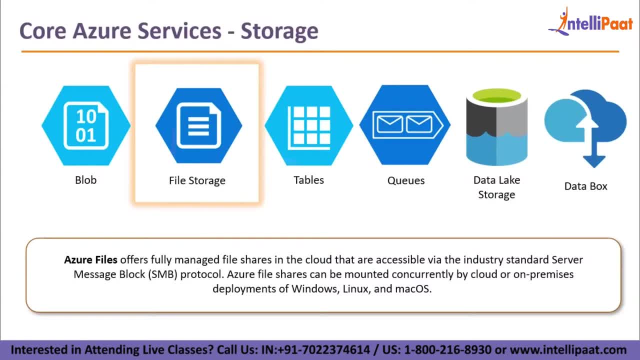 mount the file storage drive on them Right, And any change that is done from one server on the central repository of file storage would all those changes would be reflected on all the next four servers. The use that I can think of for file storage is, let's say, you have an application which 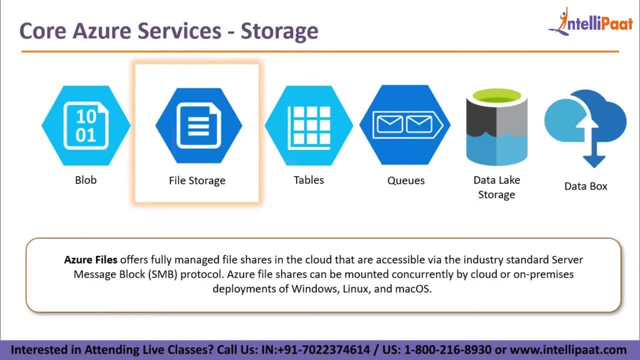 writes data On to a particular file, Right, And basically this application of yours is spread across multiple servers to ensure it is highly available. Right, Let's say you have an application which basically writes data, Right, And this application is spread across five servers. 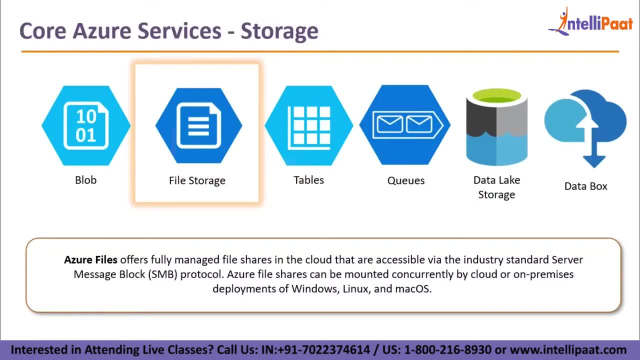 Now what happens is you. we've already discussed the role of a load balancer. You hit the load balancer and you're randomly assigned a server and you work on it. Let's say you work on server one as a customer, You would not know. 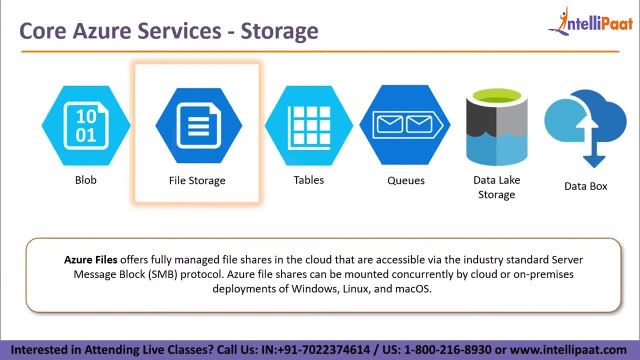 You would not know which server you're working on. Correct? Let's say you worked on server one, Right? You saved your changes and now those files are now saved on server one, But the next time you hit the URL now you're on server three. 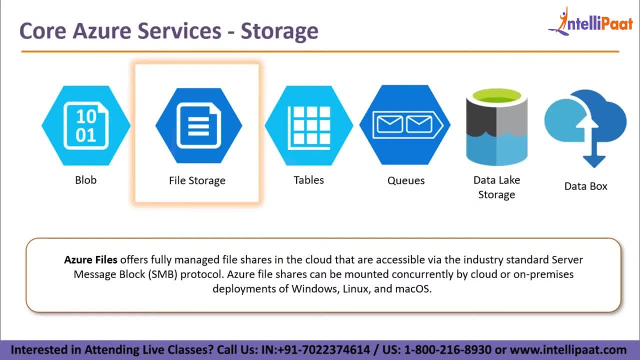 If you're on server three, you would not realize it, but your work, you would expect it to be there on server three as well. Now here comes a problem. If there is no central storage for all these five servers, they will be asynchronous in nature, in the sense that they will not sync data with each other. 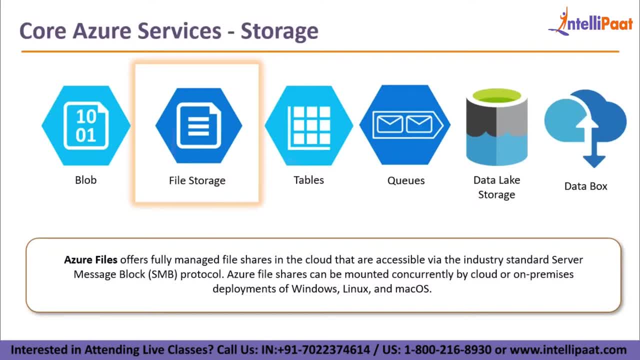 Whatever changes are done on the first server, the third server, the fourth server and the fifth server will be unaware of it. Right, And that is when the arise the need of a central storage, and that is what file storage is for. Right, You can. 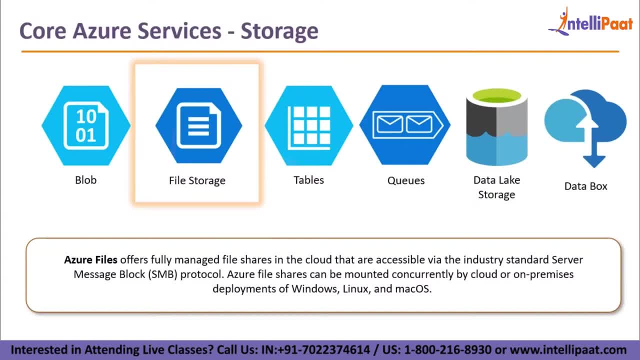 It basically uses the SMB protocol, SMB. So basically SMB 2.1 and 3.0 is compatible with file storage and recently even Linux platforms like Ubuntu, CentOS and even Mac OS have started supporting SMB Right. So it essentially would recommend you to use SMB 3.0, but there are some OS versions which 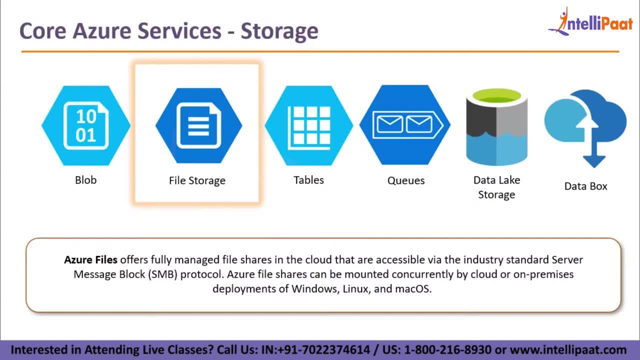 could have SMB 2.1, for example. if you're using Ubuntu 16 or Ubuntu 14.04, they are basically using SMB 2.1.. Right, So it has the backward compatibility as well for older OS like Ubuntu 14.04.. 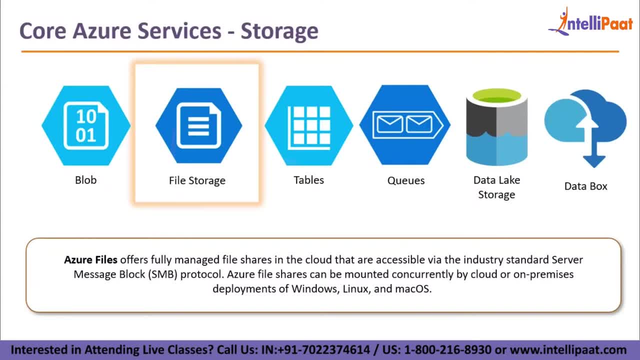 Right. So if you want to mount a drive on Ubuntu, which basically is hosted on Azure file storage, you can do that using the SMB protocol. there are a list of softwares that have to be installed. More on that we can discuss when we study file storage in detail, but for now, because 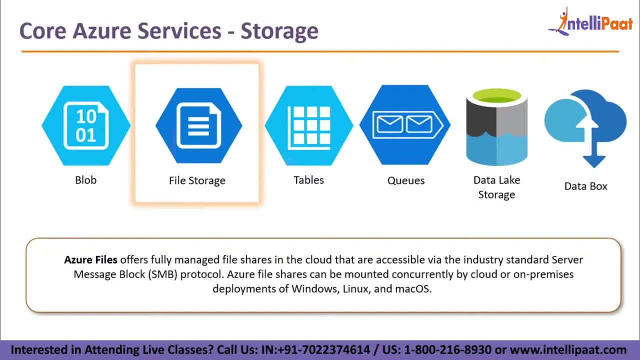 we are in a tutorial session. we are basically. I just told you what file storage is used for. So if you want to ask or if you want to think of a use case where you need a central storage kind of a thing, Now you know that you have to use Azure file storage. 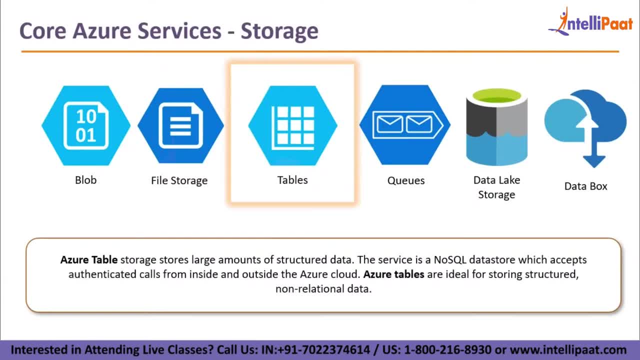 Moving on, guys. our next service is Azure table. Now, Azure table is basically a NoSQL data store, right, and it can help you to store structured data Right. It basically can store structured data. It has table, tabular columns and tabular rows in which you can save data. 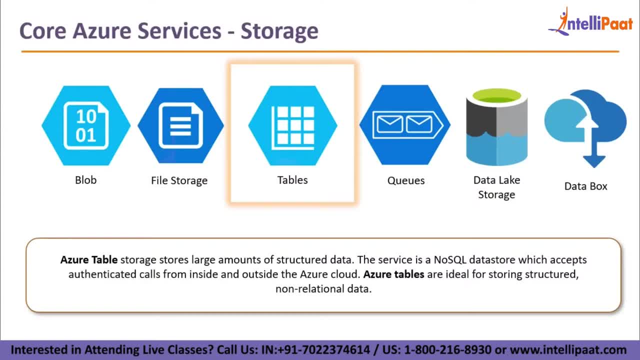 But it is NoSQL in nature, which means the data does not have to be in symmetry. Right, Right. The data could have eight columns. the third row could have two columns. the fourth row could have just five columns. it could take any kind of data, but the only condition is: 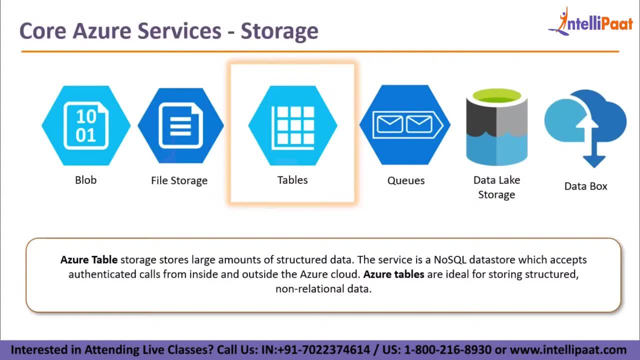 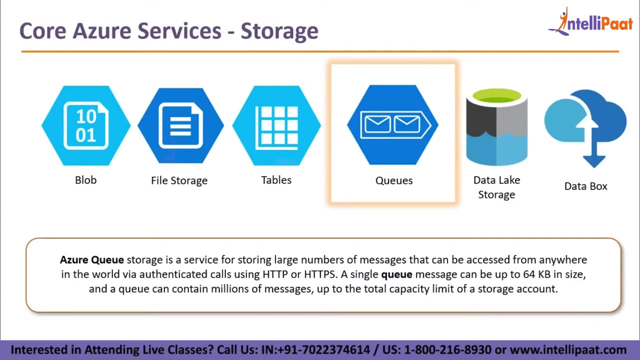 that the data should be structured among columns Right. So if there is any kind of need for storage of data of this kind, you can use Azure table. Our next storage is Azure queues, which basically is used with stateless systems- Right Systems- which do not know of what all jobs are executing on the counterpart or on the 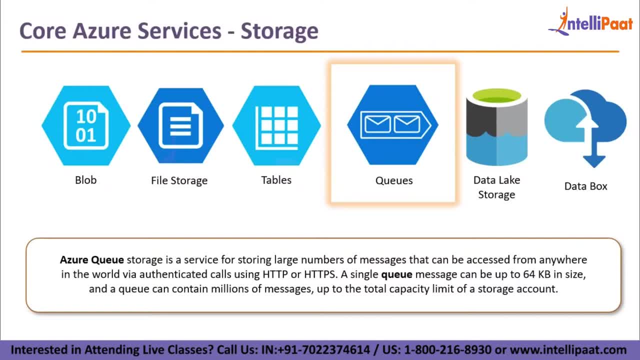 replicated servers of their application. For example, let's say there is an image processing website and what it does is the moment you upload an image, you can process the website or, sorry, process the image according to your need, Right. So what happens in this case? 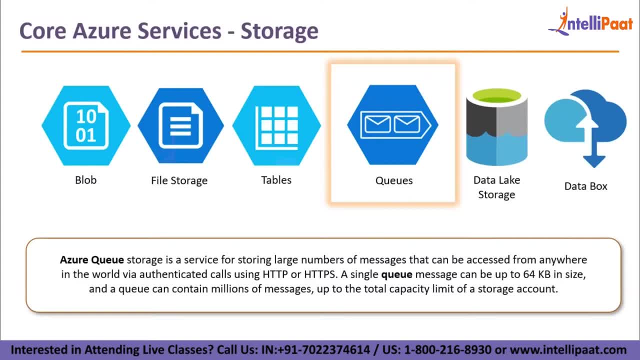 Let's say there are 200 people on the website and they've all pressed the process image button together, And what will happen? There are 200 images That have to be processed and obviously not all 200 images can be processed at the same. 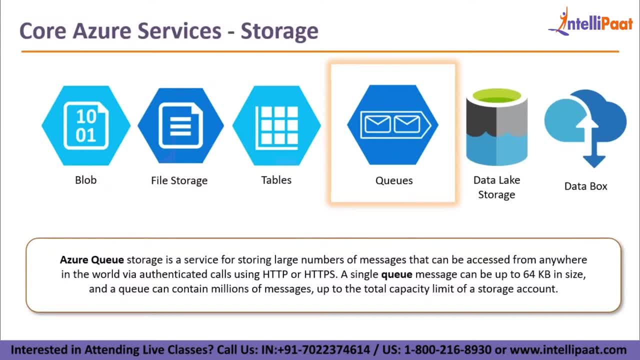 time. So what happens is the images are processed one by one and let's say, in the back end server, where the processing is done, there are five servers who are doing the processing. OK, Now, all these five servers, they pick up an image at random from the queue. 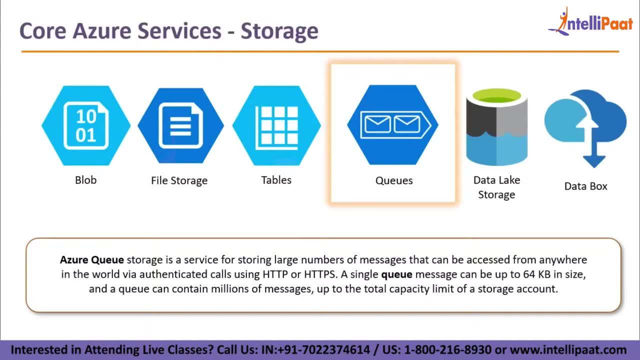 So let's say the queue is first in, first out. whichever image comes first goes out first as well. So whenever the job of the first server is done, Let's say it was Doing the processing on an image and the image processing is done. 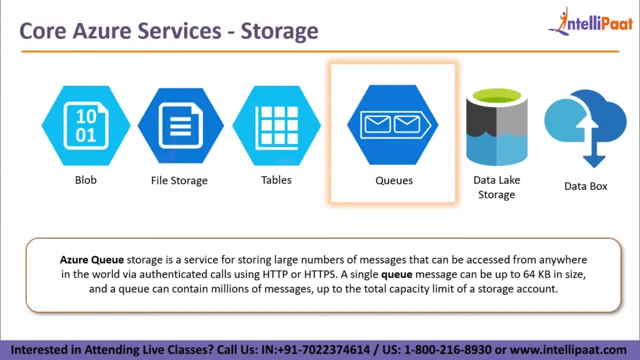 It picks up another image from the queue. The second server would also do the same. The third server would also do the same. Right? So what happens is, let's say the first server. it processed image one. Now the second, third, fourth and fifth server- they would not know whether the first image 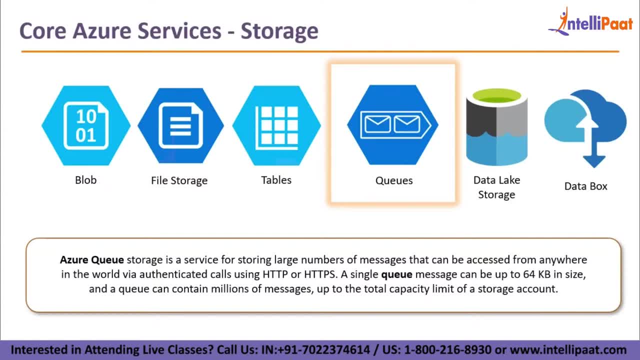 has been processed or not, and they can process it again. So for those kind of scenarios and for solving those kind of situations, we had queues which basically streamline all the content which has to be processed. And whichever content is taken up by a particular server, it deletes it from the stack and then 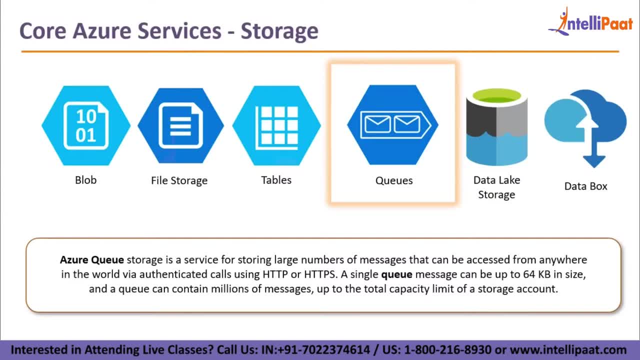 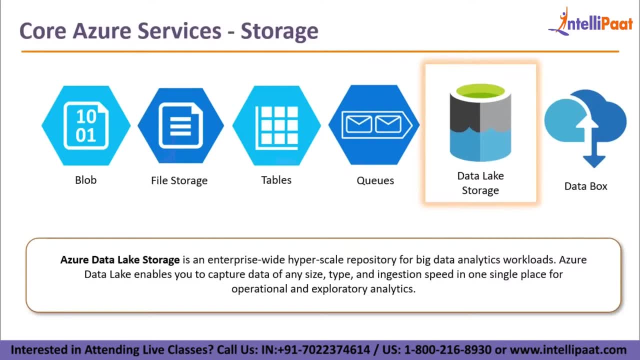 puts the second image or the second object, which basically has to be processed, Right. So for these kind of scenarios, you use Azure queues. Our next service is data lake storage. Now, data lake storage is similar to that of a blob: not a blob, but tables as your tables. 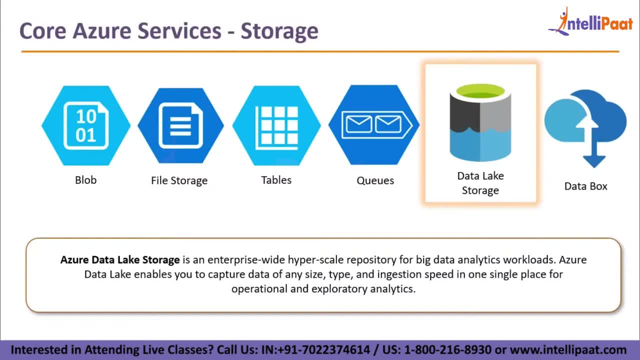 So data lake storage can store data, But It can also be used to store data for big data analytics. It specializes in that particular course segment. So if you have a big data analytic use case and you want to store data for that data lake, 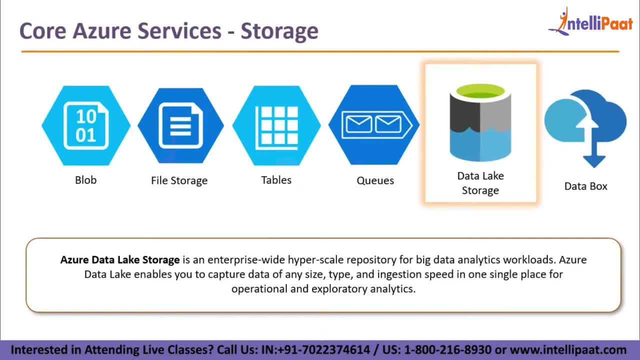 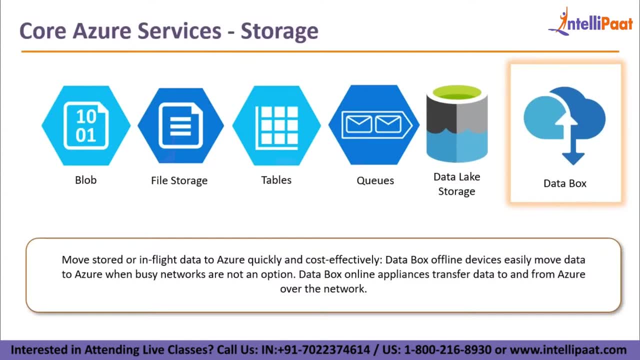 storage is should be the choice for you, Right? So this is about data lake storage, guys. The next service that we have is Azure data box. Now, what is Azure data box? Now, you might think of your company. let's say. let's say, you're working for a company. 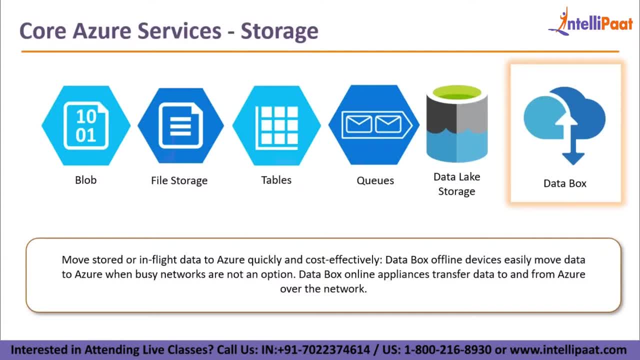 and you have all the servers on premise. You have been working since 15- 20 years in the sector that you are. I mean your company, and you did not have cloud at that time- and what I've done is you bought your own servers, you have hosted your own applications. 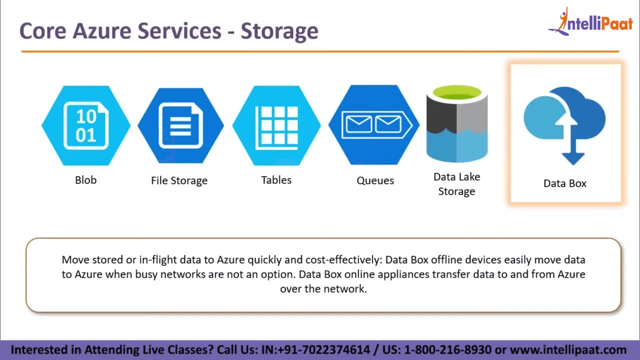 But now the cost incurring for those servers is too high when you compare it with the cost which is there in cloud computing when you opt for cloud computing. So now what I have decided is basically that you want to migrate all your applications to Azure data box. 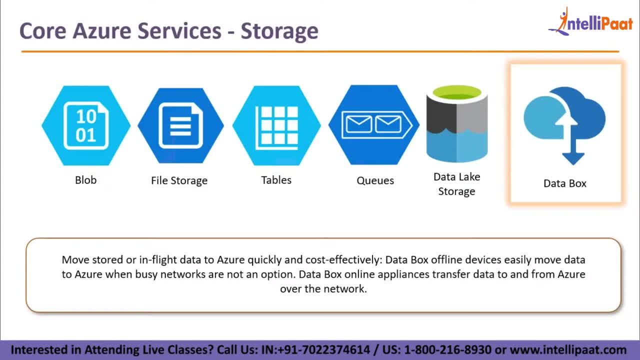 Okay Or sorry, to Azure. So let's say there are five bit, there's five petabytes, or let's say thousand terabytes of data that you have to transfer on Azure. Now, in businesses, time is very important, guys. Time is money Basically. you must have heard of that phrase. 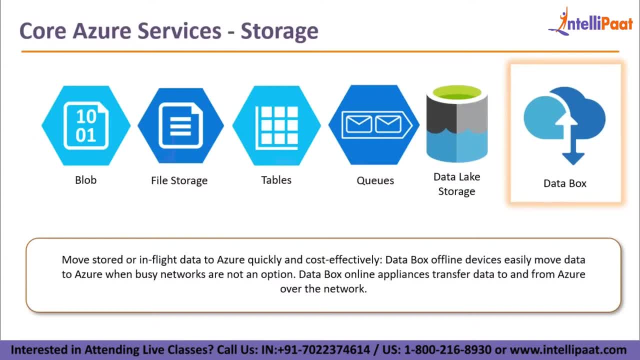 So everything is required at a fast pace And if you want to transfer a thousand terabytes of data, imagine the data transfer costs which would incur to you, and also it would take a lot of time to upload thousand terabytes of data via Internet towards your right. 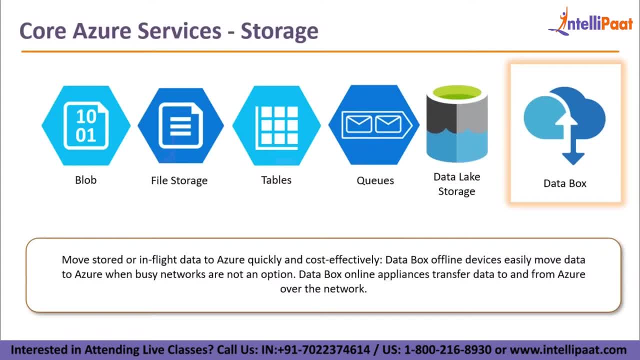 You would agree on that. now, to solve problems of this scale, when you have a large amount of data that you want to transfer on towards your cloud, What is does is it basically gives you a physical device on which you can load your data right, So as your data box is a service in which you can 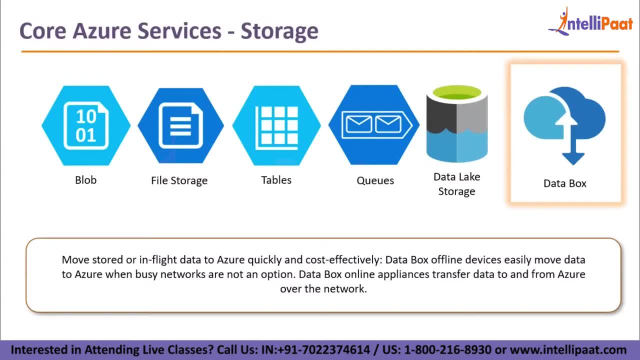 You can basically request A box, kind of a system, from Azure which basically ships to your company. You can load all your data onto it and then that box is again shipped back to Azure cloud and all your data is again uploaded to Azure cloud from their data center directly. right, 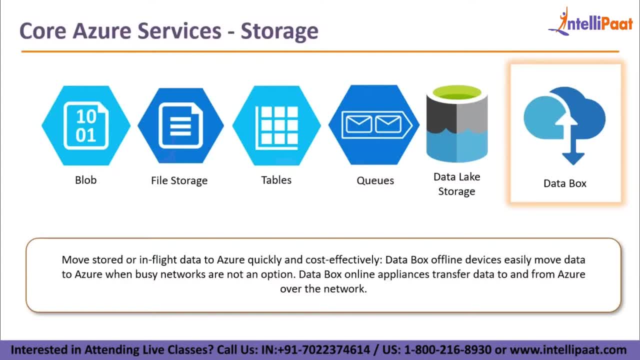 So this not only reduces the time taken to transfer data, but it also hugely reduces the cost that you would incur in the Internet charges, Because thousand terabytes is not less data guys. now, thousand terabytes is very less when I talk about a company which is existing since 15 years and when you talk about multinational. 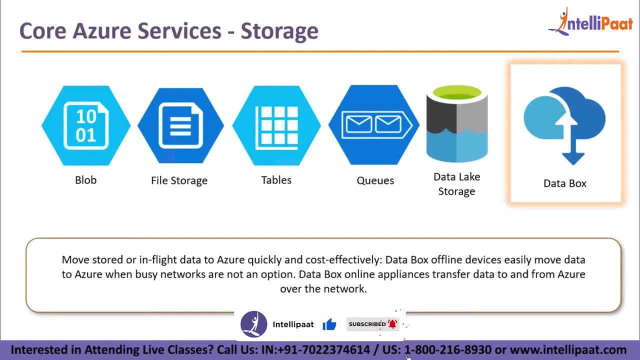 corporations, the data can be in petabytes, right, And if you have a petabyte scale data that you want to transfer to Azure, it would take weeks, if not months, to transfer that kind of data. So that is where data box comes in and data backs a data box, as your data box can. basically. 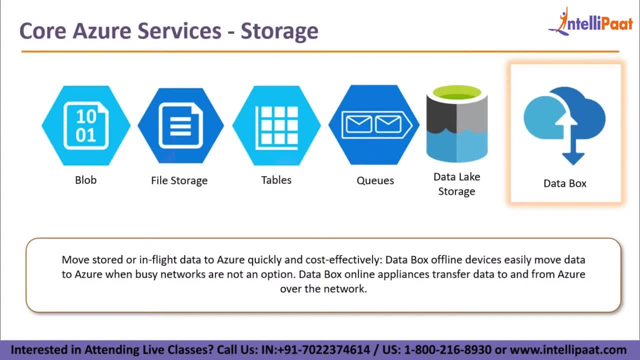 support Around 5. Petabytes of data at one time right Now. if 5 petabytes of data is less for you, you can request multiple boxes from Azure too, and multiple boxes will reach your location. you store your data onto it. I mean you copy your data onto it and then request as your back that you can take away. 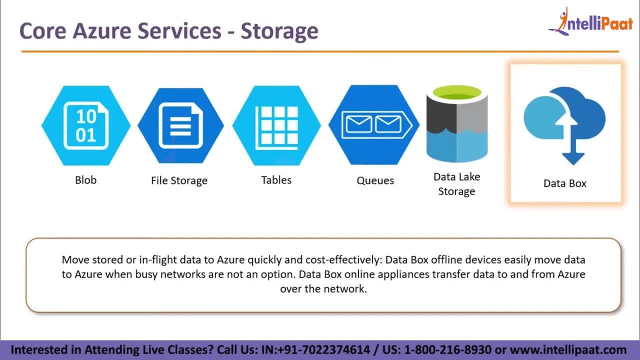 your data boxes and they will take the data boxes back to the data centers and transfer the data directly. right. This will reduce your time to around one week of time, so your data of petabyte scale can be transferred To Azure in less than a week and at the same time you would also save on huge Internet. 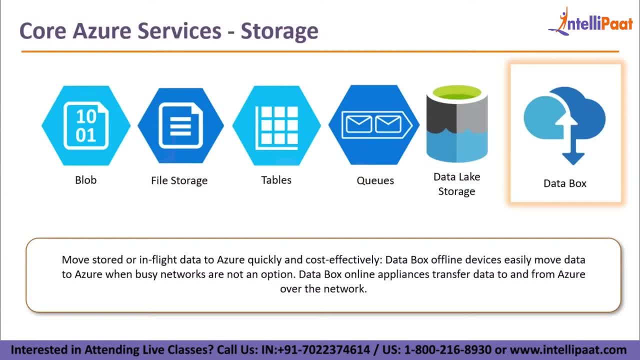 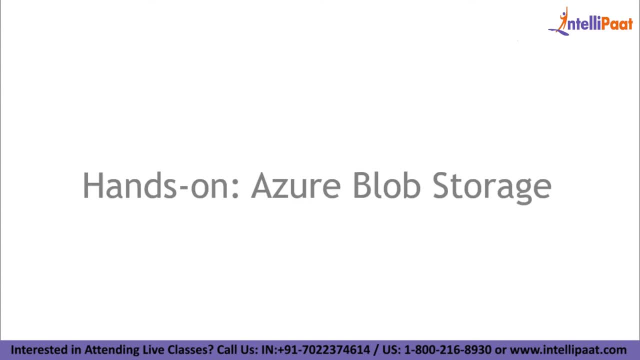 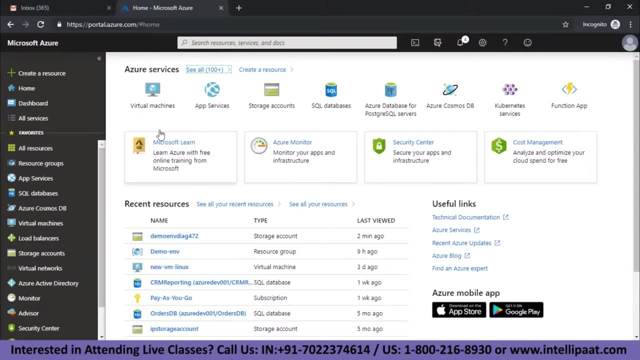 costs, Right? So this is what the data box service of Azure is. All right guys. so now let's go ahead and do this: hands on on Azure blob storage. So let me quickly switch on to my Microsoft Azure portal, which is this? All right guys, so this is my Microsoft Azure portal. what I want to do is I want to show. 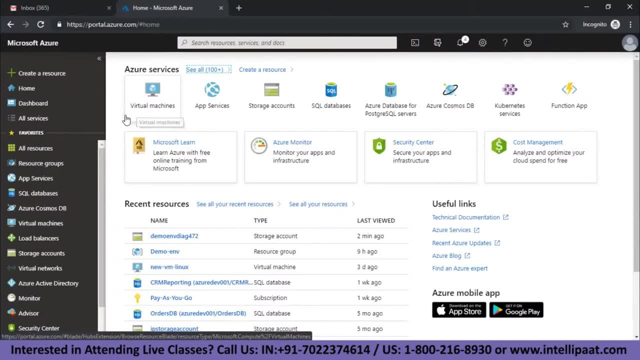 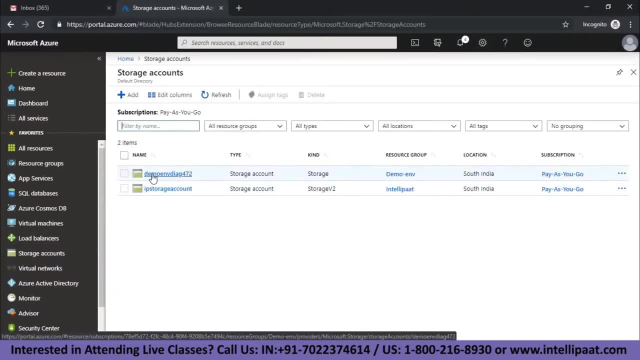 you guys how the blob storage works in Azure, Right? So the first thing that I'm going to do is I'm going to go into storage accounts and over here you will find that there is a storage account called demo environment. Why is it here? 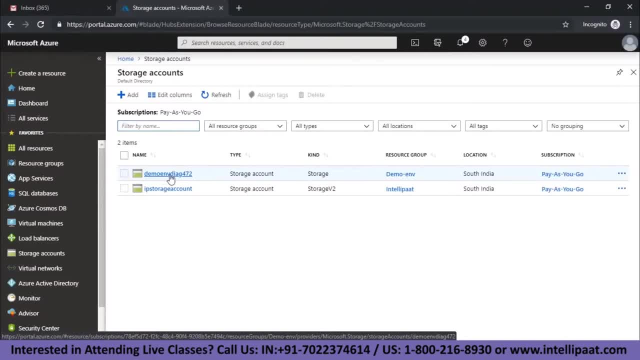 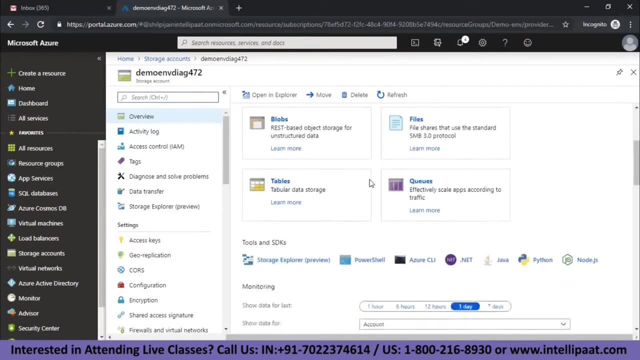 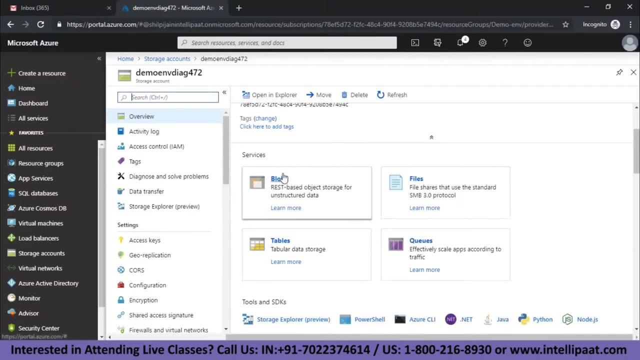 Because I created a virtual machine with the name demo environment, right, And obviously the virtual machine requires some storage. If you go inside this, you will see that you have the four options that we discussed, that are, blob, files, tables and queues. What we are interested in is blob. 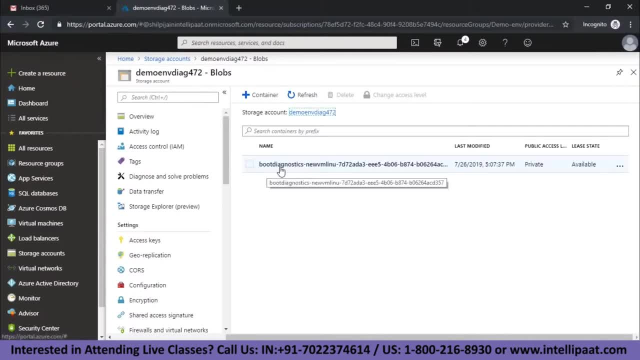 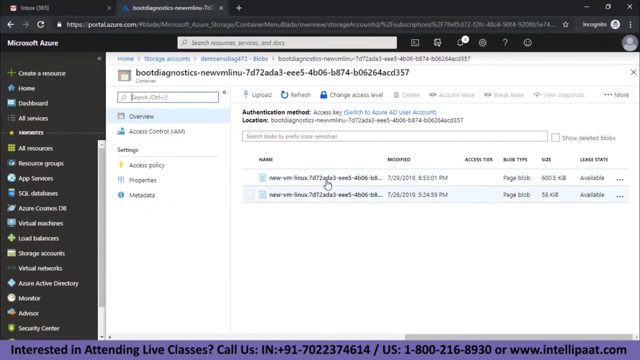 So we'll just click on that And you can see that. But this has boot diagnostics for the new VM Linux that we launched earlier, right? So all the logs for that VM are basically going inside this container. So basically, if I go inside this container, you can find that these are the two text files. 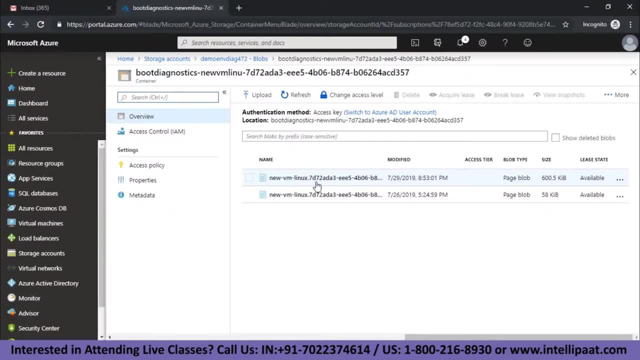 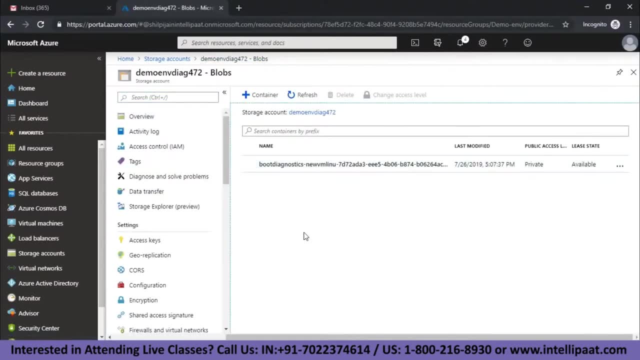 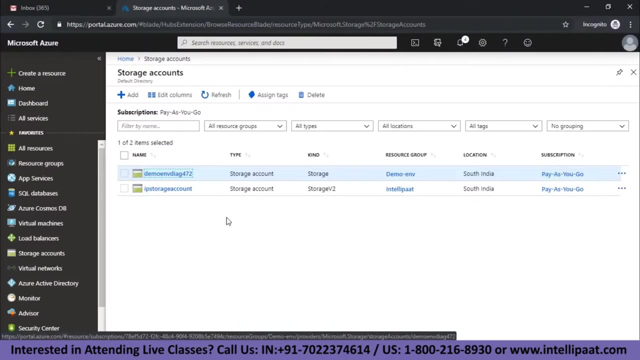 which are present will basically will have the log data of that VM that we launched, right So? but we're not here for that. What we basically want to do is I'm going to show you guys how you can use blob. Now, no matter what you are working on, if you want to create a blob, so it's for yourself. 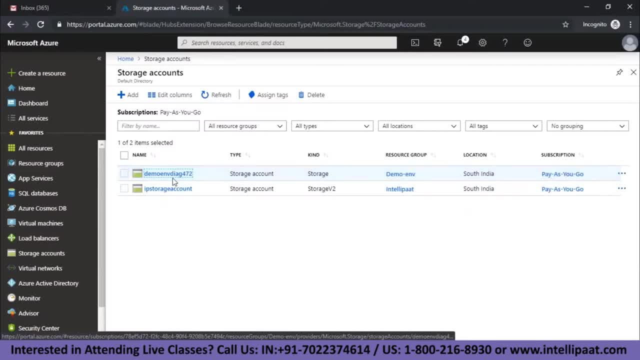 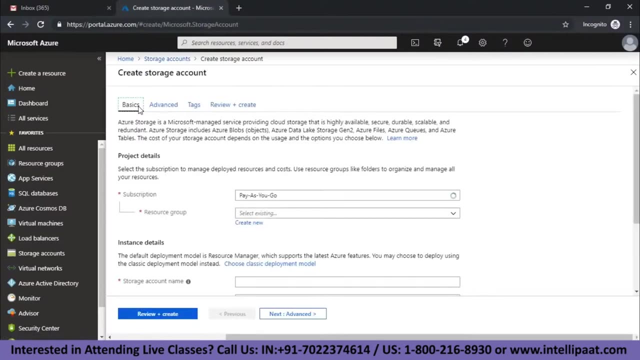 you will have to create a storage account, right. In our case, this was the VM storage account. If you are starting a fresh on Azure, you will not have any storage accounts over here, right? So let's create a storage account first and let's try to name it something relevant, which. 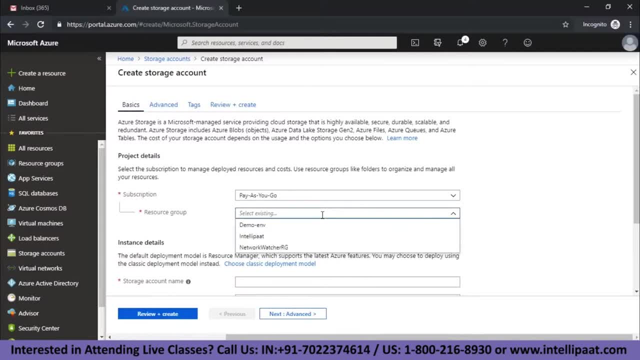 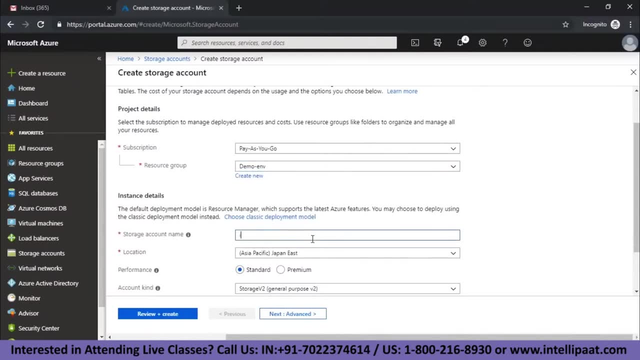 might go with the demo that we're doing. So the resource group, We want to add it in his demo environment and the storage account name that we want to give is, let's say, Intellipaat hyphen zero. let's say: this is the one that we want to. 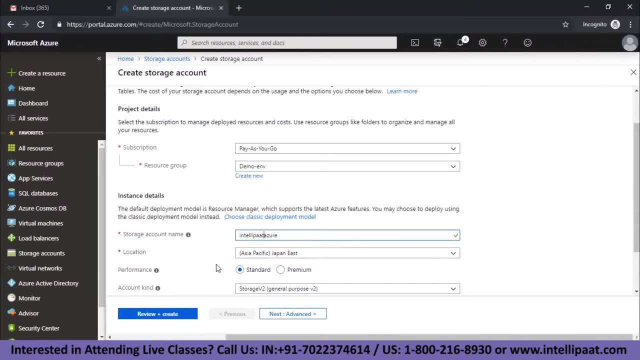 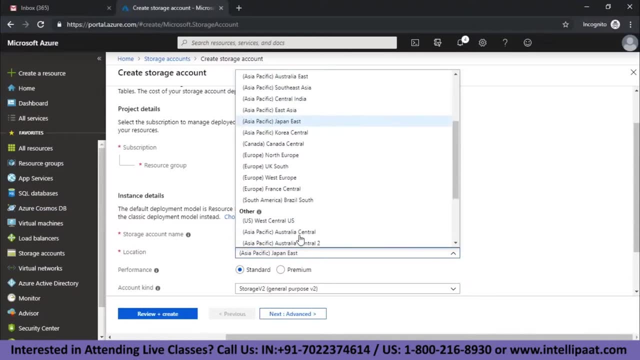 give Okay, But it's a location that we want this storage account to be in. as discussed earlier, we'll choose a nearest location to us. So in that case, the nearest location would be Asia Pacific, South India. Let's try to choose this location, right. 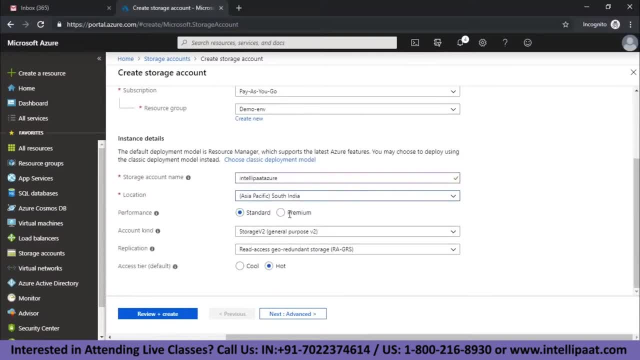 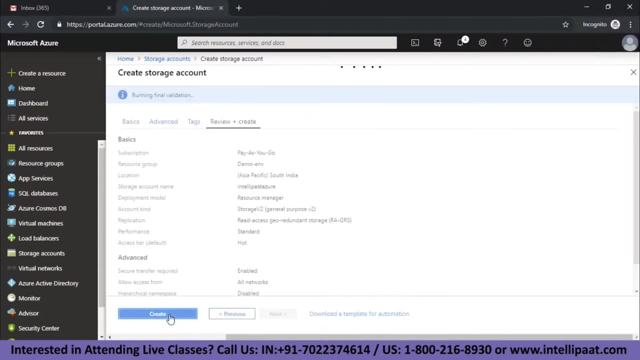 Now, how do you want the performance? It could be either standard or premium. We can discuss this later, probably when we'll discuss this service in detail in our further sessions, But for now, let's let it be at standard right, Put everything at default, and now let's click on review plus create. 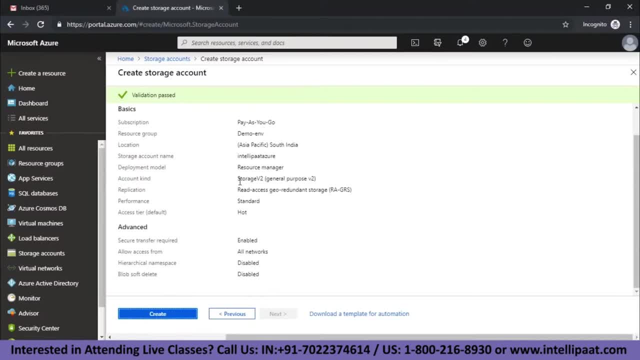 When you do that, it will ask you all the- basically show you all the information with respect to the storage account that we are creating. If everything Looks good, just click on create. Once you have clicked on create, guys, your storage account will take some time and then 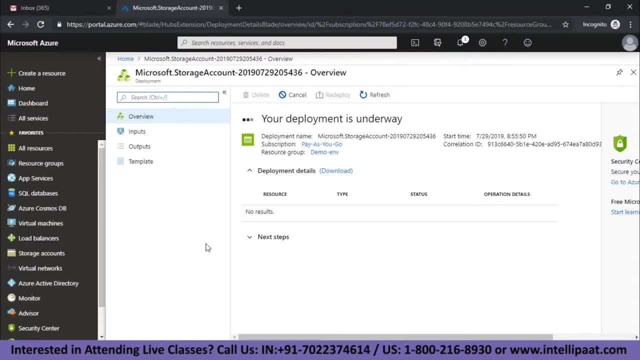 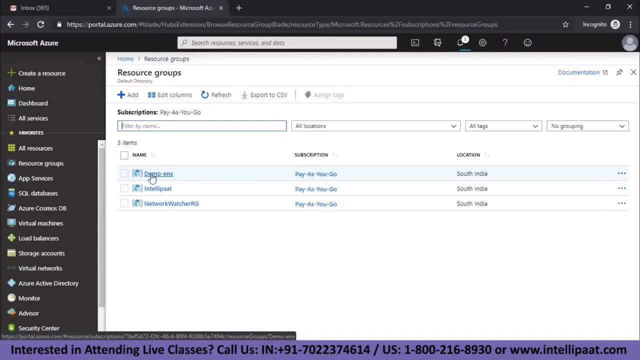 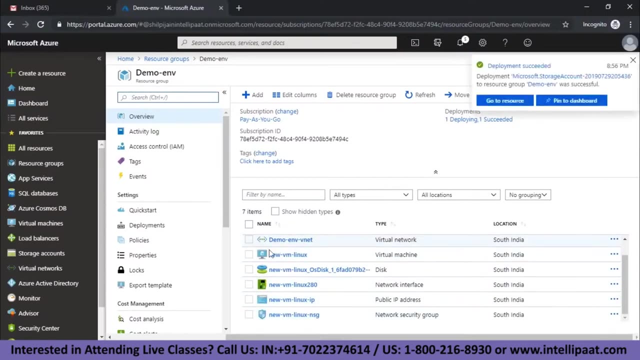 it will become ready for use And, like earlier I specify: all you have to do is go to the source groups. Let's say: this is the demo environment that we created earlier. I'll go inside this and now I can see all the things that I had launched are present over here, even the storage account. 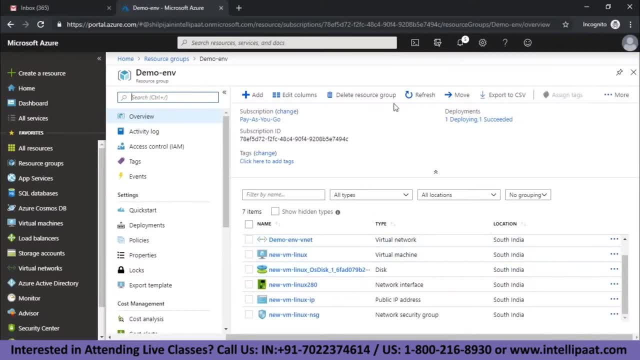 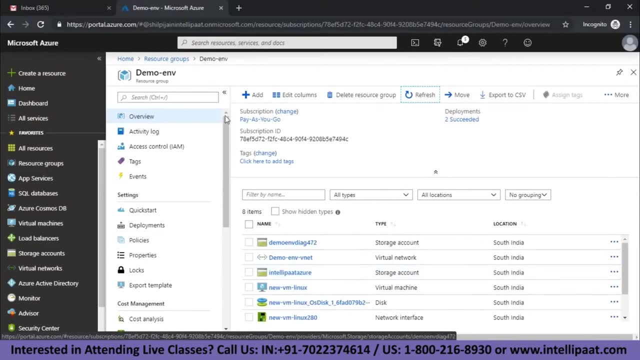 that I'm creating Because that is basically being launched right now. I can see that also over here. as you can see, it's Intellipaat Azure. This is the storage account that I created And now it is visible inside demo environment resource group. 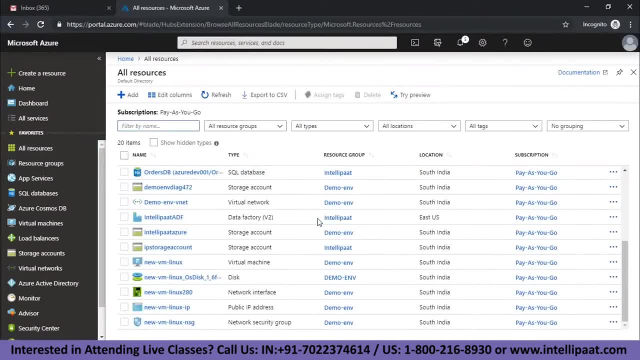 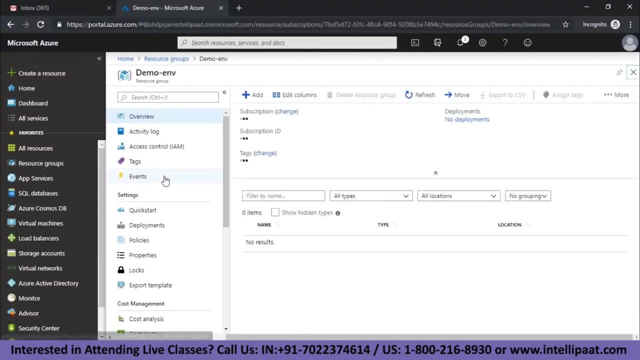 On the other hand, if I go to all resources, I'd be able to see all the resources that are there on my Azure account, but this looks a little messy, And that's why resource groups are pretty helpful, guys, because I know that my resource that I've deployed is sits inside a specific resource group. 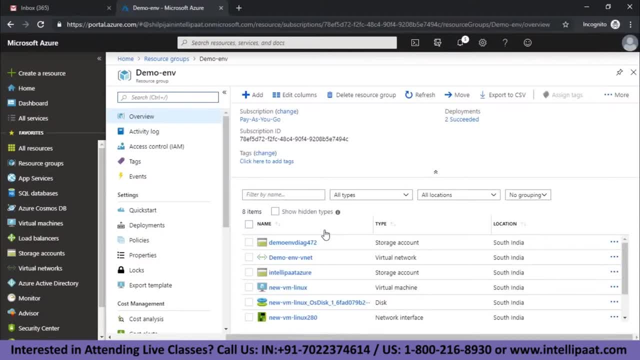 And that resource group. basically, I can name on the basis of what task that particular resource is going to do. Since ours is a demo session, what we have done is all the resources that we are basically deploying are inside the demo environment resource group And right now we just deployed this storage account, which is Intellipaat Azure and, as 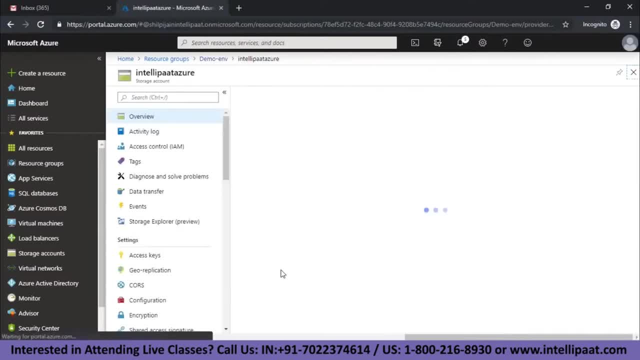 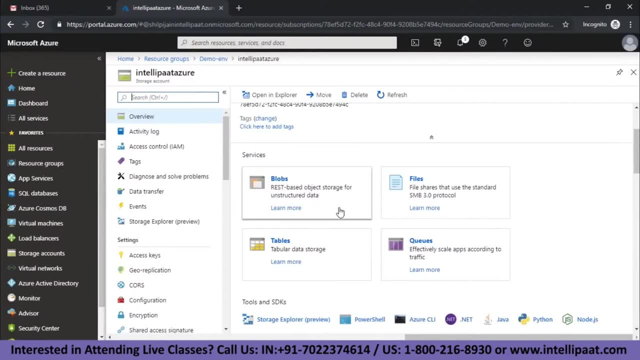 you can see it has been successfully deployed. Now let's go inside the storage account and, like we saw earlier, you see a similar user interface over here. You have four options: Either to go to the storage account, Either to go inside blob, or to go inside files or tables or queues. 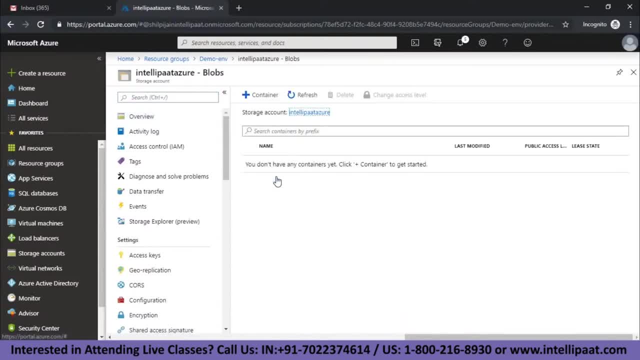 Let me demonstrate to you how blobs work. So we'll go inside blobs, guys, and, as you can see, there are no containers over here. What are containers? Containers are nothing but root folders, right? For example, on Windows, you have the desktop folder, So desktop folder becomes the root folder. or to give you a better example, let's say: 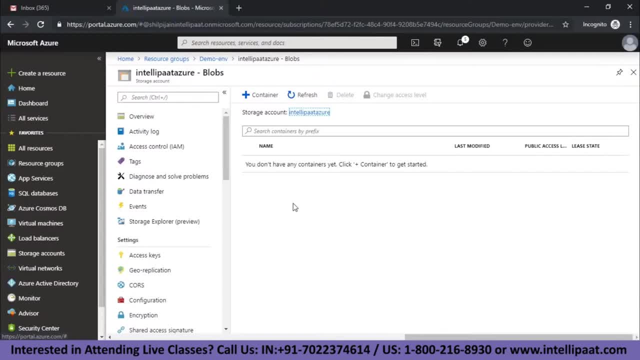 you go to the C drive of your computer, right? Whatever is inside the C drive is the root of the drive. If you create a folder inside that drive and you then put files inside that folder, that is no longer the root directory, right? So whenever you are uploading files on blobs, the first thing that you need is a root directory. 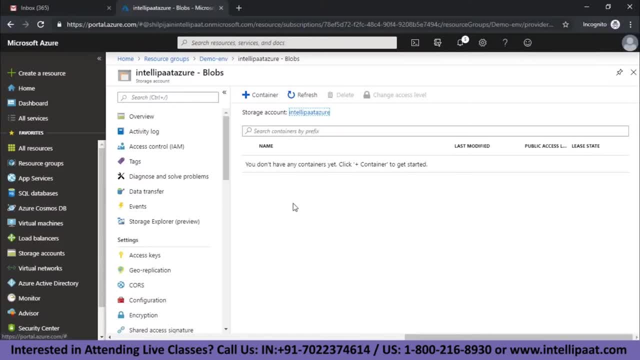 and that root directory is nothing but containers, right? So let's go ahead and create a container. so I click on a new container and let's name this container. Let's name it as Intellipaat, okay. and now let's click on: OK. 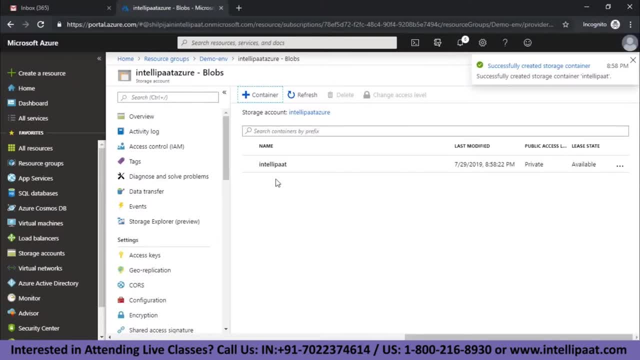 Alright, so my new container is now ready. Now you would have noticed that there is something called as access level, and right now the access level is private. More on this I'll explain to you as we move along. So right now we have not changed it to anything. it's private and let it be at private. 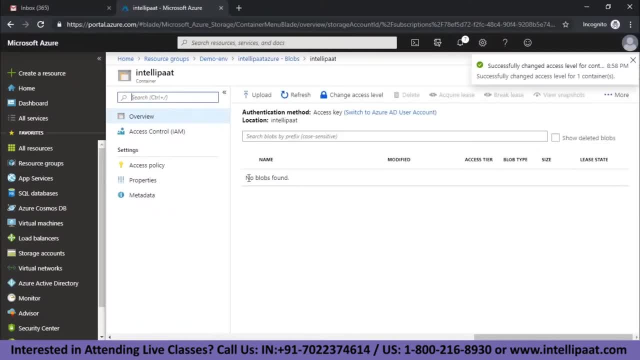 Now what I'll do is I'll go inside this container and it says: no blobs found right. So what I can do is I can upload some files onto this container, and for doing that I'll have to click on upload, and now I'll have to select the file. 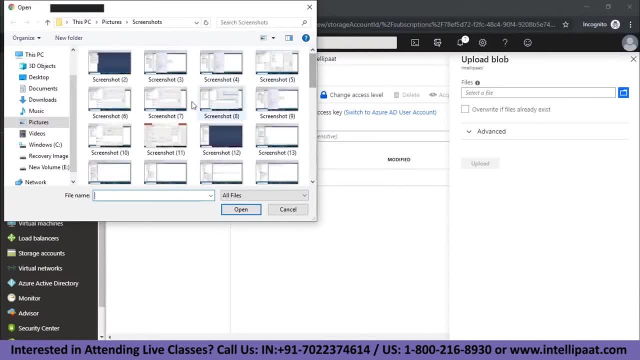 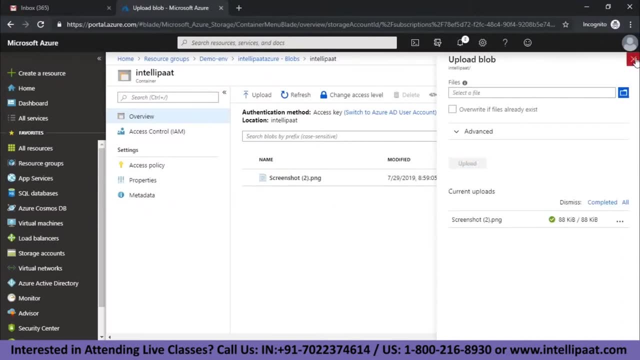 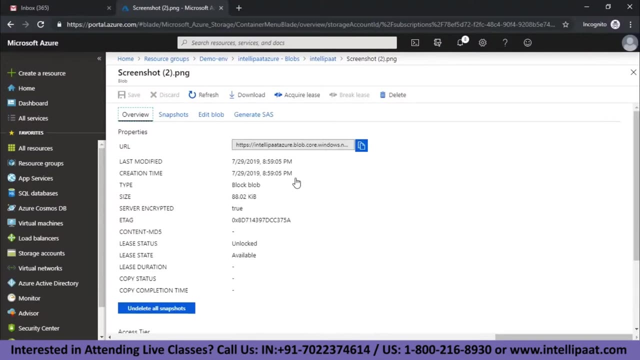 So let's. so these are some images that I have on this system, So what I'll do is I'll just select a random image and now let's upload this image onto my blob, Alright? so this image is now uploaded on the blob, and what I can do is I can just click. 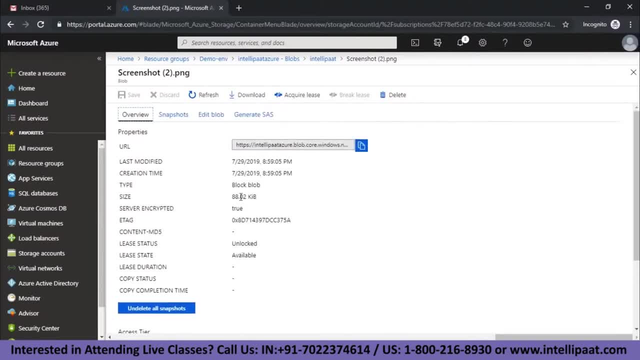 on this image and I can see all the information with respect to it. It's 88 KB in size. this is the last modified time. this is the creation time. Now here is something interesting, guys. I have the URL to the file that I have uploaded, right? 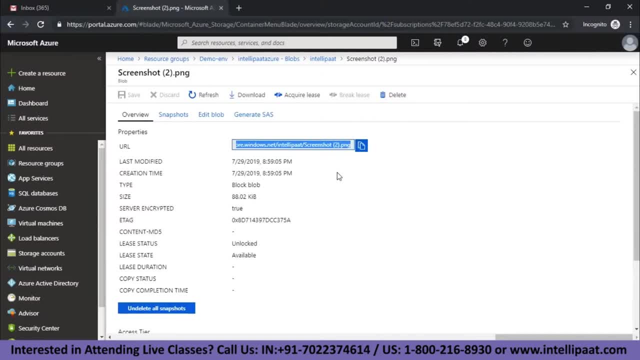 Now this URL can be embedded anywhere. it can be embedded on a website. it can be embedded on a post that you're making to social media. This, basically, is a file which is now hosted on the internet And anywhere. anyone who has access. Okay. 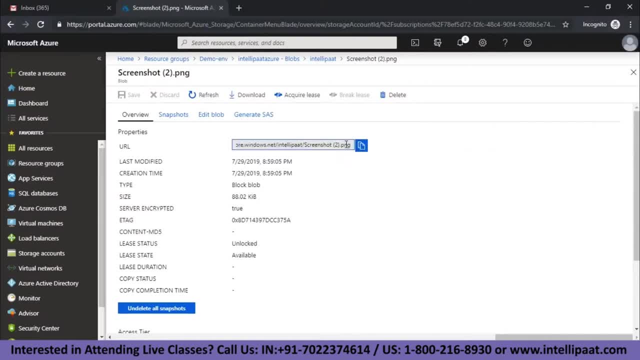 Access to this particular link would be able to see the image that you have just uploaded. Awesome, isn't it Right? So what I'm going to do is let me copy this link and let me open it in a new tab right, and I'll hit enter. 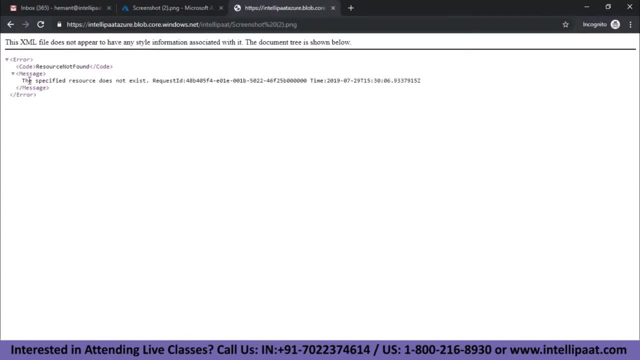 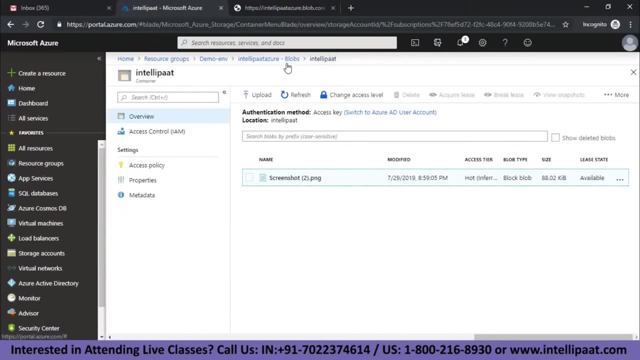 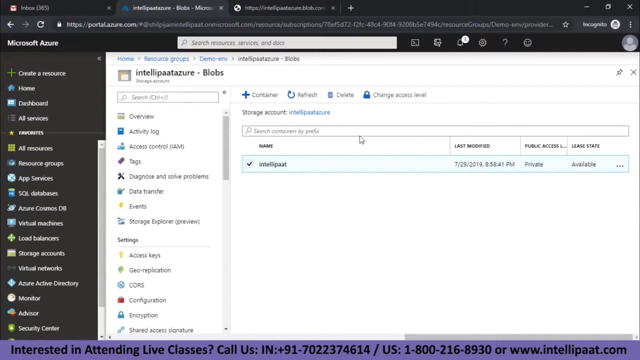 So right now it says the resource not found. the specified resource does not exist. Now why do you think this happened? This happened because we did not give access to the container for general public access Right. What do What does that mean? If I click on the container and I click on change access level, it's right now private. 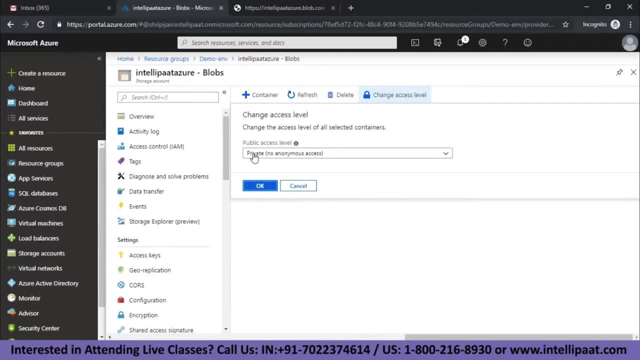 which means I can only access this blob through the Azure portal or through, you know, CLI or through some other way, But only that way would be working. Now, if I want anyone and anywhere who wants to access this file, I'll have to go ahead and choose anonymous read access for blobs only. 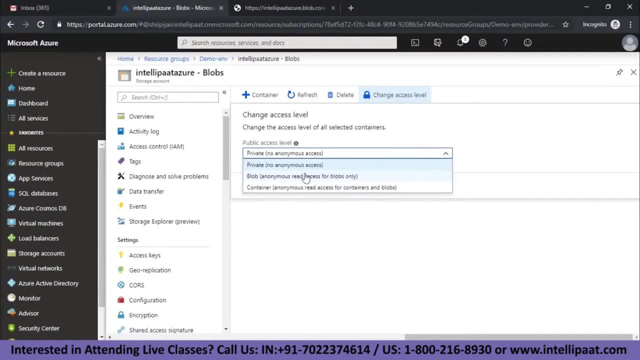 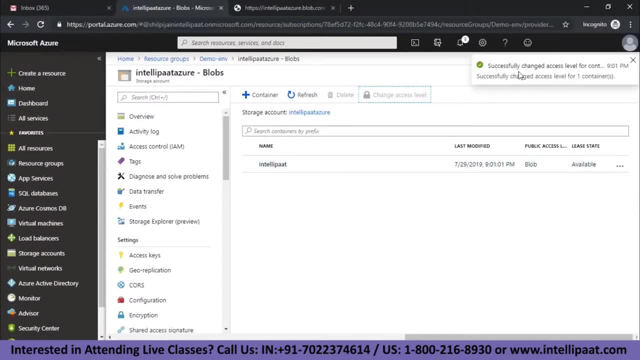 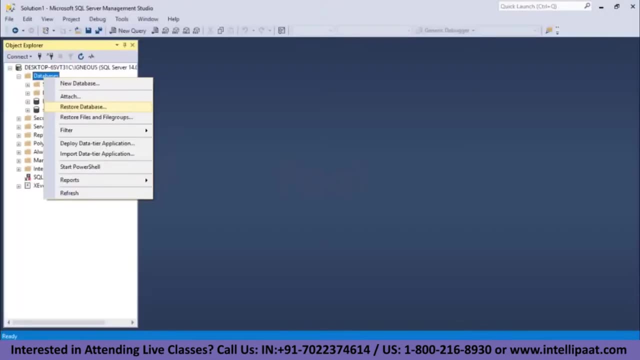 Okay. So when I do that, I just select a blob over here and I click on OK. Now the permissions for the files inside this container has changed. What does that mean? That basically means if I refresh this now, I would be able to see this image over here. 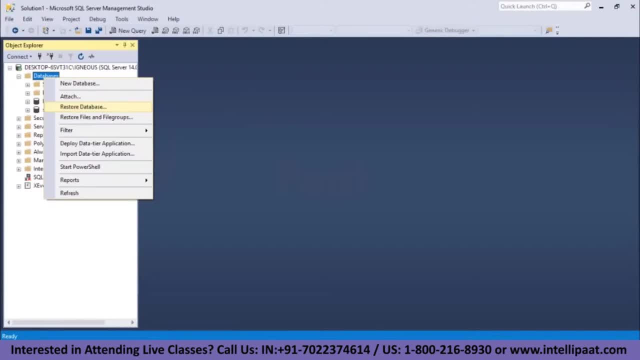 Right? Similarly, if this link is copied by you and based on a browser, you also would be able to see this particular image, Right? So, guys, this is what a blob storage is. You can use blob storage to dump data such as logs, such as images, such as videos, that 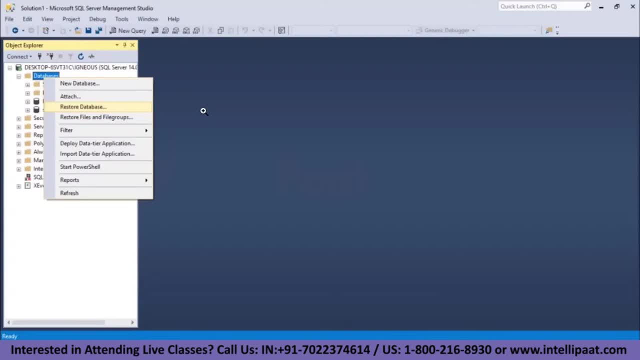 could be either private, if your application does not want to use it and you just want to keep there- keep it there for you know, just keeping it there- or what you can do is you can provide it a public read access on the blob level, that is, for all the files will. 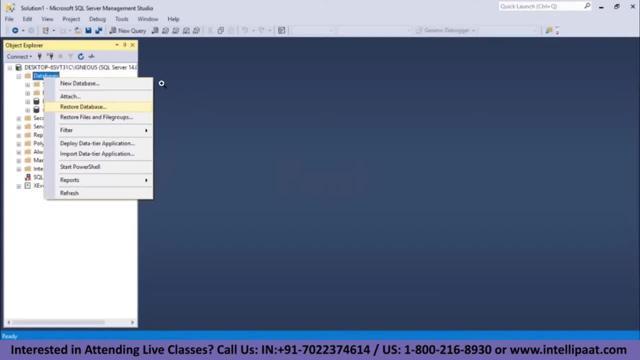 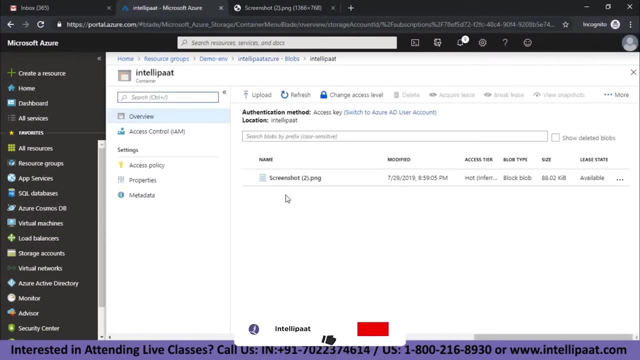 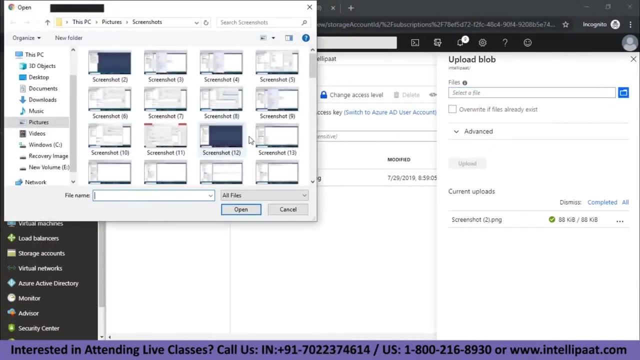 have public read access And those files will then be able to use by just going to their link. Let me upload one more file for you guys, so that you are clear with the concept of defining permissions. so I'll define the permissions on the container, so I don't have to do anything. 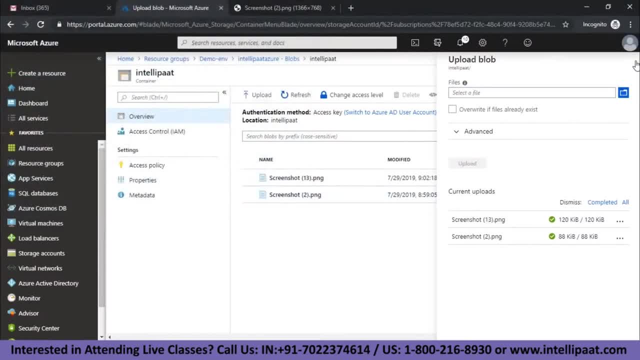 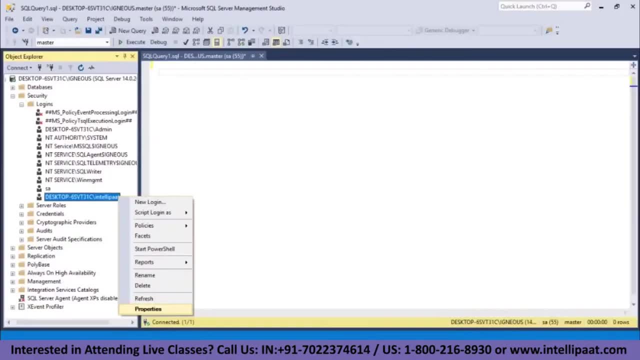 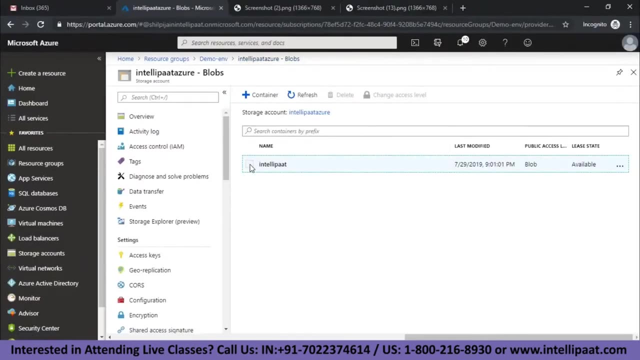 now I'll just upload the images, and this is a new image which has been uploaded. And now if I go inside the image and I copy the link and if I paste link over here, you can see I'm able to see this screenshot even here, right the moment I go out and I change the. 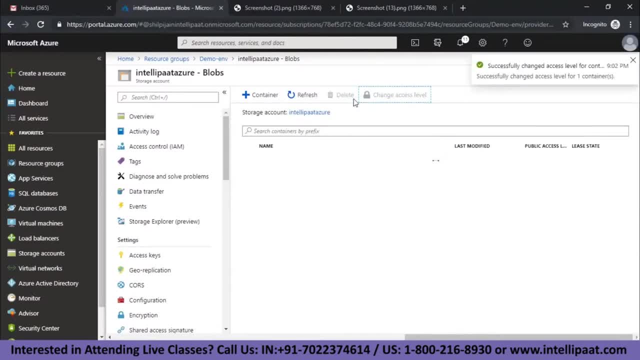 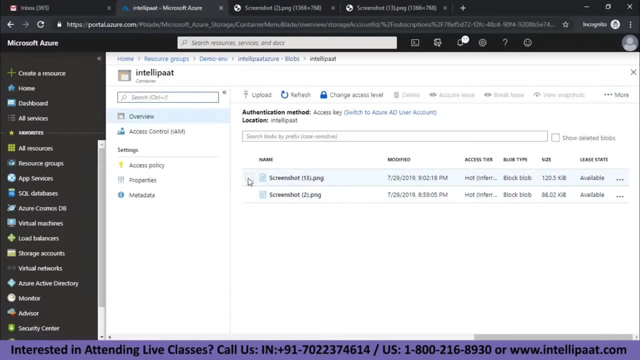 access level to private and I click on OK. Now if I refresh, OK, So it did not change the permissions of the files not visible. OK, So that basically took some time for the permission to get allocated on the container. which basically means like if I go out and if I change the access level again to 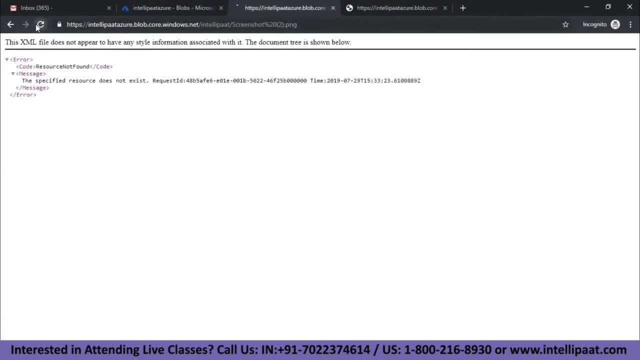 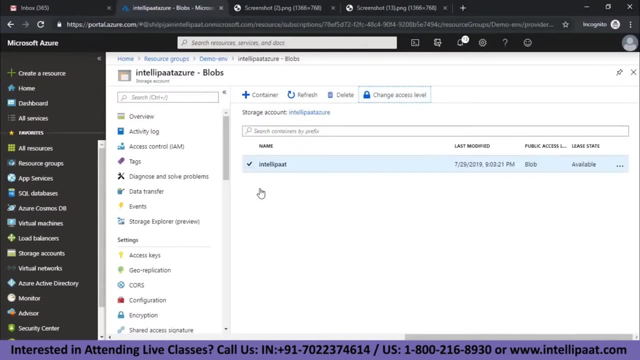 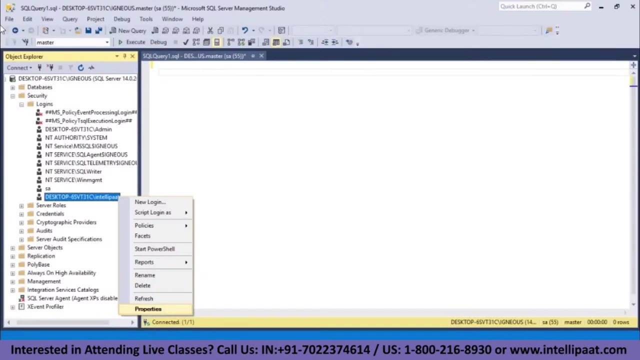 Blob. and if I refresh this files, yes, I'm able to see them right. And again, if I go out and if I change the access level to, let's say, private, again, and if I refresh, the first refresh, it is there. the second refresh, it is there. 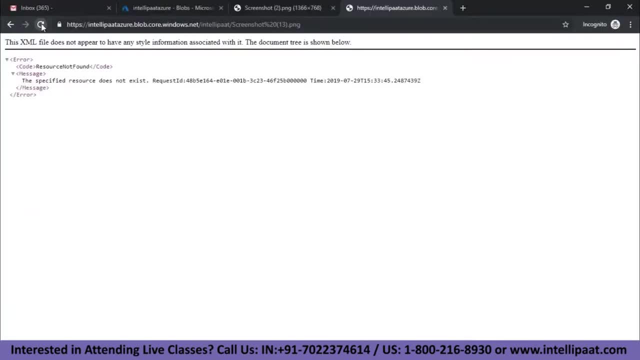 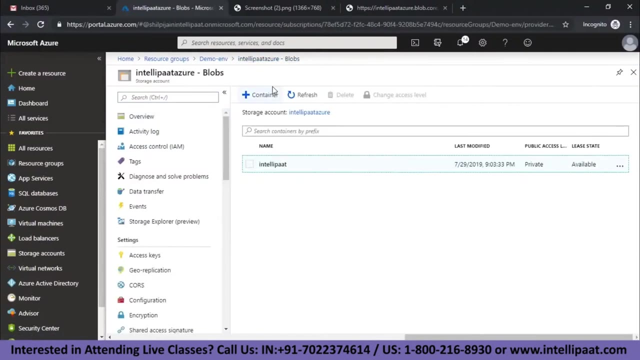 But if you wait for some time, like a minute or so, this access will basically be gone. As you can see, it now says resource not found right. So with the click of a button You can basically control all the files permissions which are there inside a container and grant. 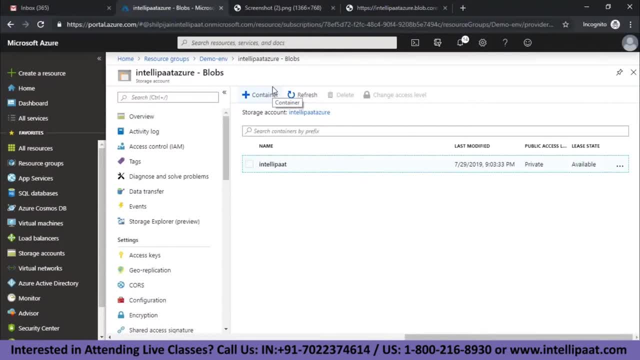 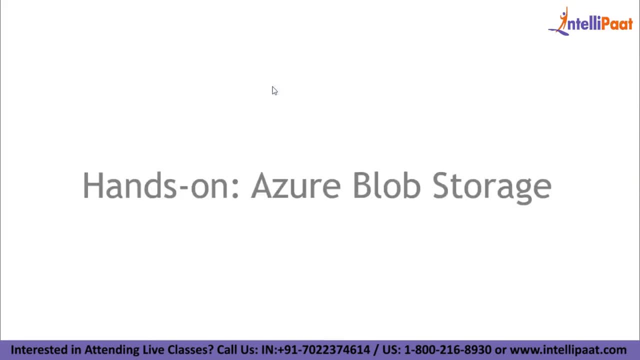 them, public or private, read access, right, guys? So guys, this was a brief demo about blob storage on Azure. Let us come back to our slides, right So, the guys? I hope now you're clear with what blob storage is. Now let's move forward and talk about our next set of services, which are the database. 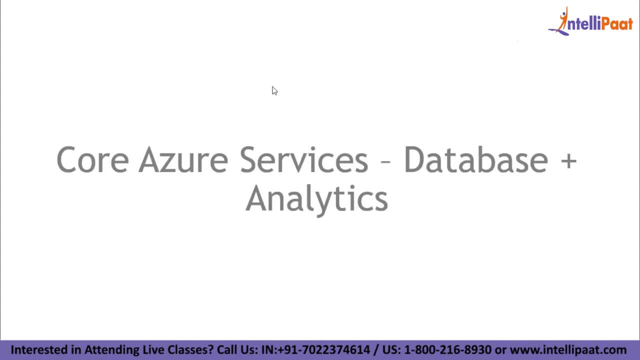 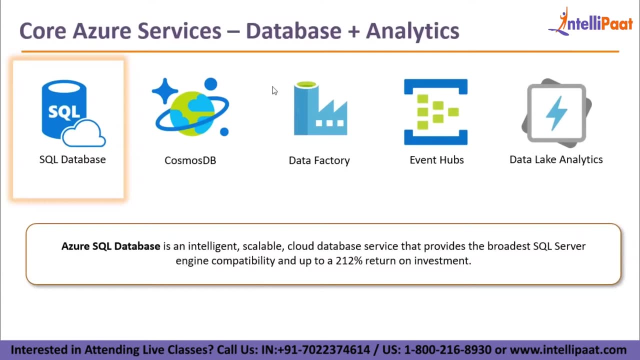 and the analytics service in Microsoft Azure. So let's move forward and talk about our next set of services, which are the database and the analytics service in Microsoft Azure, right? So basically, there are five core services that you should know of when you're dealing with Azure in terms of databases and analytics. 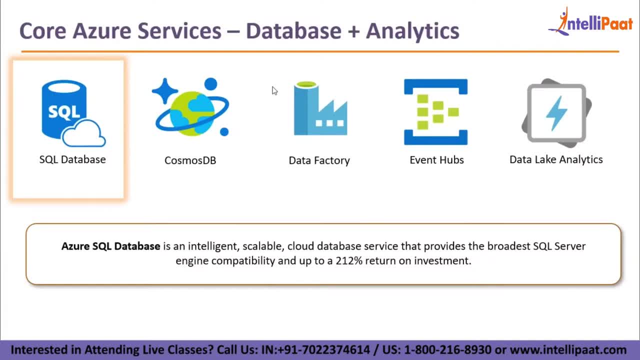 The first service is the SQL database service, which basically is a database as a service, right, You do not get an access to the operating system on which this database is installed, You basically get access to only the database And basically, if you remember what we have studied earlier, for a service which does not 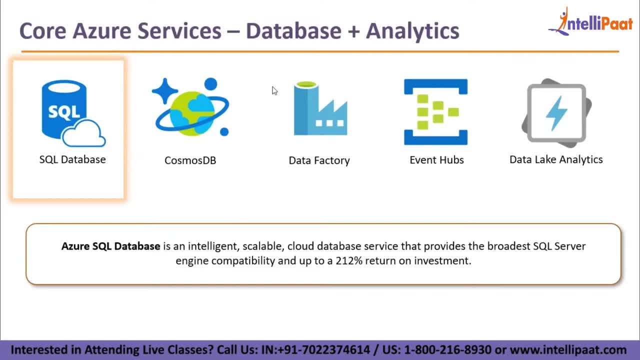 gives you access to the operating system but in turn gives you access to a platform kind of a thing where you can interact with the service and probably upload something onto the software being used is called platform as a service, So as your SQL database is basically a platform as a service, 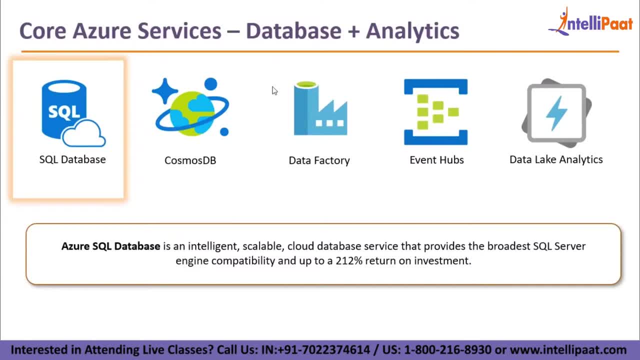 Which not only gives you the independence from the infrastructure side, but at the same time, it is highly scalable and it can provide you up to 212% of return on investment. That means that whatever money you are going to spend on Azure SQL database, the benefits. 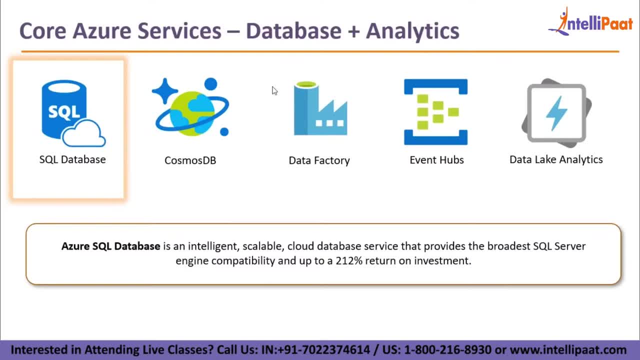 that it is going to provide you is going to give you back 212% of the money that you would be investing In using as your SQL database. isn't that interesting, right? So this was the first service among the database, and let analytic services in Azure, our next. 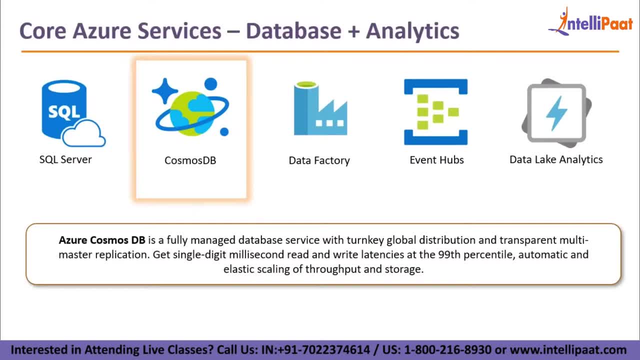 service is Cosmos DB. Now, guys, Cosmos DB is basically a fully managed database service, again just like SQL server, But in this case, what happens is your database is extremely highly available, Which means it is distributed throughout the world using Azure regions, and it is highly 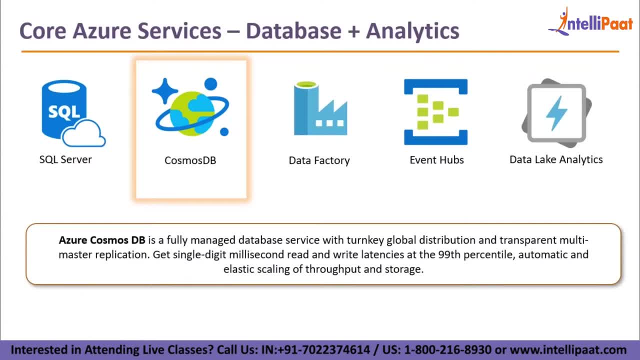 available, right? So basically, what happens is when you launch a Cosmos DB cluster, it distributes or it creates a replica of the database in multiple regions, as you specify, right. And the cool thing about Cosmos DB is whatever region you want to close or want to stop and 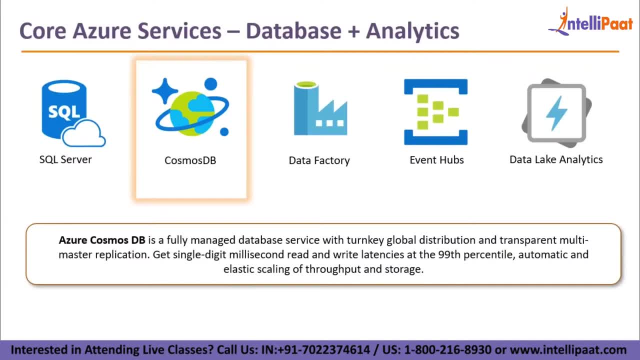 probably. If you want your database to be replicated in a particular region, you can do that with the click of a button. If you want it again in some other region, you can again do that with a click of button. So everything is fast, everything is at one. the whole control is at one central place. 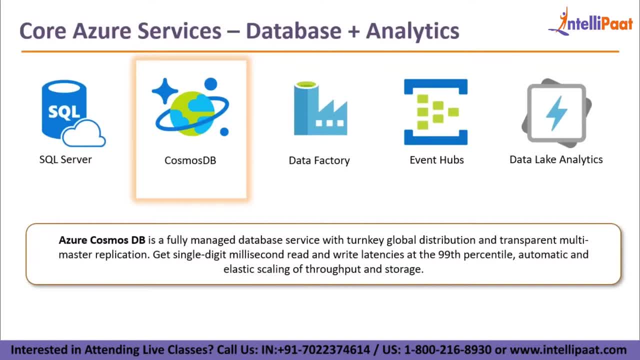 and you can replicate your database accordingly with that one platform or with one, that one Cosmos DB dashboard that you get right Now. again, you have multiple models that you can implement in Cosmos DB. For example, you can implement multi master replication or you can implement multi right. 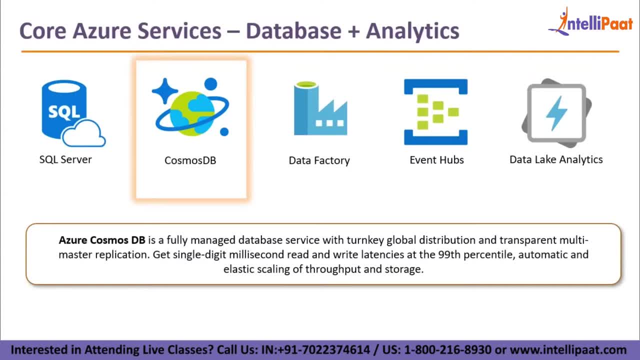 regions. replication, which basically means usually, when you have distributed database which is highly available, you have one region where all the rights take place. but the read can actually be done from any of the regions where the database has been distributed. But in case of Cosmos DB, you also have the option of configuring multi regions. 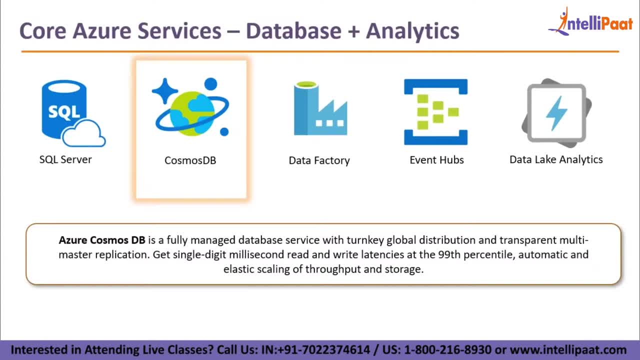 So basically, you can implement multi master replication or you can implement multi right regions, which basically means that, let's say, I want to, I'm in India and my and I'm a user who's using your application right Now. if I am using your application, probably the website is being served from the nearest. 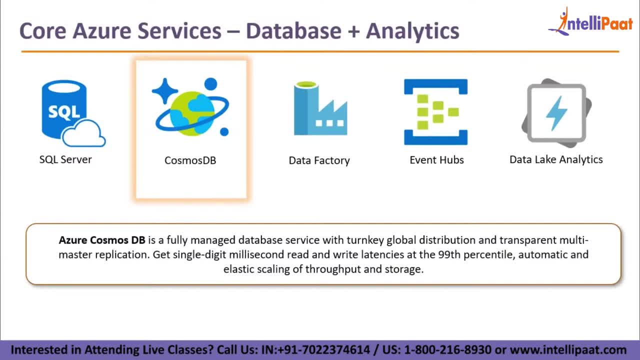 edge location of my location. for example, you must have enabled content delivery network on your website if you want to increase- or, sorry, decrease- the latency on your application right Now. to decrease the latency of your application, You've implemented CDN, so I am being served the website from the nearest location of my 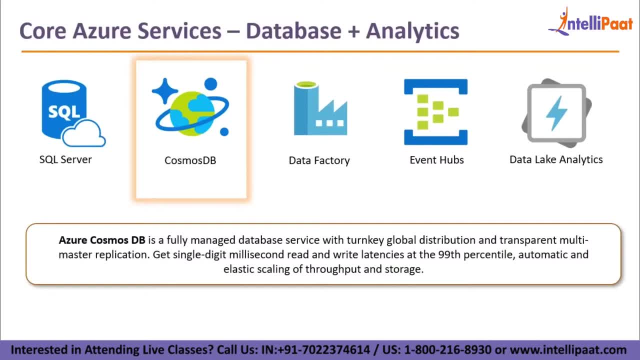 home, from where I'm accessing your application and, at the same time, the application itself is also accessing the database. right Now, imagine the website is fast, but the processing that it does, that is the data that it has to fetch from a particular database. it exists in altogether a different region, which is 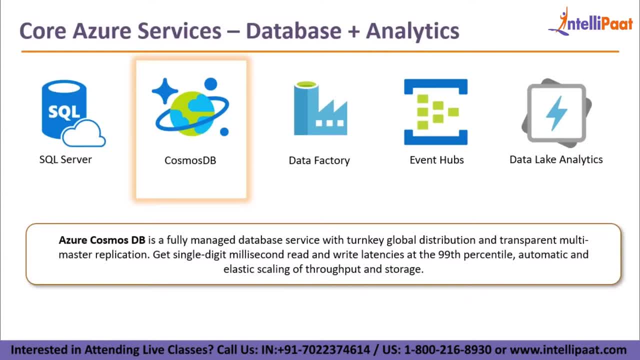 on the other part of the world right- on the- or on the other side of the world Right. That will again increase the latency of your application. so you don't only need your front end component to be highly distributed, you also need your back end and your database. 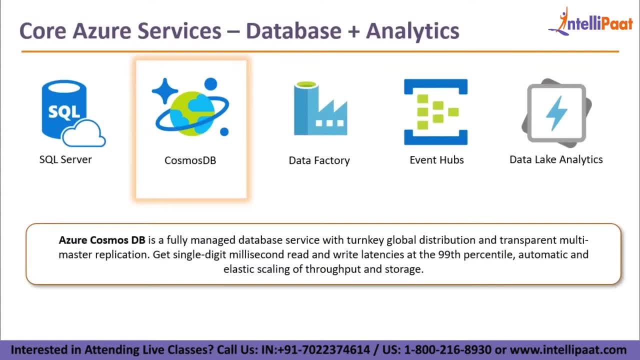 to be highly distributed and highly available. right, and that is the sole reason. when you are dealing with the audience, which is spread across the globe, you also have to take care that the processing that these, that each of these guys, are doing, would also be available to them in the lowest time possible. 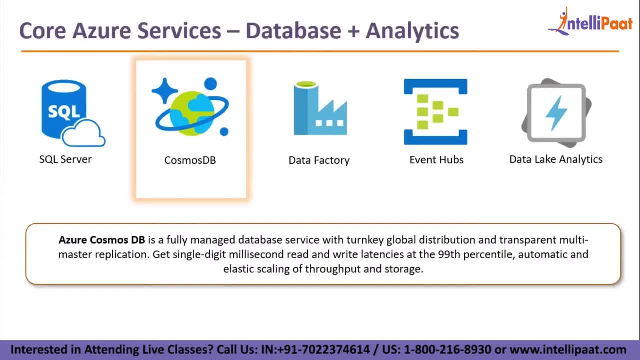 And for that what you have to do is the back end processors, or the back end servers, and the database servers also have to be near them so that whenever they're writing any information, that also information can be written faster. Now, if you have a right one and read anywhere kind of a distribution, in that case you will. 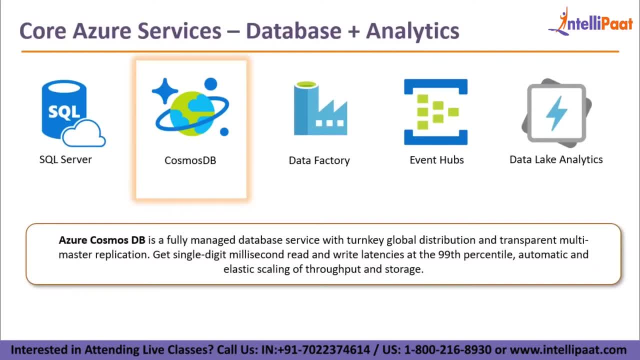 have to write at a central location. let's say the center location is the US and your databases. So basically the read replicas are actually distributed throughout the globe. What are read replicas? Read replicas are basically the copy of the central database from which you can read the 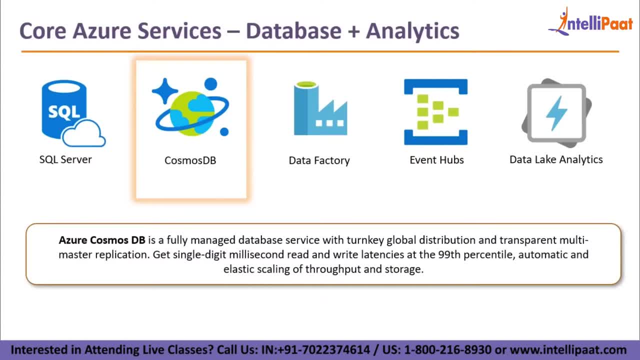 data and these read replicas basically get synced, or basically are synced with a central database, with. So whatever you write on the database is automatically and quickly replicated on the read replicas as well. So it's very fast, Right, So? So in terms of writing the data, you can get a very low latency, but in terms of writing, 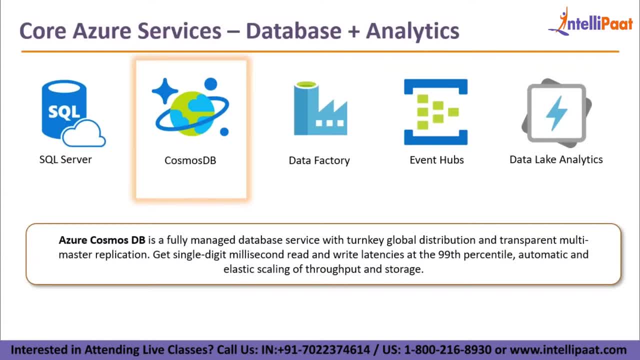 the data. if you want low latency as well, then you need to have multi write regions, and that is exactly what this feature is for. So, in a nutshell, Cosmos DB is basically a fully managed database service which provides you with a large scale deployment of databases throughout the globe, and it also gives you 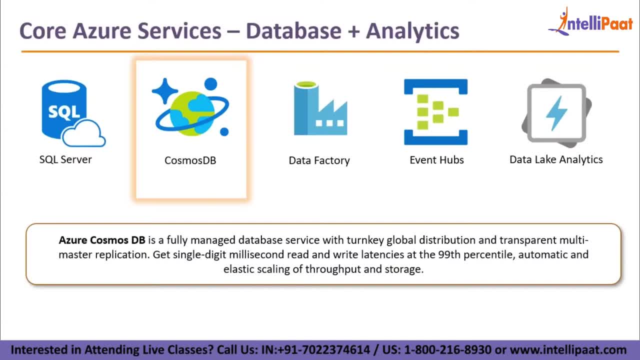 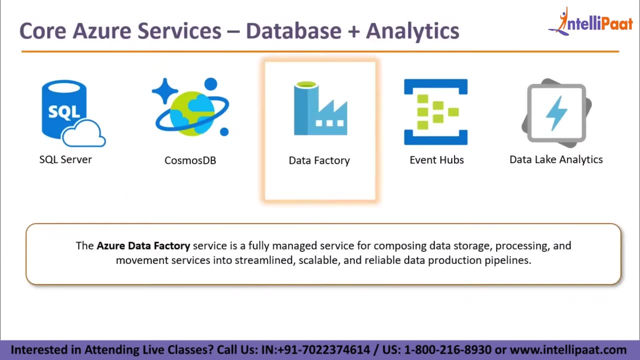 the option of Deleting, Deleting or replicating your database on a new region entirely with a single click of a button, Right? So that is what Cosmos DB is for you guys, Right? The next set of, or the next service that we have is the data factory service. 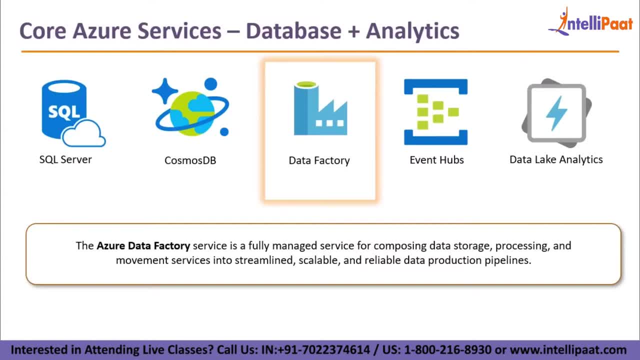 Now, what is the data factory service? It is basically an ETL service, which is an extract, transform and load service, which basically can take data from multiple sources and then transform the data according to what has been coded in the application, using a particular service which can be used in conjunction with. 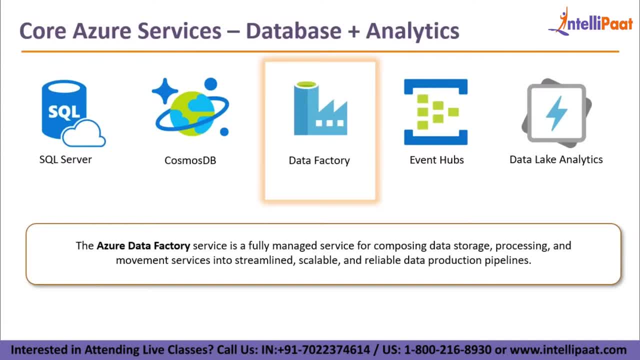 data factory and then load the resultant data into a BI service which can be used to analyze the data Right. So usually when you're doing this kind of an infra setup, you need a lot of planning, you need a lot of mediators between the technologies which are being integrated, for example the 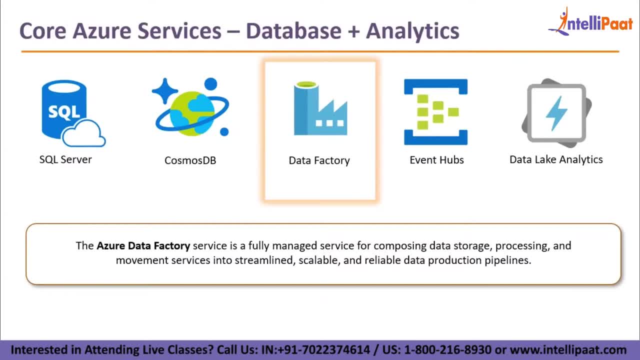 data can be coming from Multiple sources, such as social media websites, it can be coming from e-mails, it can be coming from chats, it can be coming from reviews. it could be coming from anything, right? So all these data sources are basically first of all aggregated and the data is first put. 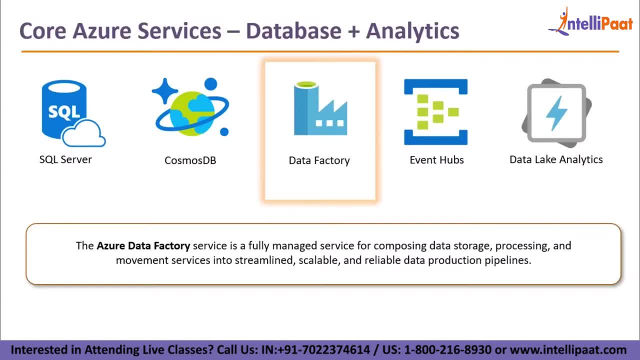 in the raw form in one particular place, Then what happens is according to the logic that you have specified for the transformation of this data. for example, you probably want to see the data in a particular view, So that basically means you would have to first transform this raw data that you've. 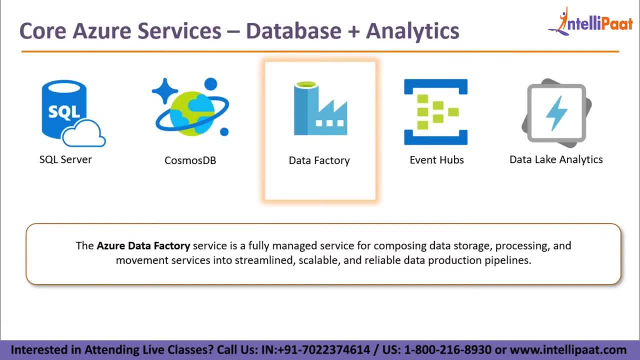 got from multiple sources into a structured format. So that is what transformation is. So, once you have the resultant data that you feel is the correct way of getting the data or representing the data, the next step that you need is, obviously, if there are a million. 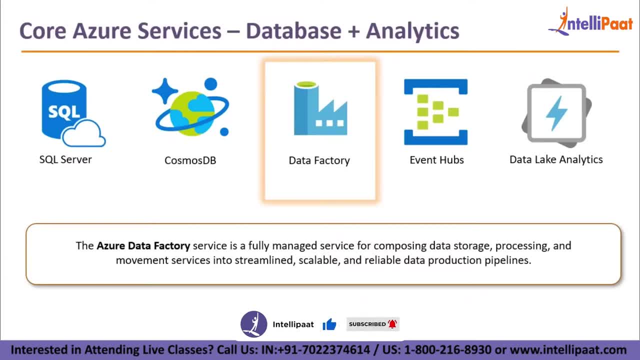 rows in your data set, you won't be able to find what you are actually looking for or, basically, it might take a lot of time, Right For you to analyze a million rows of data that you have just created. So what you can do is- or what? what the industry came up to this particular problem was that 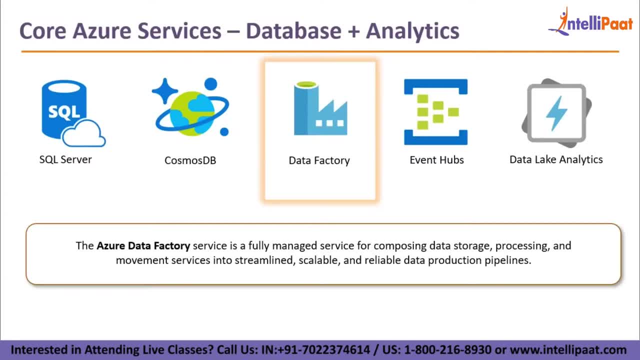 they created a business intelligence application. What is the business intelligence application? It takes in the data set and it quickly creates patterns. it creates, quickly creates graphs which can actually help you to better understand the data Right. So Data Factory also happens to have the integration capabilities. 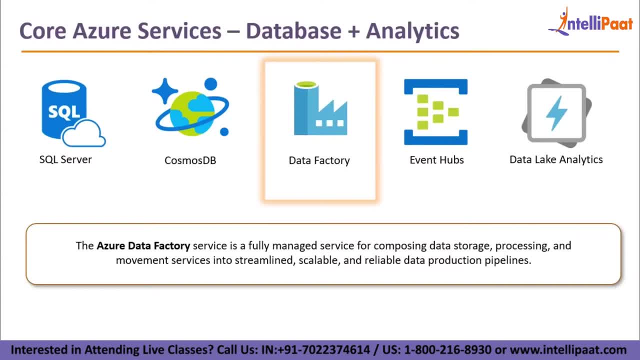 With a lot of BI tools. The most prominent one is Microsoft's own Power BI tool, but it also can integrate with Tableau and other BI systems Right. Similarly, it can be integrated with multiple data ingestion systems as well, So it's a total ETL system that you can deploy on Azure and connect your various sources. 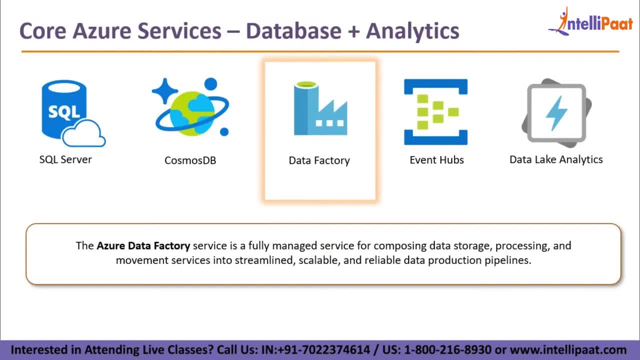 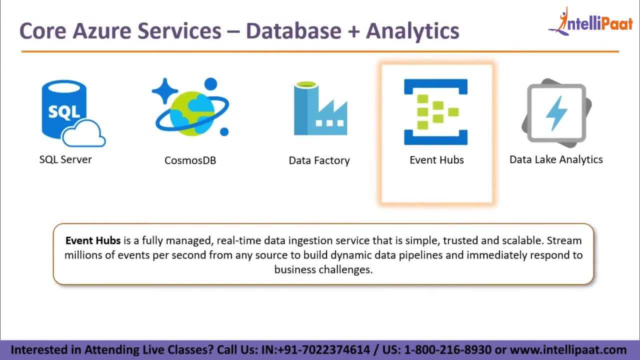 and outputs and get the resultant output. OK, OK, OK, So our next service is Event Hubs. Now, what is Event Hubs? Event Hubs is basically a place where you can again take in a lot of data. just like Data Factory, you can extract data from multiple sources. 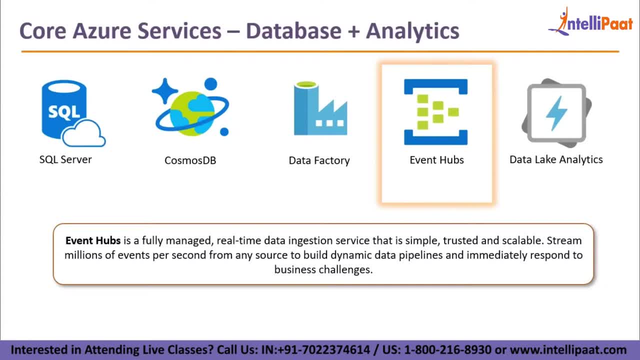 But in this case you're not actually extracting data, but the multiple sources from where the data is being generated. The data is being pushed onto Event Hubs. OK, So the data is pushed onto Event Hubs and the Event Hubs job is to process this data. 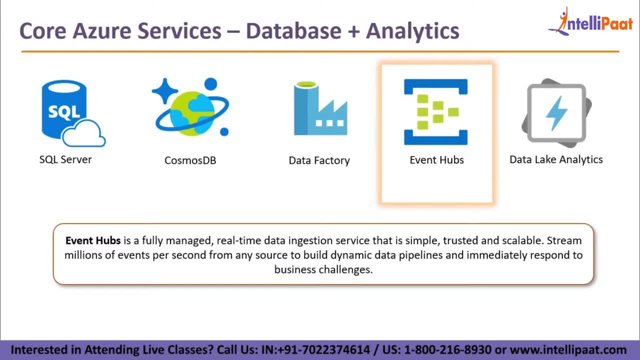 and see where this data has to go next. Right, For example, let's say the data is coming from a social media website. right, So you analyze. OK, so this data came from a social media website. it has to go to this particular service. This data is coming from this particular website. it has to go to X or Y particular service. 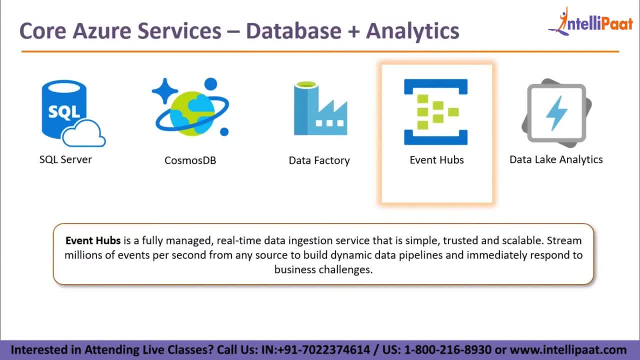 Similarly, you have millions and millions of data coming every second, or data packets coming every second. The sole job of Event Hubs is to basically analyze each packet and redirect it to the corresponding consumer of that packet Right. So this is what Event Hubs is for you. 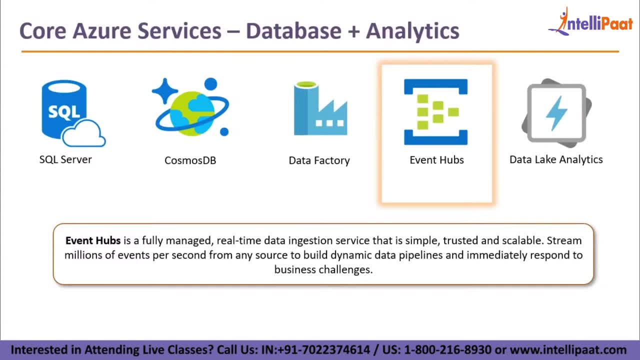 So this is done very fast. So the speeds claimed by Azure is around 1 Gbps. that, that is, it can process 1 GB of data per second. So the messages coming to Event Hubs can be processed that faster, And it Also does parallel computing of each data packet right. 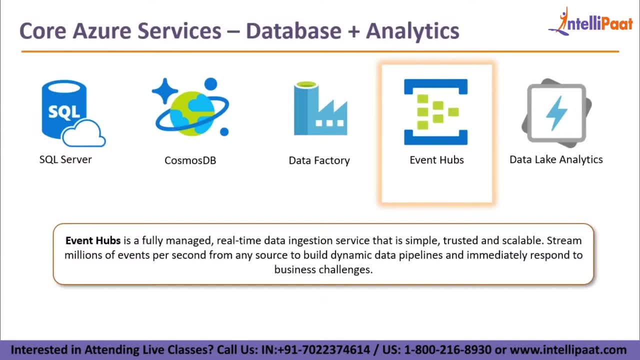 So this is how, or this is what Event Hubs is for guys. Now, obviously, Event Hubs cannot be just used alone, Right? You have to use it in conjunction with a host of applications. for example, the producers, that is, the data producing resources, have to first combine with an Event Hub and then 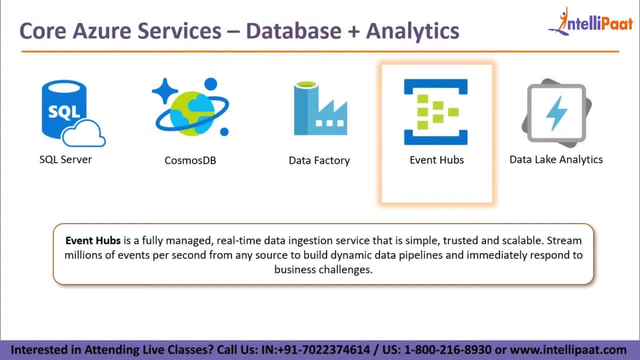 you have to define the rules in Event Hub as to what data goes where or what data goes to which consumer Right. Your consumers are defined on and they are basically connected to Event Hubs, right? So basically Event Hubs in the most basic sense is a single point of data ingestion. 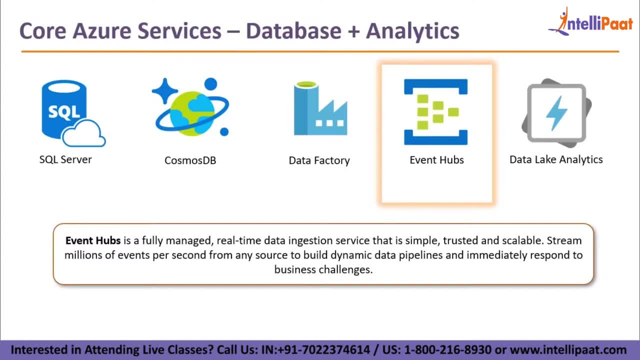 So you don't have to worry about where should I send my data? Send all your data to Event Hubs, and Event Hubs will decide where your data packet has to go, based on what rule you have defined inside that system. Okay, So guys, this is what Event Hubs is. 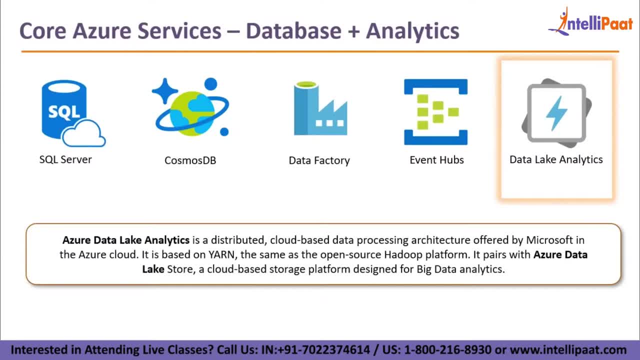 Our next service is Data Lake. Right, So we already saw what Data Lake is. So Data Lake is basically a storage for big data analytics, right? So Data Lake analytics is basically a distributed, cloud-based data processing infrastructure- right, So it is basically architected to perform data processing on the big data. I mean the 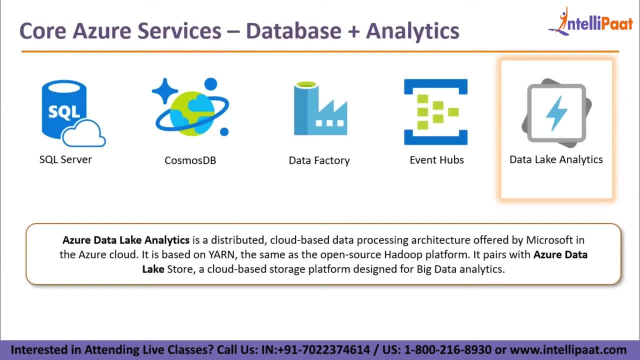 data that you stored on Data Lake is has to be processed by something right, and that processing can actually be done by Event Hubs, Data Lake analytics. So it is basically the architecture is based on Yarn, So Yarn is basically a component of the Hadoop ecosystem and it can all and basically pairs. 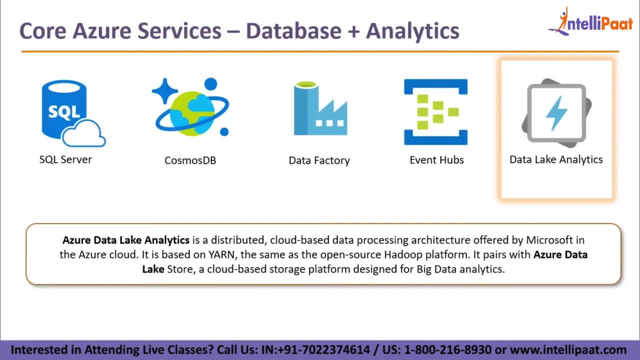 with the Azure Data Lake store or where, basically, we have stored all our data and can perform the analysis on the scale of big data. analysis, That is, big data is a huge amount of data with variety of data in it, right, so all the data has. 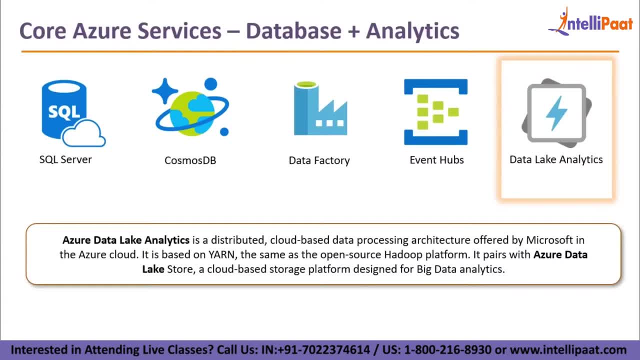 Mixed and matched fields right. the data is in the rawest form possible and the processing can be done only by using selected tools which can actually make that happen. If you use simple tools, or if you use traditional tools, the time taken by those tools to process 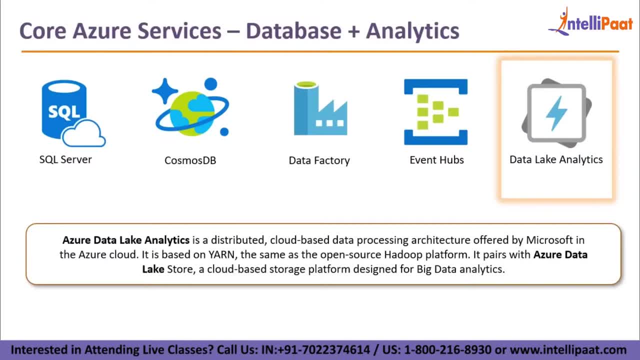 this amount of data will be huge, right, And that is why you need Hadoop tools to basically make this process faster, And Azure Has used the same technology that Hadoop uses and has made it even faster for you, right. So Data Lake analytics is used in big data analytics. it will basically use for processing. 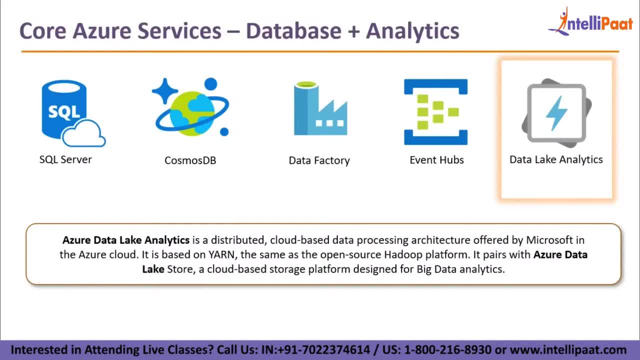 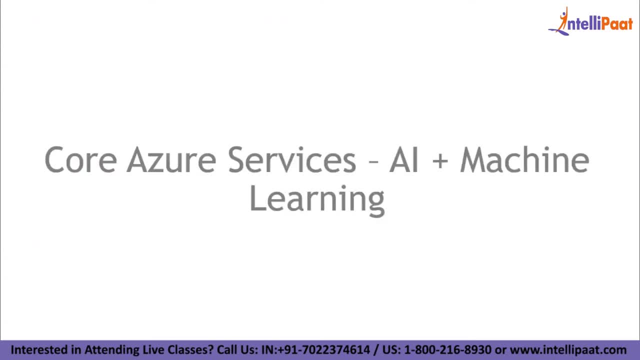 data, and what data the data which you store on Azure Data Lake store, right. So this is what Data Lake analytics is, guys: moving forward, guys. Now let's move on to our next domain, which is the AI and machine learning domain in Azure. All right guys. 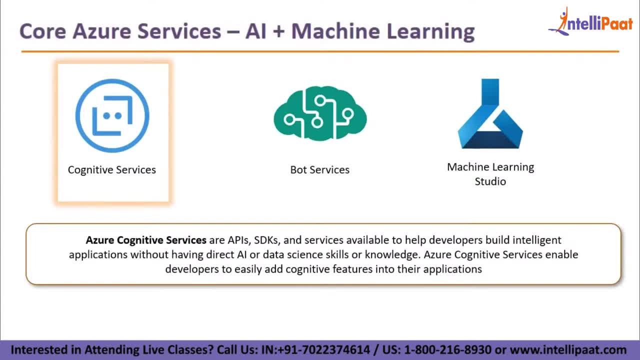 So in Azure, You basically have three core services in the AI and machine learning domain. the three core services are cognitive services, then you have bot services and then you have the awesome machine learning studio. So let's understand each of these services one by one. 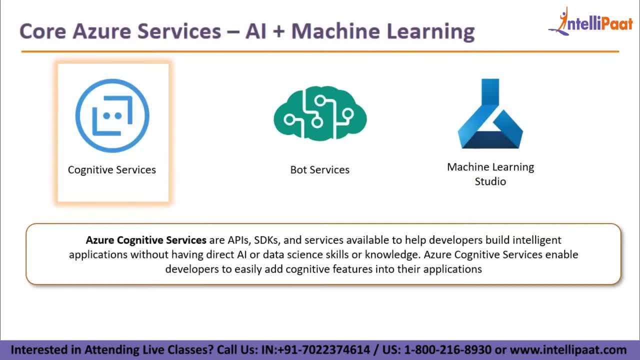 The first service is the cognitive services. now, what are cognitive services? cognitive services in Azure are basically APIs or SDKs, you know, which have been developed for a developer, which Are integrated in his application, and these APIs and SDKs basically interact with the machine learning models which have been created in Azure. right? 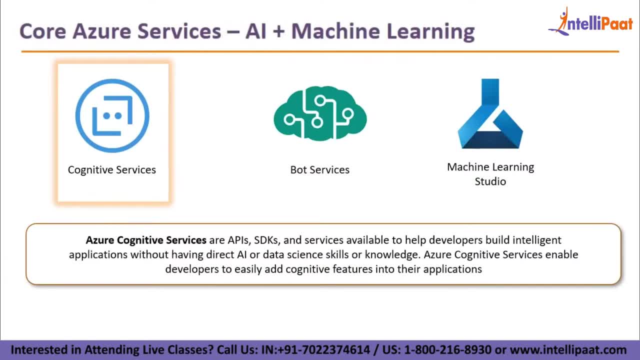 So cognitive services would include services like vision, which basically gives you image processing capabilities. It also has text analytics services, which can basically do natural language processing for you. So all these services, all these services in Azure, Are Use, And to use them you'll have to integrate them with your applications. 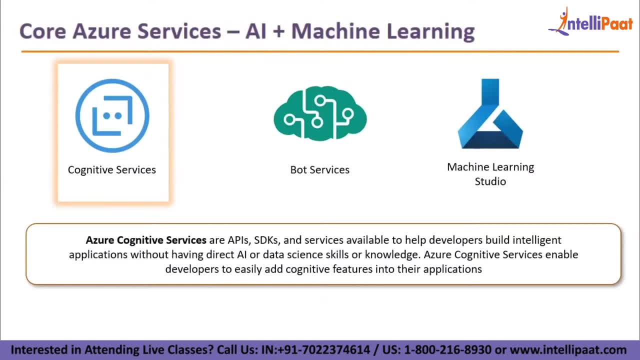 And those integration can happen with the help of APIs, can happen with the help of SDKs and once your application is integrated with these services, you're charged on the basis of the number of requests that you make to these particular service, for example, division service and the cognitive services offers. your is pretty awesome. any image study upload. 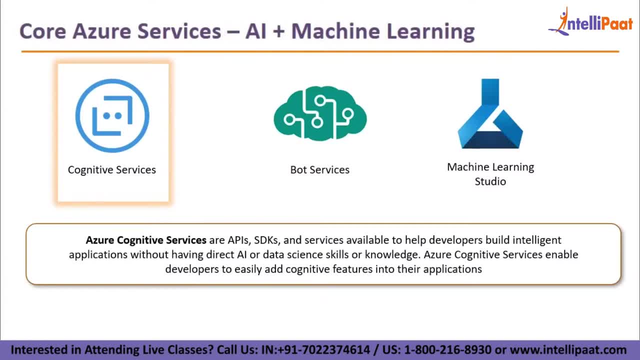 it will tell you Each In the image whatever is present. and how is that possible? basically, as your head process thousands and millions and even billions of images already, right. and they have trained the image processing machine learning model In a way that now it gives accurate results, right? so instead of creating your own machine, 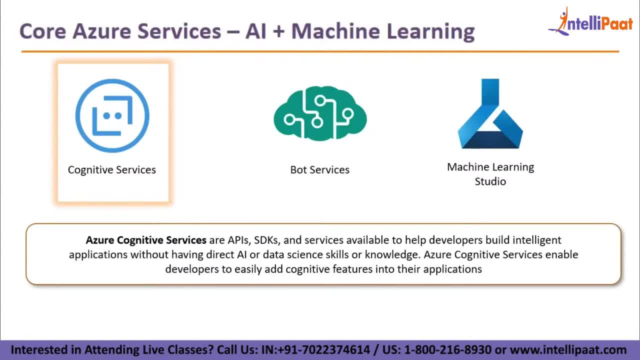 learning model for image processing. you can actually use the as yours machine learning model and you can get your work done. So it might have used deep learning, it might have used only machine learning, we do not know, but the results are very accurate And if you want to use AI and machine learning capabilities, offers your 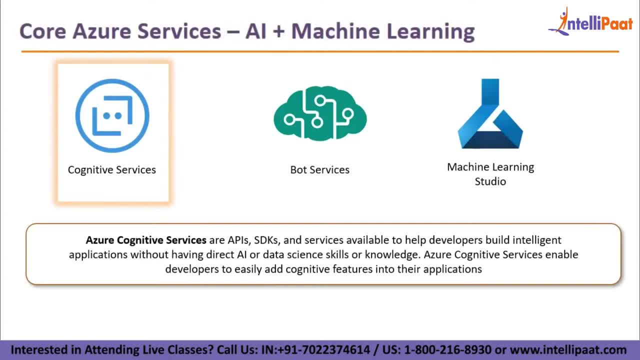 So the models which are trained by us, or, if you want to use them directly, you can actually use the cognitive services offers your and to integrate them with your applications. you have several APIs and SDKs availability. So this was about cognitive services, guys. Now there's a derivative of the cognitive services that does. your has launched. 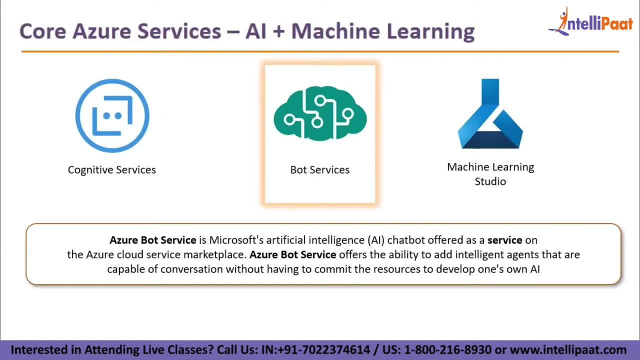 Which is basically called the bot service. Now, what is the bot service, guys? the bot service is basically a chat bot which has been developed by Azure, which is totally based on AI, and it basically makes uses of the natural language processing service or the capabilities which are basically there in the cognitive services. 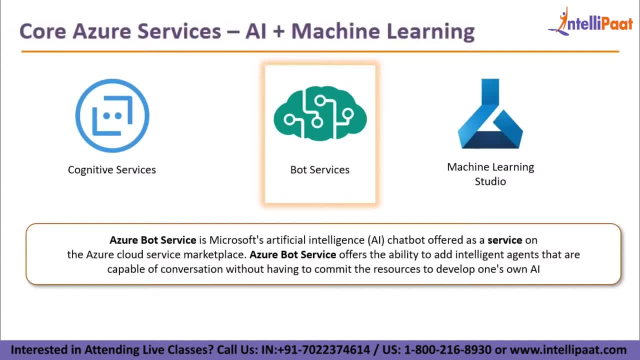 of Azure. It makes use of that right And it is very to the point and you don't have to train the model to become expert in the conversation You're having, but it can actually learn from every conversation that you have with the AI chat bot of Azure and you can actually tweak its settings so that it becomes custom. 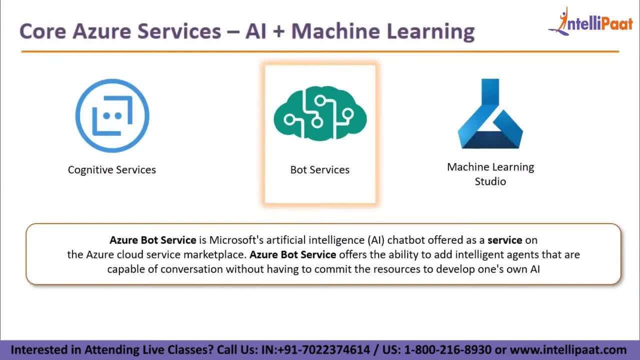 designed for you so that your customers get the right answer every time they ask a question from the bot service of Azure. So, in a nutshell, as your bot service is nothing but a chat bot service, it's a prebuilt chat bot service which you can integrate in your application and this chat bot service has 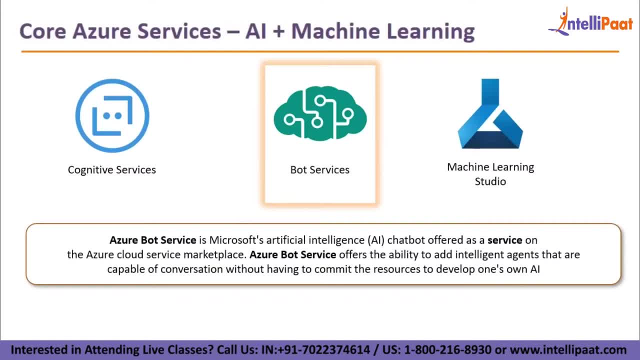 already been trained by us And it gives accurate answers to questions and but obviously your you will have to tweak it according to your applications. You'll have to do some settings so that it answers the correct way of answering. the answers would be according to you and according to your domain of application. 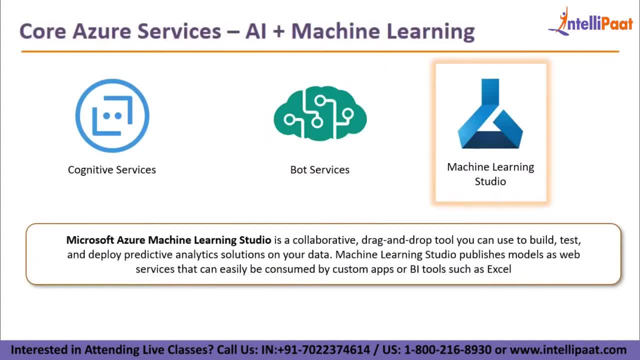 OK. so, guys, this was the bot services, and next set of service is the machine learning studio. Now, what is the machine learning studio, guys? It's basically a very simplified version of using machine learning. for example, the most simple language that I think for starting off in data science is R. right. 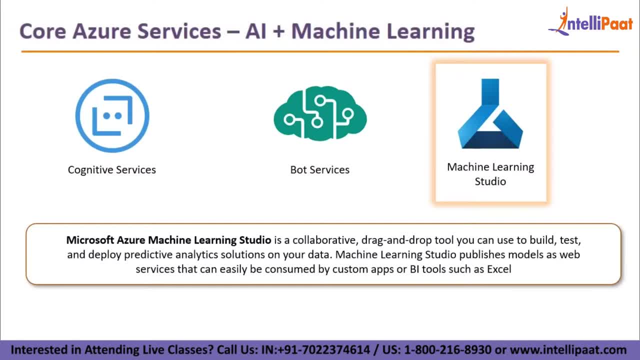 So, as a beginner, if you start using R or start learning R, you will have to spend some time to first of all understand the syntax, how it works, etc. And then you'll get a hang of how to create models, how to train them, how to test them. 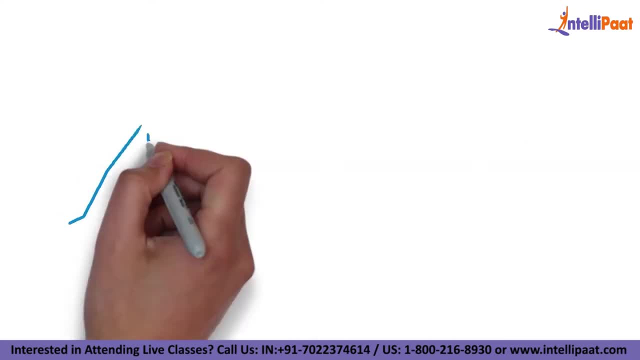 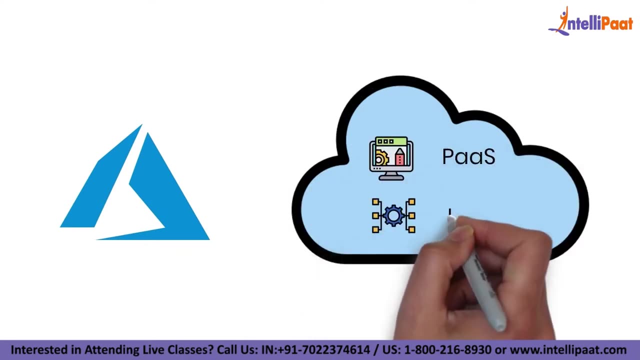 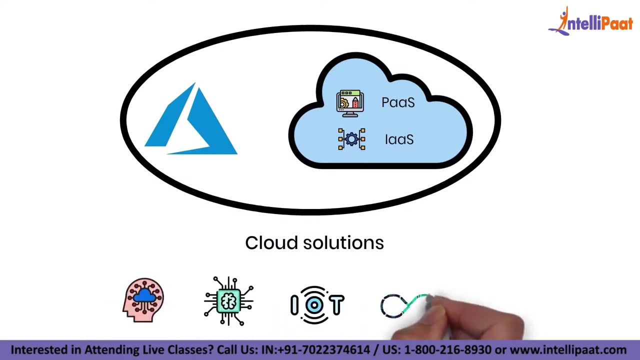 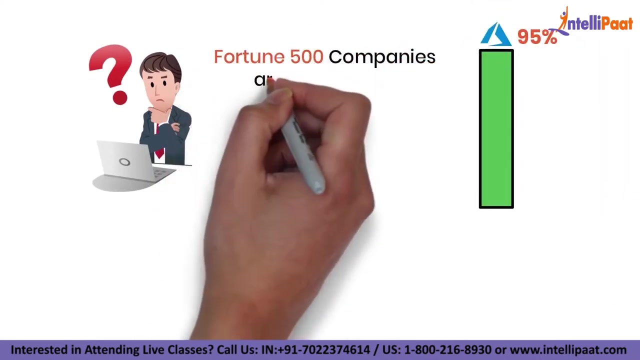 etc. So what is Microsoft Azure? Microsoft Azure is a cloud provider that provides various platform as a service and infrastructure as a service products. Azure has cloud solutions to all the infrastructural problems by providing services in various domains. Did you know that almost 95 percent of Fortune 500 companies are using Azure? 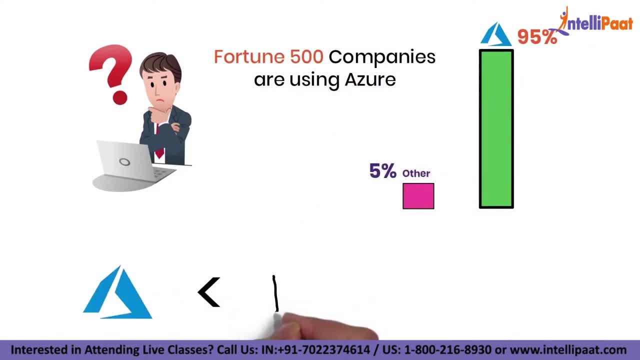 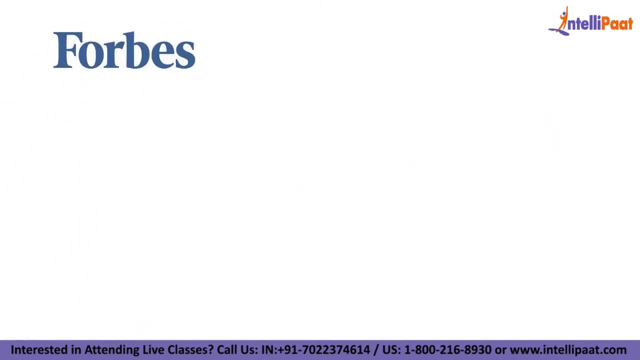 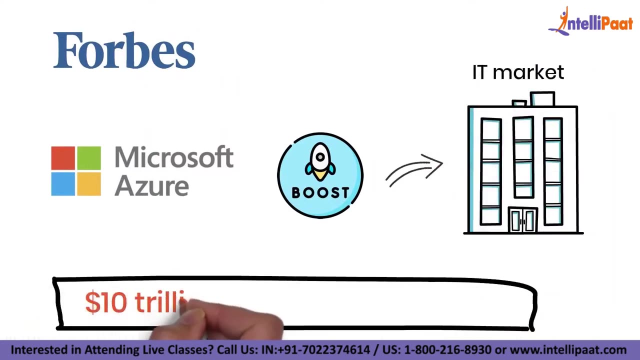 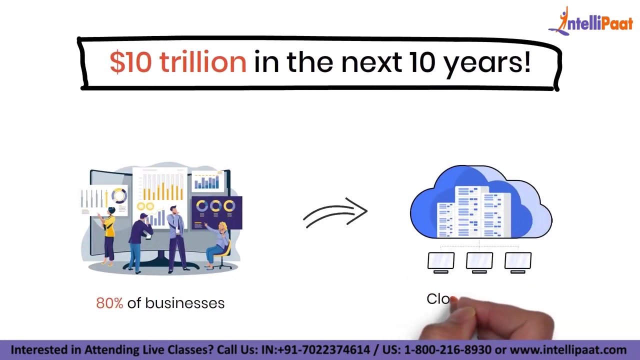 Also, it is five times cheaper than AWS in terms of Windows and SQL Server because they are also Microsoft products. Forbes say that Microsoft Azure is set to boost the size of the IT market by 10 trillion dollars in the next 10 years. As per predictions, 80 percent of the businesses will move their workload to cloud by 2025. 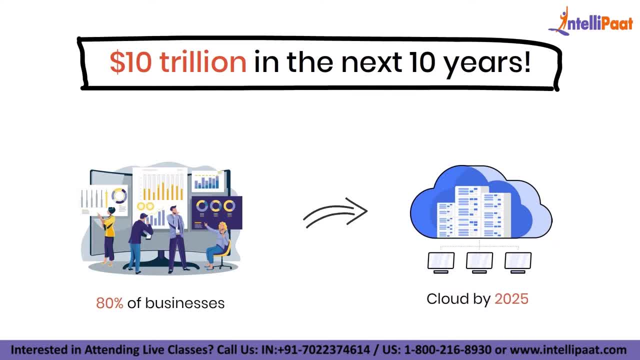 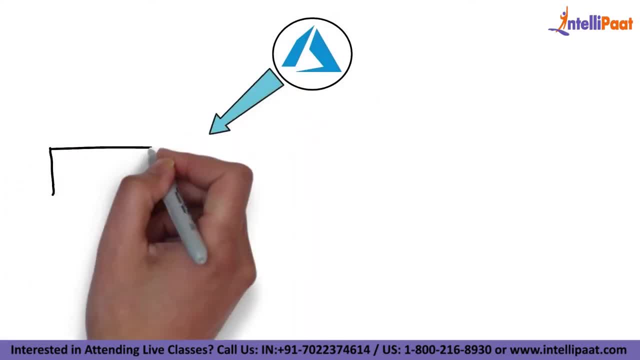 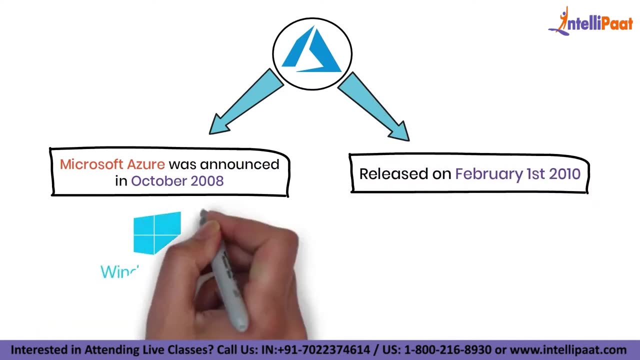 Thus making it a major career to consider transitioning to. For a better understanding of Azure, Let us start at the very beginning. Let us start at the very beginning. Microsoft Azure was announced in October 2008 and released on February 1, 2010 as Windows. 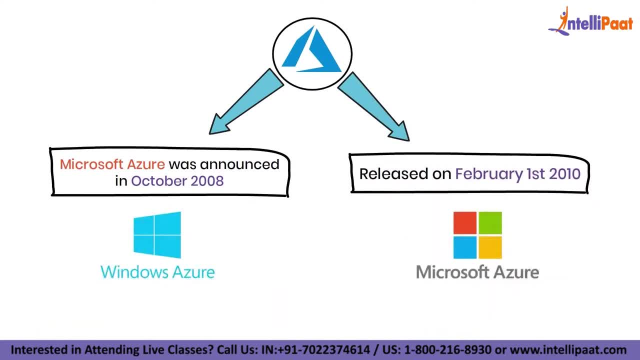 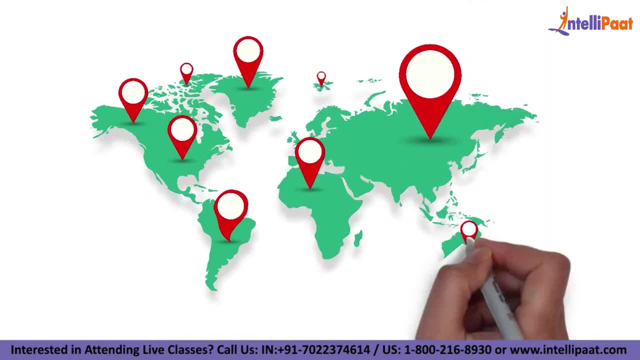 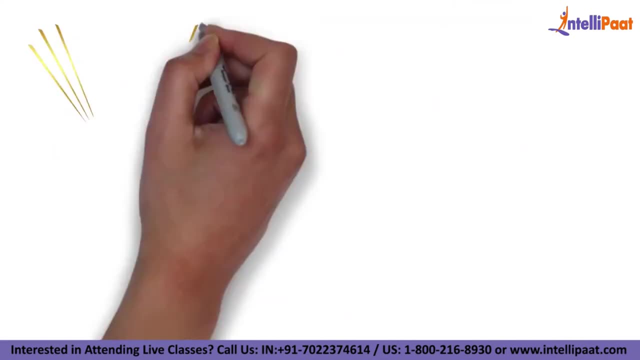 Azure, first and later named as Microsoft Azure on 25th March 2015.. In today's scenario, its reach is in 140 countries and is still expanding, which is pretty impeccable. In simpler terms, Microsoft Azure is a platform that enables users to use Azure. 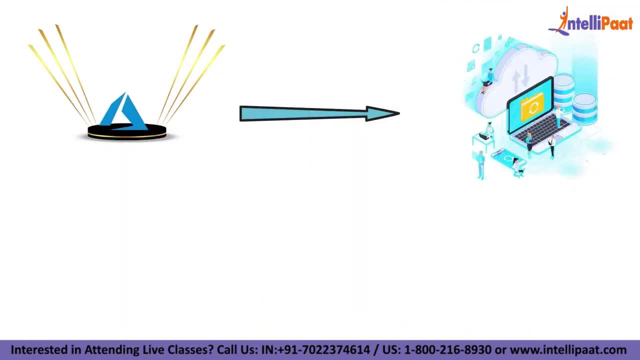 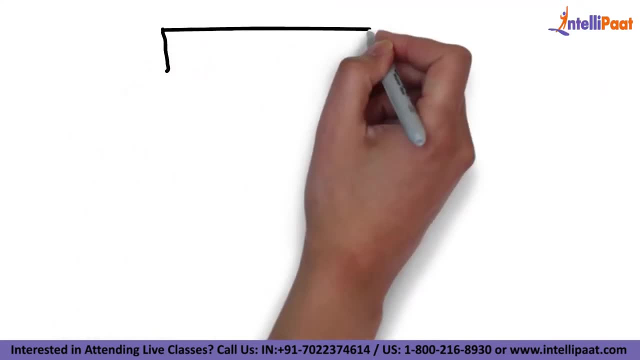 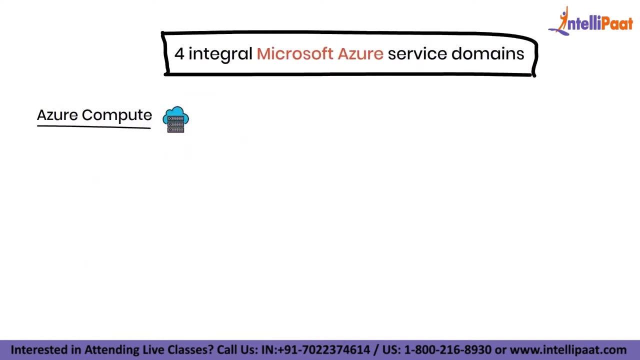 It enables users to engage in agile cloud computing and is designed for creating and managing apps through Microsoft's data center. Now there are four integral Microsoft Azure service domains. The first one is Azure Compute. Compute is the most integral domain in Azure as it brings everything together with Azure. 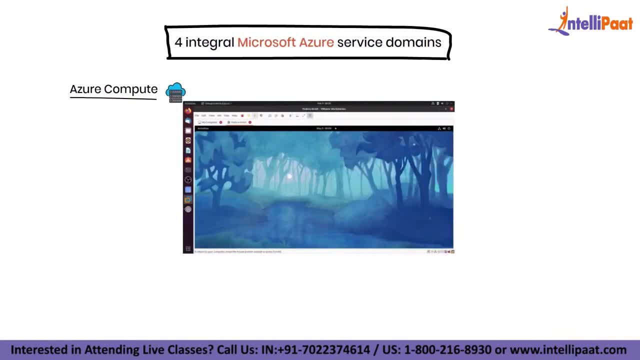 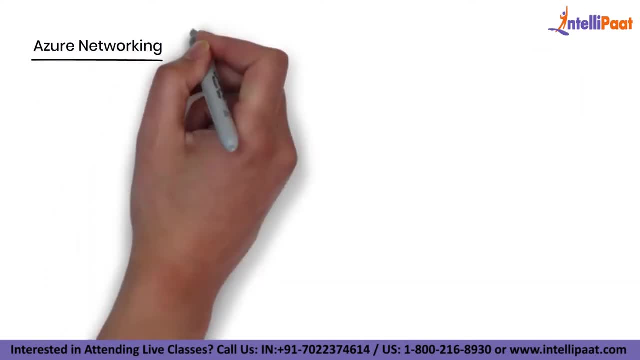 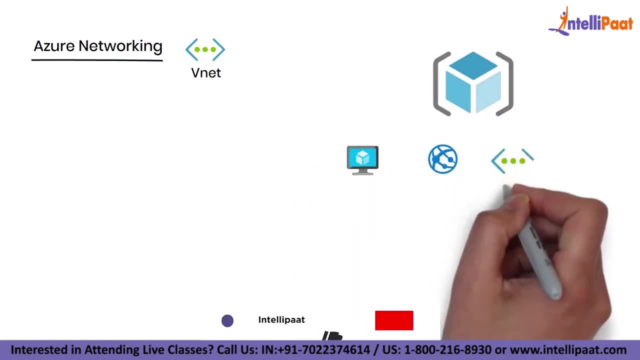 Second, we have Azure Networking Networks from the cloud networks. In azure, vnet is the networking tool that connects all azure resources together. These networking services allow enterprises to safely connect their on-premises services to the azure cloud. It is also used to manage Virtual private networks. 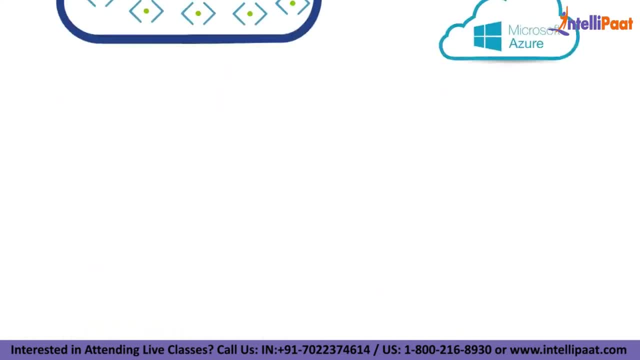 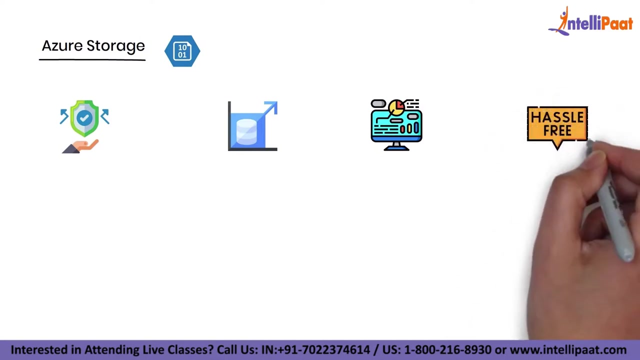 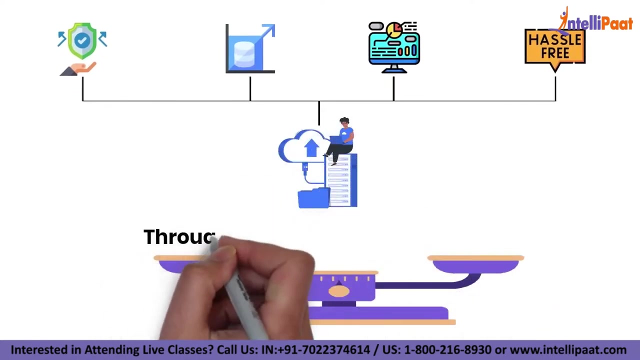 create multiple virtual networks on the cloud. the third one is azure storage. azure storage provides storage solutions that are more durable and large scale applications- data driven applications- can be built without any hassle. azure automatically scales the storage requirements according to the usage and it automatically balances throughput according to the connections. 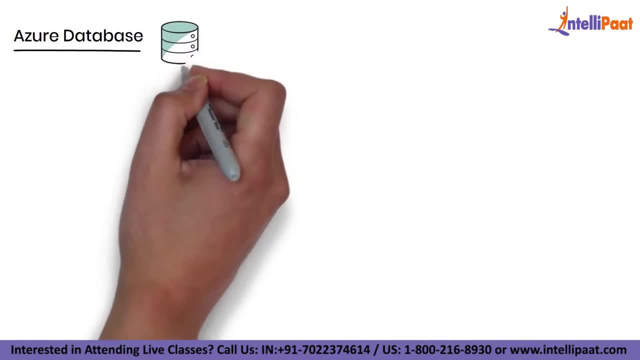 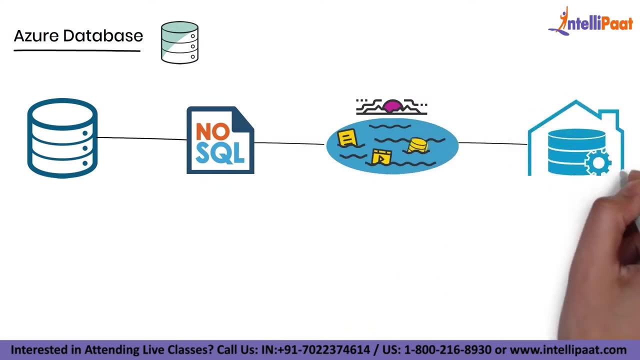 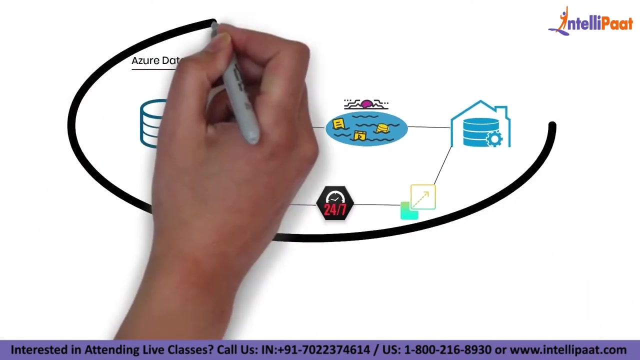 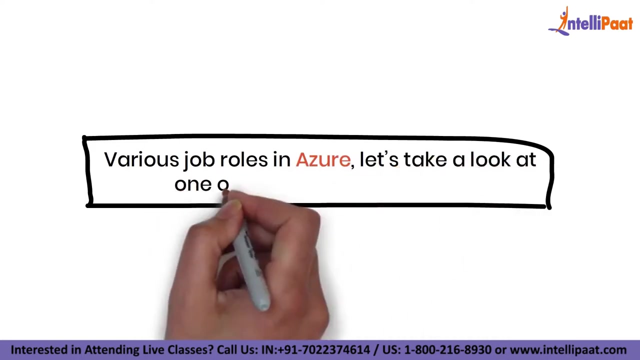 made, and the last one is azure database. azure provides relational databases, no sql databases, data lakes and data warehouses. it provides a scalable, high available and fault tolerant database server and lets you scale according to the incoming data. there are various job roles in azure. let's take a look at one of the most popular job roles as your developer. 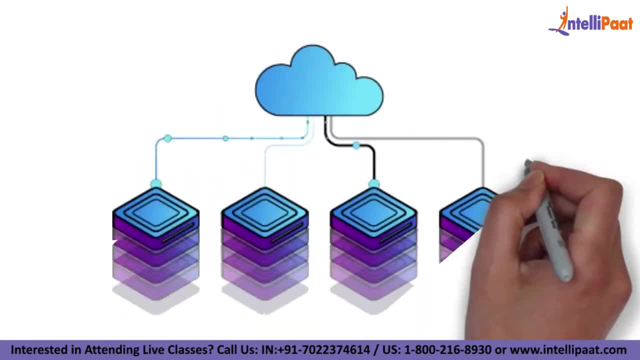 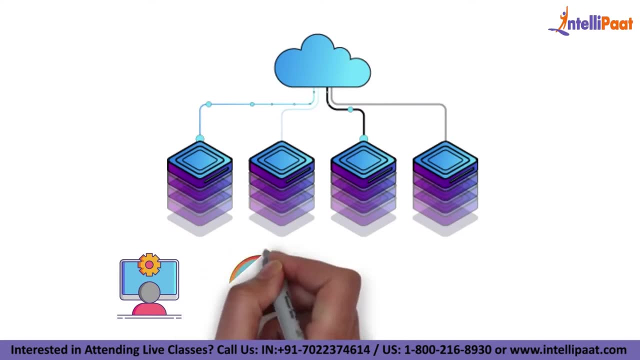 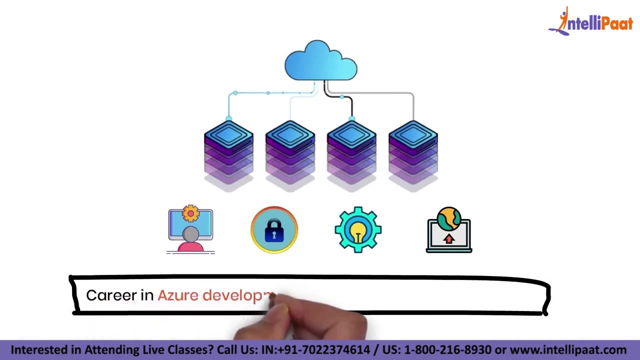 an azure developer is a cloud professional who creates cloud-based applications making use of the benefits of the cloud architecture. if you are proficient in testing, security, development and deployment, then a career in azure development is somewhere you will fit in well. the job includes responsibilities like testing of applications. 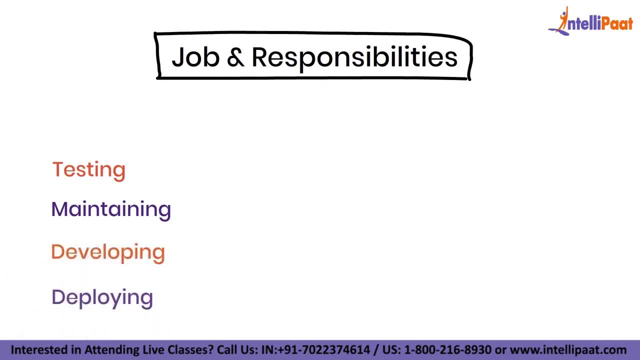 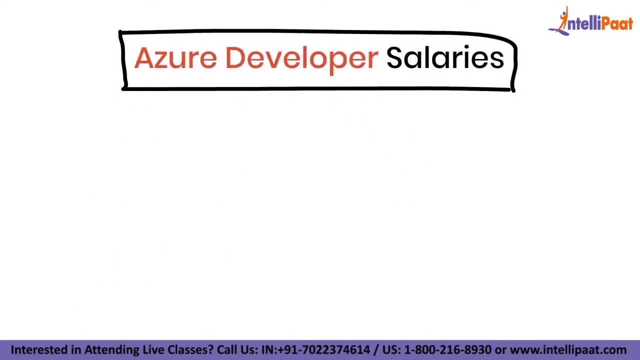 maintaining, developing and deploy them on azure. it also includes participating in all phases of development and having the ability to work side by side with cloud administrators, clients and cloud architects in united states. on average basis, an azure developer gets paid one thirty two thousand one forty eight dollars per annum. however, for an entry level developer, 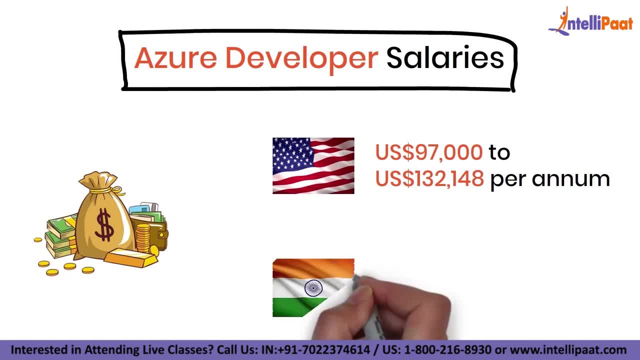 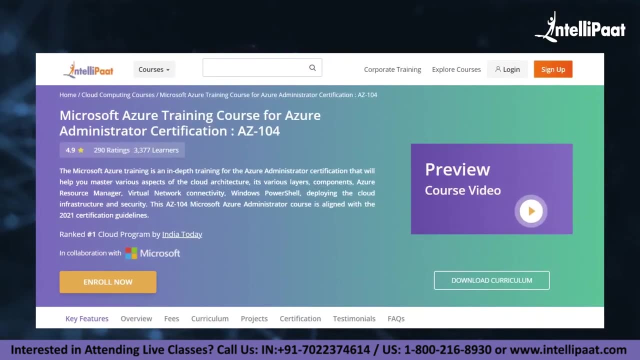 it's ninety seven thousand dollars, whereas in india the salary offered ranges from seven lakhs to twenty five lakhs per annum. just a quick info, guys: intellipaat provides microsoft azure certification training in partnership with microsoft, mentored by industry experts, the course link of which 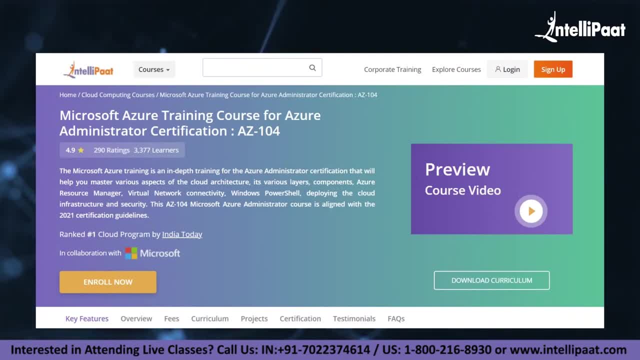 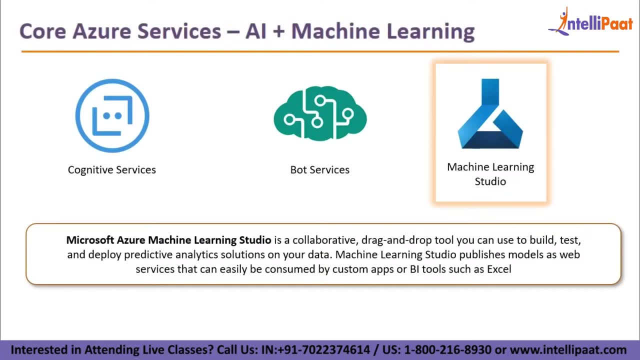 is given in the description below. now let's continue with the session. what machine learning studio says is: you do not have to learn any programming language. it has drag and drop interfaces. so all you have to know is data science, ai or machine learning conceptually. and if you 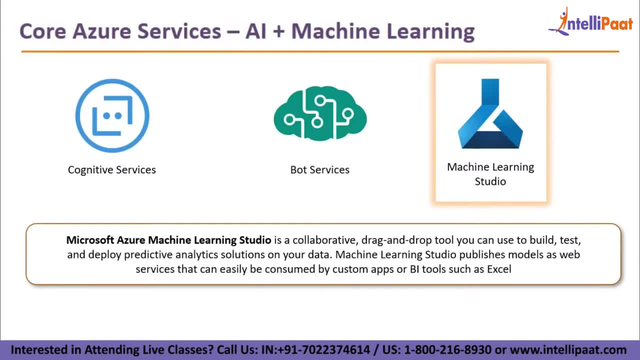 Dancing Drando. you have the principles of the data science, uh concepts, understood pretty well. what you can do is you can start off by creating your own machine learning model by just doing uh drag and drop from the ui of the azure machine learning studio and you'll be up. 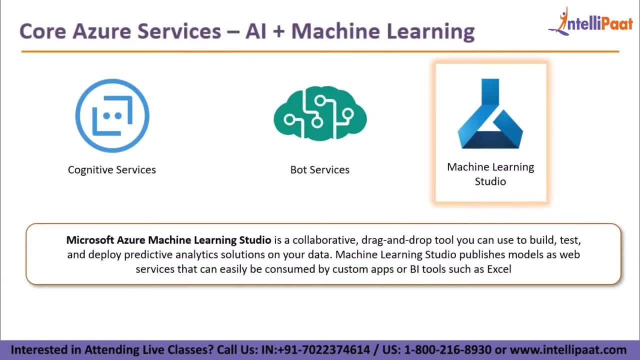 and ready with your first model in under five minutes, of course for a specific set of data set. obviously you will not be taking millions or billions of lines of data set, otherwise that will take a little more time. but yes, you can create your own machine learning model. 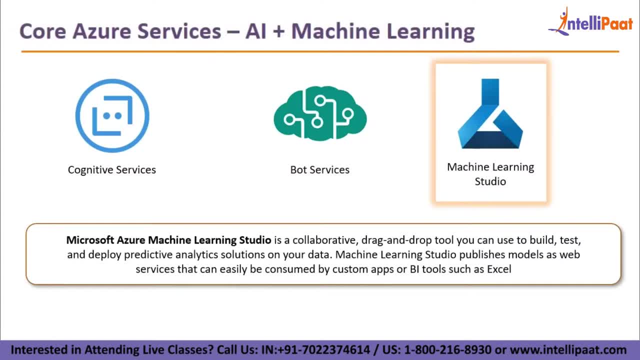 with Azure machine learning studio without knowing any programming language. right. so that is the power of machine learning studio, and the most coolest feature of it is it has a drag and drop user interface. so everything is drag and drop. you just drag and drop whatever you need, whatever data set you need, whatever algorithm you want to implement whatever thresholds you 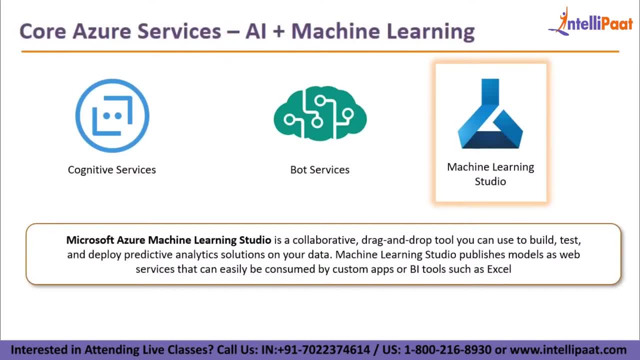 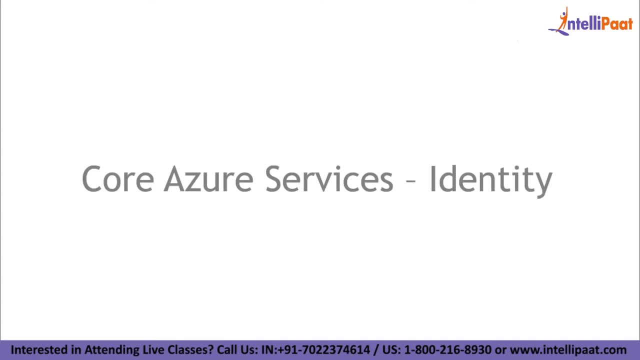 want to implement. just drag and drop everything and it will work like a charm, okay, so, guys, this was the machine learning studio application for you. the next set of services that we are going to discuss, guys, are the identity services in azure. all right, guys, so now let's go ahead and 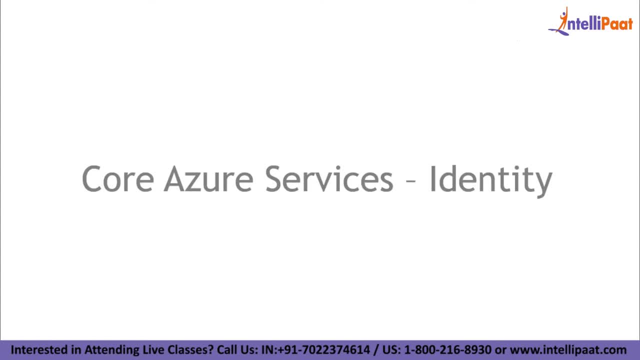 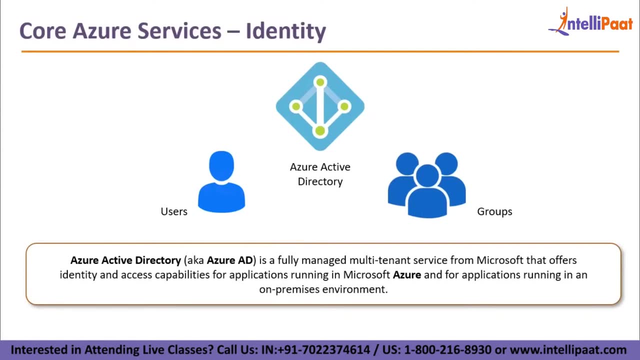 understand the core azure services in the identity domain, right? so, guys, the probably the most important service when you're dealing with identity in azure is azure active directly. now, what do you mean by identity? identity basically means when you want to give a particular person some access to a particular resource that is being used on azure cloud, right? so azure active. 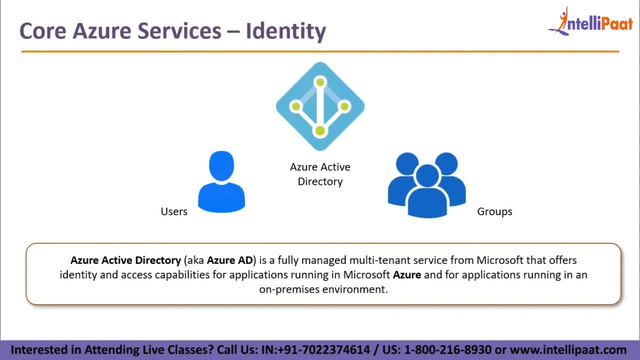 directory is basically a fully managed multi-tenant service from microsoft that basically offers identity and access to particular users in your organization. now, if you're acquainted with how a microsoft windows server works, you would know that there is a server active directory as well. right, there's a microsoft server active directory as well, in which you can specify for your on-premise 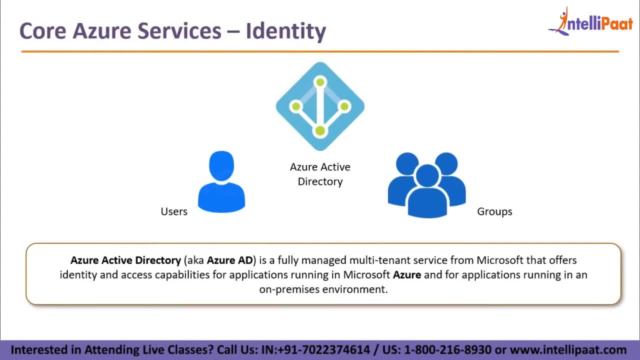 applications which users have access to what extent. right, for example, people can just have read access, or some people can have read and write access, or some people can even have admin and access to a particular application. right, and the most important part about azure active directory is that it can integrate with your on-premise server active. 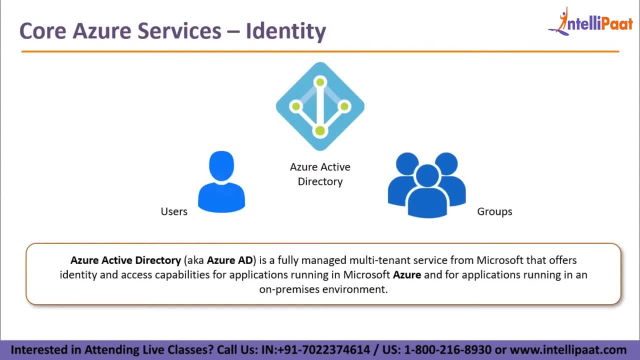 directory and can also authenticate people who are there on the on-premise infrastructure and want to use the on-premise resources. like or on-premise softwares can also be authenticated using azure active directory and if those on-premise users then you want to use resources on azure, that also will be. 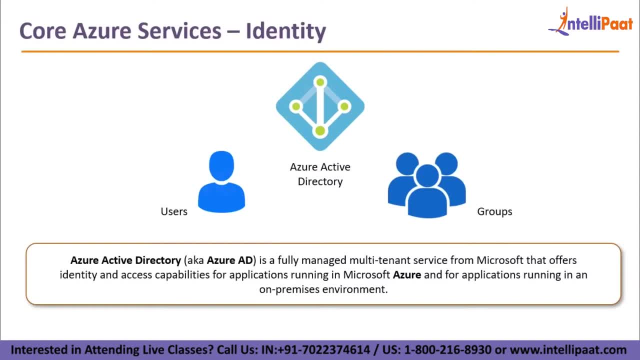 authenticated using azure active directory right now. how does all this works? so it's a very simple concept, guys, what you can do. you can actually add users in azure act directory right now. you can add individual users and you can assign individual roles to each users. for example, if there is a 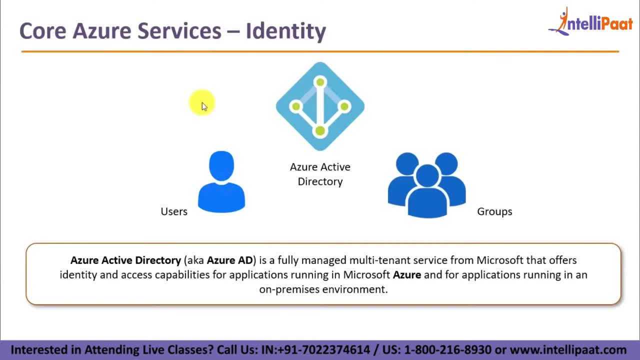 sas application which you have deployed on microsoft azure. giving access to that particular sas application to a particular user would be possible by just adding a user and giving him the access of that that sas application. right, and you can also do a mass allocation of a particular permission. for example, let's say you want to give administrator. 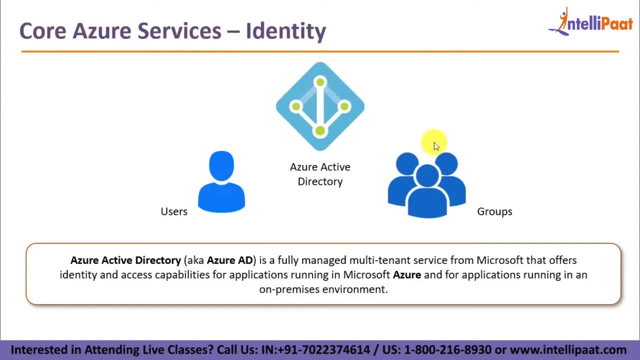 privileges to a set of people. now how would you give that so? one way is: whenever there is a person who comes into a company whom you think can be given admin access, you will add his user and provide him the admin access. or what you can do is you can actually define a group on which you have specified admin. 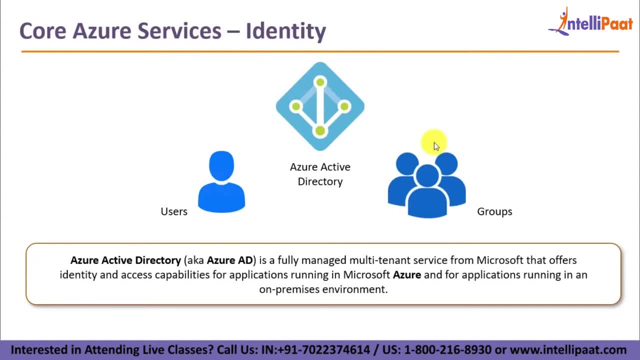 resources, also admin privileges, and whoever users will be added to this particular group will get those permissions or will get those privileges automatically, right? so in this case, what you will be doing is, whoever is coming into the organization, you are just adding him to the group and the permissions inheritance takes place automatically because that group has been assigned. 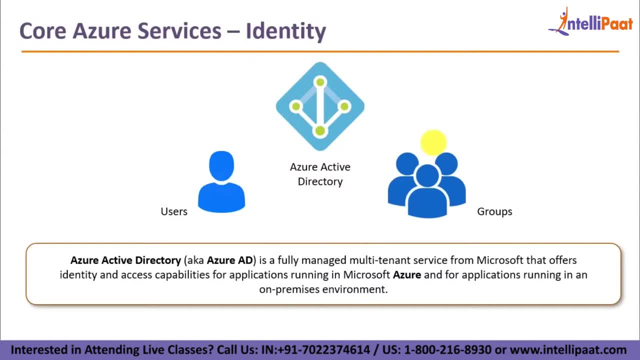 the admin privileges. Similarly, if you want to create some other group- for example, you want to create a group for some SaaS application- you can also do that right, And this concept is a part of Azure Active Directory. And again in a nutshell, Azure Active Directory is nothing, but it's basically a directory. 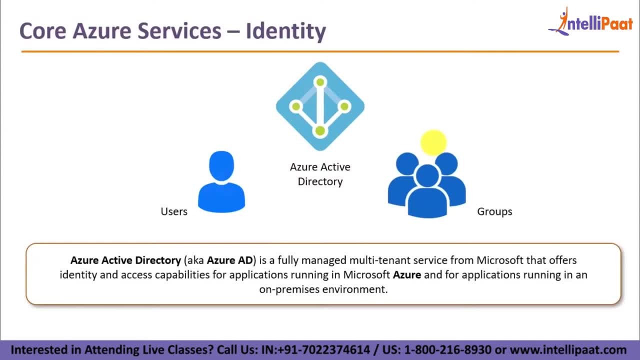 in which you can add users and specify what these users can do on Azure or on on-premise software right, And these users can be managed in two ways. or either you can manage them individually by creating a user time and again, or what you can do is you can add these users to already. 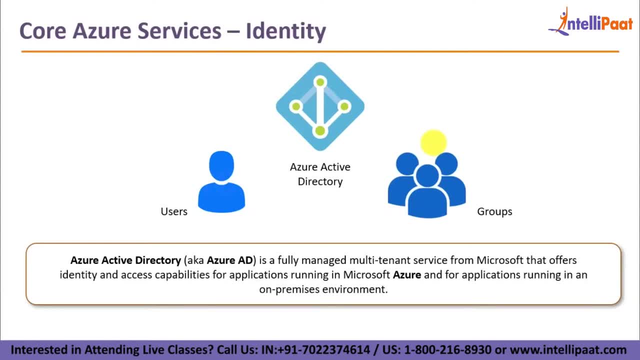 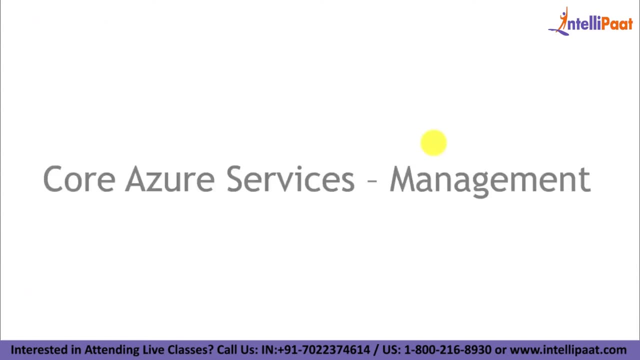 existing groups that you have created, with the respective permissions, and they'll inherit all the properties which have been specified to that group. okay, So, guys, this was the Azure Active Directory and this was about the identity domain in Microsoft Azure. Moving forward, guys. now let's talk about the management tools in Microsoft Azure. that 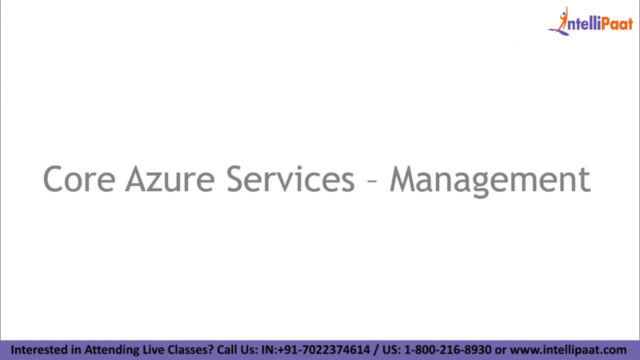 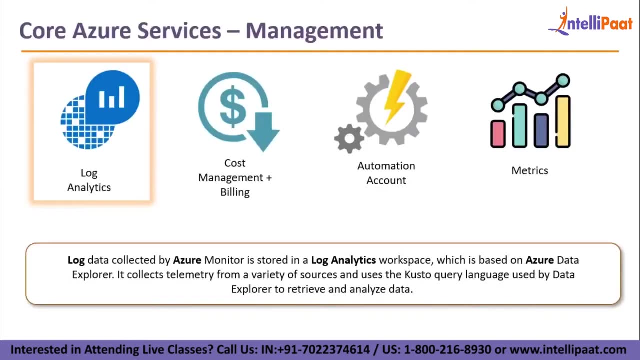 are very important for you to know while you're working as an Azure professional. Alright, guys? Okay, so let's go ahead and understand the management services of Azure. So the first service is Log Analytics. guys, Now, what is Log Analytics? So, basically, the full name of this service is Log Analytics Workspace. 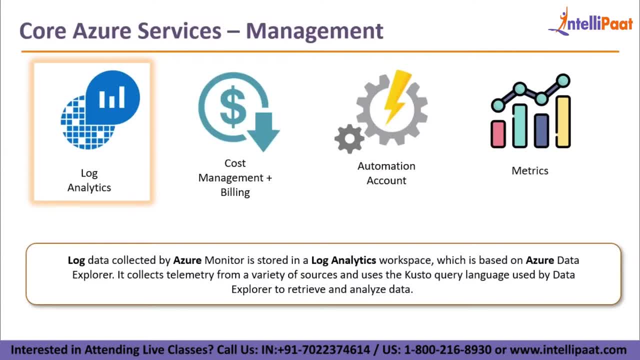 Now, what you can do with Log Analytics Workspace is you can dump all the logs with respect to what is happening on a particular Azure resource onto this workspace. Now, how do you do that? The first thing that you do is you basically go to your management console and you go. 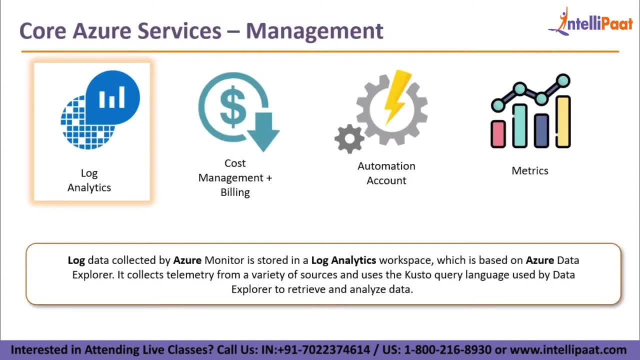 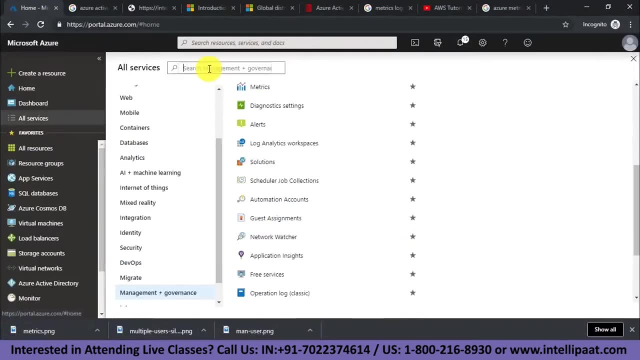 to Log Analytics Over there. you will have to create a Log Analytics Workspace and specify the name- anything right? It's pretty straightforward. Once you've specified that, the next step would be to add a data source. So if I were to show you quickly, I can just jump onto my management console. 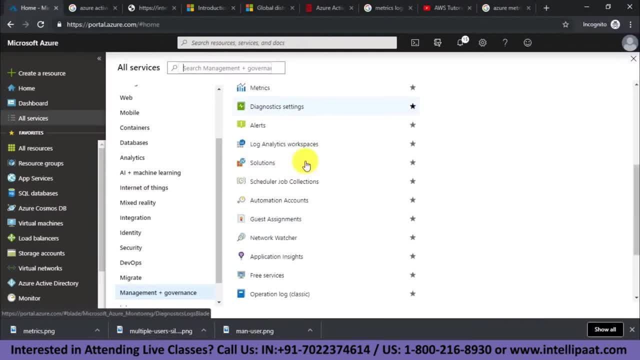 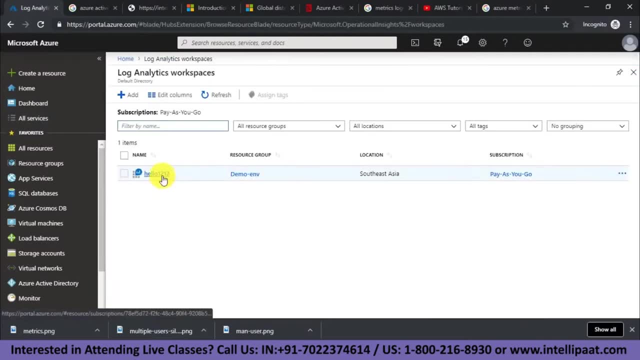 I can go to Log Analytics Workspace, which is somewhere over here. here it is Now. here's a sample Log Analytics Workspace that I've created. I'll just go inside it And, as you can see, it says connect a data source. 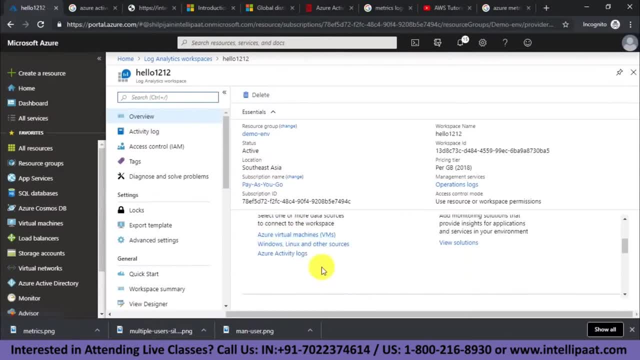 So you can create or you can basically connect Azure virtual machines over here, or you can specify some other sources if you want to, And you can also specify Azure activity logs to stream over here. right, So this will start accumulating logs in this workspace. 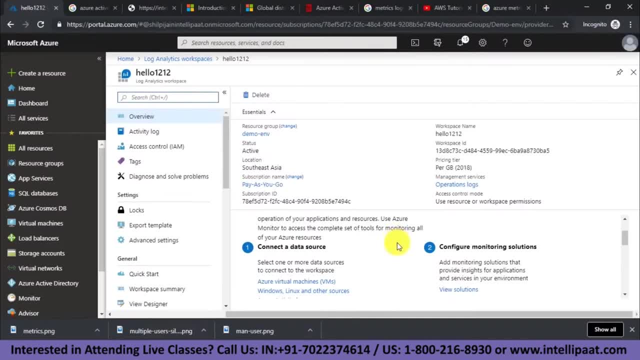 Once that is done, we'll have to specify monitoring solutions as to how you want to read the logs and what do you want to do with respect to a particular data source. So that's the first step. The second step is to create a data source. 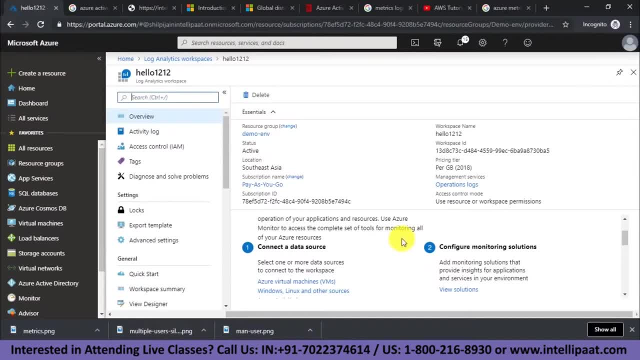 So here, what I'm going to do. what I'm going to do is to create a path. I'm just going to save this data source and I'm going to add a range of data. So let's click on load up, Let's create. 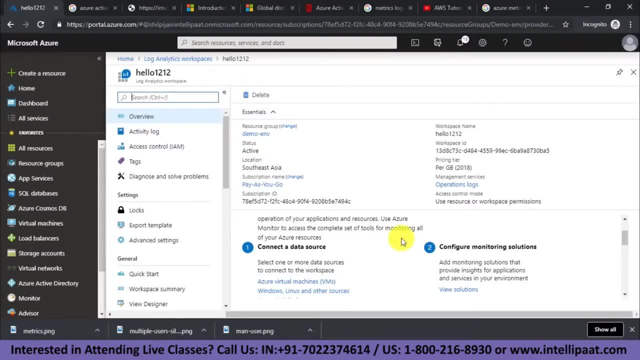 So right now I'm going to be preparing a website with this domain here And my way of creating my website is to click on load up and toys and I'm going to address the match. So someone who wants a little bit more the changes. 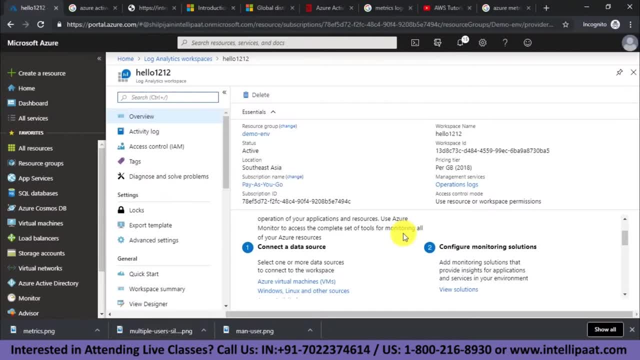 So right now I have my log with this page here and whatever database I want to run is going to appear in a new disk. I've already done that. I was able to identify certifications. now that this system is OK, This thing, let me name it. so maybe a tremendousidades may just be looking for some unique. 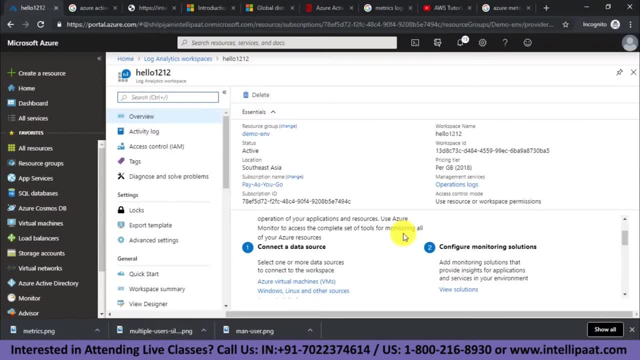 you can specify in your log notation that whenever there is an error, I would specify a term such as level okay, and I would specify that is equal to critical. but if things are okay, it's just for know-how as to which command has been executed and that command executed successfully. 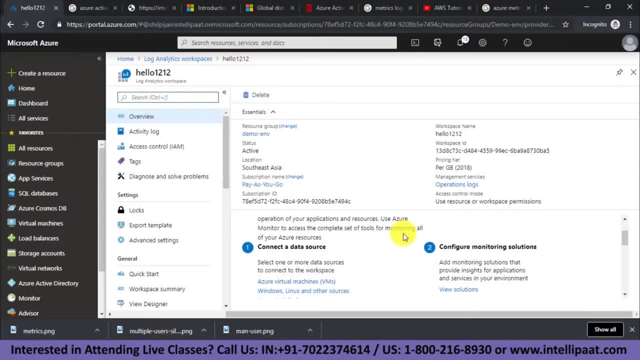 in that case I can specify the level as info, okay. and then I can specify in my monitoring solution that whatever log comes in, check the level field in that log and if the level field is critical you can flag that log. basically, so all that can be configured inside the monitoring solution. so 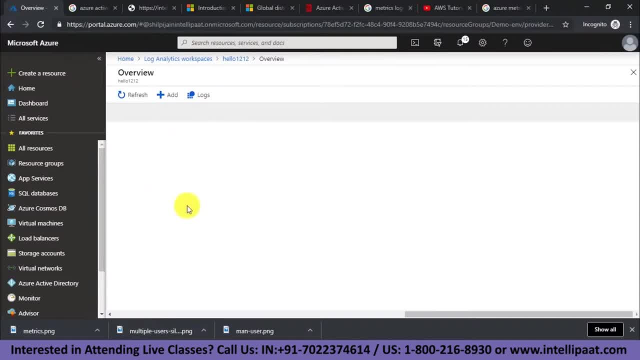 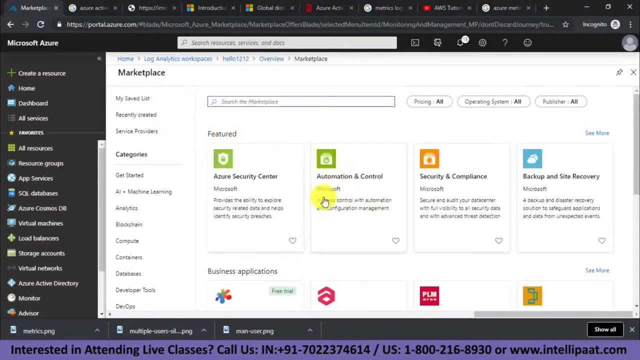 if I were to click on view solutions, you can actually check out what all monitoring components you can actually add on your log analytics workspace. so, as you can see, you can add as your security center, you can add optimized catalog. so there are a lot of things that 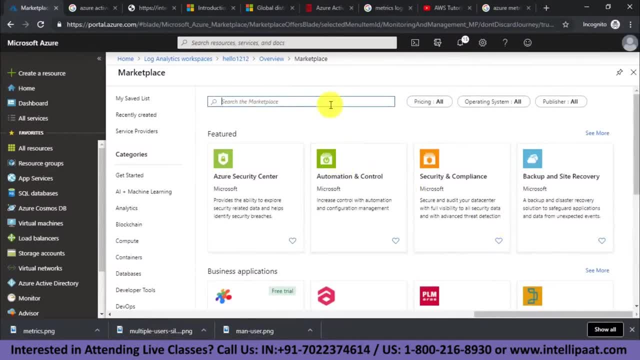 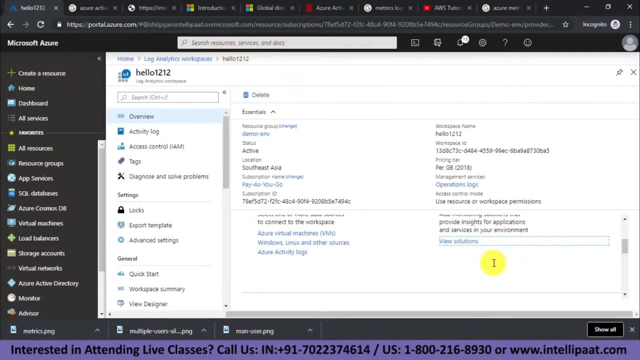 you can basically add on to monitor logs, right, you can choose according to your will. it is available in as your market face. so once you specify the monitoring solution, your log starts to flow in, and in your monitoring solution is after. specify which logs to flag, and that's how. 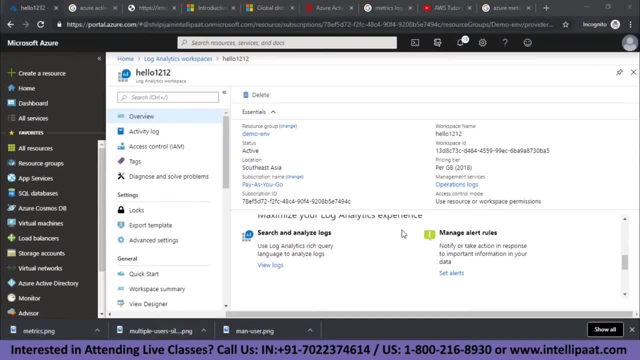 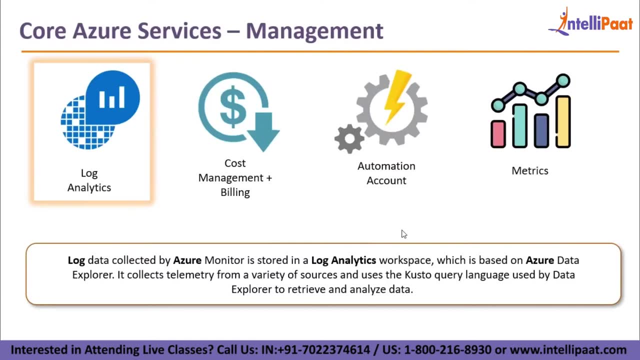 it's gonna work right. so this is the log analytics service in as your guys in, and it helps you to manage your as your resources effectively pinpoint where the problem is occurring, go over there and see the logs, see on which command problem occurred, fix that problem and then go ahead with your daily. 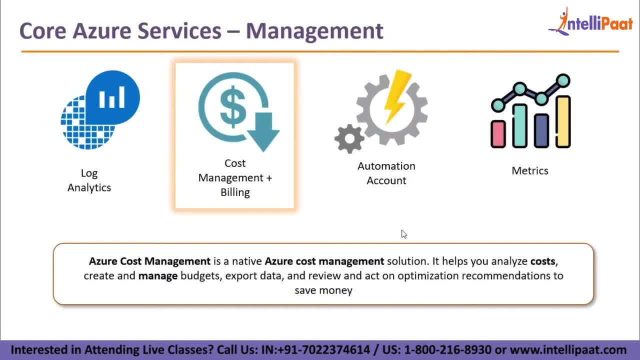 routine. so this is what log analytics is, guys. the next service is cost management and billing. so this is basically a native application of Azure, guys, which helps you to manage your bills in Azure, right? so, for a few things which I can tell you on the top of my head, which comes in is that: 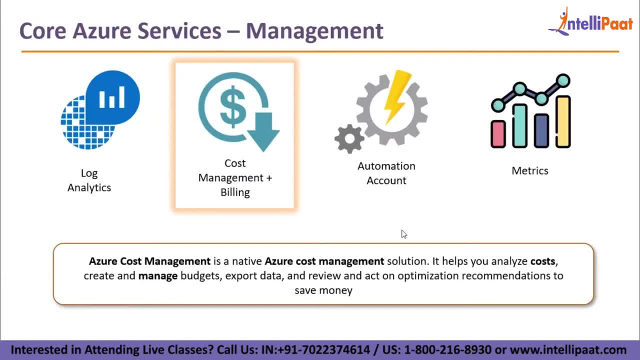 you can manage a budget. you can specify that my as your budget or my as your bill should not go over a particular limit. you can specify that, or you can so when you, when you say it should not go over a particular limit, that means, if it goes beyond that, all your services. 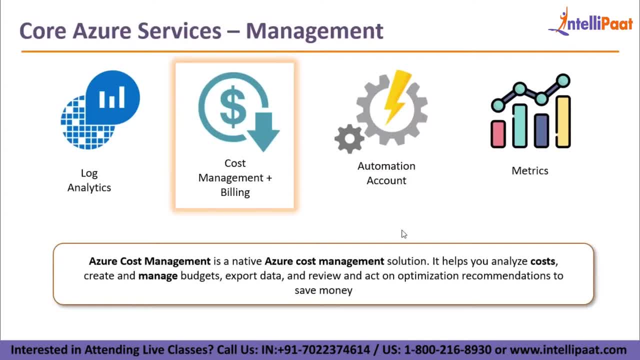 will be stopped. but when you are in a business you actually don't want that. so what? so this particular limit is called a hard limit, that is, you want to limit it to that particular cost. there is another kind of limit, which is called a soft limit, which basically means it will alert you that your budget 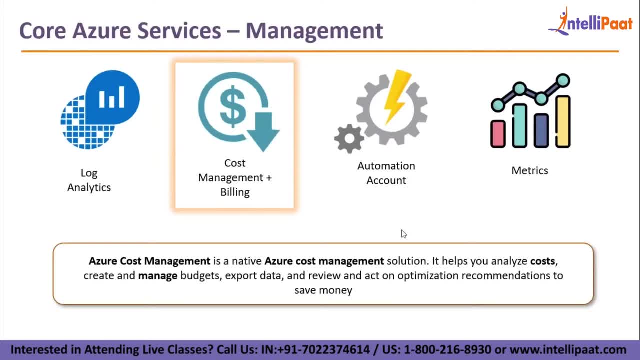 has been crossed and you can actually make forecasts also in this particular service based on your uses. let's you you have used as your heavily for five days, so it gives you a forecast that if you happen to use Azure in this similar fashion, this is what your bill is going to be at. 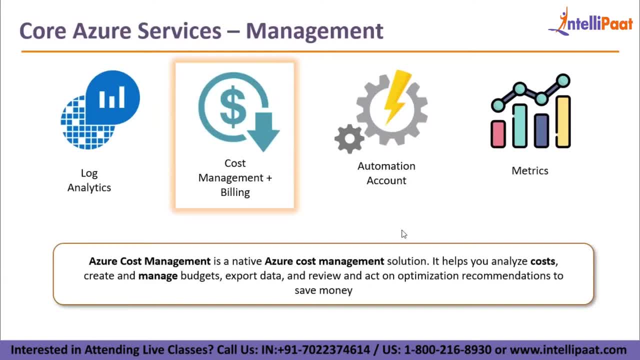 the end of the month, right, and then you can actually see what kind of tweaks you can make in your services so that your bill comes down. so all of this is possible in cost management and billing services of Azure. now this also is under the management domain. reason: 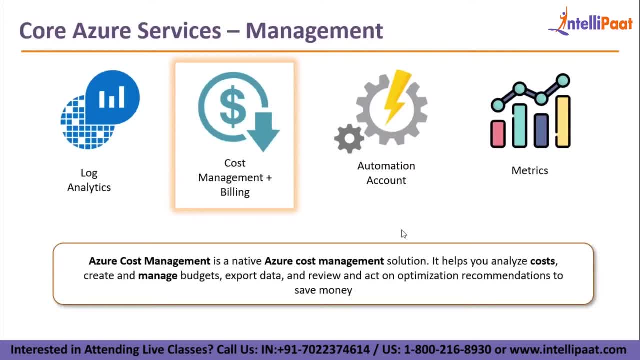 being. it helps you in managing your Azure resources in a better fashion. the next service, guys, is a very important service, which is an automation account. now, what is an automation account, guys? it is nothing, but uh, it's. it's a way of deploying Azure resources. so how do you deploy Azure? 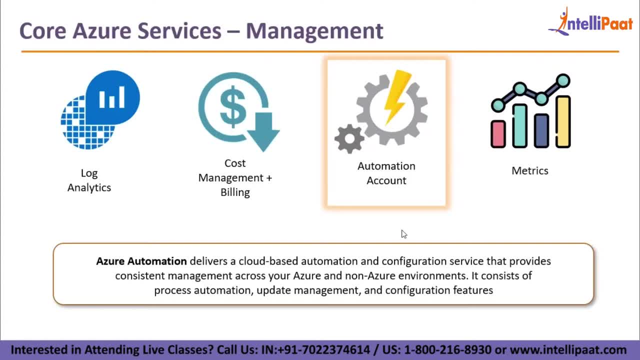 resources. so we have seen few of the resources in this session today wherein we deployed a virtual machine, we deployed a storage account, so all of that was possible one by one. I mean, I had to go manually into that service, I had to click on that, I had to specify a name and that's how you know my resources. 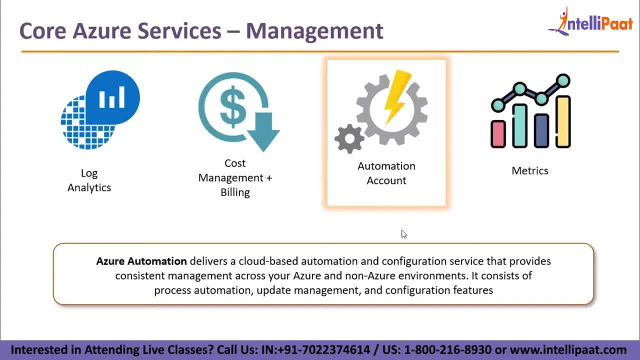 were deployed. but in automation account what happens is you can create run books. now, what are run books? you basically specify a code wherein you specify all the resources and their names and their configurations that you want to deploy, and then you upload that run book onto the automation account and then you run that runbook. then what it does is it automatically creates the. 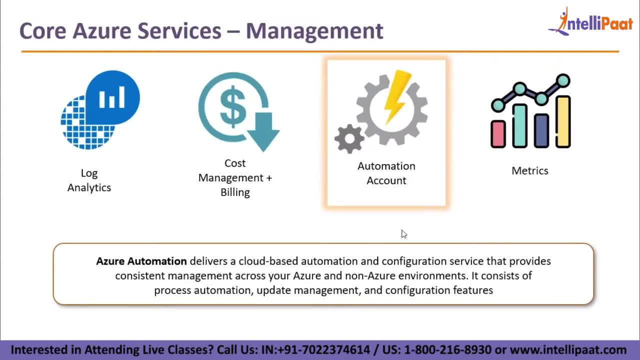 resources for you. you don't have to do anything. just put that runbook over there, click on play button and it will create all the resources for you with the exact same configurations that you have specified in the code. it is particularly helpful when you're setting up a large infrastructure. 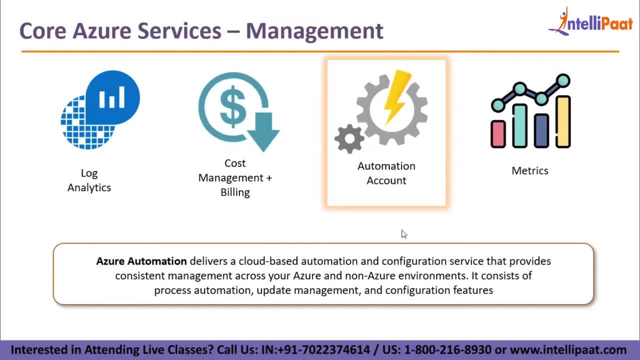 wherein you'll have to deploy thousands of 2000 machines, where each uh where the 2000 machines are basically divided into multiple sets- it could be back-end server set, it could be database server set, it could be front-end server set, all of which will 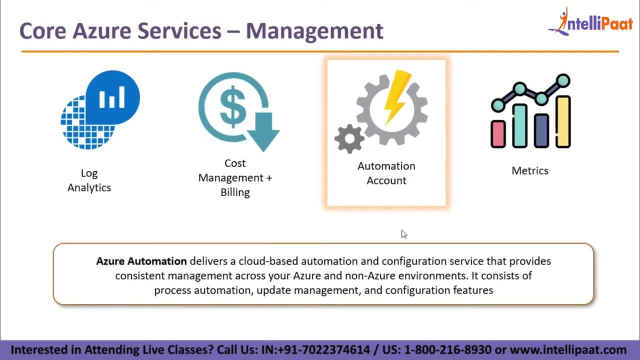 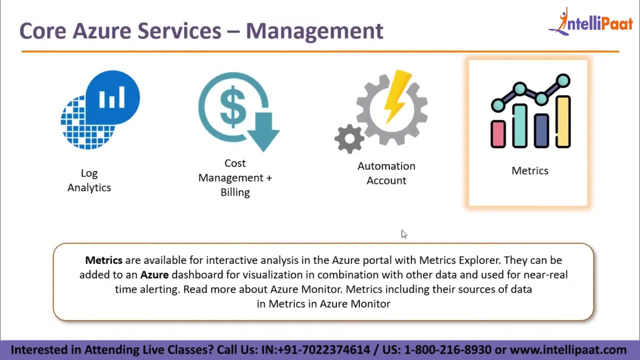 have different kind of configurations and if these, this is the kind of a scenario, then run books would be of great help, and that's where automation account also comes in, which basically helps you to play those run books. okay, our next service is metrics. guys, now, metrics is a service which helps you to 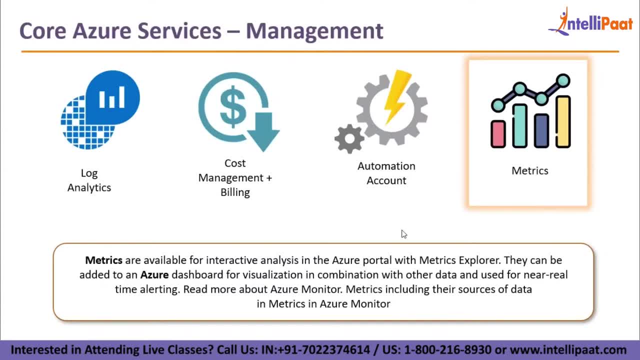 visualize what all is happening on your as your resource. for example, what is a network throughput, what is the CPU usage right, what are the memory usage. all of that you can see inside metrics. now you can actually check a 24-hour log as well in metrics and see at what point of time does your resource or your or the 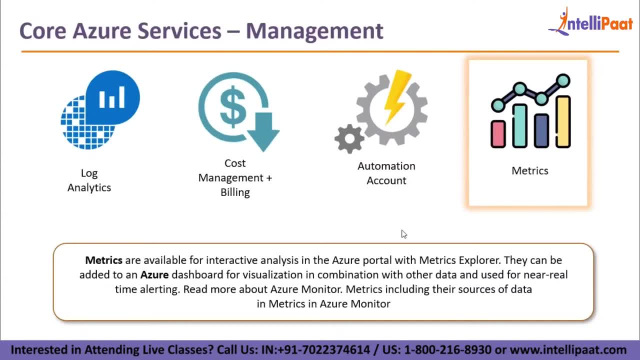 particular metric that you're checking could be CPU usage, would memory usage is actually rising, and then you can plan accordingly as to how to plan your or how to scale your infrastructure at that particular time. right, so this is what metrics are useful for. it basically gives you an. 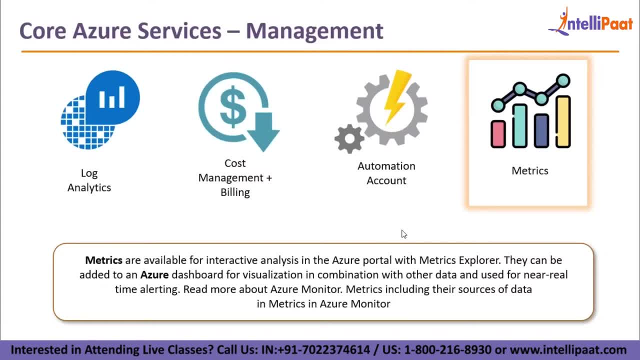 overview of how things are going. so, if you think about it, it is nothing but metrics. oh sorry, it is nothing but logs, which is basically basically getting visualized in from of graphs, but nonetheless, it's very helpful and that is a service which is being provided to you by as well, by the name metrics. 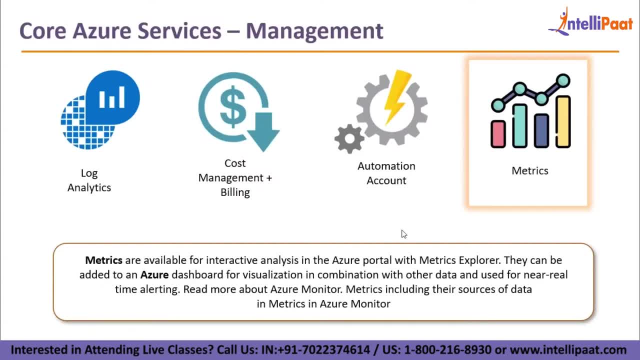 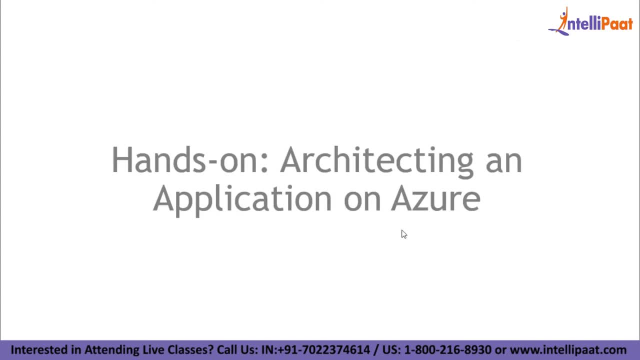 alright there. so these were all services in the management domain. guys, our next up, we'll be discussing a hands-on. so enough of theory. i guess we have discussed probably most of the important services which are there in the azure portal. now what we'll be doing is i will be showing you an application which basically exists. 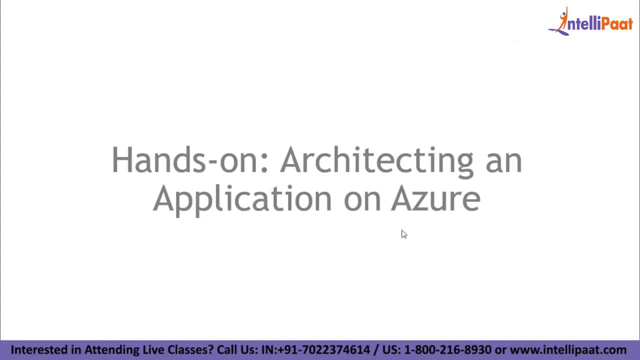 on my local host and what we'll try to do is we'll try to migrate that to azure and we'll choose the services. based on the knowledge that we have gained today, we'll choose the services accordingly, then we'll set up the infrastructure and then we'll see how it works on the cloud. so, guys, let's. 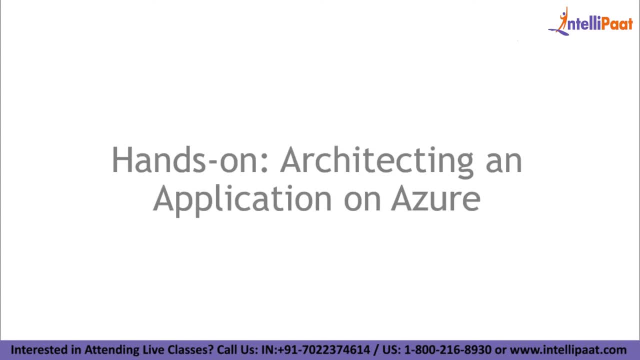 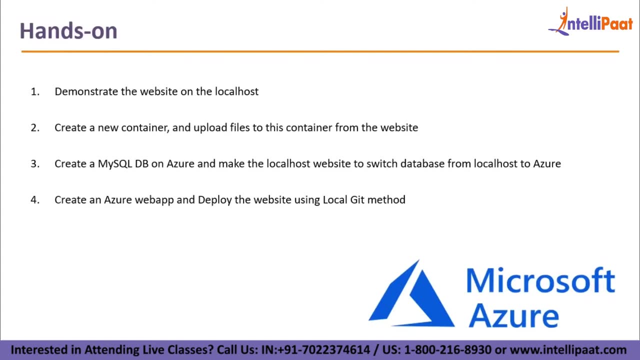 go ahead and do that, all right guys. so let's go ahead and let me show you what all we are going to do. so the first thing that we're going to do is basically i have a website that i've already created on my local host, which basically can upload data to azure blob storage through the. 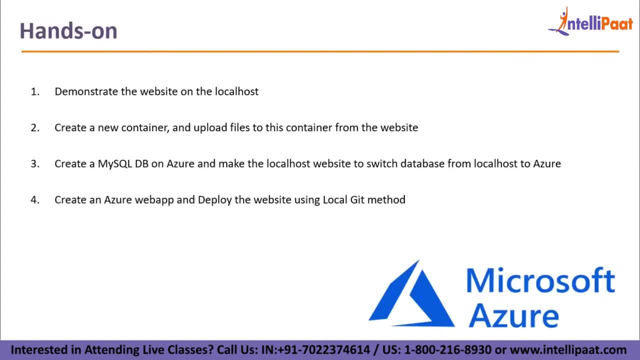 website. so i'm going to show you guys how i have configured it and how can it basically upload data to azure blob, right? so the second point is create a new container and upload files to this container from the website, right? so we'll be creating a container and our website we're going to configure to upload files to this. 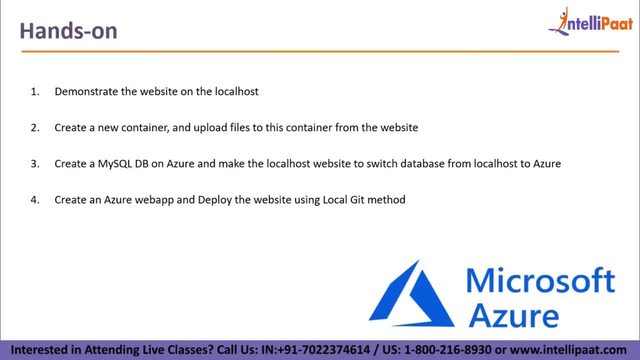 particular container. third thing is we have to create a mysql database on azure. so right now, what is happening is my website is basically storing data on the local host mysql engine. what the hands-on expects us to do is we'll have to deploy mysql database on azure blob. so we're going to create a mysql database on azure blob and we're going to 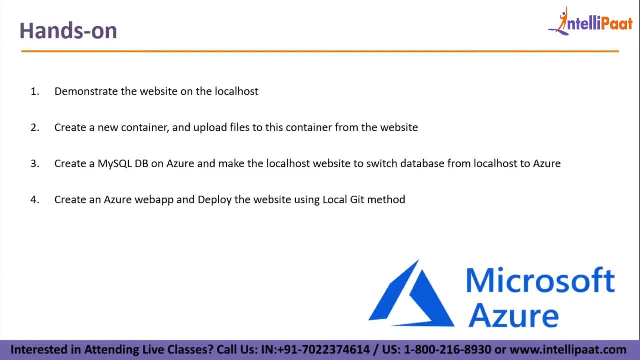 run this well, abo well, and the architecture is going to be based off of azure, and the website should basically push the data on to the mysql database, which will be there on the azure portal, right? so this is the third step and the fourth step. finally, we want our final website to be: 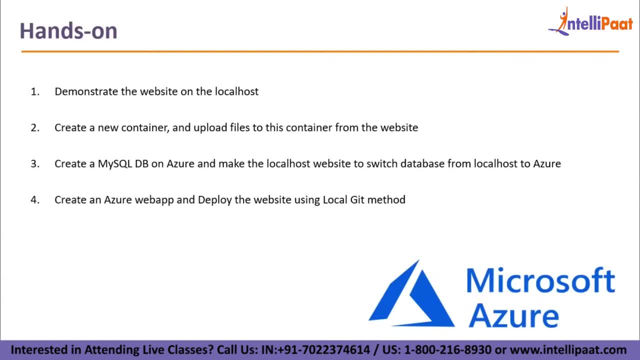 uploaded on azure webapp and basically we have to deploy it using the local git method. what it is, don't worry about it. as you move along, you'll get it all right. so let's start off at the first point right now, which is demonstrate the website on the local hosts. 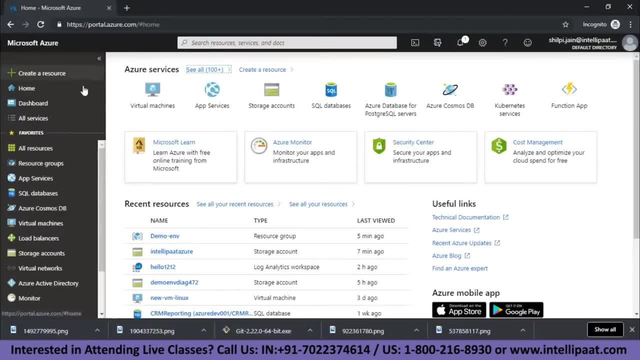 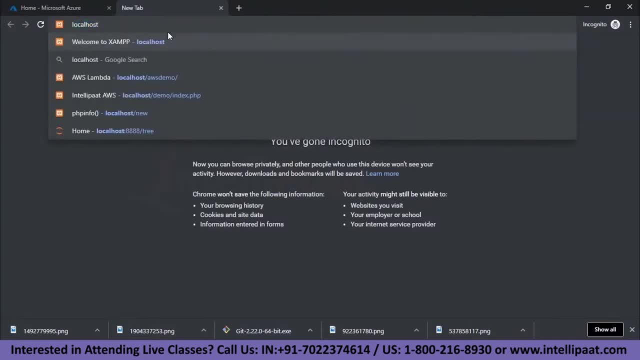 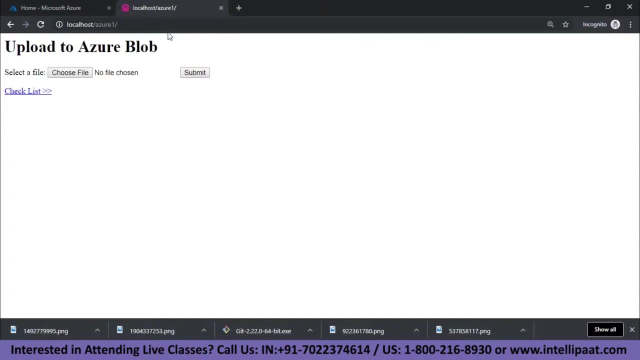 so let me switch on to my browser. so, guys, this is my as your portal, and if I have to demonstrate to you my website, it basically exists on localhost as your one, right? so this is my website, guys, and what it does is it basically can upload data on to Microsoft Azure. but right now, what I have not basically configured it. 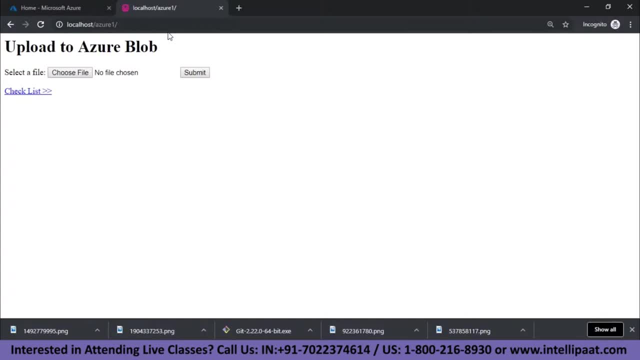 to connect to my Microsoft Azure storage account. I'll show you how we can configure it right. so once a file is uploaded on the blob, it also makes an entry of it in the database. right now, where is the database? the database exists on my localhost, so what I'm gonna do is I'm gonna just open the mysql. 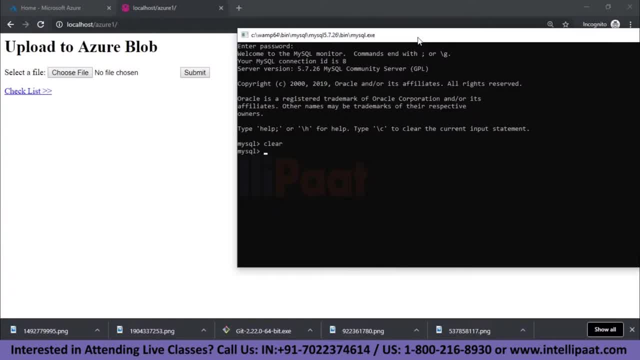 console right, and my mysql console basically has a database called images. so if I do a show databases, you can see that there is an images database. so this is the database that my website will be interacting to. so let me just use images, and in this database what I have is a table. so if I 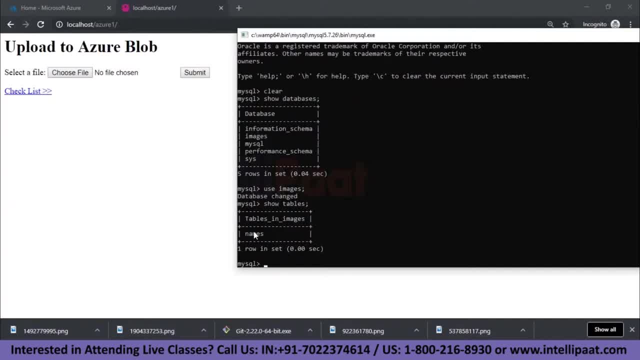 do a show tables command, you can see that I have a table called names, right, but right now there is no data inside names. right now there is no data inside names. so if I do a select star from names, as you can see, it is empty set, right? so 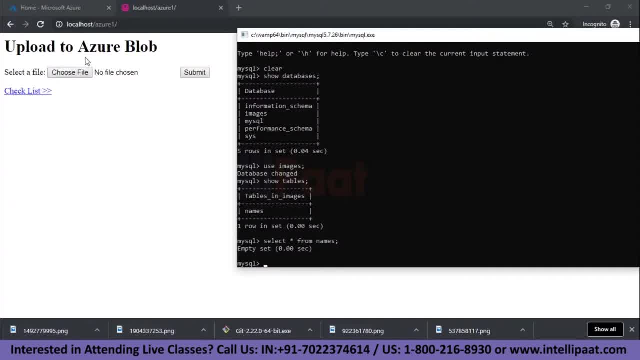 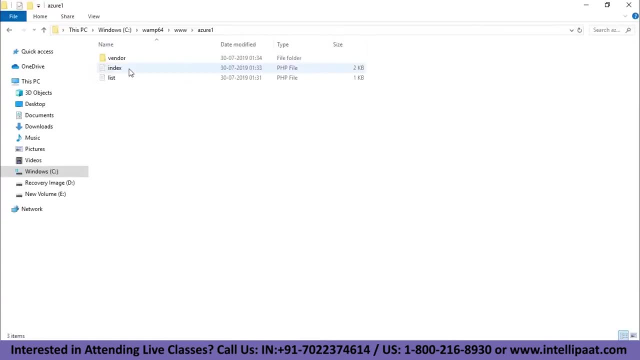 when the data, when this website will be uploading file, when it will be successfully uploaded, next step would be to basically put the data inside the database as to what is the name of the file. okay, so let me show you the code, guys. let me show you how the code looks like. this is my indexphp. let me just 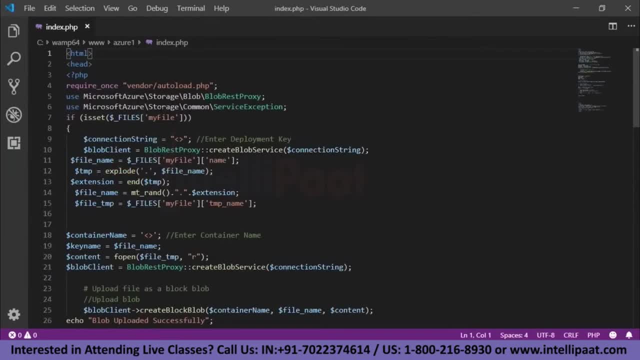 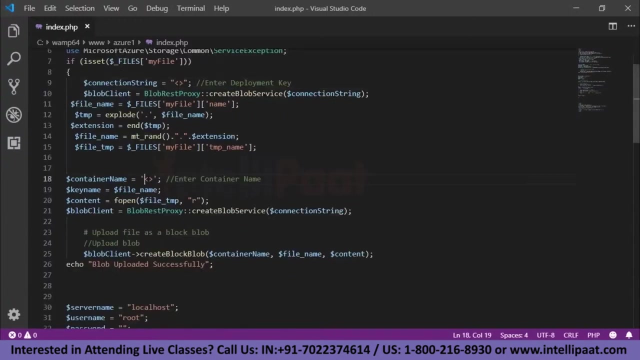 open it, alright, guys. so, guys, this is this is how my code looks like. so the first thing that I'll have to do is basically I will have to enter a deployment key over here, which will basically be my connection string, and the second thing that I'll have to do is I'll have to enter the container. 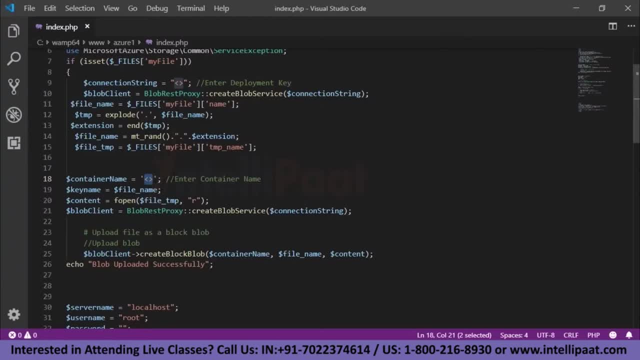 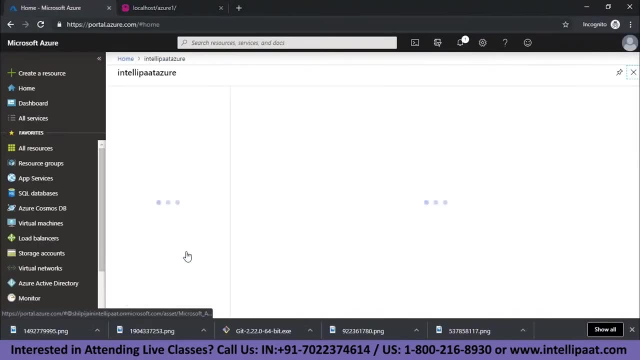 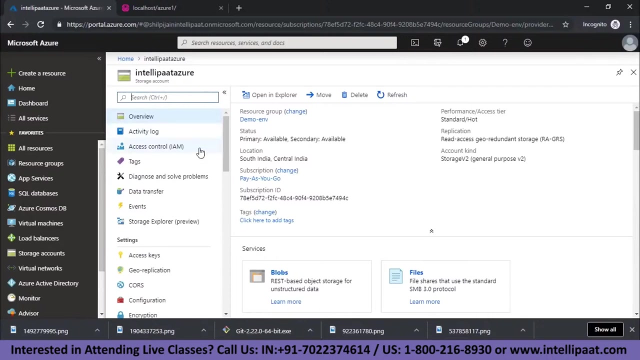 name, which I'm going to create in a little while, right, so let's first jump on to our azure portal and what we want to do is go inside our storage account. so, guys, this is my storage account and what I want is the deployment key. so in this storage account you will have to go to access keys. just go inside that. 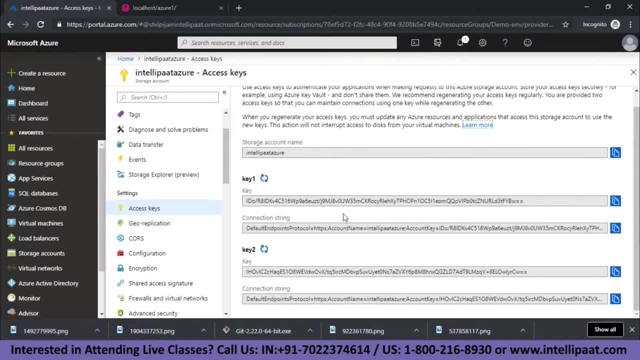 and here you will find two keys. you can take any of these two keys, so what I'll do is I, let's say, I take key one and this is the connection string. so I'll have to copy this and I'll have to come back to my code and I'll have to replace. 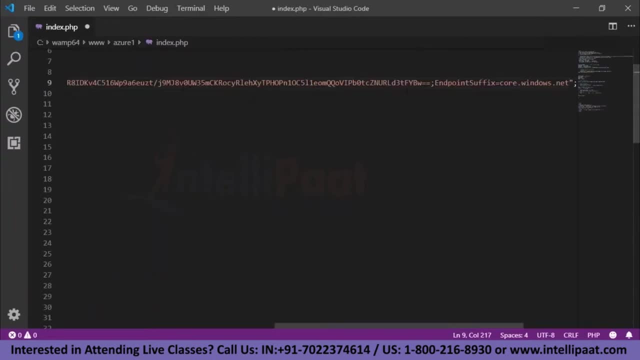 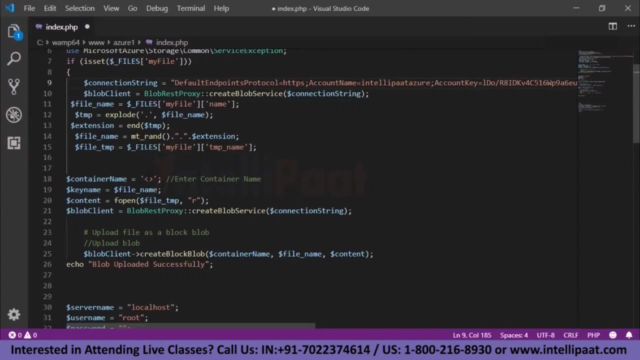 it over here. so let's replace the deployment key. and now I will have to remove this part out of the deployment key. this is not required, right, but this we will remove and this is my deployment key, guys, all right? next step is to basically enter the container name. now the hands-on basically expects us to. 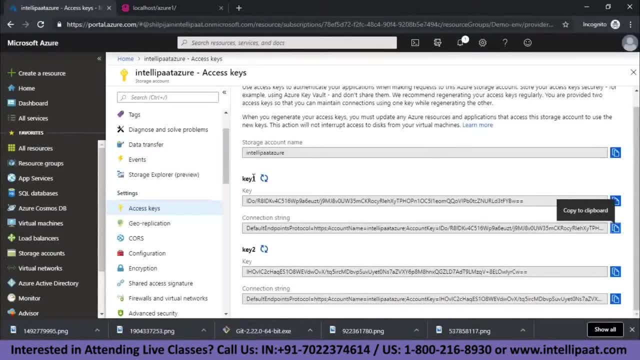 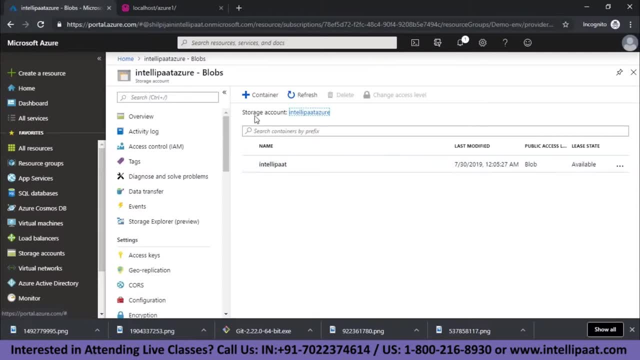 create a new container, so let us do that. so let's go inside overview and let's go to blobs. so I have a container in telepart over here. let's create one more container and let's call it new right and let's give the access as blob and 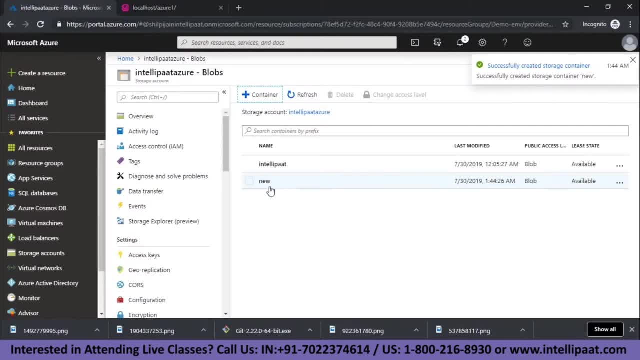 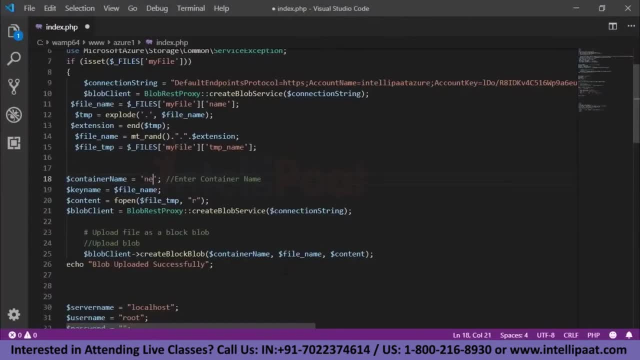 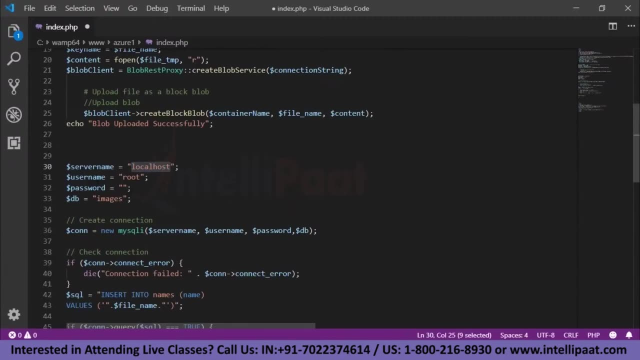 let's click on. OK, so my container is now ready and it's called new. let's name the container over here. so my container name is new. okay, everything else looks good, so right now this is. this is basically the connection information for my MySQL database. so right now it is going to upload the data on to my localhost MySQL. all right, so 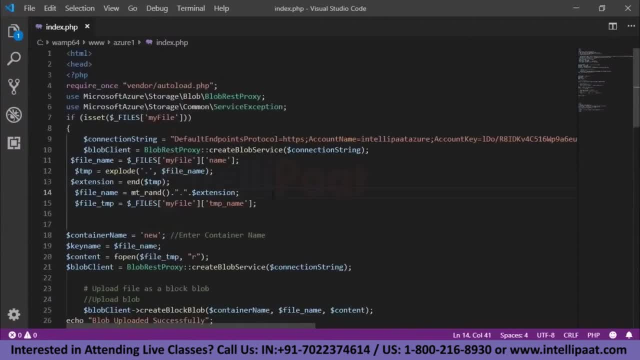 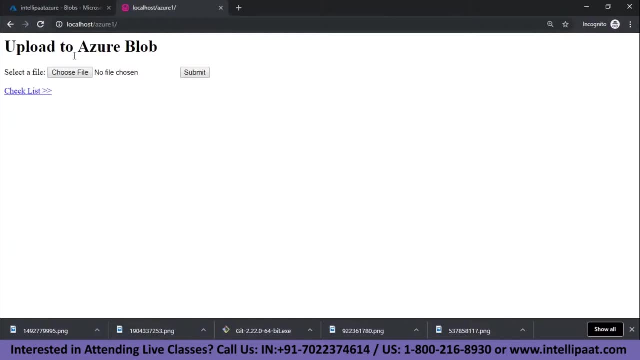 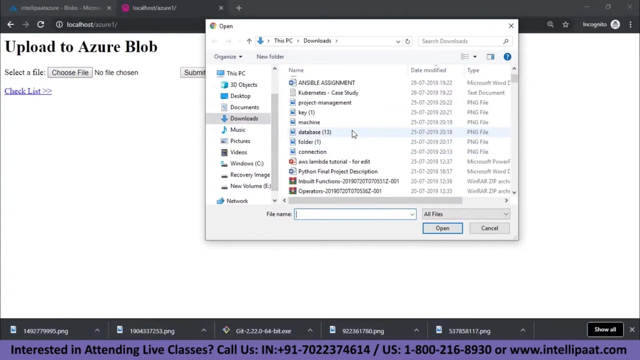 let's see if I can upload a file now. let's save this indexphp. after you've downloaded it, you will notice as I scroll down here. you'll see that we have two different spiritually broadcast resources in this folder. let's go back to our website. let's refresh it once and now. let's choose a. 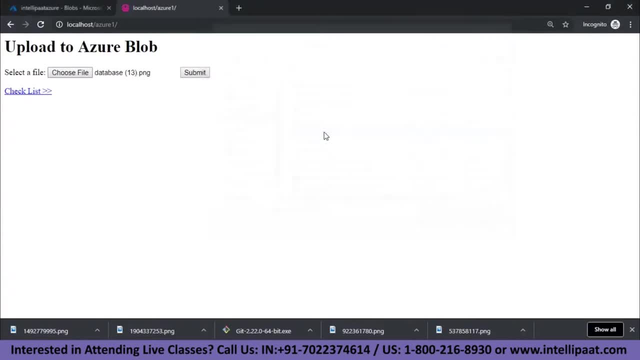 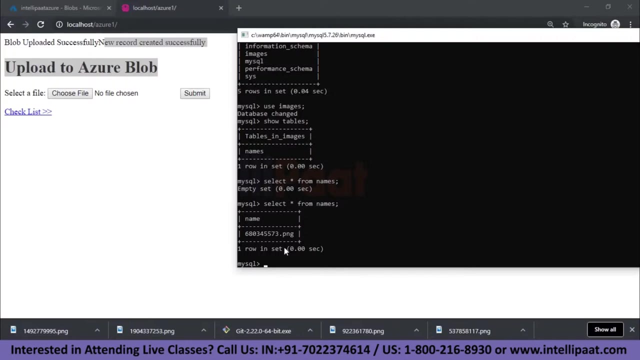 file which we want to upload. let's go inside, let's try to upload. let's say database, so this is an image which is called database. let's select this and let's click on submit. so it says blob updated uploaded successfully and new record: created successfully. see, there is a new entry over here which is 680345573. this is the name which has been assigned. 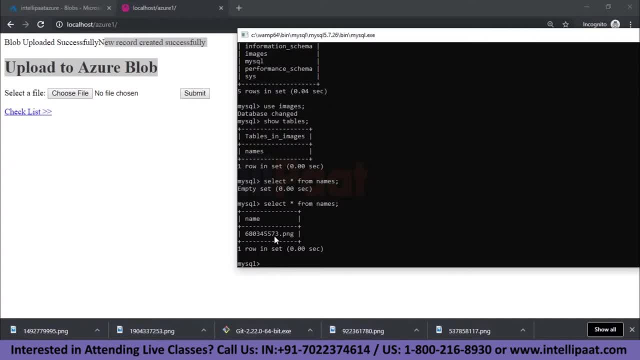 by my website, so this is basically a random name. the reason for that is that it could be that you are uploading duplicate files, and if you upload duplicate files, you don't want the names to coincide. so what i'm doing is i'm assigning a random name to every file that i'm uploading. 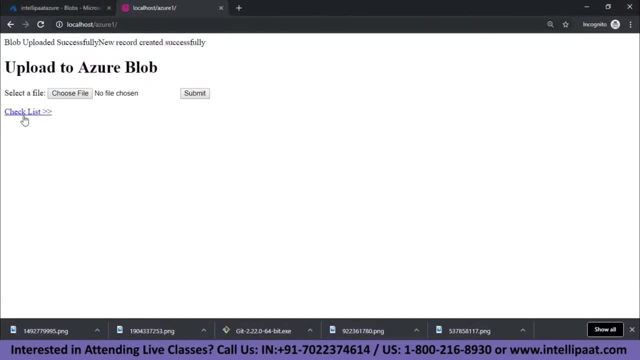 right. so this is the file which has been uploaded and we can check it over here. if i click on checklist, this is the file which has been uploaded and if i click on this file now, i can download that file, basically from azure. it says blob not found and the reason for that is that 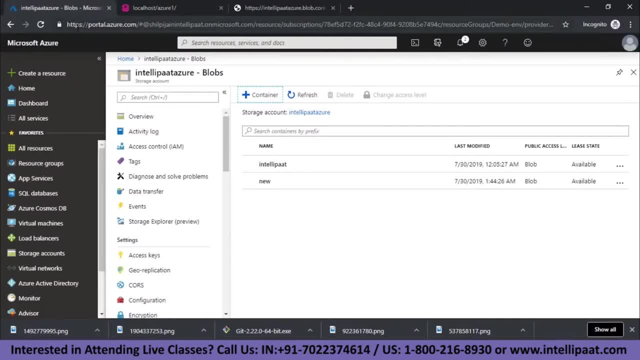 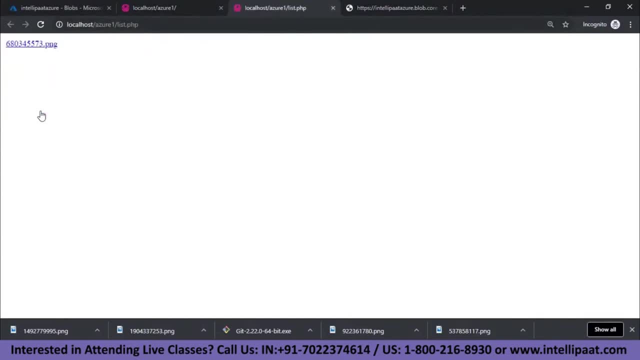 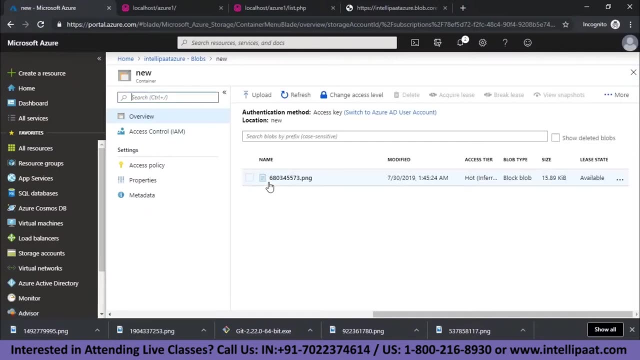 i'll have to change the url inside my list website, which is basically, if i click on checklist, this is the listphp. i'll have to change some code here. i'll show you that. but first let's go inside the new container and, as you can see, there's a png file over here. now, this png file: 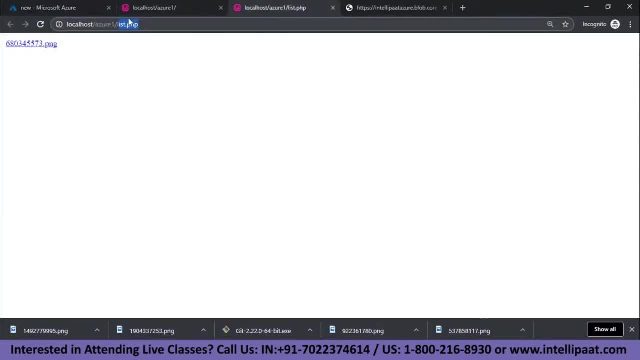 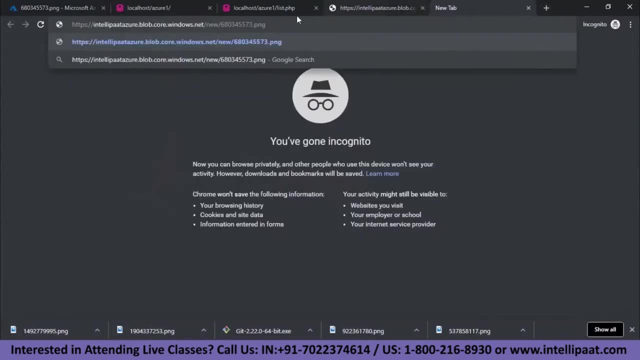 i can directly download from my list file. but in order to do that, what i'll have to do is i'll have to click on this file and i'll have to copy this url and i'll have to see what is the prefix over here. so the prefix is this. so i'll have to copy this prefix and now i will have to go inside my 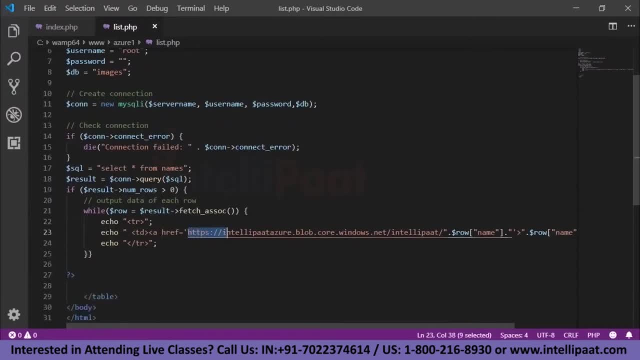 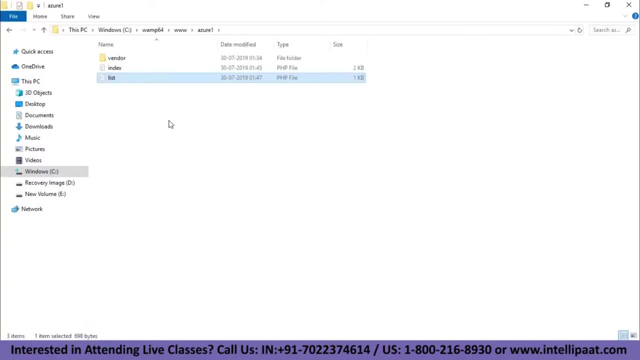 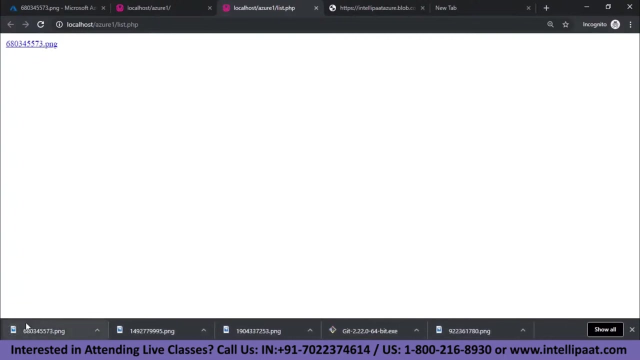 code and open the listphp code, and this is the url that i'll have to go inside my listphp code to replace. so let's replace it all right. great, now let's save it. come back to our website. this is the listphp. let us refresh this once and now. when i click on the file, you can see that i've 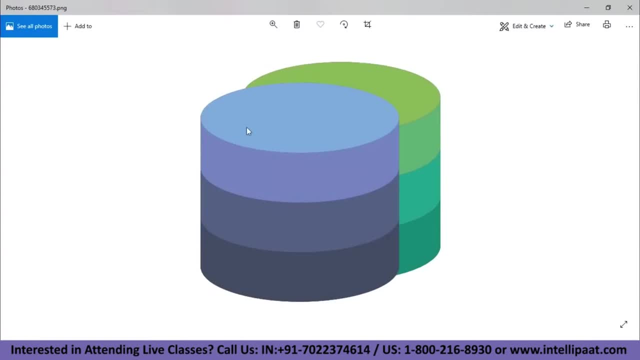 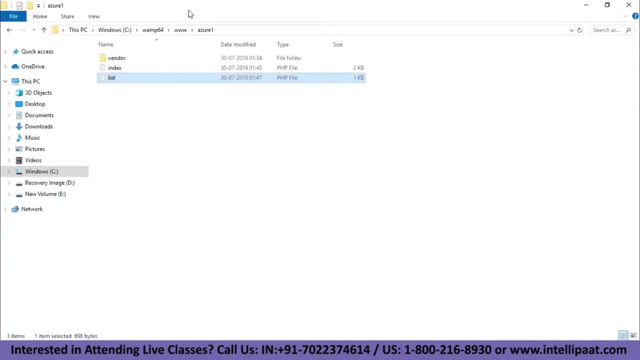 downloaded the file automatically. let's click on this file and this is an image which has been downloaded. now let's try something else. let me show you the image first, and then i'll try to upload it. so what i'll do is i'll go inside downloads and let's say i want to upload this. 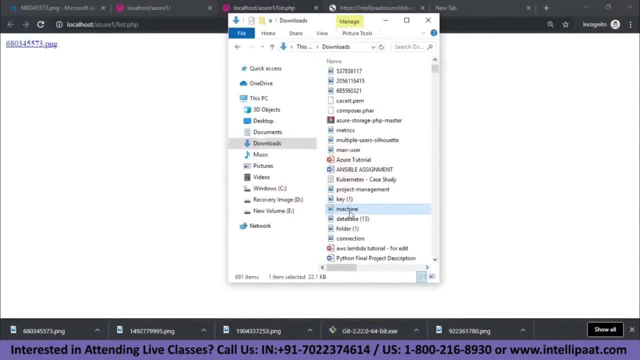 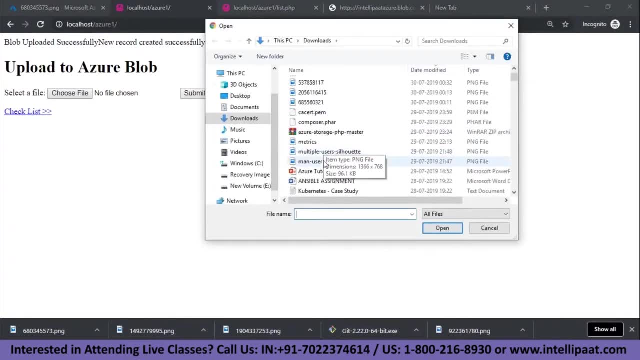 file. so this machine file looks something like this: okay, now we're going to upload this machine file. let's go inside our website, let's choose a file and now let's select the machine file, which is basically this: this we will upload, we'll click on open and we'll click on submit, so it says blog. 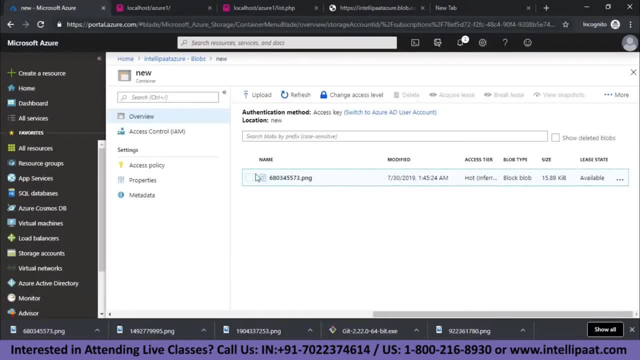 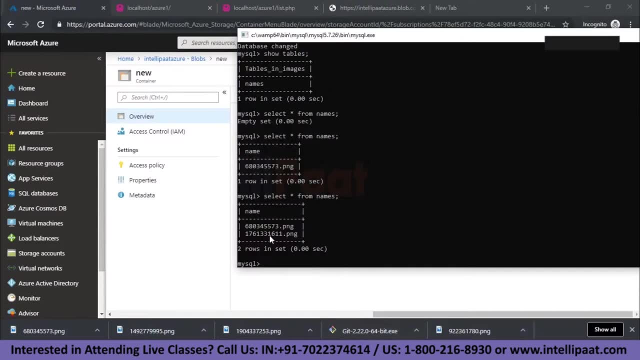 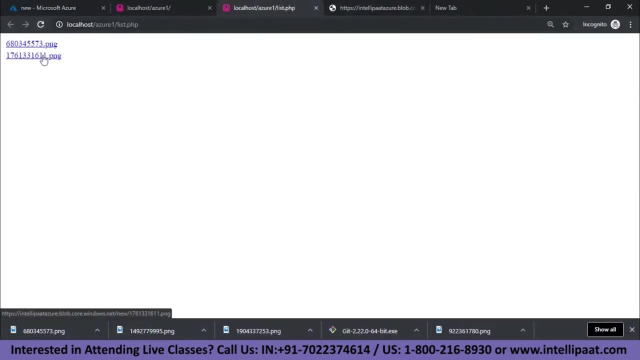 uploaded successfully. if i go inside my container and i refresh it, you can see there's a new entry over here. even in my database, if i refresh, there's a new entry over here. and now what i can do is i can basically just go to my list, refresh it. this is the new entry. click on it. file gets. 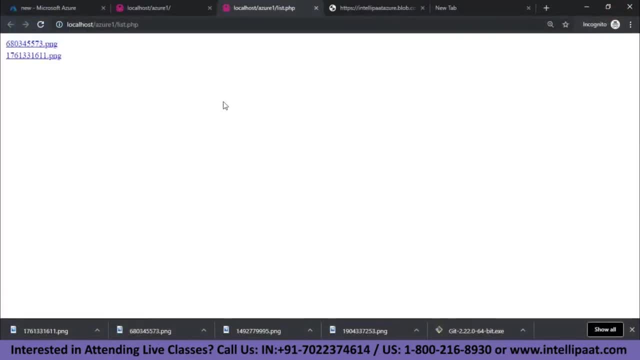 downloaded. click here, and this is the file which was uploaded. so what is basically happening over here is this file is now hosted on blog and any of you, if you click on this link, you will be able to download it, but the problem is that this website right now is only available on my local. 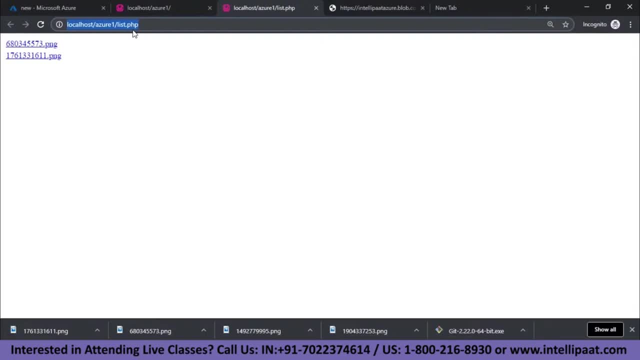 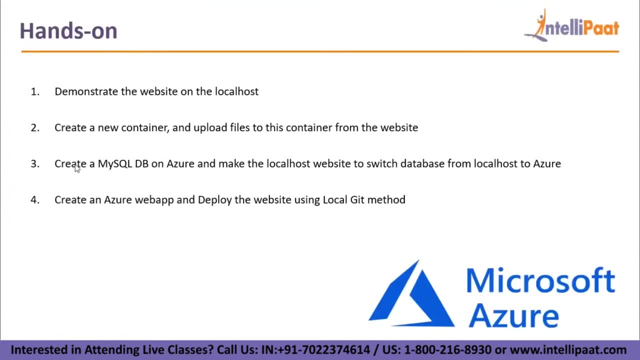 host and i have to make it available to the world. now how can i do that? so, first thing, first, let us go back to our slides and see what is our next step. so our next step is that i want to create a mysql database on azure. so right now, my database, which is being updated, is on my local host, but 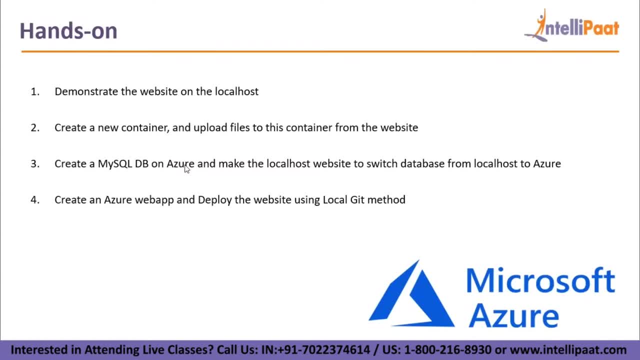 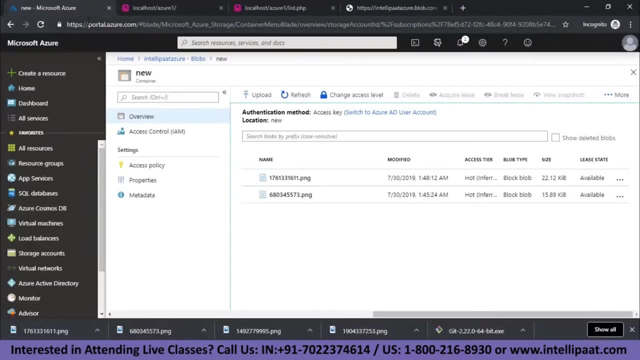 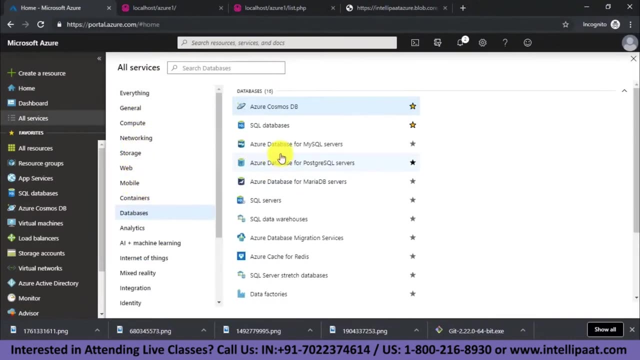 what i want is that it should be updated on my azure mysql database. now let's see how we can do that. so the first thing that i will do is i'll have to go back to my azure dashboard. i'll have to go to my database and this is the database that i want to launch: azure database for mysql server. 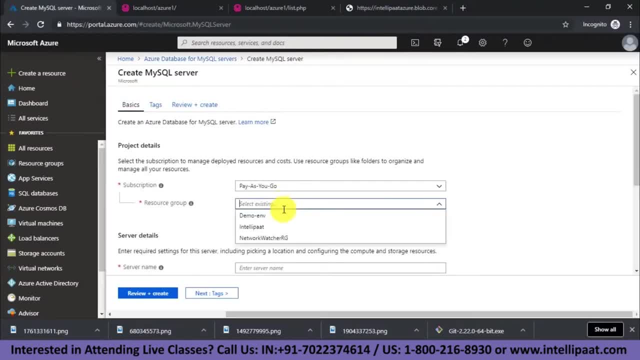 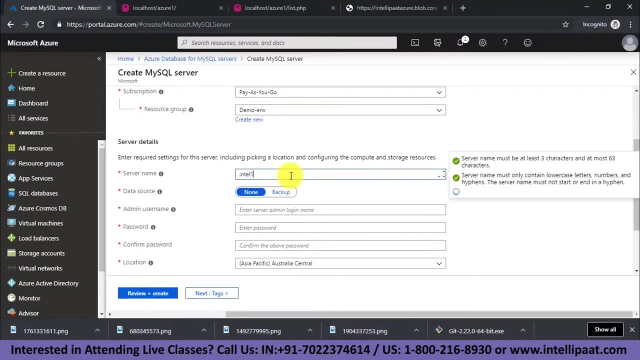 let's select it. let's add a database. i want to include it inside my demo environment resource group. the server name: let's specify it as intel one right. the admin username: let's specify it as intel. the password: let's specify it as intel at the rate one to three. okay, it says your password. 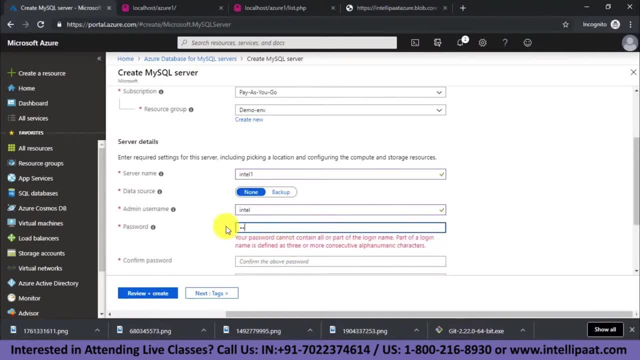 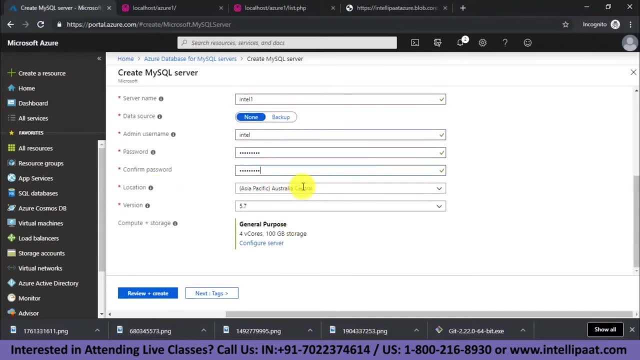 cannot contain all or part of the login name, no issues, let's name it as azure, at the rate, one to three. same is the case over here. all right, and where do i want to launch it? i want to launch it in south india. uh, the version is 5.7, which is great now. 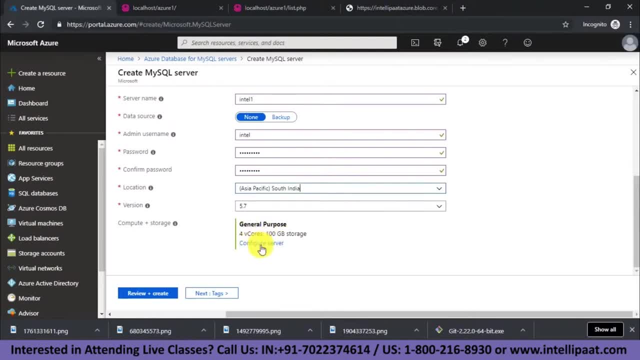 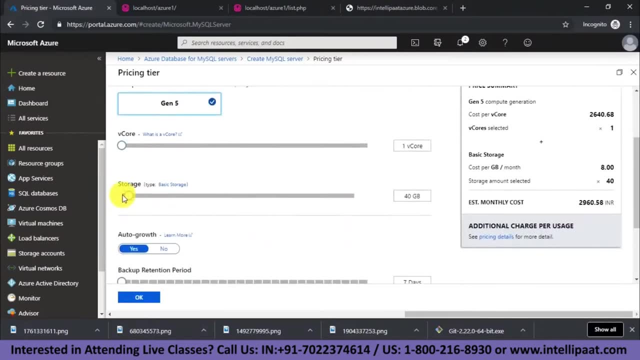 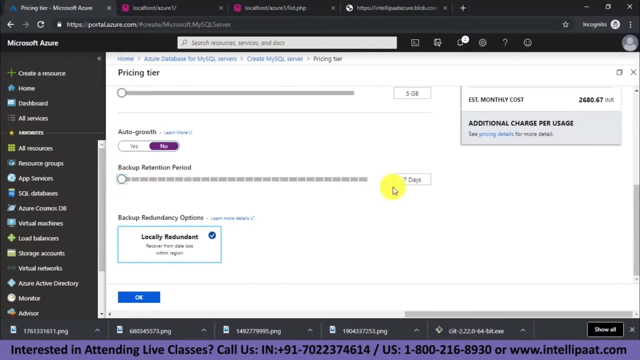 let's change the amount of specification that we have for this server. let's click on configure server. i want a basic configuration. i basically want one core and i want the least amount of storage, which is 5 gb. auto growth- no, i don't want it. backup retention period: uh, the least is seven days, which is fine, and i think that's it. 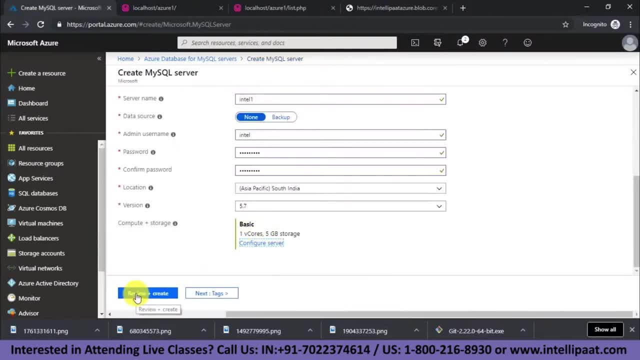 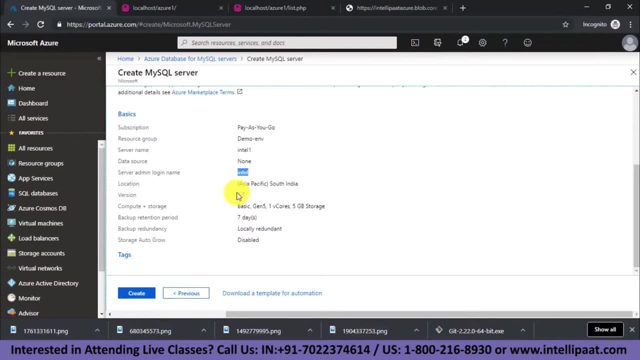 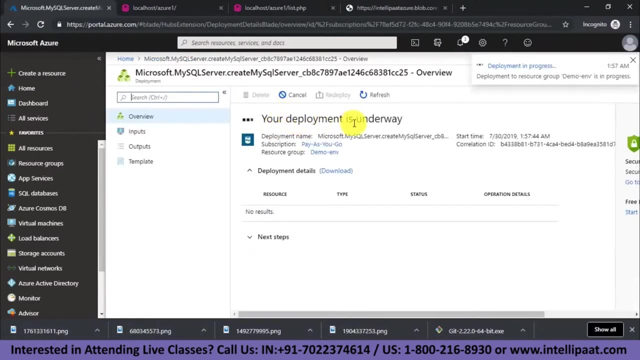 let's click on. okay, now the server has been configured. now let's click on review, let's create: okay, so our username is intel, my password is azure, at the rate one to three, and now let's click on create. all right, so my deployment is underway, which basically means my mysql database is now. 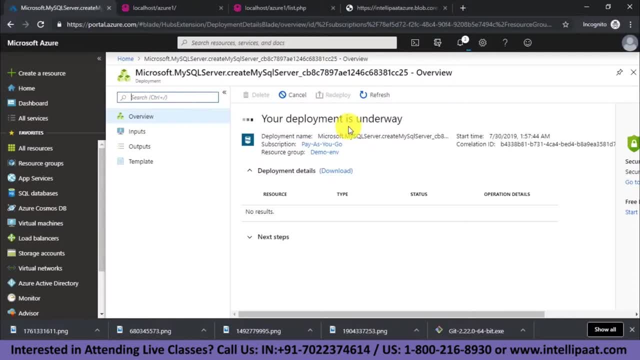 getting deployed. let's wait for some time. let's wait for some time, and then i'll show you how to complete it. we'll wait for it to be complete and then we'll proceed with our demo. all right, guys, so my deployment is now complete, so i can just click on go to resource. 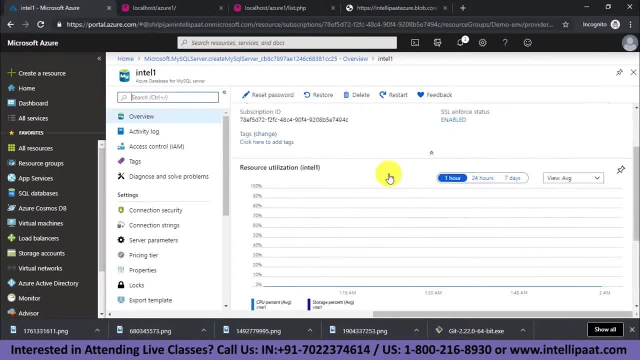 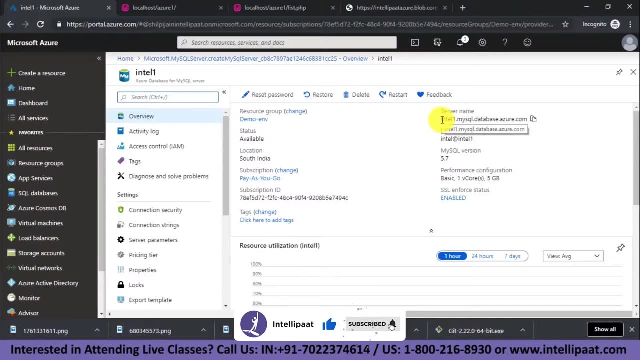 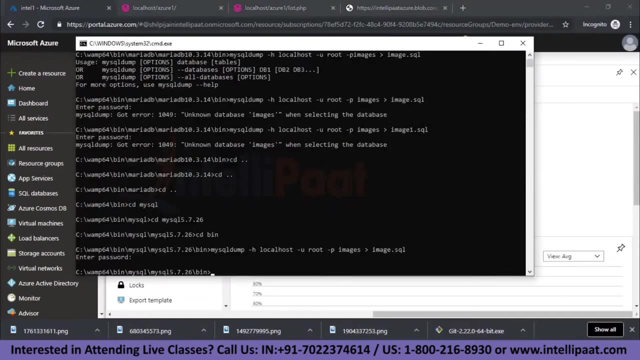 and i am in. so this is my database. guys, now, in order to see or in order to access my database, this is the server name that i'll have to use, so let's go ahead and select this. so my server name is this. let's copy it and let's come back to our command prompt and what we want to. 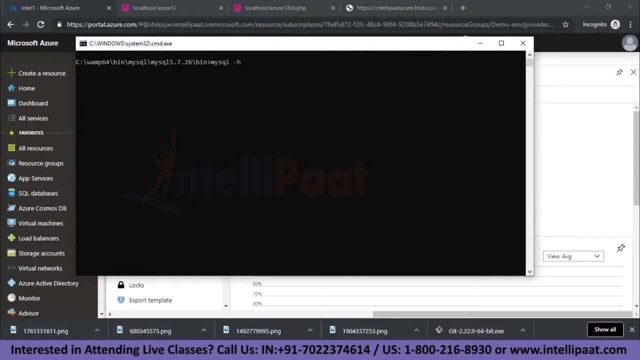 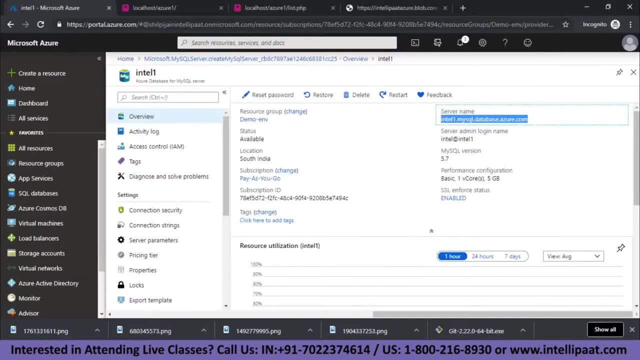 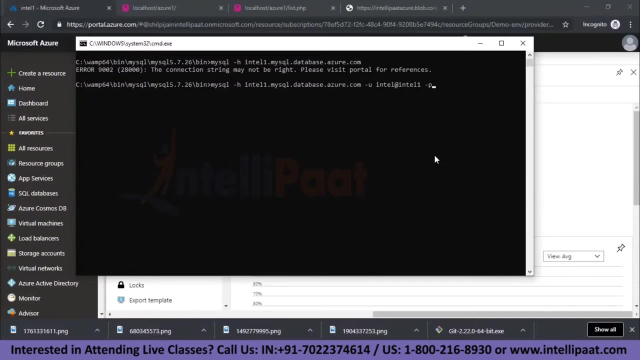 do is mysql-h. this is the connection string, or the server name. next thing is i'll have to specify the username, which in my case is this. so let's copy it, paste it here. next thing that i want is the password. so the password is azure at the rate one to three. now this will give me an error. 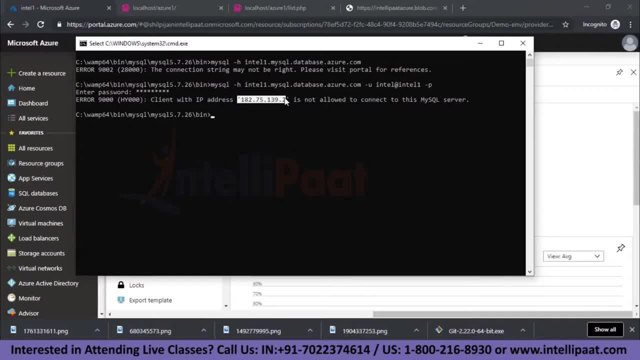 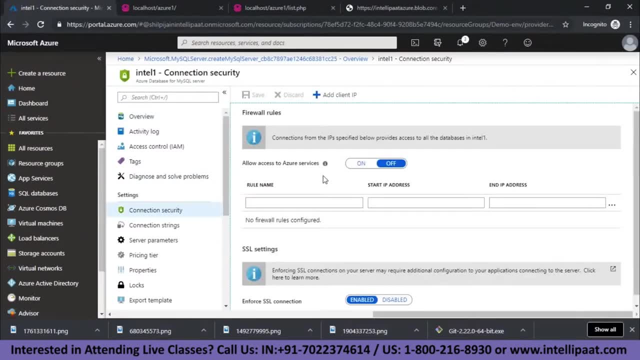 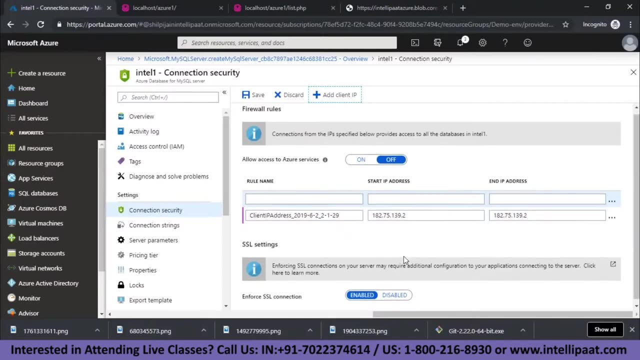 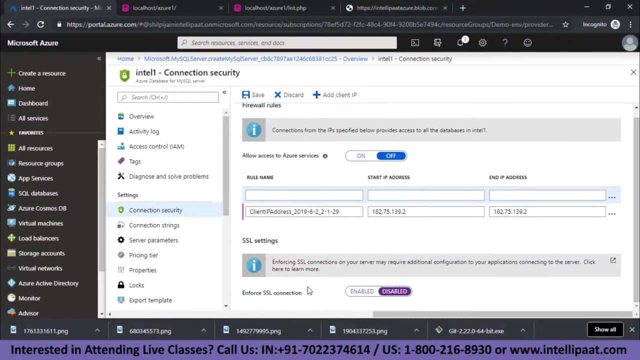 it says: client with ip address is not allowed to connect to this mysql server. So let's solve that. Let's solve that. So we will go inside connection security And what I want to do is I will specify my client IP, which is this: All right, That's been added. Also, guys, turn this enforced SSL connection off, because right now, we don't want to get into making an SSL connection, since this is a demo. 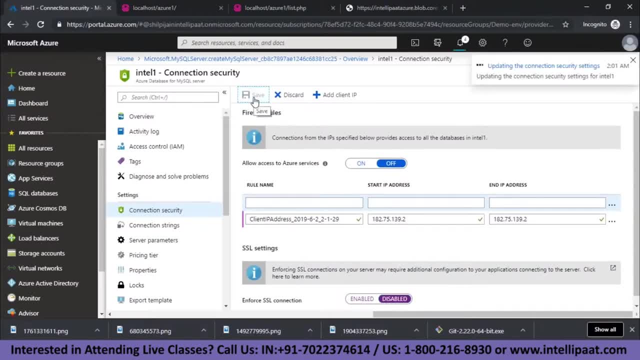 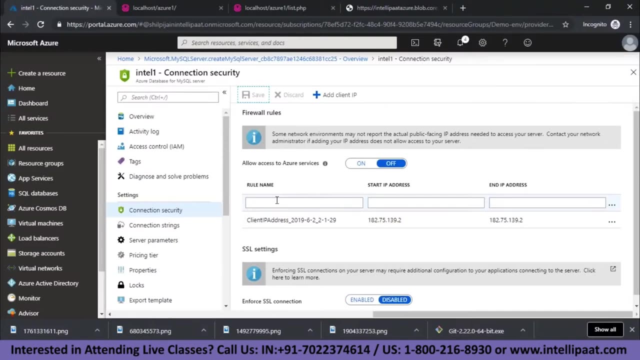 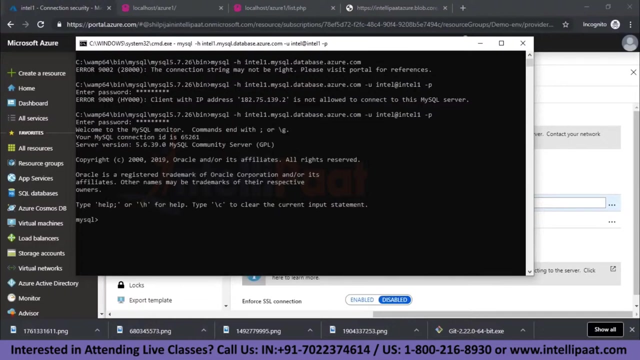 All right guys, everything looks good. now Let's click on save And once this rule has been saved, what we'll see is that we should be able to connect to our database. All right guys, so it says it has successfully updated the connection security. And now, when I go back to my command prompt and I try to enter the same command with the password Azure Ether 8, 1 to 3,, you can see I have successfully connected to my MySQL database on Azure. 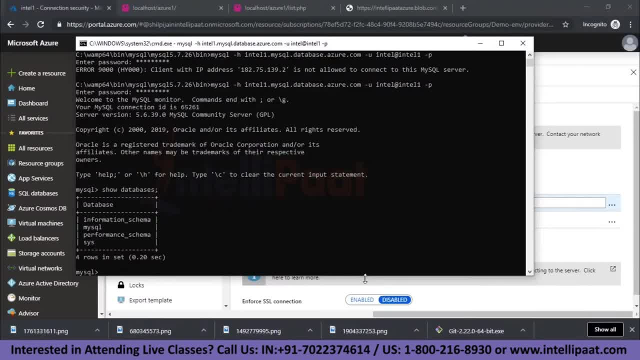 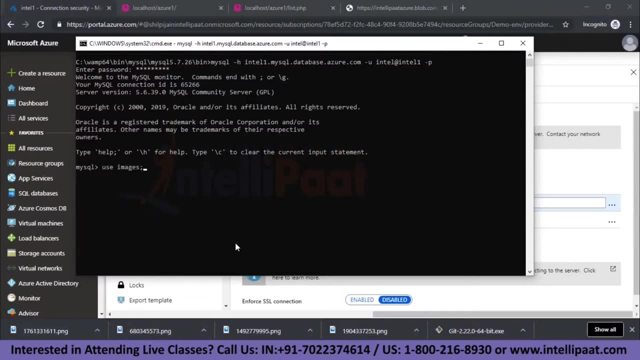 Now, if I do a show databases right now, you can see there are only the default databases present. So let us change that. So I'll just exit. or, before exiting, let us just create an empty database which is images. So we'll use images And let's create a table. So create table names And the names will be names, space, barcat, 20.. So we have created a table. 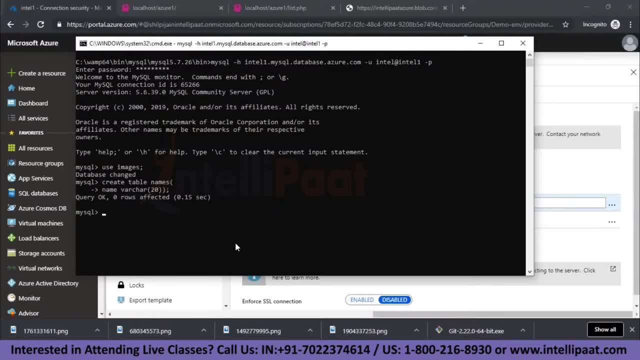 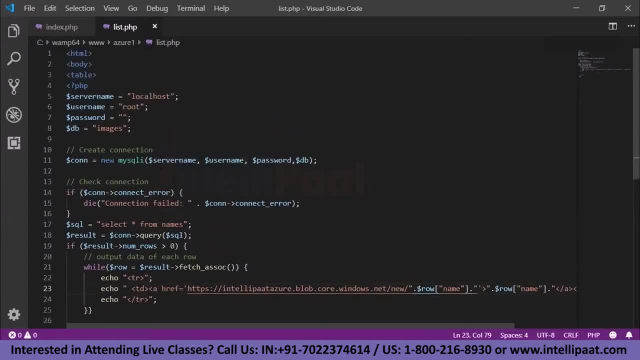 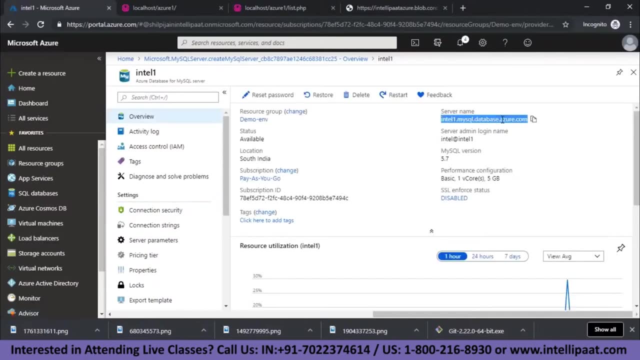 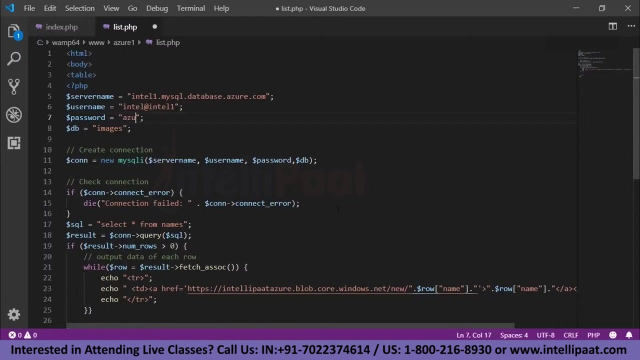 created it. and now let's just go to our code. so the code is over here. this is my code, guys. now i will have to specify the server name. so server name in my case would be this: let's copy it. this is my server name, my username is this and my password is azure. at the rate one, two, three. 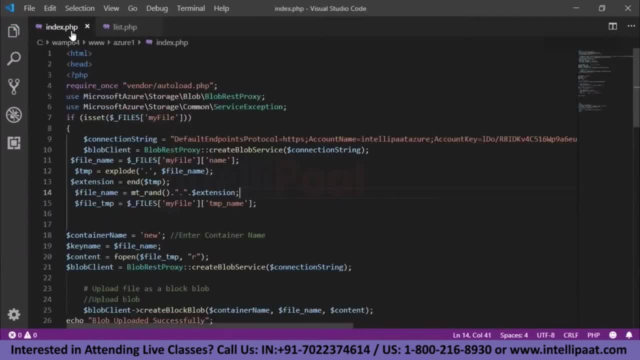 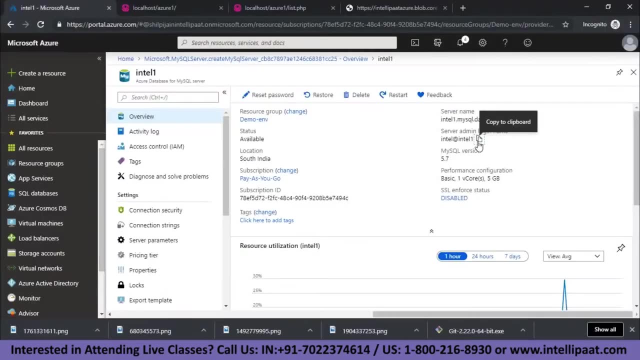 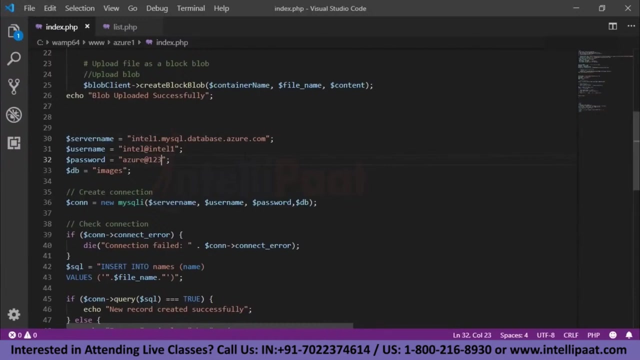 okay, everything looks good. let's save the file. similarly, in indexphp, let's do the same changes. my server name is this: let's copy it. my username is this: let's copy it. and my password is azure. at the rate. one, two, three. all right, let's save the file. and now let's go to our website. let's. 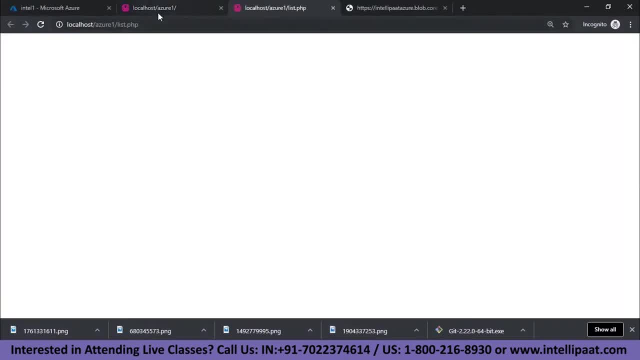 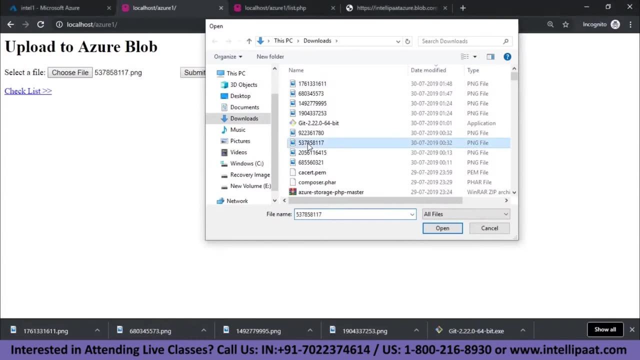 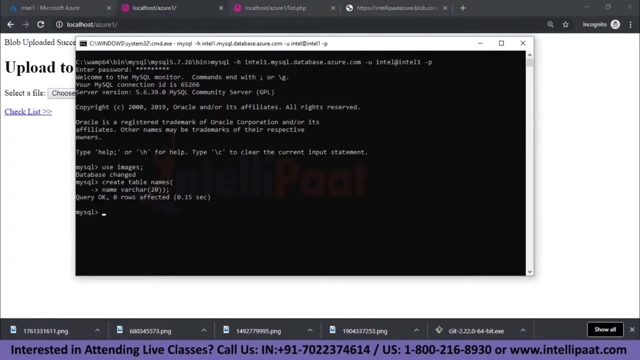 try to check the list. let's see what it shows us. it shows us empty because there's no data in the azure sql table. great, now let's choose a file. and now let's try to upload some random file. let's click on submit. it says blog updated successfully. new record created successfully. let's check that, so i'll. 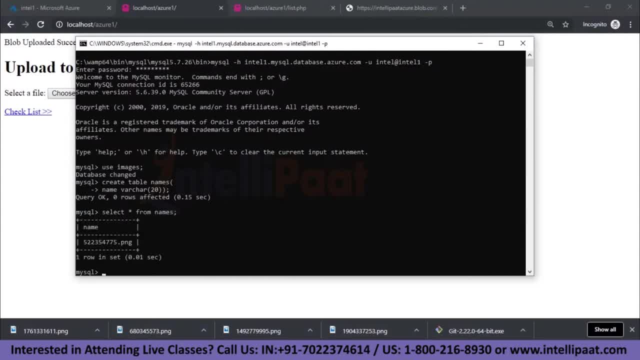 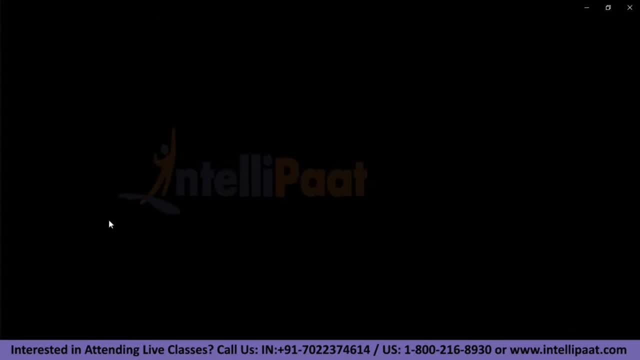 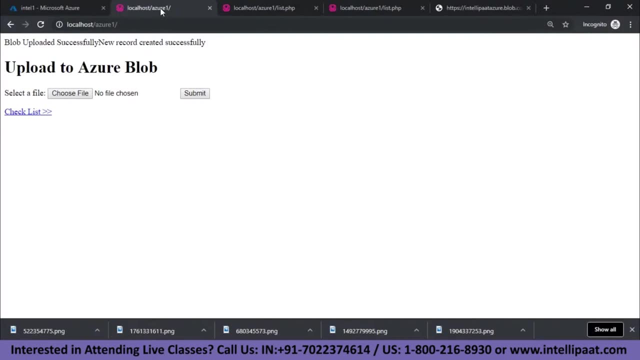 just do a select, start from names, and i can see that there is a new entry over here. if i do a checklist, this is the new entry. if i click on this, i can download the file, and this is the file that i basically uploaded. great, now my website is updating data. 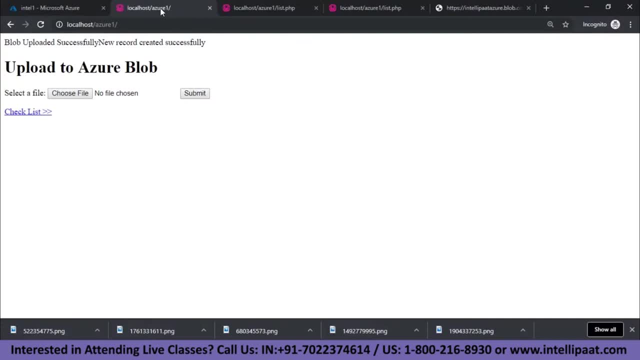 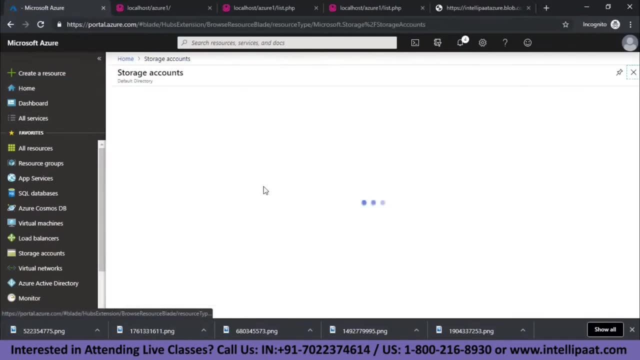 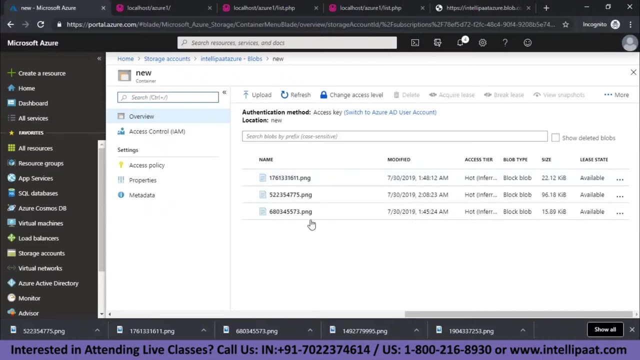 on my azure sql table. so i'm going to go to my azure sql table and i'm going to go to my azure database and at the same time, it is uploading data onto my storage account inside the container, which is new, right? so let's go inside blobs, let's go into new, and this is the. 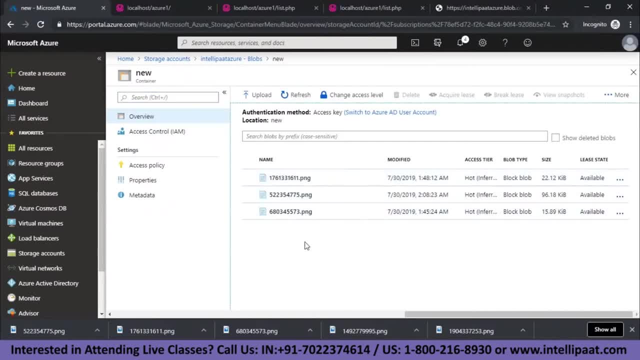 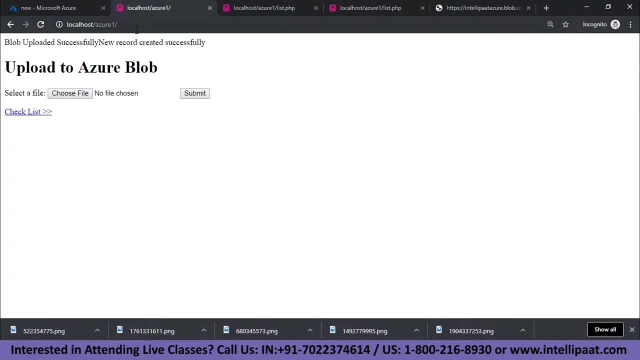 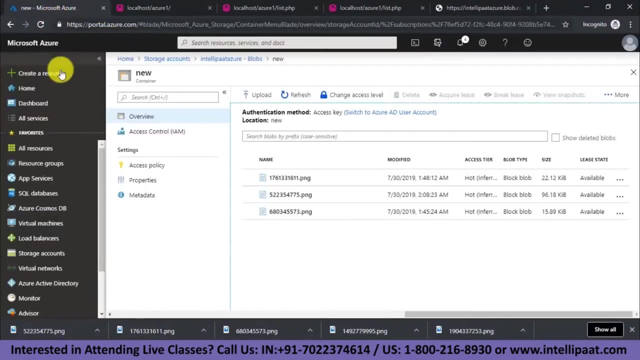 new file, which was basically just uploaded. great guys. now what i want to do is i want to make this website public, right? this website is working fine over here, so i'm going to go to my azure database, but i want this website to be used by everyone in the world. now, how can i do that? in order to do? 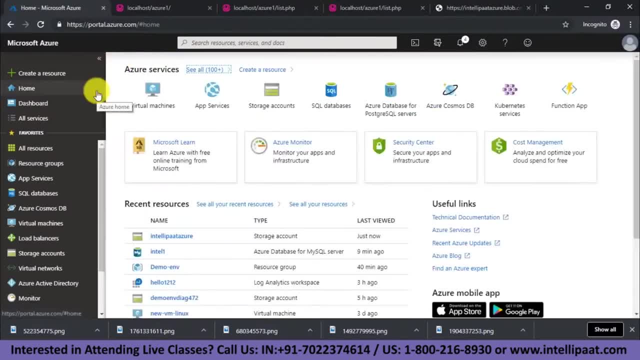 that i will have to go on to home and we studied or we saw a service which can basically just upload our website and not ask us to install any software, not ask us to log in into the operating system, do some configuration, nothing. it will just give us a dashboard through which we can upload our website. 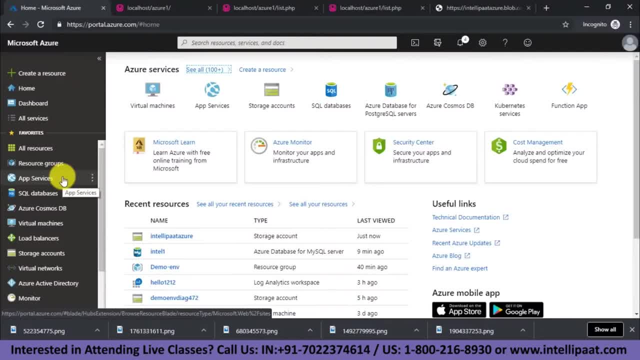 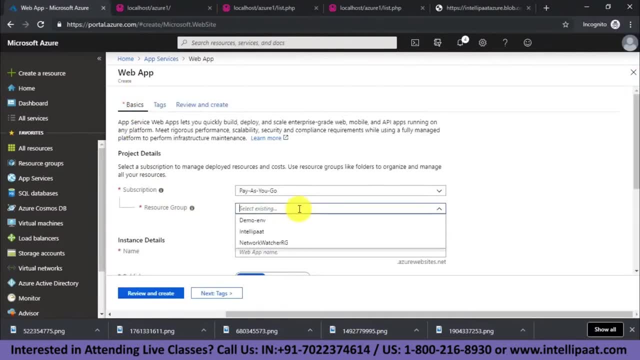 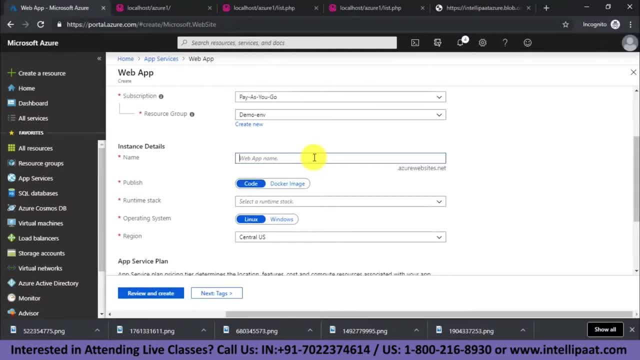 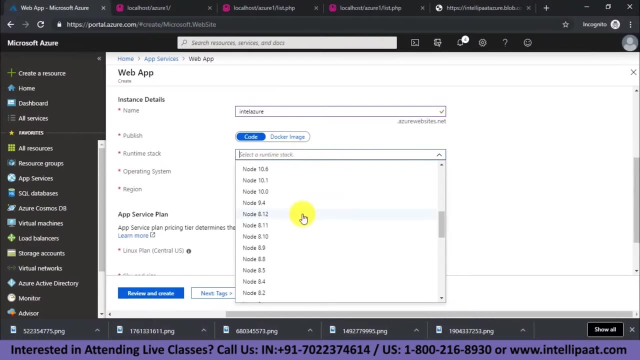 demo environment- name of the instance. let's specify it as intel demo, all right. okay, it's already been taken, so let's specify intel azure. all right, this seems to be available. uh, what do you want to publish? i want to publish the code, the runtime stack. it's actually php 5.0. 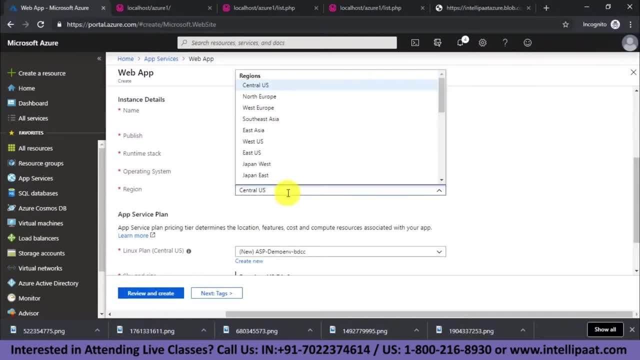 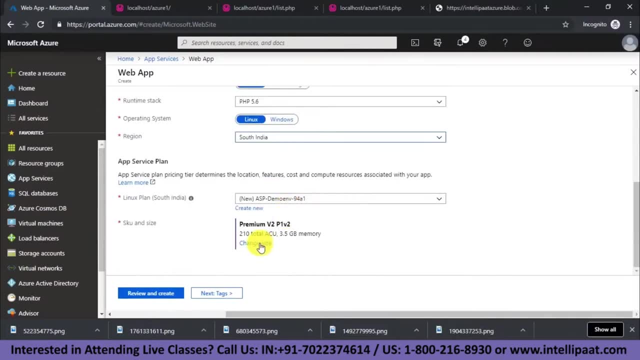 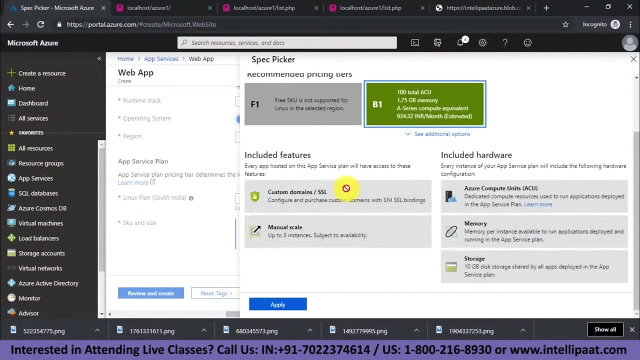 6. this is the one. what is the region that we want to deploy it in? we want to deploy it in south india. so let's select that. south india, this is the one. great. uh, let's change the size of the server which will be launched. so, basically, we are in dev or test environment, right, and this is the minimum. 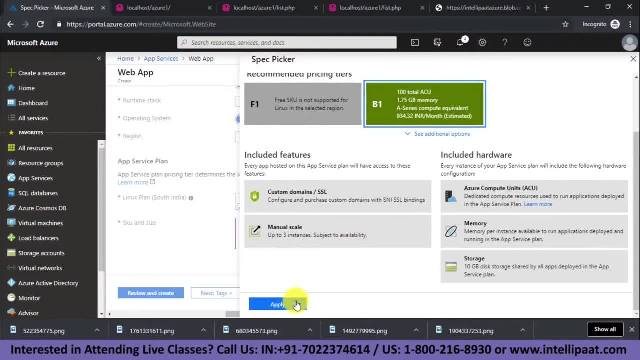 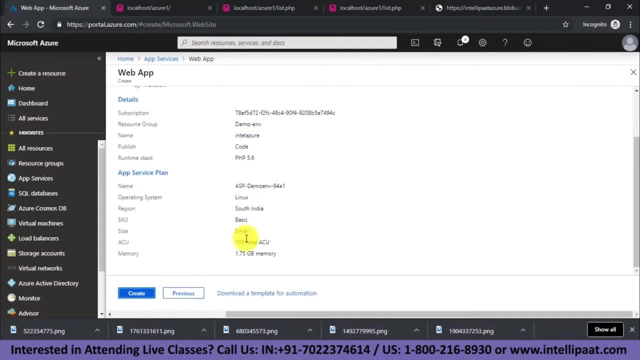 configurations that we can launch. all right, let's click on apply and now let's click on review and create. so this, over here, we can basically do all the change, uh, all the necessary review as to what all we are launching. so we just selected php 5.6 and we specified the name of the app. that's all we did. right now, let's click on create. 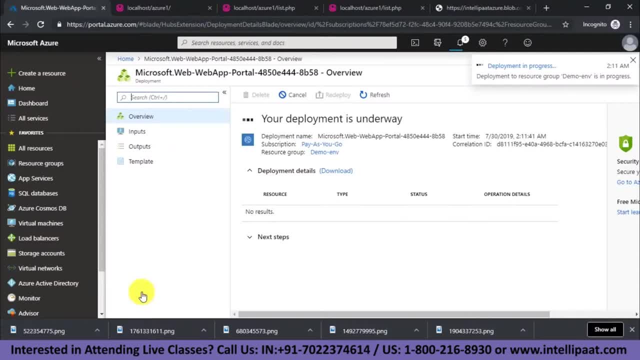 now, guys? what will happen now is it will basically deploy a server on which it will install php 5.6, install apache, and then it will give me a url and when i go to that url, i will basically see a sample app. right, it is not giving me access to the operating system. 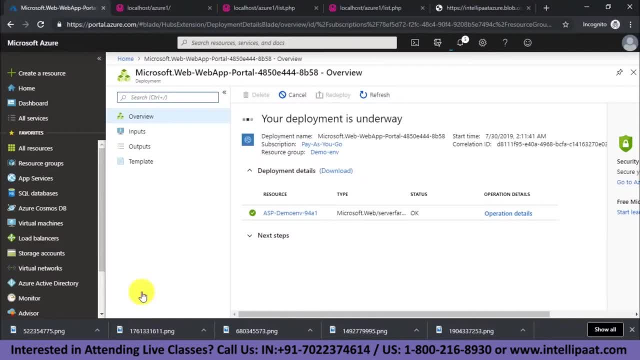 it is not asking me to install any software. all that was done over here was we selected the runtime stack, which was php 5.6, we specified the server configuration and that is all. that is all we need to configure and that is all we get access to now. once it gets deployed, i'll show you, guys, how you. 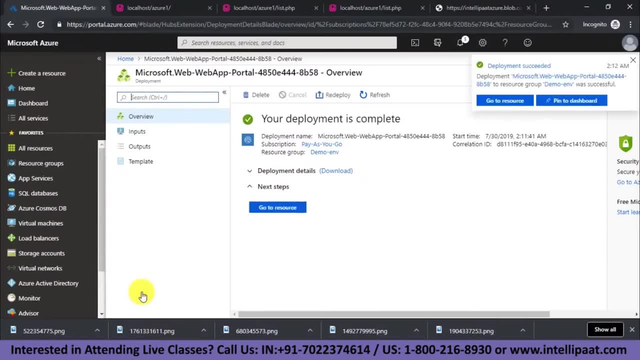 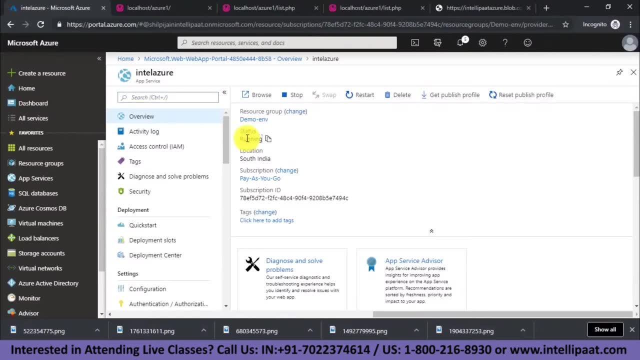 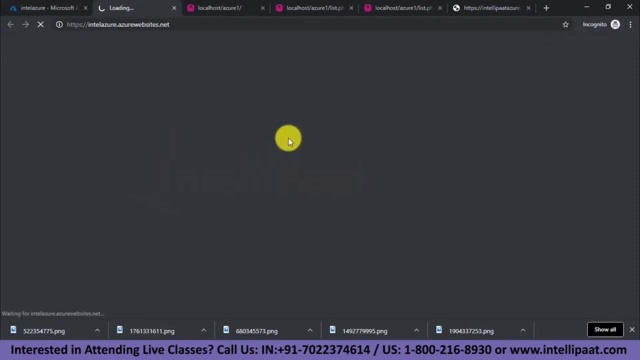 can upload your code onto this particular web app. so, as you can see, it is already deployed. now let's go to resource, and this is the resource guys. the status is: it's going to be the same as the web app. so it's running right now and if i browse this web app right now, it'll basically show me a. 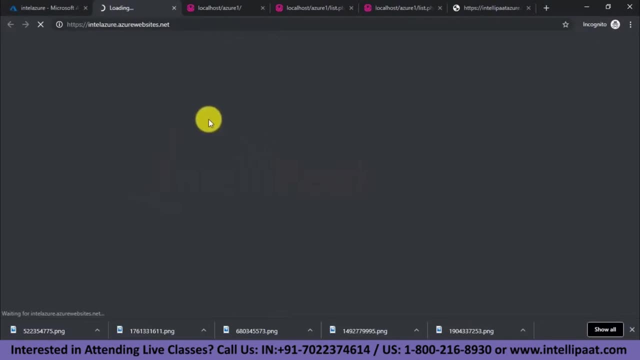 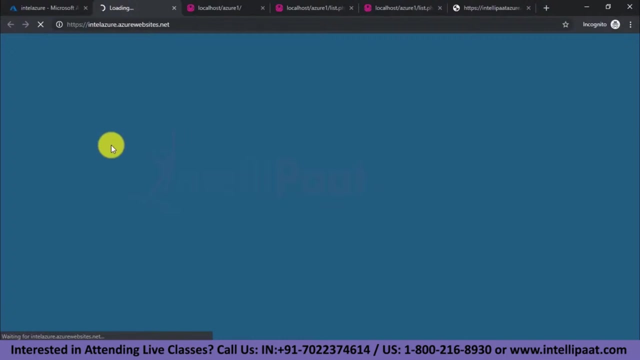 sample web app which has been deployed on it. right, let's wait for that website to appear. since this uh web app has just been launched, it might take some time for the web app to show the website, but nevertheless it will show the website, so let's wait for it to actually show us. let me 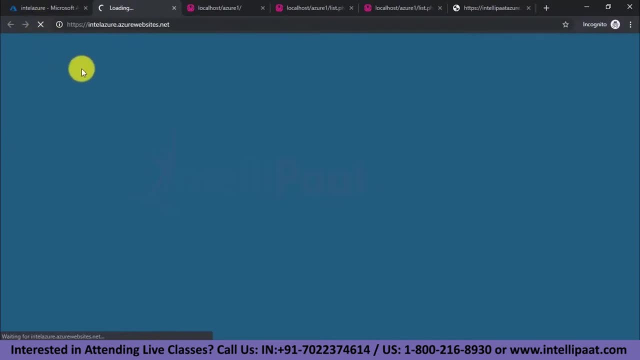 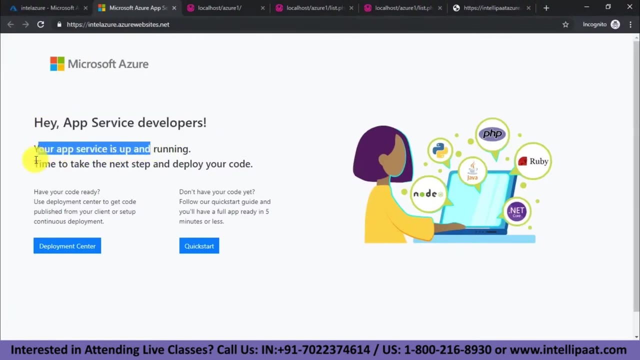 try stopping it and refreshing it once. all right, it's going to take its sweet time, so let's go with that, all right. so as you can see, hey, app service developers, your app service is up and running. time to take the next step and deploy your code. great, so this is what you want to do. 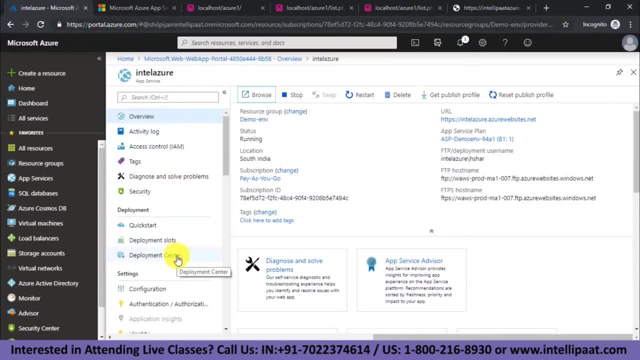 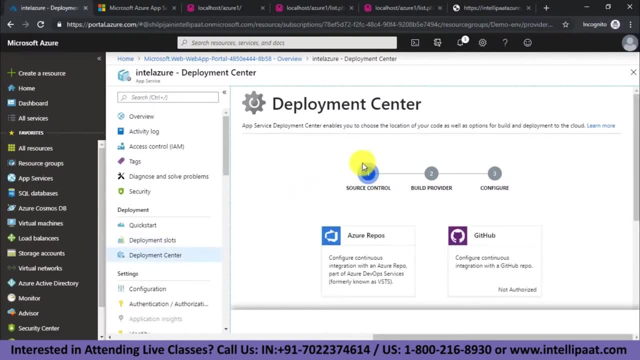 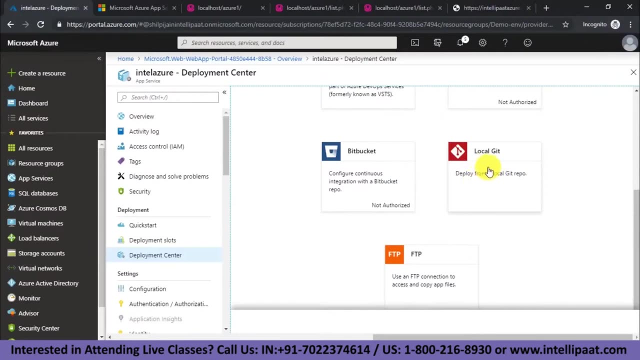 now, to deploy your code you will have to go inside deployment center. so let's go inside that. so once we're inside deployment center, it's asking me: where is my source control? right? so my source control is basically on my local, right? so? but it- my local- is not a git repository. 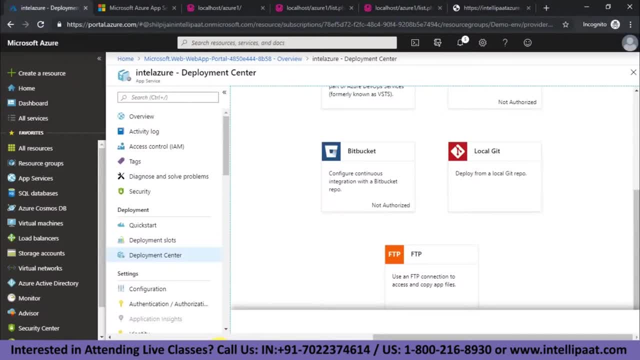 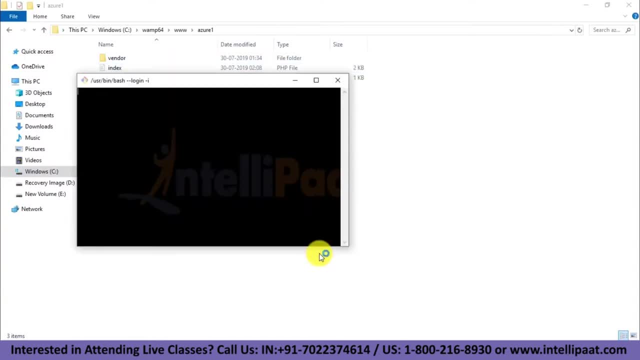 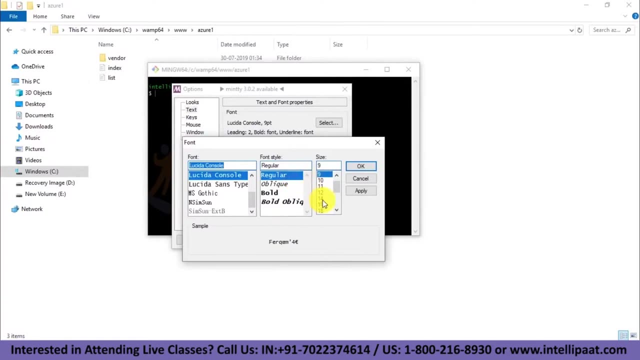 as of now. so what i can do is i can just go on my code, which is over here, as your one. this is the folder, and let me just right click here and click on git bash. right, let me just make the text a little bigger for you so that it is visible, all right. so, guys, now what i'm going to do is i'm 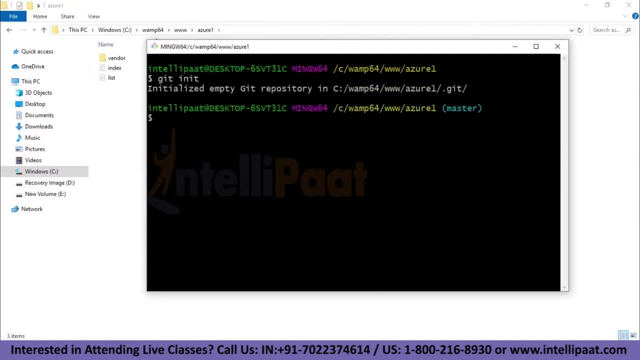 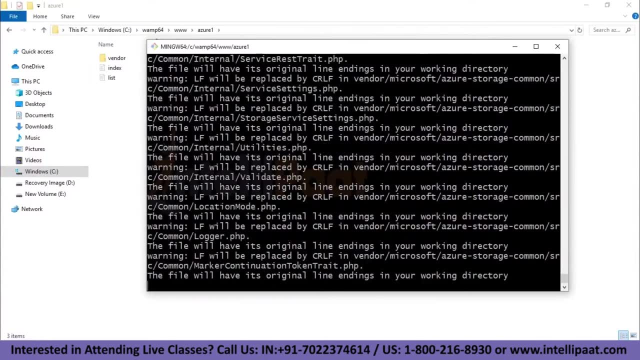 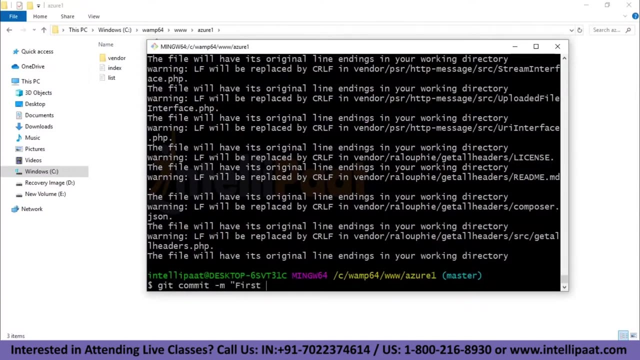 going to initialize an empty git repository, so get in it. and now i'm going to add all the files in the git file system. i'm going to stage it for the git file system. so once this process is done, i'm going to commit it. git commit hyphen m. and this is my first comment. now it's going to save the files. 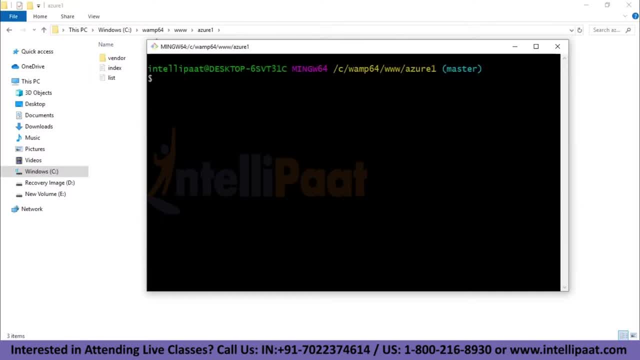 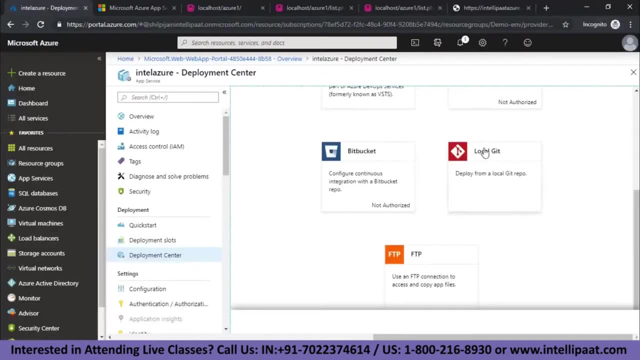 great, so the files are saved. now what i want to do is i want to upload this particular code onto my azure web app. right, so going back to the portal, i do have a local git where i have my code checked in, so let's select this option and click on. 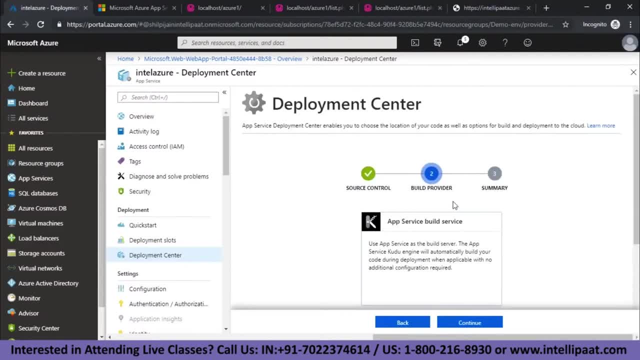 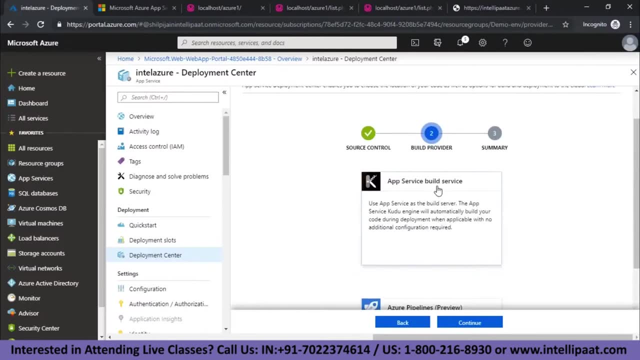 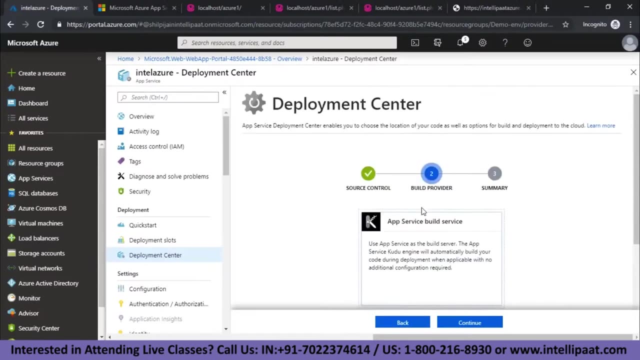 continue. now it's asking me which build provider to choose. uh, don't worry about here. don't worry about what is azure pipelines and what is kudu engine. basically, if you select kudu engine, you don't have to do any configuration. more on this we can discuss in the further sessions, but right now, 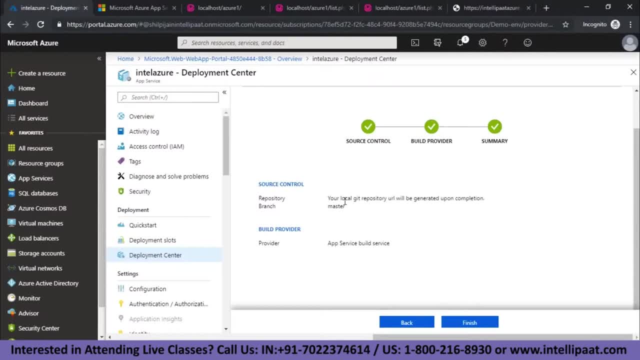 just select the kudu engine and click on continue. and now it says your local git repository url will be generated upon completion. branch would be master. app service is build service- great, let's click on finish. so now it is basically going to set up the git environment for me on the web app. 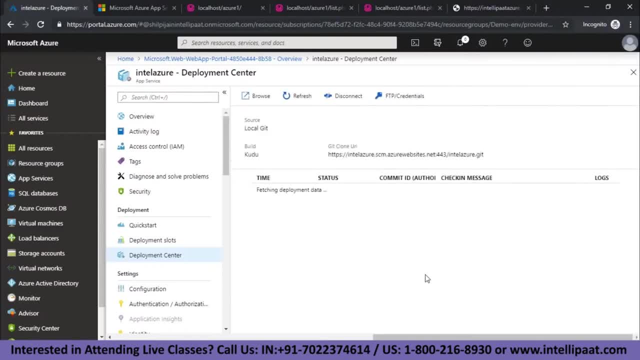 server and what i will get is basically this url, which is my git url. so this url i'll be using to upload my code. but before that i will also have to set the credentials for my git system. so to set that, i click over here- ftp or credentials, and i'll go to user credentials. 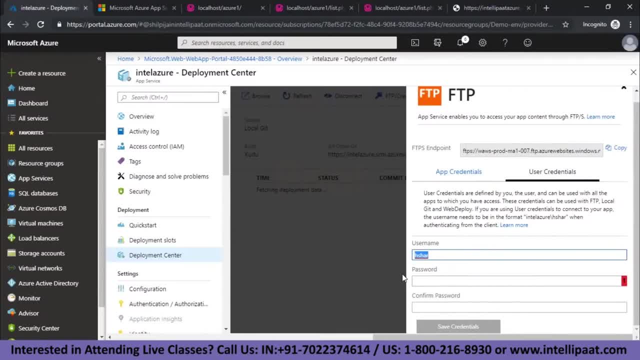 and i can specify anything over here. let's specify a username, let's say the username is intellipaat and let's say the password is intelli at the rate one, two, three. intelli at the rate one, two, three. and now let's click on save credentials. so it says saving credentials was a success- great. 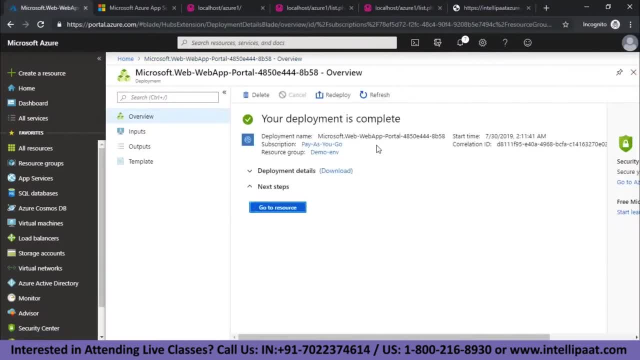 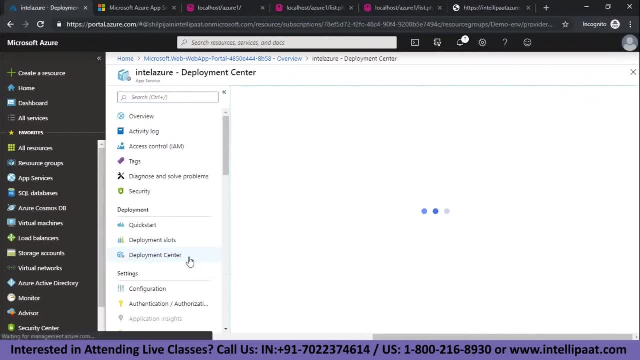 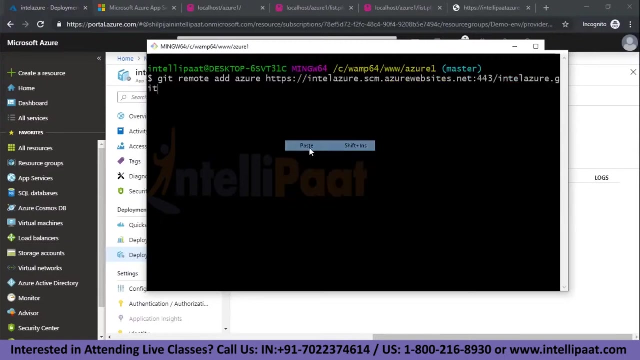 now what i can do is: i can just close this, and now i'll just have to go to my resource, i'll have to go to deployment center and now i will just take the git url over here. all right, this is a git url. let's copy this. and now git remote, add azure and let's try to paste. 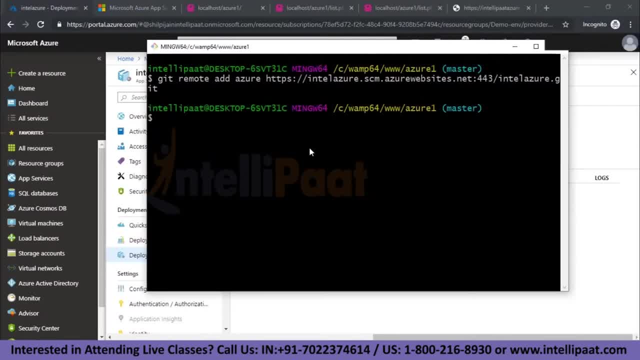 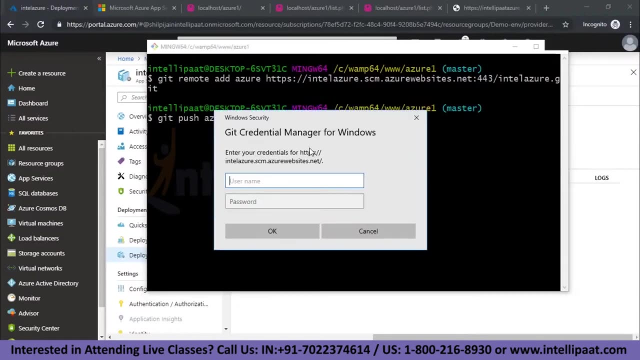 this link now. yes, so this was the syntax. git remote, add azure right. and now what i want to do is i want to push my code onto it. so git, push azure master. i'll hit enter and i'll ask me the credentials. so credentials is intellipaat and the password is intel at the rate one, two, three. 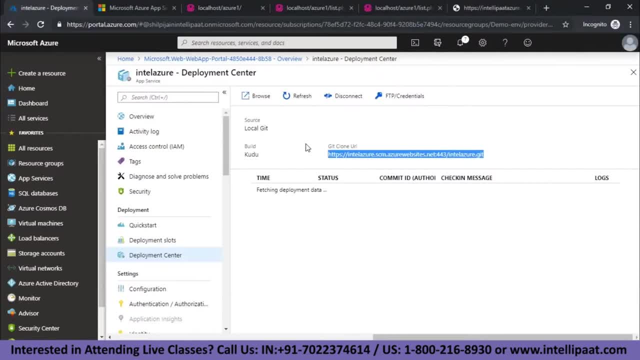 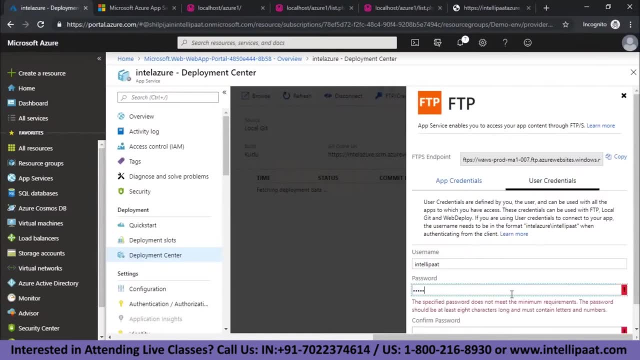 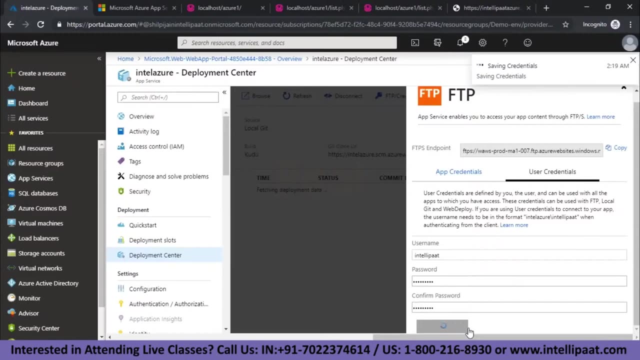 oh, authentication failed. i think i forgot the password. uh, no issues, guys, so i can just specify it again. so intel at the rate one, two, three and intel at the rate one, two, three. let's save the credentials. okay, credentials are saved, let's go back here. git push azure master. 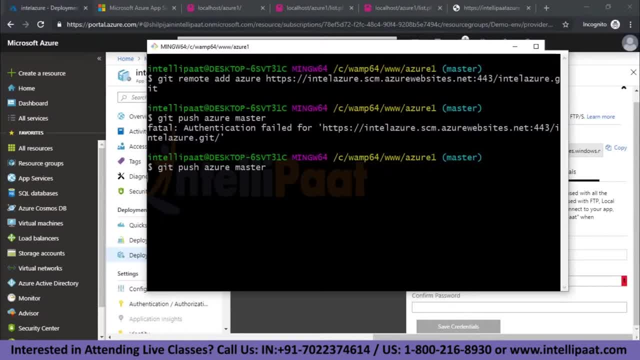 and now it should basically push my code onto the web app. now it will take some time over here, guys, don't worry about the time. it will take around a minute or so to upload your code. so let's wait for that time and let's hope everything goes well. all right, the process. 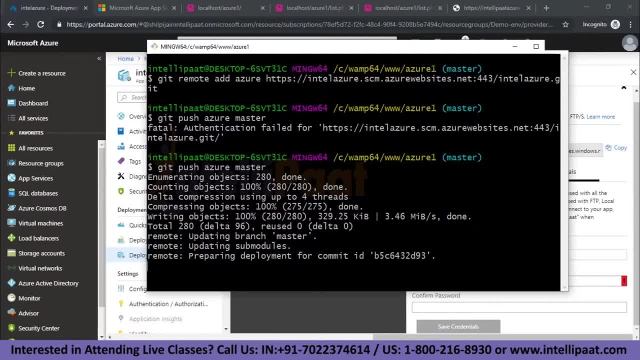 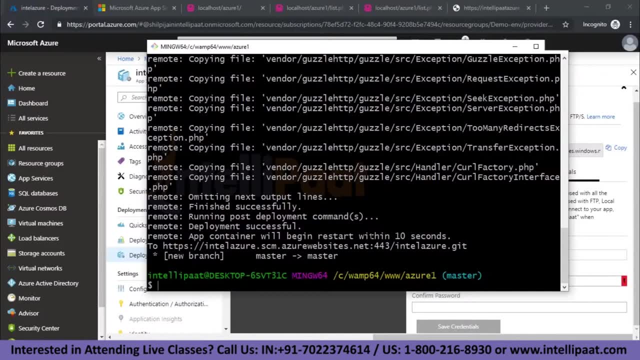 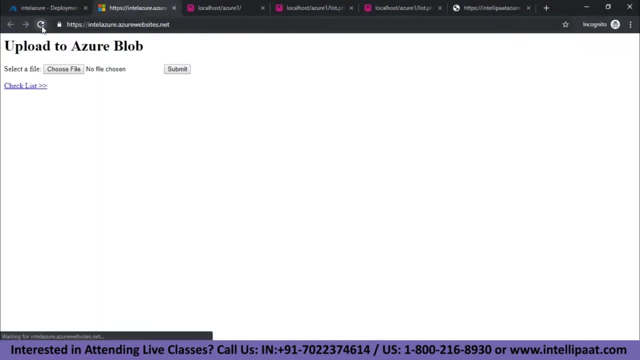 has started, so it is updating the branch now copying all the files- great. so my code is now uploaded on the app and it says it will restart in 10 seconds. great. so meanwhile, what i can do is i can go to my web app and i can just refresh this and, as you can, 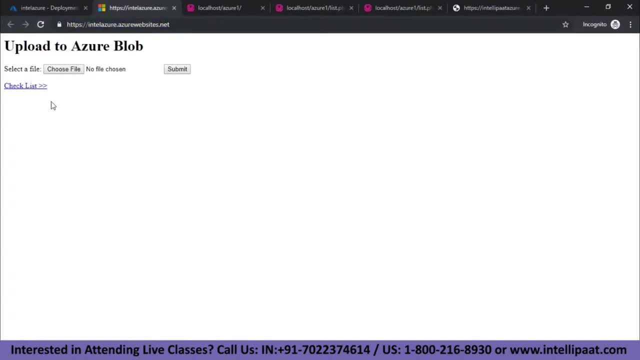 see my website is now available over here, right? if i click on checklist, you will see an error and i'll tell you why that error would be there. it says: connection failed. client with ip address is not allowed to connect to this mysql server. now how can you solve that? just go to home and go to. 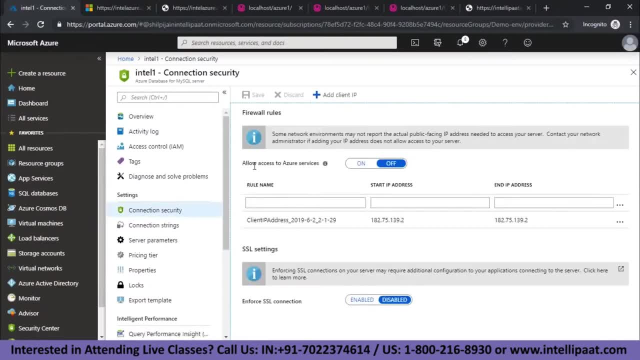 your database. go to connection security and allow this. allow access to azure services. just click on on and, as a security feature, just remove the ip address that you used earlier and now let's click on save. so now my security settings will get updated and then i would be able to use my website. 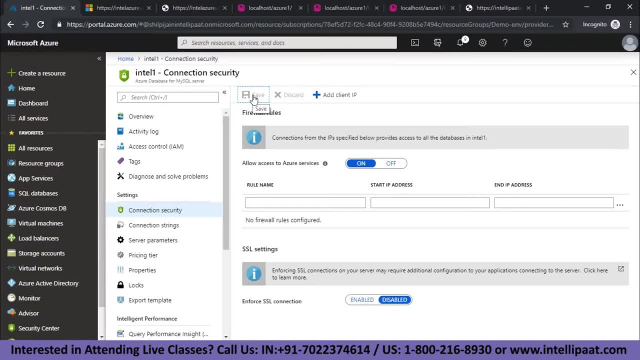 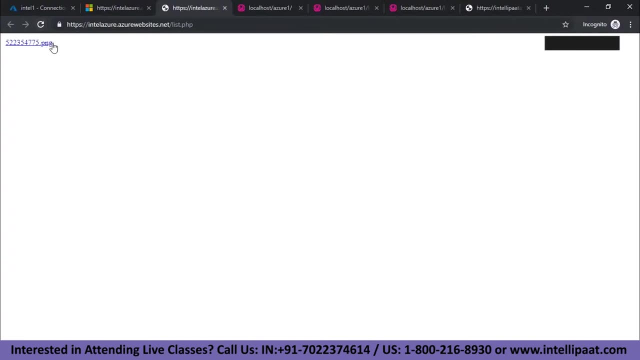 on the web app. all right, so my settings are about to be updated. let's wait for that time and then we'll go ahead. all right, guys, so my data is has been updated successfully. so if i go here back and i click on refresh, you can see the list is now being generated. let's try to upload a file, guys. 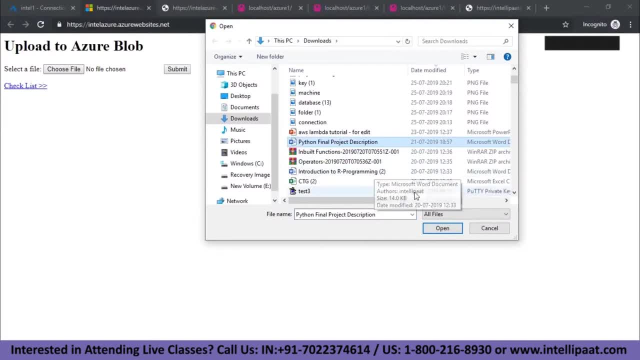 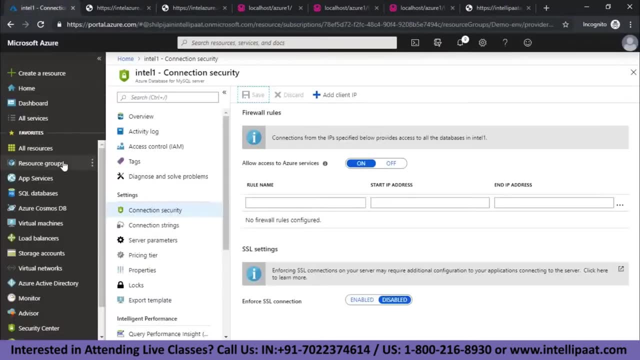 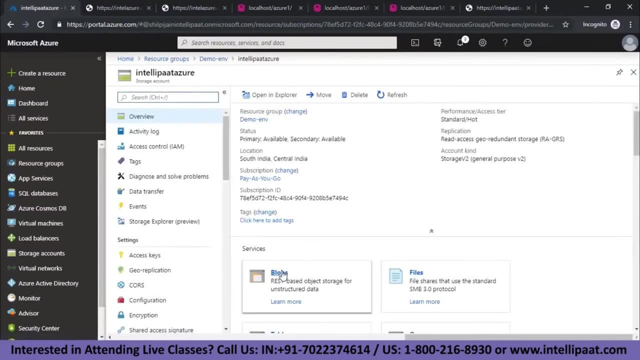 let's try to upload. let's try to upload this word file: okay, let's click on open and let's click on submit. it says blog updated successfully. let's check that. let's go to our resource group. let's go to our storage account. let's go inside blobs inside our container, and this is the docx file which was just updated. 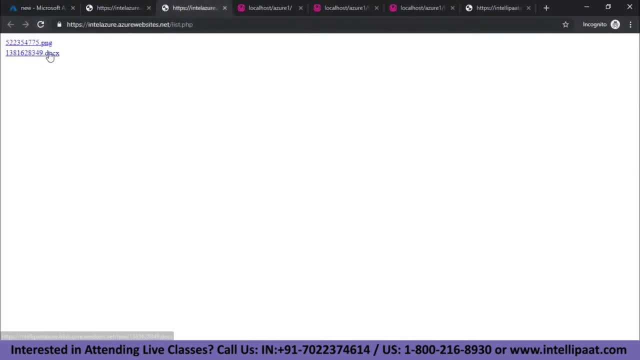 and if i refresh the list, i can see the docx file over here as well. if i click on it, i'd be able to download it. and, guys, with this we have successfully completed our demo. but let me show you a very awesome thing that comes with connecting git to your web app. right, so now i can just simply go. 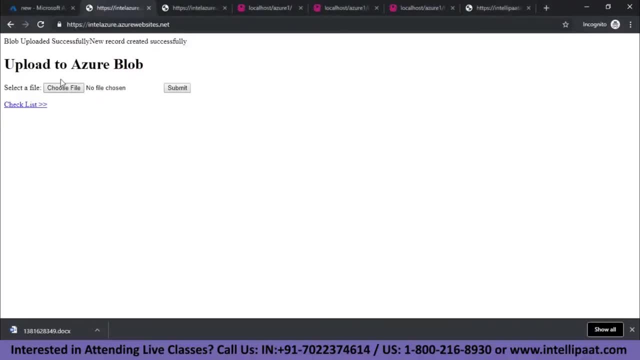 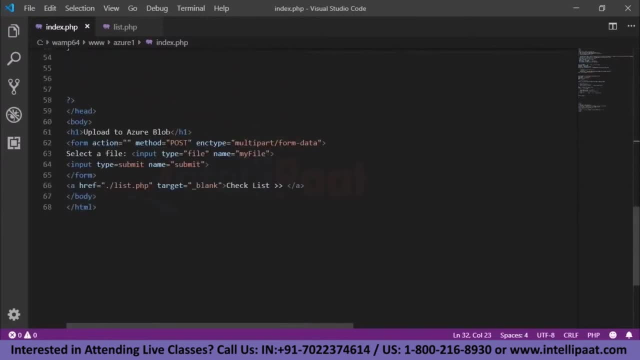 to my indexphp and let's say i want to change this heading. okay, so let's try to change the heading. i'll just go down, upload to azure blog and let's add a little bit of text. over here let's say welcome to intellipa. okay, let's save it. come back to our git terminal. let's do a git status. 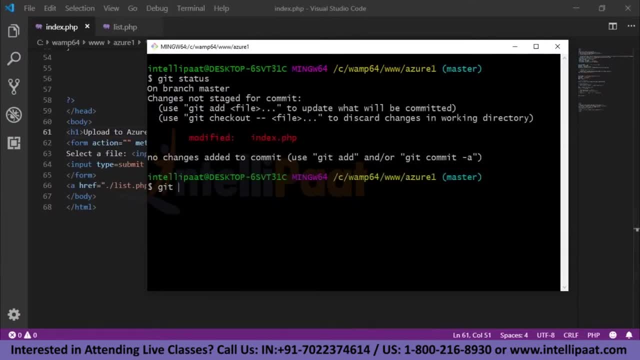 you can see that indexphp has been modified. great, let's scale this file, let's commit this file. updated index: great, and now let's push it. so git, push. azure master will again take a minute or two and then our files will get updated on the web app automatically. all right, so my code has been. 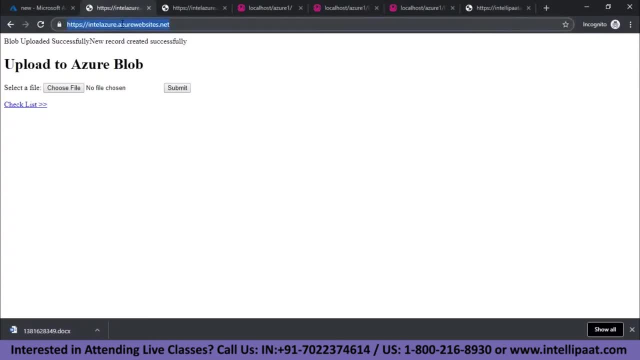 updated. let's go ahead and check it. so let me just refresh this website and, as you can see, my code has successfully updated. over here it says: upload to azure blob. welcome to intellipaat. and this is exactly what we changed. all right, so, guys, with this we have successfully completed our demo. let us summarize what all we 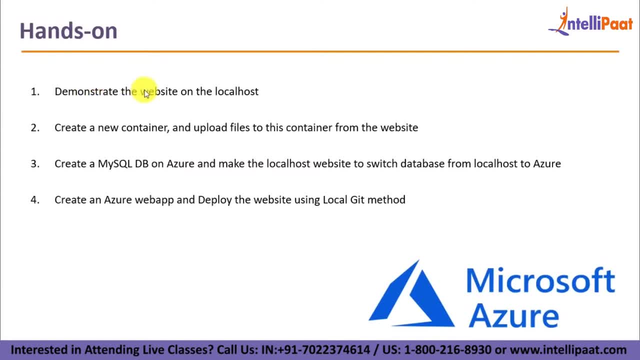 did so. let me come back to my slides. so we demonstrated the website on the localhost, which was working fine. then we created a new container and then we uploaded all the blob files over there. after that we also deployed a mysql database on azure and the localhost website. 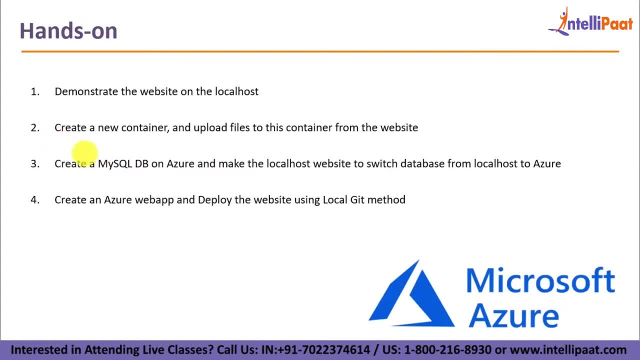 was then able to insert data onto the mysql database on azure, and then, finally, we also deployed an azure web app and we deployed our website using the local git method and finally, we also checked if we updated anything and we pushed through our git method. the files were successfully. 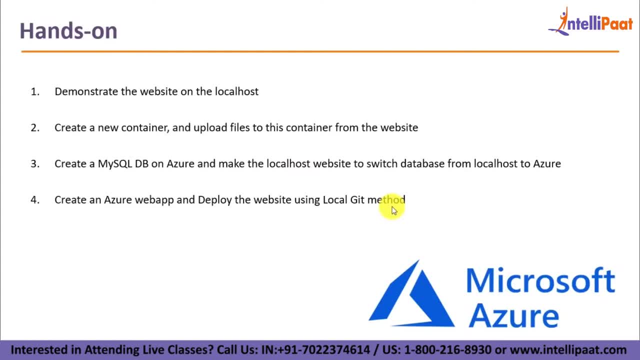 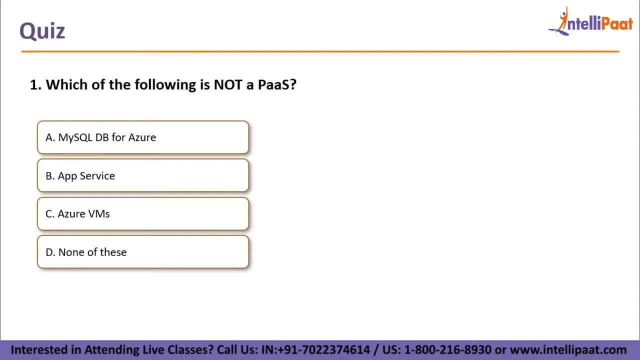 being uploaded onto my azure web app. right, all right, guys. so our first question is: which of the following is not a platform as a service? and the options are: mysql database for azure app service, azure vms, or is the answer none of them these? the answer is: as your VMs. the next question is: can we deploy as your VM? 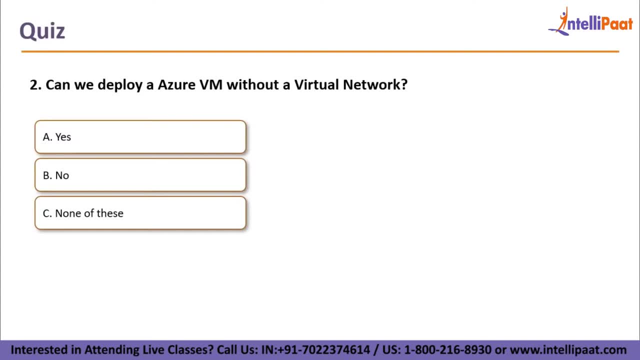 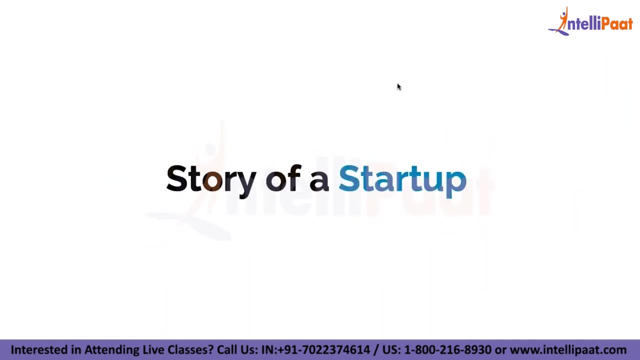 without a virtual network. so the options are yes, no or none of these. the answer is no. so let's take the example wherein let's say: you guys want to start your own company. let's talk from that perspective and then we'll understand why big companies are using cloud platforms like as you are today. all 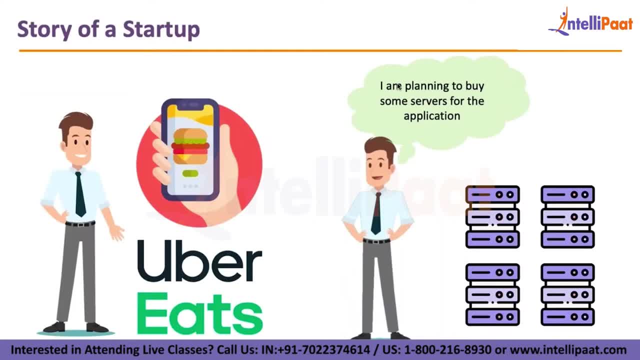 right. so let's say you're a guy who just wants to open a food platform. let's say you're, the food platform that you want to open is Uber Eats. okay. so if you want to open an application like Uber Eats, what is the first thing that you have to? 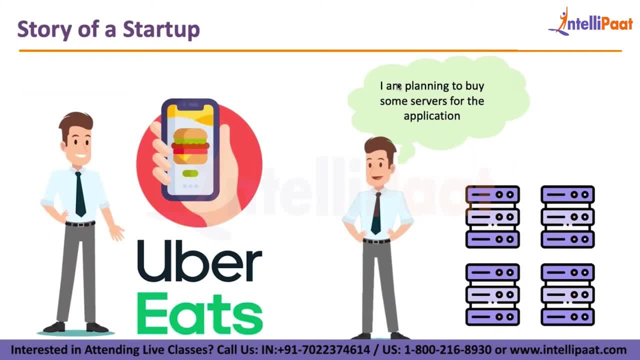 do so. obviously, first of all, you will have to have an application right which, basically you will be developing and which will basically work right. so let's say you hired a team of developers and you've done that. so now your application is ready and now the next step is basically making it available to the world, right making it. 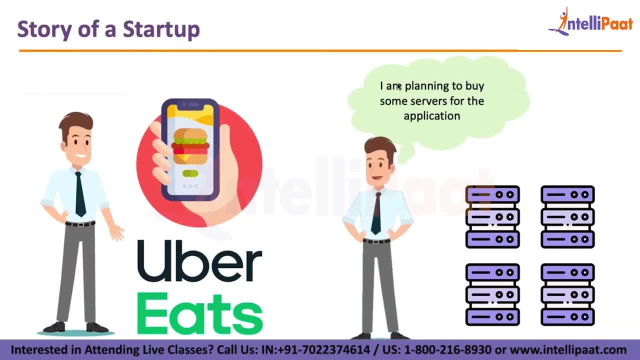 available on the internet. so how will you do that? so for doing that, guys, first of all you need to host that application on a server. okay, now, when you're starting small and let's say there are four or five people who are going to use your application, you can do that using your own laptop as well. now, when you're 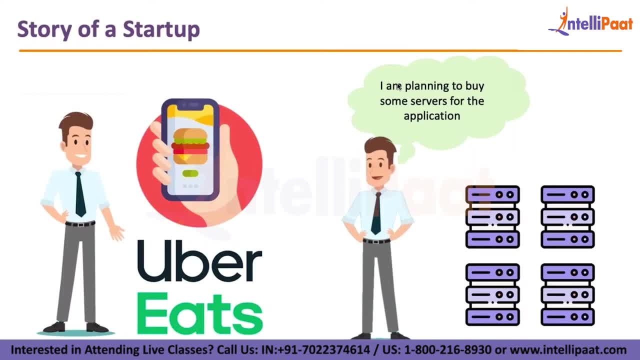 doing it from home, you're going to be able to use your own laptop as well. so now, when you're doing it from home, you're going to be able to use your own, using your own laptop. let's say you have developed the application right and now you want to push on the internet. so what you do is you basically run that. 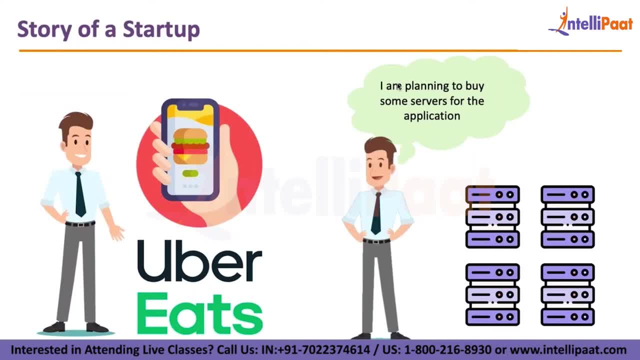 application on your laptop, you connect it to the internet, right. and obviously there are certain other things as well that you would need. for example, you would need a static IP of your laptop, which an IP which is not going to change any time, right? and at the same time, you will also need 24: 7 electricity, so that 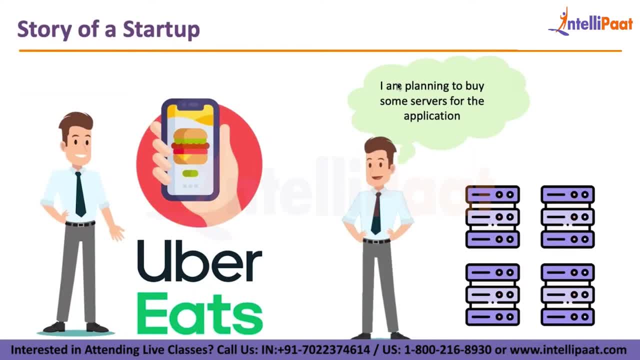 your laptop never shuts down, right? otherwise, if your laptop shuts down, the other people will not be able to use that application. okay, so, guys, this would be the basic setup that you would need to host your application. now let's talk about a scenario where in you know: 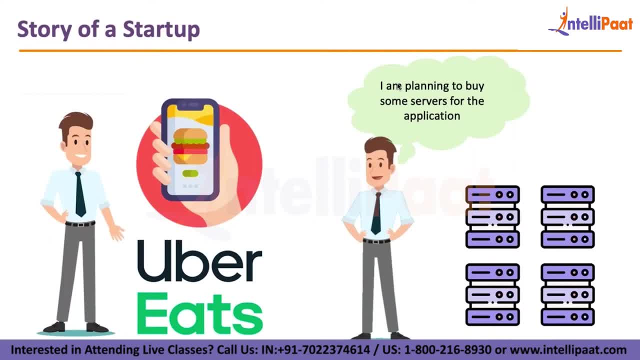 your application becomes a hit overnight and now some thousands of users are using your application. now, obviously, your laptop will not be enough, so what will you have to do so, as you know that? okay, so my application is actually working. a people want to use my application and you know it is going to be a success in the future. now, 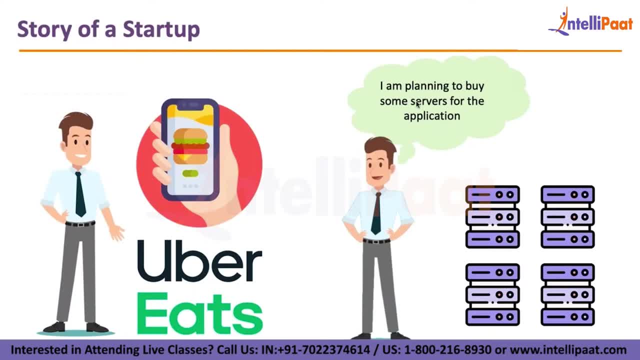 so what you do is you take a loan from some bank or you take some amount from your savings and then you basically buy a set of servers. okay, so those servers take around two to three days to basically get delivered to you. then you basically set them up for setting them up again. 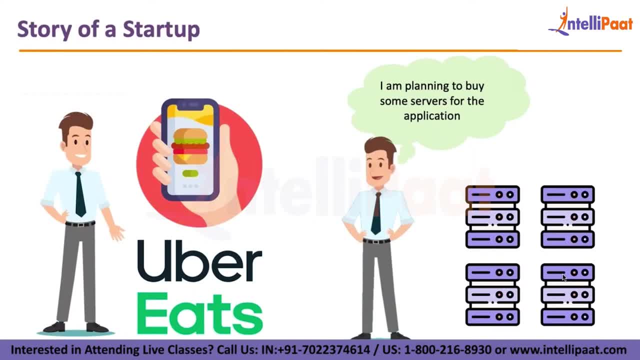 you know you need a team which can basically install the required software on it. then you need a place where you can keep these servers. so you rent some apartment, put those servers over there, you know, connect it to a power backup kind of a facility where, even if the electricity goes, 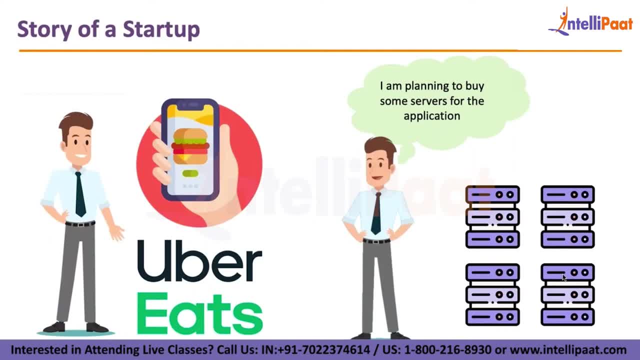 there is a generator which is going to power up your server and at the same time, you basically also contact a service provider, an internet service provider, which is going to give you good internet to your servers. seems everything sorted right, so now you've invested a huge chunk. 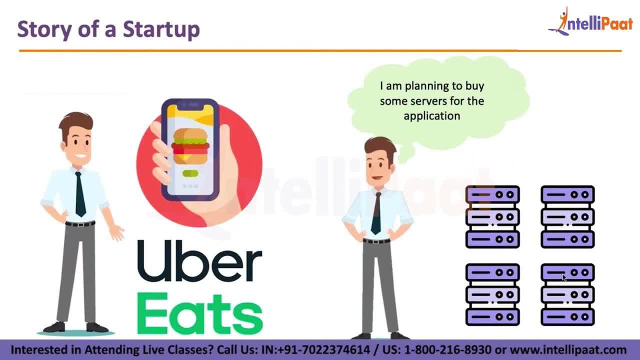 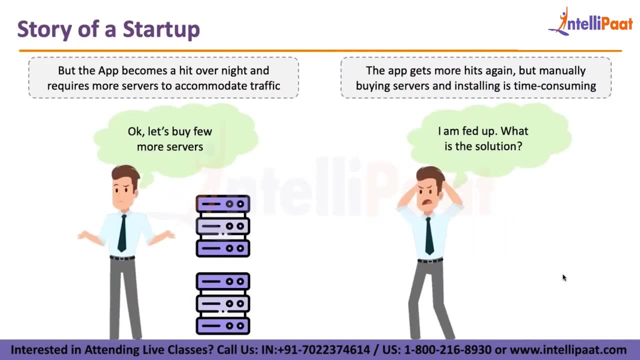 of money on your application, right, and now you have made it available on the servers where thousands of people can access it. okay, now the application again becomes a hit overnight. and now there are more customers who basically want to access your application. and now the servers that you bought, they're not enough. so 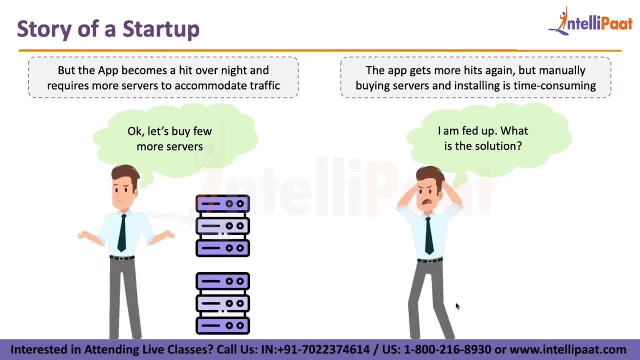 what you basically happens is: uh, you get to know, okay, so more customers are using your application now, and now you suddenly have to buy more servers because obviously the servers that you have to buy are not enough. so you have to buy more servers because obviously the servers that 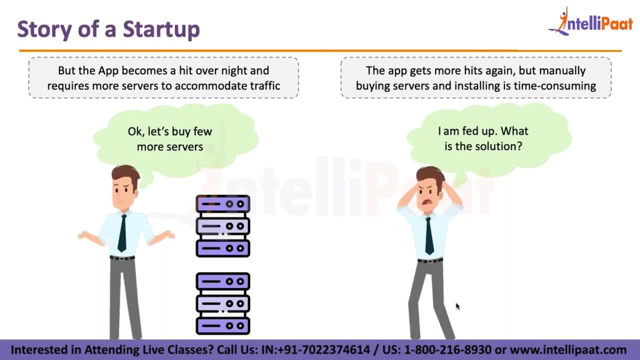 you have currently, they're not uh, giving you the- uh the right kind of performance that you need. so, again, you have to invest some money now. take one thing into account, guys: that servers are very expensive. at the same time, you've also entered a place. you are giving money for the internet. 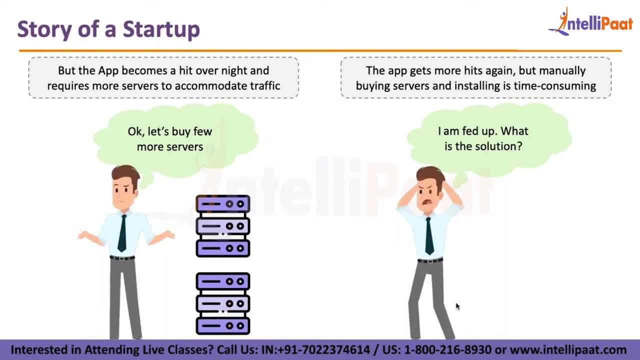 connection. you are giving money for the electricity, so there's a lot of investment required over here to make your application available online to 100 000 of users, or even a million people. right and obviously. you have to invest some money to make your application available online to hundreds of thousands of users or even a million people. right and obviously. 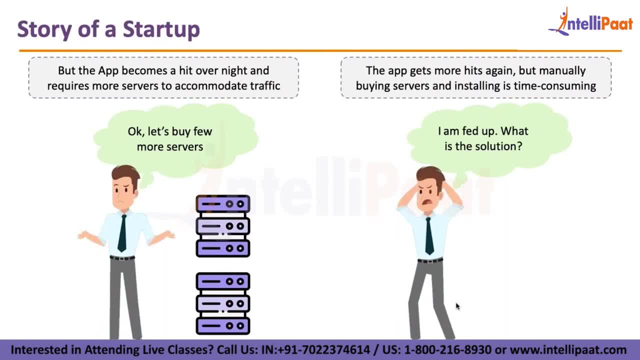 because you know you've just started out, you are not getting the kind of money that you're supposed to do because you're also doing marketing for your application. you're also giving a lot of discounts on your application, because of which you're not getting the right right kind of revenue, right? so 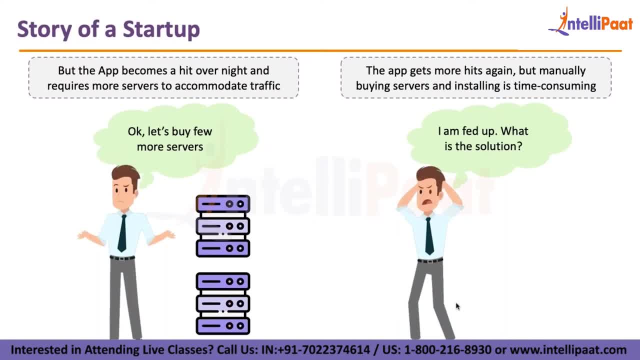 what should you do? so, as and when the traffic will grow again and again, you will have to buy more servers, and that will require more investment from your site. so you get fed up of the solution of this particular situation and now you're looking for ways to basically solve it now, if this kind of situation arose before the 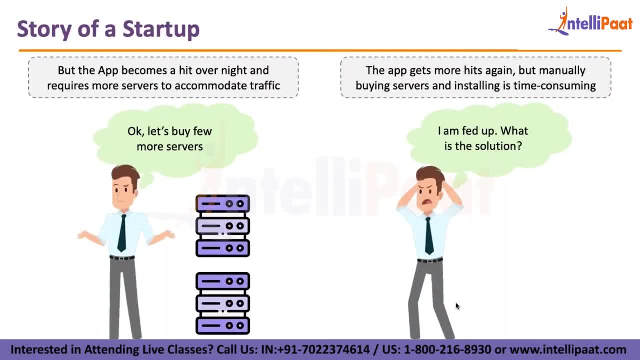 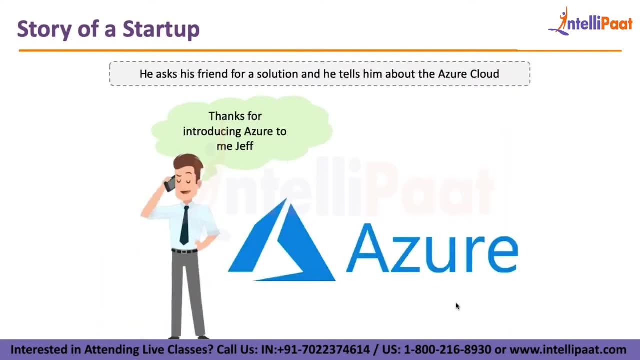 year 2006 or 2005. well, you didn't have any other option that to shut your company or take some loan from a bank and pay the interest also to the bank while you're repaying. uh, you know the amount to them, right? but now with cloud providers such as azure, such as aws, such as google cloud platform, 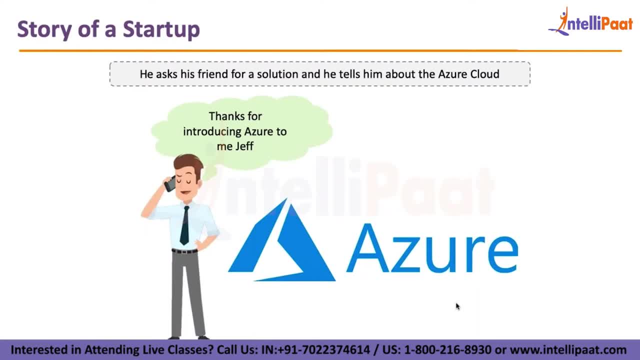 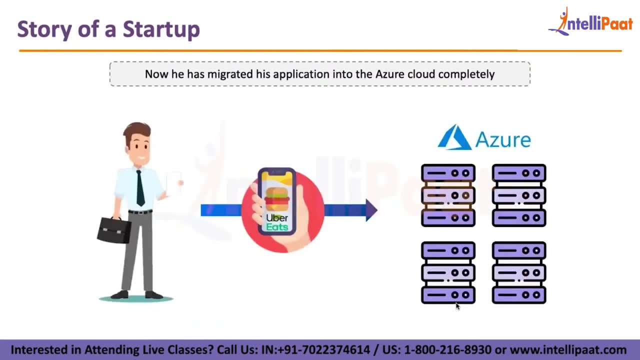 this has become very easy. so what is this cloud platform and how is it going to help you? let's understand that. so, guys, with a cloud platform, what you can do is you can rent infrastructure right. so now let's say you have an application which is ready and you want to make it available. 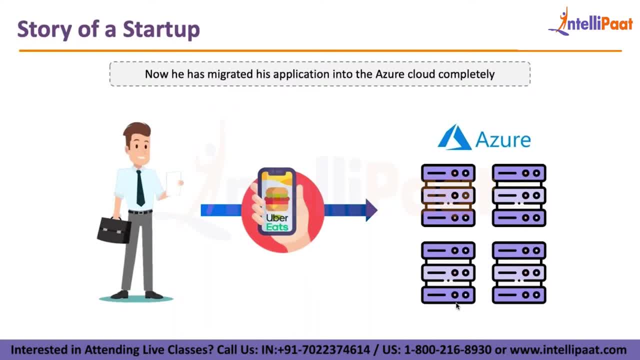 to the world. so what you will do is you can basically, uh, you know, go to, uh azure and you can just tell them: okay, you know what i need? uh, 32 gb of ram of servers and around 16 core of cpu, right, and I want 24: 7 electricity. I want that server to never go down, is that? 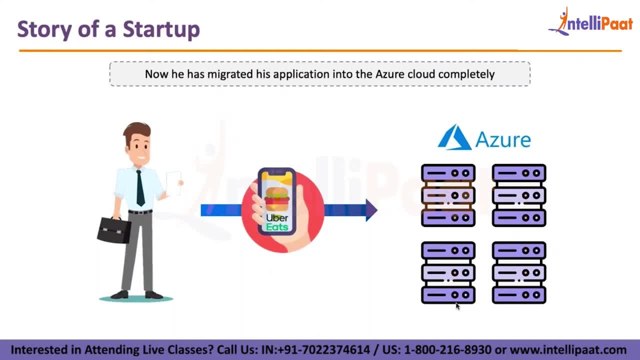 possible. so, as new people say, yes, that is possible. all you have to do is monthly. I just have to pay the rent for our servers. we will manage all the electricity, we will manage all the internet connection, we will manage everything which is required from the hardware perspective. all you have to do. 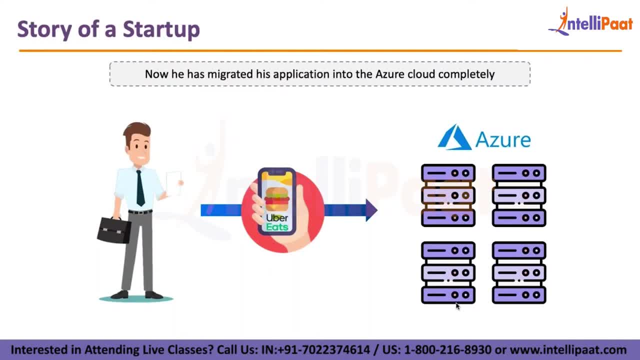 is take care of our application, which you're deploying to the server, and nothing else, and in lieu of that, you just have to pay the rent of the server that you are using. now, let's say, after one month you do not require the service anymore. so you, there is no security that you have to pay. there is nothing. you. 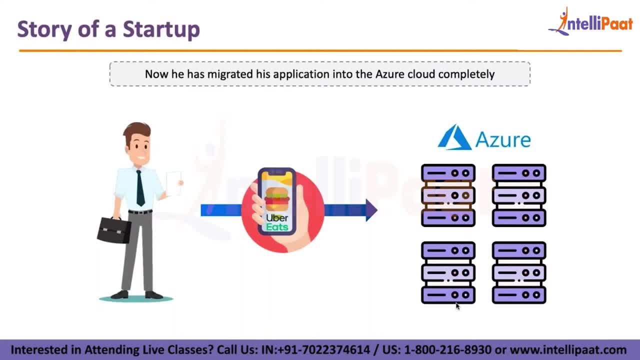 actually have to pay. just pay the amount that you used the server for, and that is about it, that we require nothing else. at the same time, let's say tomorrow, you need more servers that you want to add while you know your customers are growing, so all you have to do is take. 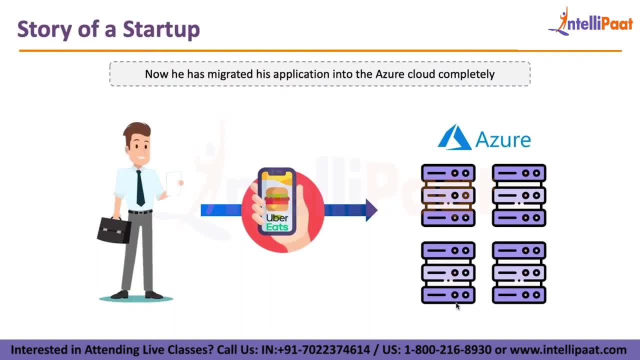 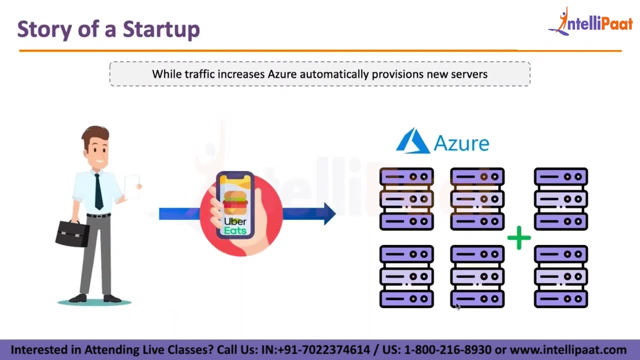 some more servers on rent and apply to your existing fleet of infrastructure and you're set and it will hardly take two to three minutes to do this right, and again, you just have to pay the rent of the servers that you are basically going to use. okay, so now with this- uh, they also give you. 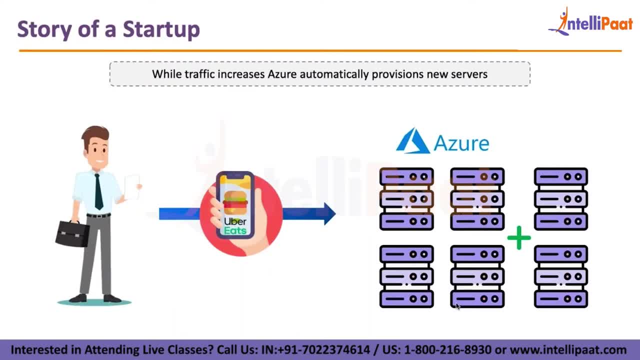 a feature wherein, let's say, the load increases on your application, the cpu usage of the servers which are hosting your application. it increases so automatically new servers will be added to your fleet and as and when the cpu usage goes down a particular number, it can also start removing. 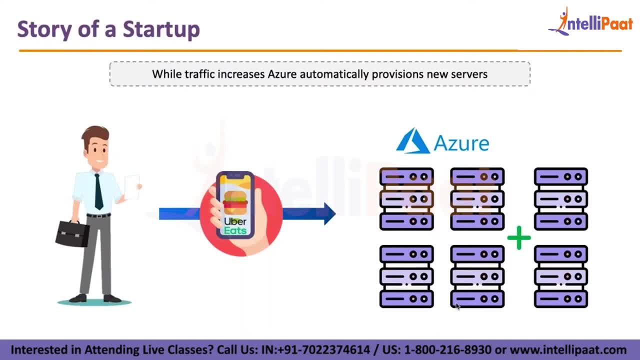 servers from your fleet right or removing servers from your infrastructure, and this is what is called as auto scaling, and with this, you never have to now worry about how many servers you need, how many people are there on your website. why? because everything is being managed automatically and at the same time. 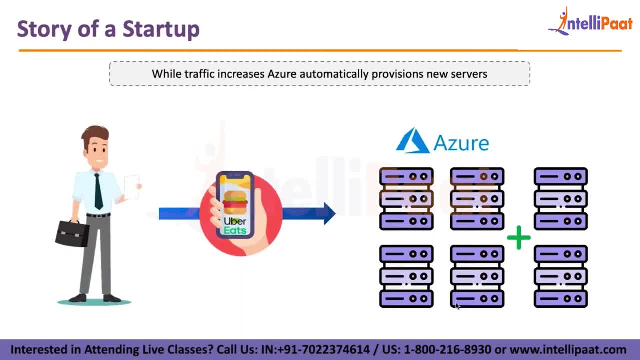 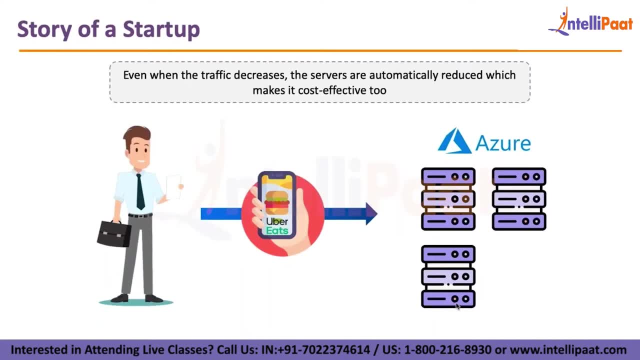 you do not have to buy servers now. you can just rent them and use it as long as you want them, right? so this came to be a very good deal for you, and that is exactly how millions of companies worldwide have now shifted to cloud. why? because azure is going to azure, or aws or any other. 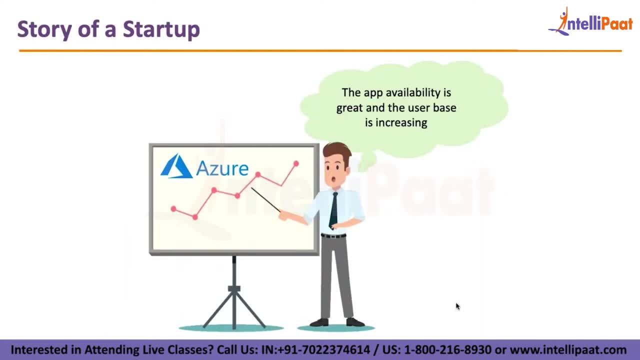 google cloud platform, for that matter- is giving you servers on rent. rent, all right, and the rent is as low as 0.005 dollars per hour, right, so that is how cheap the rent is for the servers that you're basically trying to deploy and with this- uh, you know, the internet is managed with them. 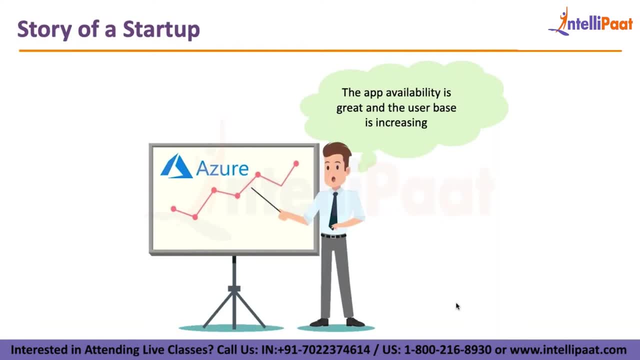 the, even the hardware updates. let's say, tomorrow, they will upgrade your hardware for free. you don't have to pay them anything extra other than your rent. they are going to manage everything and because of this your usage is going up. why? because now your application is available all the time and at the same time the traffic also, uh is. 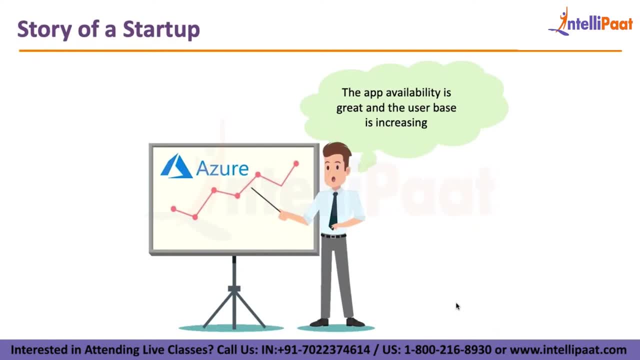 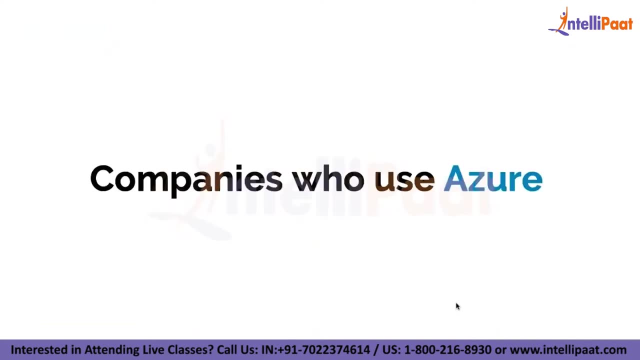 being managed automatically so that, uh, the new servers added to your fleet and are removed for your fleet as and when the traffic increases or decreases. okay, so this is the story of the startup, why it was using azure. now let me show you some of the companies who are using azure to 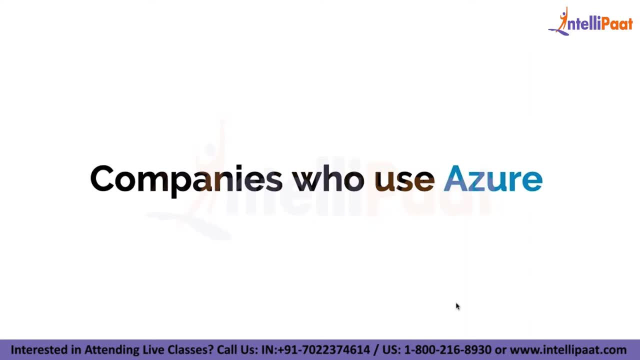 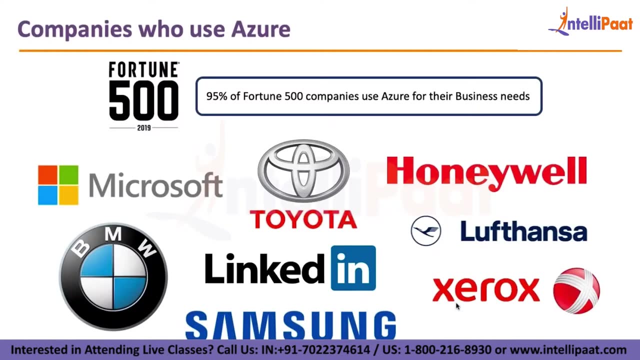 today right, or using a cloud platform, today specifically microsoft azure. so these are all the companies who are using microsoft azure for all kind of needs of infrastructure, right, and they just have their software over it. so companies like toyota, honeywell, lufthansa, linkedin, samsung. 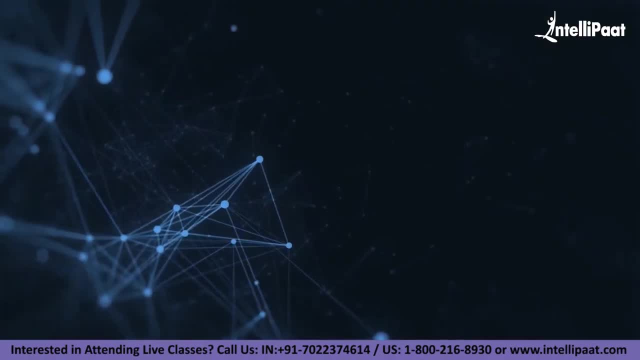 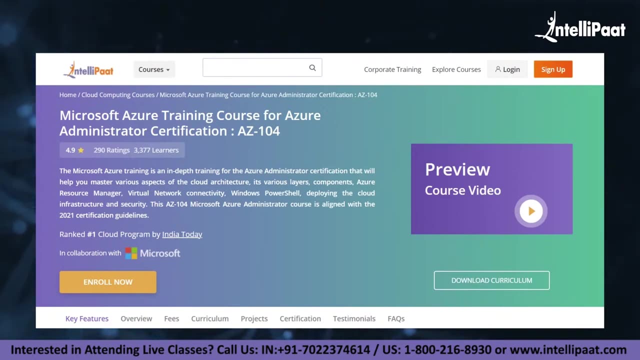 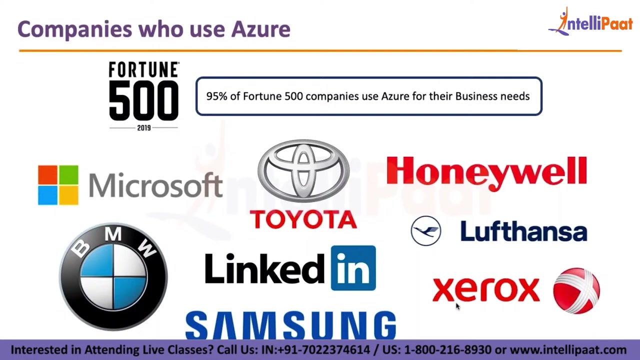 xerox bmw. just a quick info, guys. intellipad provides microsoft azure certification training in partnership with microsoft, mentored by industry experts, the course link of which is given in the description below. now let's continue with the session. and even microsoft itself. so any microsoft website that you go to is also hosted on microsoft azure, right? so all. 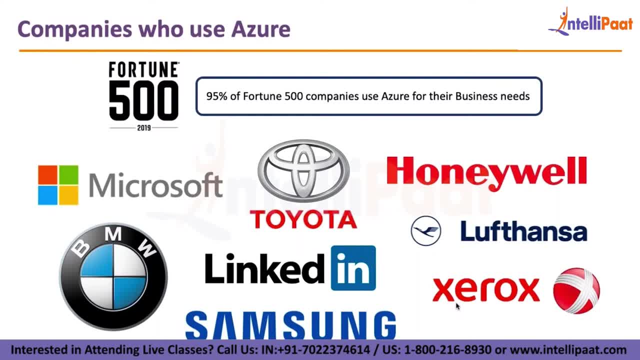 these companies are on azure for the very same reason that i've just explained you. first thing is cost effectiveness. second thing is distribution of work, because now you don't have to have your own team to manage your servers and at the same time you also are can be reliable on the infrastructure which azure has given you, because it would. 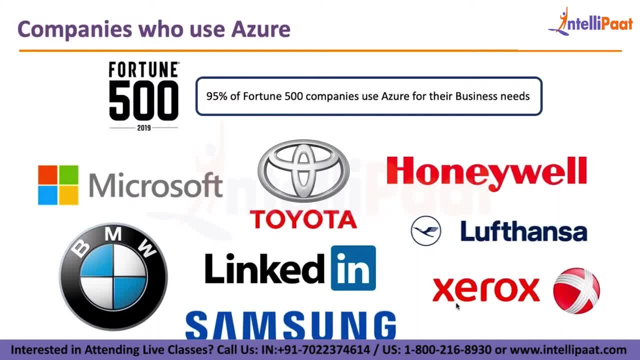 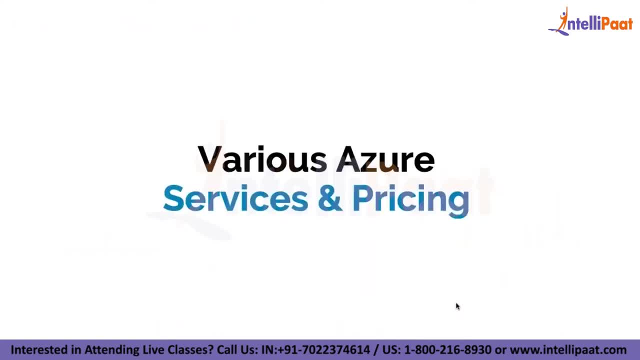 have been a pain to manage the hardware. uh, you know a team which is going to monitor your hardware all the time. if you were to set it up all by yourself, okay. so now that we have understood what azure is exactly and why we should use it, now we will move along. 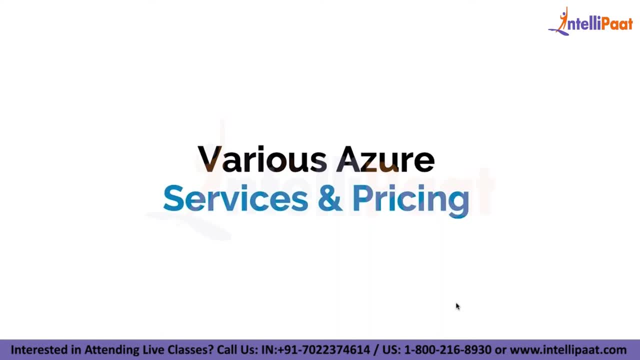 and understand some azure software. so one of the last thing i want to talk about in recent years is this case where these software are actually designed for the spotless, where the blindly done thing, our iOS, don't know what used to be our services and its pricing. so suhas is. 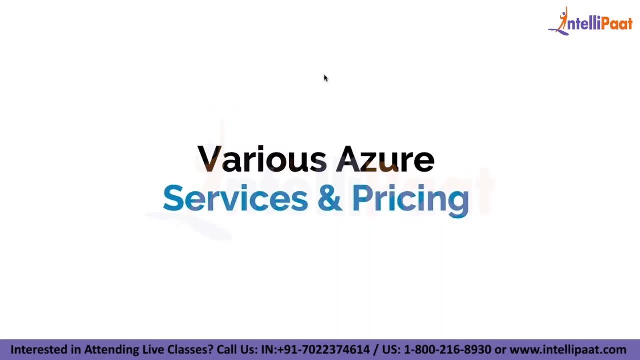 saying how much does it cost to owning a server versus, uh, buying from cloud? okay, so, so, as it depends on the size of the server, so let's say, if you, uh, let's, let's compare the price around 16 cores, right, and a 64 gigs of ram, which has around 3000 megahertz of speed. so this setup. 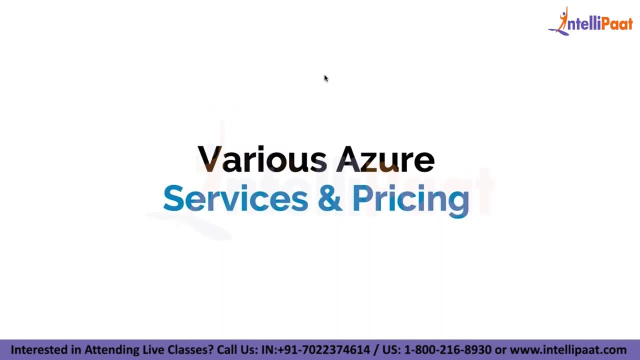 for just the cpu is going to cost you around three to four lakhs. and now this is a pc. now imagine if you have to set up a server and this pc will now be multiple times in the server rack that you have, which is basically going to cater to thousand, two thousand people. so the cost of the setup is going. 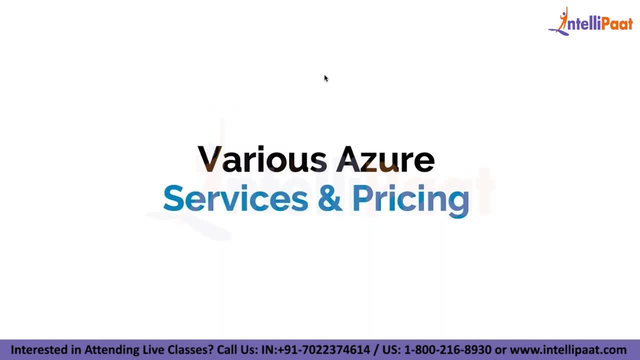 to be around six to seven lakhs per server rack right now. imagine that your server hits a hundred thousand users, or 200 000 users. this cost is going to increase exponentially. now, obviously, you will have to manage it according to the revenue that you are generating, right, but at the same time, the 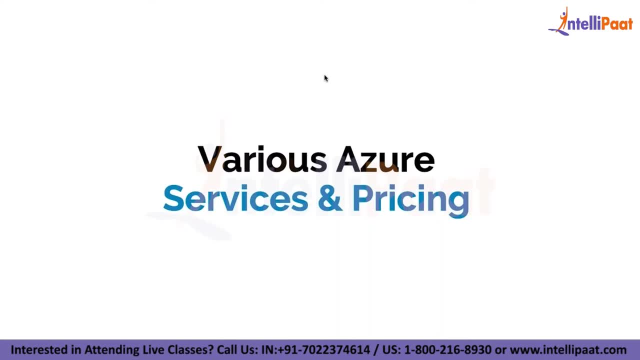 revenue will take some time to come in right, and, at the same time, if your users are increasing exponentially- which is a good thing for you, though, but, let's say, if you're not able to manage the demand of the users, which is basically the infrastructure that you have, it again becomes. 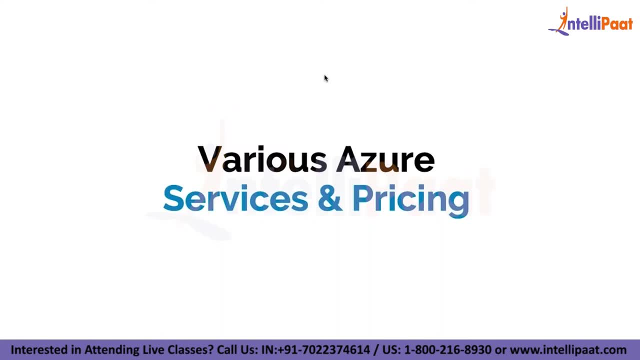 a problem. let's say you have that kind of money to buy your own infrastructure but with every increasing demand that infrastructure will take some time to come to your office. at the same time you will also have to take in headache of manage, managing or hiring a team of your own. 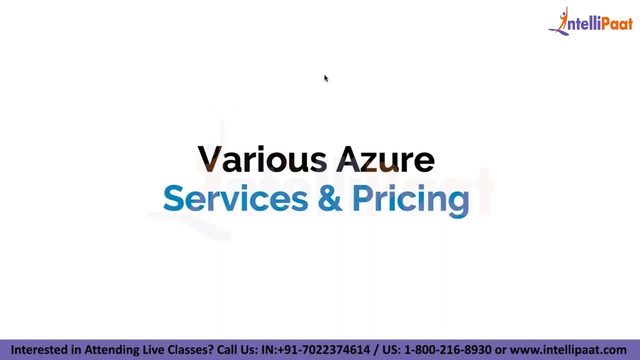 to basically manage these servers right. and obviously when you hire a team, you also have to deal with the problems that the team is facing. you have to also deal with- uh, you know what are the kind of tasks that you will be assigning them, etc. so it becomes a headache for you. because you basically wanted to. 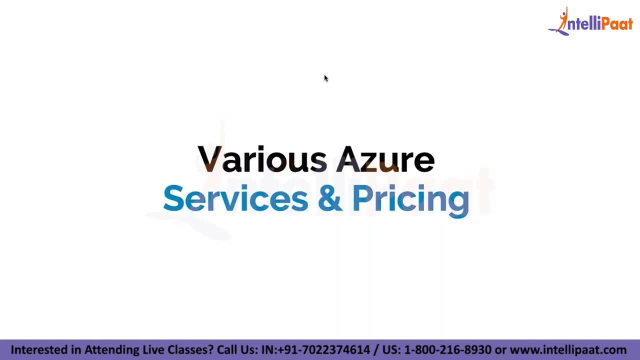 open a app which is basically a software. so not only you now have to manage the software, but you are also going to manage the hardware side of the hardware. software does giving less time to your application, which probably, if you have spent more time on it, you could have increased the. 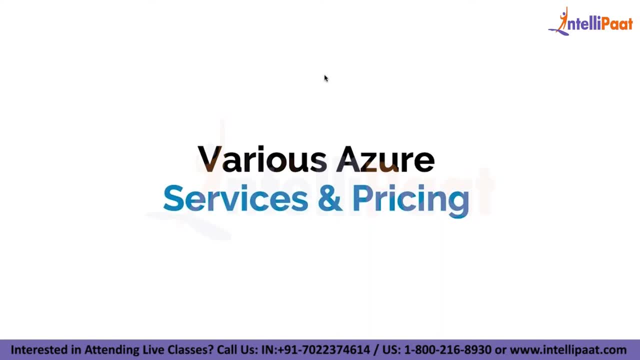 revenue of your company. right, and that is exactly why, basically, companies prefer cloud providers. okay, santosh is saying: what about security charges? so, santosh, everything you just have to include the rental charges. security, uh, from the hardware perspective. security from the perspective of, uh, you know, if you're deploying a firewall on azure so that firewalls 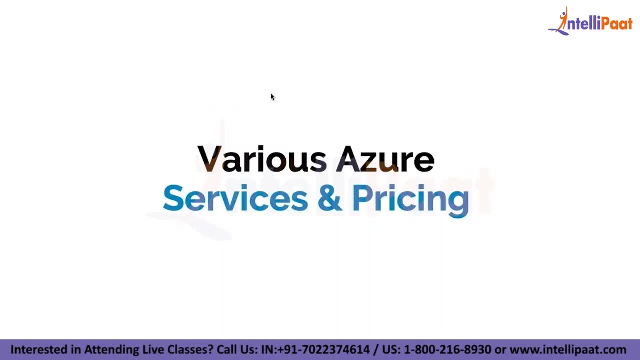 foolproofness is all guaranteed by microsoft azure. now think about it like this. let's say you have your own application that you're trying to launch in the internet space. now, obviously, the kind of security- uh, you know- aspects that you can create around your application, the kind of money that you can invest around your application just for the security needs. 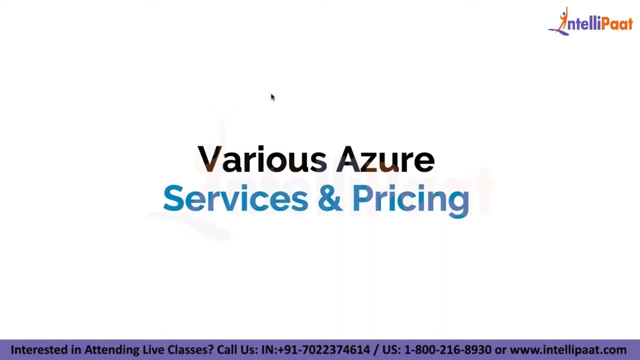 whatever that money is, it's going to be always less than what azure has already invested on their infrastructure, given the fact that microsoft itself is hosting each and every service of theirs on their own, and that's why it's so important that you have your own application and 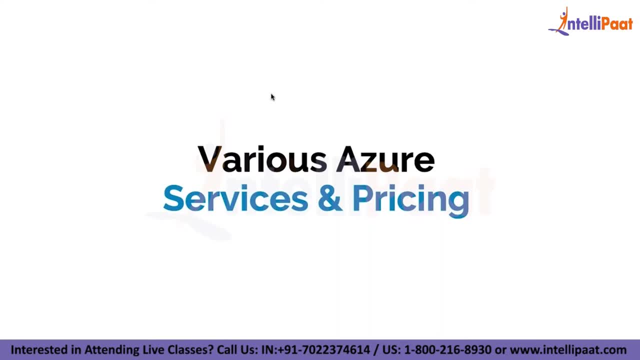 that's why it's so important that you have your own application on microsoft reserve okay, so you can be less assured that if you are hosting your application on a cloud like azure, it's getting best-in-class infrastructure and at the same time- uh, you know- the security best. 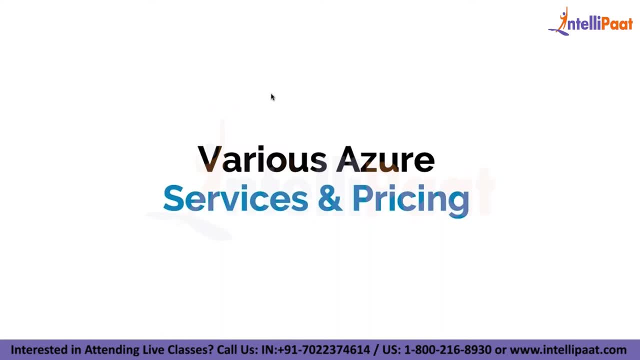 practices. now, obviously, you will have to make sure that your application, from the software perspective, is secure as well. that is not something that azure can guarantee, but the infrastructure that you're deploying on cannot be tampered with. that is something that azure will guarantee you. so, monty, uh, why is there again? a very good question. so i just told you about why cloud. 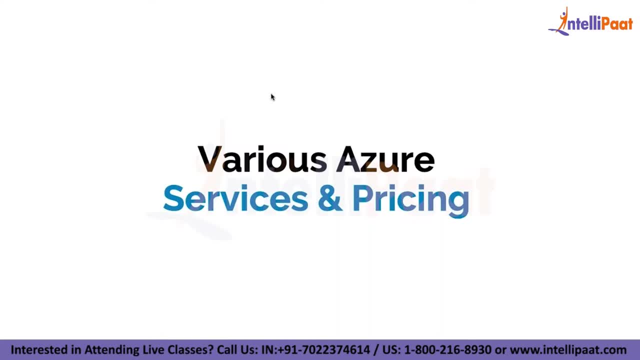 platforms are basically- uh, you know- preferred rather than owning your own infrastructure. now, why are we learning azure today? let's, let's try to answer that question. so, as you all know that amazon web services is the largest cloud provider in the market right now. right, and when i say the largest cloud provider, it has around 41 to 42 percent market share. 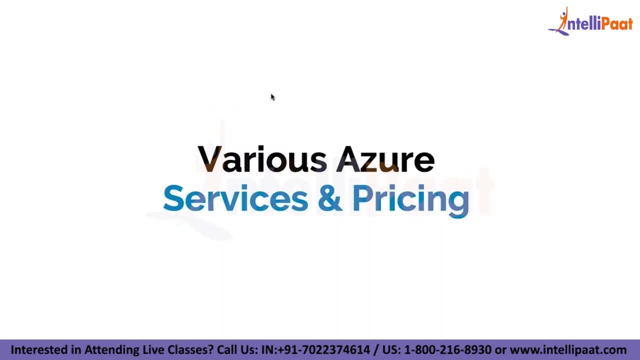 now, because it is the largest cloud provider in the market. that obviously means that there are more jobs, and because there are more jobs, there are more people who are trying to apply for the job and hence more competition. when you talk about microsoft reserve, it's the second largest cloud. 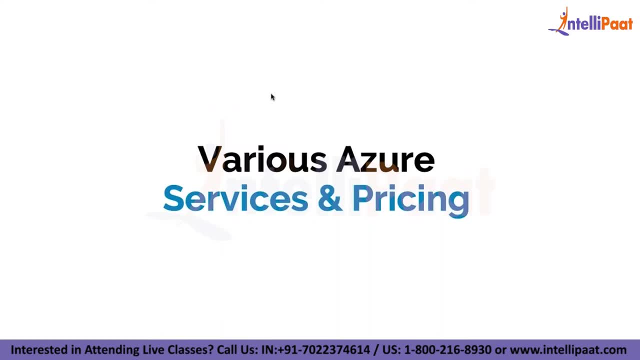 provider. now let's first talk from the market perspective. now, because it's a second large, a second largest cloud provider companies which are using aws right now. they're also taking into account a secondary cloud provider for their infrastructure needs. why? because, let's say, tomorrow, uh, you know, the whole of aws servers go down now. they do not want it to impact their own. 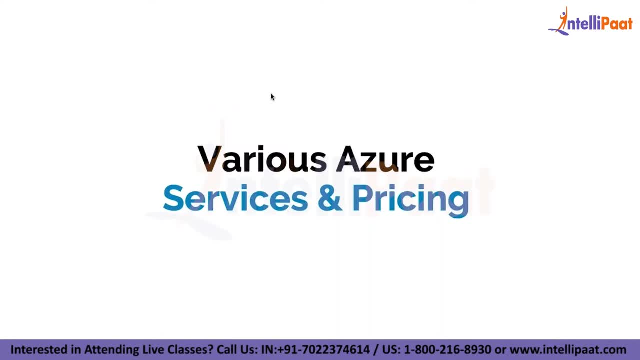 application. so what they do is they create a redundancy in place and what they do is they manage their servers on azure as well. right, and now they're using two cloud providers instead of one. this is from the market perspective, and that's why you can see the growth of azure has been. 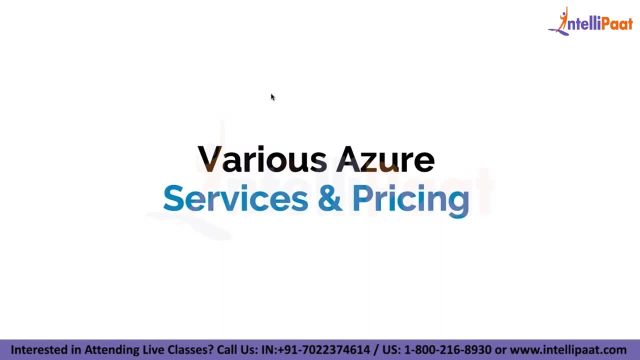 dramatic in the past two, three years. right, the kind of growth that aws has seen is less than the kind of growth that azure is seen from. uh, you know, if you, if you take into into account the last three, four years. at the same time, azure is a lot cheaper when you compare it with other. 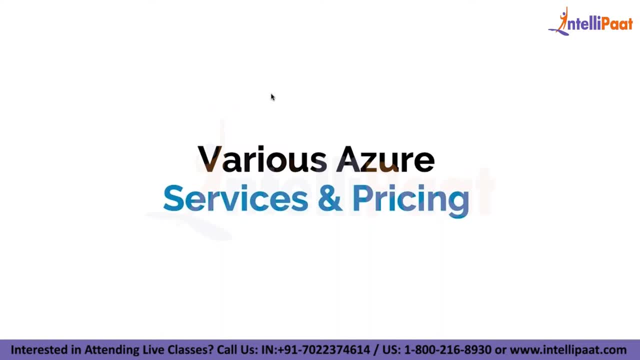 cloud providers, and the sole reason for that is the microsoft products. so if you are using any microsoft product on, let's say, aws, on google cloud platform, it is obviously going to charge you more than microsoft product that you get on azure. why? because azure is basically owned by microsoft, so because of that, even the pricing is in control and hence 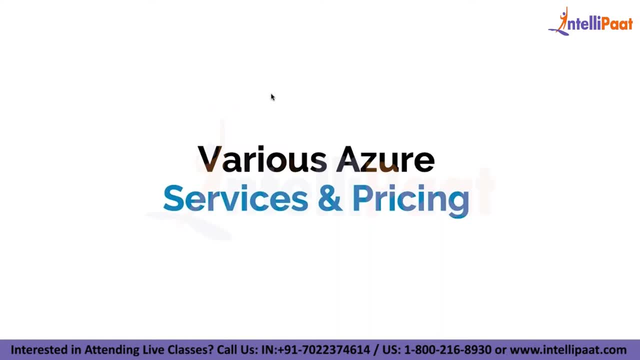 it becomes more cheap for people who want to use microsoft, uh software. third thing is now, because the aws is the largest cloud provider, there is more competition over there. azure does not have much of competition but at the same time, since constant companies have started considering azure and because of the growth rate of azure, that we have. 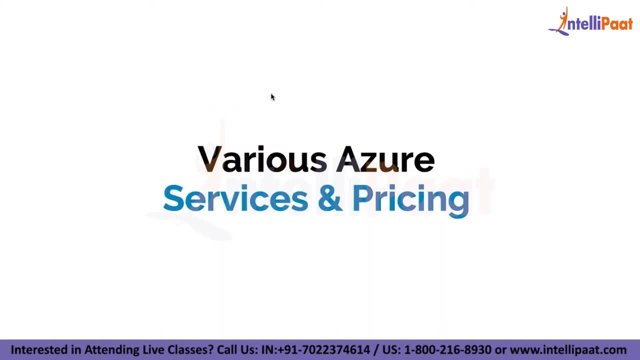 seen in the past three, four years. there's an acute shortage of people who are who, uh, basically, are certified in azure and, at the same time, know azure that well as well. nowadays, what is happening is people who know aws. they are the only ones who are also trying to- uh, you know, control the. 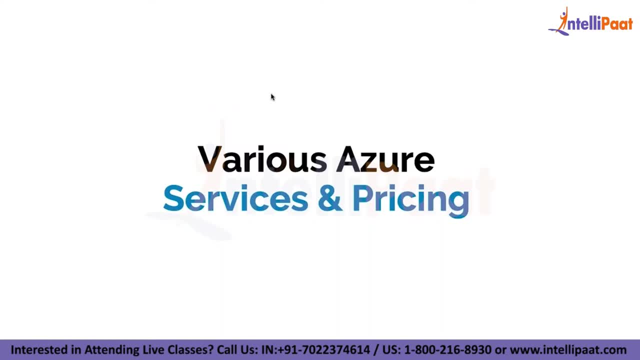 infrastructure which is there on azure in the same company, right, but that is not happening all the time. so this is the way that people are stepping out, because a lot of features are different between microsoft, azure and aws and now companies basically want to have a separate guy who can manage their separate cloud platform that they have now. obviously, if you talk about, 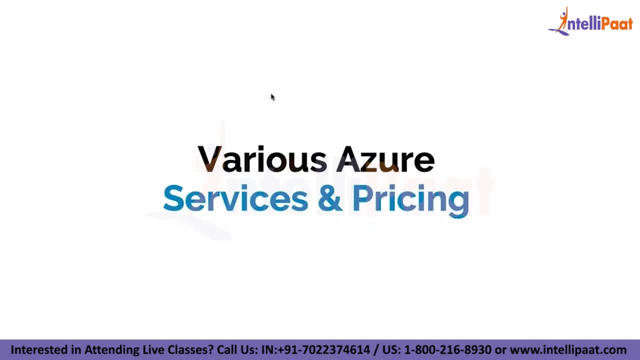 senior cloud profiles, such as senior cloud engineers or senior cloud architects. now, these guys, they are not just limited to learn only aws or only microsoft. in the long run, when you see more than one cloud provider, that is, some companies expect you to know both AWS and Microsoft Azure. some companies expect you to know all the three. 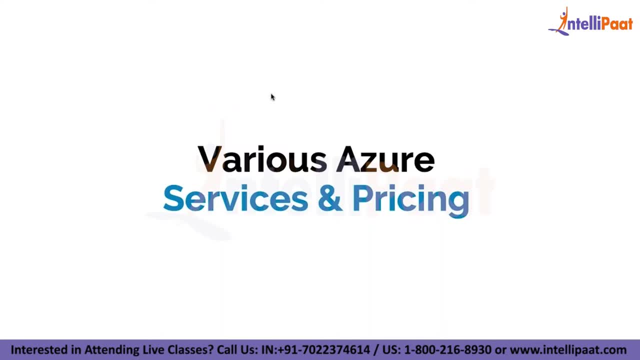 Microsoft Azure, Google Cloud Platform and AWS as well. but when you're starting out in the cloud domain, it is recommended that you start with Microsoft Azure, because it will be a lot easier for you to switch to the cloud domain because of the less competition right and while you are also growing for. 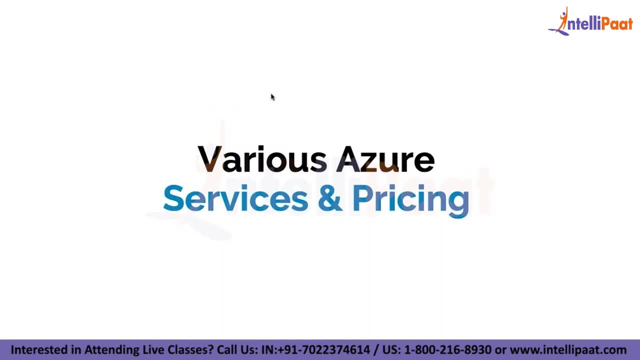 the next level, the next level of profile that you want to go for, then you should also learn AWS. you should also learn Google Cloud Platform. okay, so SK is saying: what are the difference between Azure and AWS services? well, SK, when you talk about it from the features perspective. so what are the features? 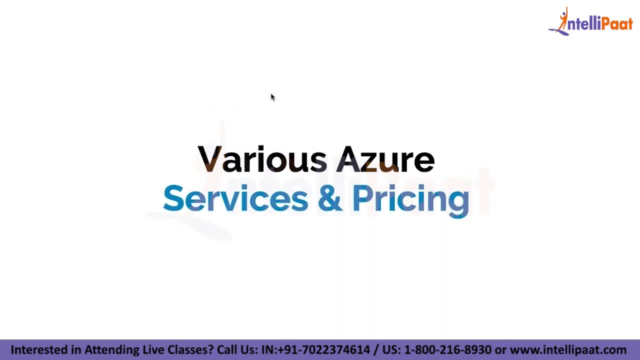 that AWS is providing, which Azure is not. all the features are same, but the way you implement them using the services is different. right, the steps that you have to do to do a particular task in Azure is obviously going to be different from what you have to do in AWS, because they are two. 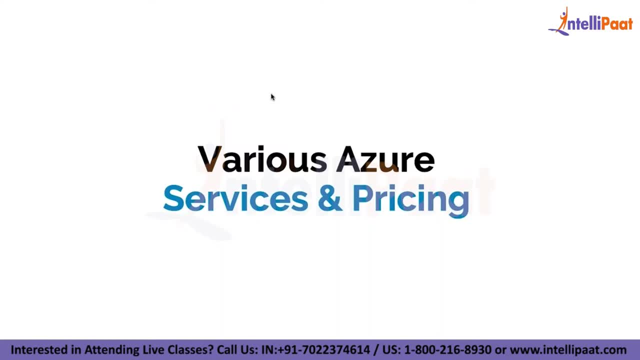 different companies. they have built their own product separately and obviously because of that, the way of implementation is also very different. right, so that is the only difference. but when you talk it from features perspective, both the cloud providers are neck-to-neck. there are giving each other competition in terms of the feature that they offer and because of that, all the 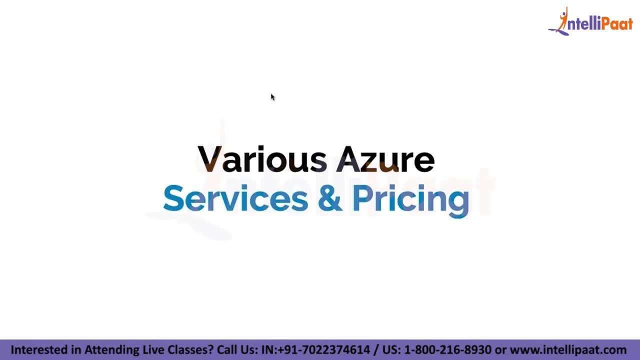 features, or most of the features, are same. okay, so how is your is different from AWS and what are? the basic process for cloud is same. so, Samir, I think I just answered your question. so both of them have the same features. it's just that because they are two different products, the same thing can be. 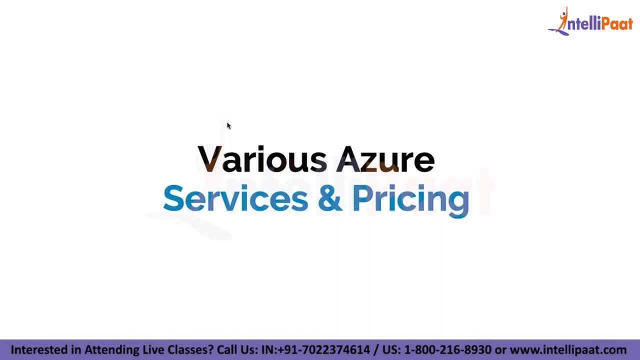 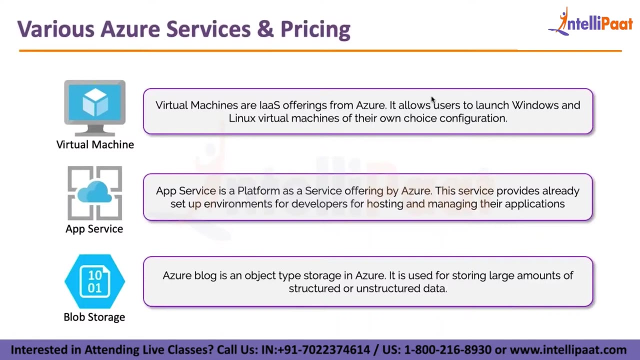 implemented in the both the cloud providers in different kind of ways as your services. so these are some of the common services and Microsoft Azure that we are basically going to discuss now. okay, so let's talk about the most common service, which every one of you is going to use. 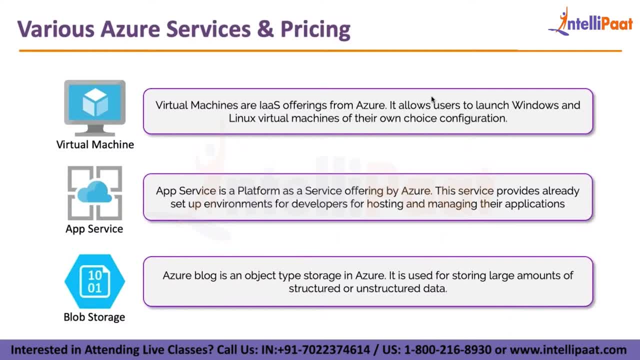 once you start using Microsoft Azure, and that service is nothing but the virtual machine service. so, guys, the virtual machine is basically, it's an infrastructure as a service, or, in other words, it's basically a server. so all that we have been discussing till now, even in the example that I told you, 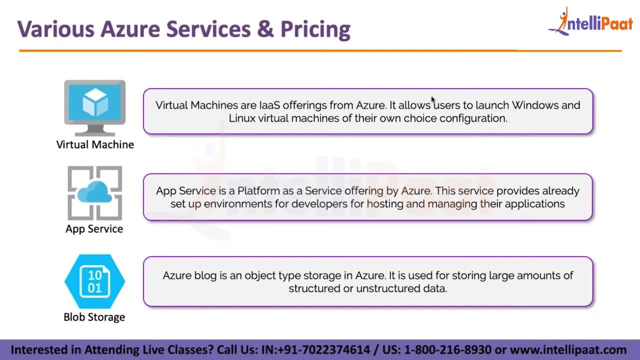 earlier was about using a server. right so whenever you deploy a server in Microsoft Azure, that is nothing but a virtual machine. right so a virtual machine is just like your own laptop or personal computer or PC. right, it's just that a virtual machine can have whatever kind of resources you want. right so when 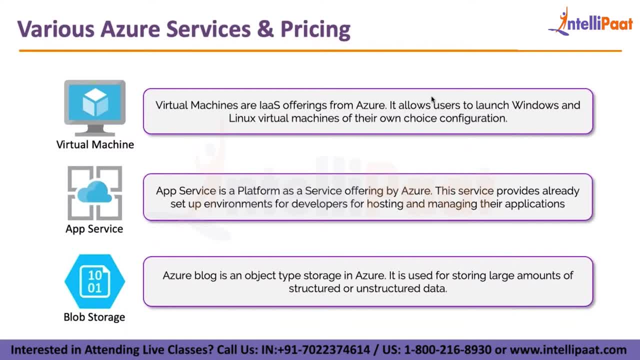 you deploy a virtual machine. you choose the amount of RAM that you need, you choose the amount of CPU that you need and then you deploy- all right. so that is exactly what a virtual machine is right. for example, in your PC, if you have a 32gb RAM right now, you cannot just change it right now. you have to buy some. 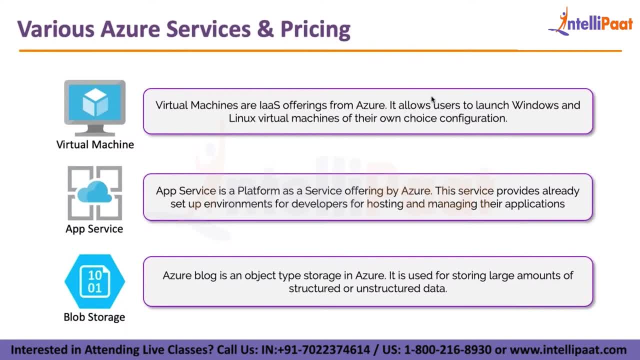 parts, include it in your PC setup and only then that configuration will increase. but with virtual machines are seen as you can do that in a matter of seconds. right, and how can you do that? because you know the infrastructure or the hardware that is basically made available to you by Microsoft Azure is. 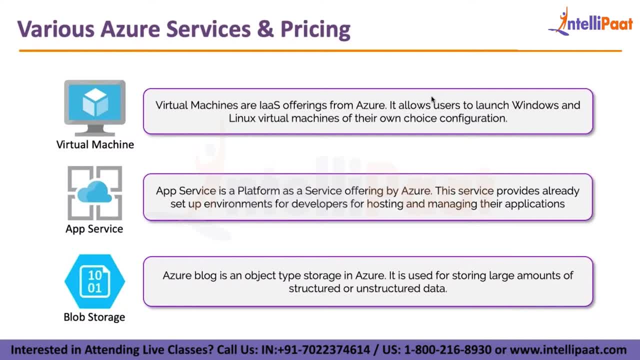 virtualized, which basically means if your virtual machine is being launched on, let's say, a certain hardware, it might be the case that the same hardware might be committing 100 or 200 of virtual machines as well. so that is the kind of resources which are available on the hardware, but the hardware can virtualize. 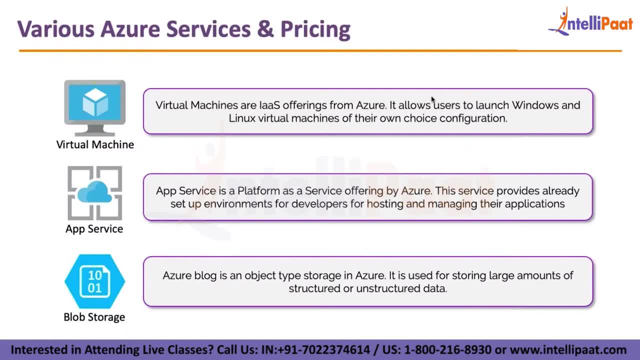 some of the resources and can make those resources available to you as a separate machine. that is exactly what virtualization is right. so a virtual machine in Azure, like I again said, it's basically a server that you deploy right and these servers are basically going to have the required ramp, the required 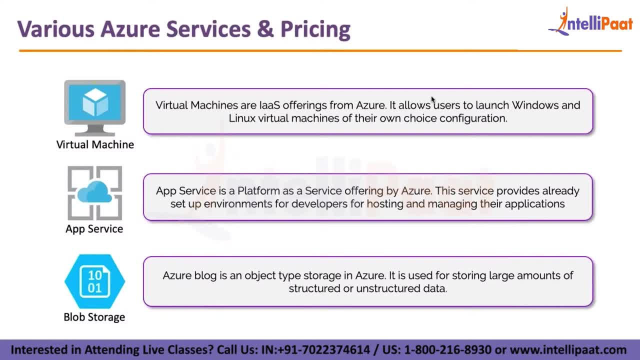 CPU that you specify. so that's what our virtual machine is, right. then the second check kind of service is called app server. so what is an app service? so an app service is basically a platform as a service, right, and in that what you get is: so, let's say, you deploy a virtual machine, right? so when you deploy a 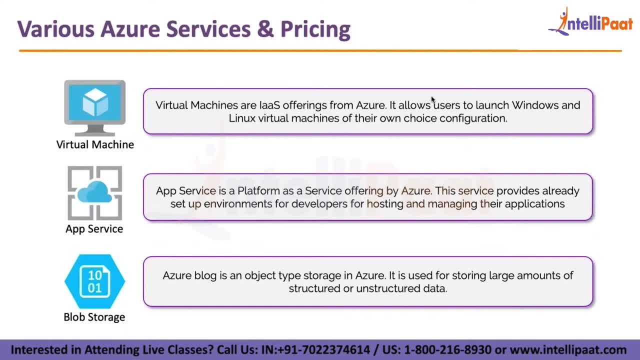 virtual machine. what happens is you get a screen to a computer which probably has the Linux operating system or the Windows operating system installed on it, and then you can use it as you want, right, but in app service this thing is not there. in app service what happens is you are given a platform, so you're not. 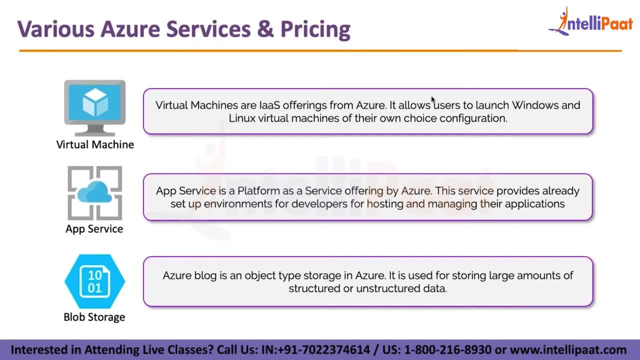 given the whole machine to work on. you basically are given a platform which basically gives you a dashboard, kind of a view, and in that dashboard you can only do the actions which are specified by the service that you reply. for example, in app service you can deploy your own website, but if you have to, 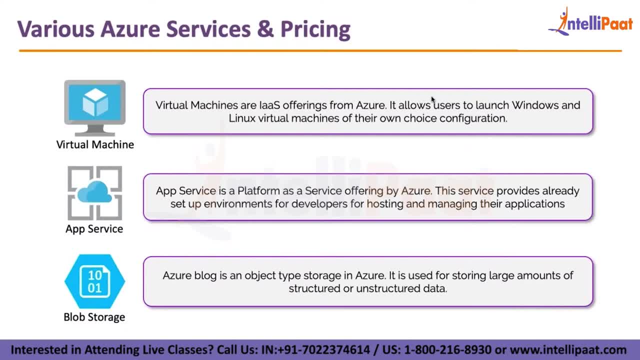 deploy your own website. let's say you want to do that on as your virtual machine. so first what you have to do is: let's say your website is based on dot net, so you will have to install dotnet on this. or let's say, your website is you. 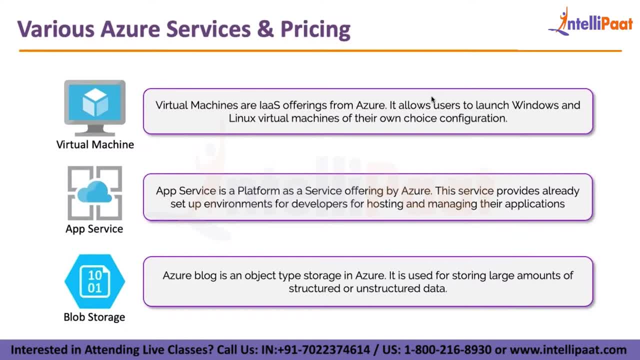 know, based on Apache software. so you will have to install the Apache software. if it's a PHP website, you will install the PHP software and once all the software that installed, only then you can deploy your website on it. So that's it, Thank you. 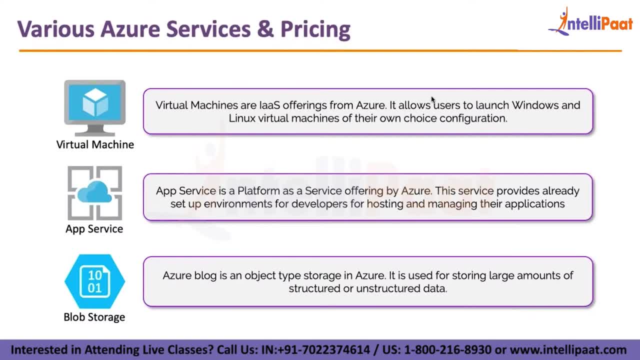 it, or you can copy the files of your website on it and then your website will become available. but the scene with app services is that everything is deployed automatically. so you just tell us your, what is the kind of website that you are going to deal with. so, let's say, if you have a PHP website, what you do is you. 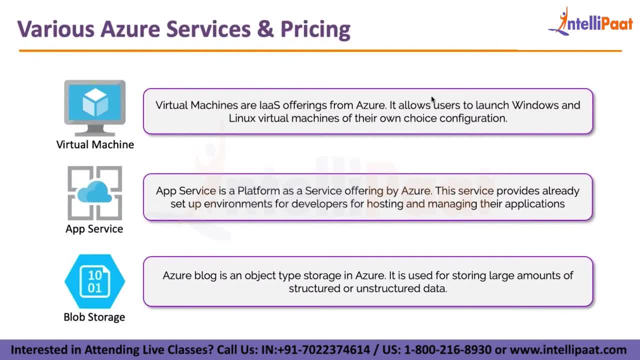 click on app services. you tell Microsoft- okay, so I'm gonna use a PHP website on the service that I'm deploying- and Microsoft themselves. they basically set up the environment for you, then install the software's and everything, and all they do is they give you a button, which is on the dashboard that you will see right, and on that button, 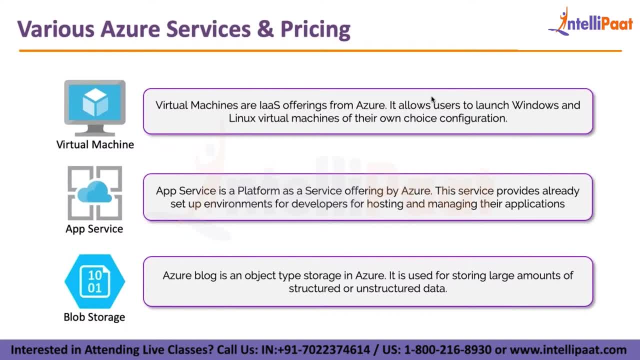 you can see, I mean through that button. if you click on it, you will be able to upload your website, and once your website is uploaded, it will automatically be deployed on the server, which is basically deployed in the background, right? so the purpose of having an app service versus a virtual machine is to 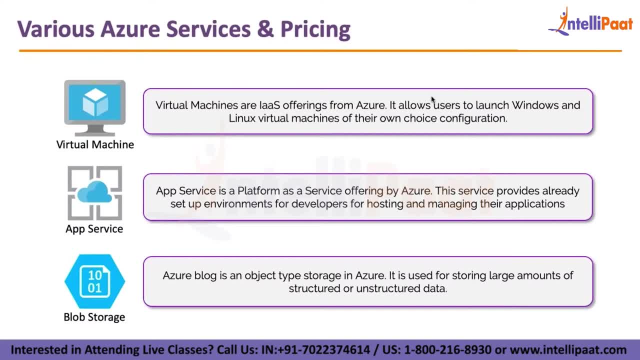 make your life easy. so you do not have to deal with the software that you are going to install with the operating system directly, as your manages the operating system on your behalf. it manages all the software is based on your behalf, and all you do is you just deploy your application. so that is what an app services, right? 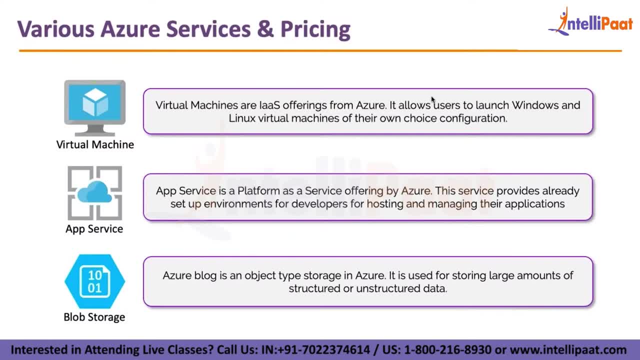 similarly, the third kind of very common service which will be used- Microsoft is your- is the blob storage. so a blob storage is just like Google Drive, so I'm pretty sure every one of you might have used Google Drive in any of your careers, right? a Google Drive is just like you know, uploading your file on the cloud. 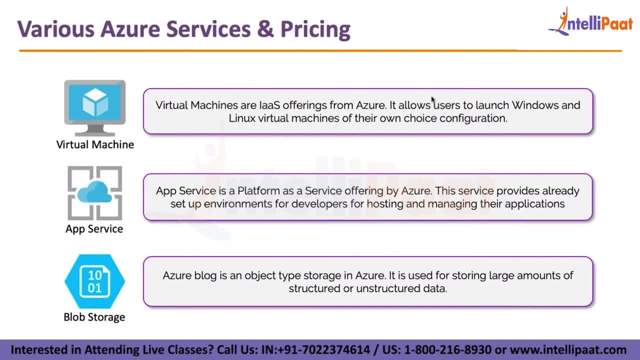 and that's about it, and that is exactly what a blob storage also is. so on blob storage you can also upload your files, but what you can do with those files is a lot different than what you can do with files on Google Cloud. Google Cloud, for example, in blob, you also have the option of, you know, keeping those files. 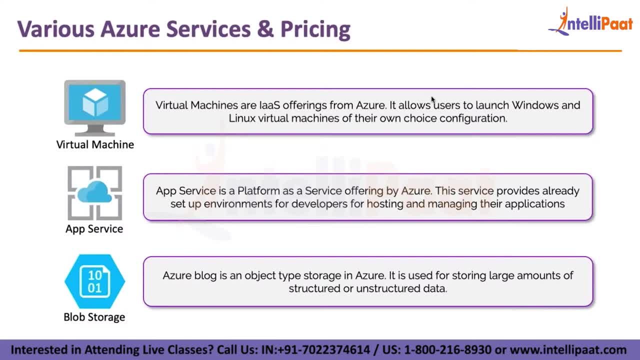 in a very, very primitive kind of storage which is going to reduce your costs drastically and, at the same time, you will see that when you're using Google Drive, you have a limit to the kind of files that you can upload. when you sign up on Google Cloud, the story I think that you get is around 30. 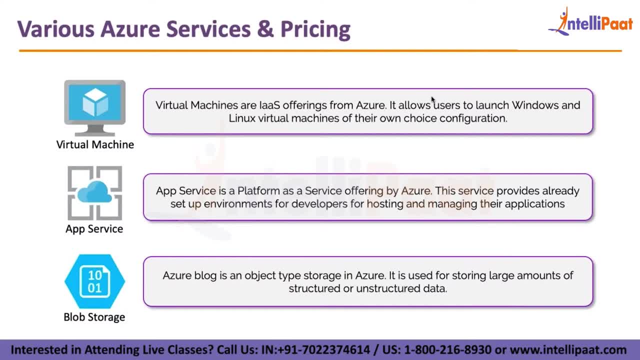 GB. so 30 GB data is free for you that you can upload, and after 30 GB you will have to buy some storage where you can upload that data. upload more data, but when you're using blog storage, you do not have any restriction of how much. 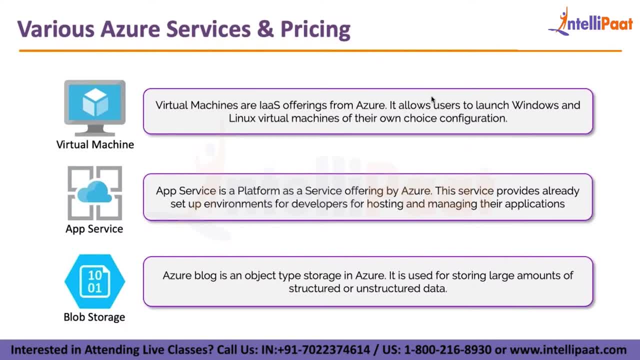 of data can you upload. it's unlimited data that you can upload and, at the same time, you are only charged for the data that you are upload per month. let's say you uploaded 1 terabytes of data, so you will only be charged for the amount of. 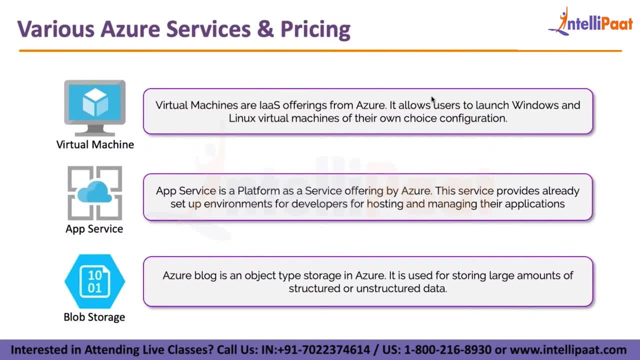 1 terabytes of data and nothing less, nothing more. now those pricings are also very different. so if you want very high speed download and upload to your, to to your file that you have uploaded on blog storage, the pricing will be different. let's say you say that this is a backup. 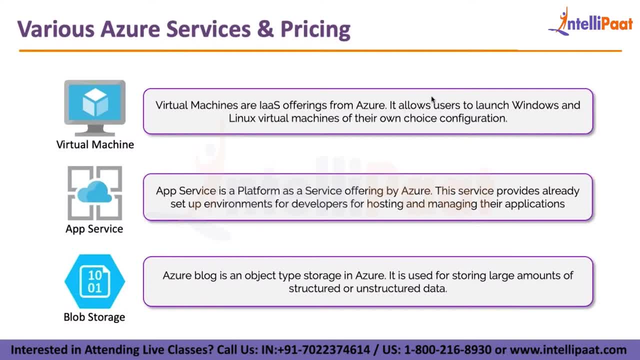 file that you're putting on blog storage, and probably you. you will never use it again. you just want it to be saved in a very safe place. so in that case, what you can do is you can change the storage class of your blob storage and that will. 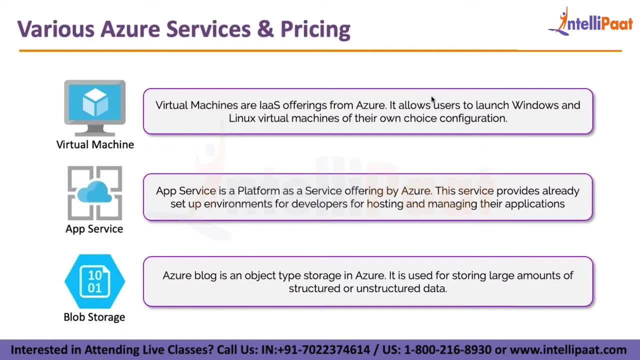 almost take, make the cost of uploading and keeping the file button right, and similarly, there are a lot more features as well, and that is exactly what blob. so they just so again, if you want to understand it, it's just like Google Drive, but with a lot more features. so that's about what blob. storage is right. then you have. 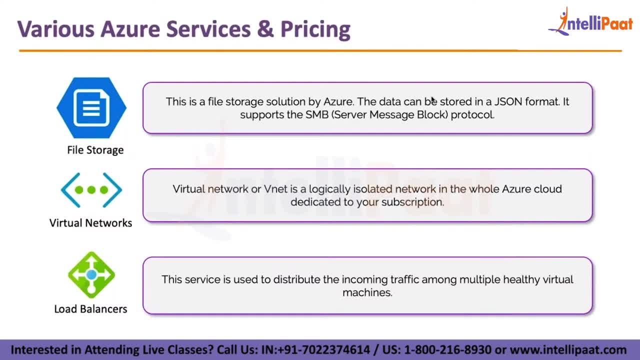 something called as file storage. so file storage is just like having a network drive right which you can map to your computer. so I just talked about Google Drive. Google Drive, you cannot map it as a C Drive or a D Drive on your system, but with file storage, if you deploy it on Microsoft Azure, it has again. you know. 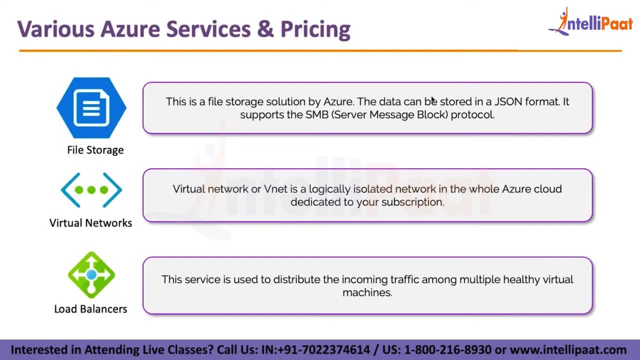 a very unlimited kind of a service where you can decide how many GBs or terabytes you need, and once you've defined that application in Microsoft Azure, you can basically connect it to your computer and mount it as a local disk drive, and then you can basically copy files to it or retrieve files from it as you want. so 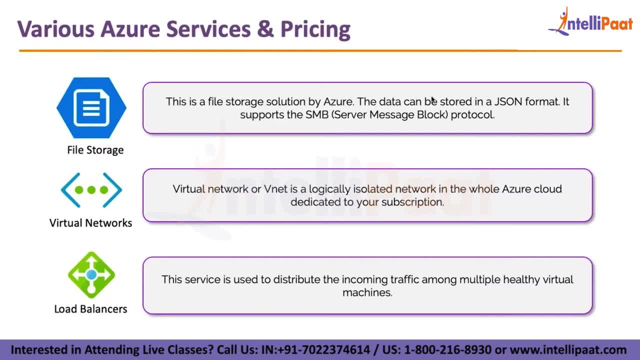 this is what a file storage is. now, the cool thing about file storage is that multiple people can be can basically mount this drive on their computer at the same time, and they can use it for as a shared drive between them while they're working on it. right? so that is what a file storage is, so each of these 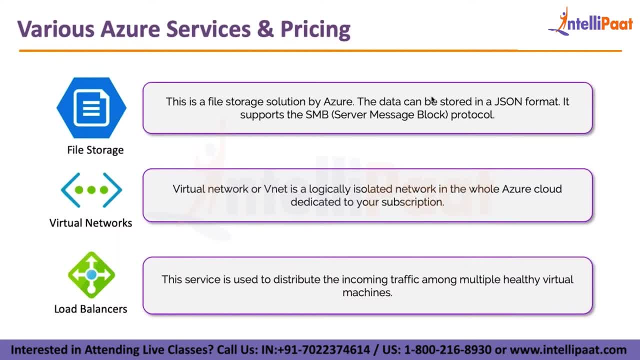 service basically plays a different role. when you are deploying an application on production cloud, right then. the next set kind of service that you have is called virtual networks. so virtual networks is just like you know, in your office you have networks, right? so if you want to deploy a network for a set of machines, 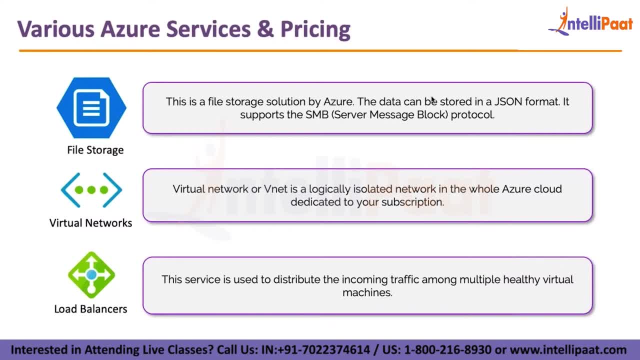 that you're running on your computer. you can deploy a network for a set of machines that you're deployed in Microsoft Azure. the way you can do that is by making use of virtual networks. now again, you can create n number of virtual networks in your Azure account, where you can have n number of servers and these virtual 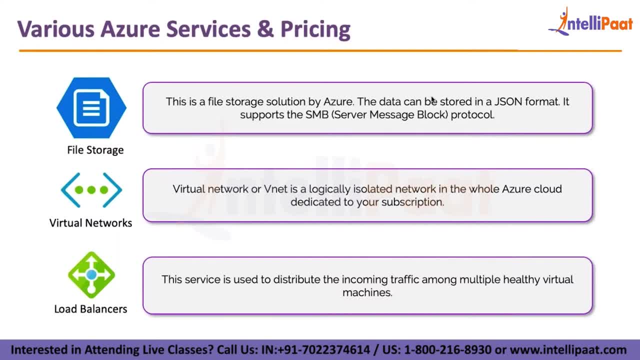 networks, again, can have n number of features that you can explore and implement, which I think you will learn more as you start using the virtual network service, right, and the final kind of service that we are going to understand is load balancers, right? so what is a load balancer? a load balancer? 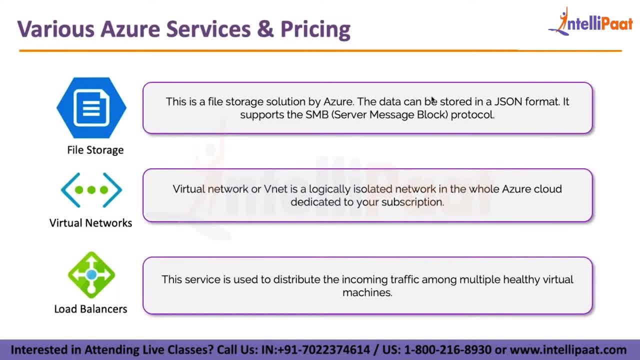 is basically a load balancer. that is that a load balancer is basically a you know it's, it's, it's more of use in production and probably for a guy who does not know about load balancers, even if they're using it, they will never get to know about it. right, and this is all. 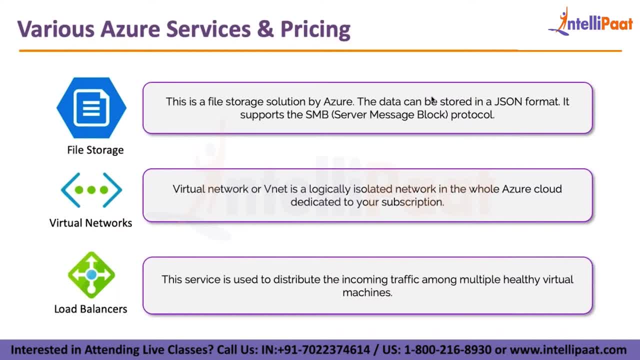 actually a service that we are actually going to make use of in today's session as well, where i'll show you the the reason people use load balancers. so i give you the example of a story in the beginning, right, where you can add more servers for your application and then, as you add more servers, 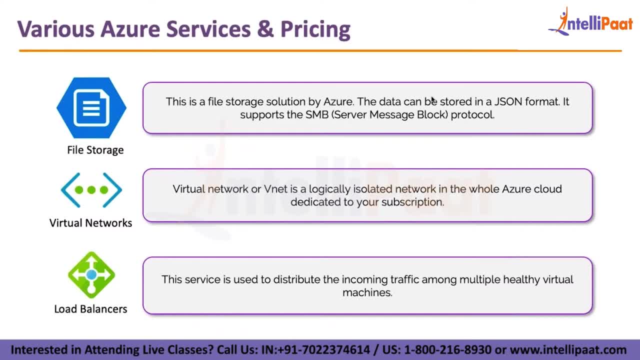 more number of users can basically be dealt with right. so how does that happen? how does how do you, how can you add hundreds of servers and then decide where a user exactly is going to land on, or which server is going to land on for basically his needs? for example, if you go to flipkartcom, 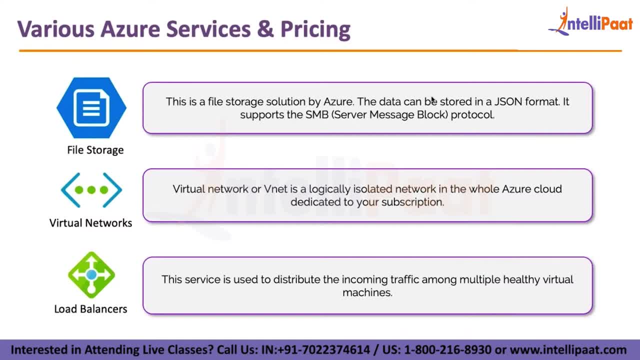 or you go to amazoncom. so when you go there you automatically are given if your internet connection is good, if your application loads just fine, right. so where is the data on that application coming from? that data is basically coming from cloud, is basically coming from a fleet of servers which have been 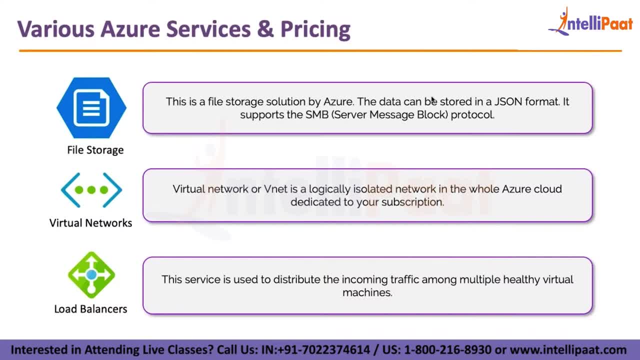 deployed on cloud and to one of those servers you connect, and that is where your data is basically coming from. so you never decide which server you have to connect to. that is automatically chosen for you, right, and that is the way it works. so when you go there, you automatically are given. 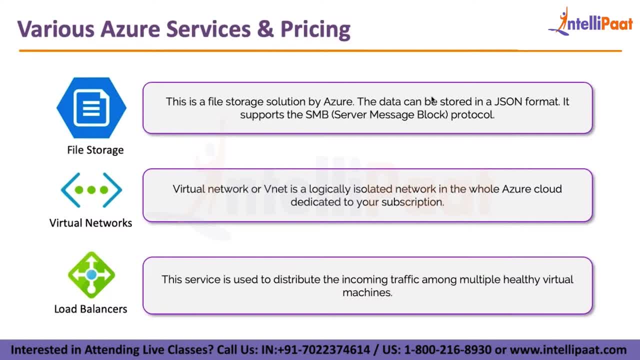 exactly what a load balancer does. it distributes the load equally among multiple servers which are deployed in your infrastructure. okay, more about this. we will understand as you move along. so, guys, this is a brief about the azure services in microsoft azure. now let's go ahead and talk about 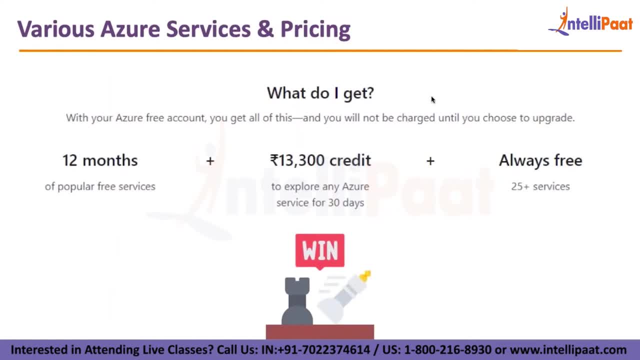 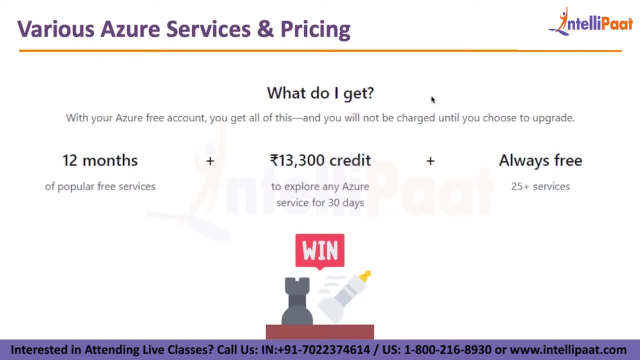 around 13,000, 300 apiece, or $200. right, so you can use this amount to learn and understand microsoft zonk. right, so you can deploy as many services you want and you can use them until and unless you exhaust the $200 or the 13 thousand 300th piece credit that you have in your microsoft. 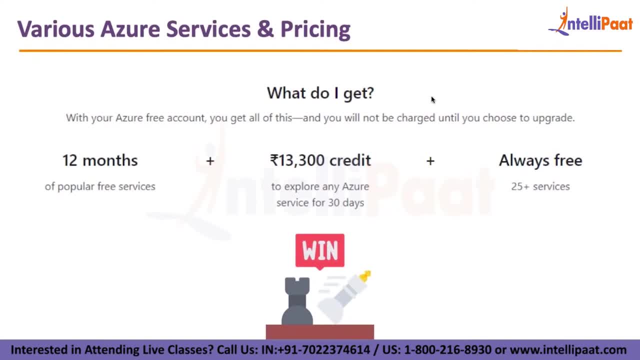 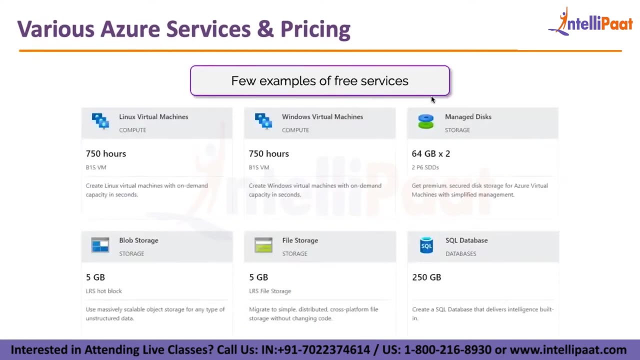 account the moment you sign up, right, so this is something which is very developer friendly, which azure has done that the moment you sign up, it makes the services available for you free so that you can practice them and learn more about it. okay, and other than that, there are some set of free services as well which are valid for- uh, you know, a lifetime. so 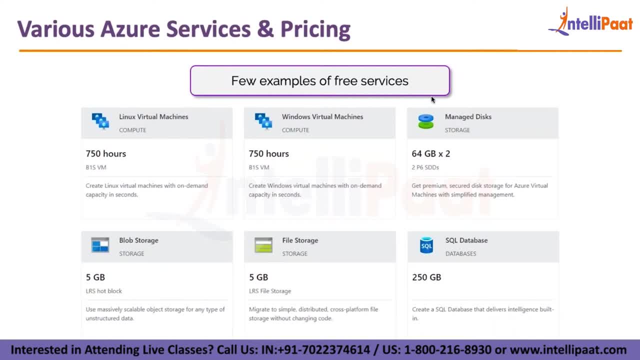 whenever you're using azure. this is uh. some of these services are valid for one year. for example, uh, when you're using linux virtual machines or windows virtual machines on microsoft azure, 750 hours every month will be given free of cost to you of the server type b1s, vm, right. so 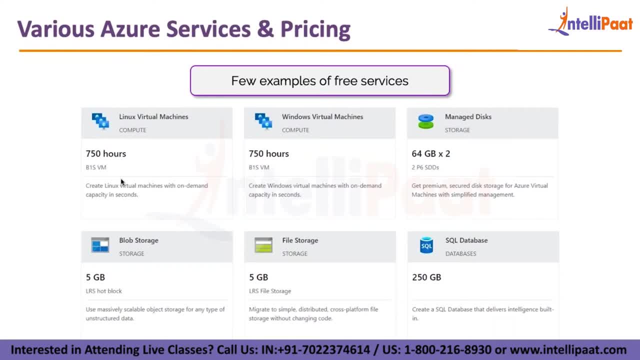 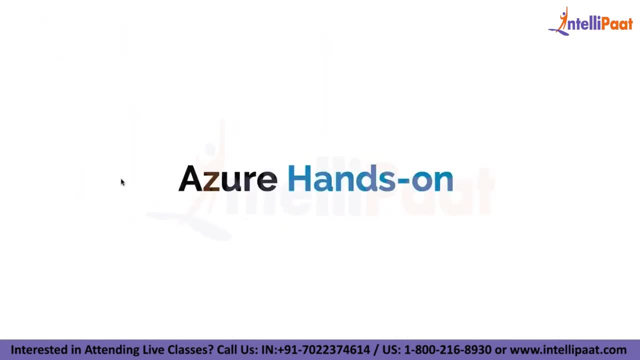 if you are using the servers, the first 750 hours of those servers will be free of cost, that is, will not be charged to you while you're using those servers, right? so now, guys, let's move on and start off with the hands-on, and what i'm first going to do is i'm going to explain you. 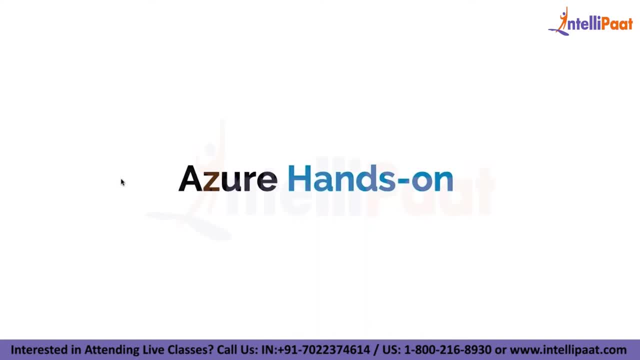 what we are basically going to make, and then we are going to go ahead and start it. okay, so, guys, let's first understand the uh website architecture that we are going to deploy on azure today. all right, so what we are basically going to do is, uh, we will have two sets of 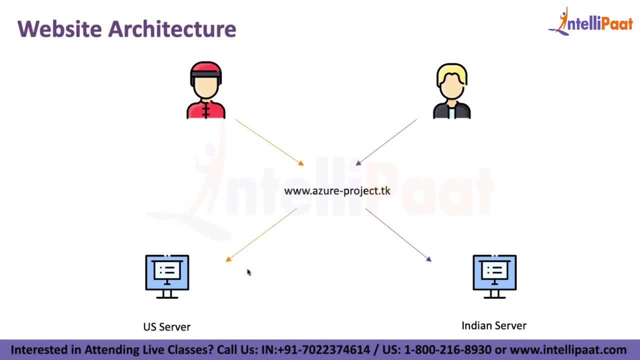 servers. right, so the first set of servers would be in the uh us region and the other set of servers would be in the indian region. all right now, since these- these will be multiple servers, what we are going to do is we will, we are basically going to have a load balancer on top of them and through 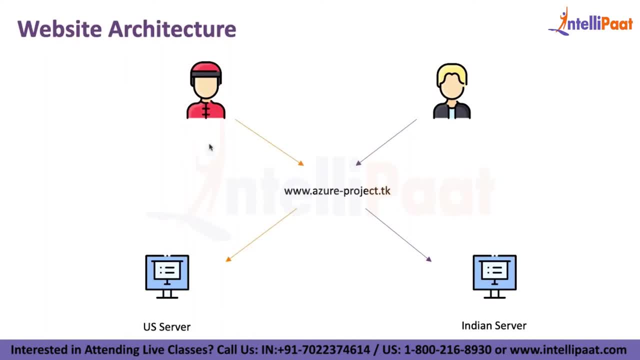 this load balancer, uh, if you are in the us region, if you go to a particular domain, basically it should be pointed to the us server automatically. and once you are pointed to the us servers, your load balancer should basically- uh, you know- divide the load between the people or between the servers. 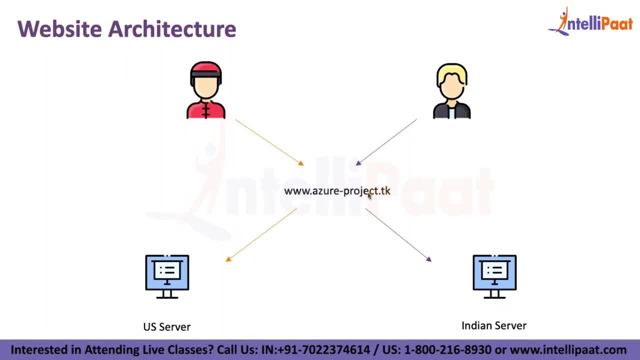 that you have in your fleet right. similarly, if let's say you are from india, you are going to have a load balancer in india, so you will also be accessing the same domain, which is, uh, this right, and once you access it, you will be basically pointed to the indian servers, and in indian. 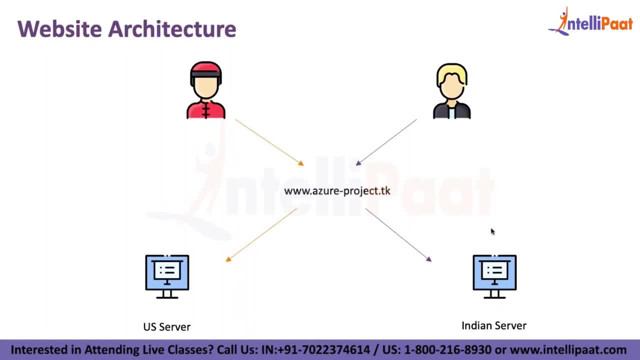 servers. we are going to have a load balancer which is basically going to route your request to a specific indian server. okay, so this is the architecture. so, uh, let me repeat it again. so, first thing, what we'll do is we basically uh, deploy some servers in us and deploy some servers in india. 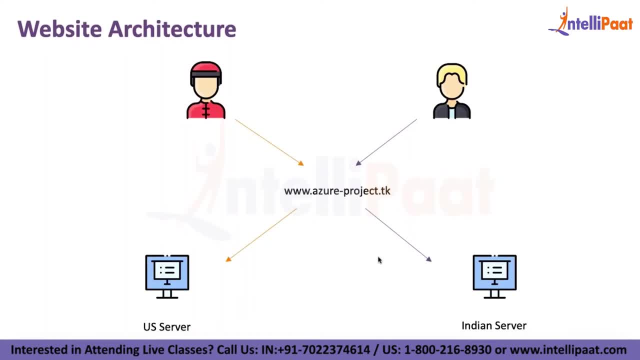 right, and these servers will have a load balancer on top of them. so now what is going to happen is, if five servers are hosting the same application, your user does not have to be concerned about which of these five servers uh, he has to reach. he will basically reach to a common point, and that 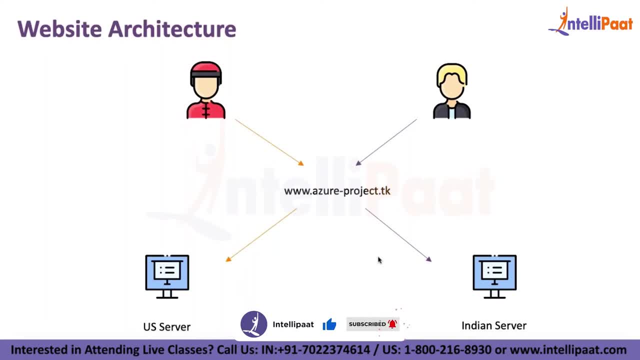 common point will be the load balancer, which is basically going to route the request based on which server is going to be more free. okay, and that is exactly what we are going to do with the us servers as well. okay. so, guys, this is the architecture. there is going to be a separate entity over here. uh, that entity is basically: 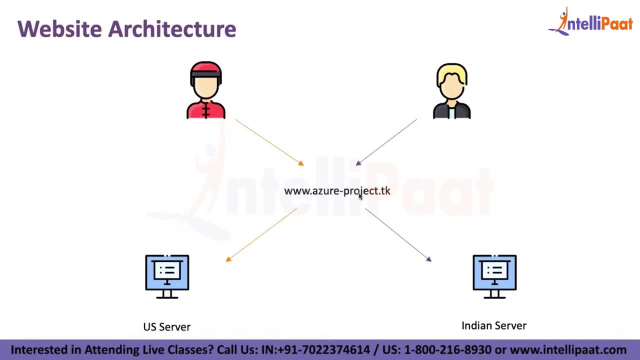 called a traffic manager. right, so that traffic manager has a feature wherein it can see according to which region the request is coming from and which, uh, which of the servers- that is, either the indian server or the us servers- based on which request, where it sends the request and where it. 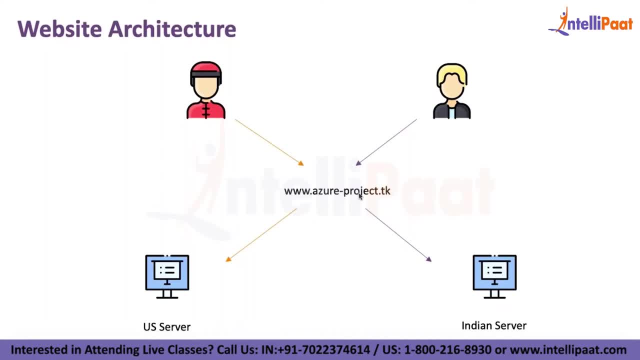 can deal. the faster uh deal the request, more faster it will route the request based on which request over there and obviously, uh, that basically has to do with the distance uh between the customer and the server. so let's say, if you are in india and you are trying to access as your project, 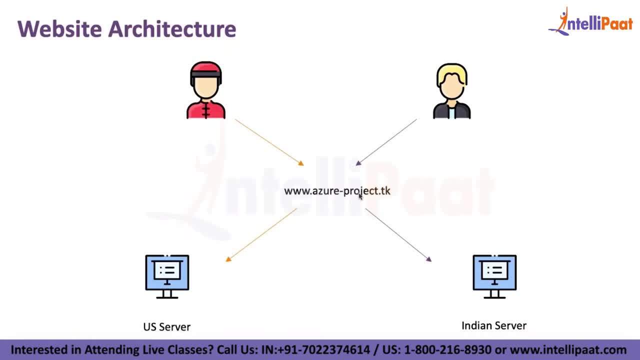 or tk right. so obviously, if your request is being served from the us servers, the uh ping will be more, or the time it will take to uh, you know to, to respond to your query would be more than the servers which are which are basically deployed in the 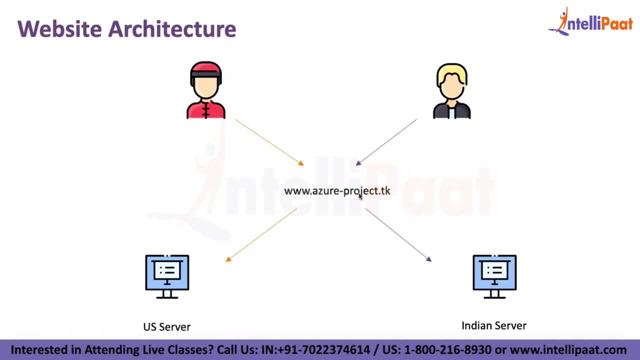 indian region. so, indian region, if you are from india, the servers can reply to you more faster. similarly, if a guy is from us, right? if he is trying to- uh, you know- ping a particular website and that website has servers in us, obviously they can serve them faster than servers which are going to be there in the indian region, right? so this? 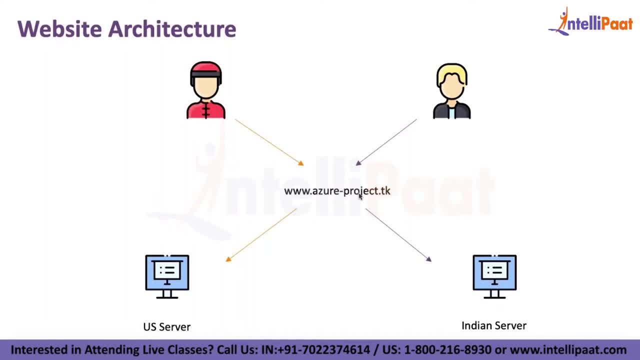 is the architecture that we are going to deploy today. this is basically how even a modern e-commerce application basically works. so if you have a look at flipkart or amazon, these are the things that they implement into the background, which normal customers usually don't know about, but they basically use every day. okay, 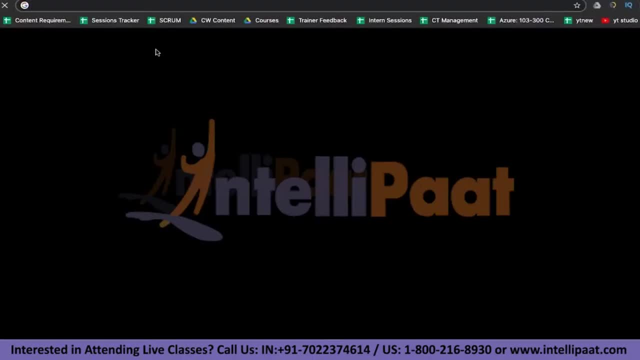 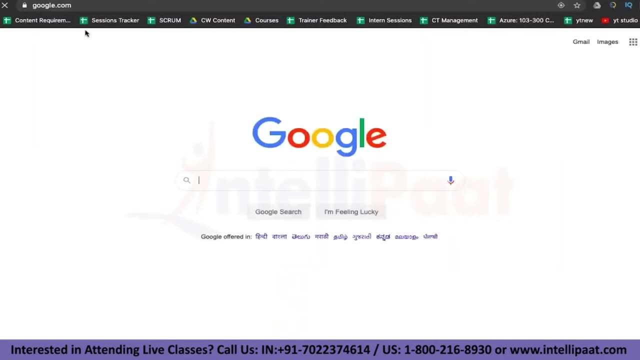 and that is exactly what we are going to do. so let's say, i type in googlecom, so you will automatically see. the moment i type googlecom, i'm automatically uh routed to the indian server. so, as you can see, it's written india over here, right? if i type in googlecom, 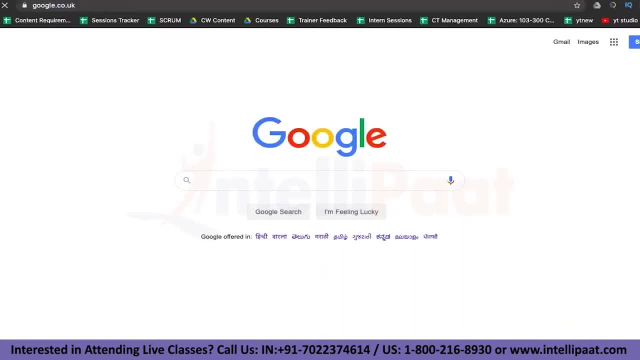 dot. co dot uk. you can again see i'm still on the indian server. why? because every time i'm trying to go to a different google website, i'm always logged to the server which is more nearer to me, and that is the indian google right. so no matter which url you are entering over, 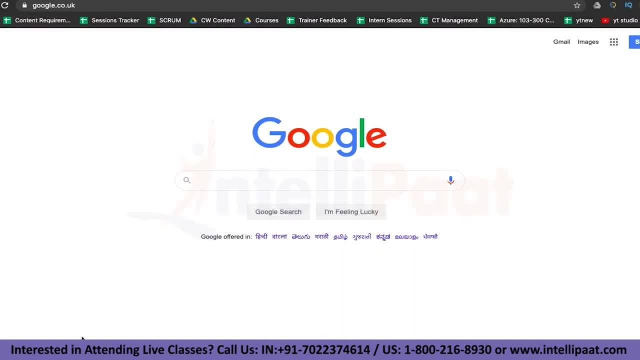 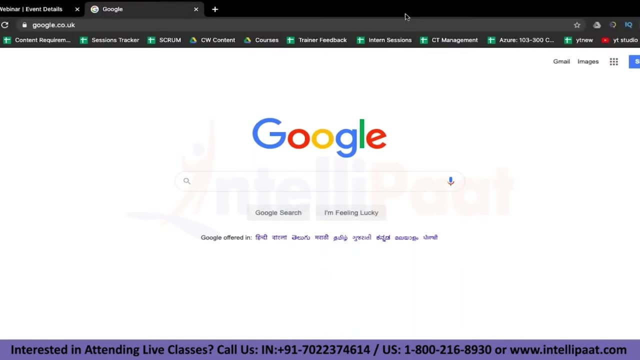 here, you're always being redirected to the indian google, right? but if you want to bypass this, so you connect to a vpn, right? let's say you connect to a vpn and you connect to a particular country, so whichever country you will be connecting to, let's say you connected to uh. 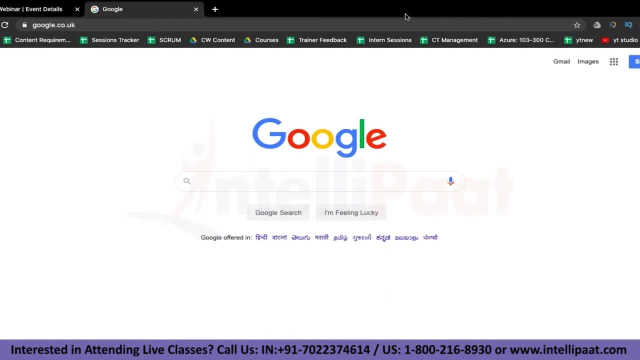 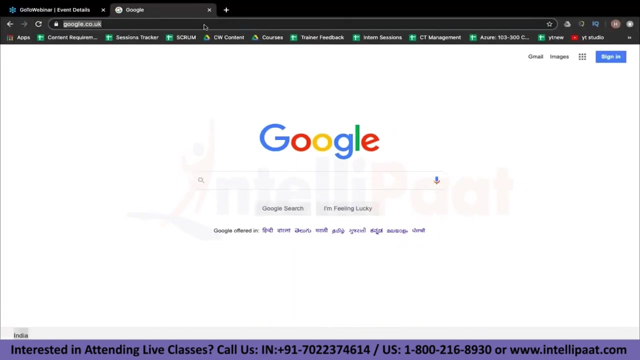 you connect to france. so now, when you will be going to your browser typing in googlecom, now you will be directed to googlefr, right? so that is exactly how it works, what we are going to implement in today's hands-on as well. let's go ahead, and the first thing that we would do 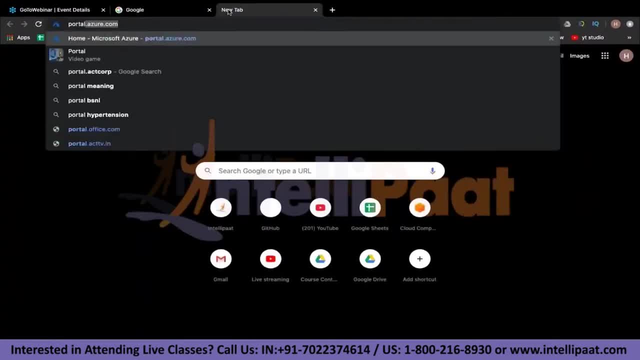 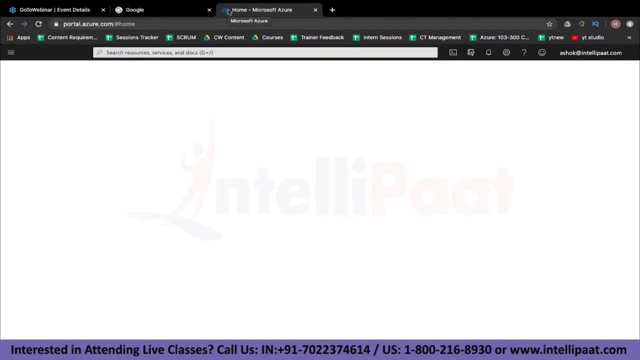 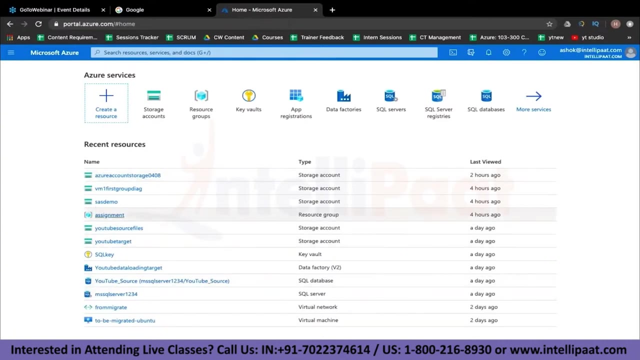 is go to the azure dashboard. so the url is portalazurecom. so once you guys log in or sign up on microsoft azure, this is how your dashboard is going to look like now. now, i already have some resources, uh, that i have deployed over here, so you 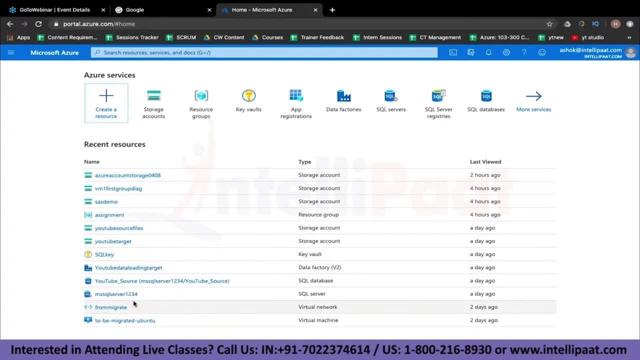 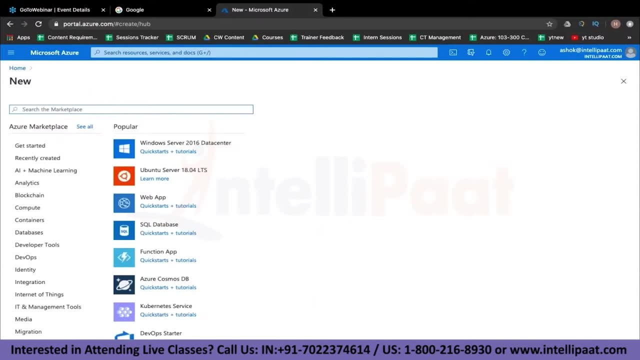 don't have to worry about them, right? so what i'm gonna do is i'm gonna create a resource and once i've created a resource, now i will choose what kind of resource that i want to deploy. so when i'm creating a new now it's asking me what kind of resource that i want to deploy. let's say i want to. 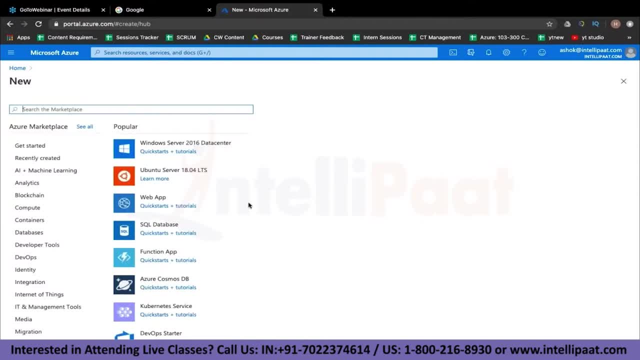 launch a linux server. so a linux server is basically uh, either an ubuntu server or it could be a centos server. but if i want to launch a windows server, i can choose this windows or i can choose some other uh operating system as well. so this gives me limited option of. 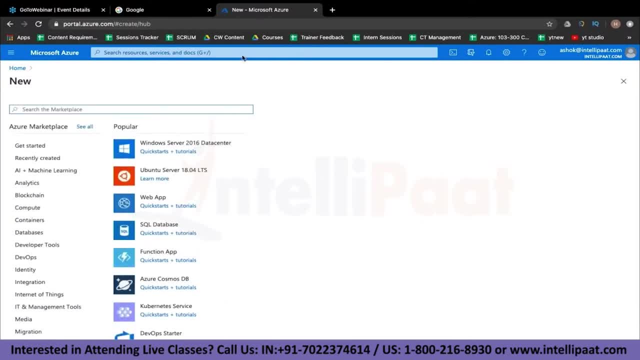 opacity. so let's agree this as an ubuntu and if i feel okay and uh, run it some more. it's gonna work out for both. i'm just gonna click on the покinna thing and then add a specific version of the composer, because i think that's going to give myself a choice. okay, i'll open up my folder and 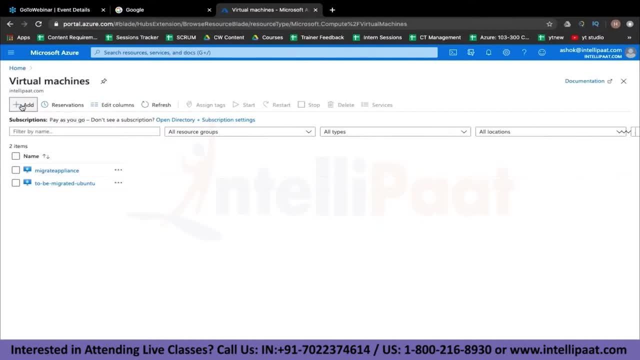 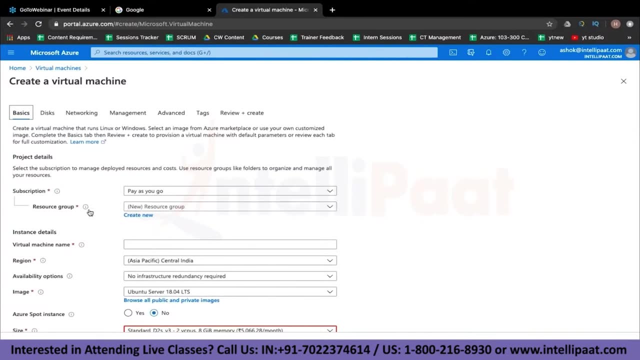 i'll just go public review my pages, i'll go back to my main folder, i'll go kubectl this one and i'll just 제일 onlinexual stack um. and now that i can do that, you guys, you can see, here i am first things. first, it will ask you a resource group to basically deploy it in. 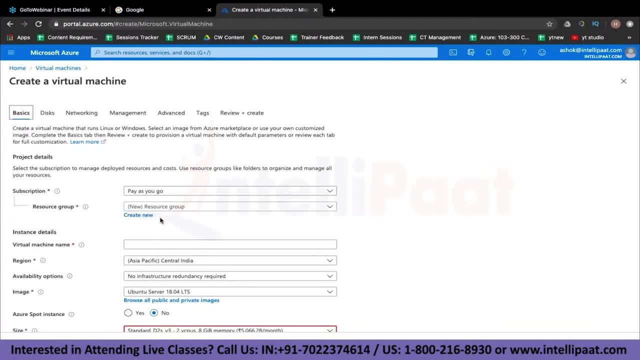 so a resource group is nothing, but it's basically a logical grouping of all the resources that you're going to deploy on the as your cloud. okay, so what we can do is we can just click on create new and let's say, this is demo- hyphen webinar. 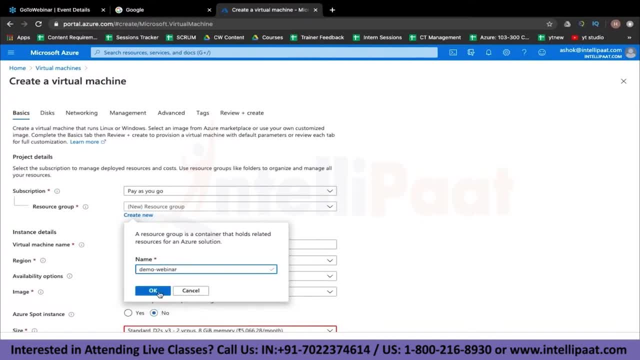 this is the resource group that I'm basically going to create right now. okay, so the resource group has been created and now we have to enter the virtual machine name. so let's say it's Indian server. so this is the server that we are going to deploy right. next thing that I'm going to see is the region that I 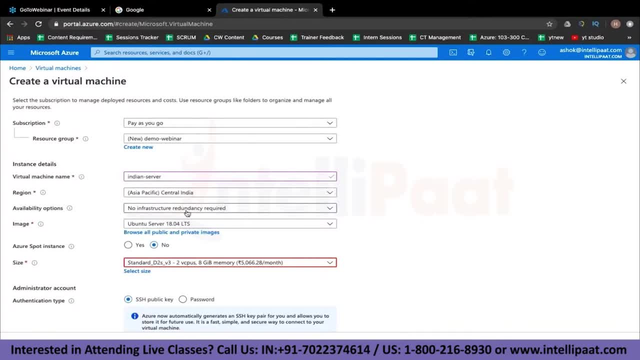 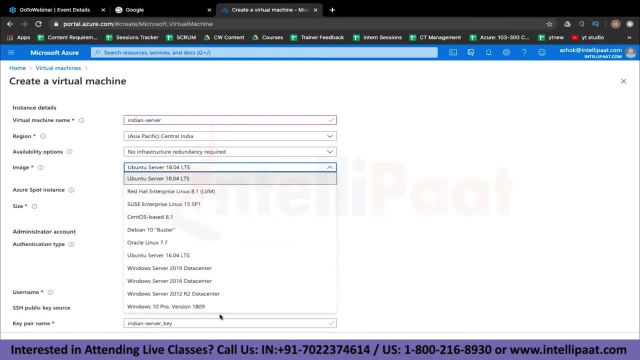 want to deploy it in, so it's in central India, which works out for me, which is great. what is the operating system that I want to launch? so these are the different kind of operating system that I can choose between. so as the Microsoft options, then I have Oracle option, I have the Linux options. 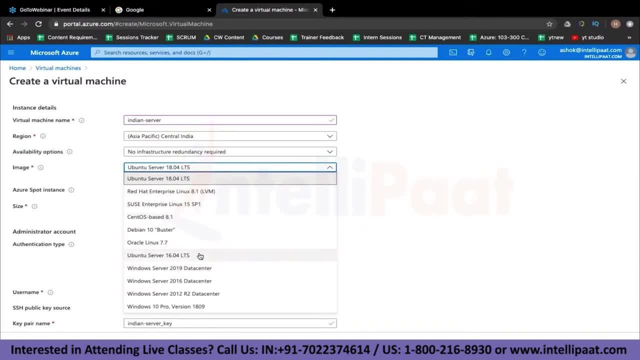 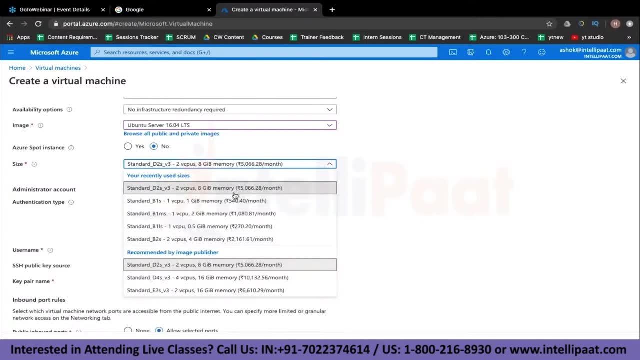 so whichever I want, I can choose. so for this demo I'm choosing the Ubuntu server. then here I can choose the size of the virtual machine that I want to deploy. so let's say, I want to deploy the lowest on this list, which is one V CPU and one GB. 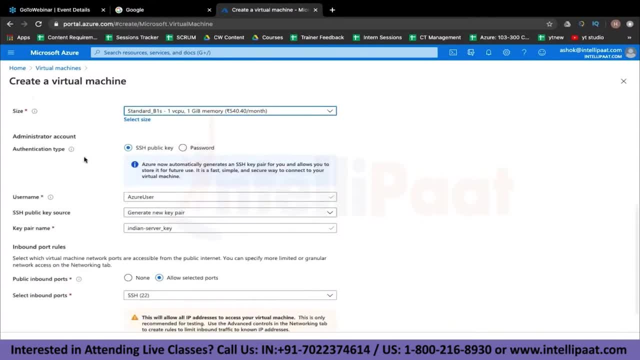 of memory. so let's choose this. then it is asking me what is the authentication type that I want to choose. do I want to log in using a public key or do I want to log in using the password? so let's choose password. let's get some username over here. let's give the username. let's say: 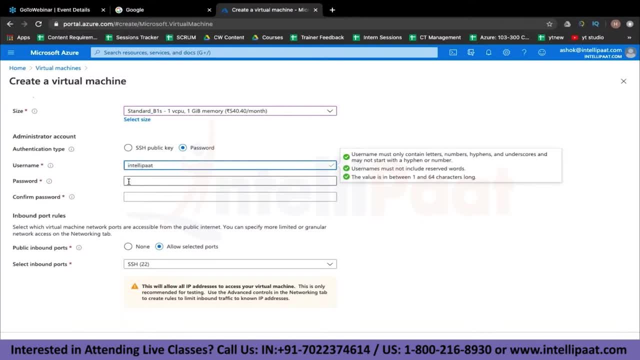 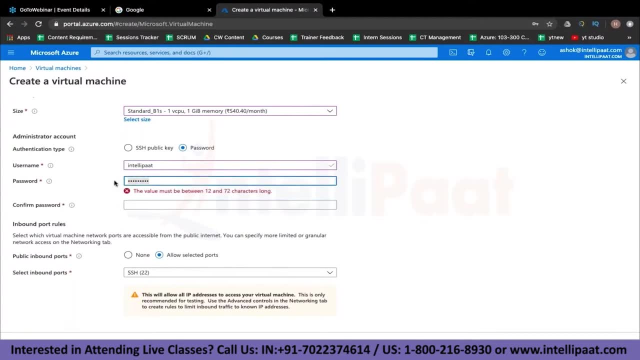 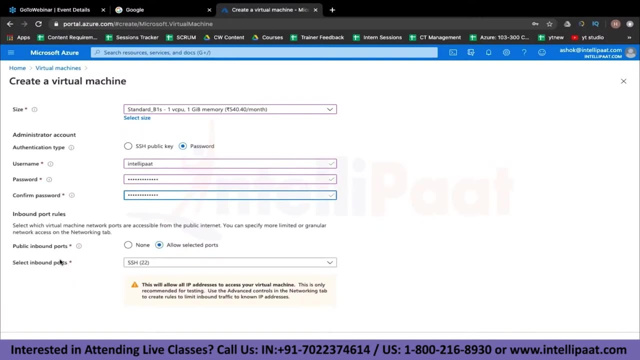 as in telepart. and now let's get some password as well. okay, it says the value must be between 12 and 72 characters. okay, let's get that value. okay now, which ports do I want to be open, to open on the firewall? so, whenever you want to connect to a Linux machine, you 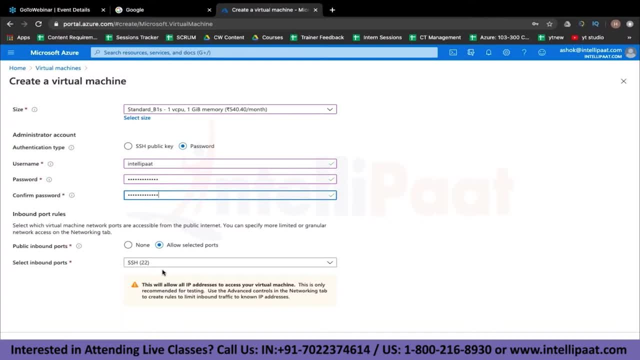 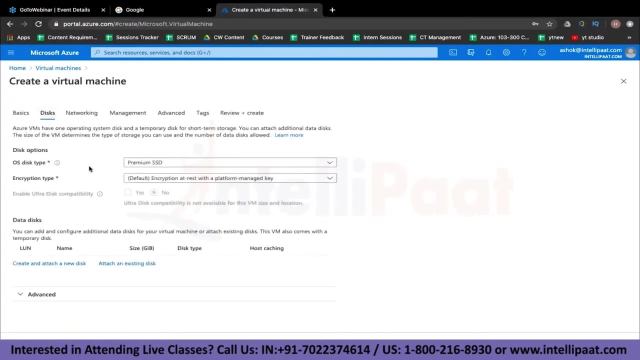 basically connect using the SSH protocol. okay, and the SSH protocol basically always works on port 22, so port 22 is going to be allowed in the firewall for us. let's click on next. so now in disks, we are being asked: which kind of disk do you want? do you want premium SSD? do you want standard HDD? do 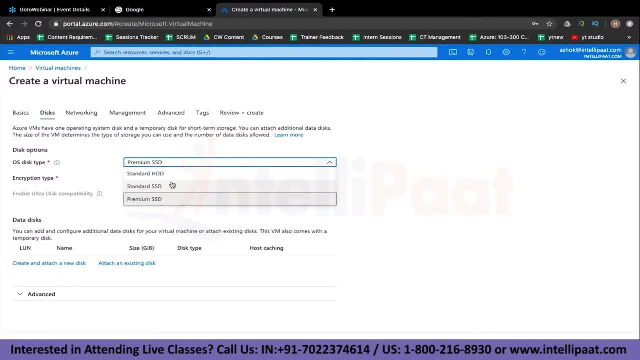 you want standard SSD, so basically, this is going to affect your performance. so HDD is basically a disk based hard drive. then you have solid-state hard drive and premium solid-state hard drive as well, so all these three will have different IO values. for this demo, let's choose standard SSD, alright, and then let's 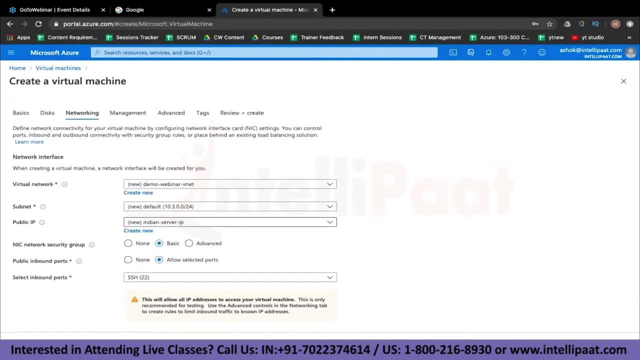 click on next. now it's going to ask me: where do I want this server to be deployed? so it's automatically creating a, you know, a virtual network for me, which is called demo webinar vnet. right, and it is automatically creating a subnet as well. it is assigning a public IP also to 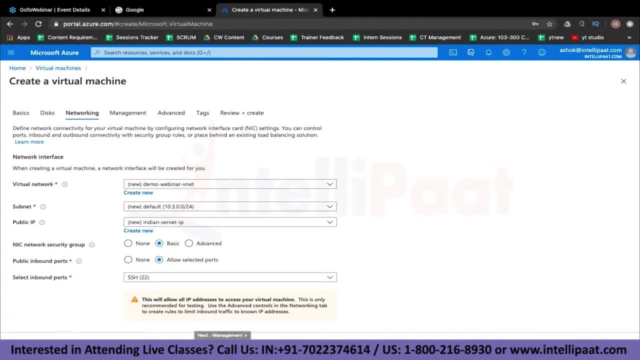 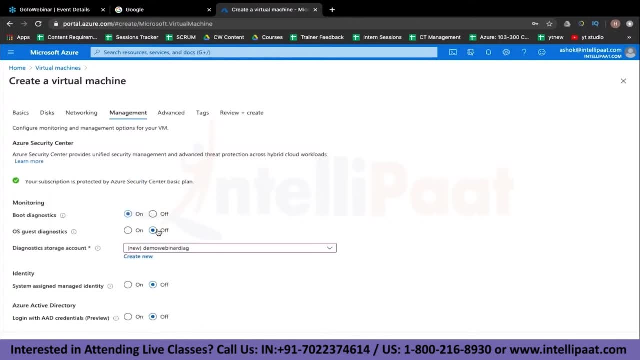 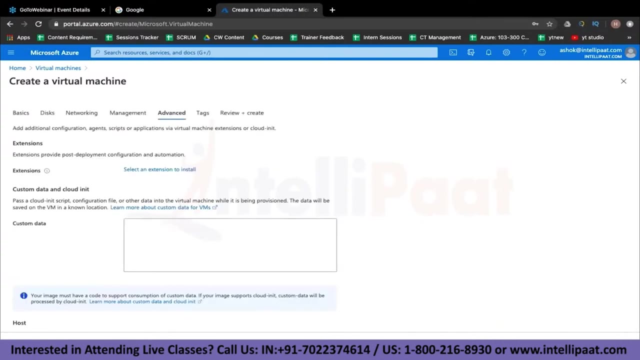 my server, etc. so let me keep everything at default. we'll click on next. now it is asking me: what kind of monitoring do I want on my server, right? so I don't want any more monitoring. so I'll just switch it off and click on next again. 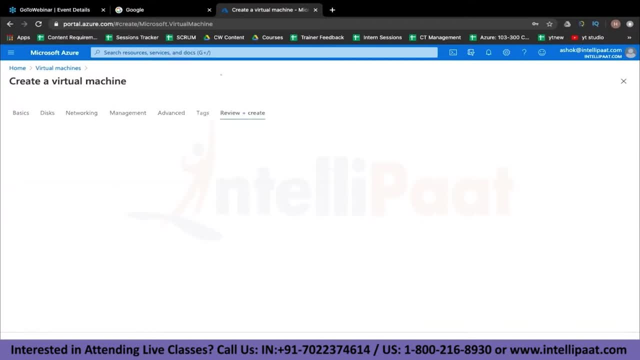 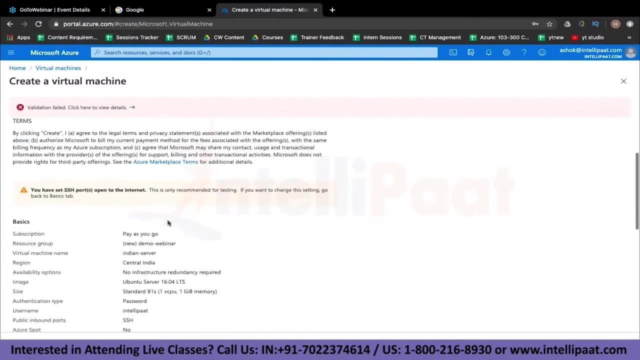 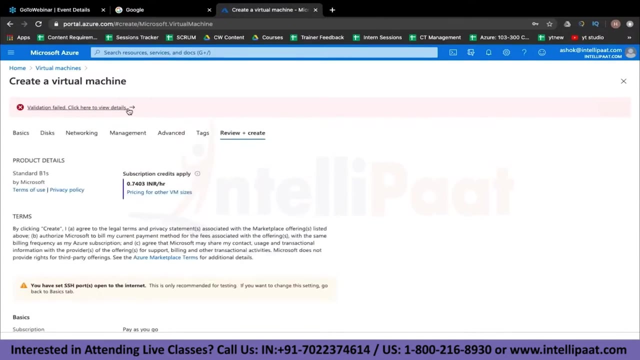 this can also be left, so you can just click on next, next again and finally. now you can basically just review all your settings, right? so it says verification failed. so probably we did not fill out some information. let's verify that, so we'll just click here. okay, it says the requested size for resource is currently. 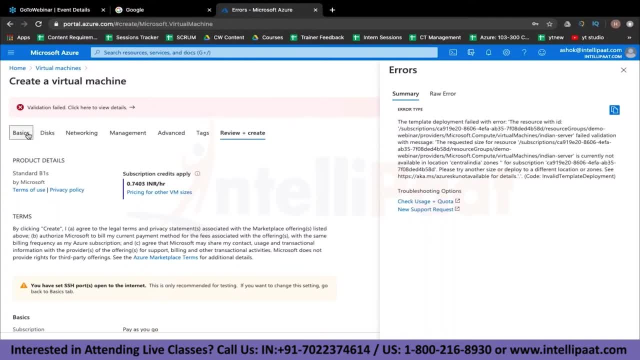 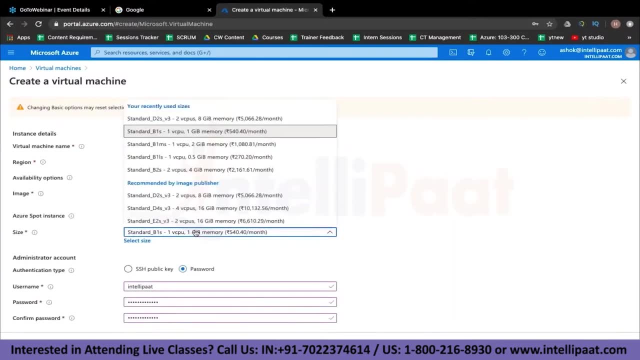 not available in central India. so it's saying the 6 О A Sound of music, S Sound of music, Sound of music that are selected, which is, uh, basically, this is not available, so let's choose some other size. uh, let's choose, let's say, an 8gb machine. 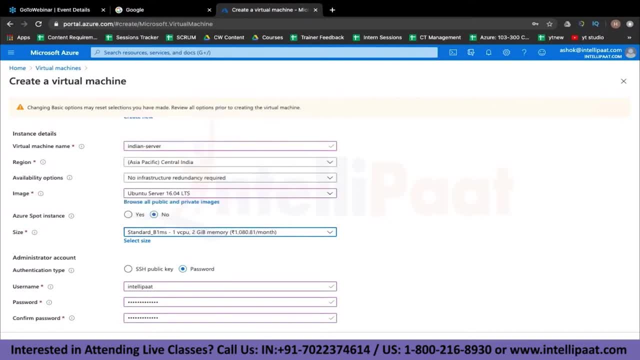 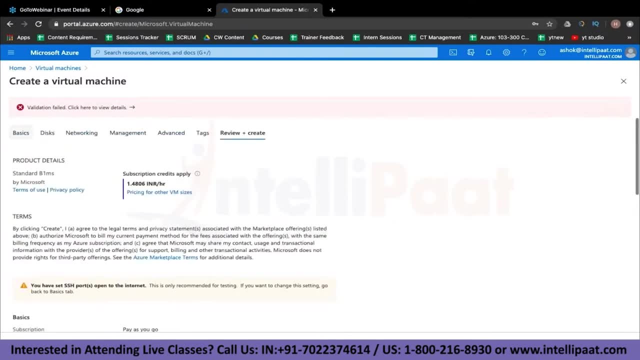 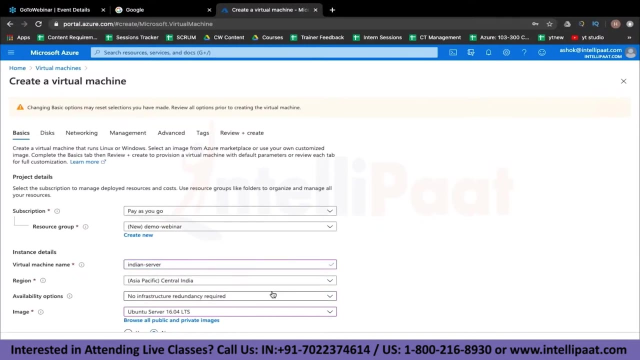 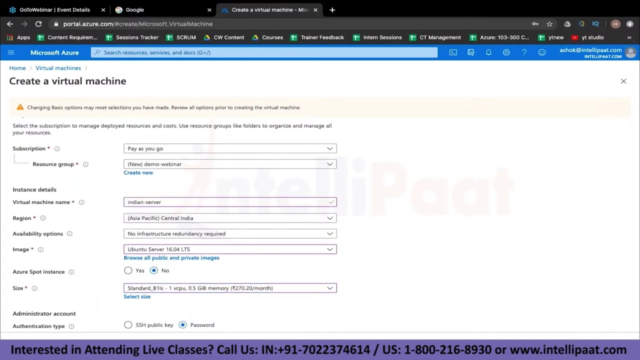 or a 2gb machine. let's say, let's click on review plus create. okay, even this is not available, all right it. so sometimes, the region that you choose, they might not have the required size that you want to launch and in that case you just have to go ahead and choose for a size. 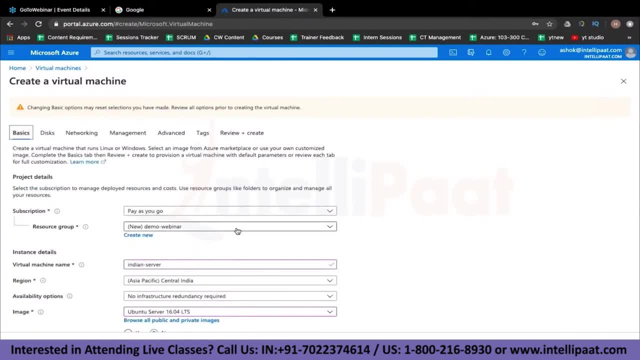 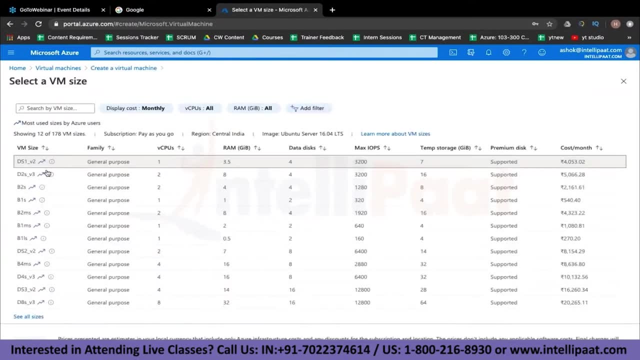 that might be available. i think if i go for a premium size, it should be available. give me a second. okay, so you can see that the high demand for all these servers and that's why they're all used, right, so what we can do is we can just go back. 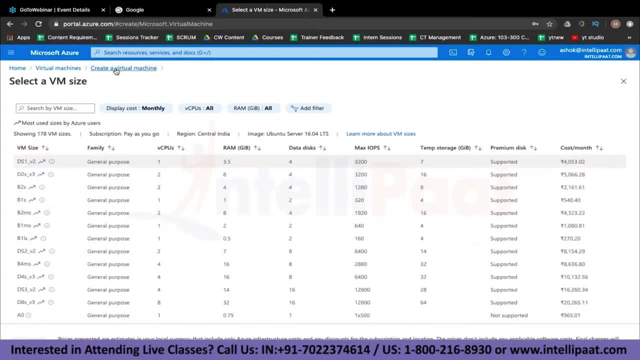 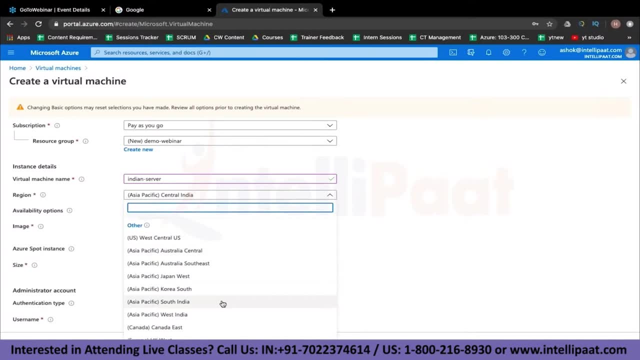 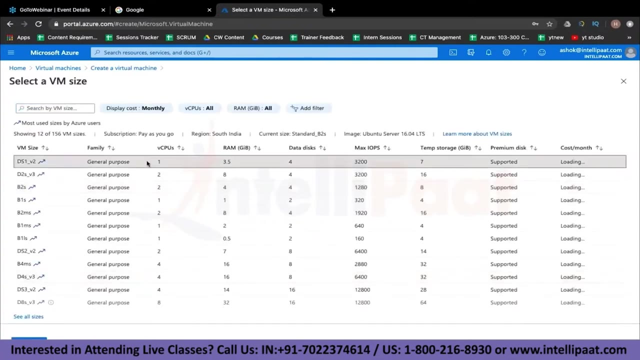 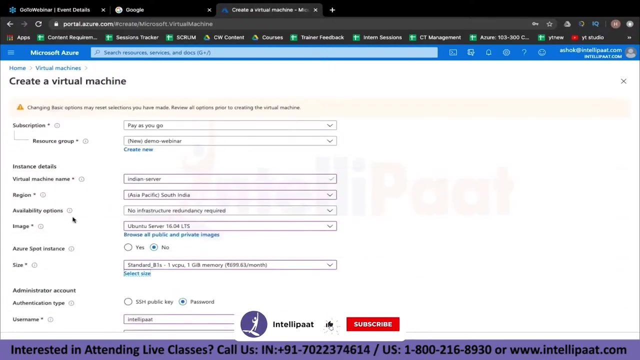 and none of the servers are available in this region. so let's go to some other region. uh, let's select, uh, south india. i think that should have some servers available for us. okay, so here are some servers are available. great, so what we can choose? let's choose the same size that we selected earlier. click on review, just create. 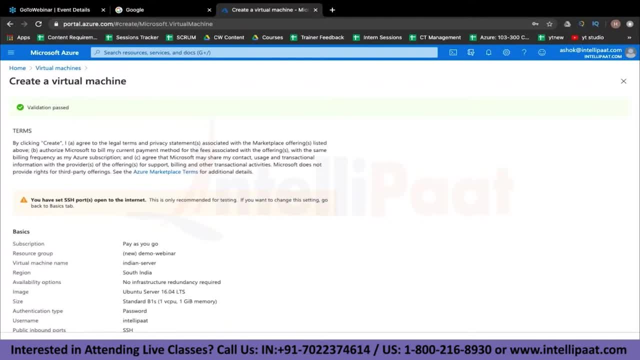 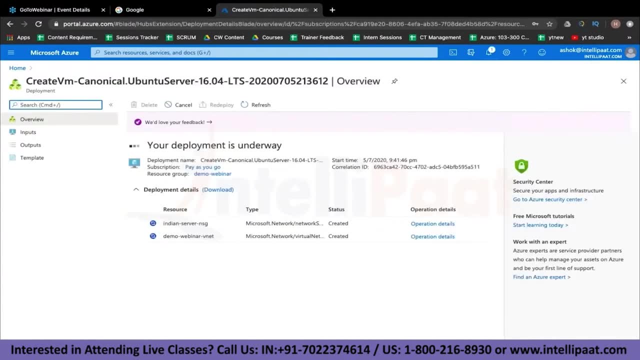 and, as you can see, the validation has now passed, so let's click on create now. with this, now my server is getting launched. okay, now it will take some time for this server to get deployed, but basically what we have done is we have deployed one server in the south india region. 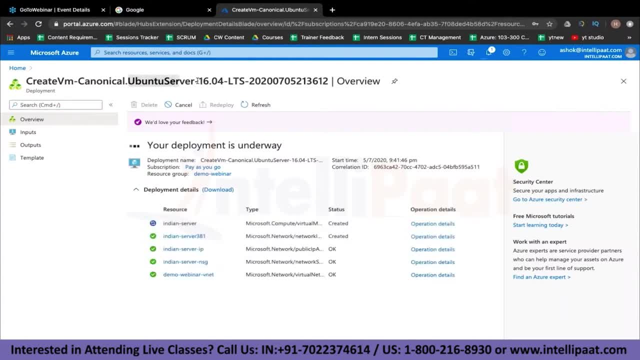 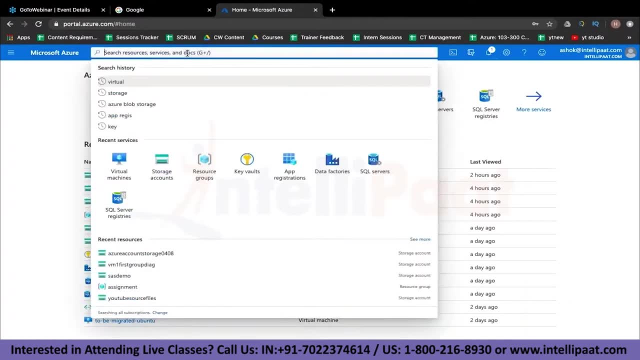 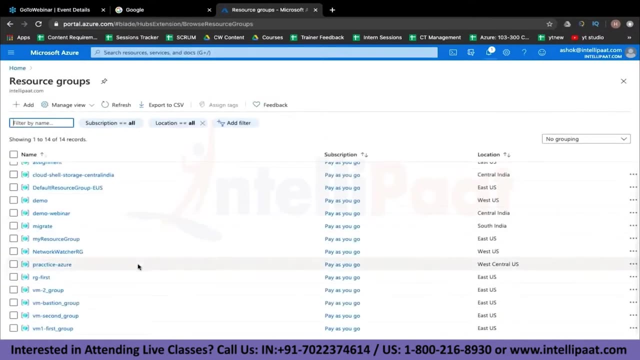 which basically, is going to make use of an ubuntu server. okay, so let's go back to the dashboard and let me show you the uh resource group which is basically getting created. okay, there are a lot of resource groups over here, but what you can basically refer to. 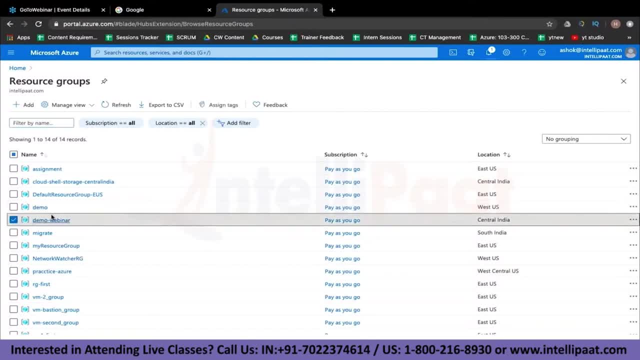 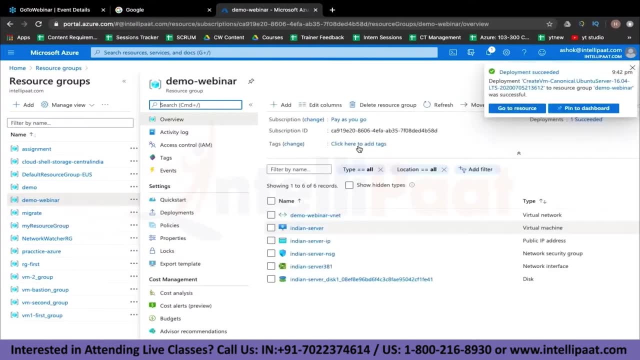 is this? so demo webinar is the resource group that i created right. so now let's go ahead inside the demo webinar, and here you can see the resource that you've just deployed: the indian server. it is getting deployed in it, so, as you can see, the deployment has got succeeded great. so let's deploy a us server as well. so again, let's click on add on. 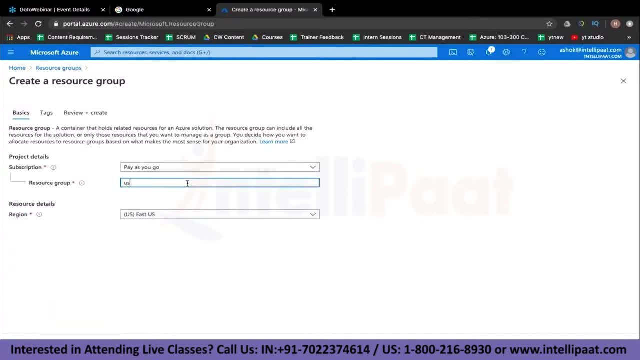 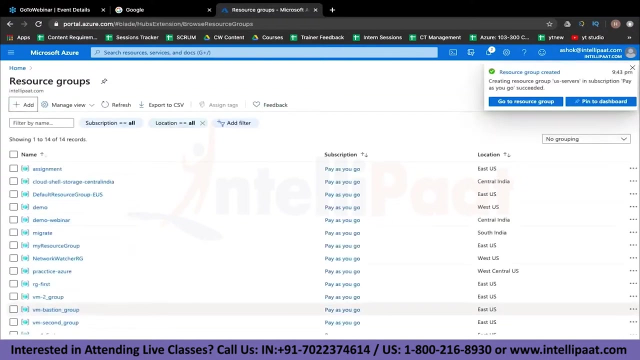 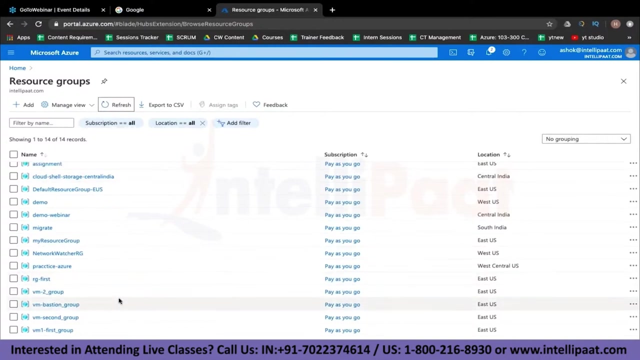 the resource group. let's create a second resource group for our us servers so that we can differentiate resources that we are going to deploy, and let's deploy it in the best us region. okay, click on review plus create and finally create this resource group. okay, so the resource group has got created and now i can just go to that resource group. 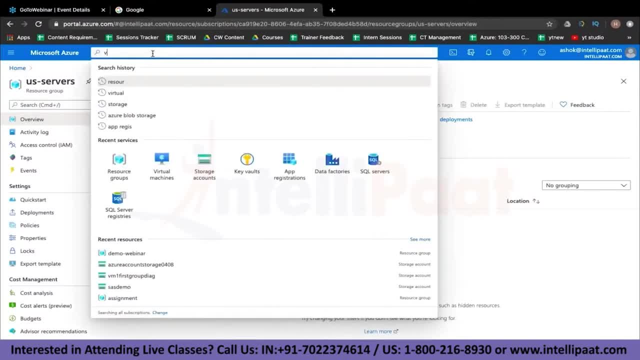 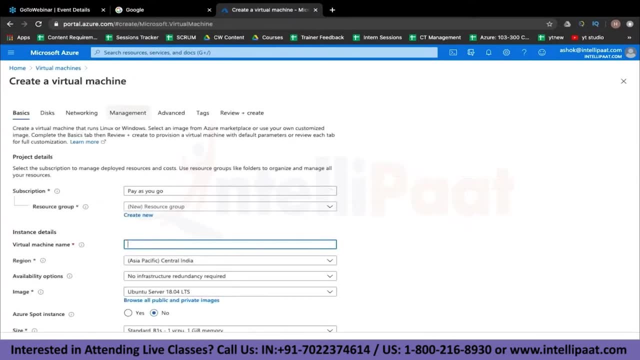 and let's go ahead and deploy it in the best us region. so let's go ahead and deploy it in the best us region, okay, so let's go ahead and deploy some resources over here. so let's do the same thing. let's deploy a virtual machine again in the us resource group. so i'll just click on create a. 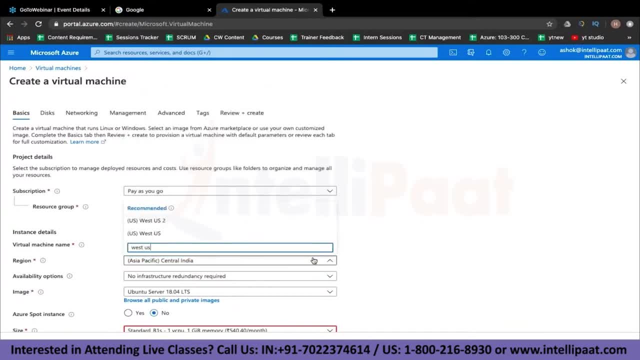 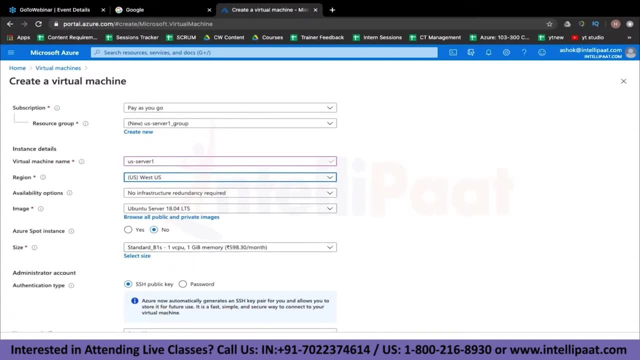 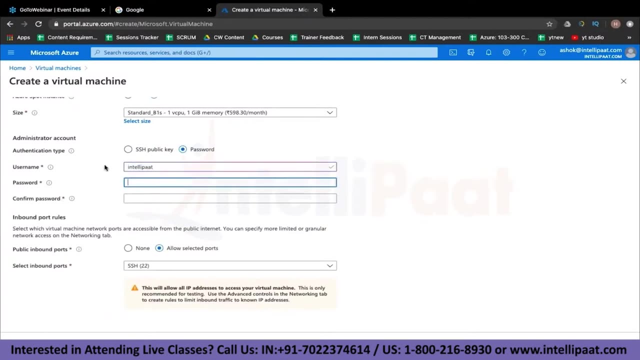 virtual machine us server one. let's get this name. let's deploy it in best us. okay, this is the image that i want to launch. uh, this is the size that is automatically selected. let's hope it is available. let's give the username as in telepart and the password as this. i think i'll keep the same. 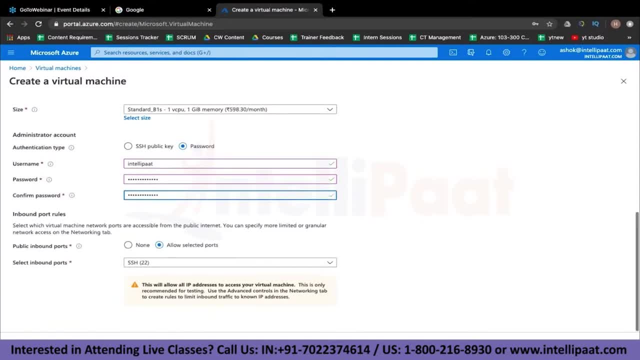 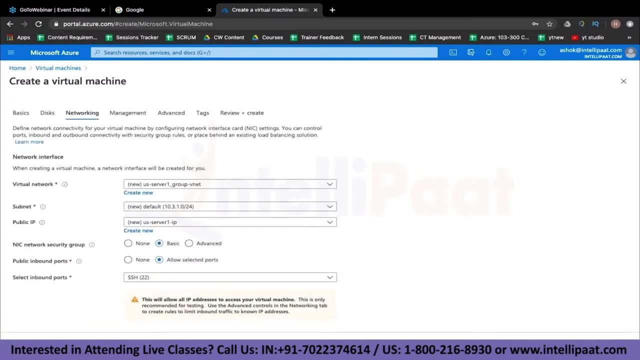 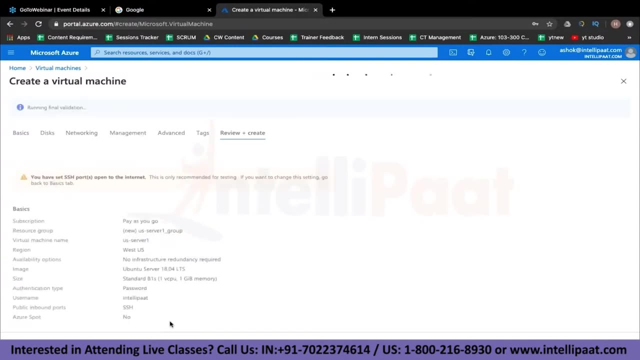 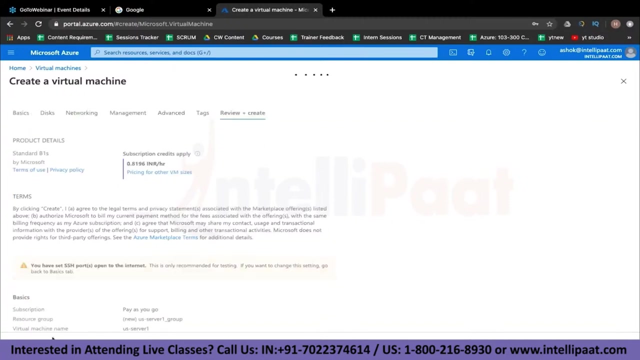 password which i used for my previous server: okay, click on disks, i think, rest everything. we can leave by default only in management. we will turn the monitoring off and click on review plus create. so, as you can see, the price is just 80 passa per hour, which is great, so we'll just create it now and now. a server is being launched. 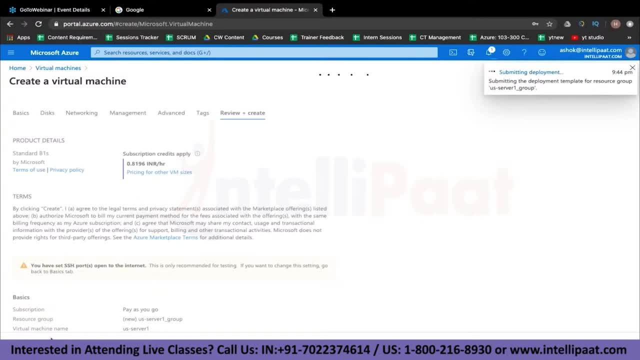 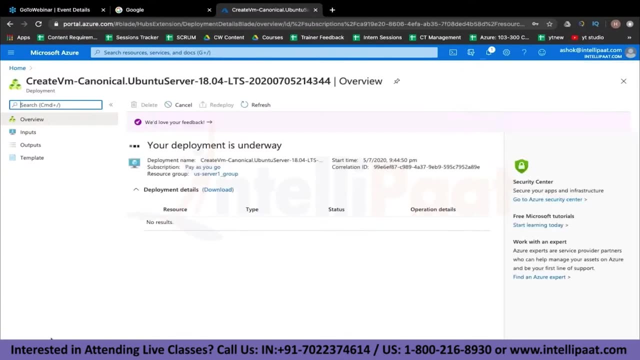 in the us region. okay, now to make it more authentic, let's deploy one, one, uh, virtual machine, more so so that we have two, and on top of these two virtual machines, then we will deploy- uh, you know, a load balancer as well, and we'll also figure out a way so that when we basically hit the load, 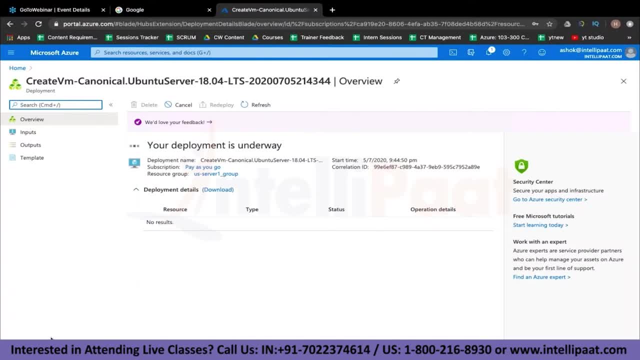 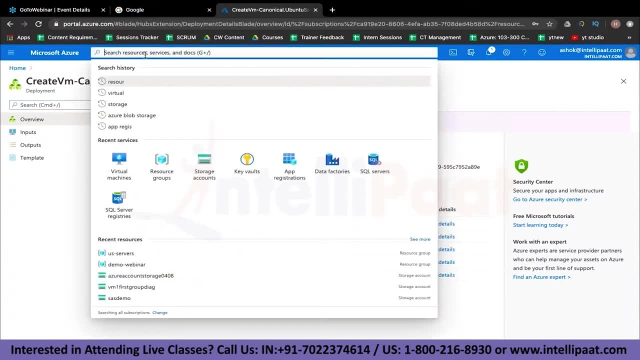 balancer, we automatically get the load balancer, and then we will deploy the load balancer as well to know which server, basically, we are trying to connect to. okay, so, while this is being deployed, let's deploy, uh, one more virtual machine in india. so let's add one more. 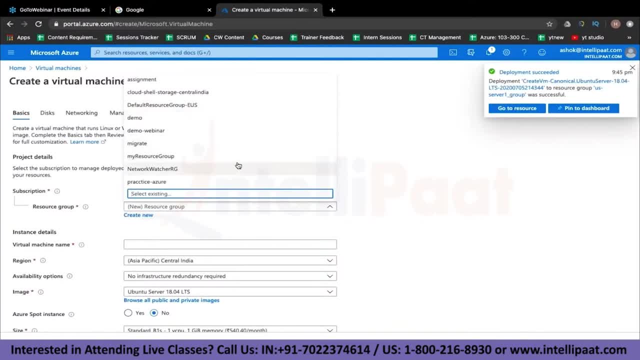 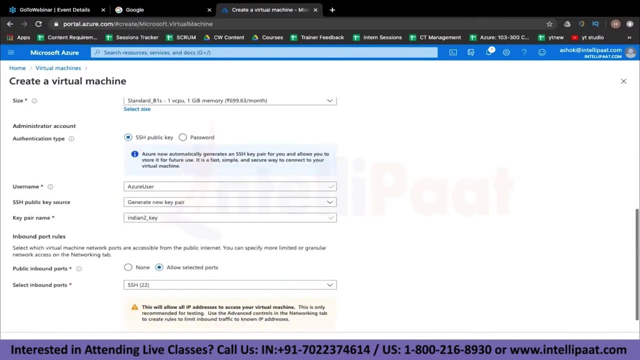 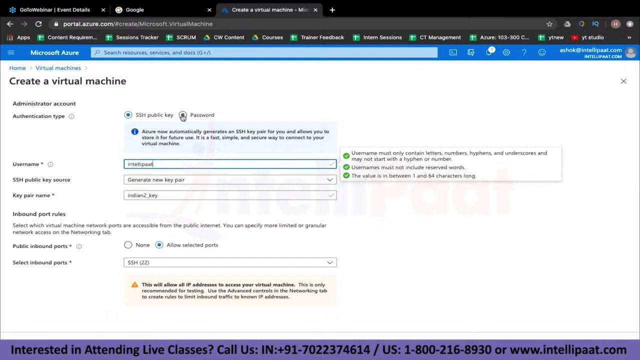 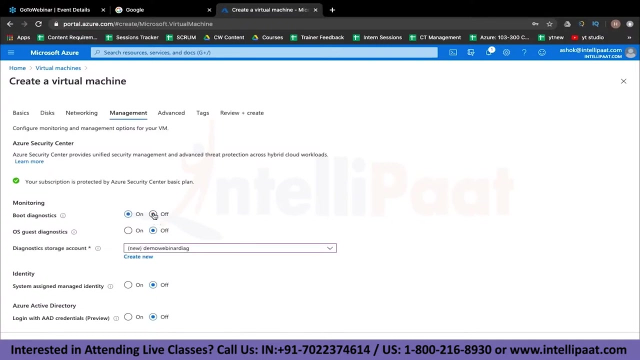 it will be in the resource group called demo webinar. what's the machine name? it will be indian two. it will be in south india region. uh, same image, same. uh, server configuration username would be entire part and let's give the password same. okay, let's go to management. uh, turn off boot diagnostics. and now let's create it. 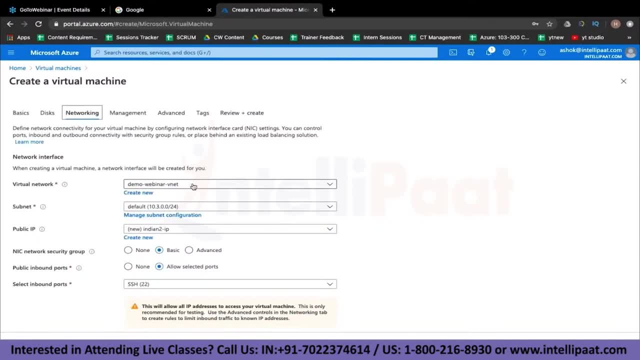 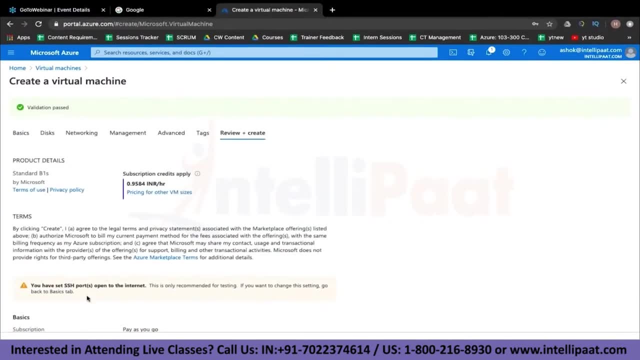 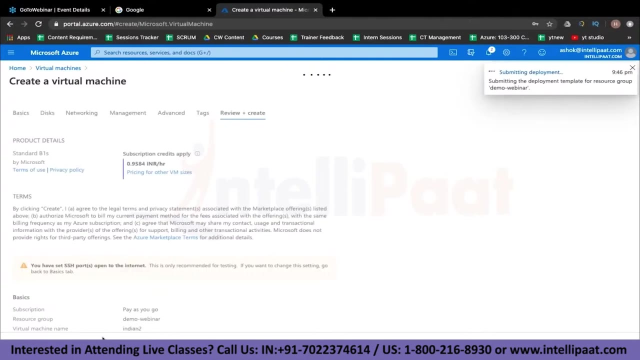 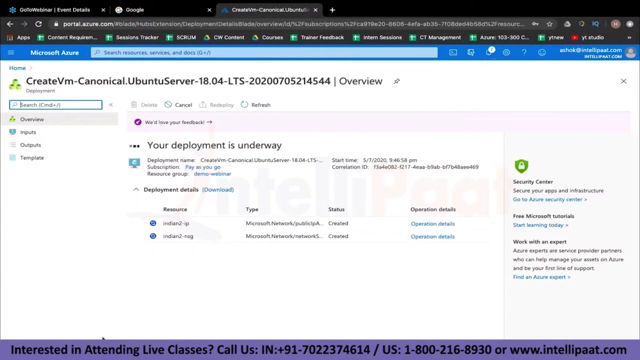 so in netflix networking? let me see. yes, so we are under the same uh network that we created earlier, and now let's just go ahead and create this, all right? so with this guys, we have now deployed uh two servers in the india region, and let's do the. 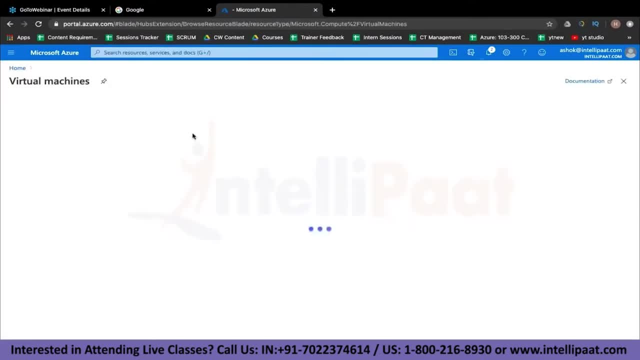 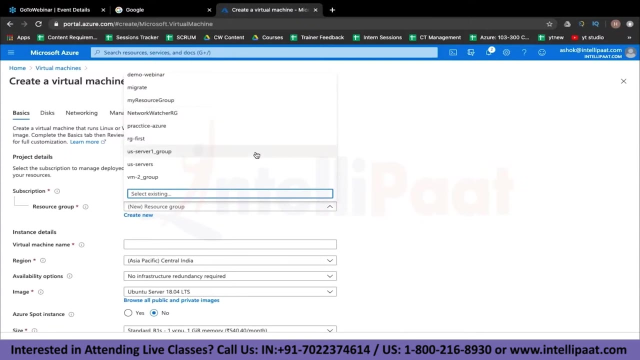 same for us as well. let's deploy one more last uh pm or a us region as well. so this will be in the uh us resource group right and the virtual machine is going to be named as uh- us, so server 2. it's going to be in the west us. 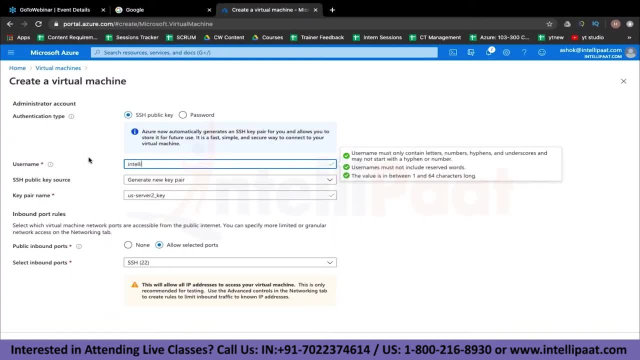 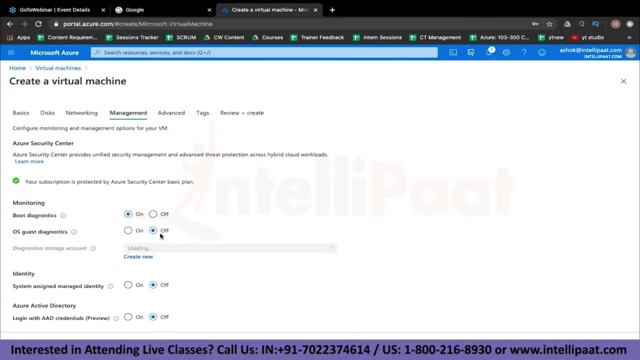 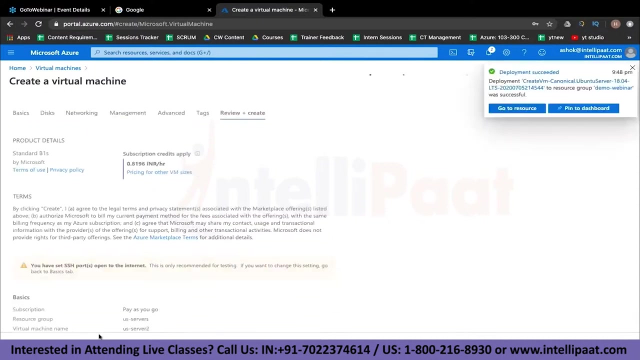 same machine. config. username would be teleport and password would be the same what i entered for those again. finally, we'll go to management, turn out diagnostics, click on review plus create and create the vm now. okay, so now this will be deployed in the background and what we can do is we can start. 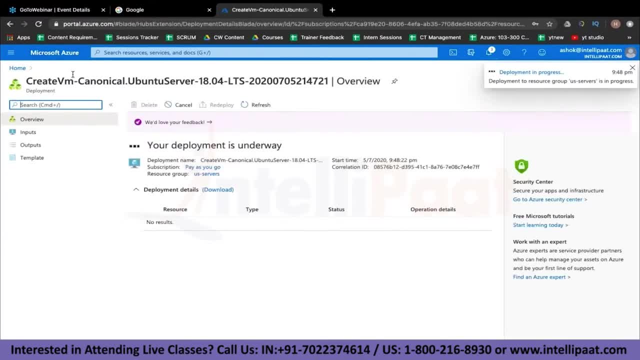 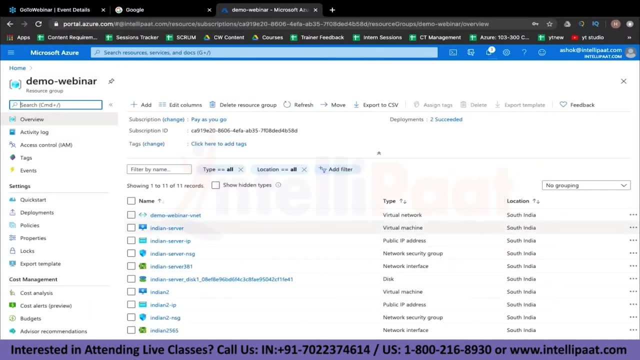 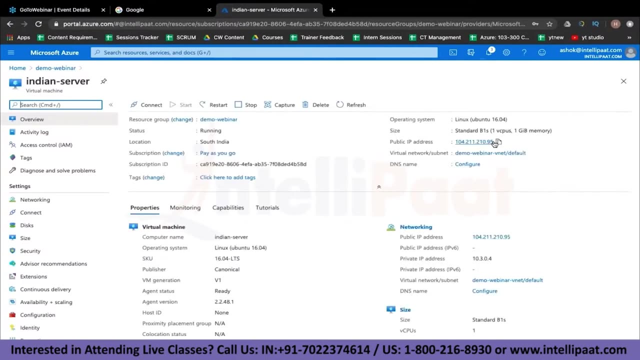 configuring our server now. okay, so let's head over to the us server- sorry, the indian servers- first, and let's try to configure the first server that we deployed. so this is the ip address of the server. let's connect to it. so for connecting you will first. 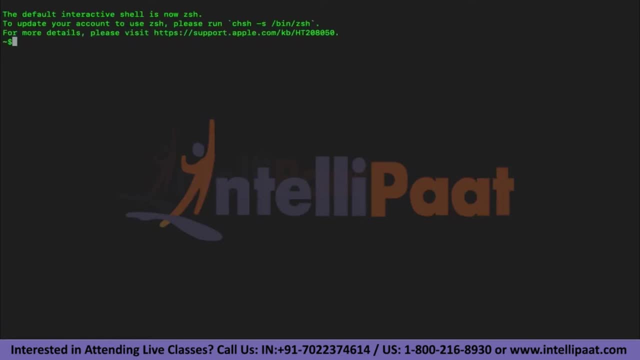 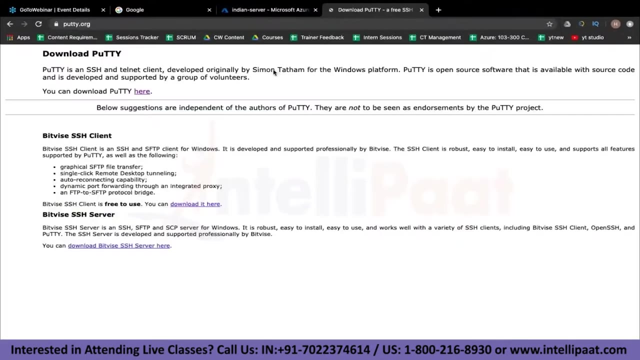 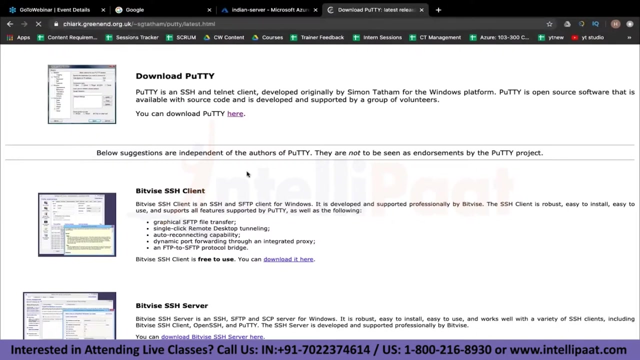 need a terminal, so people who are using windows, what you can do is you can download a software called putty, right, so you just have to go to puttyorg, go to download putty, just click over here and then what you have to do is you have to download the putty 64-bit version, which is this: 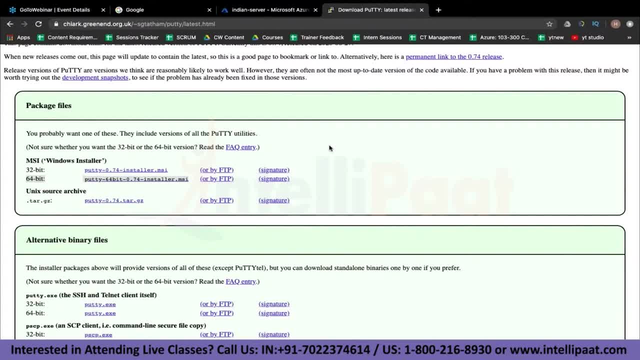 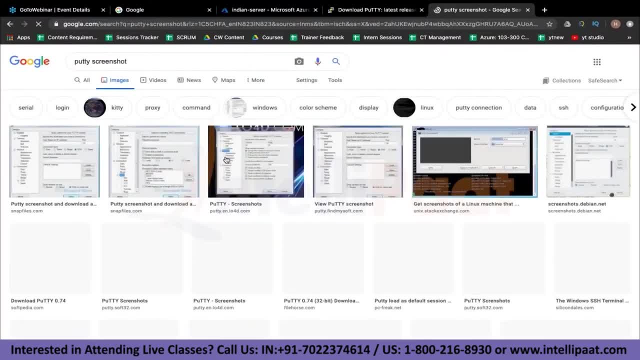 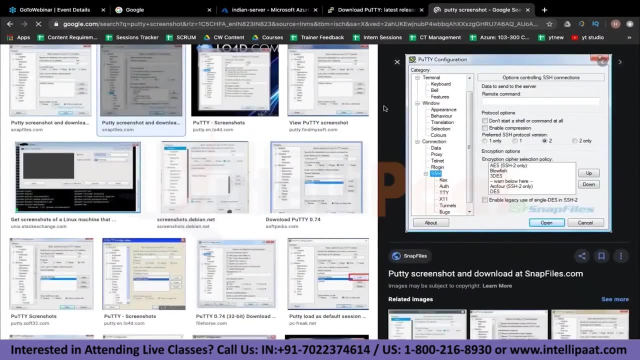 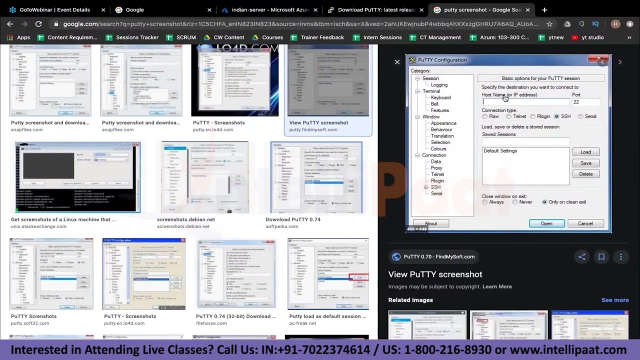 right, and once you download this, uh, you know you will see a window like this, right? so in this window, all you have to do is, uh, okay, one second. yes, this is the window that you will see, so just enter the ip address over here of the server. so, in this case, the server. 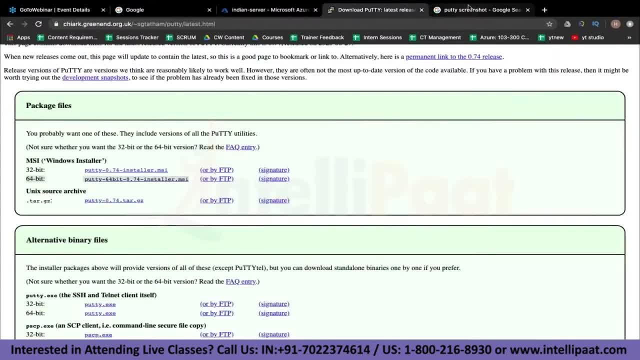 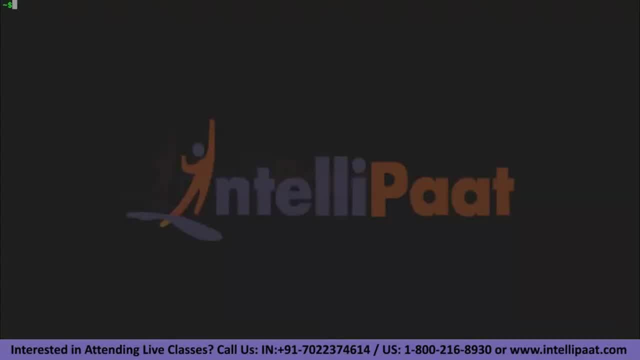 ip address is this: just enter that over here and click on open right, and that is about it same screen. then you will see as i'm seeing right now. okay, so i'll just enter ssh. so, people who are there on linux or mac, you just have to enter this command so ssh. enter apart, at the rate, the ip. 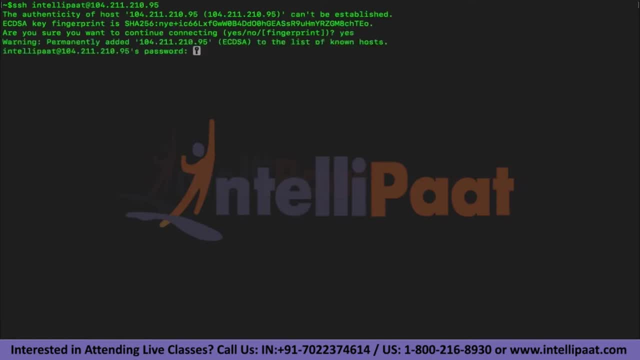 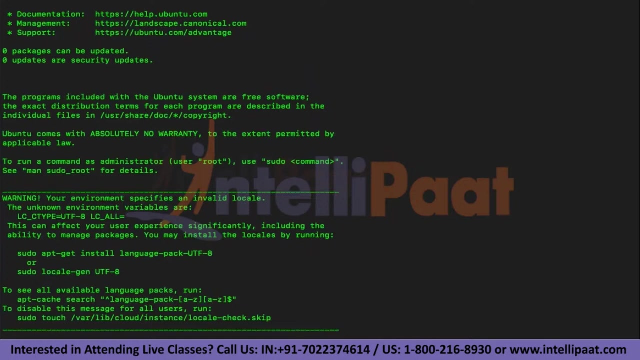 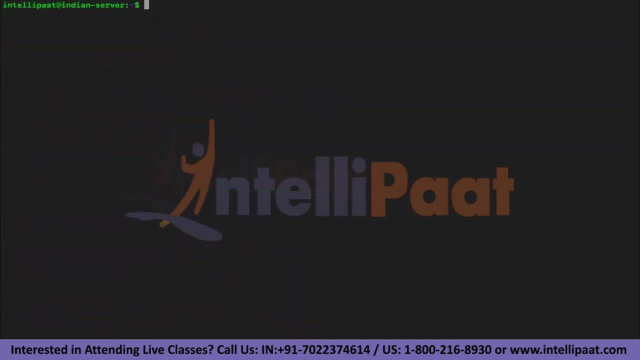 address, click enter. i think yes. it'll ask the password. so just enter the password of the server. even the putty guys will see the screen. and then you are now logged into your intellipa- sorry, your indian server in the azure region. so this is your first server. let's connect to a second server as well. so ssh and telepart. 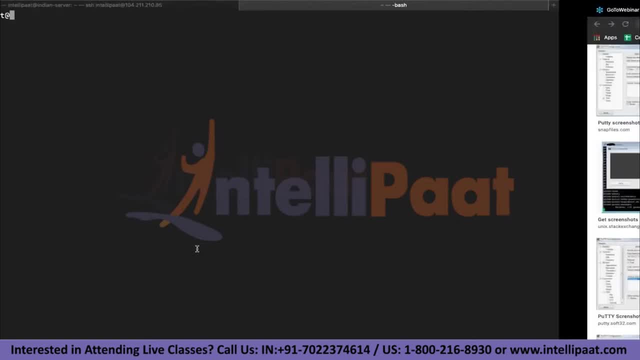 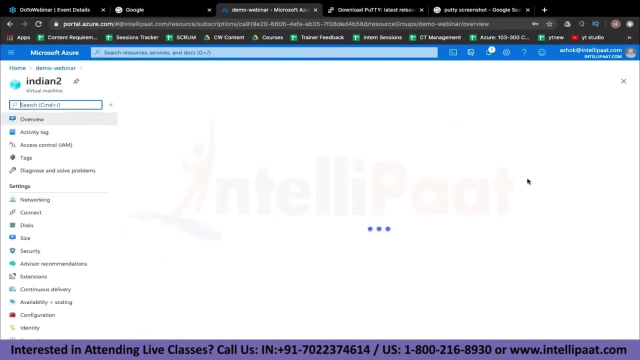 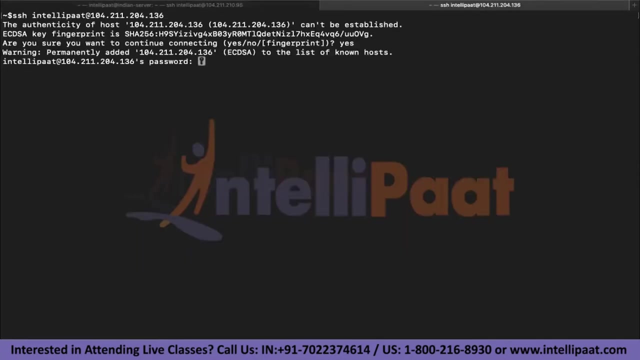 at the rate. and then the second server is this: let's copy and paste the ssh and then go to the server, and here we go, the ip for this server as well, put in here, and now it's asking the password. and yes, you are now connected to your second server as well. okay, what i've done is i have deployed four servers, two in 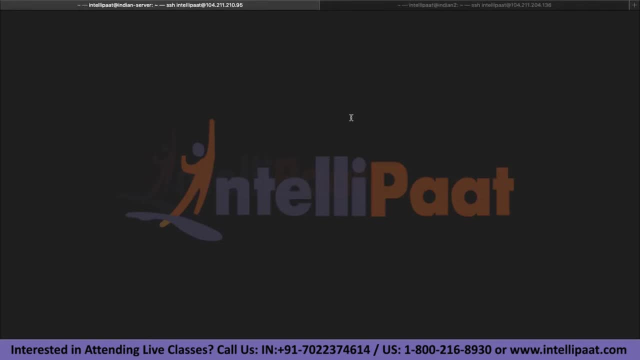 the us region, two in the india region, and now i've connected to these servers in the india region. all right, guys, so let's go ahead and configure these servers now. so what i'm going to do is, first, i'm going to basically install a web server software which is called a party apache 2.. so 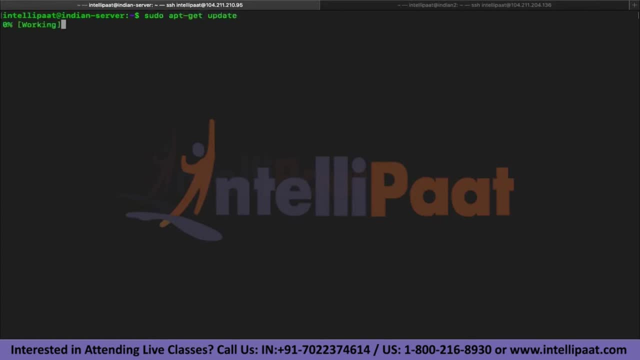 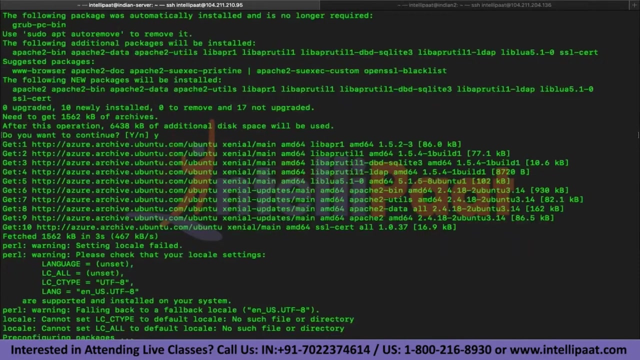 in order to install that, first we'll have to update the machine. so let's update it by typing in the command so we're able to get update, and once the servers are updated now let's install the software by using this command, which is sudo, apt-get, install apache 2.. okay, so the software is. 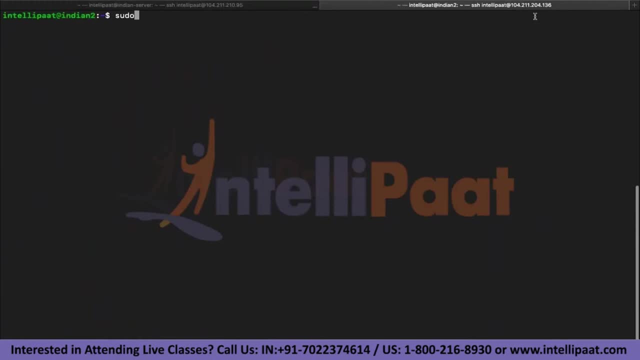 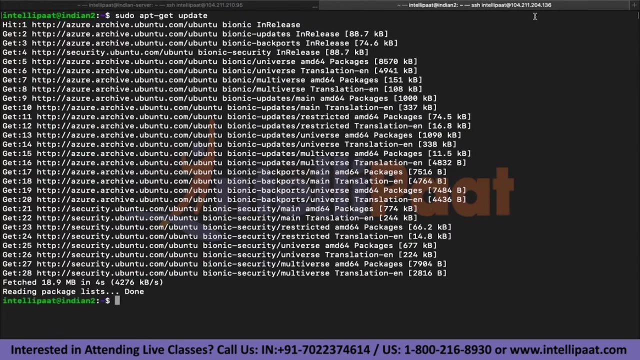 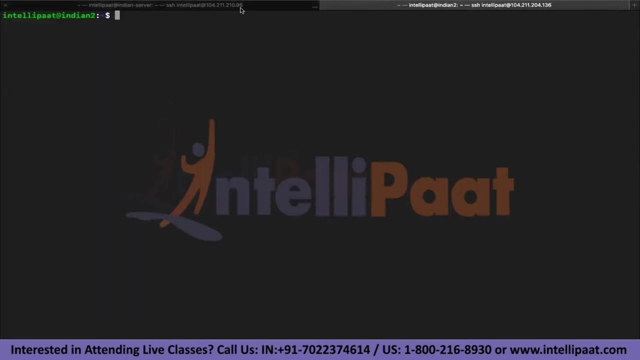 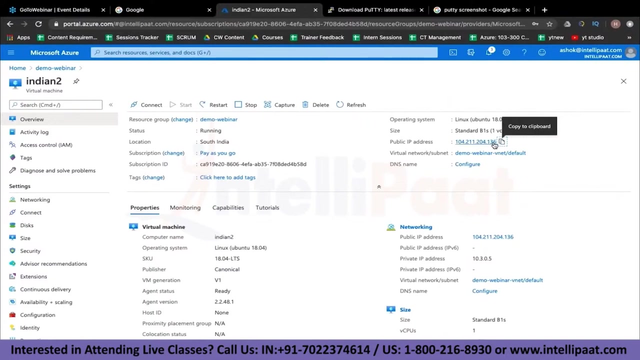 being installed over here. we can do the same on the other server as well. first update it, and once it's updated we will install the apache 2 software. so both the machines now have the apache 2 software installed, and now let's try to see if that software is working or not. so ideally, what should happen is: if you install the software, 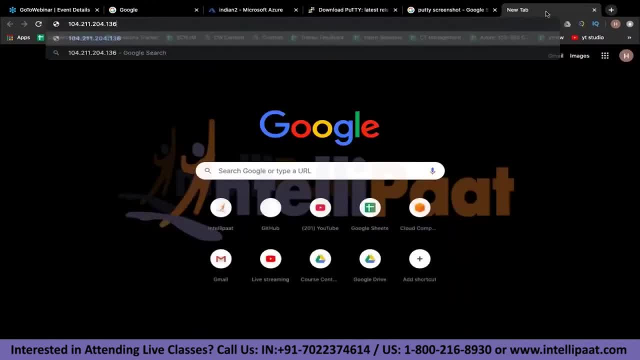 and if you copy the ip address of your server and try to paste it in the browser, you should be able to see the website that you have just deployed. but what happens is, because you know, we have not opened the firewalls for, uh, the http protocol. that's why we are not. 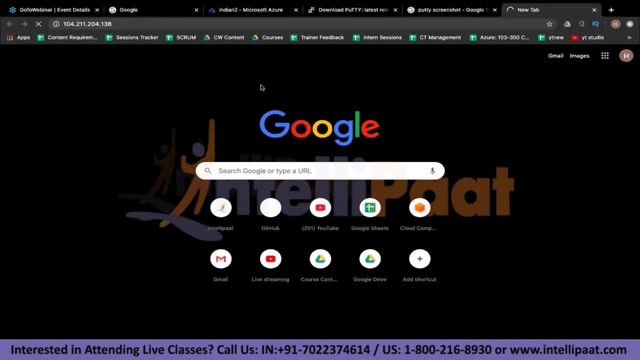 able to see this web page right now. you remember, we only opened the port 22.. so whenever your browser is trying to interact with your server, it always tries to interact on port 80, and that is exactly why you're not, uh, seeing the web page right now. 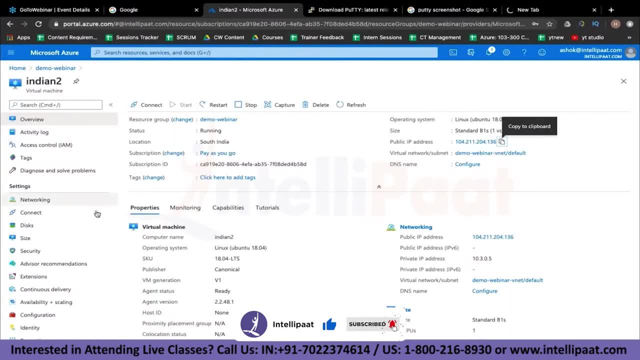 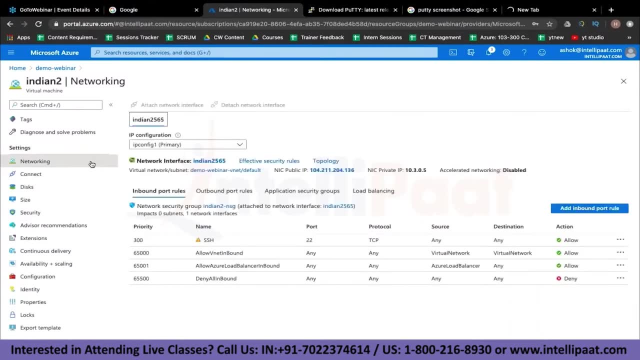 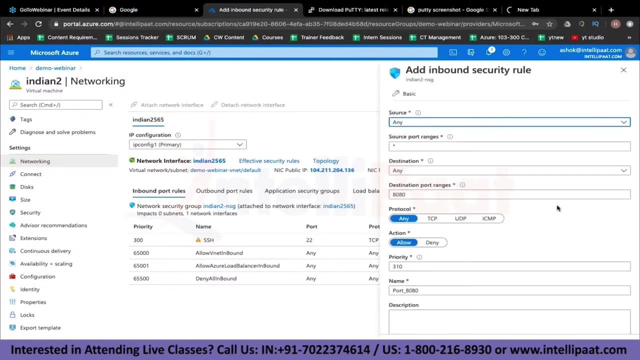 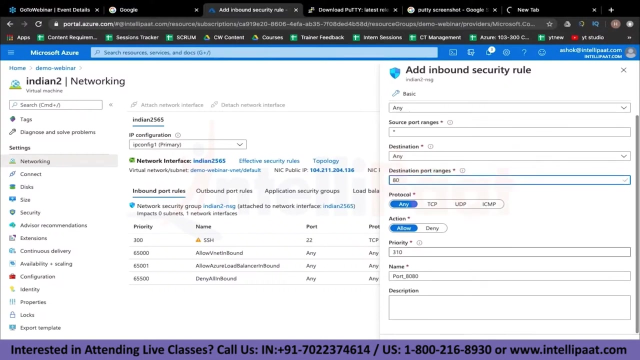 can do is, let's say, this is my indian server 2, so all i have to go to is networking, and in networking i have to add an inbound rule. so in the rule i have to specify the destination port, which is port 80, and it is going to be allowed, and i just click on add. 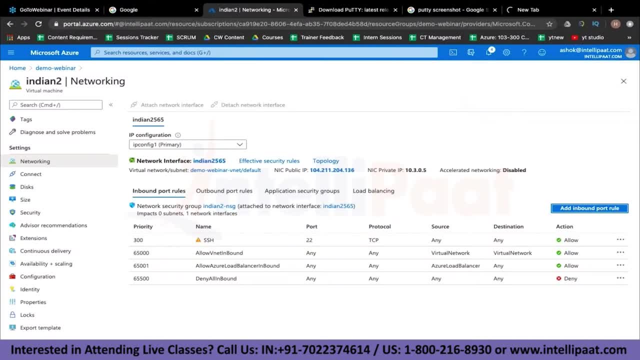 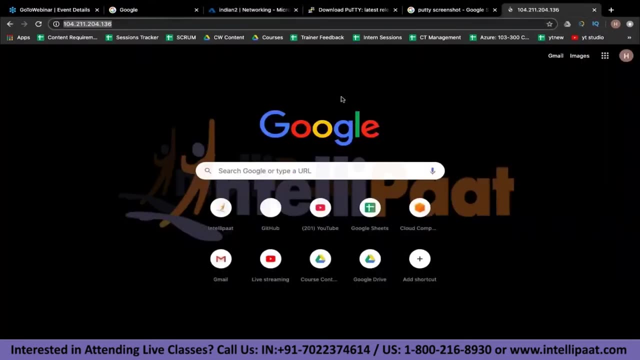 so, with this rule in place, uh, what is going to happen is the port 80 is going to be opened in the firewall and then, once the rule has been created, now, right, so this will take around, uh, you know, 30 to 40 seconds to basically get uh updated in the main firewall of azure. 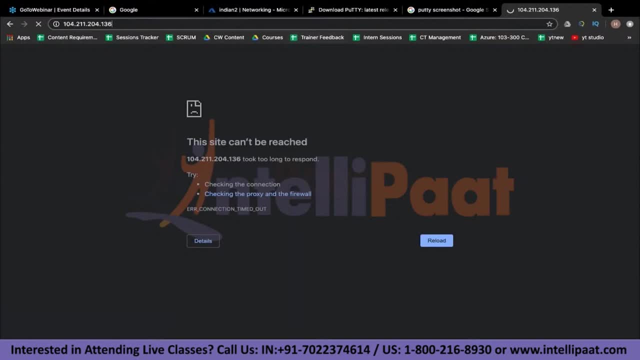 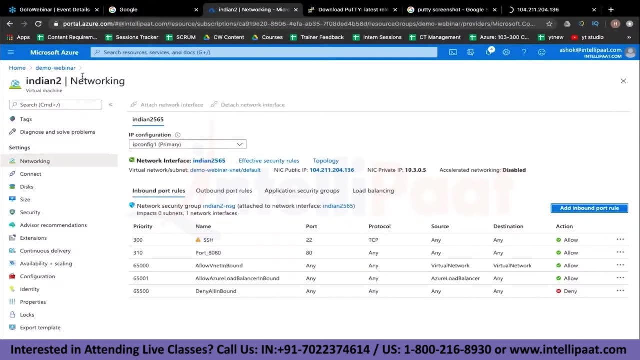 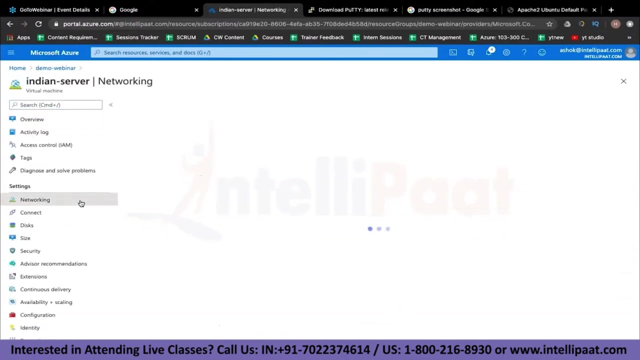 and then we should be able to see this website. so let's wait for some 30 to 35 seconds and while this is happening, let's also open the port 80 on the first indian server. so we'll just go to the first indian server, go to networking and add port 80 over here. 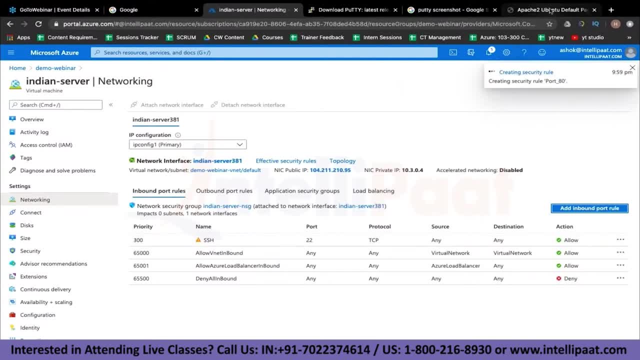 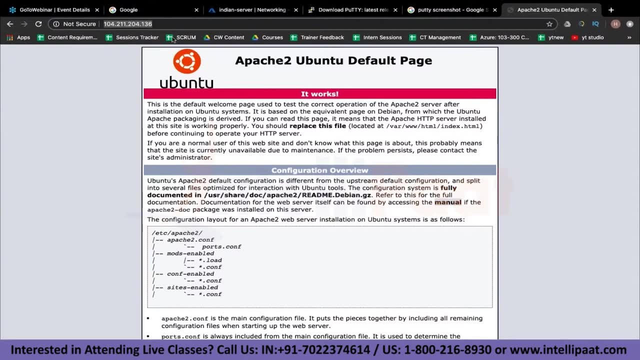 okay. so this rule is now getting created and if i go back you can see on this ip address. i am able to sustain this way. so since i've enabled it, i can still go back and style these IP disappearing to cd apache 2 page. so this is the indian tools ip address and you're going to change this web. 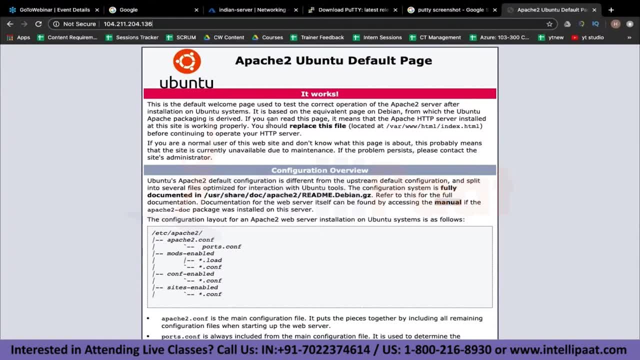 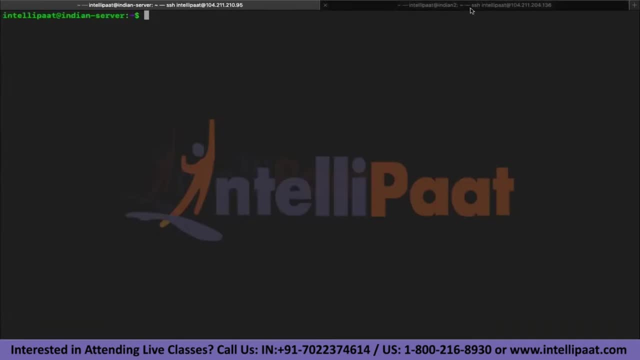 page in a little while and i'll show you how you can do that. so to replace this file, what you have to do is you have to go to slash var, slash www, slash html, and then replace indexhtml. so that is exactly what we are going to do now. so let's go to indian 2 server. let's go to the file location. 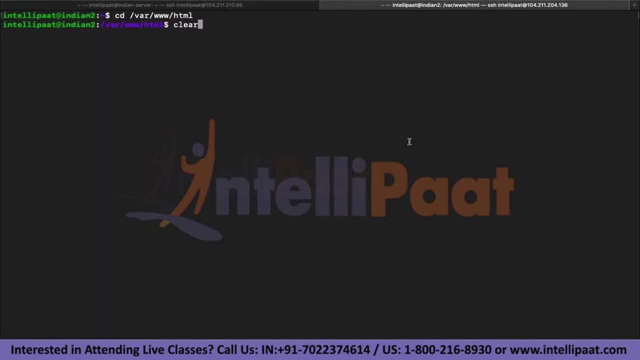 which was mentioned and in this file location. now let's delete the indexhtml which is present and let's add one more indexhtml. so to create or edit any file you have to make use of the command sudo nano. so nano is basically just like notepad that you have in windows, right? 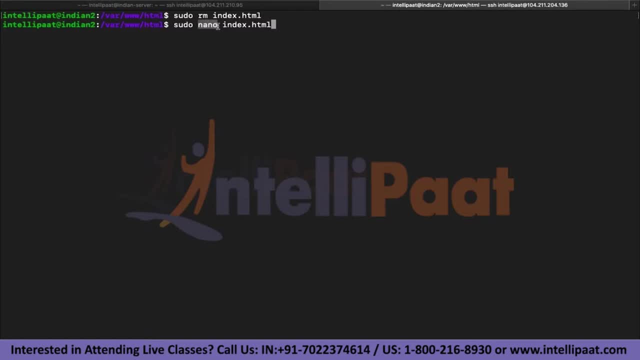 so notepad, open the notepad, uh, for you to write in or edit documents. similarly, in a book 2, there is a text editor called nano, right, so we're going to open that and, as you can see, it is now creating a file called indexhtml. so let's write a very simple html code over here. 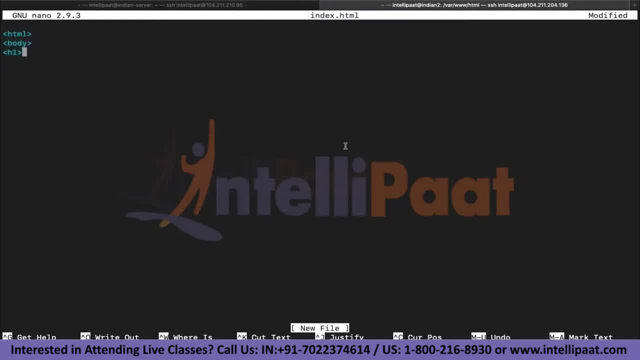 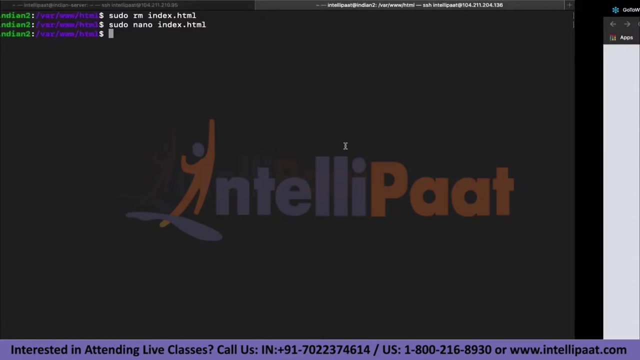 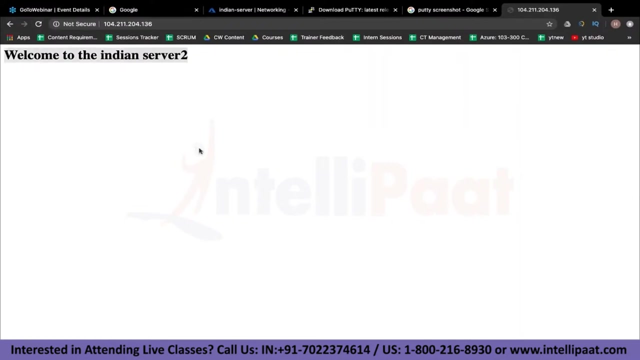 which is basically just going to have one line just saying welcome to the indian server 2. right, let's write this html done. and now, if i refresh this, you can see it says welcome to indian server 2, which is great. so now let's do the same thing for our first indian server as well. so right now, if i go to 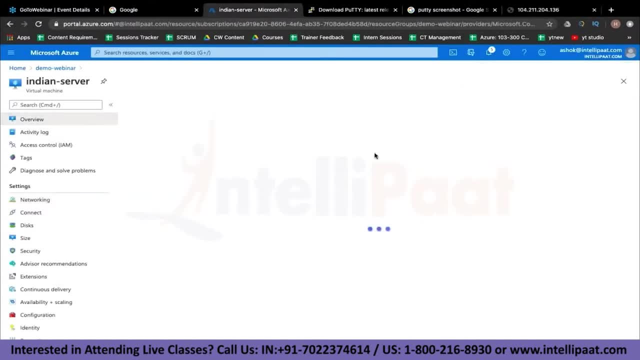 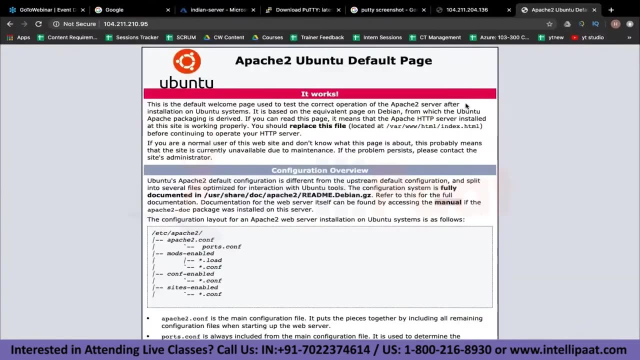 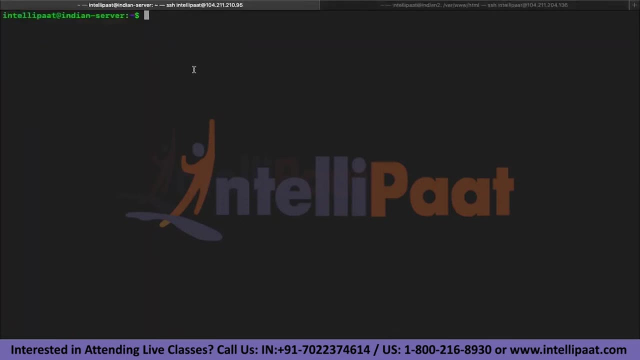 this ip address and i see that we still have the same ngl server we already created a new one for. in a new tab i've seen the default departure to page uh. let's replace that with this code. so what i'm doing is i'll first go to the file path. 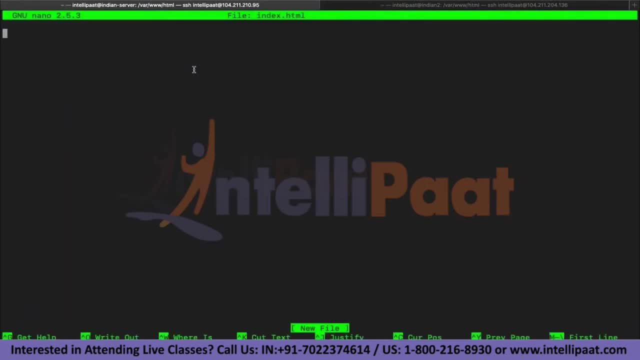 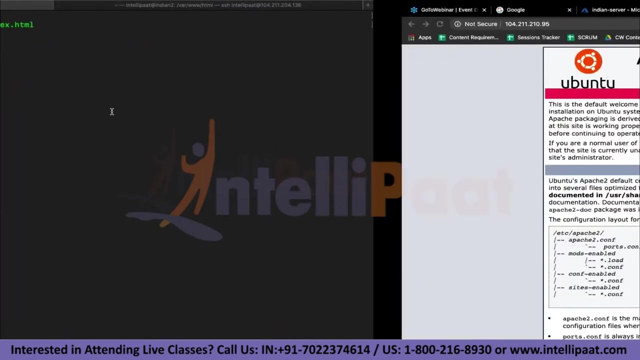 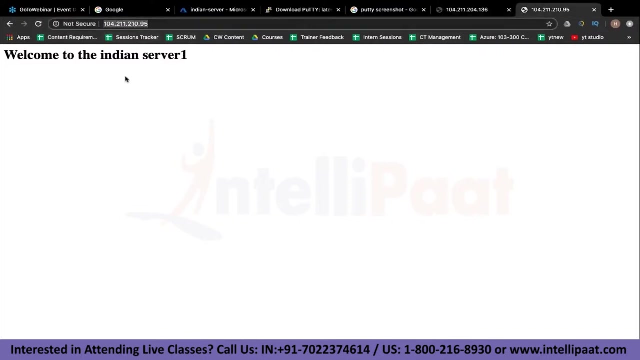 and now i am going to paste the code that we wrote over here into this file and change this to welcome to indian server one. okay, done. and now, if i refresh it, great. so now i have two ip addresses where, if i go from the browser to these ip addresses, i can going to see: 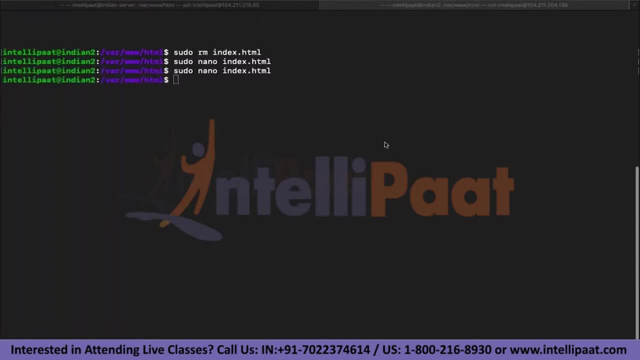 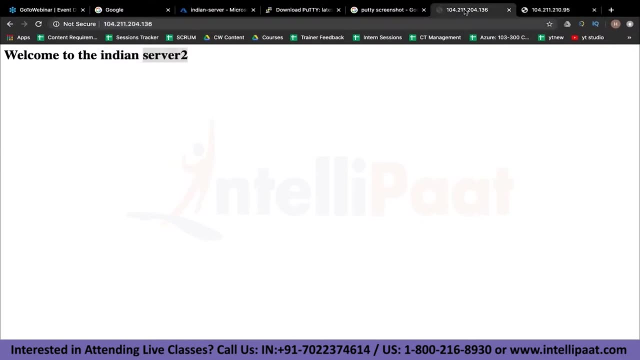 indian server one and indian server two, and now what we are going to do is we are going to put a load balancer on top of them. okay, so let's see how we can do that. so there are a lot of type of load balancers that, basically, you can deploy. uh, the load balancer that we are going to deploy, 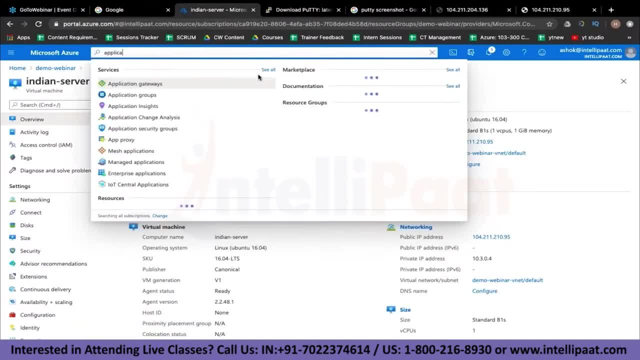 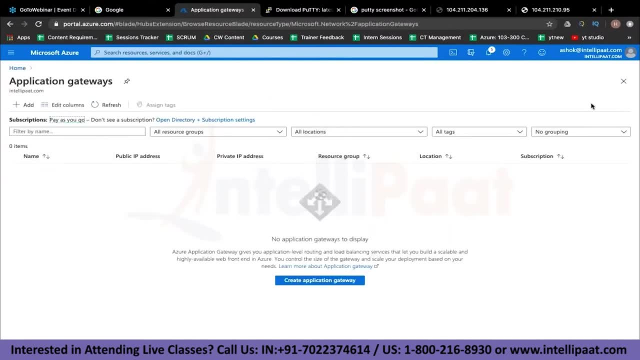 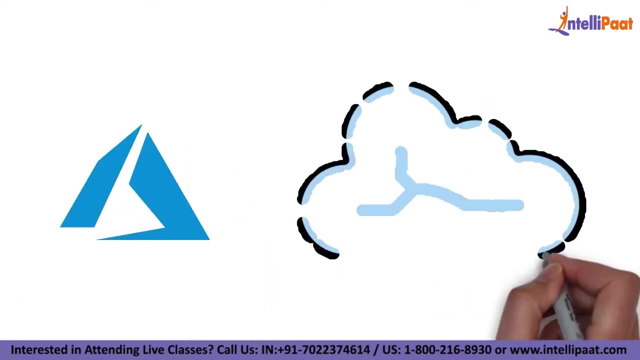 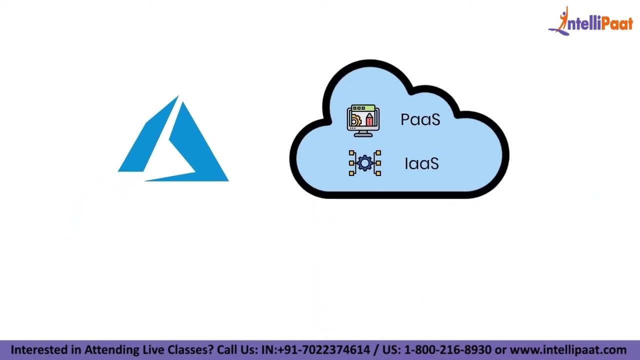 today is basically an application gateway. okay, so let's go to application gateway and in application gateway, all we have to do is: uh, so there are, yeah, so we'll just click on add. so what is microsoft azure? microsoft azure is a cloud provider that provides various platform as a service and infrastructure as a service products. azure has cloud solutions to 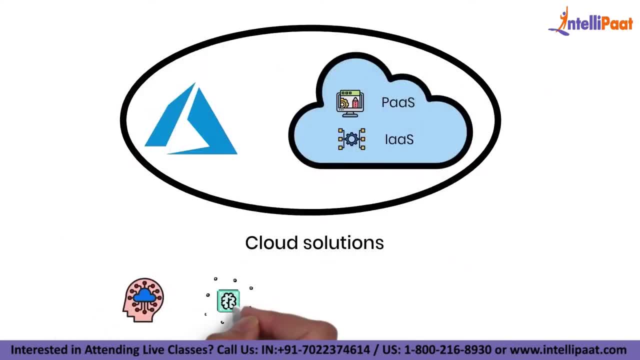 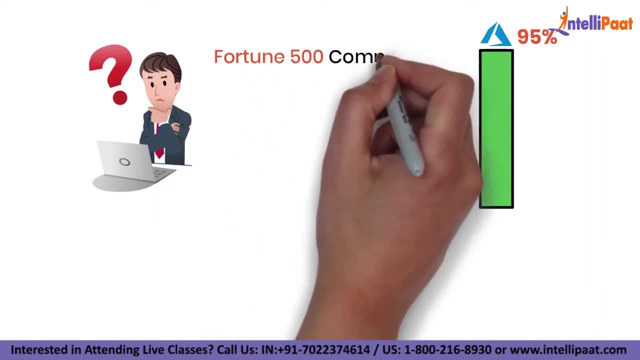 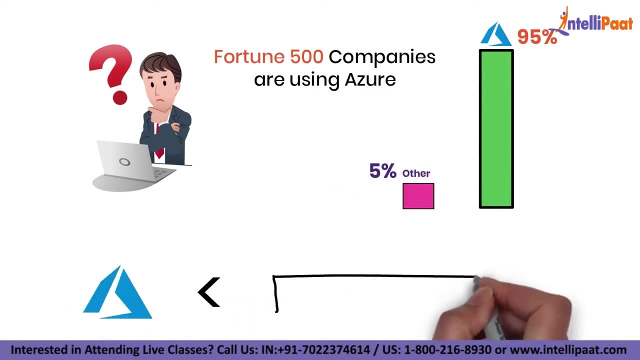 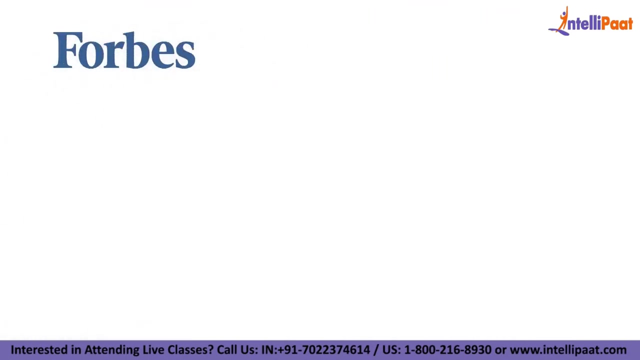 all the infrastructural problems by providing services in various domains. did you know that almost 95 percent of fortune 500 companies are using azure? also, it is five times cheaper than aws in terms of windows and sql server, because there are also microsoft products. forbes say that microsoft azure is set to boost the size of the it market. 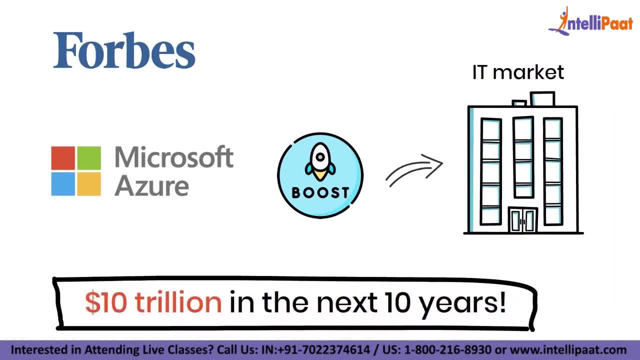 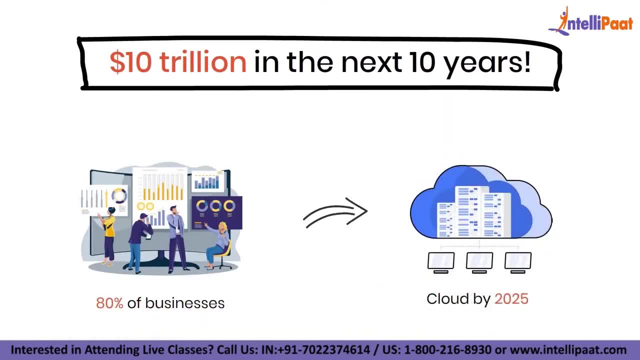 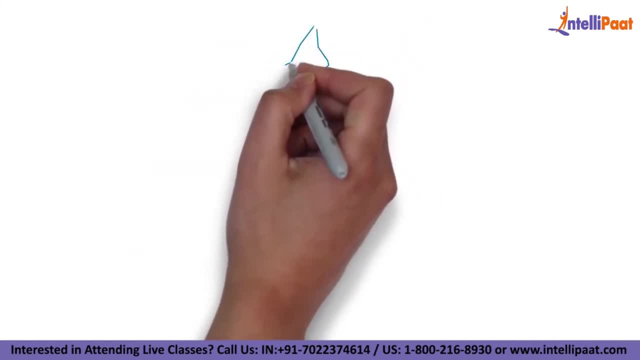 by 10 trillion dollars in the next 10 years, as, per predictions, 80 percent of the businesses will move their workload to cloud by 2025, thus making it a major career to consider transitioning to. for a better understanding of azure, let us start at the very beginning. microsoft azure was. 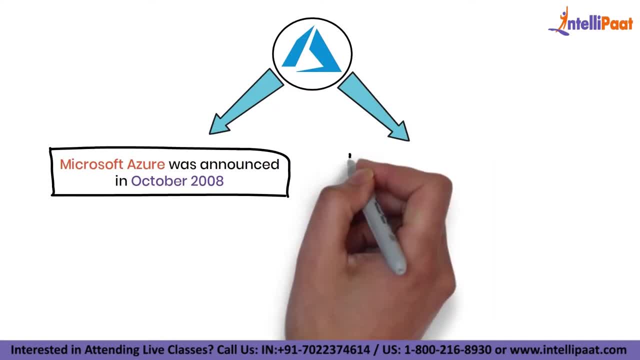 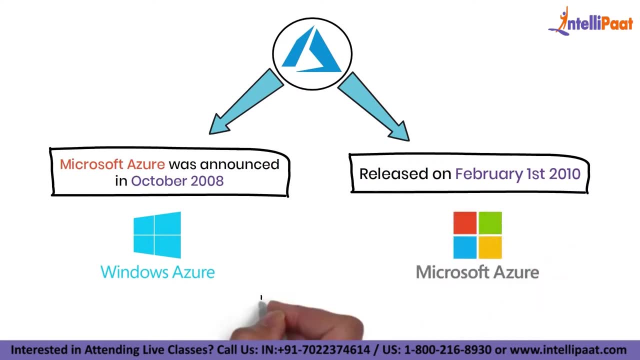 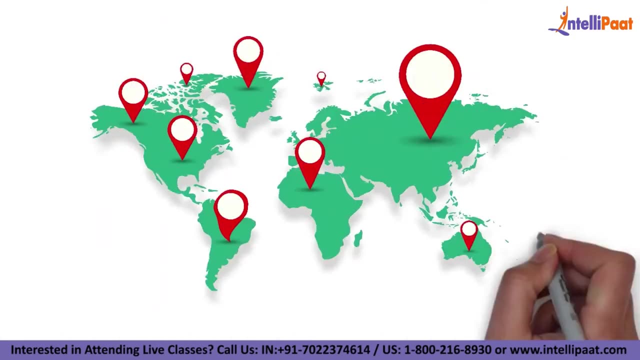 announced in october 2008 and released on february 1 2010 as windows azure first, and later named as microsoft azure on 25th march 2015.. in today's scenario, microsoft azure is going to be the first. its reach is in 140 countries and is still expanding, which is pretty. 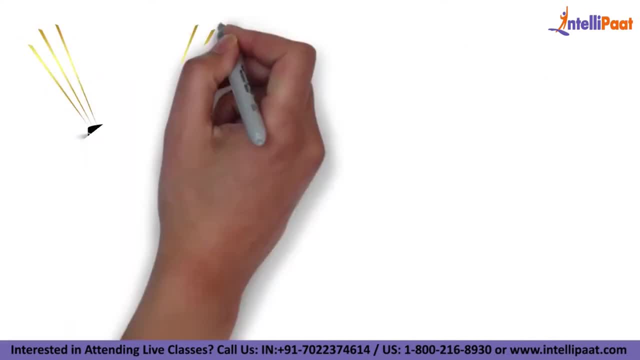 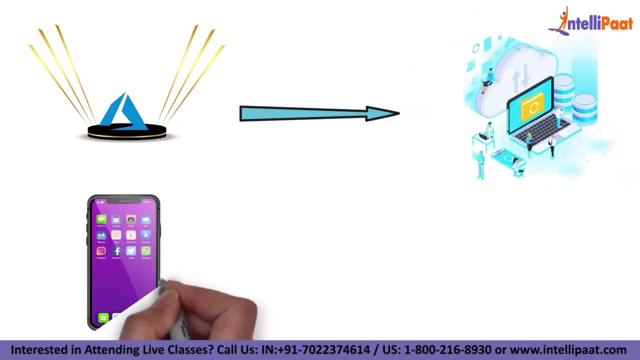 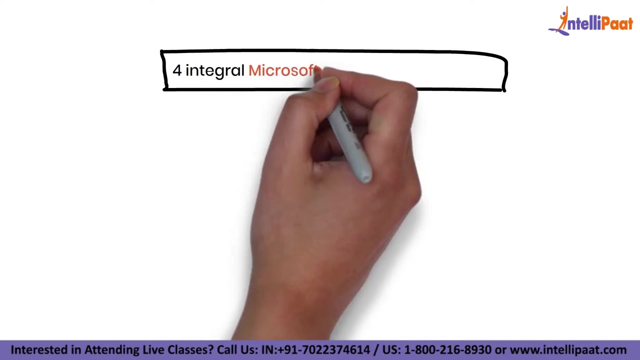 impeccable. in simpler terms, Microsoft Azure is a platform that enables users to engage in agile cloud computing and is designed for creating and managing apps through Microsoft's data center. now there are four integral Microsoft Azure service domains. the first one is as your compute. compute is the most. 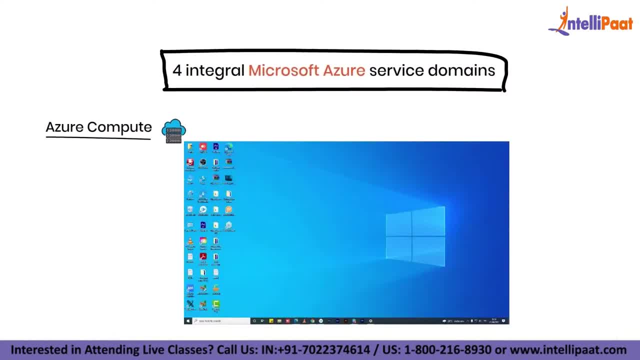 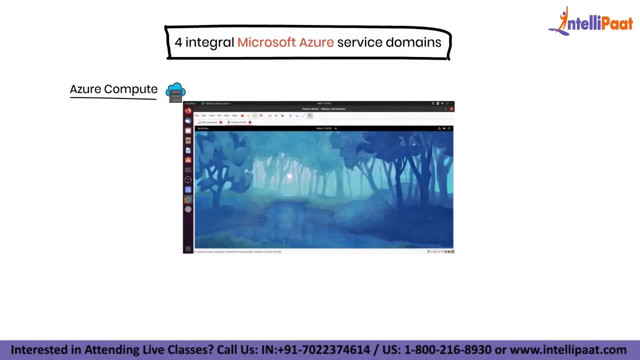 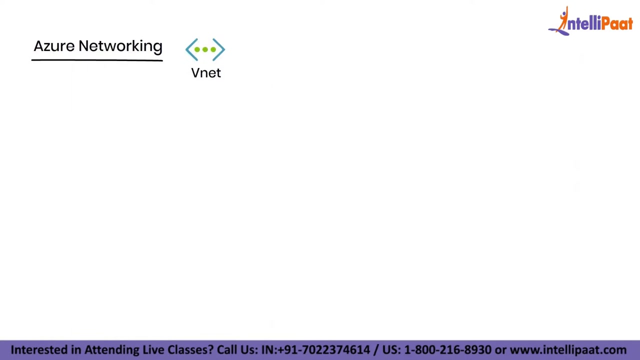 integral domain in Azure as it brings everything together with Azure virtual machines. you can get on-demand scalable compute resources as your virtual machines. app services and container instances are some popular compute services. second, we have Azure networking networks from the cloud networks in Azure, v-net is the networking tool that connects all Azure resources together. 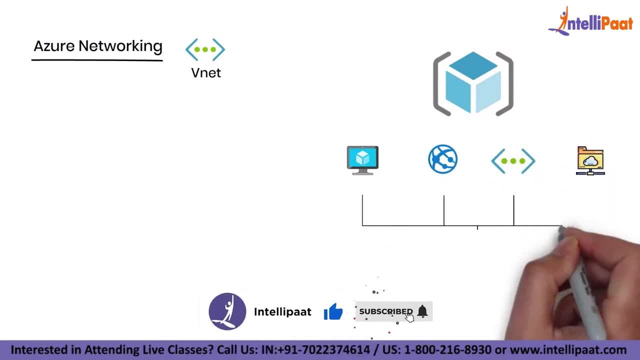 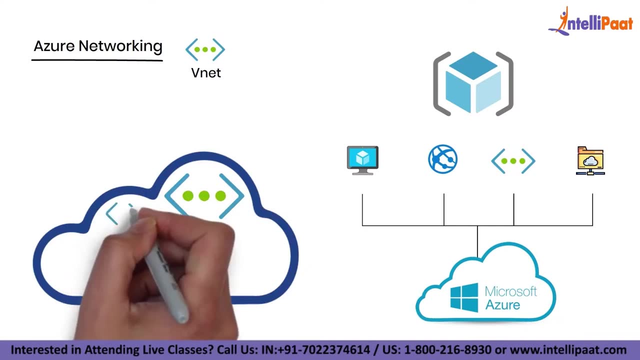 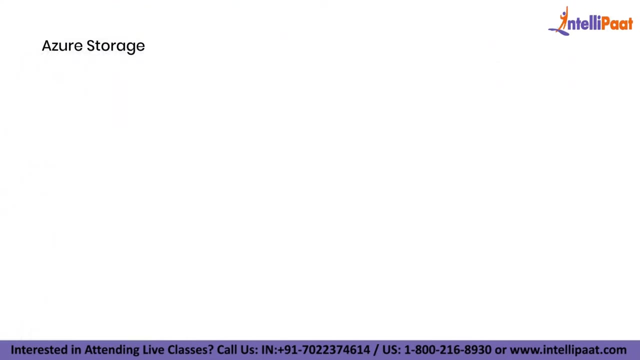 these networking services allow enterprises to safely connect their on-premises services to the Azure cloud. it is also used to manage virtual private networks and further create multiple virtual networks on the cloud. the third one is Azure storage, as your storage provides storage solutions that are more durable and large-scale applications. 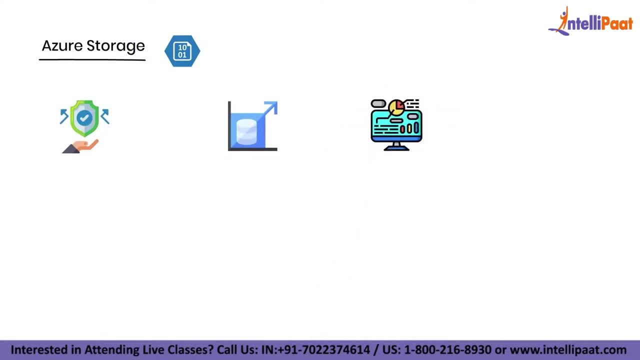 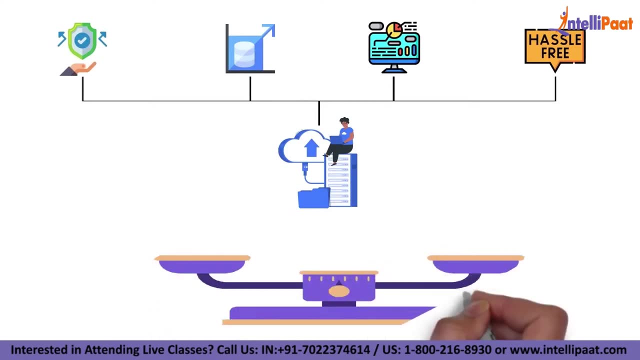 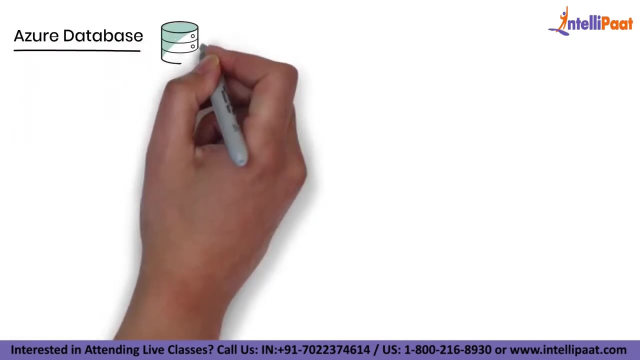 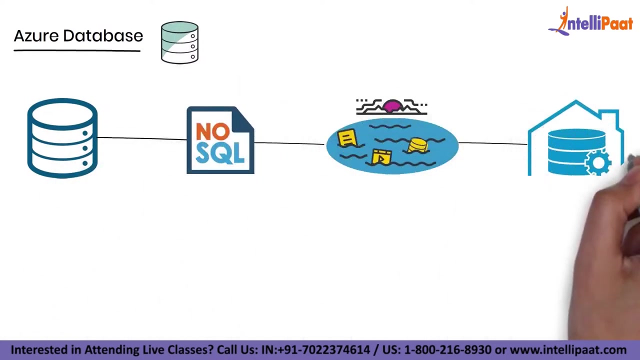 data-driven applications can be built without any hassle, as your automatically skills the storage requirements according to the usage and it automatically balances throughput according to the connections made. and the last one is Azure database, as your provides relational databases, no sequel databases, data lakes and data warehouses. it provides a scalable, high. 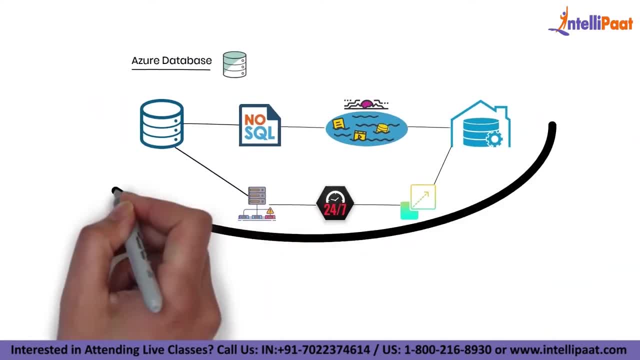 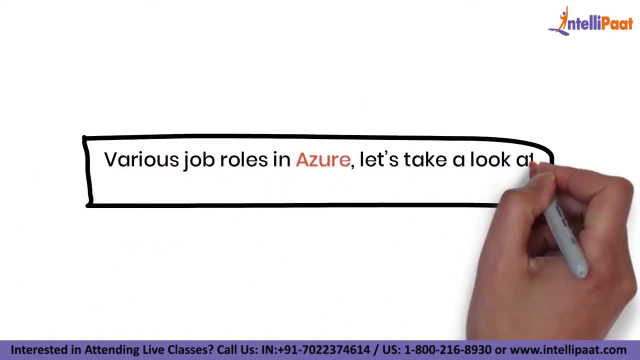 available and fault-tolerant database that can be easily managed through the data assets of your applications database server and lets you scale according to the incoming data. There are various job roles in Azure. Let's take a look at one of the most popular job roles: Azure Developer. 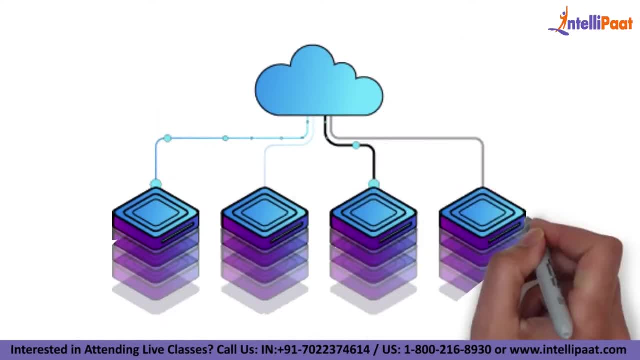 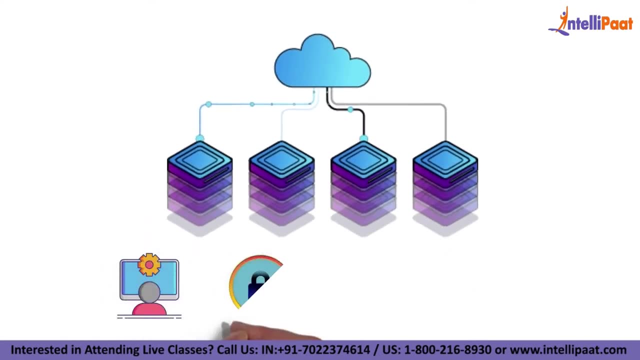 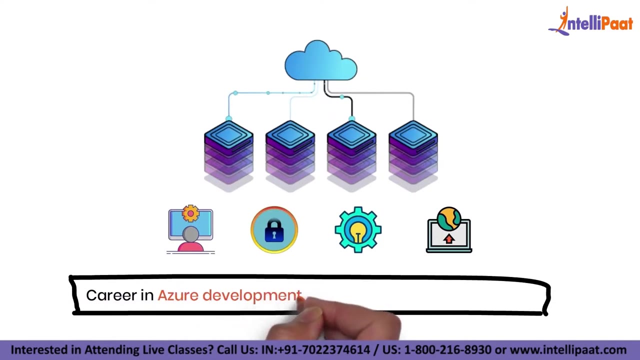 An Azure Developer is a cloud professional who creates cloud-based applications making use of the benefits of the cloud architecture. If you are proficient in testing, security, development and deployment, then a career in Azure Development is somewhere you will fit in well. 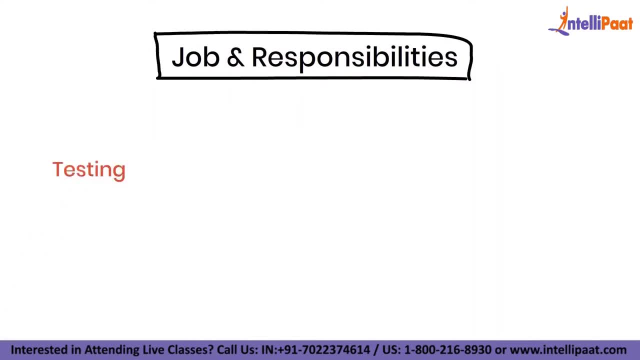 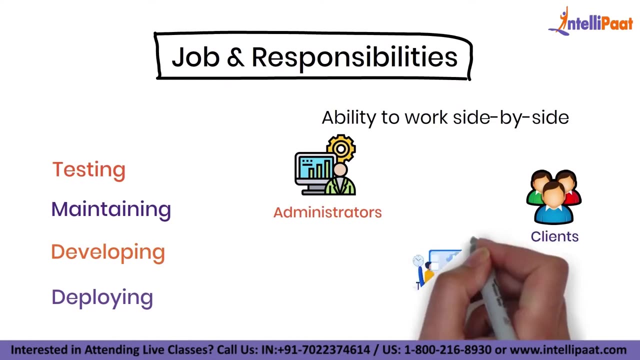 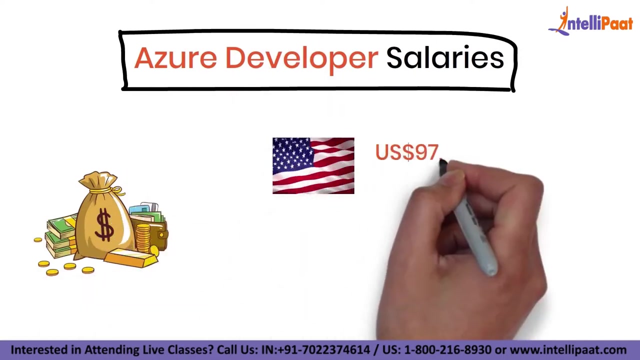 The job includes responsibilities like testing of applications, maintaining, developing and deploying them on Azure. It also includes participating in all phases of development and having the ability to work side-by-side with cloud administrators, clients and cloud architects. In United States, on an average basis, an Azure Developer gets paid $132,000 per month. 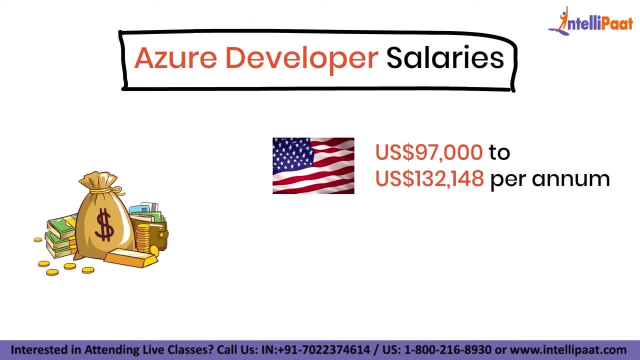 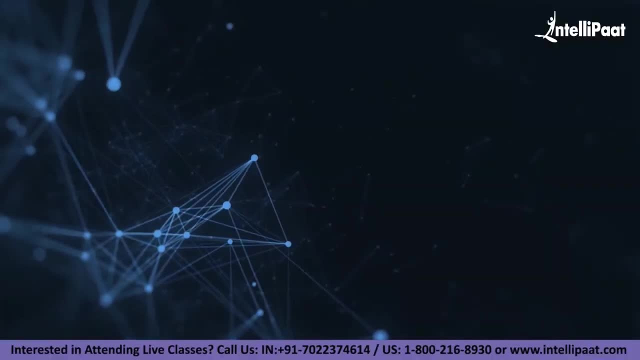 However, for an entry-level developer it's $97,000, whereas in India the salary offered ranges from 7 lakhs to 25 lakhs per annum. That's all about Azure. Just a quick info, guys. Intellipaat provides Microsoft Azure Certification training in. 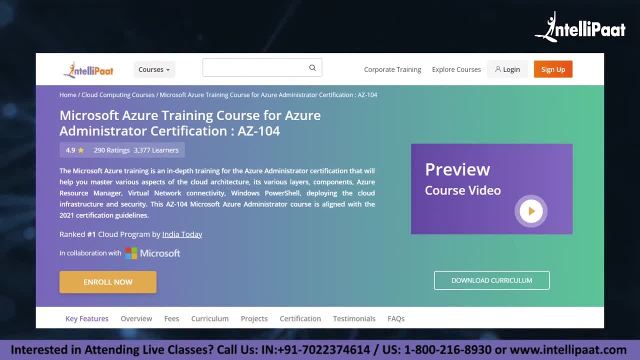 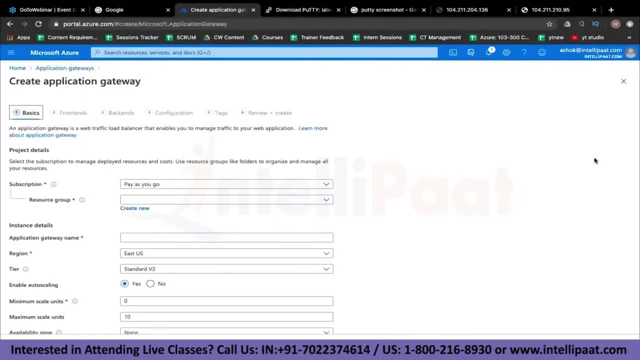 partnership with Microsoft, mentored by industry experts, The course link of which is given in the description. Thank you, Now let's continue with the session. And now it's going to ask us which resource group we want to deploy it in. 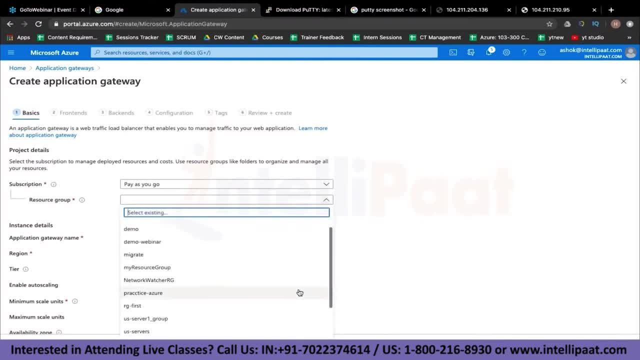 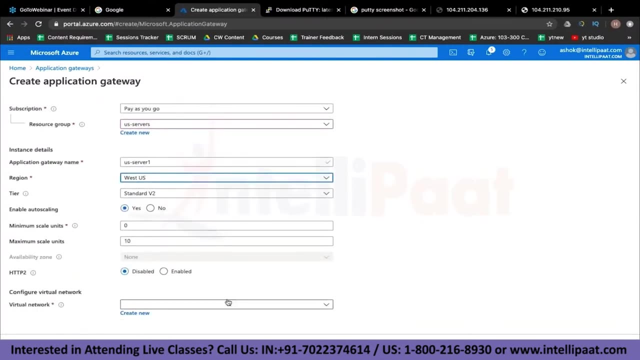 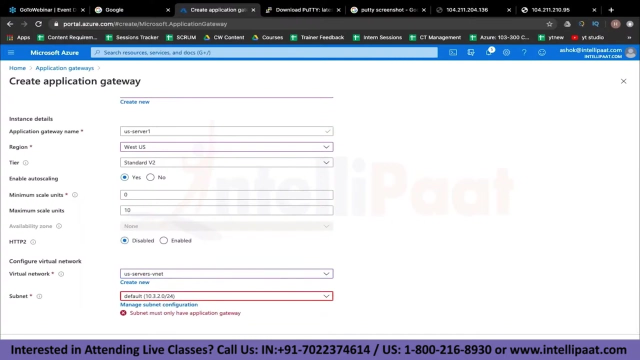 So we will, let's first apply, deploy it for the US region. So we are going to say, say US servers, application gateway, let's say US server one- The region is best US- And virtual network: This is the virtual network we want to deploy it in. 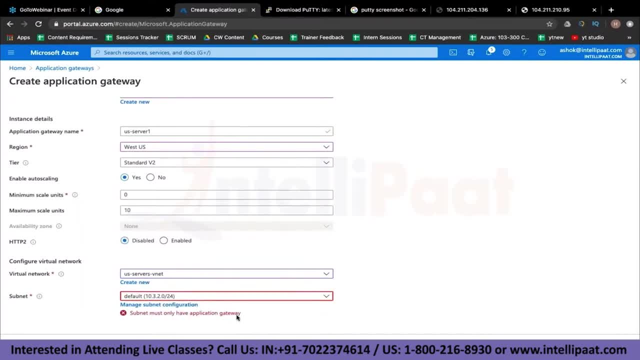 Now, this is the error that you will get. It says the subnet must only have application gateway. Now, in order to have this, what you'll have to do is you will have to create a subnet which is not going to have any other resource, right? 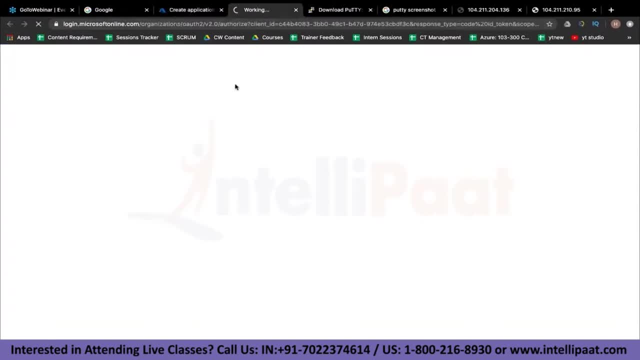 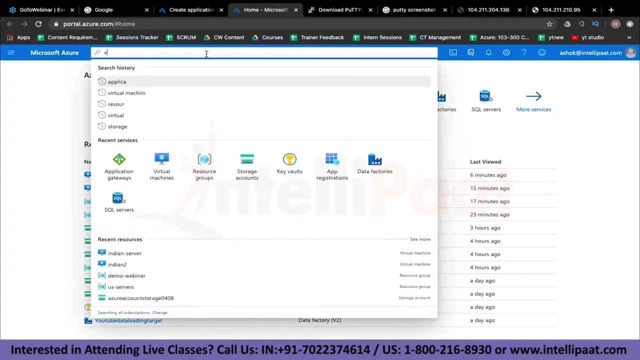 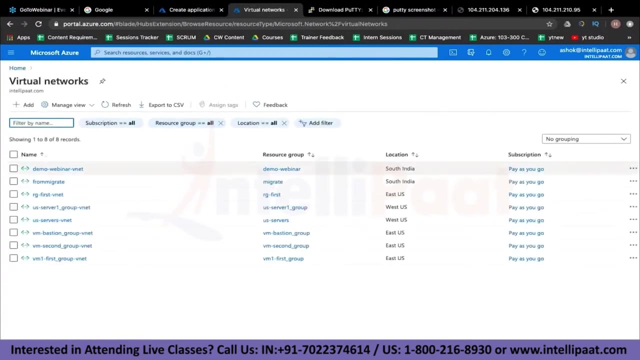 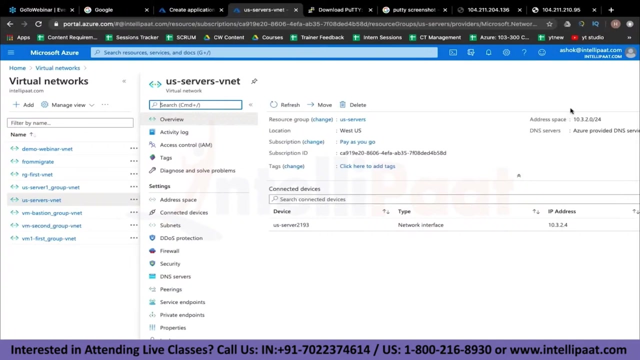 So how we can do that is just go to your Azure portal And then go to virtual networks. Okay, Now, the network that we want to configure is the US source, right, And in this, if you go to subnets, you can see there's only one subnet right now, which. 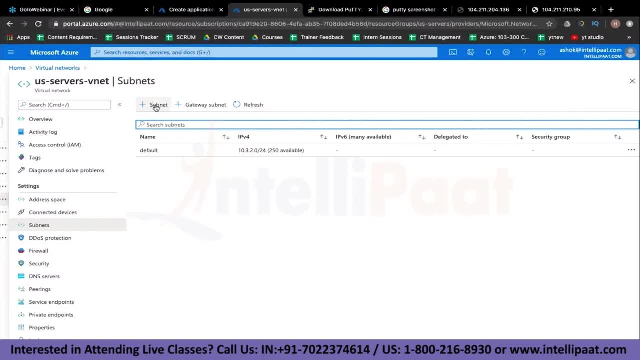 is the default subnet, So let's add one more subnet and let's the address name for this. Now the address range can be a little confusing to you, So let me make it as simple as possible for you guys. So right now you can see that address range over here is 10.3.2.0, slash 24.. 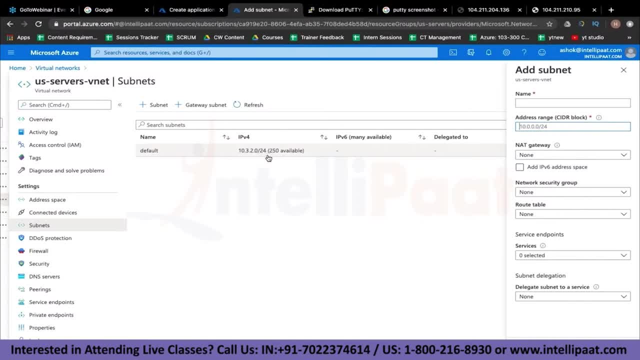 So slash 24 basically says how many IP addresses can be included. So if you type in slash 24, it gives it 250 IP addresses in the range of 10.3.2,. it could be dot one, dot two, dot three, dot 19,, dot 99.. 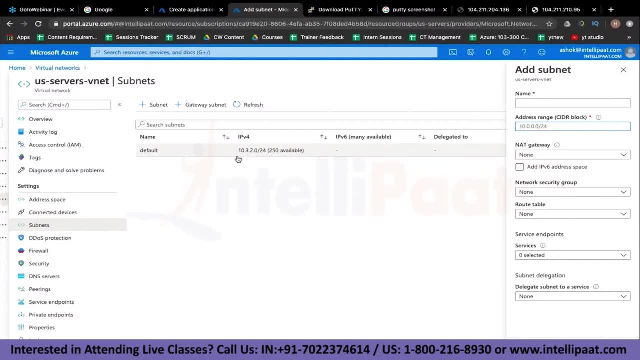 Right, Okay, So that's, that could be the range. So, similarly, we just replicate this and we'll specify 10.3 dot. uh, instead of two we can specify, let's say, five dot zero slash 24.. 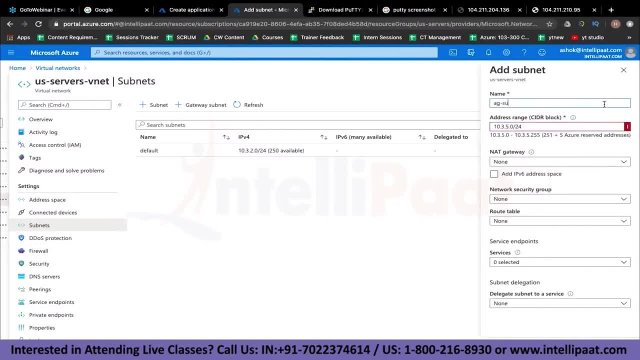 Right, And let's say this is for uh, AG, uh, subnet. Okay, So it says the subnet is not contained within these address space of the virtual network. Okay, Let's solve that as well. So we will first have to go to address space. 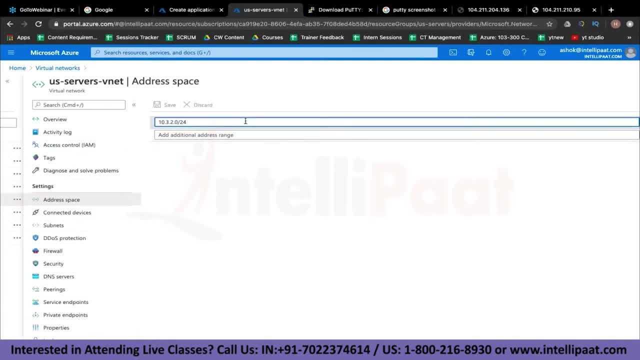 So we can. so here the address space is this: So instead of this range I can give a better range, which can be slash 16.. So the lower the number, the higher number of uh ranges you get. So as specified in slash 16 over here, 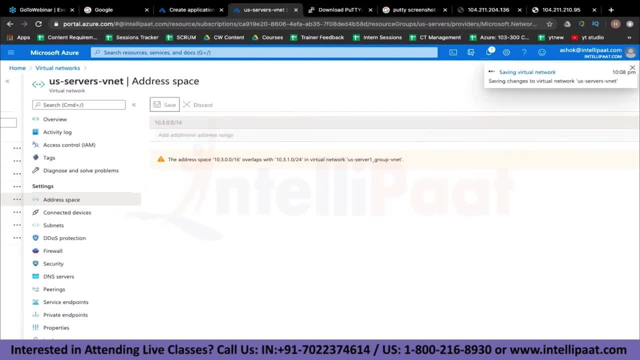 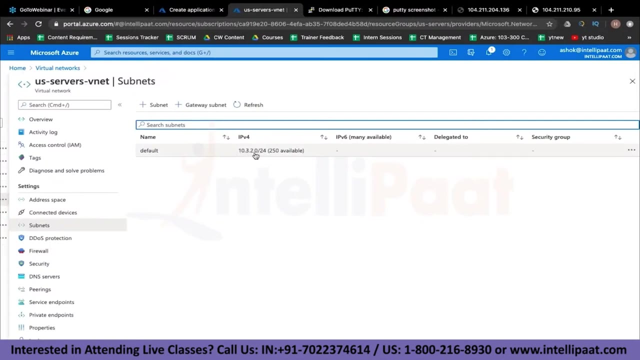 So what this basically tells us? Yeah, That the whole, uh, the whole virtual network can have IP address in these ranges, And obviously the subnets have to lie between these ranges, right? So my uh default subnet is obviously within the range of 10.3.. 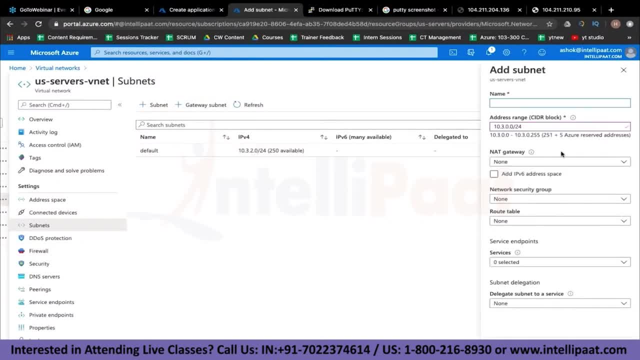 Now I'm going to specify a subnet range for my application gateway, which is going to be this: Okay, And let's call it AG hyphen subnet, Okay, Okay, All right, Let's click on. Okay, So this subnet is now being added. 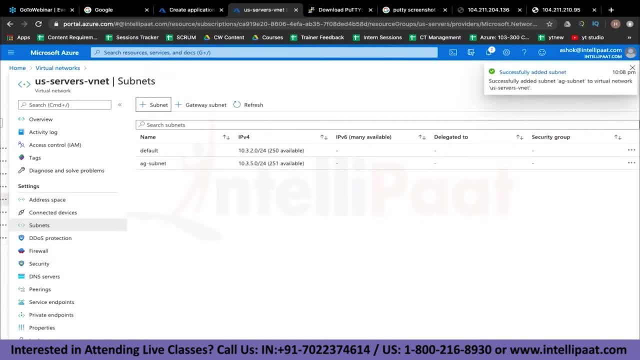 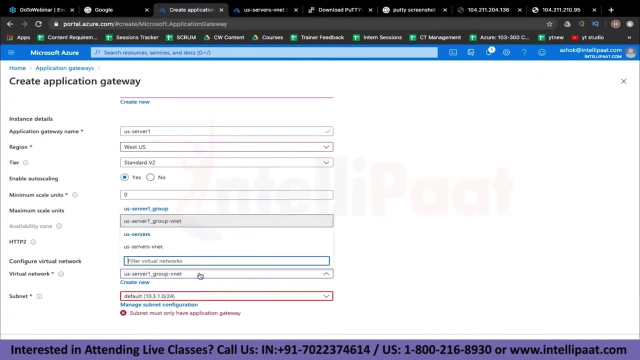 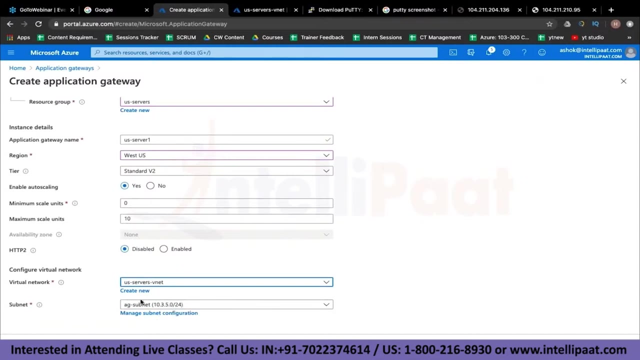 Okay, It's been added. And now, if you go back to us so as we net, you can see that AG subnet we can choose. now, Okay, And it's not giving any error now Okay. So now let's click on. next. 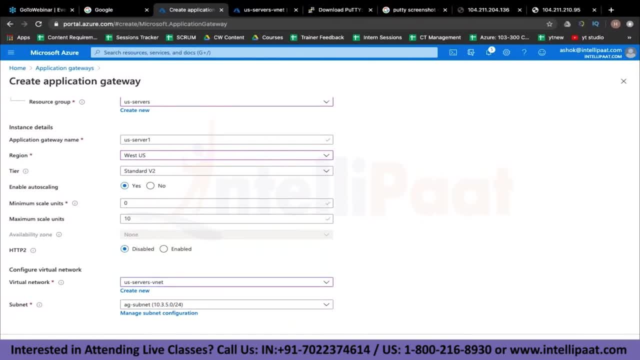 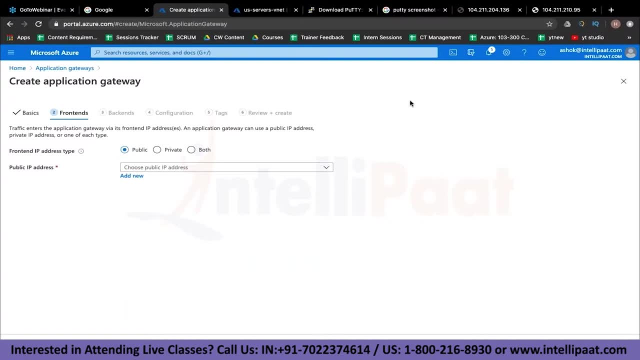 Okay, And now it is asking me what will be the front end of this load balancer? The front end is always a IP address, So there will be one IP address of the load balancer that we will be hitting And that IP address is basically going to route to the backend servers that we have. 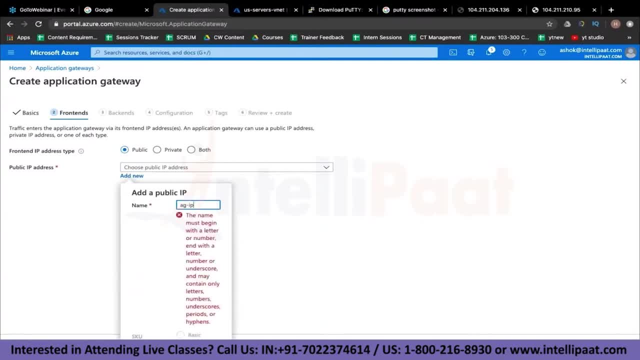 So let's add, uh, let's call this as AG hyphen, IP. Okay, Okay, Next, Uh, now it's asking me to add backends. Uh, so backends, uh, we can add, uh, we can click on: add a backend. 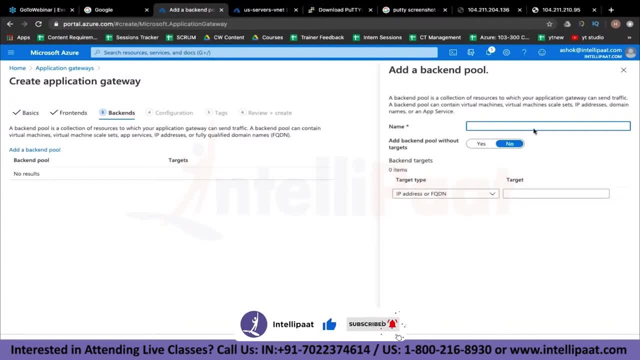 Let's name this backend pool as uh us hyphen And let's add the uh virtual machines in this. So the target type would be a virtual machine and it could be us server two. Let's add this first and again a virtual machine, and let's choose us. 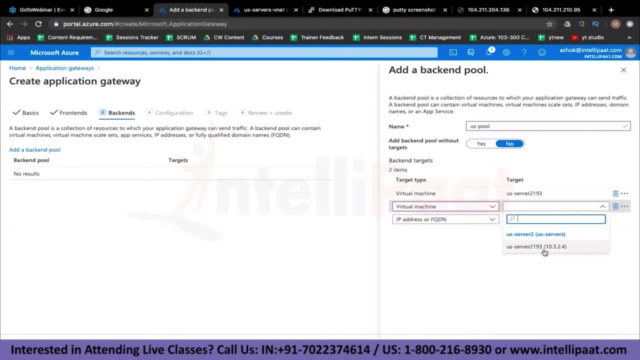 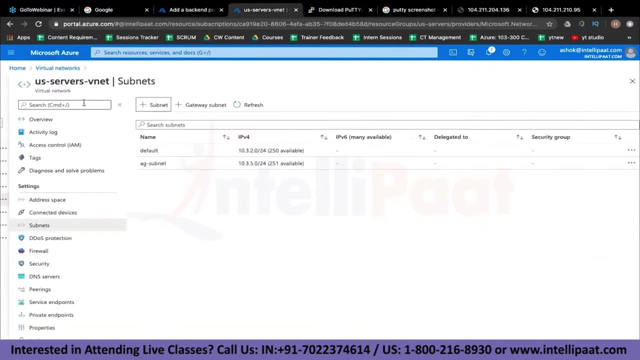 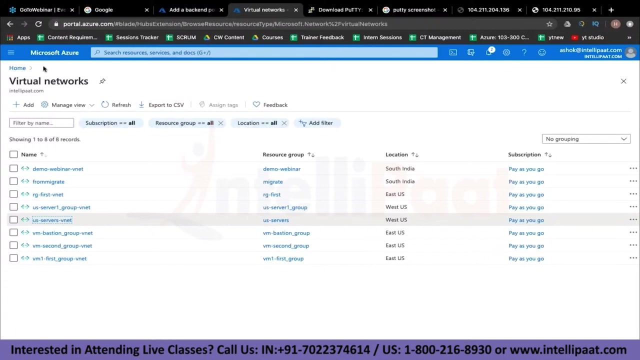 One is not being listed over here, So only those servers which are in the virtual networks of this application gateway can be added. So I think, Uh, Okay, So the server, one that we deployed, is not in the same, uh, virtual network. 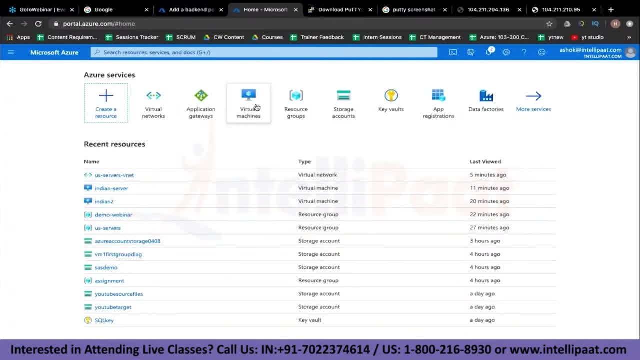 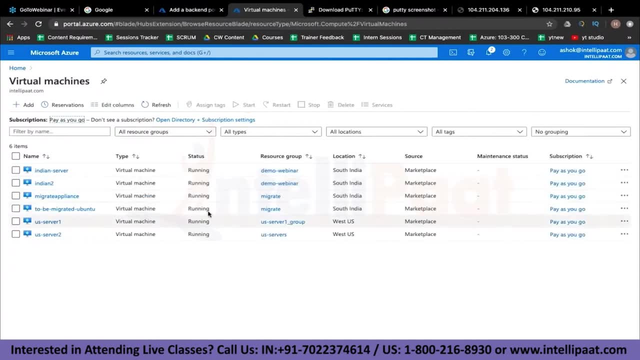 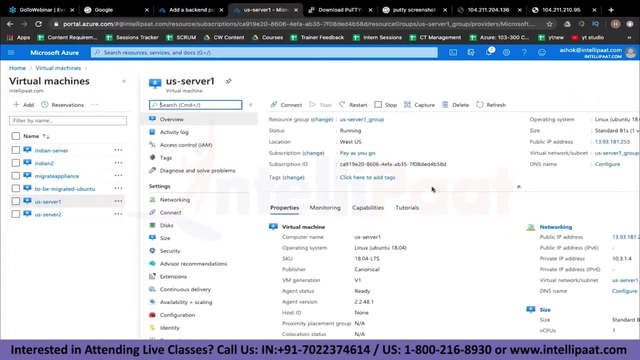 Let's verify that. So let's go to virtual machines and let's go to, okay. So I think this is a problem. So, uh, us server one is in a different network. Hmm, Okay, Let's try to fix that. 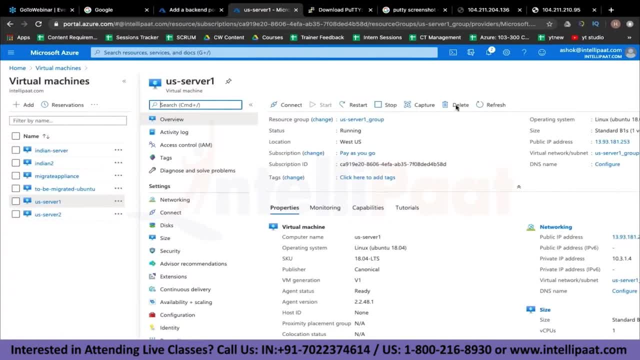 So it's a good thing. We did not configure us servers yet. So what we'll do is we'll just delete the server, that is us server one, and while it is being deleted, Uh, let's quickly add: Okay, So let's quickly add a new virtual machine. 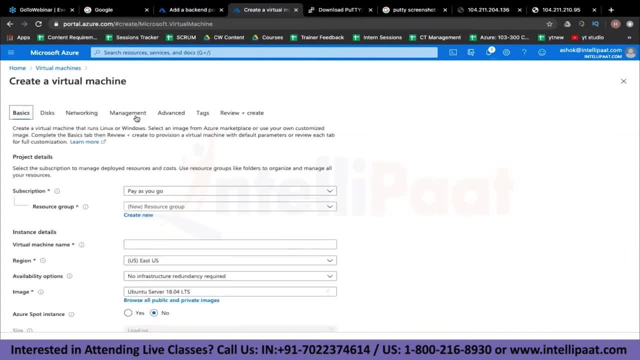 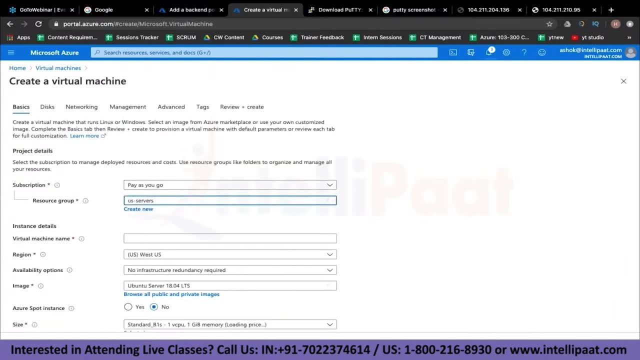 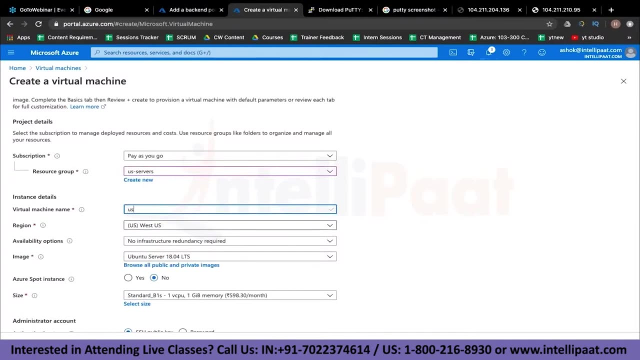 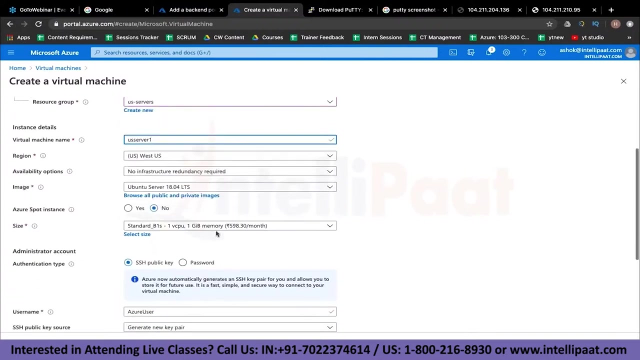 in the resource group of us servers. Uh, let's name this virtual machine as server one, us, or us server one. uh, it will be in the best us. The operating system will be Ubuntu server. This is the size of the virtual machine. 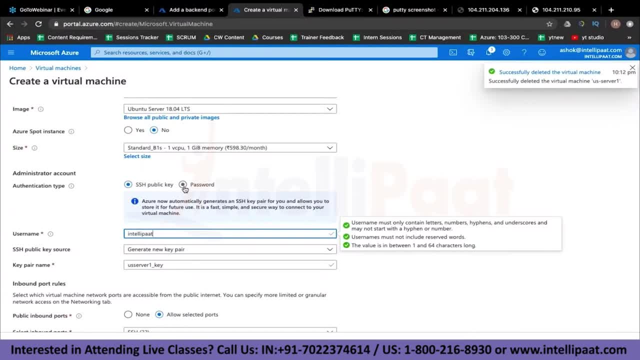 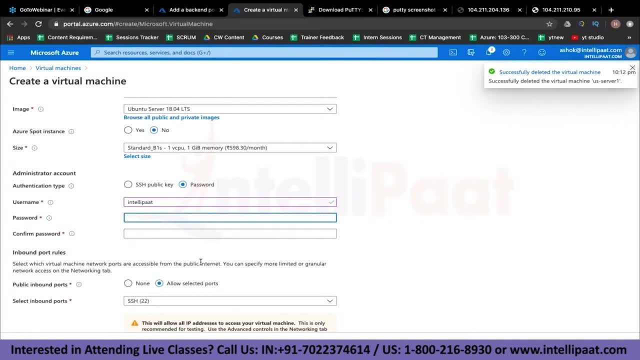 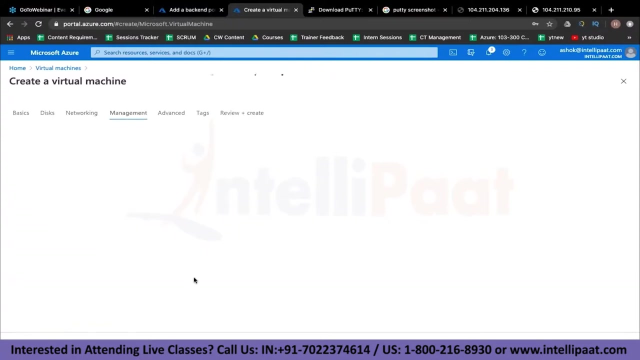 Username would be in telepart, The authentication type would be password And, as you can see, the deletion happened automatically in the background. And now let's specify the password. right? Let's go to management. Turn off the boot diagram. Okay. 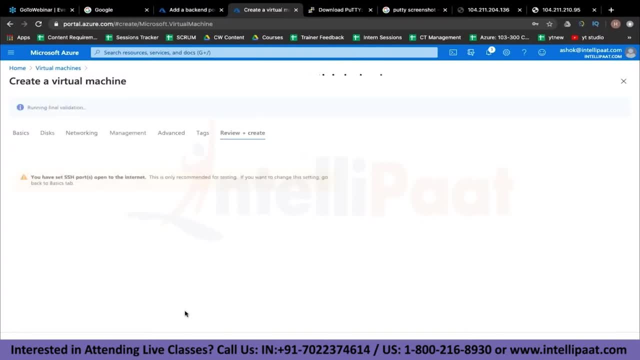 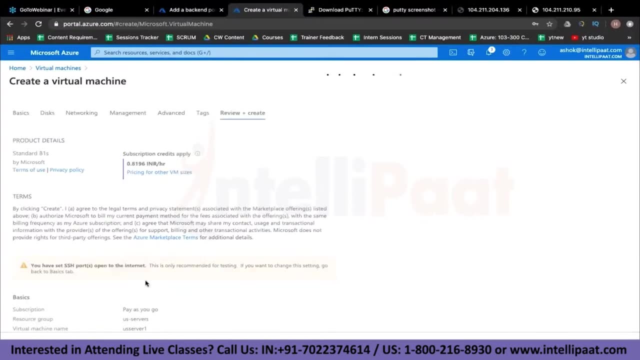 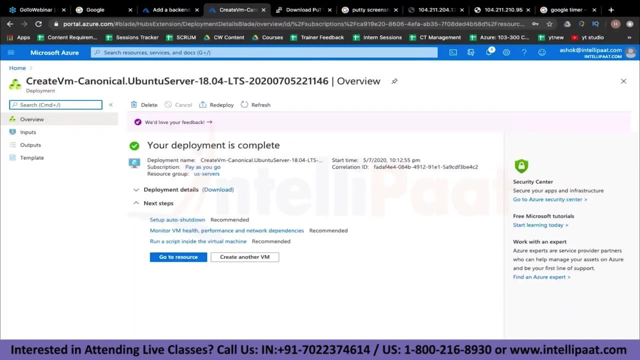 Let's go to diagnostics and click on review plus create. okay, So now my virtual machine is getting created. Now it'll take a minute or so to get the study guys. So so we have now deployed the uh us servers. uh, correctly. 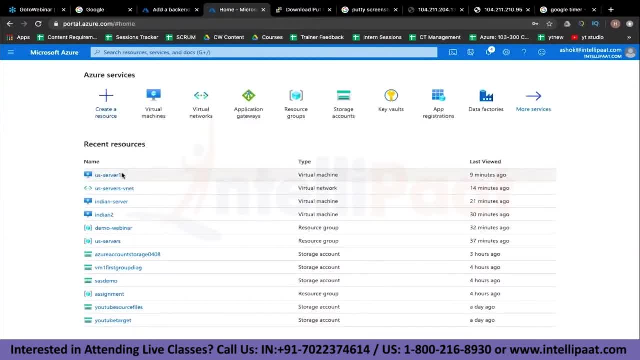 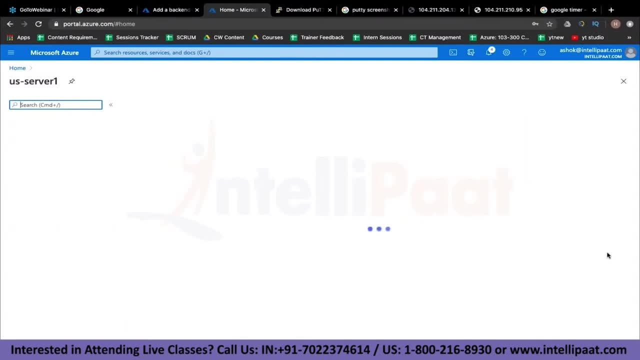 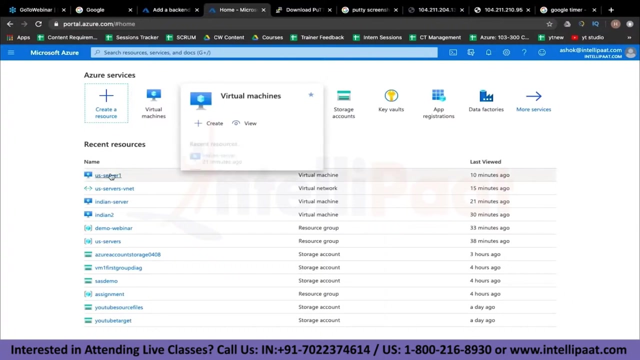 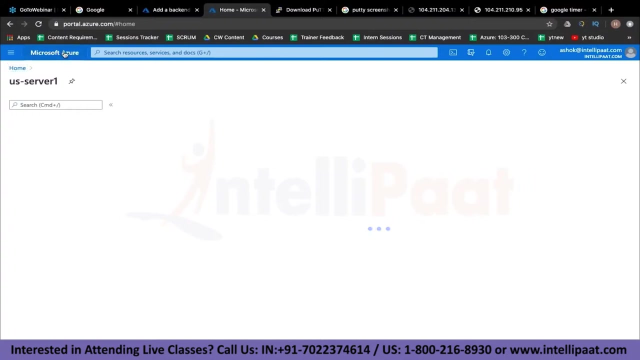 And what we can do now is let's connect to them and let's try to configure them right before. So let me just go ahead and connect to the application, Okay. So let's go to us server one. Okay, It's taking some time to load. 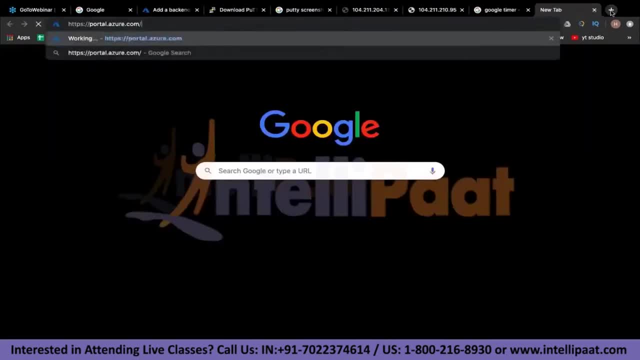 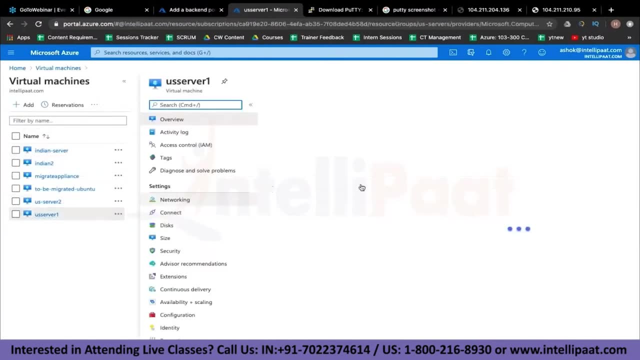 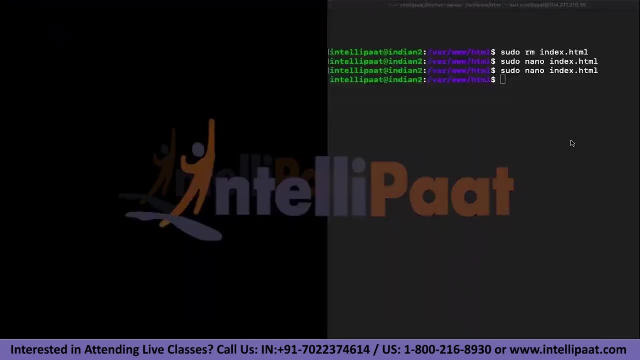 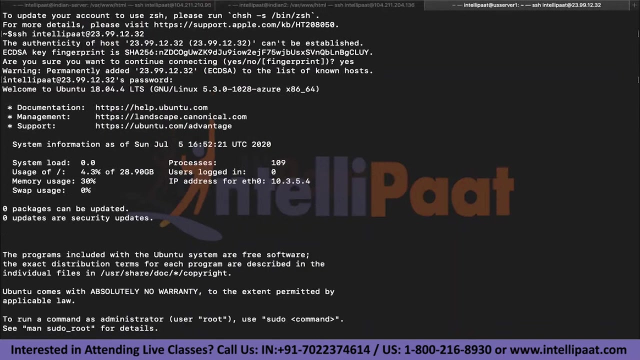 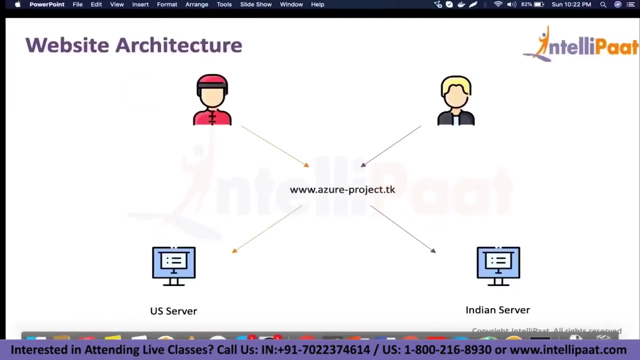 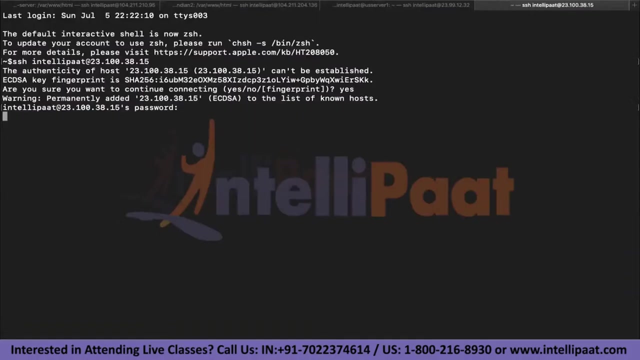 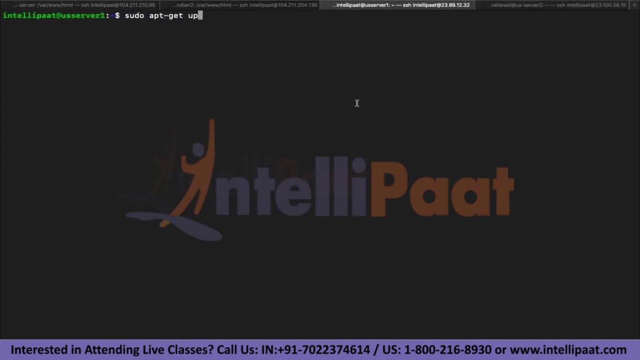 One second: okay, so this is a us server one. this is the ip address. let's try to connect to it. all right, so we are connected to us server one. let's try to connect to us server two. okay, this is the ip address. great, so we're connected to both the servers on the first server. let's update the machine. 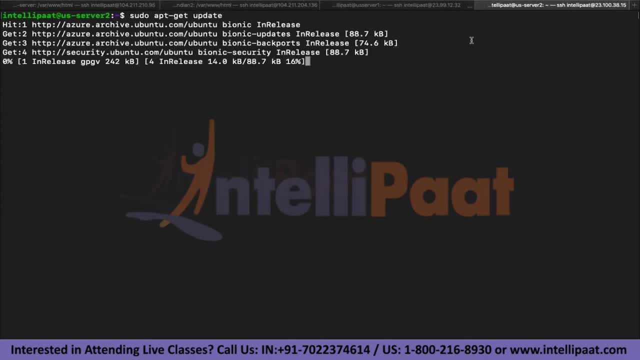 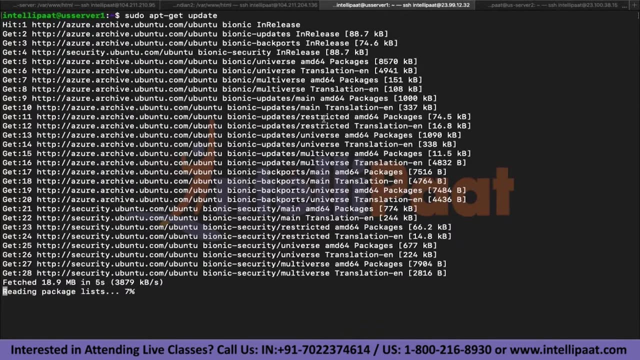 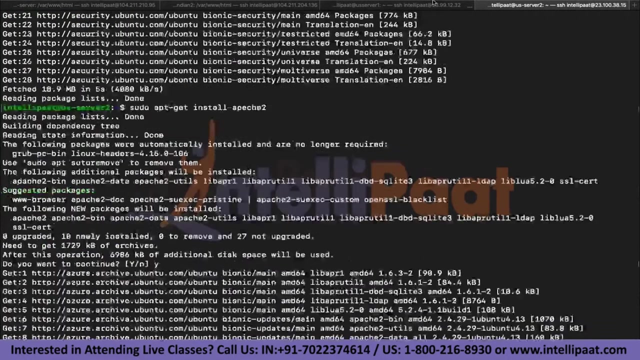 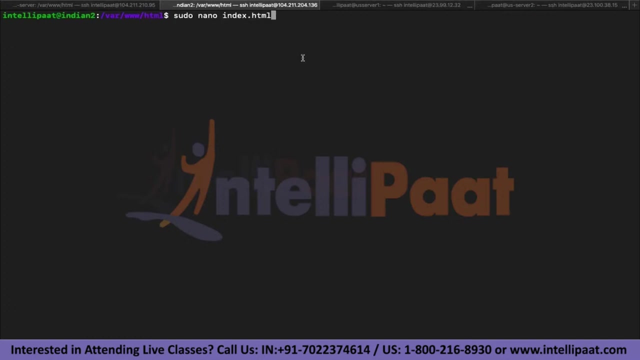 on the second server as well. let's update the machine. so same steps as we did earlier, and once they're updated, let's install the apache 2 software on this. okay, so it is being installed. similarly, over here as well, let's install the software. okay, so while this is being installed, let's copy the code that we have to put on this. 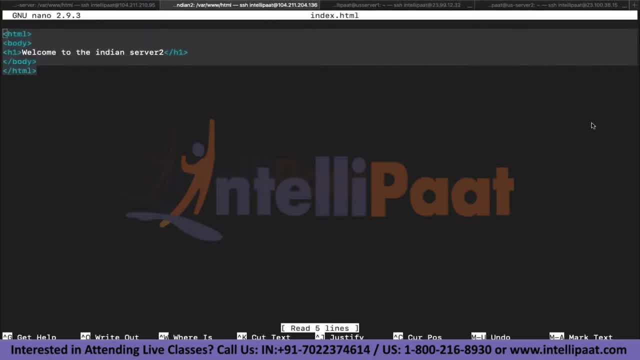 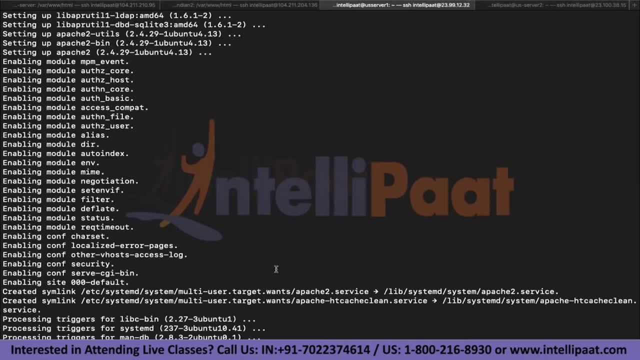 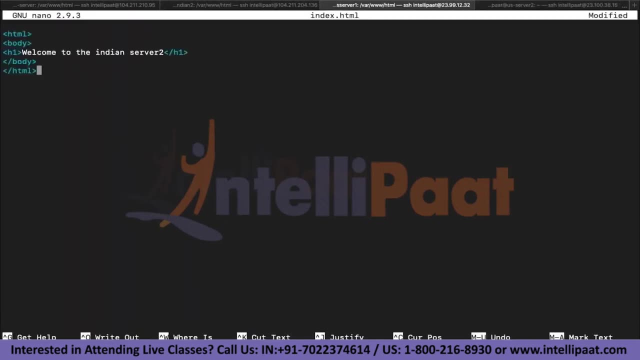 server as well. now it's taking some time to load. let's give it that time. so let's put the website for the us server now. so this is us server one, so let's put that in for there, amen. similarly, let's edit this as us server 2. 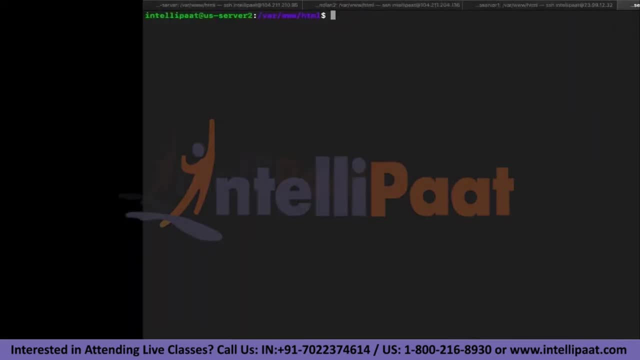 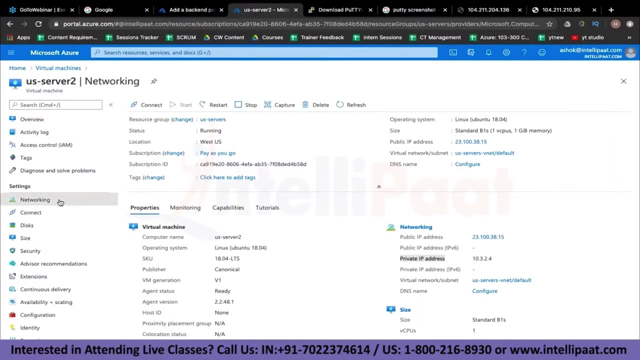 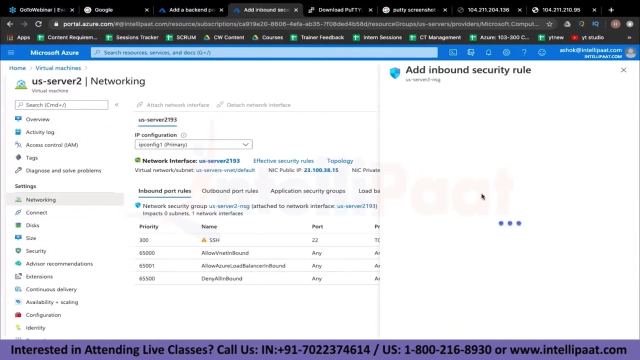 great. now let's open these ports and the servers. so this is server 2. lets go to networking. let's add the directly active login shallow, open SOLAL, the port 80 rule, and while this rule is being created, let's do the same for us. 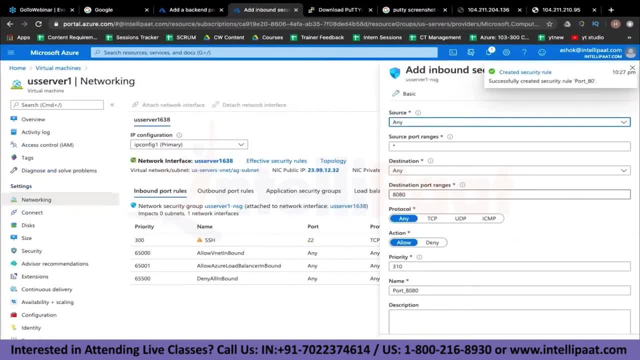 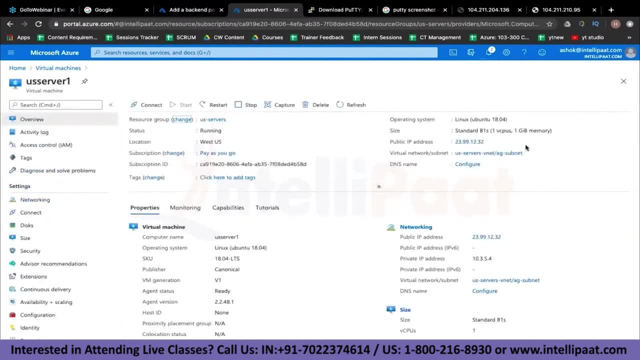 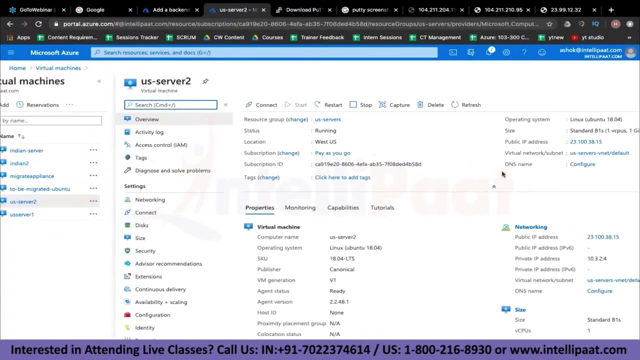 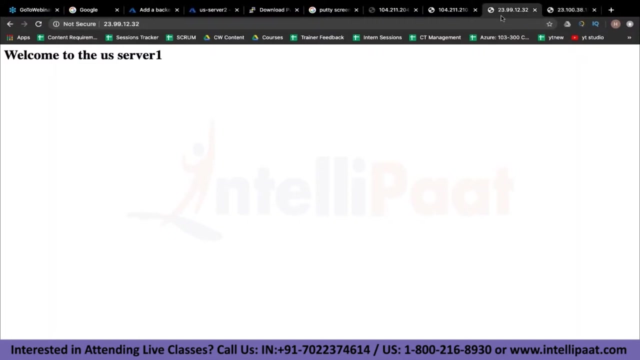 server one as well. and now what we can do is we can just put in these IP addresses in our browser to verify whether these are working or not. so us, our one, is working. similarly, let's check us over to as well, and that is working as well. so let me give you these IP address of the can in. 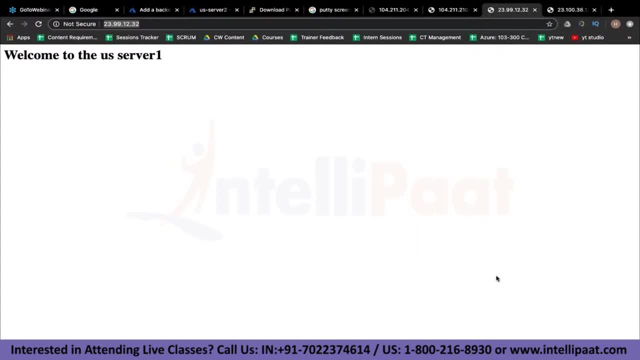 the chat so you guys can verify these are working or not- and if they are, I think you. we are good to go with at least the VM architecture and we can now start deploying the load balancers. now, based on the operating system that you choose, automatically the price of that server is adjusted. so let's say: 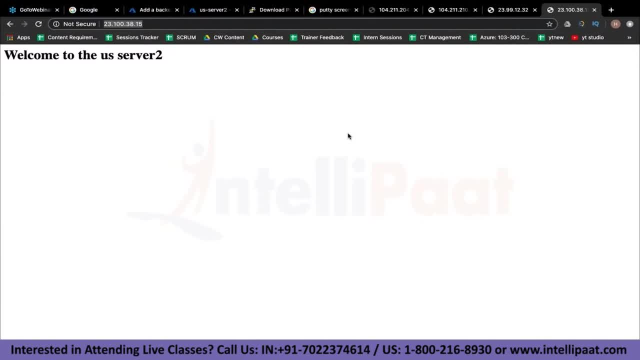 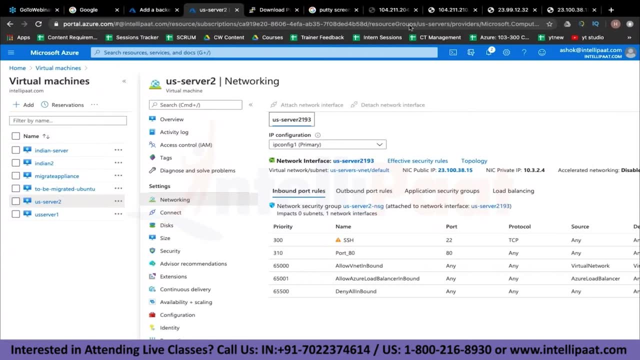 you're choosing a licensed product. that license cost is included in the rent of the server that you're going to pay. all right, so that's how it's managed. if the IP addresses are now working, let's now start configuring the application gateway. so we are in the us server application. 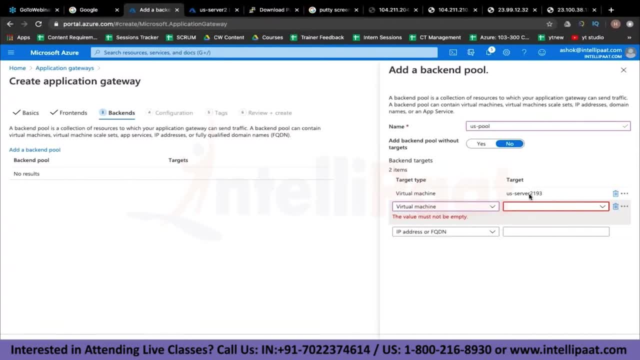 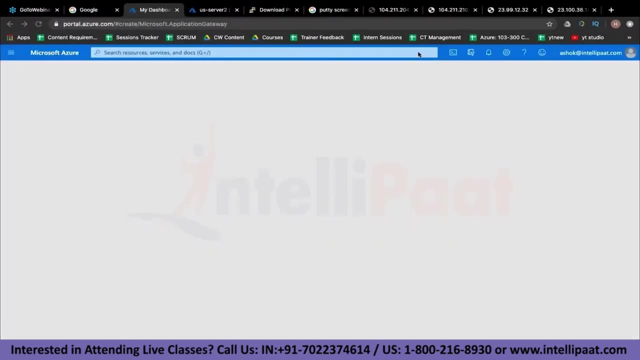 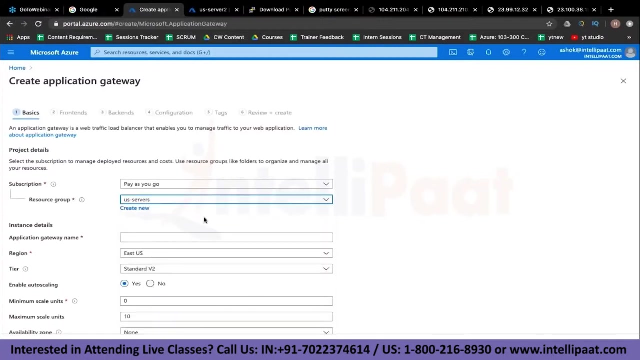 gateway. so we left off over here. so we have chose, chosen us server 2. let's choose again virtual machine and I think we will have to refresh this, so let's reload, okay, so resource group was us service. application gateway name is AG hyphen us. application gateway name is AG hyphen us. 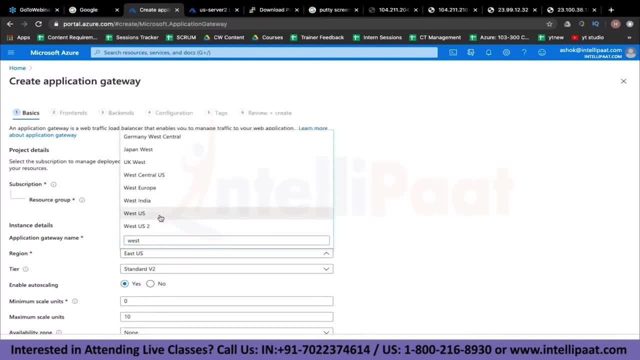 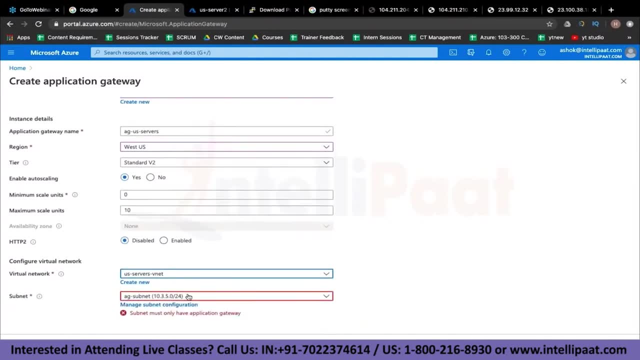 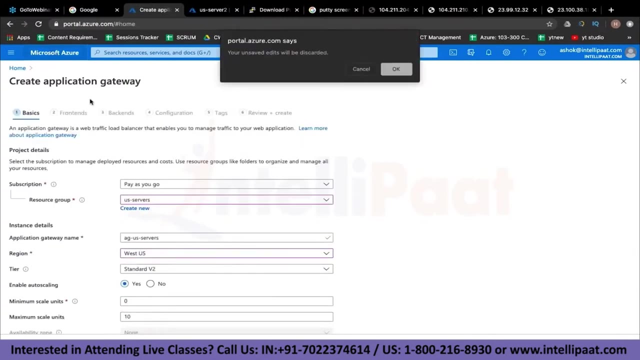 source region is west us. uh. tier is okay. uh, virtual network is us. so has been it and okay, so, okay. so in the previous one i think it was creating an application gateway, but it got left off the green. so i think let's try to configure that application gateway itself. 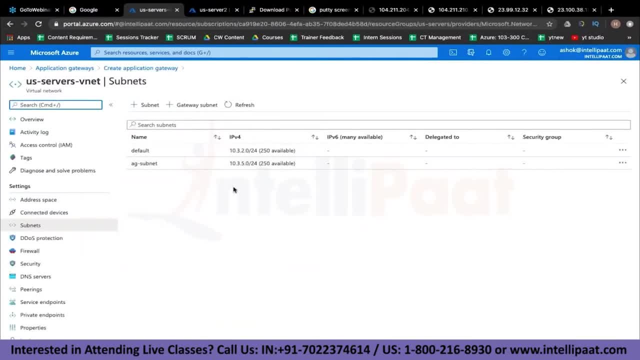 um, okay, so i think, uh, because we left off the previous application gateway, it has hindered, uh, you know, a problem in ag subnet or what i think is the us server, one that we deployed. i think we have deployed it in ag subnet. let me just double check that. 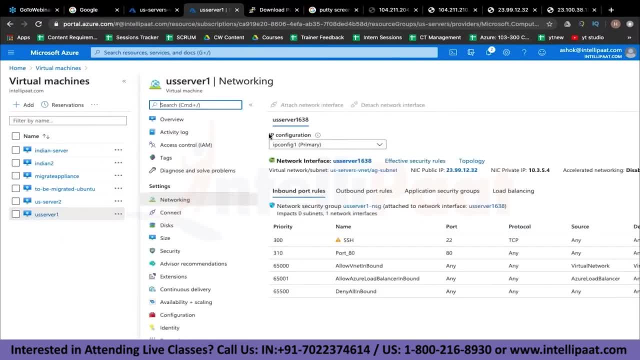 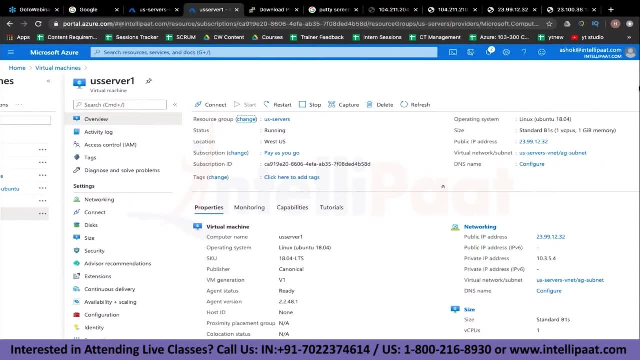 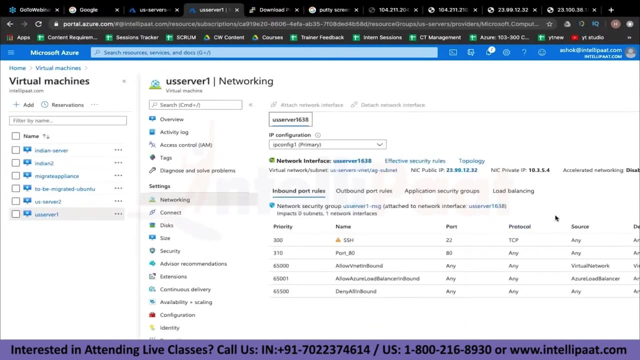 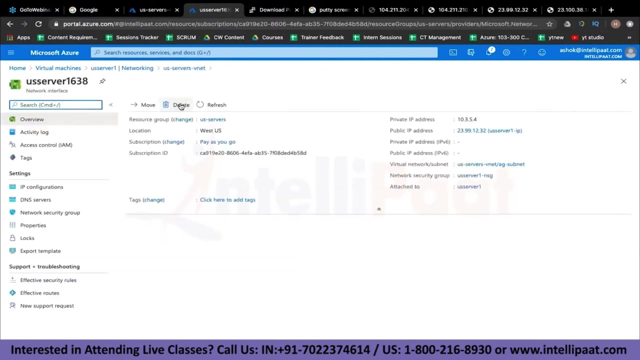 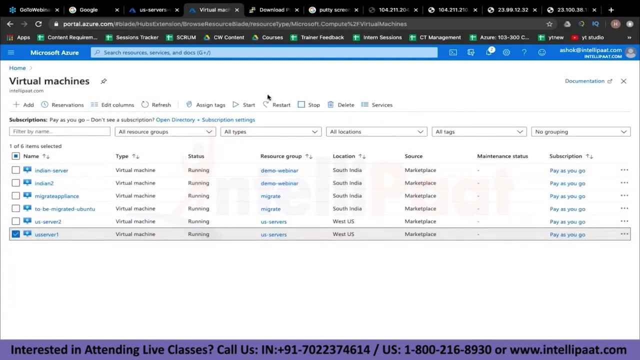 okay, so this is server one. and if you go to the overview: yes, so this is the problem. okay, so let's see if we can change that. um, so we can go to networking. uh, okay, so let's do this. guys, let's delete this again, because if we edit it, i think 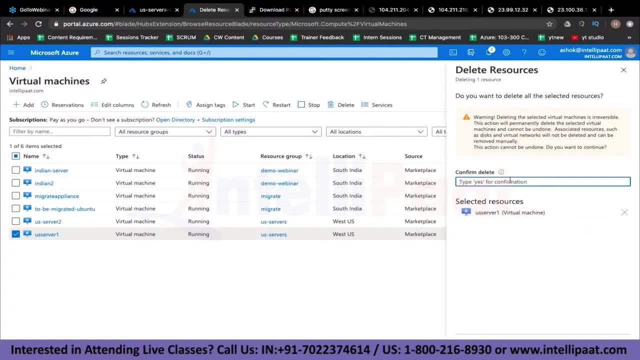 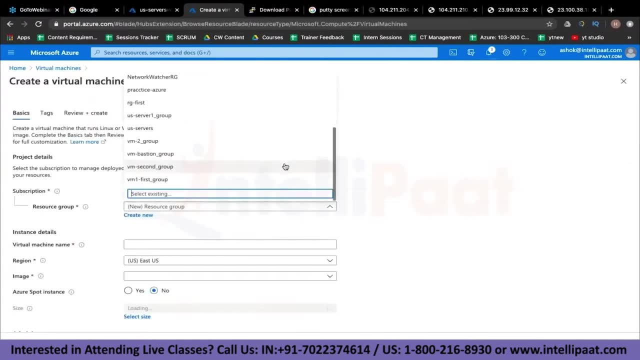 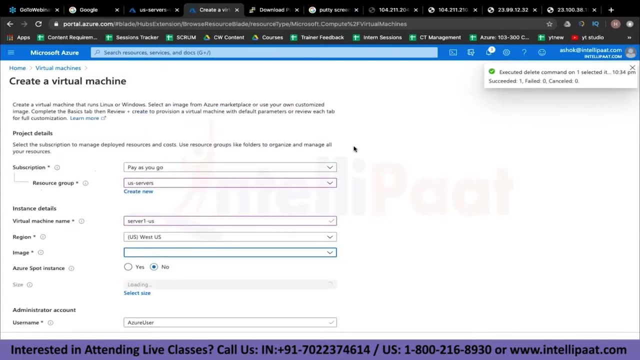 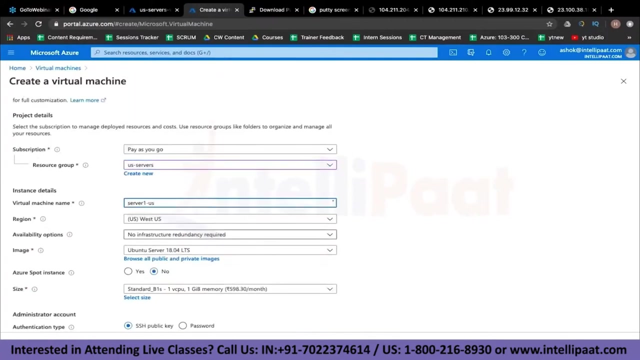 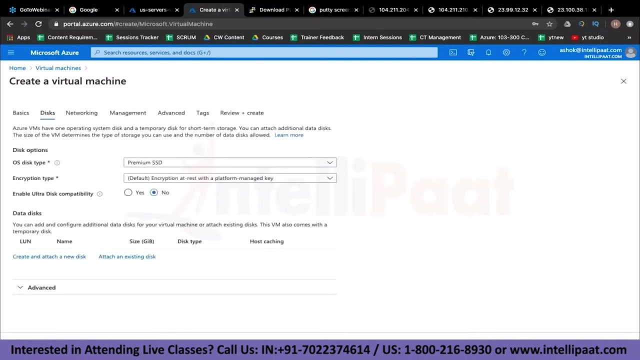 there will be a lot of steps that i have to do. it won't take much time, and in the meanwhile let's create one again. okay, so the size of the loading. so that will wait. let's quickly enter the same info, i think let's be double sure that we're defining it in the default subnet now. 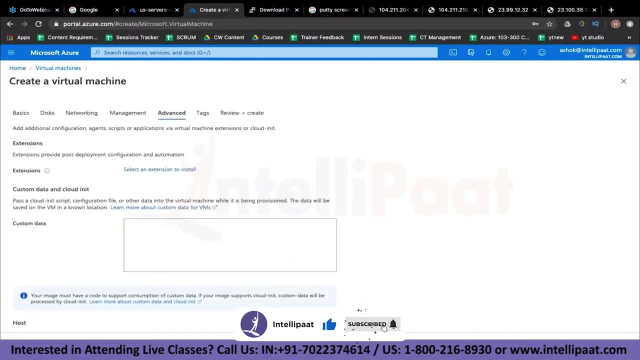 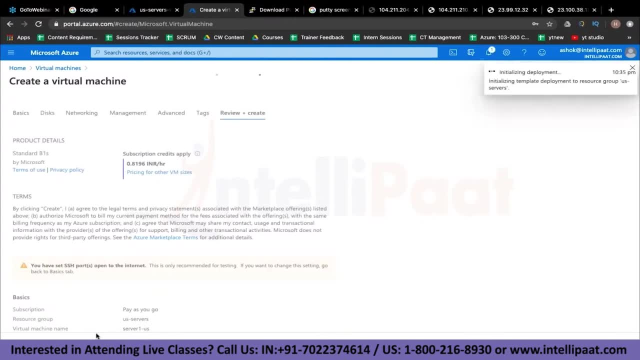 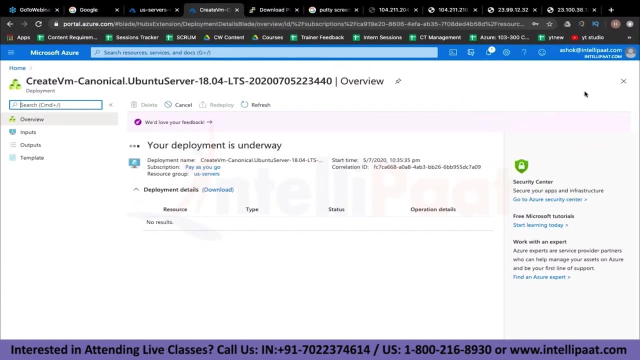 and management. let's turn off the diagnostics. if you press create, i think every good thing looks good. now let's create it. great, so it's now getting created. it'll take some 30, 40 seconds, so let's complete that and then come back to our application gateway. 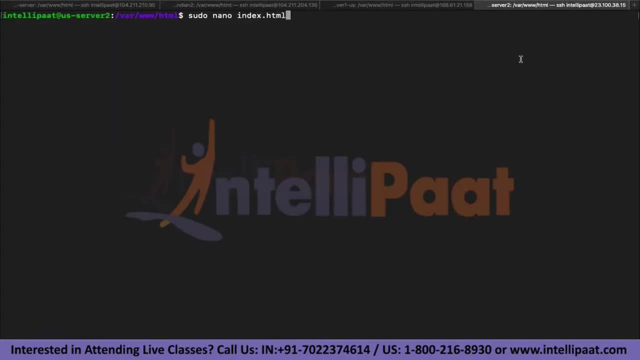 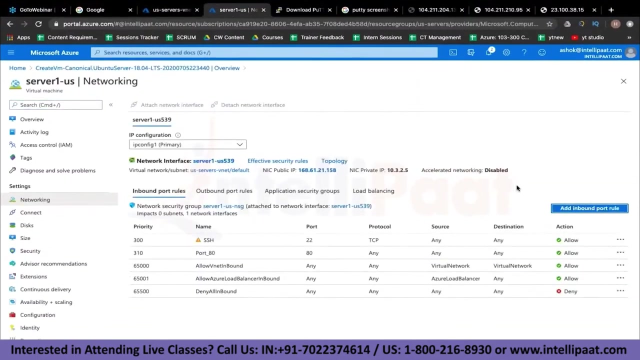 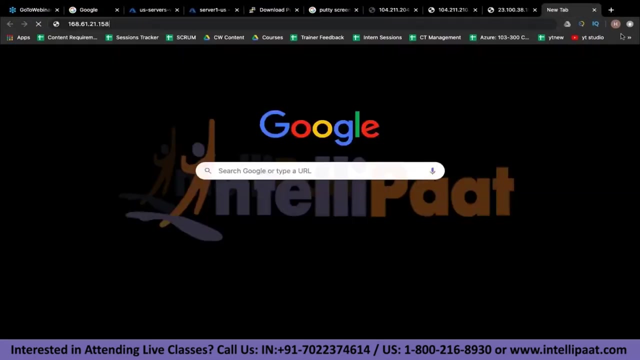 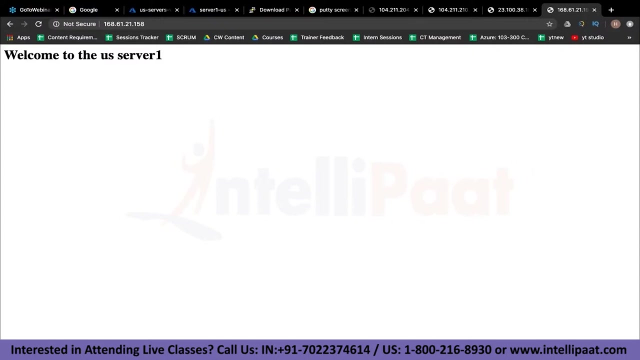 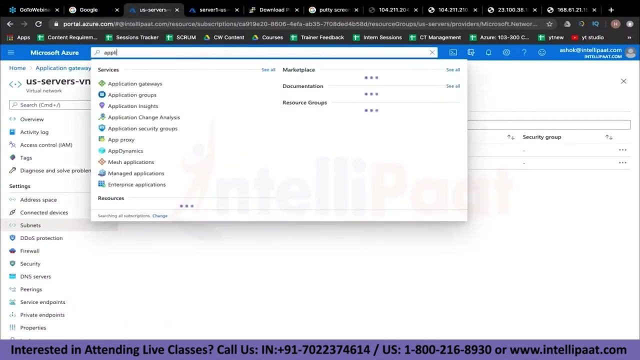 so let's copy the code, paste it here, and i think that is about it. so now we can just verify if we can see this ip on the browser. so yes, we can. great. and now what we can do is add one. this is: first of all, let's go to my uds developer, let's call our api. 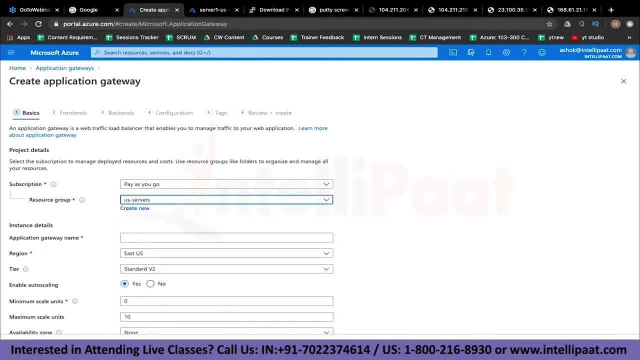 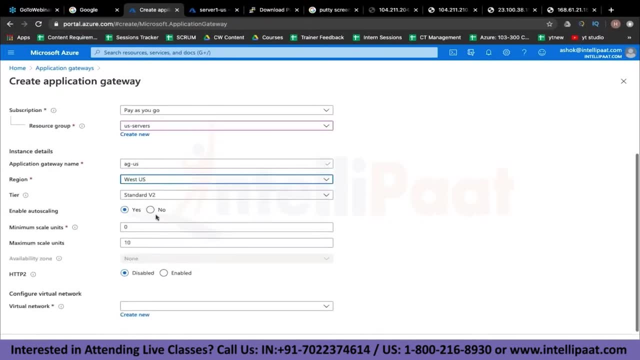 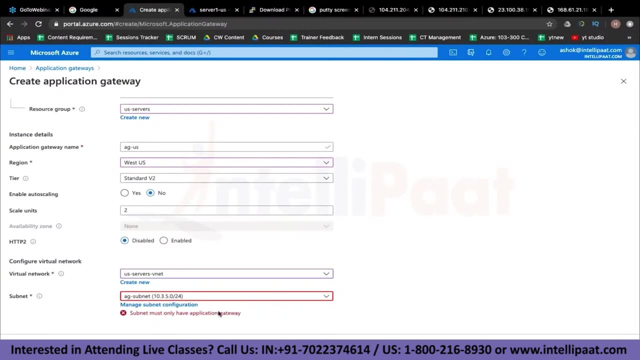 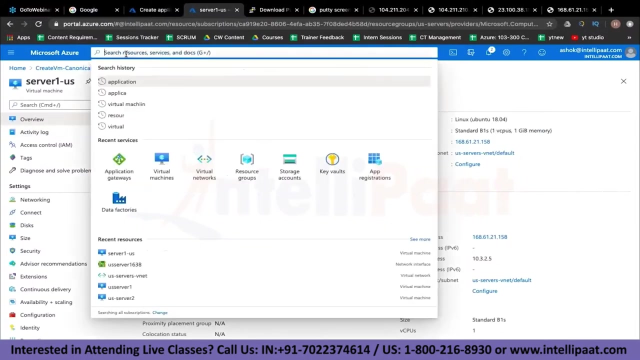 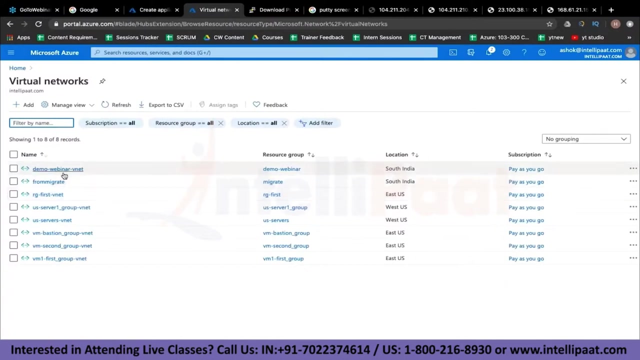 let's go to our server, go back in the browser, so i'll run the application. so, now that we have the servers configured, let's go to application gateway servers be net. okay, what is the problem now? well, this is part of. okay, let's do this. let's just delete the AG net subnet and try to connect to it again, so US. 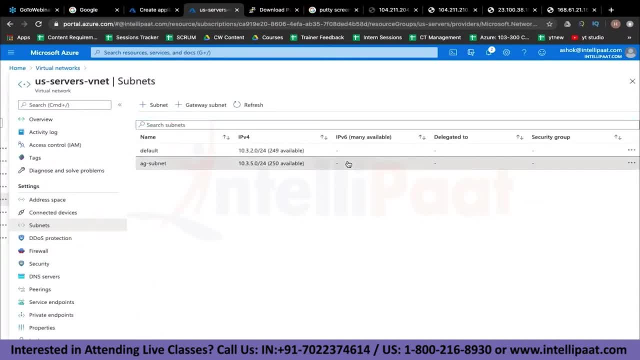 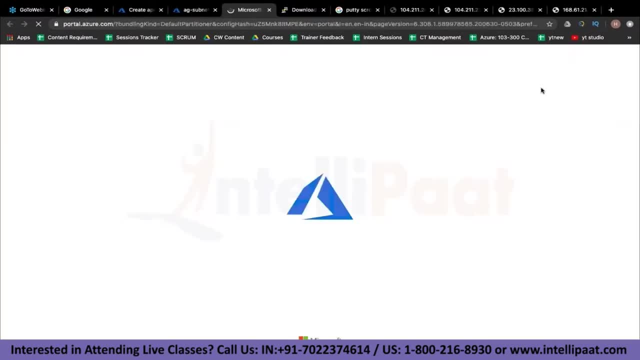 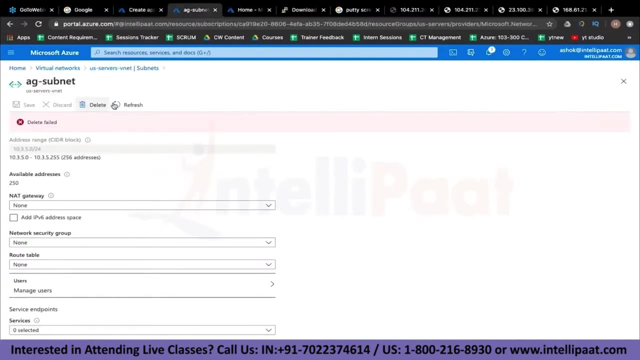 servers be net- we both subnets- or the AG subnet. let's delete it. okay, so there seems to be some network interface which I was making use of it. what we can do is let's leave this. let's create one more subnet where we can have our 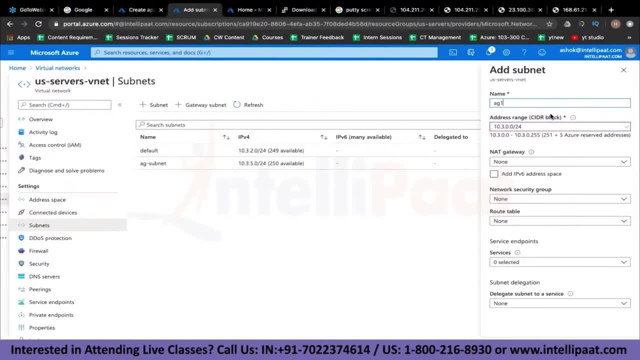 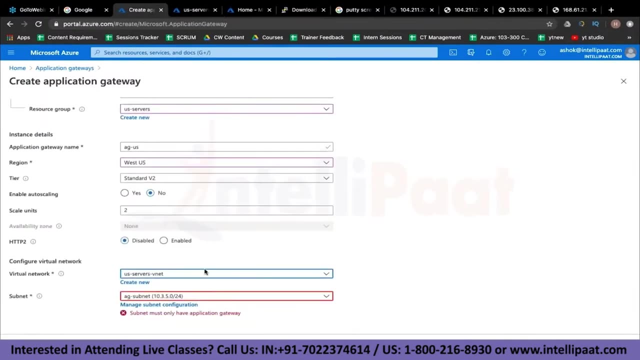 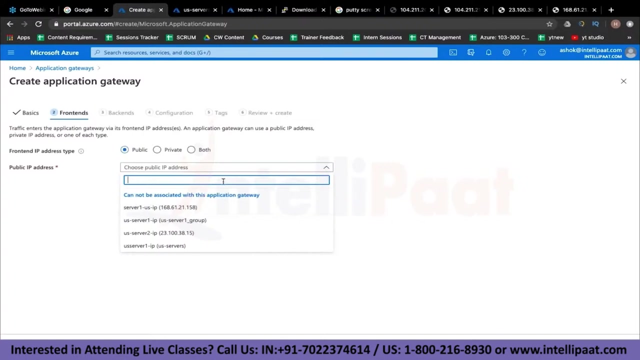 application gateway. so let's call it as eg1 hyphen subnet and this could be the range. let's create it and now, okay, this is a subnet that we want to configure. let's choose an ip address. let's add one new hyphen, ag, us. okay, let's add a back-end pool. so back-end pool is nothing but. 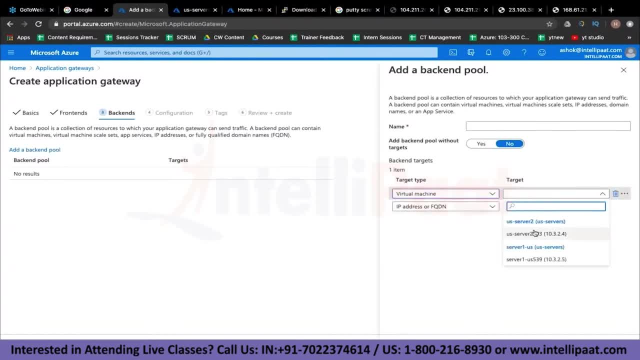 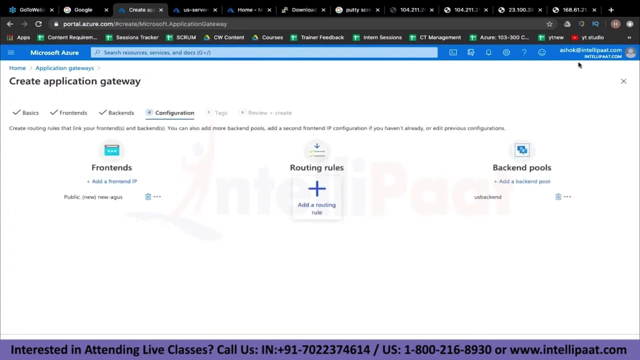 your servers. so right, so let's add them. so let's choose a virtual machine. let's choose the first virtual machine, and now let's choose the second virtual machine as well. okay, so we have added the back-end pool. let's call it as us backend. let's add it. done configuration. so is there a routing rule that you want to specify? 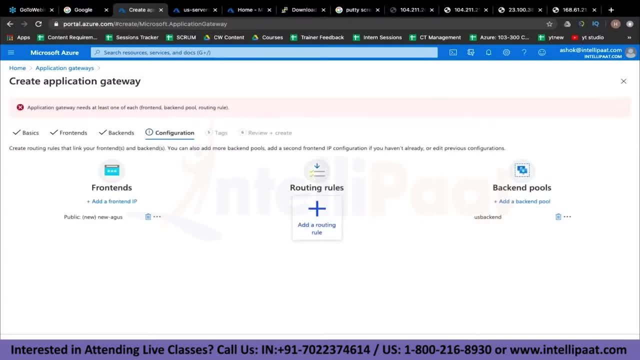 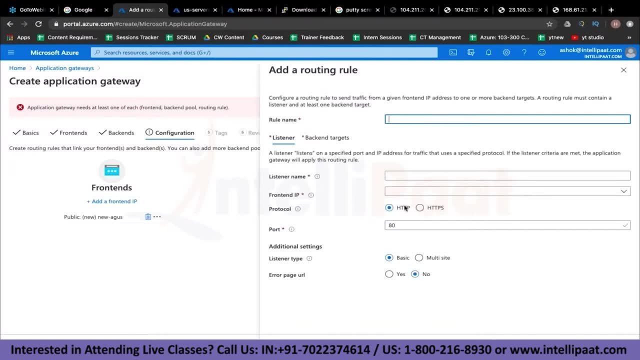 uh, let's not specify anything. so in that case we'll be here. uh, okay, I think we have to specify. so let's specify a backend rule. let's call it as uh, first rule. right, listener name would be: let's say it's listener iphone. us front-end ip would be public. let's not type in basic error pages, url. back-end targets. 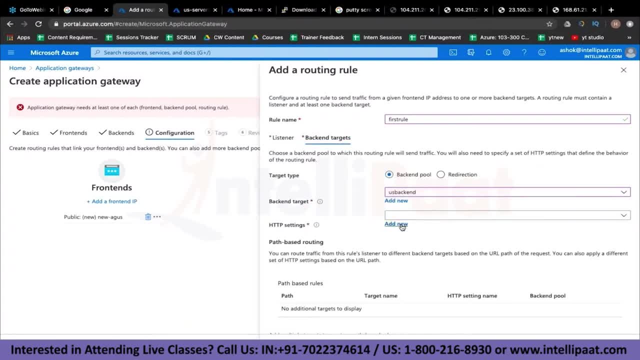 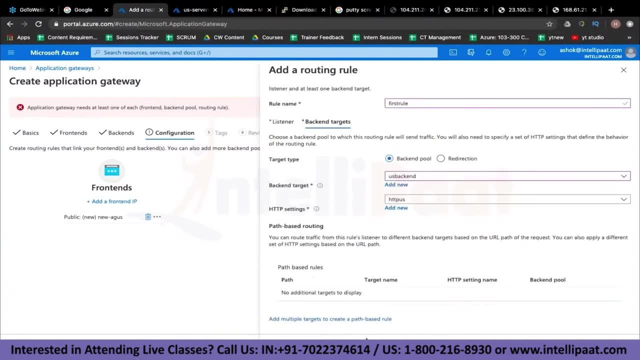 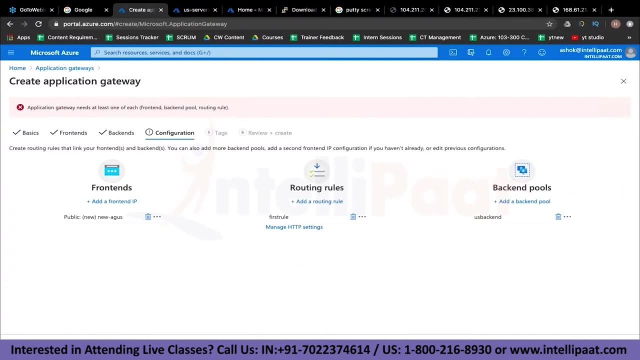 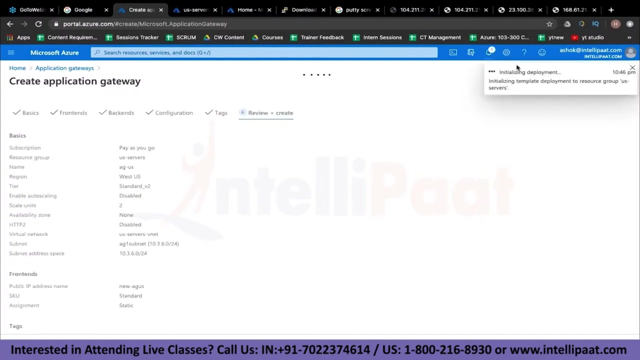 so it will be us back-end http. second setting. let's add new http setting. let's call it as http: us added us back-end data log. we're not adding any path-based rules in this load balancer. okay, let's hit an add and finally, let's just click on review plus create and create it. so with this, now we have. 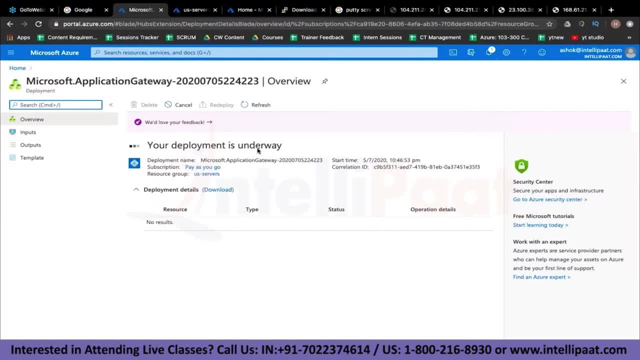 created the load balancer. uh, that is required for these us servers now. I think it will take a minute or two to deploy, so let's give it that time. meanwhile, uh, we can deploy the same for our our Indian servers as well. so for our Indian servers, I think the first thing 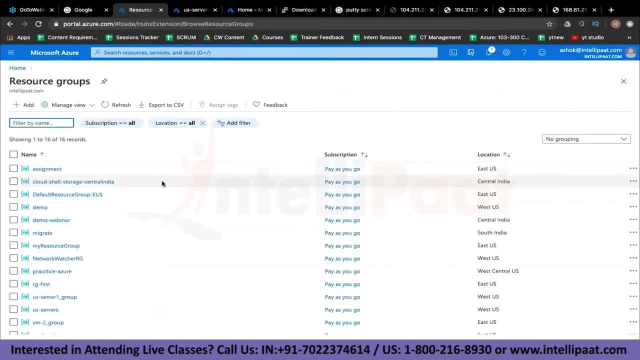 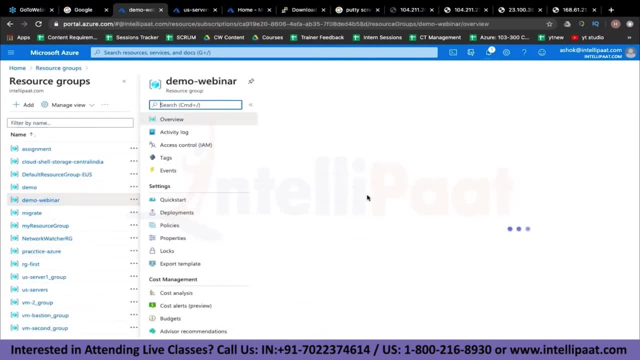 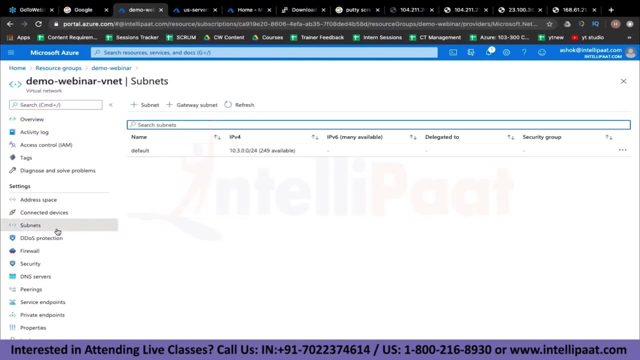 that we would need is the virtual network to be configured. so let's go to demo: webinar: resource group. now in this, the virtual network, the subnets. in this we just have the default one. so first we'll change the address space saved, now we'll go to subnets. okay, let's add a subnet and let's call it the AG subnet. 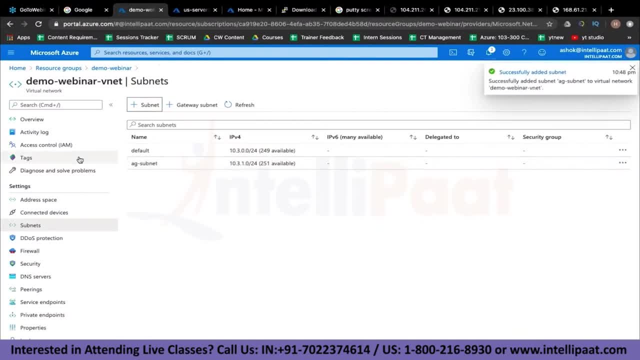 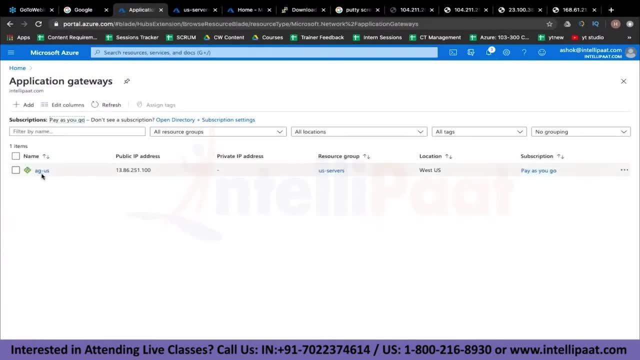 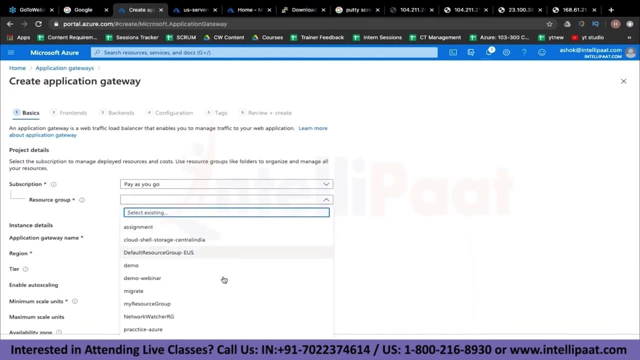 so now we have a subnet for the application gateway, right, and now let's go to application gate this and this is the us one which is getting created, right. let's add one more and it will be in the demo webinar resource group. we'll call. 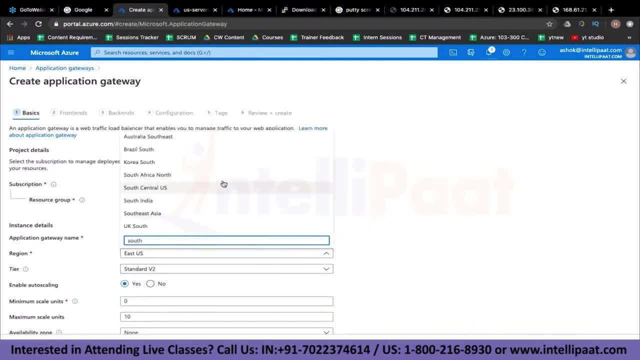 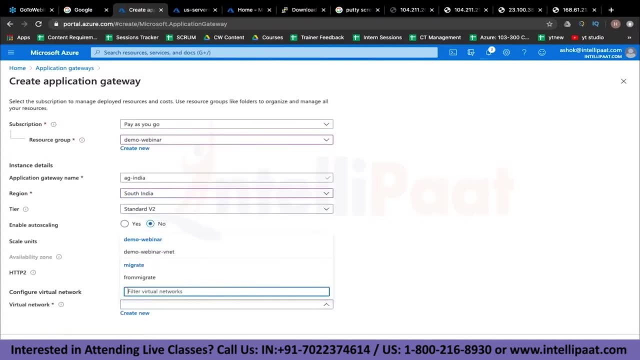 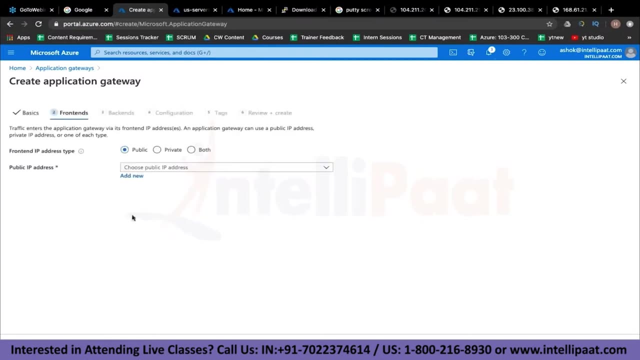 it as AG-India will be part of the south India region. not scaling virtual network would be Demo webinar, vnet and, yes, the subnet would be AG- Subnet. it's great. now let's add a public IP address to it and let's call it EG. 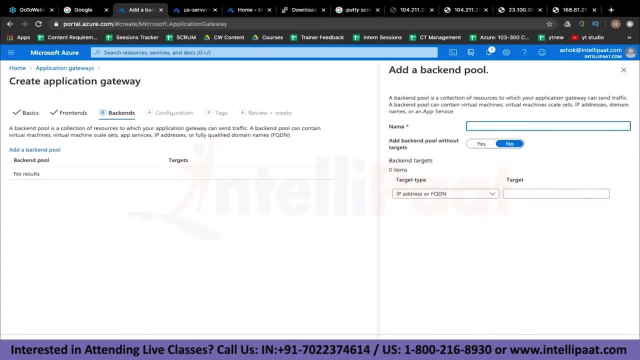 hyphen: India. again the back-end. so let's add a back-end pool. it'll be of type: what's the machine? so let's first add the first Indian server and then the second Indian server. okay, and let's call this as the India packet. so back-end. 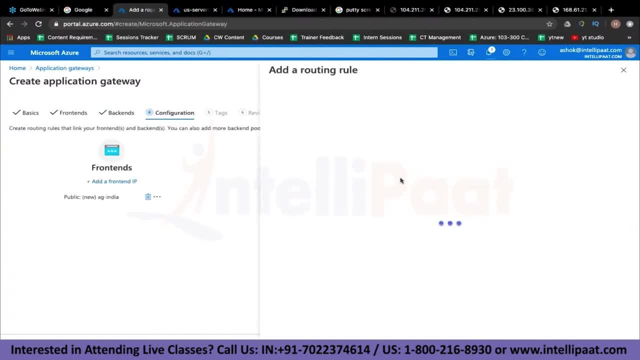 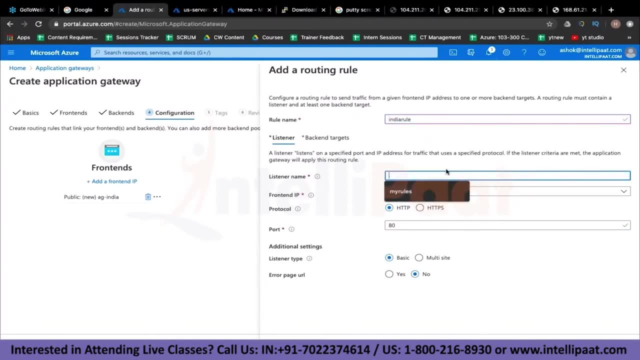 pool has been added. now let's add an outing rule. so again the same configuration, guys, the rule name. let's call it as India rule listener name. you can give it anything. let's call it my listener front-end IP. it would be public, obviously. then let's specify the back-end. 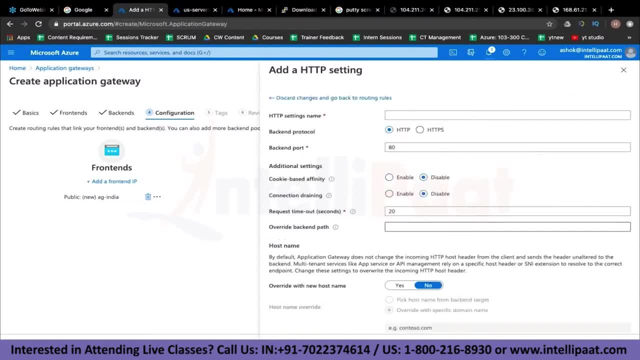 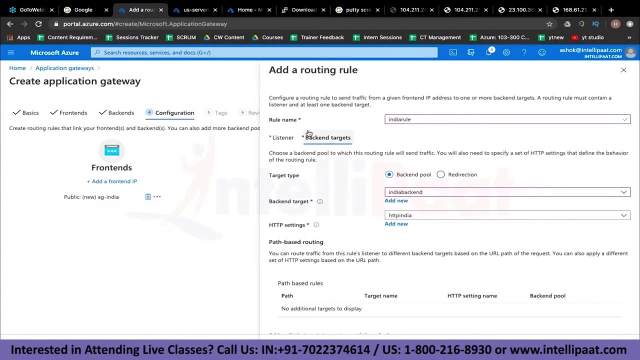 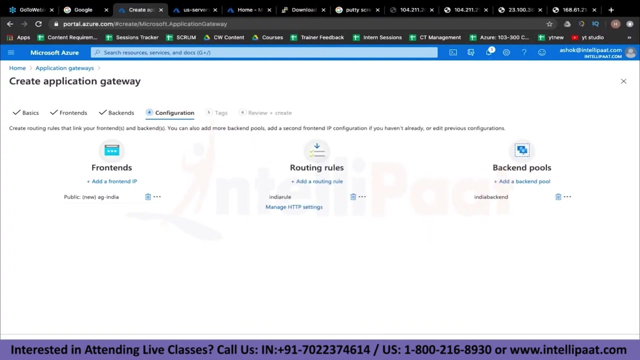 target. so back-end pool would be India. back-end HTTP seconds. you will have to add a new setting. let's call it as HTTP India here, nothing to be specified, just create the rule, the HTTP setting, and I think that should be about it. we're not adding any parts and let's just click on create now. 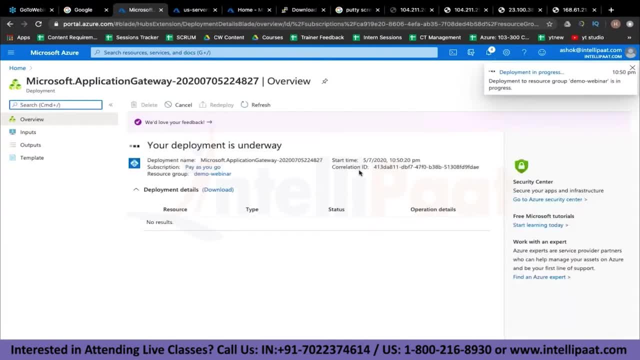 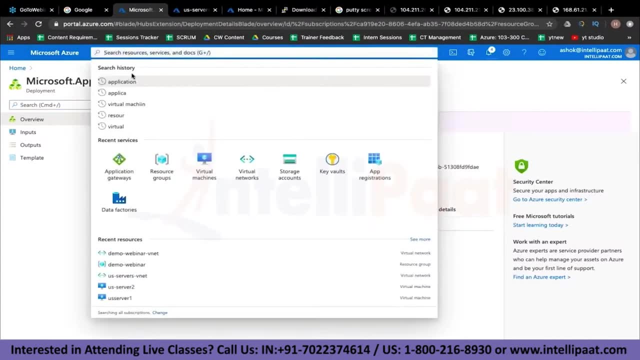 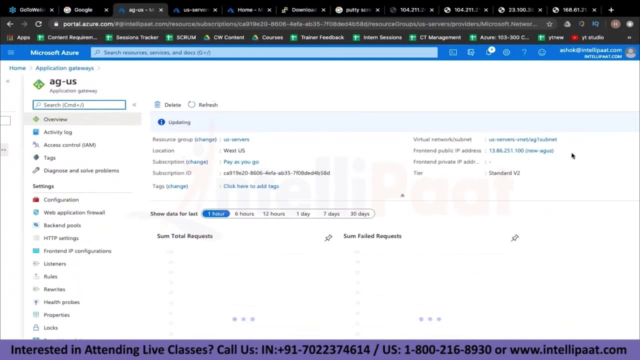 so with this, my application gateway has been created. this application gateway is now being deployed for India. I think my us one should already be deployed, so I let's check that out. so if I go to a g-h of them us, this is the IP address. let's 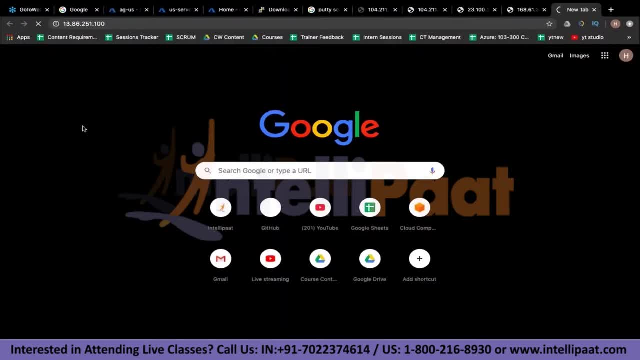 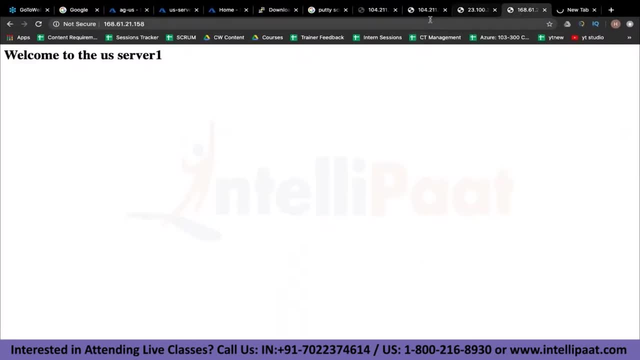 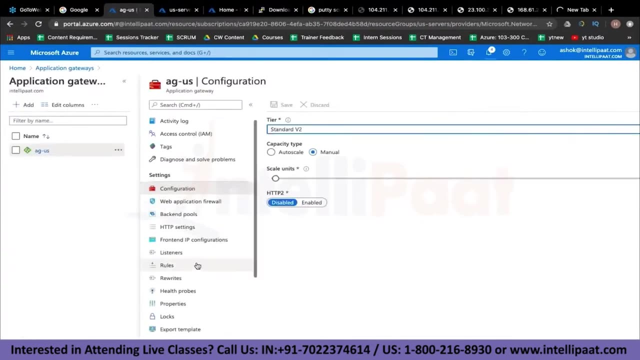 copy it, paste it on that browser and, as of now, I'm not able to connect to anything right now. right, so what I'll do is I'll just go back to my US application gateway. let me check. so there are a couple of things which can go wrong, because of which it is not connecting. so let's first check the. 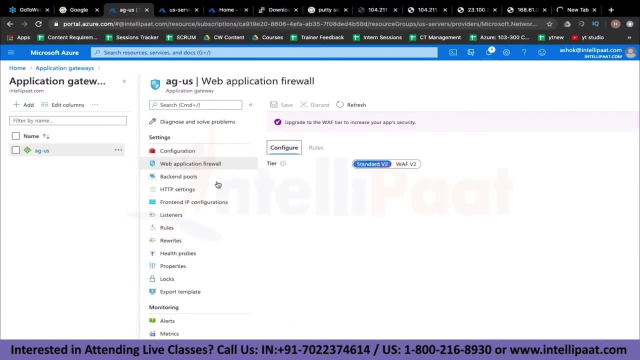 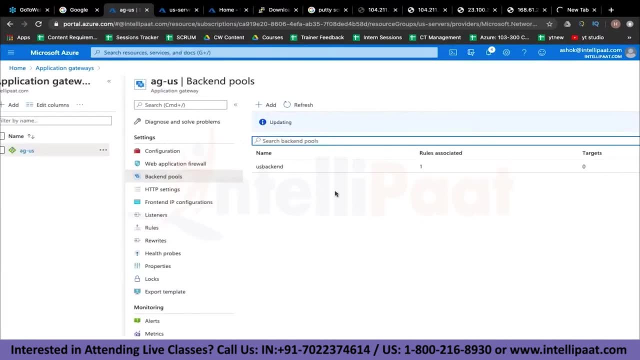 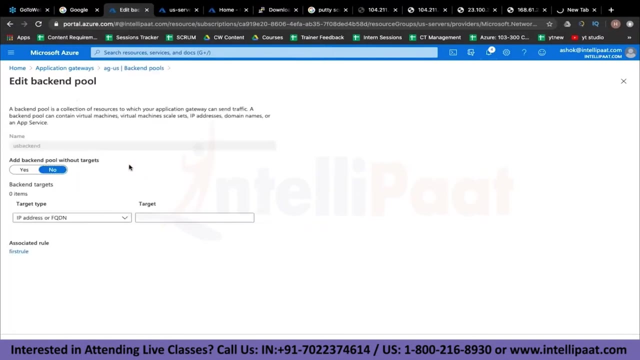 firewall. so here everything seems okay. let's go to configuration. here everything seems to be okay. go to back-end pools. okay, so there are no targets according to the rules associated. let's check that. okay, so there are no targets in the back-end pool for us. let's add it, although I think we did. 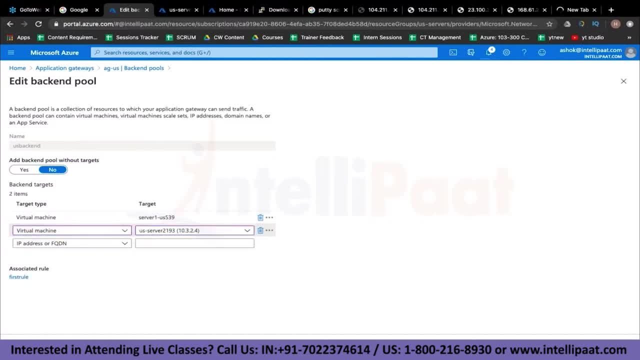 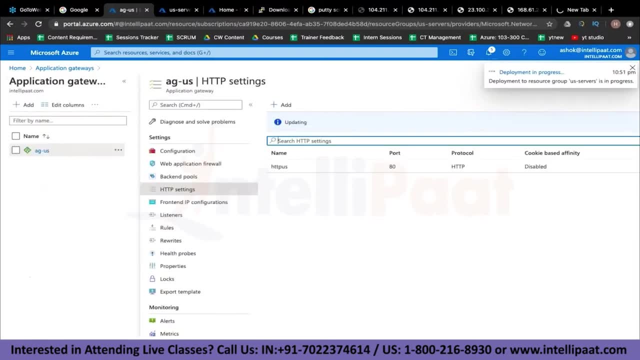 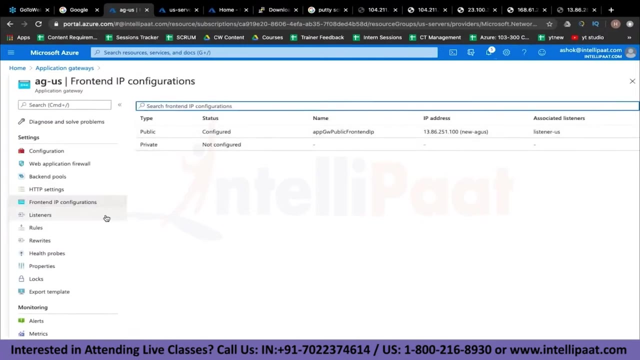 add it, but it's not there, so that's not waste any time you and save this, okay. while this is happening, we can also check out the other settings. so HDB settings look good. front-end IP configuration: public. we have configured it looks good. we have added a list now, which is okay. 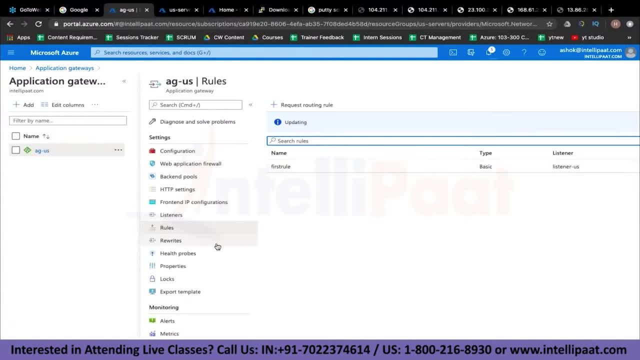 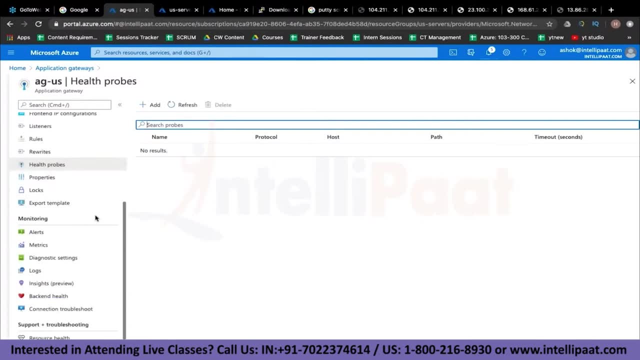 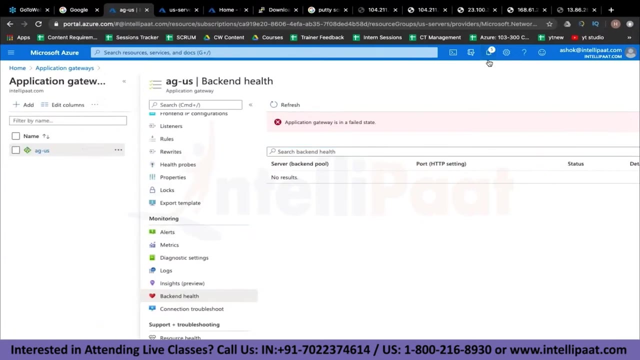 rules look good for school health probes. yeah, nothing here. then I think you also something have something called as back-end health, okay, so application gateway right now is in the deployment phase, right? so that's why you cannot see it right now, so let's wait for it to get completed. I think our application 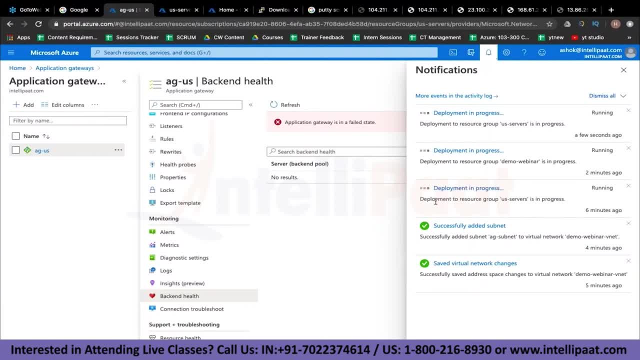 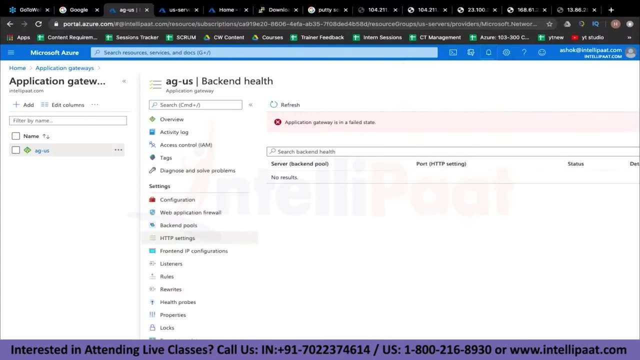 gateway is still in the deployment phase. so as you can see, that deployment to group US so is a still in progress. so I guess the application gateway has not deployed fully and that's why you know it's taking some more time. so load balance is a very, very heavy resource guy so it usually takes around some five. 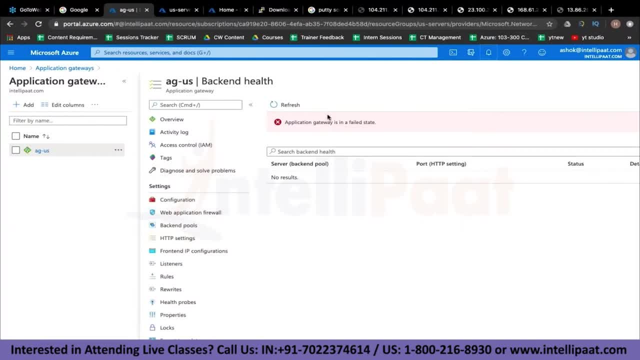 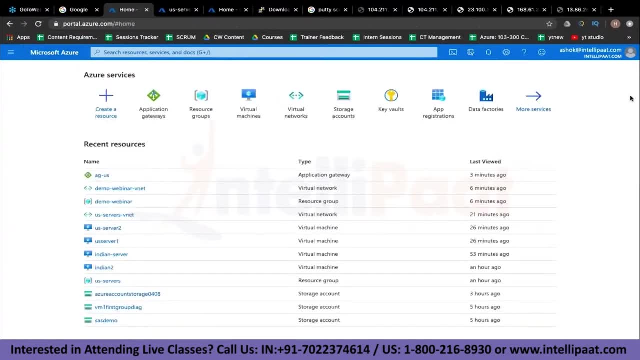 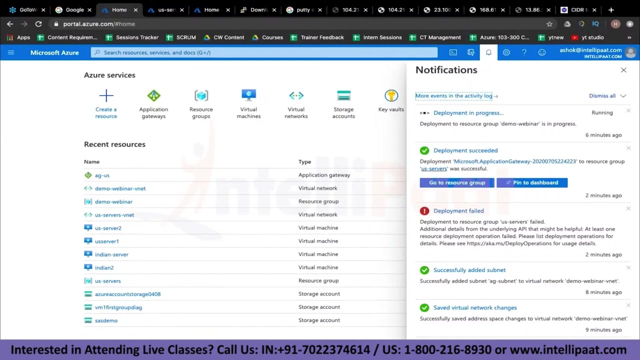 to six minutes to deploy. so let's wait for that, that time, while this is completed, right, and while it is being completed, let me see if you have any more questions. so you, okay, so us. so one is failed, one is succeeded. let's see if we have. 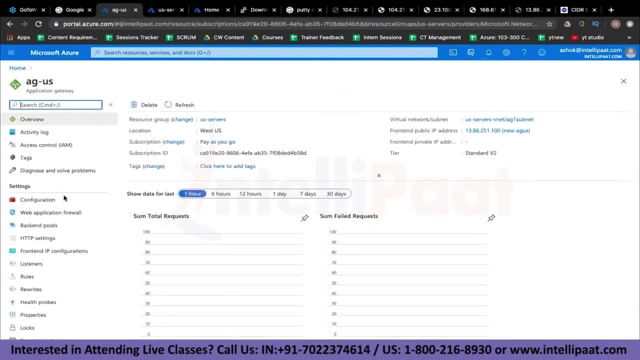 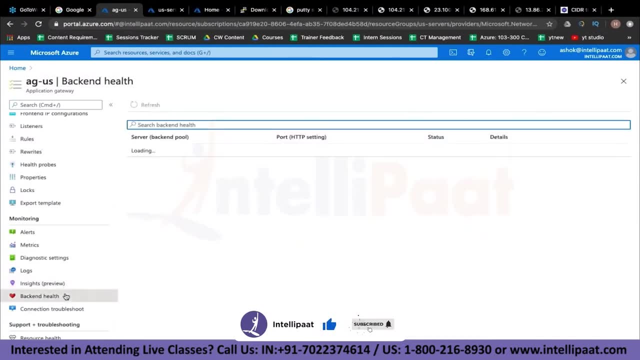 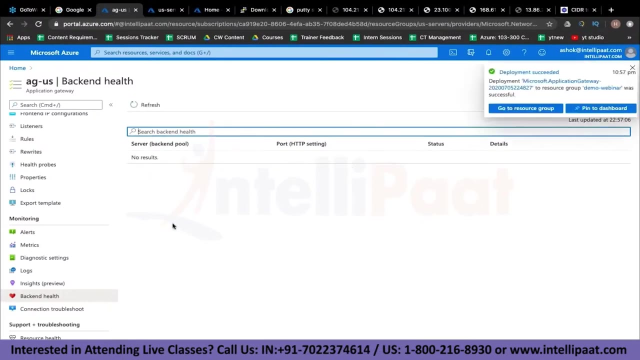 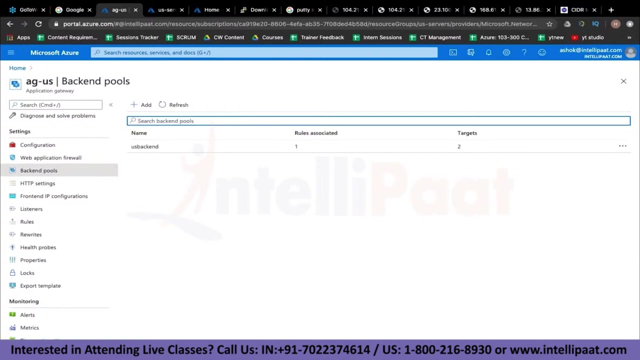 everything in my application gateway. okay, this is my US application gateway, guys, as you can see from the name. let's check the back-end health. so now you should have two servers listed over here which are not listed. okay, let's go to back-end pools. so there are two targets, which is good. 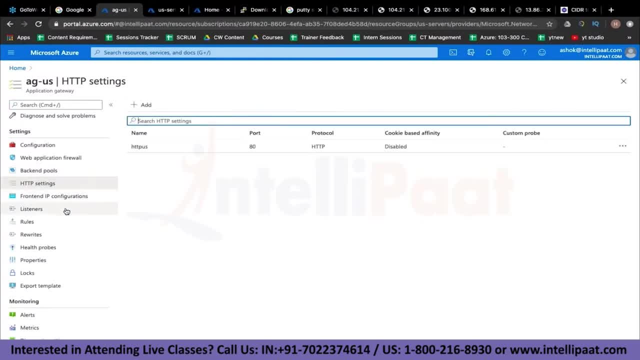 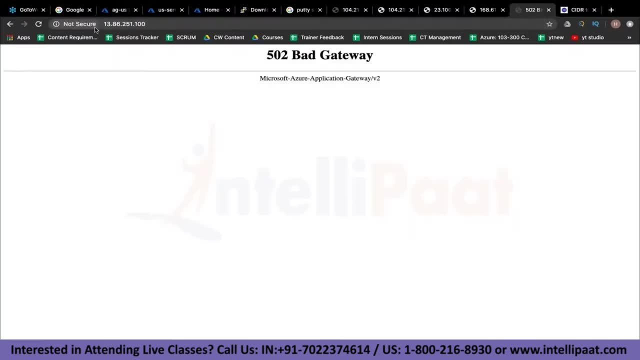 let's go to HTTP settings. this looks okay. rules looks okay, okay. let's try to go here, okay, and try to refresh this. okay, so, at least our application gateway has been deployed. it just says that there's a. okay, so at least our application gateway has been deployed. it just says that there's a. 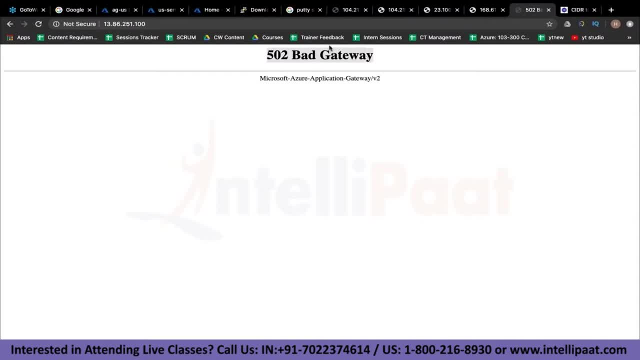 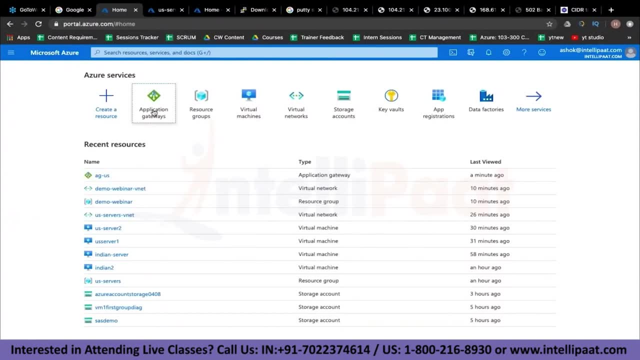 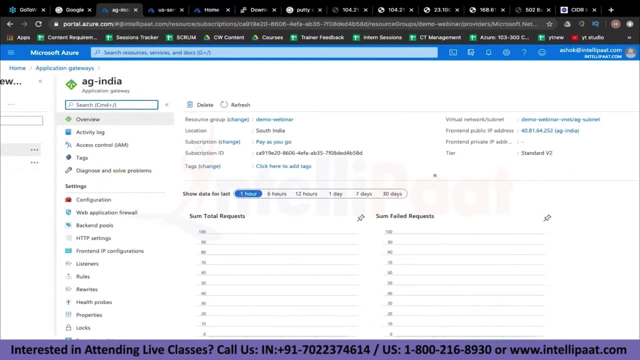 bad gateway. so we will see how we can fix this. meanwhile, even shower Indian server has been deployed. I'm sorry, Indian application and gateway. let's see how that is working out for us. so go to the application gateway India. let's copy the IP address, paste it in the browser. 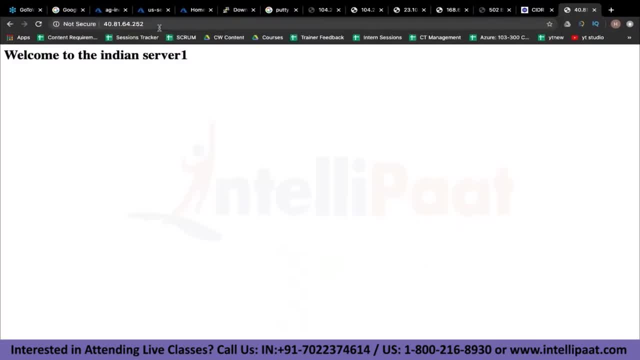 it enter: okay, this seems to be working. okay, this should open as well. so this is, this seems to be working, just fine. so it says: welcome to Indian server one. great, if you keep hitting, refresh it, as you can see, it is now routing you to Indian server 2 as well. right, again, it is out into one. again to two, again to one again. 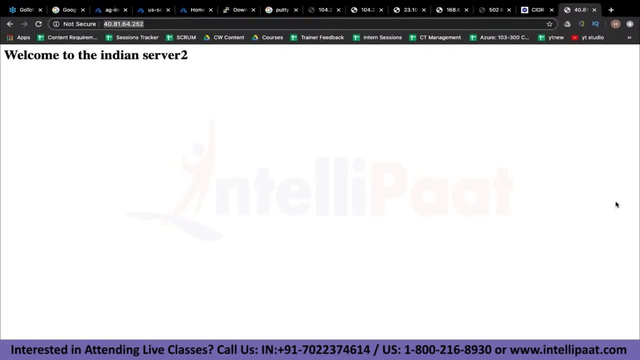 to two. so it randomly basically takes up your request and it is now routing it to you, routing to one of the servers. usually on the production of architectures. what happens is, once there is a load balancer through which the servers can be accessed on the browser, the servers firewall is restricted to. 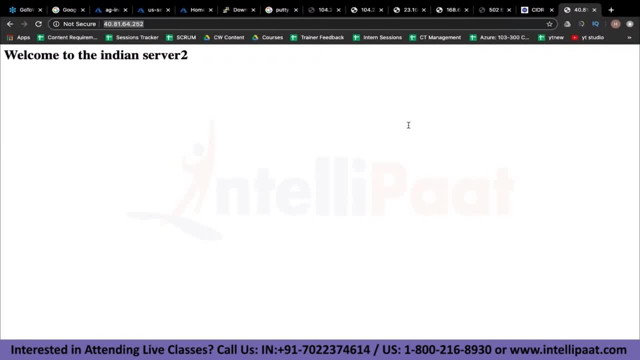 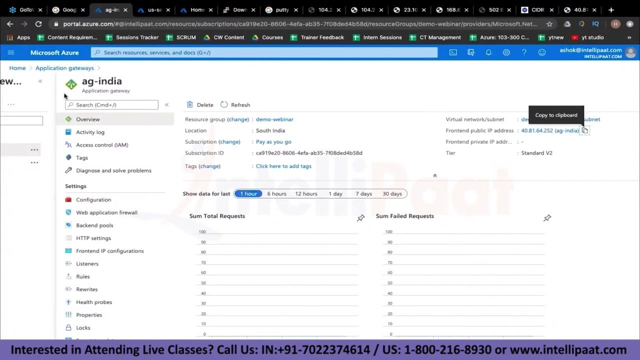 just a low connection from the load balancer. obviously, this is done as a security reason, but you will have to do it by yourself, right? and that's a architectural best practice. okay, so this is working fine and the US application gateway is giving some issues to us, so let's see how we can figure that out. let me just go to the US. 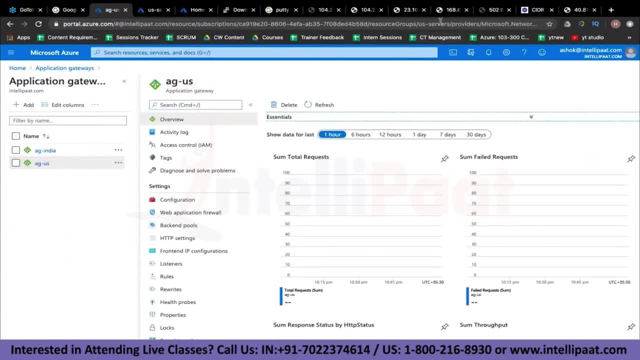 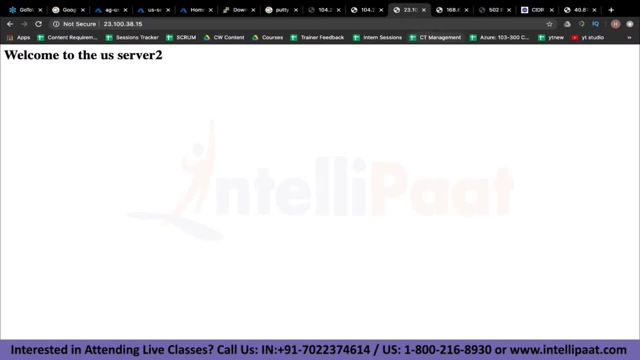 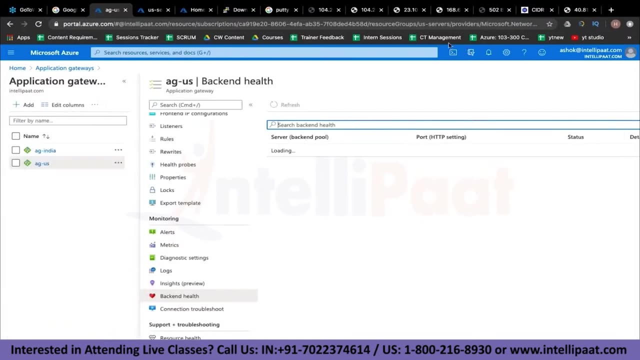 application gateway. so first things first, let's see if the US servers are working fine. yes, the first server is working fine and the second server is also working fine, great. so I think the problem is that the backend health is still not restored over here, and because of this I 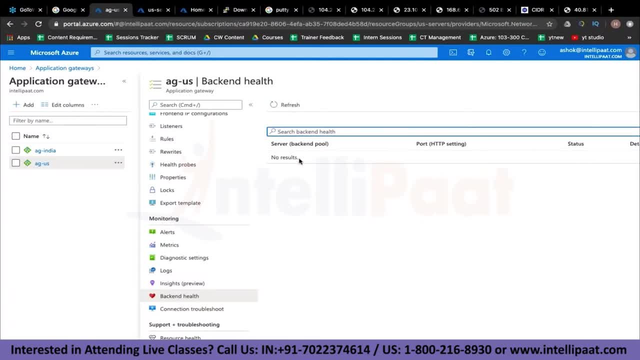 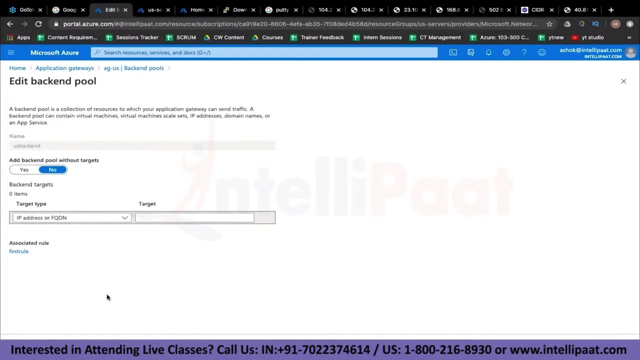 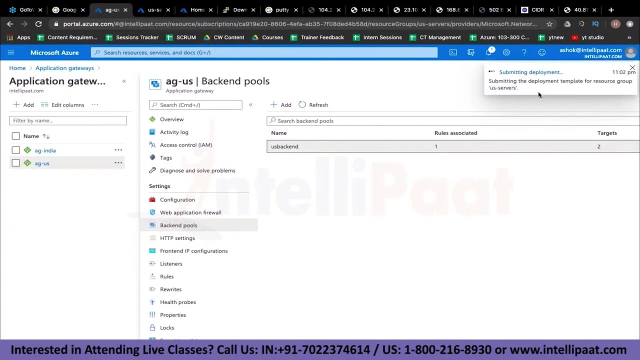 think it's giving you as 502 error. okay, so to fix this, what we can do is we can go to back in pools and we can just delete these targets, save it and once this deployment is successful, we can add the new two targets. again the two targets and I. 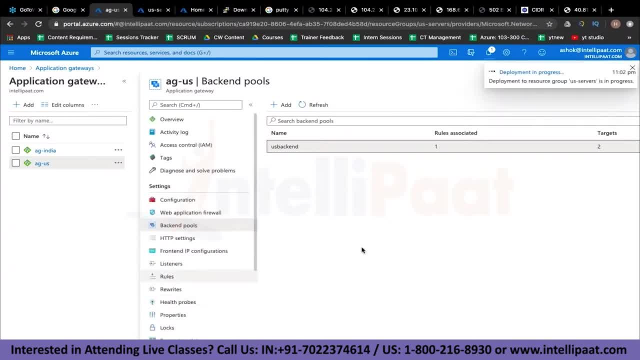 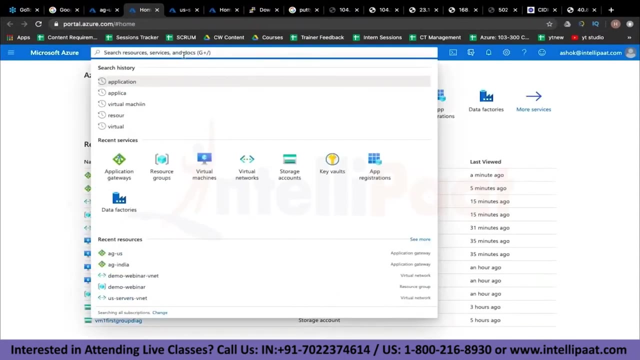 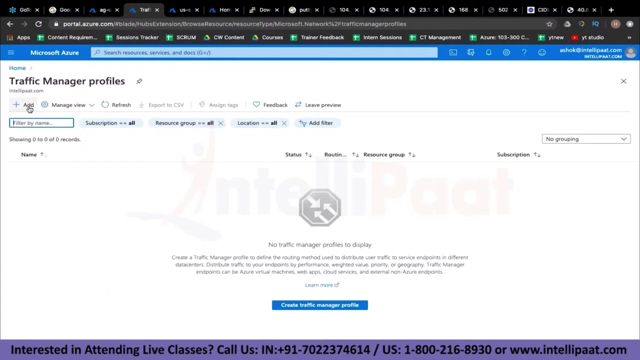 think that should solve the problem. okay, so while this is happening, let's go ahead and configure a traffic manager now, so we can see that the India load balancer is working perfectly fine. so now what we'll do is: let's create a traffic manager. okay, so let's create a new traffic manager, let's click on add and let's 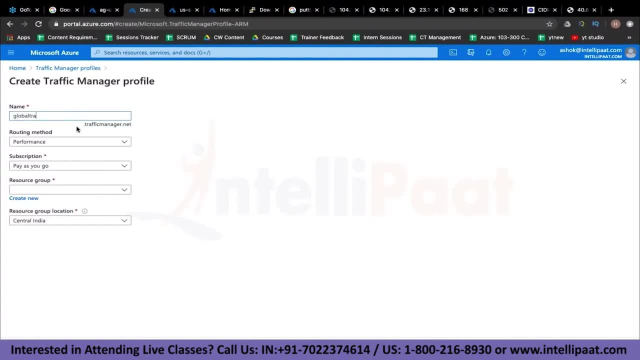 call it as global traffic manager, and we can deploy it in any region. let's say we are deploying it in us. okay, resource group would be usos. okay, this is very important. the routing method: so we want to route it according to geography, right, so wherever the 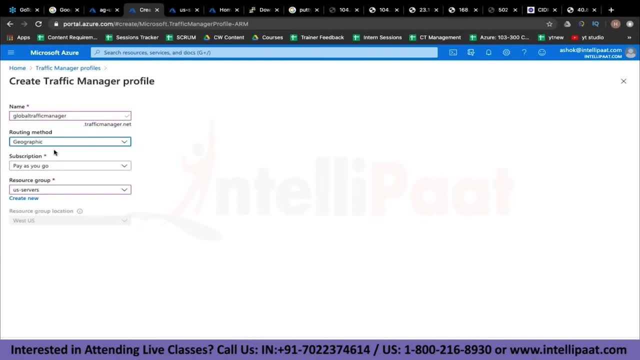 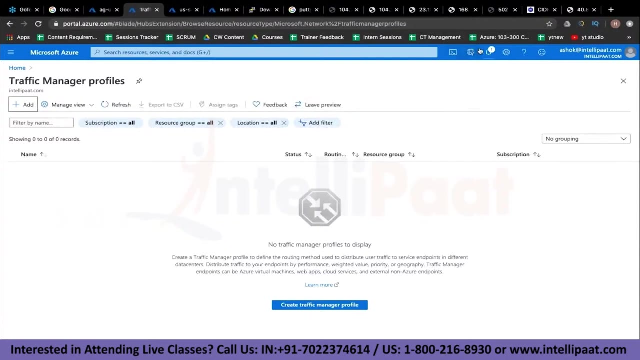 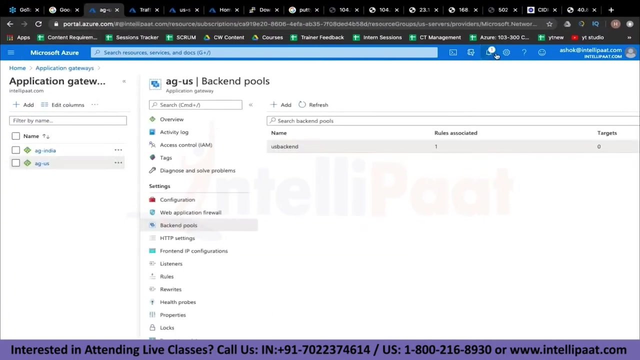 request is coming from. that request should basically be routed to the servers which are near to it, so we have chosen the routing method as geographic. let's click on create and with this, our traffic manager has now been created. okay, now this will take some time, so let's give that time to it. and now let's. 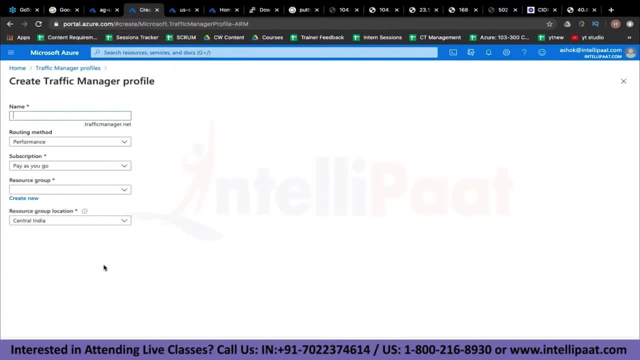 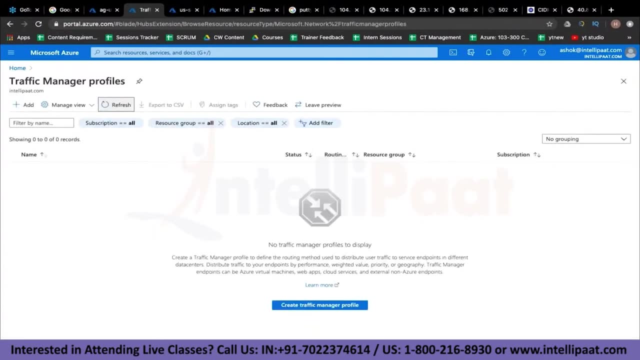 click on add, so in the traffic manager profile. okay, we've already added it, so it should list here. let's refresh, so it will take some time to. okay, so deployment has succeeded. great, so the traffic manager, we can see it over here. now the status is enabled, so we can go. 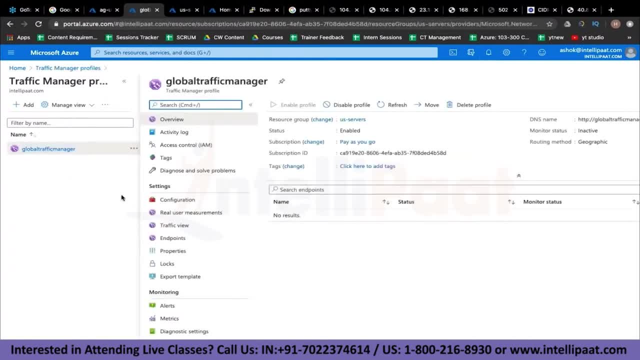 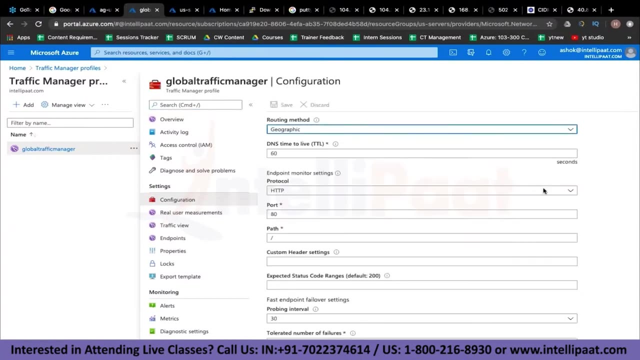 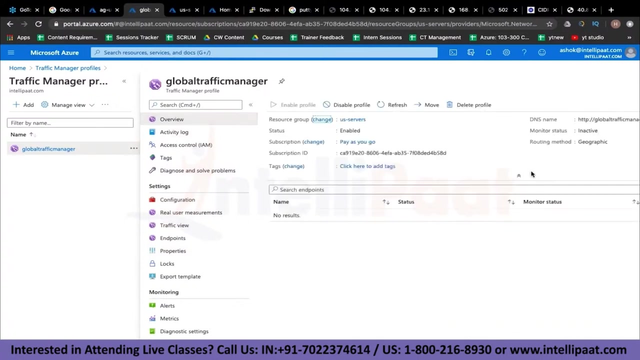 inside this traffic manager. now what we can do is we can configure it to connect to our load balancers. okay, so for doing that you will have to go to configuration. okay, everything looks good over here, so now we will have to add endpoints, and so there are no endpoints over here, so we 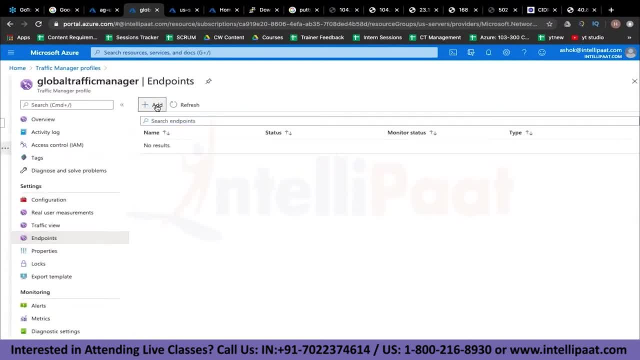 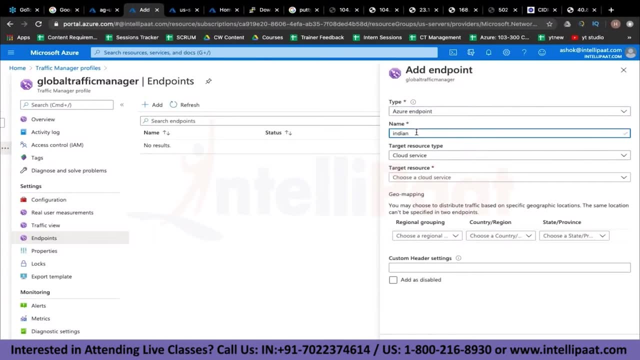 will go to endpoints. add an endpoint, so let's add it for the Indian server first. right, so the. so whenever you're adding the, you have to make sure of one thing, which I'm going to show you in a little while. so, first of all, let's select the public IP address, and the IP address would be: 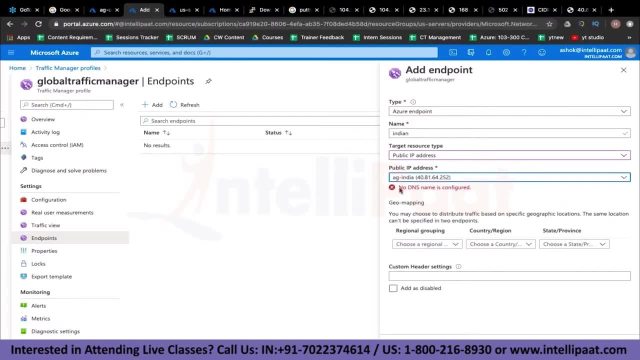 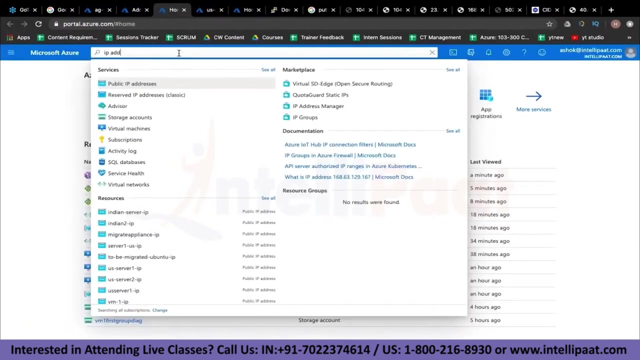 for AG India. so, as you can see, it says no DNS name is configured, right, so what you have to do is for the AG India IP address- AG India is with nothing but the application gateway of India- you will have to configure their DNS, okay, so let's see how we can do that. let's go to the IP addresses page. 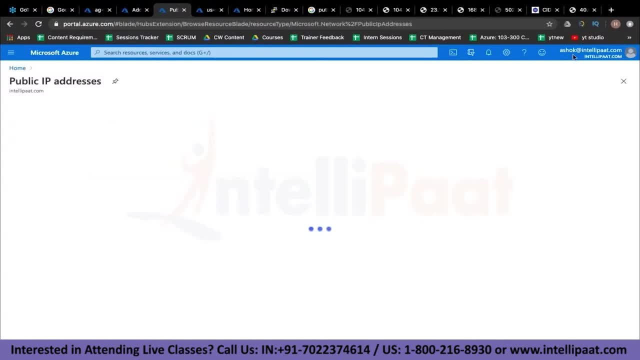 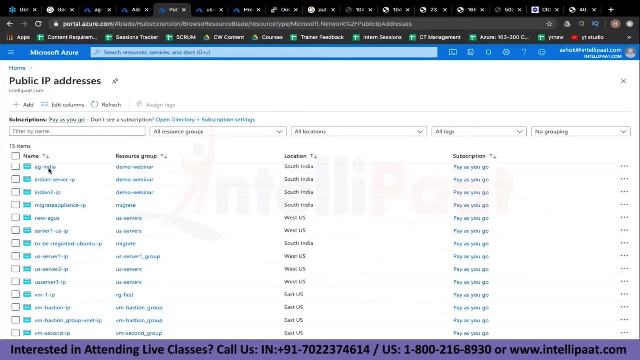 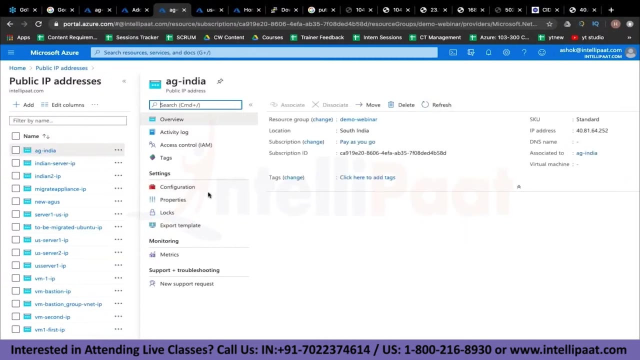 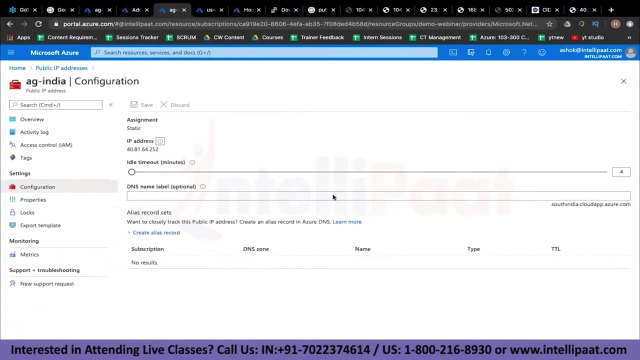 go to public IP addresses. here we'll go to AG hyphen India, which is this and AG hyphen India. now what we'll do is we'll go to configuration. in configuration we can get the DNS name right. so all our Holelije's DNS names. 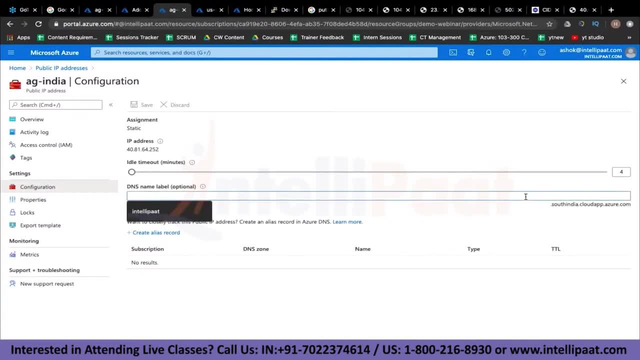 will. a book to help this suffix attached with it. so let's give this as a gee IP. now it is checking whether it's a way, emperor, so it's available, and now we can just click on save. with this, our public IP address is now going to have a DNS name. okay, so it's done, and now over here. 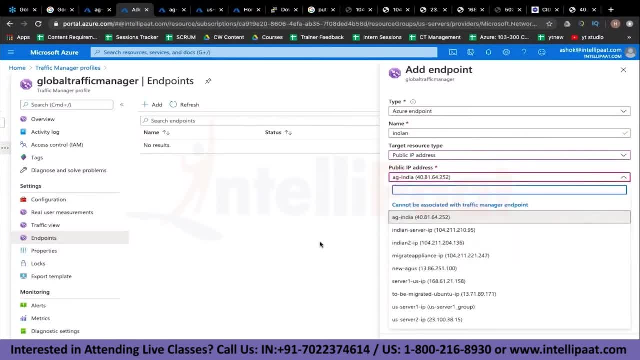 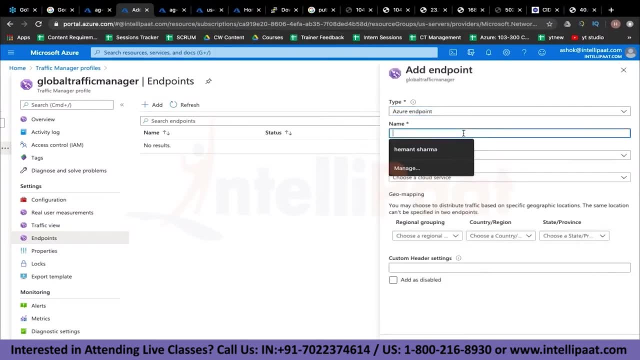 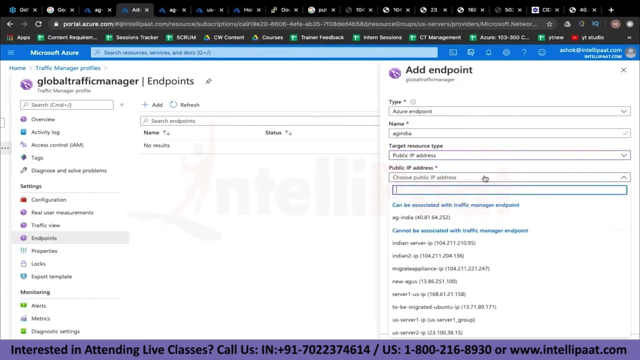 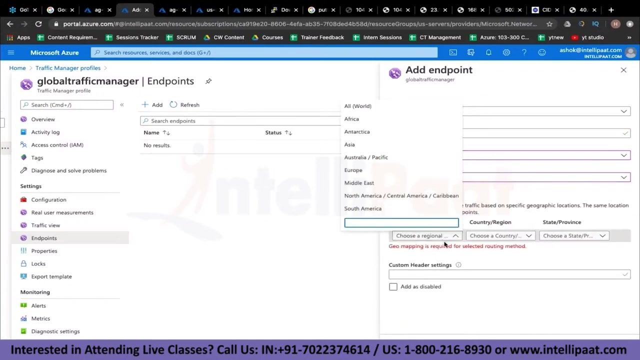 I will have to, I think, refresh this. so let's add an endpoint again. let's call it as AG India endpoint. it's going to be an public IP address and the IP addresses is in there. great, so let's click on add and now I can just do a regional mapping. 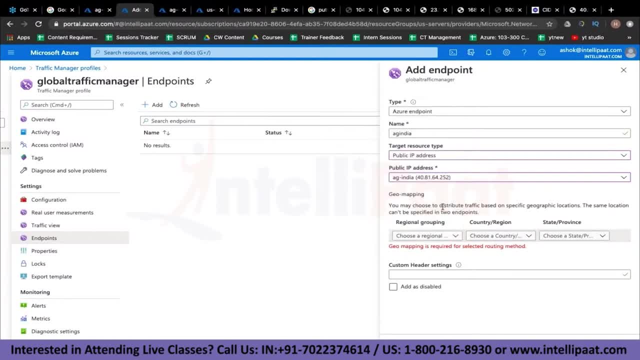 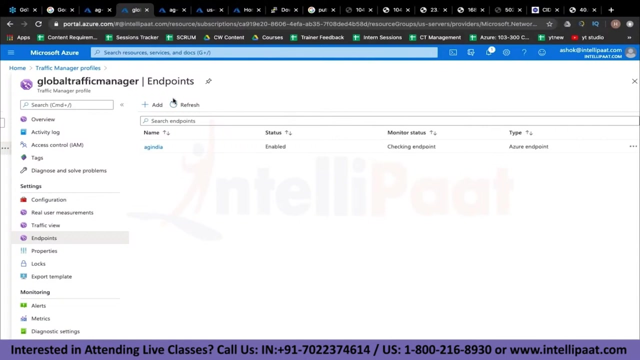 over here which is going to be mapped to it. so here we can choose to distribute traffic based on specific geographic locations. okay, so anybody who's springing from Asia in Asia, let's say India, then they should basically be routed to this endpoint. okay, so with this, your endpoint has now been configured in the traffic. 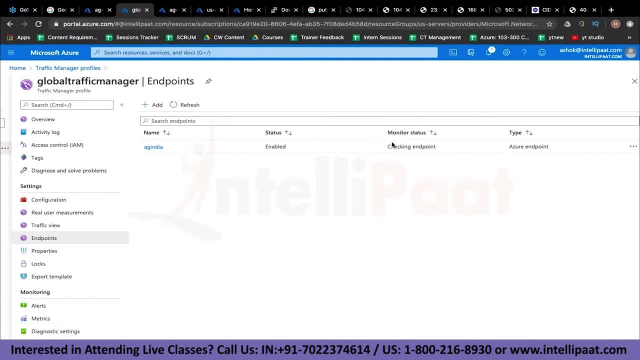 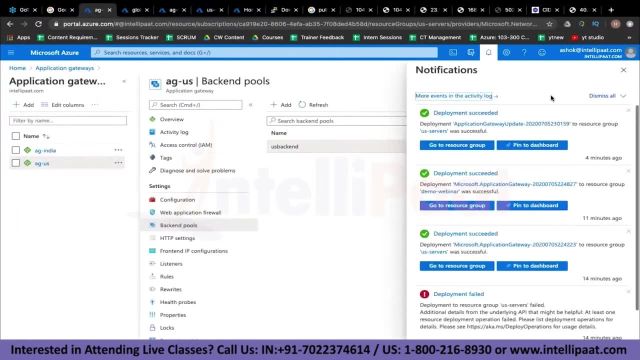 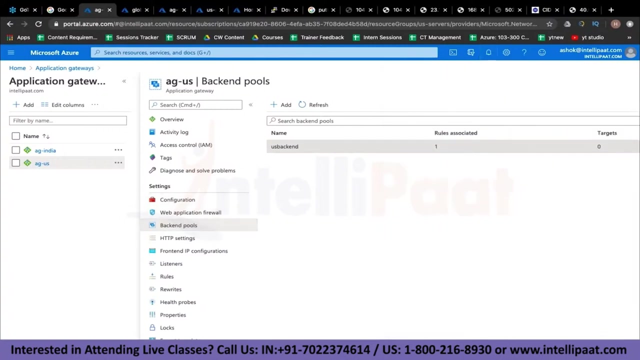 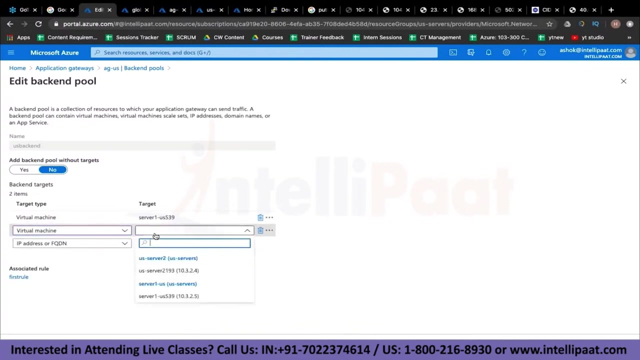 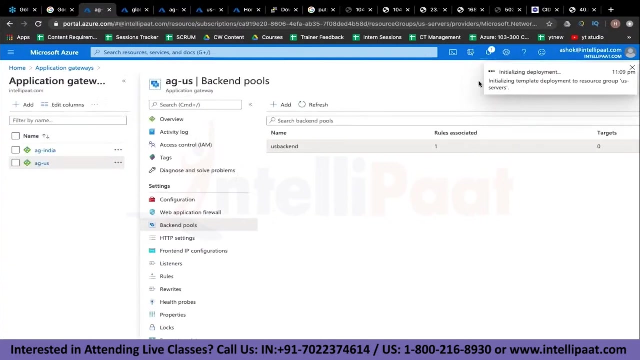 manager to connect to your Indian servers. so now let's verify if my AG us: yes, so an application gateways the for the US server. that was successful, great. so now what I can do is I can again add the targets and that should solve our problem. okay, so the deployment is now happening. meanwhile, let's verify if we go to our 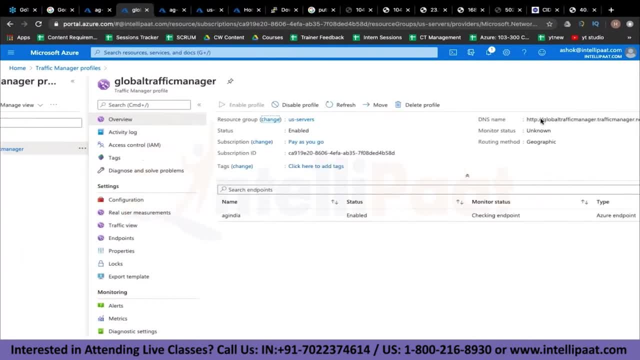 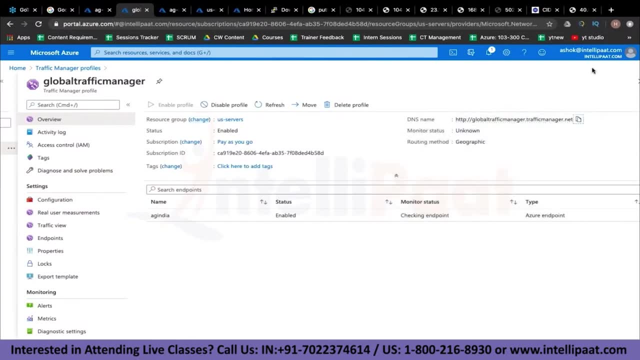 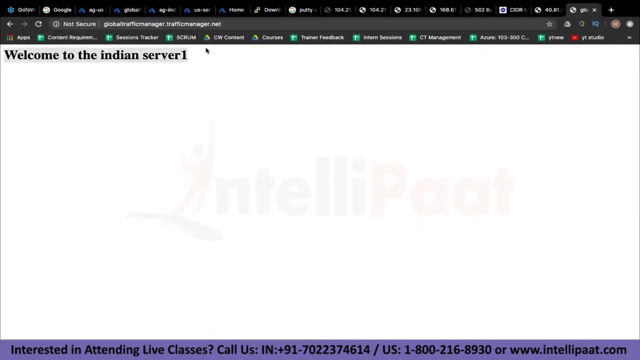 traffic manager is having this DNS. are we able to access the source or not? so yes, we are able to access the Indian source, right? so that means our traffic manager is working just fine, so I can give you this IP address as well. so, right now, because only Indian IP addresses are there. that's why our Indian servers are. 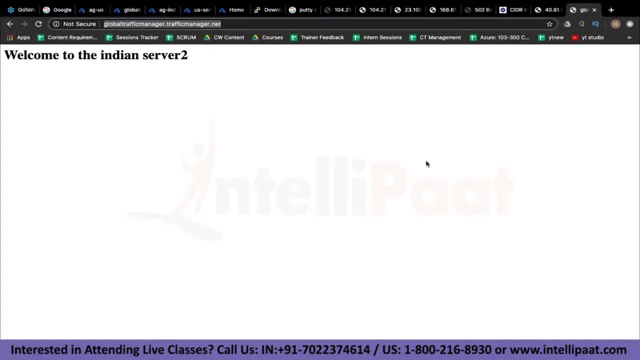 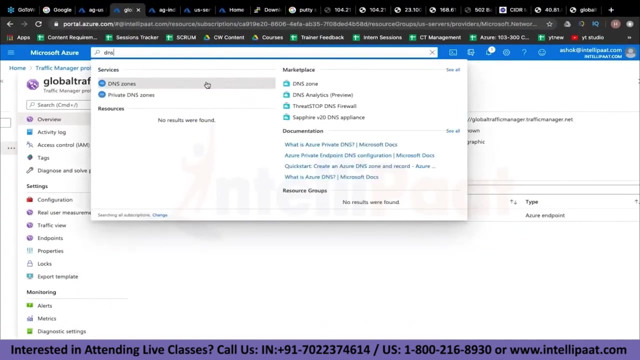 connected to it or Indian endpoint has been added. that's why only the Indian servers are connected. but as soon as we also add the application gateway for us people who are from outside Asia, they will be able to connect to it right. so, while this is happening, DNS name. so we will just search for DNS, this select. 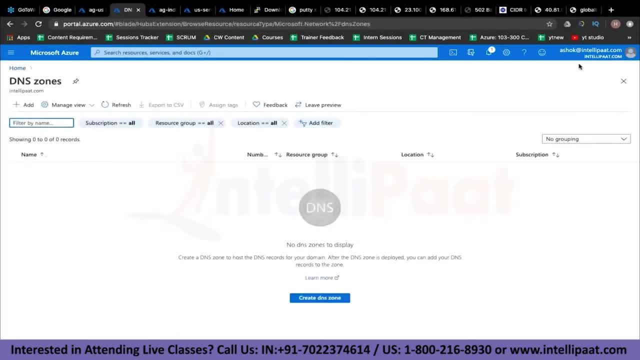 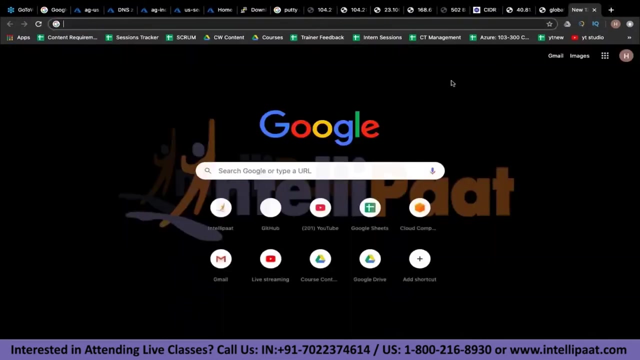 DNS zones. so here you can basically add a rule that, or you can configure a custom URL which can connect to your traffic manager, and let's see how we can do that. so if you want to do that, guys, the simplest thing to do over here would be to first go to. so there's a website called free norm. 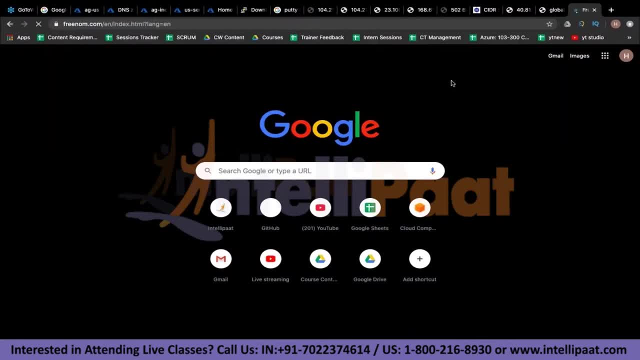 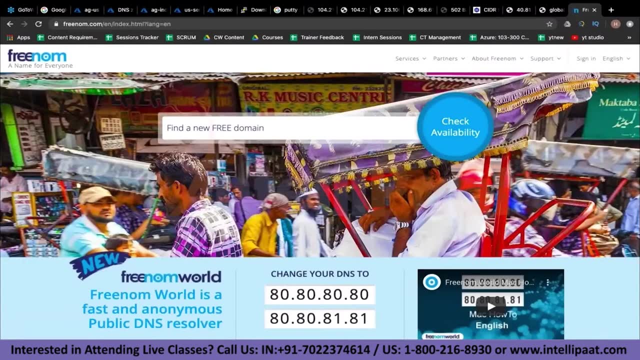 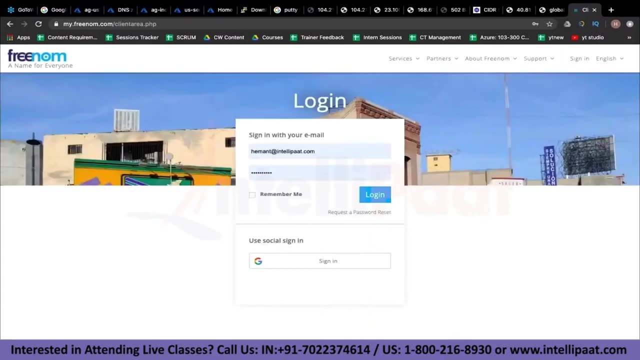 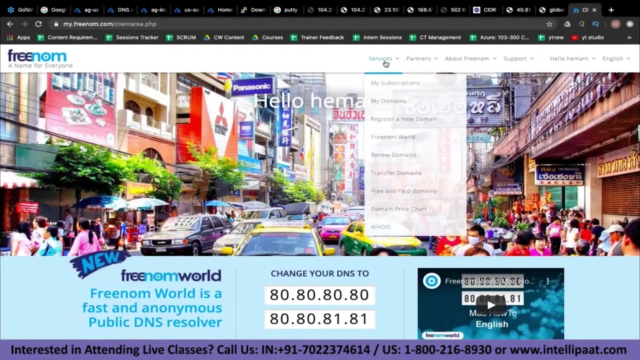 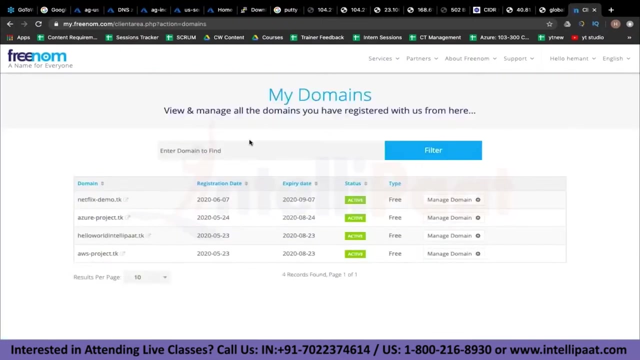 just go over there. so free norm gives you the information about the domain. again, you already have a free domain which you can create. if you just check is like: so let's sign in. I already have signed up over here, so you guys can also sign up and with this, what you're gonna get is you're gonna get domain that you can use. 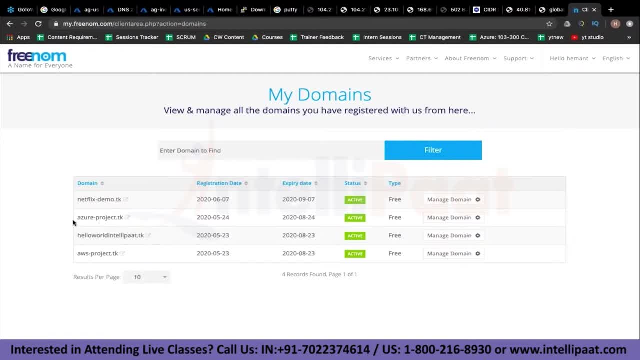 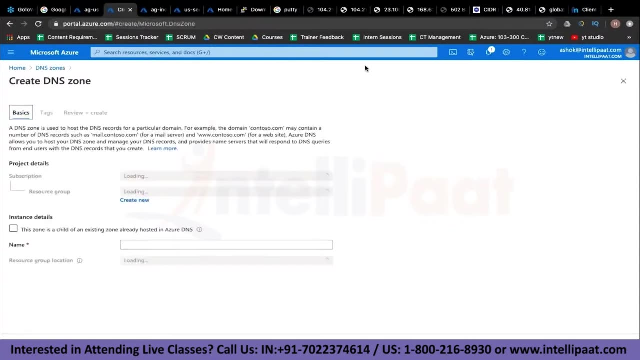 that I have specified and then all I have to do is, the moment I go to as your hyphen project or TK, I would be able to see the website that I've deployed. okay, so in order to do that, just go to DNS. so first you will have to add a DNS zone. 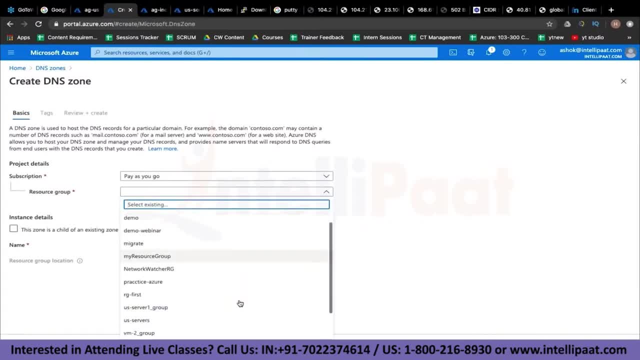 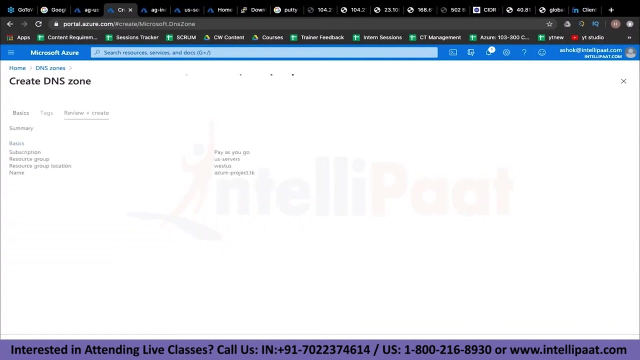 let's specify it in us again and the name that we will give them is DNS, hyphen, public. okay, or basically it's expressing expecting us to give the domain name itself, so it'll be as your hyphen: project, dot, TK. okay, let's click on review plus create. 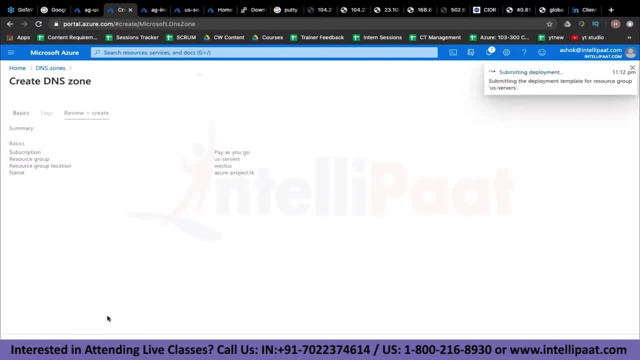 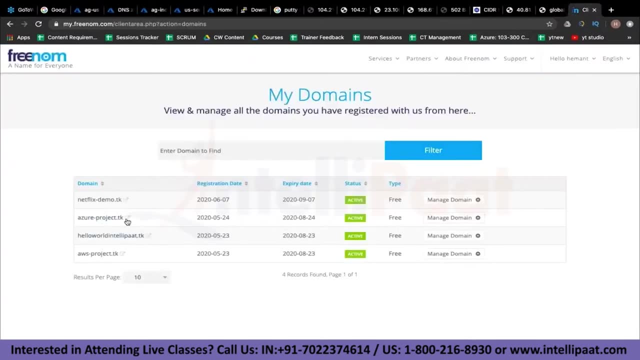 created and with this, our DNS zone will now be created. and this DNS zone we will have to connect our domain to this DNS zone and then we will configure a DNS zone to connect to our traffic manager. so that is how the flow is going to happen. so 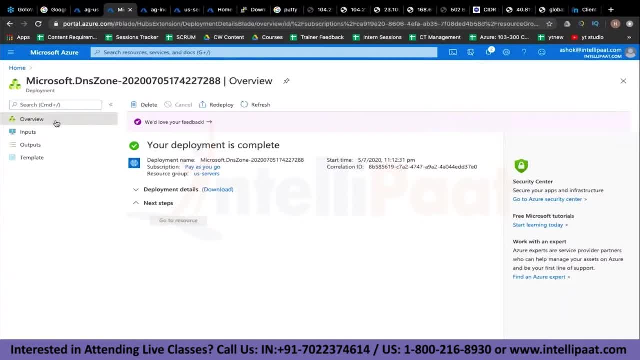 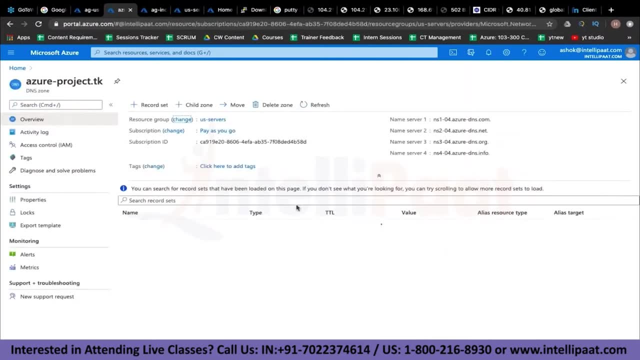 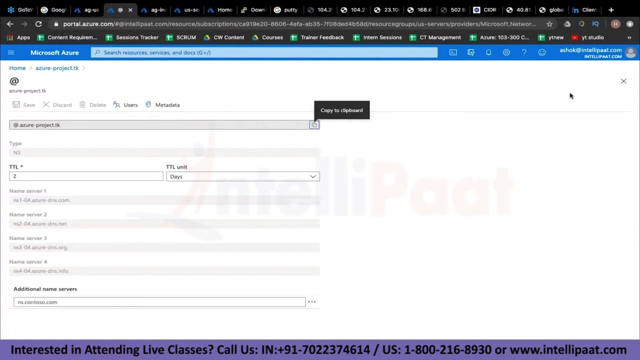 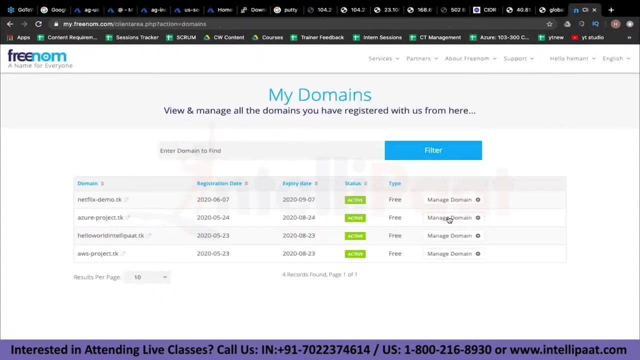 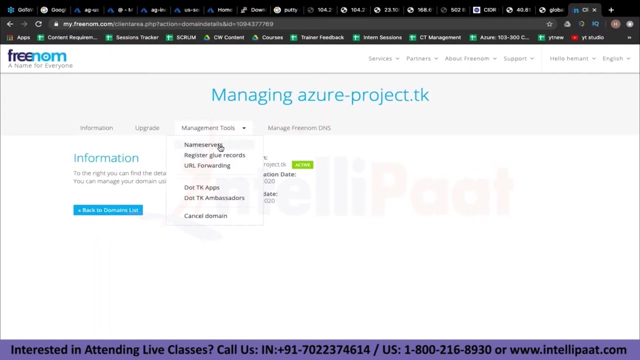 the DNS zone deployment is complete, so we can just go to the resource. so here we are, and here this is the most important thing, guys. you get names project, so we'll click on manage domain and in manage domain we'll go to management tools and then name servers. so just replace the name servers that. 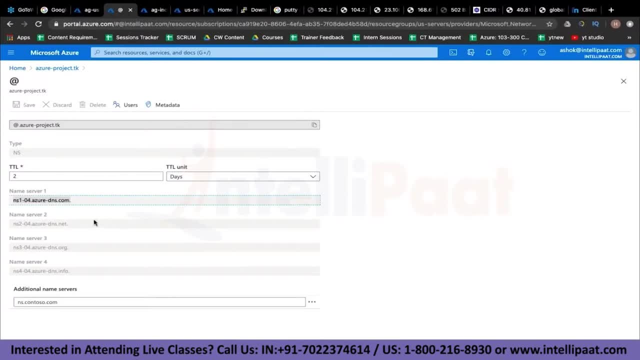 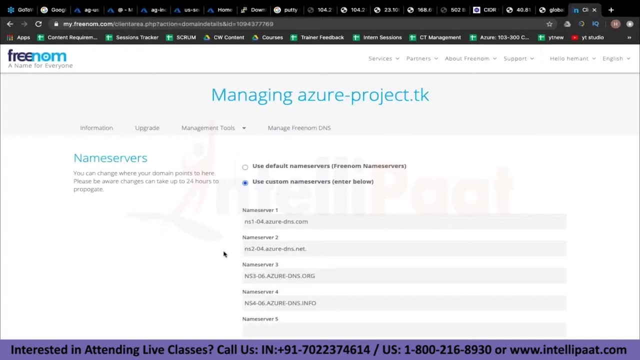 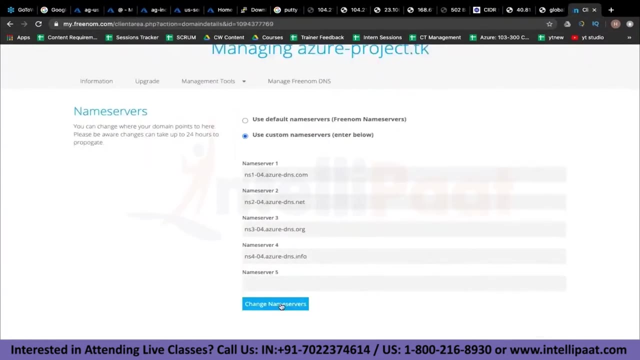 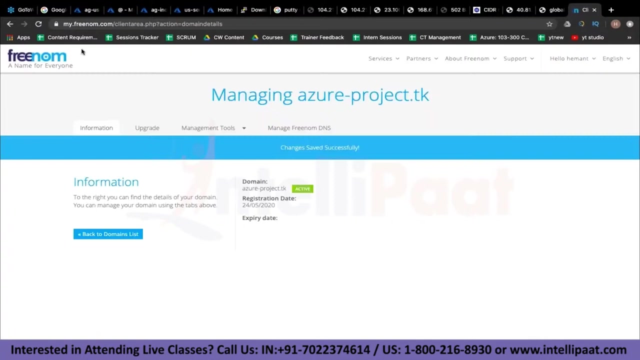 are there with the new ones, and that should be it. that's about it: how to configure your domain to basically connect. so let's copy it one by one. okay, so now just click on change name service and that's it. that's all you have to do on the Freenom website. okay. 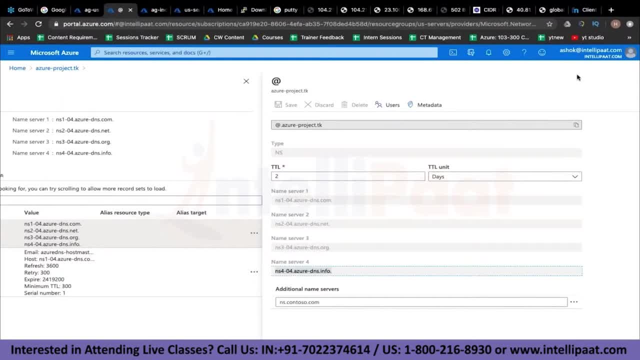 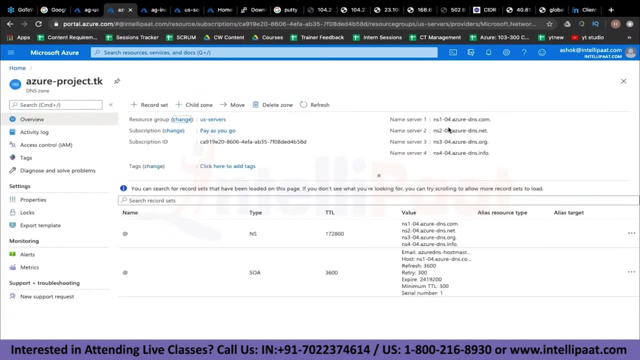 now come back to your DNS zones over here, and now what you can do is just close this. okay, now you just have to point your DNS zone to your traffic manager. so just click on record, add a record, set and this: let's configure it to be CNAME and it is the global traffic manager. 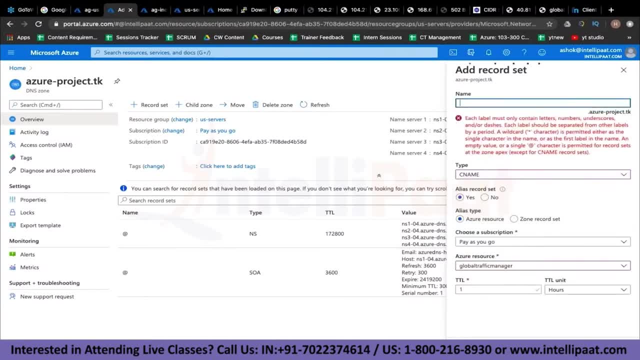 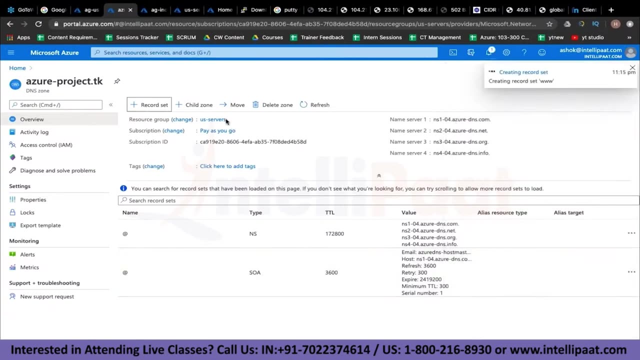 that we want to point on. okay, let's click on OK. so here we have to enter something. so that's a blue double W and let's click on OK, okay. so with this our record set has now got created, and it will take like a minute or two, or sometimes that even takes 24 hours, to basically make a 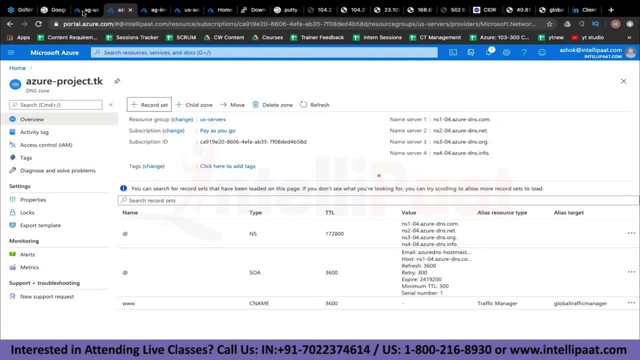 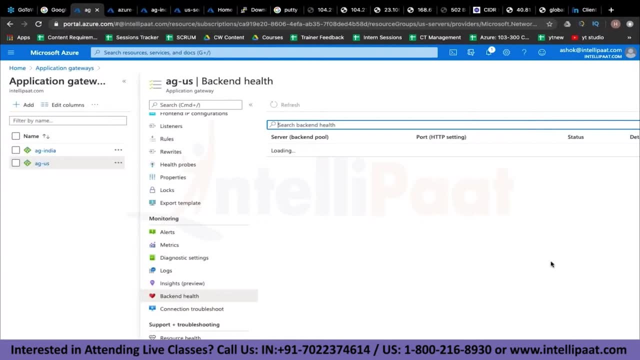 change in the DNS server, so we'll check that. meanwhile, let's come back to my DNS server. next one is the DNS server to our application gateway. check the back-end health now and let's see if this has loaded great. so now it is showing us both the 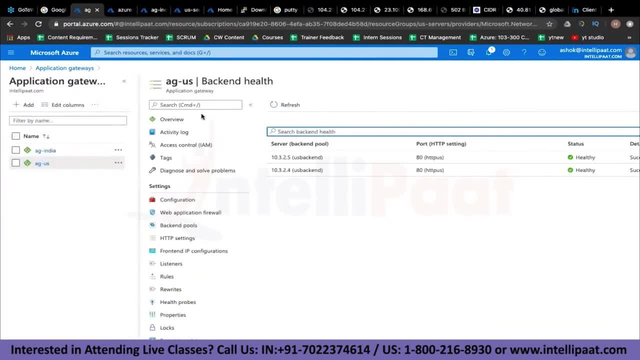 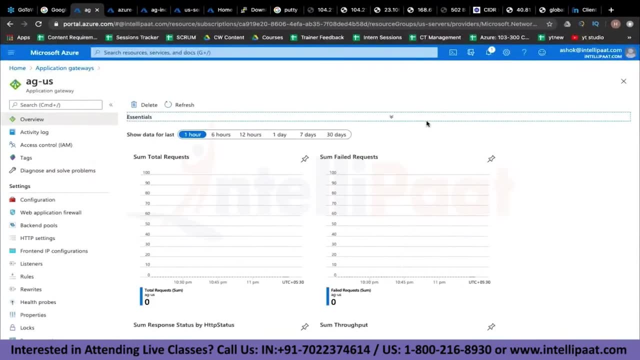 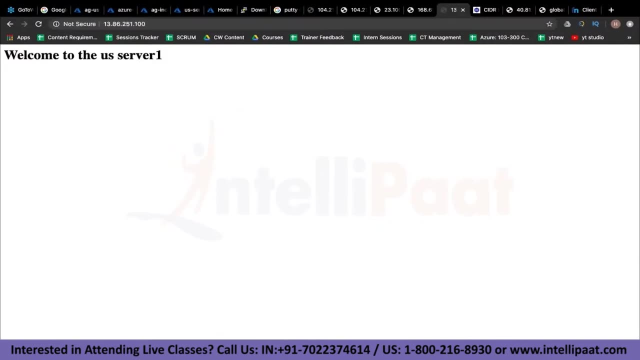 us backends right in the application gateway of us, and now, if we go ahead and try to connect to it, this is the ip address. great, we are able to connect to the us servers and we can see that it first connected to the one one, then the second one. so let's copy. 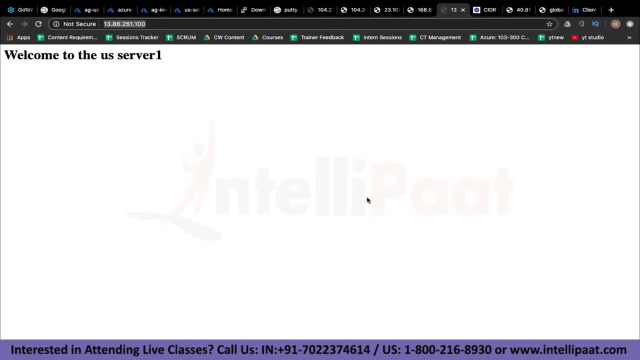 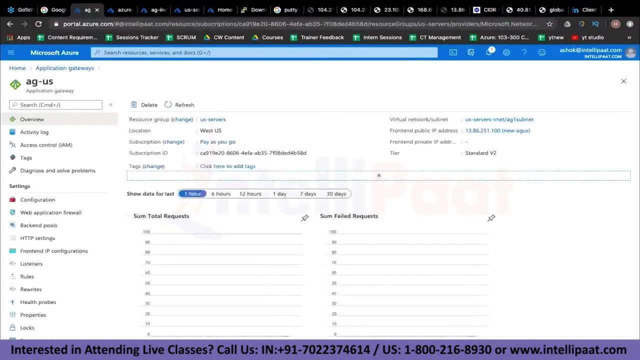 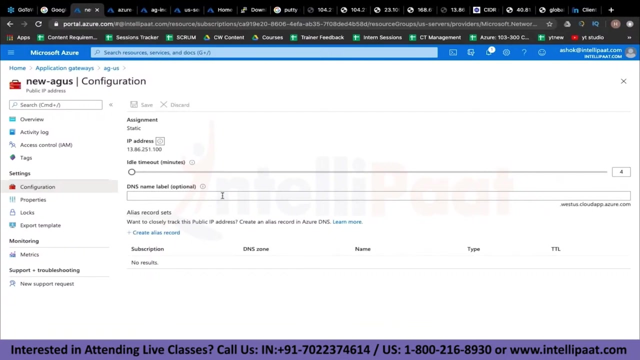 this and let me give it to you guys so you can test it out. now what i'll do is, on this application gateway, the ip address that we have just got, let's configure that to have a dns name. so go to configuration. this would be ag us. 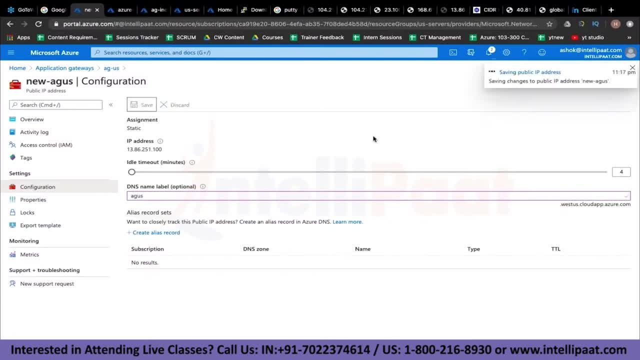 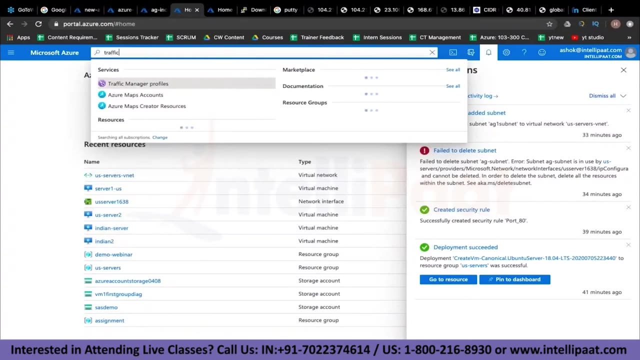 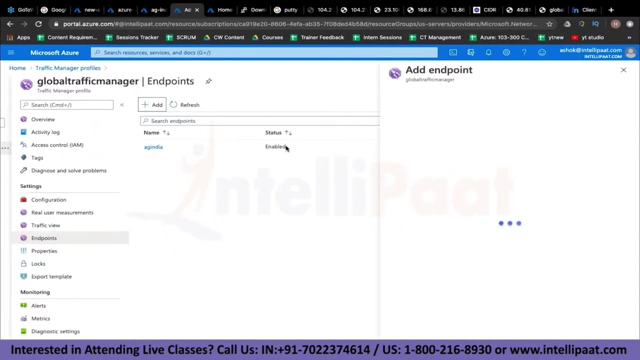 so it's available, let's save it and then, once this is configured, we can just go to the traffic manager now and add an endpoint for the us source. so we'll go to endpoints, add an endpoint over here and this will be for ag india. uh, it's a public ip address, the target resource type: 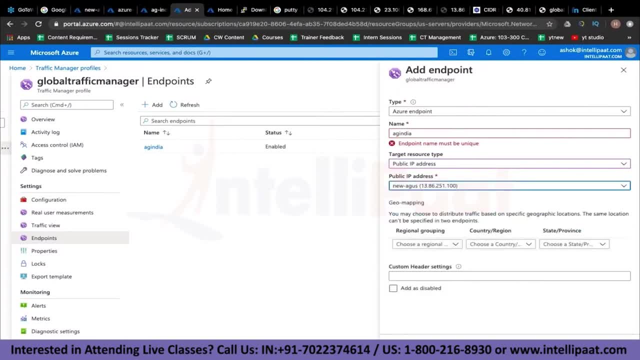 and we have to connect to new ag us click on add. okay, so again, we will have to do the regional grouping. so in this case, now anybody can connect, right, so any, the whole world can connect. and if the whole world is connecting, uh, sorry, this will not be ag india, this. 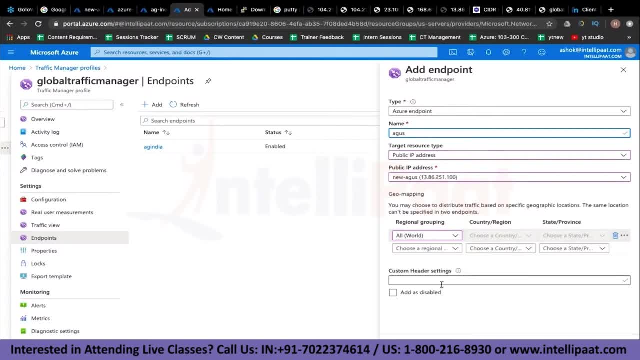 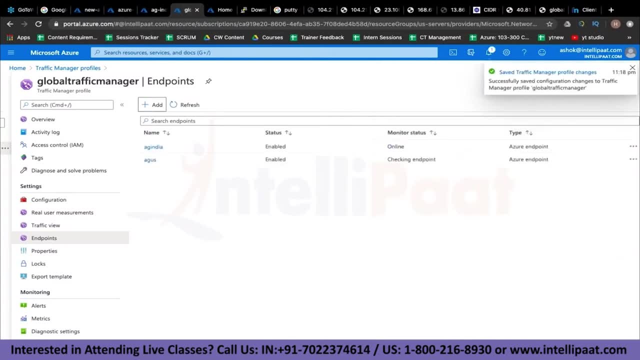 will be ag us, the whole world can connect and if they want to connect, they will be able to go to this endpoint. so now let's see what happens. so once let's make, let's wait for this to come online and once it is, we will just check. if you go to the 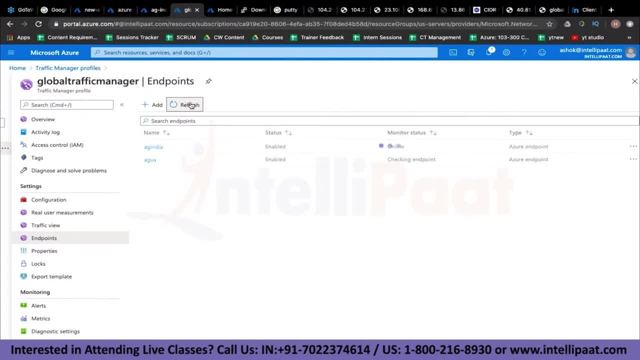 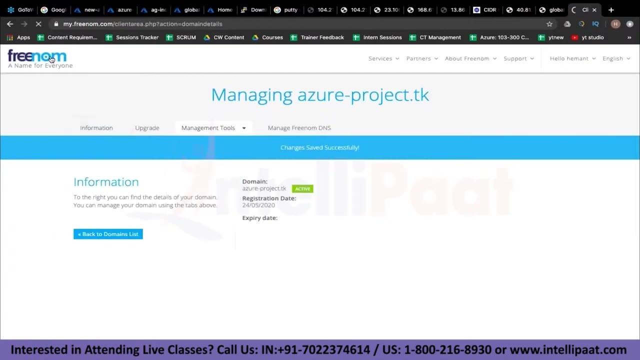 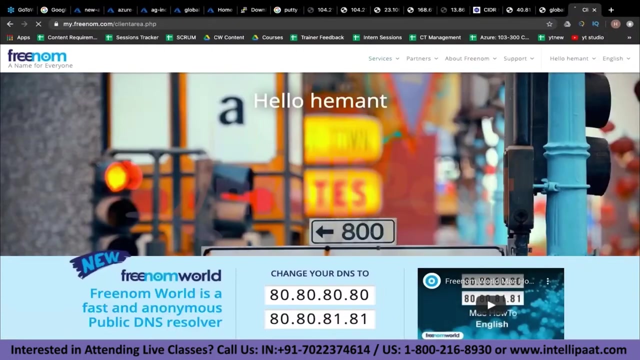 traffic manager, which server it is basically pointing us to, given the fact that this particular endpoint is for the whole world to access. so, once you have signed up, go to the home page, then go to services, go to register a new domain, and once you go to register a new domain, 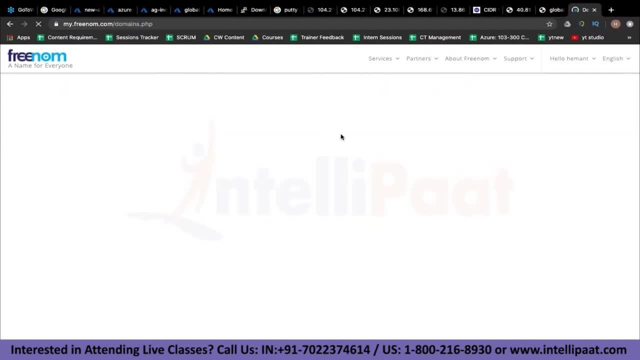 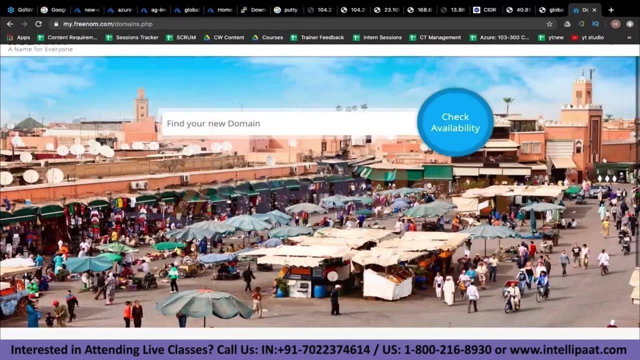 it will basically ask you which domain you want to go for. just enter the name over here and find your new domain. you will get a list of available options, choose the one that you want and then do the steps that i just told you. so that should help you. 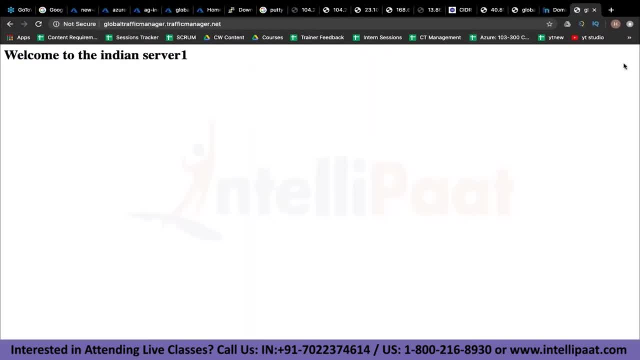 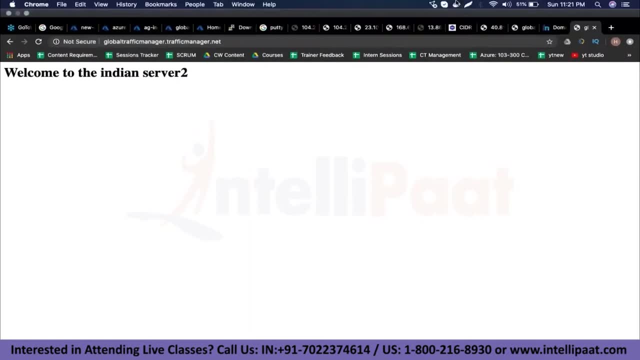 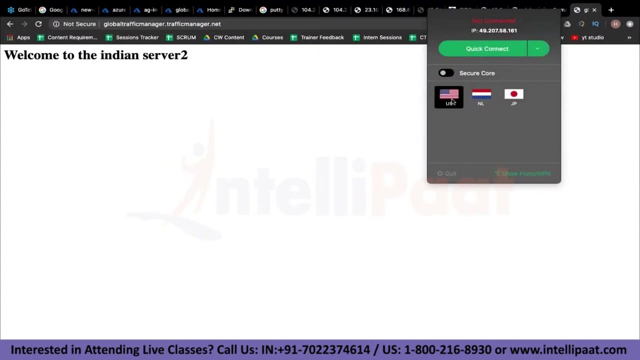 out okay, so i'm being routed to the indian servers- always great. now what i can do is i can connect to a us server, right, and then through vpn, and then we can see if it is working out for us. uh, so sometimes there are inconsistencies. uh, sometimes people in 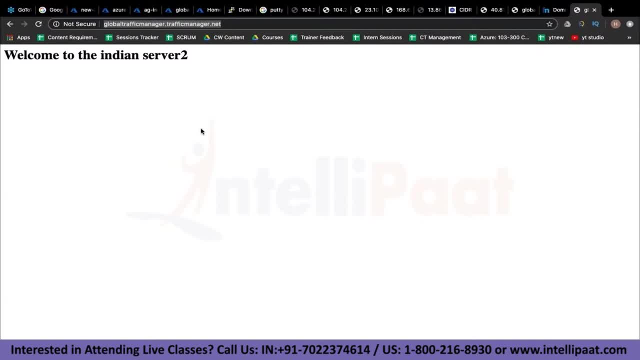 other regions might get redirected to uh the region, to uh some other region in the another uh service. but i think that is just because the service has just been started. if you leave it for 24 hours to work or 30 hours to work, it will start functioning properly and 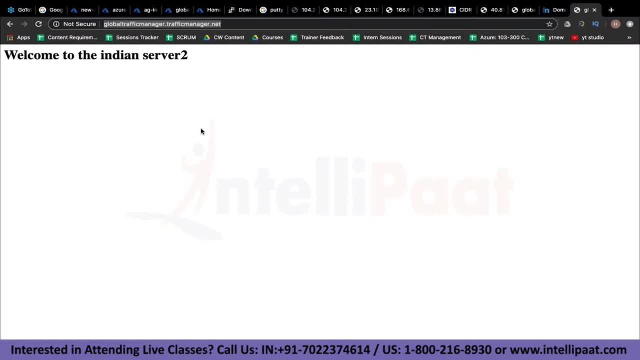 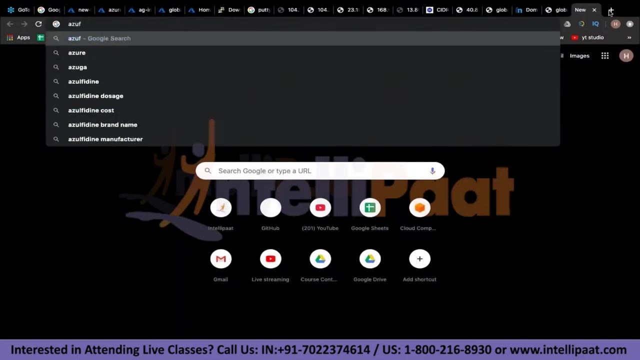 then everyone- i think 95 percent of us- got the right uh answer. right: people from india are able to access the indian servers and people from us are able to access the usos. great guys, so. and now let's check the final part of our project. so now, 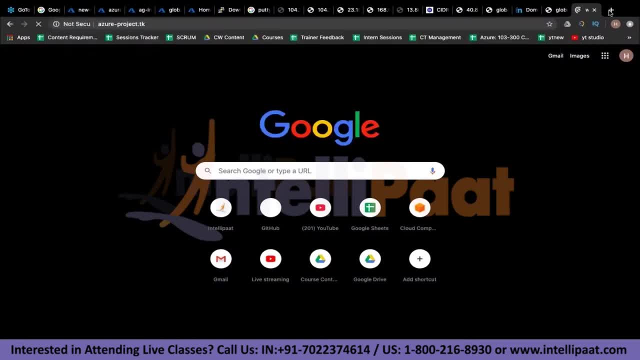 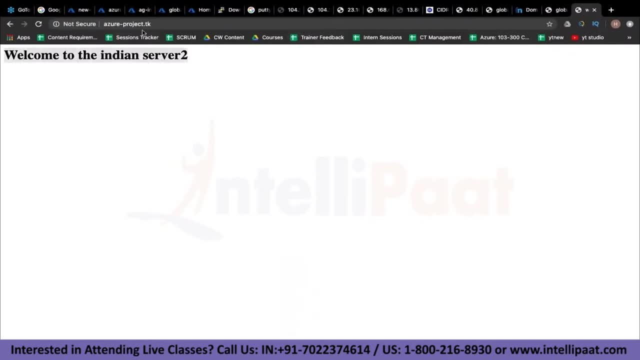 just let's go to azure hyphen project dot tk and let's see if that is working out for us. great. so now even the azure hyphen project dot tk url is pointing to our servers. write it out and let me know what the results are. so now the people from us also. 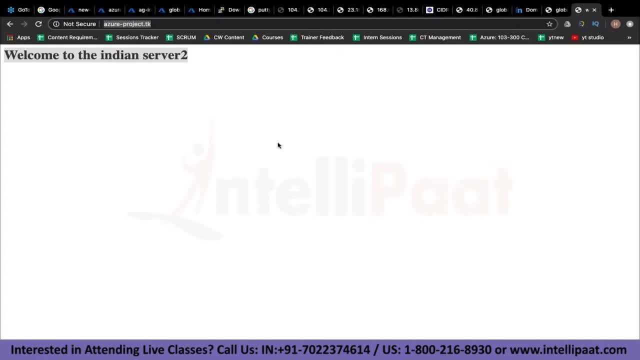 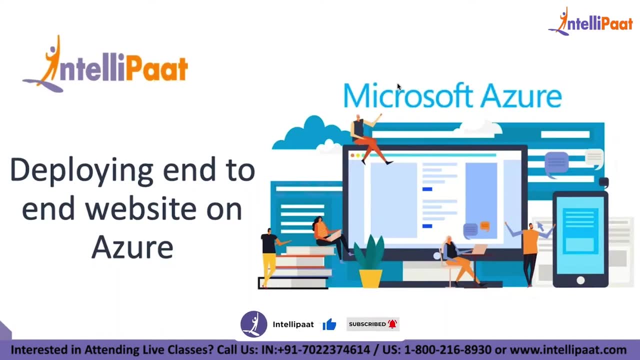 should be seeing the us page and indian one should be seeing from the indian page. so firstly, let's understand why azure is important, because i understand a lot of people over here will not even understand what cloud is right, what azure is. so let me go ahead and show you, guys. 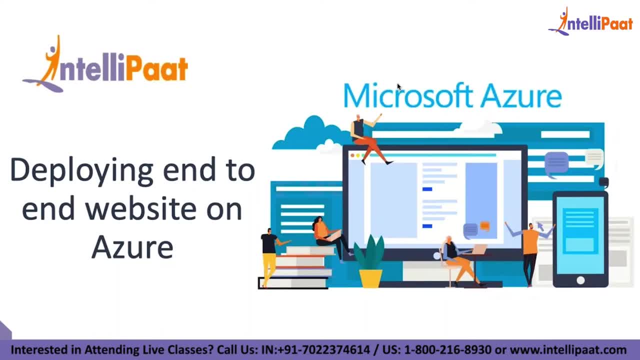 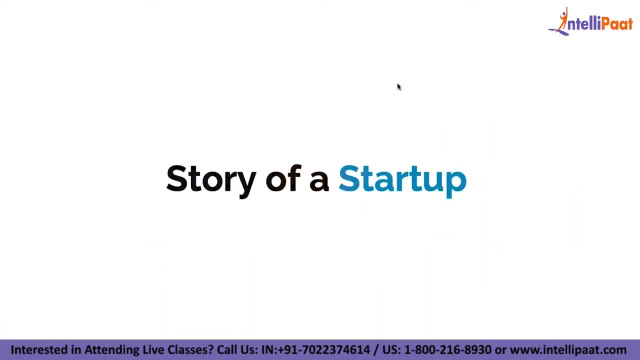 why is there a need of cloud? okay, and let's understand that using a story. so let's take the example, uh, wherein let's say: you guys want to start your own company. let's talk for from that perspective and then we'll understand why big companies are using uh cloud platforms, like azure today. 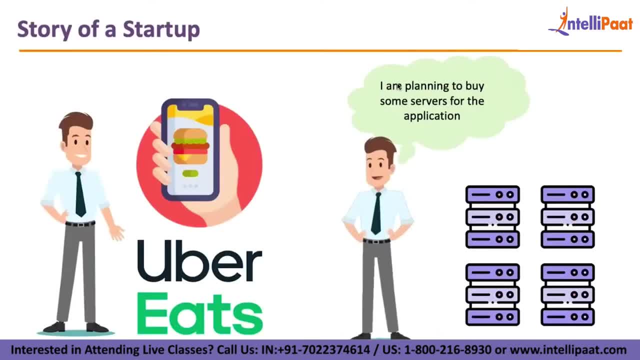 all right. so let's say you're a guy who just wants to open a food platform. let's say you're the food platform that you want to open is uber eats. okay, so if you want to open an application like uber eats, uh, what is the first thing that you have to do? so, obviously, first of all, you will. 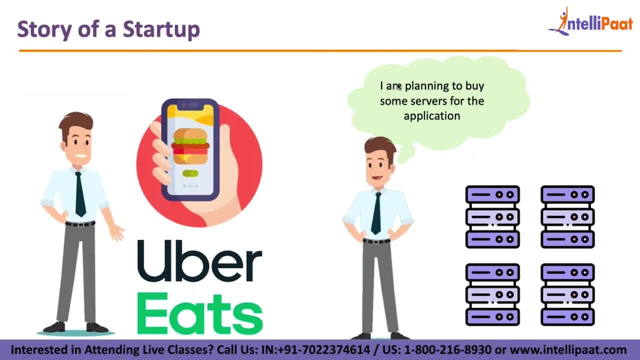 have to have an application right which basically you will be developing and which will basically work right. so let's say, you hired a team of developers and you've done that. so now your application is ready and now the next step is basically making it available to the world. right, making it available. 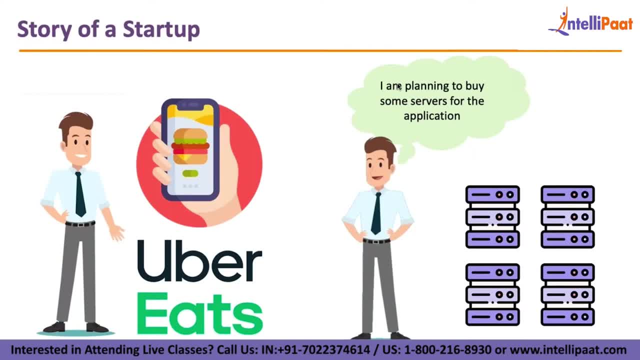 on the internet. so how will you do that? so for doing that, guys, first of all you need to host that application on a server. okay, now, when you're starting small and let's say there are four or five people who are going to use your application, you can do that using 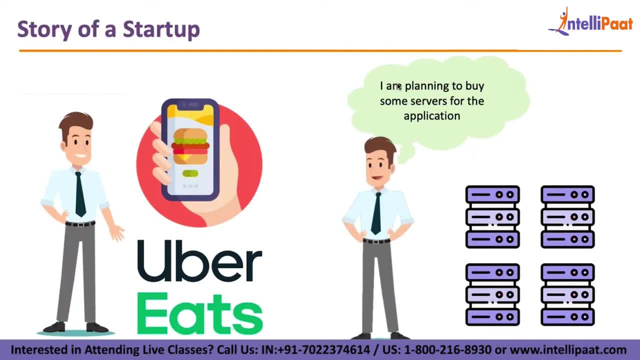 your own laptop as well. now, when you're doing it using your own laptop, let's say you have developed the application right and now you want to host on the internet. so what you do is you basically run that application on your laptop, you connect it to the internet, right? 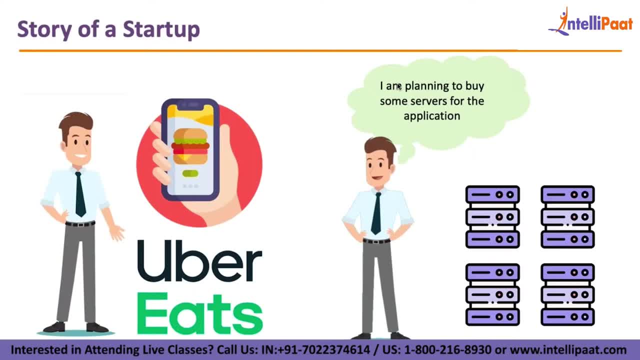 and obviously there are certain other things as well that you would need. for example, you would need a static ip of your laptop, which an ip which is not going to change any time, right, and at the same time, you will also need 24: 7 electricity so that your laptop will be. 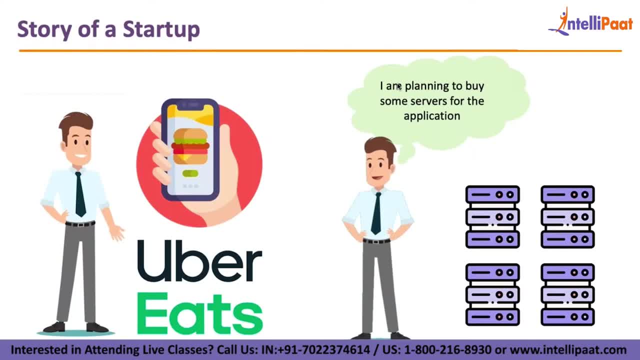 able to run those applications on the internet. so this is going to be the first step in making sure that your laptop never shuts down, right? otherwise, if your laptop shuts down, the other people will not be able to use that application. okay, so, guys, this would be the basic setup that you would need. 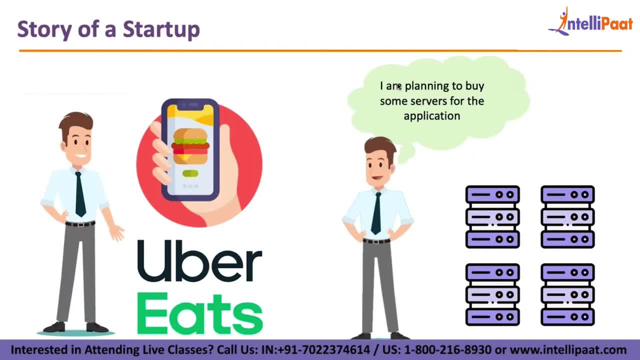 to host your application now. let's talk about a scenario, uh, wherein you know, your application becomes a hit overnight and now some thousands of users are using your application. now, obviously, your laptop will not be enough, so what will you have to do? my application is actually working. a lot of people want to use my application and 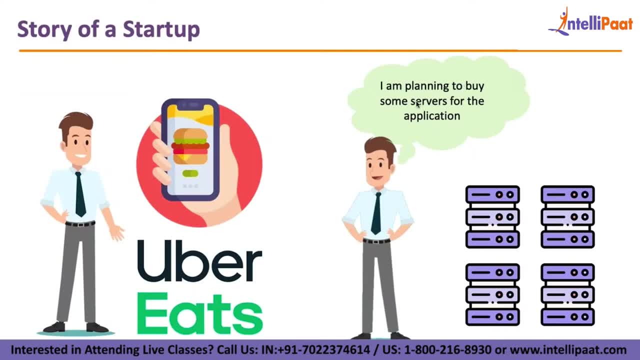 you know it is going to be a success in the future now. so what you do is it take a loan from some bank, or you take some amount from your savings and then you basically buy a set of servers. okay, so those servers take around two to three. 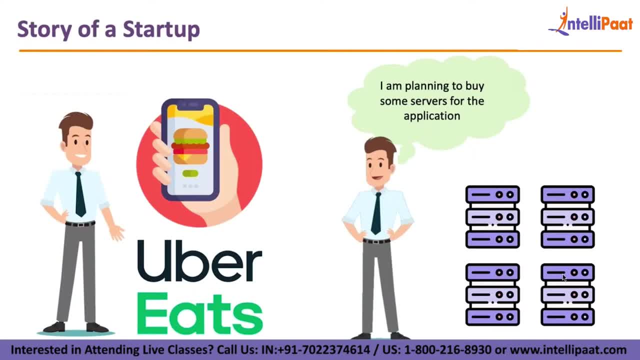 days to basically get delivered to you. then you basically set them up. for setting them up again, you know you need a team which can basically install the required software on it. then you need a place where you can keep these servers. so you rent some apartment, put those servers over there, you know, connect it. 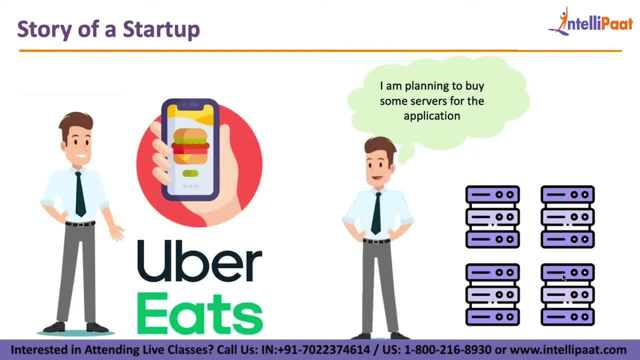 to a power backup kind of a facility where, even if the electricity goes, there is a generator which is going to power up your server and at the same time you basically also contact a service provider and an internet service provider which is going to give you good internet to your servers, seems. 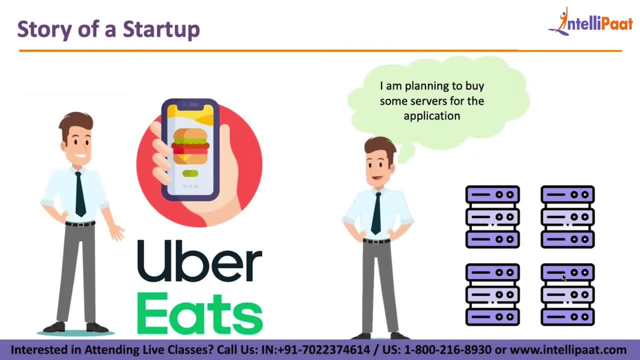 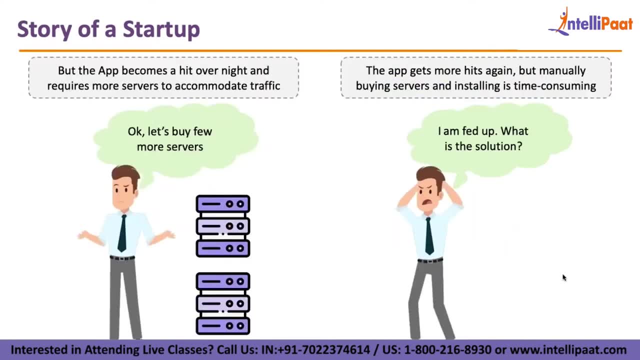 everything sorted right. so now you're in a situation where you have invested a huge chunk of money on your application right, and now you have made it available on the servers where thousands of people can access it. okay, now the application again becomes a hit overnight. and now 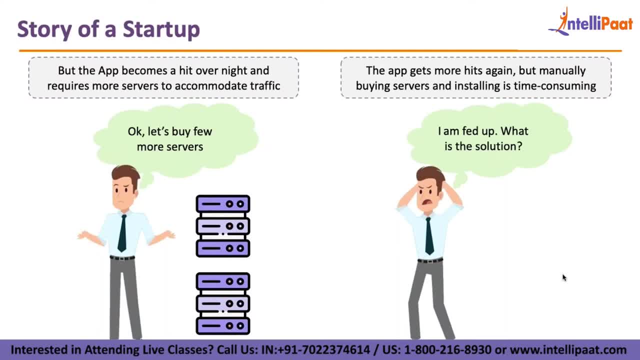 there are more customers who basically want to access your application, and now the servers that you bought they're not enough. so what you basically happens is you get to know: okay, so more customers are using your application now and now you can get more customers because, obviously, the servers that you have 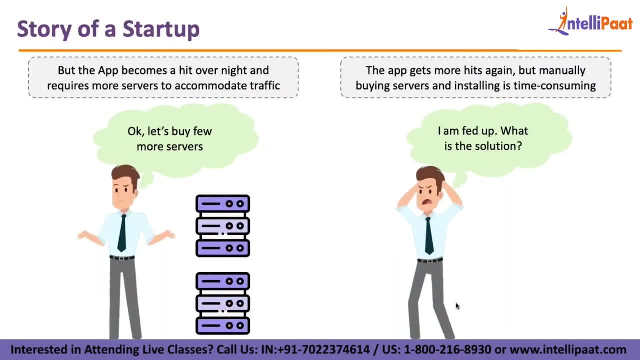 currently they're not giving you the correct, the right kind of performance that you need. so, again, you have to invest some money now. take one thing into account, guys: that servers are very expensive. at the same time, you also entered a place. you are giving money for the internet connection. you are giving 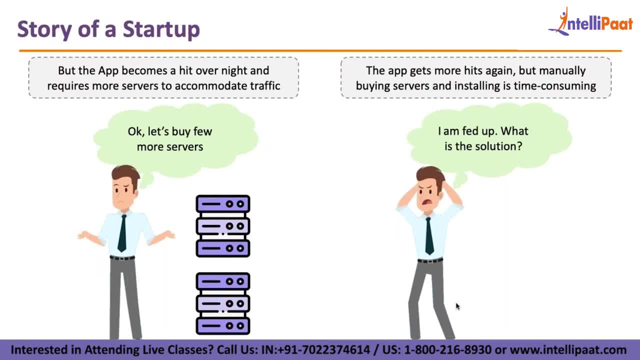 money for the electricity. so there's a lot of investment required over here to make your application available online to hundred thousands of users or even a million people. to make your application available online to hundred thousands of users or even a million people. right and obviously, because you know you have just started out. you are not. 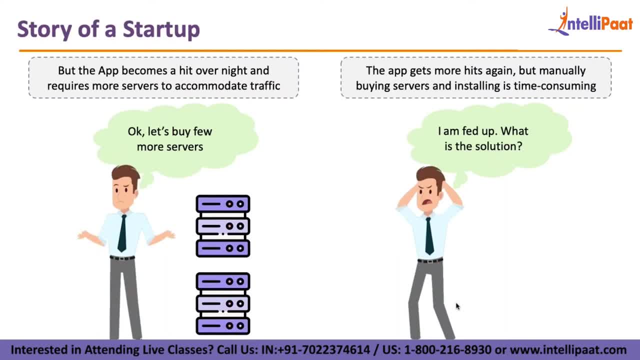 getting the kind of money that you are supposed to do, because you are also doing marketing for your application. you're also giving a lot of discounts on your application, because of which you're not getting the right right kind of revenue in, right. so what should you do? so, as and when the traffic will grow? 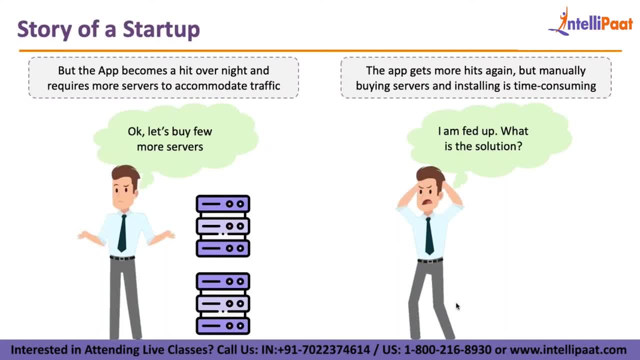 again and again. you will have to buy more servers and that will require more investment from your site. so you get fed up of the solution of of this particular situation and now you're looking of ways to basically solve it now. if this kind of situation arose before the year 2006 or 2005, well, you 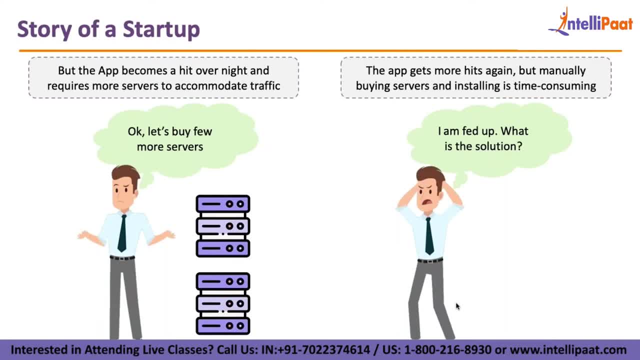 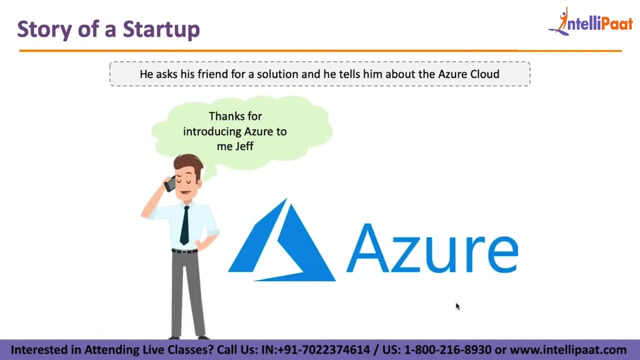 didn't have any other option- that to shut your company or take some loan from a bank and pay the interest also to the Bank. while you are you paying, you know the amount to them right. but now, with cloud providers such as azure, such as aws cloud platform, this has become very easy. so, what is this cloud platform and how? 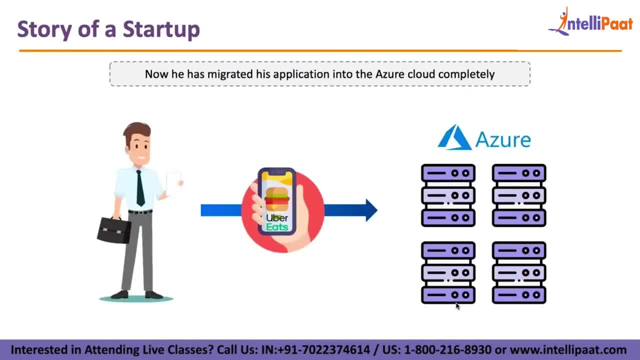 is it going to help you? let's understand that. so, guys, with a cloud platform, what you can do is you can rent infrastructure right. so now let's say you have an application which is ready and you want to make it available to the world. so what you will do is you can basically, you know, go to as your and you. 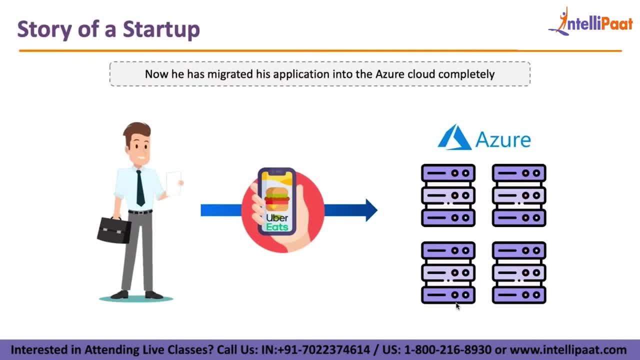 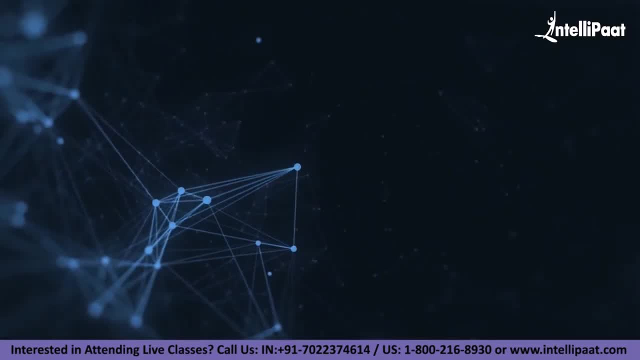 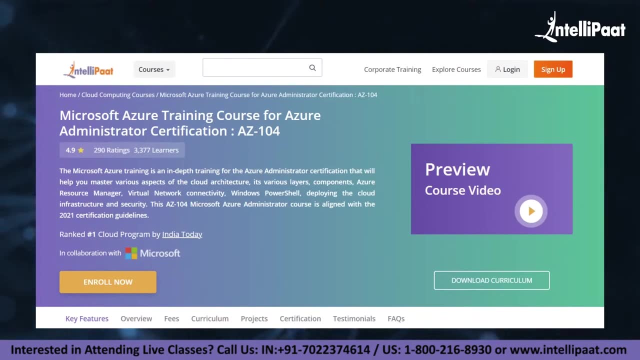 can just tell them: okay, you know what I need: 32 GB of RAM of servers and around 16 core of CPUs. just a quick info, guys. Intellipaat provides Microsoft Azure certification training in partnership with Microsoft, mentored by industry experts, the course link of which is given in the description below. now let's. 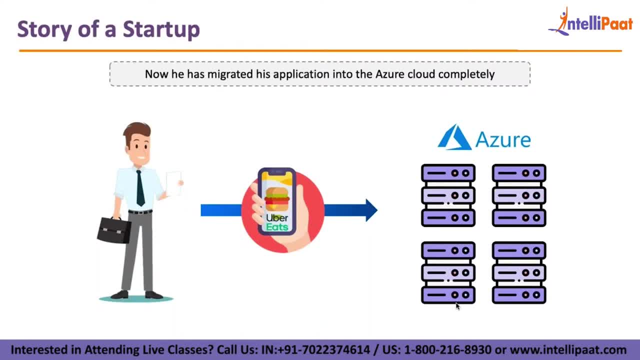 continue with the session. right, and I want 24: 7 electricity. I want that server to never go down. is that possible? so, as you people say, yes, that is possible. all you have to do is monthly. I just have to pay the rent for our servers. we will manage all the electricity. we will manage all. 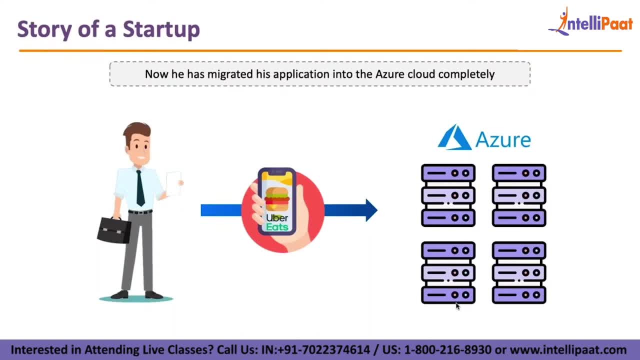 the internet connection. we will manage everything which is required from the hardware perspective. all you have to do is take care of our application, which you're deploying to the server, and nothing else, and in lieu of that, you just have to pay the rent of the server that you are using now, let's say after one. 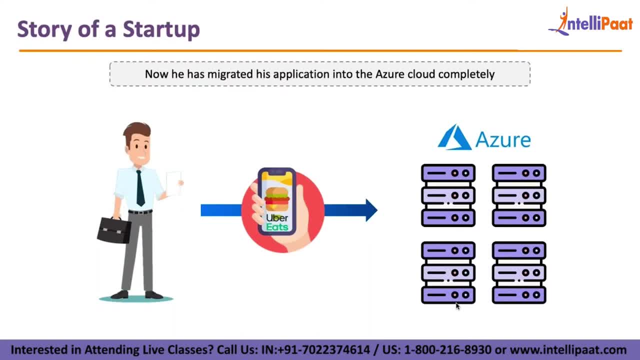 month you do not require the servers anymore. so you, there is no security that you have to pay, there is nothing you have to. you have to pay. just pay the amount that you use the server for and that is about it, that we require nothing else. at the same time, let's say, tomorrow you need 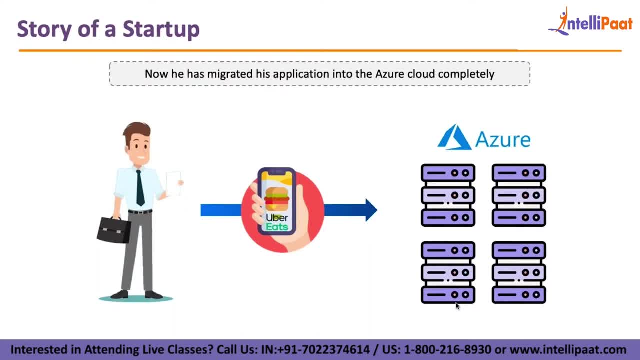 more servers that you want to add while you know your customers are growing. so all you have to do is take some more servers on rent and apply to your existing fleet of infrastructure and you're set, and it should hardly take two to three minutes to do this right. and again, the response to that is always a 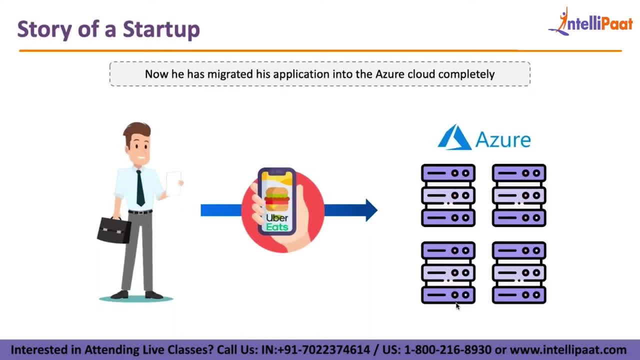 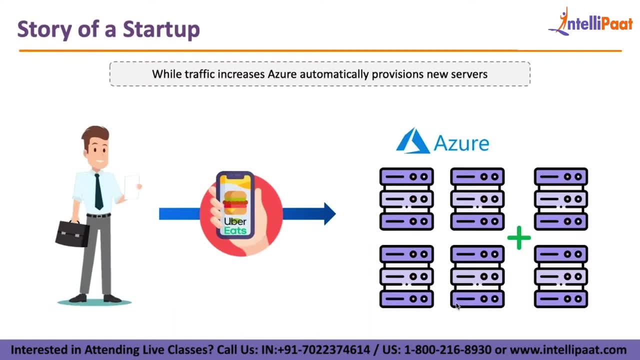 SUBSCRIBE to my YouTube channel so I will see you in the next video. so, thank you so much. you just have to pay the rent of the servers that you are basically going to use. okay, so now with this, uh, they also give you a feature wherein, let's say, that load increases on your application, the 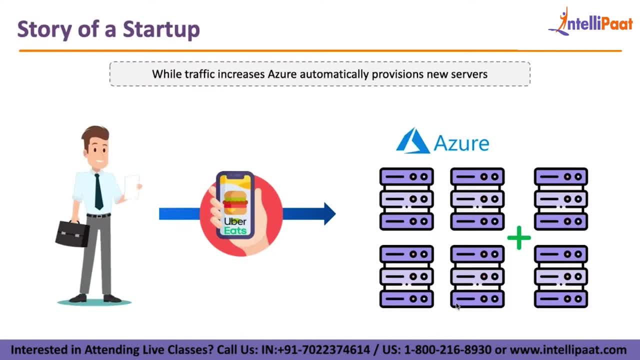 cpu usage of the servers which are hosting your application. it increases, so automatically new servers will be added to your fleet and even when the cpu usage goes down a particular number, it can also start removing servers from your fleet right or removing servers from your infrastructure, and this is what is called as auto scaling, and with this you never have to now worry. 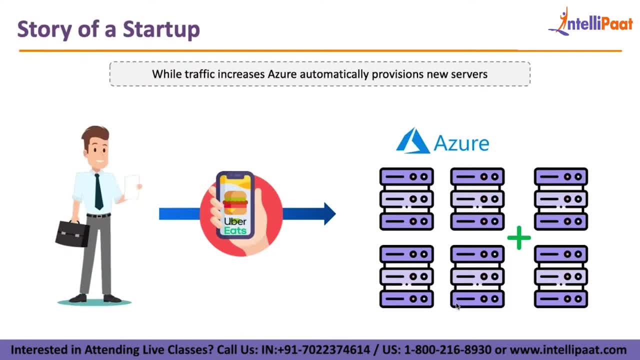 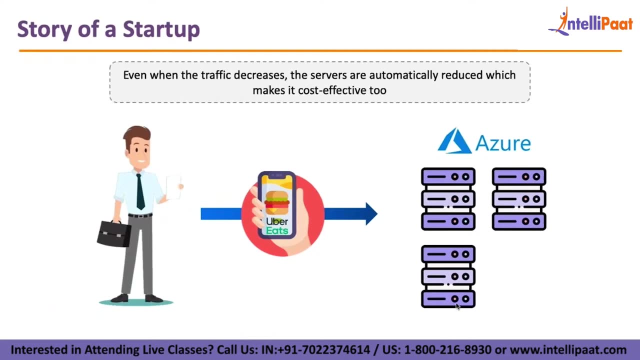 about how many servers you need, how many people are there on your website. why? because everything is being managed automatically and, at the same time, you do not have to buy servers now. you can just rent them and use it as long as you want them, right? so this came to. 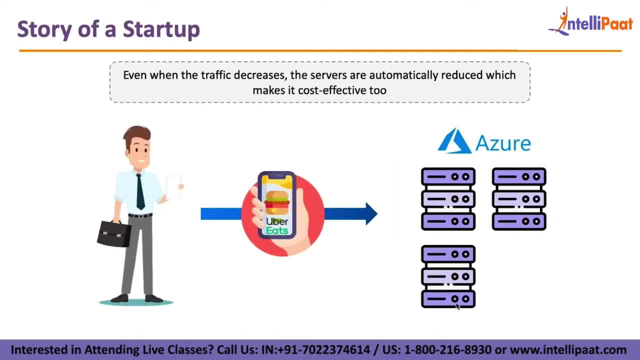 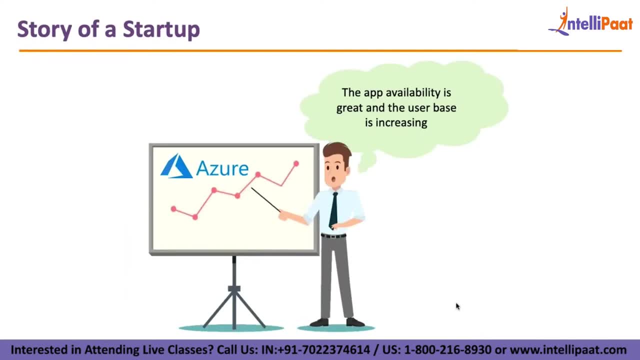 be a very good deal for you, and that is exactly how millions of companies worldwide have now shifted to cloud. why? because azure is going to azure, or aws, or any other google cloud platform for that matter, is giving you servers on rent. rent, all right, and the rent is as low as 0.005 dollars. 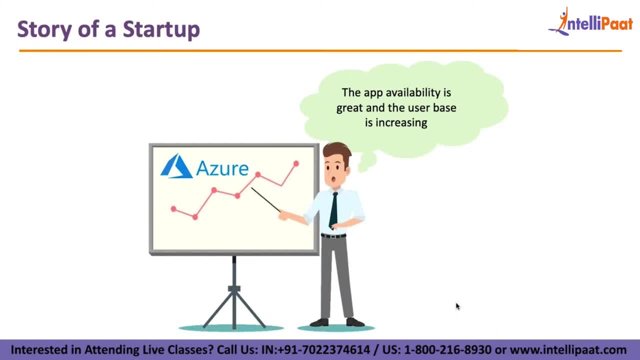 per hour. right, so that is how cheap the rent is for the server that you're basically trying to deploy. and with this, uh, you know, the internet is managed with them, the. even if the hardware outdates, let's say tomorrow, they will upgrade your hardware for free. you don't have to pay them. 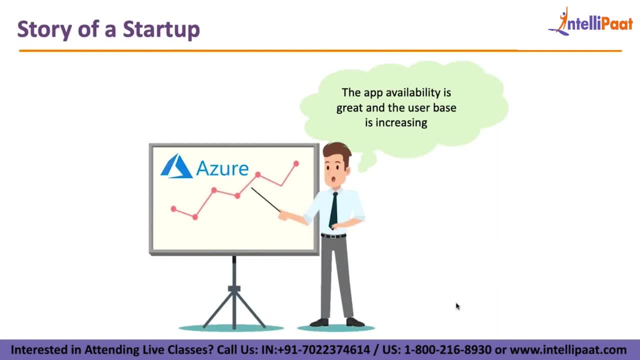 anything extra other than your rent. they are going to manage everything and because of this your usage is going up. why? because now your application is available all the time and at the same time, the traffic also is being managed automatically, so that the new server added to your fleet and i 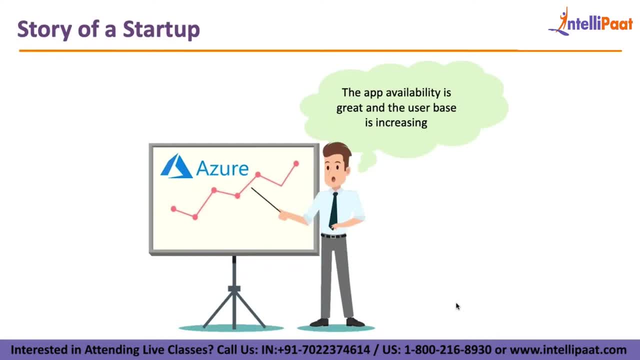 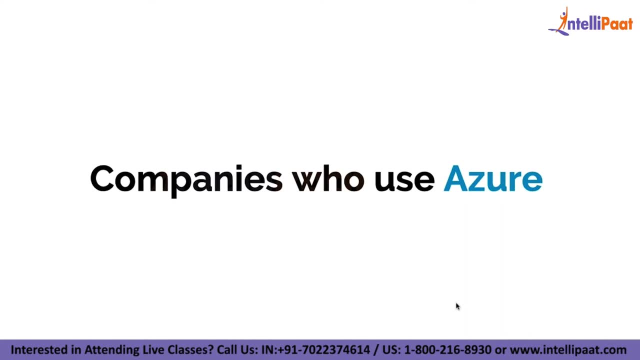 removed for your fleet as and when the traffic increases or decreases. okay, so this is the story of a startup, why it was using azure. now let me show you some of the companies who are using azure today, right, or using a cloud platform today, specifically microsoft azure. so these are all the companies who 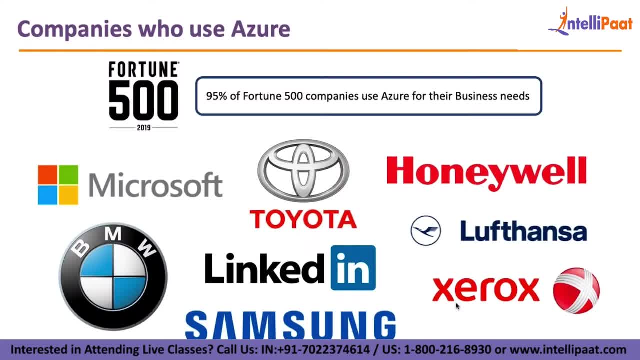 are using microsoft azure for all kind of needs of infrastructure, right, and they just have their software over it. so companies like toyota, honeywell, lufthansa, linkedin, samsung, xerox, bmw and even microsoft itself. so any microsoft website that you go to is also hosted on microsoft azure. 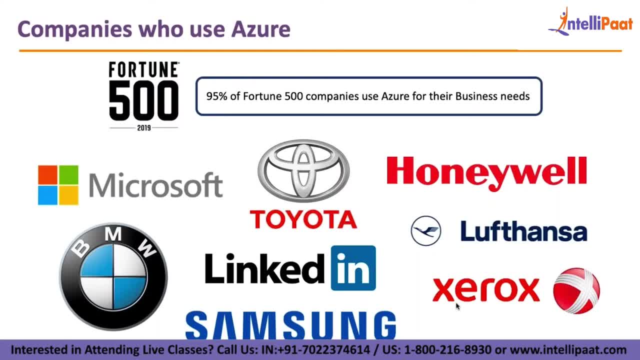 right. so all these companies are on azure for the very same reason that i just explained you. first thing is cost effectiveness. second thing is distribution of work, because now you don't have to have your own team to manage your servers and at the same time you also are can be reliable. 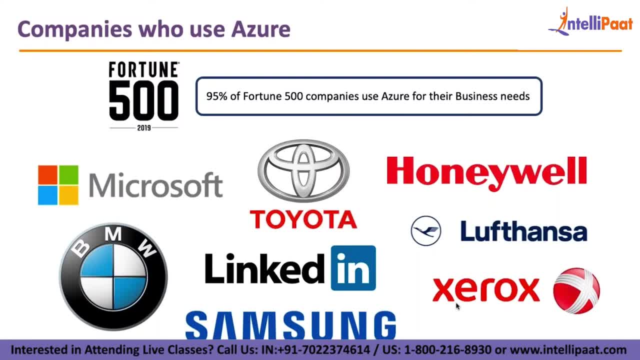 on the infrastructure which azure has given you, because it would have been a pain to manage the hardware. uh, you know a team which is going to monitor your hardware all the time. if you want to set it up all by yourself, okay. so now that we have understood what azure is, 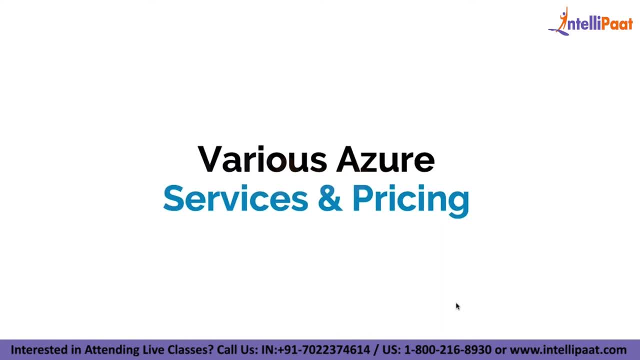 exactly and why we should use it. now we will move along and understand some azure services and its pricing. so suhas is saying: how much does it cost owning a server versus, uh, buying from cloud? okay, so so, as it depends on the size of the server, so let's say, if you uh, let's, let's compare the price. 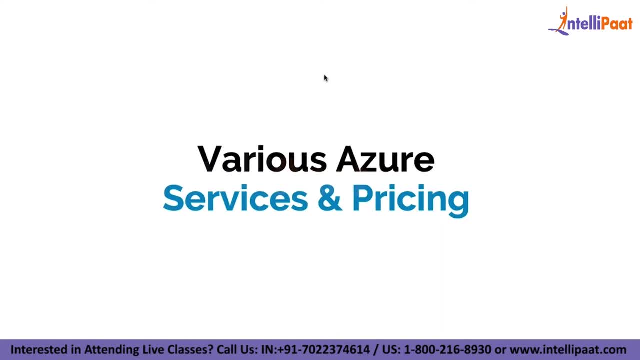 of having a pc today, right? so if you buy a pc with which has a very good gpu, right, let's, let's say you ATTI graphic card with an i9 core CPU which has around 16 cores, right, and a 64 gigs of RAM, which 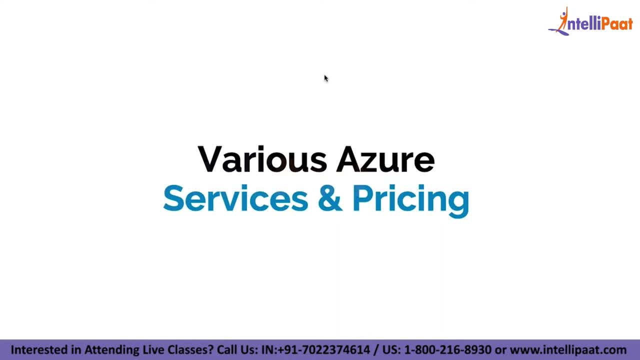 has around 3000 megahertz of speed. So this setup for just the CPU is going to cost you around 3 to 4 lakhs. and now this is a PC. Now imagine if you have to set up a server and this PC will now be. 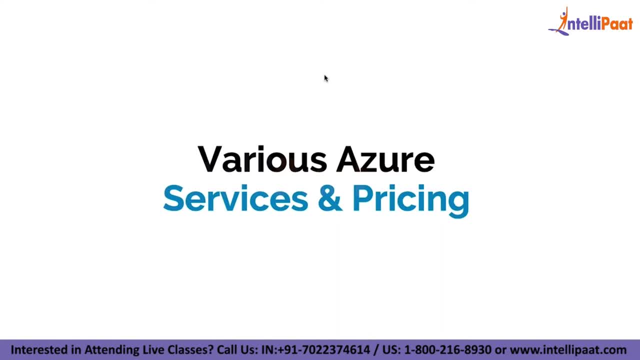 multiple times in the server rack that you have, which is basically going to cater to 1000-2000 people. So the cost of this setup is going to be around 6 to 7 lakhs per server rack right Now. imagine when your server hits 100,000 users or 200,000 users. this cost is going to increase. 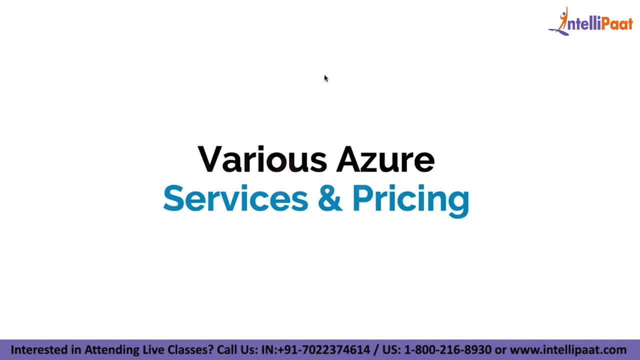 exponentially. Now, obviously, you will have to manage it according to the revenue that you are generating, right, but at the same time, the revenue will take some time to come in right, and at the same time, if your users are increasing exponentially, which is a good thing for you, though, 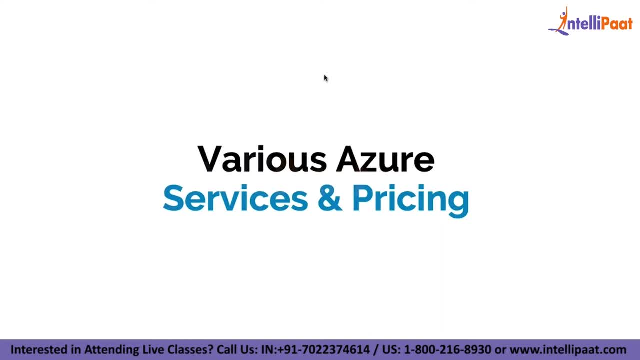 but let's say, if you are not able to manage the demand of the users, which is basically the infrastructure that you have, it again becomes a problem. Let's say, you have that kind of money to buy your own infrastructure, but with every increasing demand that infrastructure will take. 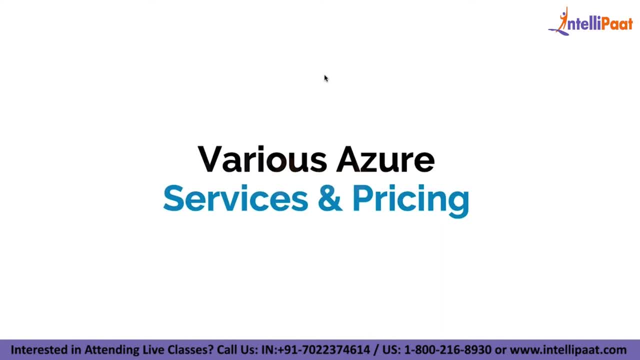 some time to come to your office. At the same time, you will also have to take a headache of managing or hiring a team of your own to basically manage these servers right. and obviously, when you deal with the problems that the team is facing, you have to also deal with you know what are the 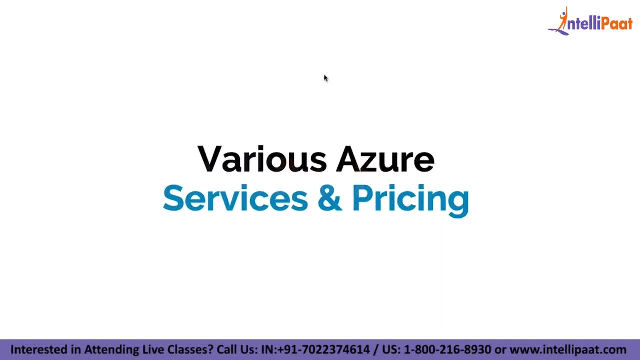 kind of tasks that you will be assigning them, etc. So it becomes a headache for you because you basically wanted to open a app which is basically a software. So not only you now have to manage the software, but you are also going to manage the hardware side of the hardware. 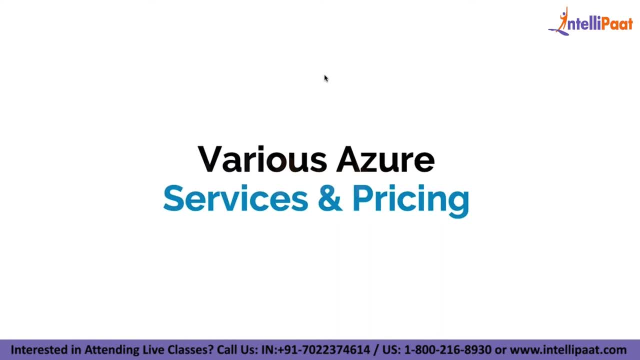 software, thus giving less time to your application, which probably, if you have spent more time on the app, you could have increased the revenue of your company. right, and that is exactly why, basically, companies prefer cloud providers. Okay, Santosh is saying: what about security charges? So, Santosh, 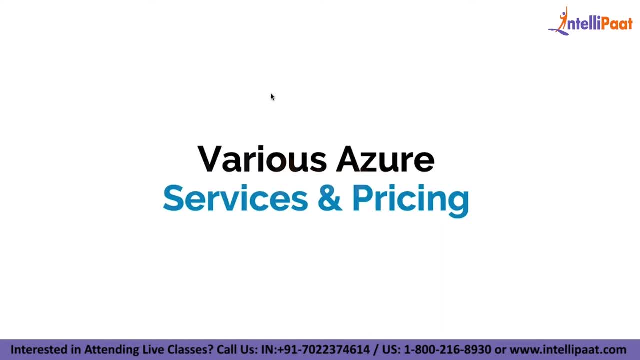 everything. you just have to include the rental charges. security from the hardware perspective, security from the perspective of you know if you're deploying a firewall on Azure so that firewalls foolproofness is all guaranteed by Microsoft. Okay, Now think about it like this. let's say you have your own application that you're trying to launch. 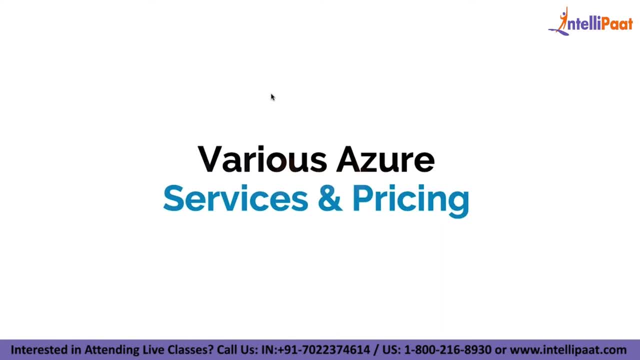 in the internet space. Now, obviously, the kind of security you know aspects that you can create around your application, the kind of money that you can invest around your application just for the security needs. whatever that money is, it's going to be always less than what Azure has. 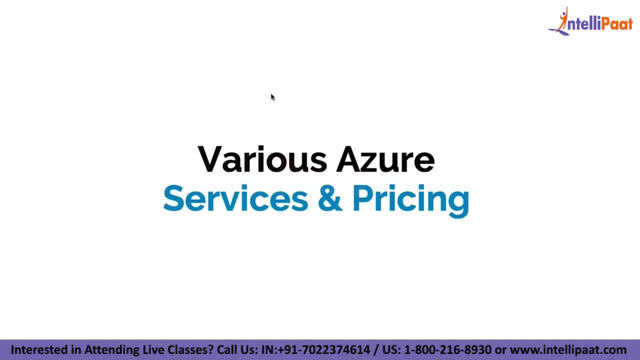 already invested on their infrastructure. given the fact that Microsoft itself is hosting the applicationBI, ought up and curt. Okay, do you want to add that? Are you totally correct to worry about security at the most Page and all of a sudden, everybody else is continuously obtains credentials for each and every service of theirs on Microsoft. so okay, so you can be, should that? if you are hosting your application on a cloud like Azure, it's getting best-in-class infrastructure and at the same time, you know the security best practices increasing. you will have to make sure that your application from the Considering is secure, that you've moved your applications securely, and it is not something that, as your can guarantee. but 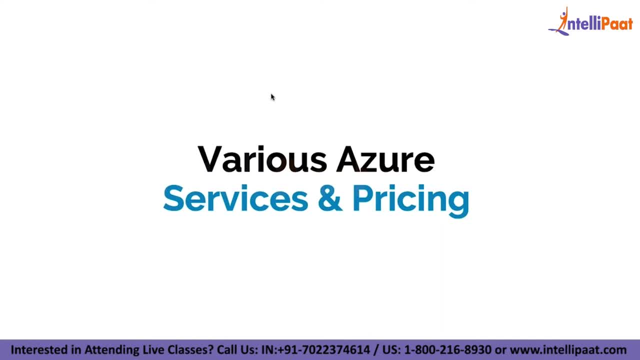 cannot be tampered with. that. there's something that azure will guarantee. i just told you about why cloud platforms are basically- uh, you know- preferred rather than owning your own infrastructure. now, why are we learning azure today? let's, let's try to answer that question. so, as you all know, 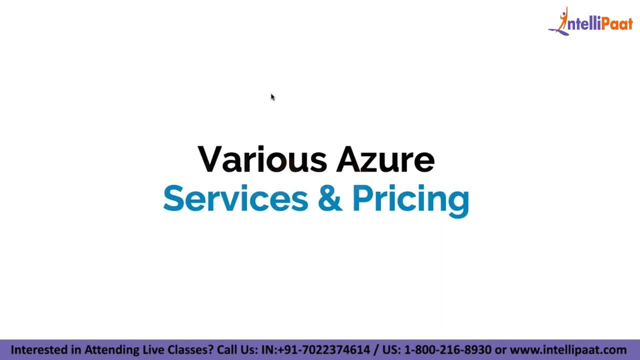 that amazon web services is the largest cloud provider in the market right now. right, and when i say the largest cloud provider, it has around 41 to 42 percent market share now. because it is the largest cloud provider in the market, that obviously means that there are more jobs, and because there 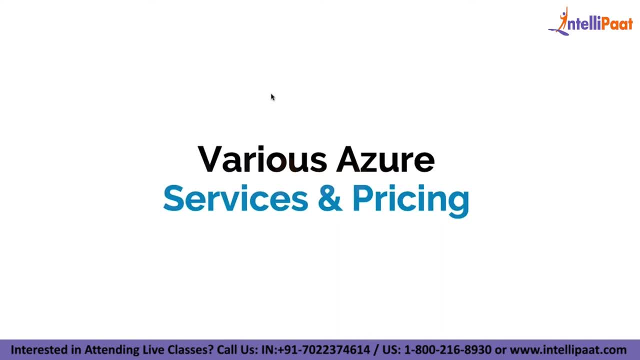 are more jobs, there are more people who are trying to apply for the job and hence more competition. when you talk about microsoft azure, it's the second largest cloud provider now. let's first talk from the market perspective now, because it's the second large, second largest cloud provider. 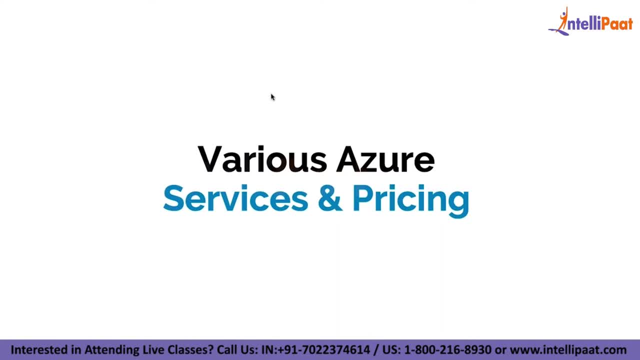 company companies which are using aws right now. they're also taking into account a secondary cloud provider for their infrastructure needs. why? because, let's say tomorrow, uh, you know, the whole of aws servers go down now. they do not want it to impact their own application. so what they do, 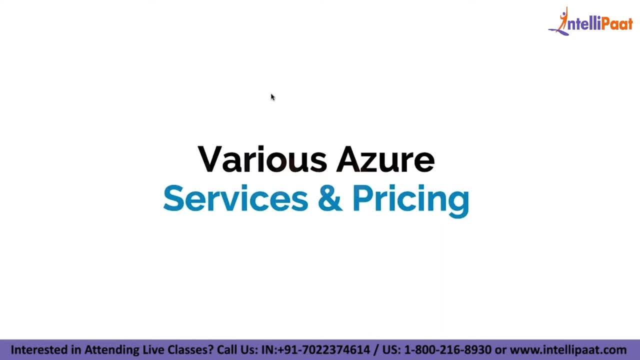 is they create a redundancy in place and what they do is they manage their servers on azure as well. right, and now they're using two cloud providers instead of one. this is from the market perspective, and that's why you can see the growth of the azure has been. 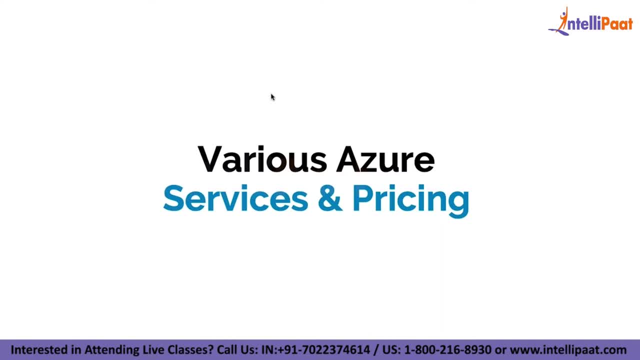 dramatic in the past two, three years. right, the kind of growth that aws has seen is less than the kind of growth that azure has seen from. uh, you know if you, if you take into account the last three, four years. at the same time, azure is a lot cheaper when you compare it with other. 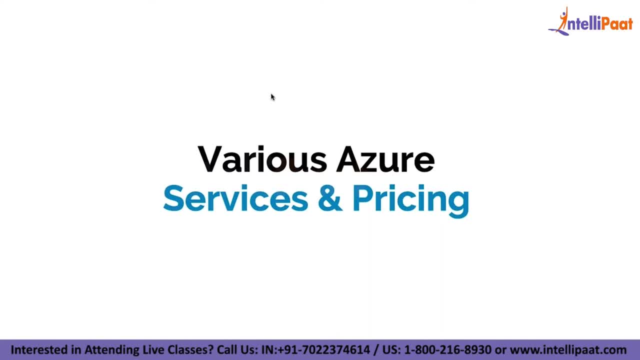 cloud providers and the sole reason for that is the microsoft products. so if you are using any microsoft product on your azure app, this is less profitable, so that's probably going to focus on class on, let's say, aws on google cloud platform. it is obviously going to charge you more than microsoft. 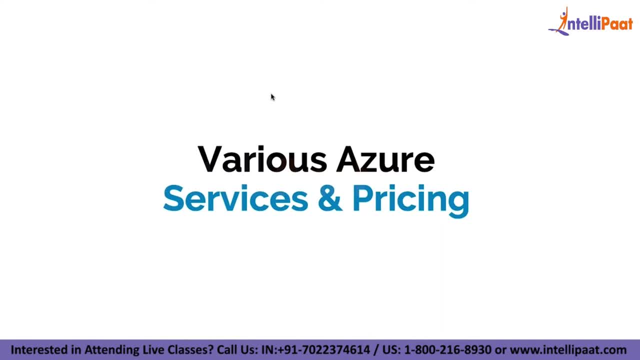 product that you get on azure. why? because azure is basically owned by microsoft, so because of that, even the pricing is in control and hence it becomes more cheap for people who want to use microsoft uh software. third thing is now because the aws is the largest cloud provider there is. 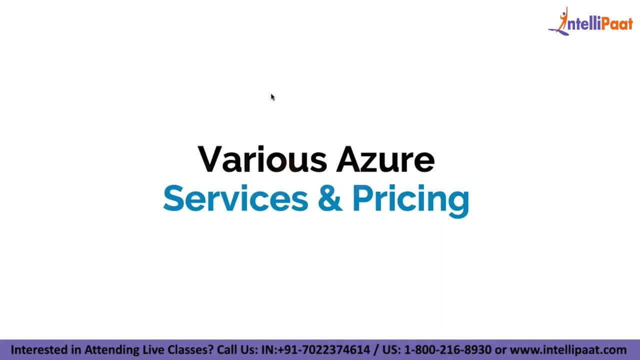 more competition over there. azure does not have much of competition but at the same time, since companies have started considering azure and because of the growth rate of azure that we have seen in the past three, four years, there's an acute shortage of people who are who? basically? 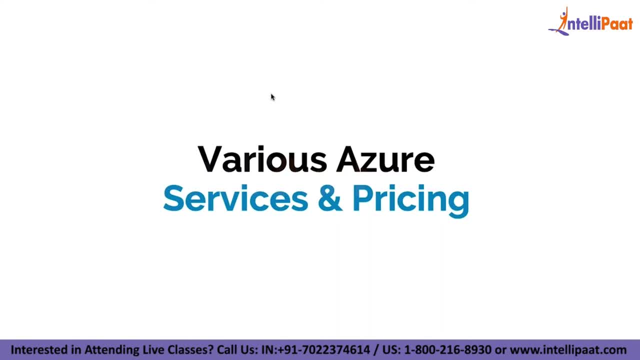 are certified in azure and, at the same time, know azure that well as well. nowadays, what is happening is people who know aws. they are the only ones who are also ılmış trying to control the infrastructure which is there on Azure in the same company, right. 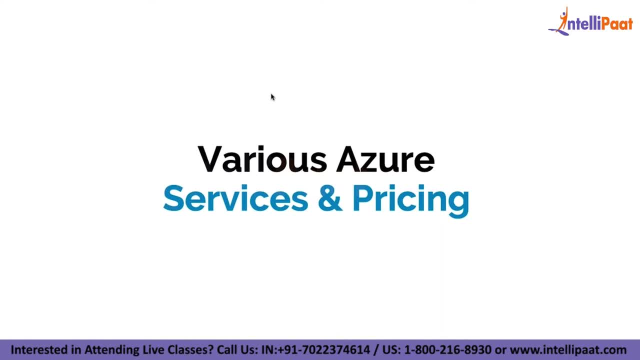 But that is not helping out because a lot of features are different between Microsoft Azure and AWS And now companies basically want to have a separate guy who can manage their separate cloud platform that they have. Now, obviously, if you talk about senior cloud profiles, 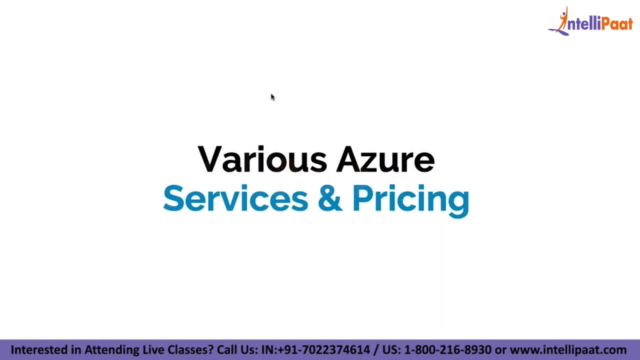 such as senior cloud engineers or senior cloud architects. Now, these guys, they are not just limited to learn only AWS or only Microsoft Azure. In the long run, when you see yourself you can actually, you will actually have to learn more than one cloud provider. 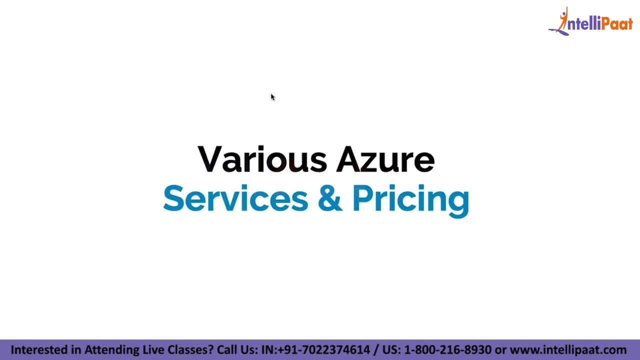 That is. some companies expect you to know both AWS and Microsoft Azure. Some companies expect you to know all the three- Microsoft Azure, Google Cloud Platform and AWS- as well, But when you're starting out with the cloud domain, it is recommended that you start with Microsoft Azure. 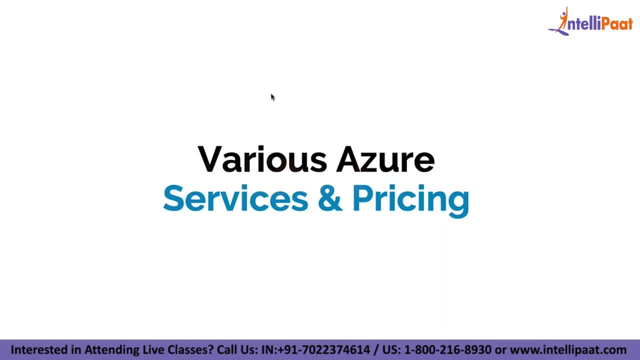 because it will be a lot easier for you to switch to the cloud domain because of the less competition right. And while you're also growing for the next level, the next level of profile that you want to go for, then you should also learn AWS. 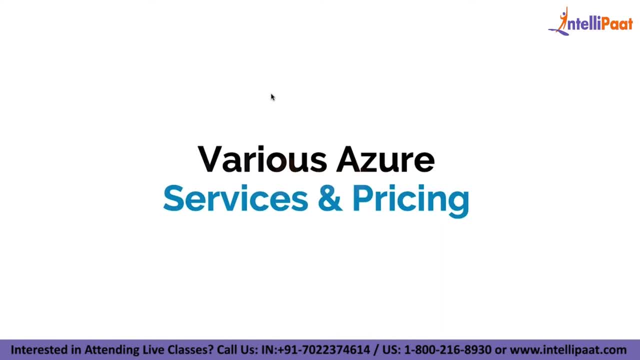 You should also learn Google Cloud Platform. Okay, when you talk about it from the features perspective. So what are the features that AWS is providing, which Azure is? not All the features are the same, but the way you implement them using the services. 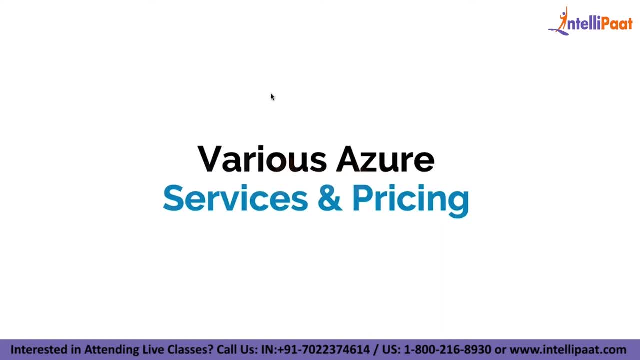 is different. right, The steps that you have to do to do a particular task in Azure is obviously going to be different from what you have to do in AWS, because they are two different companies. They have built their own product separately And obviously because of that, 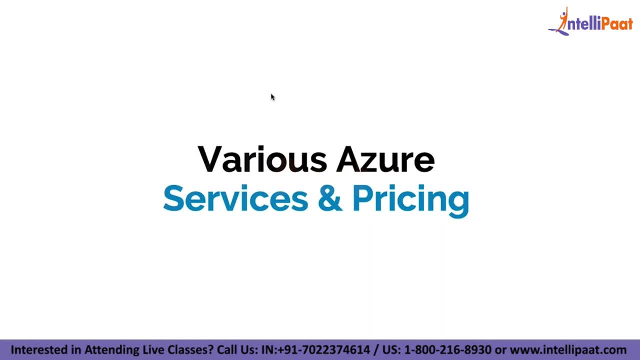 the way of implementation is also very different, right, So that is the only difference. But when you talk it from features perspective, both the cloud providers are neck to neck. They are giving each other competition in terms of the feature that they offer. 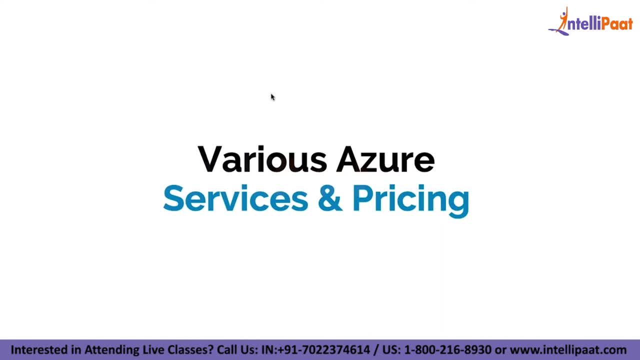 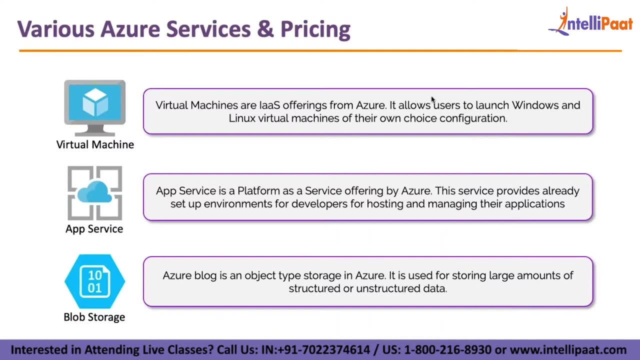 And because of that, all the features, or most of the features, are same. Okay, so let's talk about the most common service, which every one of you is going to use once you start using Microsoft Azure, And that service is nothing but the virtual machine service. 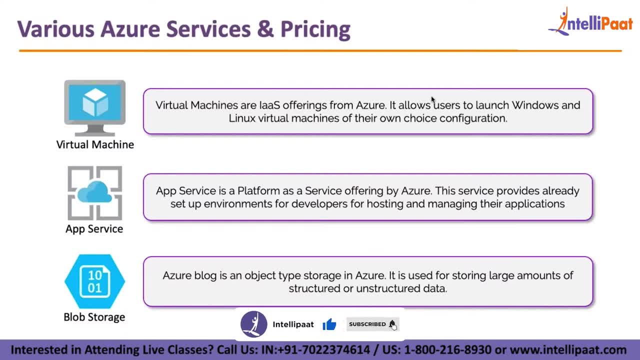 So, guys, the virtual machine is basically, it's an infrastructure as a service, or in other words, it's basically a server. So all that we have been discussing till now, even in the example that I told you earlier, was about using a server right. 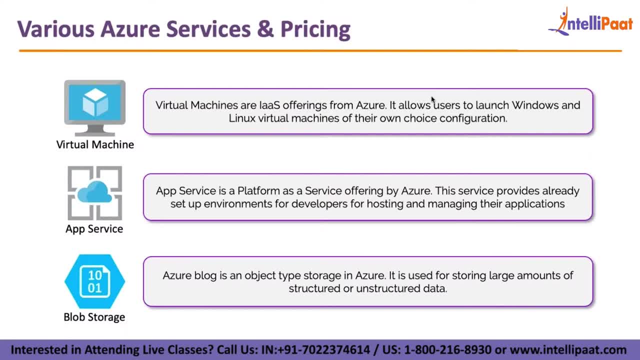 So whenever you deploy a server in Microsoft Azure, that is nothing but a virtual machine, right? So a virtual machine is just like your own laptop or personal computer or PC, right? It's just that a virtual machine can have whatever kind of resources you want, right? 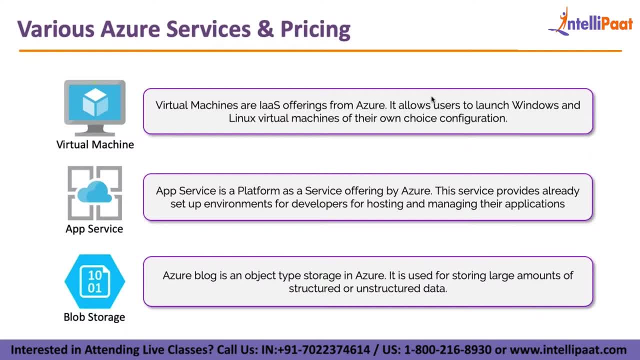 So when you deploy a virtual machine, you choose the amount of RAM that you need, you choose the amount of CPU that you need, and then you deploy it right. So that is the most common service. That is exactly what a virtual machine is right. 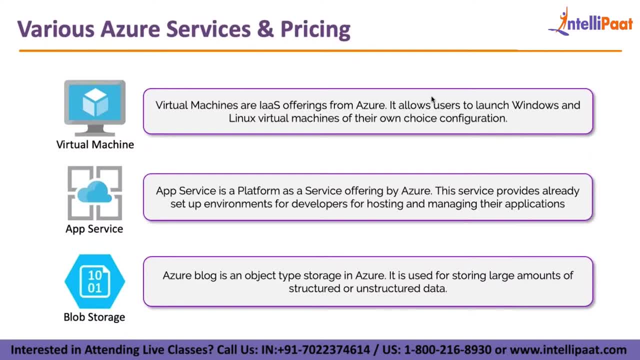 For example, in your PC, if you have a 32 GB RAM right now, you cannot just change it right now. You will have to buy some parts, include it in your PC setup and only then that configuration will increase. But with virtual machines. 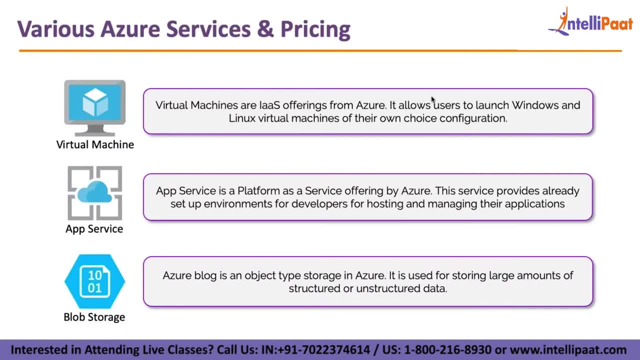 the thing is, you can do that in a matter of seconds. right, And how can you do that? Because the infrastructure, or the hardware that is basically made available to you by Microsoft Azure, is virtual. It's virtualized, which basically means if your virtual machine is being launched, 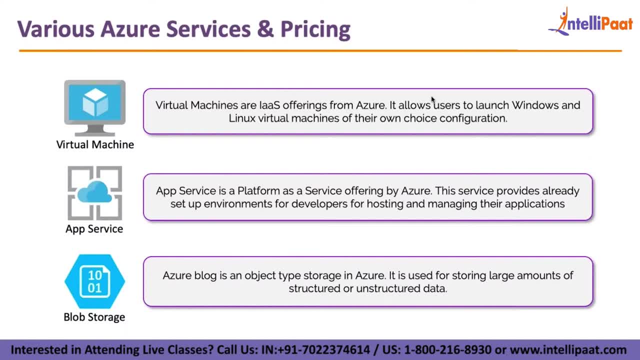 on, let's say, a certain hardware. it might be the case that the same hardware might be accommodating 100 or 200 of virtual machines as well. So that is the kind of resources which are available on the hardware. but the hardware can virtualize some of the resources. 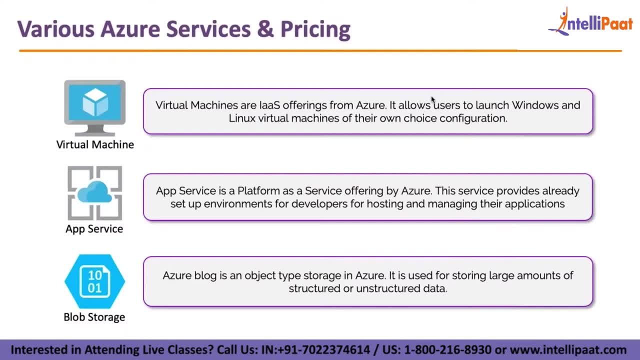 and can make those resources available to you as a separate machine. That is exactly what virtualization is right, So a virtual machine can be virtualized right. So a virtual machine can be virtualized right. So a virtual machine in Azure, like I again said. 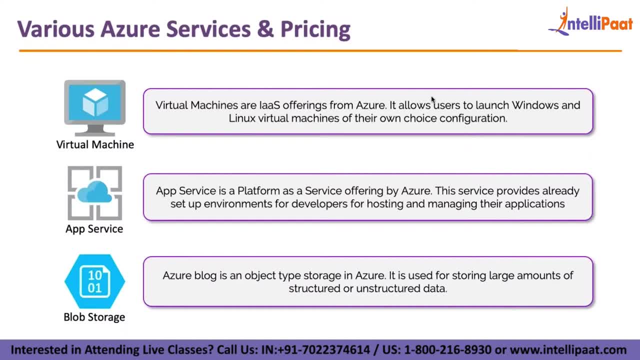 it's basically a server that you deploy, right, And these servers are basically going to have the required RAM, the required CPU that you specify. So that's what a virtual machine is right. Then the second type kind of service is called app service. 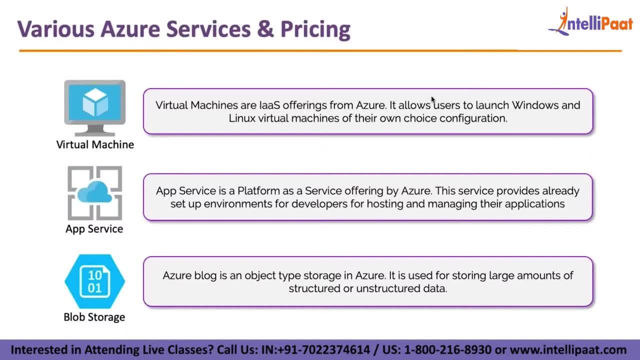 So what is an app service? So an app service is basically a platform as a service, right, And in that what you get is: so, let's say, you deploy a virtual machine, right? So when you deploy a virtual machine, what happens? 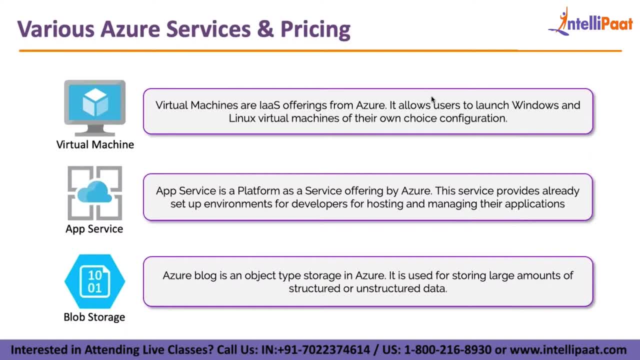 You get a screen to a computer which probably has the Linux operating system or the Windows operating system installed on it, And then you can use it as you want, right? But in app service this thing is not there. In app service what happens is you are given a platform. 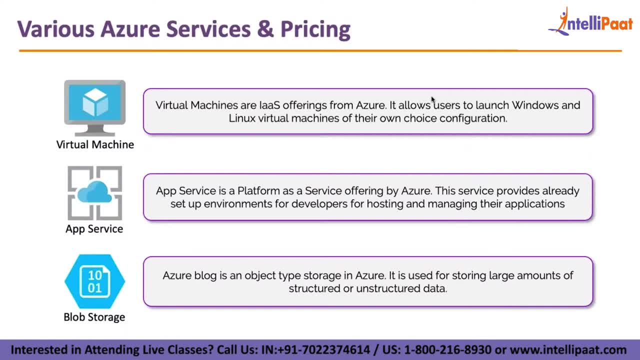 So you're not given the whole machine to work on. You basically are given a platform which basically gives you a dashboard, kind of a view, And in that dashboard you can only use it to do the actions which are specified by the service that you're applying. 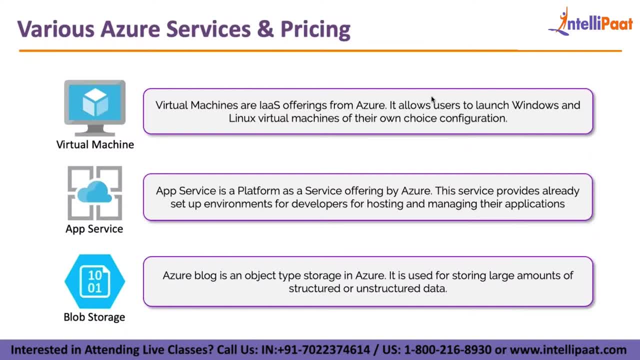 For example, in app service, you can deploy your own website. But if you have to deploy your own website, let's say you want to do that on Azure Virtual Machine. So first what you'll have to do is, let's say, your website is based on NET. 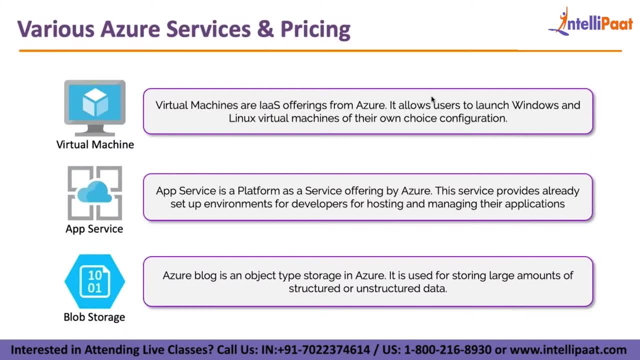 So you will have to install NET on the server. or let's say, your website is based on Apache software, So you will have to install the Apache software. If it's a PHP website, you will install the PHP software. And once all the softwares are installed, 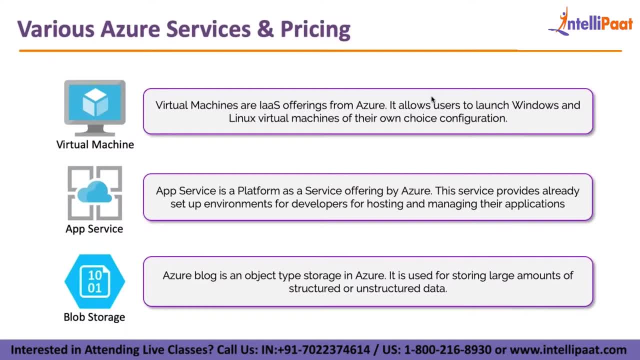 only then you can deploy your website on it, or you can copy the files of your website on it, and then your website will become available. But the scene with app services is that everything is deployed automatically. So you just tell Azure what is the kind of website. 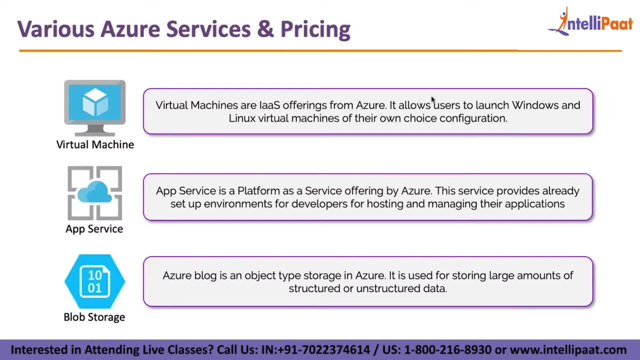 that you are going to deal with. So, let's say, if you have a PHP website, what you do is you click on app services. you tell Microsoft: okay, so I'm gonna use a PHP website on the service that I'm deploying. 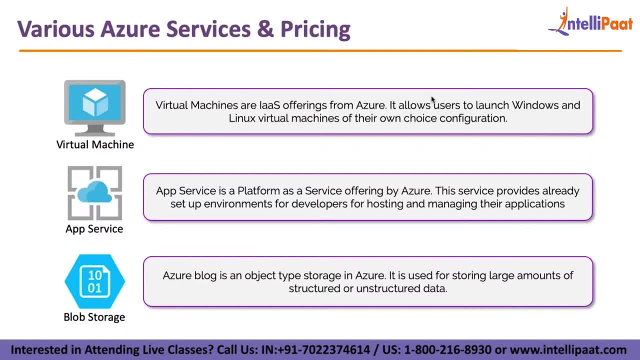 Microsoft themselves. they basically set up the environment for you. They install the softwares and everything, and all they do is they give you a button which is on the dashboard that you will see And on that button you can see. I mean through that button if you click on it. 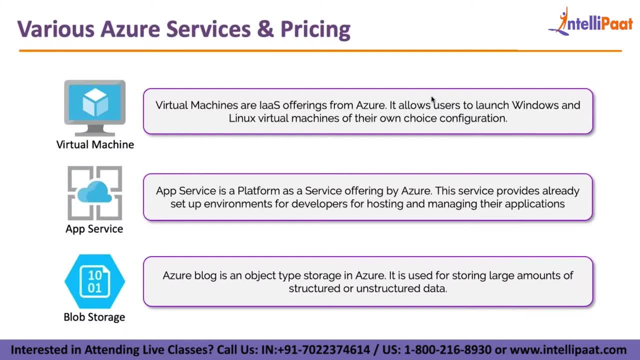 you will be able to upload your website And once your website is uploaded, it will automatically be deployed on the server, which is basically deployed in the background. So the purpose of having an app service versus a virtual machine is to make your life easy. 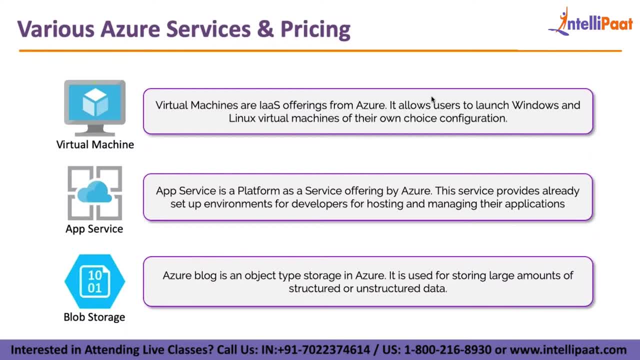 so you do not have to deal with the operating system directly. Azure manages the operating system on your behalf. It manages all the softwares based on your behalf, And all you do is you just deploy your application. So that is what an app service is. 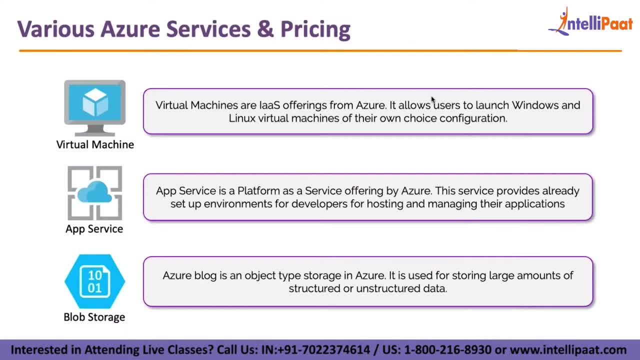 Similarly, the third kind of very common service which will be used in Microsoft Azure is the blob storage. So a blob storage is just like Google Drive, So I'm pretty sure every one of you might have heard or might have used Google Drive in any of your careers, right? 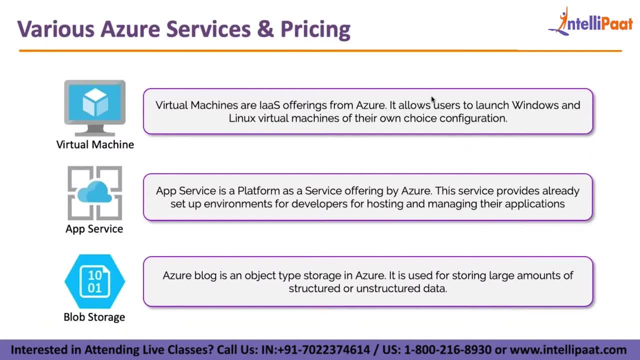 A Google Drive is just like uploading your file on the cloud and that's about it, And that is exactly what a blob storage also is. So on blob storage, you can also upload your files, but what you can do with those files is a lot different. 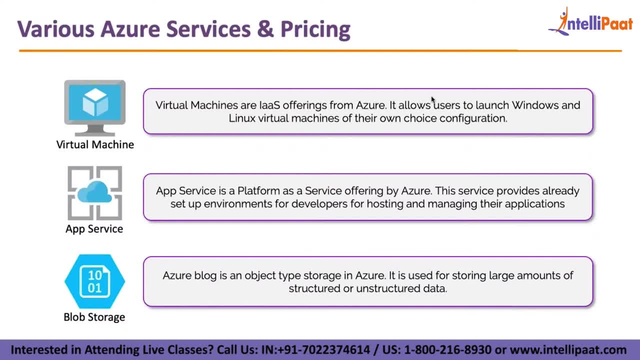 than what you can do with files on Google Cloud, For example. in blob, you also have the option of keeping those files in a very primitive kind of storage, which is going to reduce your costs drastically And at the same time, you will see that when you're using. 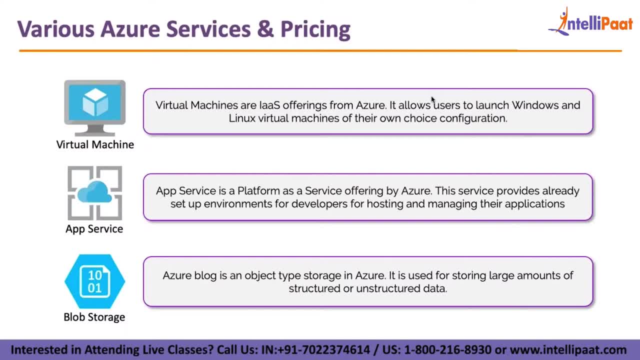 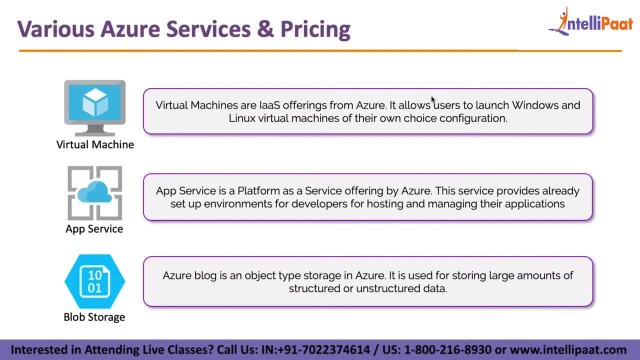 And after 30 GB you will have to buy some storage where you can upload that data. But when you're using blob storage you do not have any restriction of how much of data can you upload. it's unlimited data that you can upload. 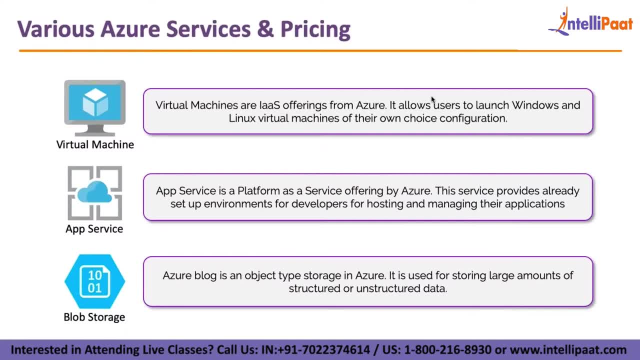 And, at the same time, you are only charged for the data that you upload per month. Let's say, you uploaded one terabyte of data, so you will only be charged for the amount of one terabyte of data, and nothing less, nothing more. 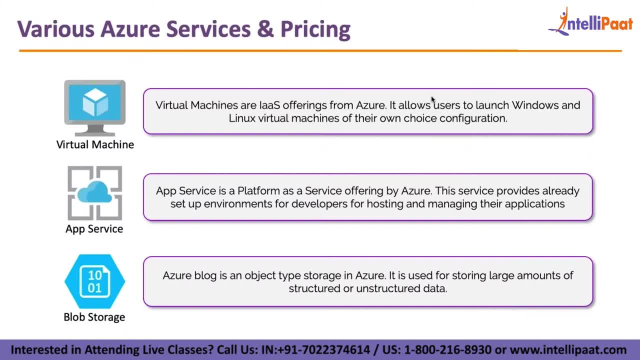 Now those pricings are also very different. Now those pricings are also very different. So, if you want very high speed intelligence, So if you want very high speed intelligence, download and upload to your, to your file that you have uploaded on blog stories. 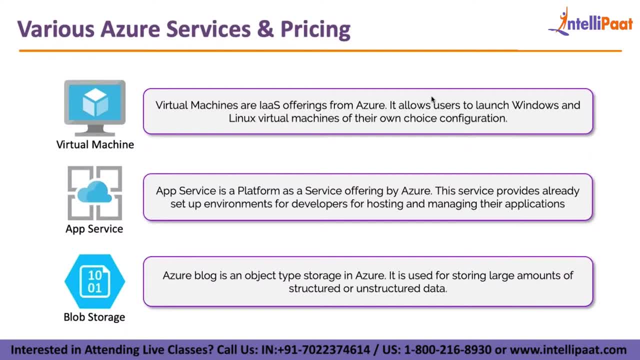 the pricing will be different. let's say you say that this is a backup file that you're putting on blog story, and probably you. you will never use it again. you just want it to be saved in a very safe place. so in that case, what you can? 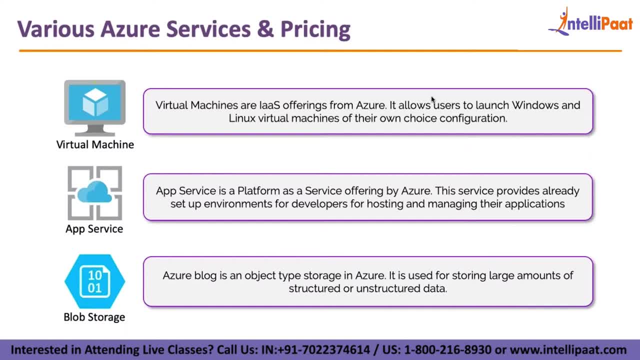 do is you can change the storage class of your blog storage, and that will almost take make the cost of uploading and keeping the file one tenth right, and similarly, there are a lot more features as well, and that is exactly what blob shortage is. so again, if you want to understand it, it's just like Google. 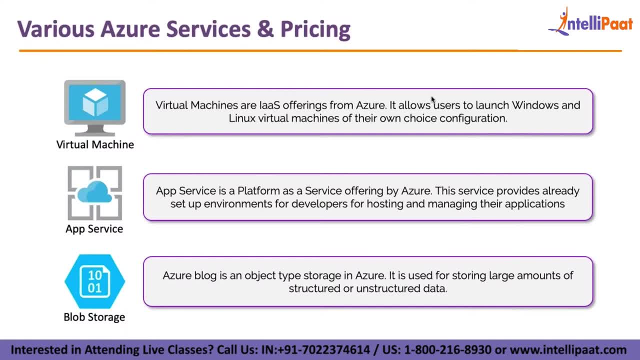 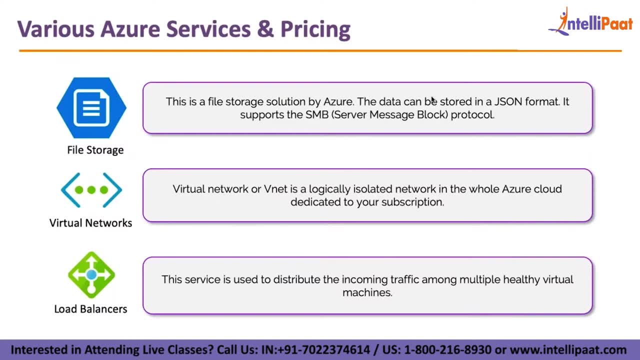 Drive, but with a lot more features. so that's about what blob storage is right. then you have something called as file storage. so file storage is just like having a network drive right, which you can map to your computer. so I just talked about Google Drive. Google Drive- you. 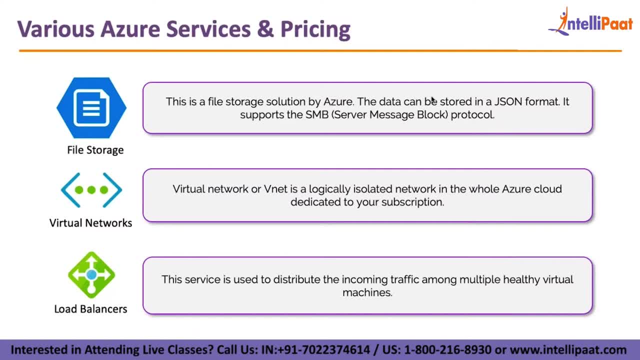 cannot map it as a C Drive or a D Drive on your system, but with file storage. if you deploy it on Microsoft Azure, it has again, you know, a very unlimited kind of a service where you can decide how many GBs or terabytes you need, and once you, 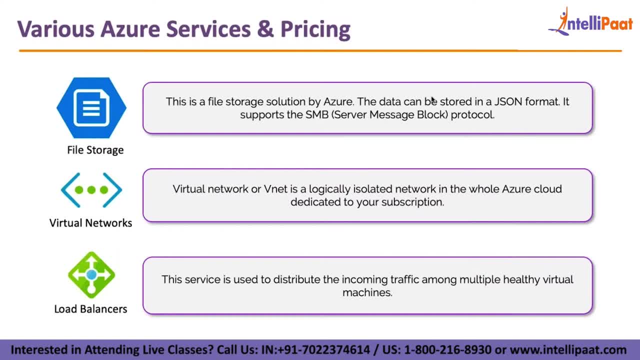 defined that application in Microsoft Azure. you can basically connect it to your computer and mount it as a local disk drive, and then you can basically copy files to it or retrieve files from it as you want. so this is what a file storage is now. the cool thing about file storage is that multiple people can be can basically. 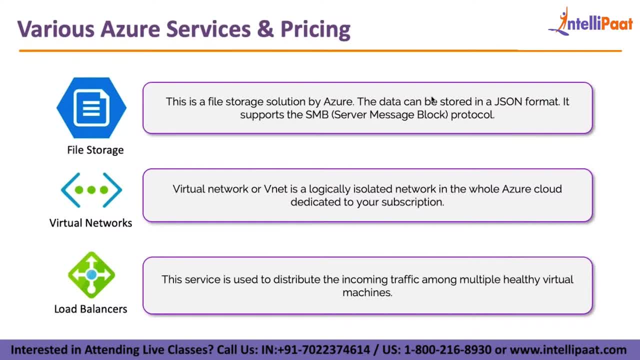 mount this drive on their computer at the same time, and they can use it for as a shared drive between them while they're working on it. right, so that is what a file storage is, so each of these service basically plays a different role. when you are deploying an application on production cloud, right then the next. 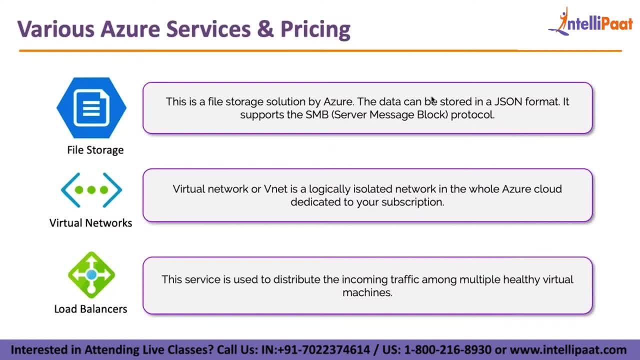 set kind of service that you have is called virtual networks. so virtual networks is just like a. you know, in your office you have networks right. so if you want to deploy a network for a set of machines that you have deployed in Microsoft Azure, the way you can do that is by making use of virtual networks. now again, you can. 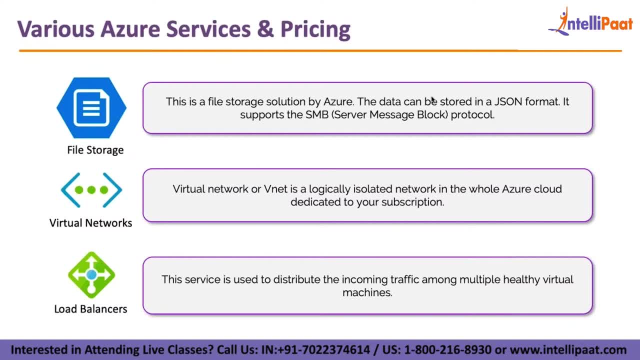 create n number of virtual networks in your as your account, where you can have n number of servers, and these virtual networks again can have n number of features that you can explore and implement, which I think you will learn more as you start using the virtual network service. all right and the final. 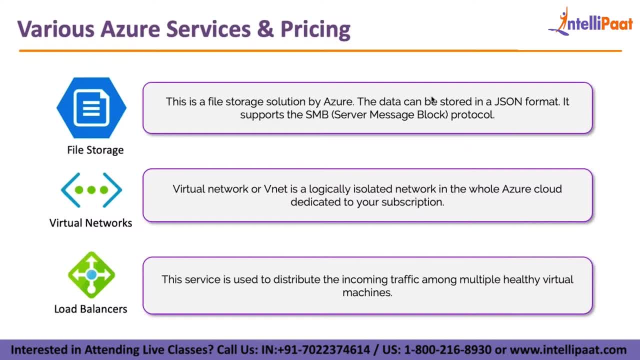 kind of service that we're going to understand is load balancers, right? so what is a load balancer? a load balancer is basically, you know it's, it's, it's more of use in production and probably for a guy who does not know about load. 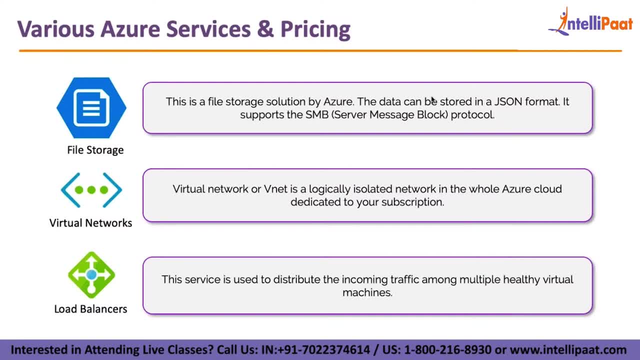 balances. even if they're using it, they will never get to know about it, right, and this is all actually a service that we are actually going to make use of in today's session as well, where I'll show you the reason. people are using the virtual network that's available at home for load balancing. 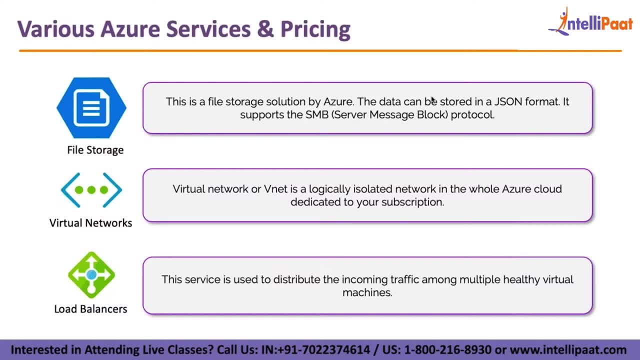 use load balancer. so I give you the example of a story in the beginning, right, where you can add more servers for your applications and then, as you add more servers, more number of users can basically be dealt with, right. so how does that happen? how does, how do we, how can you add hundreds of servers and then? 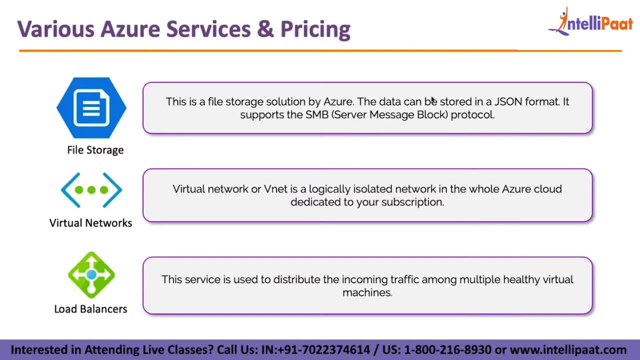 decide where a user exactly is going to land on or which server is going to land on, for basically is needs. for example, if you go to the flipkartcom or you go to amazoncom, so when you go there you automatically are given. if your internet connection is good, if your application loads, just fine, right. so where is the 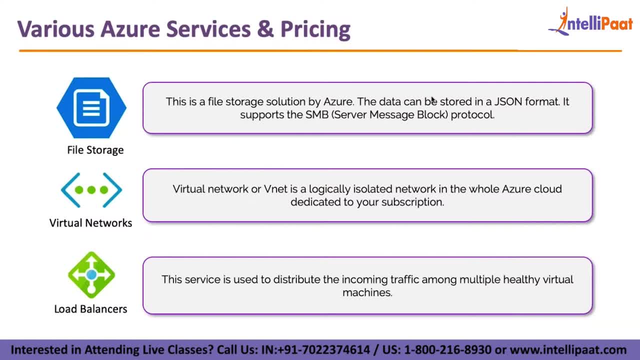 data on that application coming from. that data is basically coming from cloud, is basically coming from a fleet of servers which have been deployed on cloud and to one of those servers you connect and that is where your data is basically coming from, so you never decide which server you have to connect to. that is. 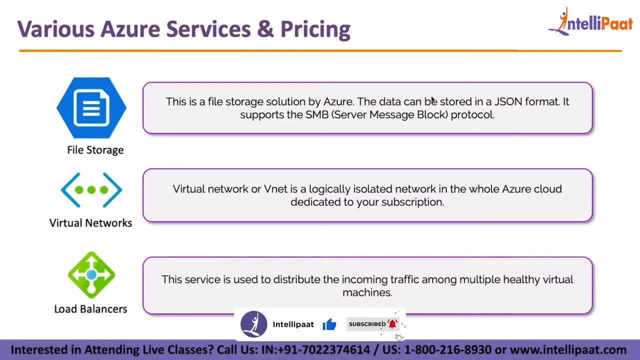 automatically chosen for you. and that is exactly what a load balancer does. it distributes the load equally among multiple servers which are deployed in your infrastructure. okay, more about this. we will understand as you move along. so, guys, this is a brief about the as your services in Microsoft Azure. now let's go. 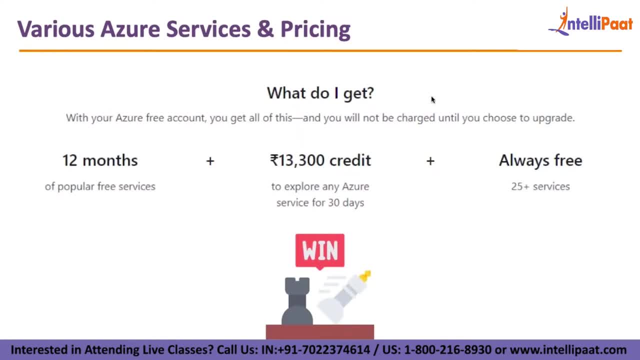 ahead and talk about the pricing. so the moment you sign up on, as your what it is: one month free usage of Microsoft Azure with a free credit of around thirteen thousand three hundred rupees or two hundred dollars. right, so you can use this amount to learn and understand. Microsoft is your right, so you can. 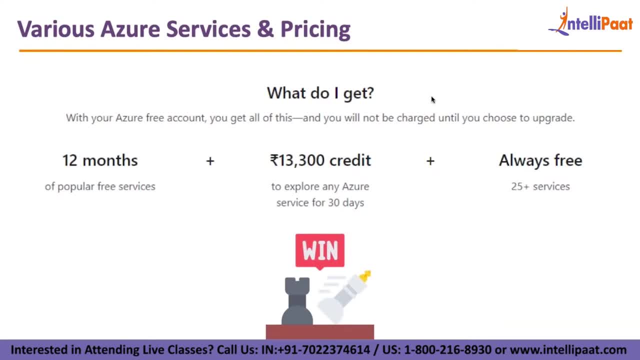 deploy as many servers as you want, and you can use them until and unless you exhaust the two hundred dollar or the thirteen thousand three hundred piece credit that you have in your Microsoft account the moment you sign up, right. so this is something which is very developer friendly, which is your has done that the moment you. 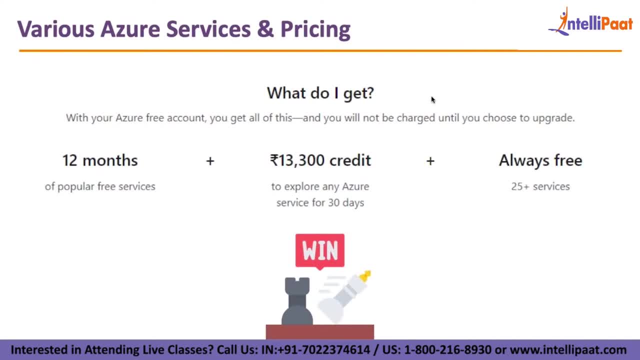 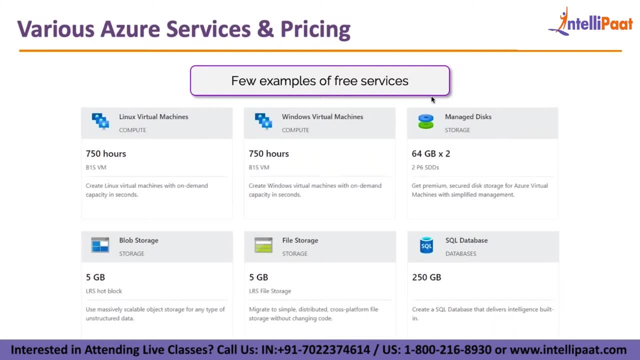 sign up. it makes the services available for you free so that you can practice them and learn more about it. okay, and other than that, there are some set of free services as well which are valid for you know, a lifetime. so whenever you're using a zone- this is some of these services- are valid for one year for. 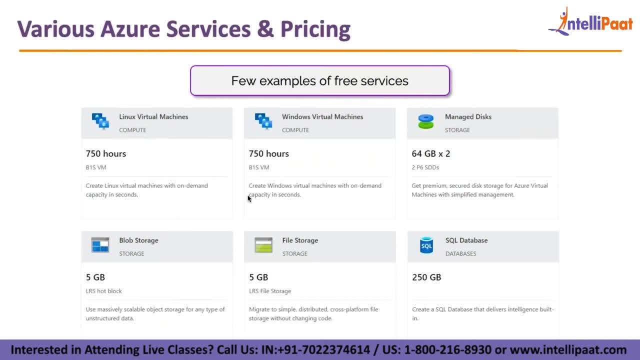 example, when you're using Linux or two machine, the Windows virtual machines on Microsoft Azure, 750 hours every month will be given, free of course, to you of the server type B 1, SVM. alright, so if you are using the servers, the first 750 hours of those servers will be free of cost, that is, will not be charged to you. 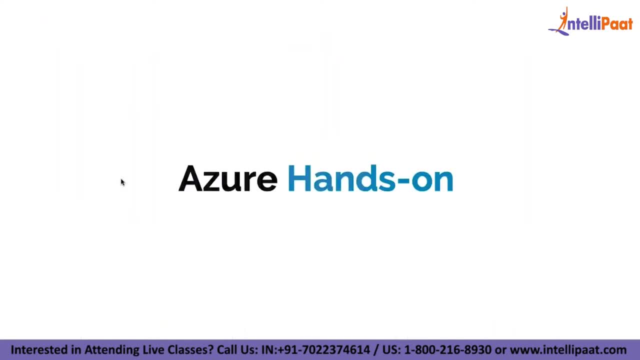 while you are using those servers, right? so now, guys, let's move on and start off with the hands-on, and what I'm first going to do is a I'm gonna explain you what we are basically going to make, and then we are going to go ahead and start it. okay? so, guys, let's first understand the website. 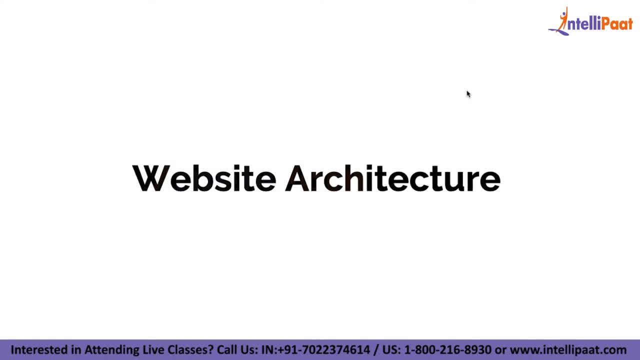 architecture that we are going to deploy on as your today. alright, so what we are basically going to do is we will have two sets of those, right? so the first set of servers would be in the US region and the other set of servers would be in the. 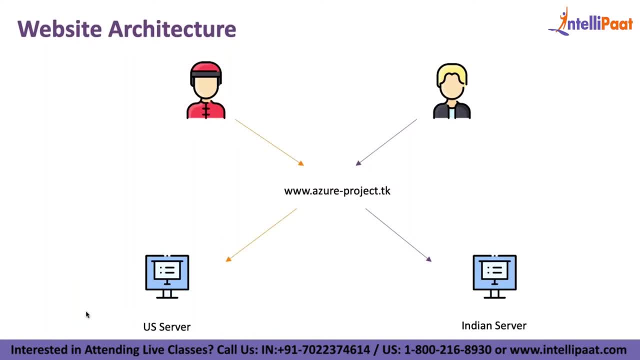 Indian region right now. since the in these will be multiple servers, what we are also going to do is we are, we are basically going to have a load balancer on top of them and, through this load balancer, if you are in the US region, if you go to a particular domain, basically it should be pointed to the US server. 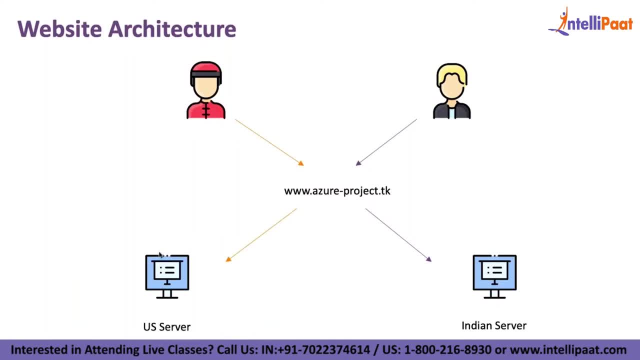 automatically and once you are pointed to the US servers, your load balancer should basically, you know, divide the load between the people or between the servers that you have in your fleet right. similarly, let's say you are from India, so you will also be accessing the same domain, which? 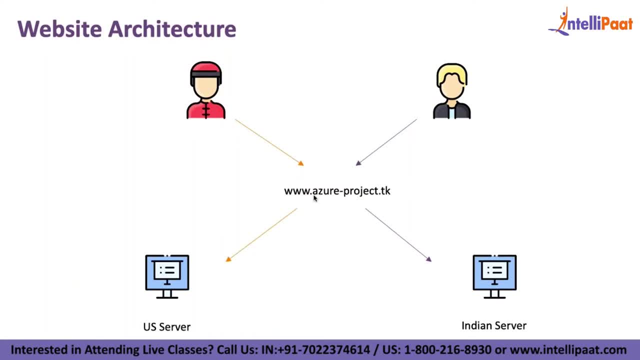 is this right? and once you access it, you will be basically pointed to the Indian servers and in Indian servers we are going to have a load balancer which is basically going to route your request to a specific Indian. so let me repeat it again: so, first thing, what we'll do is we basically deploy some servers in US and 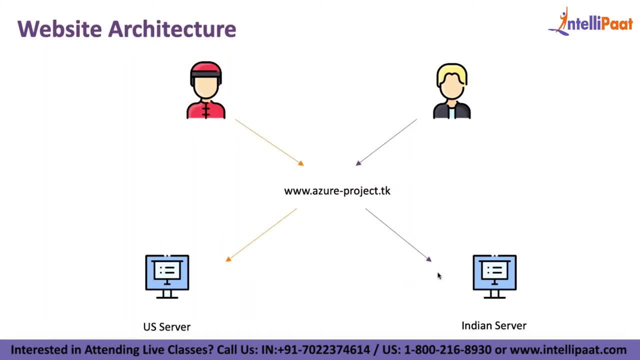 deploy some servers in India, right, and these servers will have a load balancer on top of them. so now what is going to happen is, if five servers are hosting the same application, your user does not have to be concerned about which of these five servers he has to reach. you will basically reach to a common point. 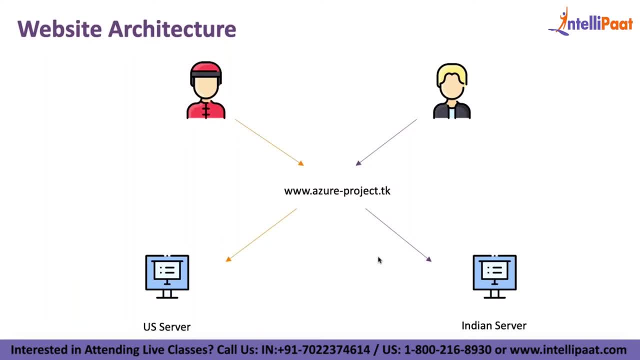 and that common point will be the load balancer, which is basically going to route the request, based on which server is going to be more free. okay, and that is exactly what we are going to do with the US server. okay. so, guys, just let's say, if you are in India and you are trying to access, 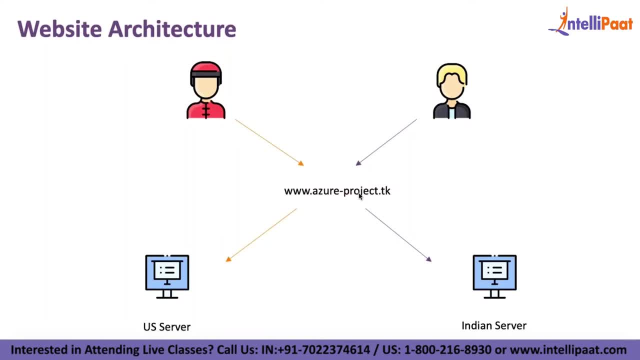 as your project or TK right. so obviously, if your request is being served from the US servers, the ping will be more or the time it will take to you know, to respond to your query would be more than the servers which are, which are basically deployed in the Indian region. so Indian region, if you are from India, the 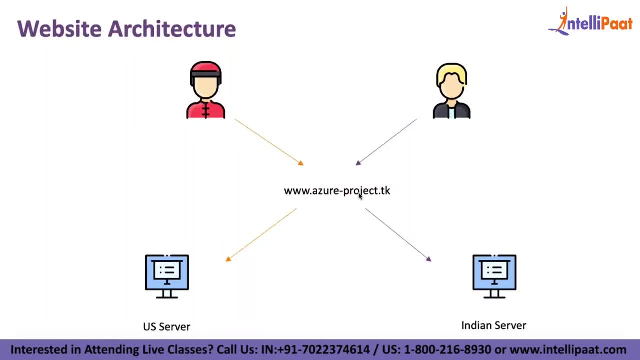 servers can reply to you more, faster. similarly, if a guy from us- right, if he is trying to, you know- ping a particular website and that website has servers in US, obviously they can serve him faster than servers which are going to be there in the Indian region, right? so this is. 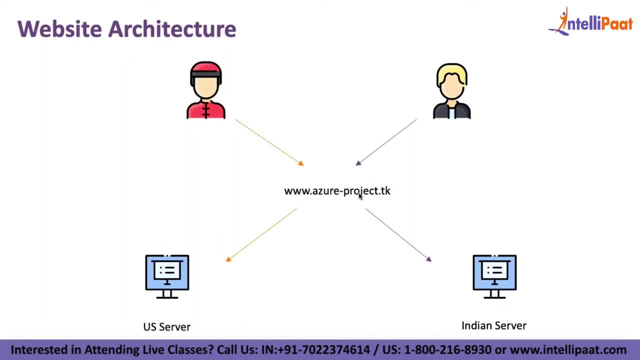 the architecture that we are going to deploy today. this is basically how even a modern e-commerce application basically works. so if you have a look at Flipkart or Amazon, these are the things that they implemented in background, which normal customers usually don't know about, but they basically use every. 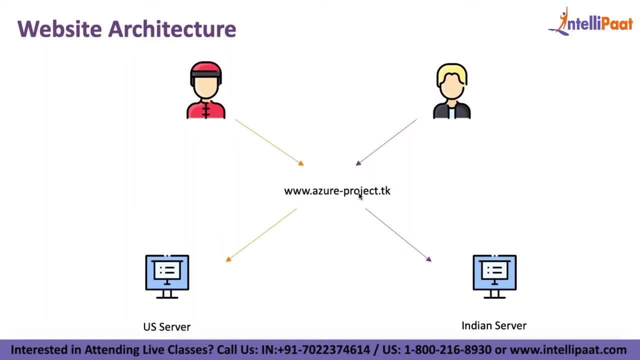 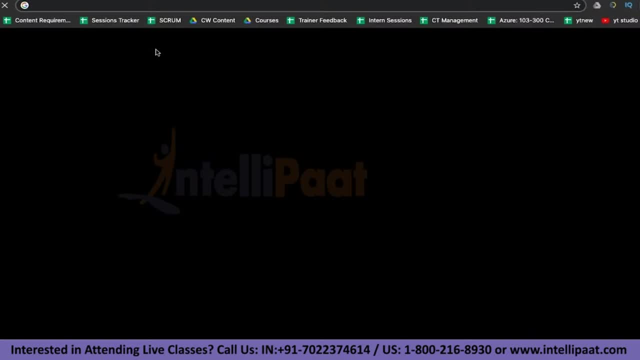 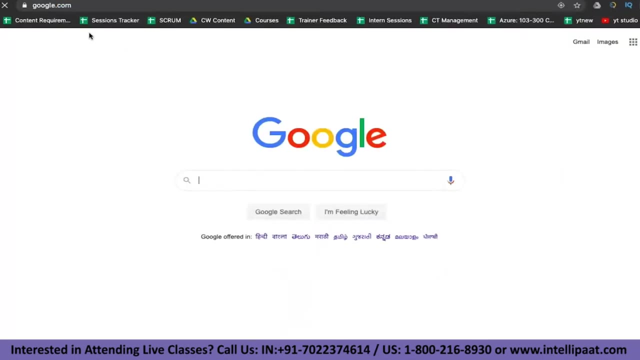 day, okay, and that is exactly what we are going to do today in this session. if we go to, let's say, a browser, so let's say I type in googlecom, so you will automatically see, the moment I type googlecom, I'm automatically routed to the Indian server. so, as you can see, it's written India over here, right, if I type? 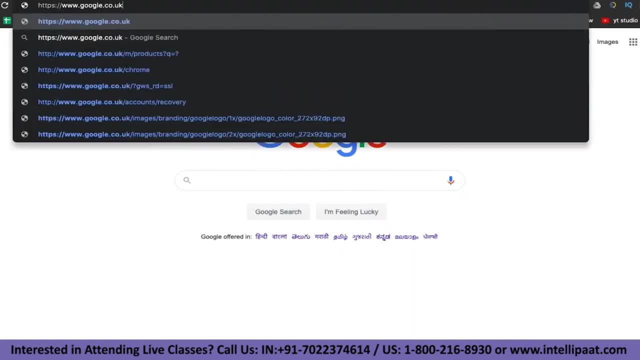 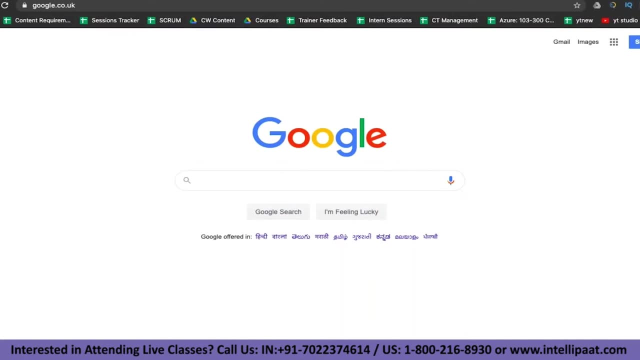 in googlecom dot UK. you can again see I'm still on the Indian server. why? because every time I'm trying to go to a different Google website, I'm always logged to the server which is more nearer to me, and that is the Indian Google right. so no matter which URL you are entering over here, you always been. 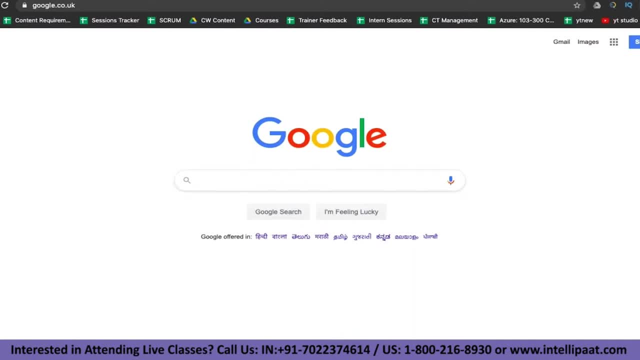 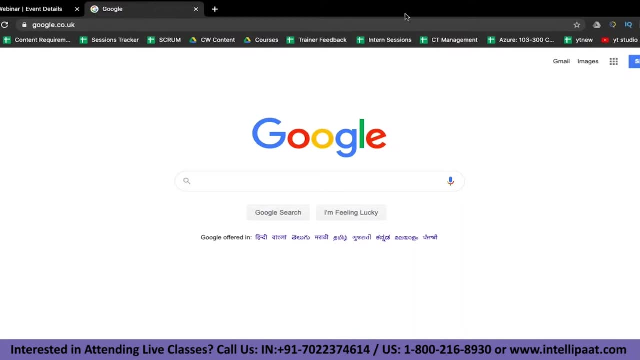 redirected to the Indian Google right. but if you want to bypass this, so let's say you connect to a VPN, right? let's say you connect to a VPN and you connect to a particular country. so whichever country you will be connecting to, let's say you connected to. 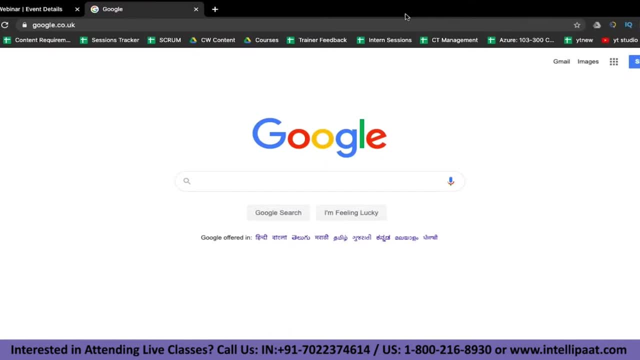 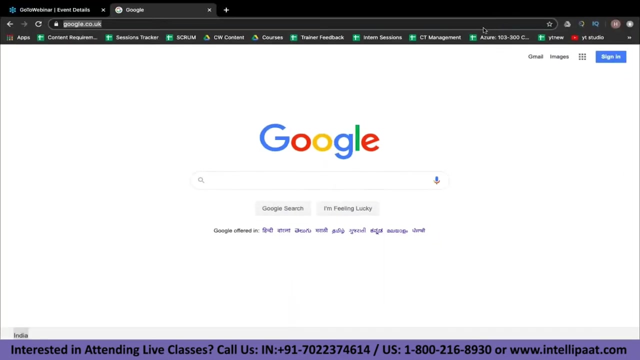 you connect to France. so now, when you will be going to your browser typing in googlecom, now you will be directed to googlefr, right? so that is exactly how it works, what we are going to implement in today's hands-on as well. let's go ahead, and the first thing that we would do is go to the 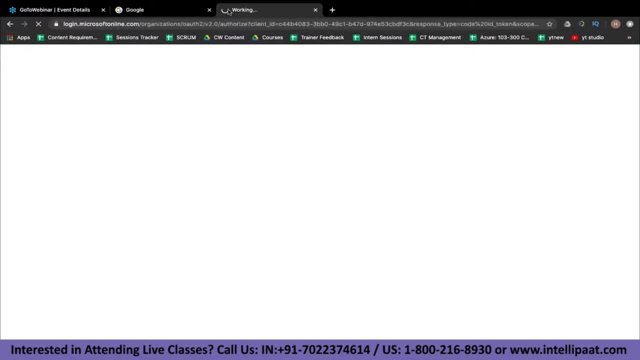 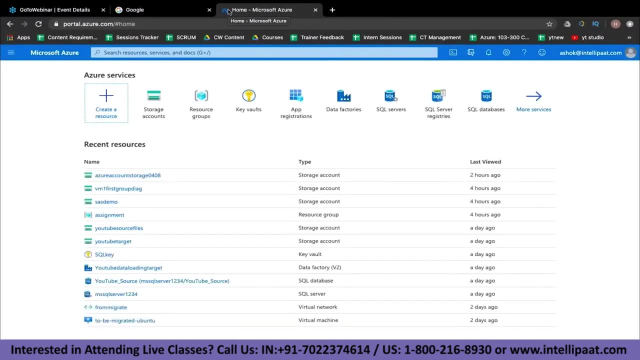 Azure dashboard. so the URL is portalazurecom. so once you guys log in or sign up on Microsoft Azure, this is how your dashboard is going to look like. now I already have some resources that I have deployed over here, so you don't have to worry about them, right? so what I'm gonna? 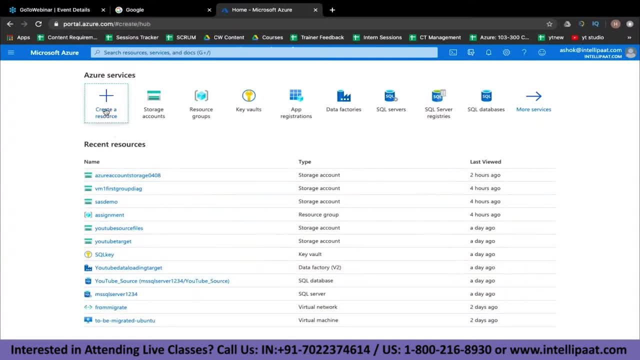 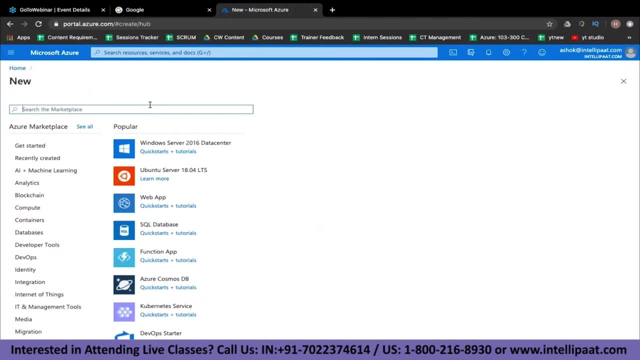 do is I'm gonna create a resource and once I've created a resource now, I will choose what kind of resource that I want to deploy. so when I'm creating a new now, it's asking me what kind of resource that I want to deploy. let's say I want. 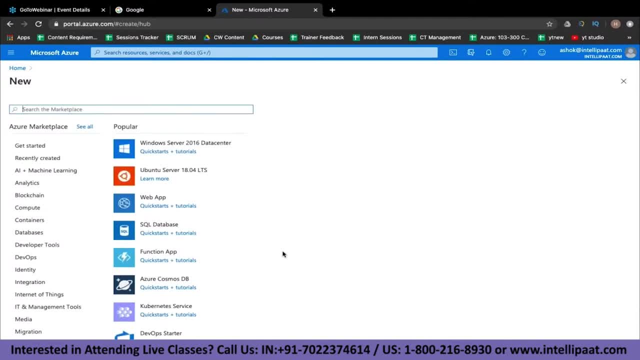 to launch a Linux server. so a Linux server is basically either an Ubuntu server or it could be a sent to a server. but if I want to launch a windows server, I can use a server like this and I can use a server like this and I can use a. 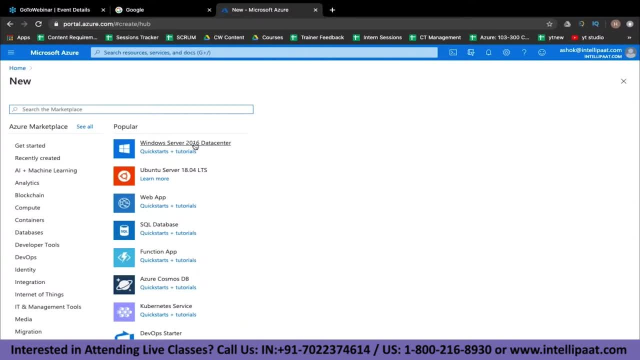 server like this and I can choose this windows or I can choose some other operating system as well, so this gives me a limited option over here. these are the popular options that people basically deploy. so what we can do is we can just search for virtual machines. I can click on that service. 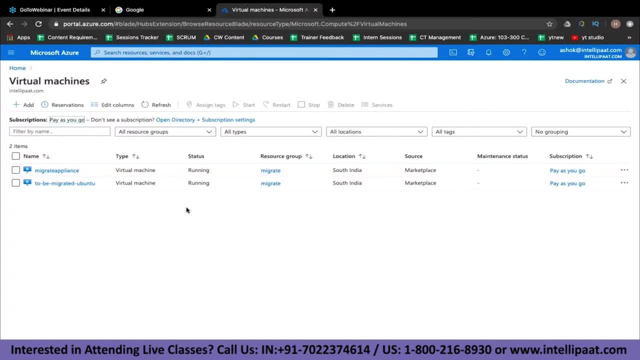 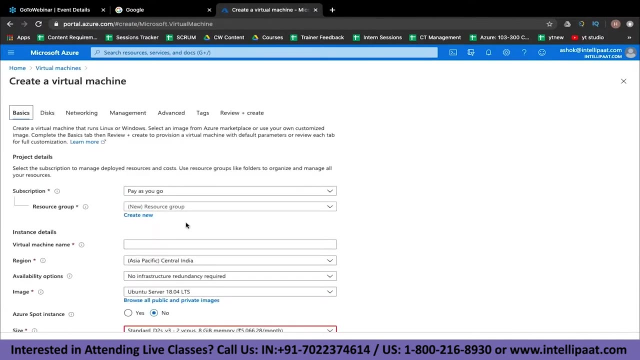 and, as you can see, I have some machines which are already running over here, so we are going to ignore them. so first let's deploy our first virtual machine, so we'll click on add and now i can fill in all these things that i want. okay, so first things. 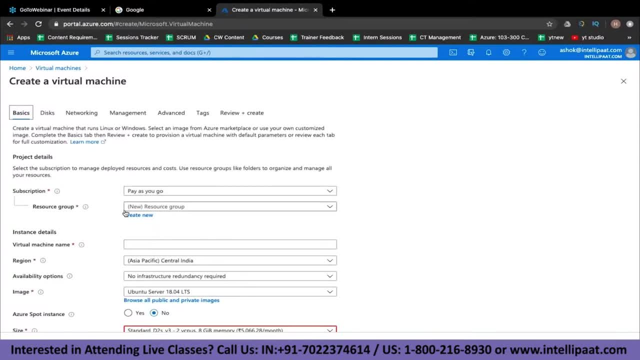 first it will ask you uh, a resource group to basically deploy it in. so a resource group is nothing, but it's basically a logical grouping of all the uh resources that you're going to deploy on the azure cloud. okay, so what we can do is we can just click on create new and let's say this is: 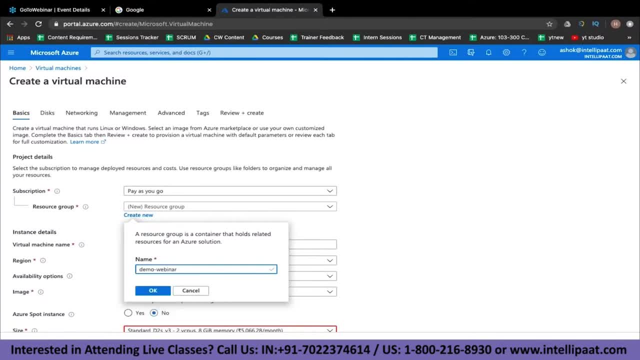 demo hyphen webinar. this is the resource group that i'm basically going to create right now. okay, so the resource group has been created and now we have to enter the virtual machine name. so let's say it's uh, indian server. so this is the server that we are going to deploy. 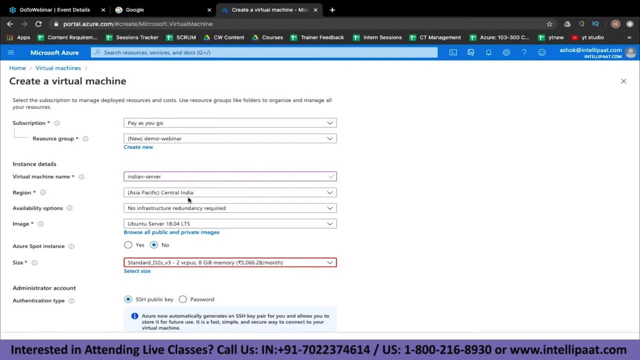 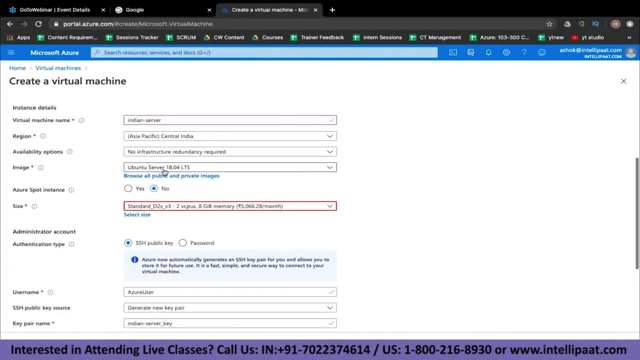 right, uh, next thing that i'm going to see is the region that i want to deploy it in. so it's in central india, which works out for me, which is great. uh, what is the operating system that i want to launch? so these are the different kind of operating systems that i can choose. 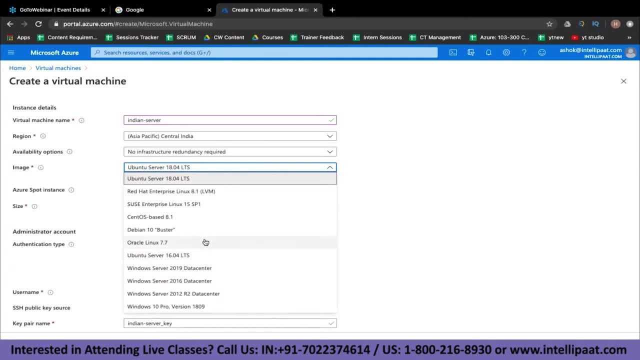 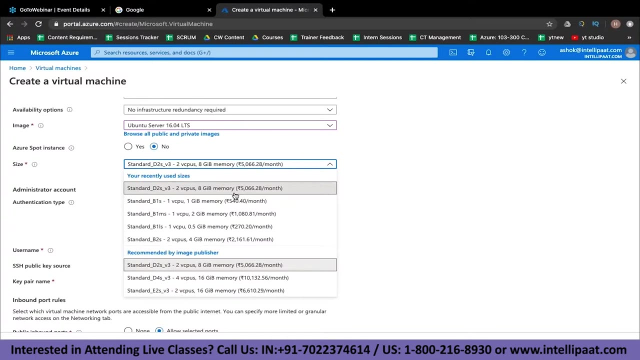 between. so i have the microsoft options, then i have oracle option, i have the linux options. so whichever i want i can choose. so for this demo i'm choosing the ubuntu server. then here i can choose the size of the virtual machine that i want to deploy. so let's say i want to deploy 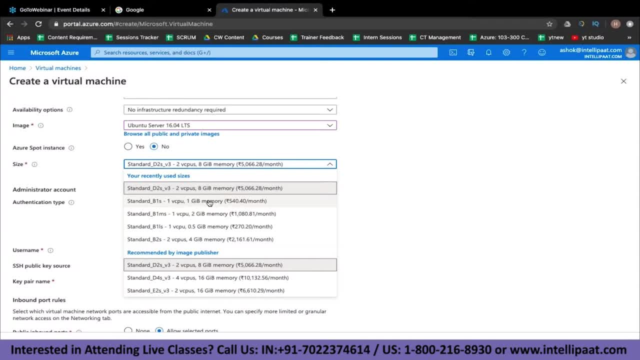 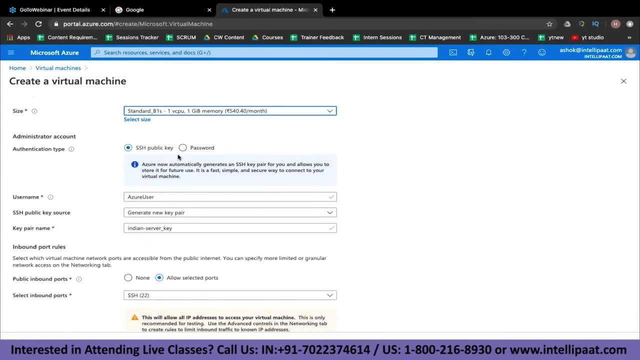 uh, the lowest on this list, which is one vcpu and one gb of memory, so let's choose this. then it is asking me what is the authentication type that i want to choose. do i want to log in using a public key or do i want to log in using a password? so let's choose password. 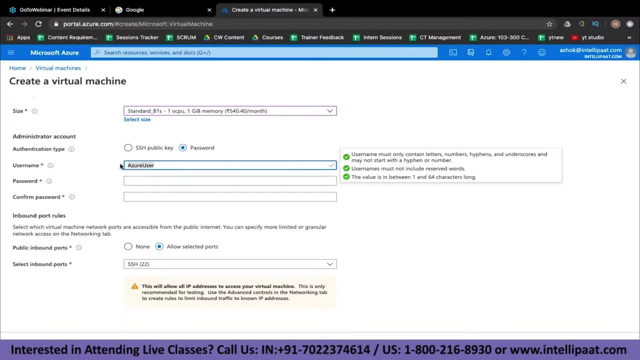 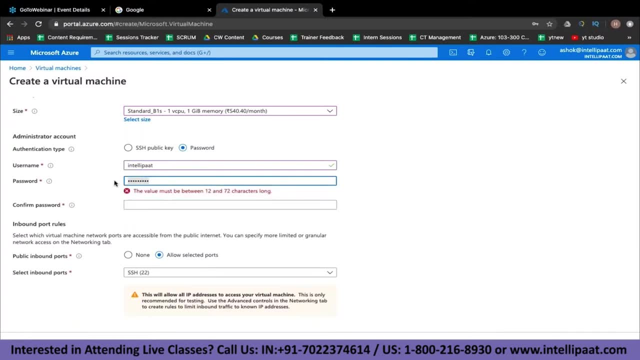 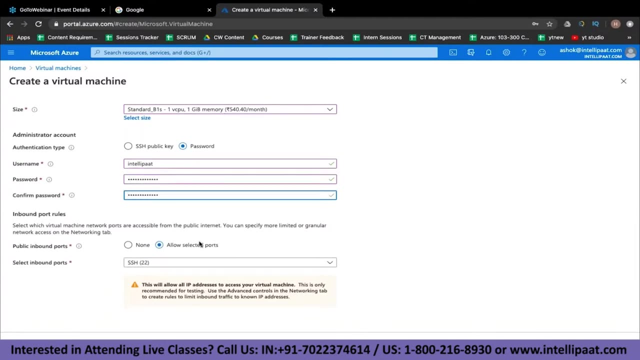 let's give some username over here. let's give the username. let's say as: uh, intellipaat. and now let's give some password as well. okay, it says the value we have in 1272 characters. okay, let's give that value. okay, now, which ports do i want to be opened on the firewall, so whenever you want to connect to a 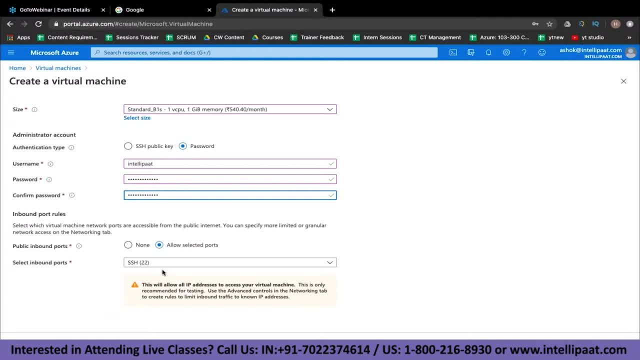 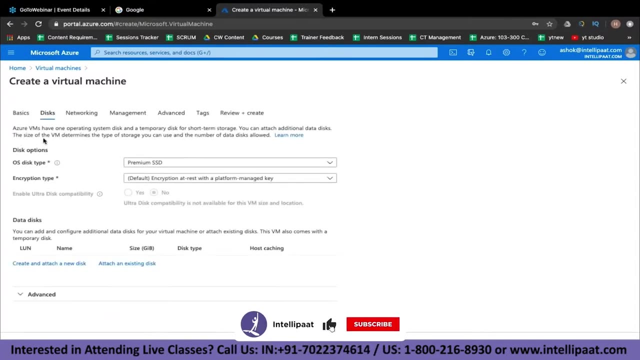 linux machine. you basically connect using the ssh protocol. okay, and the ssh protocol basically always works on port 22.. so port 22 is going to be allowed in the firewall for us. let's click on next. so now in disks, we are being asked: which kind of disk do you want? do you want premium ssd? 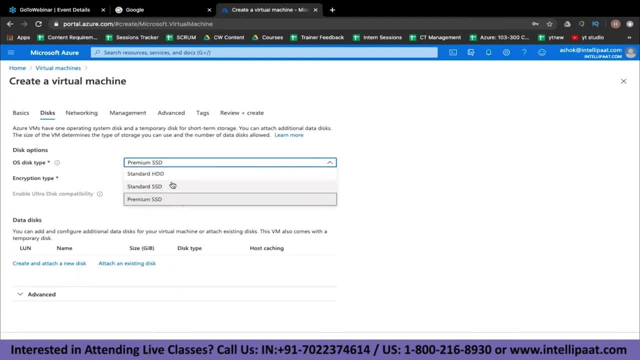 do you want standard hdd? do you want standard ssd? so basically, this is going to affect your performance. so hdd is basically a disk based hard drive. then you have solid state hard drive and premium solid state hard drives as well. so all these three will have different io values. 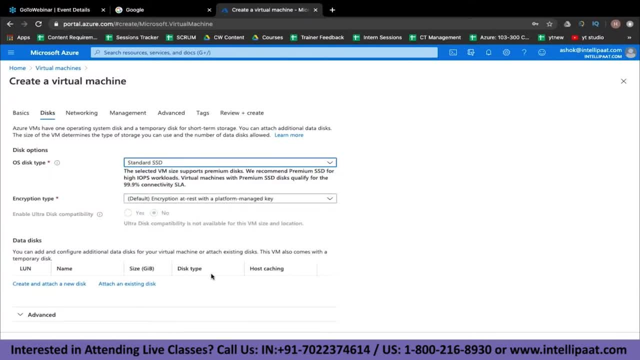 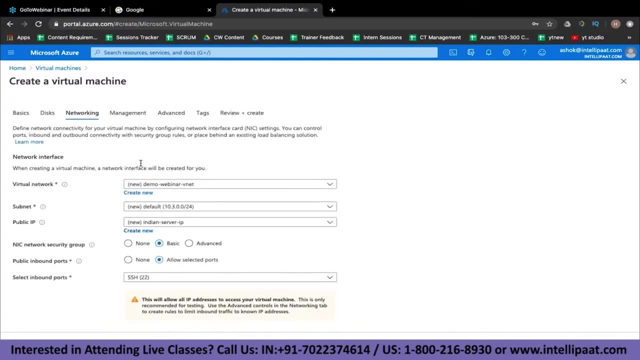 for this demo, let's choose standard ssd, all right, and then let's click on next. now it's going to ask me: uh, where do i want this server to be deployed? so it's automatically creating, uh, you know, a virtual network for me which is called demo webinar vnet. right, and it. 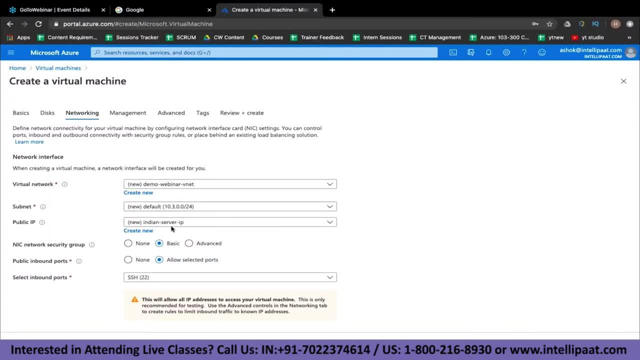 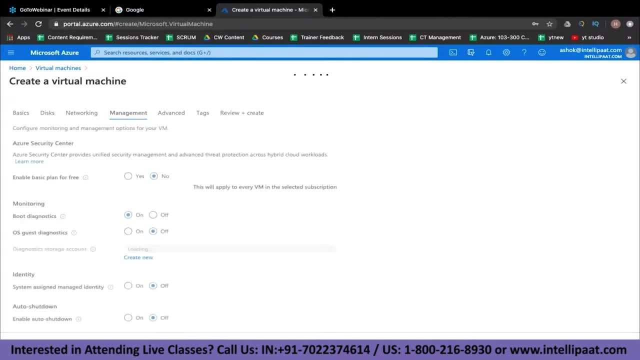 is automatically creating a subnet as well, it is assigning a public ip also to my server, etc. so let me keep everything at default. we'll click on next. uh, now it is asking me what kind of monitoring i want on my server, right? so i don't want any monitoring, so i just switch it off and click on. 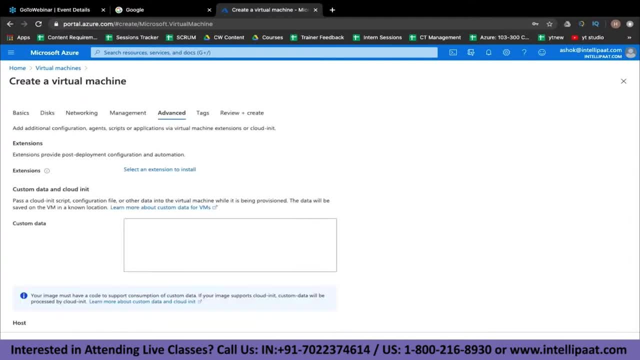 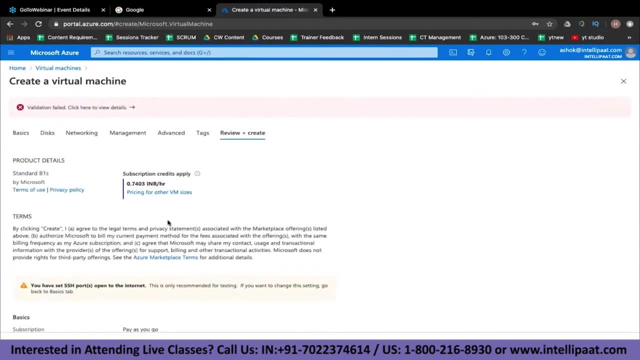 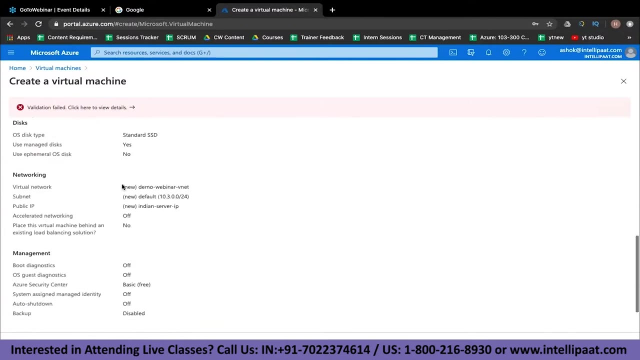 next again. uh, this can also be left, so you can just click on next, next again and finally. now you can basically just review all your settings. right, so it says verification failed. so probably we did not fill out some information. let's verify that, so we'll just click here. 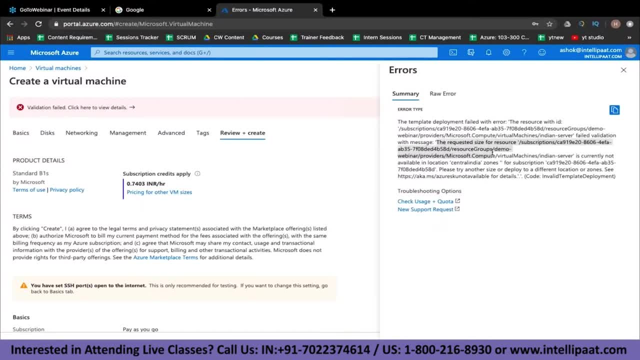 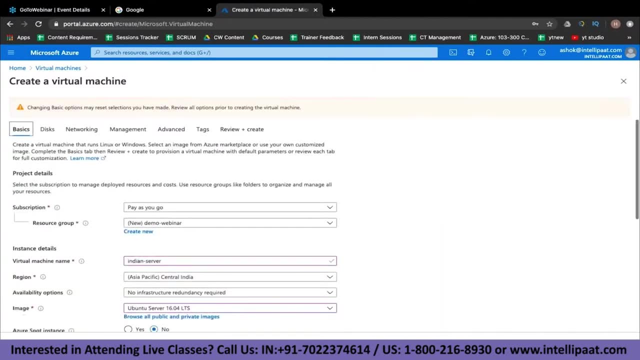 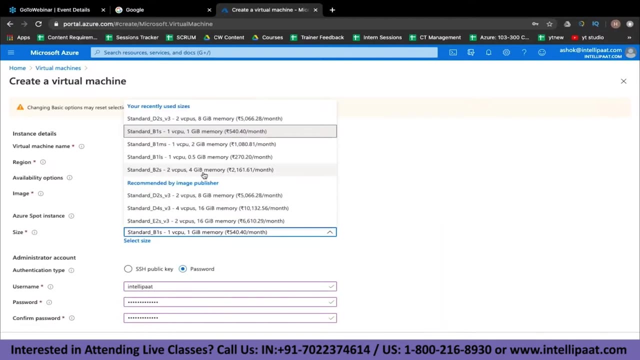 okay, it says the requested size for resource is currently not available in central india. so it's saying: the size that i selected, which is basically this, is not available, so let's choose some other size. uh, let's choose. let's say, an 8gb machine or a 2gb machine. let's say: let's click on review plus create. 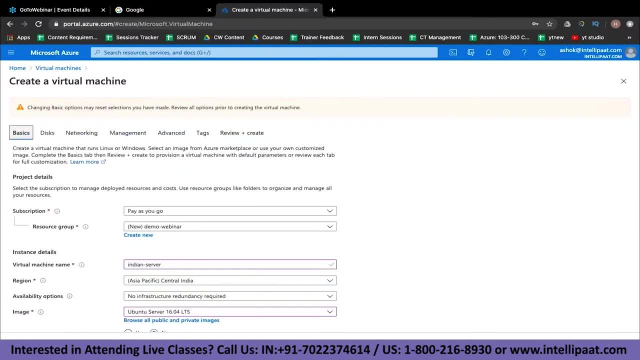 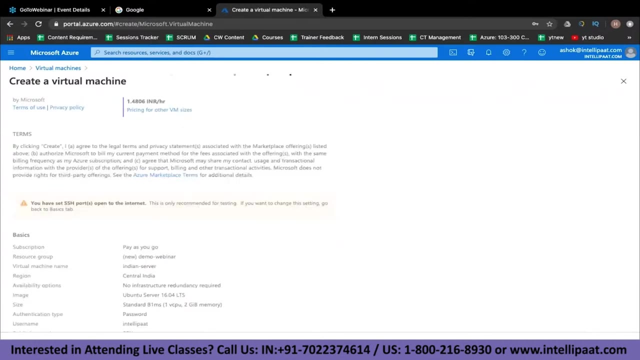 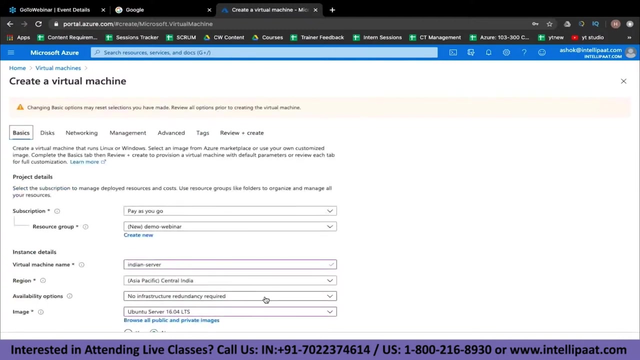 okay, even this is not available, all right. so sometimes the region that you choose, they might not have the required size that you want to launch and in that case you just have to go ahead and choose for a size that might be available. i think if i go for a premium size, it should be available. give me a second. 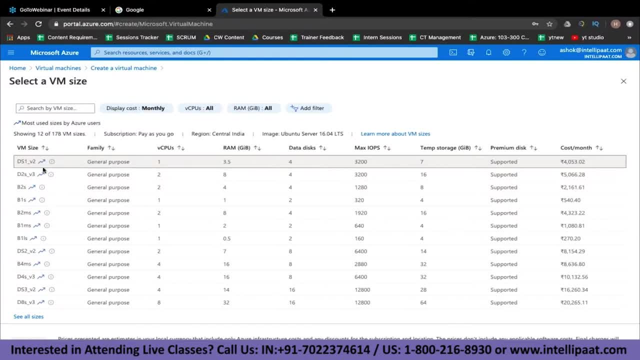 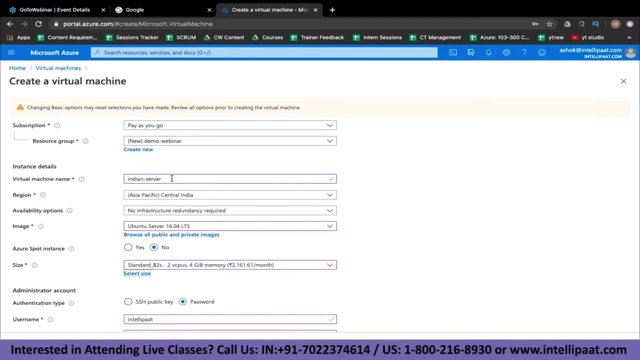 okay, so you can see that the high demand for all these servers and that's why they're all used, right. so what we can do is we can just go back and none of the servers are available in this region. so let's go to some of the region. uh, let's. 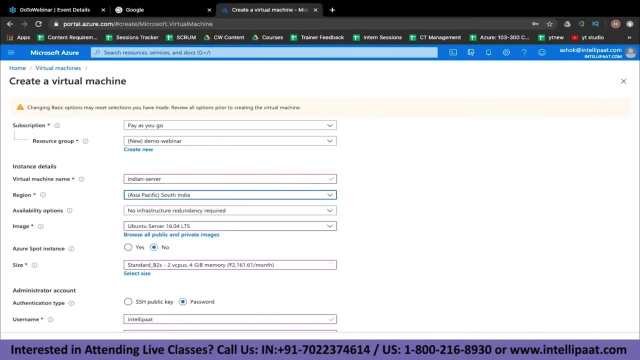 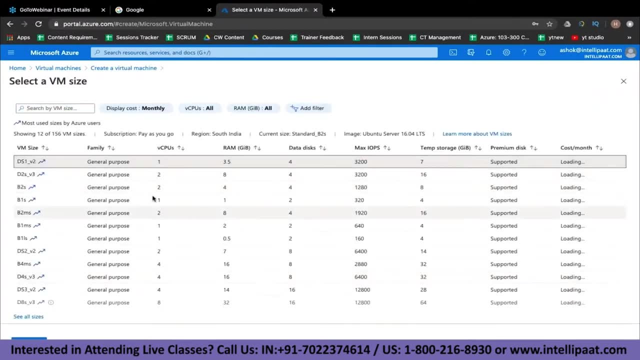 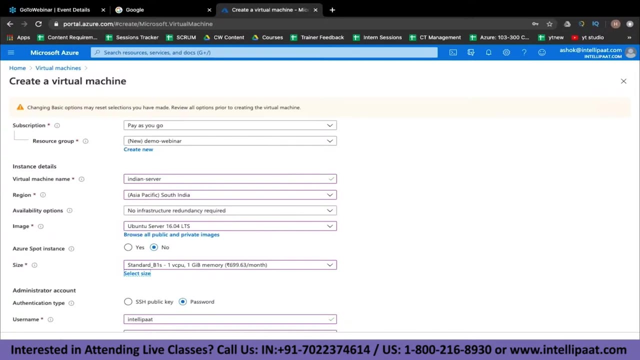 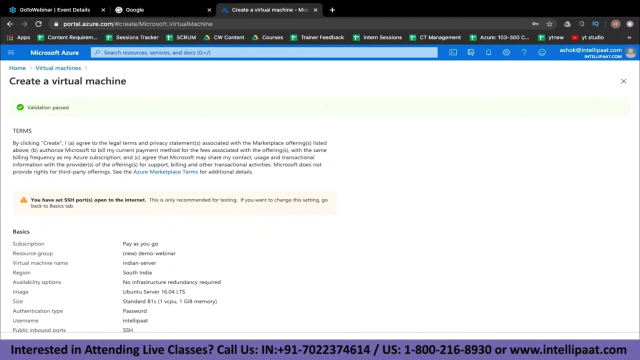 select uh, south india. i think that should have some servers available for us. okay, so here some servers are available. great, so what we can choose? let's choose the same size that we selected earlier, click on review plus create and, as you can see, the validation has now passed, so let's click on create now. 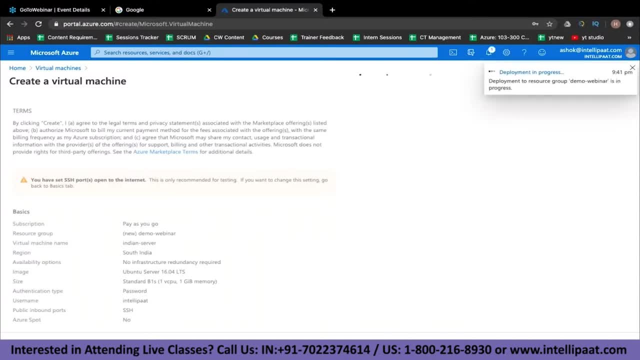 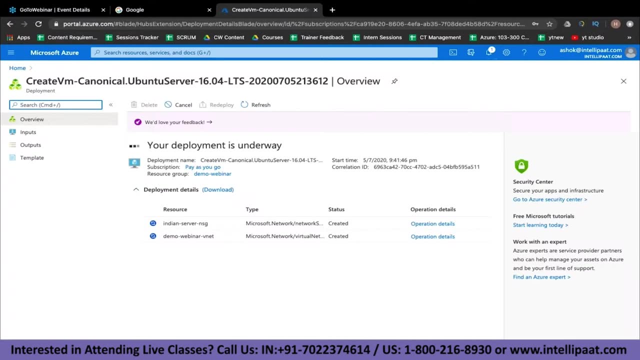 and with this, now my server is getting launched. okay, now it will take some time for this server to get deployed, but basically what we have done is, uh, we have deployed one server in the south india region which, basically, is going to make use of an ubuntu server. 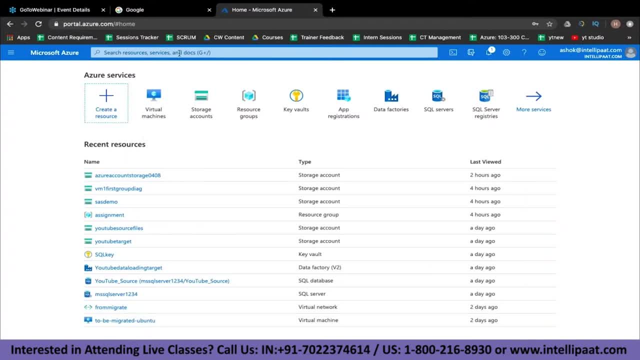 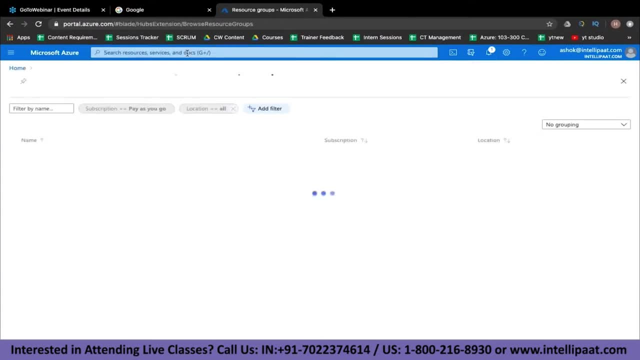 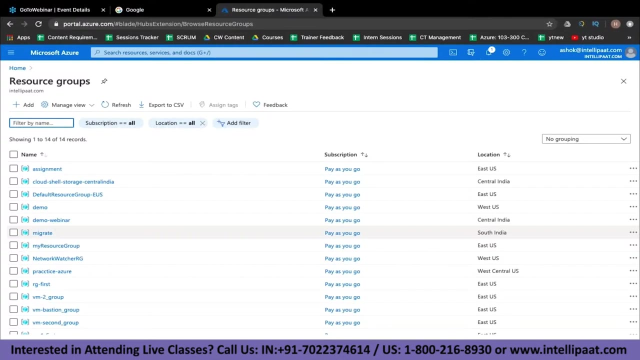 okay, so let's go back to the dashboard and let me show you the uh resource group which is basically getting created. okay, there are a lot of resource groups over here, but what you can basically refer to is this. your demo webinar is here. then you can see the link if you want, like this. 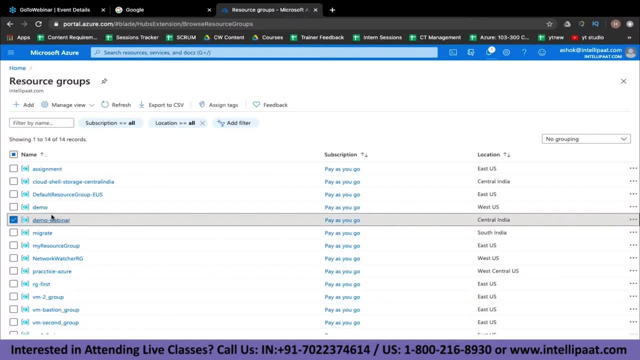 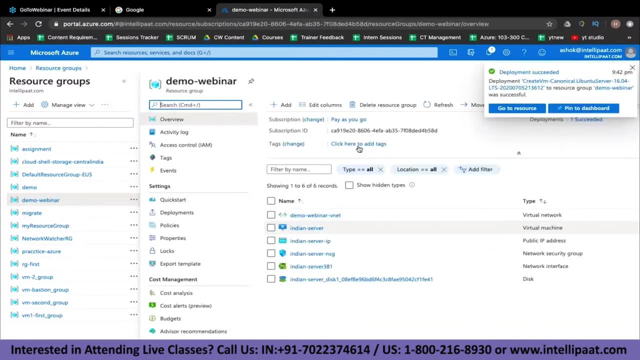 so there you go. okay, all of that is clocks. i will get back in a second webinar- is a resource group that i created right. so now let's go ahead inside the demo webinar, and here you can see the resource that you've just deployed: the indian server. 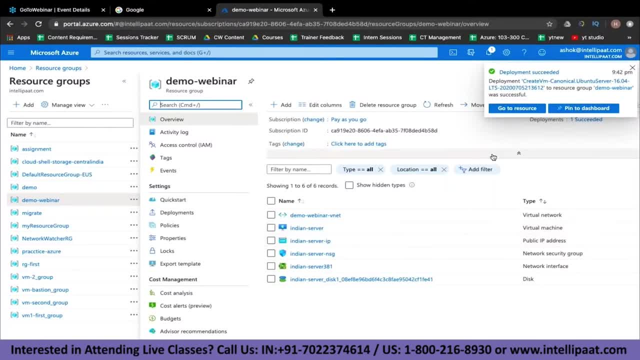 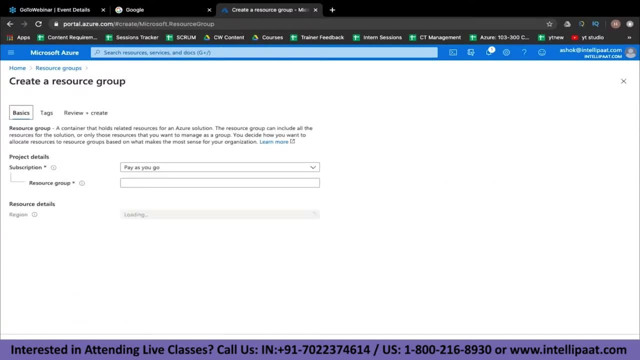 it is getting deployed in there. so, as you can see, the deployment has got succeeded great. so let's deploy a us server as well. so again, let's click on add on the resource group. let's create a second resource group for our us servers so that we can differentiate between, uh, the resources that we're. 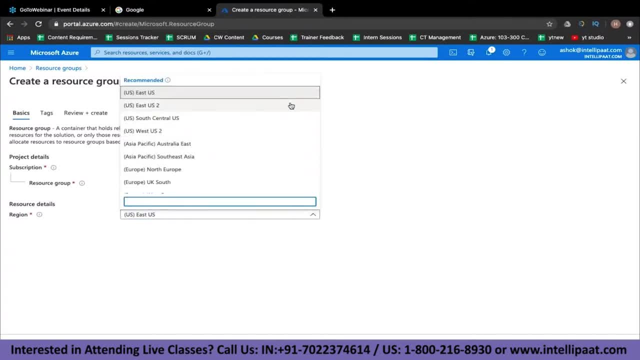 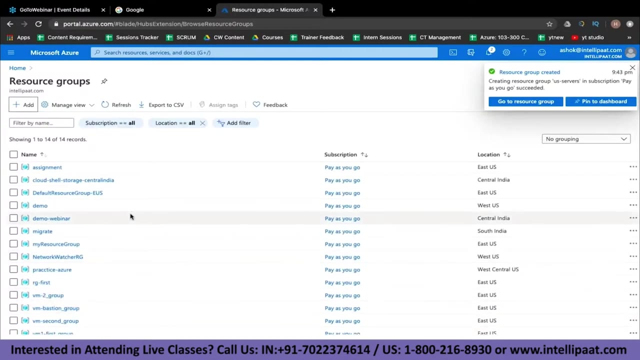 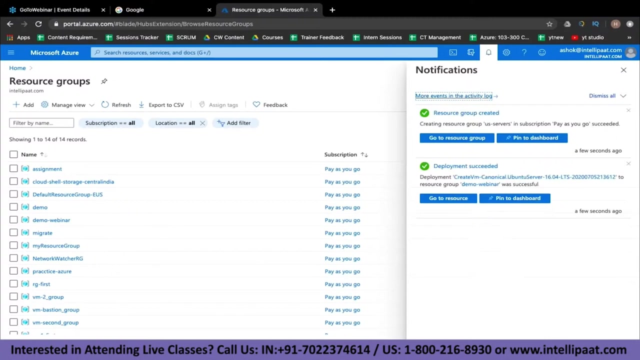 going to deploy- and let's deploy it in the best us region. okay, click on review plus create and finally create this resource group. okay, so the resource group has got created and now i can just go to that resource group and you can deploy some resources over here. so let's do. 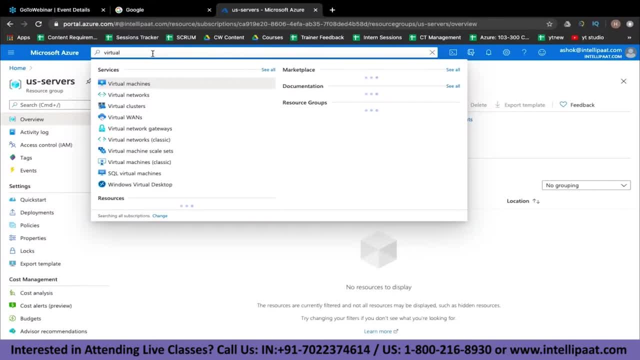 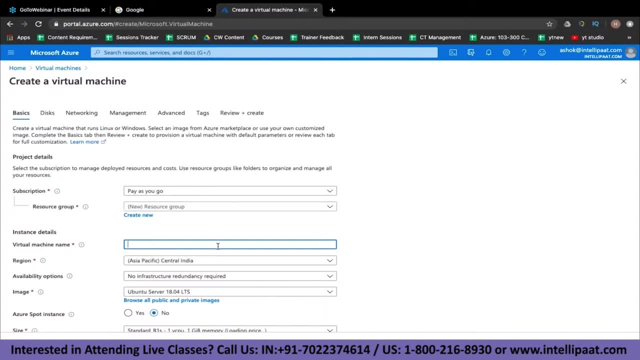 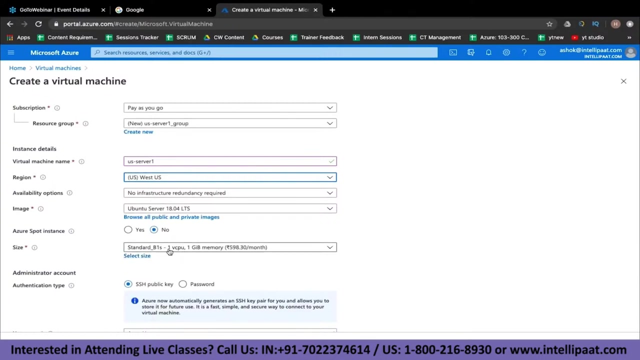 the same thing. let's deploy a virtual machine again in the us resource group. so i'll just click on create a virtual machine, us server one. let's get this name. let's deploy it in best us. okay, this is the image. uh, this is the size. that is automatically selected. let's hope it is available. let's give the username. 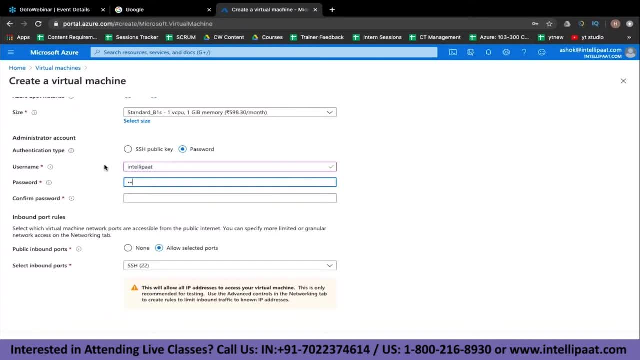 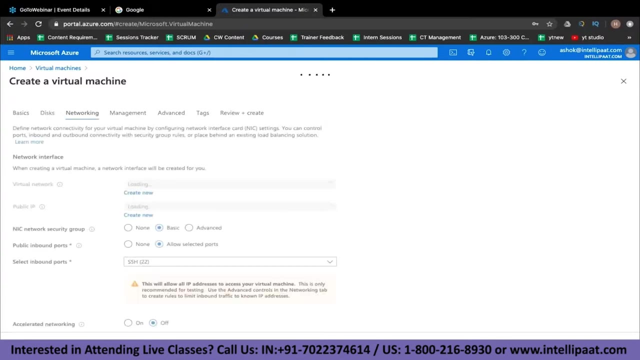 as in telepart, and the password as this. i think i'll keep the same password which i used for my previous. so okay, click on disks. i think rest everything we can leave at default. only in management we will turn the monitor on, okay off, and click on review plus create. so, as you can see, the price is just 80. 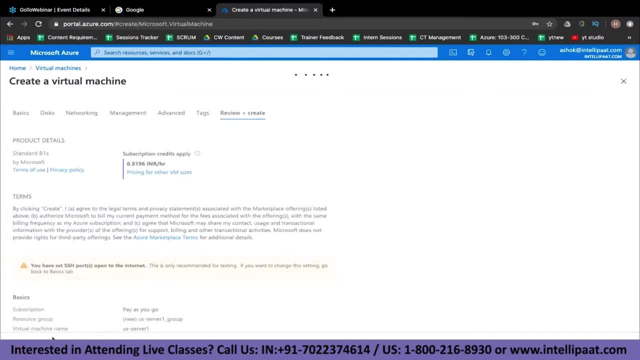 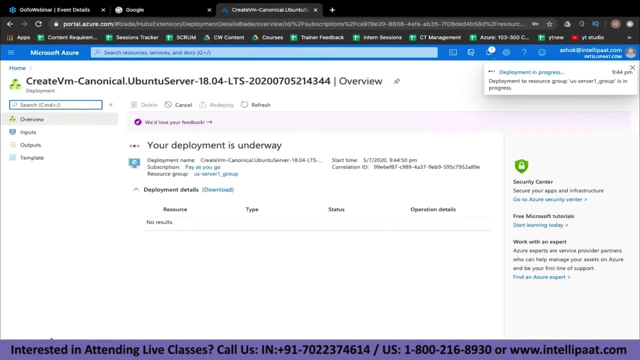 Pasa, but which is great, so we'll just create it now and now. a server is being launched in the US region. okay, now to make it more authentic, let's deploy one, one virtual machine more, so that we have two. and on top of these two virtual 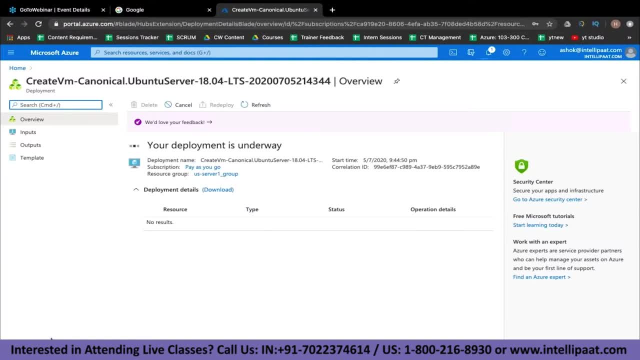 machines, then we will deploy, you know, a load balancer as well, and we'll also figure out a way so that when we basically hit the load balancer, we automatically get to know which server basically we are trying to connect to. okay, so, while this is being deployed, let's deploy one more virtual machine in. 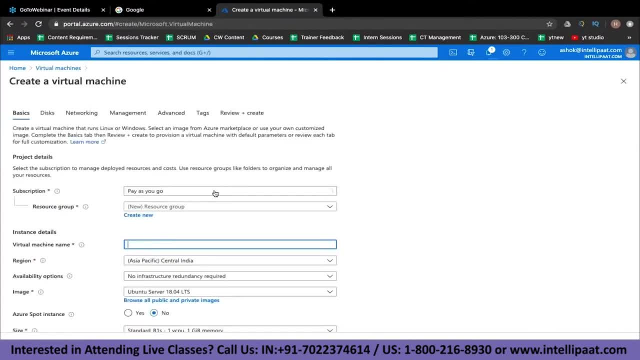 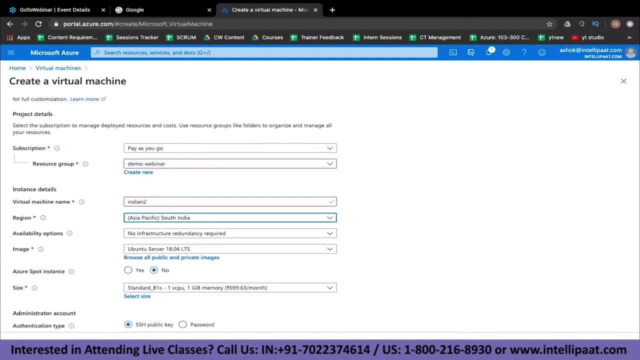 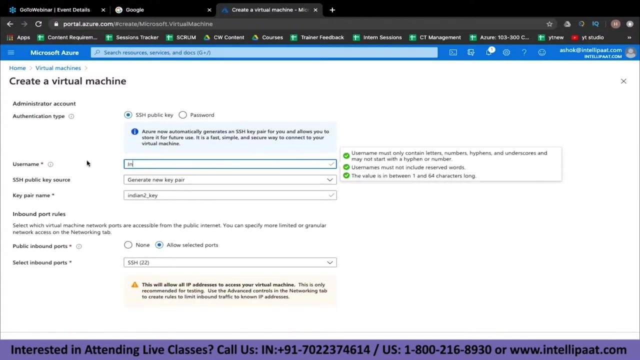 India. so let's add one more. it will be in the resource group called demo webinar. what's the machine now name? it will be Indian to it. even south, in a region. same image, same server configuration. you know the name would be entire part and let's kill the password. same, okay, let's go to. 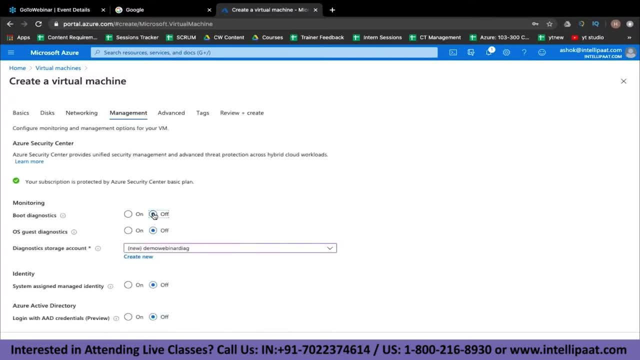 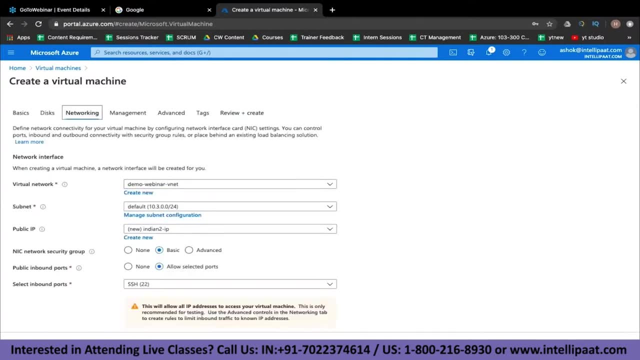 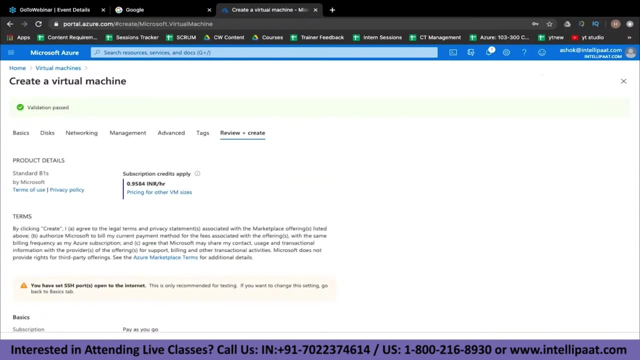 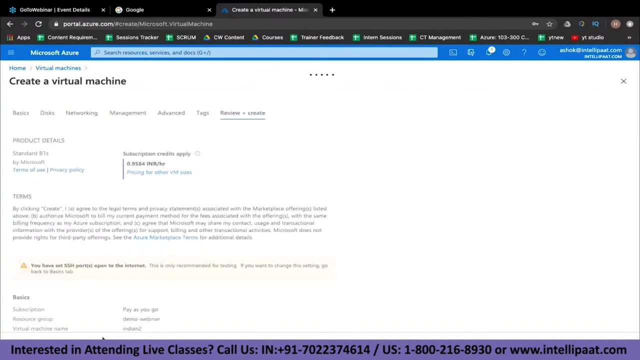 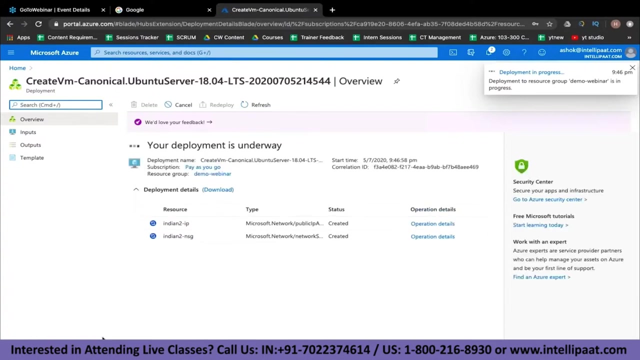 management, turn off boot diagnostics, and now let's create it so in networking. let me see, yes, so we are under the same network that we created earlier, and now let's just go ahead and create this. you all right? so, with this, guys, we have now deployed two servers in the India region. 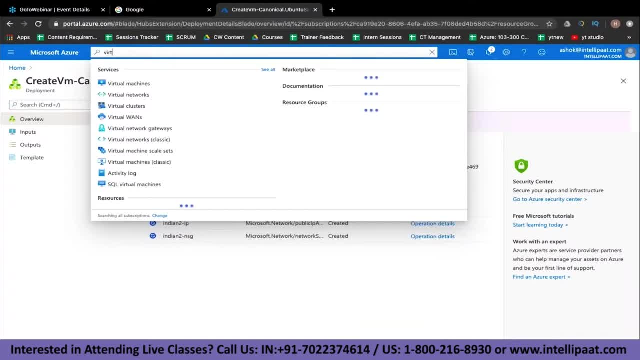 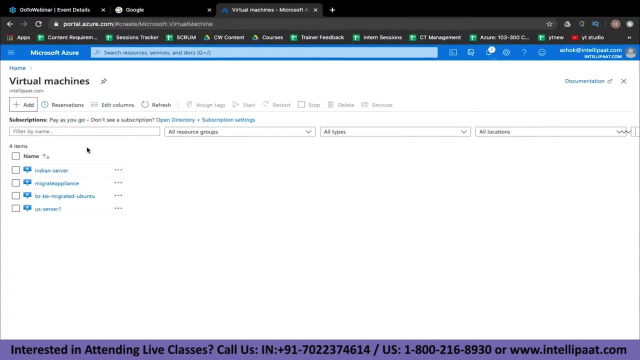 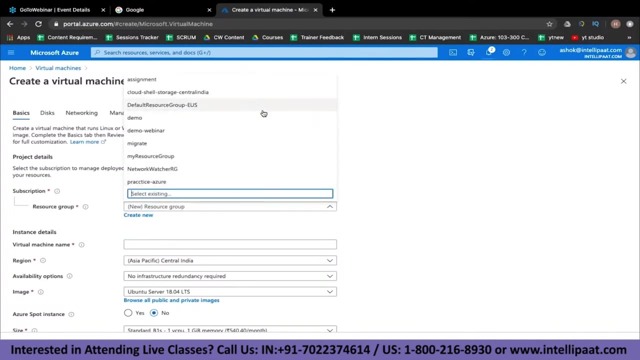 and let's do the same for us as well. let's deploy one more last pm or a US region as well, so this will be in the US resource group. you, okay, we have 500 components here, 0 ever current. okay, so let's do this. we are in. 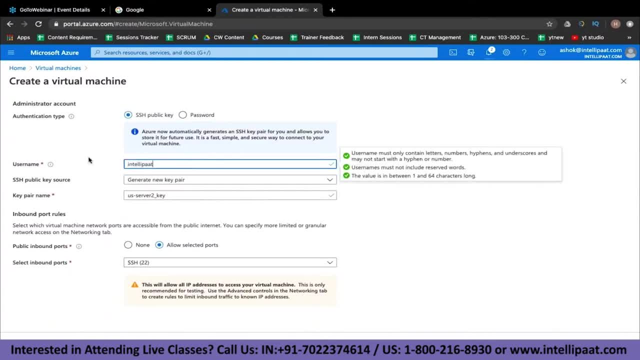 India which machine right, and what your machine is going to be named as USכולan server out to. it's going to be in the best you s same machine config, user name would be impressed and password would be the same what I entered for those again. finally, we filled out test. but hey, go ahead and go next example and develop by that. we'll do that as well. let's begin with congressional mechanics and CPU together as we go ahead and move on to this next example, and I think there's a lot of information involved there, because it is here between 2-4 to 5-9 most lt boys questions. that is basically near quero cantilevers, nothing else, because we created this. well, what if the operation is it is released directly on one console network, orников úcthis example. it is here. ok, and I will see that. second is that Lehman Street and India was in a global, beautiful static in terms of. 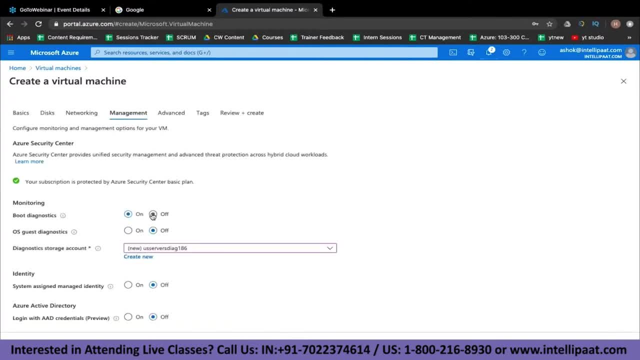 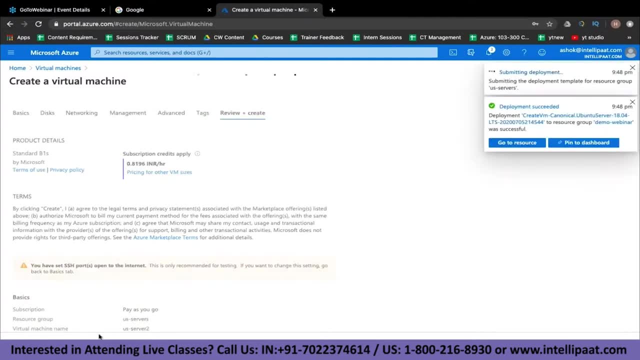 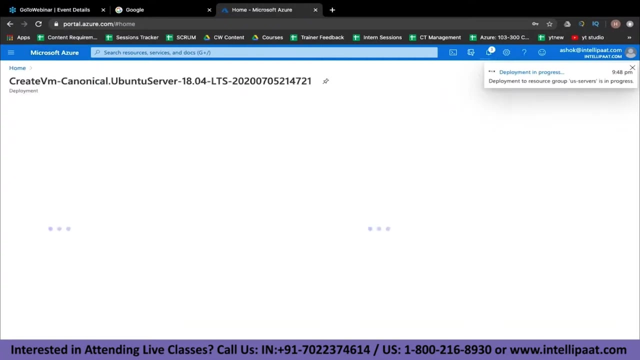 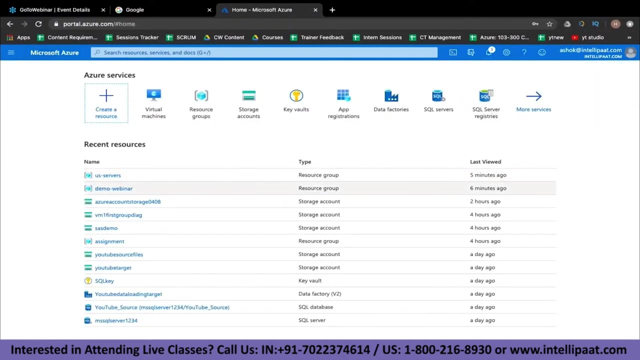 finally, we'll go to management, turn out diagnostics, click on review plus, create and create the vm now. okay, so now this will be deployed in the background and what we can do is we can start configuring our server now. okay, so let's head over to the us server. sorry, the 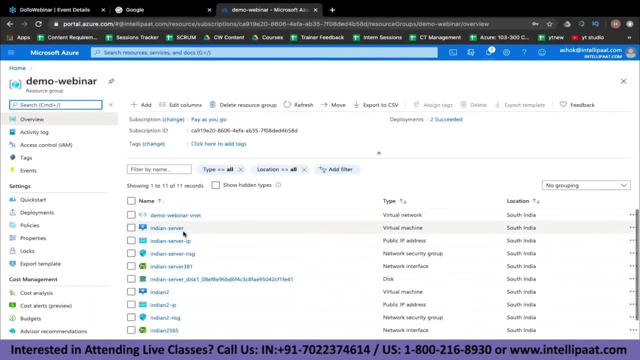 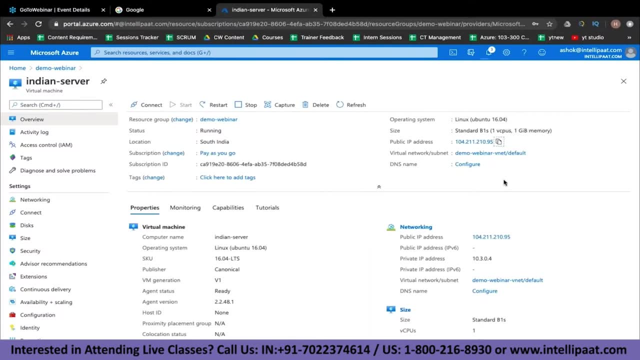 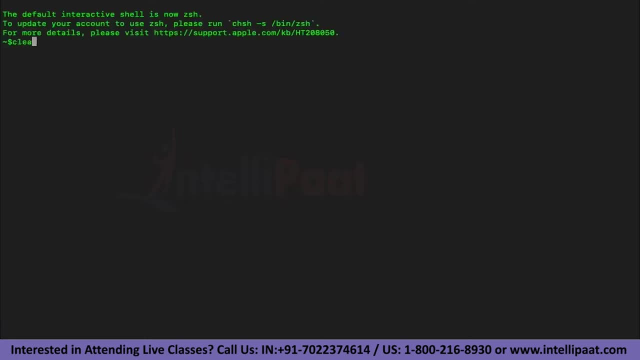 indian servers first and let's try to configure the first server that we deployed. so this is the ip address of the server. let's connect to it. so for connecting you will first need a terminal. so, people who are using windows, what you can do is you can download a software. 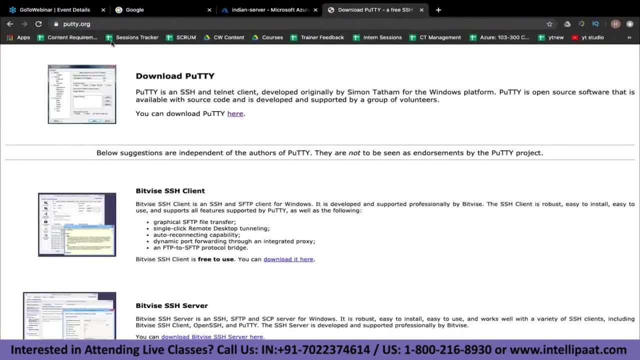 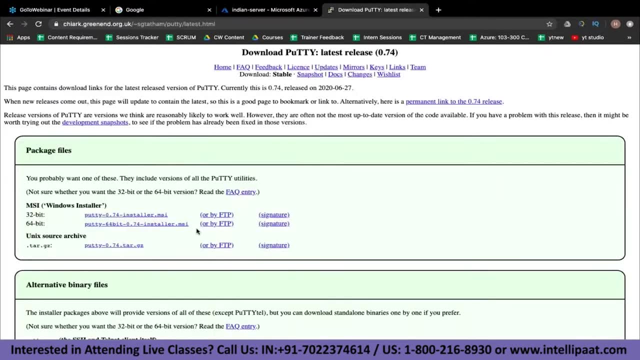 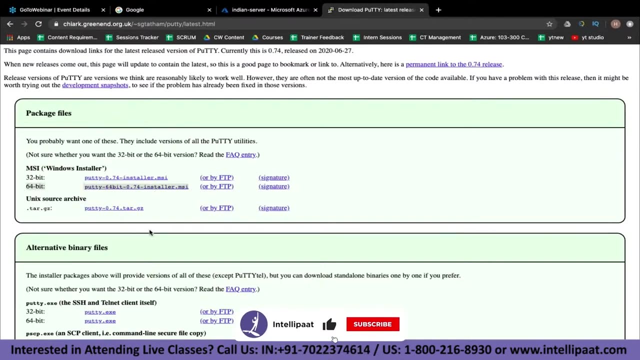 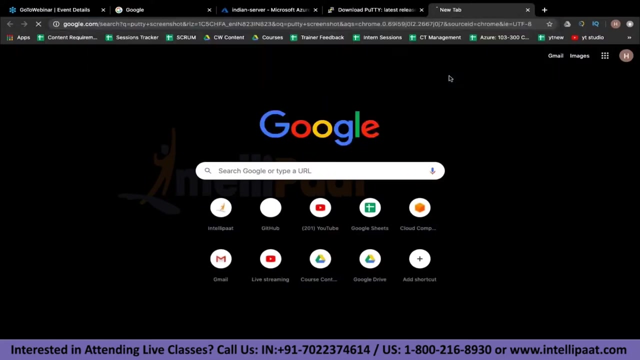 called putty, right, so you just have to go to puttyorg, go to download putty, just click over here and then what you have to do is you have to download the p64 bit version, which is this, right. and once you download this, uh, you know you will see a window like this: 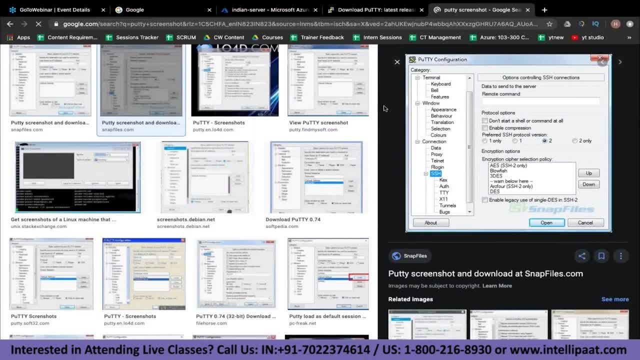 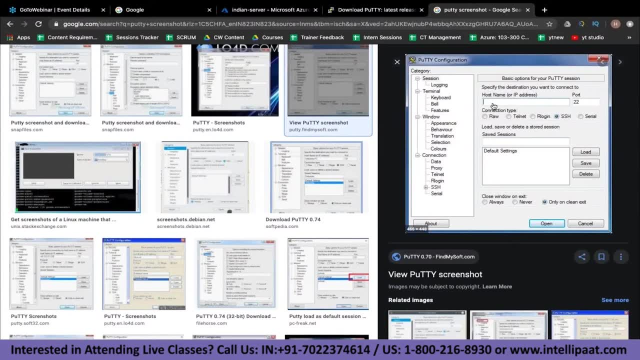 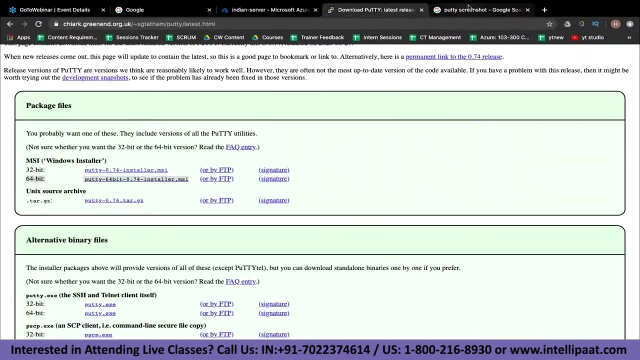 right. so in this window, all you have to do is, uh, okay, one second. yes, this is the window that you will see, so just enter the ip address over here of the server. so in this case, the server's ip address is this: just enter that over here and click on open. right, and that is about it. same screen then. 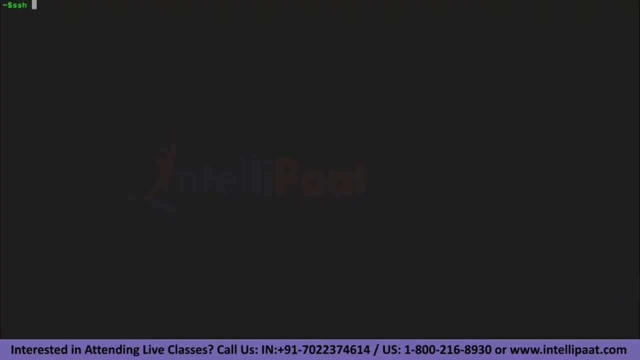 you will see, as i'm seeing right now. okay, so i'll just enter ssh. so, people who are there on linux or mac, you just have to enter this command, so ssh, and teleport, at the rate, the ip address. but enter, i think yes, it'll ask the password, so just enter the password of the server. 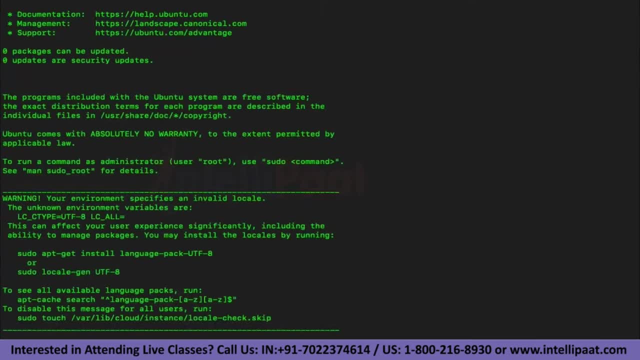 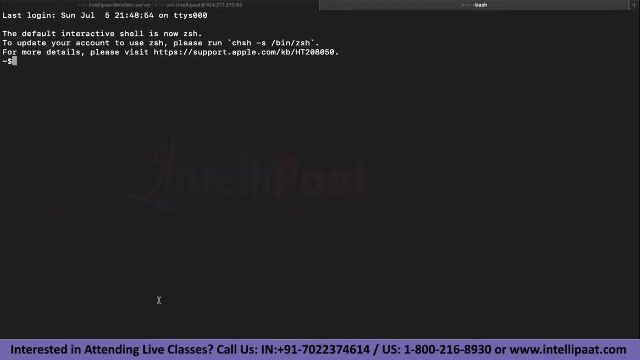 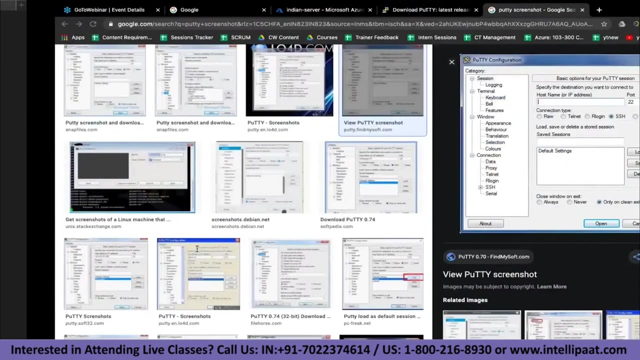 even the putty guys will see the screen. and then you are now logged into your intellipa- sorry, your indian server in the azure region. so this is your first server. let's connect to a circuit second server as well. so ssh and telecom at the rate, and then the second server. 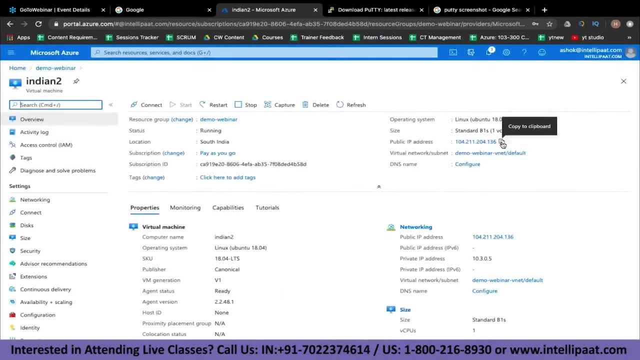 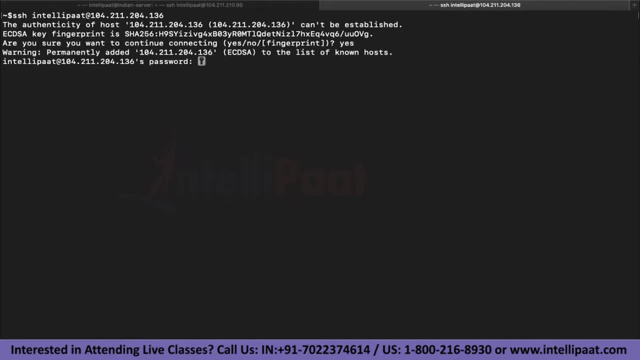 is this: uh, let's copy the ip for this server as well, put in here, and now it's asking the password and, yes, you are now connected to your second server as well. okay, what i've done is i have deployed four servers, two in the us region. 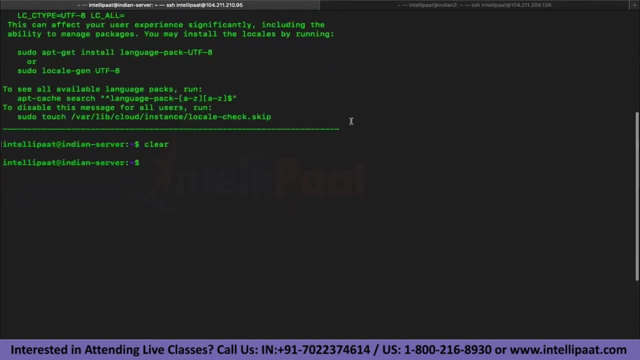 india region, and now i've connected to these servers in the india region. all right, guys, so let's go ahead and configure these servers now. so what i'm going to do is first, i'm going to basically install a web server software, which is called a party apache 2.. so, in order to install that first, 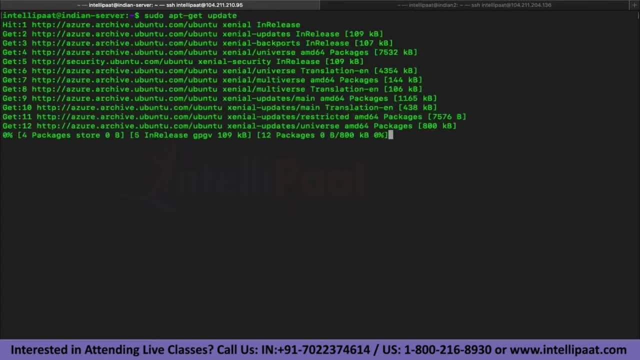 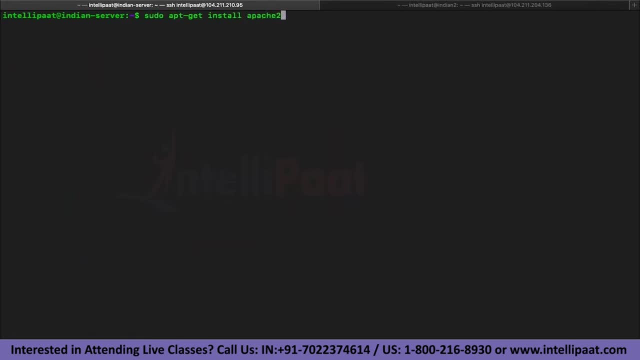 we'll have to update the machine. so let's update it by typing in the command so we get update, and once the servers are updated, now let's install the software by using this command, which is able to get install apache 2.. now let's install the software by using this command, which is able to get install apache 2.. 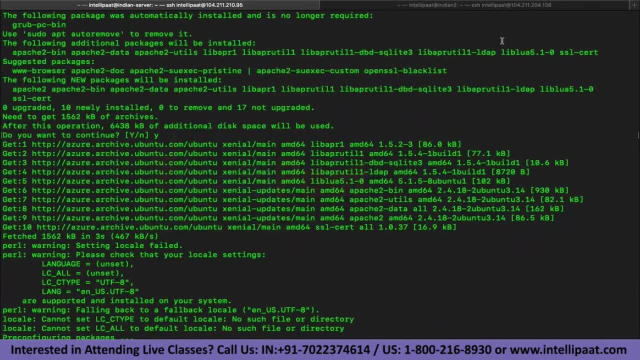 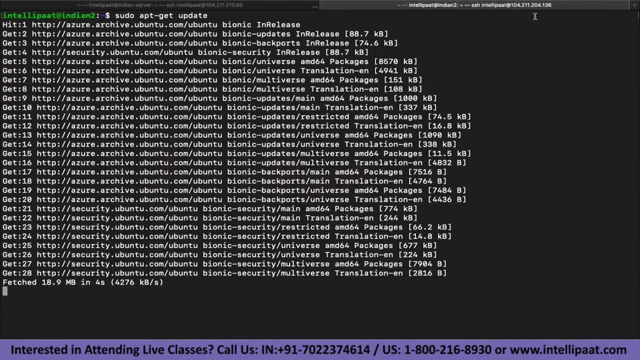 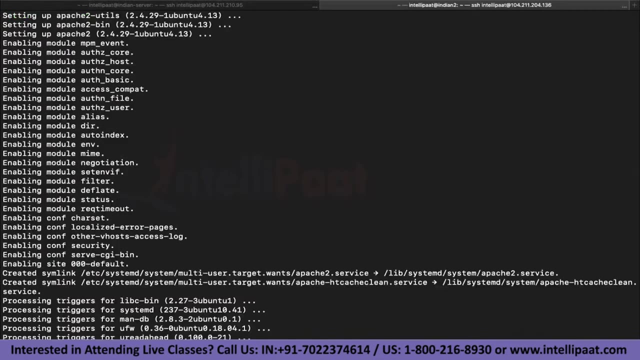 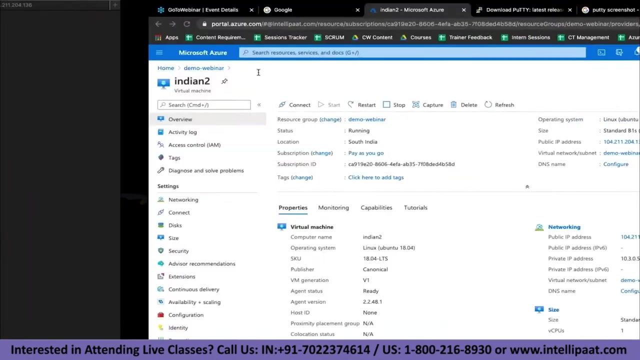 okay, so the software is being installed over here. we can do the same on the other server as well. first update it, and once it's updated we will install the apache 2 software. so both the machines now have the apache 2 software installed, and now let's try to see if that software is working or not. so ideally, what should happen is if: 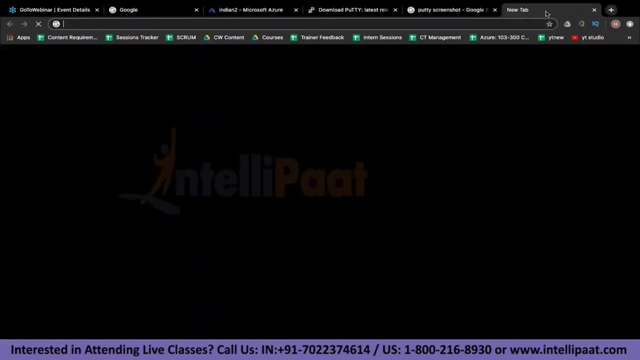 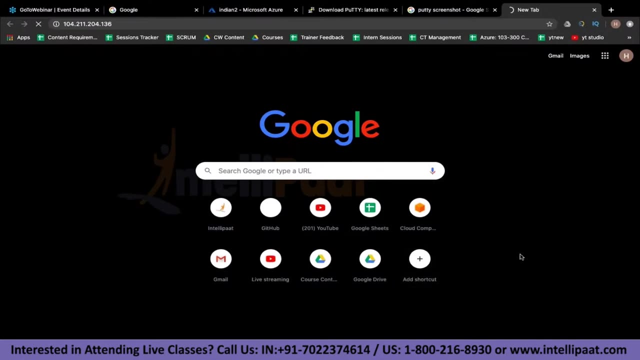 you install the software and if you copy the ip address of your server and try to paste it in the browser, you should be able to see the website that you have just deployed. but what happens is because you know, we have not opened the firewall for, uh, the http protocol. that's why we are not able to. 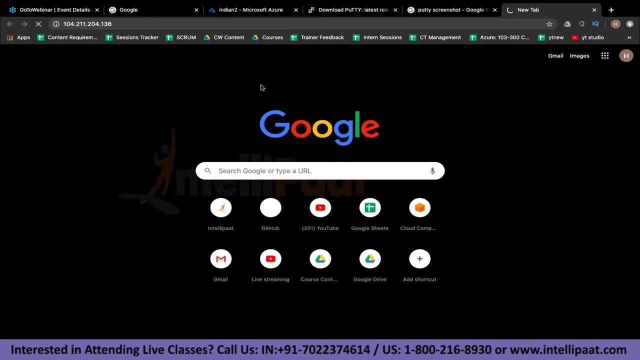 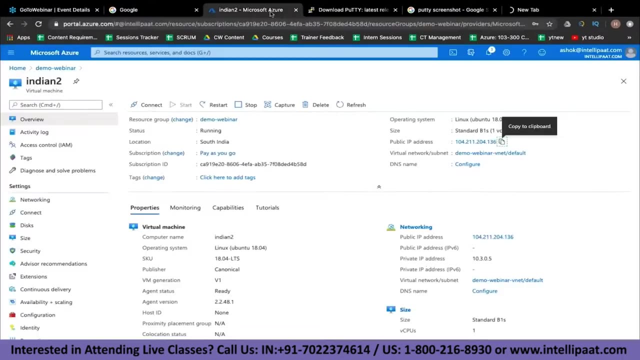 see this webpage right now. you remember, we only opened the port 22, so whenever your browser is trying to interact with your server, it always tries to interact on port 80, and that is exactly why you're not, uh, seeing the web page right now. so what we can do is, let's say, this is my indian server 2. 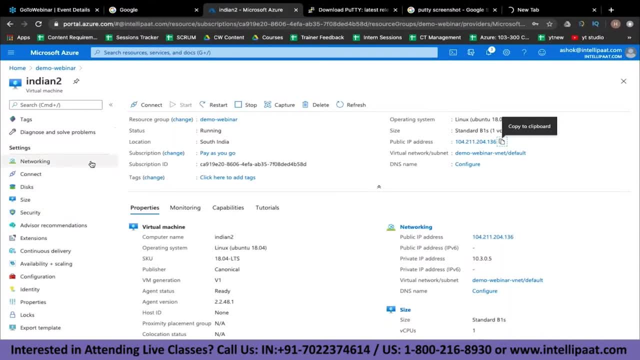 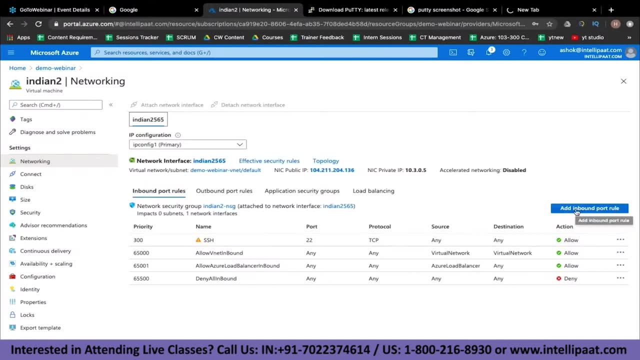 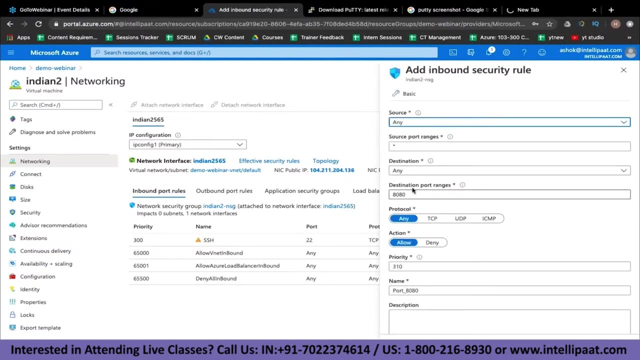 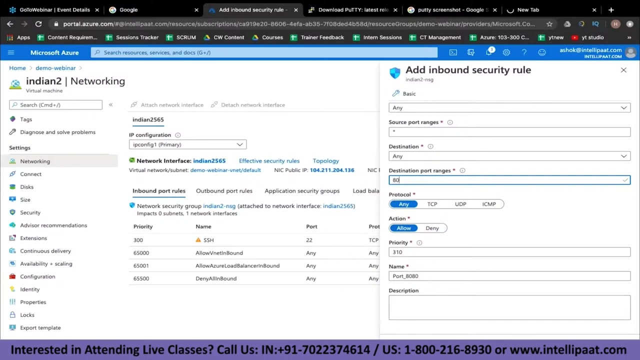 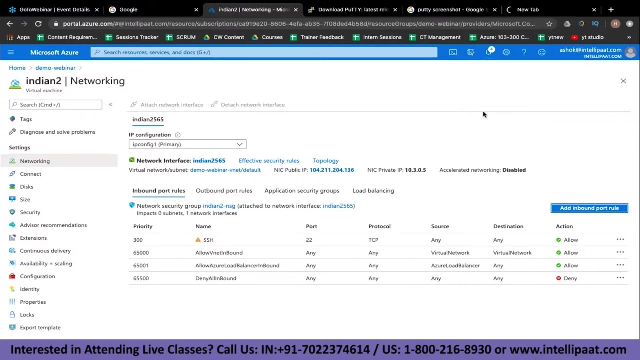 so all i have to go to is networking, and in networking i have to add an inbound rule. so in the rule i have to specify the destination port, which is port 80, and it is going to be allowed, and i just click on add. so with this rule in place, uh, what is going to happen is the port 80 is going to be opened in. 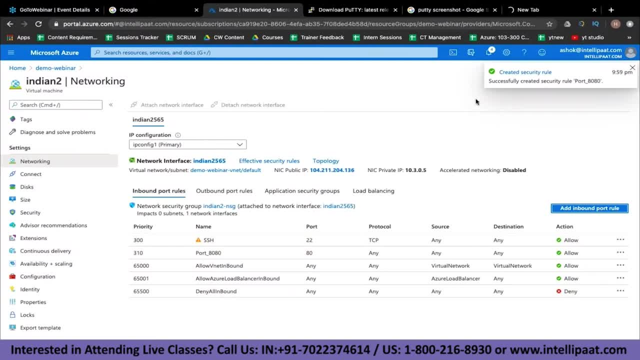 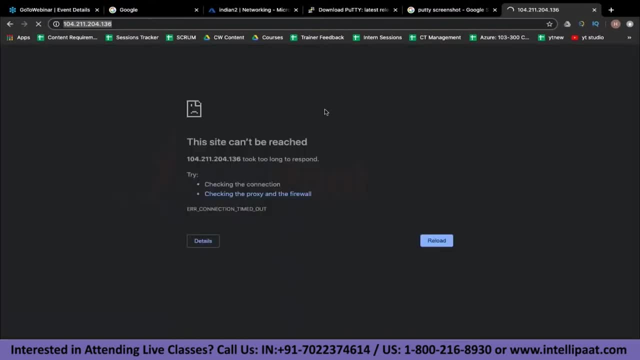 the firewall and then, once the rule has been created, now, right, so this will take around, uh, you know, 30 to 40 seconds to basically get uh a little bit of time, and then we should be able to see this website. so let's wait for some 30 to 35. 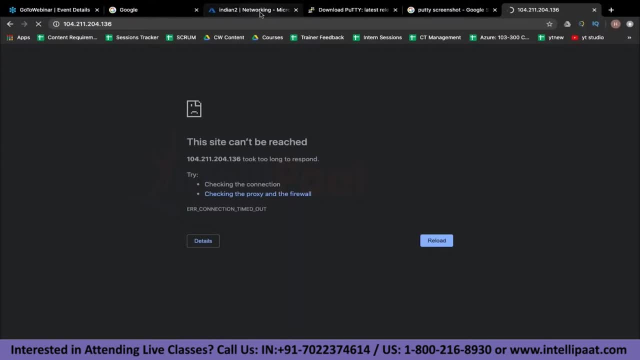 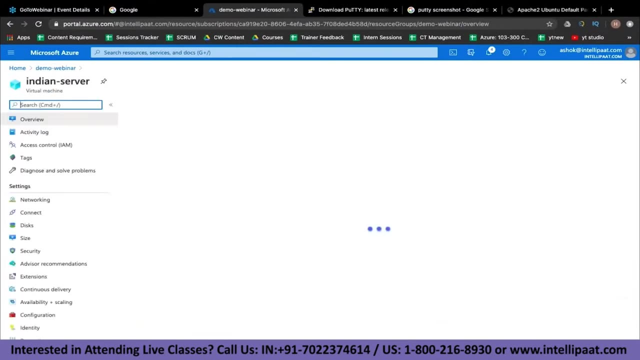 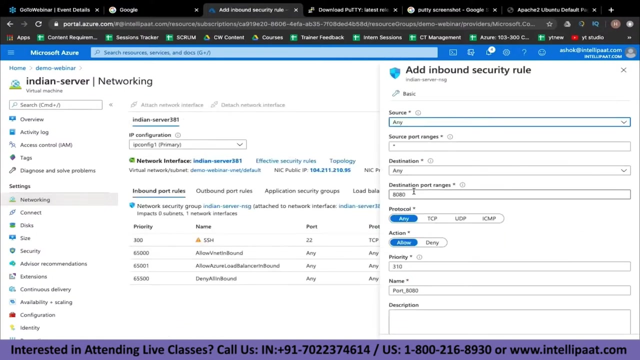 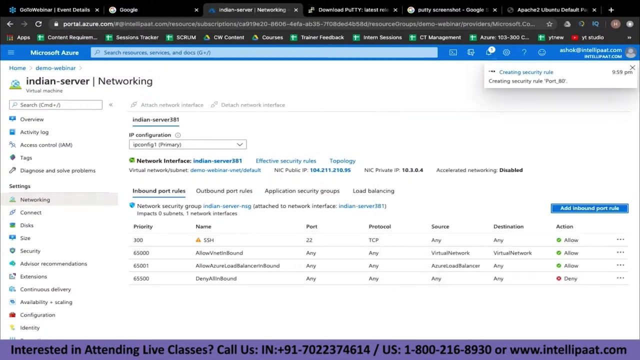 seconds and while this is happening, let's also open the port 80 on the first indian server. so we'll just go to the first indian server, go to networking and add uh, port 80 over here. okay, so this rule is now getting created and if i go back you can see on this ip address i am able. 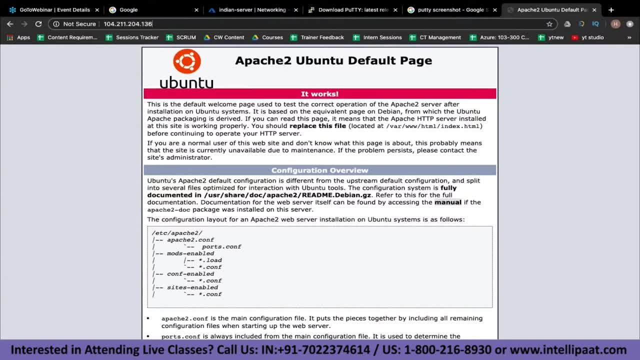 to see the apache 2 page. so this is the indian tools ip address and you're going to change this web page in a little while and i'll show you how you can do that. so to replace this file, what you have to do is you have to go to slash var, slash www, slash html, and then replace indexhtml. 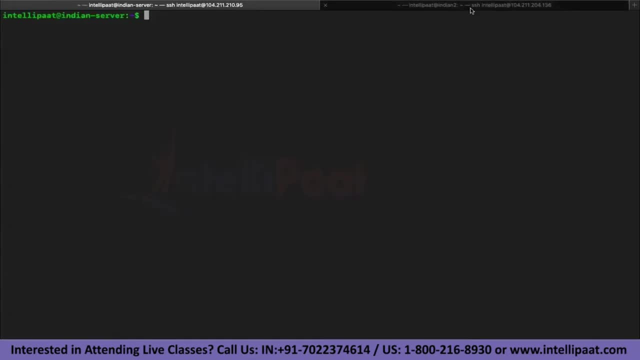 so that is exactly what we are going to do now. so let's go to indian 2 server, let's go to the file location which was mentioned and in this file location now let's delete the indexhtml which is present and let's add one more indexhtml so to create or edit any file. 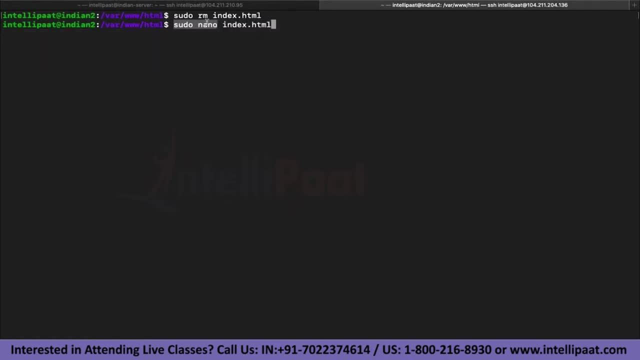 you have to make use of the command sudo nano. so nano is basically just like notepad that you're have in windows, right? so notepad, open the notepad, uh, for you to write in or edit documents. similarly, in ubuntu there is a text editor called nano, right, so we're going to open that and, as you can see it, 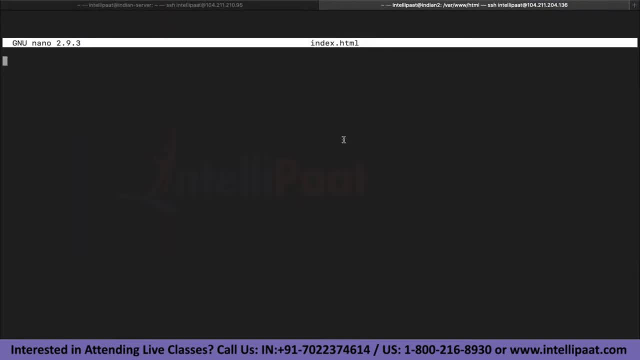 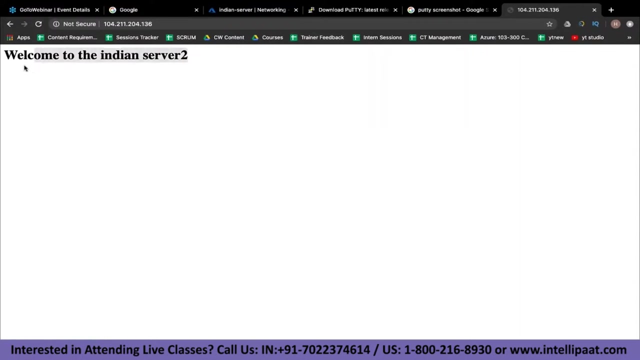 is now creating a file called indexhtml. so let's write a very simple html code over here which is basically: we're just going to have one line which is saying welcome to the indian server. two, right, let's write this html done and now, if i refresh this, you can see it says welcome to indian server. 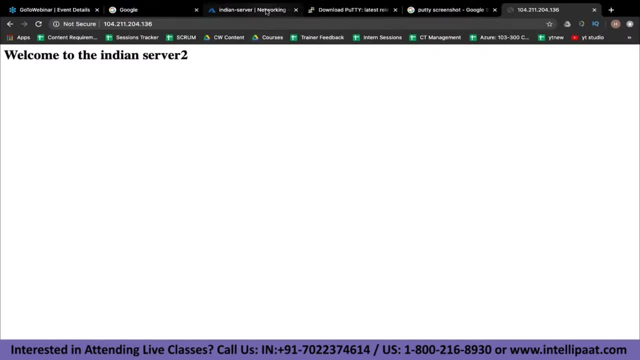 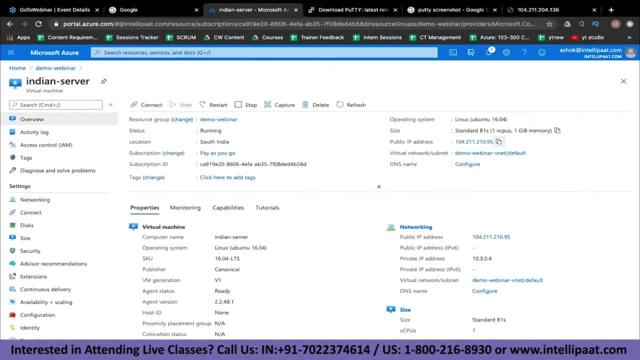 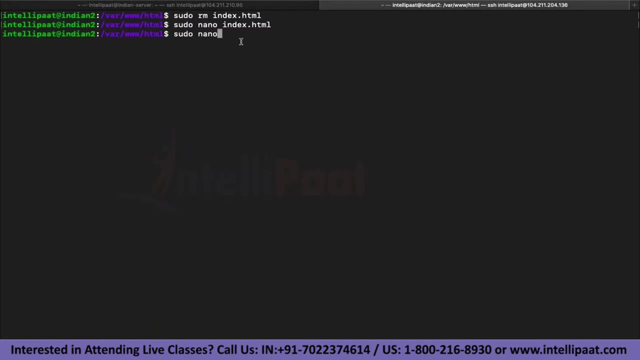 two, which is great. so now let's do the same thing for our first indian server as well. so right now, if i go to this ip address in a new tab, i'll be seeing the default departure to page uh, let's replace that with this code. so what i'm doing is i'll first 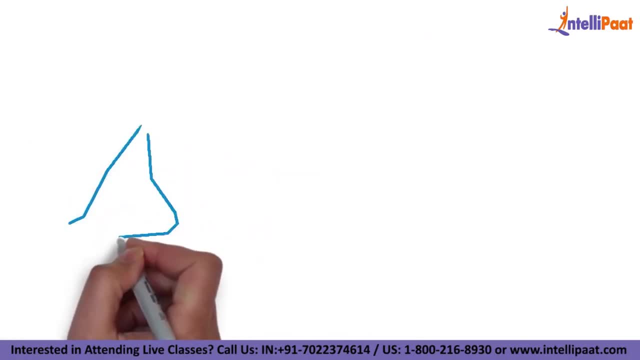 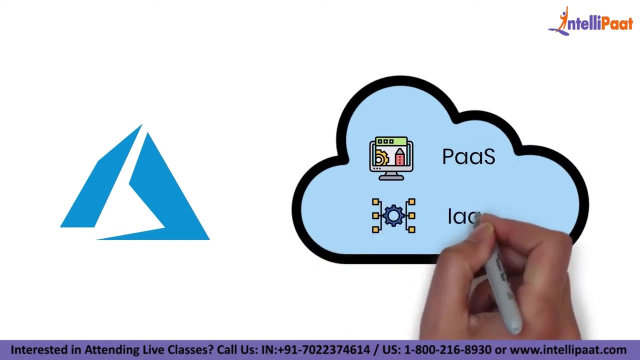 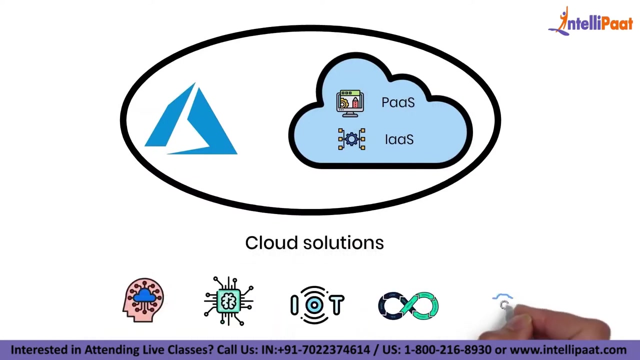 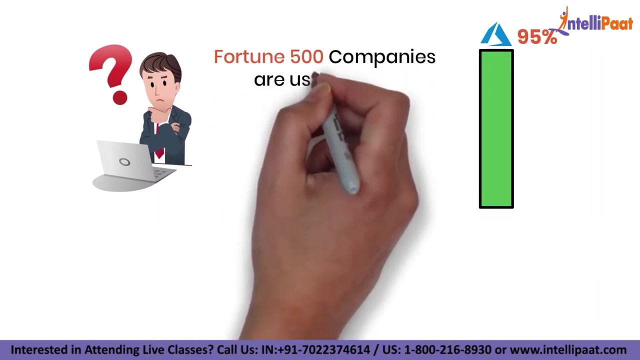 so what is microsoft azure? microsoft azure is a cloud provider that provides various platform as a service and infrastructure as a service products. azure has cloud solutions to all the infrastructural problems by providing services in various domains. did you know that almost 95 of fortune 500 companies are using azure? also, it is five times cheaper than aws in terms of windows. 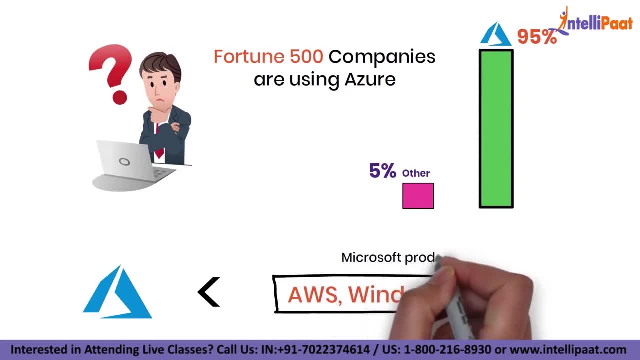 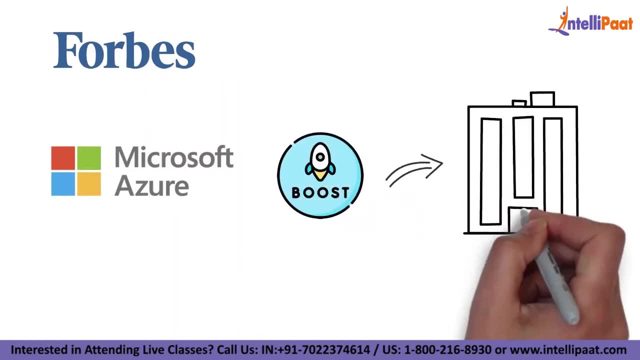 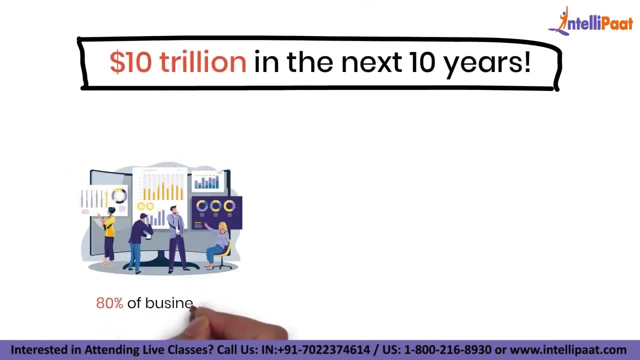 and sql server, because there are also microsoft products. forbes say that microsoft azure is set to boost the size of the it market by 10 trillion dollars per year. that is almost the same as the trillion dollars in the next 10 years. as per predictions, 80 percent of the businesses will 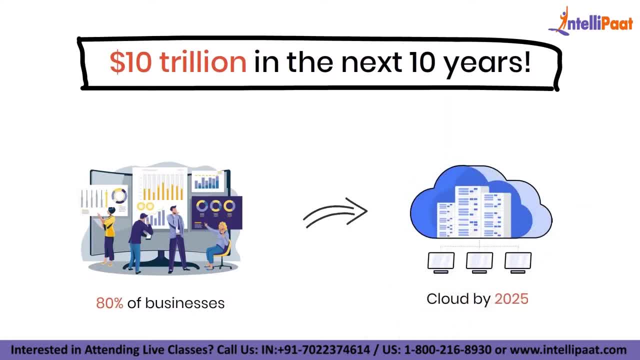 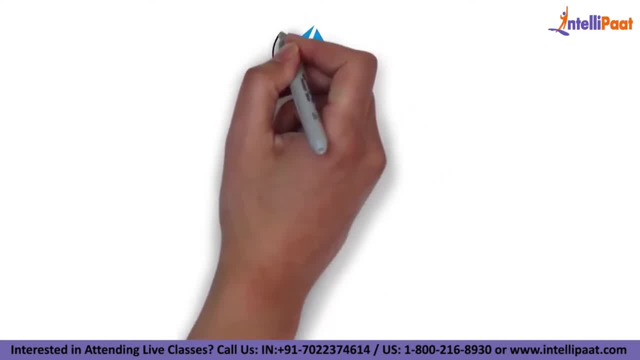 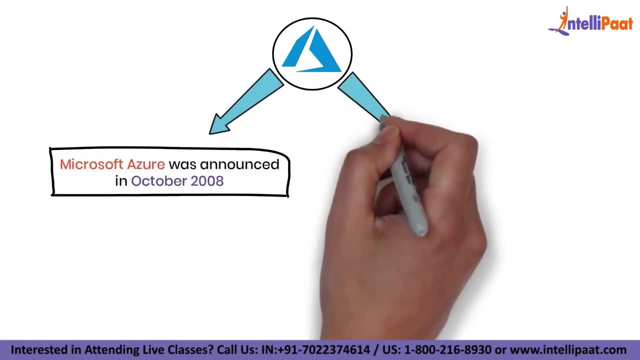 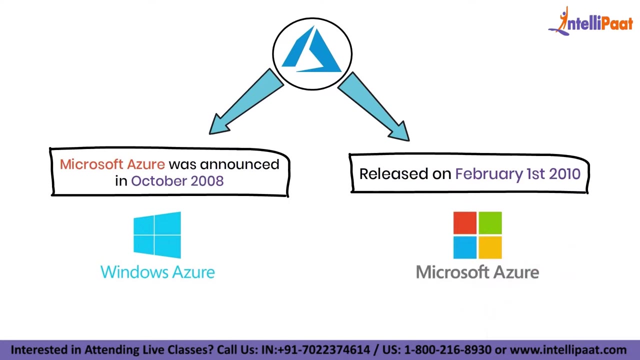 move their workload to cloud by 2025, thus making it a major career to consider transitioning to. for a better understanding of azure, let us start at the very beginning. microsoft azure was announced in october 2008 and released on february 1 2010 as windows azure, first and later named as microsoft. 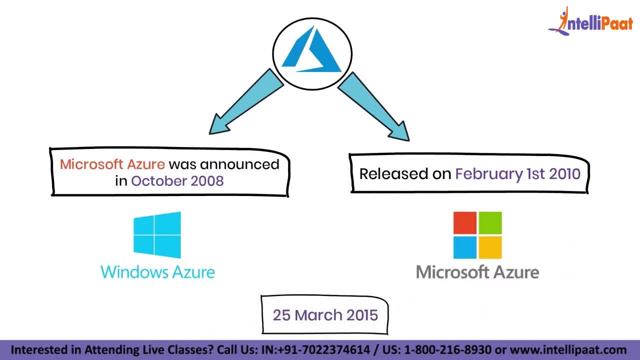 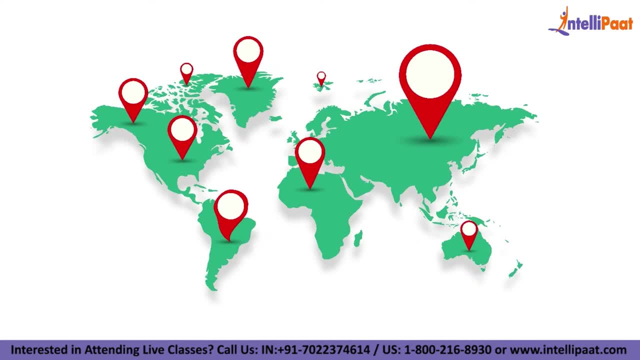 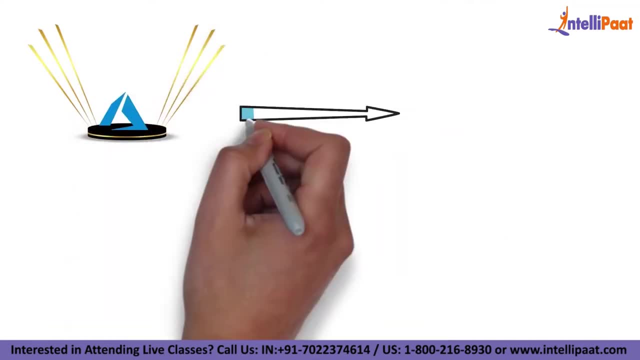 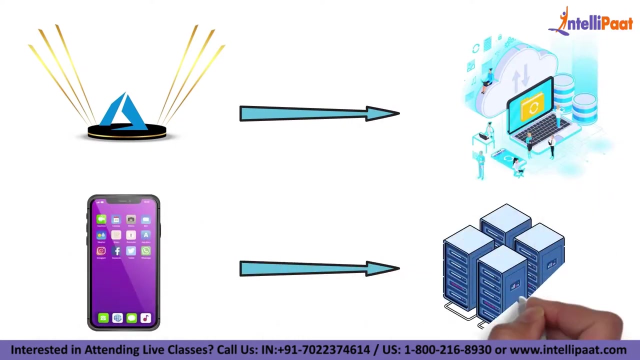 azure on 25th march 2015.. in today's scenario, its reach is in 140 countries and is still expanding, which is pretty impeccable. in simpler terms, microsoft azure is a platform that enables users to engage in agile cloud computing and is designed for creating and managing apps through microsoft's data center. now there are 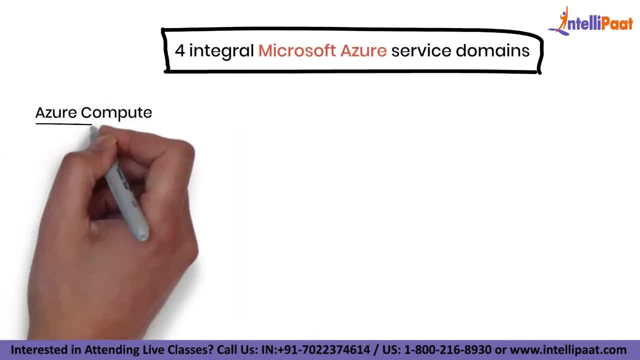 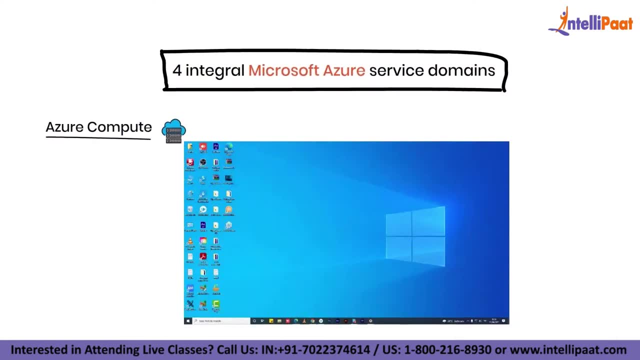 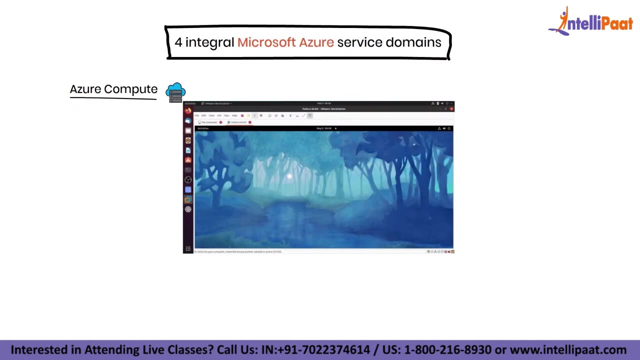 four integral microsoft azure service domains. the first one is azure compute. compute is the most integral domain in azure as it brings everything together with azure virtual machines. you can get on-demand scalable compute resources. azure virtual machines, app services and container instances are some popular tools for creating and managing apps through microsoft's data center. 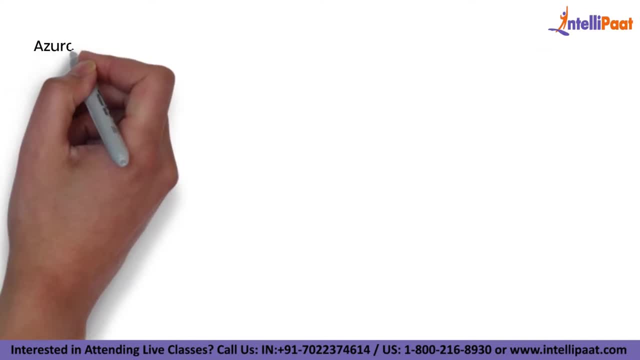 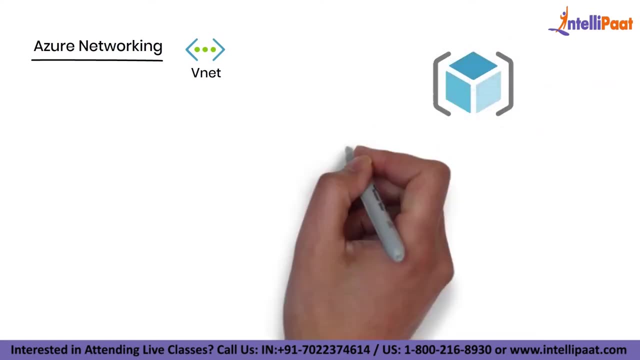 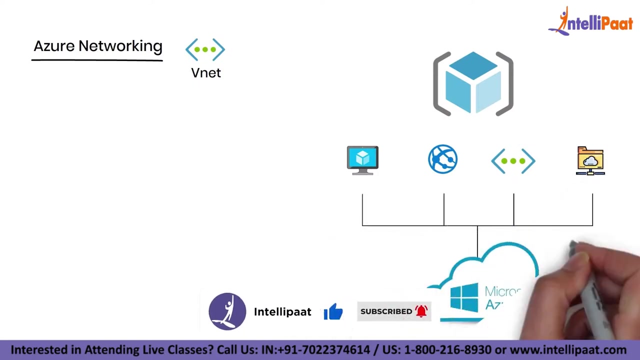 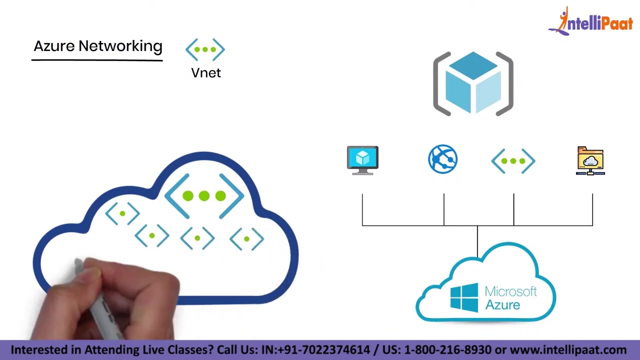 second, we have azure networking networks from the cloud networks. in azure, vnet is the networking tool that connects all azure resources together. these networking services allow enterprises to safely connect their on-premises services to the azure cloud. it is also used to manage virtual private networks and further create multiple virtual networks on the cloud. the third one is: 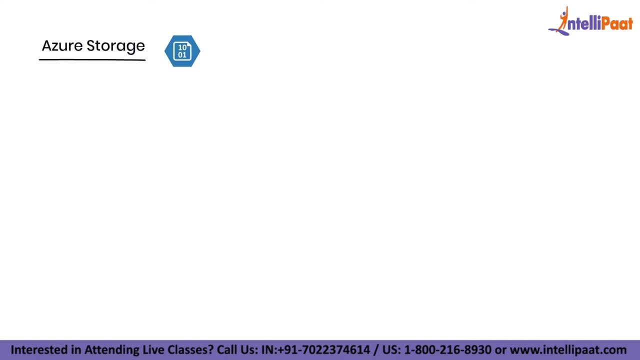 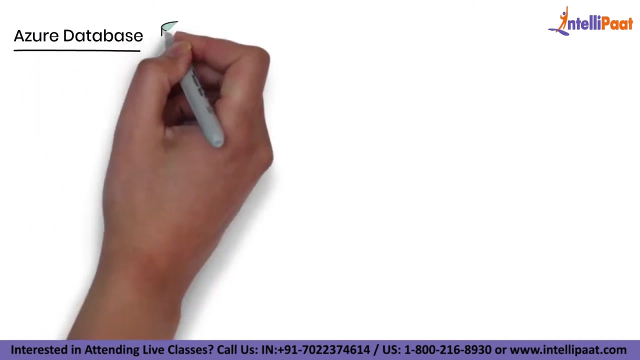 azure storage. azure storage provides storage solutions that are more durable and large-scale applications. data-driven applications can be built without any hassle. azure automatically scales the storage requirements according to the usage and it automatically balances throughput according to the connections made. and the last one is azure database. azure provides relational databases, no sql databases. 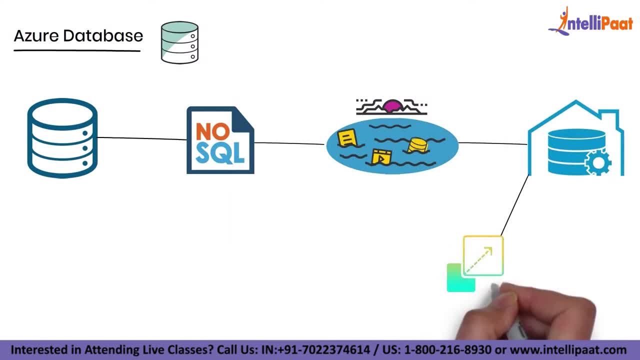 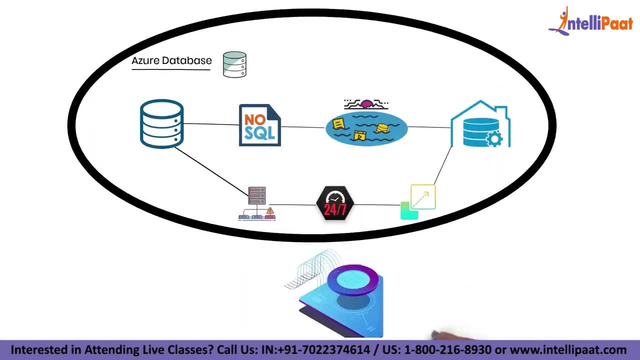 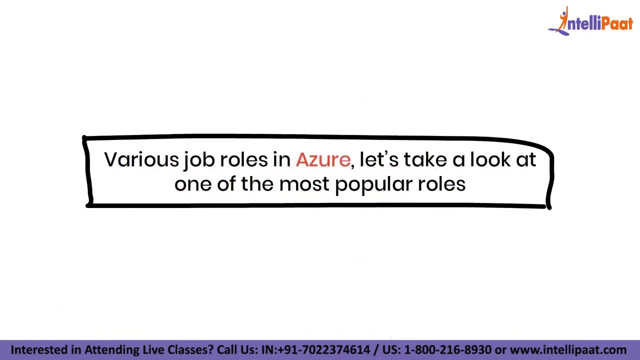 data lakes and data warehouses. it provides a scalable, high available and fault tolerant database server and lets you scale according to the incoming data. there are various job roles in azure. let's take a look at one of the most popular job roles: azure developer. an azure developer is a. 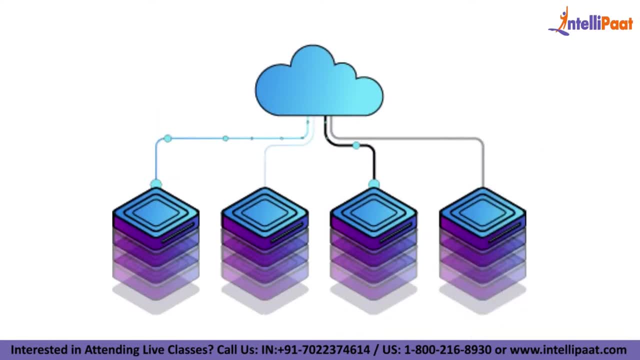 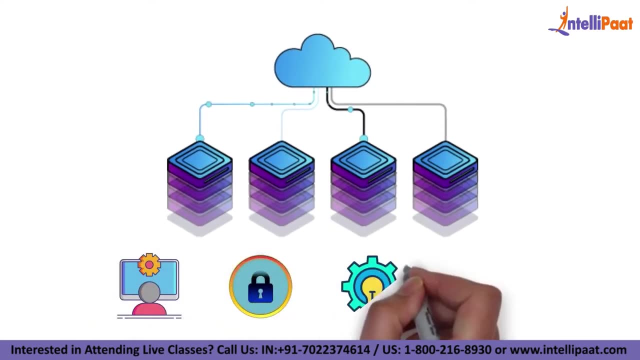 cloud professional who creates cloud-based applications making use of the benefits of the cloud architecture. if you are a professional cloud developer, you can create cloud-based, cloud-based applications making use of the benefits of the cloud architecture. if you are efficient in testing, security, development and deployment, then a career in azure development. 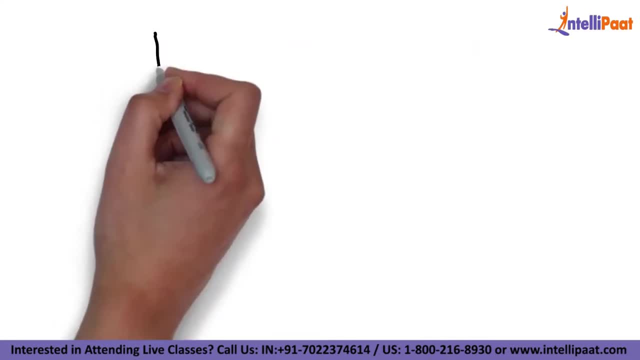 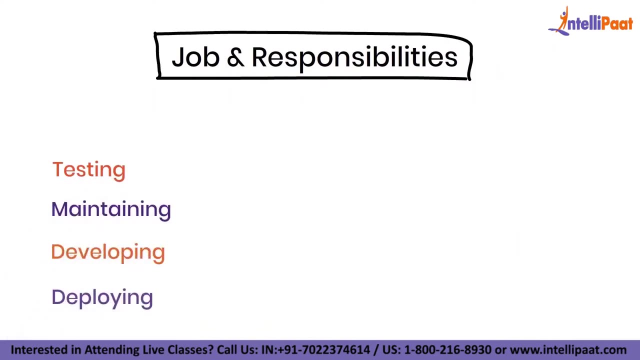 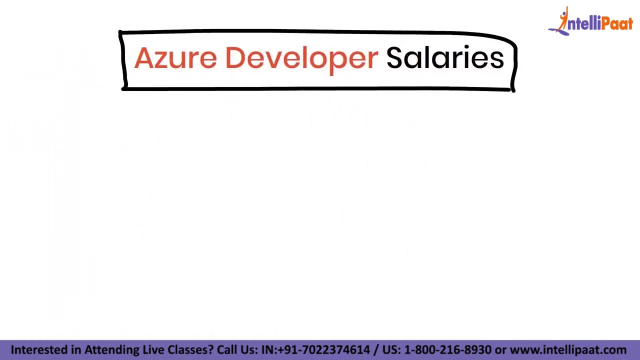 is somewhere you will fit in well. the job includes responsibilities like testing of applications, maintaining, developing and deploy them on azure. it also includes participating in all phases of development and having the ability to work side by side with cloud administrators, clients and cloud architects in univ In the United States, on average basis, an Azure developer gets paid $132,148 per annum. 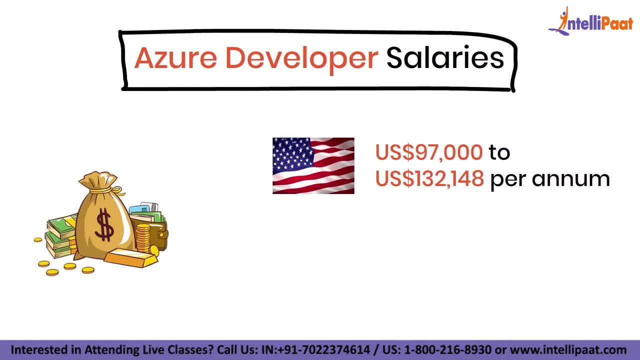 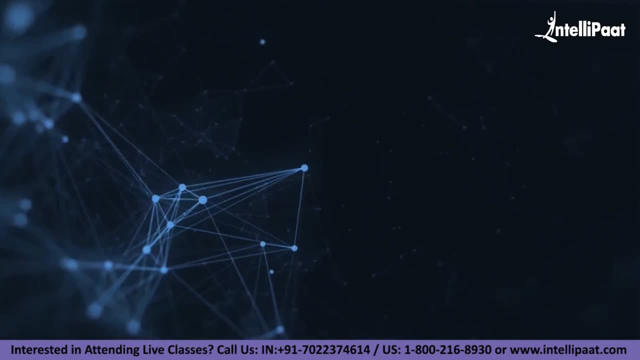 However, for an entry-level developer, it's $97,000.. Whereas in India, the salary offered ranges from 7 lakhs to 25 lakhs per annum. That's all about Azure. Just a quick info, guys. Intellipaat provides Microsoft Azure certification training. 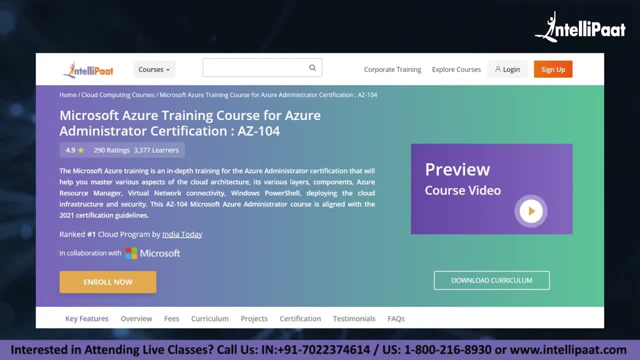 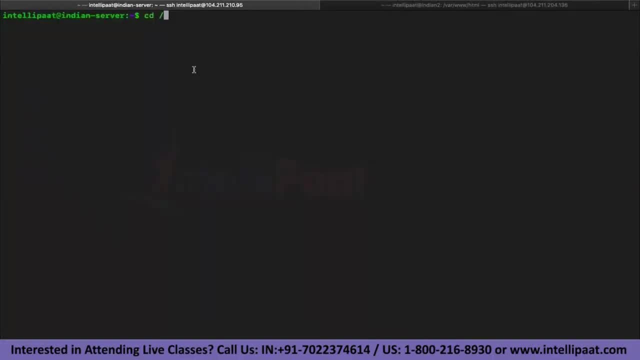 in partnership with Microsoft, mentored by industry experts, The course link of which is given in the description below. Now let's continue with the session, Go to the file path, And now I'm going to paste the code that we wrote over here. 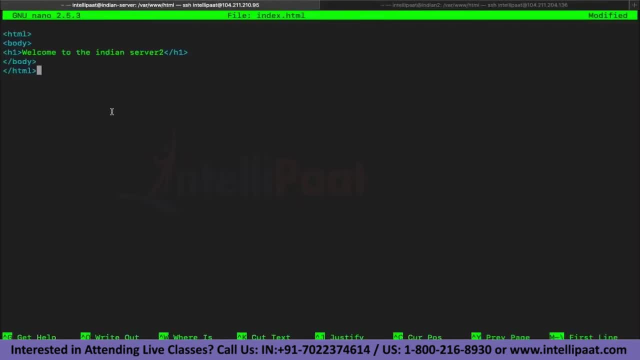 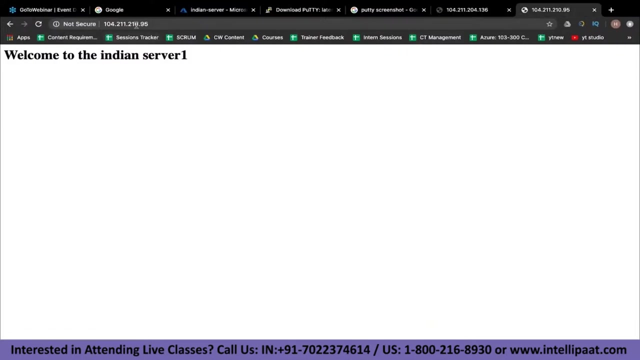 Into this file And change this to Welcome to Indian Server 1.. Okay, done, And now, if I refresh it, Great. So now I have two IP addresses where, if I go from the browser to these IP addresses, I am going to see Indian Server 1 and Indian Server 2.. 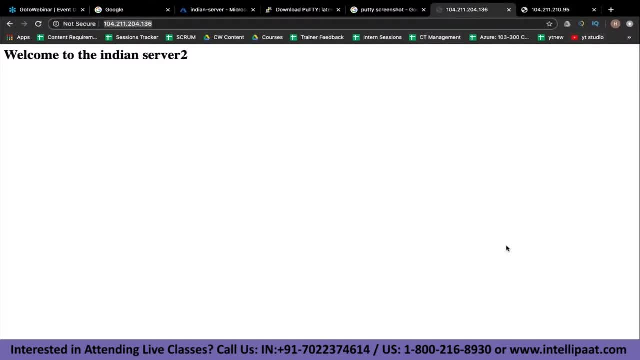 So let me give these IP addresses to you guys as well. So just open your chat section And you should get these IP addresses. Just try it in your browser. I'm going to put a load balancer on top of them, Okay. 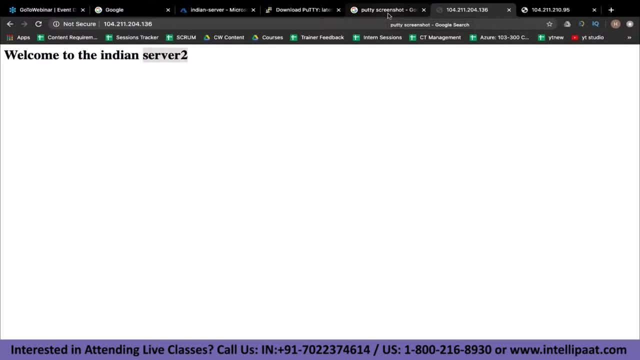 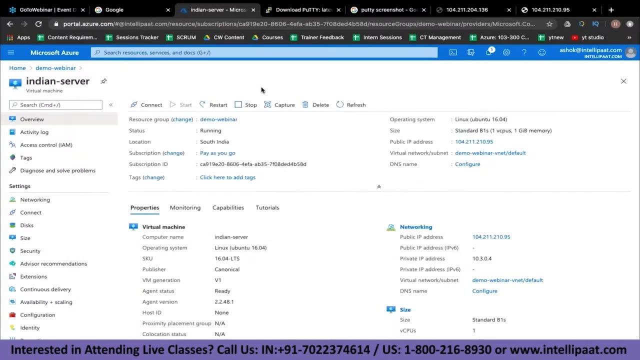 So let's see how we can do that. So there are a lot of type of load balancers that basically you can deploy. The load balancer that we are going to deploy today is basically an application gateway. Okay, So let's go to application gateway. 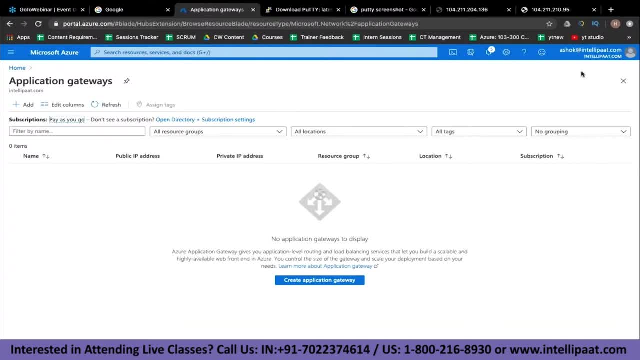 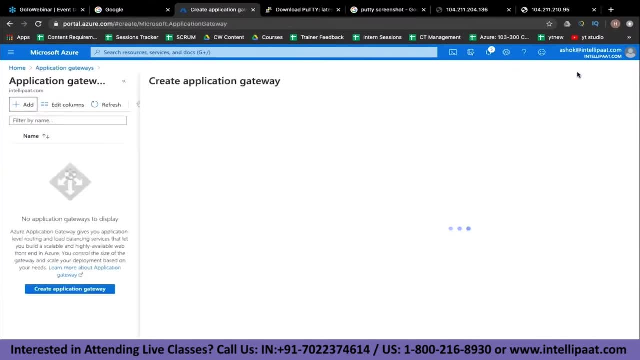 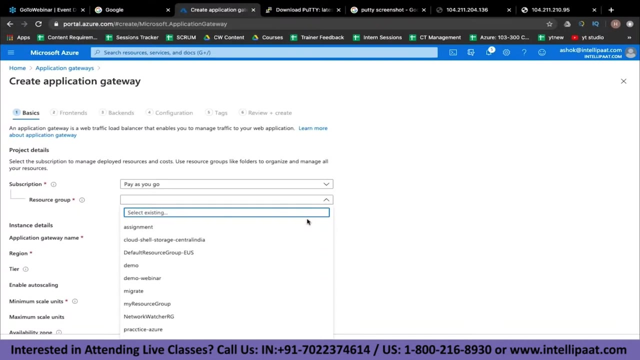 And in application gateway. all we have to do is So there are. Yeah, So we'll just click on add. And now it's going to ask us which resource group we want to deploy it in. So we will, Let's first apply. deploy it for the US region. 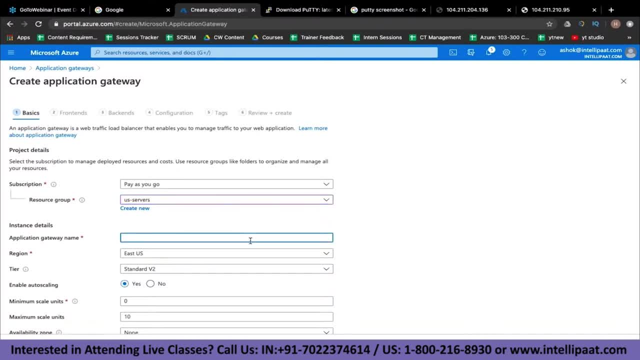 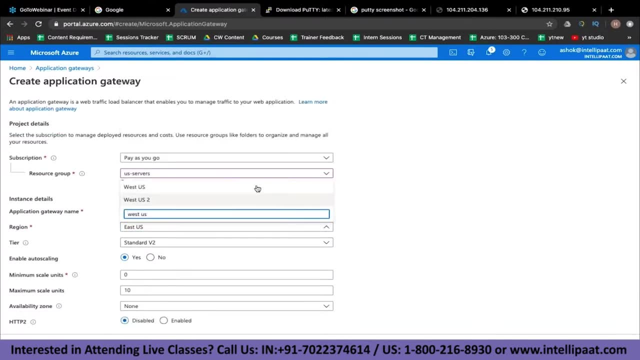 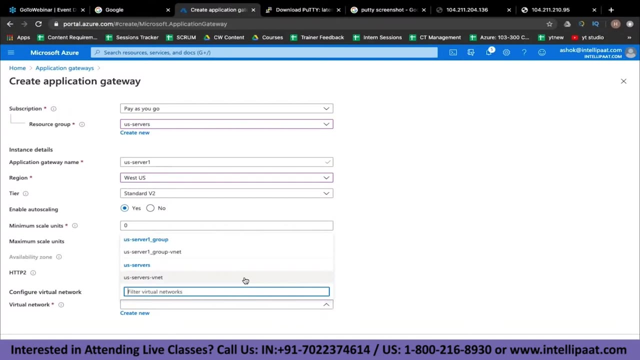 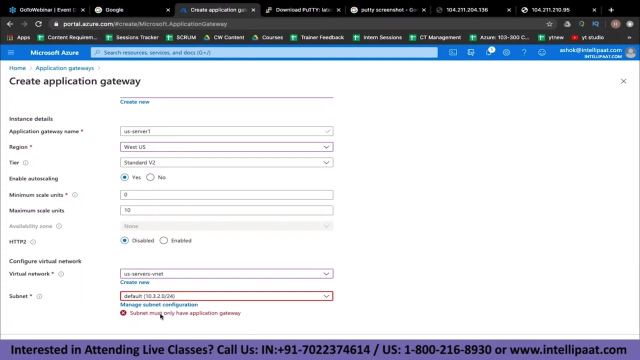 So we are going to say US servers, application gateway, Let's say us server one- The region is best us- And virtual network. This is the virtual network to deploy it in. Now this is the error that you will get. It says the subnet must only have application gateway. 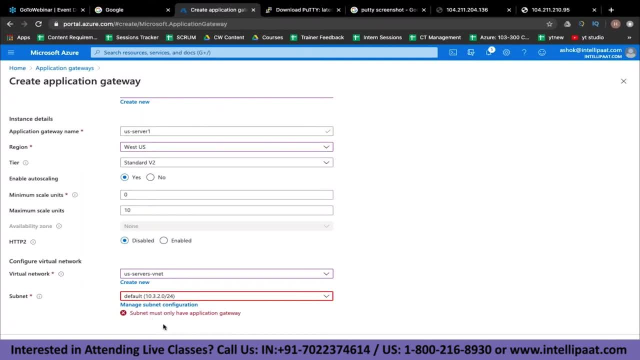 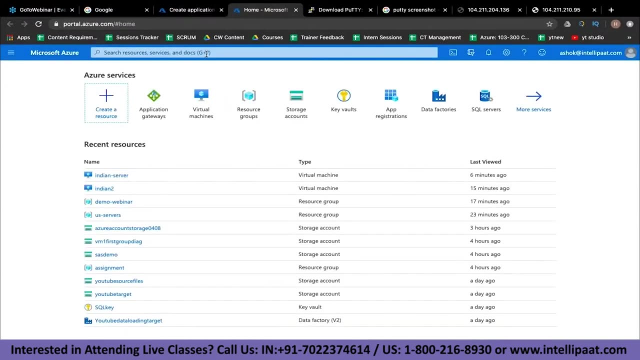 Now, in order to have this, what you'll have to do is you will have to create a subnet Which is not going to have any other resource. All right, So how we can do that is just go to your as your portal. 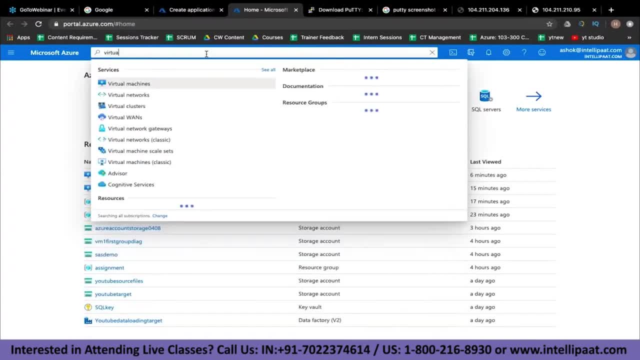 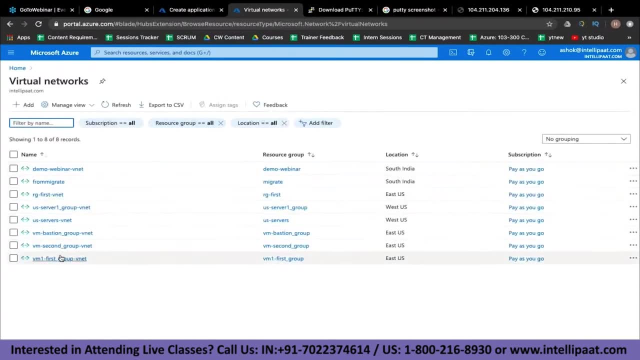 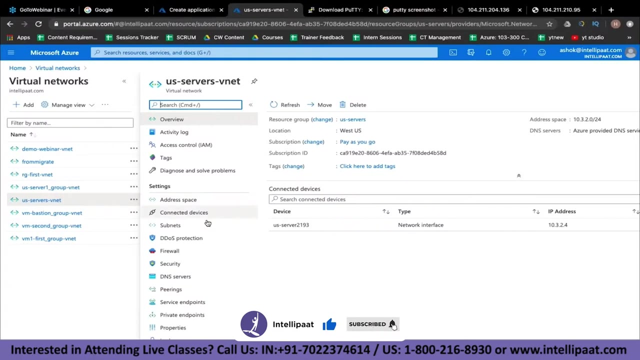 And then go to virtual networks. Now, the network that we want to configure is the Usos Right And in this, If you go to subnets, you can see there's only one subnet right now, Which is the default subnet. 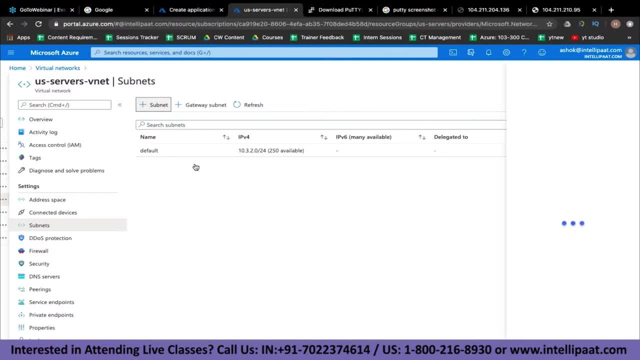 So let's add one more subnet And let's the address name for this. Now the address range can be a little confusing to you, So let me make it as simple as possible for you guys. So right now you can see the address range. over here is 10 dot 3, dot 2, dot 0, slash 24.. 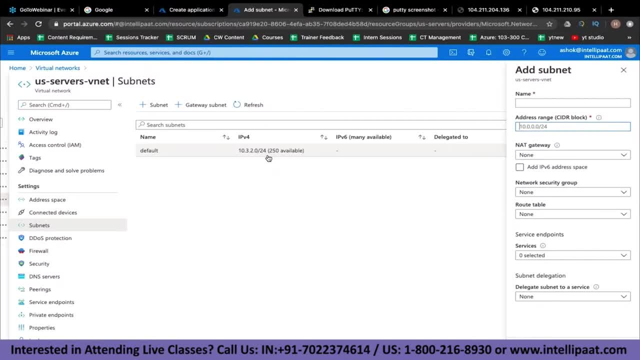 So slash 24 basically says how many IP addresses Can be included. So if you type in slash 24, it gives it 250 IP addresses in the range of 10 dot, 3, dot 2.. It could be dot 1, dot 2, dot 3, dot 19, dot 99.. 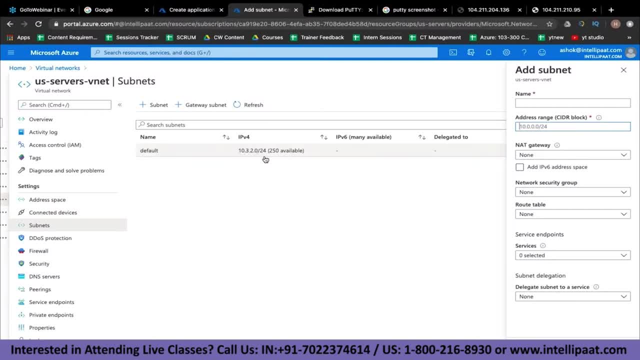 Right, Etc. So that could be the range. So, similarly, we just replicate this and we'll specify 10 dot, 3 dot instead of two. we can specify, Let's say, five Dot 0 slash 24. Right. 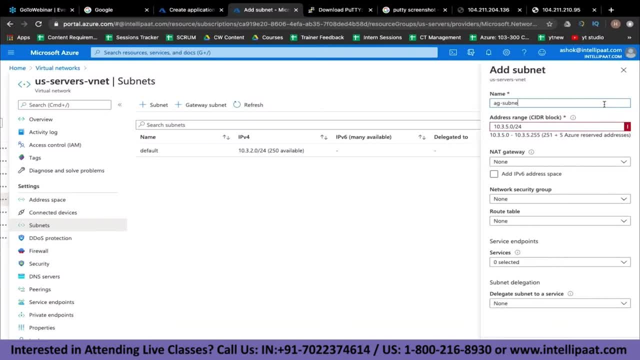 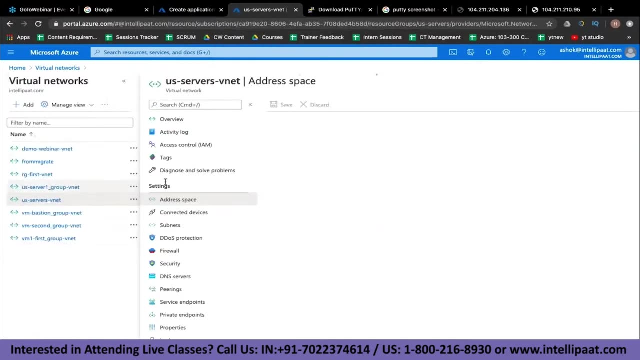 And let's say this is for our AG subnet. Okay, So it says the subnet is not contained within these address space of the virtual network. Okay, Let's solve that as well. So we first have to go to address space So we can. 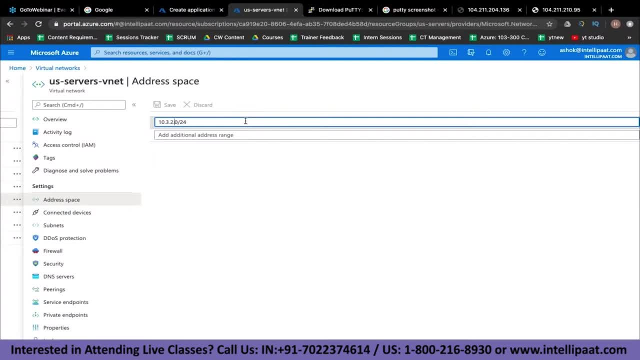 So here the address space is this. So instead of This range I can give a better range, which can be slash 16.. So the lower the number, the higher number of ranges you get. So, as specified in slash 16 over here, 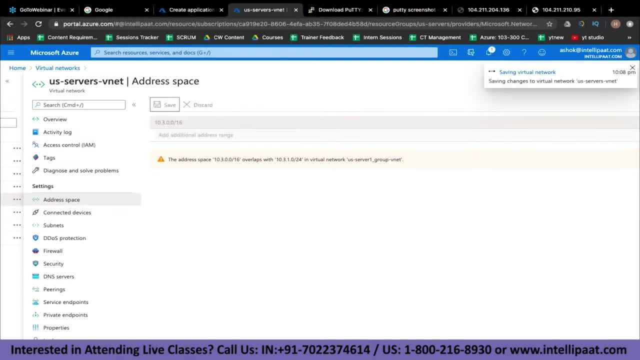 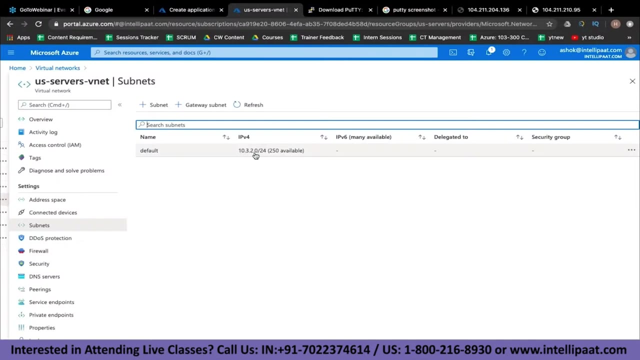 So what this basically tells us? that the whole, The whole virtual network can have IP address in these ranges And obviously the subnets have to lie between these ranges, Right? So my default subnet, Default subnet, is obviously within the range of 10 dot 3.. 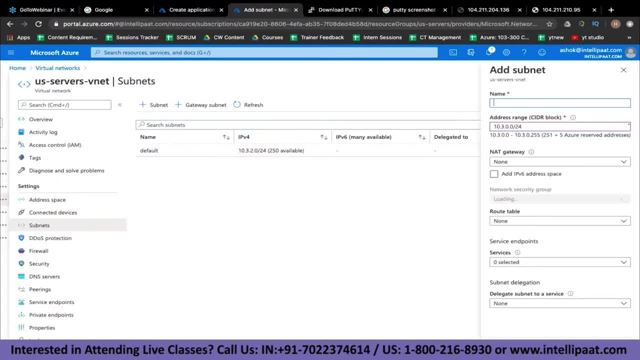 Now I'm going to specify a subnet range for my application gateway, which is going to be this: Okay, And let's call it AG hyphen subnet, Right, Let's click on Okay, So this subnet is now being added, Okay. 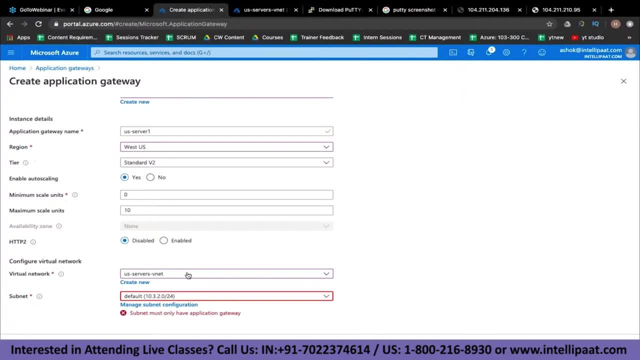 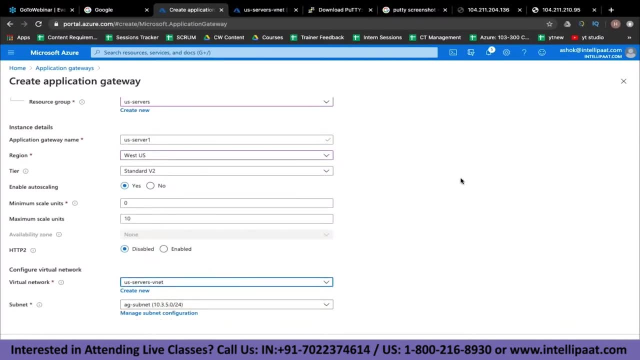 It's been added And now, if you go back, Okay To US, So as we net, You can see that EG subnet. We can choose. now Okay, And it's not giving any error now Okay. So now let's click on next. 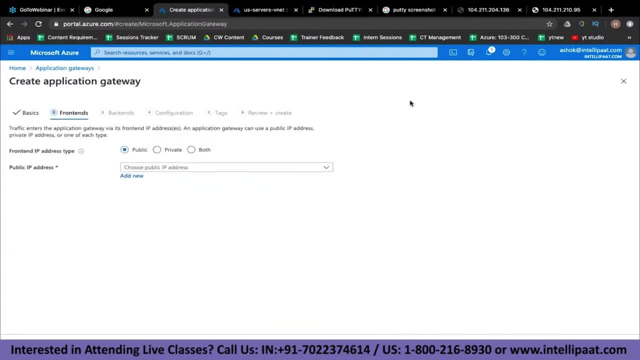 And now it is asking me what will be the front end of this load balancer? The front end is always a IP address, So there will be one IP address. So there will be one IP address of the load balancer that we will be hitting. 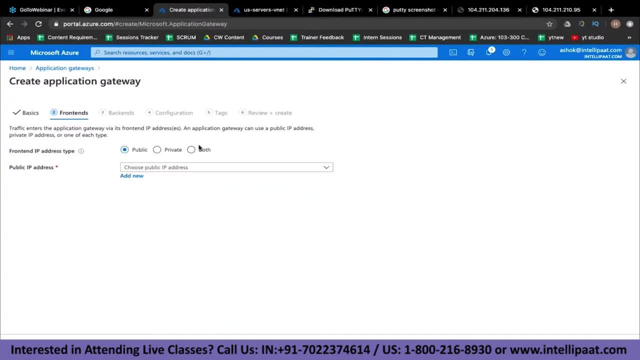 And that IP address is basically going to route to the backend servers that we have. So let's add. let's call this as ag-ip-us, okay. Next, now it's asking me to add backends. So backends we can add. 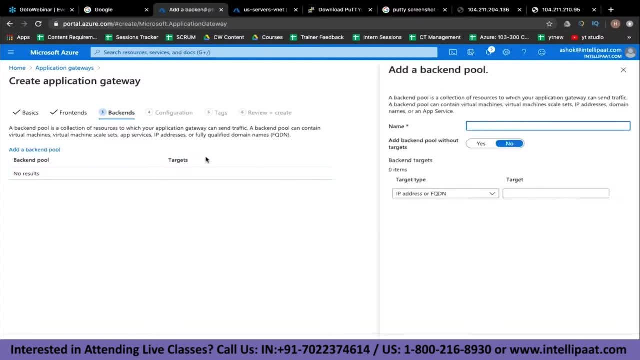 We can click on add a backend pool. Let's name this backend pool as us-pool And let's add the virtual machines in this. So the target type would be a virtual machine And if it could be us-server2,, let's add this first. 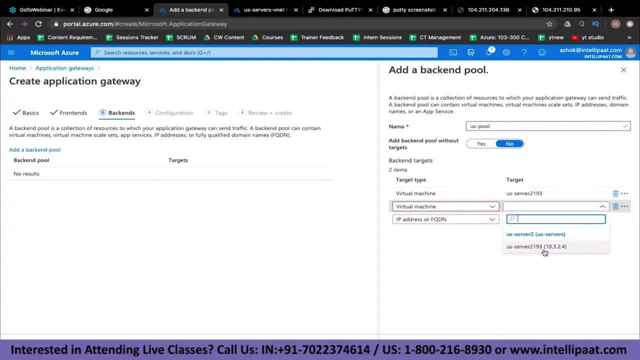 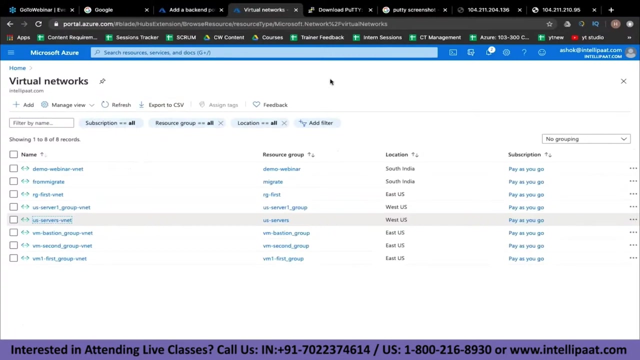 And again a virtual machine, and let's choose us-server1 is not being listed over here, So only the servers which are in the virtual network of this application gateway can be added. So I think the server1 that we deployed is not in the same virtual network. 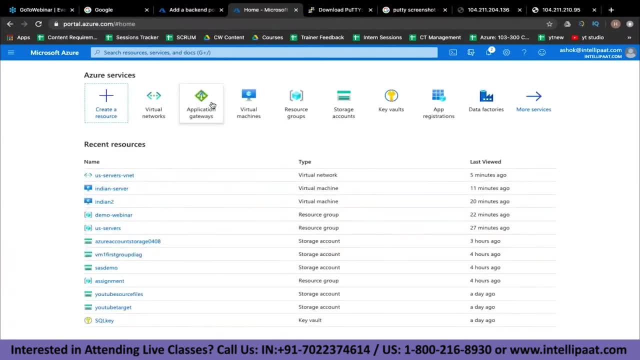 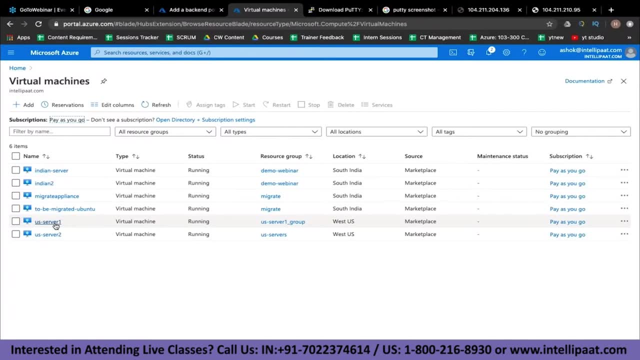 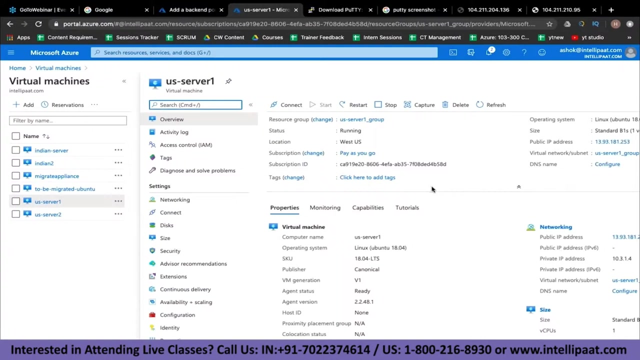 Let's verify that. So let's go to virtual machines And let's go to: okay. So I think this is a problem. So our us-server1 is in a different network. Hmm, okay, let's try to fix that. 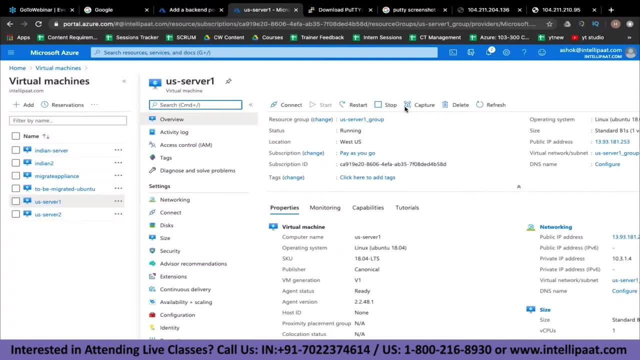 So it's a good thing. So let's try to fix that. So it's a good thing. So it's a good thing. So let's try to fix that. It's a good thing. we did not configure us-servers yet. 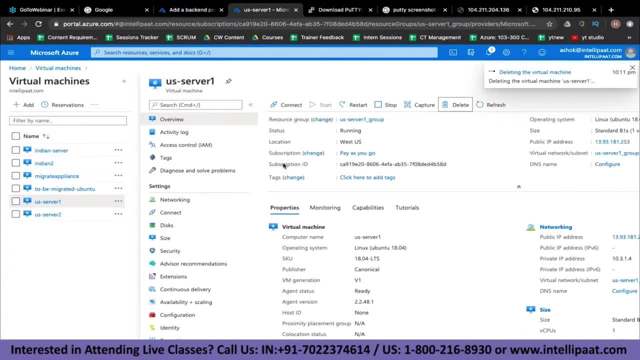 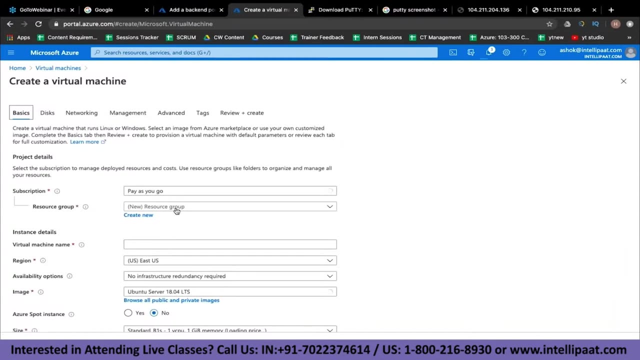 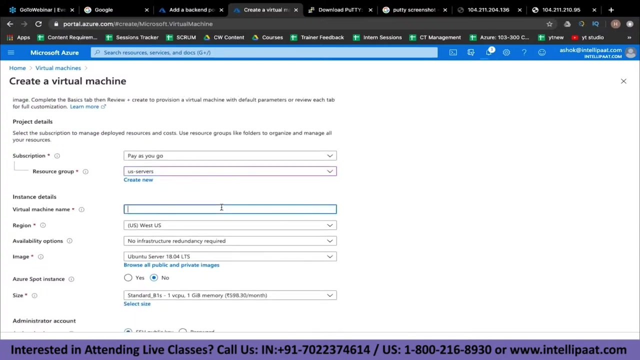 So what we'll do is we'll just delete this server That is, us-server1.. And while it is being deleted, let's quickly add a new virtual machine in the resource group of us-servers. Let's name this virtual machine as server1.. 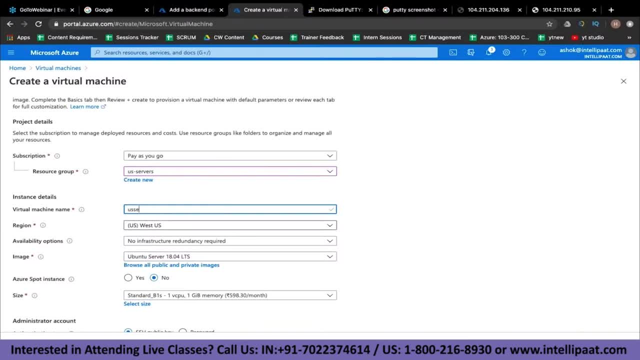 Let's name this virtual machine as server1.. So let's go to server1.us or us-server1.. So let's go to server1.us or us-server1.. So let's go to server1.us or us-server1.. 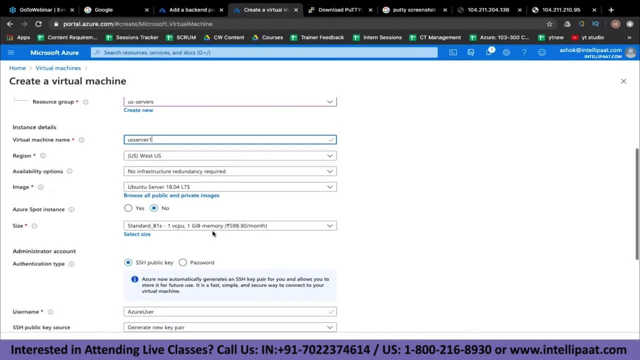 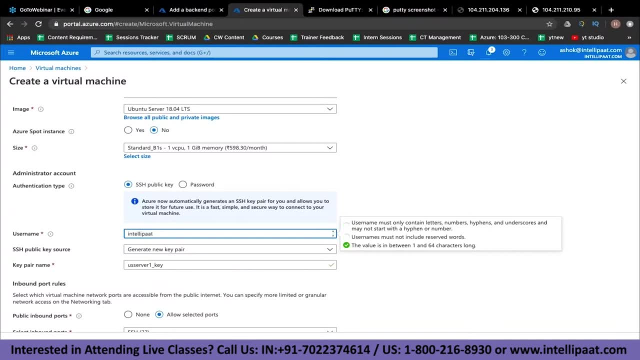 It will be the best US. the operating system will be Ubuntu server. This is the size of the virtual machine. This is the size of the virtual machine. Username would be Intellipaat, The authentication type would be password And, as you can see, 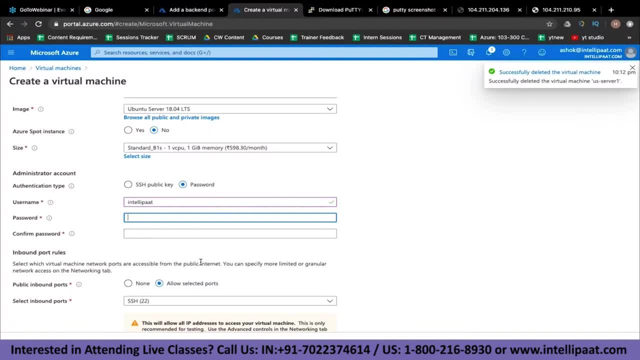 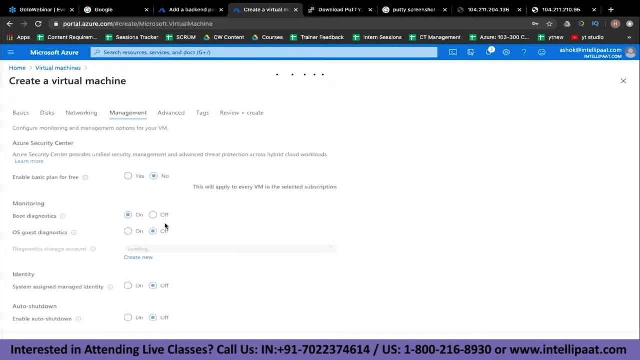 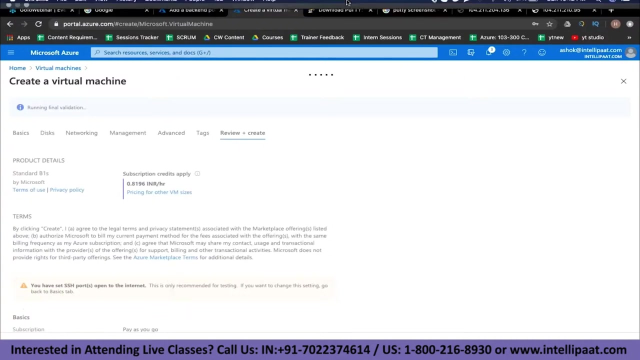 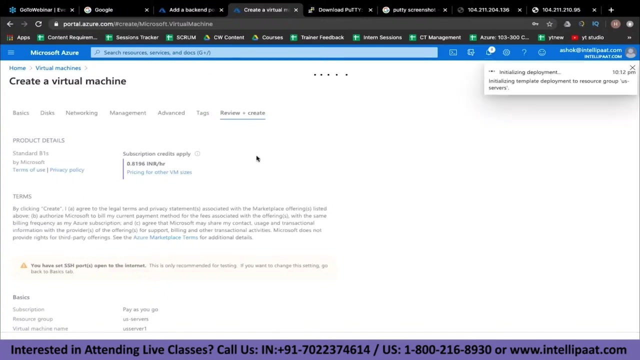 the deletion happened automatically in the background. And now let's specify the password right. let's go to management, turn off the boot diagnostics and click on review plus create. okay, so now my virtual machine is getting created. now it will take a minute or so to get this ready, guys. so 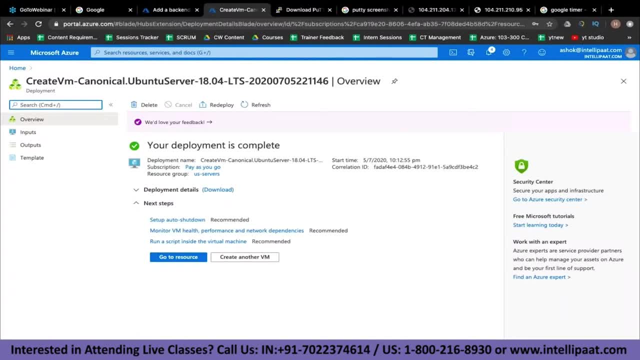 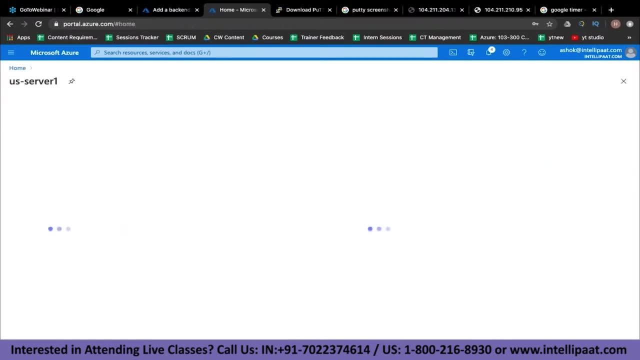 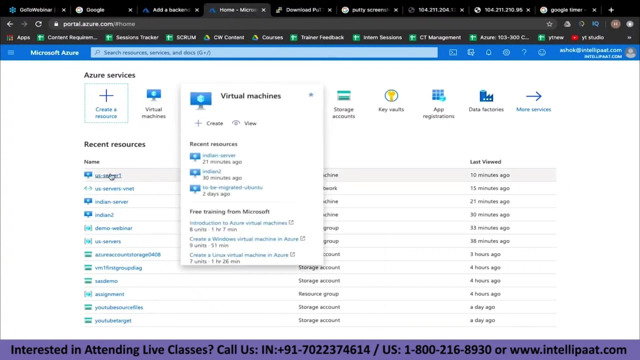 so we have now deployed the uh us servers- uh, correctly, and what we can do now is let's connect to them and let's try to configure them right before we can actually go ahead and connect to the application gateway. okay, so let's go to us server one. okay, it's taking some time to load. 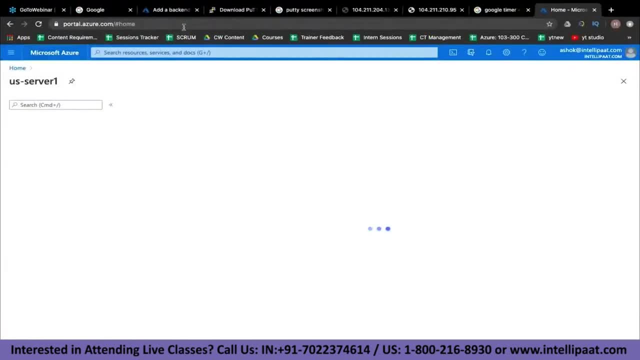 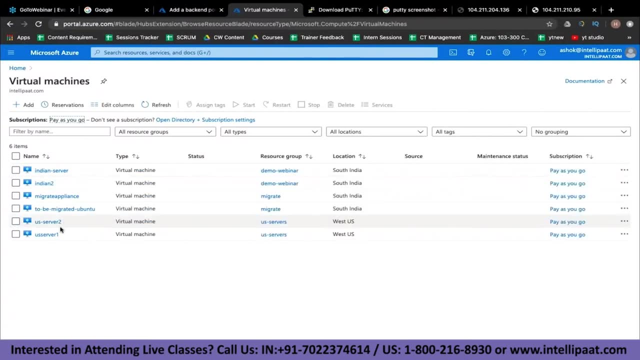 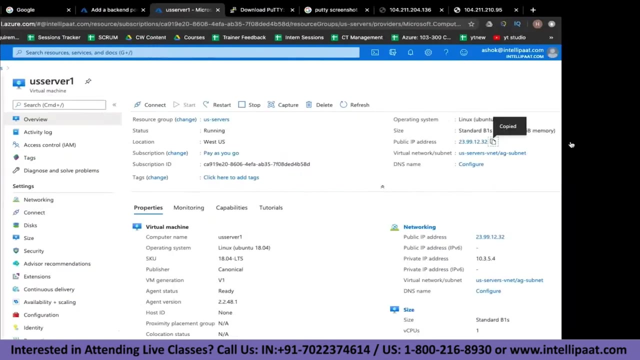 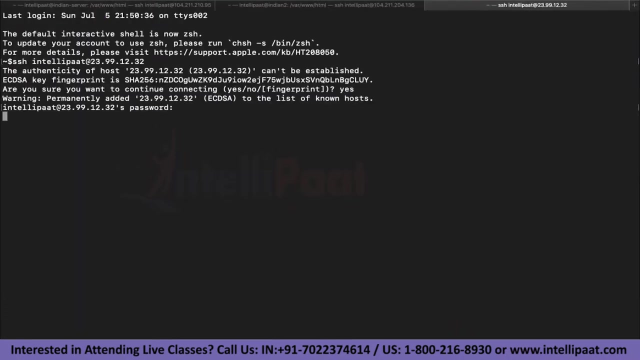 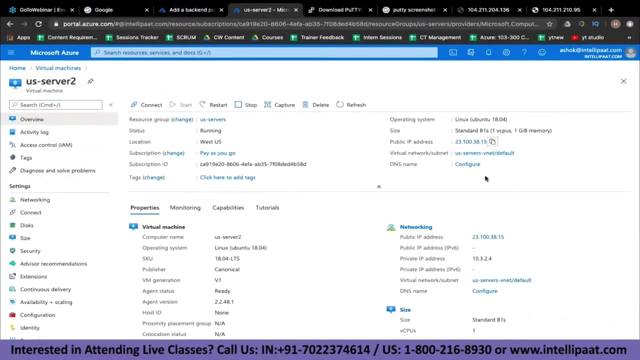 one second, guys. okay, so this is a us server one. this is the ip address. let's try to connect to it, all right. all right, so we are connected to us server one. let's try to connect to us server 2 as well. okay, this is the ip address. 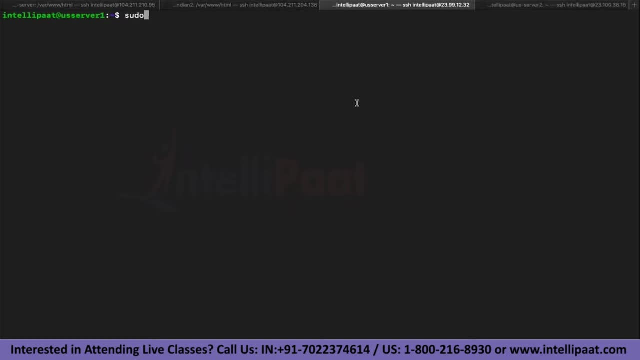 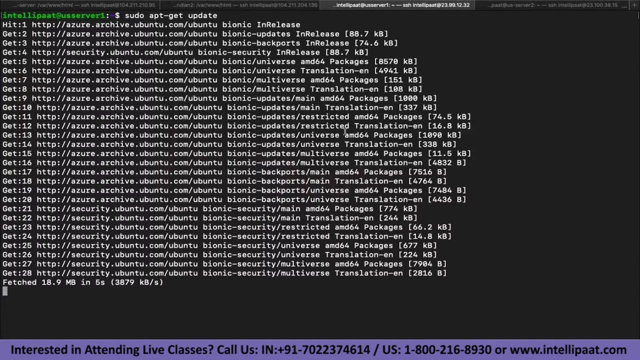 great, so we're connected to both the servers. on the first server, let's update the machine on the second server as well. let's update the machine, so same steps as we did earlier and once they're updated, let's install the Apache to software on this. okay, so it is being installed. similarly, over here is 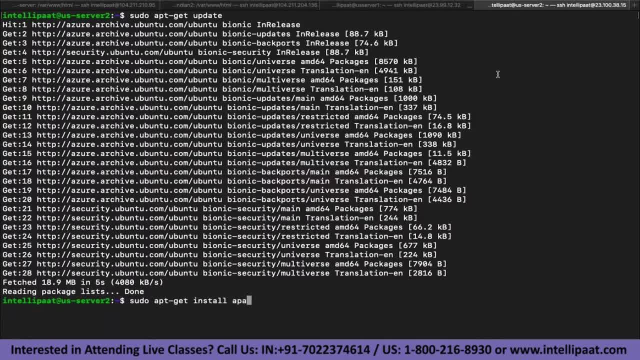 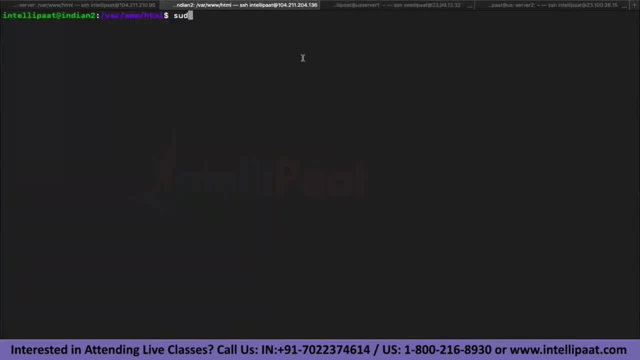 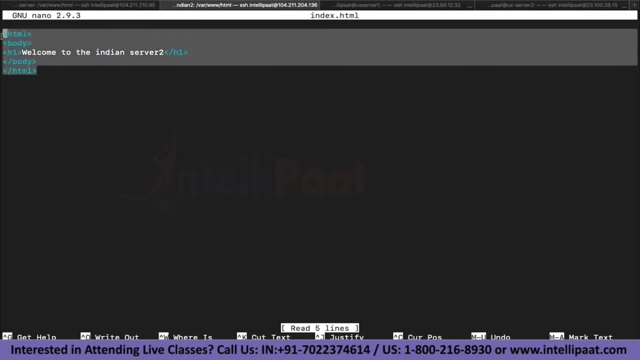 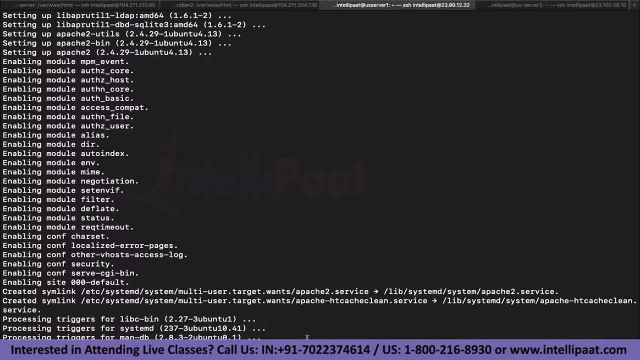 well, let's install the software. okay, so while this is being installed, let's copy the code that we have to put on this over as well. now it's taking some time to load. let's give it that time. if you don't want to use Apache server, you can also make use of. you can make. 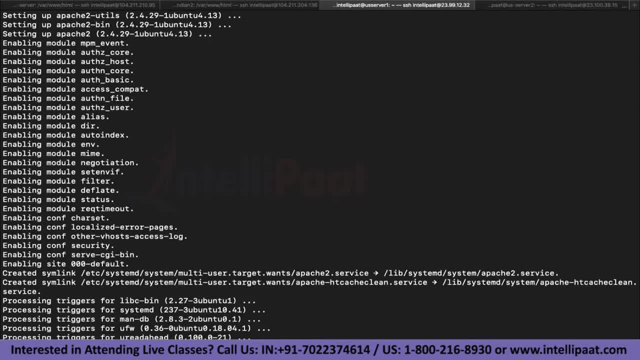 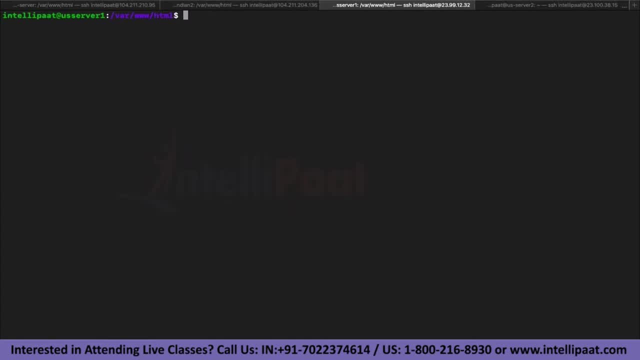 use of nginx. so nginx is basically again a web server which is doing exactly what Apache do does, but at the same time it's a different company, right? so it also hosts HTTP websites for you. so if you don't want to use this software, you can use that. 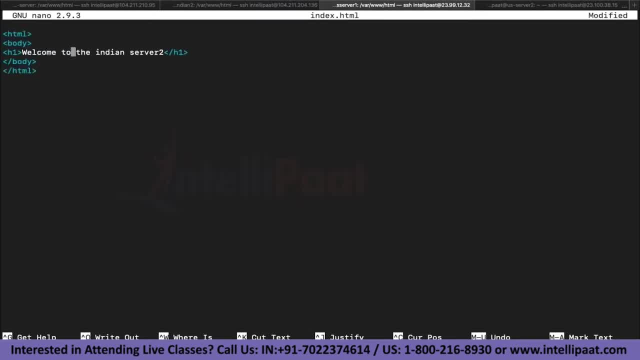 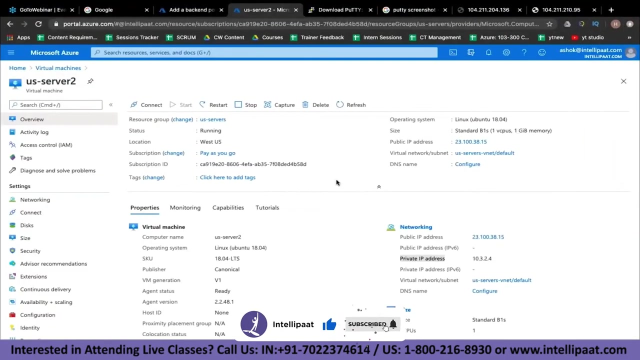 so let's put the website for the us server now. so this is us one, so let's put that in for their. similarly, you, you let's edit this as us server 2. great, now let's open these ports and the. 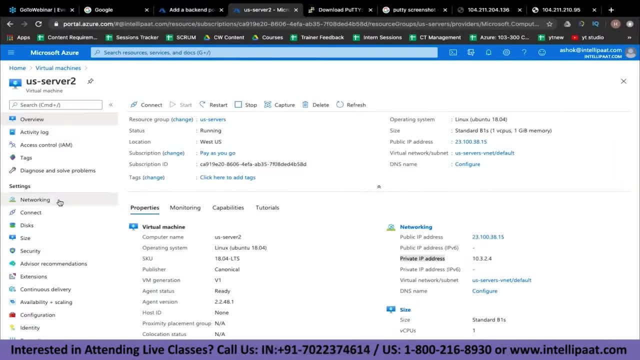 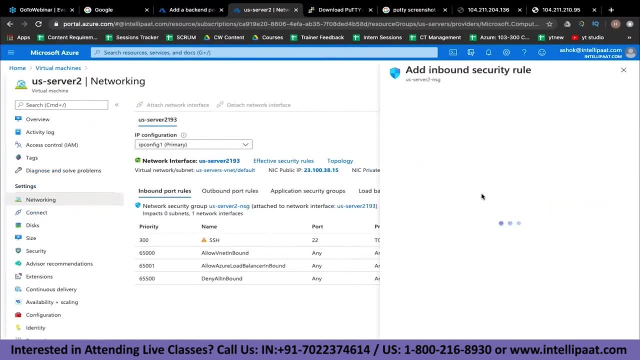 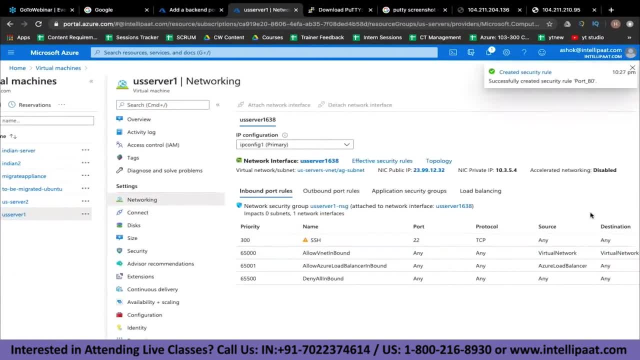 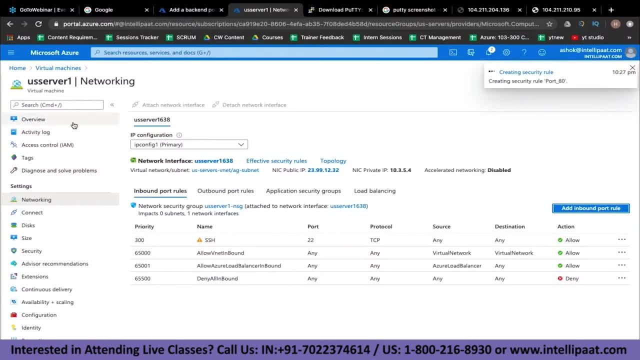 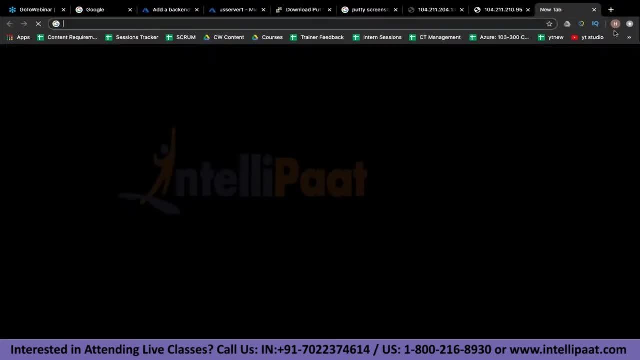 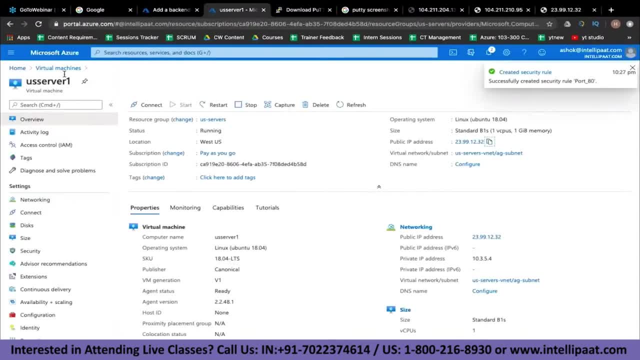 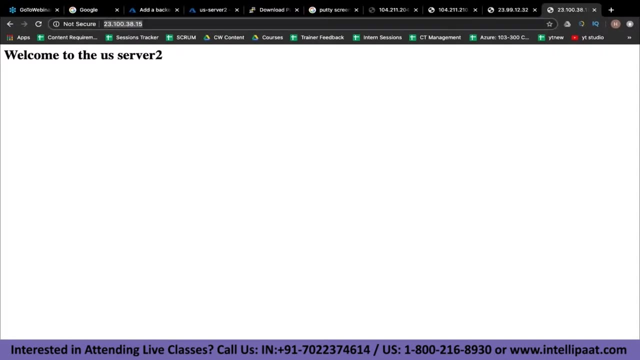 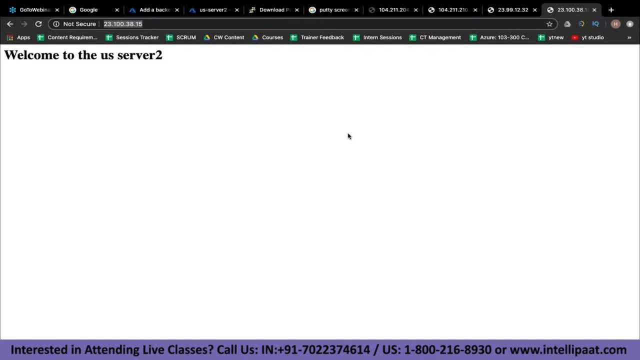 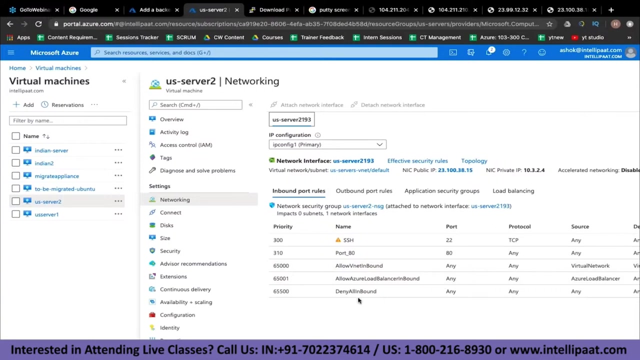 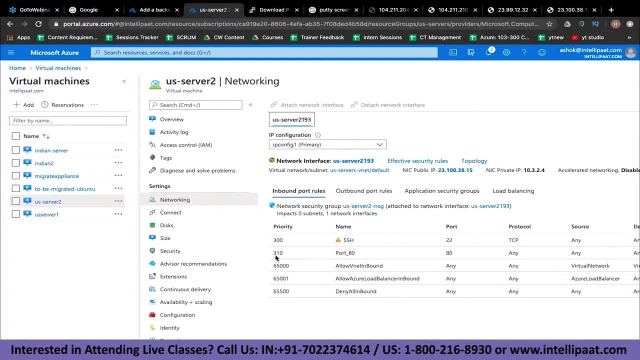 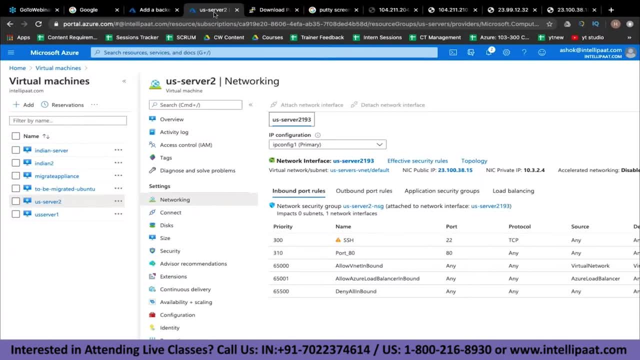 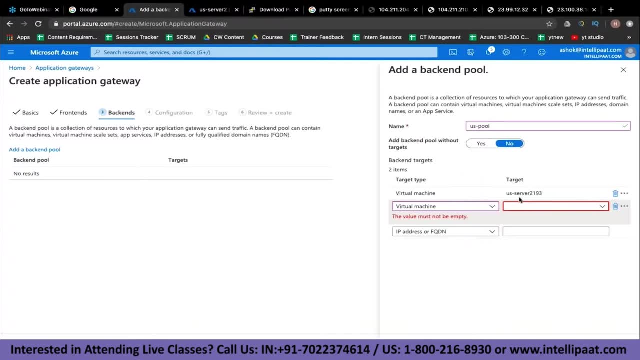 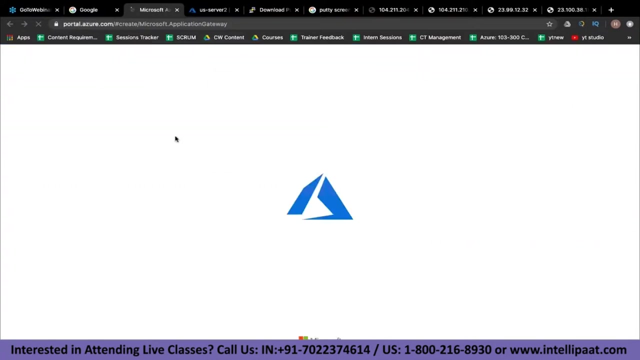 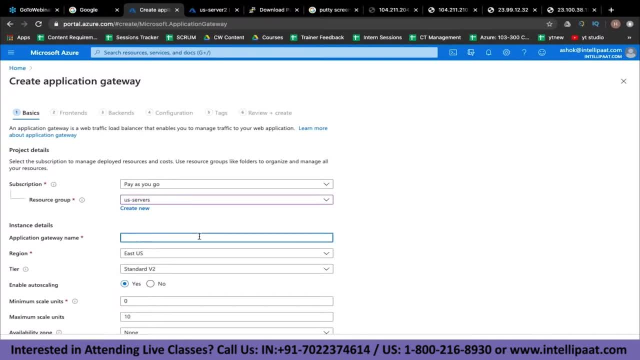 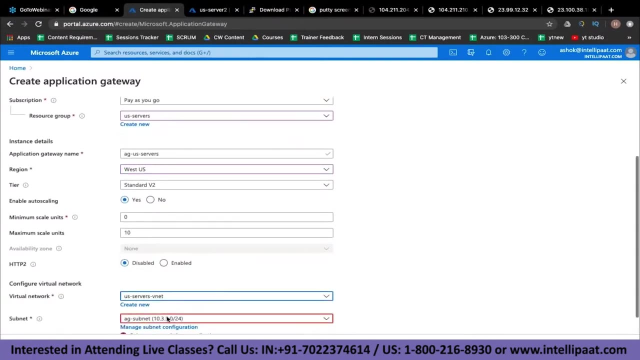 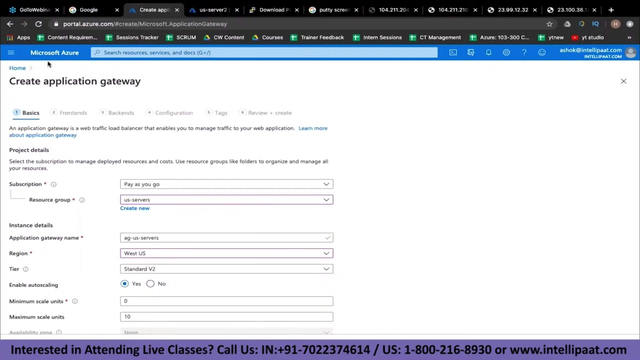 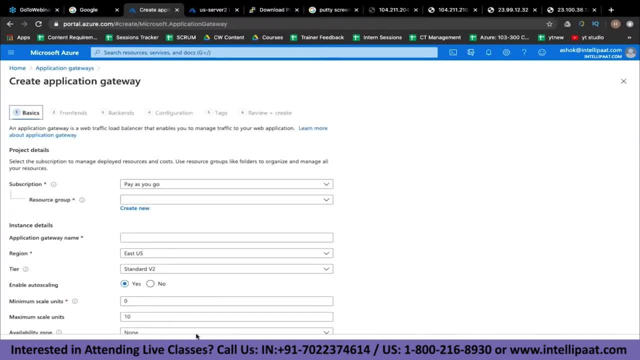 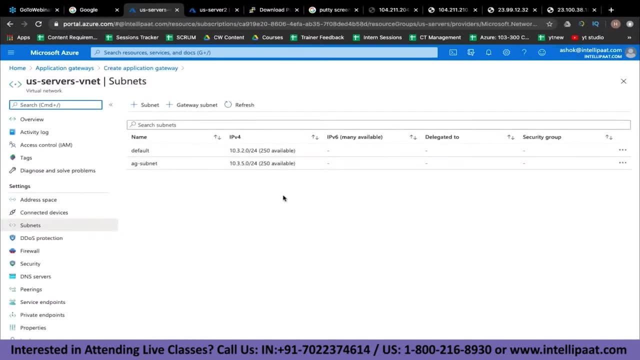 configure that application gateway itself. okay. so I think because we left off the previous application gateway, it has hindered. you know a problem in AG subnet or what I think is the US server, one that we deployed. I think we have deployed it in AG subnet. let me just 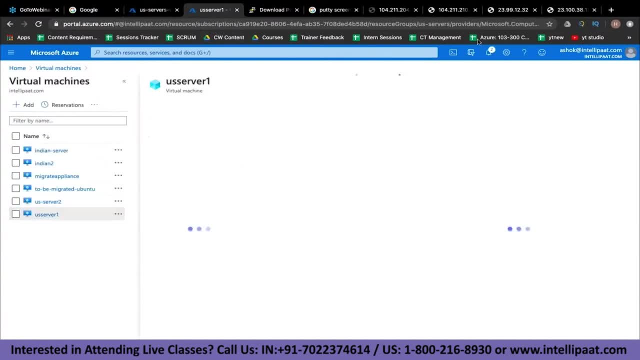 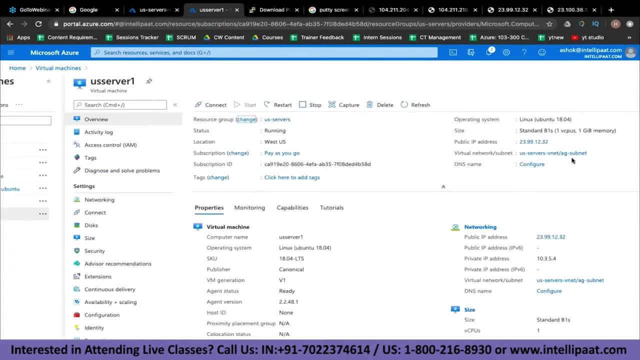 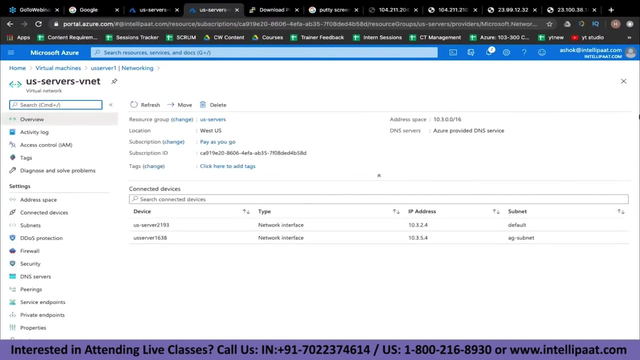 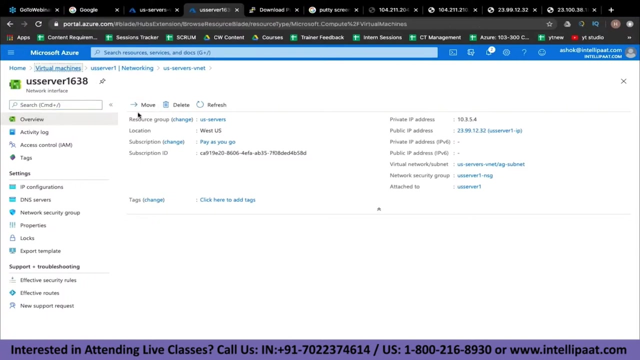 double check that. okay, so this is server one and if you go to the overview: yes, so this is the problem. okay, so let's see if we can change that so we can go to networking. okay, so let's do this. guys, let's delete this again, because if we edit it, I think 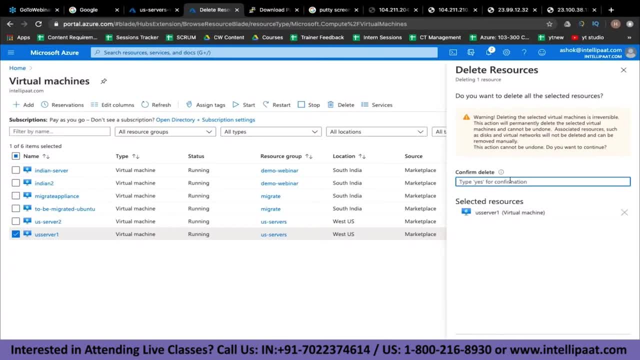 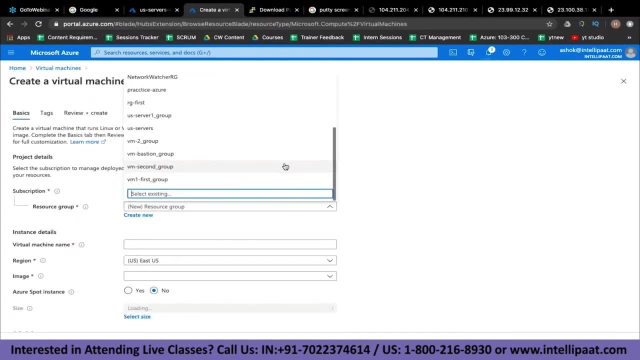 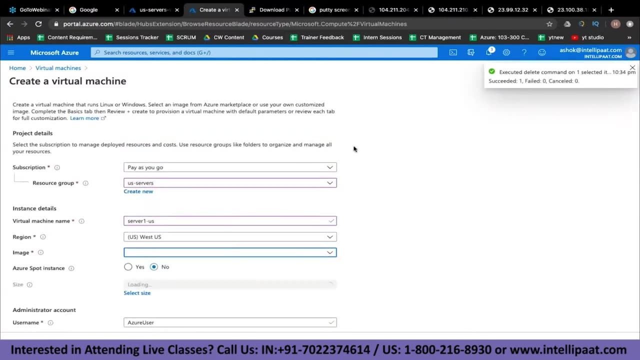 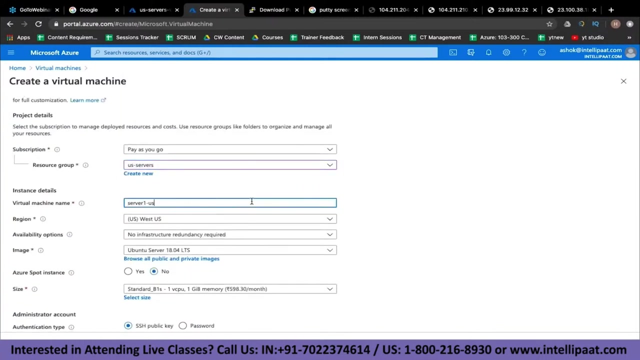 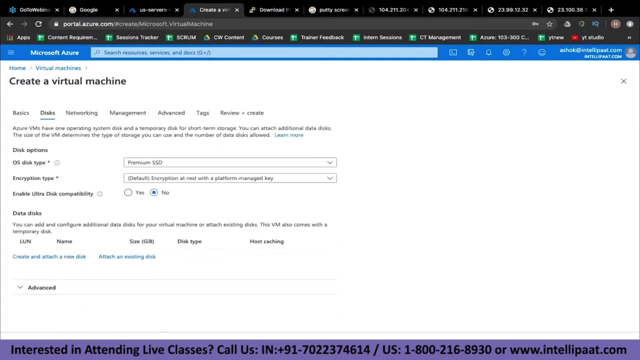 there will be a lot of steps that I have to do to want it much time, and in the meanwhile, let's create one again. okay, so the size of the loading. so that will wait. don't be hurrying around to edit this one. let's quickly enter the same in for. 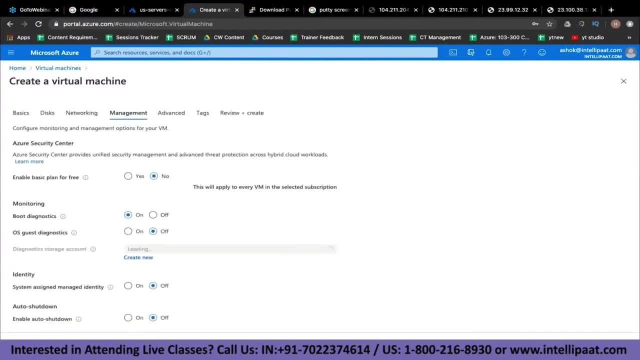 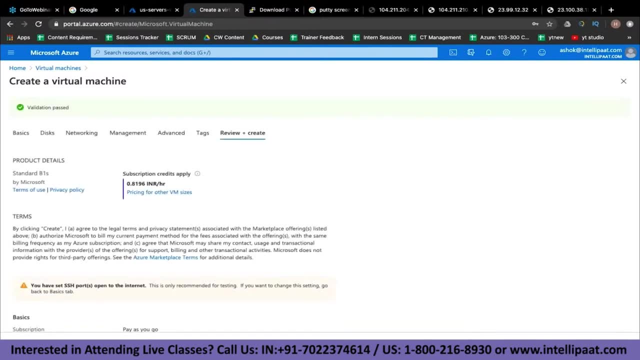 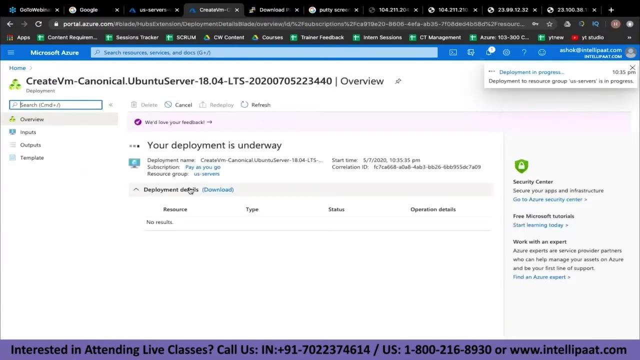 I think let's be double sure that we define it into theDuPol: equipo now and management. let's turn off the diagnostics, let's create. I think a good thing looks good now that's created, great, so it's now getting created. so, guys, so say, oh wait, you need to delete this first. please leave the job to click on any cuest to see whether it works or not. 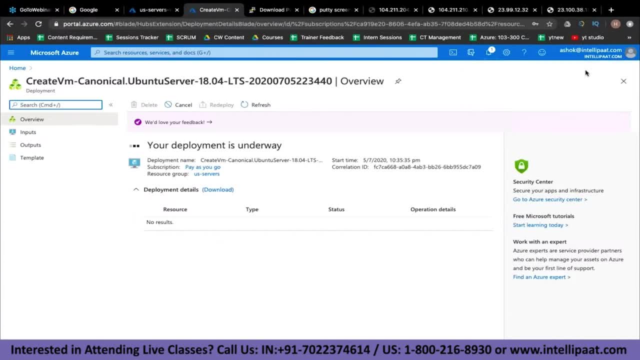 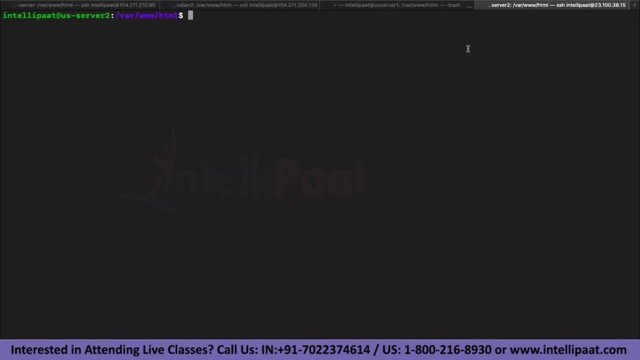 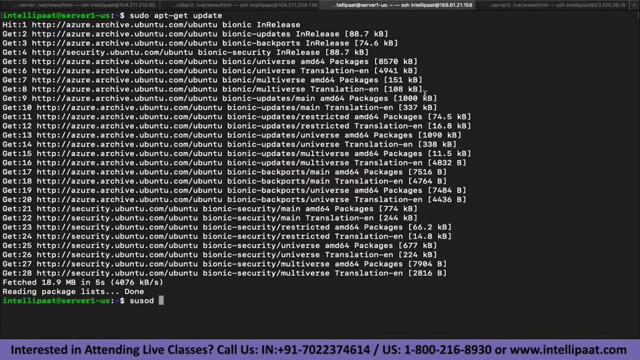 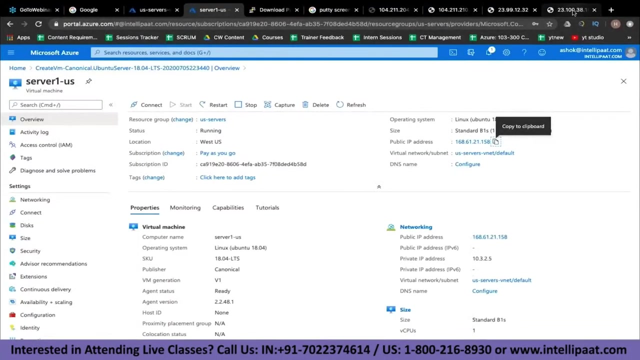 great, so it's now getting created. it'll take some 30, 40 seconds. uh, let's try to copy this ip. come back to terminal. i think server one we will have to reconnect. okay, let's quickly update it and now install the software. okay, so the software is being installed and now what it can do is. 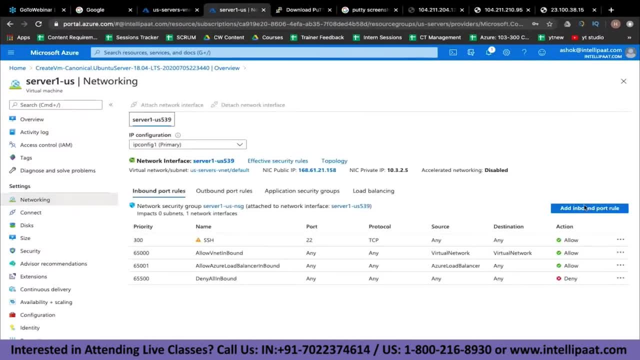 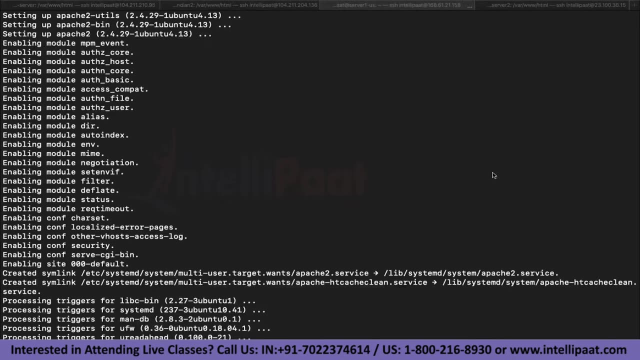 go back to server one. go to networking, add an inbound port rule. port range would be 80 added. great, that rule is now being added and at the same time the software are also getting installed. network load balancer can redirect based on networks. application load balancer can redirect based on, uh, the user parts. okay, so that would be the. 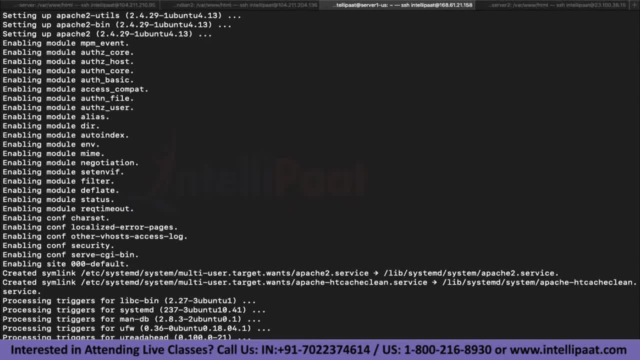 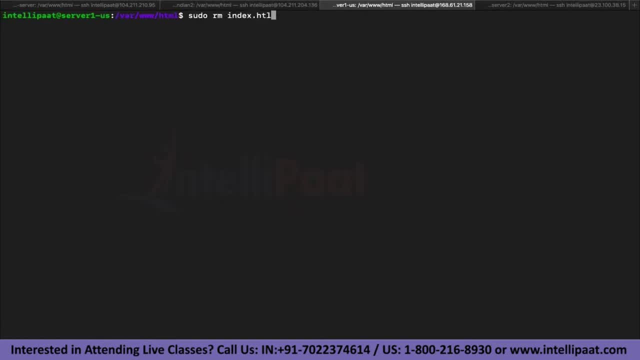 difference. but i think if you don't know about azure, uh, it is okay if you do not understand it right now, because there are a lot of things to learn in azure. right, it's okay if we miss out on some today, because the main idea of today's session is to understand how, uh, you know companies. 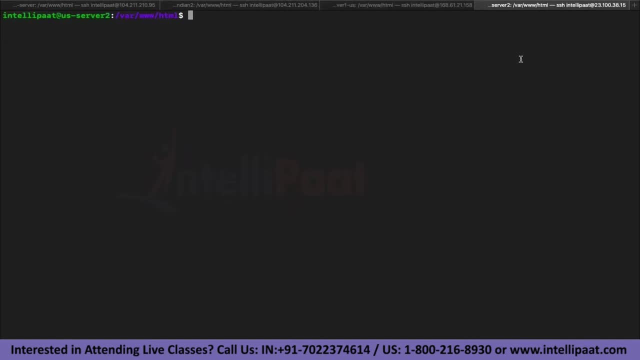 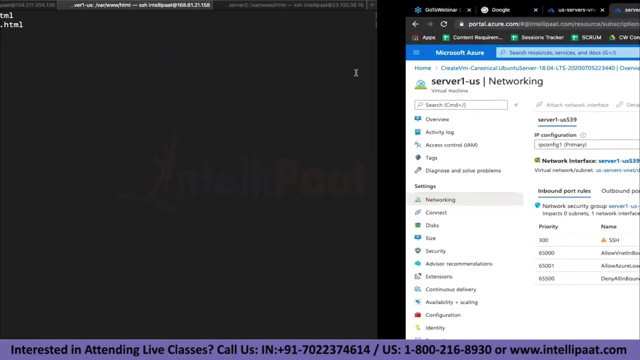 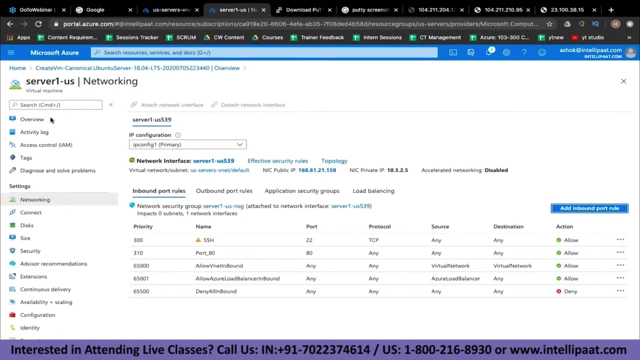 like google or, uh, other big companies. they're making use of cloud for basic things that you do not notice every day, but today you're noticing. okay, so let's copy the code, paste it here. i think that is about it. so now we can just verify, if we can. 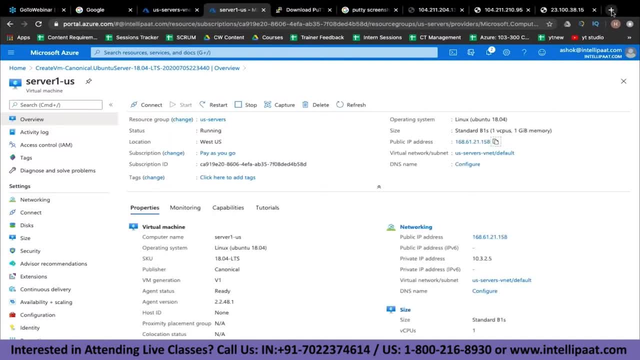 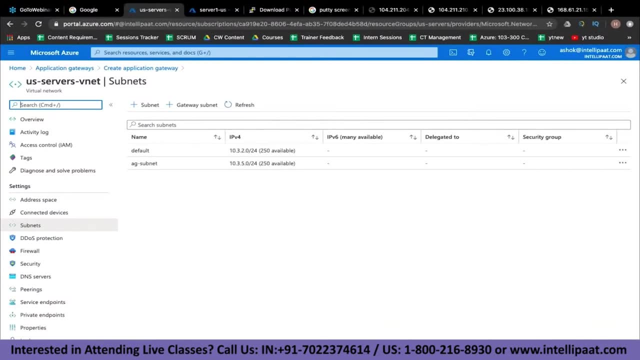 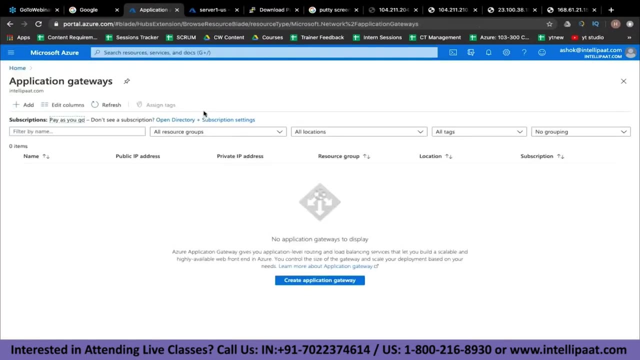 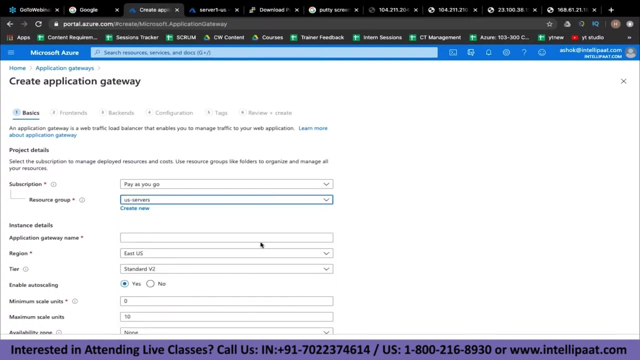 see this ip on the browser. so, yes, we can. great. so now that we have the servers configured, uh, let's go to application gateway. uh, add one. uh, we're gonna add it to the uh us server first, us servers resource group. let's call it at eg, hyphen us. it's gonna be a part of west us. 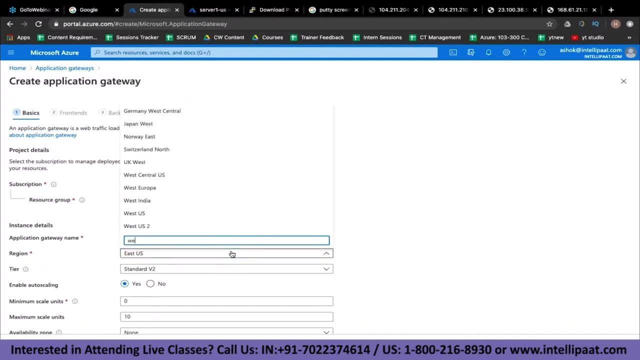 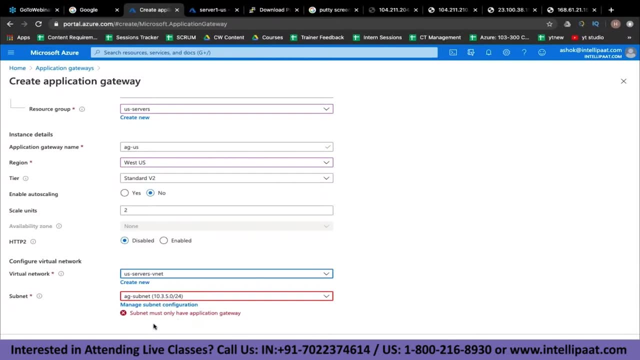 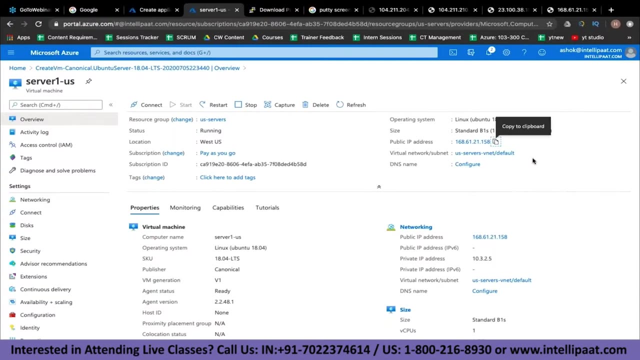 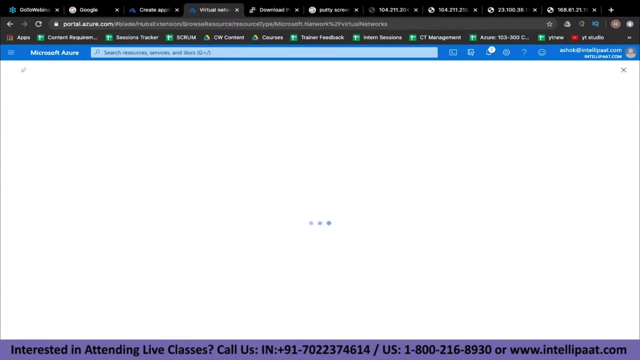 so we're gonna add it to the us server first: us server resource group. let's call it at ag hyphen: us best, us auto scaling. we don't want it. virtual network would be us service bnet. okay, what is the problem now? well, this is part of. okay, let's do this. uh, let's just delete the ag net subnet and let's 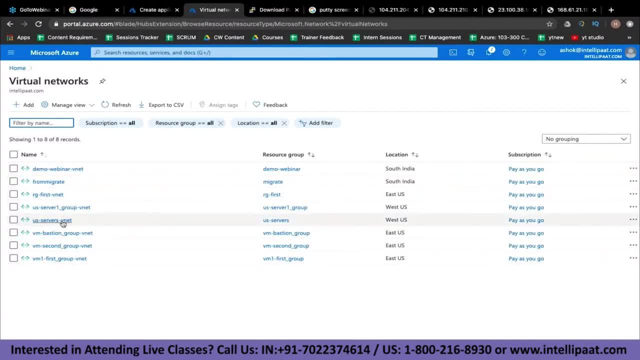 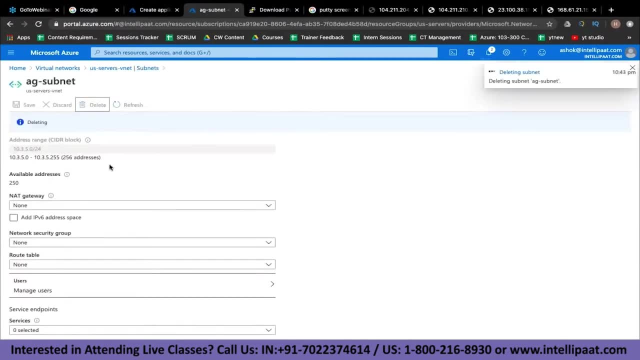 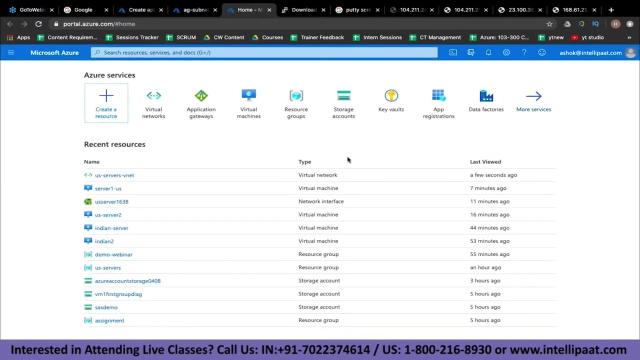 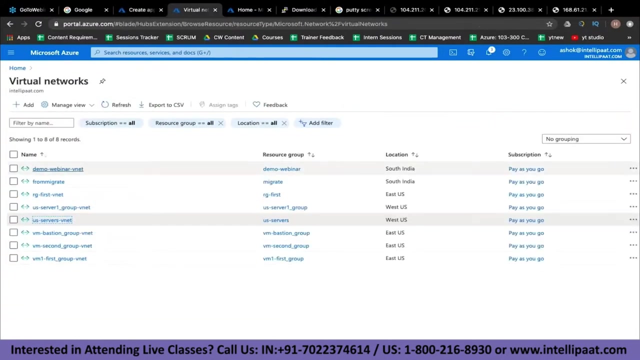 try to connect to it again. so us servers, vnet. uh, we go to subnets over the ag subnet. let's delete it. okay, so there seems to be some network interface which I was making use of it. what we can do is let's leave this. let's create one more subnet where we can have. 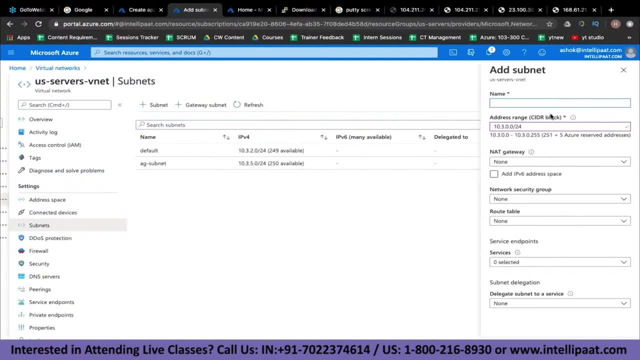 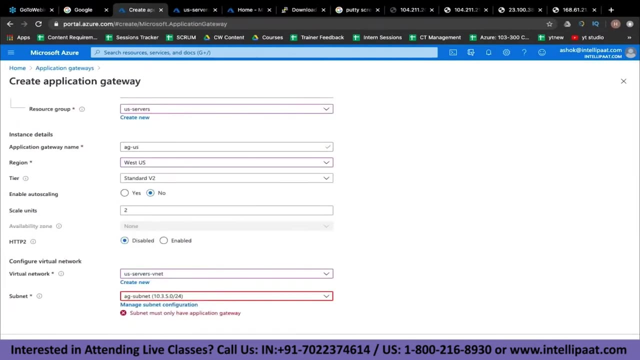 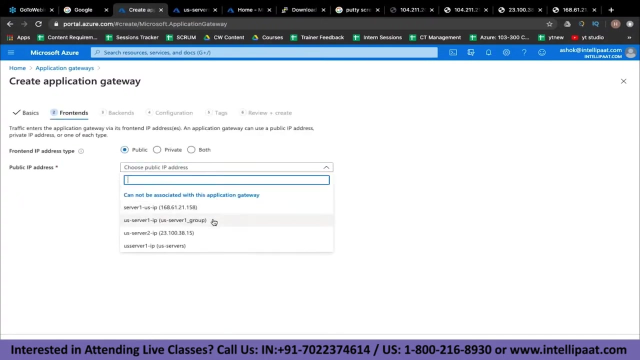 a application gateway, so let's call it as eg1-subnet and this could be the range. let's create it and now, okay, this is a subnet there you want to configure. let's choose an IP address. let's add one new hyphen: AG- us. okay, let's add a back-end pool, so back-end. 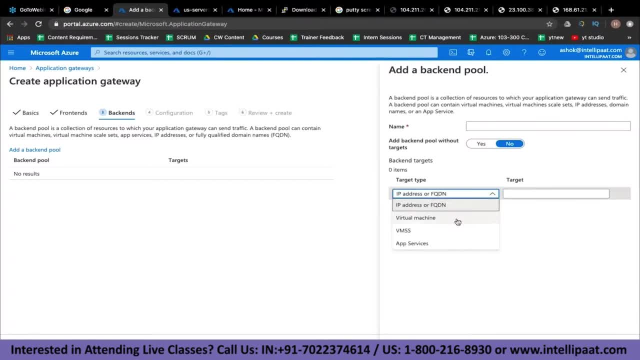 pool is nothing but your servers, right, so let's add them. so let's choose a virtual machine. let's choose the first virtual machine. let's choose the first virtual machine. let's choose the first virtual machine, and now let's choose the second virtual machine as well. okay, so we have. 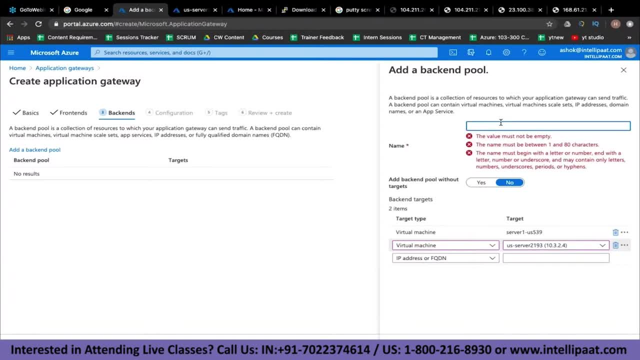 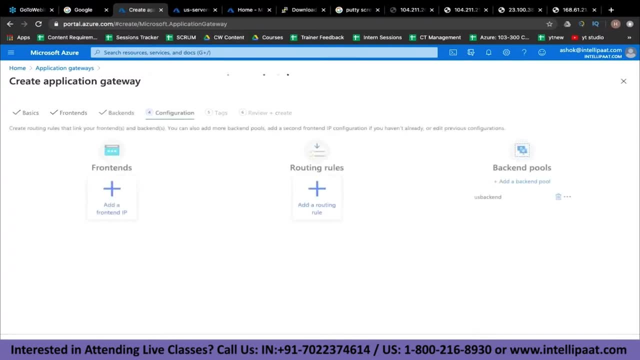 added the back-end pool. let's call it as us back-end. let's add it. done configuration. so is there a routing rule that you want to specify? let's not specify anything, so in that case will be a okay, I think we have to specify, so let's. 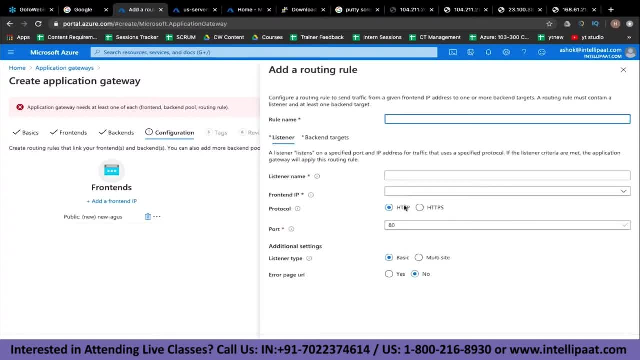 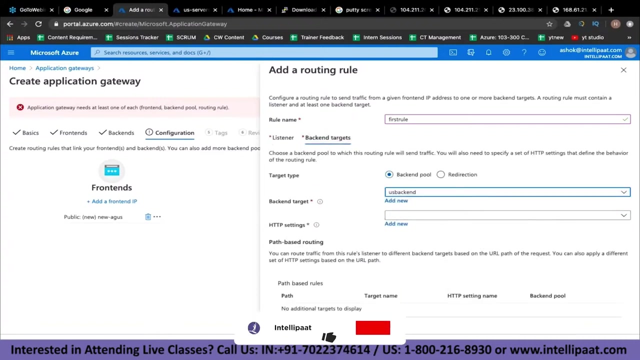 specify a back-end rule. let's call it as first rule. right listener name would be: let's say it's listener I from us. front-end IP would be public. this prototype is basic at a page of URL back-end targets, so it will be us back and I should be. second setting: let's add new HTTP setting. 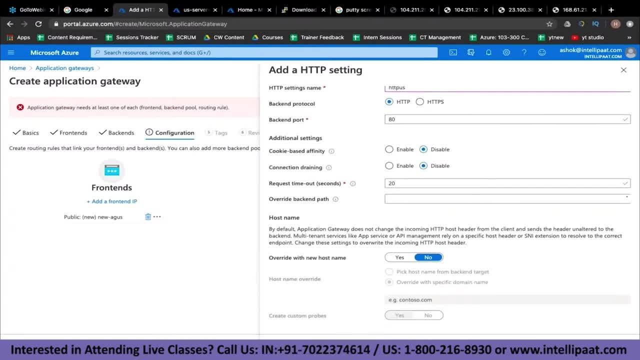 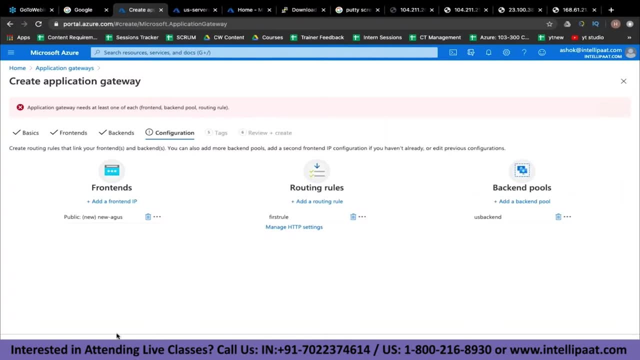 let's call it as HTTP us added. we're not adding any path based rules and this load balancer. okay, let's take an ad and finally, let's just click on review plus create and create it. so with this, now we have created the load balancer. 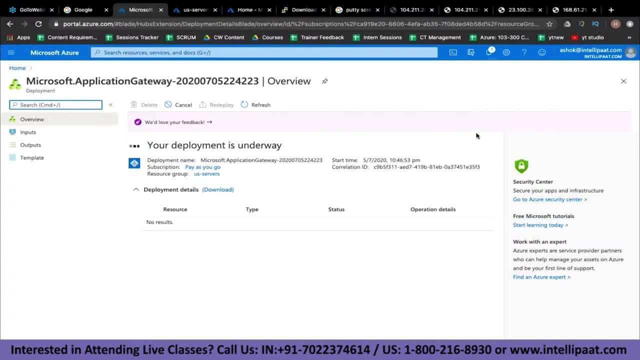 that is required for these US servers. now I think it will take a minute or two to deploy, so let's give it that time and we'll be right back. so let's go ahead and meanwhile we can deploy the same for our Indian services. well, so for our Indian. 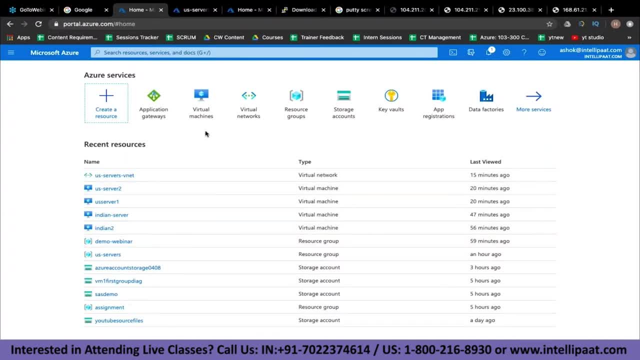 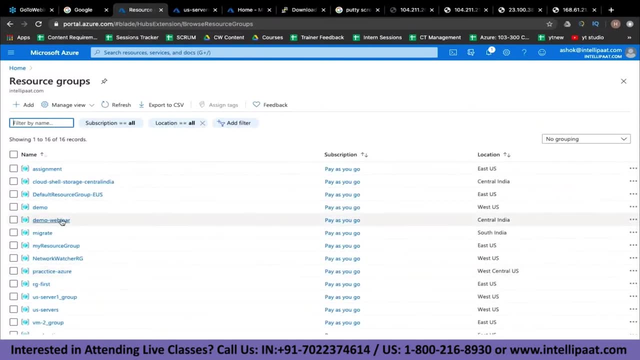 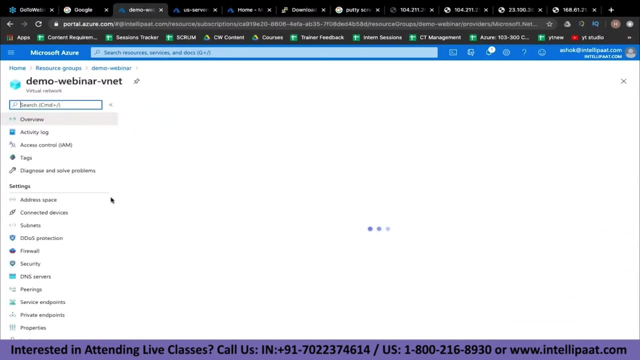 servers. I think the first thing that we would need is the virtual network to be configured. so let's go to demo webinar resource group. now in this, the virtual network, the subnets- in this we just have the default one. so first we change the address space saved, now we go to subnets. okay, let's add a subnet and let's call. 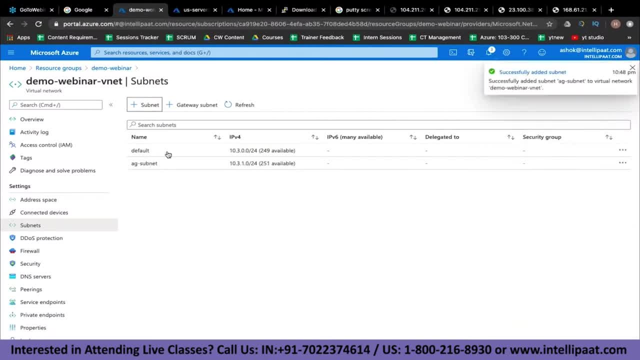 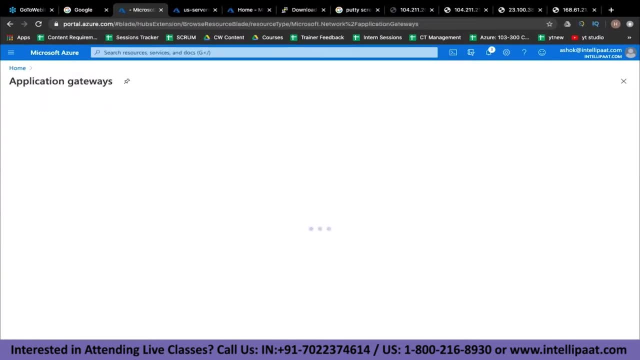 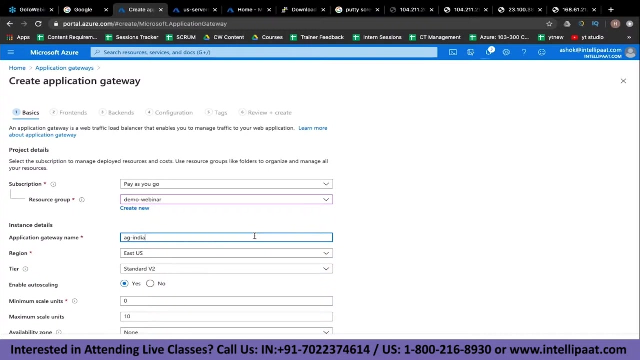 it the AG subnet. so now we have a subnet for the application gateway, right, and now let's go to application gate with. this is the US one which is getting created. right, let's add one more and it will be in the demo webinar resource group. will call it as a GI for India. 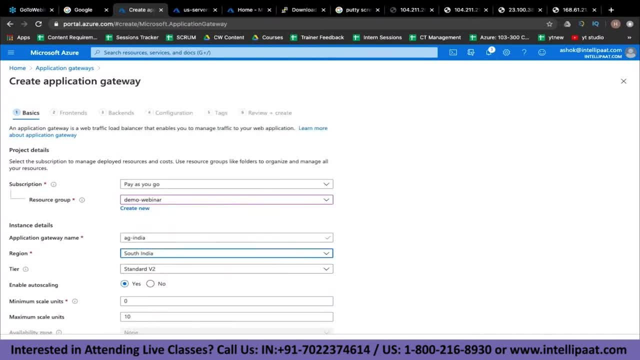 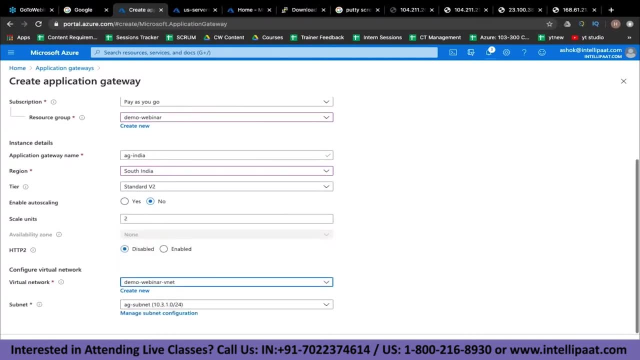 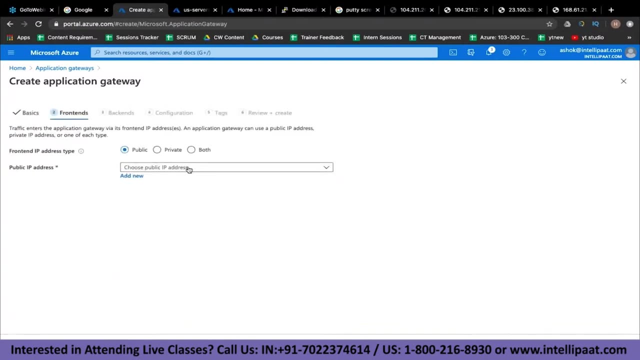 would be part of the South India region. not scaling. virtual network would be demo, webinar, be net and, yes, the subnet would be AG high fence of it's great. now let's add our GIFs and I'll be adding GIFs right here. so the subnet for the 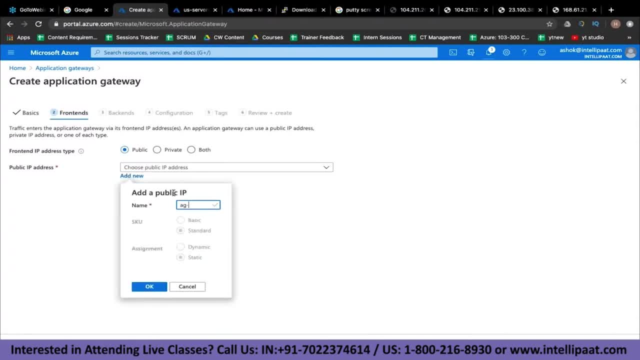 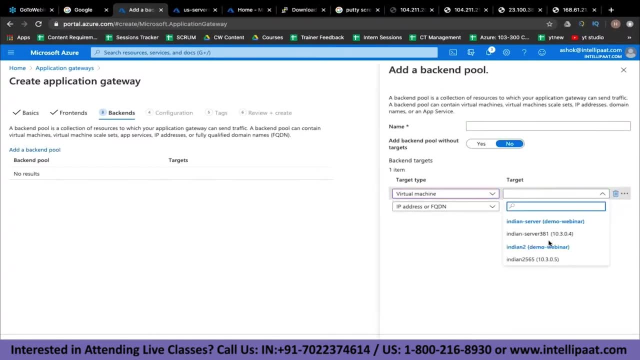 a public IP address to it and let's call it eg- India. again, the back-end, so let's add a back-end pool. it'll be of type virtual machine, so let's first add the first Indian server and then the second Indian server. okay, and let's call this: 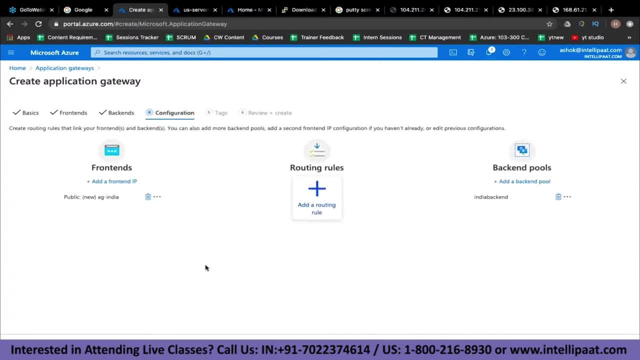 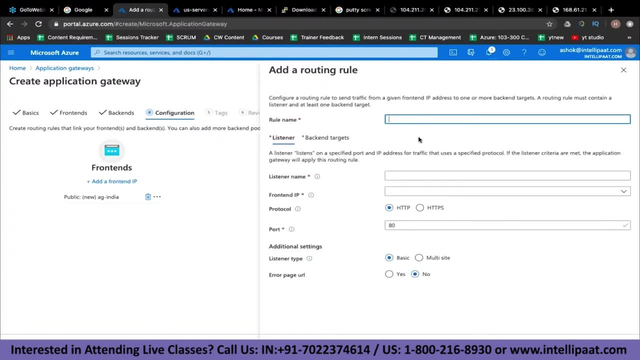 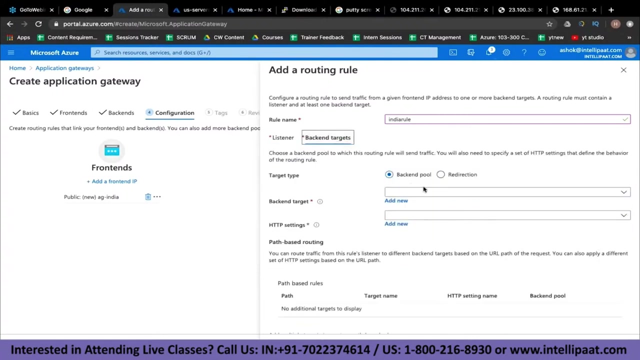 as the India packet. so back-end pool has been added. now let's add an outing rule. so again the same configuration, guys, the rule name. let's call it as India rule listener name. you can give it anything. let's call it my listener front-end IP. it would be public, obviously. then let's specify the back-end target. so back-end. 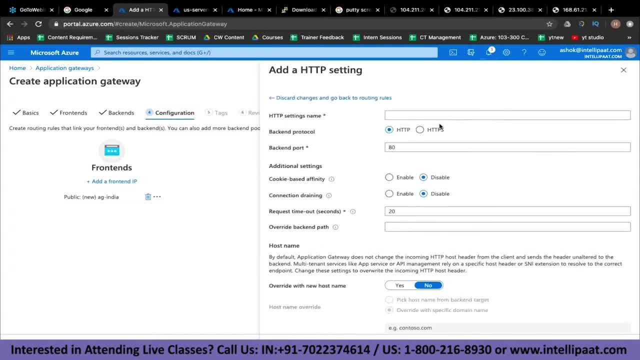 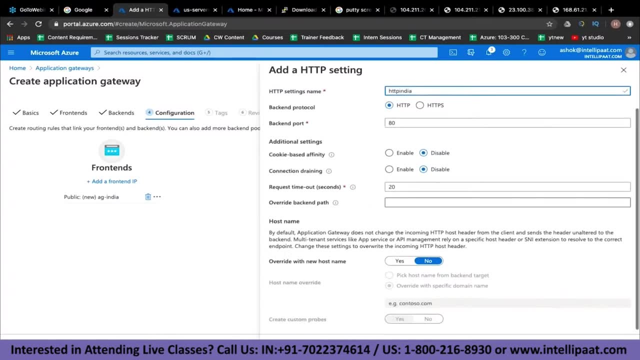 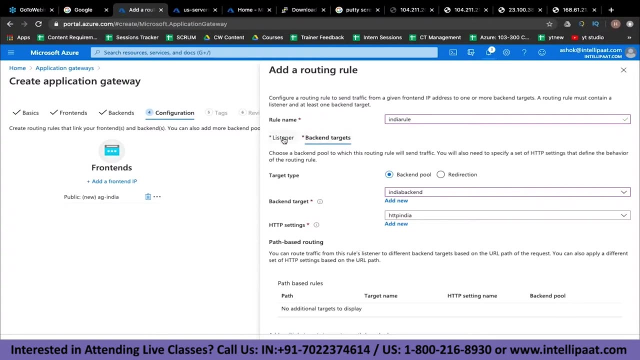 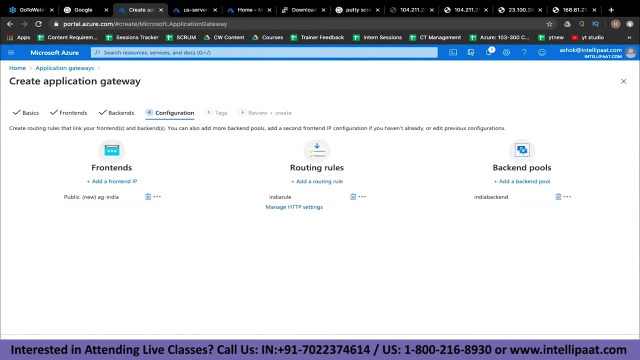 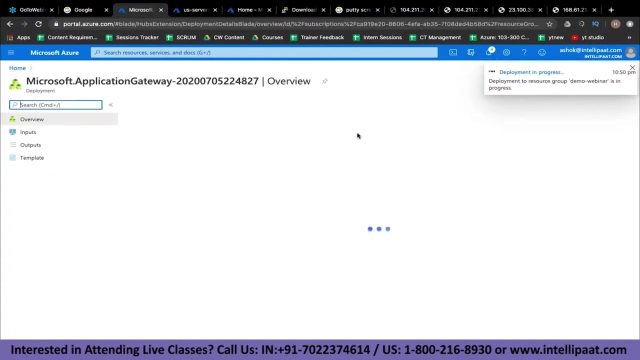 pool would be India back-end HTTP seconds. you will have to add a new setting. let's call it as HTTP India. here, nothing to be specified, just create the route, the HTTP setting, and I think that should be about it. we're not adding any parts and let's just click on create now. so with this, my 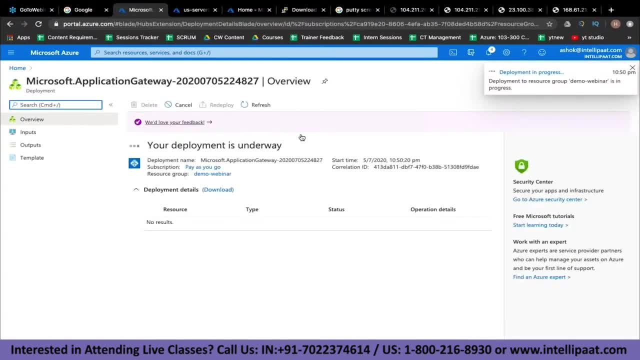 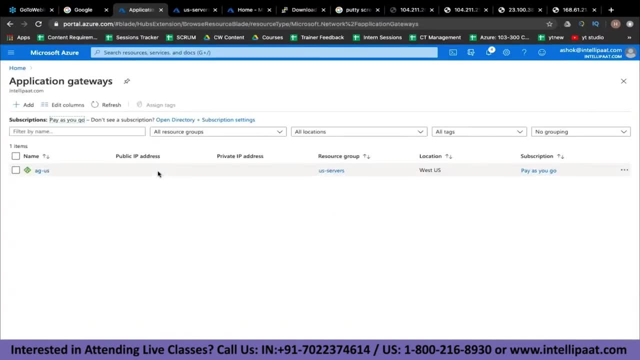 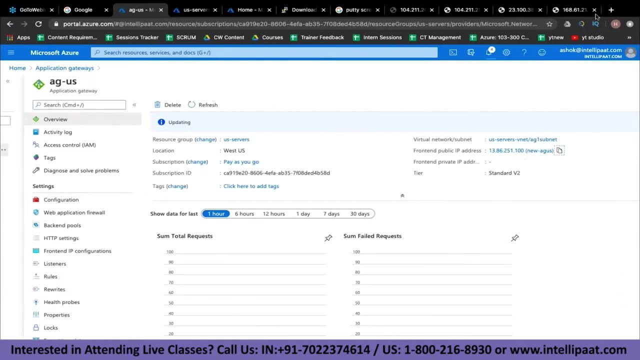 application gateway has been created, and this application gateway is now being deployed for India. I think my us one should already be deployed, so let's check that out. so if I go to AGI from us, this is the IP address. let's copy it, paste it on my browser and as of now, I'm. 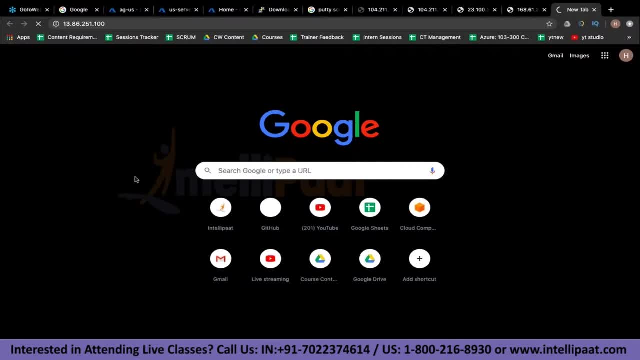 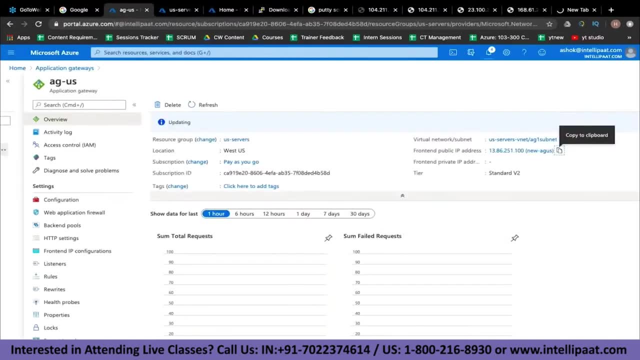 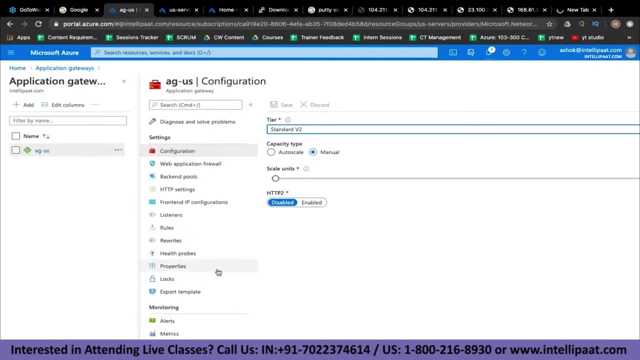 not able to connect to anything right now. right, so what I'll do is I just go back to my us application gateway and let me check. so there are a couple of things which can go wrong, because of which it is not connecting. so let's first set the firewall, so sure everything. 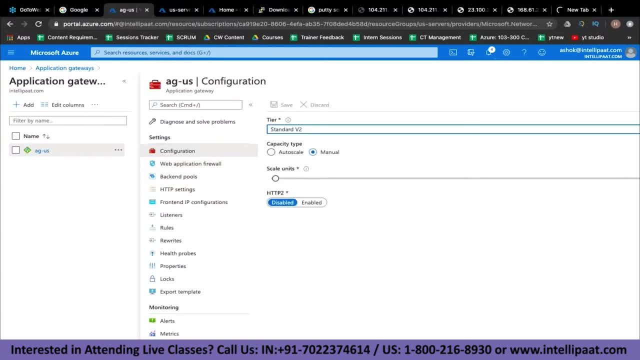 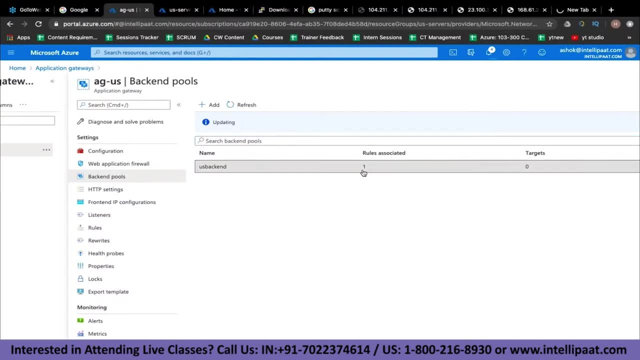 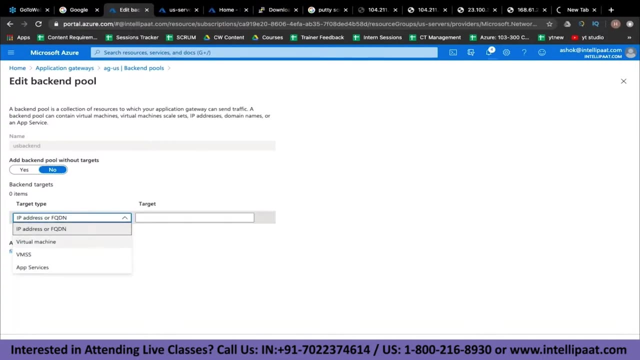 seems okay. let's go to configuration here. everything seems to be okay. go to back-end pools. okay, so there are no targets according to the rules associated. let's check that. okay, so there are no targets in the back-end pool for us. add it, although I think we did add it, but it's not there, so that's not waste. 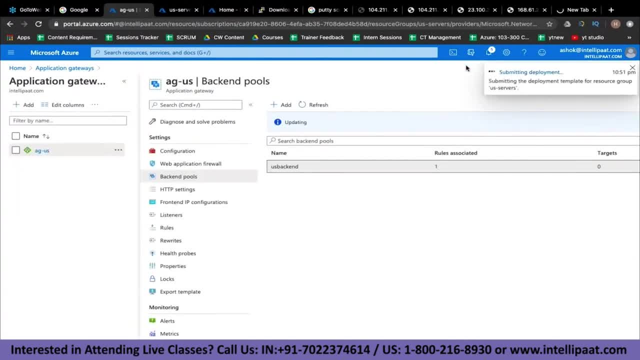 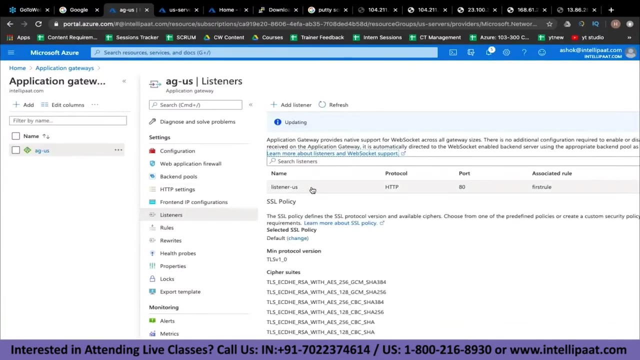 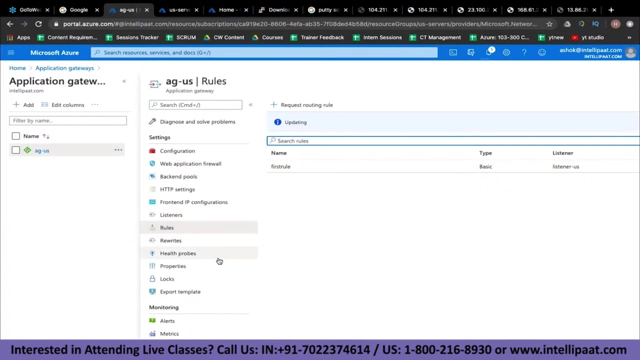 any time and save this. okay, while this is happening, we can also check out the other settings. so HTTP settings look good. front-end IP configuration: public- we have configured. it looks good. we have added a listener, which is okay. rules look good for school, hence probes: yeah, nothing here. then I think you also. 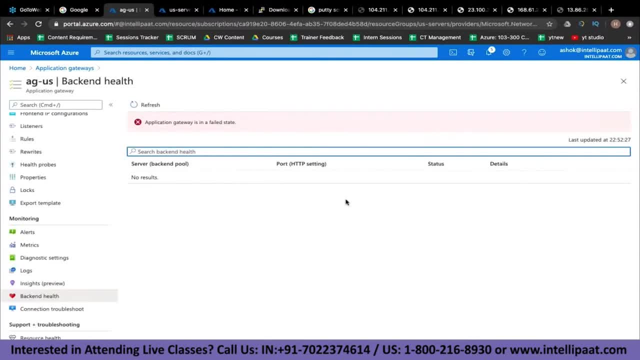 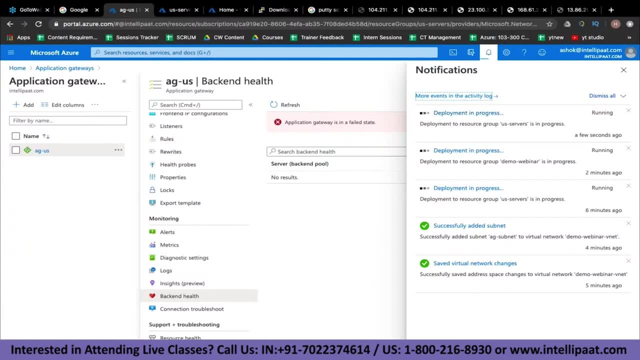 something, have something called as back-end health. okay, so application gateway right now is in deployment phase, right? so that's why you cannot see it right now, so let's wait for it to get completed. I think our application gateway is still in the deployment phase, so, as you can see, that deployment to group US servers is still in progress. so 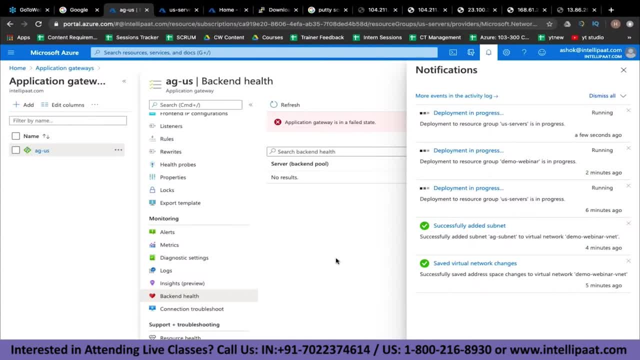 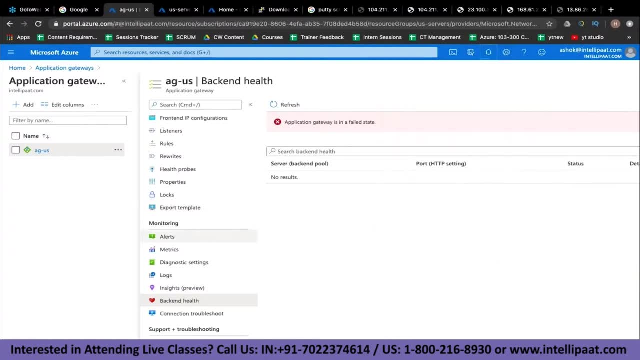 I guess the application gave they have not deployed fully and that's why you know it's taking some more time. so load balances are very, very heavy resource guys, so it usually takes around some five to six minutes to deploy. so let's wait for that that time. okay, so us so was one is filled when I succeeded, let's 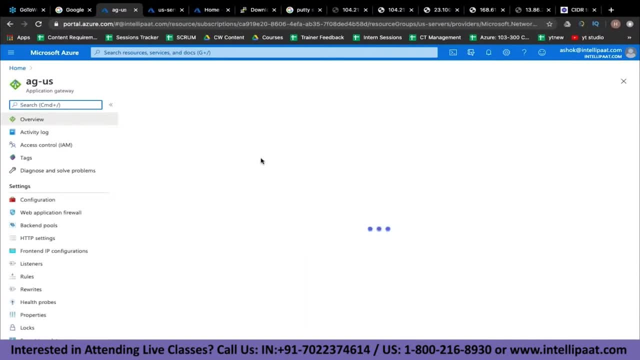 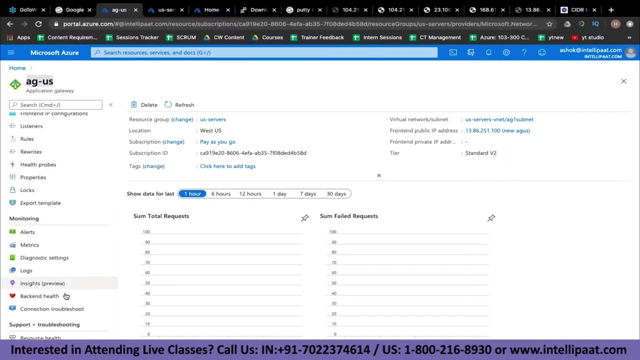 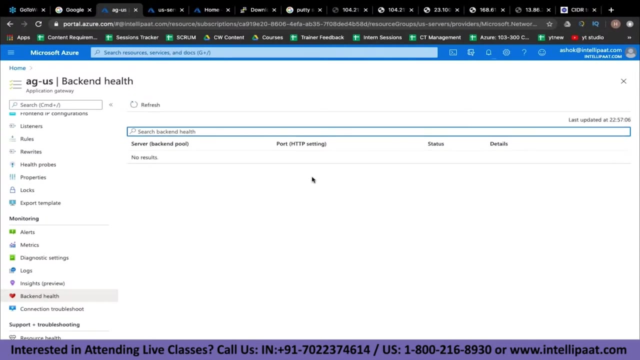 see if we have everything in my application gateway. okay, this is my us application gateway, guys, as you can see from the name. let's check the back-end health. so now you should have two servers listed over here which are not listed. okay, let's go to back-end pools. so there are. 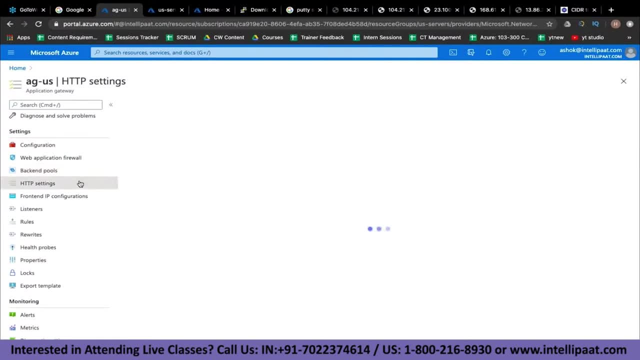 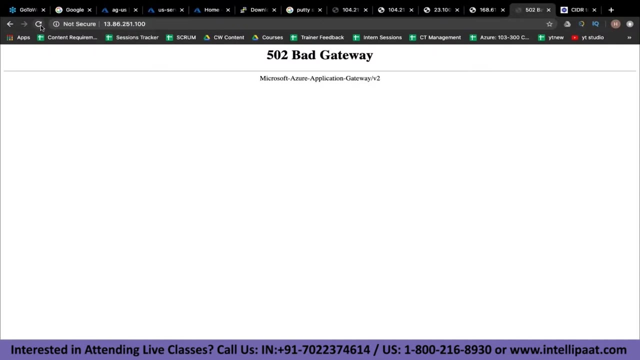 two targets, which is good. let's go to HTTP settings. this looks okay. rules looks okay. okay, let's try to go here, okay, and try to refresh this. okay, so at least our application gateway has been deployed. it just says that there's a bad gateway, so we will see how we can. 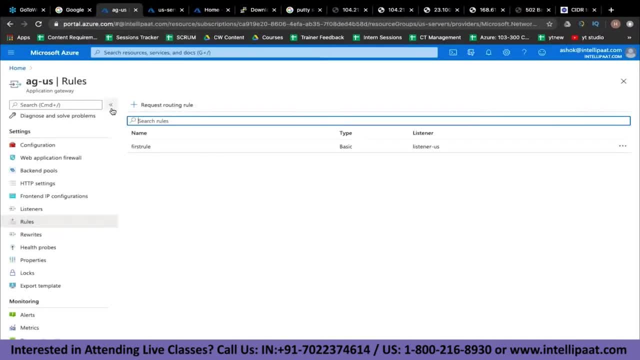 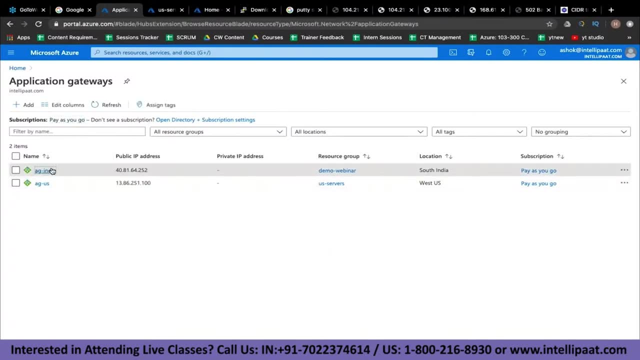 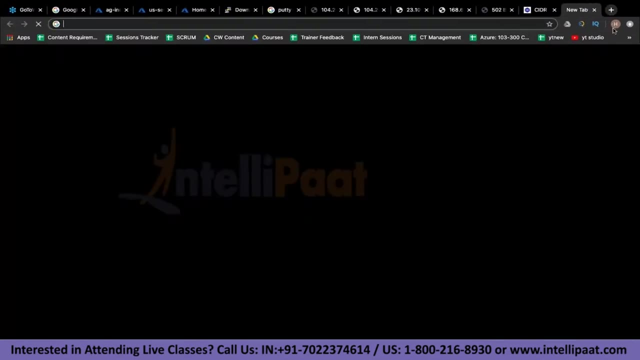 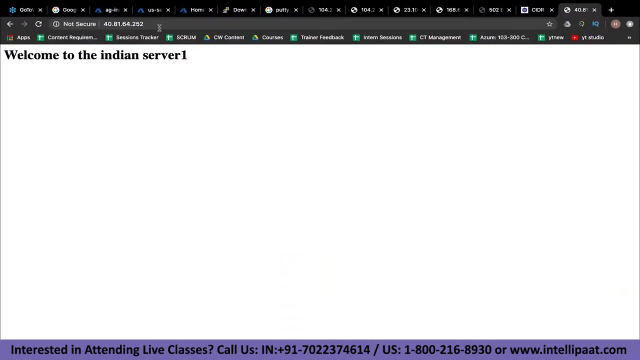 fix this. meanwhile even our Indian server has been deployed. I'm sorry, Indian application gateway. let's see how that is working out for us. so we'll go to the application gateway in there. let's copy the IP address, paste it in the browser. it enter. okay, this seems to be working just fine. so it says: welcome to Indian. 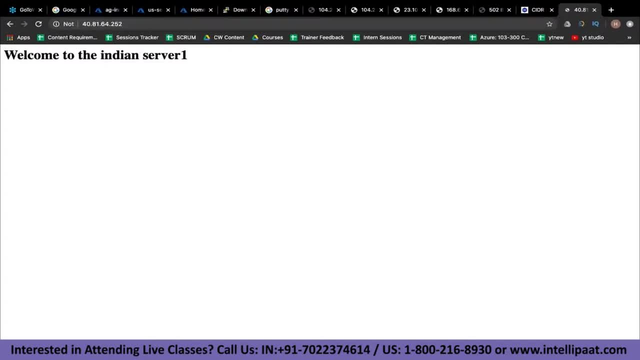 server one. great, if you keep hitting, refresh it. as you can see, it is now routing you to Indian server 2.0.. as well, right, again, it is out into one, again to two, again to one, again to two, so it randomly basically takes up your request and it is now routing it to you. 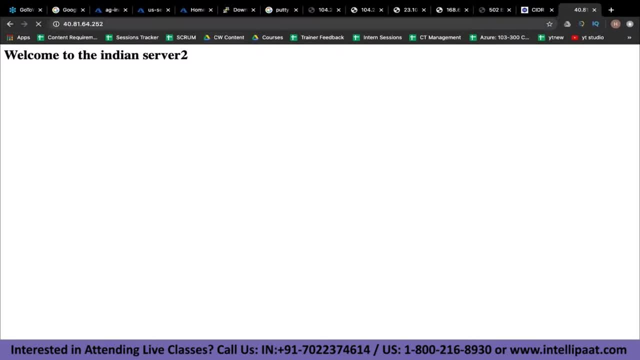 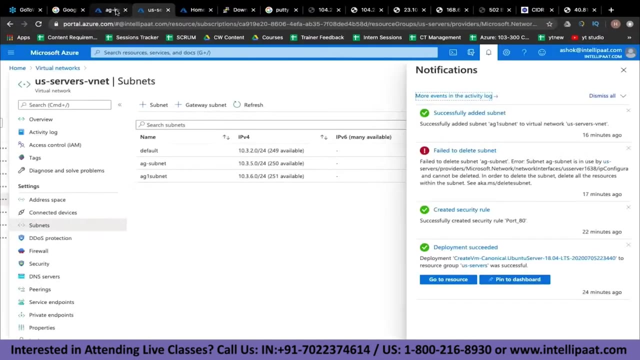 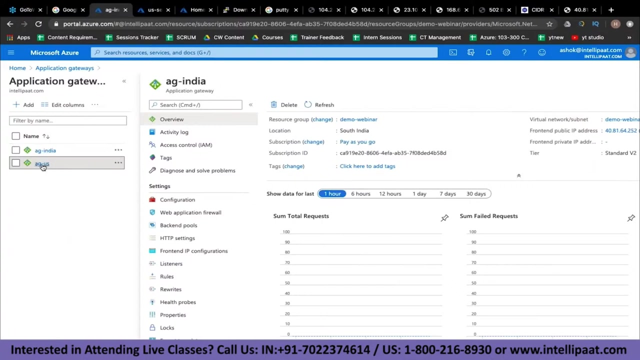 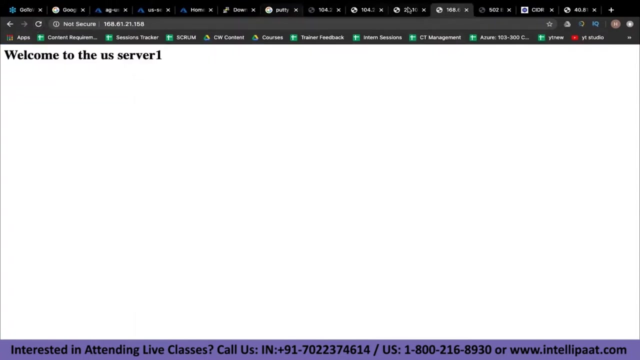 routing to one of the servers. so this is working fine, and the US application gateway is giving some issues to us. so let's see how we can figure that out. let me just go to the US application gateway. so first things first, let's see the US servers are working fine. yes, the first. 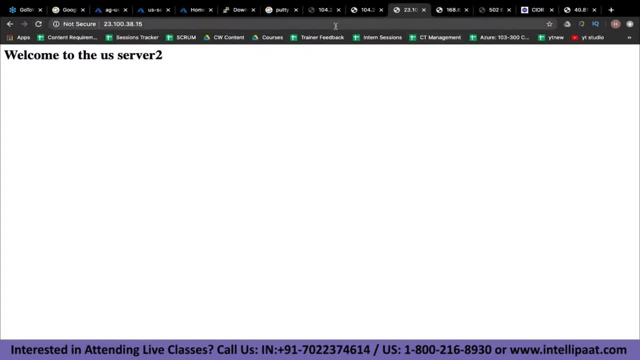 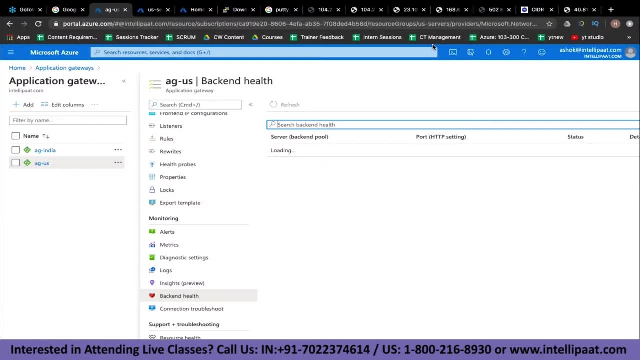 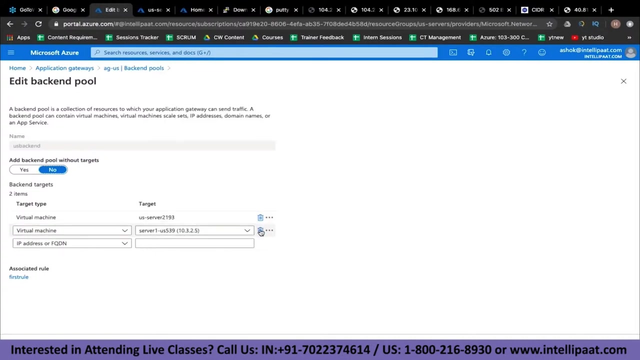 server is working fine and the second server is also working fine, great. so I think the problem is that the backend health is still not restored over here and because of this, I think it's giving you as a 502 error. okay, so to fix this, what we can do is we can go to back in pools and we can just delete these. 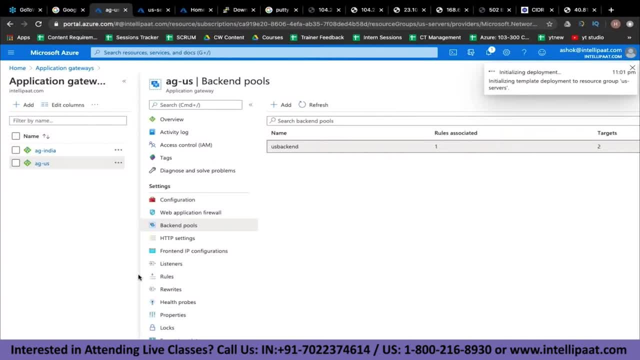 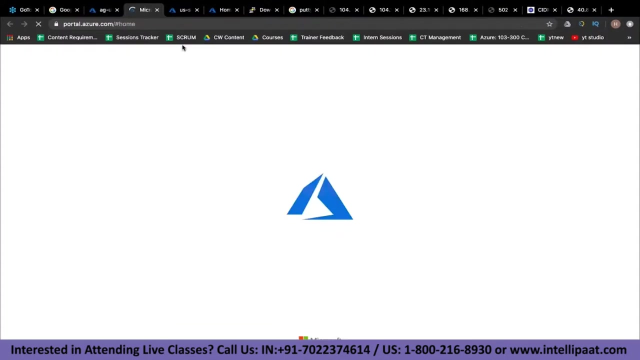 targets, save it and once this deployment is successful, we can add the new two targets- again the two targets, and I think that should solve the problem. okay, so while this is happening, let's go ahead and configure a traffic manager now so we can see that the India load. balancer is working perfectly fine. so now what we'll do is: let's create a traffic manager, okay. so let's create a new traffic manager, let's click on add and let's call it as global traffic manager, and we can deploy it in any region. let's say, we are deploying it in US. okay, resource group would be US. 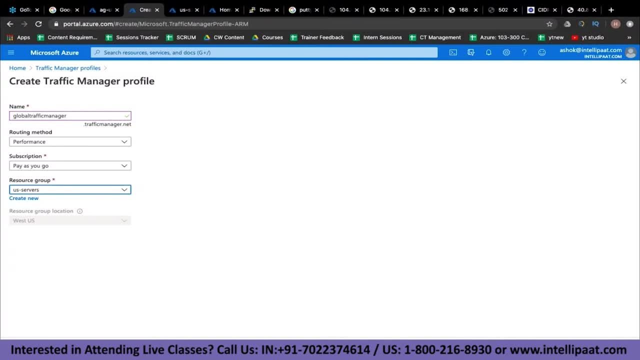 servers. okay, this is very important: the routing method. so we want to route it according to geography, right? so wherever the request is coming from, that request should basically be routed to the servers which are near to it. so we have chosen the routing method as geographic. let's click on create and with this, our traffic manager has now. 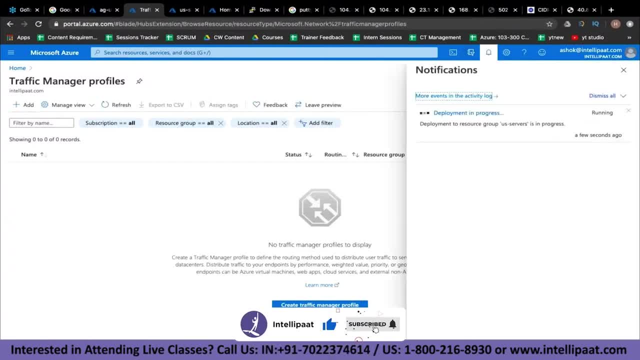 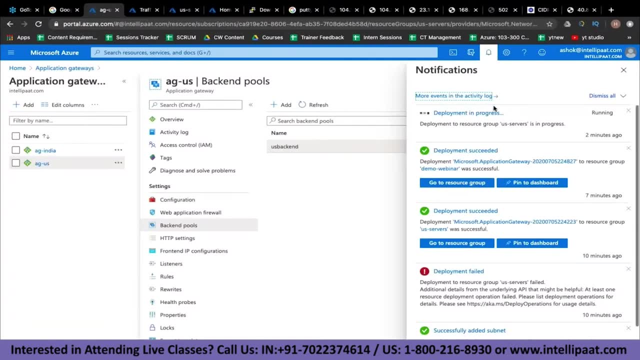 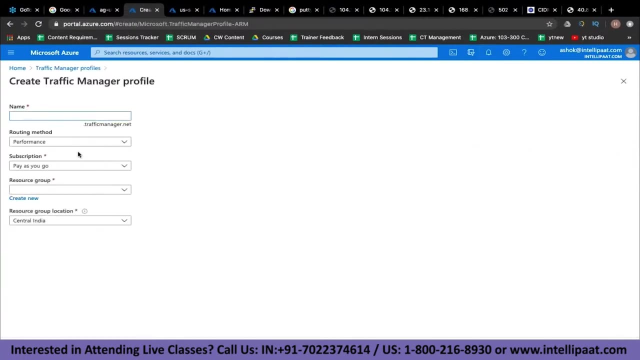 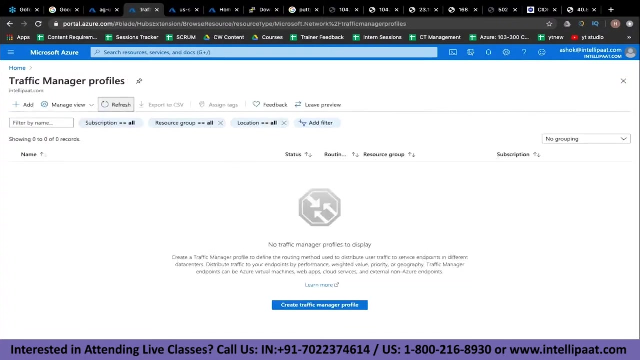 been created. okay, now, this will take some time, so you let's give that time to it. and now let's click on add. so in the traffic manager profile- okay, we've already added it, so it should list here- let's refresh. so it will take some time to. okay, so deployment has succeeded. great, so the 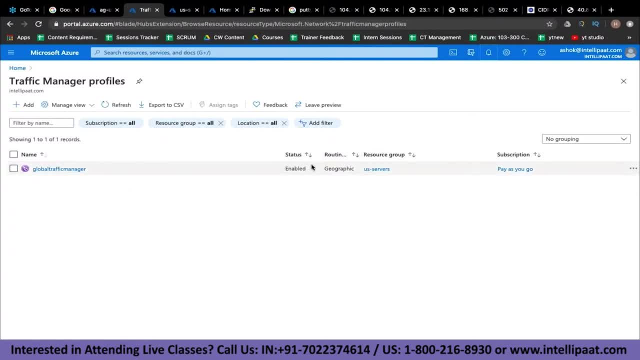 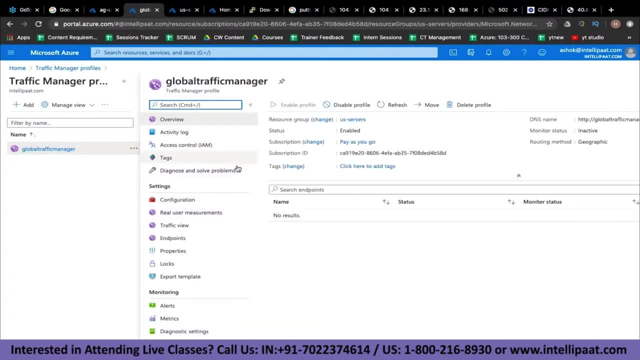 traffic manager. we can see it over here. now the status is enabled, so we can go inside this traffic manager now and what we can do is we can configure it to connect to our load balancers. okay, so for doing that you will have to go to configuration. 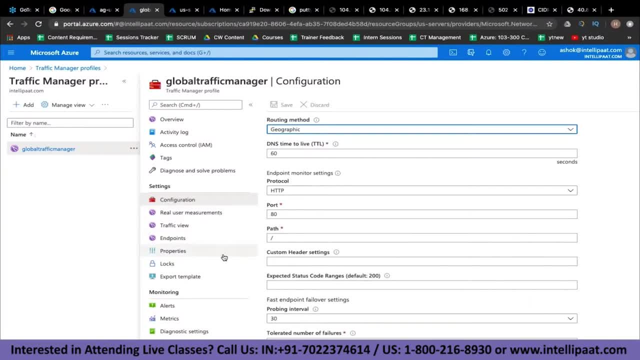 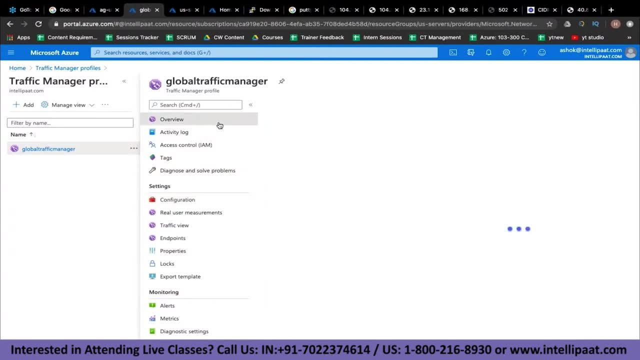 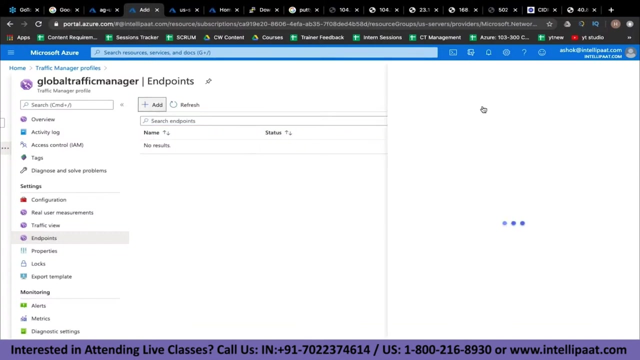 okay, everything looks good over here. so now we are, we have to add endpoints, since there are no endpoints over here. so we'll go to endpoints- add an endpoint. so let's add it for the Indian server first, right, so the so whenever you're adding the end points, you have 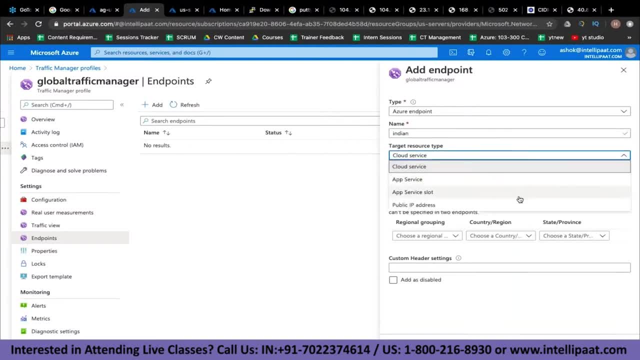 to make sure of one thing, which I'm going to show you in a little while. so first of all, let's select the public IP address, and the IP address would be for ag in there. so, as you can see, it says no dns name is configured. right, so what? 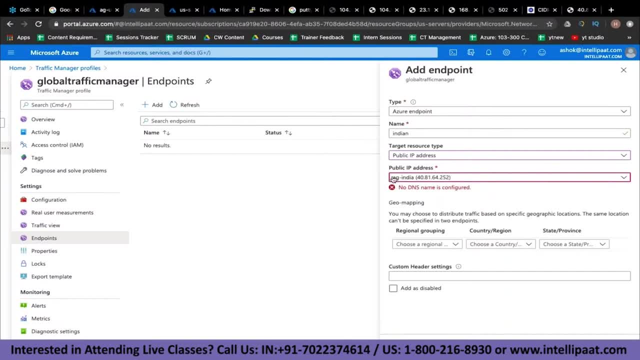 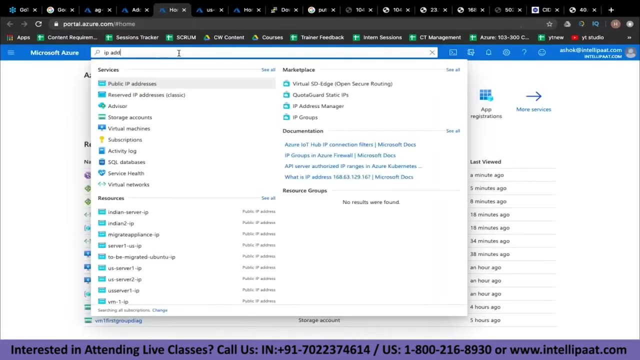 you'd have to do is for the ag india ip address- ag india is with nothing but the application gateway of india- you will have to configure the dns, okay. so let's see how we can do that. let's go to the uh ip addresses page. go to public ip addresses. 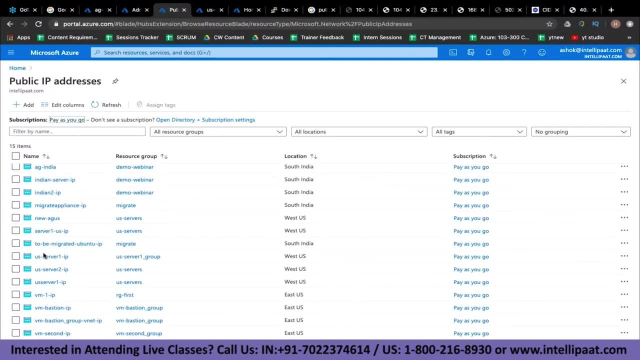 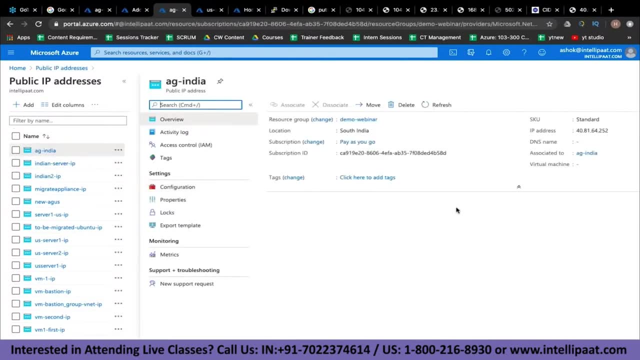 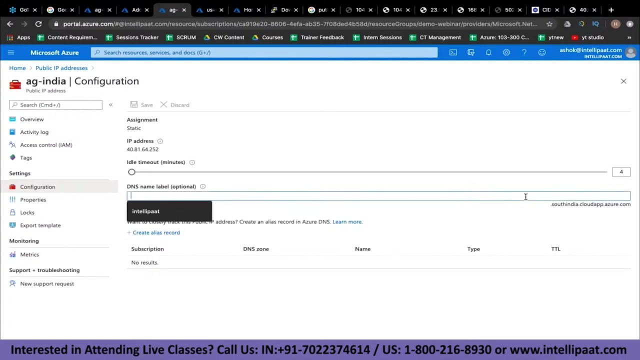 here we'll go to ag hyphen india, which is this and ag hyphen india. now what we'll do is we'll go to configuration. in configuration, we can give the dns name right. so all our ds, dns names we're going to have this suffix attached with it. so let's give this as ag. 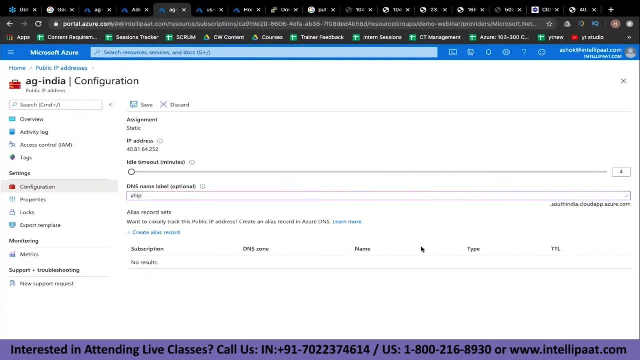 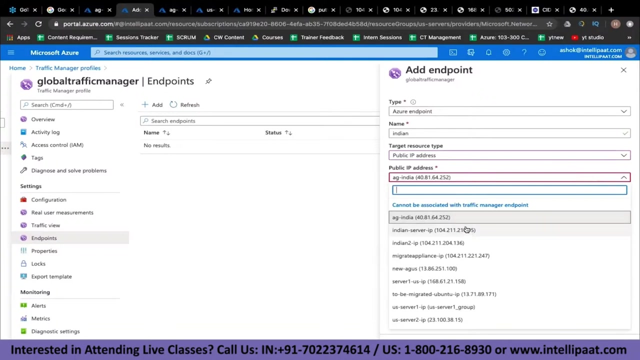 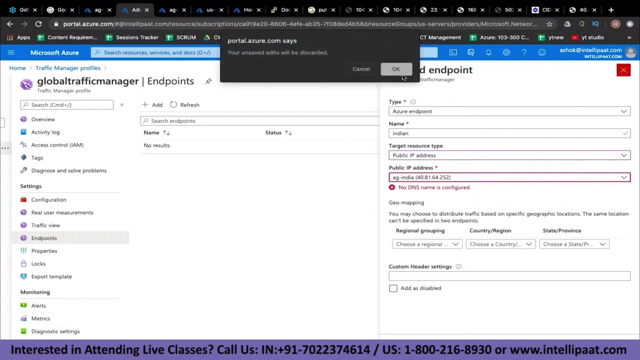 ip. now it is checking whether it's available, so it's a gip, so it's available, and now we can just click on save. with this, our public ip address is now going to have a dns name. okay, so it's done. and now, over here, i will have to, i think, refresh this, so let's. 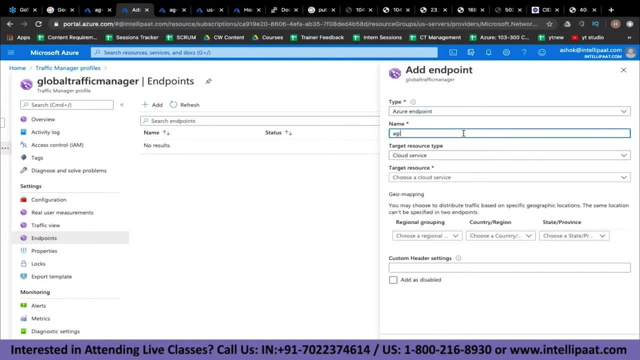 add an endpoint again. let's call this as, eg, india endpoint. it's going to be a public ip address and the ip address is aging great, so let's click on add and now i can just do a regional mapping over here which is going to be mapped to it, so here we can choose to distribute traffic based. 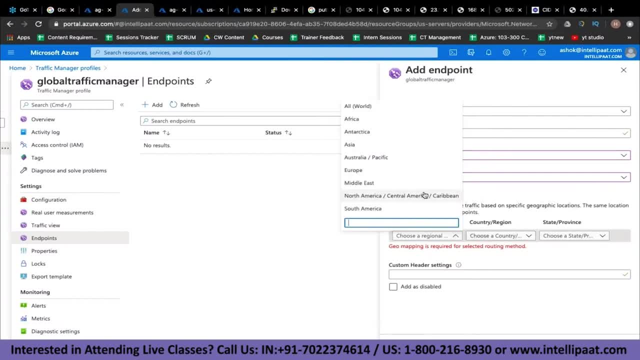 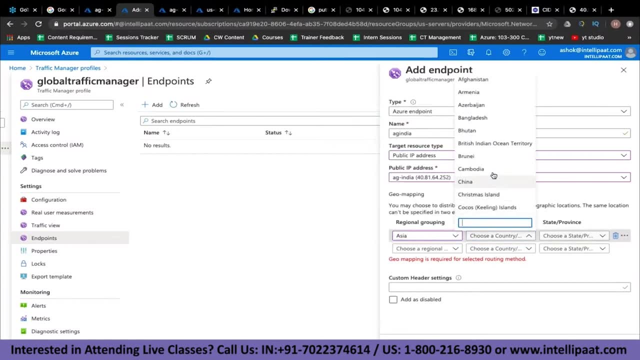 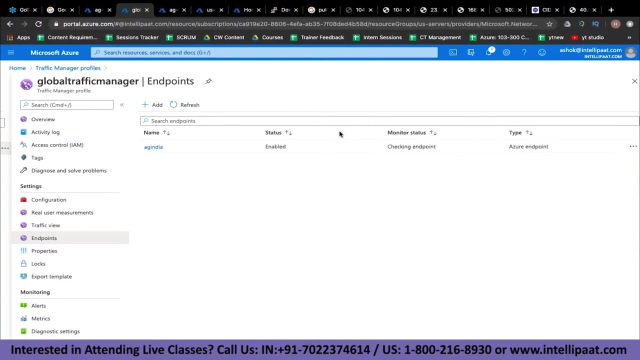 on specific geographic locations. okay, so anybody who's pinging from asia in asia- let's say india- then they should basically be routed to this endpoint. okay, so with this, your endpoint has now been configured in the traffic manager to connect to your asian servers. so now let's verify. 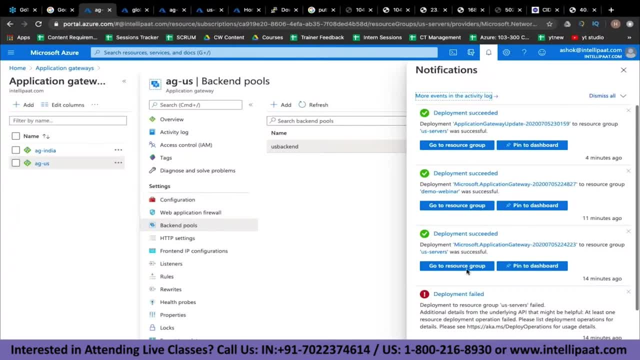 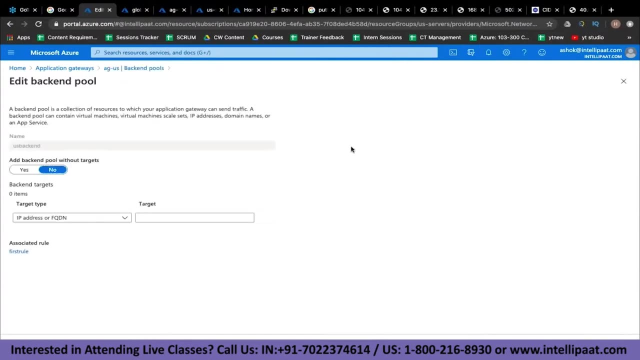 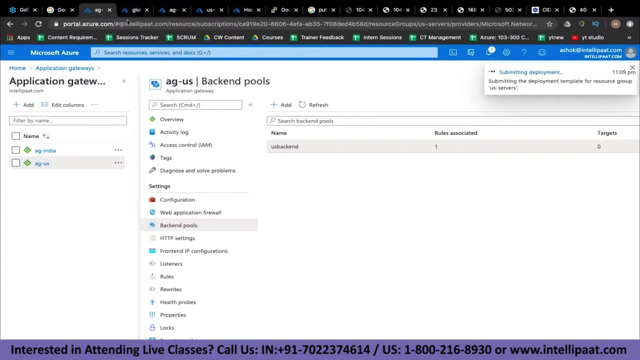 uh, if my ag us, yes, so an application gateway, the for the us servers. it was successful, great. so now what i can do is i can again add the targets and that should solve our problem. okay, so the deployment is now happening. meanwhile, let's verify if we go to our traffic manager. 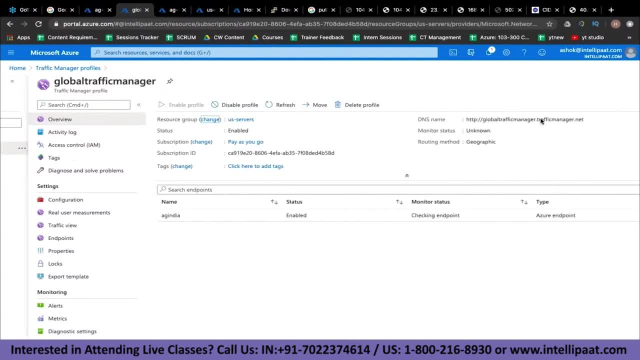 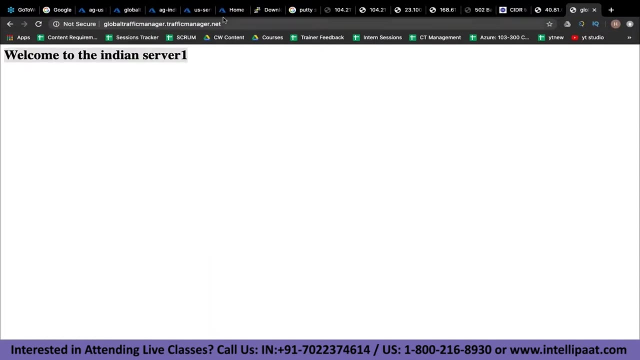 which is having this dns. are we able to access the servers or not? so yes, we are able to access the indian servers right. so we are able to access the indian servers right. so that means our traffic manager is working just fine. so i can give you this ip address as well. 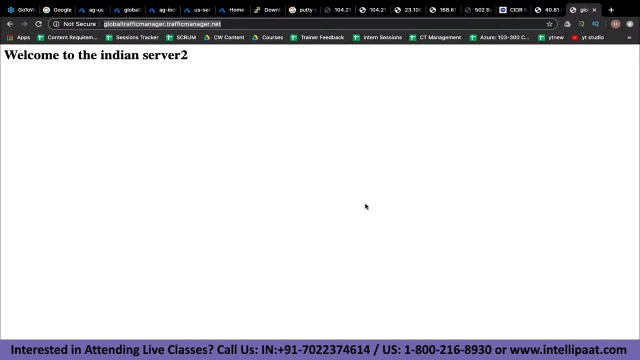 so right now because only indian ip addresses are there. that's why our indian servers are connected to it. our indian endpoint has been added. that's why only the indian servers are connected. but as soon as we also add the application gateway for us people who are from outside asia, they will be able to connect to it. we will just 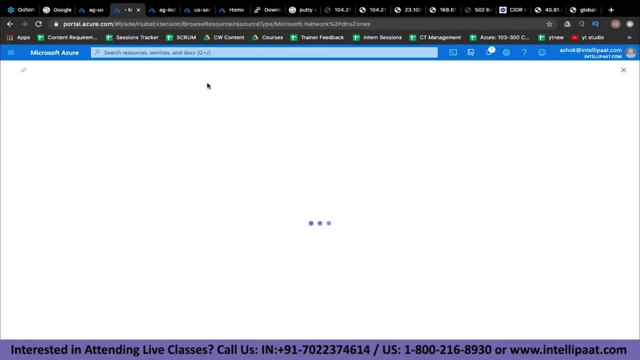 search for DNS. this select DNS zones. so here you can basically add a rule, or you can configure a custom URL which can connect to your traffic manager, and let's see how we can do that. so if you want to do that, guys, the simplest thing to do over here would be to first go to. so there's a website called free norm. 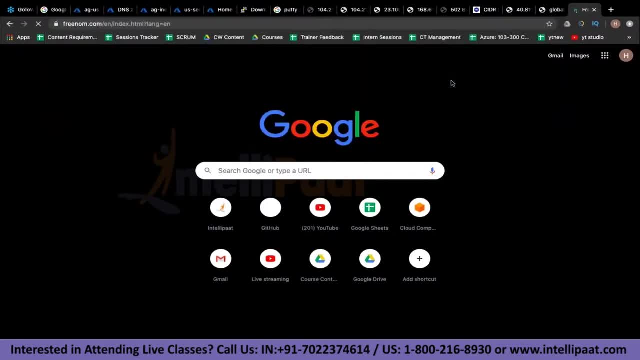 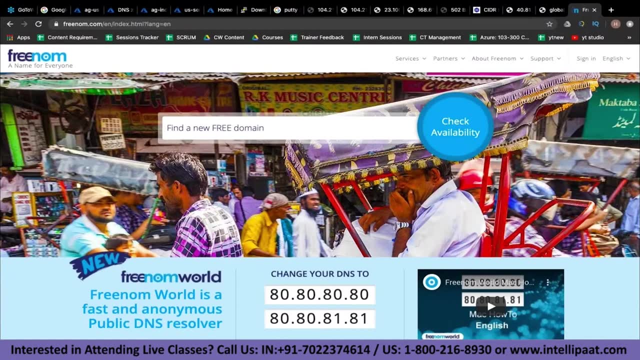 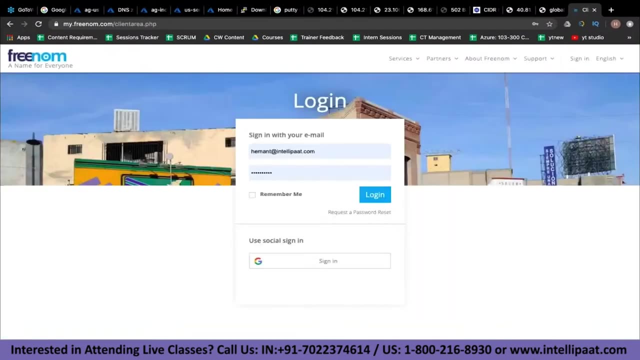 just go over there. so free norm is a website which basically gives you a free domain to work with. okay, so let's sign in. I already have signed up over here, so you guys can also sign up, and with this, what you're going to get is you're gonna get. 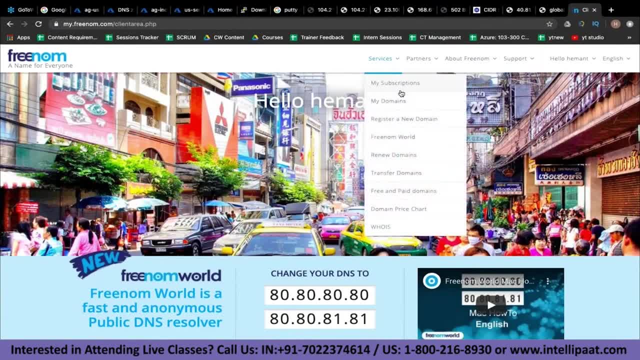 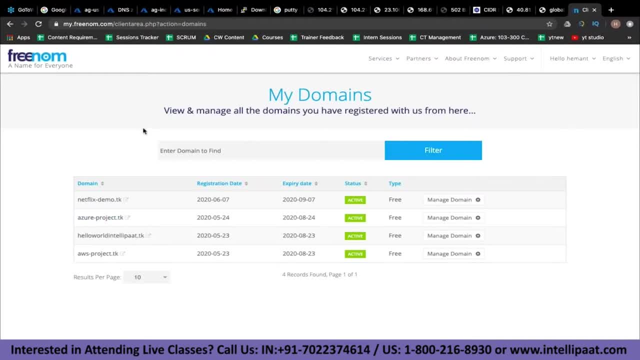 a domain that you can use for free. so, for example, I have a as your hyphen project or TK domain, which now I'm going to configure to connect to this traffic manager that I have specified, and then all I have to do is the moment I go to. 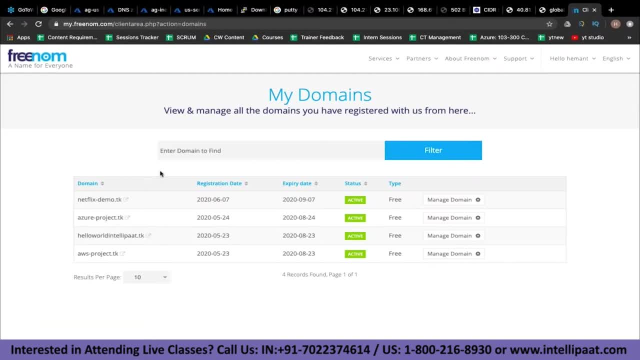 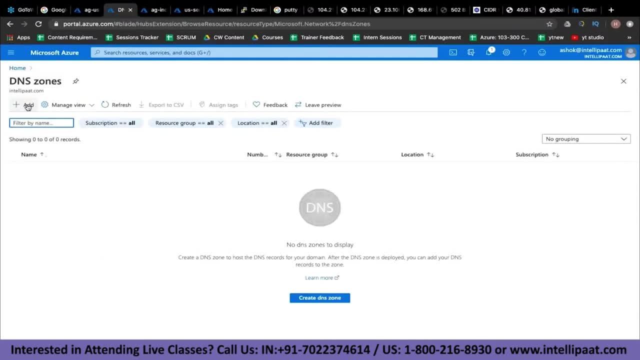 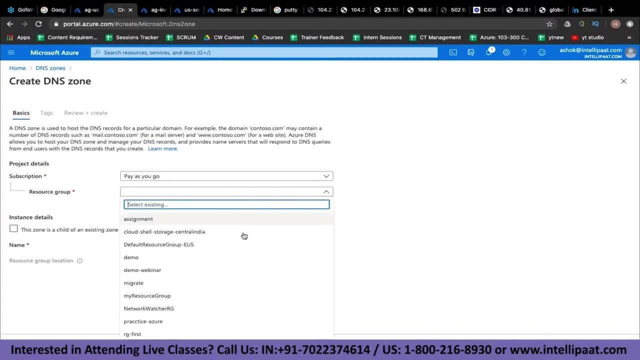 as your hyphen project or TK, I would be able to see the website that I've deployed. okay, so in order to do that, just go to DNS. so first you will have to add a DNS zone. let's specify it in us again and the name that we will give. 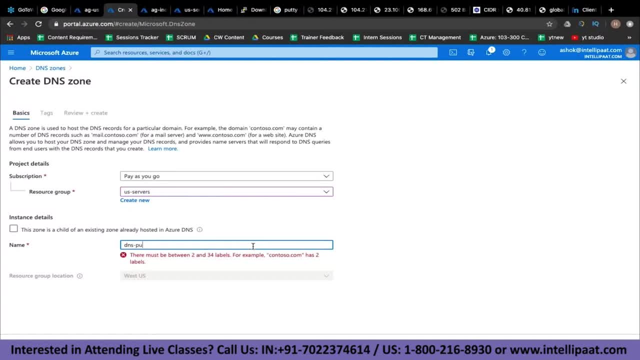 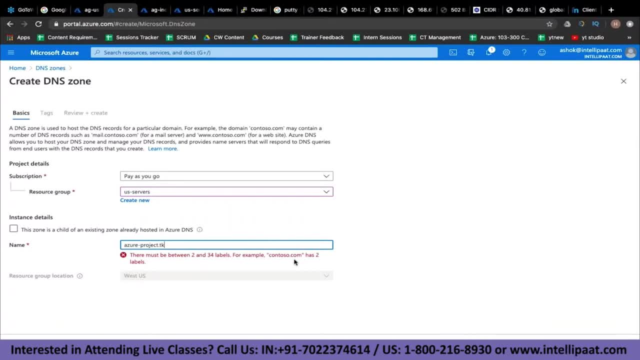 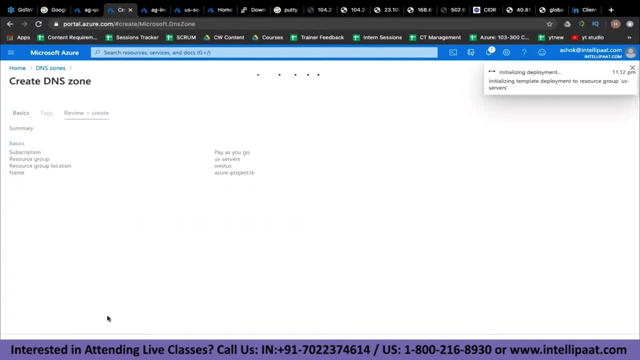 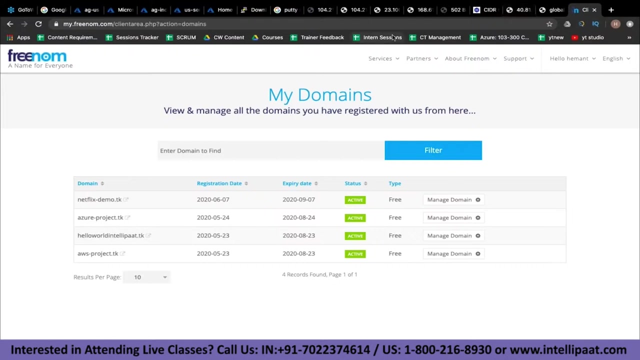 hyphen project: dot TK. okay, let's click on review plus create. create it and with this, our DNS zone will now be created. and this DNS zone we will have to connect our domain to this DNS zone and then we will configure a DNS zone to connect to our traffic manager. so that is how the flow is going to work. so let's. 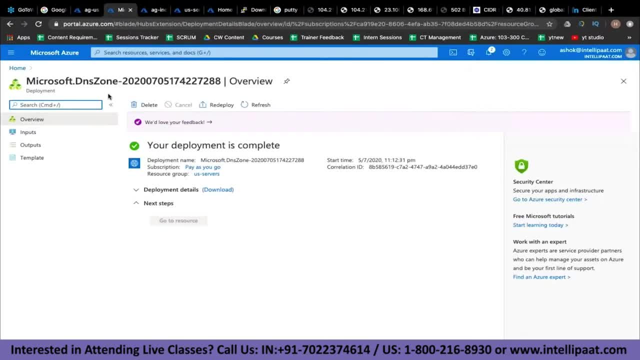 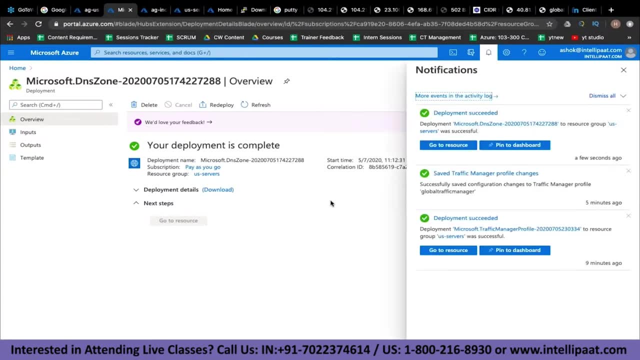 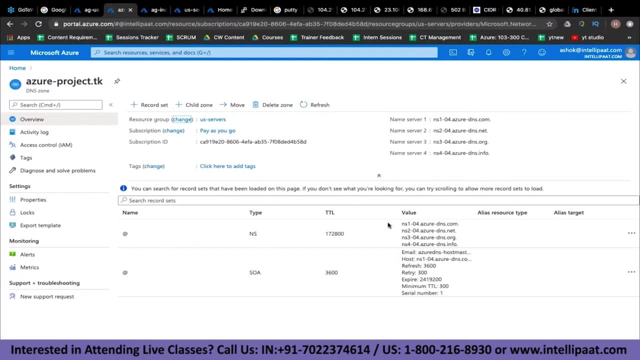 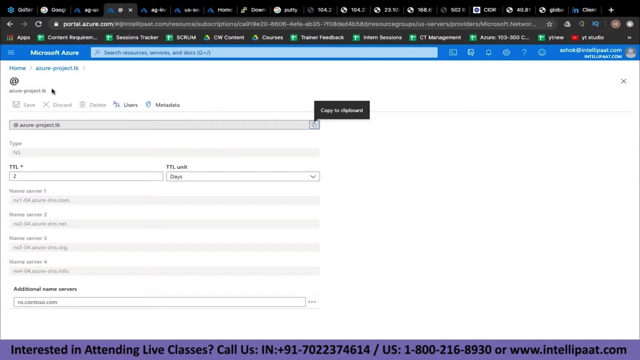 see what happens. so the DNS zone deployment is complete, so we can just go to the resource. so here we are, and here- this is the most important thing, guys- you get name servers. you get four name servers over here, and these name servers you basically have to configure in your website, which is basically giving you 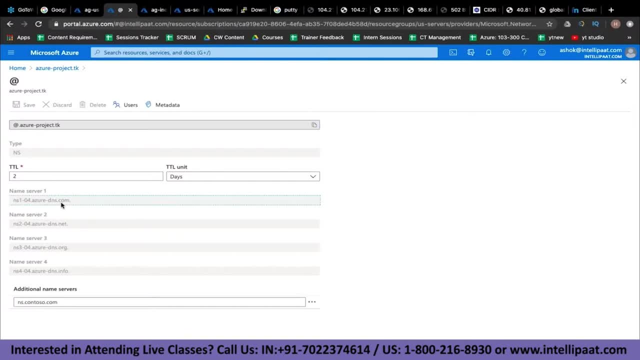 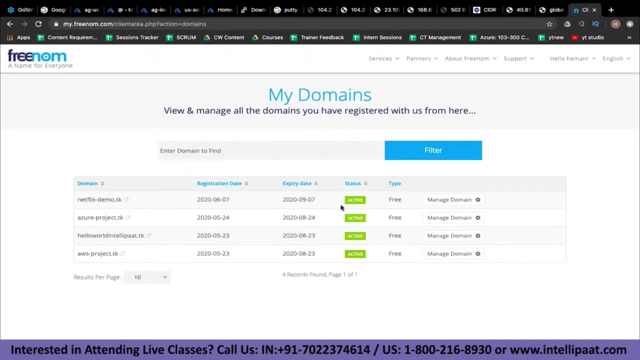 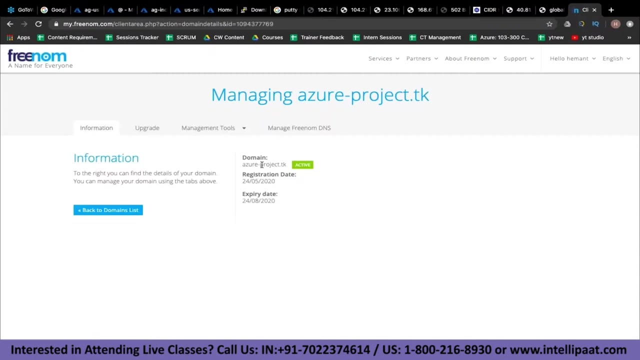 the DNS name. okay, so let's copy these. let's go to a free norm website. go to the domain that we want to configure. it's going to be as your hyphen project, so we'll click on manage domain and in manage domain will go to management. 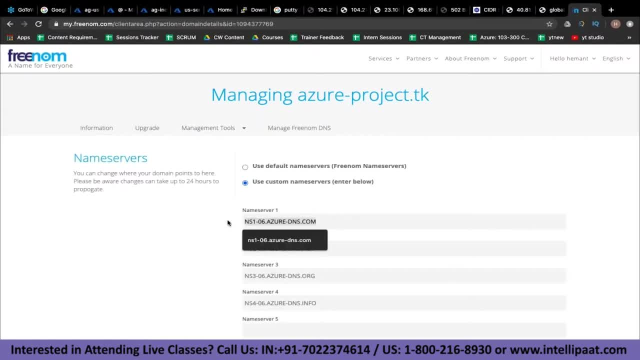 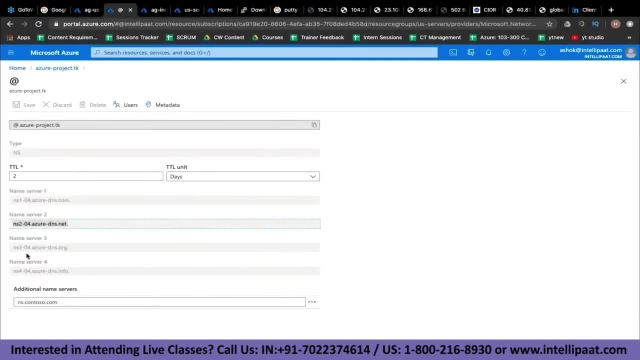 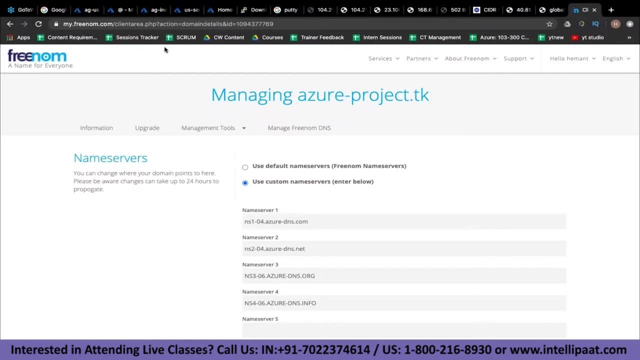 tools and then name servers. so just replace the name servers that are there with the new ones, and that should be it. that's about it: how to configure your domain to basically connect. so let's copy it one by one, okay, so now just click on change name. 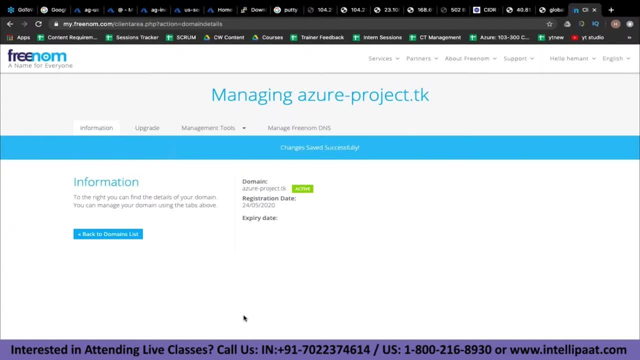 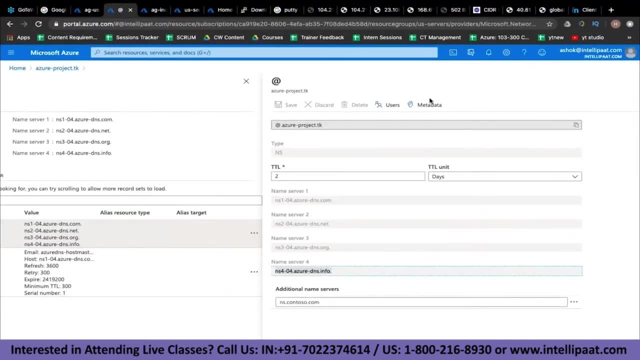 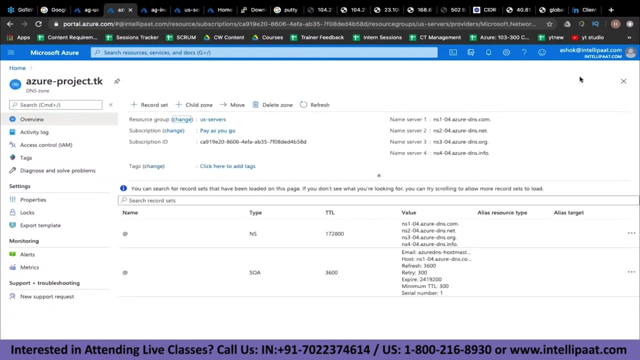 service, and that's it. that's all you have to do on the free norm website. okay, now come back to your DNS zones over here and now what you can do is just: you can choose this. okay, now you just have to point your DNS zone to your traffic manager, so just. 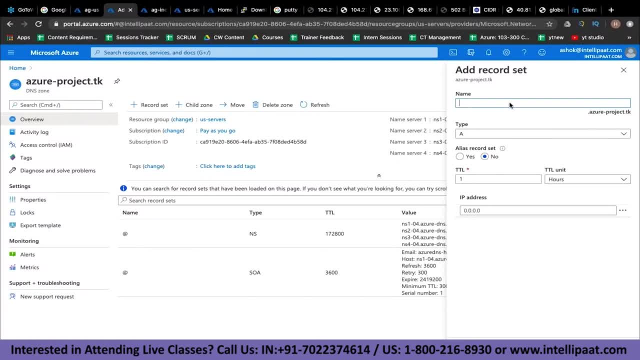 click on record, add a record set and this let's configure it to be CNAME. and it is the global traffic manager that we want to point on. okay, let's click on OK. so here we have to enter something. so let's enter www and let's click on OK. okay. so with this our record set has now got created, and it will take like a minute or two, or sometimes it even takes 24 hours, to basically make a change on the DNS server. so we'll check that. meanwhile, let's come back to our application gateway. check the back-end health now and let's see if this has. 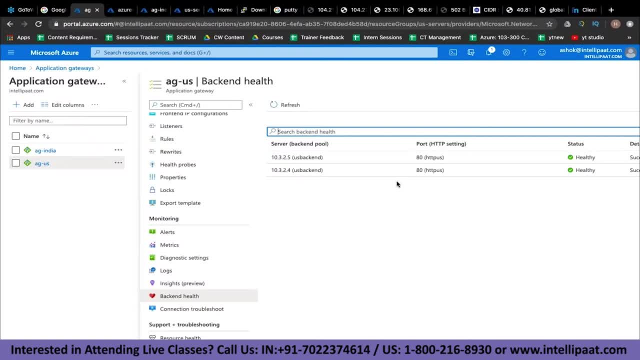 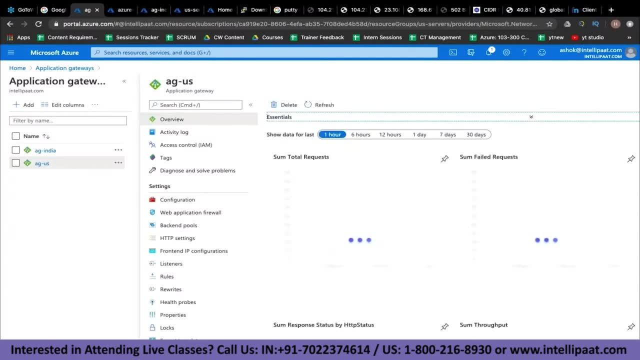 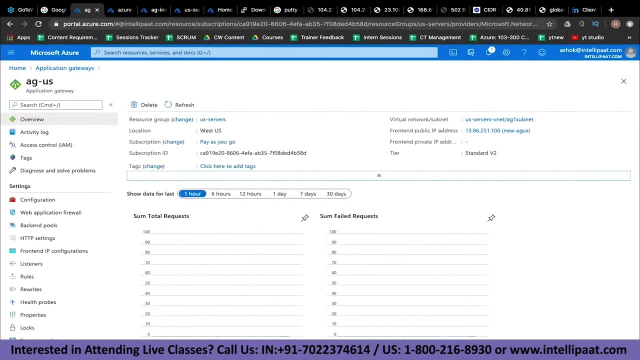 loaded. great. so now it is showing us both the US back-ends right in the application gateway of us. and now if we go there, and now if we go there, and now if we go there ahead and try to connect to it, this is the IP address. great, we are able to. 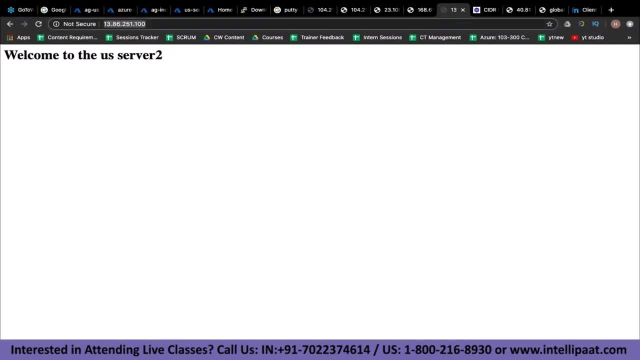 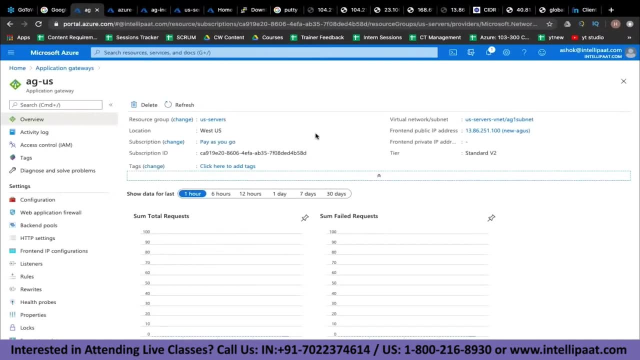 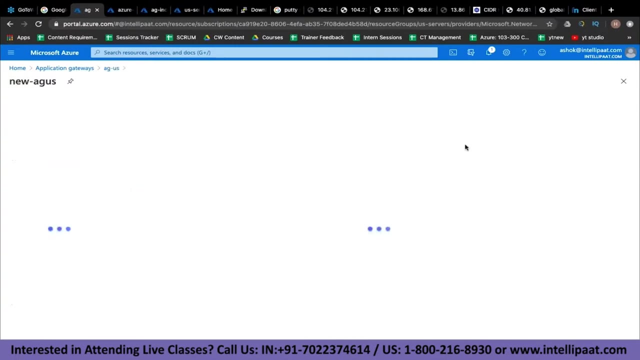 connect to the us servers and we can see that it first connected to the once one, then the second one. so let's now what I'll do is, on this application gateway, the IP address that we have just caught, let's configure that to have a. 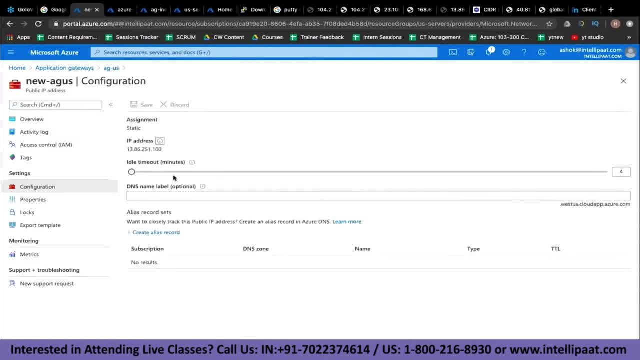 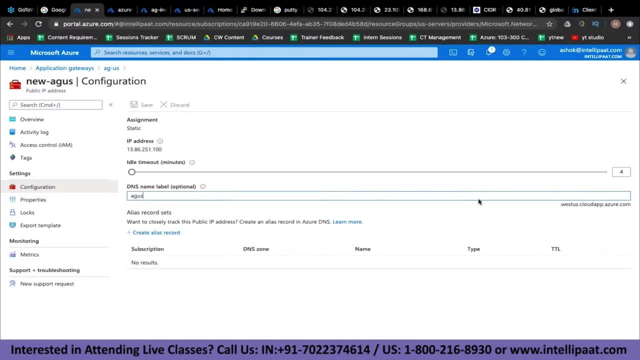 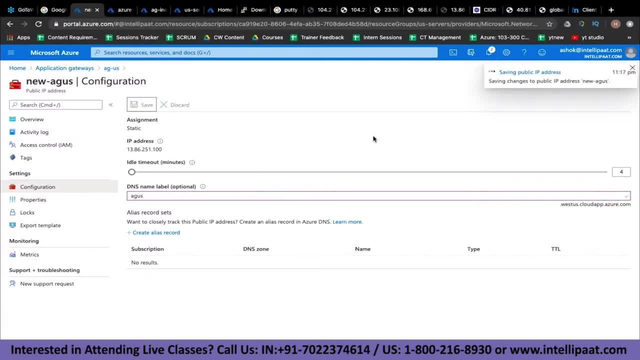 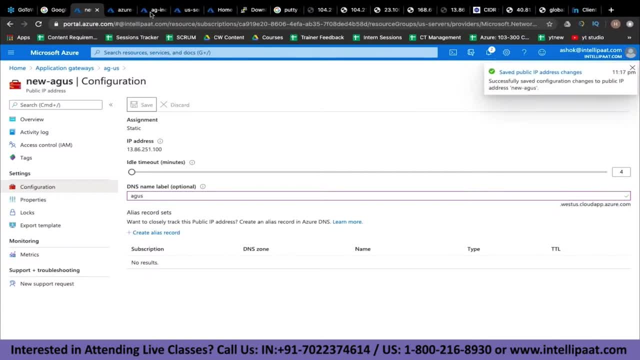 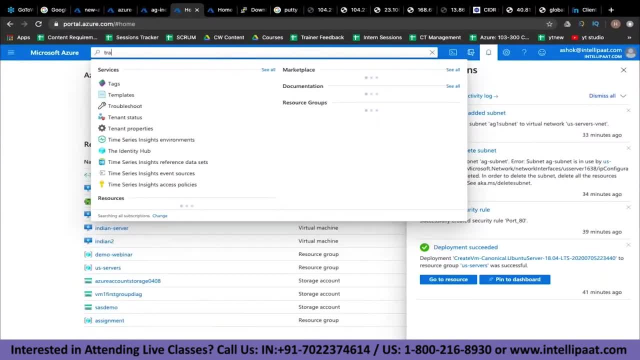 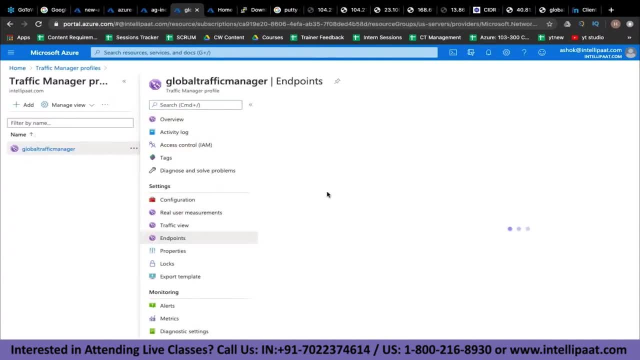 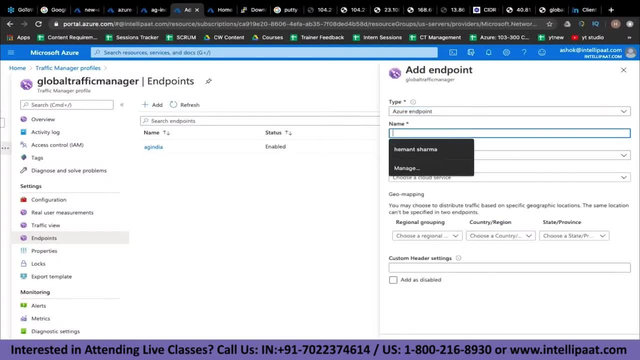 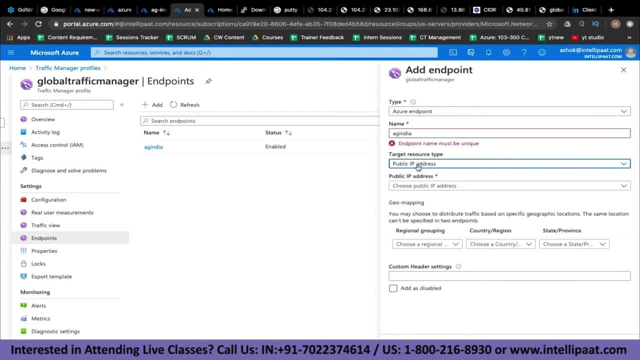 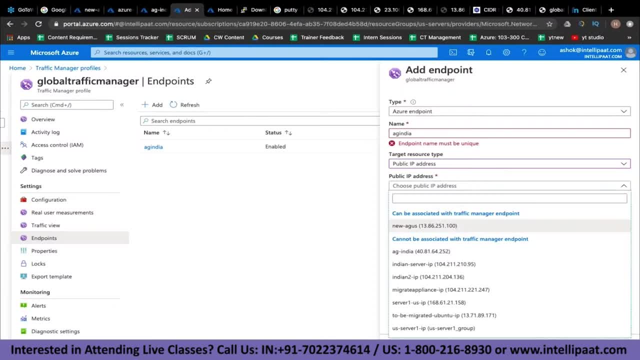 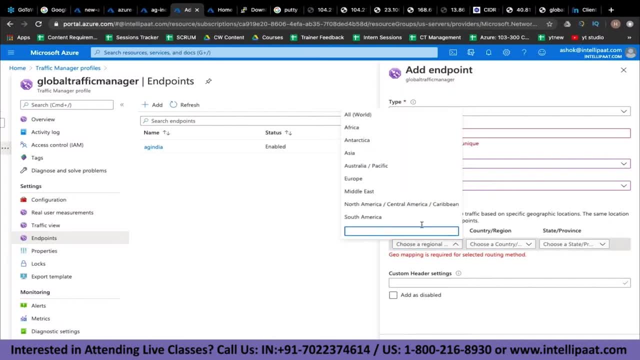 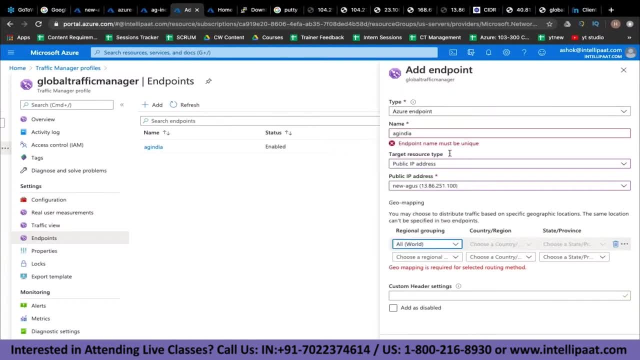 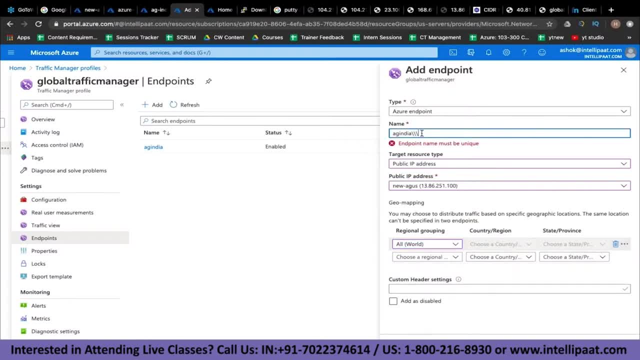 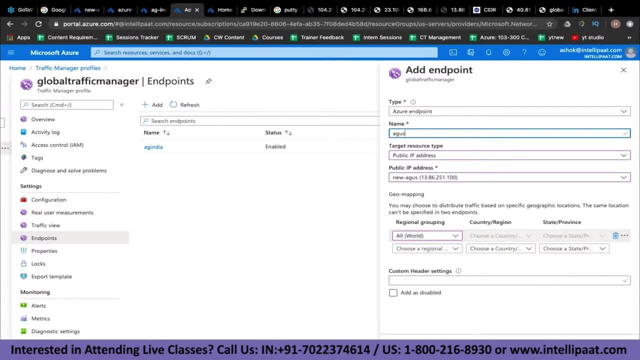 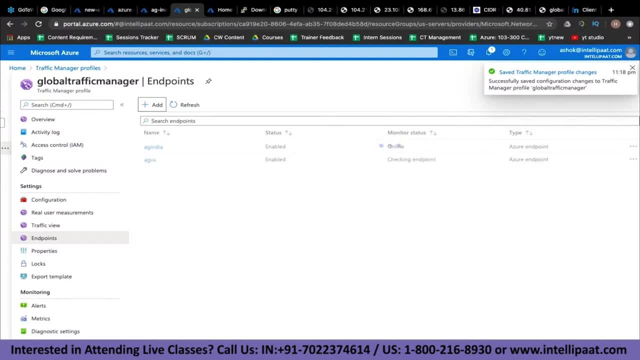 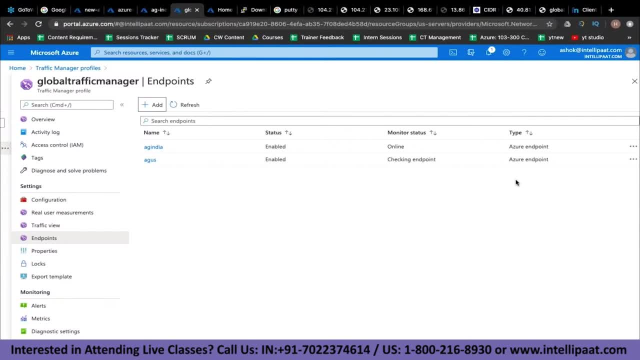 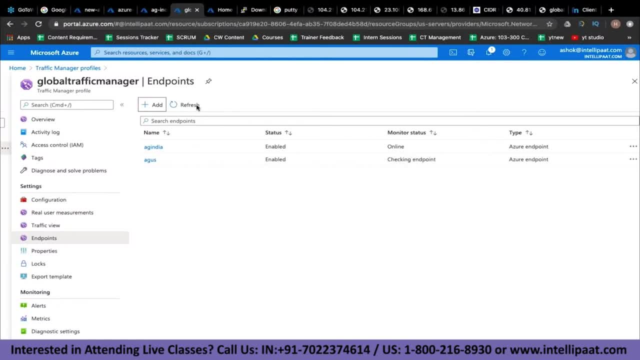 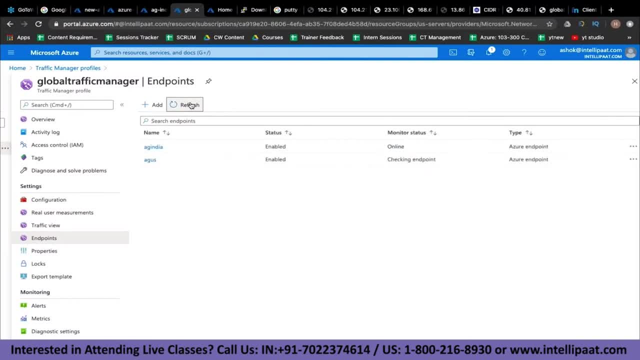 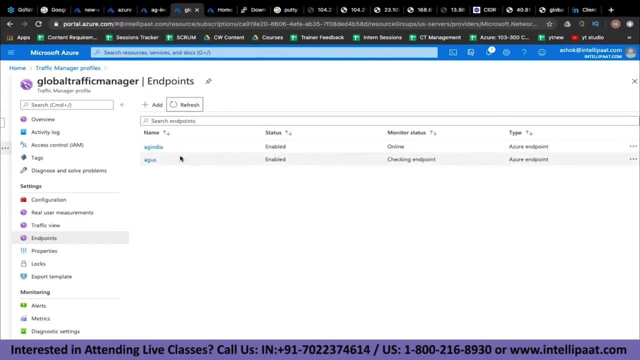 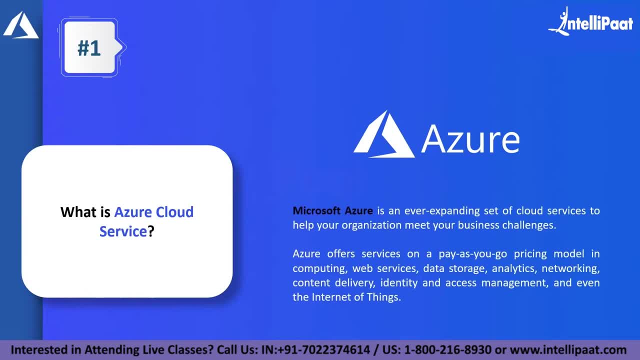 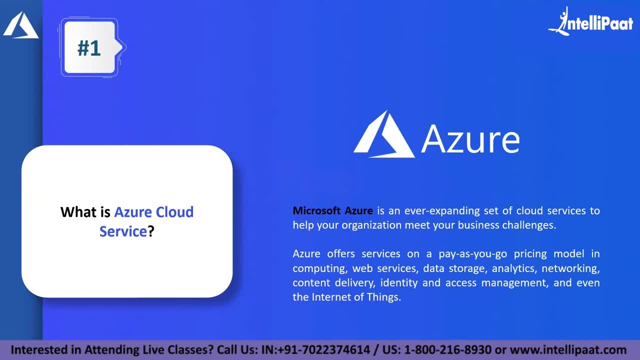 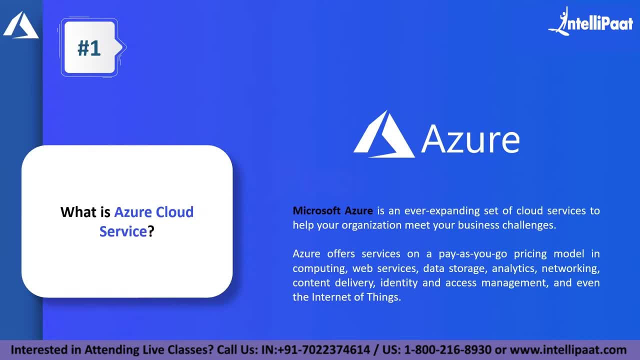 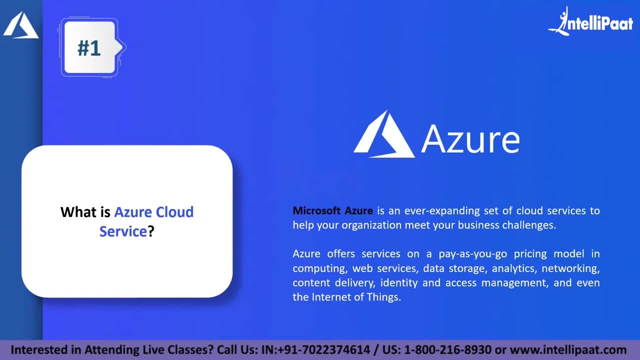 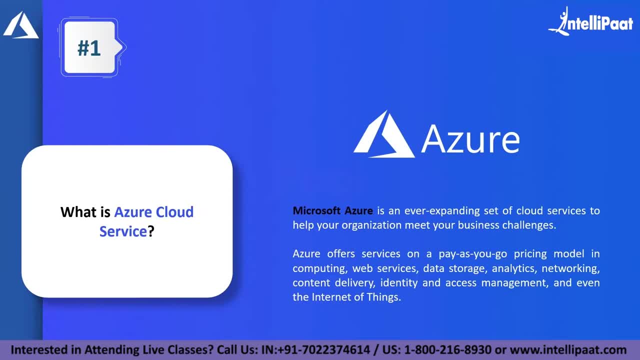 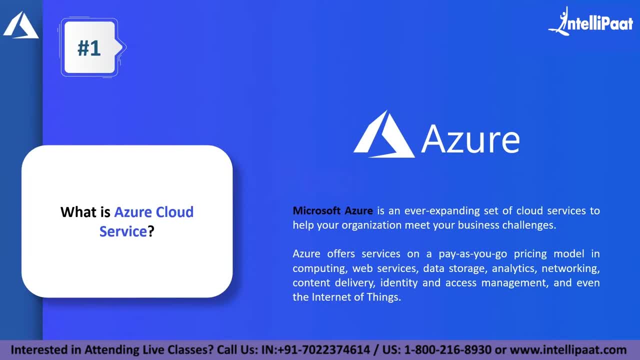 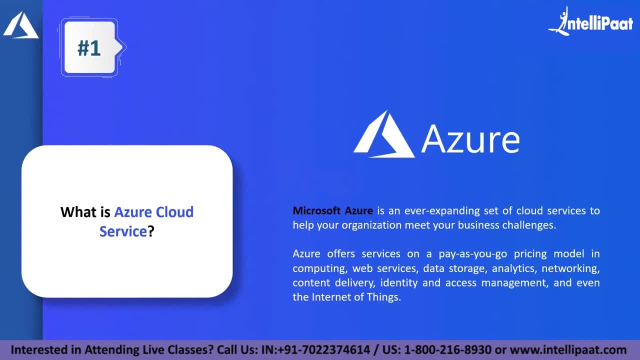 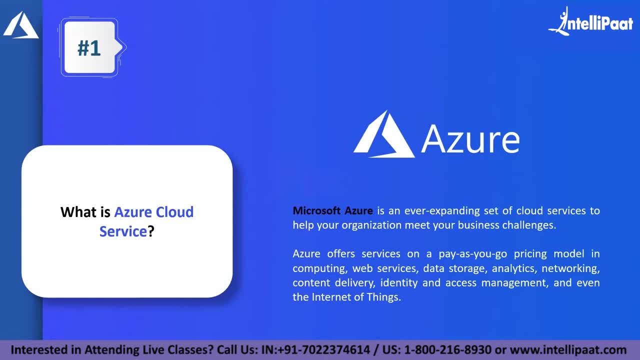 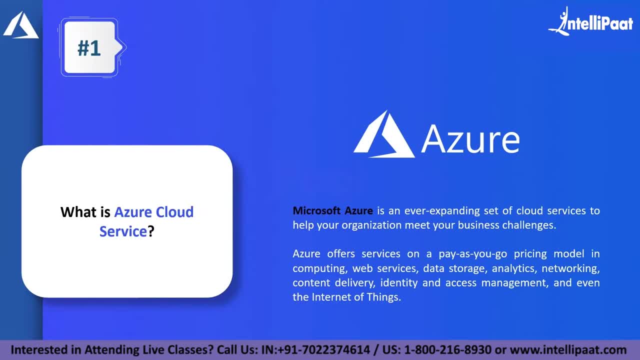 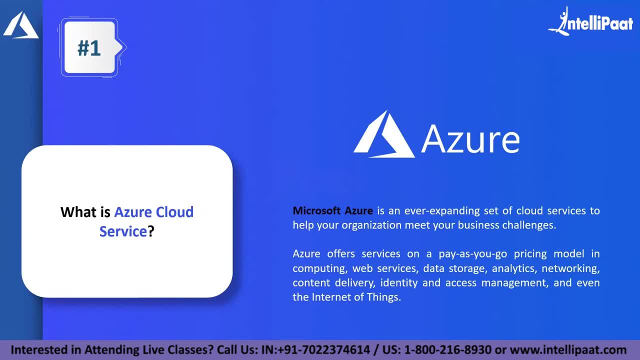 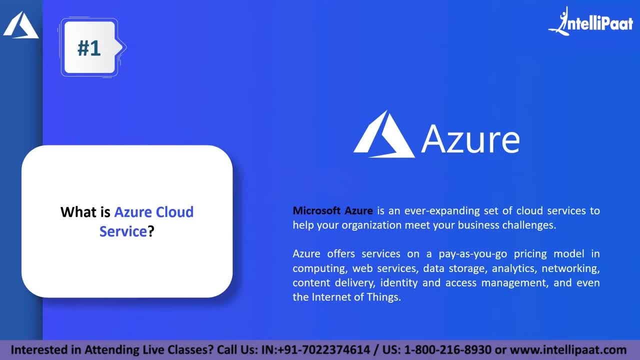 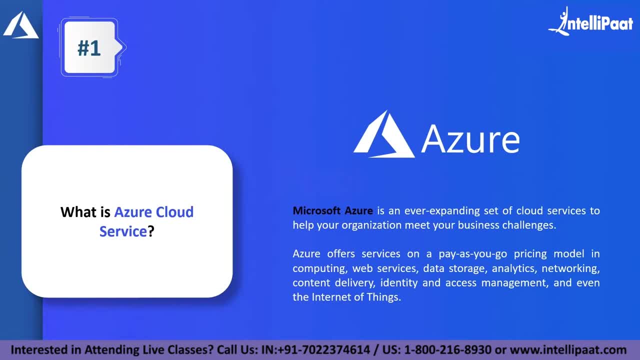 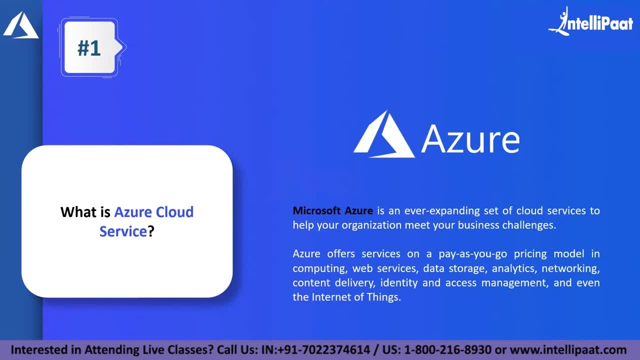 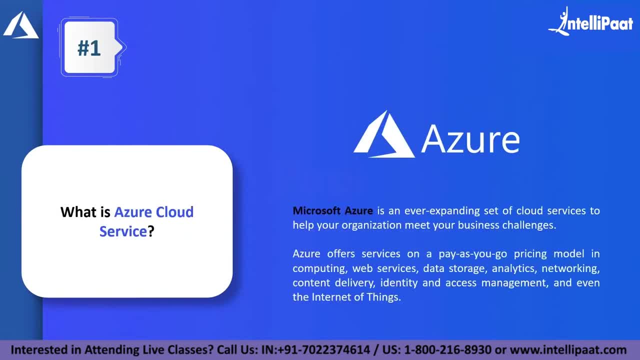 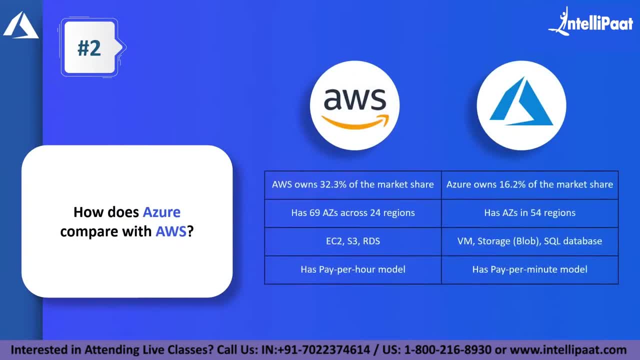 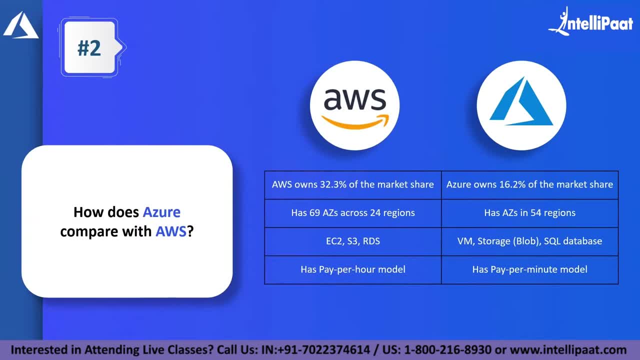 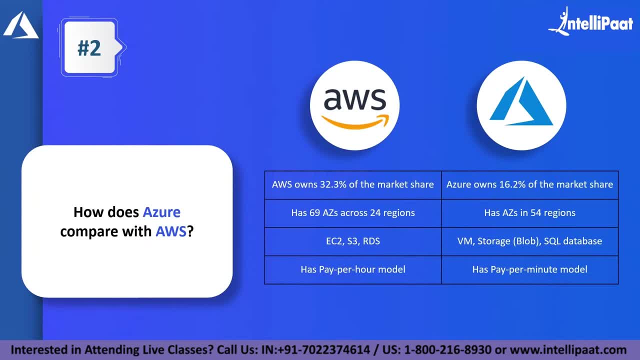 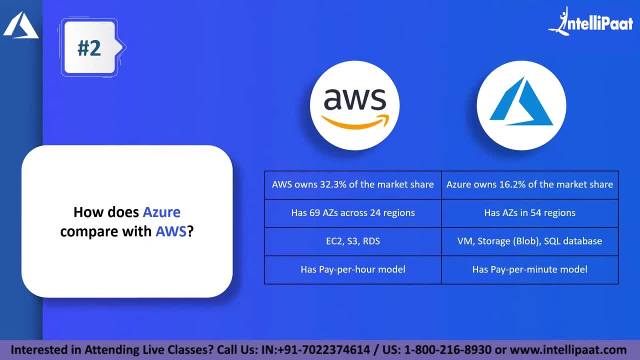 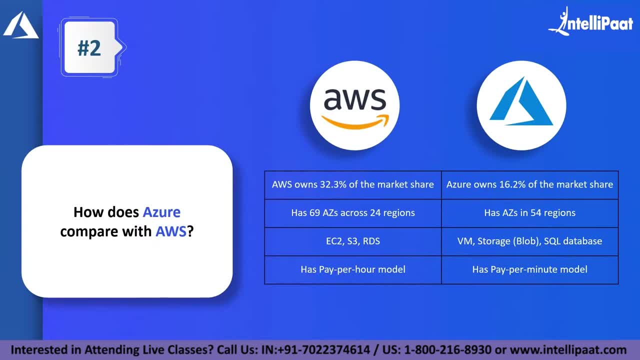 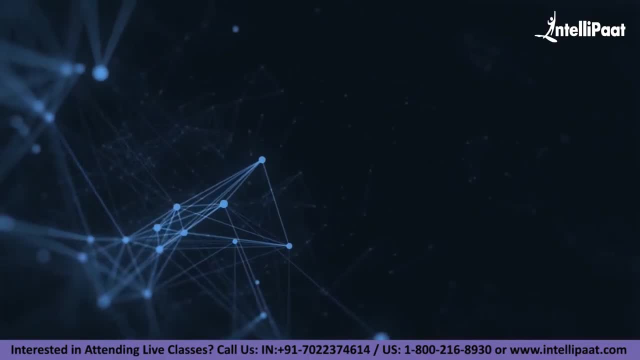 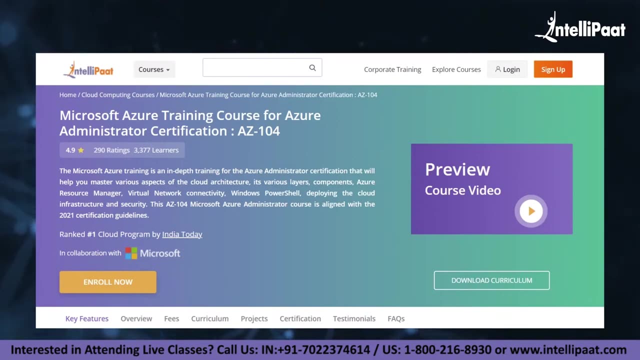 geographically located regions, for example. just a quick info, guys: Intellipaat provides Microsoft Azure certification training in partnership with Microsoft, mentored by industry experts, the course link of which is given in the description below. now let's continue with the session. Azure has regions like 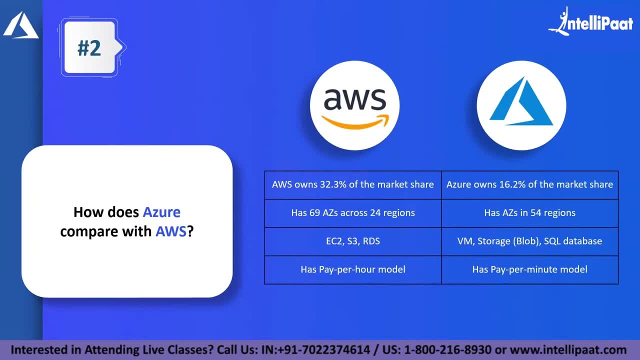 South India, North India, East US, West US, Central US Europe, Central Europe. so there are so many different regions like that. so, like that, there are 24 different regions, but within those regions, AWS has 69 availability zones, but as you has 54 regions, it has 54 regions, it has 54 availability zones and it's currently. 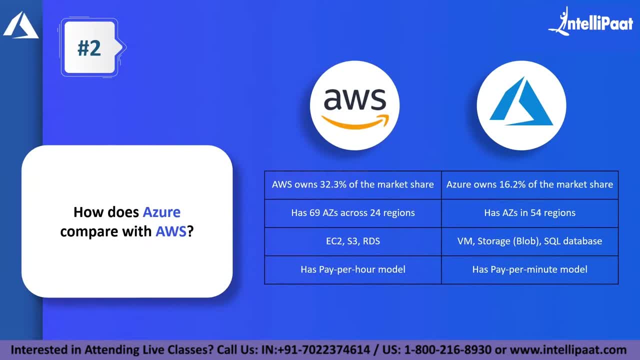 growing. so this basically shows us: your is better in availability zones, that is, data centers, because it has a wide range of data centers in various regions. next, comparing the services: if you already know about cloud, AWS, an Azure, then this would be easy. easy to s3 RDS. 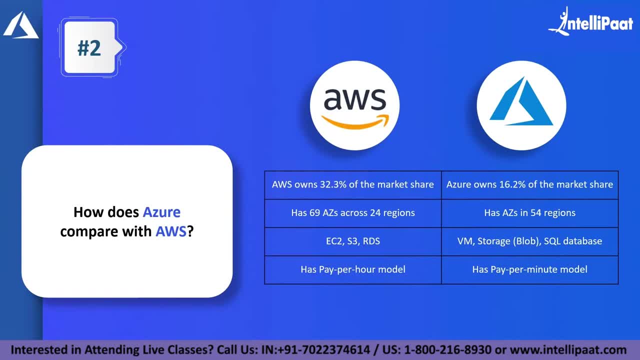 ah, are AWS services the same exact service. EC2 is equal to virtual machine, Azure virtual machines. S3 is equal to storage, blob storage, RDS is equal to SQL databases in Azure. so EC2 is used to launch and create servers named as VM does, and then S3 and blob storage are for storing objects. 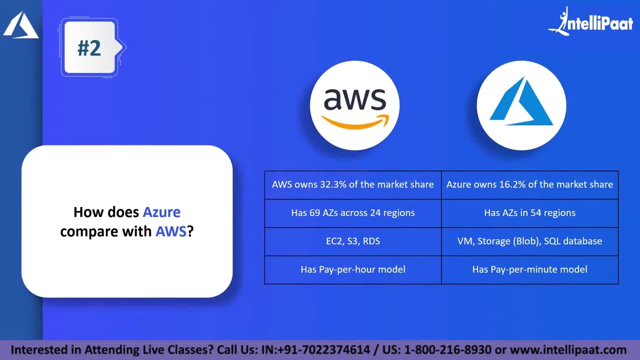 RDS and SQL databases can create relational databases running on the cloud so you can distinguish between different services. and then, finally, the pay per hour model and pay per minute model. so this is one of the important difference you'll have to note down, because AWS does not have 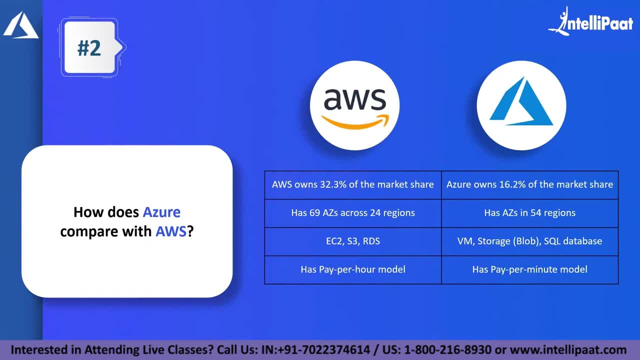 a pay per minute model, yet it charges you for the hour which you used, but Azure will charge you only for the minute. for example, if you're running a service- let's say you're running the same server- Linux server- in AWS and Azure- for five minutes in AWS will be charged the 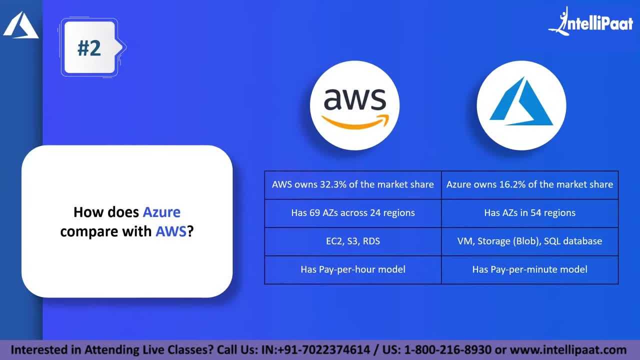 you hour. for example, if the hour charged in both AWS and Azure is five dollars, so it would be five dollars for for 60 minutes. if it's five dollars, so you will be charged for the whole five dollars in AWS, but in Azure that would be not the same because you will be charged per minute. so if it 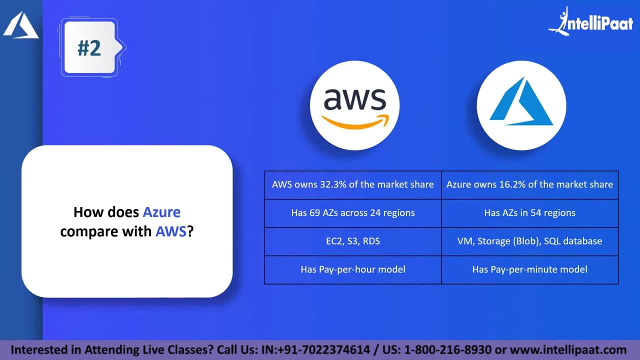 is five dollars for the hour. that is 60 minutes, so that will be reduced to one minute, so that would be multiplied into five. so you will be charged very, very, very less in Azure compared to AWS if you are using services for a very less period of time. 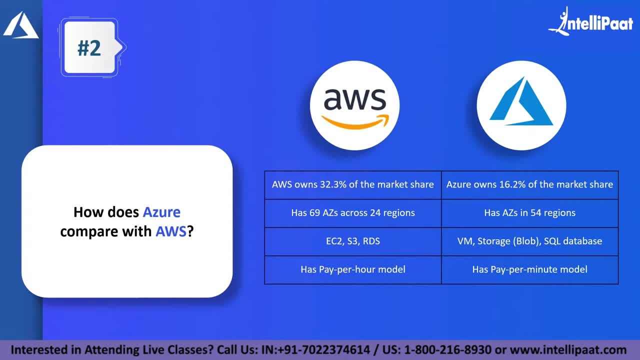 so if you're using some service for two to 10-15 minutes, then go with Azure, because that will not charge you as much as AWS. okay, so we've seen the second question, so i think you can coagulate it into an answer and give it. uh, i'm just explaining you the differences, but you'll have to provide it. 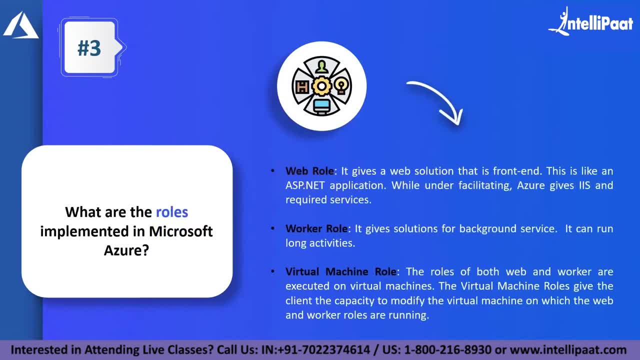 more of a answer, and then comes the roles implemented in Microsoft Azure. so you've got the role implemented in Microsoft Azure and then you have the time you need to provide an answer. so So there are three main roles: the web role, the worker role and the virtual machine role. 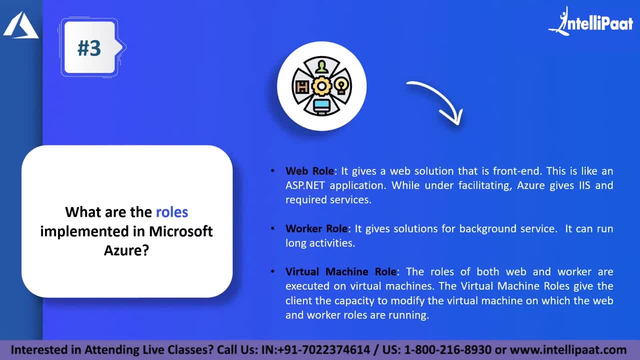 First, the web role. this gives a web solution, that is, the front-end. This is like an ASPNET application, while under-facilitating. Azure provides IIS, which is basically a web server and required services. So web role provides a web solution. 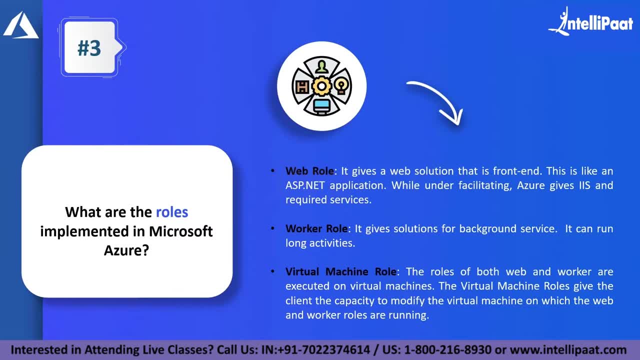 Basically it's a front-end. It can be a website's front-end. The worker role is a solution for background service. It can run long activities. For example, if you have a log activity, if you want to monitor the log activity, you can use a worker role. 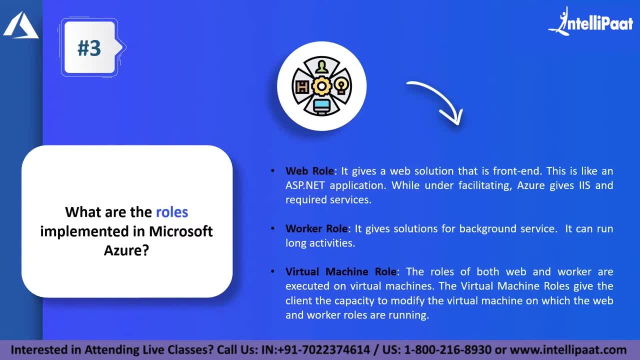 And then finally a virtual machine role. So this can act both as a web and a worker role, and this is executed by virtual machines. The virtual machine role gives the client the capacity to modify the virtual machine on which the web and worker roles are running. 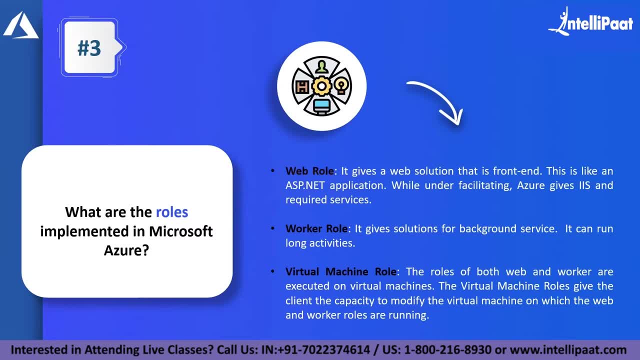 So, for example, web role only contradicts to the virtual, The front-end worker role only contradicts to the business logic, which is the background or the back-end part. So in virtual machines you can run both a web role and a worker role, which means you can have a website running as well as a background process running. 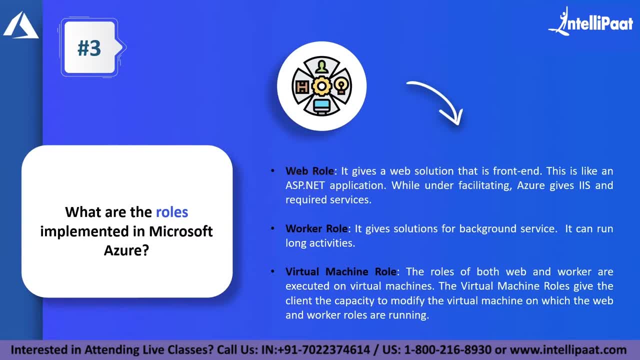 So these are the three main roles which are implemented in Microsoft Azure. So I think you get the point of this. So basically, in Azure mostly it is used to launch applications. So for an application, obviously there will be a web role which would be the application. 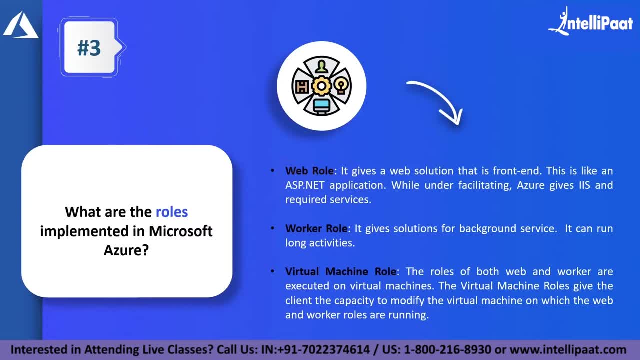 It's self-hosted. And then the worker role, which is background processes. For example, if a person wants to retrieve an image from the website, so they'll enter the information. click a button and a background code will run, So that code would be your worker role. 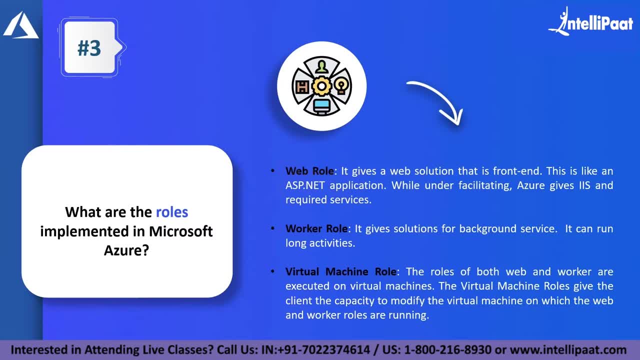 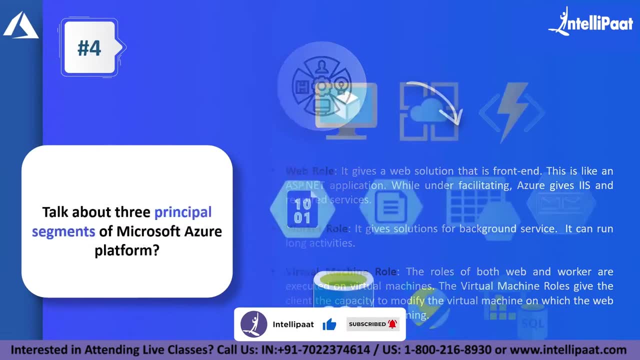 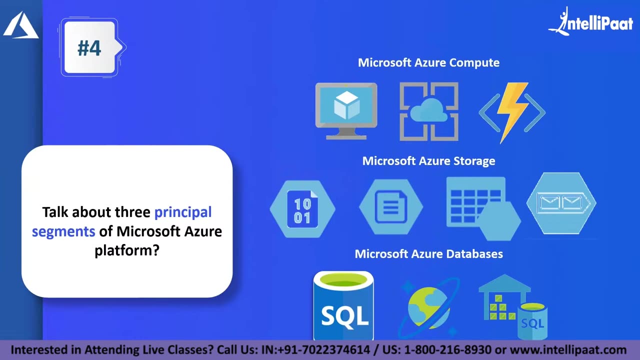 And these both can be run on a virtual machine, which makes it a virtual machine role. So these are the three most basic roles, And the next question is: So this might be a question which may be asked, But this does not have a certain answer. 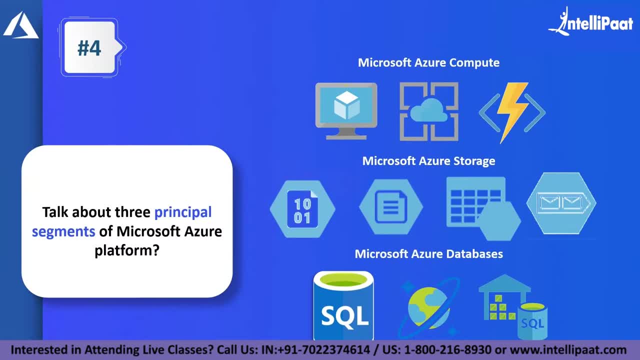 I'm just giving you the three most popular and commonly used services, So talk about the three principal segments of Microsoft Azure platform. Okay, So first of all, compute and storage comes by default because they are the most used Compute services and storage services are the most used services in any cloud platform. 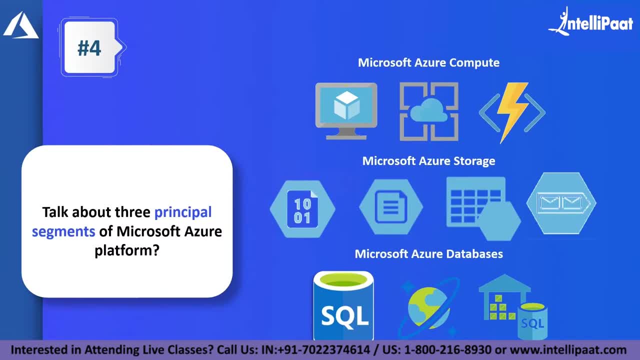 And then you can choose one as per your need. For example, you can choose database, Or you can choose monitoring, managing, governance. You can choose anything, So here I've chosen databases, For example. you can tell the answer like this: 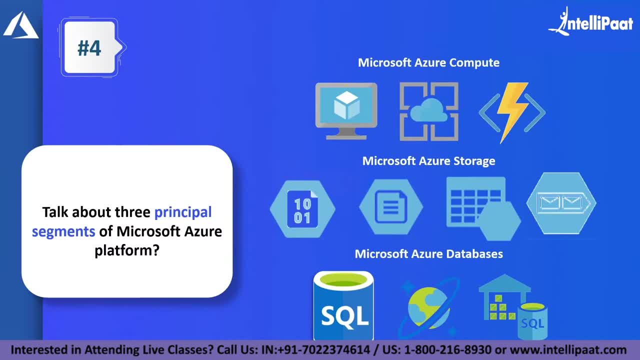 So the principal segments of Microsoft Azure platform. it can be basically anything, But here the most commonly used services comes under the compute and storage platform And I also would say databases, because every single application needs a compute, needs storage and also database. 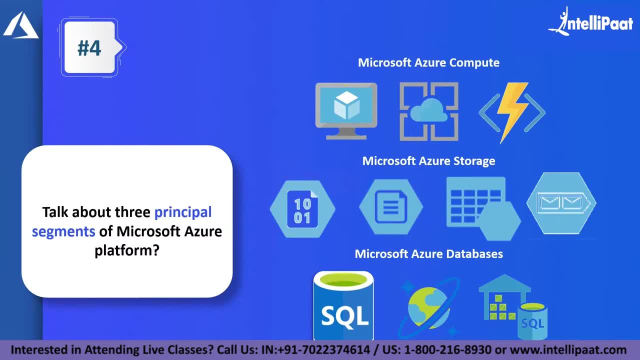 So, for example, In compute There is virtual machines, apps, services and function apps Which can be used to develop an application and also host that application with the back-end code. And then there is Microsoft Azure storage, Where we have block storage, table storage. 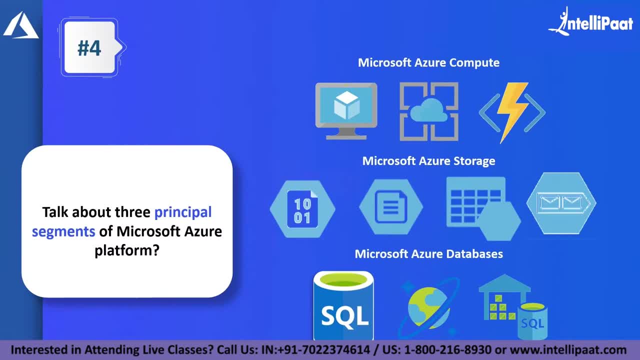 Where we have file storage. We have Azure queues, So we can use all of them to store objects. We can use them to store images, videos, audio files, We can use them to store NoSQL data And finally comes databases. 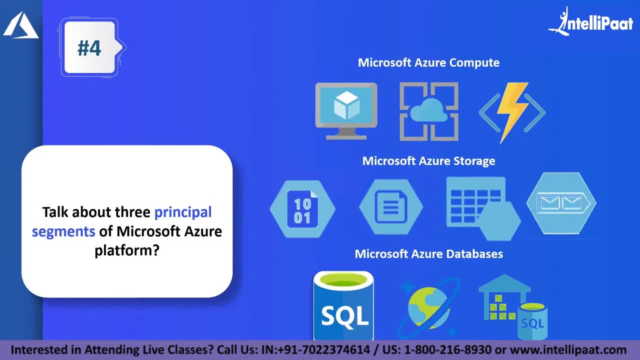 Where we can store, record or structure information. and also there is a Cosmos DB, which is for no sequel. and also, if your application needs a analytical database, we have a SQL data warehouses for that purpose too. so compute storage and databases, I would say they are the most. they are the three principal segments of Microsoft. as your 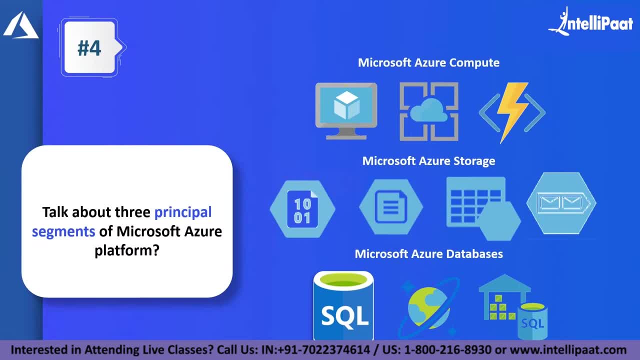 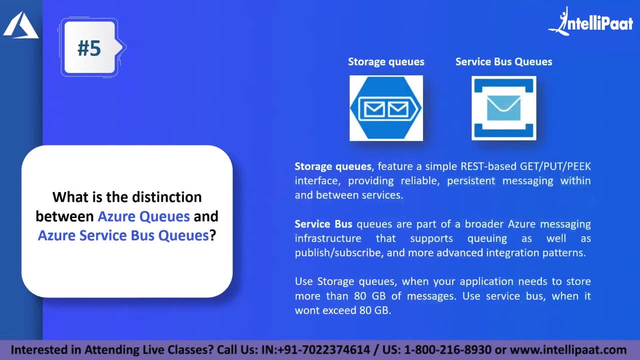 platform because they provide so many different services. pretty sure, even Azure uses them for their own benefit. okay, so this is the fourth question. so we have seen four questions up till now. so the fifth question is: what is the distinction between as your cues, as your service, bus queues? okay, first of all, 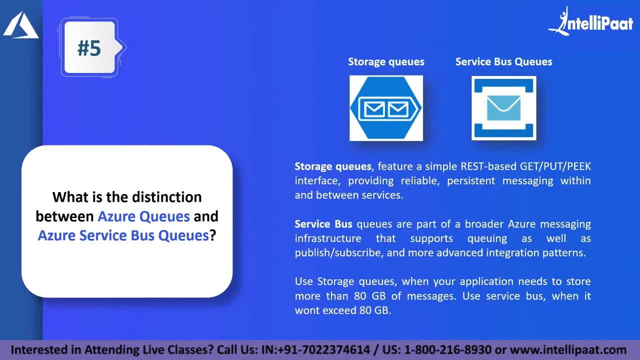 storage queues and service bus queues are different. so first, water storage queues: storage queues featuring a simple rest based I get put peak interface providing reliable, persistent messaging system within and between services. service bus use are part of a broader Azure messaging infrastructure that supports queuing, as well as published or subscribed and more advanced integration. 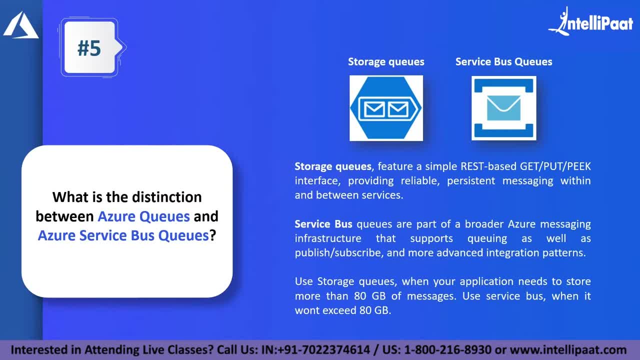 patterns. ok. so the simplest thing you'll have to know is if your application needs to store more than 80 GB of messages, go with storage queues, but if it needs only less than that and it won't exceed a thumbs up, you can go with a service bus queue. so the thing is storage use are mainly used to or move. 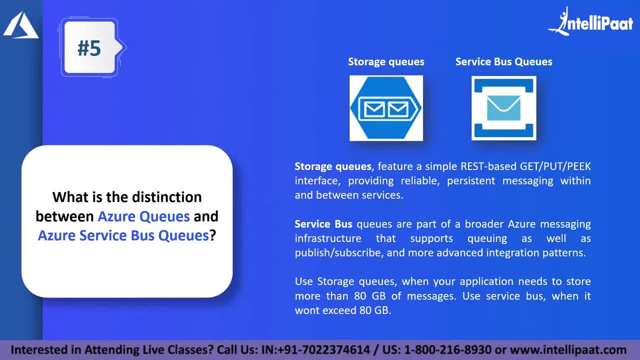 messages between services like broadcast and 언제 se juntar huge, сейчас tienen deathạt services or to an end user. so you can see it's a rest based get put peak interface. basically you can get a message from it, you can upload or send a message through it and in service bus you can do. 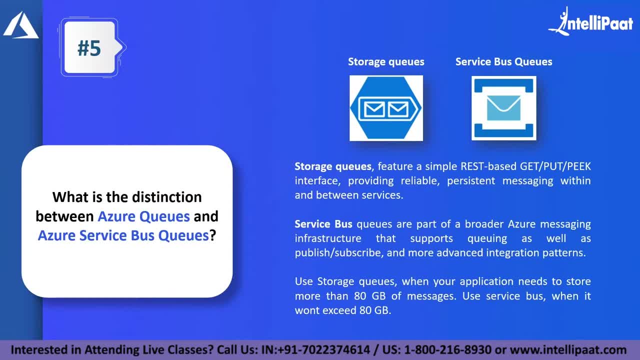 the same, but also you can integrate advanced patterns. for example, you can integrate a queuing system which basically filters multiple messages according to their priority, and that does not come with storage queues. also, storage queues are very easy to use. you can use it between services. you can create a queue within minutes. service bus is has a broader usage in azure itself, so these are: 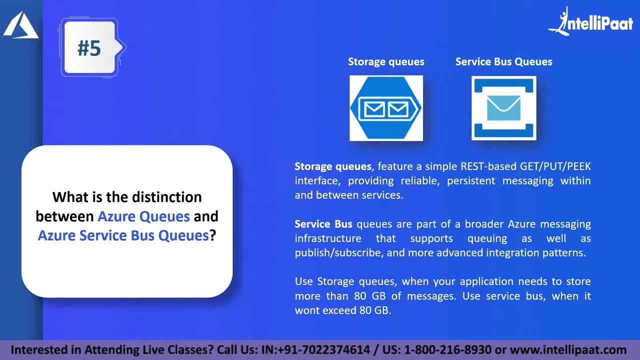 the main two differences that if you want to use an application for your own personal use, go with storage queues. if it is a bigger application which needs shorter message storing, go with service bus queues. so the just the main distinction between them is storage queues and storage queues. 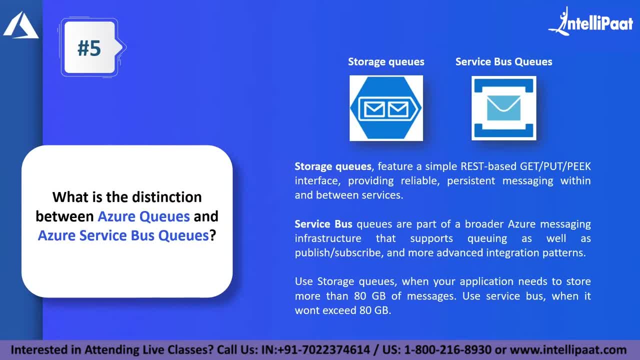 are simple, rest based get put peak interface. but service bus queues is involved with the azure messaging infrastructure itself and this supports queuing as well as normal publish and subscribe, which comes with storage queues as well. also, you can integrate advanced integration patterns, but which cannot be done in storage queues, where you can filter different. 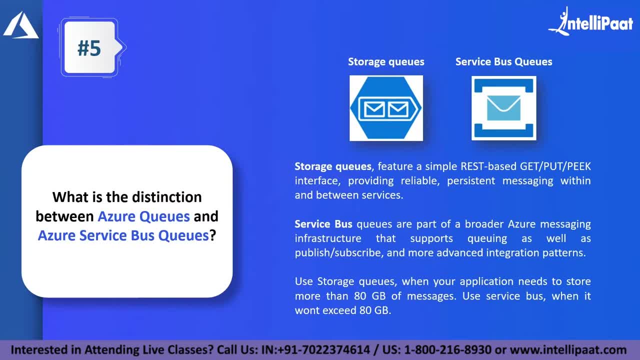 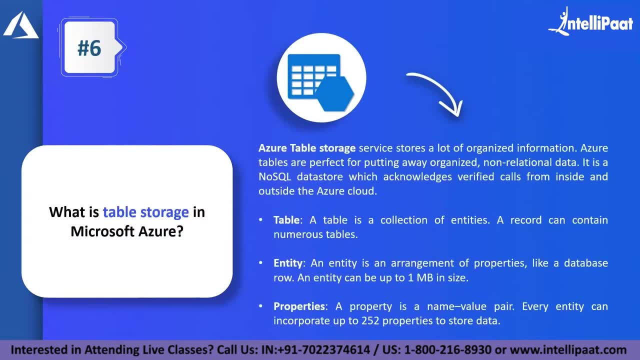 messages according to their priority and various other features and factors. okay, so the next question is: what is table storage in microsoft azure? so azure table storage service stores a lot of organized information. azure tables are perfect for putting away organized, non-relational data. it is a no sql data store which acknowledges verified calls from inside. 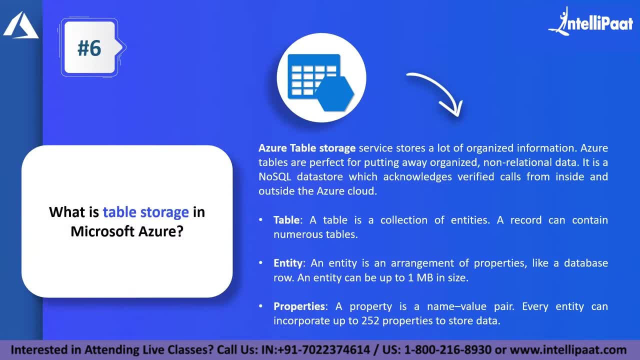 and outside the azure cloud. so basically, table storage is a no sql data store where you can store non-relational data. that's basically no sql, non-relational database. okay, so now, what exactly is table storage? first, let's look into what exactly it is. first of all, a table is a collection. 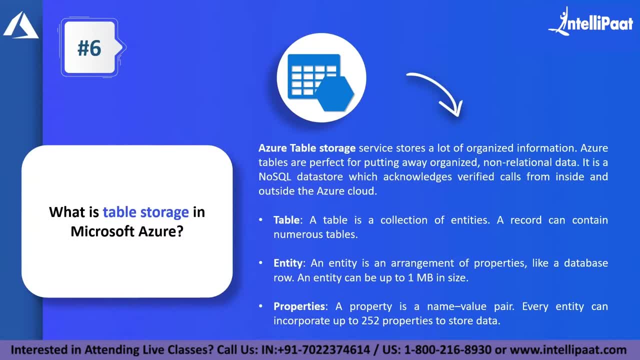 of entities. a record can contain numerous tables. basically, when you create a table, you can have multiple tables or a single table and it it is a collection of entities. so what are entities? entities is an arrangement of properties, like a database row. an entity can be up to one mba in size, so basically an entity is an item within the table. for example, if 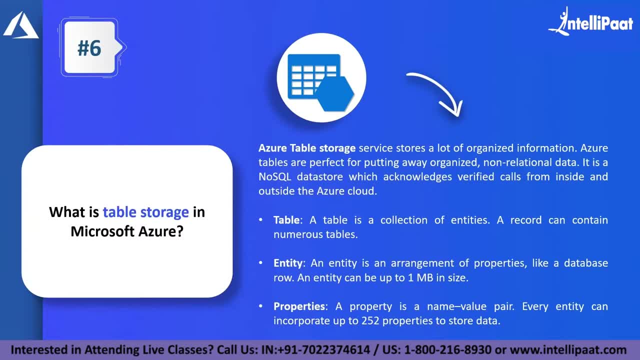 it is a table for shoes and inside that every single shoe name would be a entity. next comes properties. a property is a name value pair. every entity can incorporate up to 252 properties to store data. for example, let's say in entity we have three different shoe types. one is 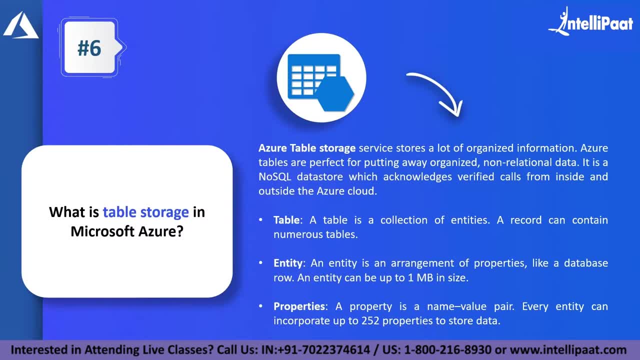 adidas, one is reebok, one is nike and inside adidas you can have 252 properties like color, type, shoe model, number and so many different properties under that entity, which defines that particular entity. so inside a table there can be any number of entities and inside those entities there 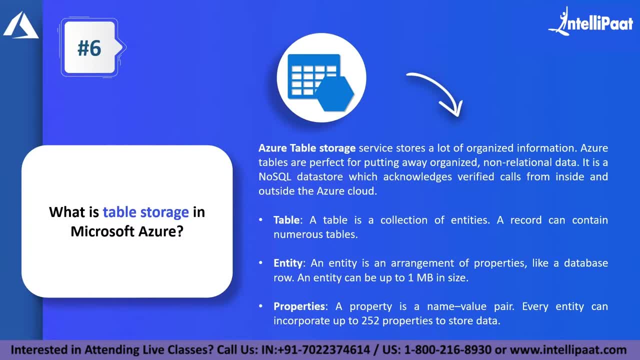 can be 252 different types of properties to store data. so that's what azure table storage is used for. it is a service used to store a lot of organized information in which you- uh- you- can store non-relational data. it's a no sql data store which acknowledges verified. 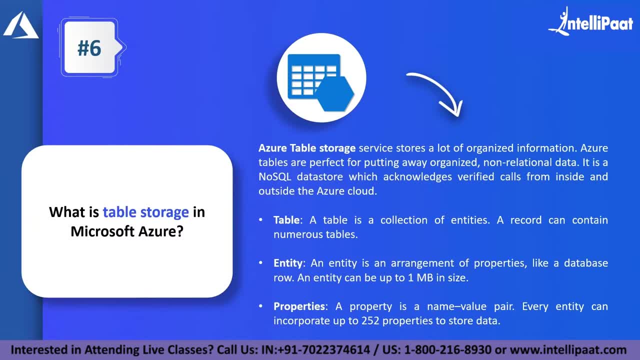 calls from inside and outside the azure cloud, that is, you can integrate it with azure services inside the cloud as well as third-party services from outside. the cloud and table is a collection of entities. entities is basically the main item inside a table and properties are the sub. basically, a property explains what an 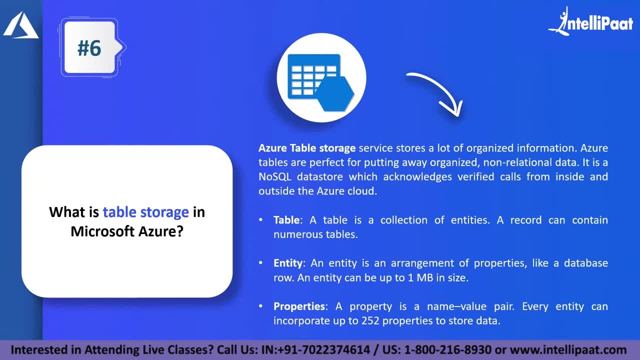 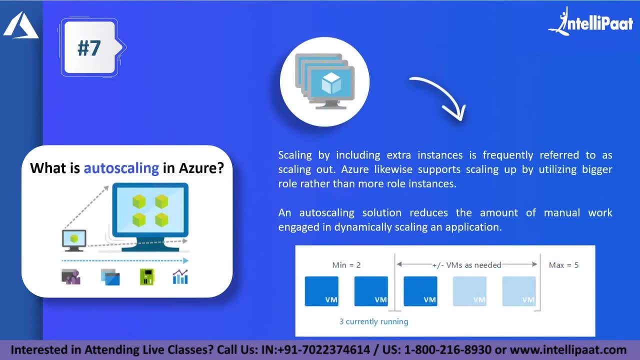 entity is, and the entity is completely, uh, explained what a table is. so that's it. that's what that is what table storage is. the next question is: what is auto scaling in azure? so what is auto scaling in azure? scaling by including extra intense instances is frequently 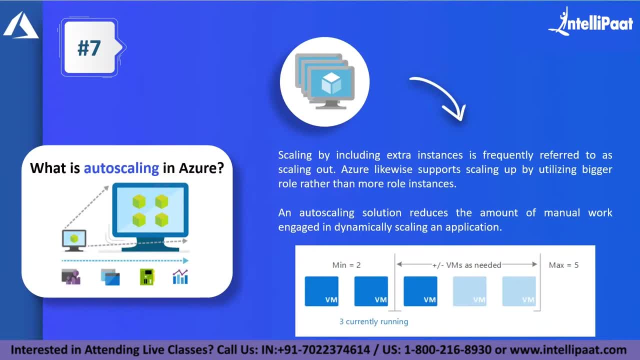 referred to as scaling out, so this is a commonly used term which is called scaling out. so azure likewise supports scaling up by utilizing bigger role rather than more role instances, and auto scaling solution reduces the amount of manual work engaged in dynamically scaling an application. so this is pretty simple, guys. so let's say you have a virtual machine which 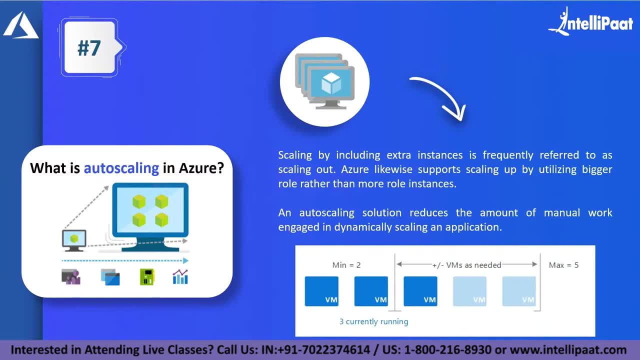 has a? uh, let's say it has a website running on it now there are a lot of users using it right now, but that one particular virtual machine is able to handle them. so let's say there are 20 users now. right now this particular virtual machine is able to handle all the 20 users and the website is not. 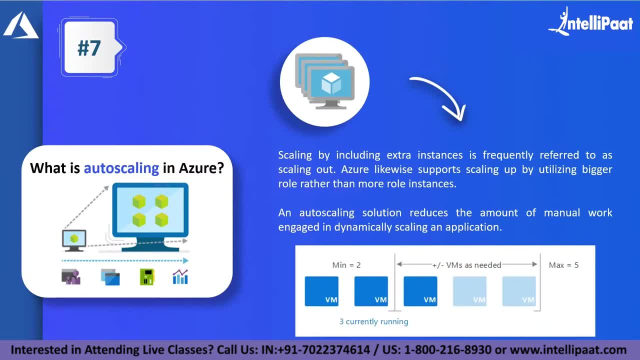 crashing, but suddenly your website has gone viral and there are 200 users now your virtual machine will not be able to handle because there are more users and the cpu utilization will go high. the traffic by hinder our traffic that we installed, shown in this video, to be걸 kwe flower anit. 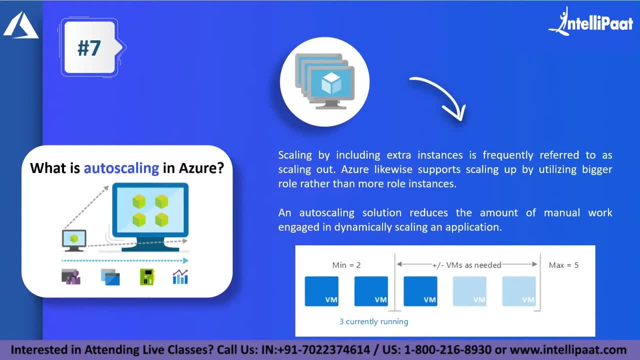 the overload of your server will go high. because of that, the usage also will increase and then your website might crash. so what you'll have to do? you'll have to again start up a virtual machine or another server. once you have done that, you will have to configure your website and make it run. 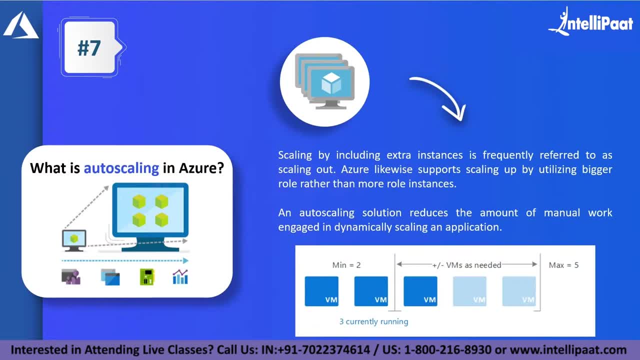 again. so this will take some time. until then you would have lost a lot of users. so instead you can start off with using auto scaling. so, for example, you can see the image in the right corner below in which the to the left there are two virtual missions, which is written as minimum two: that 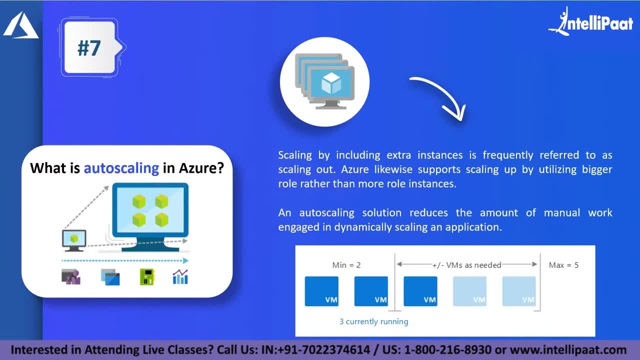 basically means, let's say, you have a website and right now your website has two virtual missions, and that is the minimum number of virtual missions and it will never go below that even a virtual mission is. let's say, even a virtual mission has been terminated accidentally. it'll launch one more. 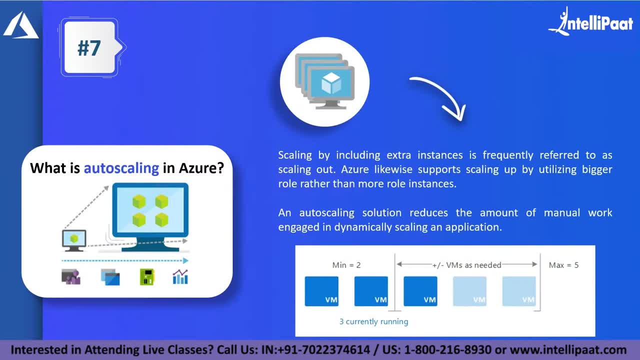 virtual mission within a span of a minute and that will be ready for your website. so now, to the right side you can see virtual machines needed and maximum is equal to five. so the maximum number of virtual missions you will get is five. the minimum number of virtual missions running will be two. 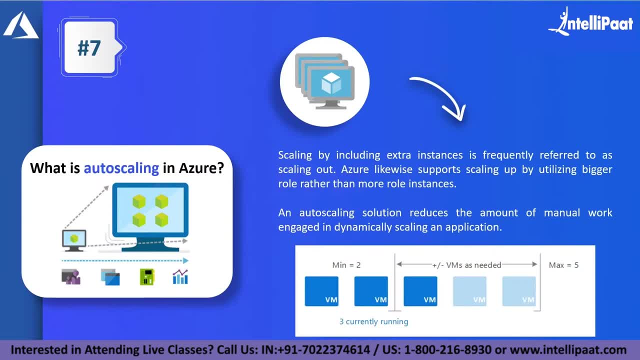 and there you can add or subtract three virtual missions. for example, if you have two virtual missions right now, you can add three more or two more or one more, or you don't need to add at all, but you cannot go below number two or you cannot go above number five. you can use auto scaling solution to do this, for example. 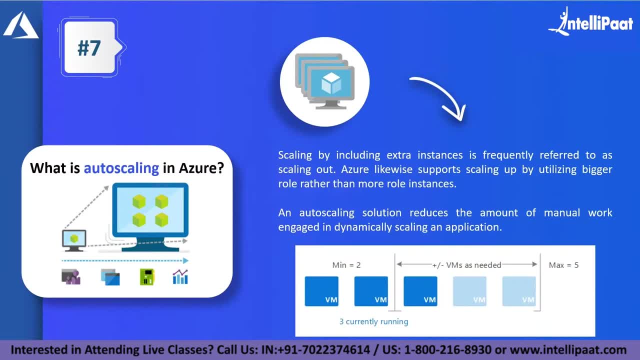 right now you have two virtual missions and the work overload goes very, very high. so right now you want one virtual machine. so it will launch one virtual mission now. it will monitor all of the three virtual missions. again. if the user count is completely increasing, it will launch one more and again if the users 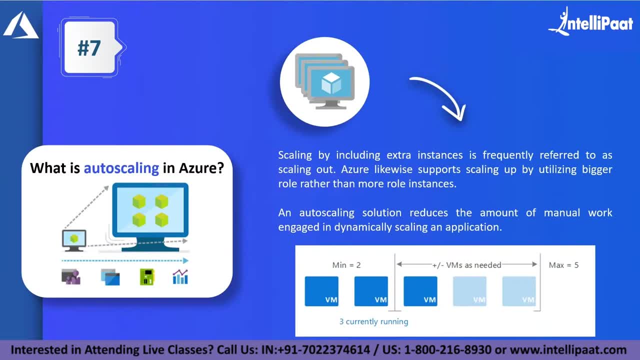 are increasing, the traffic is overloading. then again it will launch one more virtual mission. so here the maximum is number five. so it will launch up to five virtual missions after that. even though the user base is increasing, it won't go above that. you will have to change that in the 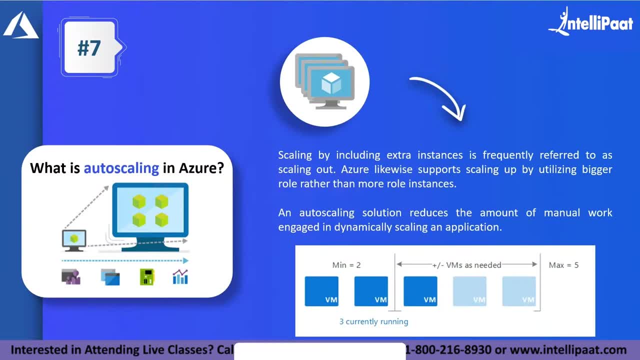 configuration. for example, max is equal to ten, so it can launch up to ten different virtual missions. okay, so got it. so I think you understood what exactly is auto scaling is. so you can explain it simply. for example, you can tell: auto scaling solution reduces the manual work engaged in dynamically. 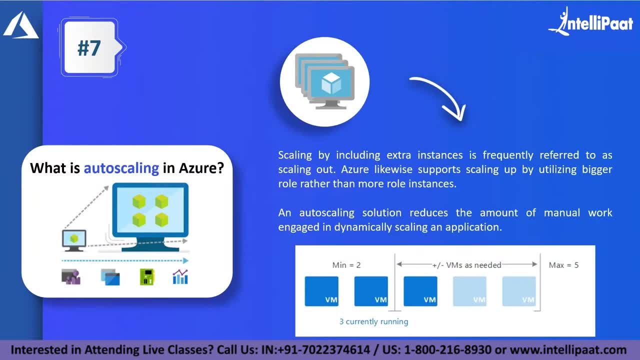 scaling an application. instead, we can set up an auto scaling solution in Azure, where it gives you the number of required instances, as such as whenever the traffic increases, it will give you more instances. when the traffic decreases, it will reduce the number of resources being used, which is also cost. 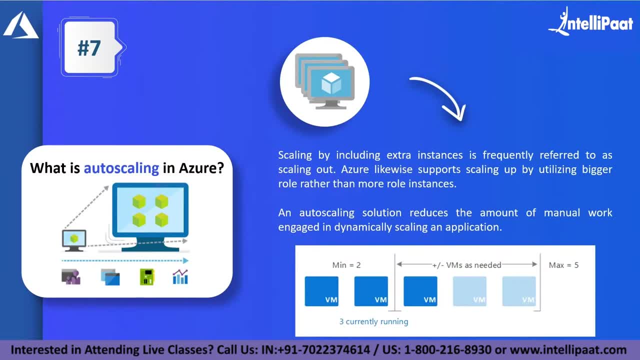 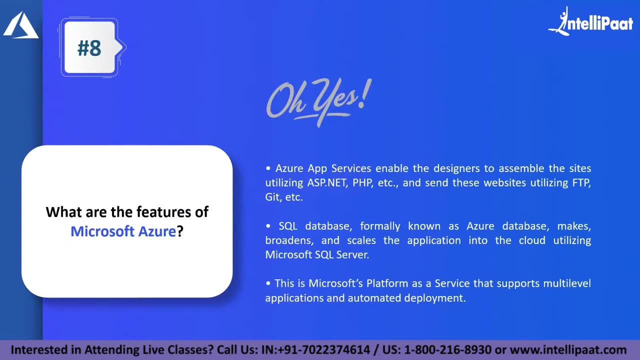 optimized and this will reduce your billing cost. so now let's look into the next question, which would be: what are the features of Microsoft Azure? so, what are the features of Microsoft Azure? so there are so many different features, so let's just look into three features. so first, as your app services enables, 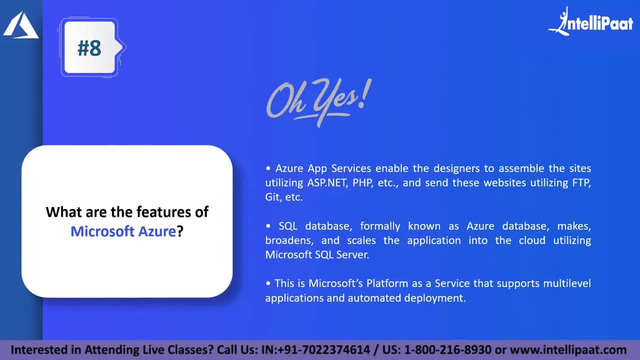 designers to assemble the sites utilizing various different programming languages. you can use ASP, NET, PHP, you can use Java, Python and send these websites utilizing FTP or git. basically, you can use github to have this code and you can integrate it with as your app services so that 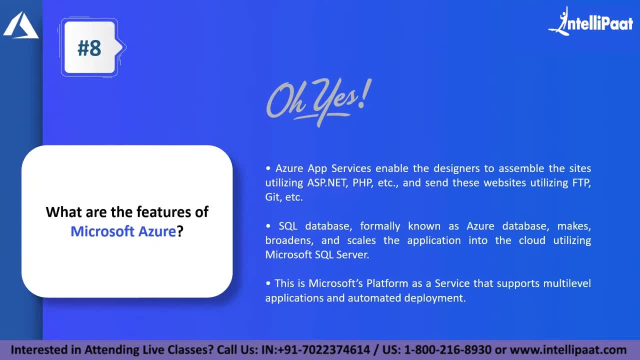 Azure itself will launch your website for you. it will maintain your website for you. you just have to work on your code. next comes SQL databases, formerly known as Azure database, makes, broadens and scales the application into the cloud utilizing microsoft sql server. so in sql databases provided by azure, 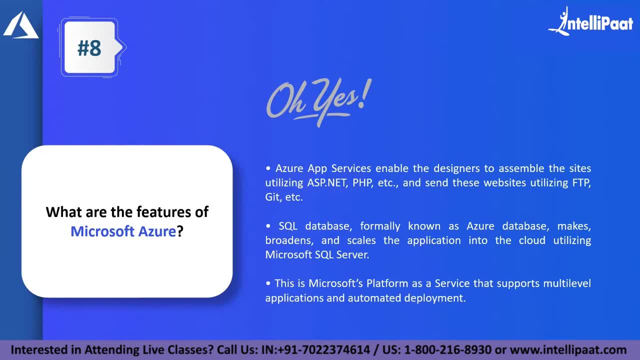 you don't need to scale out anything. for example, if you have set up a maximum size, whenever the size of the database increases, it will automatically scale the storage and also you can manually scale the compute. and finally, this is microsoft's platform as a service that supports multi-level. 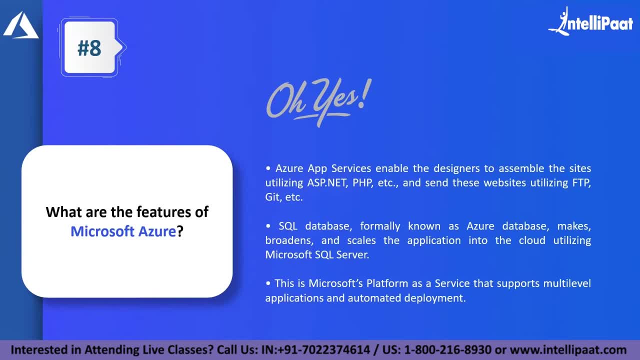 applications and automated deployment. that is, azure, is microsoft's platform as a service, because they are giving you a platform to work on various different services. even though services like virtual machines are infrastructure as a service, it comes under iaas, but microsoft azure as a whole is a platform as a service because they are giving you a platform which you can work on. 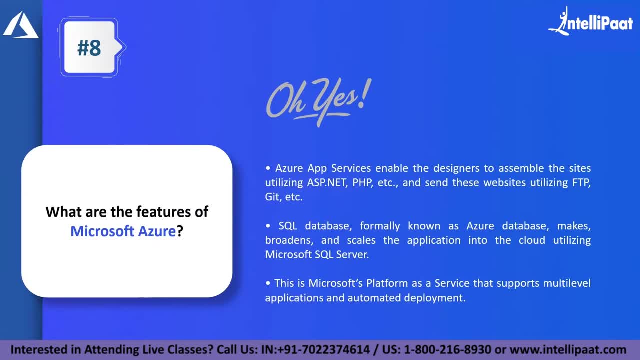 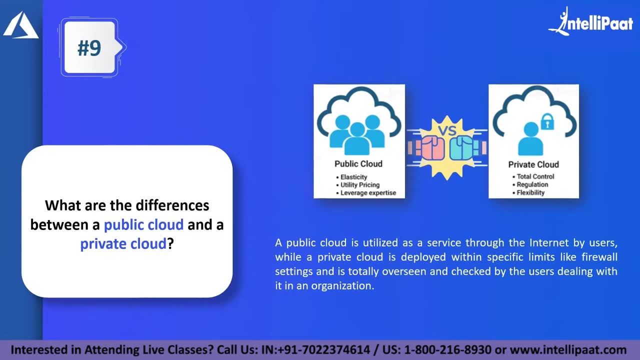 different cloud services. so these are some features about microsoft azure. you can talk about them. so next question is: what are the difference between a public cloud and a private cloud? this is one of the most basic questions. you can easily answer them. so look at the image at the. 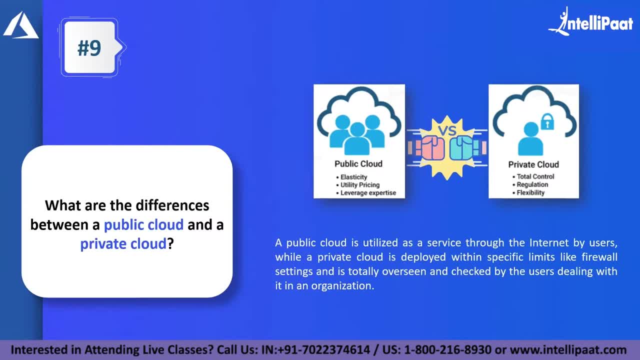 top. so, first of all, public cloud elasticity, utility, pricing, leverage, expertise, and then private cloud total control, regulation, flexibility. so let's compare this. first of all, elasticity, that is, you can launch any number of services, can go up, it can go down, you can have any number of users, you can provide the access to users. 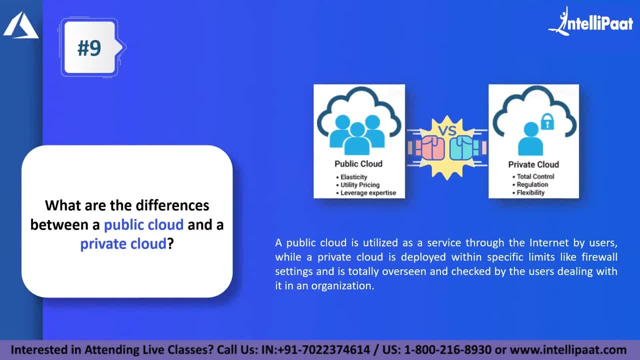 you can cut off the access whenever you want, so it's more elastic. and then, coming to write its total control, you can mention the administrator and only they will have control over the private cloud. so this basically increases security in private cloud, but public cloud is widely used. 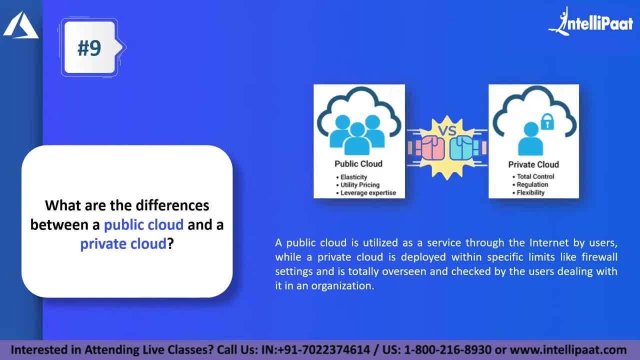 and also you can see leverage expertise. that means if you're using microsoft azure as a public cloud, then you will be able to leverage expertise because they have so many different security professionals working for microsoft and they will be guarding your virtual missions because you have taken a virtual mission from azure itself and coming to private cloud, you'll have to maintain. 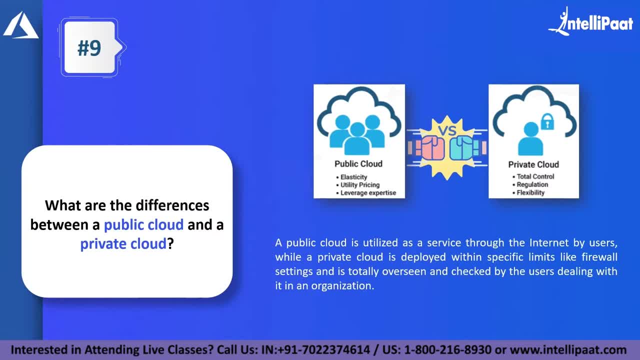 monitor all of that. and then comes utility pricing and regulation. so utility pricing in the sense you only pay for what you use in private cloud, you will pay for everything you have taken up. and also regulation in the sense you can stop someone to access something. you can stop a service overall. 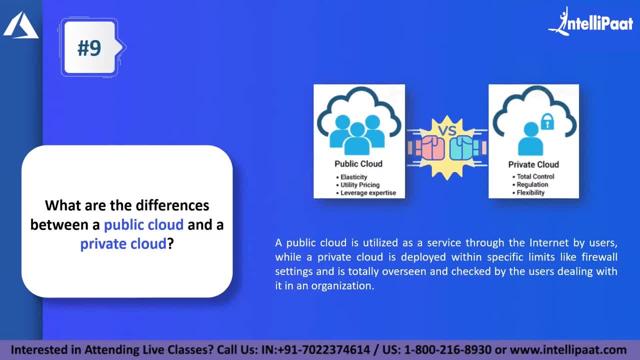 you don't need to use a service. you can stop a service. you can stop a service. you can stop a service. so in private cloud, you have the whole control. in public cloud, you have partial control. okay, so now let's look into the most basics of them. a public cloud is utilized as a service through the internet. 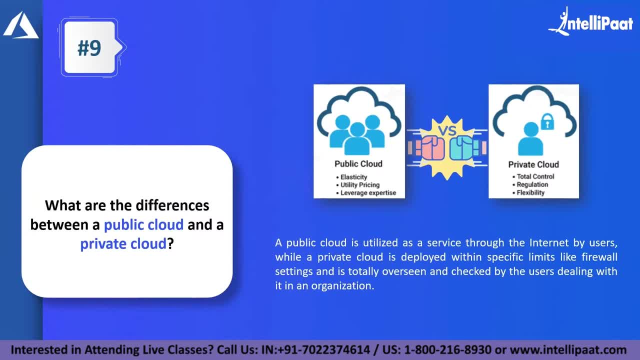 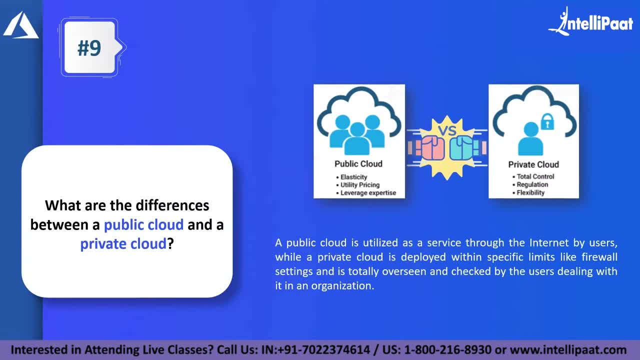 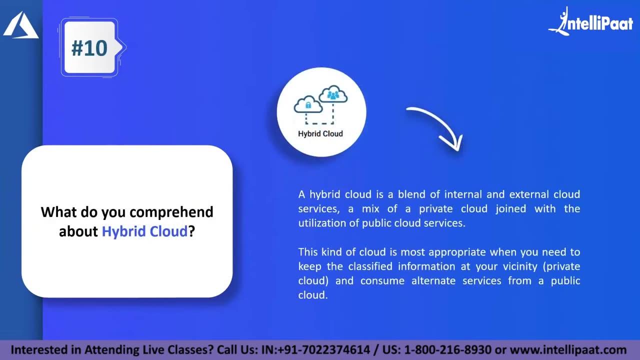 end user use. private cloud is used, mostly used for deploying applications within a specified limit. for example, within an organization, you can launch applications, so you can do that using private cloud. so this is the basic differences between public and private cloud. so the next question would be hybrid cloud: what you comprehend about hybrid cloud? so basically, a company can use both public. 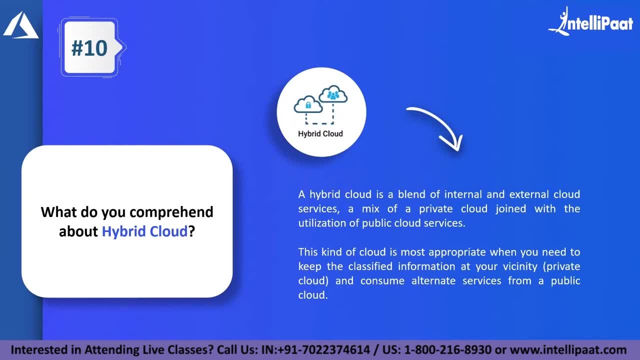 and private cloud, so a combination of them is a hybrid cloud. so hybrid cloud is a blend of internal, external cloud services, so internal in the sense within the organization, external in the sense for users, a mix of private cloud joined with the utilization of public cloud services. this kind 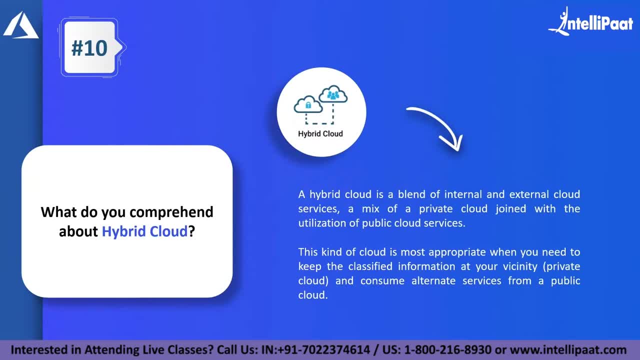 of cloud is most appropriate when you need to keep the classified information at your vicinity- private cloud- and consume alternate services from a public cloud. for example, if you have mission critical data, you can store that in the private cloud and the application itself can be running on the public cloud, because the application does not have any important information and even though 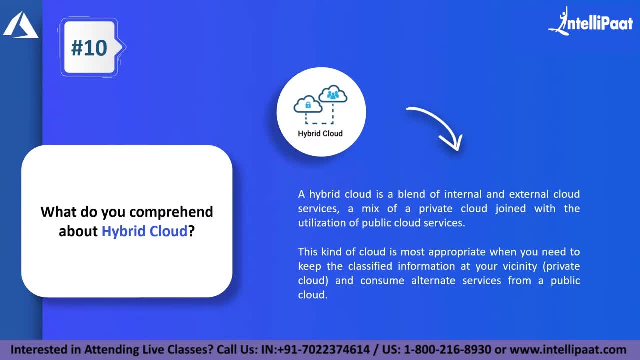 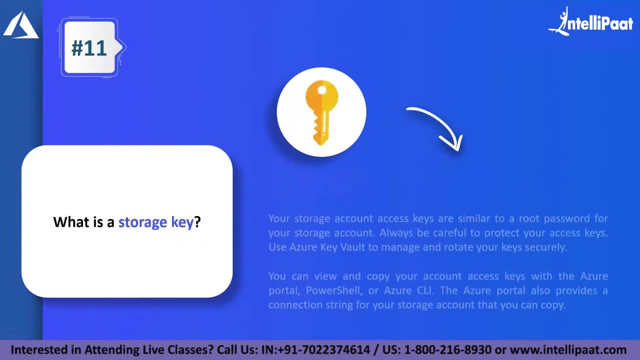 there is a security breach. there can be nothing taken from that, but your mission critical data and code is stored in a private cloud which only you can access. so this is hybrid cloud. and the next question is: what is a storage key? so your storage key- access keys- are similar to a root. 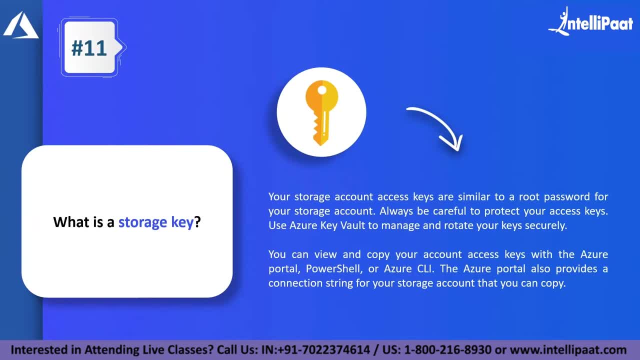 password for your storage account. always be careful to protect your access keys. use azure key vault to manage and rotate your keys securely. you can view and copy your account access keys with the azure portal, powershell or azure cli. the azure portal also provides a connection string for your storage. 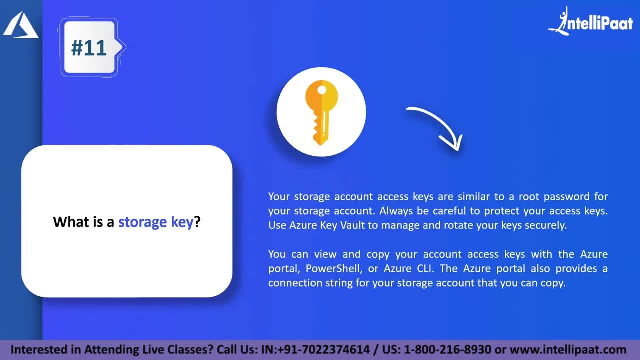 account that you can copy. for example, if you are logging into your storage account in azure portal, it's pretty simple to log in. you can just enter. you can just enter as such. but if you are trying to access your storage account from powershell or as your cli, you will have to use your storage. 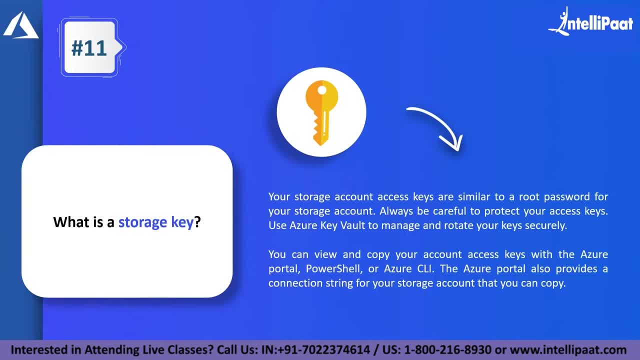 keys. so it's pretty. it's basically uh, an entry point for your storage account, so you can use that also. your portal provides a connection string for your storage account that you can copy and use it in your azure, cli or powershell. so to be simple, it is a uh. it is similar to a root password for your storage. 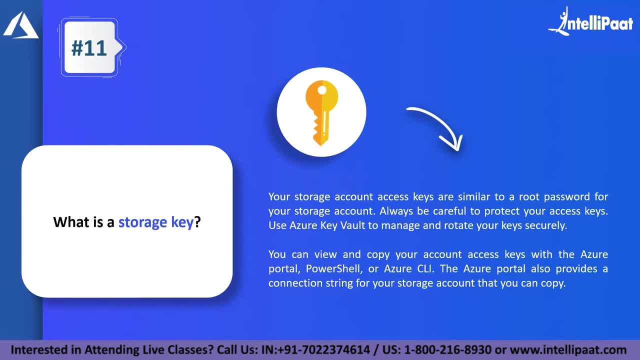 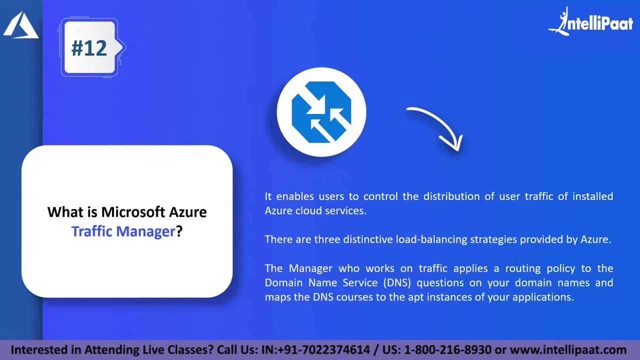 account and it is a key which you can use to log in into your storage account to check out the storage containers, like blob storage, table storage within the storage account itself. so it's pretty simple storage account. and then comes what is microsoft azure traffic manager. so it enables users to control the distribution of user traffic of installed azure cloud services. 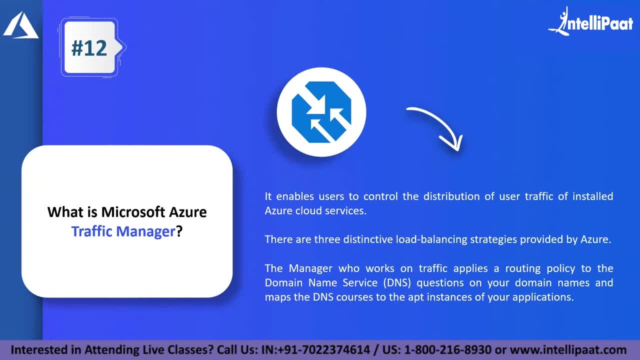 there are three distinctive load balancing strategies provided by azure. the manager who uses on traffic applies a routing policy to the domain name servers, questions on your domain names and maps the dns courses to the apt instances of your application. so let me explain to you in simple words. so, first of all, azure traffic manager is a dns based traffic. 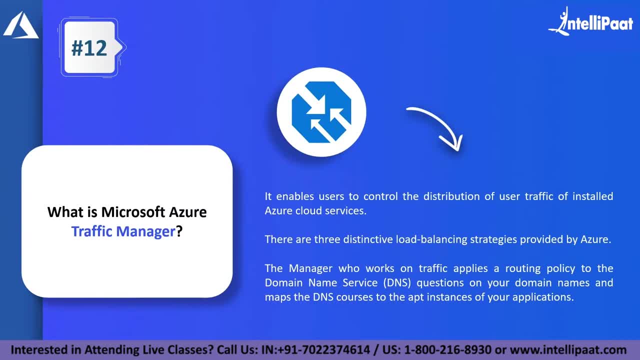 load balancer that enables you to distribute traffic optimally to services across global azure regions while providing high availability and responsiveness. so, basically, traffic manager uses a dns to direct client requests to the most appropriate endpoint on traffic routing method. so, basically, let me explain to you this. so let's say you are trying to access a website. 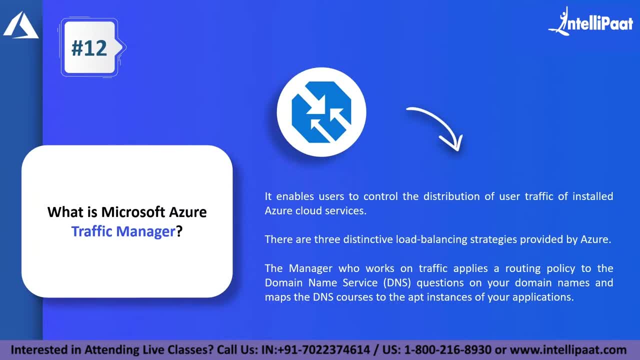 using a website's url name. now, when you type that your first point of entry would be the traffic manager. so once you hit that, the traffic manager will use dns and it will check to which ip address should this particular url name is should be redirected. so once when it finds that it will 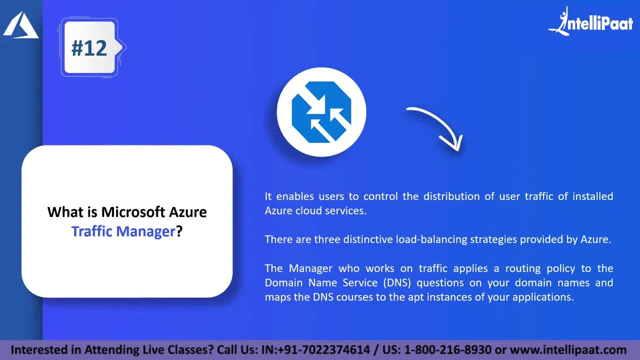 redirect the client request to the most appropriate service. for example, in intellipadcom we have intellipadcom, which is the main page, and intellipadcom site will transfer me to the blog. therefore, the traffic manager will be using that trade manager. 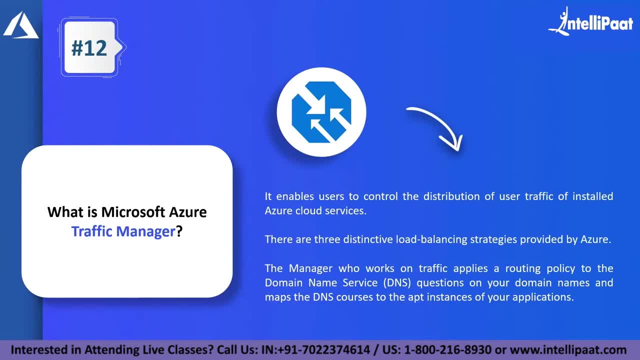 so let's say, i'm working on a project and i'm down here in friendsjohncom and this project is looking for a blog. so i'm just going to choose gentaries blog. so, for example, i'm searching for intellipadcom blog. now, this will go to the traffic manager. 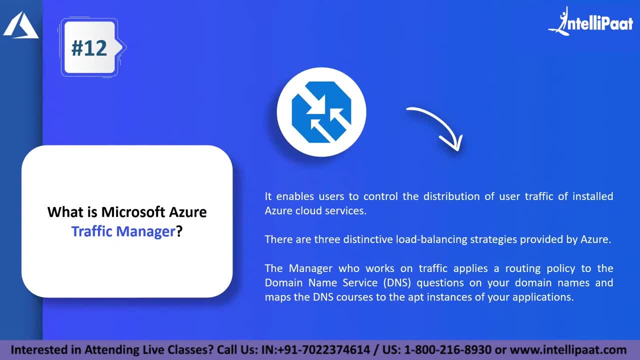 once it hits the traffic manager, it will check out the ip address for this particular url. once it gets the ip addresses, it will transfer me to the blog page, not the main intellipadcom page- auto scaling so that it is better to use. so if you're using traffic manager with auto scaling, 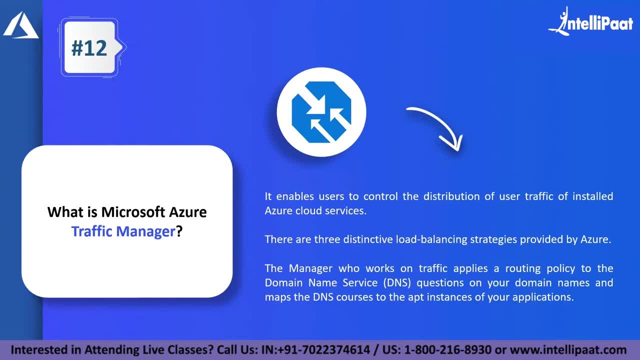 basically what you do. you will be able to launch and terminate multiple virtual machines, as well as you'll be able to launch multiple applications in different virtual machines and connect two auto scaling groups together, in which the traffic manager is the first entry point and, for example, in one auto scaling group there is app one. in another auto scaling group, there is app two. so 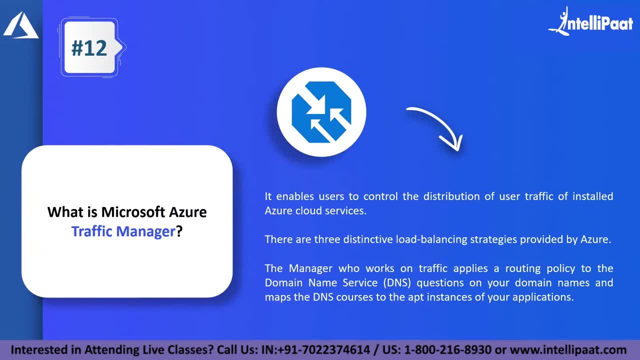 now it hits the traffic manager. if you're trying to access app two, it will take you to app two. if you're trying to access app one, it will take you to the app one auto scaling group. so this is how you can use traffic manager. the next question is: what is microsoft azure portal? this is again a. 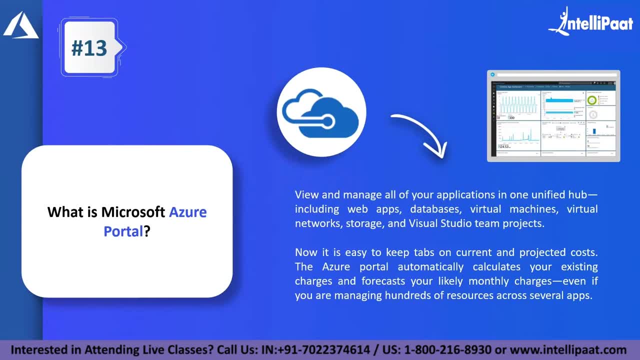 basic question. so microsoft azure portal is the website which you are logging into when you are using azure. so view and manage all of your applications. and sometimes you'll find that it is the� IO microsoft azure portal, so i'll just applications in one unified hub. you can view your web applications, your databases, your virtual. 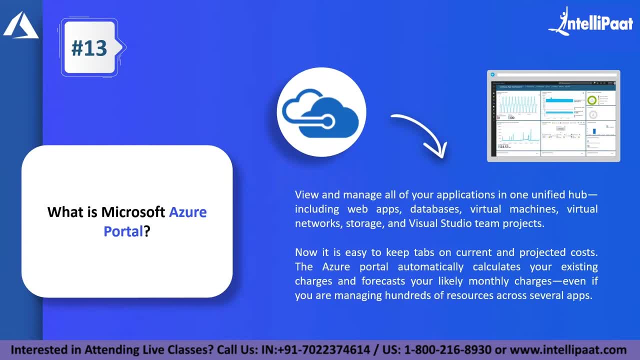 missions, your network storage and VST projects. Now it is easy to keep tabs on current and projected costs. so Microsoft Azure is not just for managing all your- all your applications and services. it can also be used to manage your current and projected billing costs. So Azure 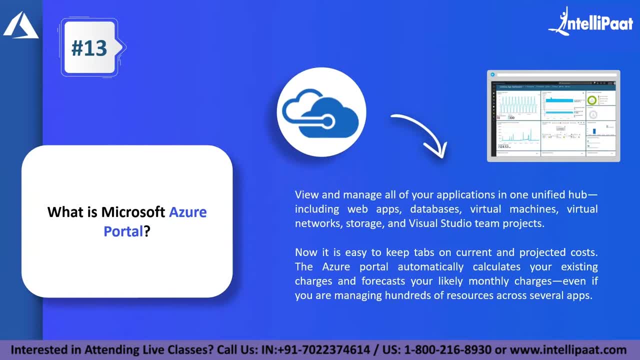 portal automatically calculates your existing charges, as well as it will forecast your future or monthly charge, even if you're managing hundreds of resources across several applications. For example, if you're using only one service, still it will give you the bill demand for right now and also the projected bill. If you are also using hundreds of services, again it will do the same. 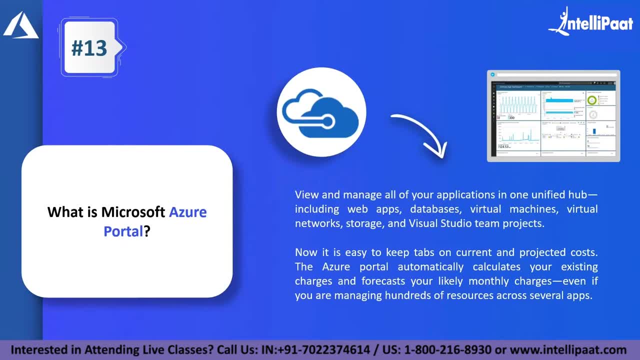 thing for you, regardless of the scale. So Microsoft Azure portal is the website which you're using to access Microsoft Azure services. that is more than enough. if you want to tell more, you can tell. it's a unified hub to manage all the Azure services. It also provides cost. 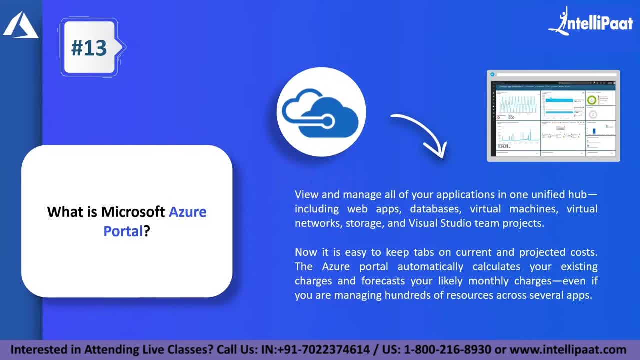 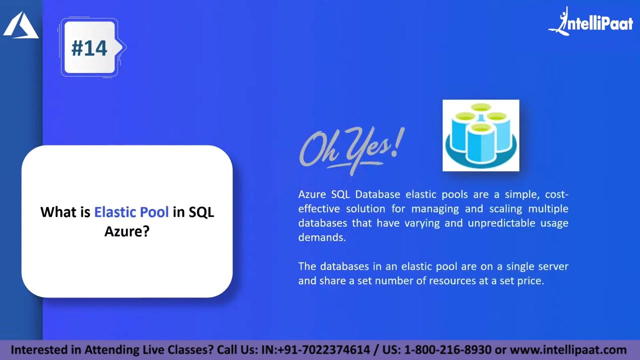 management services. You can say it has a different web page for every single service. You can access every single service directly from the portal itself and also manage, monitor and do everything else through Azure portal itself. and also you can access Azure portal from any internet connected device. Okay, so we've seen that. the next question is: what is elastic pool? 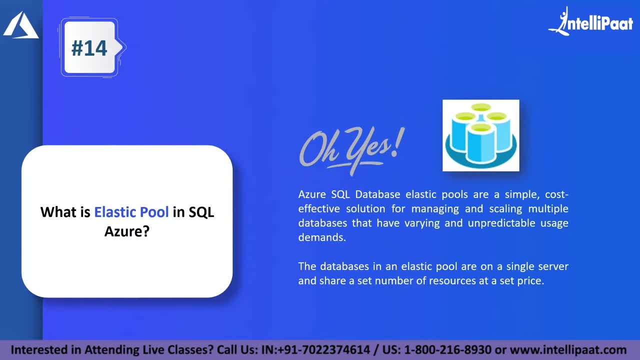 In SQL Azure. so we already saw what exactly is an SQL database. So now Azure SQL database. elastic pools are a simple, cost-effective solution for managing and scaling multiple databases that have varying and unpredictable usage demands. Databases in an elastic pool are on a single server and 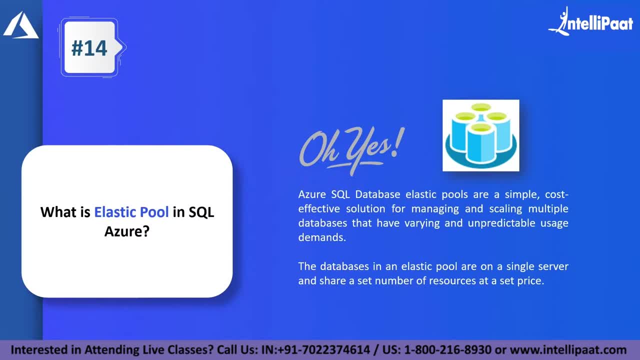 share a set of resources at a set price. Okay, let me make it simple for you. So right now, you hope you want various databases for different applications and all of them are going to be different. So all these databases need to have a different set of specifications. Now what you can. 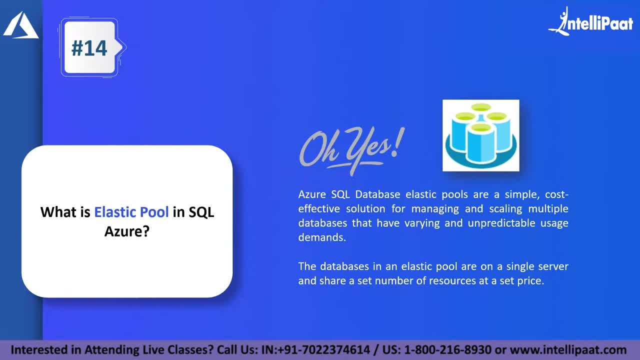 do is you can launch an elastic pool, which is basically a single server with different sets of resources within it. You can launch multiple databases and you can specify the required set of resources for a particular database. within the elastic pool itself, You can launch any number of 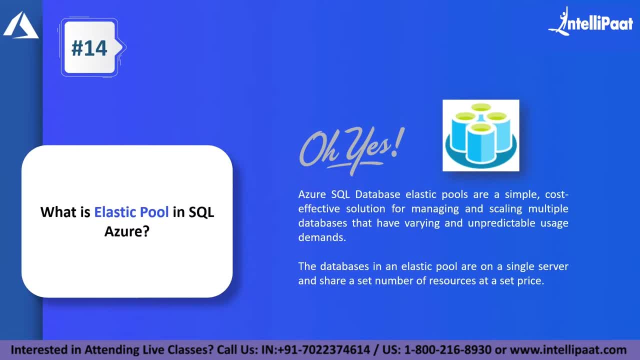 databases within that server and how much that server can handle. and all of the databases is shared, will use shared resources and the price for that will be the same, even though you're using any number of databases. So let's say you can have 10 databases within that elastic pool. 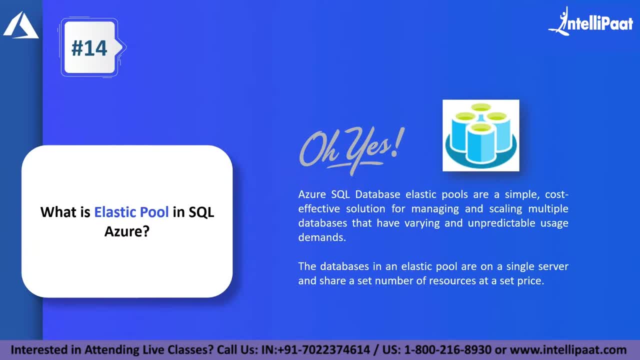 or you can have five databases, or you can have only one database, but you'll be charged the same because you are sharing the same number of resources across all the databases. So this is elastic pool. Next is: what is your SQL database? So an SQL database is just a single server with 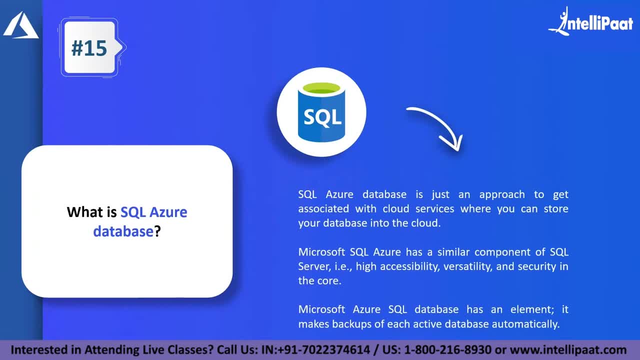 a single database. It's just an approach to get associated with cloud services, where you can store your database into the cloud. If you already know what SQL database is- for example, MySQL, PostgreSQL or MSSQL database- you will understand this easily, because it is basically the same. 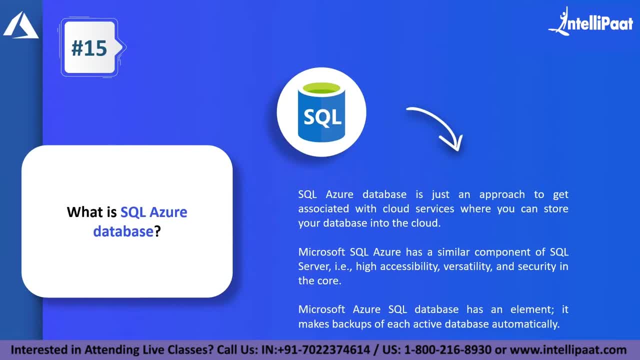 relational database on your local system, hosted on a cloud system and given remote access to you. So you can tell it pretty simply: SQL Azure database is a database server running in the Azure data center and to which you are given remote access to so that you can access that SQL. 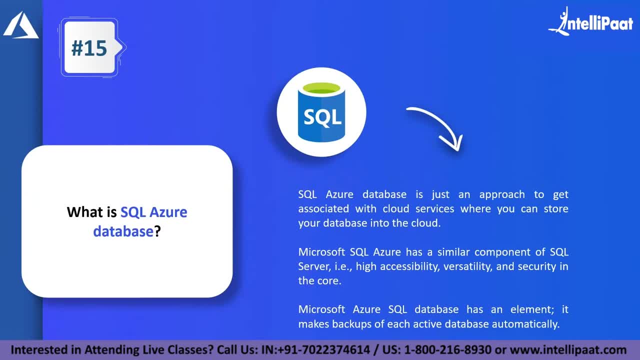 database. Microsoft SQL Azure has a similar component of SQL server, that is, it provides high accessibility, versatility and security. in the core, Microsoft Azure SQL database has an element: It makes backups of each active database automatically. So this feature does not come with a local database because it does not take backup. It has only one storage where the data is stored. 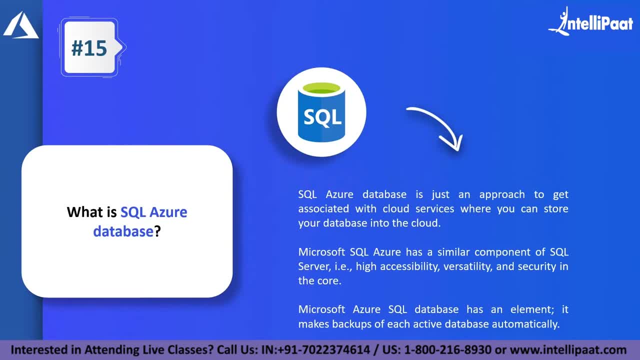 actually stored And if that is lost, your data is lost. But in Microsoft Azure SQL databases it's not the case. You can enable automatic database backups. So if your database is active and new data is coming in, it will automatically back it up. So even though your database has been, 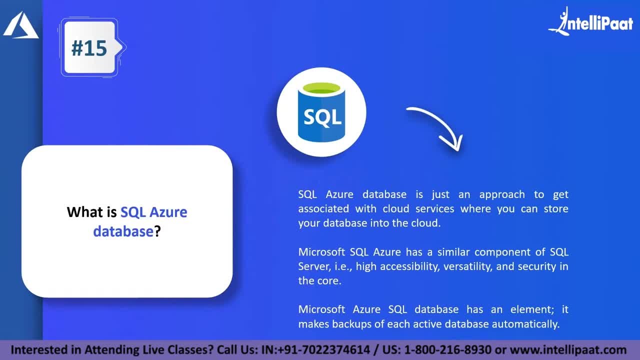 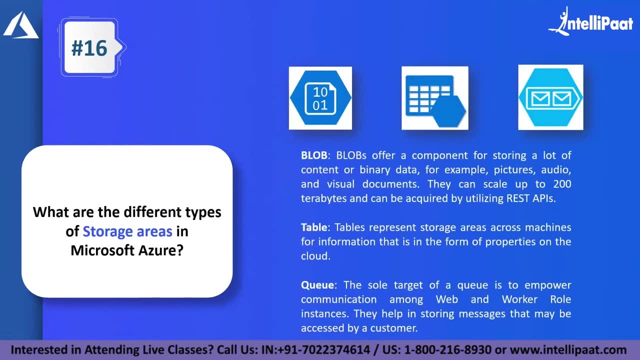 terminated, you can use the backup to launch a database with the same existing data set. So this is Azure SQL databases. Now let's look into the next question, which is: what are the different types of storage areas in Microsoft SQL? So let's look into the next question, which is: what are the 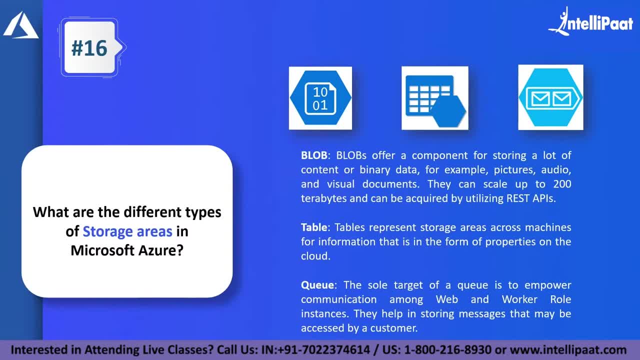 different types of storage areas in Microsoft SQL And there are still more, but you can talk about three of maximum. So within Make sure you so you can also talk about that if you want. but right now I will be looking at Blob table and 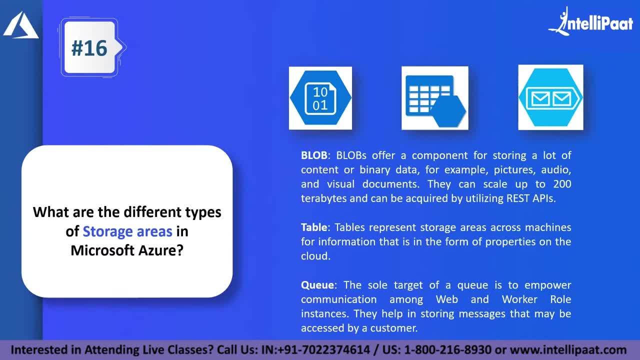 more because you can talk about Portable storage. so there is also file storage, which is basically a shared access file storage. So your data will be viene f passar, laid out into Android software as uh. so you can also talk about that if you want. But right now 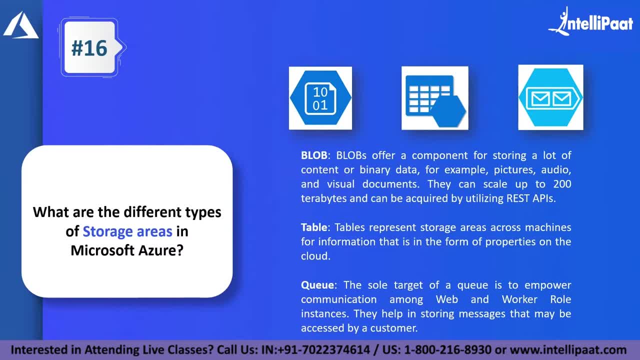 I will be looking into Blob, Table and�uece. so Qs we already looked into. you will look into Blobs and Table storage. even Table storage was a separate question, so you can also answer that. So, First of all, what is resource storage? As you can say, kind of into polling basic. 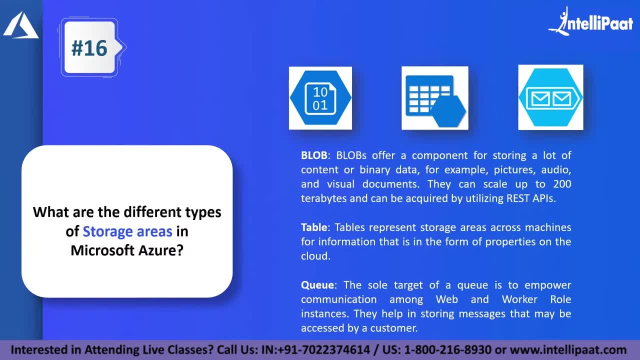 gesprochen. like route here is between records tables and folders, just with other words on blob. so blob is the most commonly used storage type in azure. so the full form of blob would be binary large objects. so you can see that bl? ob, which is basically binary large objects, blobs. 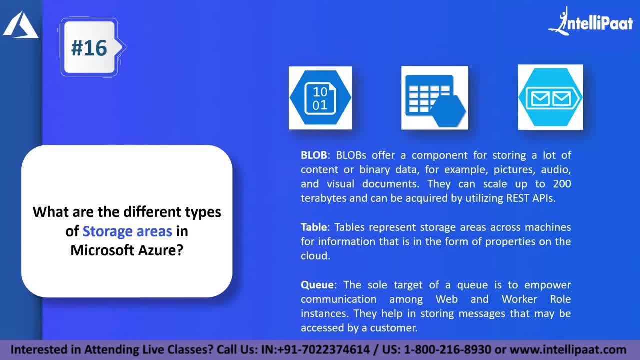 so blobs are a component for storing a lot of content or binary data. you can store pictures, audio visual documents. you can store video. you can store any type of data. they can scale up to 200 terabytes and can be acquired by utilizing risk apis. very, very simple to start off with blob. 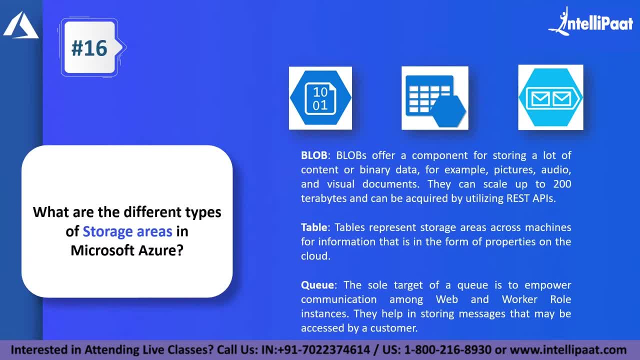 storage. we can create a storage account and create a blob container in which you can upload images, videos, documents, anything you want. you can store any type of binary data within blob storage. so that is one of the main area in microsoft azure. next comes table storage, which is a non-relational 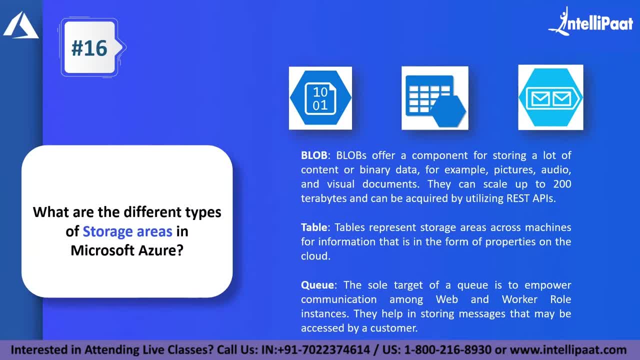 data store where you can store organized information and also you can store them using a format which is table entity, and with an entity you can have properties, so that we saw. next is queue. the sole target of a queue is to empower communication among the web and worker role. 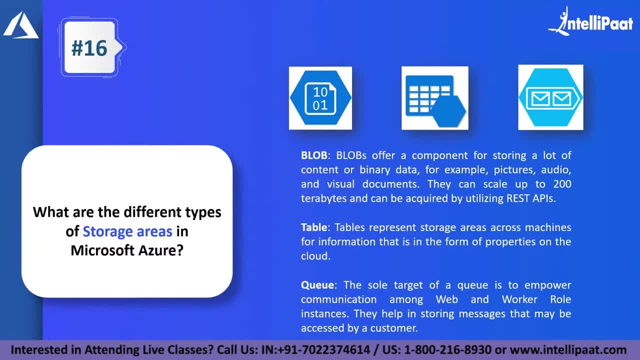 instances they help in storing messages that may be accessed by a customer. so, as told, queues can be used to connect multiple services as well as services with the end user. so these are three main storage areas. one more is a file storage, which is basically a shared storage access, which you can use to connect the same storage to multiple virtual. 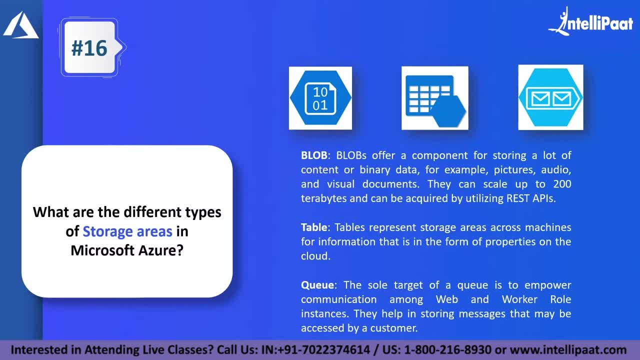 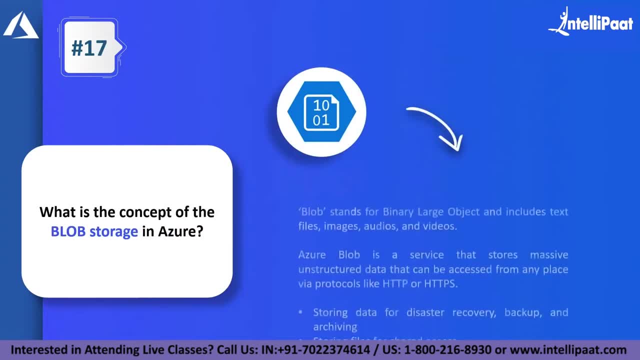 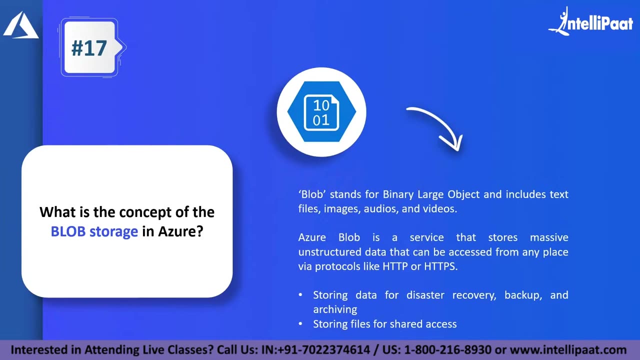 missions, so every single user in every single virtual machine will be able to access the same data store, which will save you a lot of storage as well as cost. next question is: what is the concept of blob storage? I explained to you what exactly is blob, so let me just go into that more. so blob? 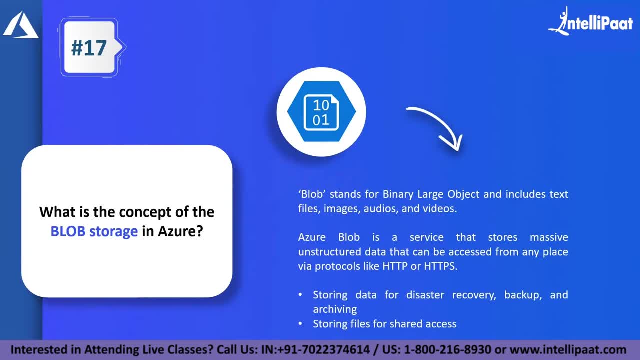 as told again, it is binary, large objects and includes text files, images, audios and videos, as your blob is a service that stores massive, unstructured data that can be accessed from any place via protocols like HTTP or HTTPS. so how does this work? how can you access these objects? 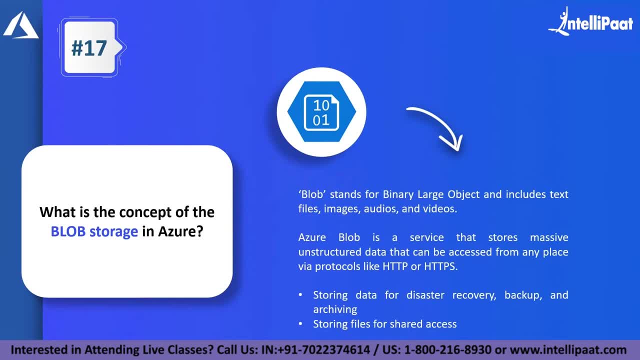 using HTTP or HTTPS, so it's pretty simple. whenever you upload an object like image or audio into the blob storage, it will have a URL, so it will be provided a URL, and it will be provided a URL and you can use that URL to access that particular object. for example, if I am uploading an image, 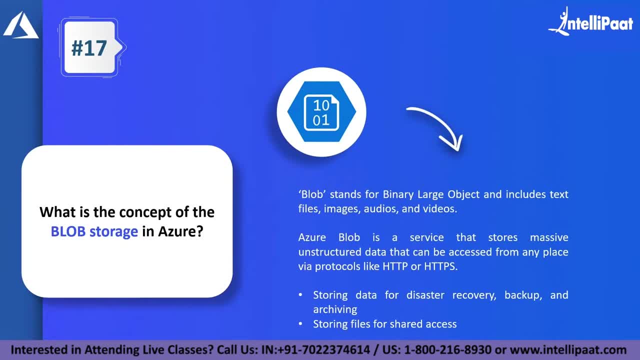 that image will have a URL for that image itself. now you can use that URL to access that particular image. so how will you access that using protocols like HTTP or HTTPS? so now, what else you can use as your blobs for storing data, for disaster recovery, backup and archiving. also storing files for shared. 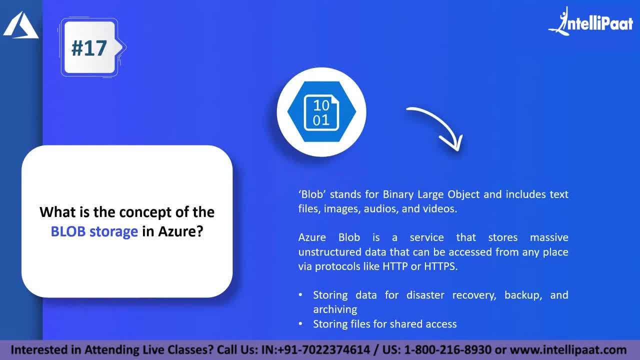 access. shared access is in the sense, if you are uploading an object and you have a link for it, you can share that link with multiple users so that they all can use that particular blob storage as a star shared storage. so that can happen also, you can use it for disaster recovery, that is, you can store data in different regions in blob storage. 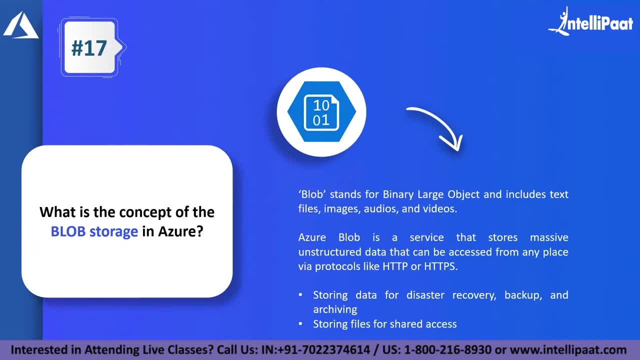 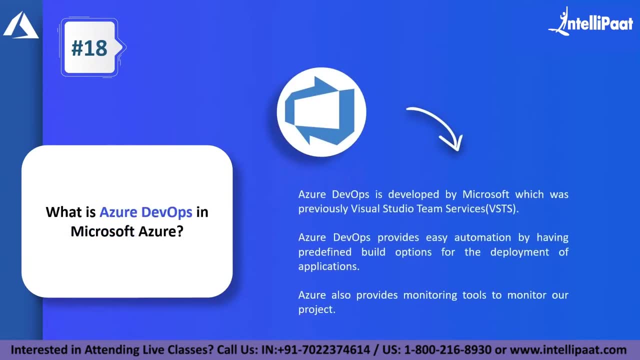 itself and use it for backup and then also archiving data. so this is blob storage. now let's look into the next question. so now this question is: what is your devops in Microsoft Azure? so if you are already familiar with devops methodologies, then this would be easier to understand. if you're not, I'll explain to you what exactly is devops in a. 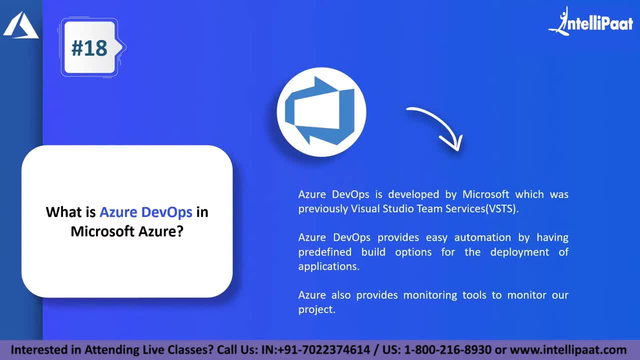 few sentences. so, first of all, devops is not a tool, it is a methodology which companies follow and implement in their software development life cycle to automate the entire life cycle. so Azure devops is not a methodology, it is a service. you may be confused by the name. but devops is the methodology, but Azure devops is a devops service. 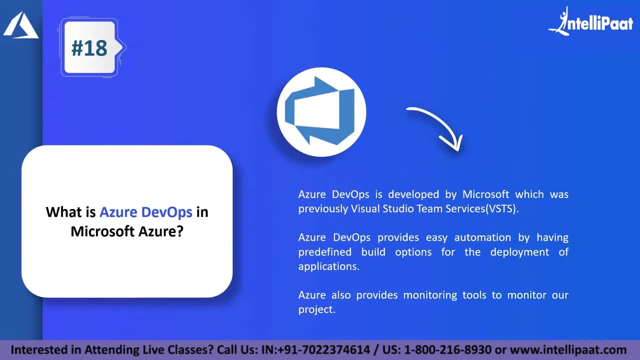 provided by Azure and it is developed by the Microsoft team. it was previously called as vsts or visual studio team services. Azure devops provides easy automation by having predefined build options for the deployment of applications. for example, if you are trying to launch an angular application, it already has build options for it. it has npm packages in build. you can have a build. 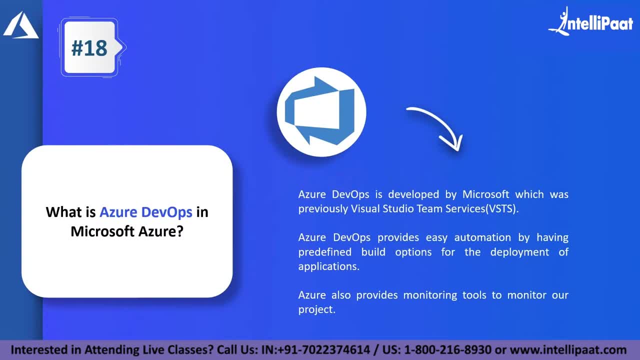 you can basically create a build in a matter of minutes. for example, if you are also launching a Java application, it has a maven build option. you can use that to build that application. so that's why they are saying it provides you easy automation and also free define predefined build options and 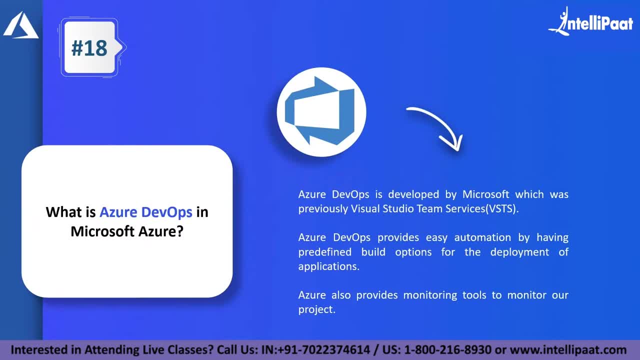 finally, it also monitors your tools and it uses monitor to monitoring tools to monitor your application or your project which you have launched within Microsoft Azure devops. okay, so Azure devops has various different tools, so let me explain to you those tools. so one tool is Azure repos, which is a repository like GitHub, so it's pretty similar. 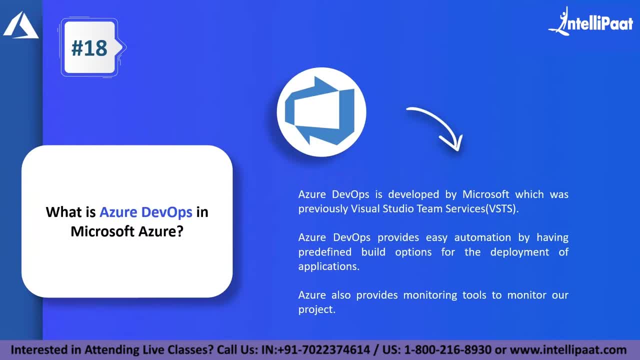 it's basically the same. and then comes Azure pipelines. pipelines is the tool which you use to implement a CI CD pipeline. a CI CD pipeline is the one which you use to automate the software life cycle. and then comes test plans, which is basically used to test these application. 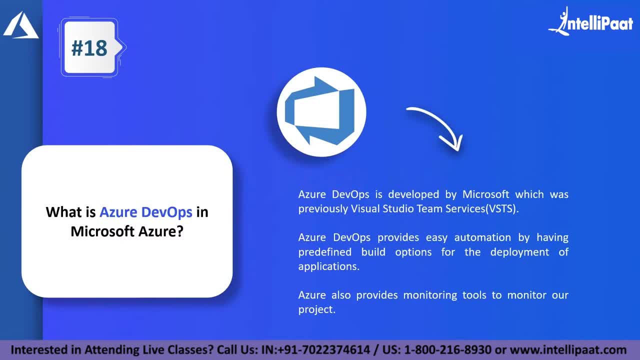 and then comes Azure boards, which is a Kanban board, which is basically like Jira, where you can implement work items, you can implement sprints, and then, finally, you have Azure artifacts, where you can store the packages, like npm, nougat, in the same place so that it is easier to access them. 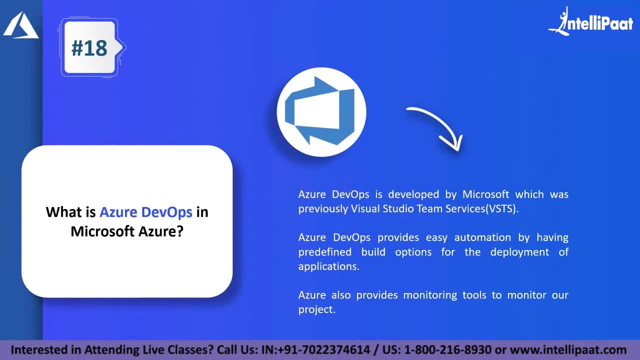 also, finally, you get an Azure dashboard where you can access and also create and launch widgets where which will be helpful for your application. for example, you can see how many builds have been succeeded, how many have failed, how much time it is taking to build a particular project, how many times it has been deployed and how many users are using. 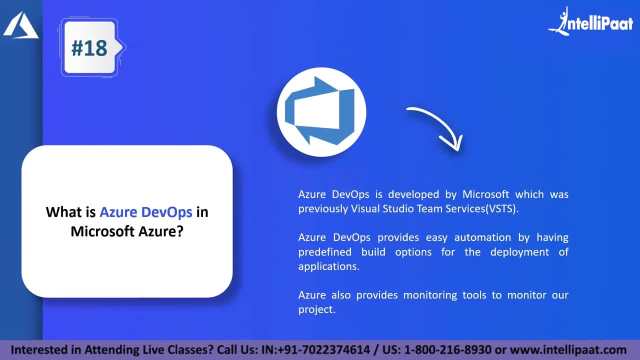 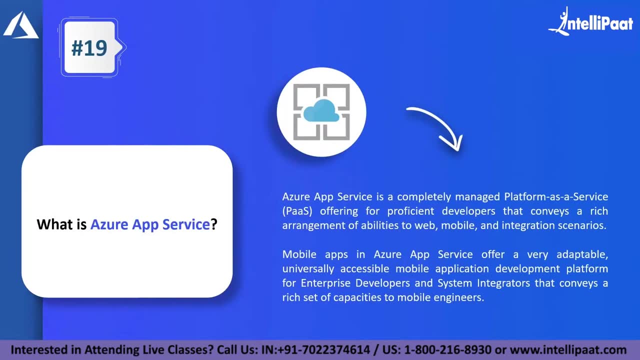 our application right now, so all these widgets can be used in Azure devops. so you've seen that the next question is: what is Azure app service? we've already discussed this, but still I'll explain to you once again, so to be very simple, as your app service is a completely a managed 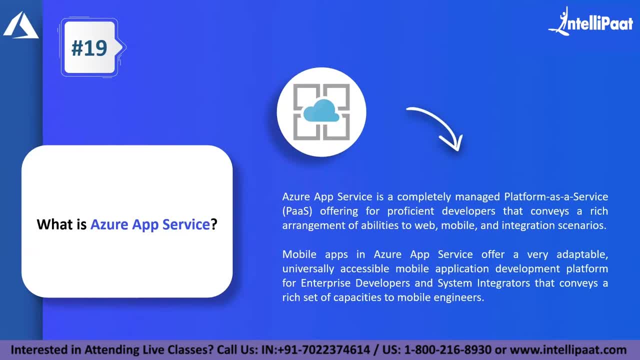 service provided by Microsoft Azure. so within Azure, Azure app service is a completely managed platform as a service, not infrastructure as a service, but a pass. it is a pass offering for proficient developers that conveys a rich arrangement of abilities to web, mobile and integration services. so if a developer wants to just concentrate on the code which is developing, 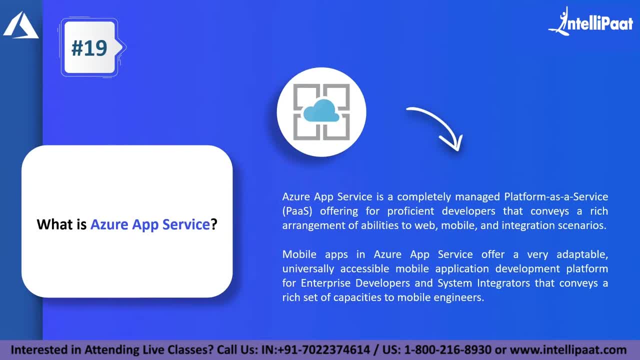 and doesn't want to manage the servers and the other side of it, that is, the backend part of it. so what he can do, he can opt for Azure app service, where he can launch one and he can just upload his code into Azure app service, which will take care of provisioning. 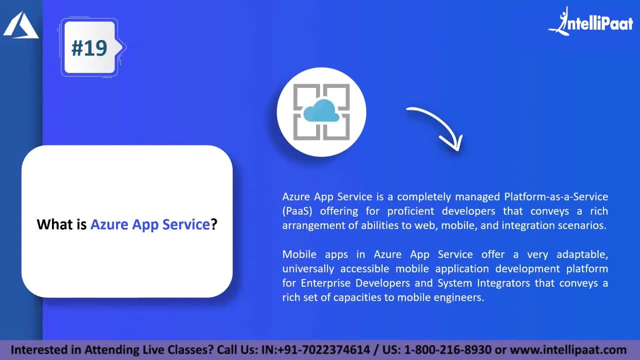 servers, uploading the code with the server and also serving that website, and also provide you an URL which you can use to look into the website. so you can do all of this using Azure app service and you don't need to manage anything. Azure will manage everything for you. it will as told it. 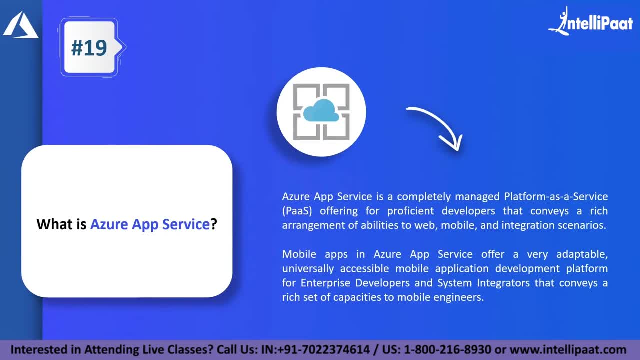 won't servers, it'll also monitor and manage them for you. and if you want anything else, if you want to scale it up again, you have an option for that. if you want to look into the server which it has launched again, you have a shell option for that. mobile applications in Azure app service offer a 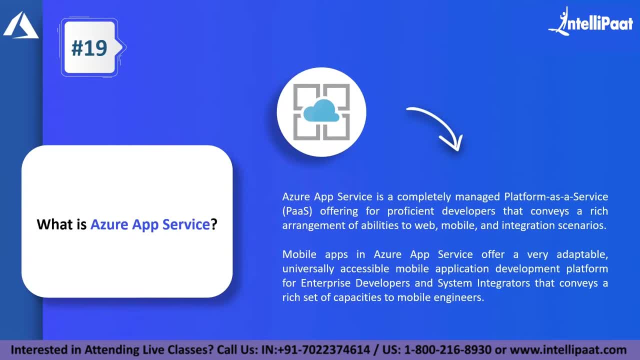 very adaptable, universally accessible mobile application development platform for Enterprise developers and system integrators that conveys a rich set of capacities to mobile engineers. so basically, using Azure app services, you cannot just launch websites, you can also launch mobile applications, and they are very adaptable and universally accessible mobile application development. 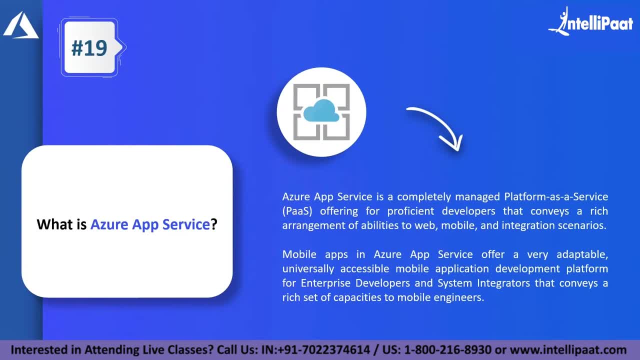 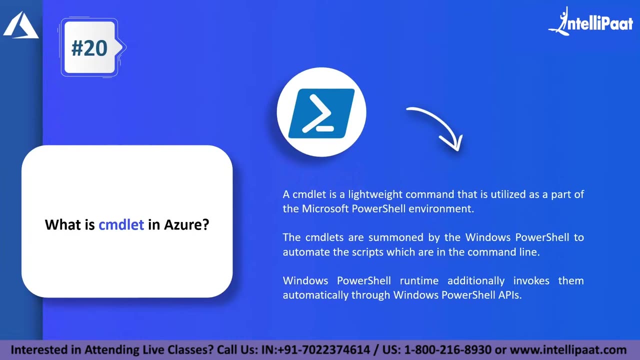 platform. for example, you might be using Android studio or xcode, so in this you will be able to launch both of them and they will run successfully. so next we'll look into cmd let in Azure. so it's it's a pretty simple answer. so cmd let is a command. basically it's a 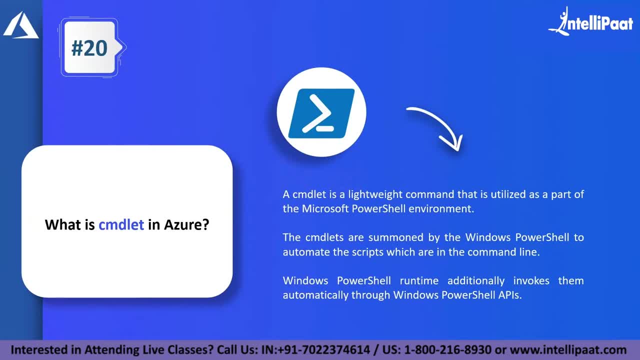 PowerShell command and this is utilized as a part of the PowerShell environment. so cmd- let's, command, let's are summoned by the Windows PowerShell to automate the scripts which are in the command line. for example, you have created a script. now you want to automate the script. you. 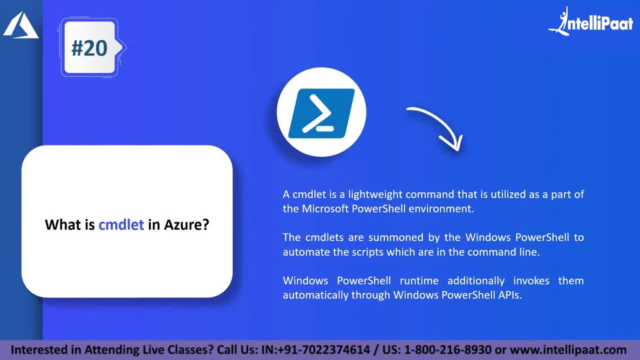 can go with command let. Windows PowerShell runtime additionally invokes them automatically. through Windows PowerShell APIs you can also automate cmd let commands, which will automate other scripts using PowerShell APIs. so to be pretty simple, cmd let is a lightweight command which you can use in the PowerShell environment and it is used to automate scripts. for example, if you want, 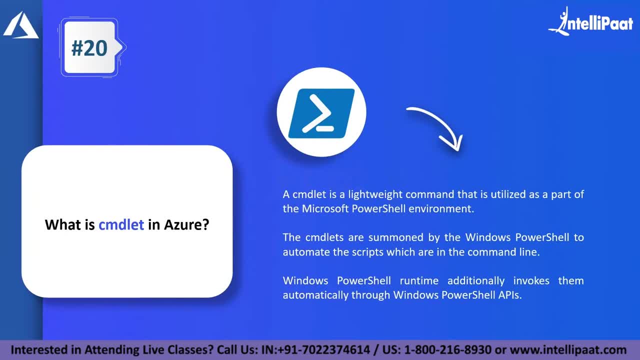 to launch virtual mission at a particular time or if you want to monitor a virtual mission at 5 pm in the evening, every single day, you can launch that script and you can automate it using cmd let and it will run that script every every day at 5 pm. 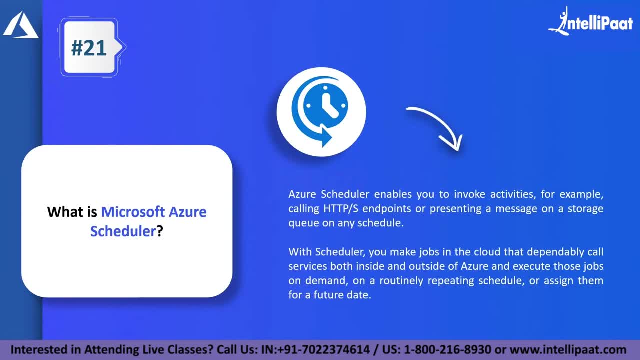 okay, so the next one is Microsoft Azure scheduler. so Azure scheduler enables you to invoke activities- for example, calling HTTPS endpoints or presenting a message on a storage queue- on any schedule. with scheduler, you make jobs in the cloud that dependably call services both inside and outside of Azure and execute jobs on demand on a routinely repeating schedule or assign them on a for a future. 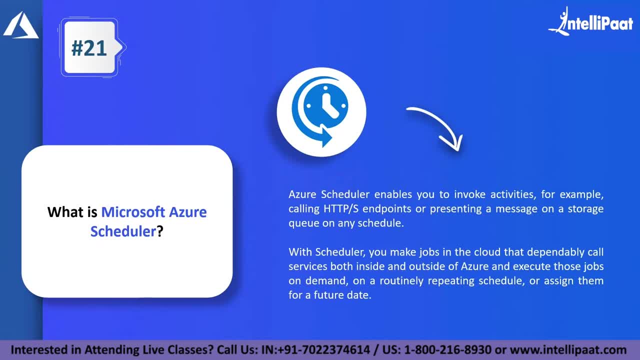 date. so in the name itself you can understand Microsoft Azure scheduler. so it basically schedules certain things for you. but what does it schedule? it schedules jobs on the cloud, so it can be within Azure or outside of Azure and, as mentioned, it will execute those jobs on demand and it can be done on a repeating scale. 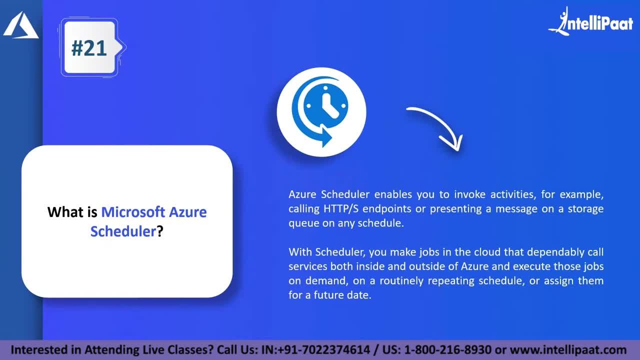 that is, for example, every day or every week, or you can assign them for a future date to run only once, so that you can do using Microsoft Azure scheduler. for example, it can call an HTTPS endpoints or it can present a message on a storage queue on any. 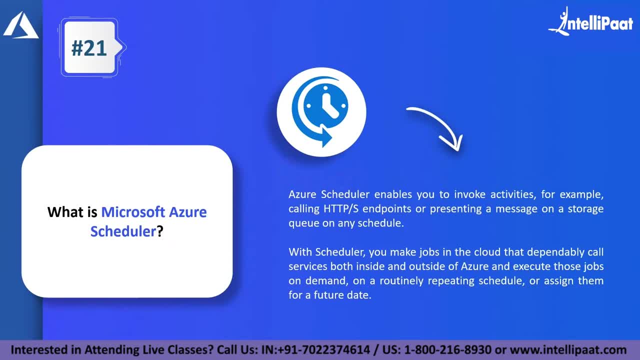 schedule, so you can use the scheduler for any service on Azure or outside of Azure. so it's pretty simple. it is, uh explainable mine by name itself. so to be simpler, you can tell this: Microsoft Azure scheduler is a service which you can use to schedule a certain task in Microsoft Azure or 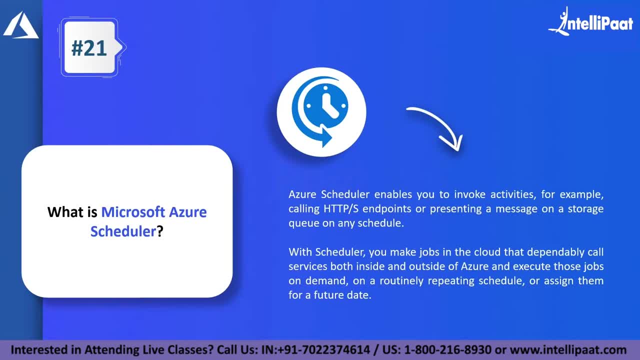 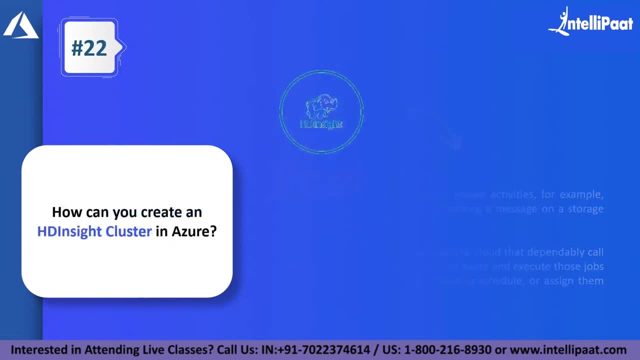 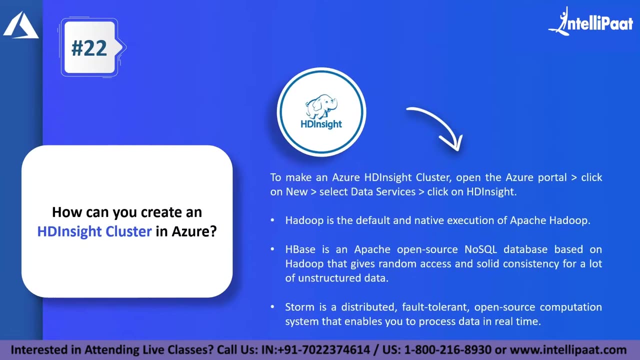 outside of Microsoft Azure, execute a job on demand which can be executed repeatedly, or it can be set to a future date for execution only once. so the next question is: how can you create an HD insight cluster in Azure? so let me explain to you in in a very simple way, so you can tell this, because this is an interview. you. 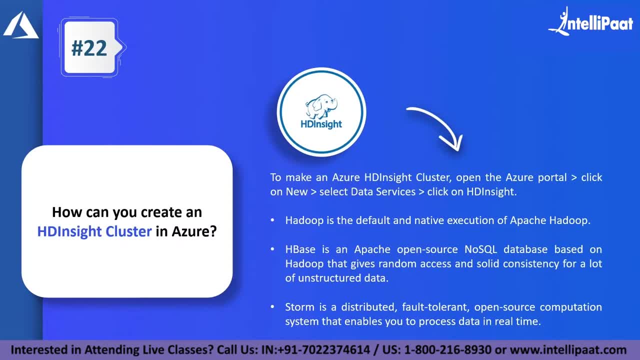 will be asked questions. you will be able to answer them with words. so to make an HD inside cluster, first of all you'll have to open as your portal, then click on new. you can select data services and you can click on HD inside, or you can just search HD inside and get into it. so once 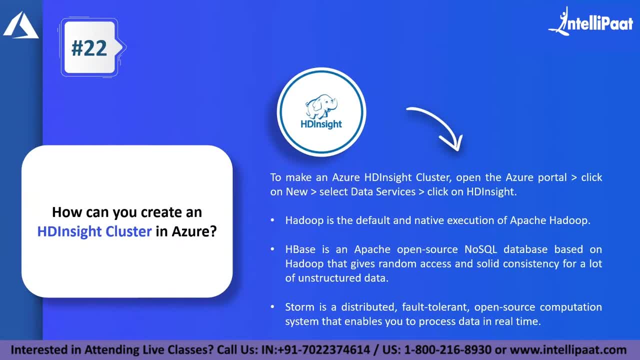 you get into it, you will have multiple options. you will have Hadoop, you will have HBase and storm and more options as well. so Hadoop is the default and native execution of our Apache. Hadoop and HD inside provides you, uh, Hadoop as the default option, and then comes HBase, which is an Apache. 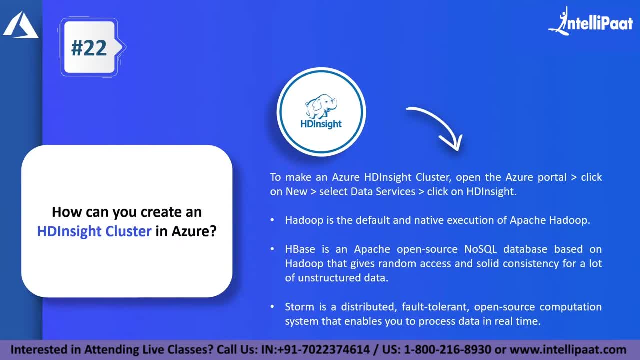 open source, no sequel database based on Hadoop that gives random access and solid consistency for a lot of unstructured data storm. as such, it is a distributed, fault tolerant open source computation system that enables you to process data in real time. so the thing is, I'm 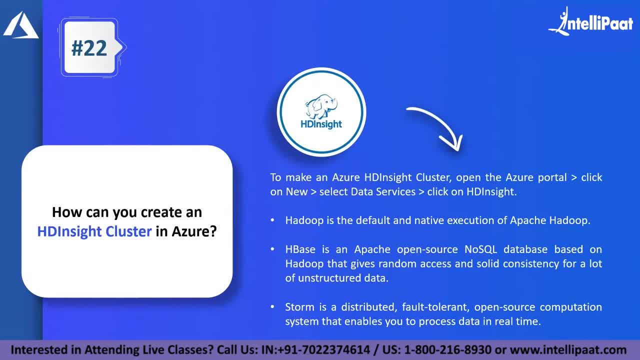 not going to explain how to pitch base and storm right now. I'm just going to explain to you what is HD insight. so HD insight is an analytic service which you can use to launch Hadoop on the Azure cloud or other Hadoop ecosystem services like HBase, storm or spark on Azure. 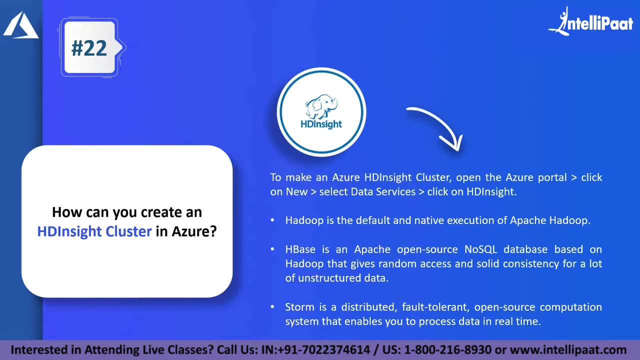 cloud. so to launch HD insights it's pretty simple, but to work with it it is a little tough. so to launch HD inside, you will just have to go to the HD inside uh cluster and you can choose the service which you want and you can launch it. so it changed side again, it's an analytic service and you can. 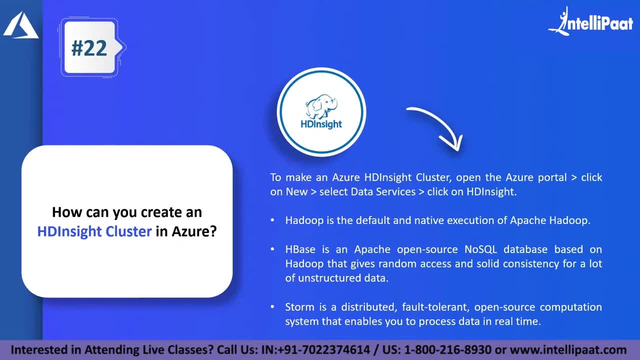 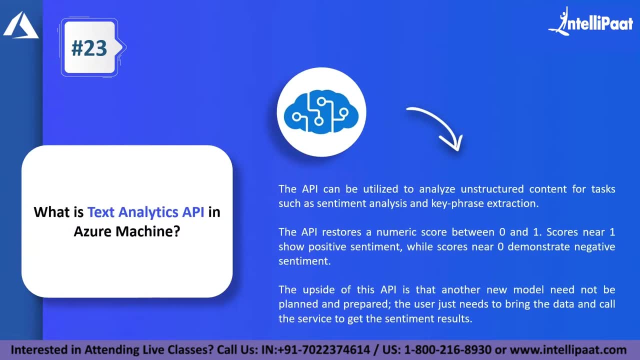 launch the big data or analytic service which you want from it. next question is: what is text analytics API in Azure mission? so let me put it simply. first of all, text analytics APIs comes under cognitive services, so API, the application program interface. so this particular API is for text analytics which can be used to search a particular word, or it can be used 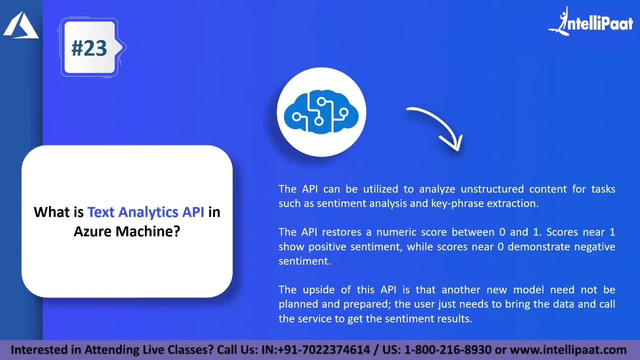 for keyword mining. okay, now let me let us just read this. once the API can be used or utilized to analyze unstructured content for tasks such as sentiment analysis and key phrase extraction: sentiments- sentiment analysis in the sense, let's say, you have a complete page of content. now you want to see. 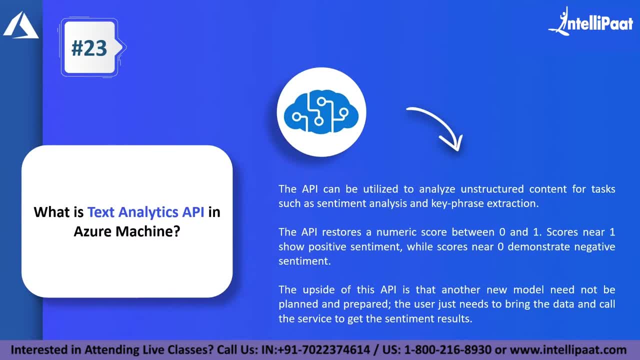 the sentiment of that content, whether the statement is happy or sad or neutral. so you can check out that using various keys and you can enter those words into the API so that when it runs it will check whether it is positive or negative. so you can see it as a numeric score. 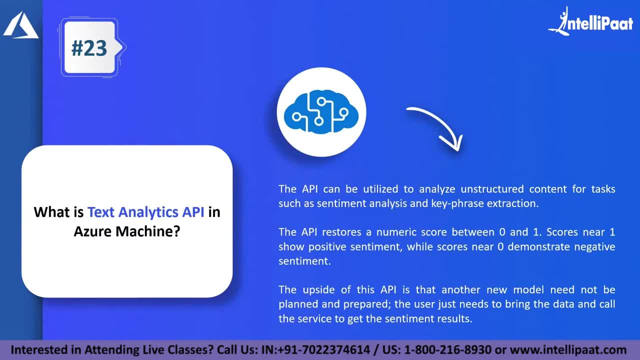 between zero and one and when it comes near one, it is highly positive and it when it comes near zero, it is highly negative. sentiment so that you can see this for sentiment analysis and key phrase extraction. in the sense, if you have a very huge document and if you want to check whether this 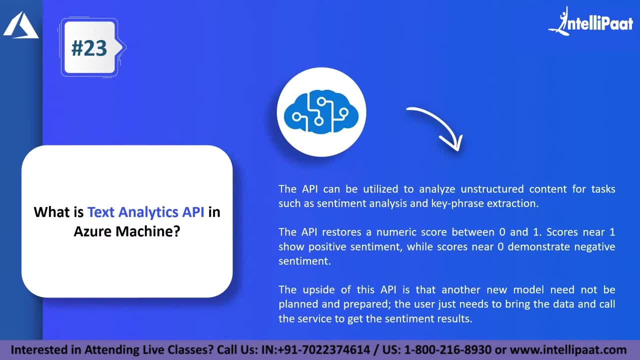 particular key phrase comes inside it and you can use the text analytics API to check out the entire document. the upside of this API is that another new model need not be planned and prepared. the user just needs to bring the data and call the service to get the sentiment results. so 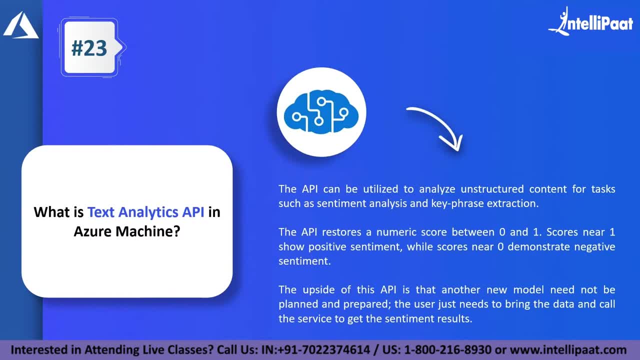 they are telling that the best part of this API is that you don't need to call another service to run this API. instead, you just have to bring the data set and call this API to run on the data set and get the sentiment results immediately. so I think you got it. it is a text analytics API. 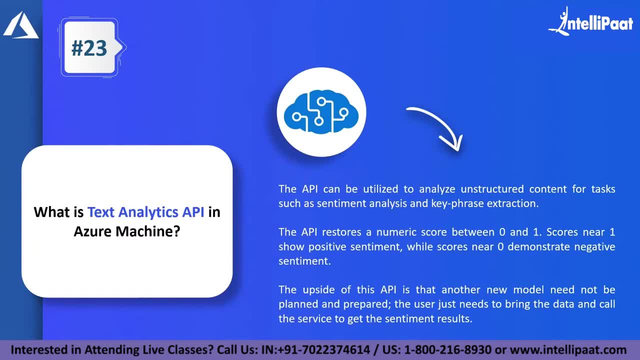 mainly used for tasks like sentiment analysis and key phrase extraction. you have two numeric scores- zero and one. near zero it is negative and near one it is highly positive. it's basically sentiment, and the upside is you don't need to call any other service. you can directly call this API and upload a data set and it will give you the sentiment results. 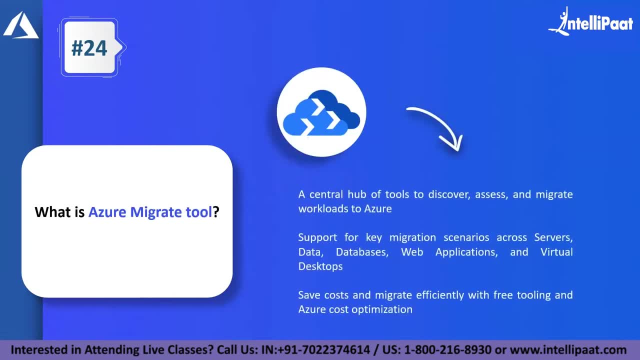 next question is: what is migrate tool? so, again in the name itself, you can get this answer: migration, a migration from the on-premise setup to the cloud or from the cloud to the on-premise setup. this is the central hub of tools to discover, access and migrate. 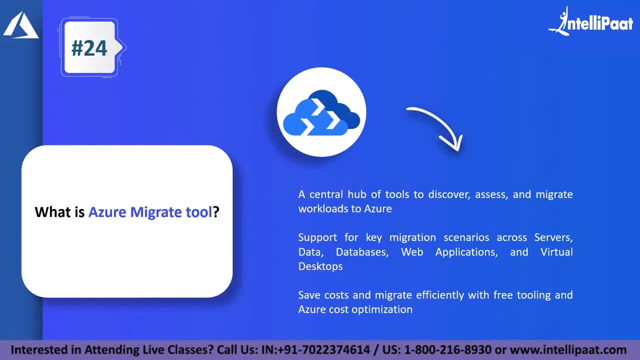 workloads to Azure so you can migrate any type of workload into Azure. so it provides support for key migration scenarios across servers, data databases, web applications and virtual desktops. it saves costs and migrate efficiently with free tooling and Azure cop optimization so you can use them as your migrate tool to migrate databases or servers or web applications from. 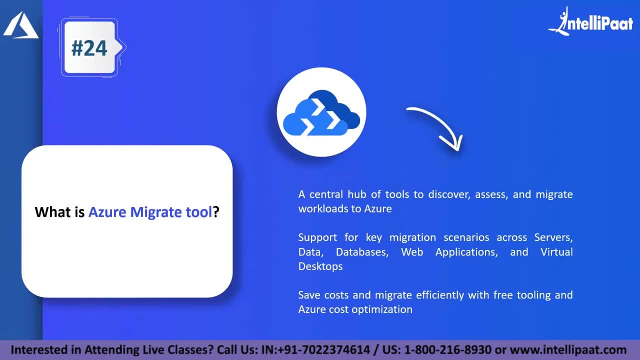 your on-premise setup to the Azure cloud seamlessly. so, for example, if you want to migrate to your database, you will have to provide the details, like the endpoint. then you'll have to provide the username and password and then the destination would be a Azure database. you can. 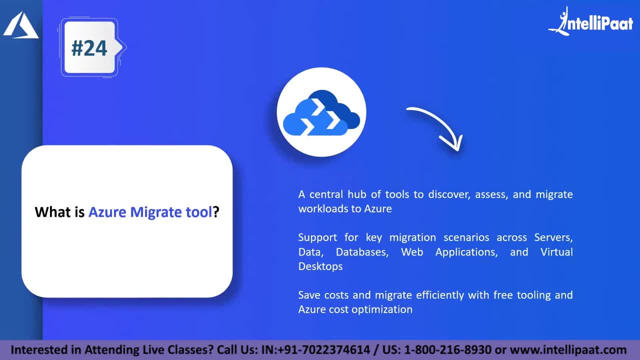 provide the details of the as your database and once you click start, it will migrate the data from the on-premise database into the Azure database, and it's very, very simple to start with. so this is basically as your migrator. you can easily explain this with two or three sentences and we've 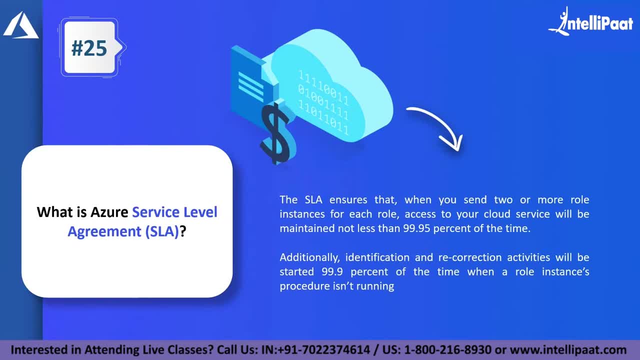 Azure service level agreement. First of all, the SLA ensures that when you send two or more role instances for each role, access to your cloud service will be maintained not less than 99.9% of the time. Additionally, identification and recorrection activities will be started. 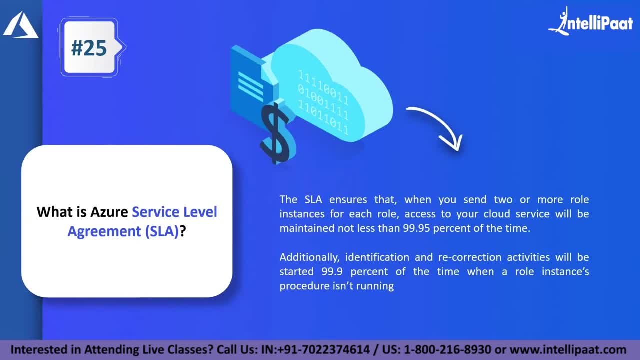 99.9% of the time when a roles instance procedure isn't running. So let me explain to you SLA in simple words. It's an agreement in which Azure tells you that this particular service will be running for this amount of time. So, for example, if you're using a service for 10 minutes, Azure